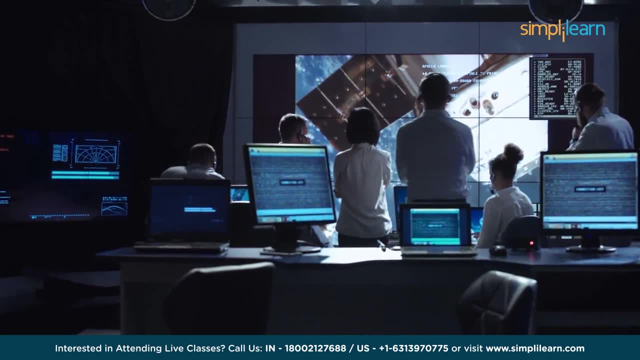 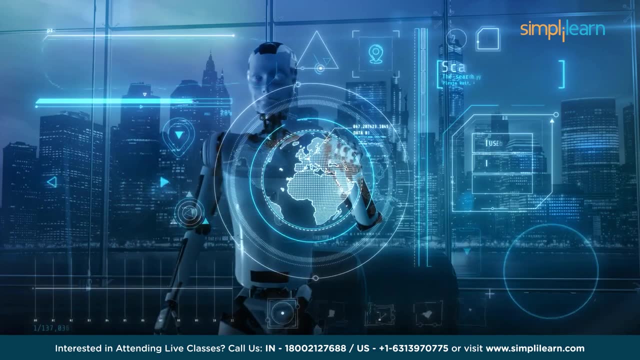 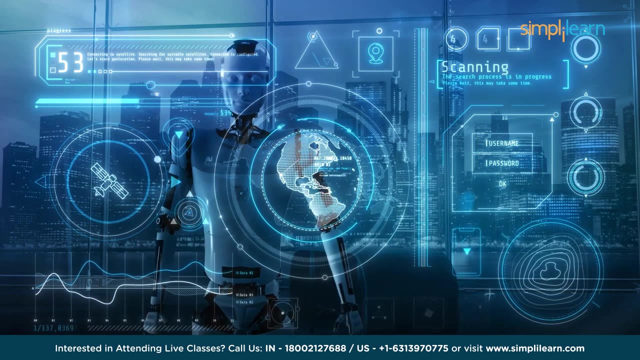 state-of-the-art tools and technologies utilized by the industry leaders. From data science fundamentals to statistics, from basics of machine learning to the basics of data science, to critical machine learning algorithms, and from programming fundamentals to data science with Python and R, this course pushes the boundaries of traditional analytics and unraveling. 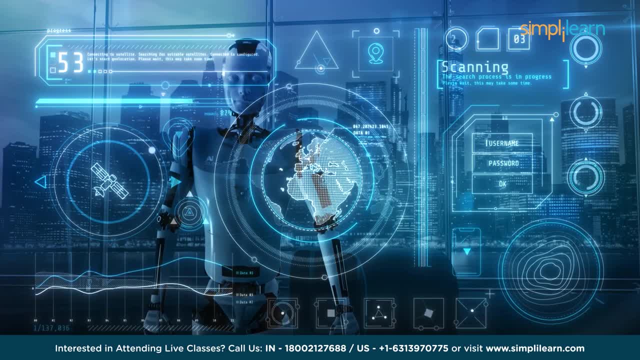 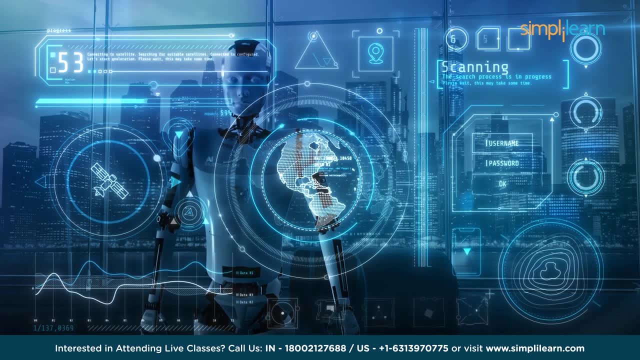 the true potential of big data. Through practical projects and real-world case studies, you will gain the expertise to extract valuable insights, uncover hidden patterns and transform data into a strategic asset. Join us in the transformative adventure and let advanced data science unleash your analytical powers. 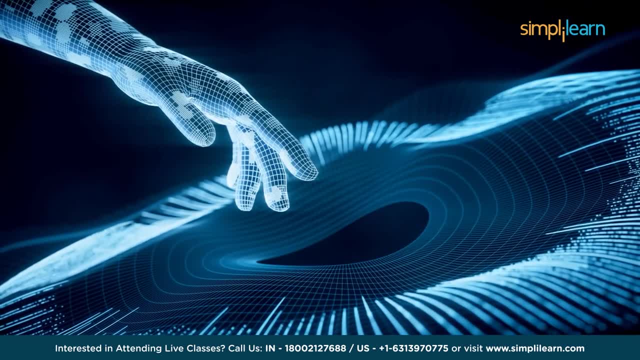 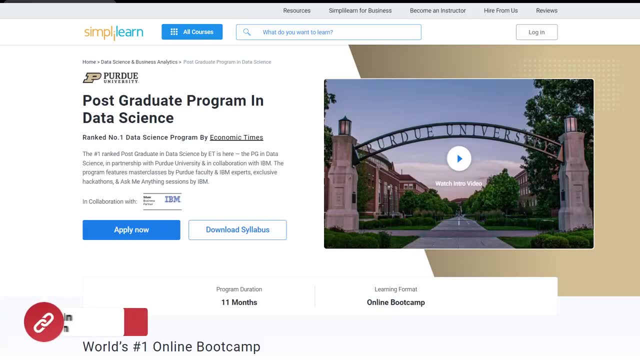 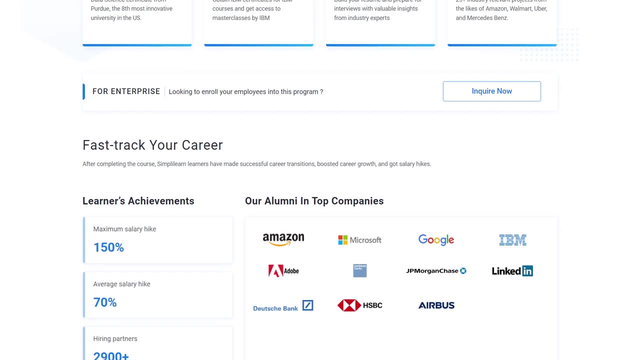 If these are the type of videos you'd like to watch, then hit the subscribe button and press the bell icon to never miss out on our future content. Also, if you're a data scientist looking for online training and certification programs from the best universities, or a professional who elicits to switch careers with data science, 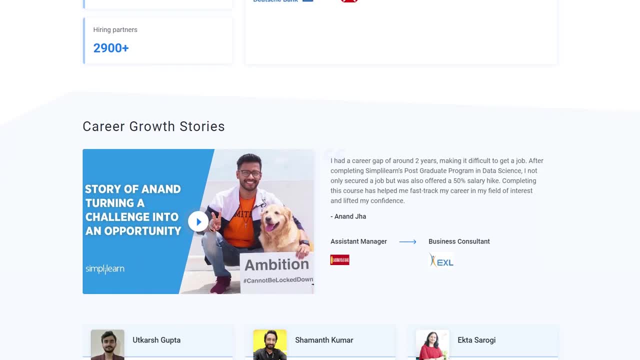 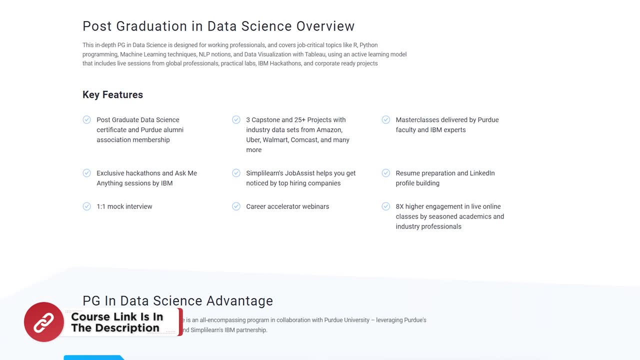 then try giving Simply Learn's postgraduate program in data science a shot. The link in the description box below should navigate you to the homepage where you can find the complete overview of the program being offered. Now over to our guest Training experts Murray. 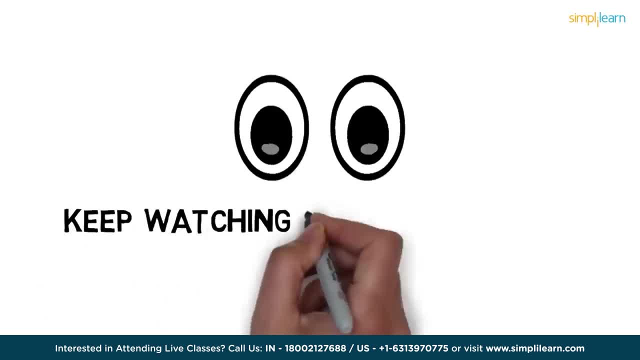 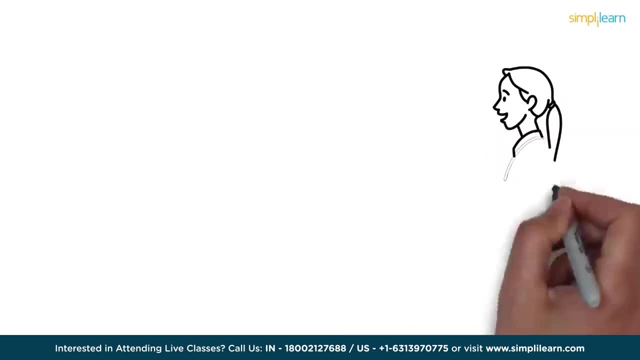 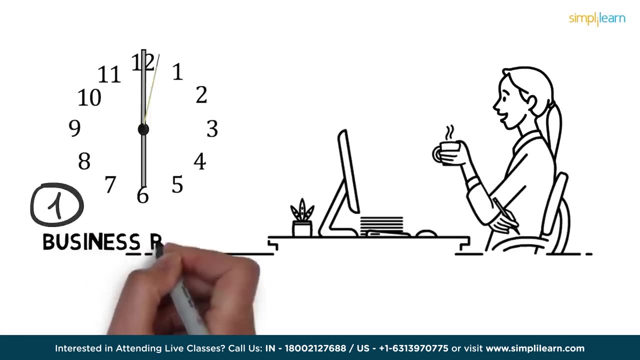 Are you one of the many who dreams of becoming a data scientist? Keep watching this video if you're passionate about data science, because we will tell you how does it really work. under the hood, Emma is a data scientist. Let's see how a day in her life goes while she's working on a data science project. Well, it is very important to understand the business problem first. 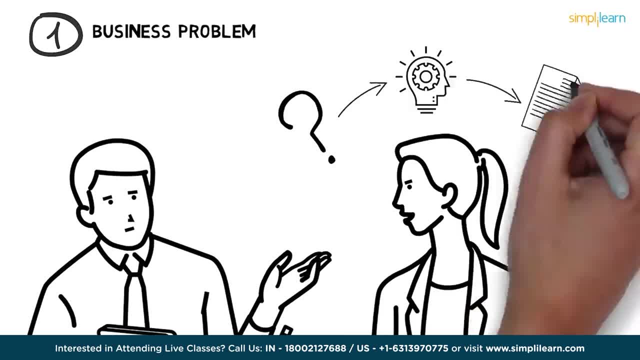 In our meeting with the clients, Emma asks relevant questions, understands and defines objectives for the problem that needs to be tackled. She is a QA, She's a CTO, So I'll leave you with that for now and we will see you in the next video. Bye for now. 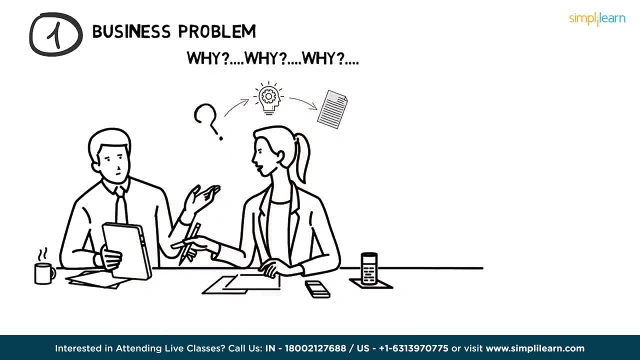 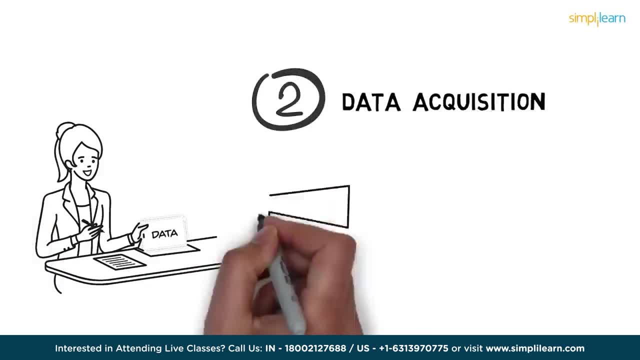 Bye, curious soul who asks a lot of eyes, one of the many traits of a good data scientist. Now she gears up for data acquisition, to gather and scrape data from multiple sources like web servers, logs, databases, APIs and online repositories. 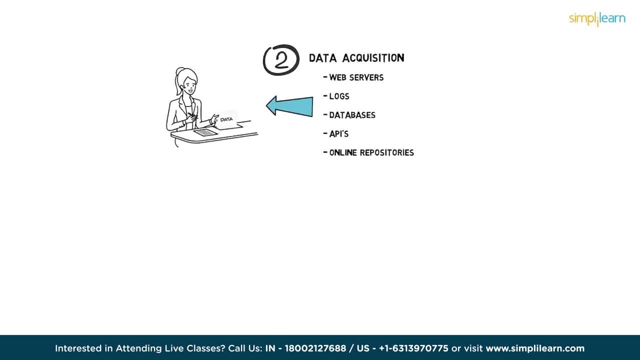 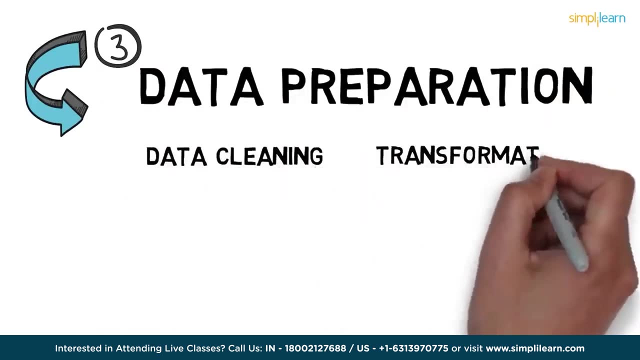 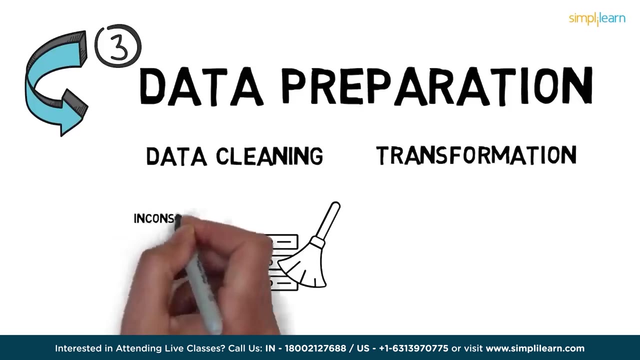 Oh, it seems like finding the right data takes both time and effort. After the data is gathered comes data preparation. This step involves data cleaning and data transformation. Data cleaning is the most time-consuming process, as it involves handling many complex scenarios. Here Emma deals with inconsistent data types, misspelled attributes, missing values, duplicate. 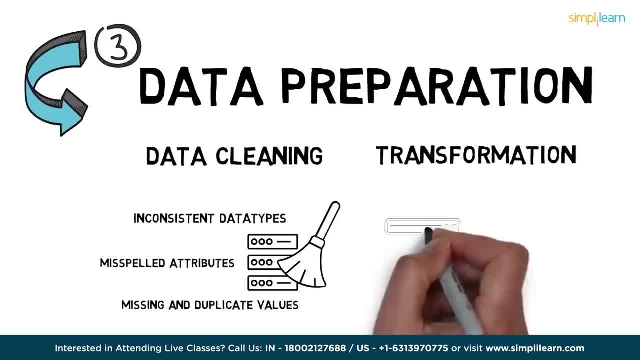 values and what not. Then in data transformation, she modifies the data based on defined mapping rules. In her project ETL, tools like Dalent and Informatica are used to perform complex transformations. that helps the team to understand the data structure better. 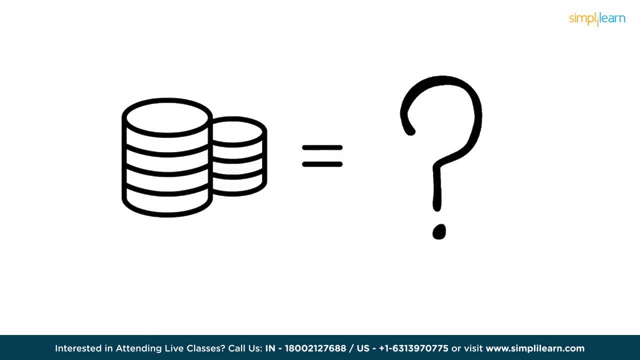 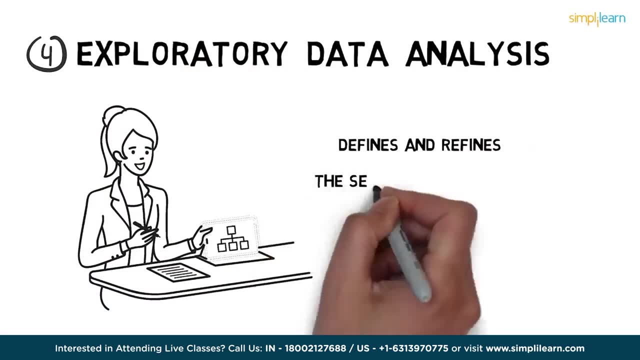 Then understanding what you actually can do- So what you can do with your data- is very crucial. For that, Emma does exploratory data analysis. With the help of EDA, she defines and refines the selection of feature variables that will be used in the model development. 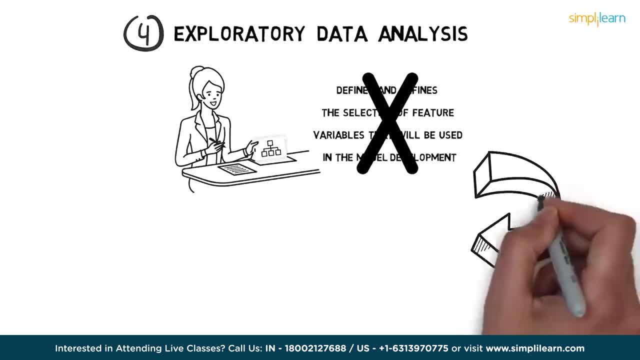 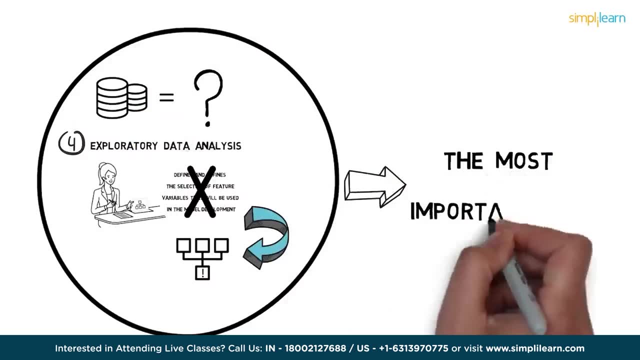 But what if Emma skips this step? She might end up choosing the wrong variables, which will produce an inaccurate model. Thus exploratory data analysis becomes the most important step. Now she proceeds to the core activity of a data science project, which is data modeling. 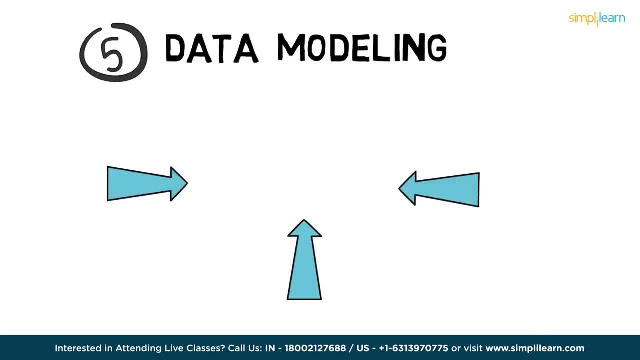 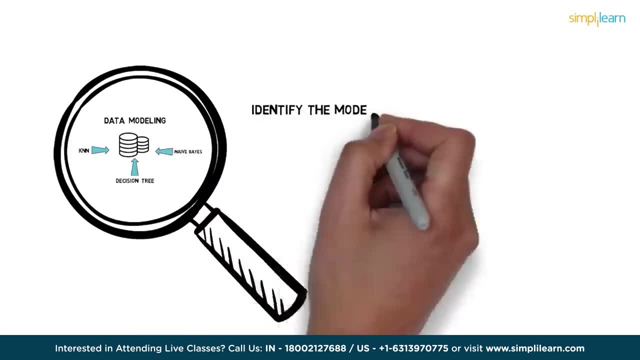 She repetitively applies data analysis to the model. This is called data modeling. Emma applies diverse machine learning techniques, like KNN, Decision Tree, KnifeBase, to the data to identify the model that best fits the business requirement. She trains the models on the training dataset and tests them to select the best-performing. 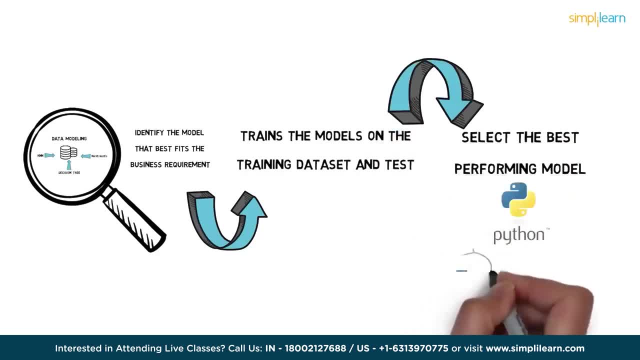 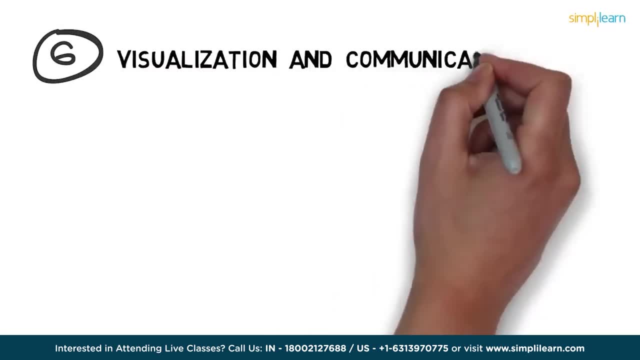 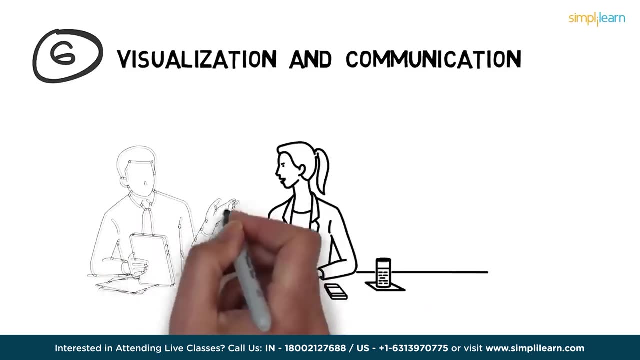 model. Emma prefers Python for modeling the data. However, it can also be done using R and SAS. Well, the trickiest part is not yet over: visualization and communication. Emma meets the clients again to communicate with business partners. She uses the tools like Tableau, Power BI and QlikView that can help her in creating. 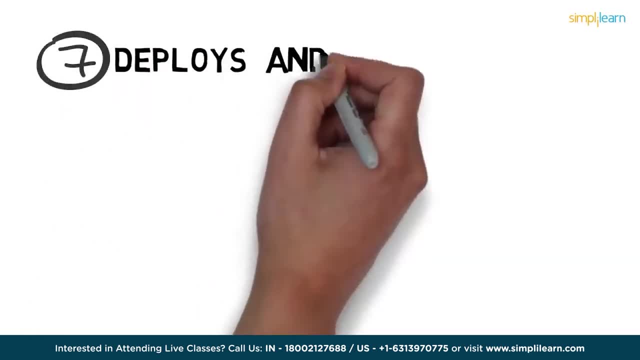 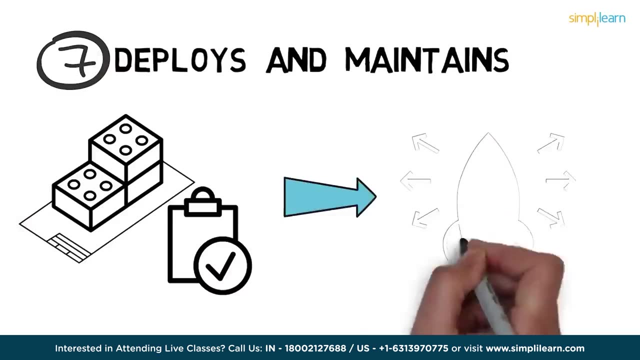 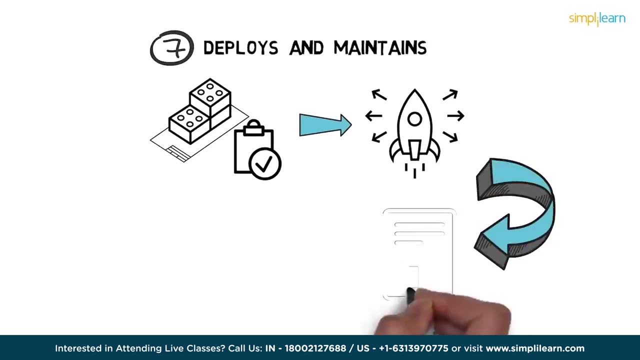 powerful reports and dashboards. And then, finally, she deploys and maintains the model. She tests the selected model in a pre-production environment before deploying it in the production environment, Which is the best practice. right After successfully deploying it, she uses reports and dashboards to get real-time analytics. 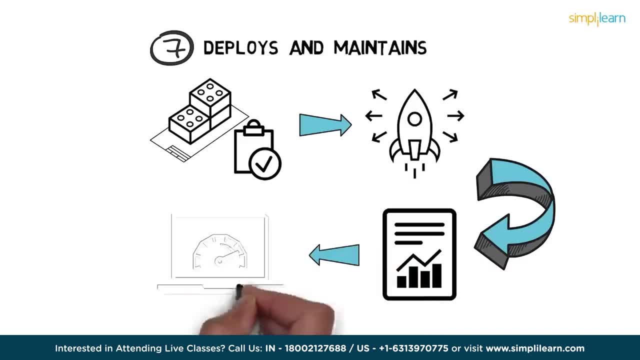 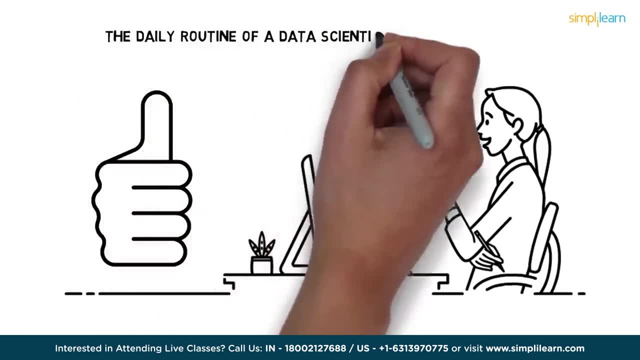 Further, she also uses the data analysis to get real-time analytics. Emma also monitors and maintains the projects' performance. Well, that's how Emma completes the data science project. We've seen the daily routine of a data scientist is a whole lot of fun, has a lot of interesting. 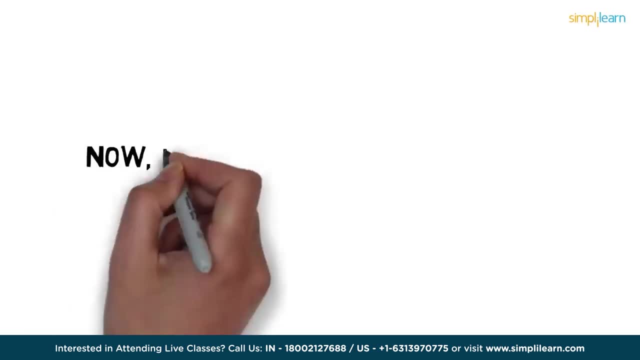 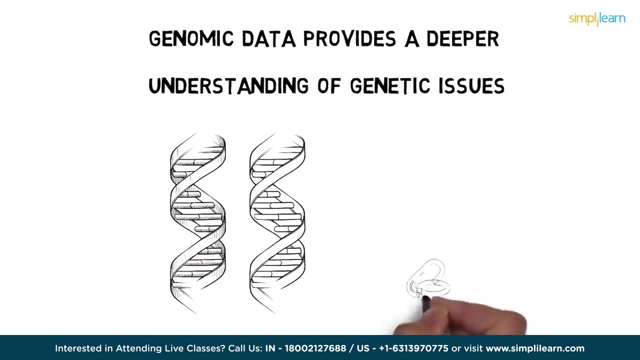 aspects and comes with its own share of challenges. Now let's see how data science is changing the world. Data science techniques, along with genomic data, provide a deeper understanding of genetic issues and reactions to particular drugs and diseases. A data science project is a farming engineering project that is designed for domestic economic 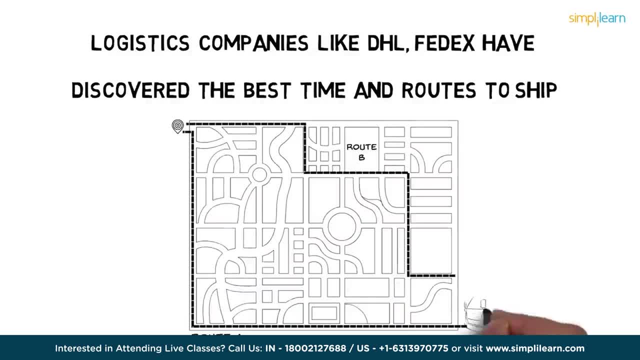 and industrial use Logistics companies like DHL and Fedex have developed a lot of data science. software for data science: discover the best routes to ship, the best suited time to deliver, the best mode of transport to choose, thus leading to cost efficiency. 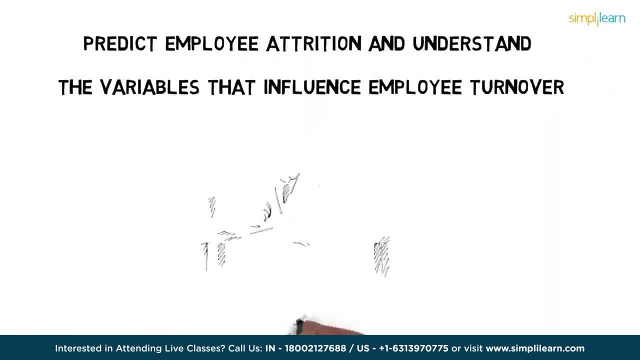 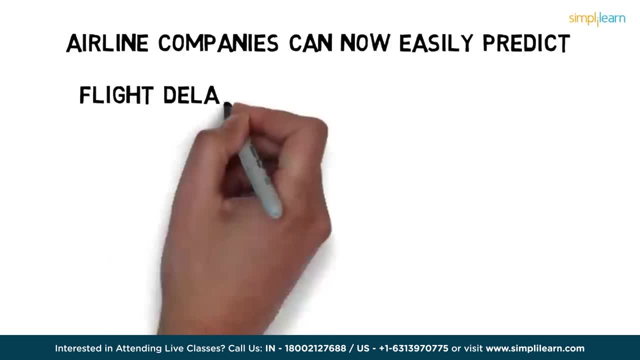 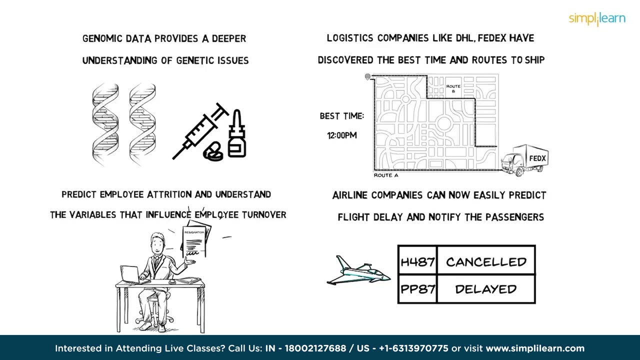 With data science, it is possible to not only predict employee attrition, but to also understand the key variables that influence employee turnover. Also, the airline companies can now easily predict flight delay and notify the passengers beforehand to enhance their travel experience. Well, if you're wondering, there are various roles offered to a data scientist. like data, 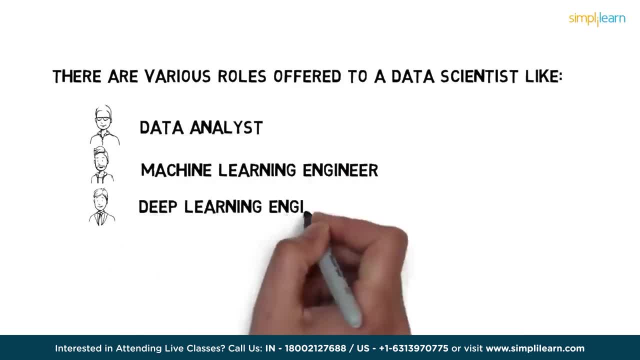 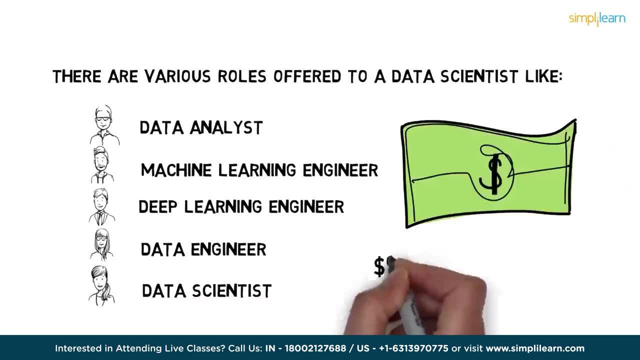 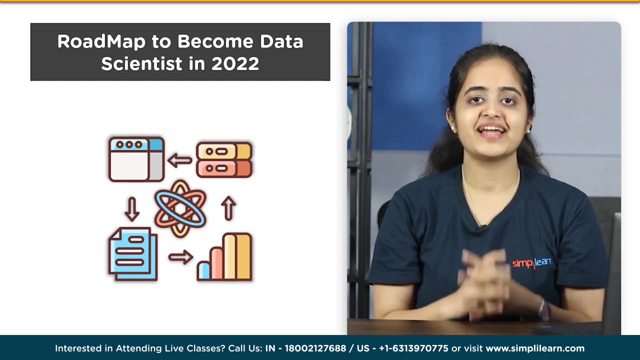 analyst, machine learning engineer, deep learning engineer, data engineer and, of course, data scientist. The median base salaries of a data scientist can range from $95,000 to $165,000.. So that was about the data science. Google had gathered 5 exabytes of data between the beginning of time 2003.. 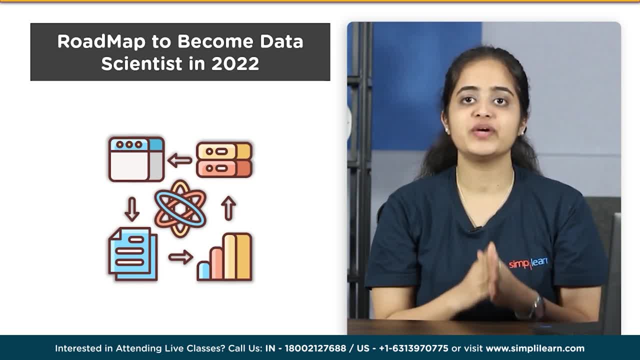 This amount of data started to be produced in the early 2000s. This amount of data started to be produced in the early 2000s. This amount of data started to be produced every two days in 2010 and every 40 minutes. 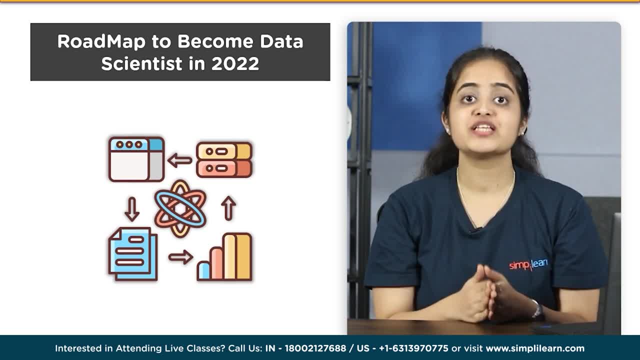 by 2021.. The responsibility of a data scientist is to gather, clean and present data, and have a keen business sense and analytical abilities. Let us have a discussion about it in the upcoming slides. How can you become a data scientist as a beginner? 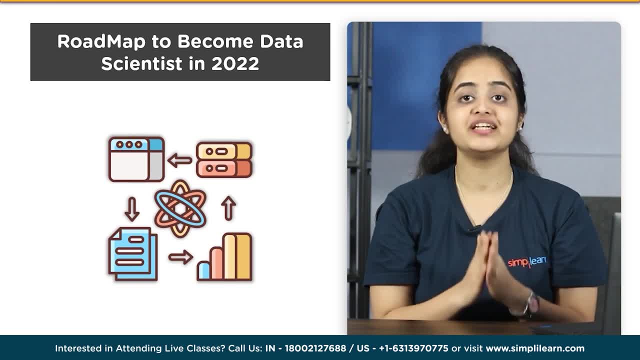 I guarantee you, after watching this video, you will have a clear understanding on how to drive your career as a data scientist. Hey guys, welcome to Simply Learn. If you are new to the channel, please make sure you subscribe to Simply Learn's YouTube. 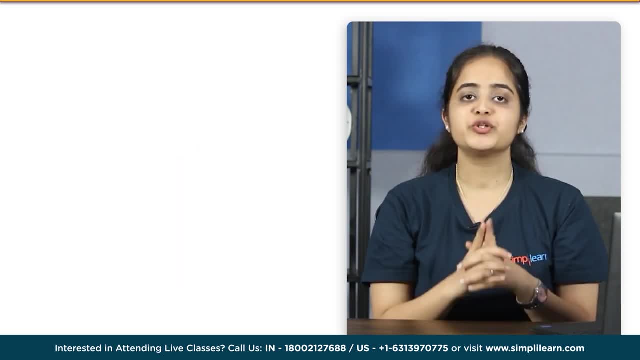 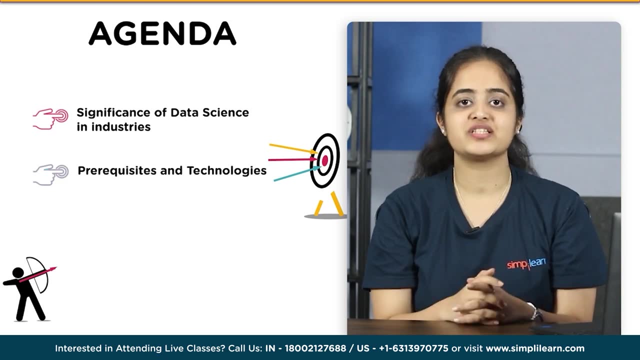 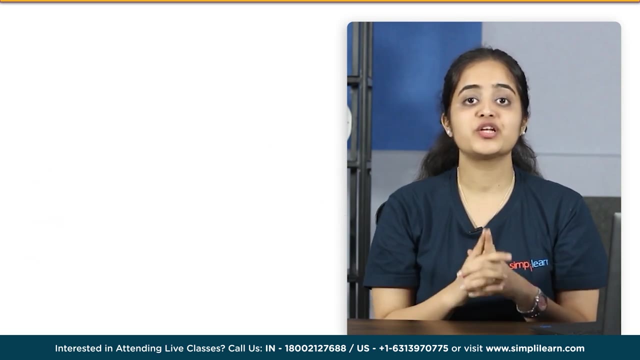 channel and press the bell icon to never miss any updates. Today we are going to cover significance of data scientist in industries. After that, prerequisites and technologies required for a data scientist And finally, salary of a data scientist. I have a query for you: which technology is used by Google Maps to predict traffic jams? 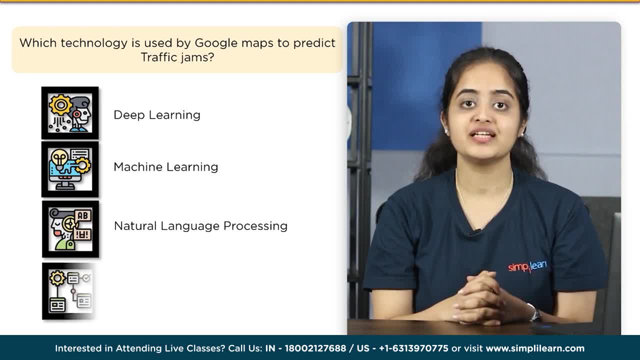 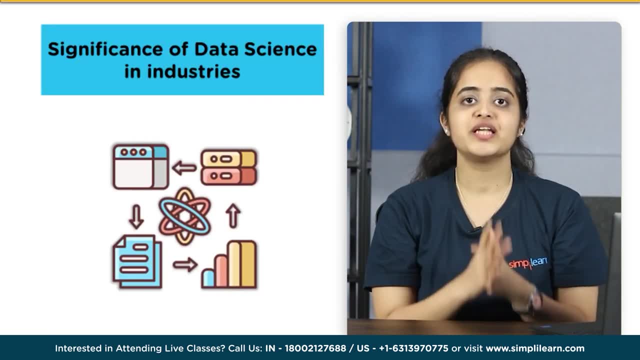 Deep learning, machine learning, natural language, processing, data structure. Please leave the answer in the comment section below And stay tuned to get the answer. Significance. Now we will see how top industries are involved in the field of data science. By 2025, the data science industry is anticipated to grow to a value of $16 billion. 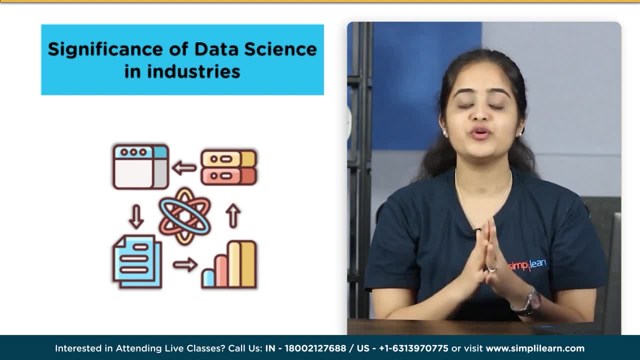 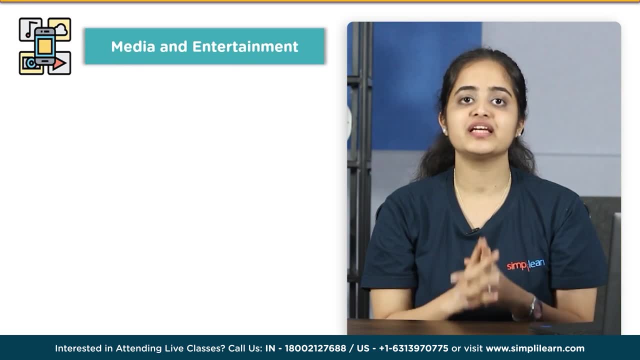 There is an abundance of data science jobs all over the world. Now let's list out crucial areas where data science is used. Media and entertainment: The major player in the media and entertainment sector, such as YouTube, Netflix, Hotstar, etc. have begun to use data science to better understand their audience. 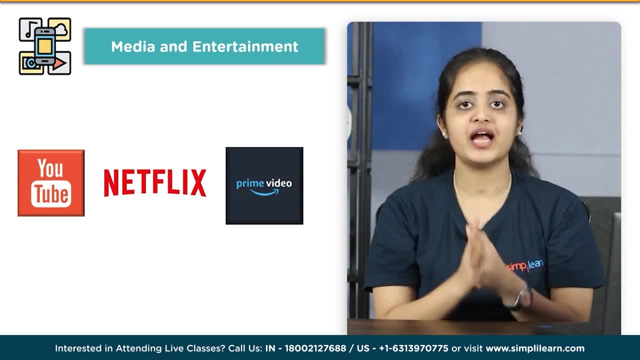 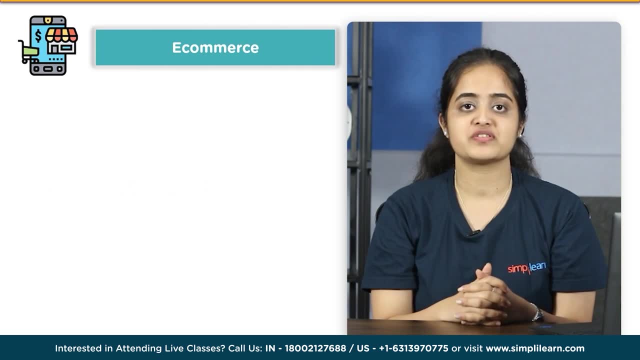 and provide them with recommendations that are both relevant and personalized. E-Commerce Data science has aided retail companies in better meeting their expectations, As they bring a unique combination of deep data knowledge, technology skills and statistical experience. data scientists are in high demand in the retail industry. 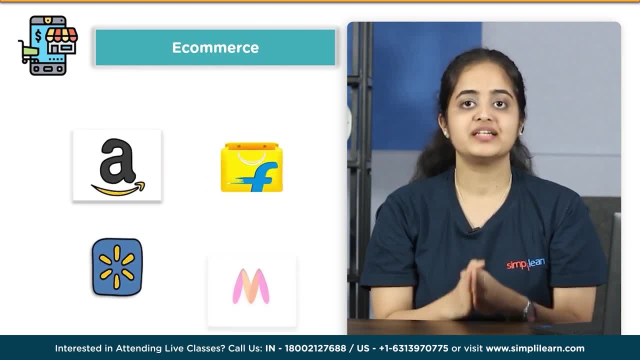 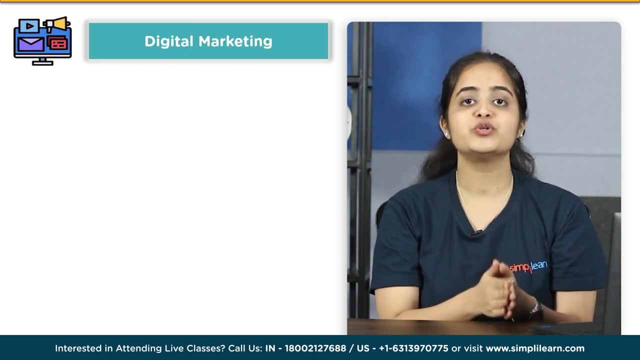 Top recruiters are Amazon, Flipkart, Walmart, Myntra, Digital marketing. Large volumes of data are currently being fetched from its users through search pages, social networks, online traffic display networks, movies, web pages, etc. A high level of business intelligence is needed to analyze such large amounts of data and 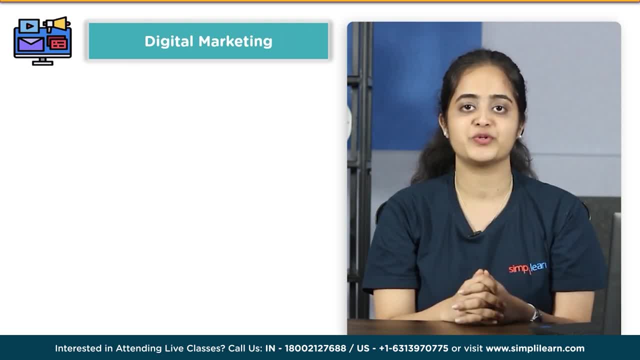 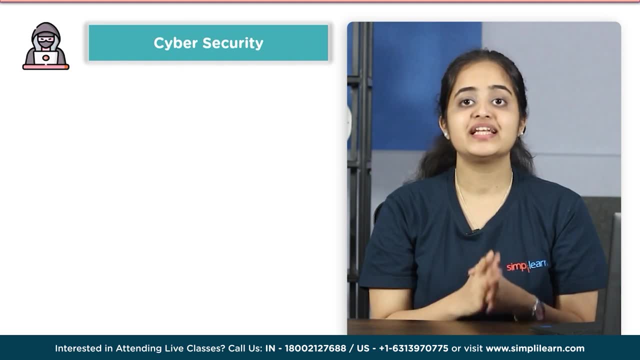 this can only be done with the proper use of data science approaches. Top recruiters are Amazon, Flipkart, Facebook, Google. famous companies, Amazon, Facebook, Cybersecurity, Data science and AI are now being used by the cyber security industry to prevent the 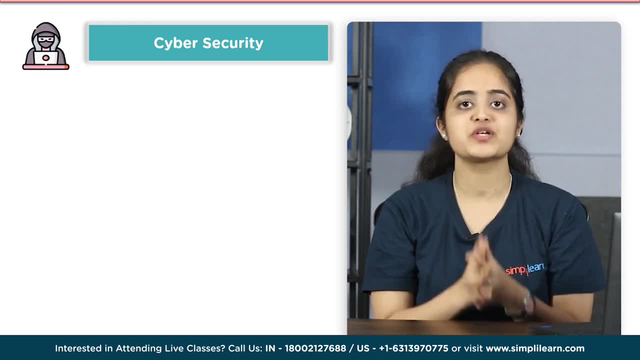 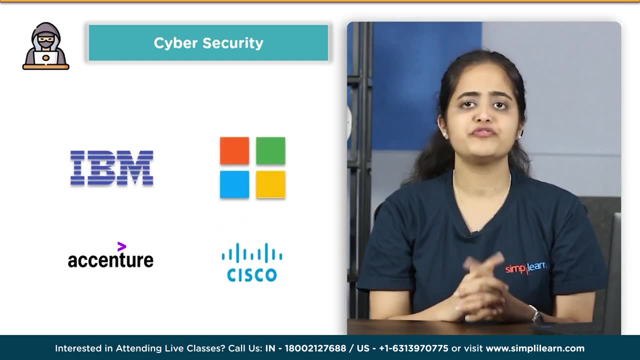 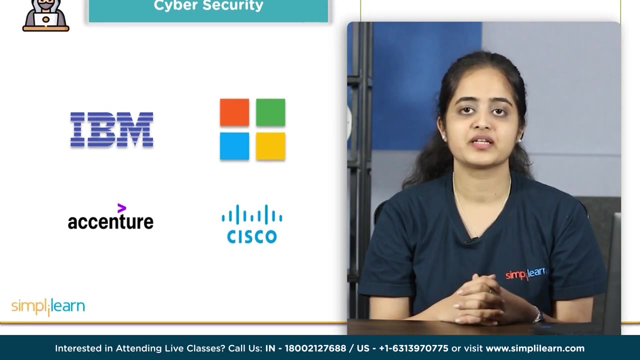 growing usage of algorithms for harmful purposes. Top recruiters include IBM, Microsoft, Accenture, Cisco and many more. Before moving forward, what is the response to the Google map question that I asked? Answer is Machine Learning Coming to Pre-requisites Now that we know significance of data science. 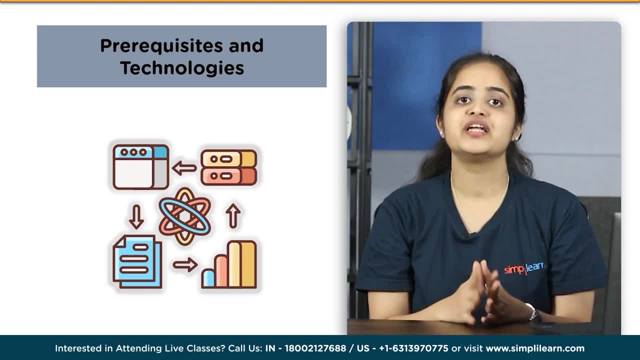 let us explore the prerequisites and technologies required for a data scientist. Seeing the demand of data scientists in every industry, it is obvious that the scope of a data scientist is very high. So how to start? There is no necessity that you should be knowing any technology or programming language. 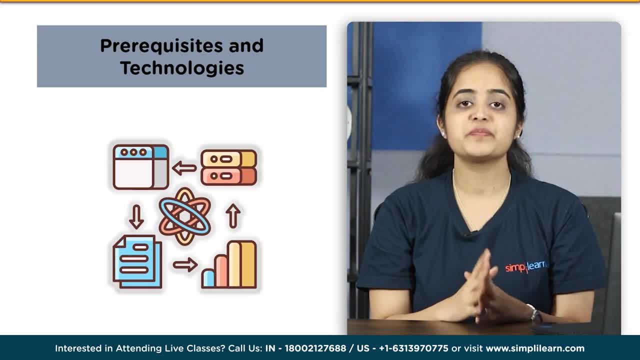 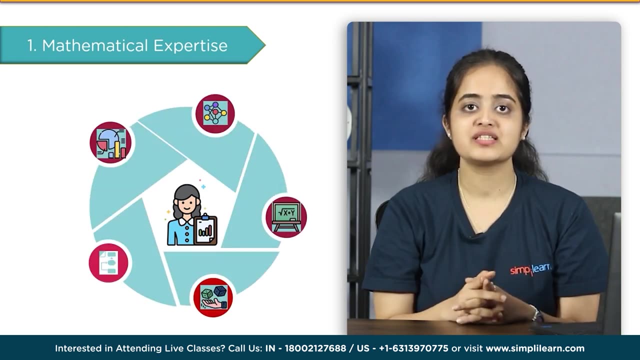 You can be a layman too. Data scientists typically have a variety of educational and professional experiences. Most should be proficient in four crucial areas. Important skill is mathematical expertise. Three concepts like linear algebra, multivariable calculus and optimization technique are crucial because they aid in our understanding of numerous machine learning algorithms. 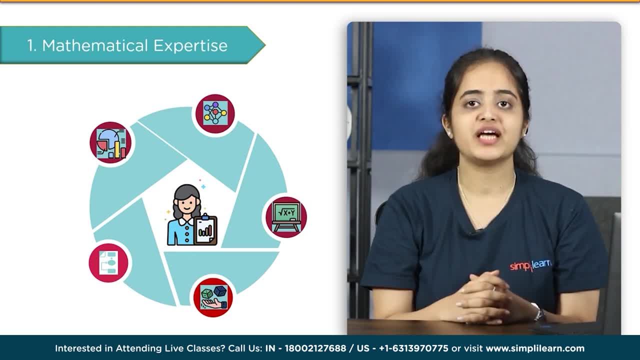 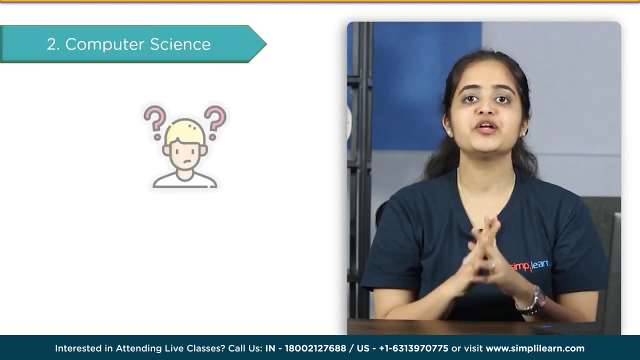 that are crucial to data science, Similar to that, knowing statistics is crucial because they are used in data analysis. Additionally important to statistics, probability is regarded as a must for mastering machine learning. Next is computer science. In the field of computer science, there is a lot to learn. 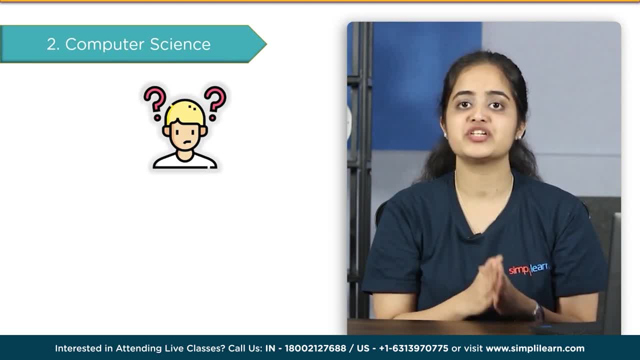 But one of the key inquiries that arises in relation to programming is R or Python language. There are many factors to consider when deciding which language to choose for data science, because both have a comprehensive collection of libraries to implement complex machine learning algorithms In addition to learning a programming language. 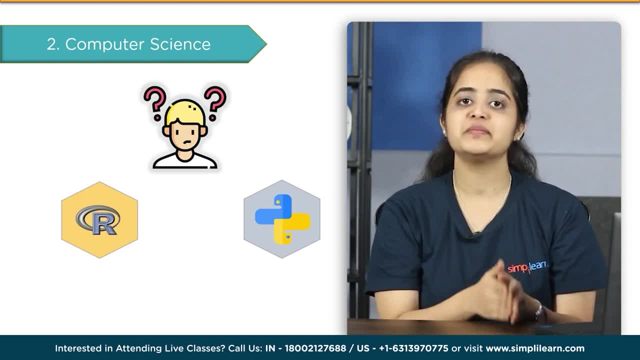 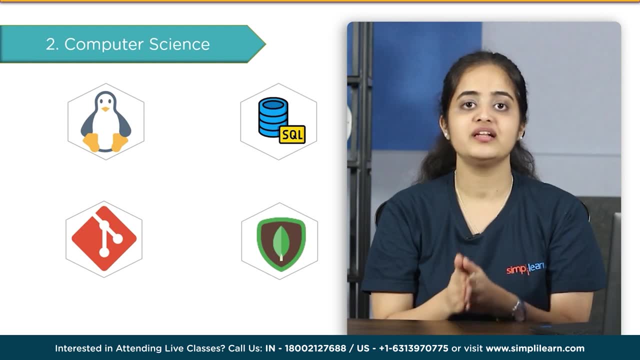 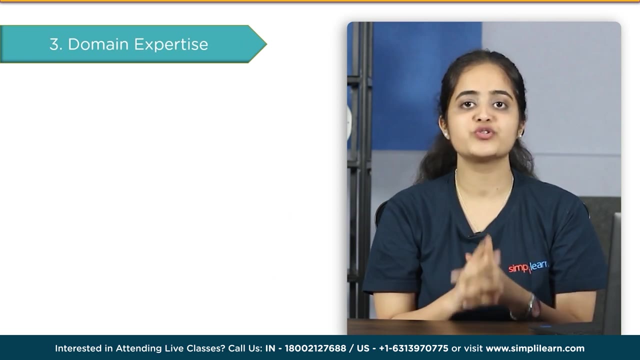 you should learn the following computer science skill: Fundamentals of algorithm and data structures, distributed computing, machine learning, deep learning, Linux, SQL, MongoDB, etc. Domain expertise: Most individuals strongly believe that domain expertise is not crucial to data science. 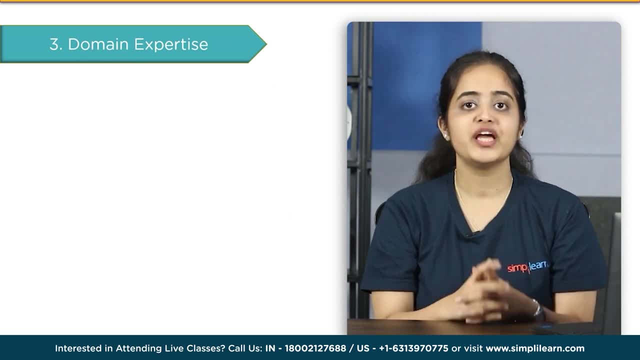 Yet it is. Consider the following scenario: If you are interested in working as a data scientist in a banking industry and you already know a lot about it- For instance, you are knowledgeable about stock trading, finance, etc- This will be very advantageous for you. 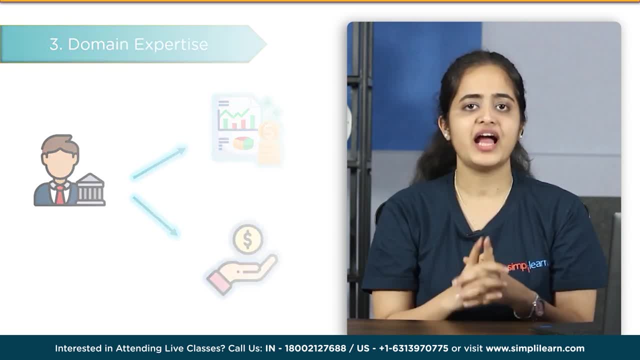 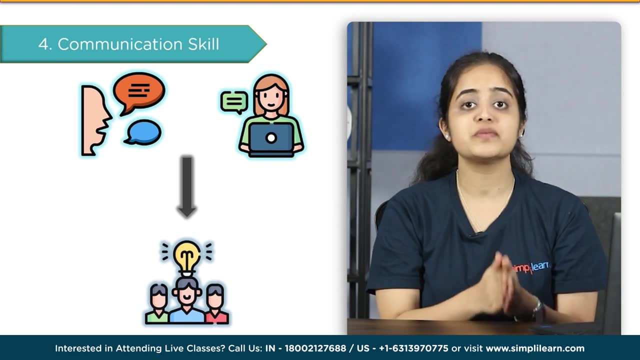 And the bank itself will favour you over other applicants. And finally, communication skill. It covers both spoken and written communication In a data science project. the project must be explained to others when findings from the analysis have been reached. This can occasionally be a report that you provide to your team or employer at work. 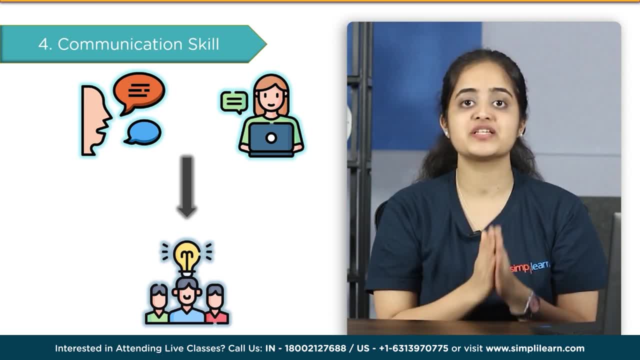 Sometimes it might be a blog entry. It is frequently a presentation to a group of co-workers. Regardless, a data science project always involves some form of communication of the project's findings. Therefore, having a good communication skill is a requirement for being a data scientist. 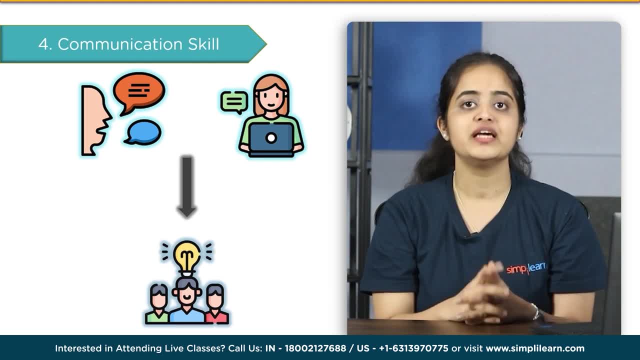 Apart from all this, practicing is very important. Keep using different tools. Also, start reading blogs on data science. Start building projects on data science which can be added to your resume. Also, you can find many interesting courses on data science by Simply Learn. 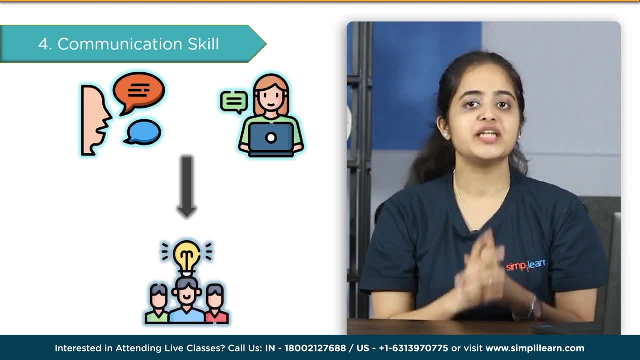 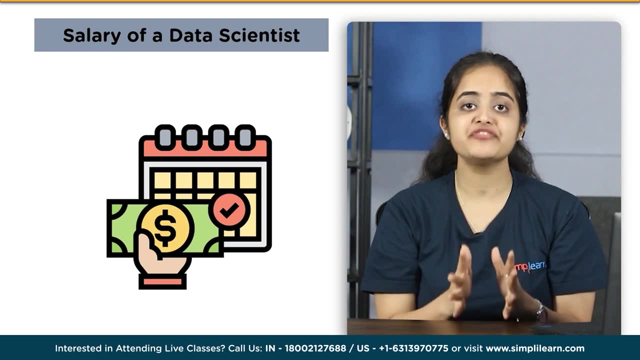 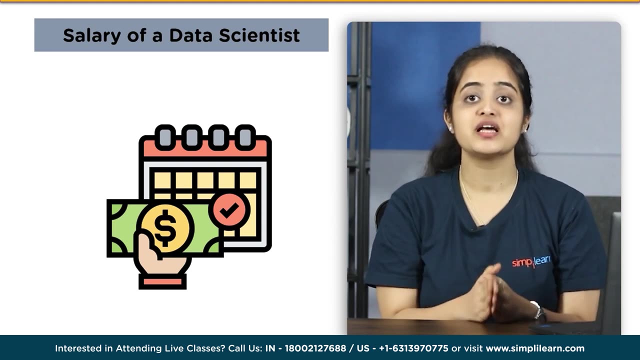 Salary reward. Salary reward is the result of good work. Now we shall discuss salaries that a data scientist will get. It should come as no surprise that data scientist may add significantly to a business. Every step of the process, from data processing to data cleansing, requires persistence. 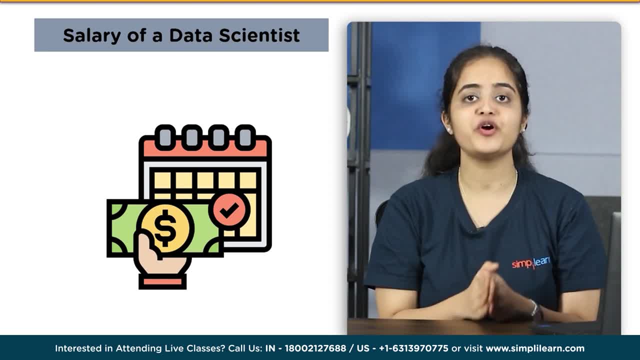 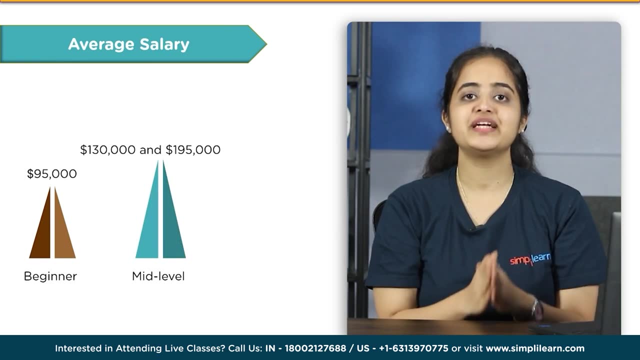 a lot of arithmetic and statistics, as well as scattering of engineering skills. One of the most important factors in a data scientist's salary is experience. At the beginner level, a data scientist can make $95,000 annually. The typical annual compensation for a mid-level data scientist is between $130,000 and $195,000. 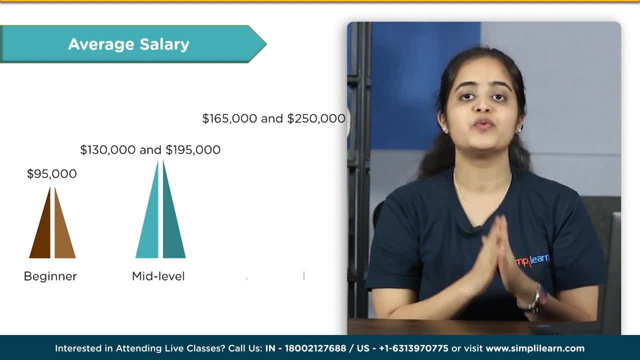 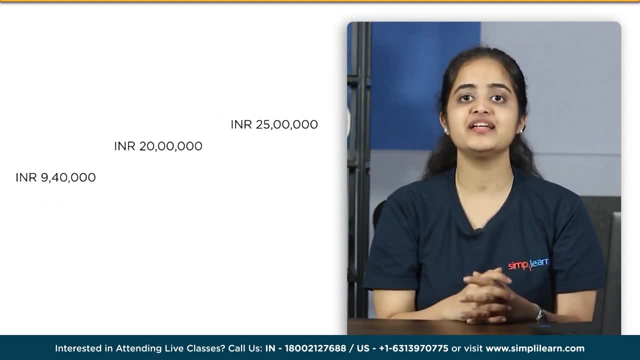 A seasoned data scientist typically earns between $165,000 and $250,000 per year In India. at the beginner level, a data scientist can make 9,40,000 rupees on average per year. At mid-level, a data scientist can make 20,00,000 rupees per year. And if you are at the advanced level, you will get paid an average of rupees 25,00,000 annually. This salary will vary in different countries. The top hiring businesses in the US that provide the highest salaries for data scientists are Apple, with $180,000 per year. 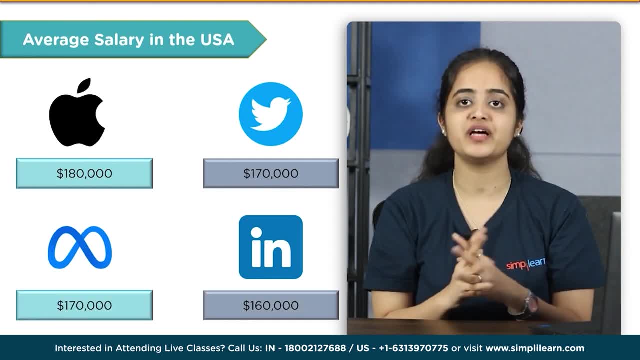 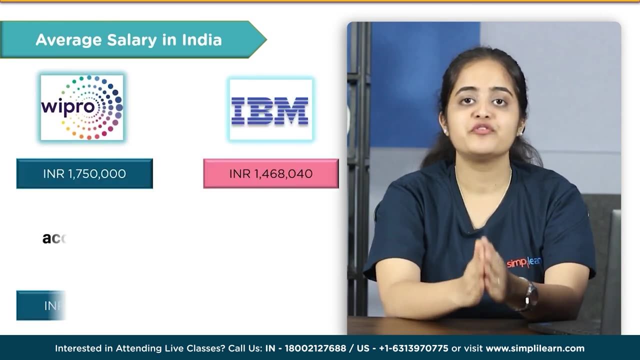 Next is Twitter, with $170 per year, Meta technology $170 annually, LinkedIn, $160,000 per annum. Wipro technology provides $17,50,000 per annum, IBM provides $14,00,000 per annum And Accenture will provide you with $19,00,000 per annum. And finally, American Express will provide on average of $13,00,000 per annum, What this buzz is all about. So now let's talk about the lifecycle of a data science project. Okay, The first step is the concept study. In this step, it involves understanding the business problem. 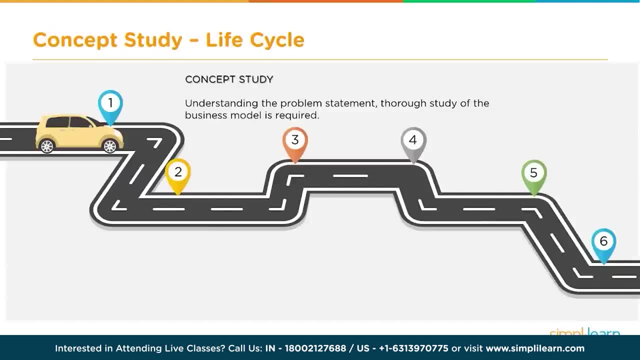 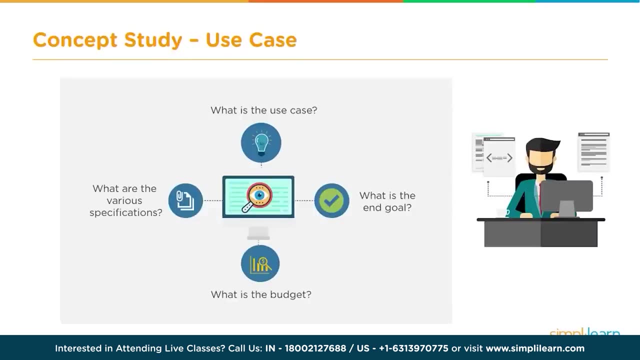 asking questions, get a good understanding of the business model, meet up with all the stakeholders, understand what kind of data is available, And all that is a part of the first step. So here are a few examples. We want to see what are the various specifications and then what is the end goal. 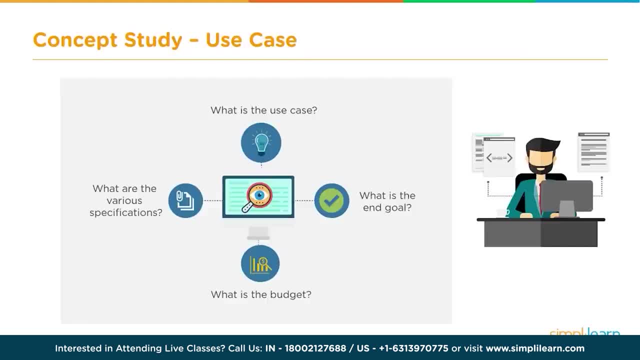 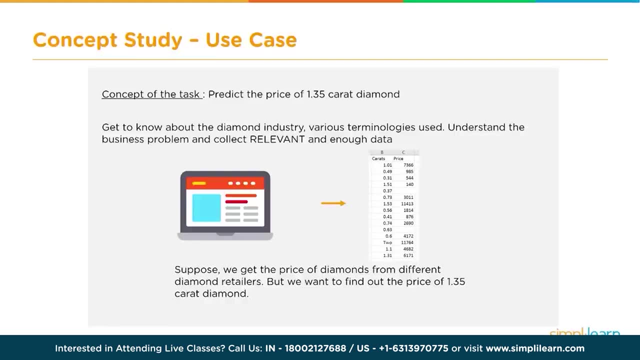 What is the budget? Is there an example of this kind of a problem that has been maybe solved earlier? So all this is a part of the concept study, And another example could be a very specific one: to predict the price of a 1.35 carat diamond. 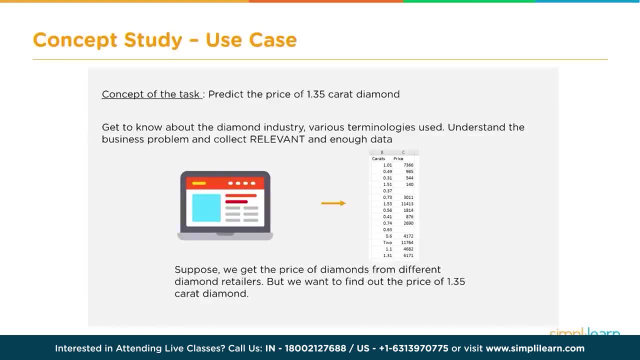 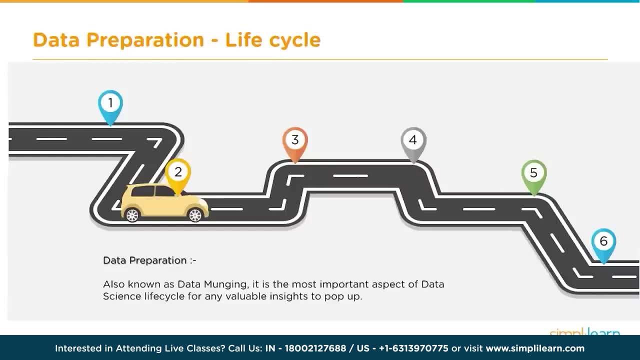 And there may be relevant information inputs that are available And we want to predict the price. The next step in this process is data preparation: data gathering and data preparation, also known as data munging, Or sometimes it is also known as data manipulation. 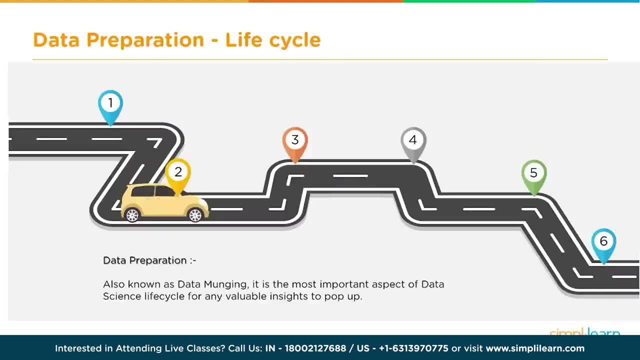 So what happens here is the raw data that is available may not be usable in its current format for various reasons. So that is why, in this step, a data scientist would explore the data. He will take a look at some sample data. Maybe there are millions of records. 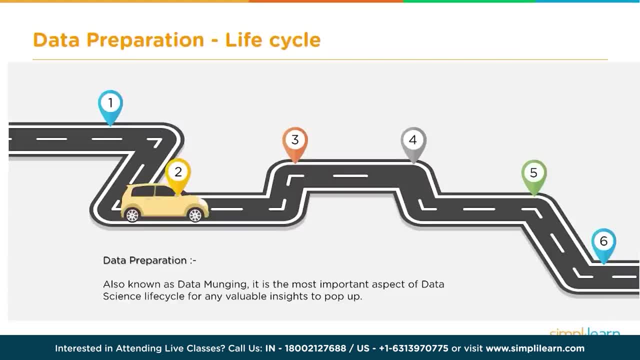 Pick a few thousand records and see how the data is looking. Are there any gaps? Is the structure appropriate to be fed into the data? Are there some columns which are probably not adding value may not be required for the analysis. Very often these are like names of the customers. 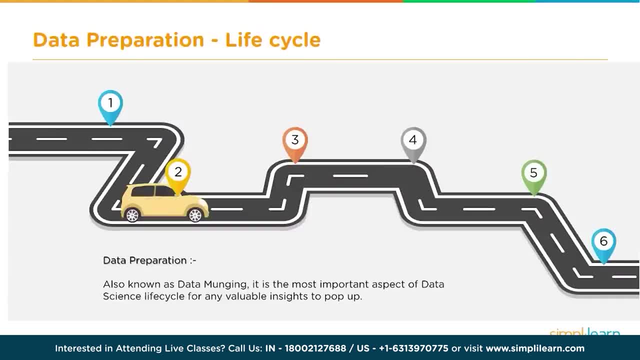 They will probably not add any value or much value from an analysis perspective. The structure of the data: maybe the data is coming from multiple data sources and the structures may not be matching. What are the other problems? There may be gaps in the data. 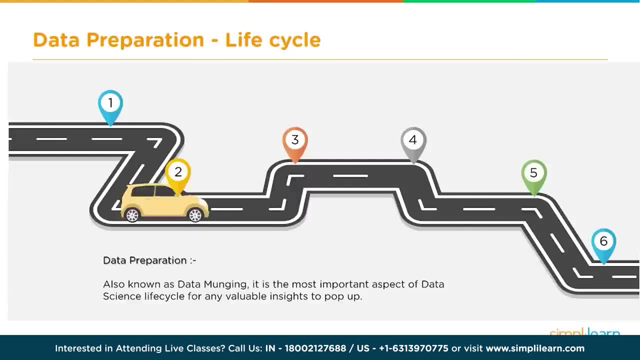 So the data, all the columns, all the cells are not filled. If you're talking about structured data, there are several blank records or blank columns. So if you use that data directly, you'll get errors or you will get inaccurate results. 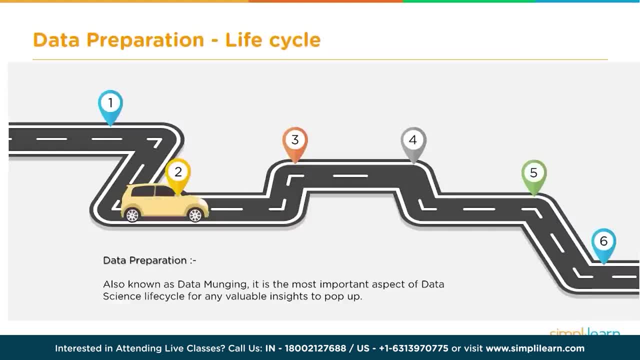 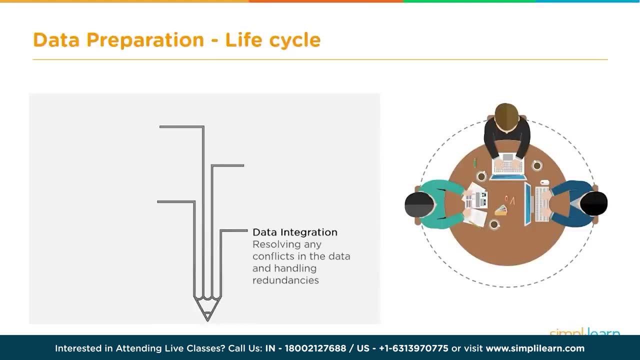 So how do you either get rid of the data or how do you fill those gaps with something meaningful? So all that is a part of data munging or data manipulation. So these are some additional subtopics within that. So data integration- Data integration is one of them. 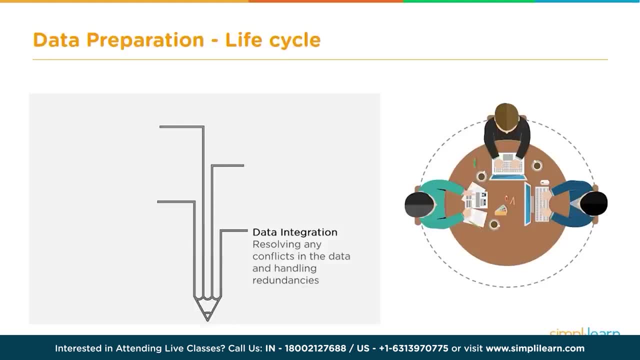 If there are any conflicts in the data there may be. data may be redundant. Data redundancy is another issue There may be. you have, let's say, data coming from two different systems and both of them have customer table, for example, customer information. 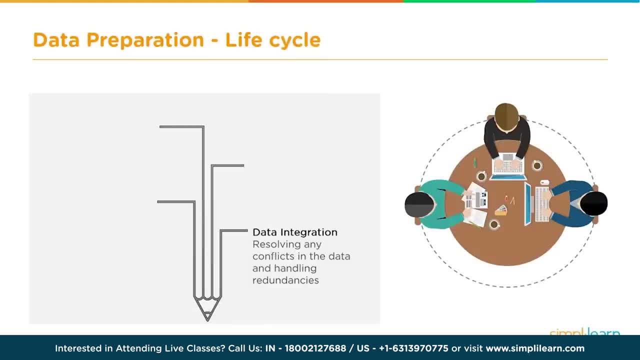 So when you merge them, there is a duplication issue. So how do we resolve that? So that is one Data transformation. As I said, there will be situations where data is coming from multiple sources And then when we merge them together, 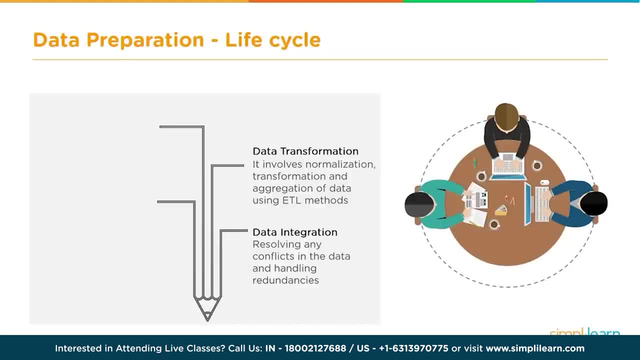 there will be matching, So we need to do some transformations to make sure everything is similar. We may have to do some data reduction. If the data size is too big, you may have to come up with ways to reduce it meaningfully without losing information. 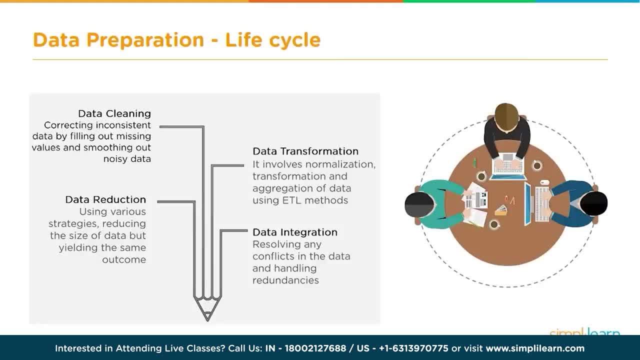 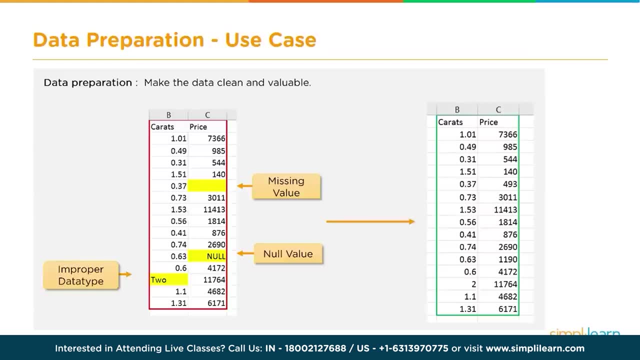 Then data cleaning. So there will be either wrong values or null values, or there are missing values. So how do you handle all of that? A few examples of very specific stuff. So there are missing values. How do you handle missing values Or null values? 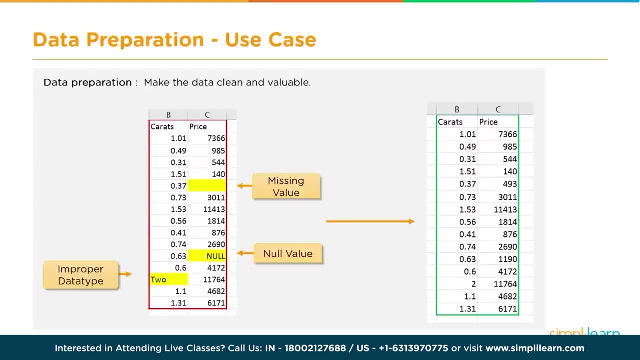 Here, in this particular slide, we are seeing three types of issues. One is missing value. Then you have null value. You see the difference between the two right. So in the missing value there is nothing, Blank Null value. it says null. 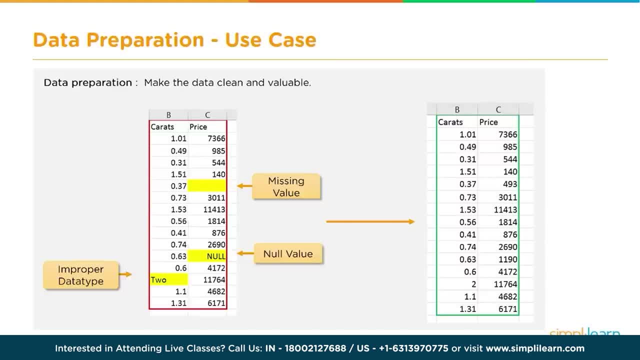 Now the system cannot handle if there are null values. Similarly, there is improper data, So it's supposed to be numeric value, but there is a string or a non-numeric value. So how do we clean and prepare the data so that our system can work flawlessly? 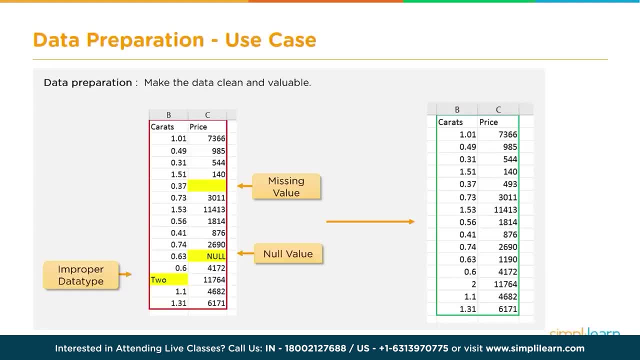 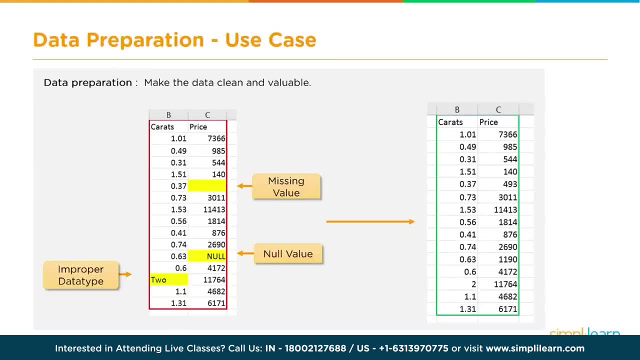 We need to clean the data. So there are multiple ways and there is no one common way of doing this. It can vary from project to project. It can vary from what exactly is the problem you're trying to solve. It can vary from data scientist to data scientist, organization to organization. 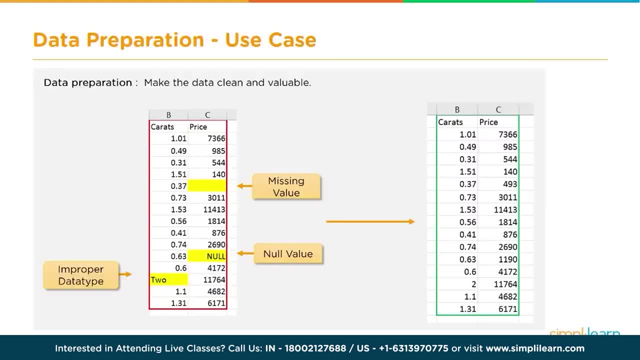 So these are, like some standard practices people come up with, And, of course, there will be a lot of trial and error. Somebody would have tried out something and it worked and will continue to use that mechanism, So that's how we need to take care of data cleaning. 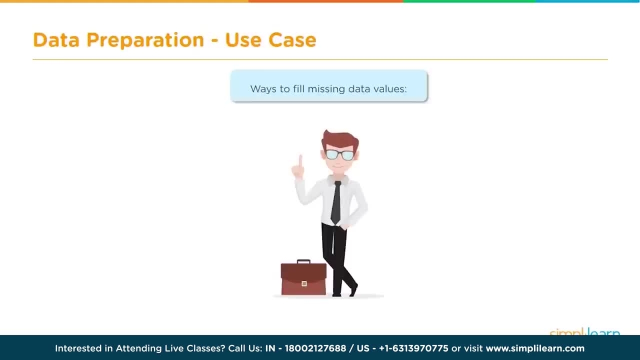 Now what are the various ways of doing? you know, if values are missing, how do you take care of that? Now, if the data is too large and only a few records have some missing values, then it is okay to just get rid of those entire rows, for example, 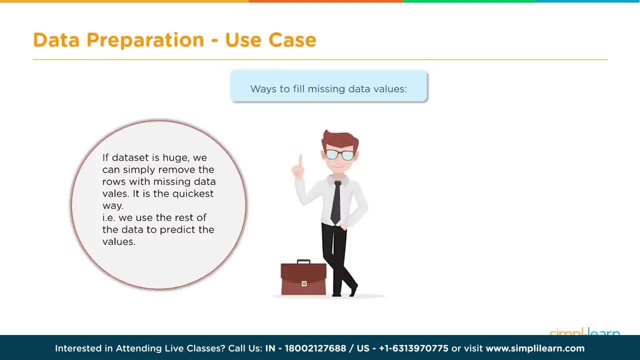 So if you have a million records and out of which 100 records don't have full data, so there are some missing values in about 100 records. So it's absolutely fine because it's a small percentage of the data, So you can get rid of the entire records which are missing values. 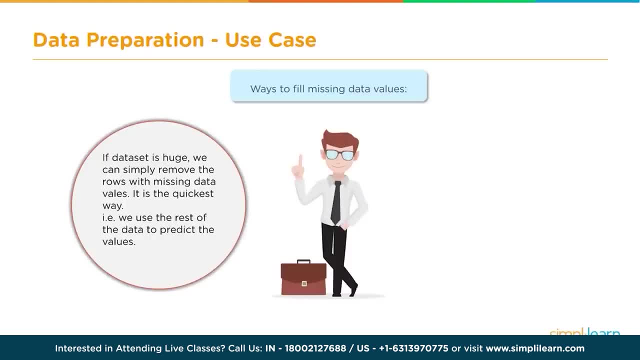 But that's not a very common situation. Very often you will have multiple or at least a large number of data set. For example, out of a million records, you may have 50,000 records, which are like having missing values. Now, that's a significant amount. 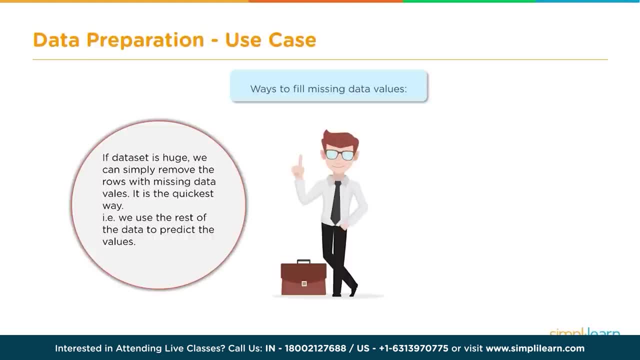 You cannot get rid of all those records, Your analysis will be inaccurate. So how do you handle such situations? So there are, again, multiple ways of doing it. One is you can probably, if a particular values are missing in a particular column, you can. 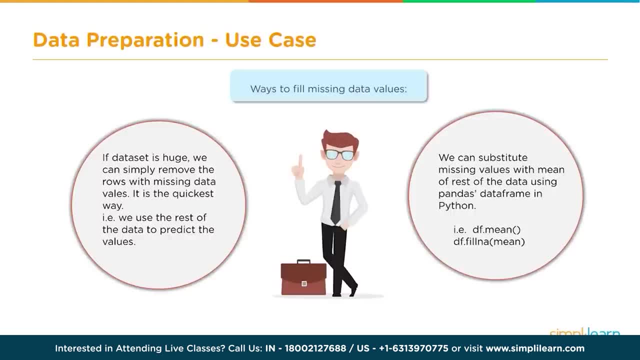 probably take the mean value for that particular column and fill all the missing values with the mean value, So that, first of all, you don't get errors because of missing values And, second, you don't get results that are way off because these values are completely. 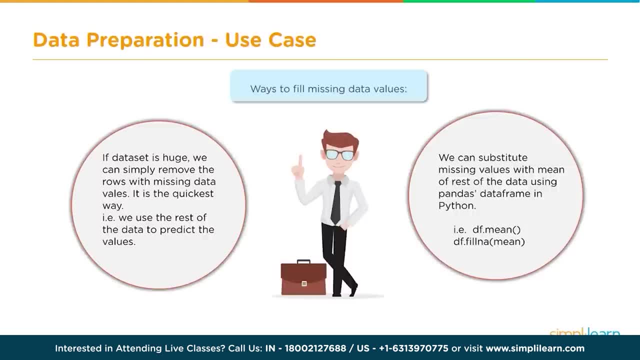 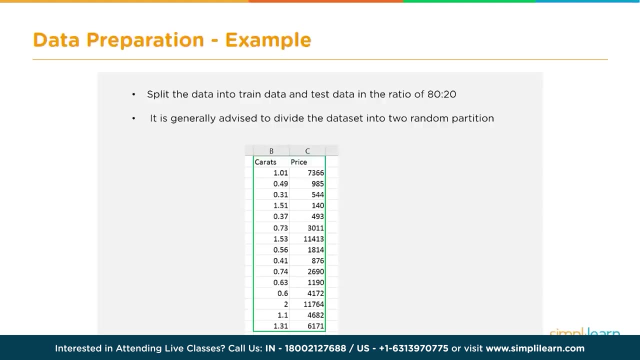 different from what is there. So that is one way. Then a few other could be, either taking the median value or, depending on what kind of data we are talking about, So something meaningful we will have put in there. If we are doing some machine learning activity, then obviously as a part of data preparation. 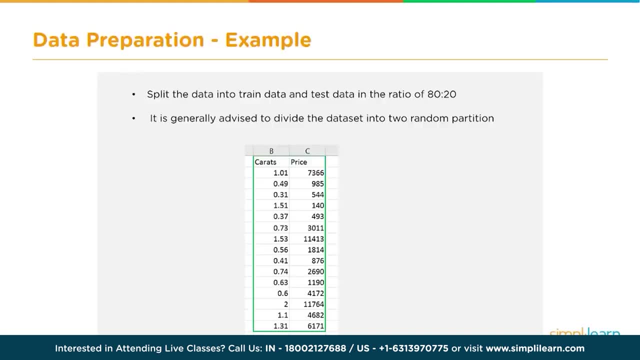 you need to split the data into training and test data set. The reason being, if you try to test with a data set which the system has already seen as a part of training, Then it will tend to give reasonably accurate results because it has already seen that data. 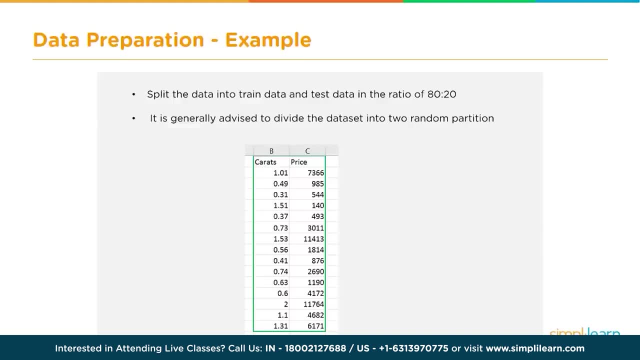 And that is not a good measure of the accuracy of the system. So typically you take the entire data set, the input data set, and split it into two parts And again the ratio can vary from person to person, individual preferences. Some people like to split it into 50- 50.. 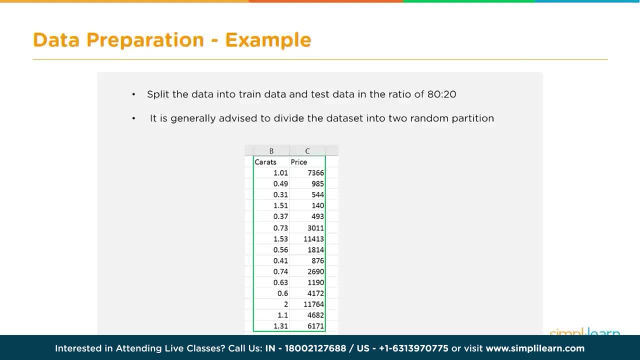 Some people like it as 63.33 and 33.3 is basically two thirds and one third, And some people do it as 80, 20,, 80 for training and 24 testing. So you split the data, perform the training with the 80% and then use the remaining 20%. 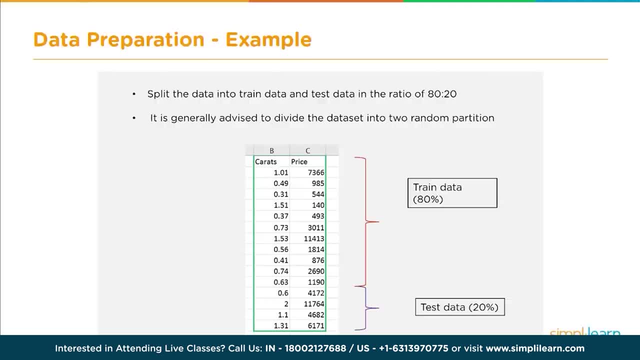 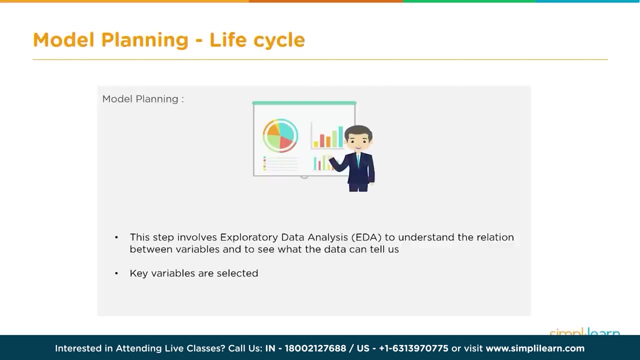 for testing. All right, So that is one more data preparation activity that needs to be done before you start analyzing or applying the data or putting the data through the model. Then the next step is model planning, or this models can be statistical models, This could be machine learning models. 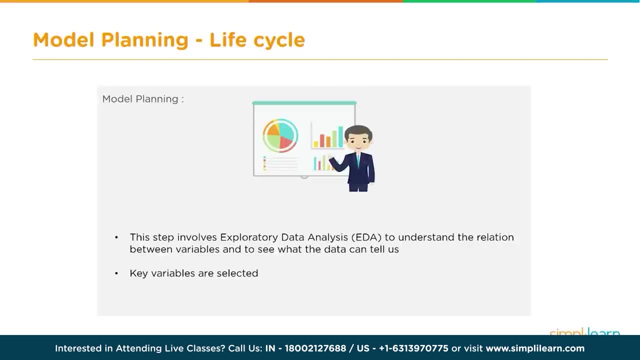 So you need to decide what kind of models you're going to use. Again, it depends on what is the problem you're trying to solve. If it is a regression problem, you need to think of a regression algorithm and come up with a regression model. 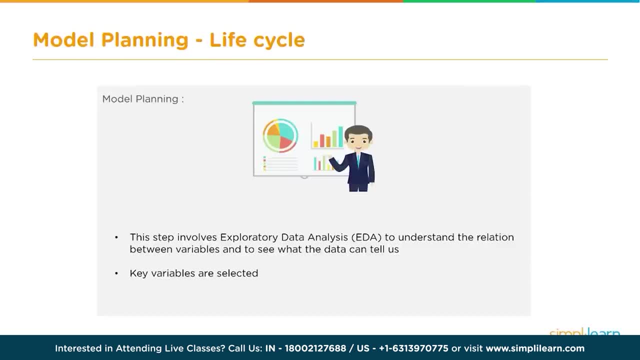 So it could be linear regression. or if you're talking about classification, then you need to pick up an appropriate classification algorithm, like logistic regression or decision tree or SVM, and then you need to train that particular model. So that is the model building or model planning process. 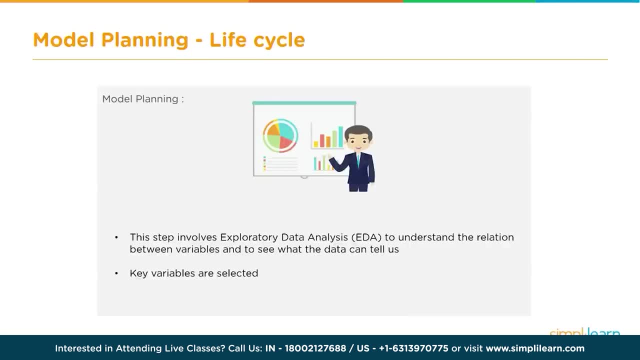 And the cleaned up data has to be fed into the model And, apart from cleaning, you may also have to in order to determine what kind of model you will use. you have to perform some exploratory data analysis to understand the relationship between the various variables and see if the data is appropriate, and so on, right. 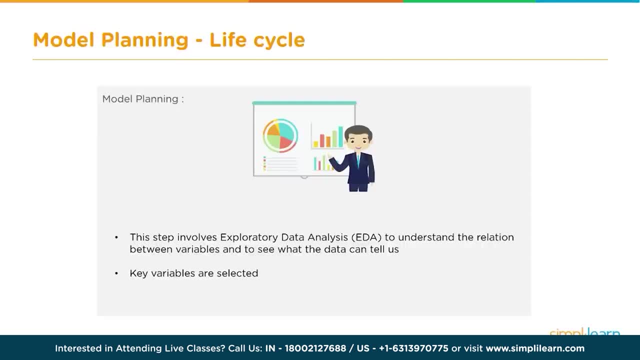 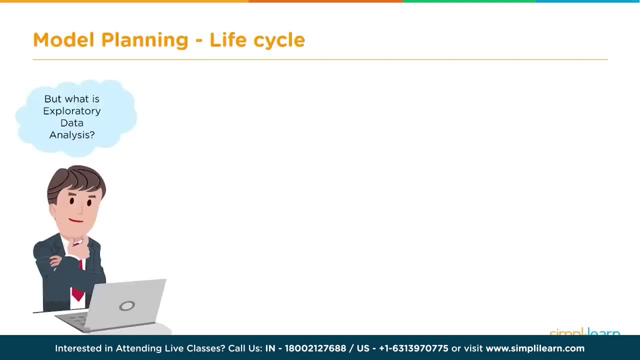 So that is the additional preparatory step that needs to be done. So, And then? what else about exploratory data analysis? So what exactly is exploratory data analysis? is basically to, as the name suggests, you're just exploring. you just receive the data and you're trying to explore and find out. 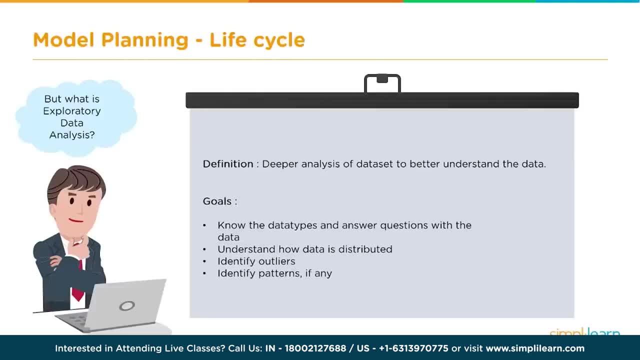 what are the data types and what is the? is the data clean in each of the columns? What is the maximum minimum value? So, for example, there are out of the box functionality available in tools like R. If you just ask for a summary of the table, it will tell you. for each column it will give some details. 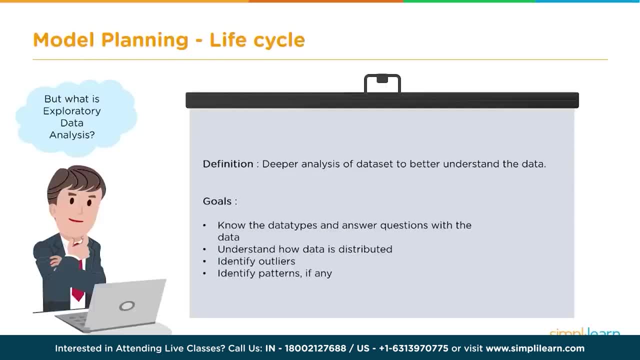 as to what is the mean value, what is the maximum value, and so on and so forth. So this exercise, or this exploratory analysis, is to get an understanding of your data And then you can take steps to. during this process, you find there are a lot of missing. 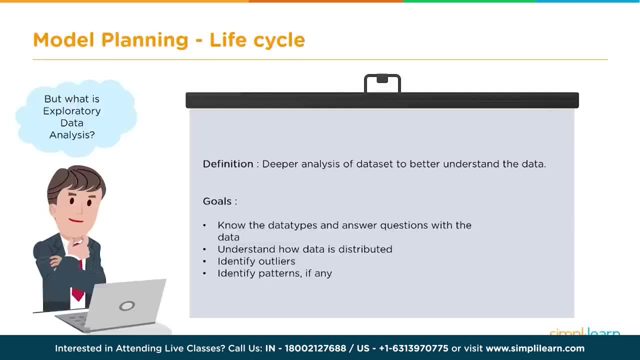 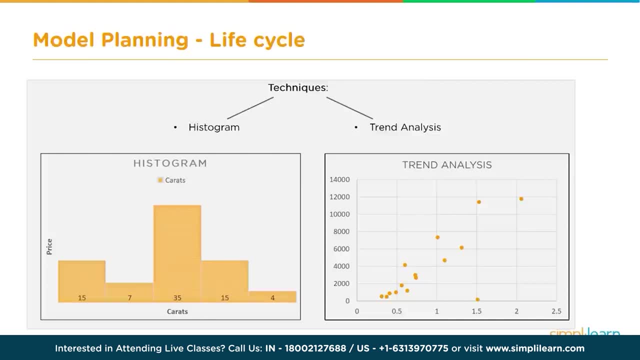 values. You need to take steps to fix those. You will also get an idea about what kind of model to be used, and so on and so forth. What are the various techniques used for exploratory data analysis? Typically, these would be visualization techniques. 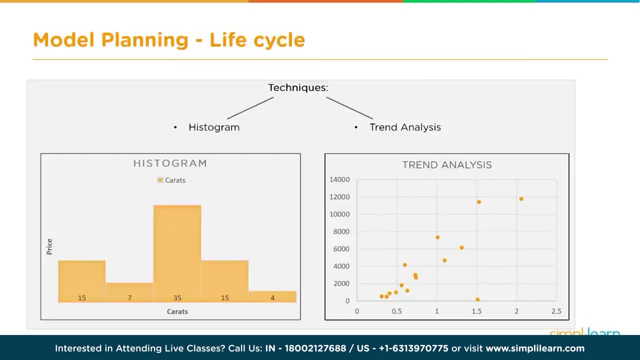 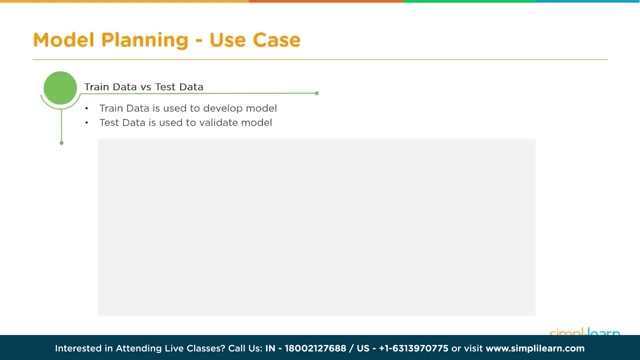 Like, you use histograms, You can use box plots, you can use scatter plots, So these are very quick ways of identifying the patterns or a few of the trends of the data, and so on. And then, once your data is ready, you decided on the model: what kind of model, what kind? 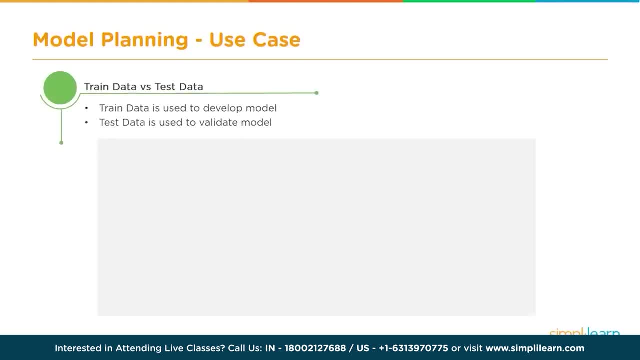 of algorithm you're going to use. If you're trying to do machine learning, you need to pass your 80% of the training data, or rather, you use that training data to train your model. The training process itself is iterative, So the training process you may have to perform multiple times. 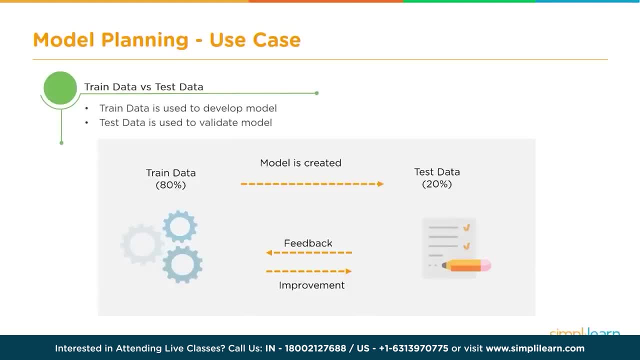 And once the training is done and you feel it is giving good accuracy, then you move on to test. So you take the remaining 20% of the data. Remember, we split the data into training and test. So the test data is now used to check the accuracy, or how well our model is performing. 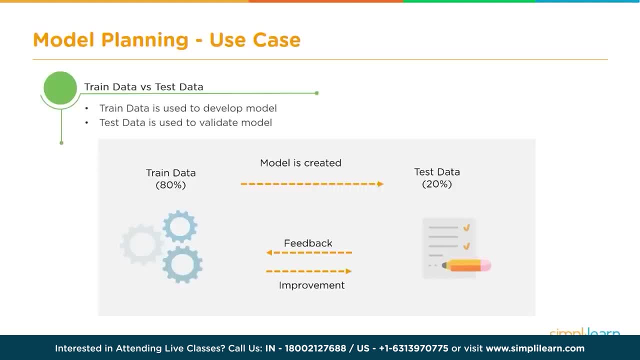 And if there are further issues- let's say, Okay, The model is still during testing and the accuracy is not good- Then you may want to retrain your model or use a different model. So this whole thing again can be iterative. But if the test process is passed, or if the model passes the test, then it can go into. 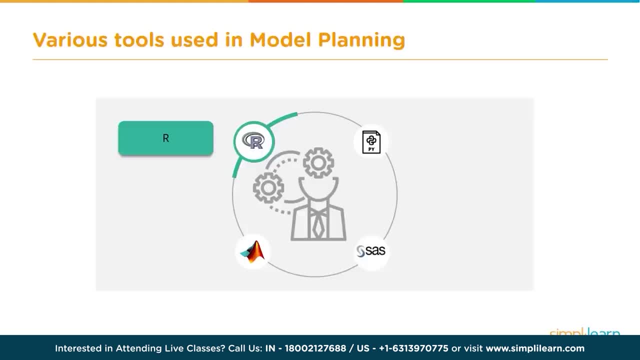 production and it will be deployed All right. So what are the various tools that we use for model planning? R is an excellent tool in a lot of ways, whether you're doing regular statistical analysis or machine learning or any of these activities are in. along with RStudio provides a very 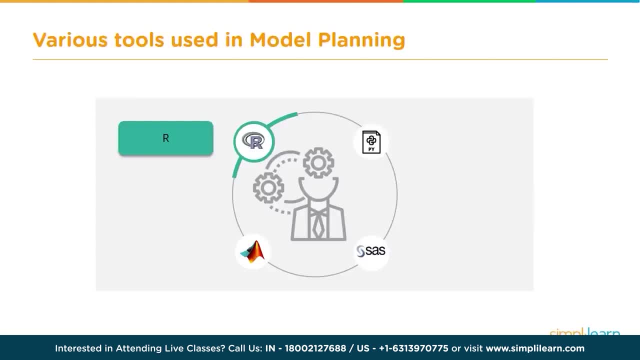 powerful environment to do data analysis, including visualization. It has a very good integrated visualization or plot mechanism which can be used for doing exploratory data analysis and then later on to do analysis, detailed analysis and machine learning, and so on and so forth. 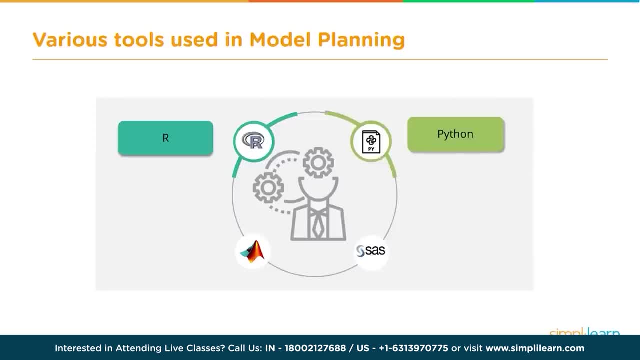 Then, of course, you can write Python programs. Python offers a rich library for performing data analysis. Okay, Python offers a rich library for performing data analysis and machine learning, and so on. MATLAB is a very popular tool as well, especially during education, So this is a very easy to learn tool. 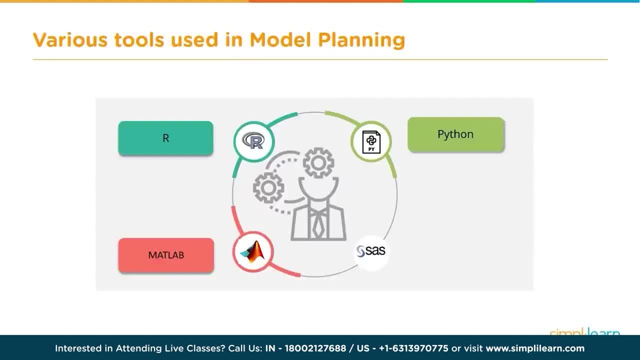 So MATLAB is another tool that can be used. And then, last but not least, SAS. SAS is again very powerful, It is a proprietary tool and it has all the components that are required to perform very good statistical analysis or perform data science. So those are the various tools. 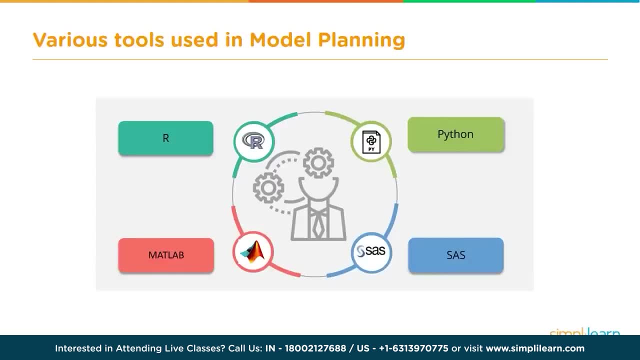 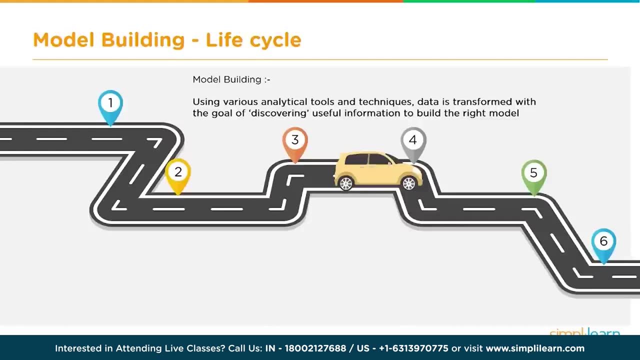 That would be required for, or that can be used for, model building. And so the next step is model building. So we have done the planning part. We said, okay, what is the algorithm we are going to use, What kind of model we are going to use? 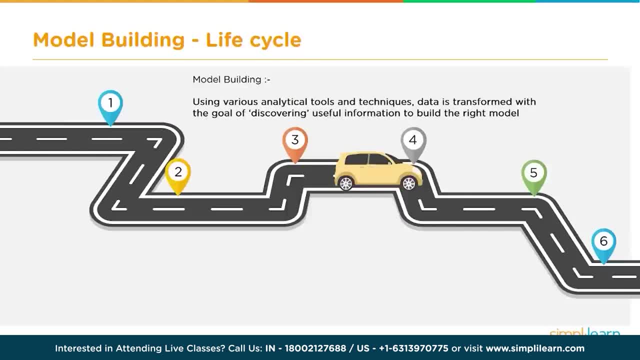 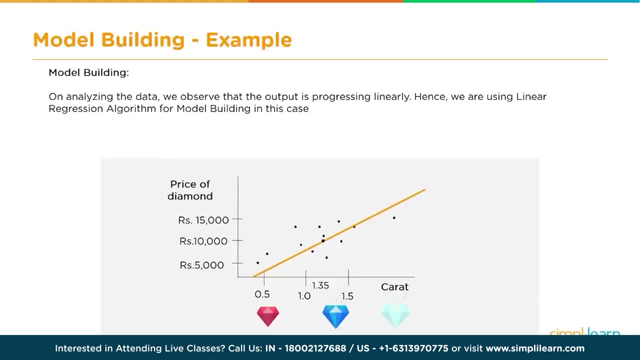 Now we need to actually train this model, or build the model, rather, so that it can then be deployed. So what are the various ways or what are the various types of model building activities? So It could be, In this particular example that we have taken, you want to find out the price of 1.35 carat. 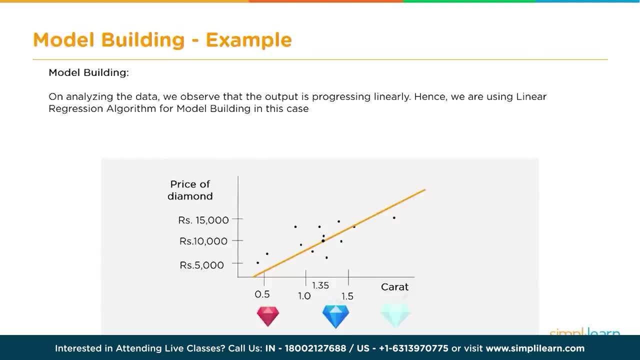 diamond. So this is, let's say, a linear regression problem. You have data for various carats of diamond and you use that information, You pass it through a linear regression model or you create a real linear regression model which can then predict your price for 1.35 carat. 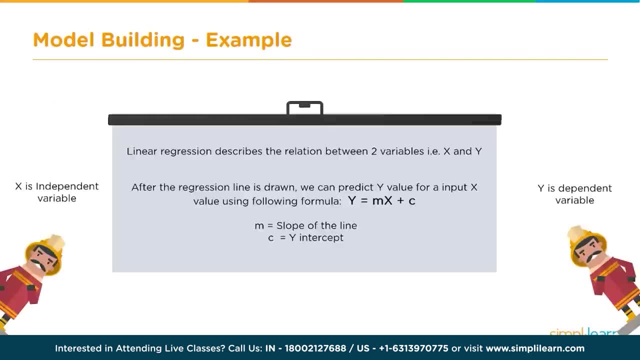 So this is one example Of model building and then a little bit details of how linear regression works. So linear regression is basically coming up with a relation between an independent variable and a dependent variable, So it is pretty much like coming up with equation of a straight line which is the best fit. 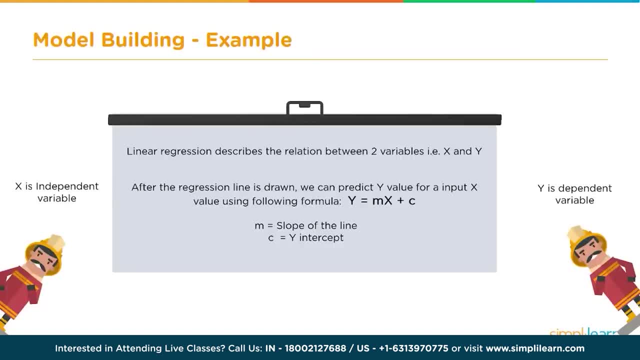 for the given data. So like for example here: Y is equal to MX plus C. So Y is the dependent variable and X is the independent variable To determine the values of M and C for our given data. So that is what the training process of this model does. at the end of the training process, 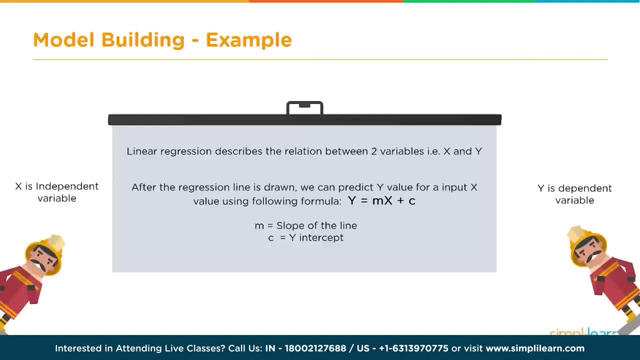 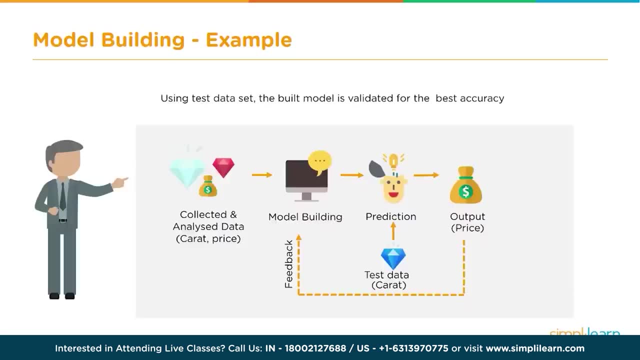 you have a certain value of M and C and that is used for predicting the values of any new data. that comes All right. So the way it works is we use the training and the test data set to train the model and then validate. Okay, 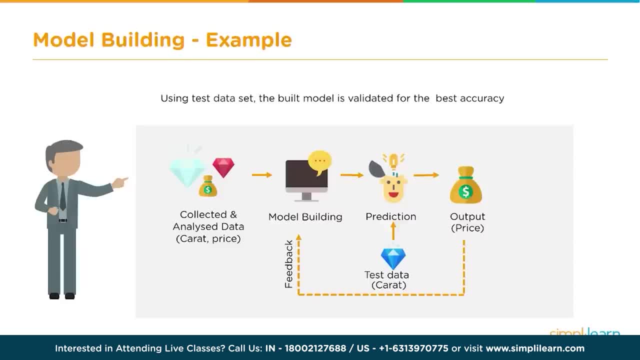 So the training problem is whether the model is working fine or not, using test data. And if it is working fine, then it is taken to the next level, which is put in production. If not, the model has to be retrained. If the accuracy is not good enough, then the model is retrained, maybe with more data or 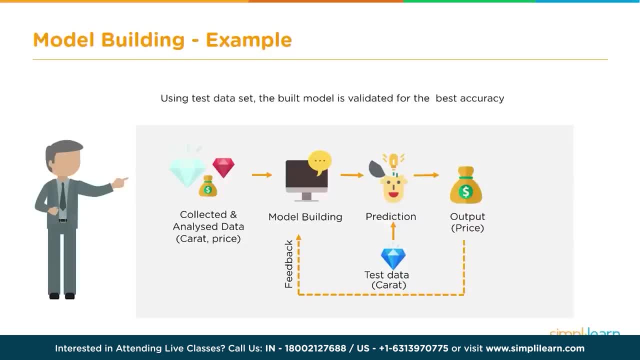 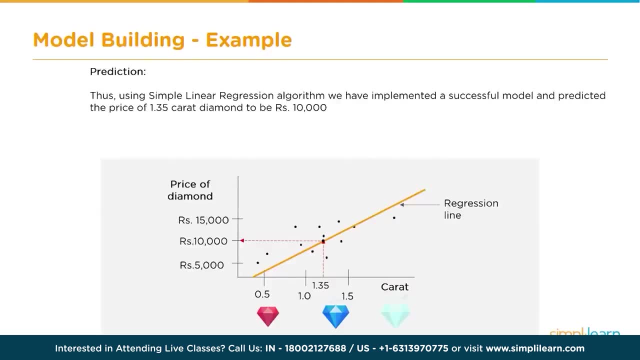 you come up with a newer model or algorithm and then repeat that process. So it is an iterative process. Once the training is completed- training and test- Then this model is deployed and we can use this particular model to determine what is the price of 1.35 carat diamond. Remember, 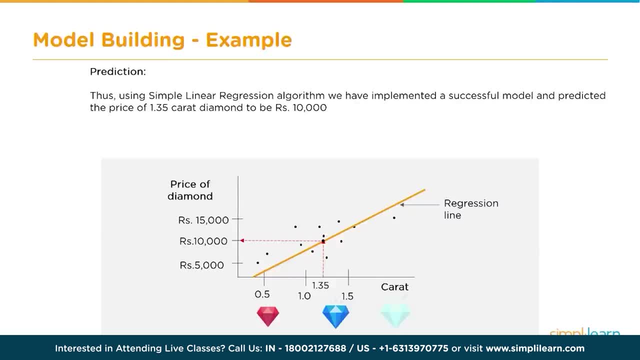 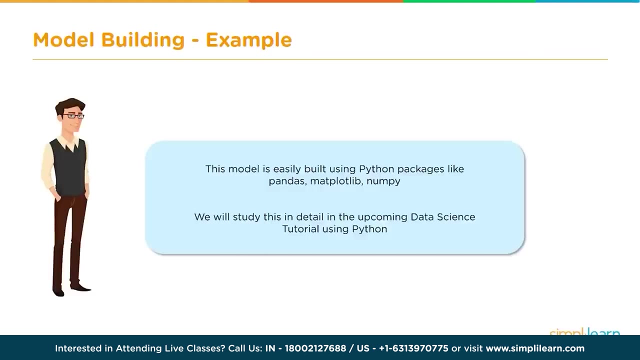 that was our problem statement. So now that we have the best fit for this given data, we have the price of 1.35 carat diamond, which is 10,000.. So this is one example of how this whole process works. Now how do we build the model? There are multiple ways. You can use Python, for example. 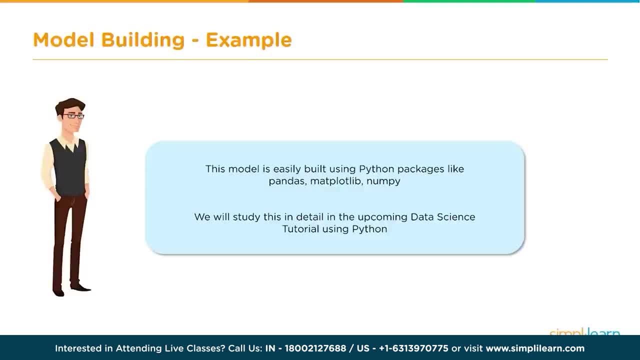 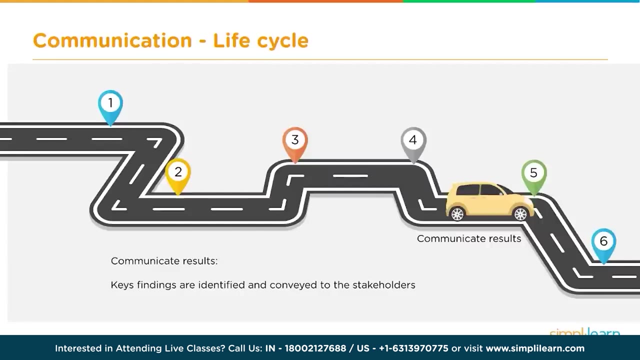 and use libraries like Pandas or NumPy to build a model and implement it. This will be available as a separate tutorial, a separate video in this playlist. So stay tuned for that Moving on. once we have the results, the next step is to communicate these results to the appropriate. 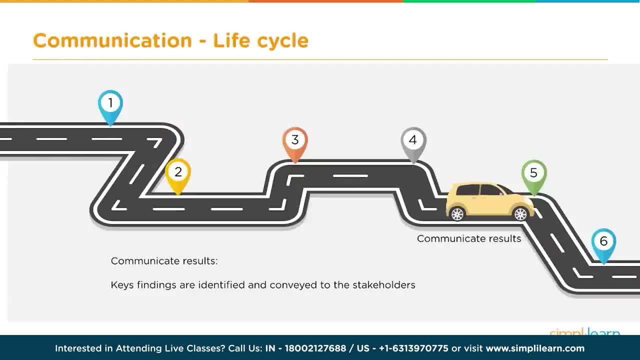 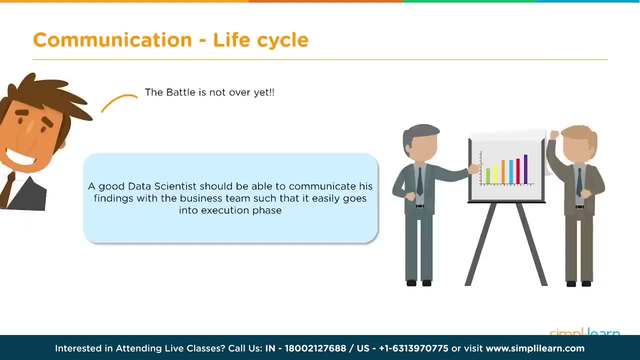 stakeholders. So it is basically taking these results and preparing like a presentation or a dashboard and communicating these results To the concerned people. So finishing or getting the results of the analysis is not the last step, but you need to, as a data scientist, take these results and present it to the team that has given. 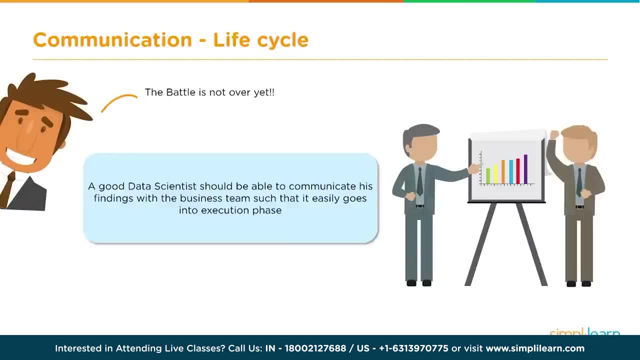 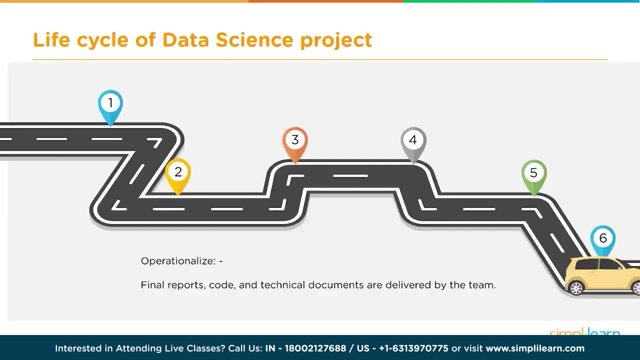 you this problem in the first place and explain your findings, explain the findings of this exercise and recommend maybe what steps they need to take in order to overcome this problem or solve this problem. So that is the pretty much. once that is accepted, The last step is to operationalize. So, if everything is fine, your data scientist. 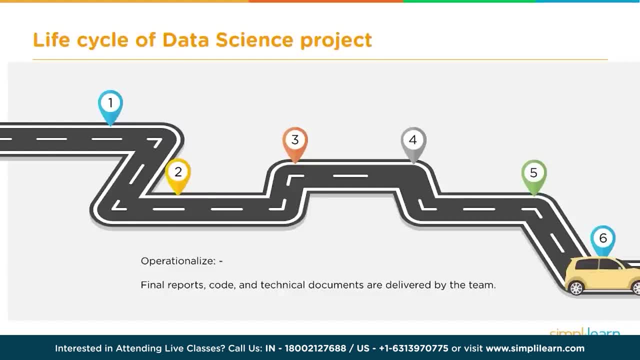 presentations are accepted, then they put it into practice and thereby they will be able to improve or solve the problem that they stated in step one. Okay, so quick summary of the life cycle. You have a concept study, which is basically understanding the problem, asking the right. 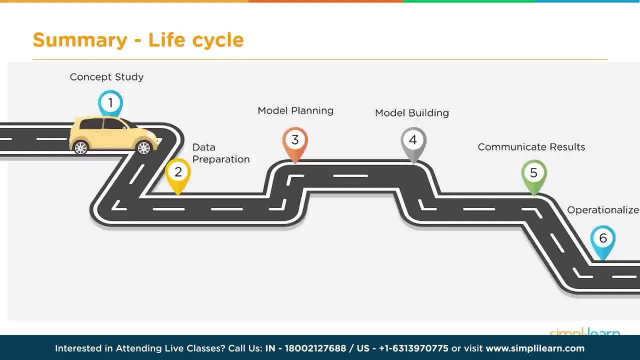 questions and trying to see if there is enough data to solve this problem and then even maybe gather the data. Then data preparation, the raw data needs to be manipulated, need to do data munging so that you have the data in a certain proper format to be used by the model or our analytics system, And then you need 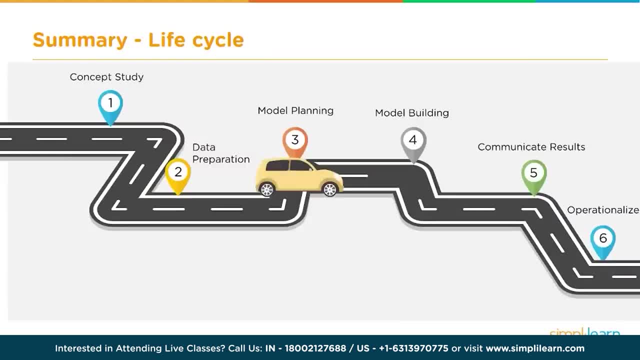 to do the model planning- what kind of a model, what algorithm you will use for a given problem- and then the model building. So the exact execution of that model happens in step four and you implement and execute that model and put the data through the analysis in this step and then you get the results. These results are then: 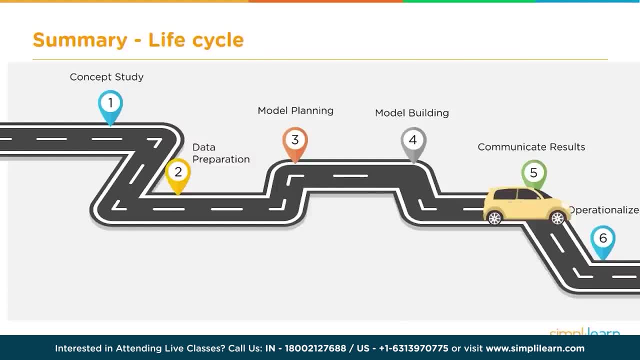 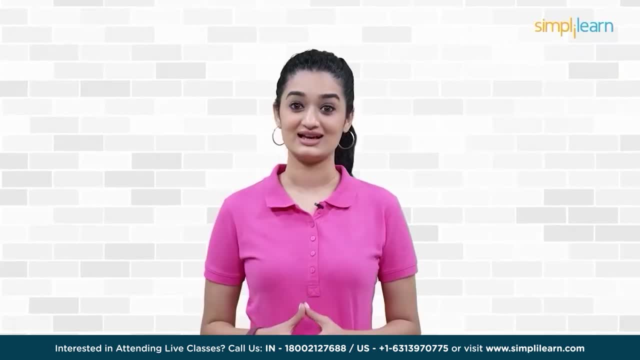 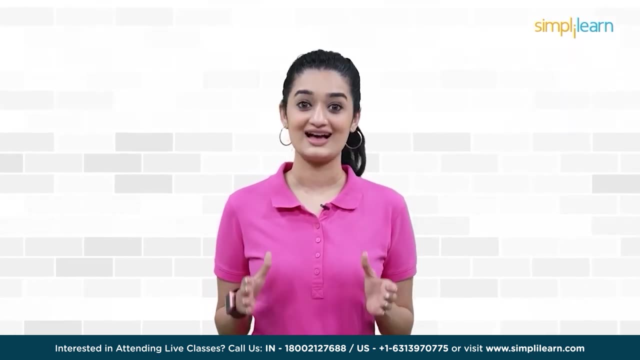 communicated, packaged and presented and communicated to the stakeholders And once that is accepted, that is operationalized. So that is the final step. Data scientist is one of the hottest, highest paid and most enthusiastic job roles in the current IT industry. Business organizations are actively hiring professionals who could collect data, analyze the market to 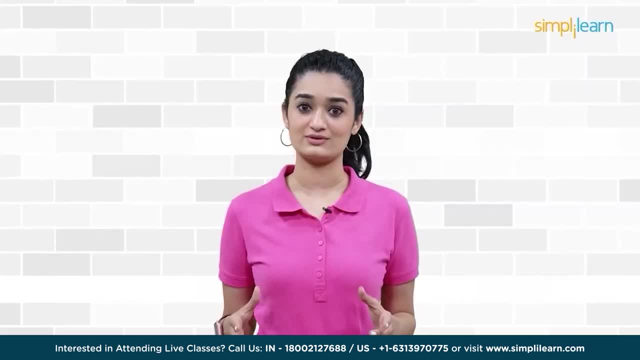 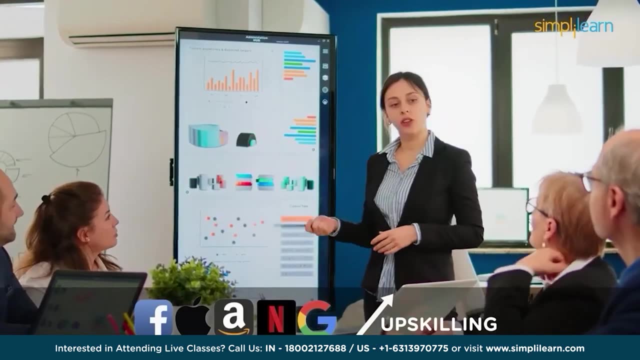 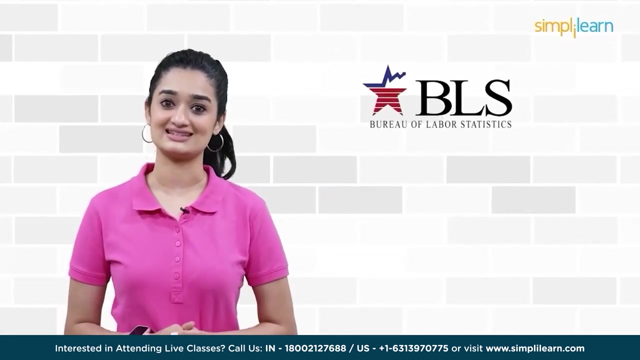 help the companies diagnose and overcome economic barriers to lead the industry. many mncs, including the fan companies, are actively upskilling their employees to bridge the gap in the world of fast space and intelligent technologies. according to the us bureau of labor statistics, now is the best. 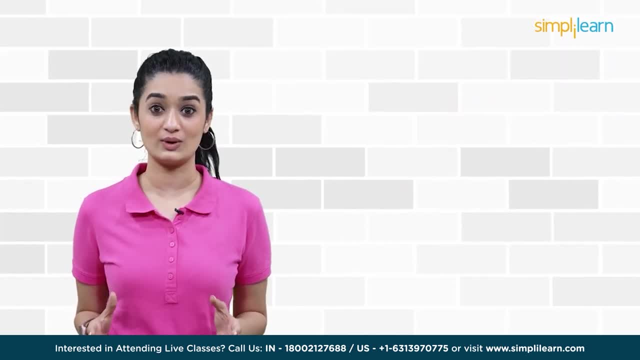 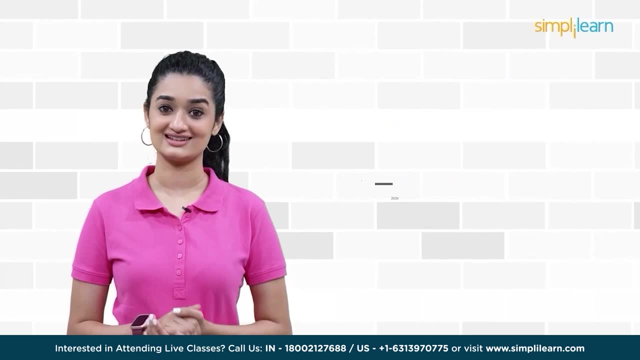 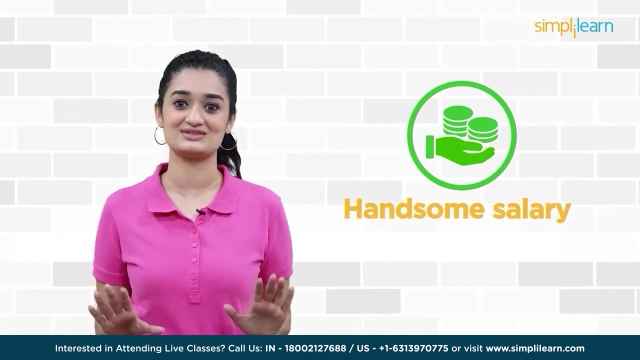 time to start a career in data science, as the number of jobs requiring data science skills alone is expected to grow by 27.9 by 2026.. the potential recruiters are actively looking for data scientists and are willing to compensate their employees with handsome salaries. according. to the leading websites like, indeed, glassdoor, nokri and linkedin. the average salary of a data scientist is anywhere between 10 lakhs rupees to as high as 80 lakh rupees per annum in india. depending on your experience in the united states of america, the salary of a data scientist ranges from hundred thousand dollars to 250 000. 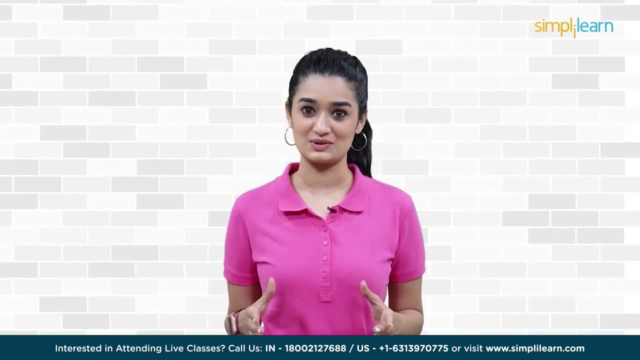 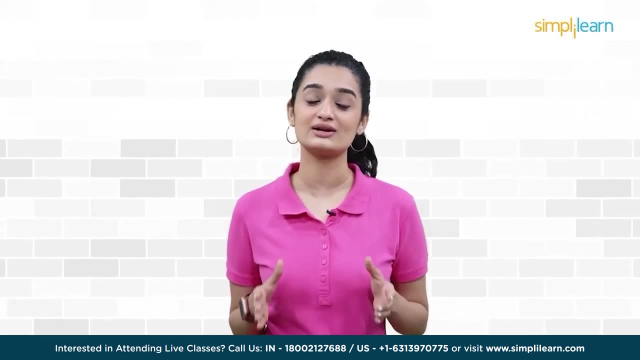 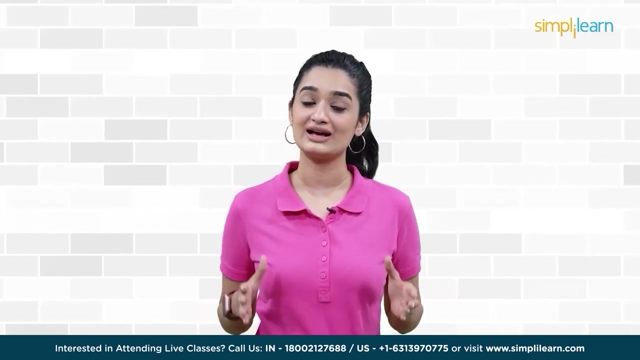 per annum on an average. should you be interested in becoming a successful data scientist, but don't know how, don't you worry, as we have got you covered with our rigorous survey reports, which will help you to not only choose from the top 10 data scientist certifications, but will also. 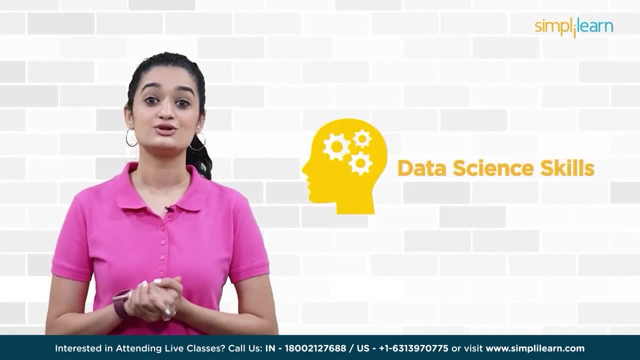 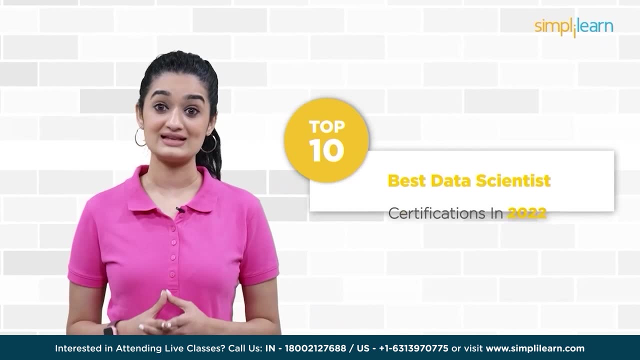 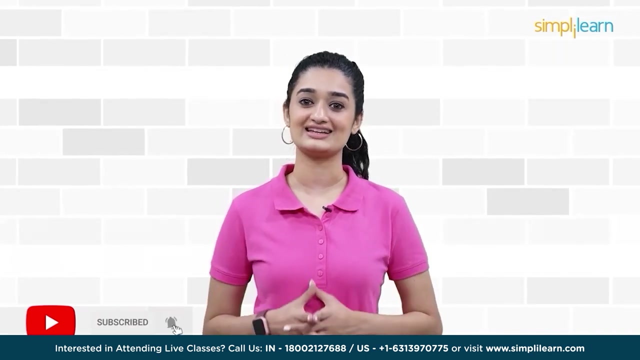 help you develop and enhance your data science skills to give your career the boost they deserve. so, without much further ado, let's get started with the top 10 best data scientist certifications in 2022. while we are at it, please feel free to get subscribed and hit the bell icon to keep yourself. 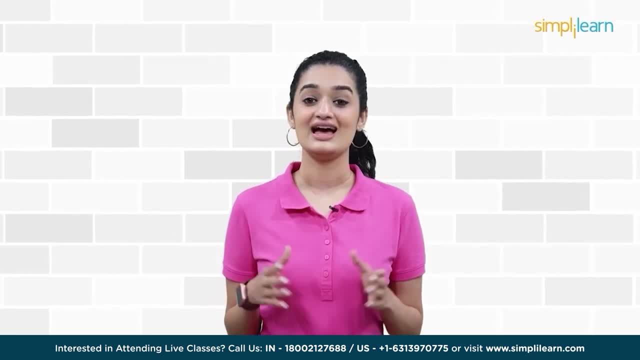 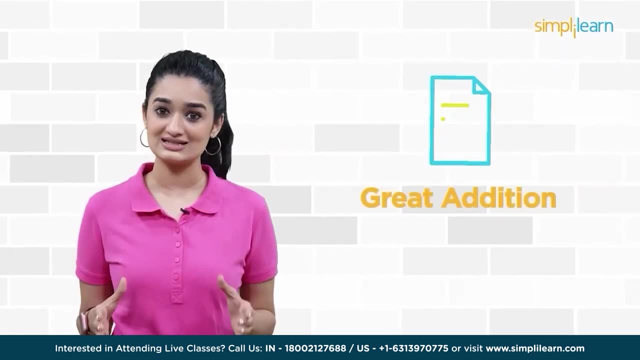 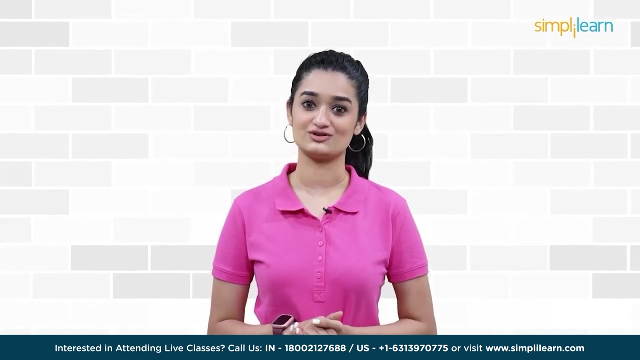 updated with the latest id trends in the industry. at number 10 we have cap, which is aka certified analytics professional will be a great addition to your resume, as the certification is valued by many driven organizations. if you're looking forward to becoming a data scientist, this certification is 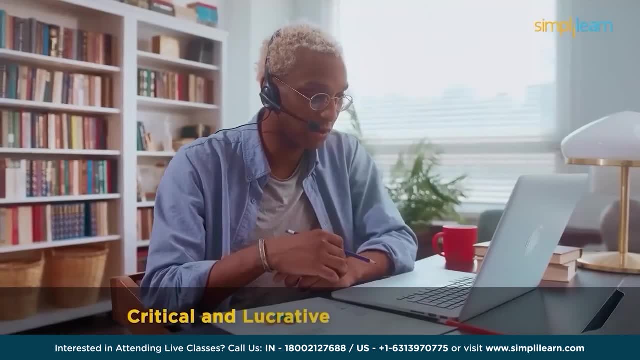 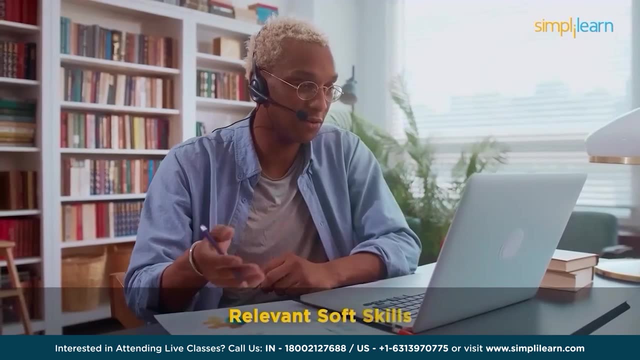 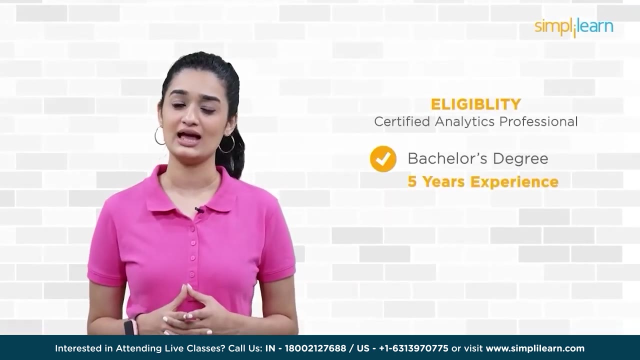 proof that you possess the critical and lucrative technical expertise, understand risk management, information security procedures and possess relevant soft skills required by a data science and analytics professional: aspiring data scientists with a bachelor's degree and five years of professional analytical experience, or master's degree with three years of experience. 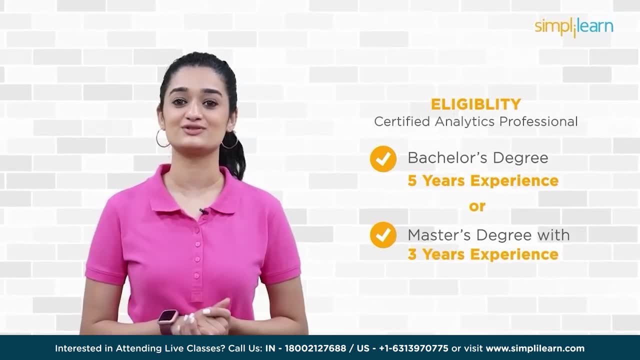 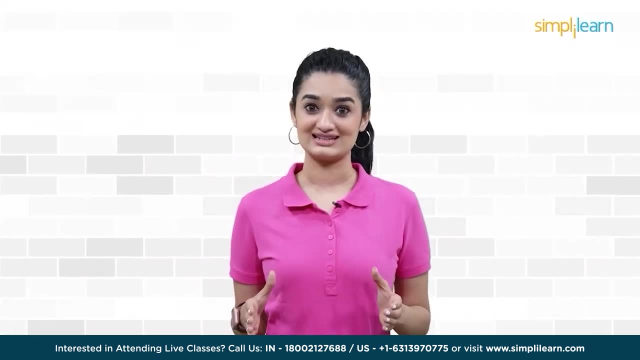 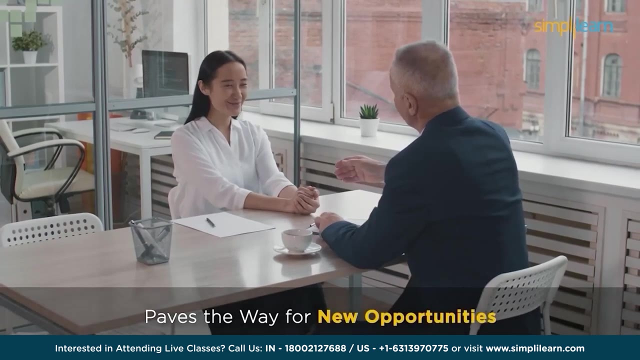 experience or master's degree with three years of experience or master's degree with three years of experience are eligible to face cap certification exam. there are numerous benefits to the certification. apart from getting exposure to new and updated technical skills, the certification also paves way for new opportunities, as the certification proves your credibility. 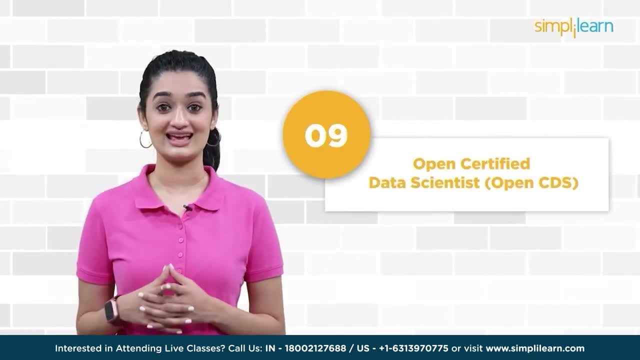 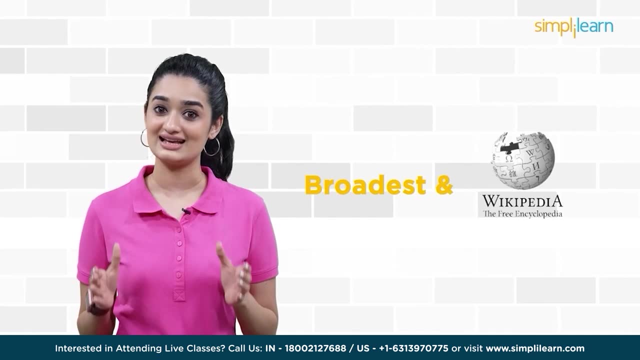 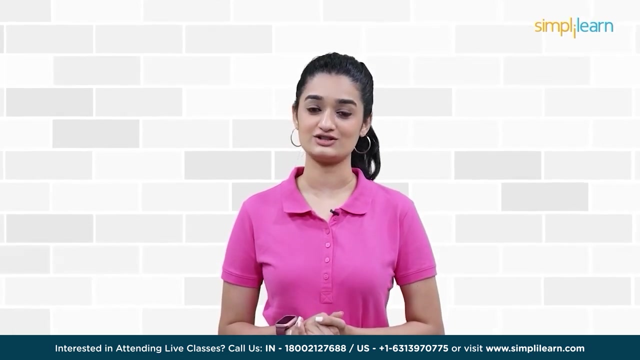 for the role we have. the open certified data scientist, aka open cds on number nine, open cds is considered the broadest and encyclopedic certification for a data scientist. Organizations choose OpenCV as certified professionals to fill up the most critical job roles responsible for. 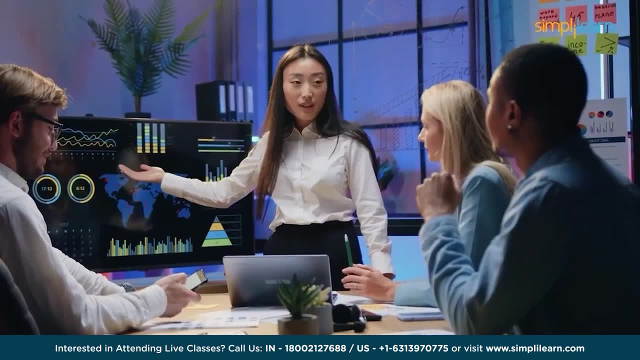 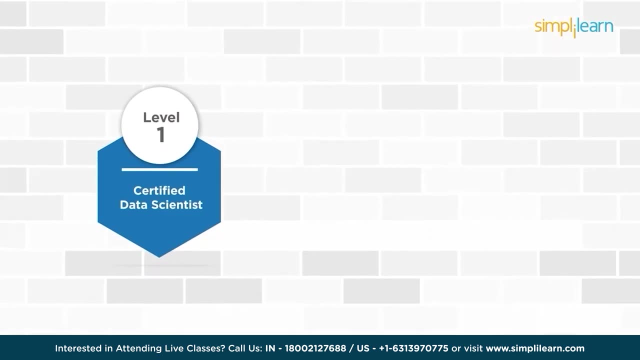 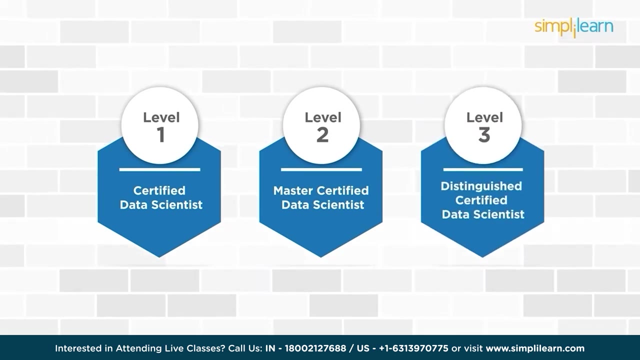 producing an effective analysis of data to improve the business. The certification is available in three different levels: Level 1- certified data scientist. level 2- master certified data scientist. level 3- distinguished certified data scientist. However, there is a prerequisite for candidates where the 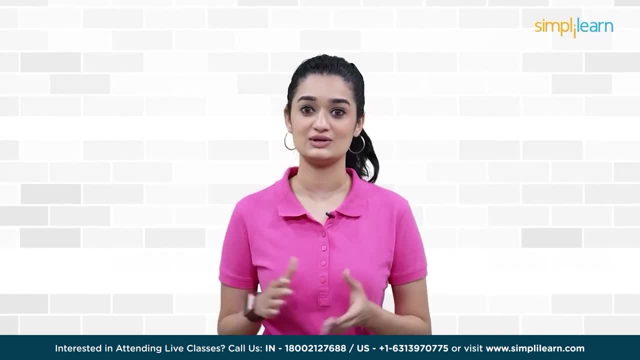 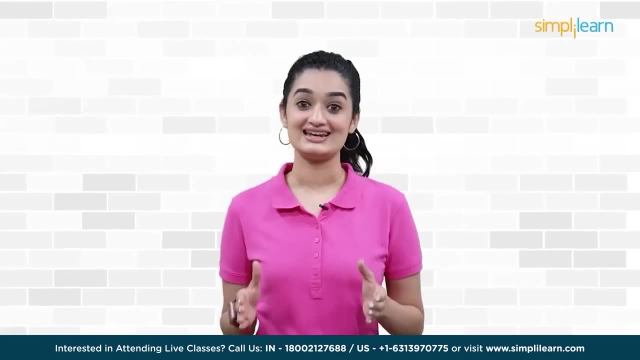 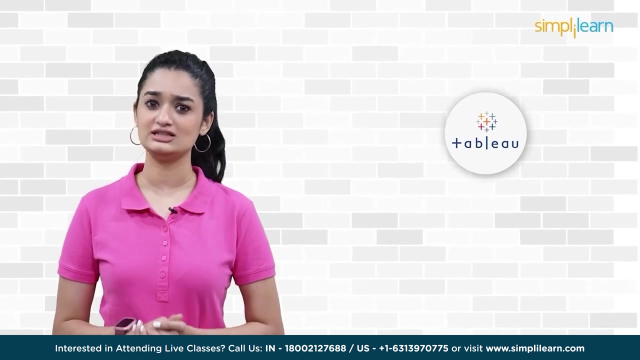 applicants are expected to demonstrate skills and experience against a set of conformance frequency requirements through written applications and peer interviews. next on our list is an interesting one: tablu. data scientist and desktop specialist. tablu is one of the leading business intelligence tools, leading in. 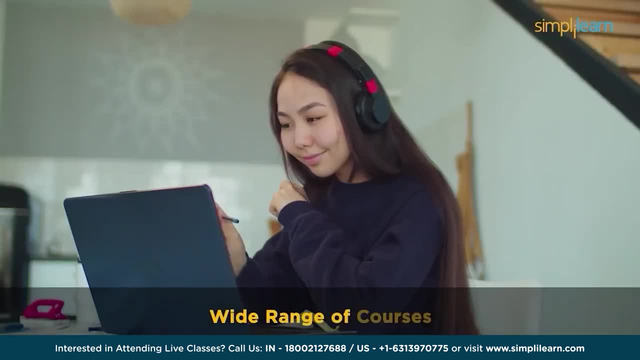 Gartner's Quatrates. tablu offers a wide range of courses and offers core courses from the need to bargain to many workforce talented percentile Journaling. Justinson is one of the leading business intelligence tools leading in darkness. votre tableau offers a wide range of courses and 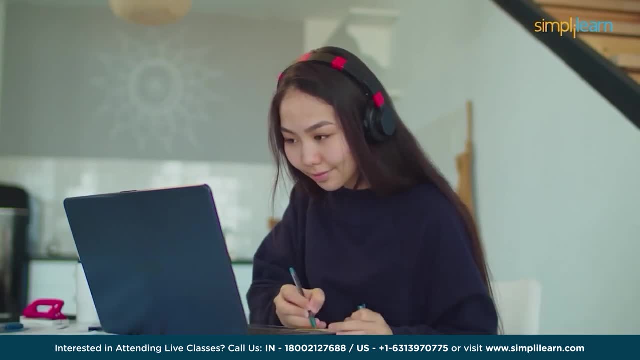 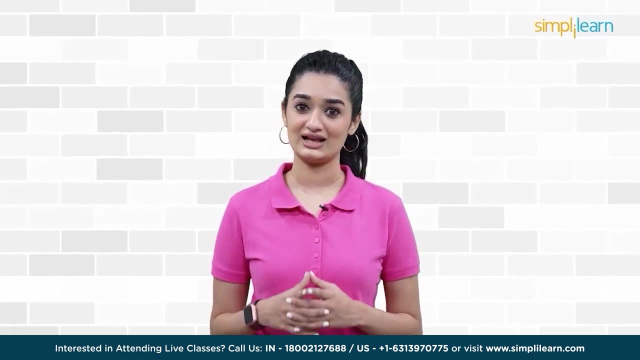 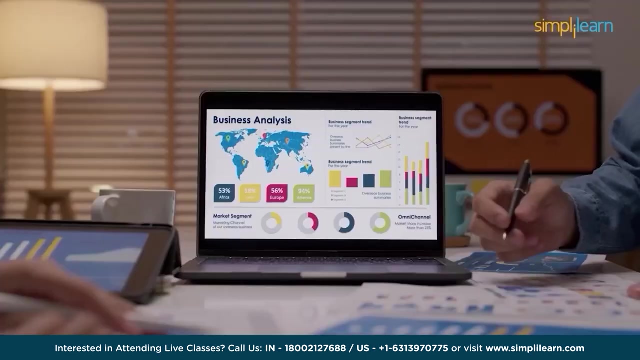 but this certification is absolutely for free. Another similar certification is based on data analytics. for interested candidates, Pursuing this certification will help you with data science fundamentals and also enhance your data visualization skills. The course covered data prep with Tableau. visual analytics, data science with Tableau. 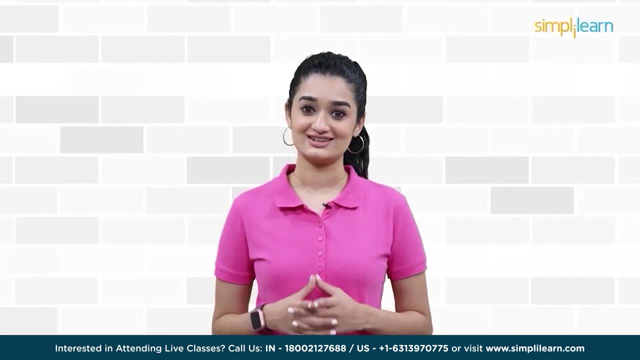 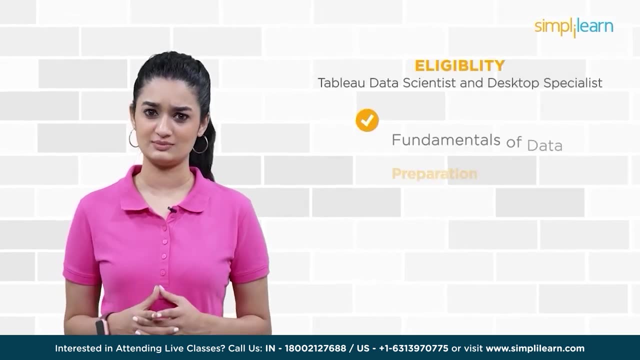 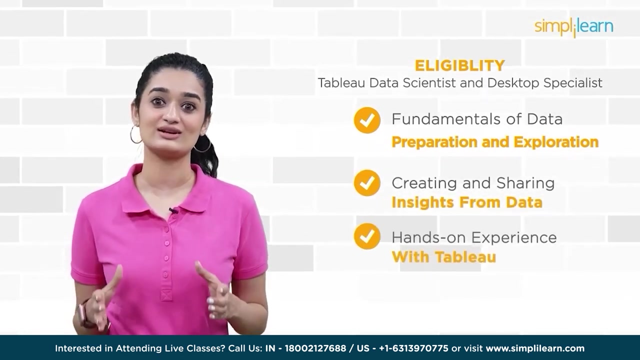 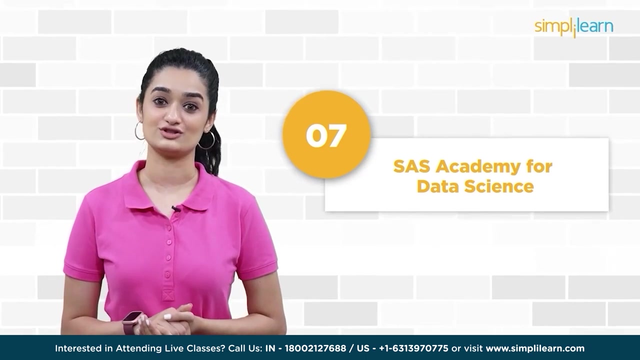 and finally, to put your learning to the test, The course also includes a data scientist skills assessment. The course requires the candidates to possess some fundamentals of data preparation and exploration, creating and sharing insights from data and some hands-on experience with Tableau. Up ahead, we have SAS Academy for Data Science Certification. in seventh position, 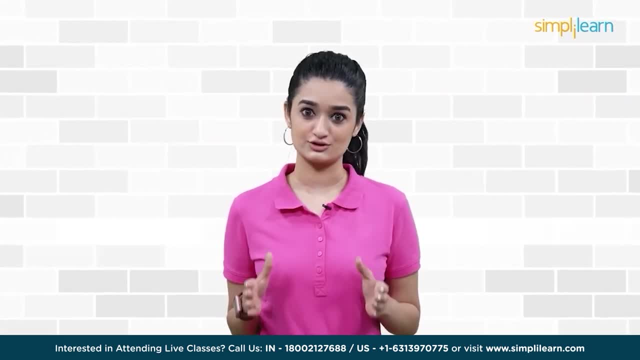 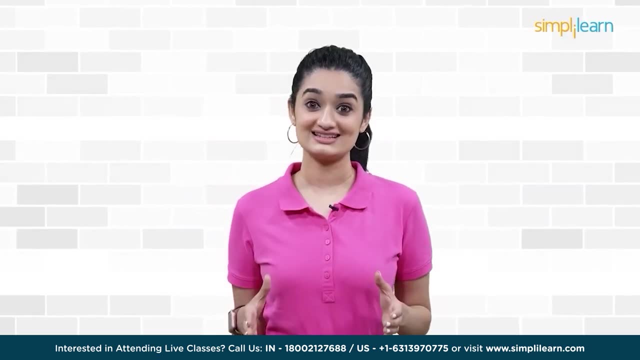 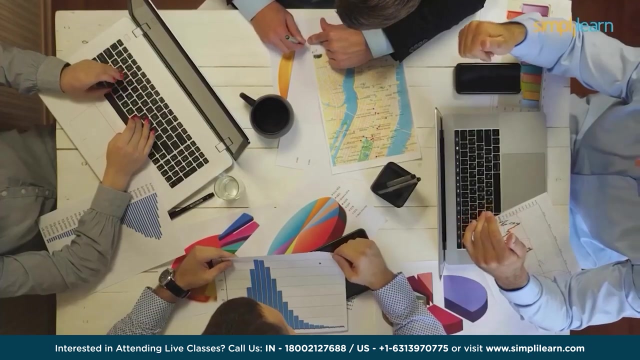 Statistical analytical system is a sophisticated tool purpose-built for carrying out advanced analytics and complex statistical operations. Getting certified as an SAS expert will help your resume to stand out. The course features hands-on experience with powerful tools like Learn using SAS R, Python, PIG, Hive and Hadoop. 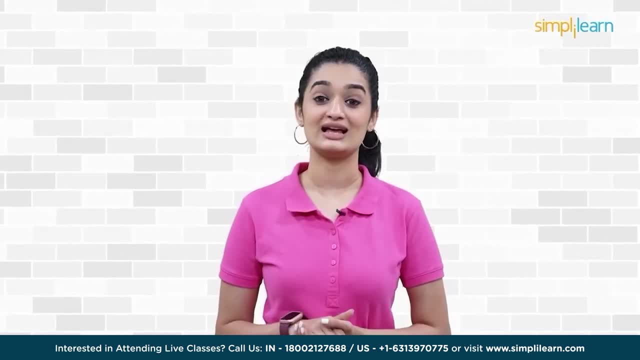 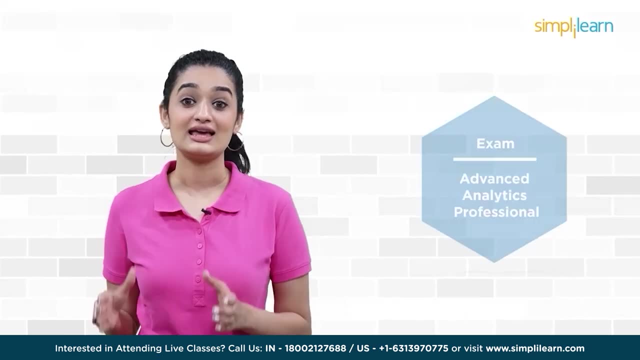 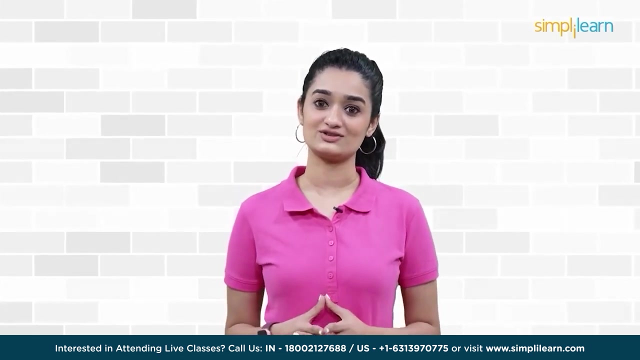 The global recognized tailor-made certification will help you prepare for all three exams, namely data curation- professional- advanced analytics- professional AI and machine learning professional as well. The course will enhance your learning with practical application based on actual SEAS studies that will feature data curation- advanced analytics. 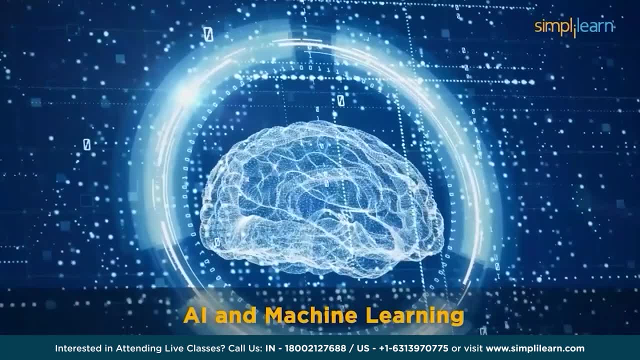 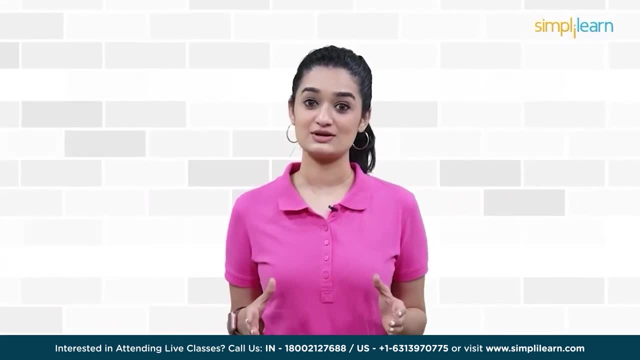 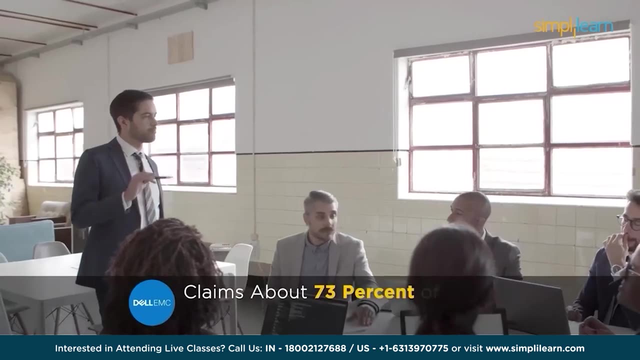 AI and machine learning your way at your own pace. We have Dell EMC proven professional certification program in the top 6th grade. The Dell EMC proven professional certification program is a tried and tested certification with affirmed results. Dell claims about 73% of individuals found the program to be effective in their career. 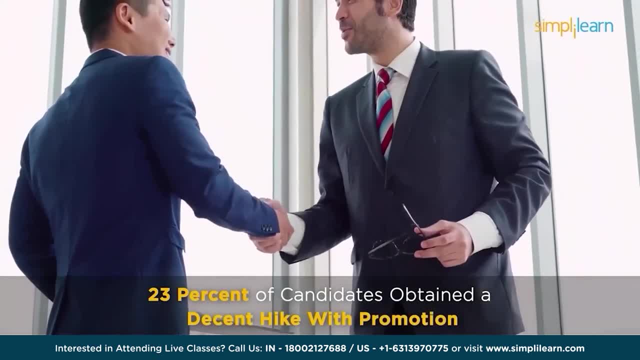 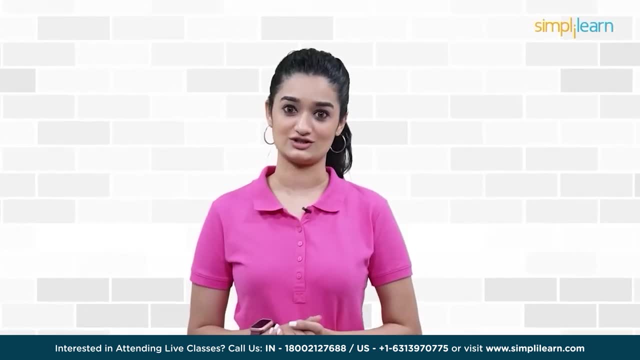 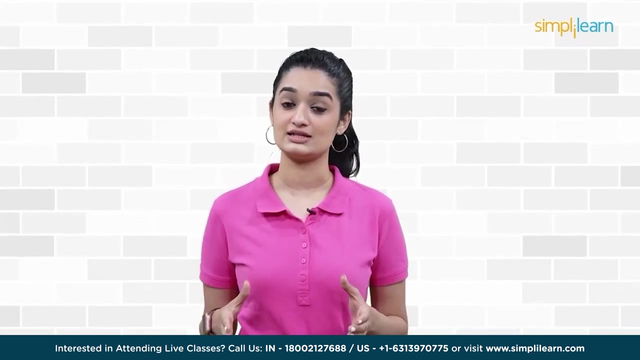 23% of candidates obtained a decent hike with promotion as well. About 86% of HRs admitted to selecting the candidates with this certification. With these groundbreaking numbers, this certification has nothing more to prove. The program is segmented into two categories: the associate level certification. 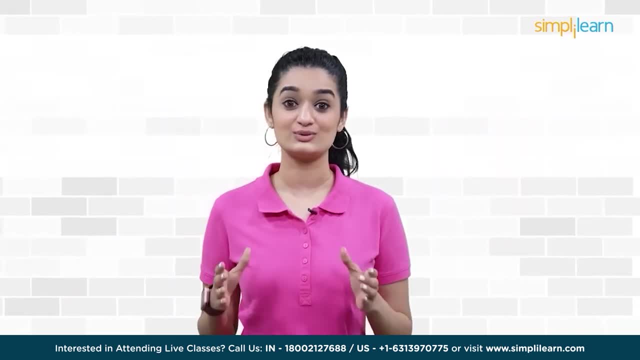 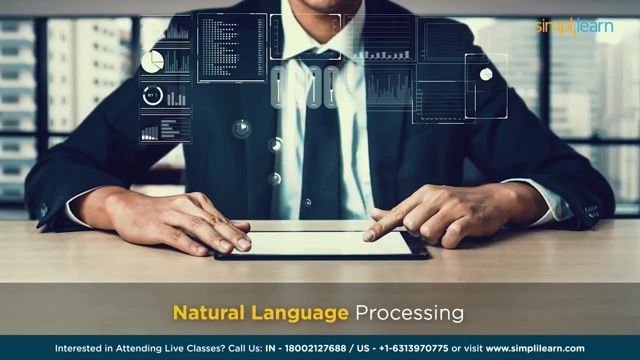 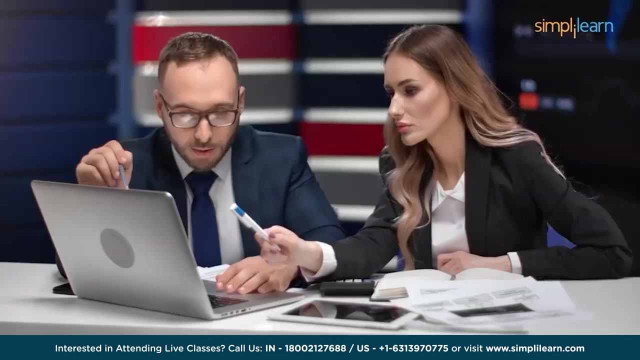 and specialist level certification. The main growth areas include advanced analytical methods- Hadoop and PIG, Hive, social network analysis, natural language processing and visualization methods. The development of these skills and the use of these methods allow the data scientists to identify and communicate conclusions and recommendations to solve business challenges. 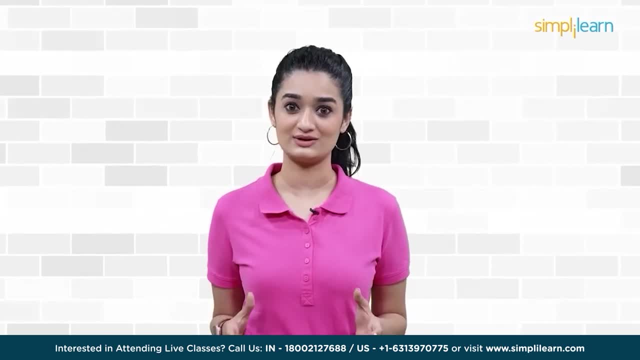 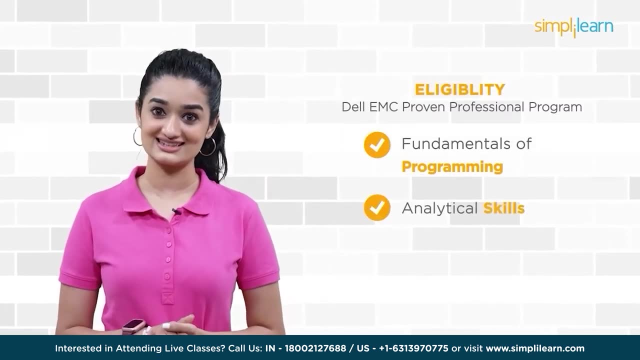 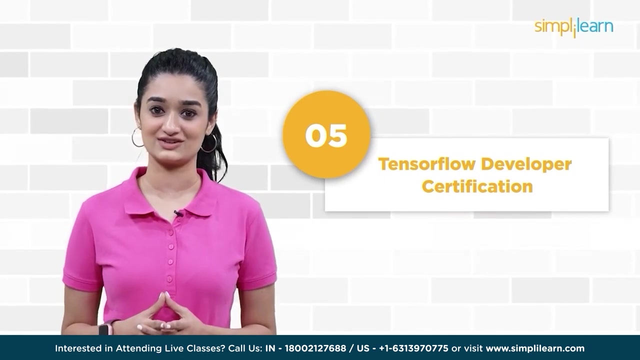 across many domains. If you are interested in wondering about the prerequisites needed, that's good news for you. The program expects only fundamental programming and analytical skills and have a good understanding of cloud computing. On the top 5th position, we have TensorFlow Developer Certification. 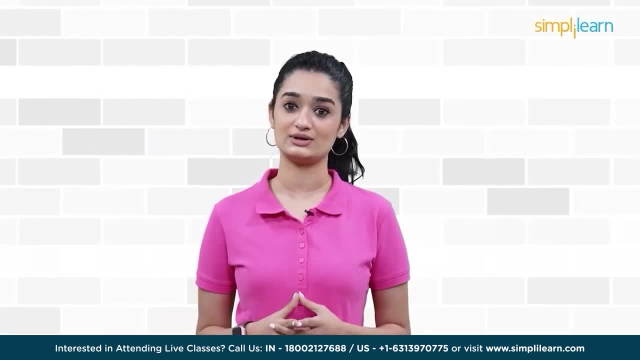 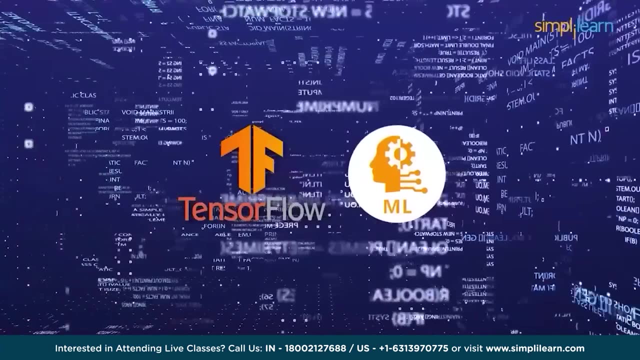 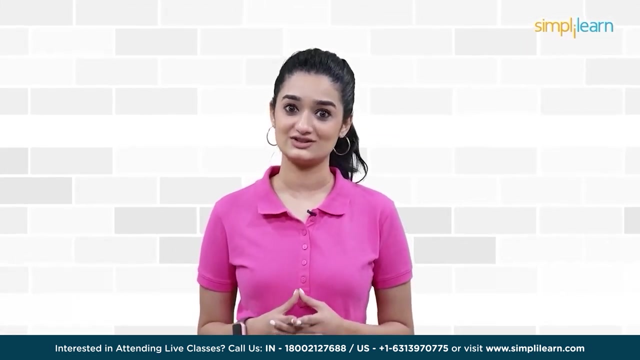 The main goal of this certification is to help aspiring data scientists get well versed with TensorFlow and showcase their expertise in machine learning. The TensorFlow Developer Certification can be considered as one of the best foundational certifications for demonstrating training and deployment of the machine learning model. 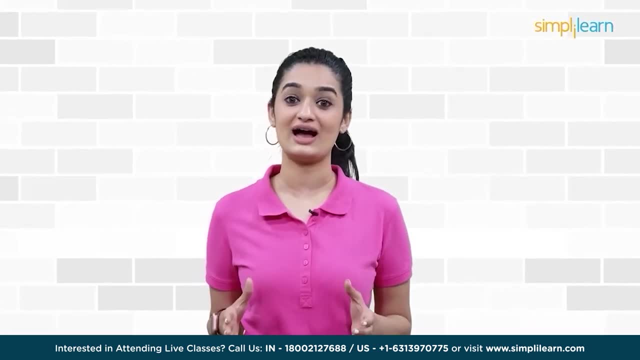 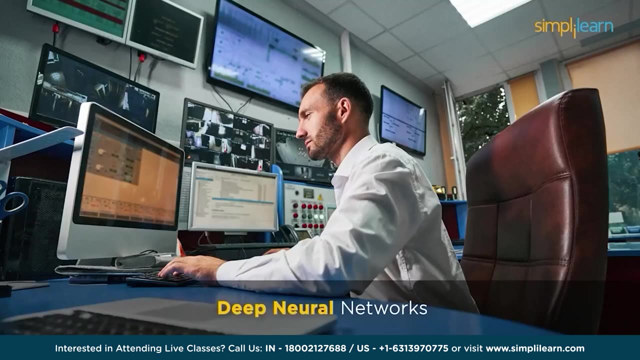 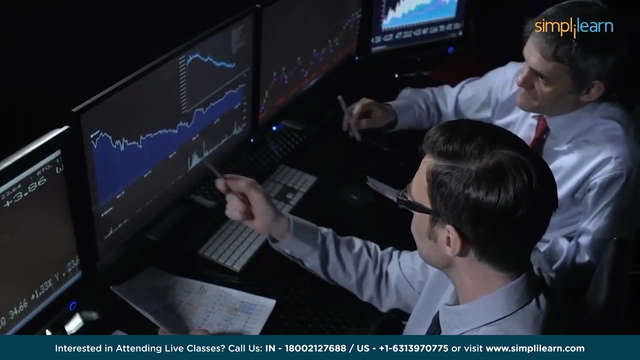 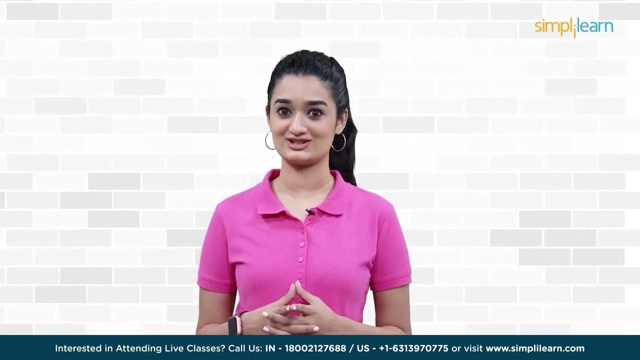 The candidates appearing for this certification are expected to have a final fundamental knowledge of image recognition, object detection, test recognition algorithms with deep neural networks, convolutional neural networks and exploring strategies to prevent overfitting, including augmentation and dropout. The best part of the certification is it does not have an expiration date. 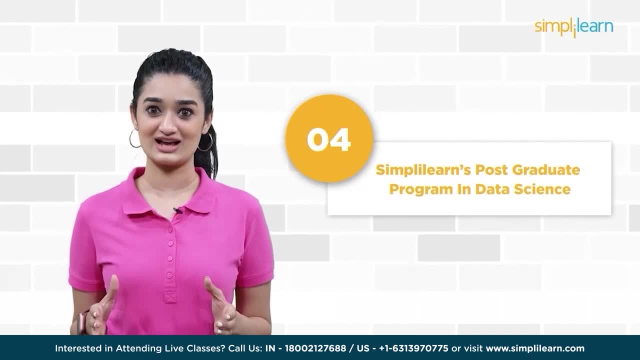 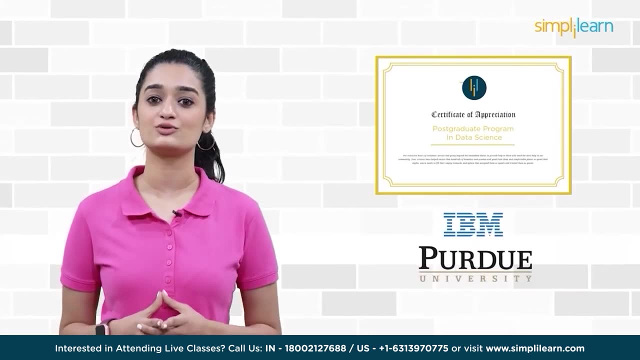 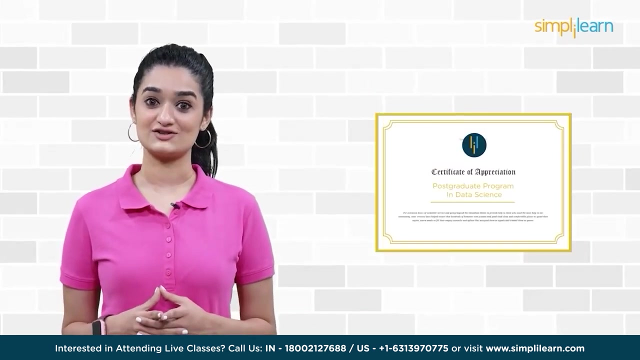 One amongst the top 5 is Simply Learn's postgraduate program in data science. Simply Learn collaborates with IBM and Windows IBM and with the best and world renowned Purdue University for providing postgraduate certification in data science. Simply Learn's data science certification is ranked as the number one by Economic Times. 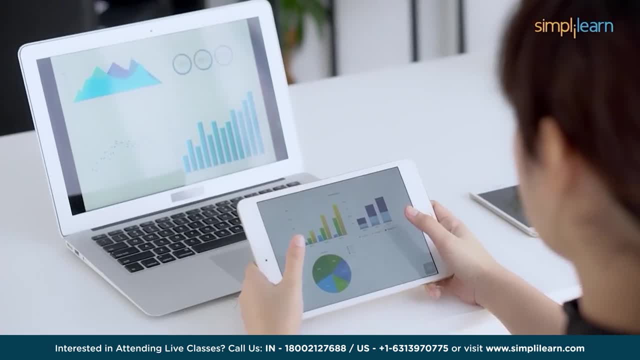 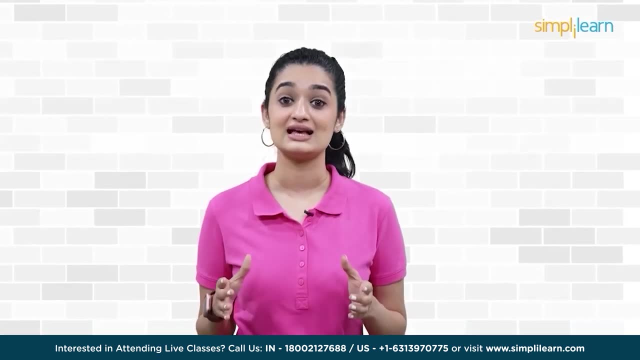 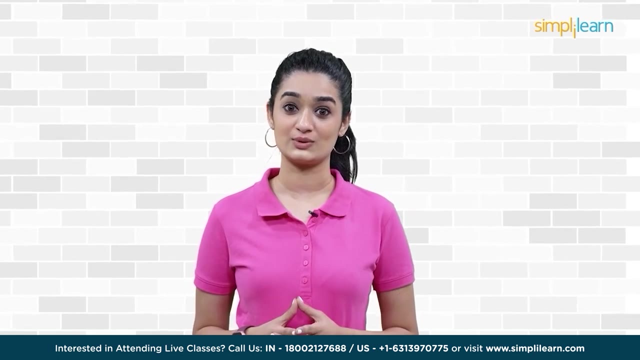 The course focuses on the comprehensiveness of content and skills required to tackle real world business problems. The best part of the certification program is that it does not concentrate on one language like the others. Here you get into the master data science with both Python and R programming languages. 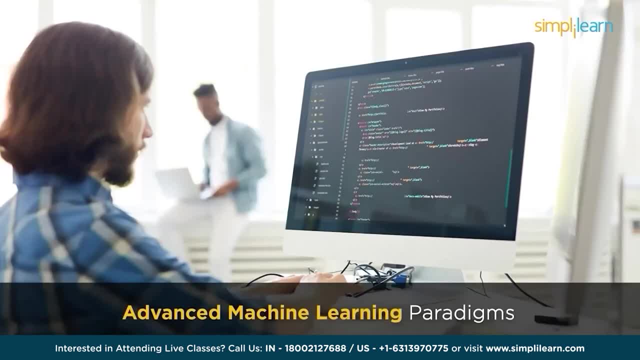 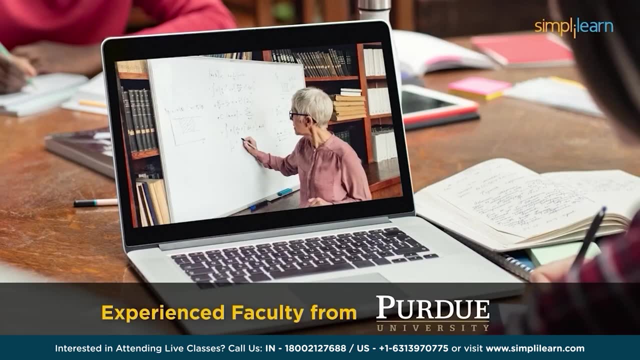 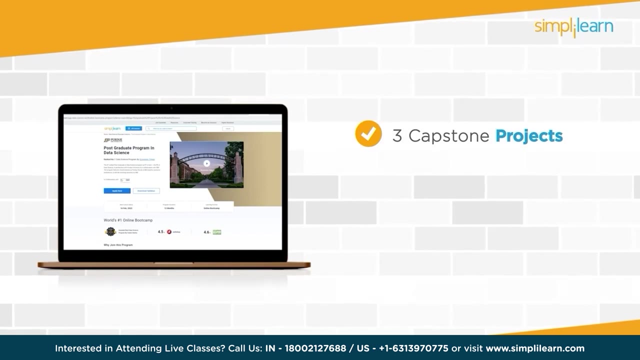 The course then navigates you through advanced machine learning paradigms with real time industry professionals and experienced faculty from Purdue University. By the end of the program you will get hands on experience with three capstone projects And also you will have lifetime access to 25 plus real time business problems and their 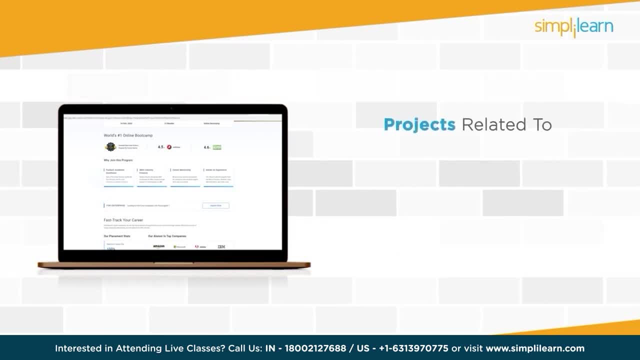 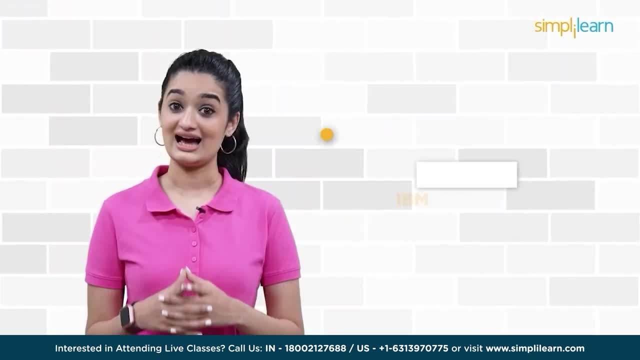 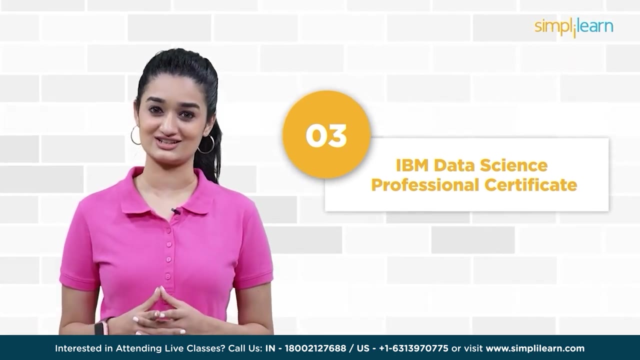 solutions for future reference. The projects are related to top organizations like Amazon, Uber, Walmart, Comcast, to name a few. The IBM Data Science Professional Certificate stands at the third position of top data science certifications. You will learn to import and clean data sets, analyze and visualize data, and build and. 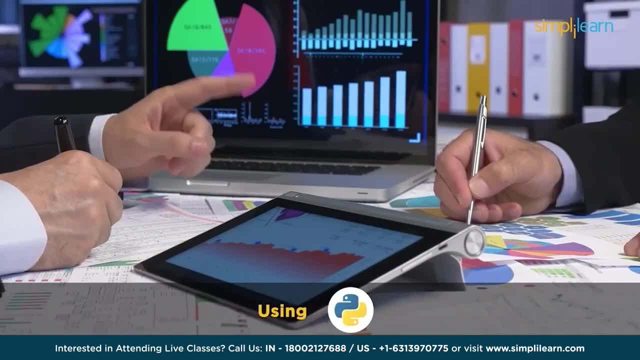 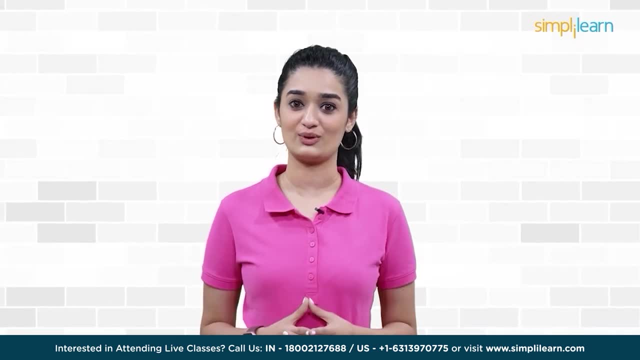 evaluate machine learning models and pipelines using Python. You will apply various data science skills, techniques and tools to complete a project and publish a real time report by the end of the course. The course revolves around Python, so it happens to be one of the major prerequisites and along 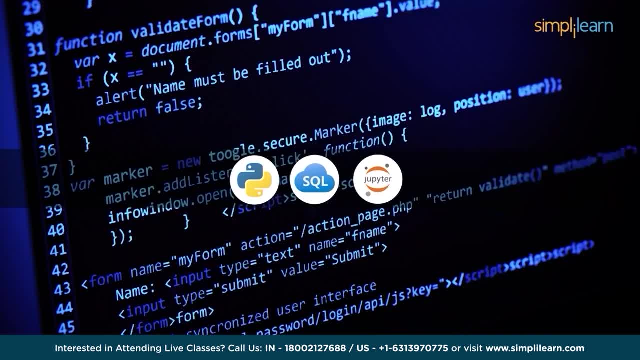 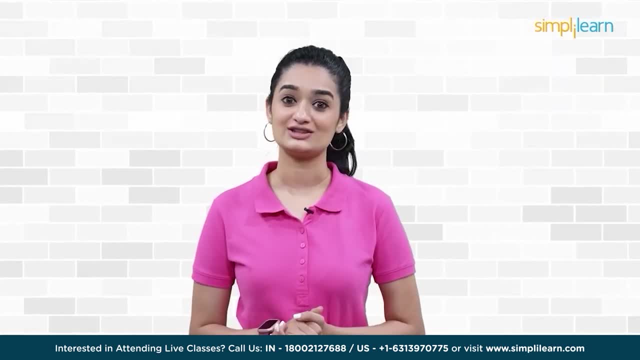 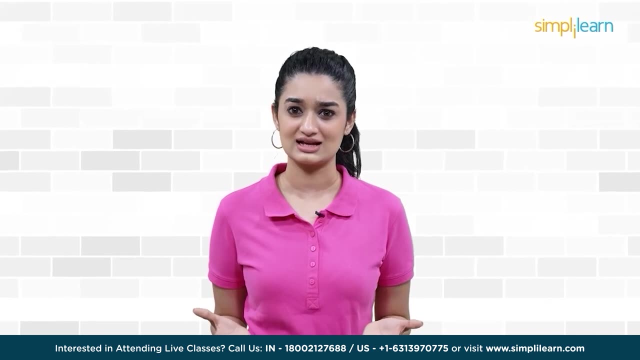 with that comes SQL and Jupyter notebook. IBM claims that the course gives people the foundational blocks to learn and master data sources. We are now at the top. second certification: the Google Certified Professional Data Engineer. You might be wondering why are we discussing data engineering? 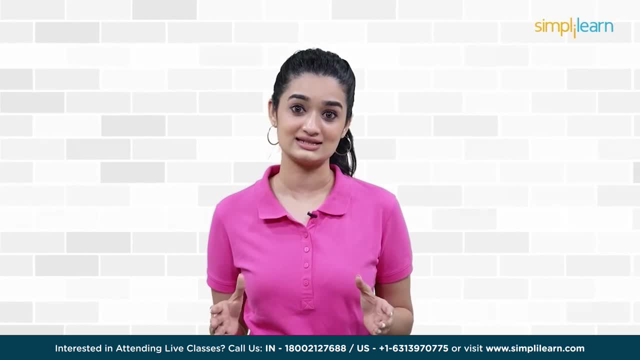 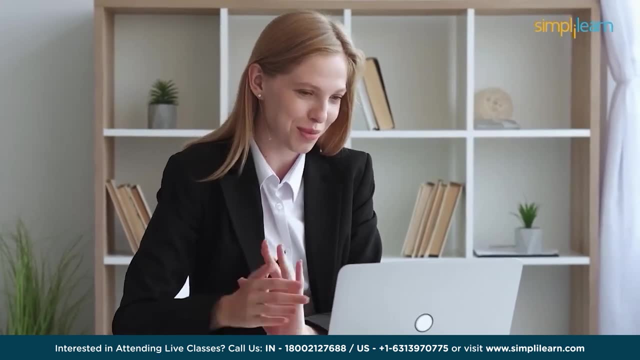 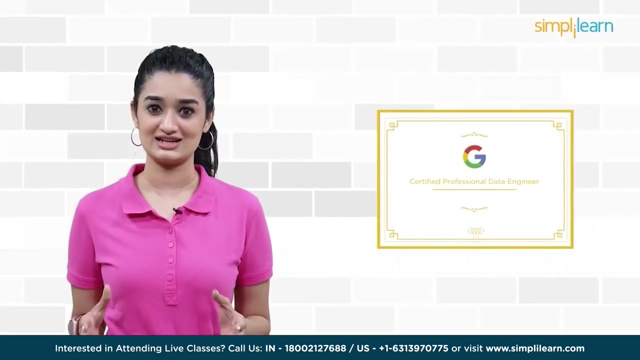 It is a fact that to become a successful data scientist, you need to possess a good grip over the data that you are working with. Data Engineer certification will give you an edge over the other candidates, proving your caliber while handling data. This certification will take you through various stages, where you will learn to design and 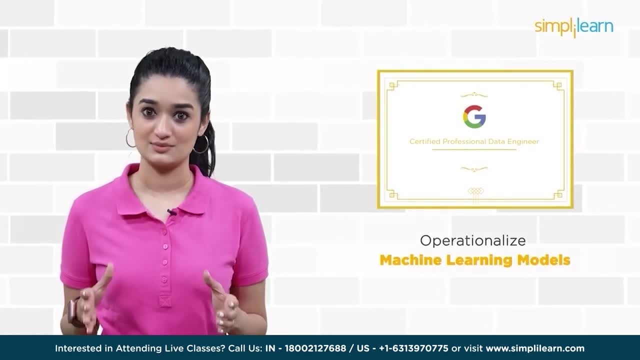 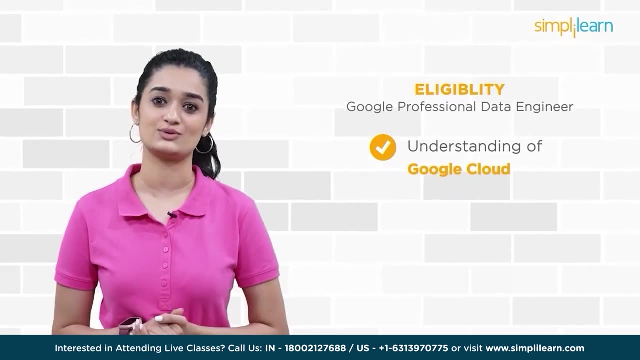 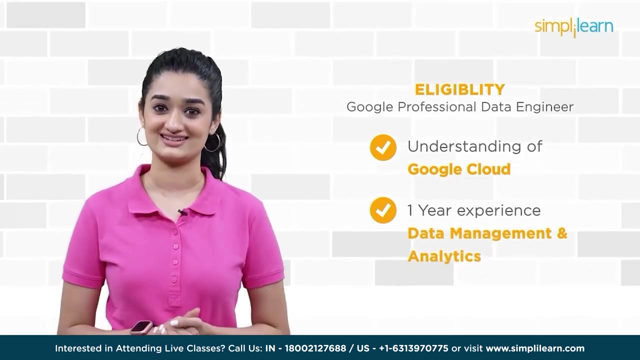 build data processing systems, operationalize machine learning models and deliver the best solution. Having a comfortable understanding of Google Cloud would be necessary. A good one year of experience with data management and analytics could add to taking up the certification On the number one position we have: Google Data Machine Learning Engineer. 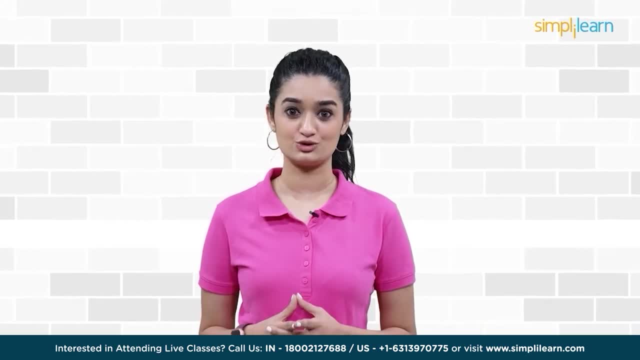 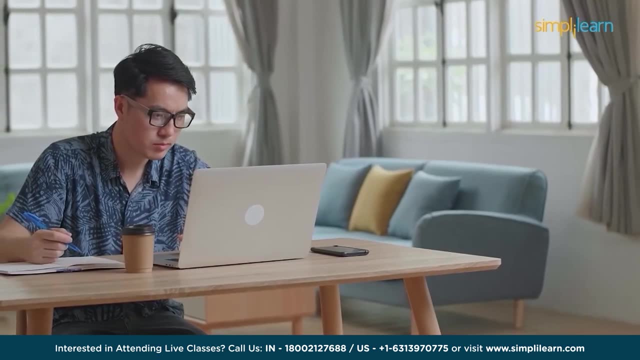 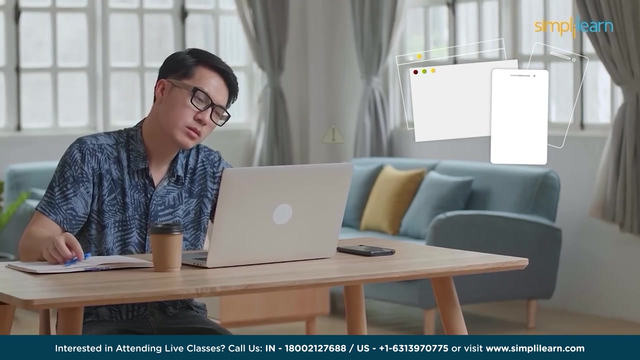 Most of the time, data scientists are comfortable working with Jupyter notebook. This could be feasible in normal conditions, But if you wish to spend your model production on the website or mobile devices, things can escalate real quick. Unexpected issues might pop up from nowhere and hinder the production environment. 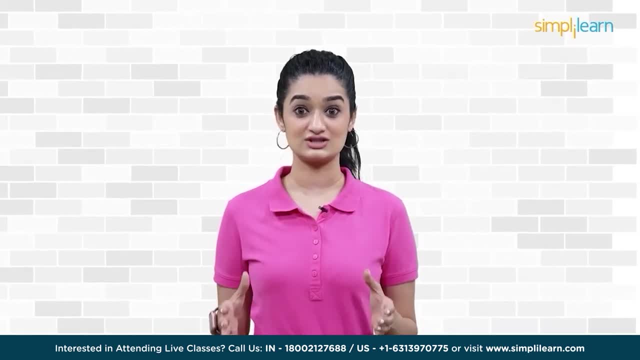 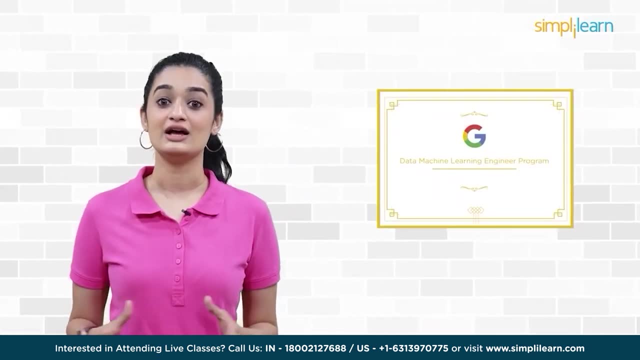 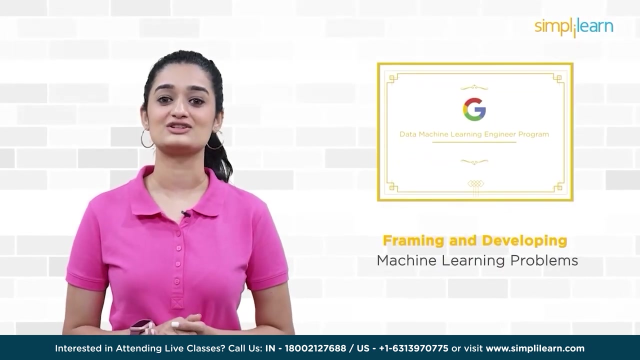 Although it is obvious and many educational programs teach this concept, it is preferred to learn it from the experts. In Google's Data Machine Learning Engineer program. you will get hands-on experience in various domains, A few important ones like framing and developing, machine learning problems, automation and 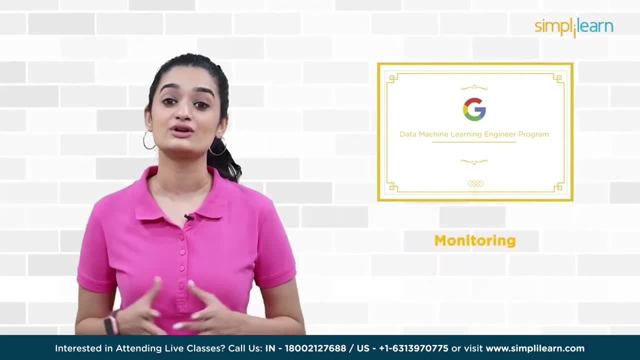 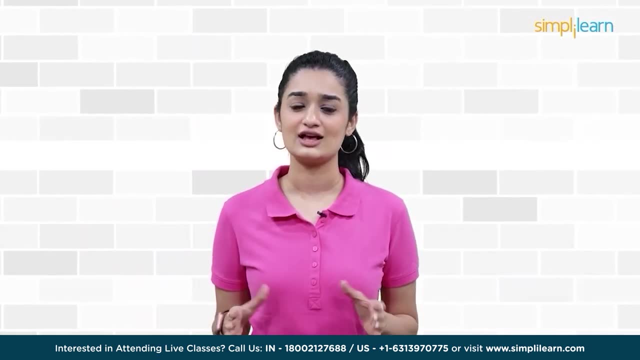 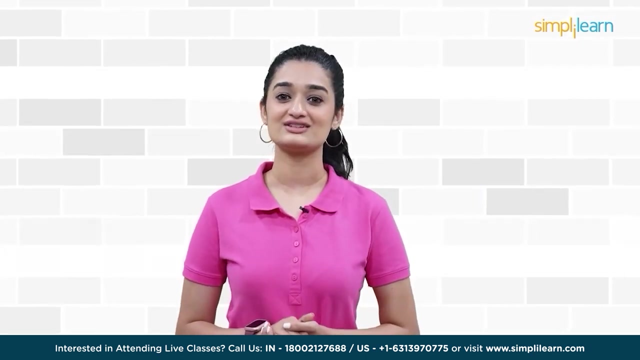 orchestrating machine learning pipelines might help Monitoring, optimizing and maintaining machine learning solutions. The best part of this certification program is you do not need to have any concrete prerequisite to take up this certification program. With that, we have come to the end of this session on the top 10 data scientist certifications. 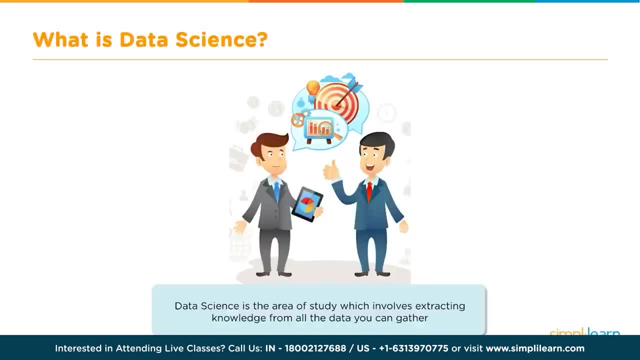 for 2022.. So what is data science? As the name suggests, it is nothing but study of using data and trying to find out the insights, or extracting some insights or knowledge using all the data that is at your disposal. So that's pretty much what data science is all about. 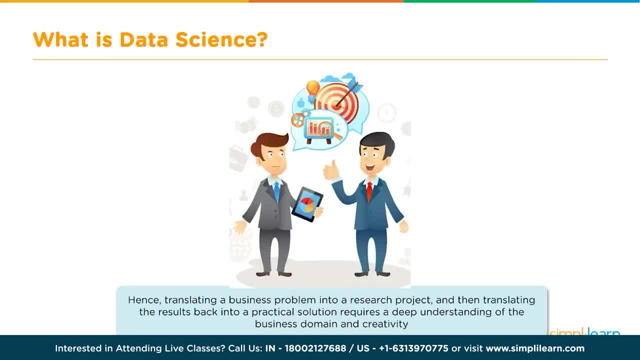 So you take the data and apply certain methodologies, certain algorithms and your business domain knowledge as well, And, of course, a certain amount of creativity, to extract some insights. Very often they are also known as actionable insights, Because once you have the insights, you should be in a position to take some action to let's 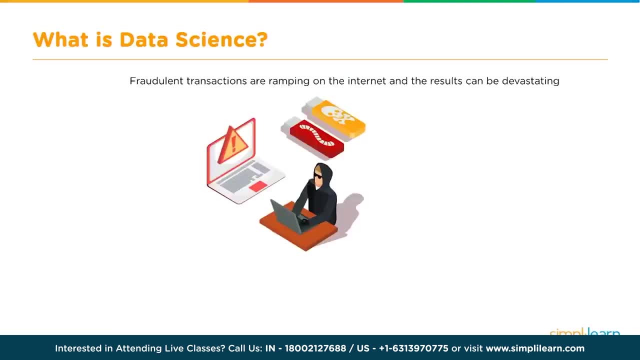 say, solve a problem or improve a situation. There are a lot of areas where data science can be used. One of the very common one is fraud detection or fraud prevention. There are a lot of fraudulent activities or transactions, primarily on the Internet. 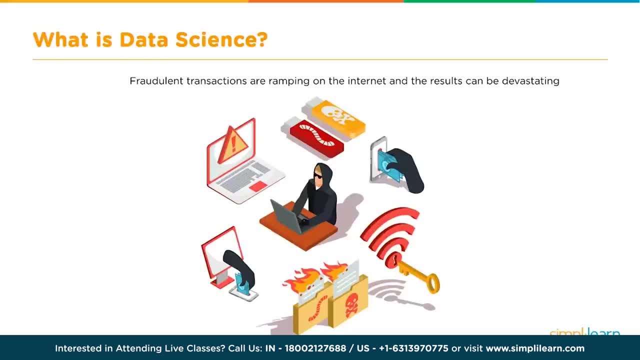 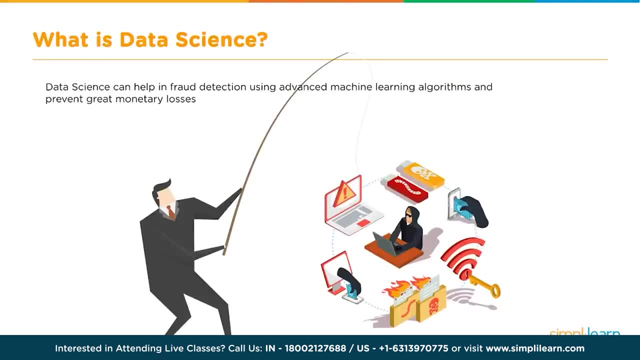 It's very easy to commit fraud And therefore we can use data science to either prevent or detect fraud. There are certain algorithms- machine learning algorithms- that can be used, like, for example, some outlier techniques, clustering techniques- that can be used to detect fraud and prevent. 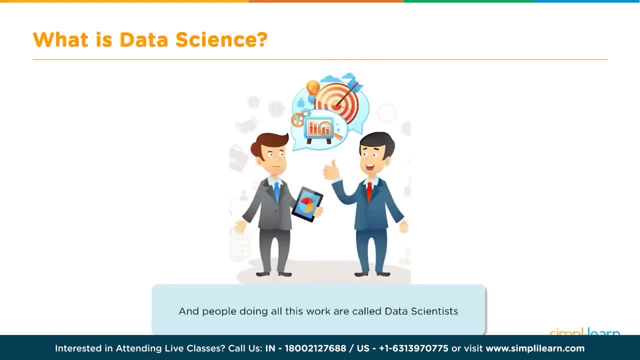 fraud as well. So who is a data scientist? It is actually a very generic role that defines. somebody who is working with data is known as a data scientist, But there can be very specific activities and the roles can be actually much more specific: What exactly a person does within the area of data science? 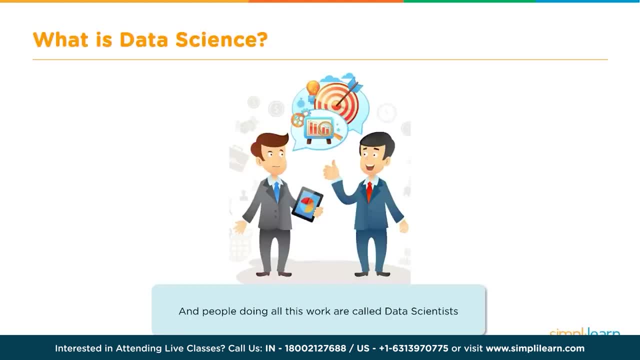 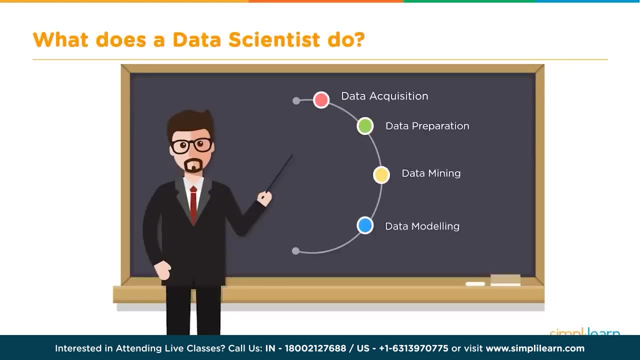 Data science can be much more specific, But broadly, anybody working in the area of data science is known as a data scientist. So what does a data scientist do? These are some of the activities: data acquisition, data preparation, data mining, data modeling. 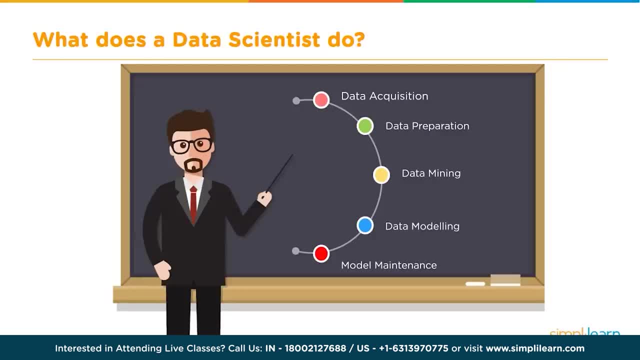 and then model maintenance. We will talk about each of these in great detail, But at a very high level. the first step, obviously, is to get the raw data, which is known as data acquisition. It can be all kinds of format, It can be multiple sources. 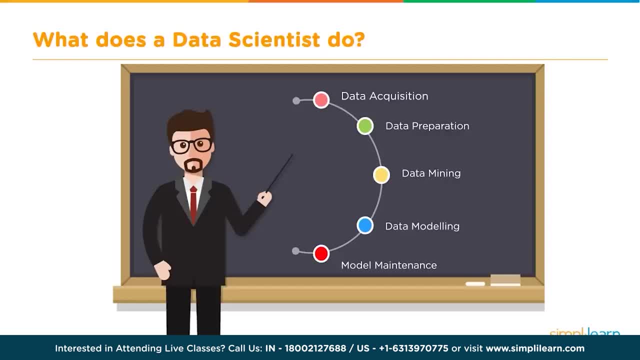 But obviously that raw data cannot be used as it is for performing data mining activities or data modeling activities. So the data has to be planned and prepared for using in the data models or in the data mining activity. So that is the data preparation. Then we actually do the data mining, which can also include some exploratory activities. 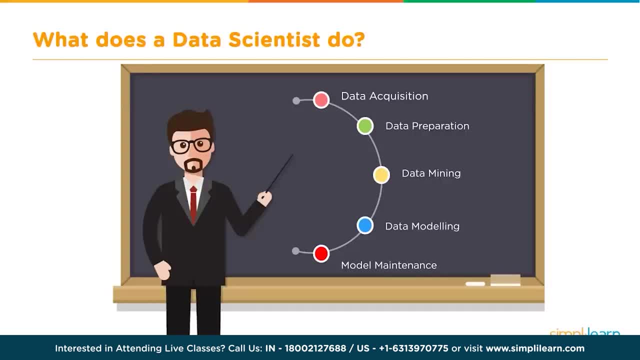 And then if we have to do stuff like machine learning, then you need to build a machine learning model and test the model, Get insights, Get science out of it, And then, if the model is fine, you deploy it. And then you need to maintain the model because over a period of time it is possible that 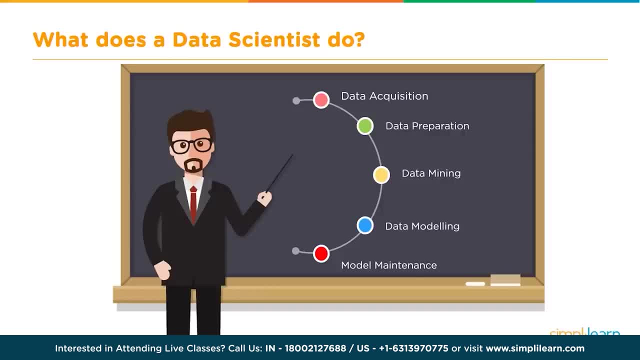 you need to tweak the model because of change in the process or change in the data and so on, So that all comes under the model maintenance. So let's take a deeper look at each of these activities. Let's start with data acquisition, So the stage of data acquisition. basically, the data scientist will collect raw data from. 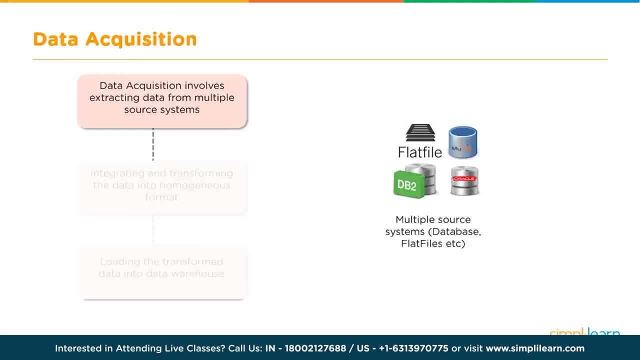 all possible sources. So this could be typically an RDBMS, which is a relational database, or it can also be a non-RDBMS, or it could be flat files or unstructured data and so on. So we need to bring all that data from different sources if required. 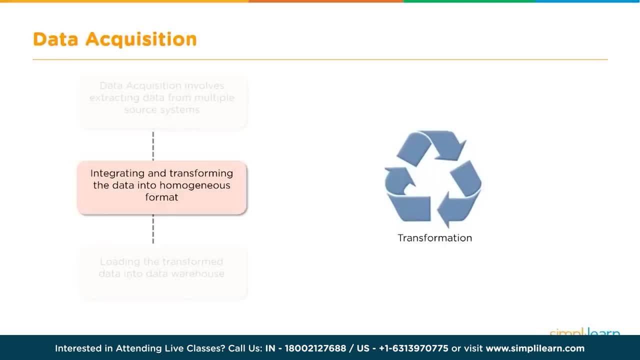 We need to do some kind of homogeneous formatting so that it all fits into, looks at least format. from a format perspective it looks homogeneous, So that may be requiring some kind of transformation. Often this is loaded into what is known as data warehouse. 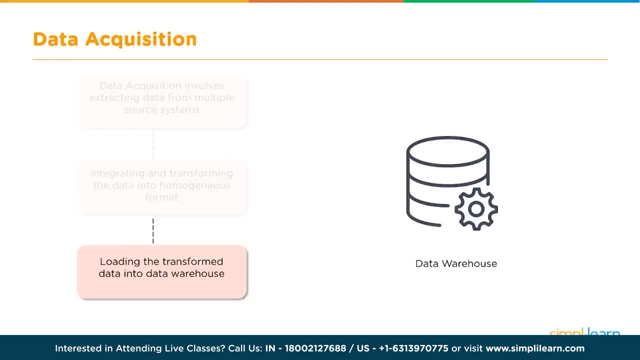 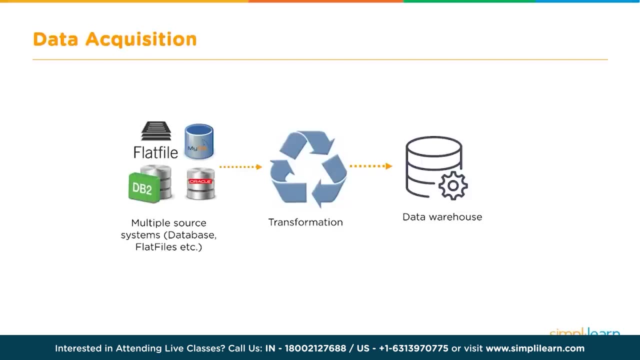 So this can also be sometimes referred to as ETL, or extract, transform and load. So a data warehouse is like a common place where data from different sources is brought together so that people can perform data science activities like reporting or data mining or statistical analysis and so on. 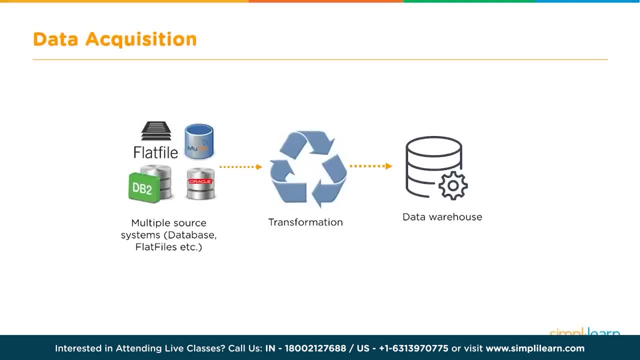 So data from various sources is put in a centralized place, which is known as a data warehouse. So that is also known as ETL, And in order to do this, there can be data scientists can take help of some ETL tools. There are some existing tools that a data scientist can take help of, like, for example: 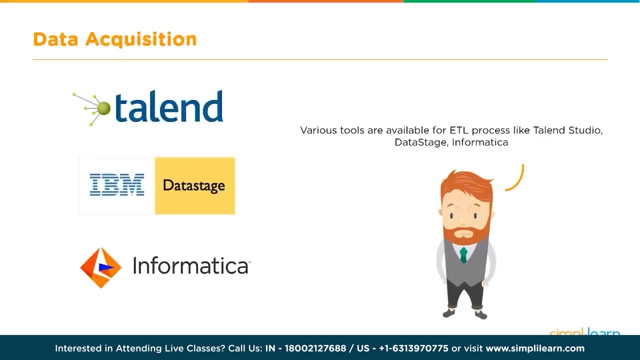 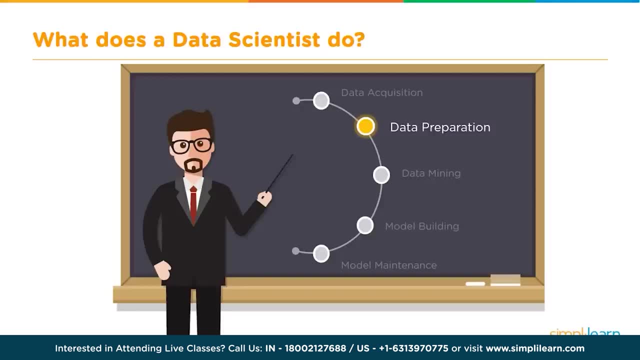 Data Stage or Talent or Informatica. These are pretty good tools for performing these ETL activities and getting the data. The next stage, now that you have the raw data into a data warehouse, you still probably are not in a position to straight away use this data. 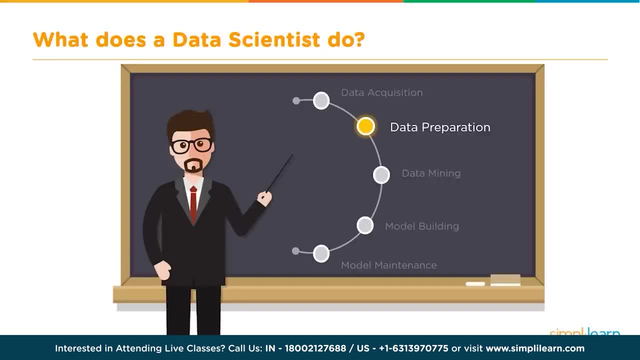 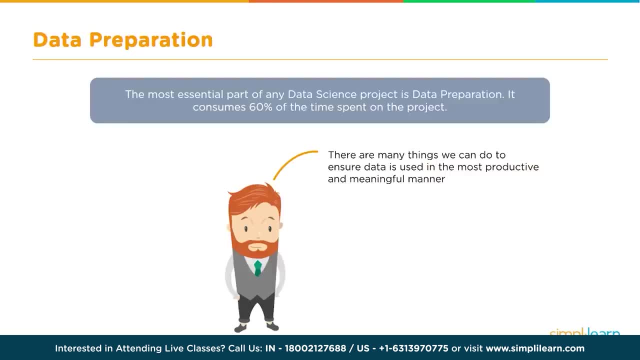 And there are multiple reasons for that. One of them could be the data is dirty, There are some missing values and so on and so forth. So a lot of time is actually spent in this particular stage. So a data scientist spends a lot of time- almost 60 to 70% of the time- in this part. 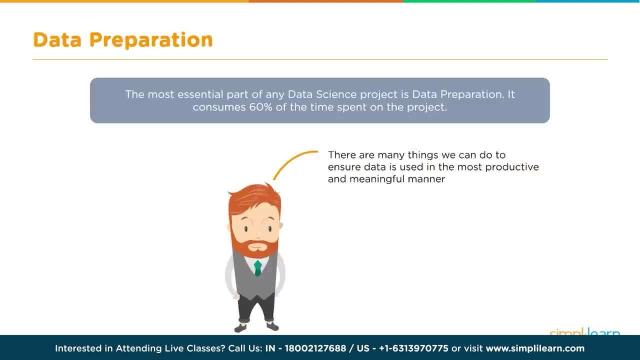 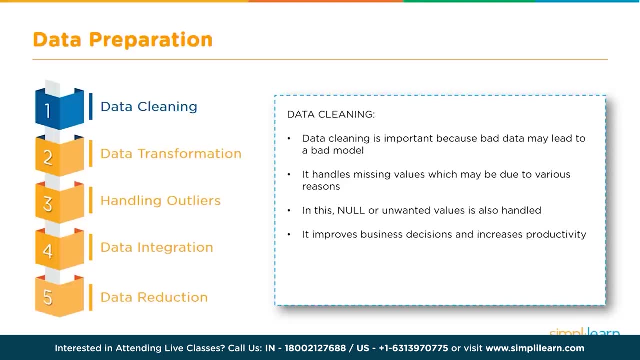 of the project or the process which is data preparation. So there are again within this, there can be, multiple tools that can be used to take care of the data. There can be multiple sub activities, starting from, let's say, data cleaning. you will probably 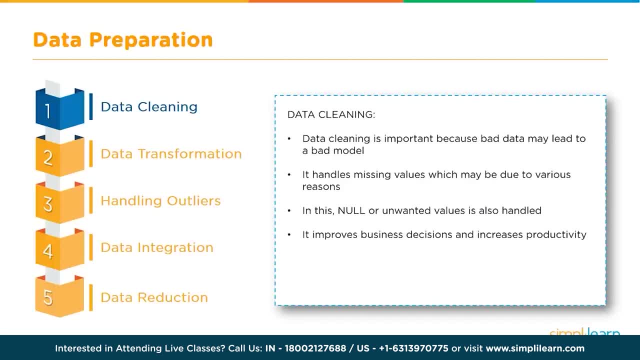 have missing values, the data, there is some columns, the values are missing or the values are incorrect, There are null values, and so on and so forth. So that is basically the data cleaning part of it. Then you need to perform certain transformations like, for example, normalizing the data and 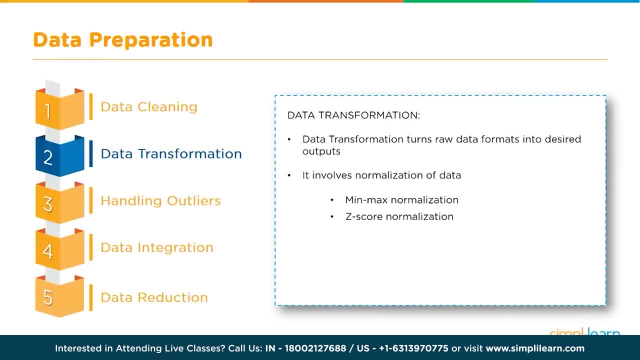 so on, right, So you could probably have to modify a categorical values into numerical values And so on and so forth. So these are transformational activities. then we may have to handle outliers, So the data could be such that there are a few values which are way beyond the normal. 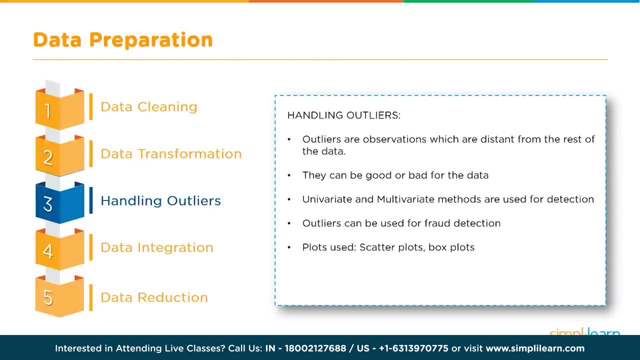 behavior of the data. for whatever reason, either people have keyed in wrong values or for some reason some of the values are completely out of range, So those are known as outliers. So there are certain ways of handling these outliers and detecting and handling these. 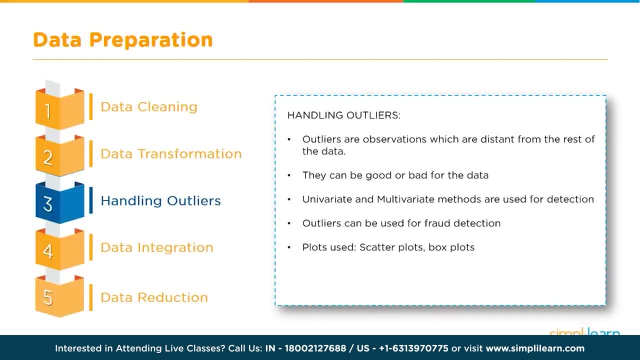 outliers, And this is a part of what is known as exploratory analysis. So you quickly explore the data to find out, are there so? and you can use visual tools like plots and identify what are the outliers and see how we can get rid of the outliers. 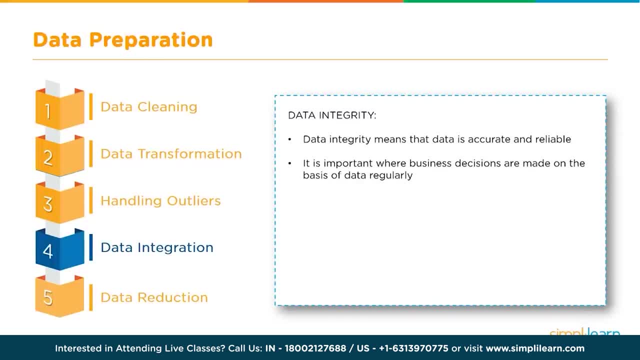 and so on. Then the next part could be data integrity. Data integrity is to validate, for example, if there are some primary keys, that all the primary keys are populated. there are some foreign keys, then at least most of the foreign keys should be populated. 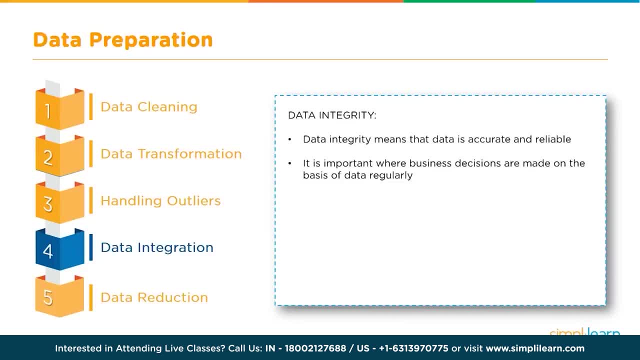 And otherwise, when we are trying to query the data, you may get wrong values and so on. So that is the data integrity part of it, And then we have what is known as data reduction. Sometimes we may have duplicate values, we may have columns that may be duplicated because 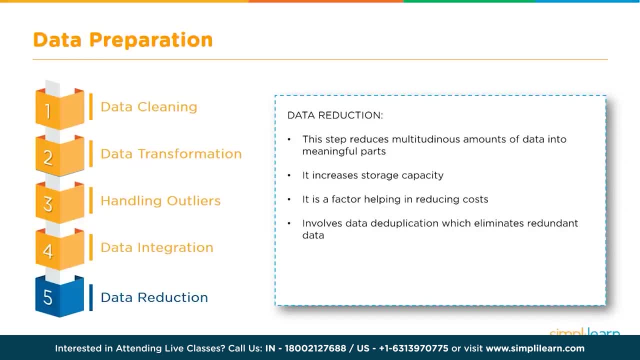 they are coming from different sources, the same values are there, and so on. So a lot of this can be done using what is known as data reduction, And thereby you can reduce the size of the data drastically, because very often it's could be written and data which can be removed, and so on. 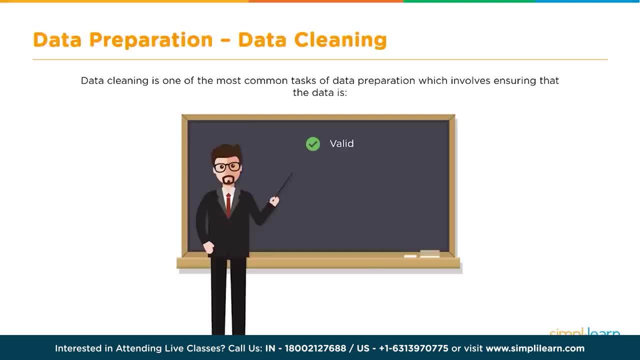 So let's take a look at what are the various techniques that are used for data cleaning. So we need to ensure that the data is valid and it is consistent and uniform and accurate. So these are the various parameters that we need to ensure as a part of the data cleaning. 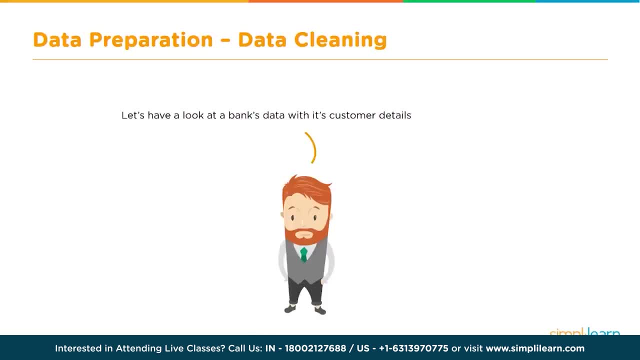 process. Now, what are the techniques that that are used for data cleaning are? so we will see what each of these are in this particular case. Okay, And so what is the data set that we have? we have data about a bank and its customer. 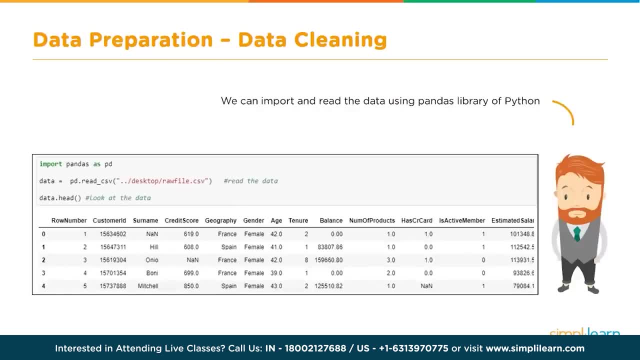 details. So let's take an example and see how we go about cleaning the data. And in this particular example we are assuming we are using Python. So let's assume we loaded this data, which is the raw file, dot CSV. This is how the customer data looks like. 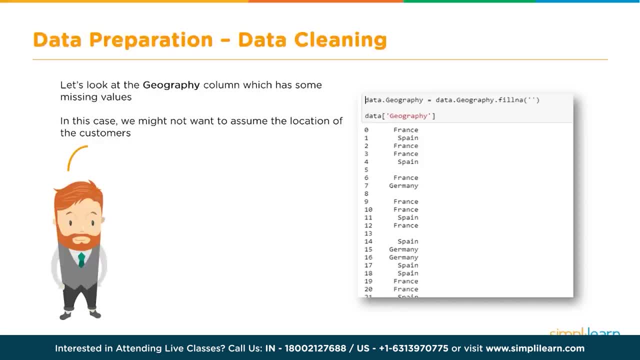 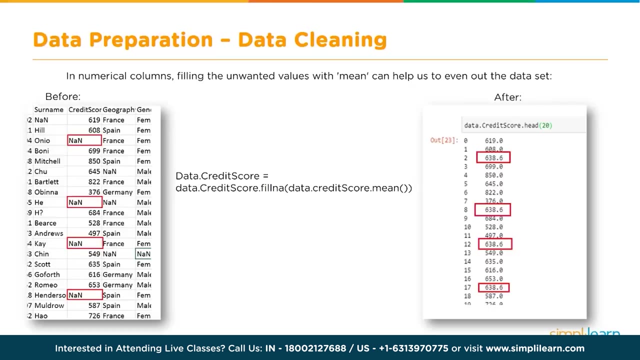 And we will see. for example, we take a closer look at the geography column, we will see. we see that there are quite a few blank spaces. So how do we go about when we have some blank spaces? or if it is a string value, then we 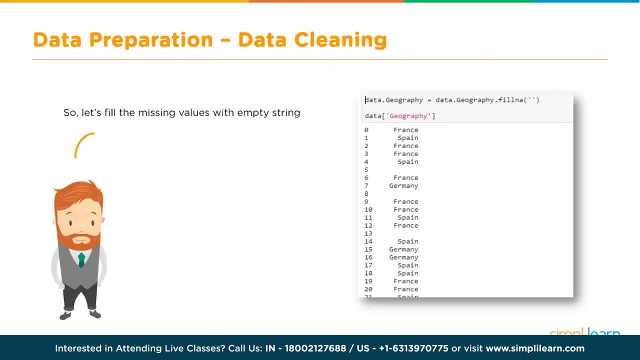 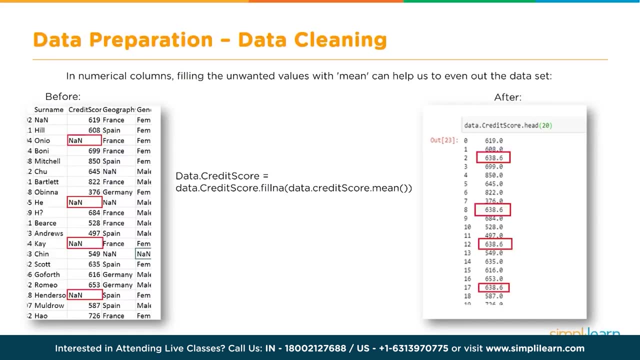 put an empty string here, or we just use a space or empty string. if they are numerical values, then we need to come up with a strategy. For example, we put the mean value, so wherever it is missing, we find the mean for that particular. 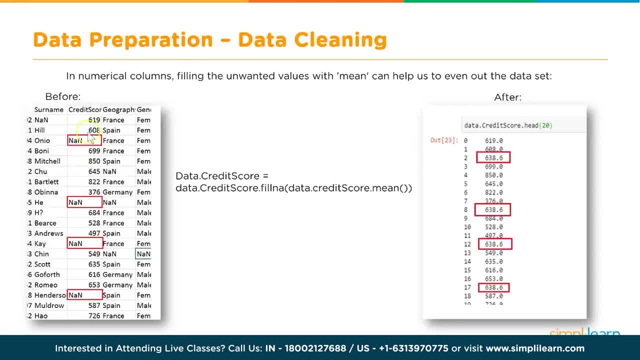 column And in this case, let's assume we have credit score and we see that quite a few of these values are missing. So what do we do here? we find the mean for this column, for all the existing values, and we found that the mean is equal to 638.6. 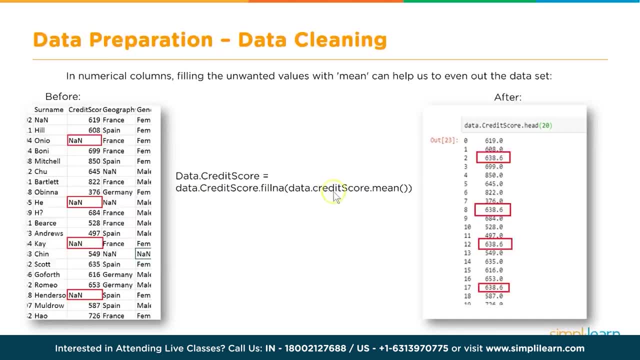 So we kind of write a piece of code to replace wherever there are blank values in and is basically like now, and we just go ahead and say fill it with the mean value. So this is a piece of code we are writing to fill it. 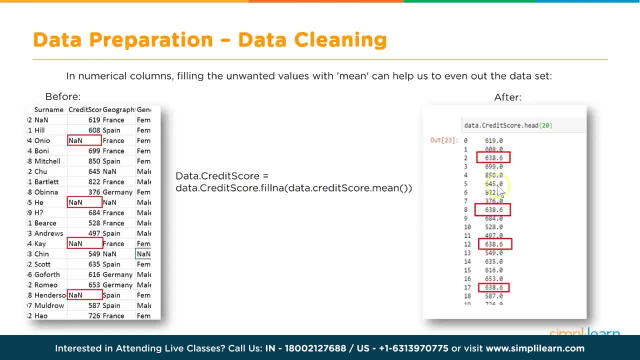 So all the blank spaces- All the blanks are all the null values- get replaced with the mean value. Now, one of the reasons for doing this is that, very often, if you have some such situation, many of your statistical functions may not even work. So that's the reason you need to fill up these values or either get rid of these records. 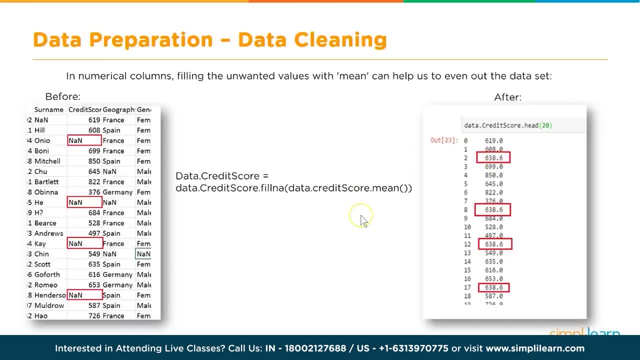 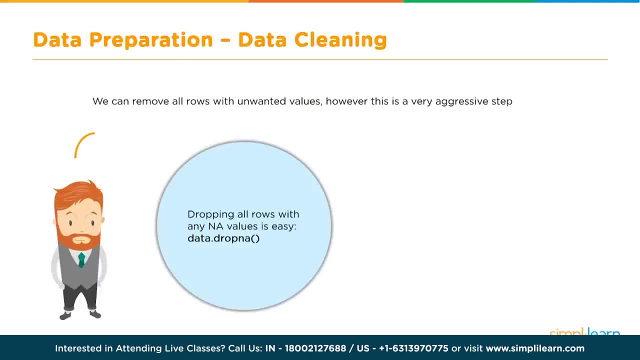 or fill up these values with something meaningful. So this is one mechanism which is basically using a mean. there are a few others. as we move forward we can see what are the other ways. for example, we can also say that any missing value in a particular row, if even one column, the value is missing. you just 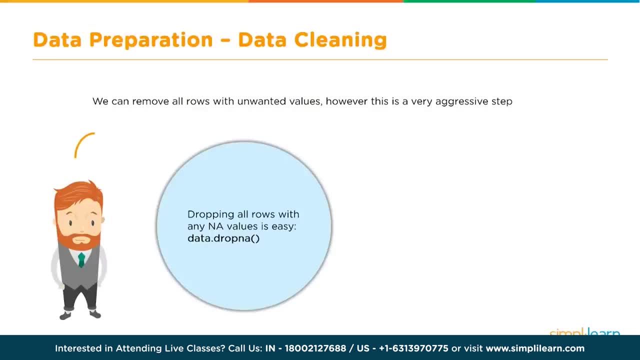 drop that particular row or delete all rows where even a single column has missing values. So that is one way of dealing. now the problem here can be that if a lot of data has, let's say, one or two columns missing and we drop many such rows, then overall you may lose. 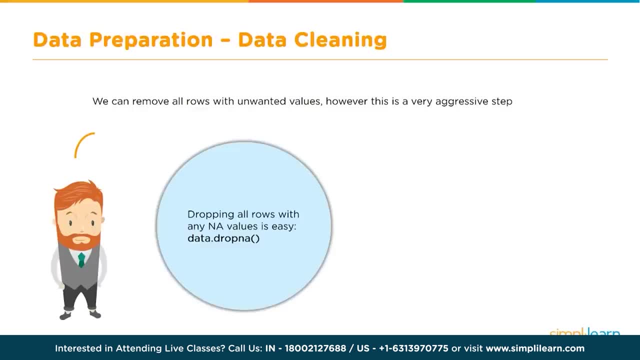 out on. let's say, 60% of the data has some value or the other missing 60% of the rows, then it may not be a good idea to delete all the rows like that manner, because then you're losing pretty much 60% of your data. therefore your analysis won't be accurate. 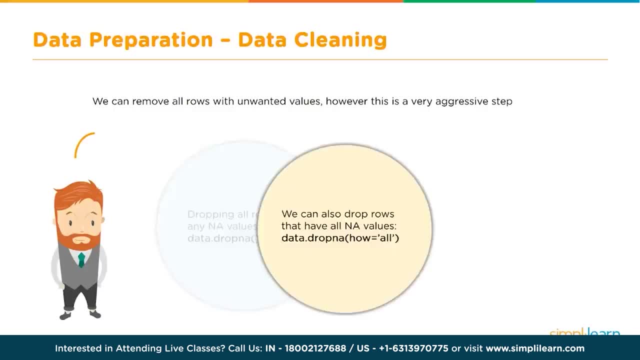 But if it is only five or 10%, then this will work. under way is only to drop values where, or rather drop rows, where all the columns are empty, which makes sense, because that means that record is of really no use because it has no information in it. 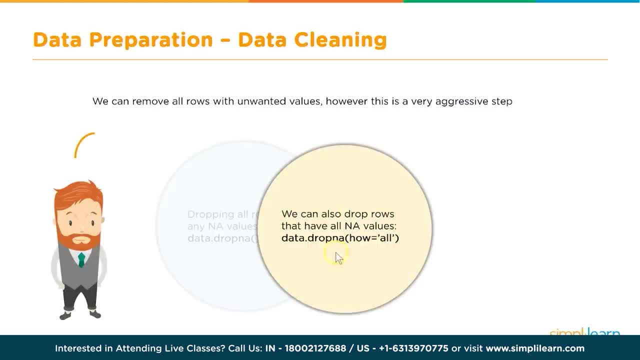 So there can be some situations like that. So we can provide a condition. I'm saying that drop the records where all the columns are blank or not applicable. We can also specify some kind of a threshold. let's say you have 10 or 20 columns in a row. 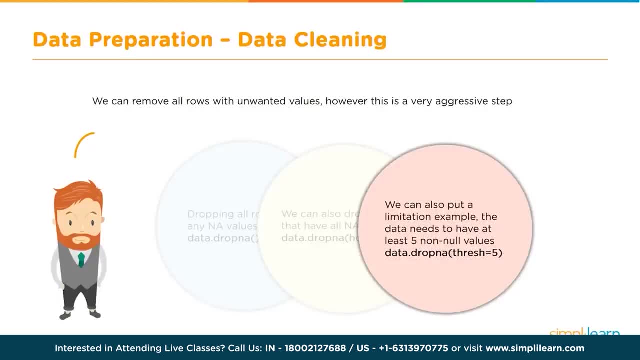 you can specify that maybe five columns are blank or null, then you drop that record. So again, we need to take care that such a condition, such a situation, the amount of data that has been removed or excluded, is not large, if it is like maybe 5% maximum. 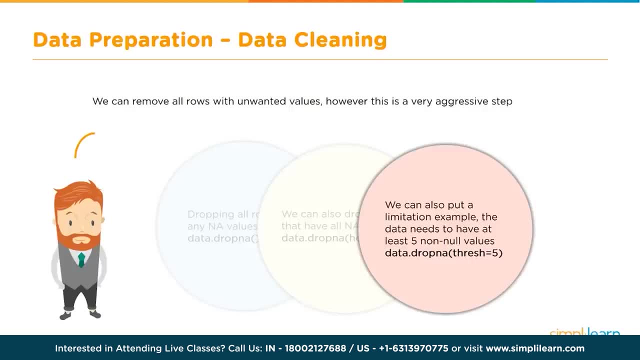 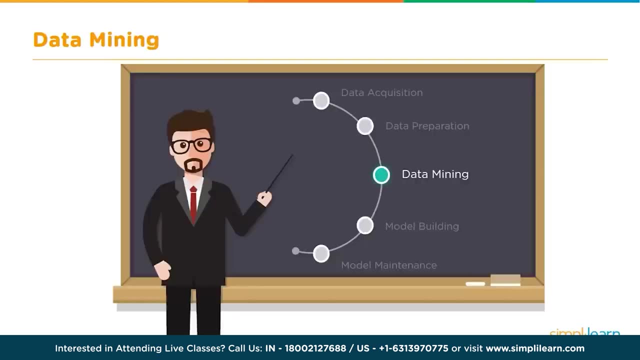 10%, then it's okay, But by doing this, if you're losing out on a large chunk of data, then it may not be a good idea. you need to come up with something better. What else we need to do next is the data preparation part is done. 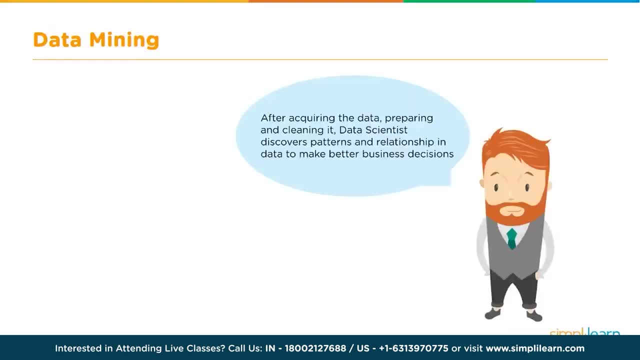 So now we get into the data mining part. So what exactly we do in data mining? primarily, we come up with ways to take meaningful decisions. So data mining will give us insights into the data, what is existing there, and then we can do additional stuff, like maybe machine learning and so on. 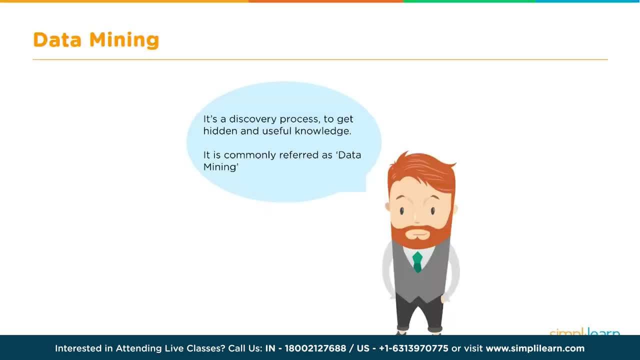 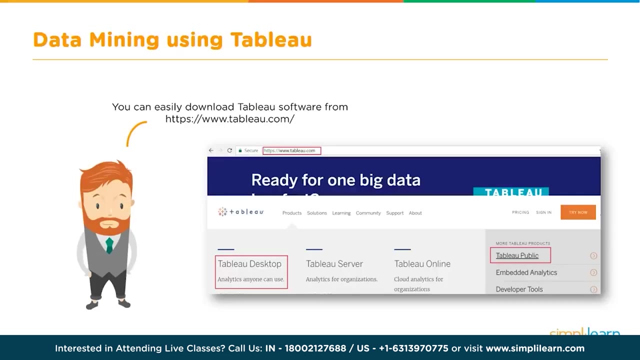 We can perform advanced analytics and so on. So one of the first steps we do is what is known as data discovery, and which is basically like exploratory analysis, So we can use tools like Tableau for doing some of this. So let's just take a quick look at how we go about that. 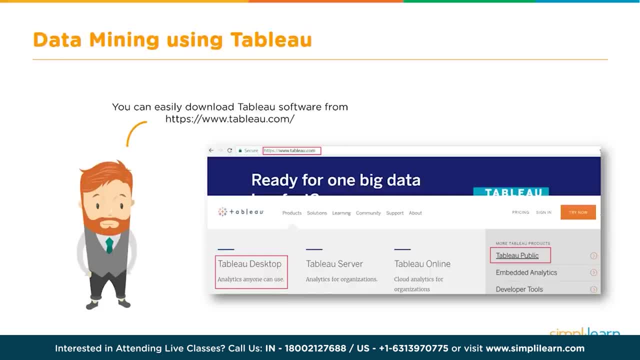 So Tableau is excellent data mining or actually more of a reporting or a BI tool, And you can download a trial version of Tableau at tableaucom. There is also Tableau public, which is free and you can actually use and play around. 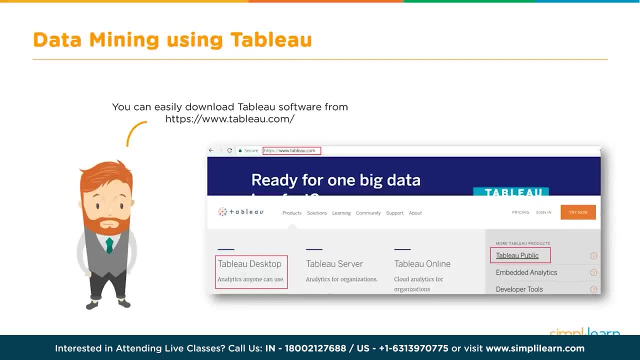 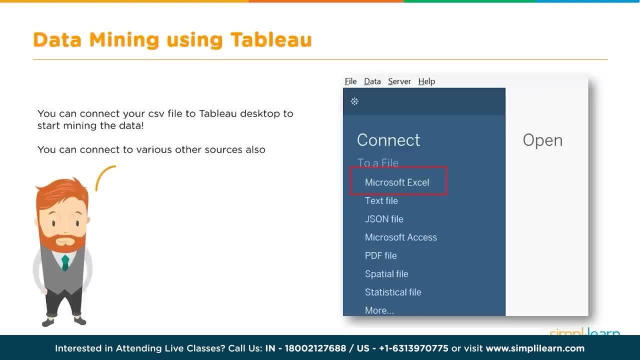 However, if you want to use it for enterprise purpose, then it is commercial software, so you need to purchase license And you can then run some of the data mining activities. say, your data source. your data is in some Excel sheet, So you can select the source as Microsoft Excel or any other format and the data will. 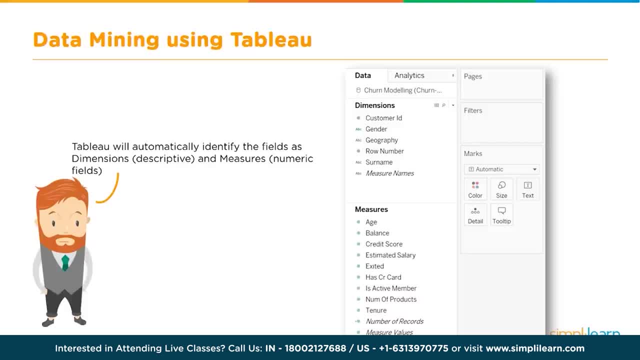 be brought into the Tableau environment, And then it will show up, And then it will show up, And then it will show you what is known as dimensions and measures. So dimensions are all the descriptive columns, and Tableau is intelligent enough to actually. 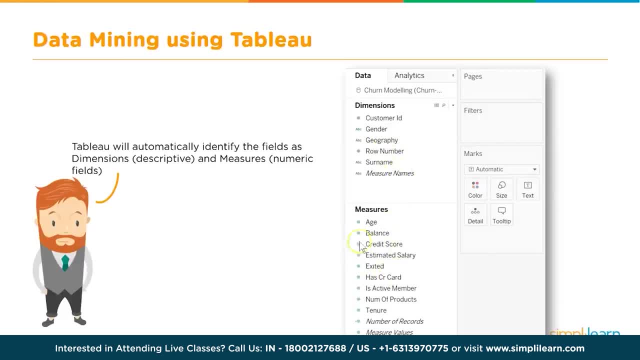 identify these dimensions and measures. So measures are the numerical values. So, as you can see here, customer ID, gender, geography- these are all dimensions, non-numerical values, whereas age, balance, credit score and so on are numeric values. 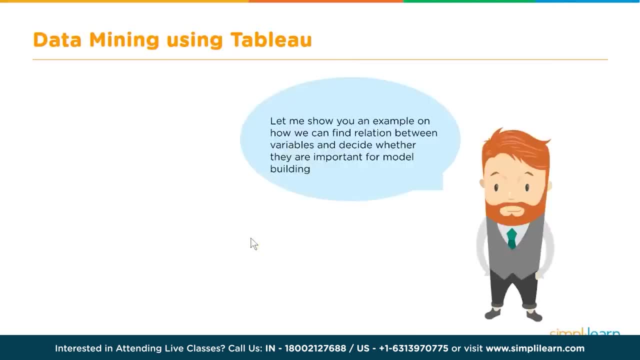 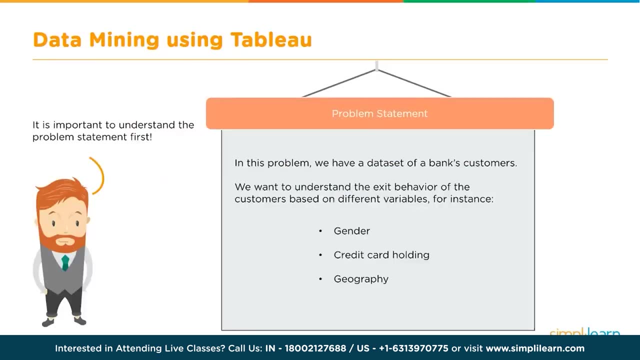 So they come under measures. So you've got your data into Tableau and then you want to, let's say, build a small model and you want to, let's say, solve a particular problem. So what is the problem statement? 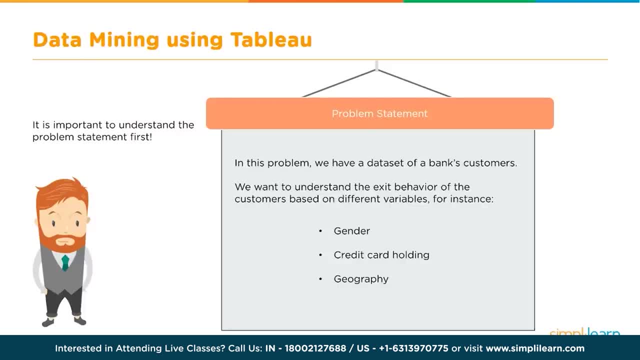 All right, let's say we want to analyze why customers are leaving the bank, which is known as exit, And we want to analyze and see what are some of the factors for exiting the bank. And we want to, let's assume, consider these three of them like, let's say, gender credit. 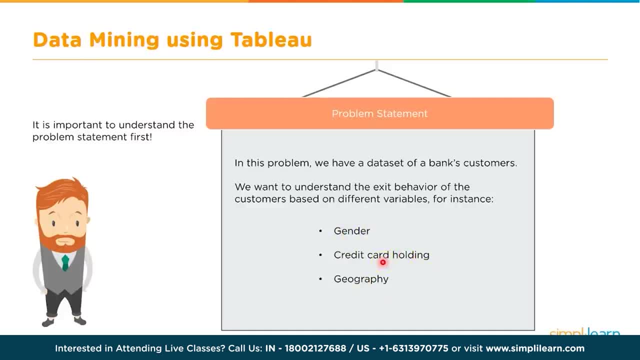 card and geography these as criteria And analyze See if these are in any way impacting or have some bearing on the customer exiting or the customer exit behavior. okay, So let's use Tableau and very quickly we will be able to find out how these parameters 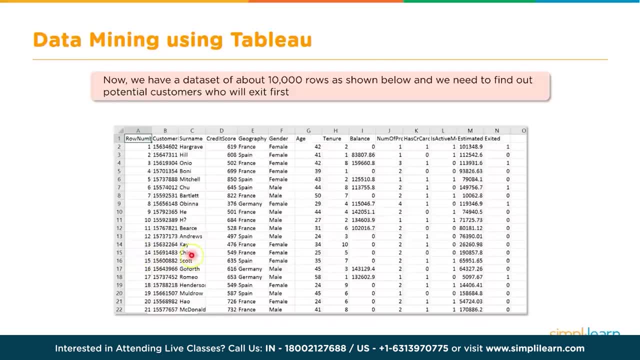 are affecting. all right, So let's see. So this is our customer data. So from our Excel sheet we have data set about, let's say, 10,000 rows and we want to find out what is the criteria. 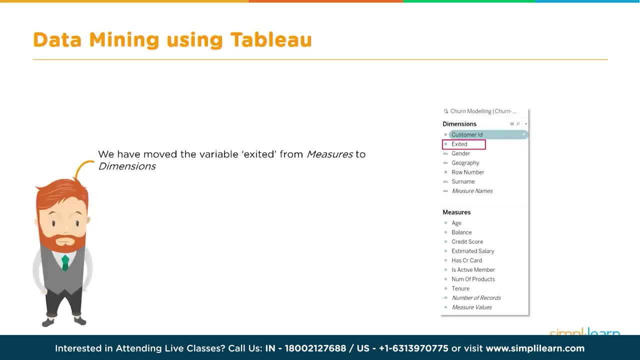 Let's start with gender. Let's say we want to first use gender, We want to first use gender as a criteria. So Tableau really offers an easy drag and drop kind of a mechanism. So that makes it really really easy to perform this kind of analysis. 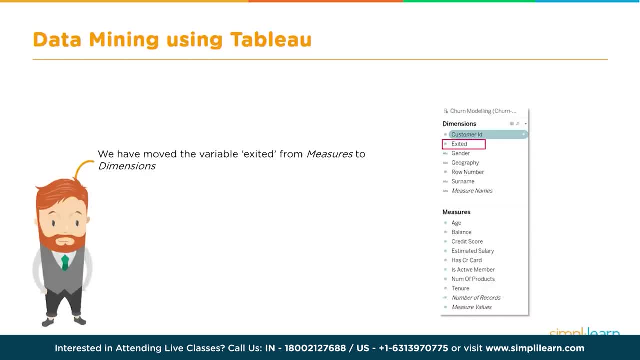 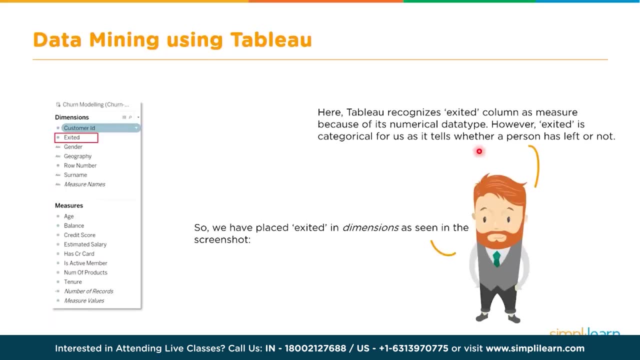 So what we need to do is exit. it says whether the customer has exited or not, So it has a value of zero and one, and then of course, you have gender and so on. So we will take these two and simply drag and drop, okay. 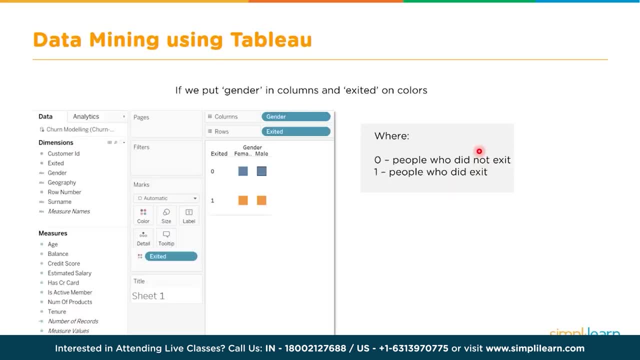 So exit it and then we will put gender And if we drag and drop it to the analysis, So okay, So that's the side of Tableau, All right. So here what we are doing is we are showing male, female as two different columns here. 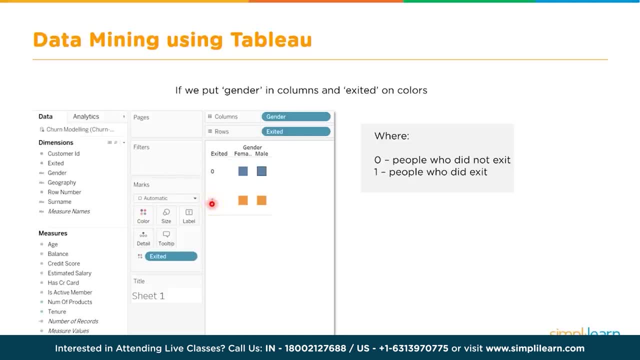 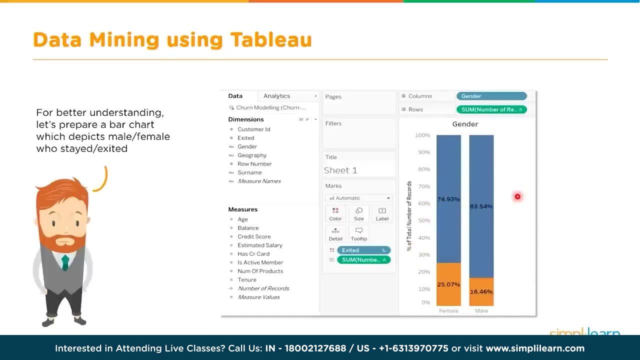 and zero for people who did not exist and one for people who exited, and that is color coded. So the blue color means people who did not exit and this yellow color means people who did exit. All right, So now if we pull the data here, create like bar graphs. this is how it would look. 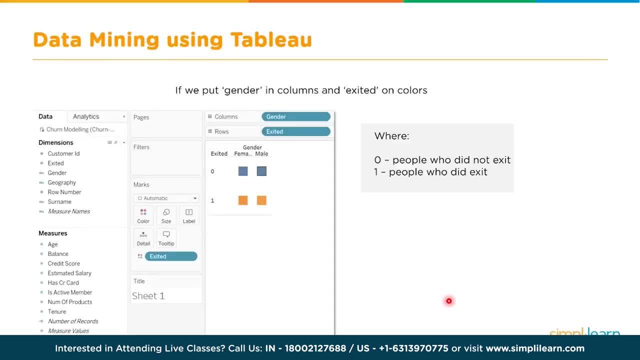 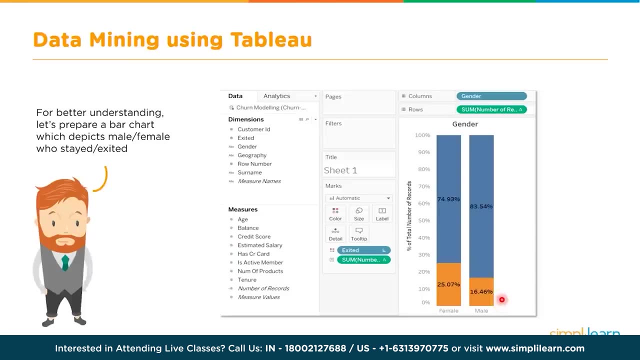 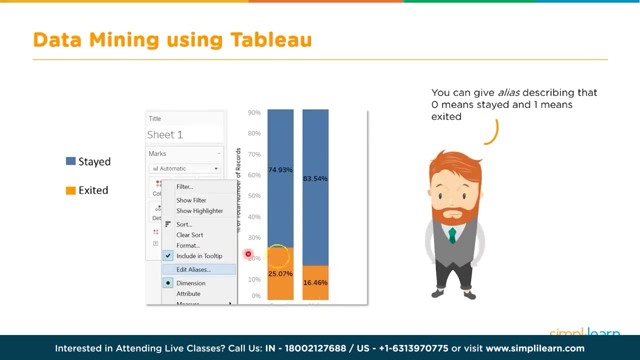 So what is yellow? Let's go back. So yellow is who exited, And for the male, only 16.45% have exited, And we can also draw a reference line that will help us or even provide aliases. So these are a lot of fancy stuff that is provided by Tableau. 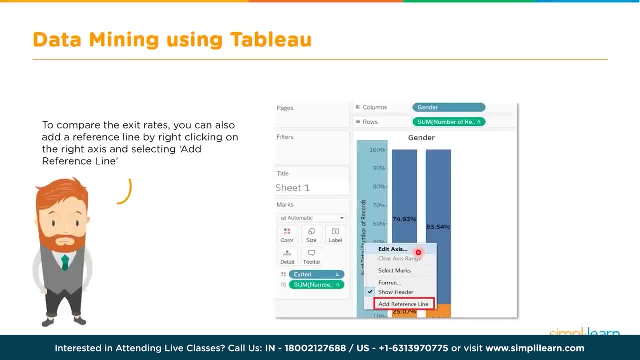 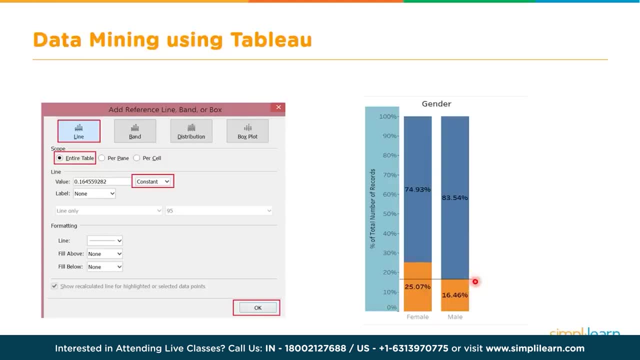 You can create aliases and so that it looks good rather than basic labels, And you can also add a reference line. So you add a reference line, something like this: from here we can make out that on an average female customers exit more. 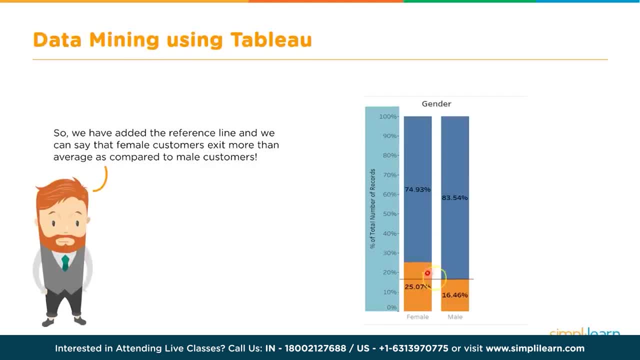 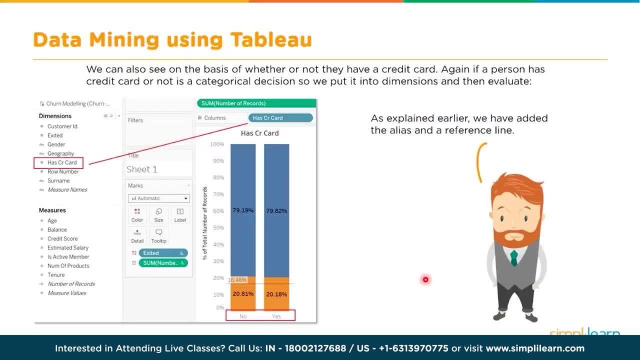 So that is what we are seeing here on an average. So we have analyzed based on gender. we do see that there is some difference in the male and female behavior. Now let's take the next criteria, which is the credit card. So let's see if having a credit card has any impact on the customer exit behavior. 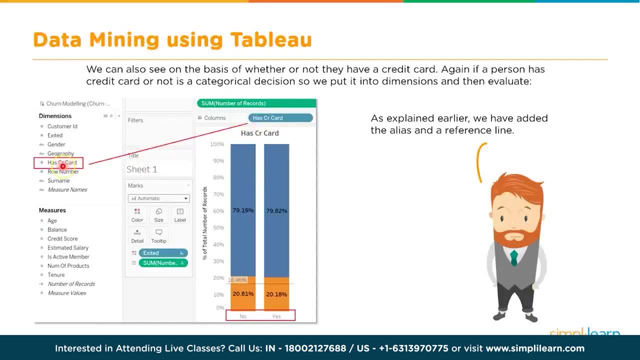 So, just like before we drag and drop the credit card, has credit card a column? if we drag and drop here And then we will see that there is pretty much no difference. The difference between people having credit card and not having credit card: 20.81% of. 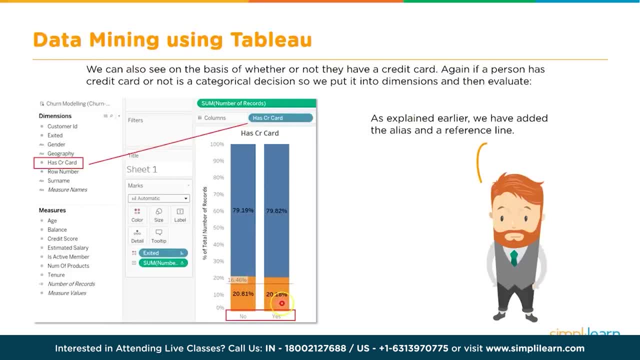 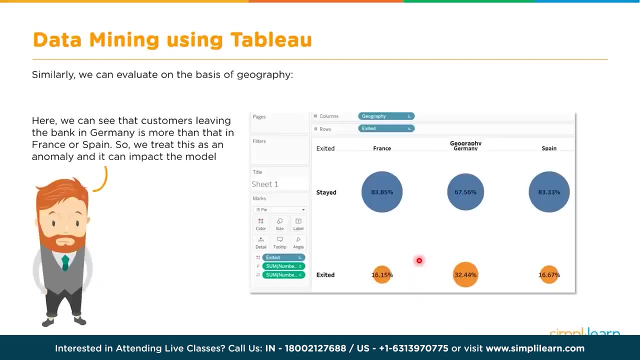 people who have no credit card have exited And similarly, 20.18% of people who have credit card have also exited. So the credit card is not having much of an impact. That's what this piece of analysis shows. Last, we will basically go and check how the geography is impacting. 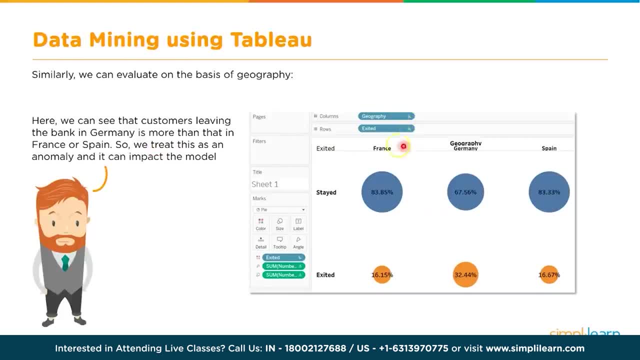 So once again we can drag and drop geography column And if we see here there are geographies like- I think there are about three geographies like France, Germany and Spain, And we see that there is some kind of impact with the geography as well. 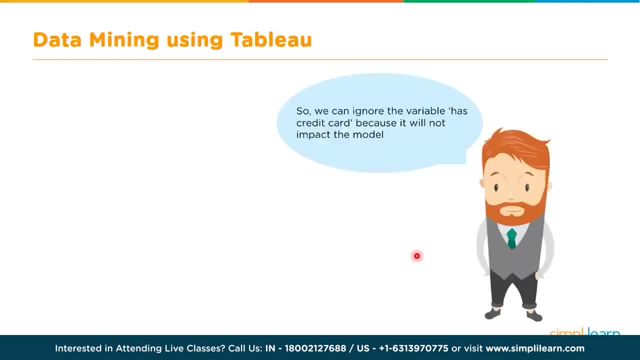 So what we derive from this is that the credit card is really. we can ignore the credit card variable or feature from our analysis because that doesn't have any impact, But gender and geography we can keep And do further analysis. Okay, All right. 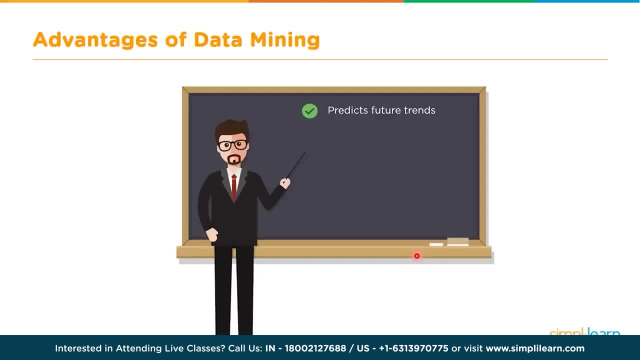 So what are some of the advantages of data mining bit? more detailed analysis can help us in predicting the future trends, and it also helps in identifying customer behavior patterns. Okay, so you can take informed decisions because the data is telling you or providing you with. 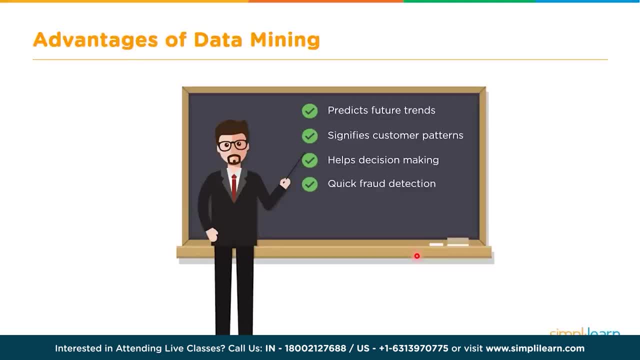 some insights and then you take a decision based on that. If there is any fraudulent activity, data mining will help in quickly identifying such a fraud as well, And, of course, it will also help us in identifying the right algorithm for performing more advanced data mining activities, like machine learning and so on. 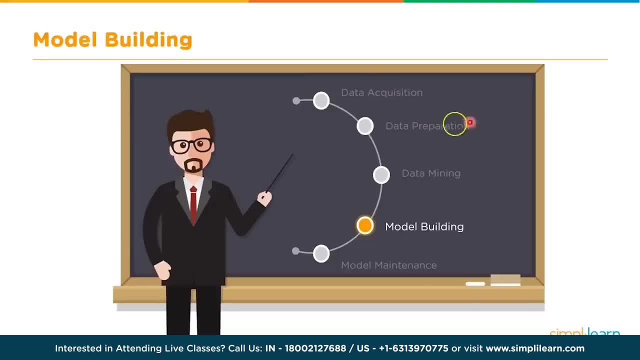 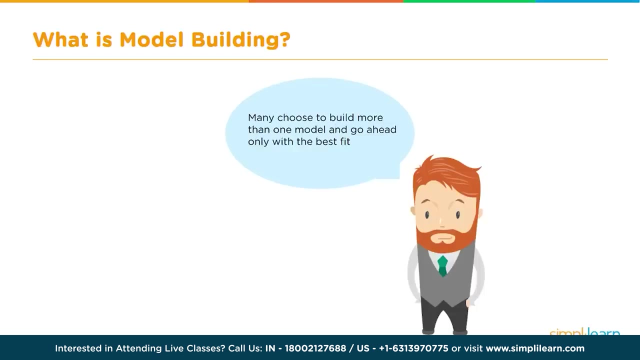 All right. so the next activity, now that we have the data, we have prepared the data and perform some data mining activity- The next step is model building. Let's take a look at model building. So what is a model building if we want to perform a more detailed data mining activity? 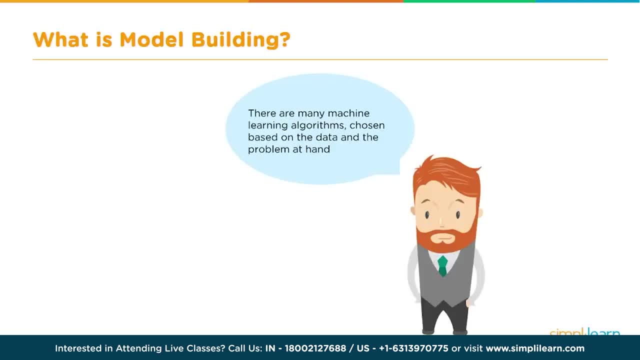 like, If we perform some machine learning, then you need to build a model. and how do you build a model? First thing is you need to select which algorithm you want to use to solve the problem on hand, and also what kind of data that is available, and so on and so forth. 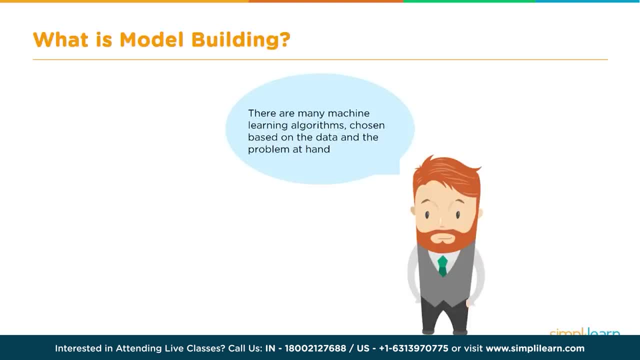 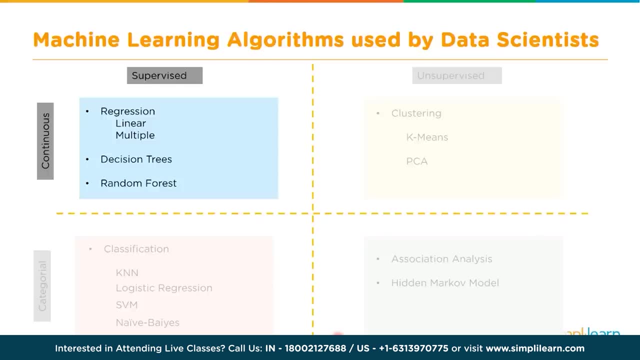 So you need to make a choice of the algorithm and based on that you go ahead and create a model, train the model and so on. Now machine learning is kind of at a very high level, classified into supervised and unsupervised. So if we want to predict a continuous value- it could be a price or a temperature or a. 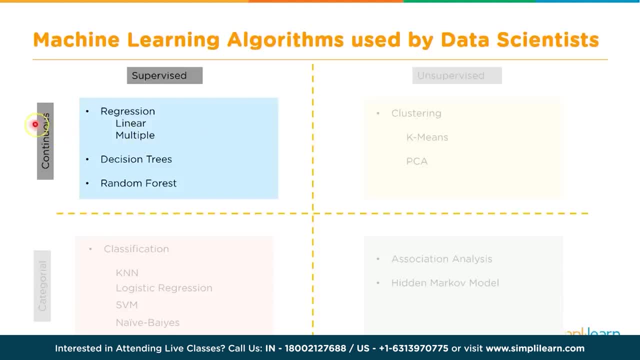 height or a length or things like that. So those are continuous values, and if you want to find some of those, then you use techniques like regression, linear regression, simple linear regression, multiple linear regression, and so on. So these are the algorithms. 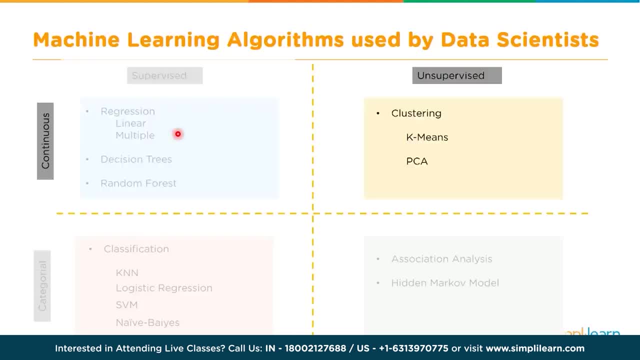 On the other hand, there will be situations, or there may be situations, where you need to perform unsupervised learning. case of unsupervised learning: You don't have any history. You don't have any history. You don't have any historical labeled data to learn from. 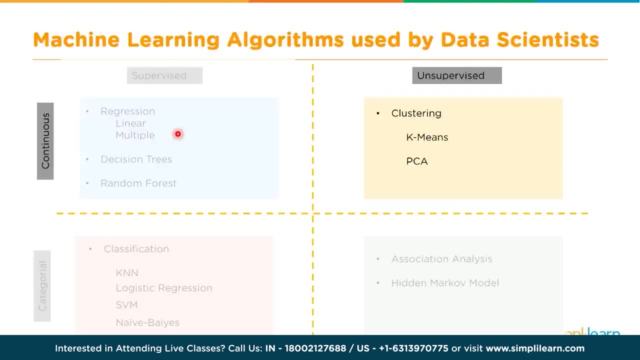 So that is when you use unsupervised learning, and some of the algorithms in unsupervised learning are clustering. K-means clustering is the most common algorithm used in unsupervised learning And similarly in supervised learning, if you want to perform some activity on categorical 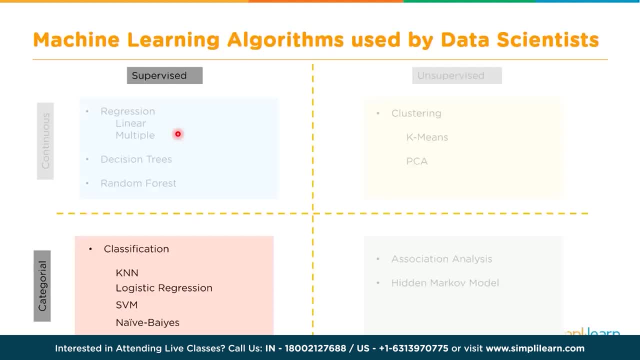 values like, for example, it is not measured, but it is counted. like you want to classify whether this image is a cat or a dog, Whether you want to classify whether this customer will buy the product or not, or you want to classify whether this email is spam or not spam. 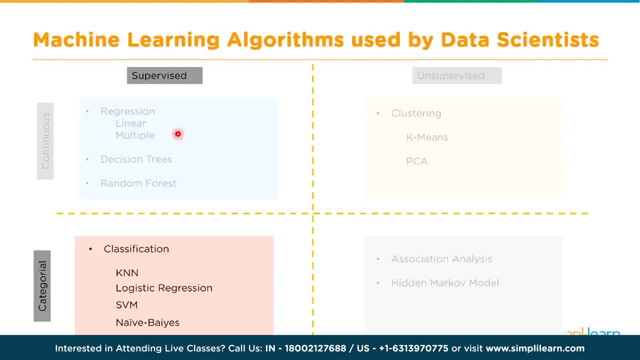 So these are examples of categorical values and these are examples of classification. Then you have algorithms like logistic regression, k-nearest neighbor or KNN and support vector machine. So these are some of the algorithms that are used in this case And similarly in case of unsupervised learning, if you need to perform on categorical values. 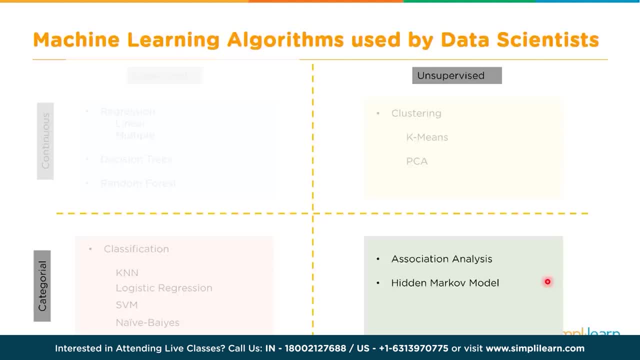 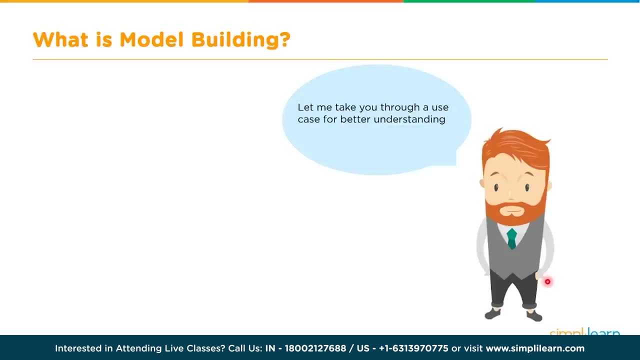 you have some algorithms, Algorithms like association analysis and hidden Markov model. Okay, so in order to understand this better, let's take an example and take you through the whole process, And then we will also see how the code can be written to perform this. 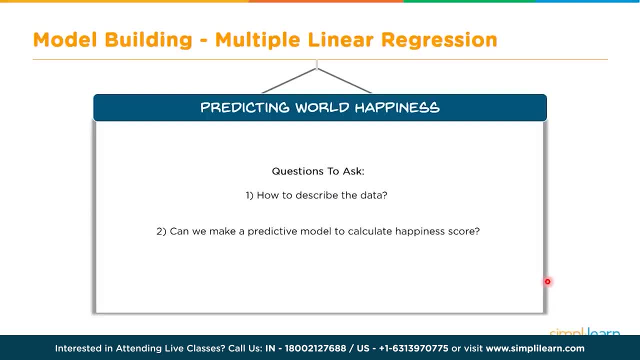 Now let's take our example here, where we want to perform a supervised learning, which is basically we want to do a multilinear regression, which means there are multiple independent variables, And then we want to perform a linear regression to predict certain values. So in this particular example, we have world happiness data. 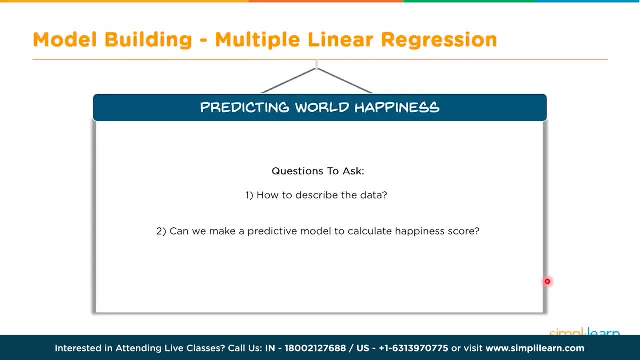 So this is the data about the happiness quotient of people from various countries, And we are trying to predict and see whether our, how, our model will perform. So what is the question that we need to ask? first of all, how to describe the data. 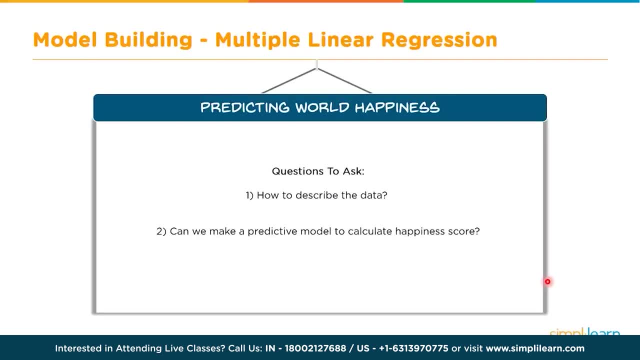 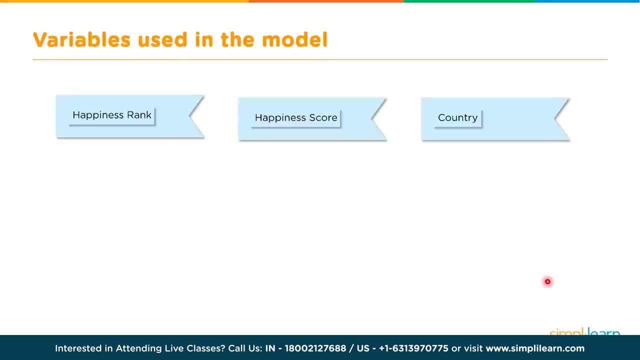 And then can we make a predictive model to calculate the happiness score, right? So based on this, we can then decide on what algorithm to use and what model to use, and so on. So this is the list of variables that are available or used in this model. 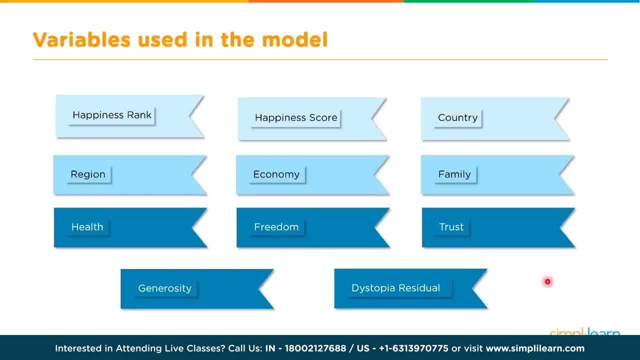 This is a list of variables that are available. There is a happiness rank. I'll load the data and I'll show you the data in a little bit So it becomes clear what are these. So there is what is known as a happiness rank, happiness score, which is happiness score. 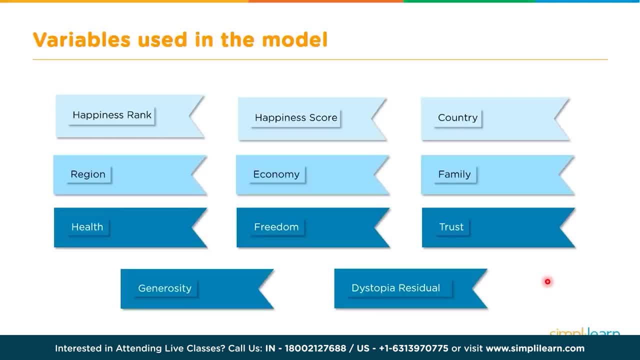 is more like absolute value, whereas rank is: what is the ranking? and then which country we are talking about and within that country, which region and what kind of economy, and whether the family, which family and health details and freedom, Trust, generosity, and so on and so forth. 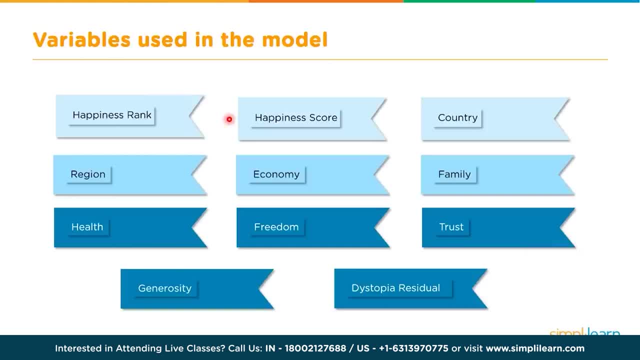 So there are multiple variables that are available to us and the specific details probably are not required, And there can be in another example the variables can be completely different. So we don't have to go into the details of what exactly these variables are, but just 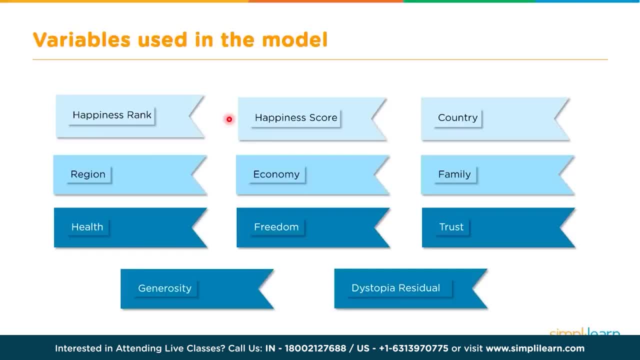 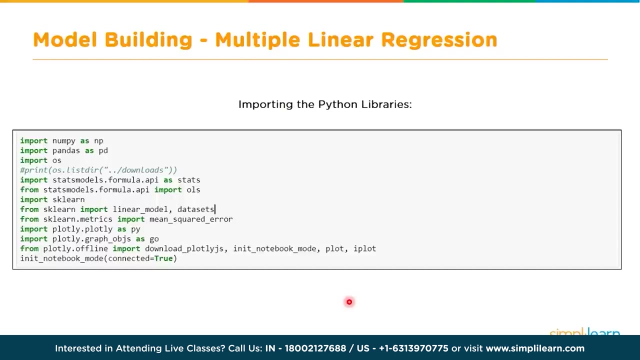 enough to understand that we have a bunch of these variables and now we need to use either all or some of these variables and then, which we also sometimes refer to as features, And then To build our model and train our model. All right, So let's assume we will use Python in order to perform this analysis or perform this machine. 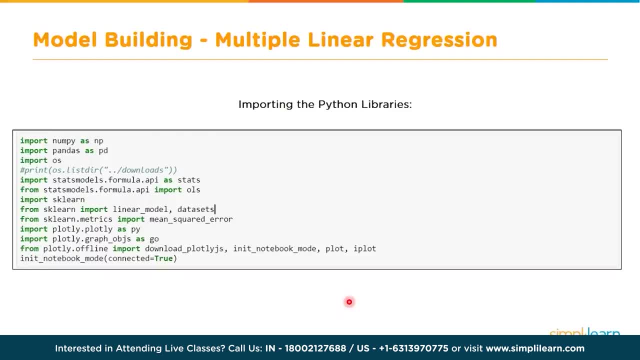 learning activity And I will actually show you in our lab in a little bit this whole thing. we will run the live code, but quickly I will run you through the slides and then we will go into the lab. So what are we doing here? 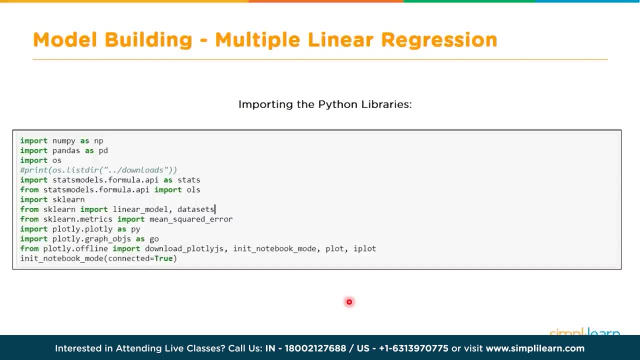 First thing we need to do is import a bunch of libraries in Python which are required to perform our analysis. Most of these are for manipulating the data, the preparing the data, and then scikit-learn or sklearn is the library which we will use actually for this particular machine learning. 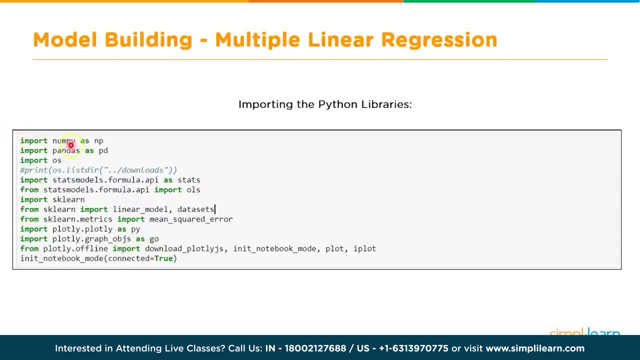 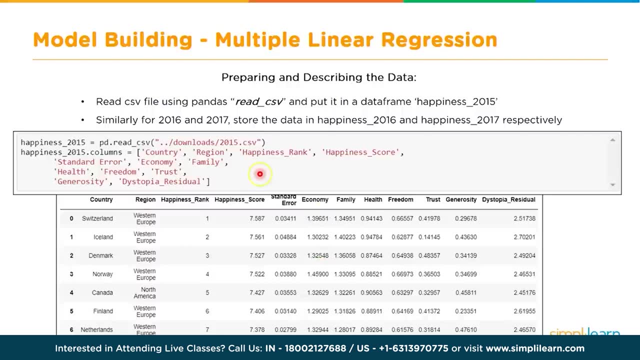 activity, which is linear regression. So we have NumPy, we have pandas and so on and so forth. So all these libraries are imported and then we load our data and the data is in the form of a CSV file, and there are different files for each year. 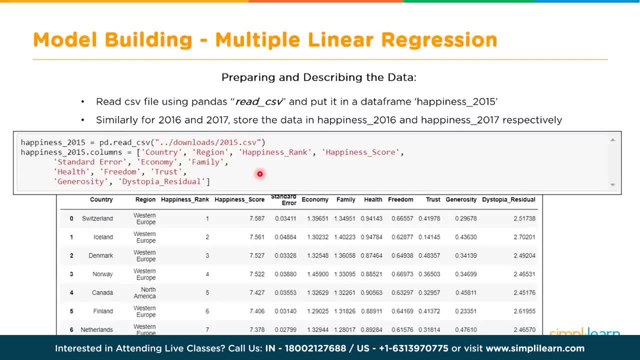 So we have data for 2015,, 16 and 17.. And So we will load this data and then combine them, concatenate them to prepare a single data frame. And here we are making an assumption that you are familiar with Python. so it becomes: 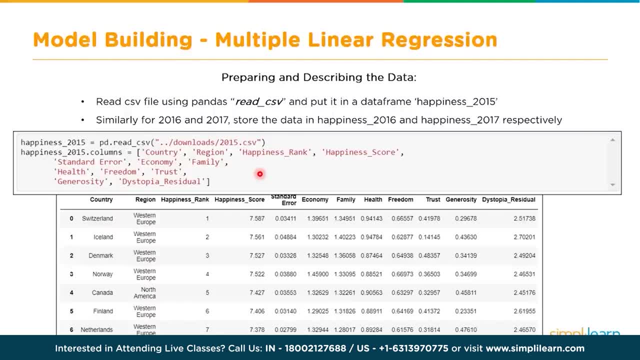 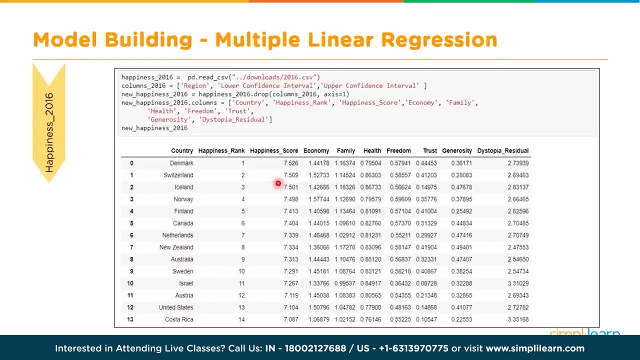 easier if you are familiar with Python programming language, or at least some programming language, so that you can at least understand by looking at the code. So we are reading the file, each of these files for each year, and this is basically. we are creating a list of all the names of the columns that we will be using later on. 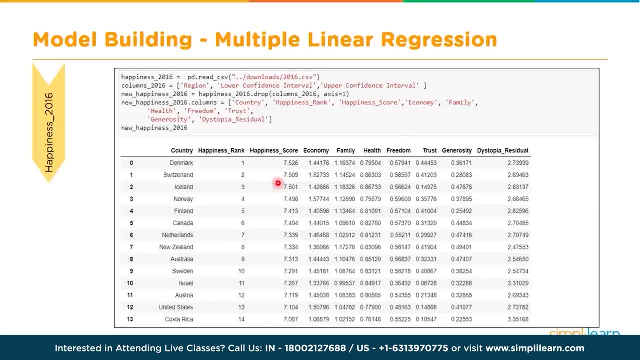 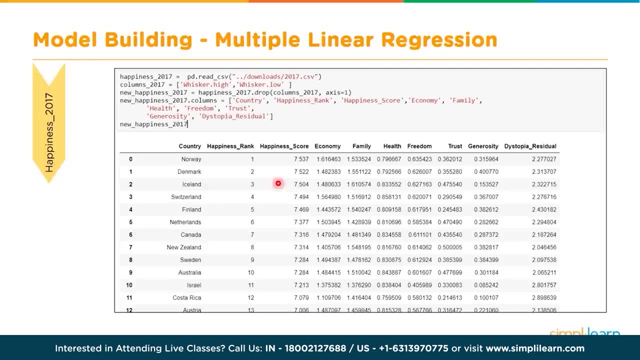 You will see in the description, You will see in the code. So we have loaded 2015,, then 2016 and then also 2017.. So we have created three data frames and then we concatenate all these three data frames. This is what we are doing here. 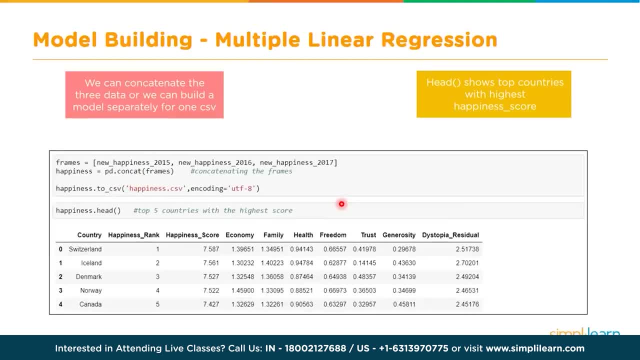 Then we identify which of these columns are required. which, for example, some of the categorical values. do we really need? We probably don't. Then we drop those columns so that we don't unnecessarily use all the columns and make the computation complicated. 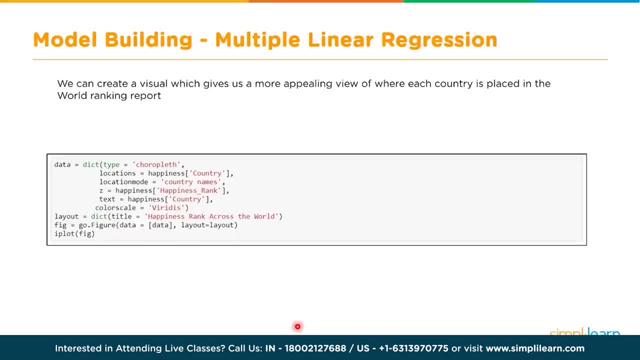 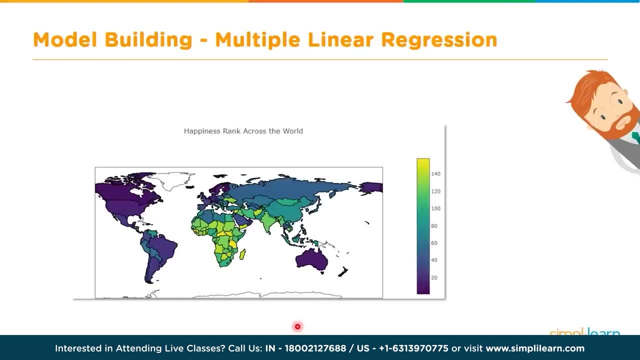 We can then create some plots. It's using plotly library and it has some powerful features, including creation or creation of maps and so on, Just to understand the pattern, the happiness quotient or how the happiness is across all the countries. So it's a nice visualization. 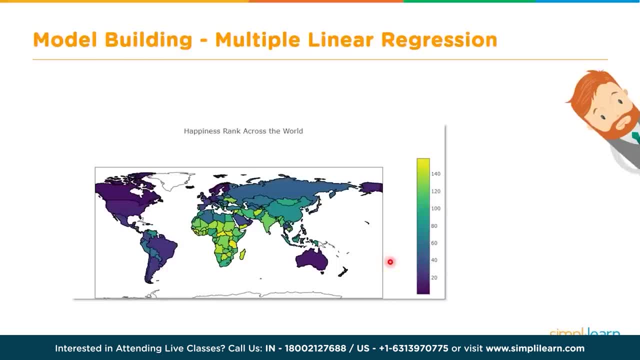 We can see each of these countries how they are in terms of their happiness score. This is the legend here. So the lighter colored countries have lower ranking, And so these are the lower ranking ones and these are higher ranking, which means that the ones with these dark colors are the happiest ones. 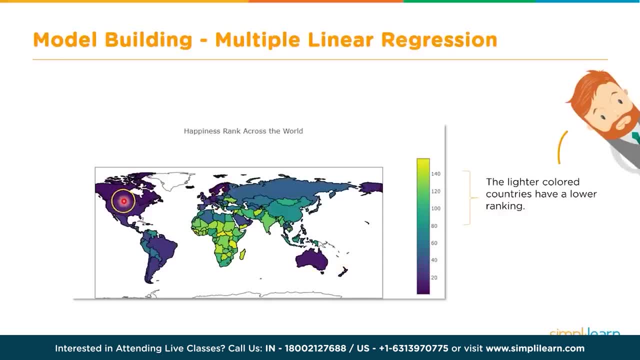 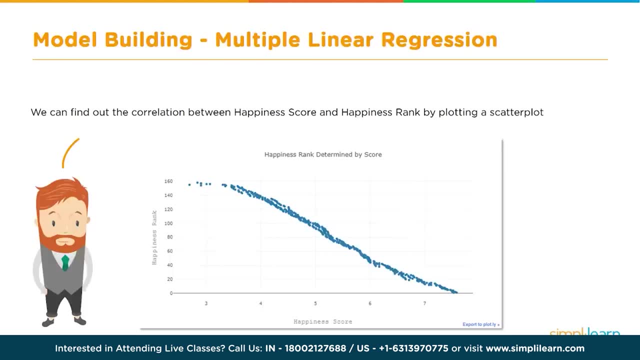 So, as you can see here, Australia and maybe the US and so on, are the happiest ones. The other thing that we need to do is the correlation between the happiness score and happiness rank. We can find a correlation using a scatterplot and we find that, yes, they are kind of inversely. 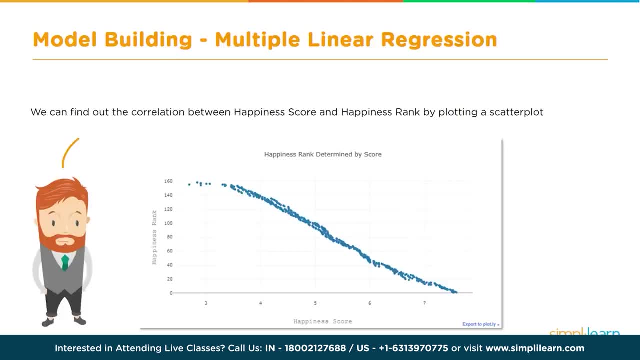 proportionate, which is obvious. So if the score is high, happiness score is high, then they are ranked number one. for example, highest is scored as number one. So that's the idea behind this. So the happiness score given here and the happiness rank is actually given here. 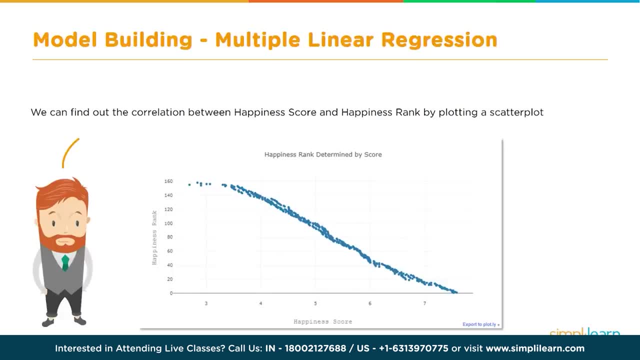 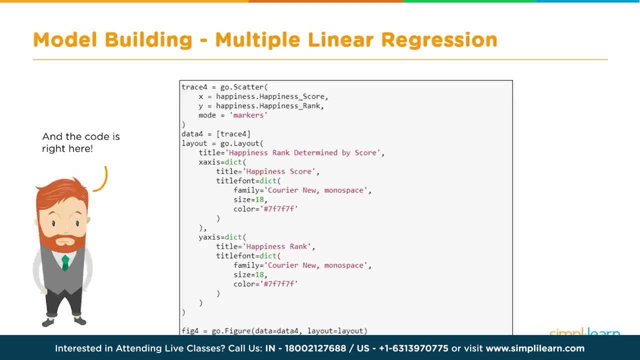 So they are inversely proportional, because the higher the score, the absolute value of the rank will be lower. right Number one has the highest value of the score, and so on. So they are inversely correlated, But there is a strong. what this graph shows is that there is a strong correlation between: 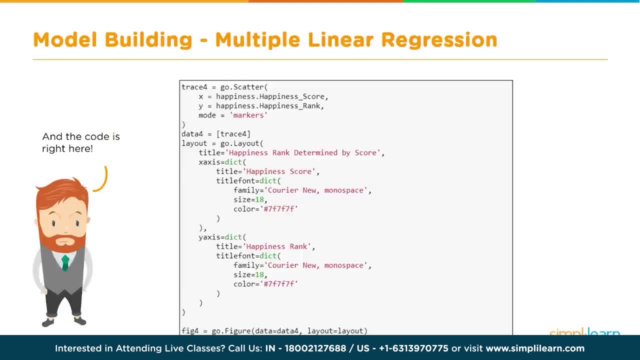 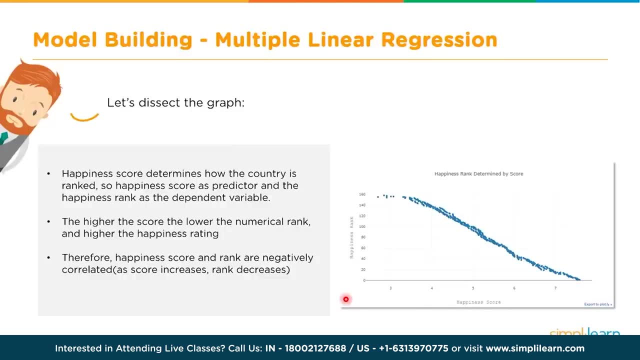 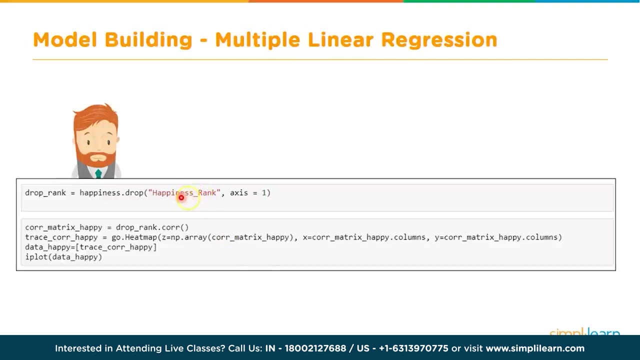 happiness rank and happiness score. And then we do some more plots To visualize this. we determined that probably rank and score are pretty much conveying the same message, So we don't need both of them. So we will kind of drop one of them, and that is what we are doing here. 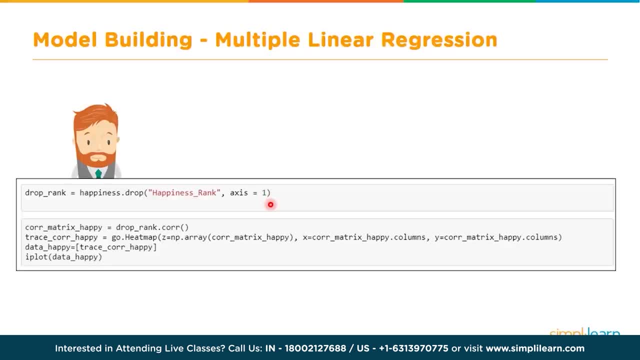 So we dropped the happiness rank And similarly so. this is one example of how we can remove some columns which are not adding value, So we will see in the code as well how that works. Moving on, this is a correlation between pretty much each of the columns with the other columns. 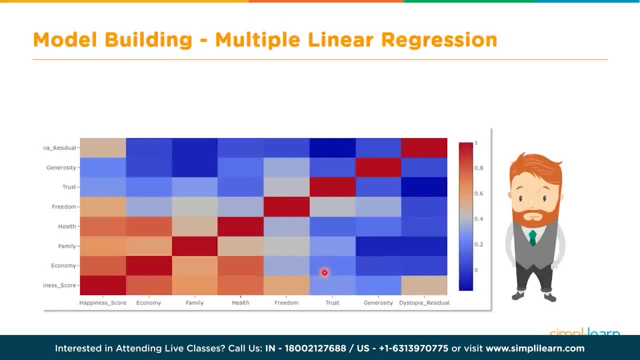 Okay, So this is a correlation you can plot using plot function and we will see here that, for example, happiness score and happiness score are correlated. strongest correlation, right, Because every variable will be highly correlated to itself. So that's the reason. So the darker the color is, the higher the correlation and as so the correlation in numerical. 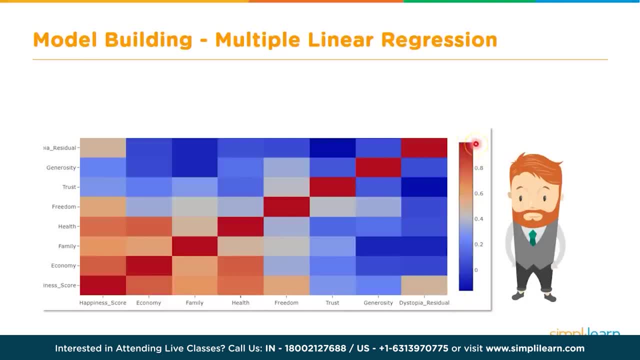 terms goes from zero to one. So one is the highest value and it can only be between zero and one. correlation between two variables. It can only have a value between zero and one, So the numerical value can go from zero to one, And one here is dark color and zero is kind of dark but it is blue color from red. 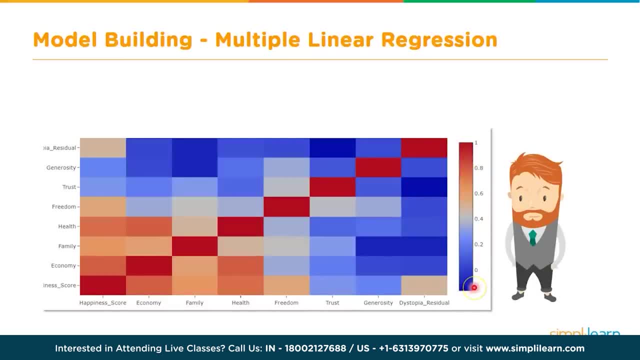 It goes down. The dark blue color indicates pretty much no correlation. So from this heat map we see that happiness and economy and family are probably also help, probably are the most correlated. and then it keeps decreasing after freedom kind of keeps decreasing. Yeah. 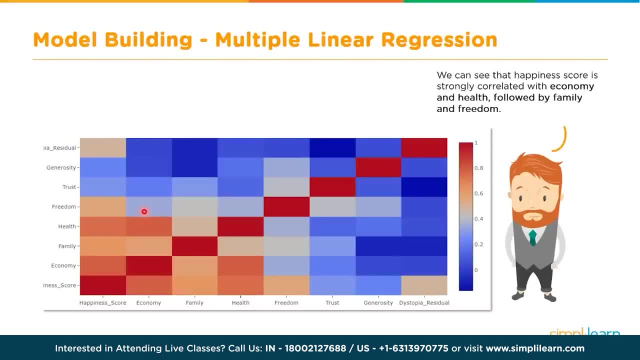 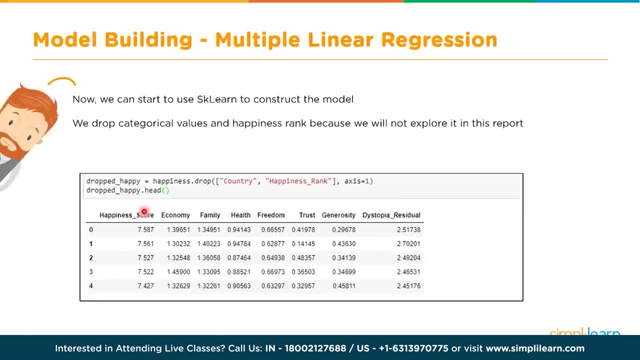 So that's pretty much all right. So that is a correlation graph, and then we can probably use this to find out which are the columns that need to be dropped and do not have very high correlation, and we take only those columns that we will need. 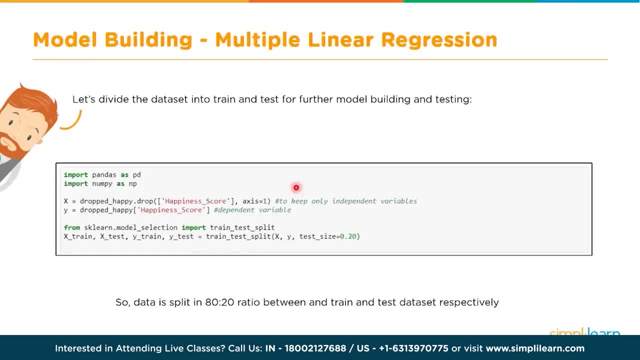 So this is the code for dropping some of the columns Once we have prepared the data. when we have the required columns, then we use scikit-learn to actually split the data. First of all, this is a normal machine learning process, Yeah. 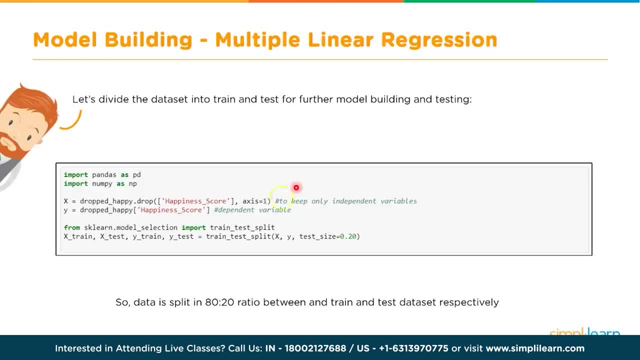 You need to split the data into training and test data set. In this case, we are splitting into 80, 20.. So 80 is the training data set and 20 is the test data set. So that's what we are doing here. 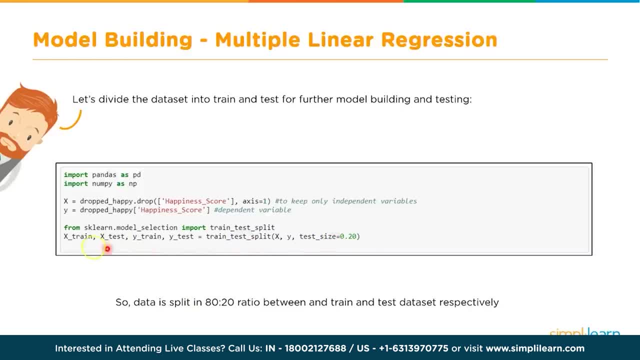 So we use train test split method or function. So you have all your training data in X underscore train, the labels in Y underscore train. Similarly, X underscore test has the test data, the inputs, whereas the labels are in Y underscore test. 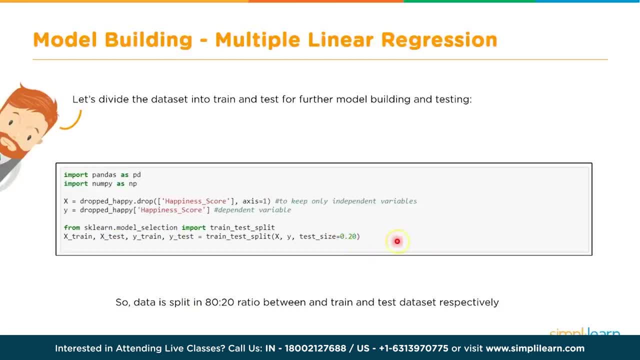 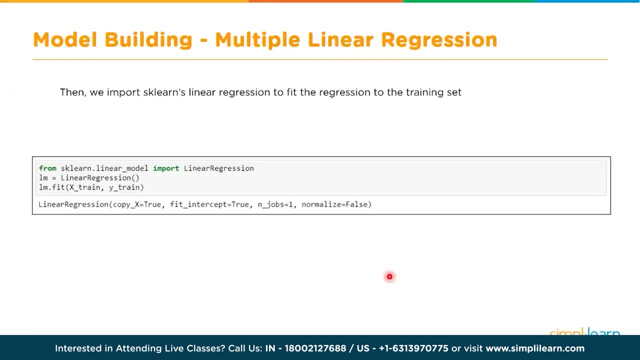 So that's all. And this value- whether it is 80, 20 or 50, 50,, that is all individual preference. So in our case, we are using 80, 20.. All right, And then the next is to create a linear regression instance. 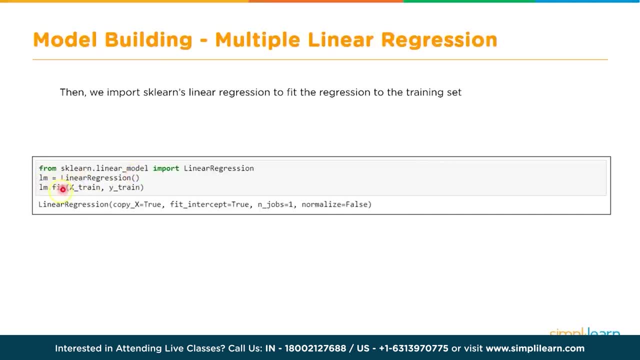 So this is what we are doing: We are creating an instance of linear regression and then we train the model using the fit function And we are passing X and Y, which is the X value, and the label data- regular input- and the label data, label information. 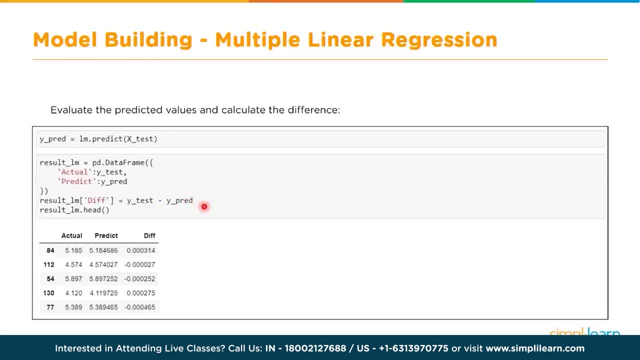 Then we do this, Okay, And then we do the test, We run or we perform the evaluation on the test data set. So this is what we are doing with the test data set And then we will evaluate how accurate the model is using the scikit-learn functionality. 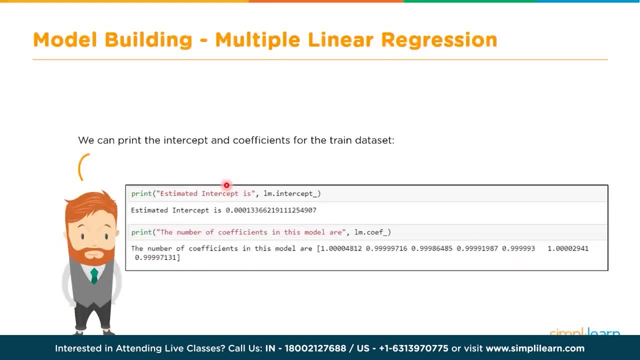 itself. We can also see what are the various parameters and what are the various coefficients, Because in linear regression you will get like an equation of, like a straight line: Y is equal to beta 0 plus beta 1, X1 plus beta 2, X2.. 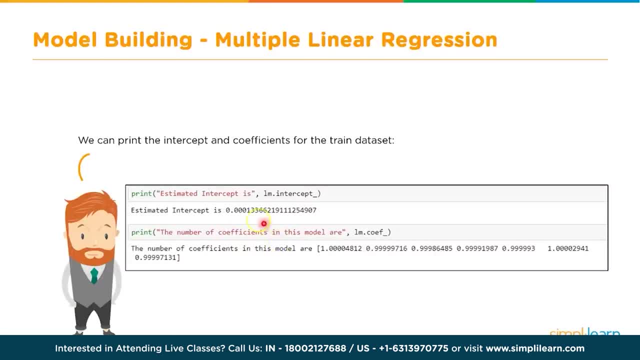 So those beta 1, beta 2, beta 3.. Beta 1, beta 2, beta 3 are known as the coefficients and beta 0 is the intercept. After the training you can actually get these information of the model. 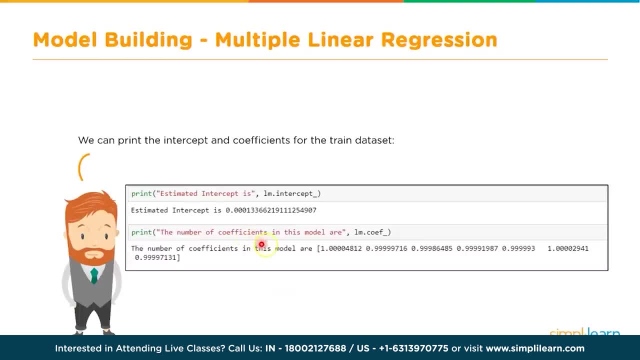 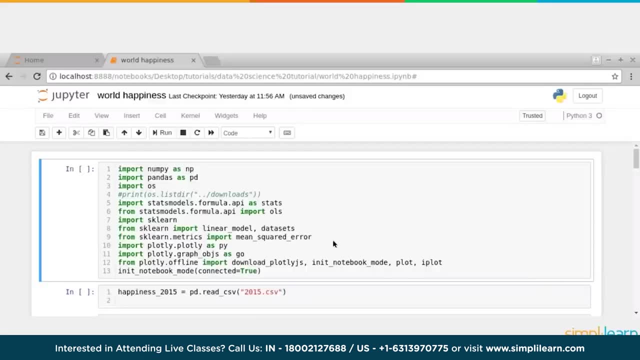 What is the intercept value, What are the coefficients, and so on, by using these functions. So let's quickly go into the lab and take a look at our code. Okay, So this is my lab, This is my Jupyter notebook, where the code. I have the actual code and I will take you. 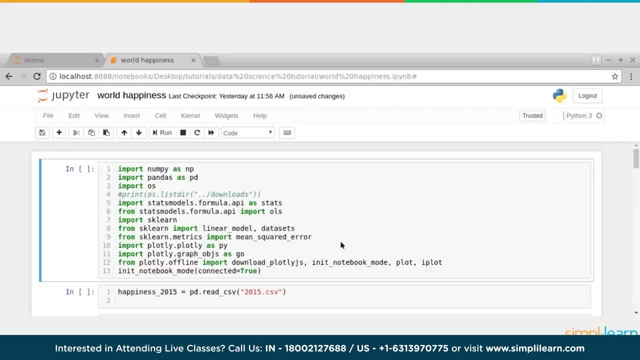 through this code. Okay, So I have code to run this linear regression on the world happiness data. So we will import a bunch of libraries: NumPy, Pandas, Plotly, and so on. Also, yeah, scikit-learn, that's also very important. 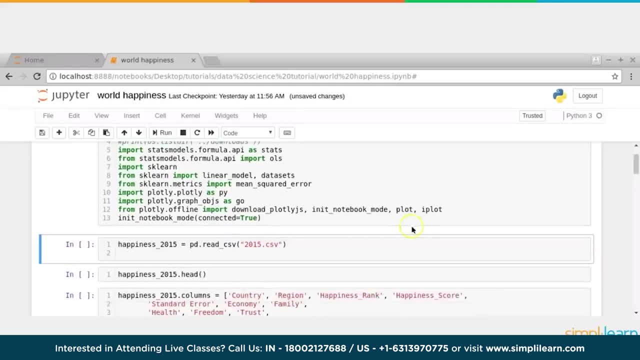 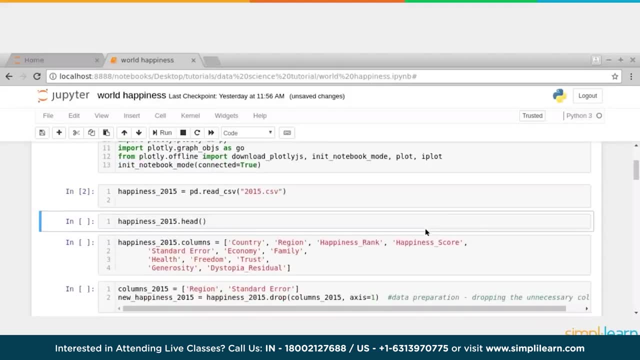 So that's the first step. Then I will import my data, and the data is in three parts. There are three files, one for each year- 2015,, 2016, and 2017, and it is a CSV file. 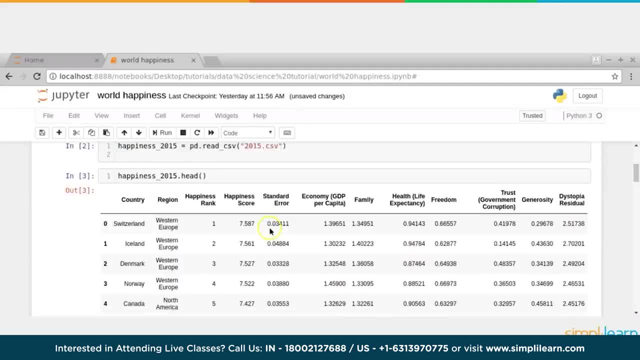 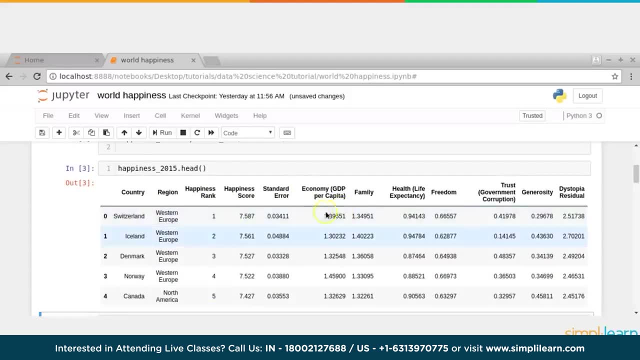 So I've imported my data. Let's take a look at the data quickly. glance at the data. So this is how it looks. We have the country, region, happiness rank and then happiness score. There are some standard errors, and then what is the per capita family, and so on. 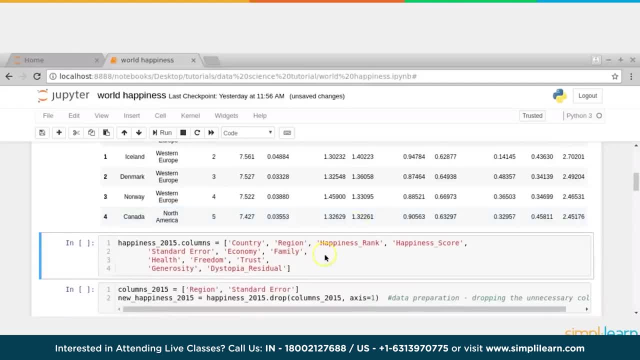 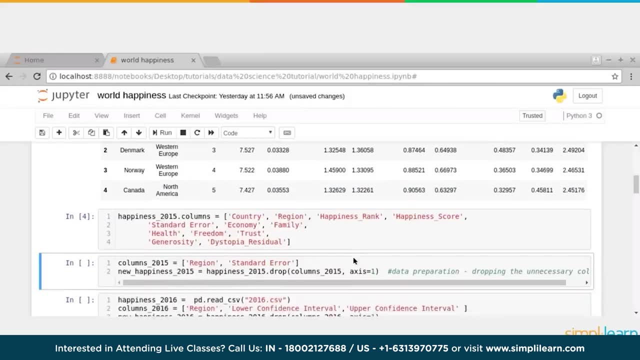 So then we will keep going. We will create a list of all these column names we will be using later. So for now, just I will run this code and no need of major explanation at this point. We know that some of these columns probably are correct. 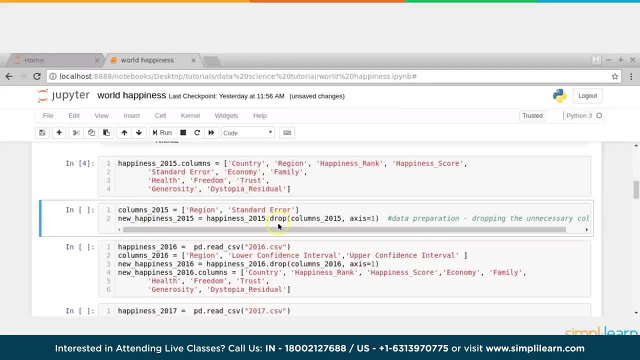 Okay, They are not required, So you can use this drop functionality to remove some of the columns which we don't need, Like for example, region and standard. error will not be contributing to our model, So we will basically drop those values out here. 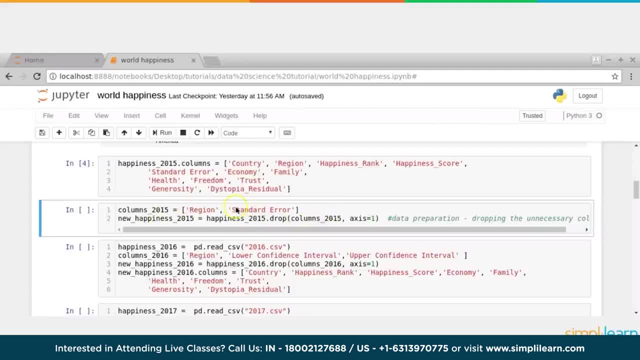 So we use the drop and then we created a vector of it. these names column names. that's what we are passing here. Instead of giving the names of the columns here, we can pass a vector. So that's what we are doing. 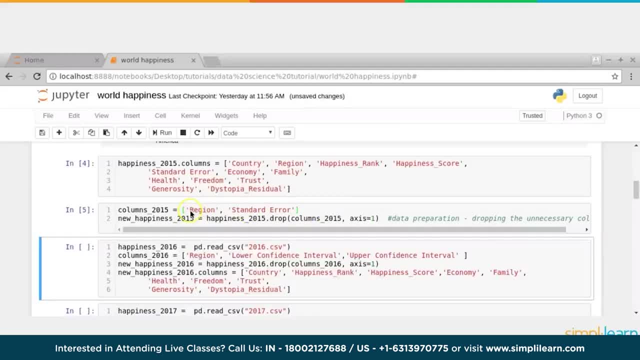 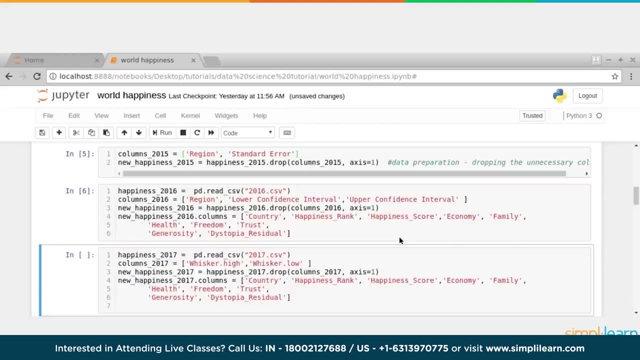 So this will drop from our data frame. It will remove region and standard error, these two columns. Then the next step: we will read the data for 2016 and also 2017 and then we will concatenate this data. So let's do that. 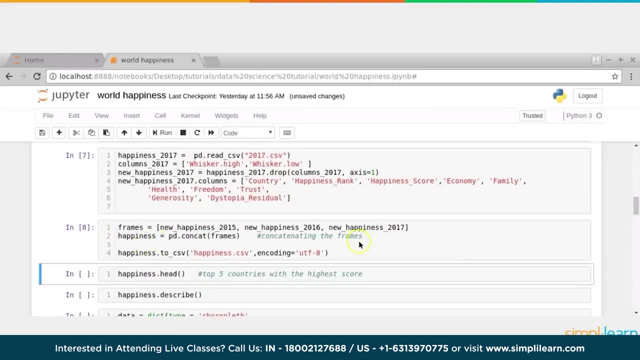 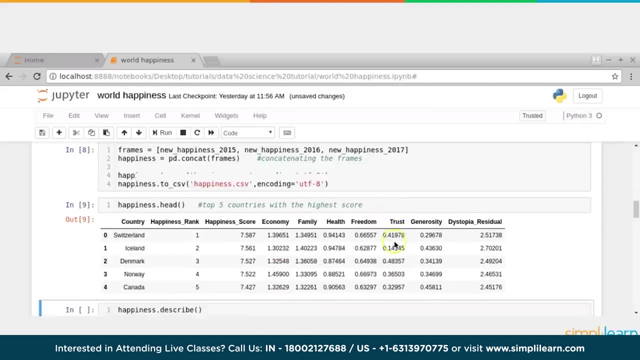 So we have now data frame called happiness, which is a concatenation of both all the three files. Let's take a quick look at the data now. So most of the unwanted columns have been removed and you have all the data in one place for all the three years. 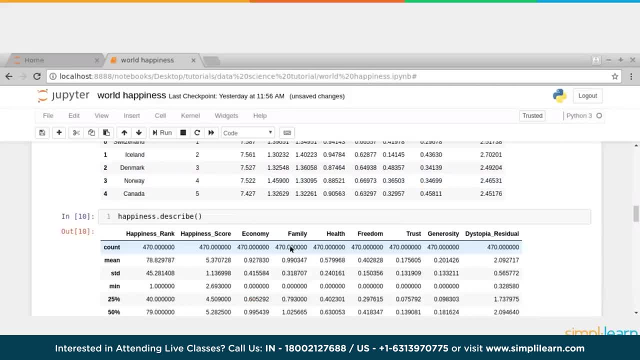 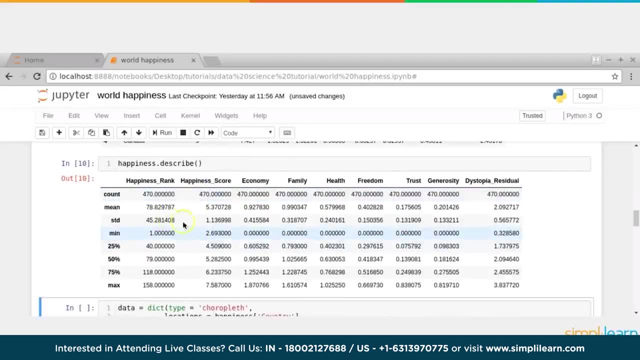 And this is how the data looks. And if you want to take a look at the summary of the columns, you can say describe and you will get this information. For example, for each of the columns: what is the count? what is the mean value standard? 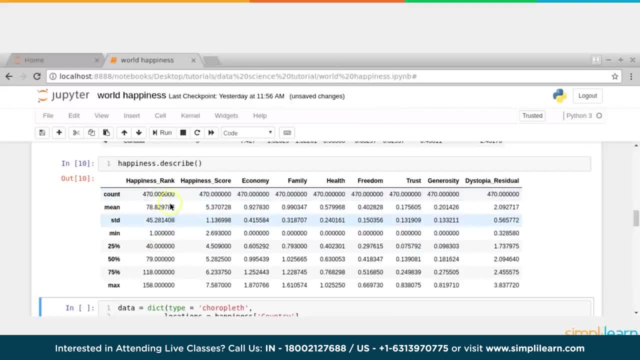 deviation, especially the numeric values, not the categorical values. So this is a quick way to see how the data is and initial little bit of exploratory analysis can be done here. So what is the maximum value, What's the minimum value, And so on. 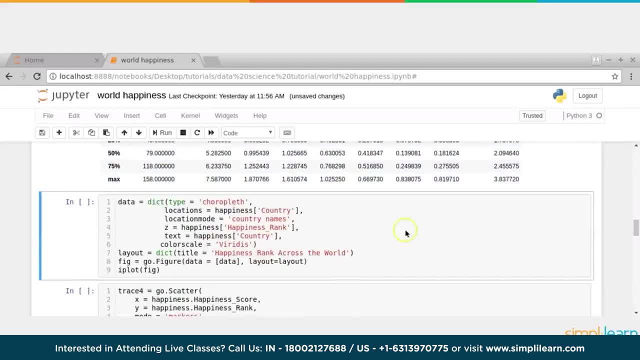 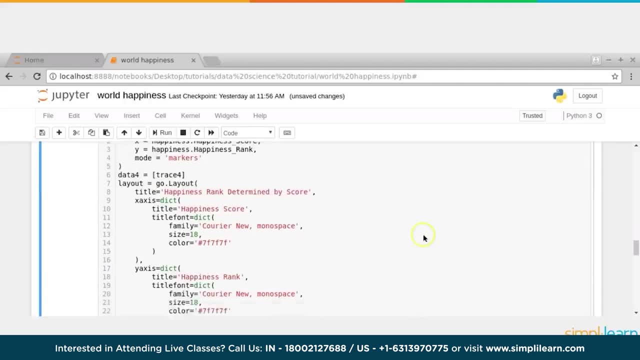 So let's take a look at the results of the columns. All right, so then we go ahead and create some visualizations using Plotly. So let us go and build a plot. So if we see here now, this is the relation correlation between happiness, rank and happiness. 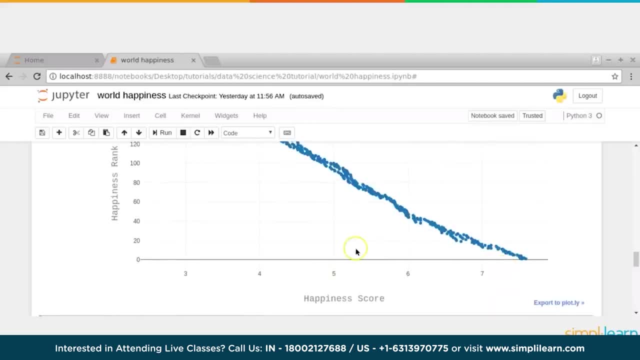 score. This is what we have seen in the slides as well. We can see that there is a tight correlation between them. Only thing is it is inverse correlation, but otherwise they are very tightly correlated, which also says that they both probably, Probably- 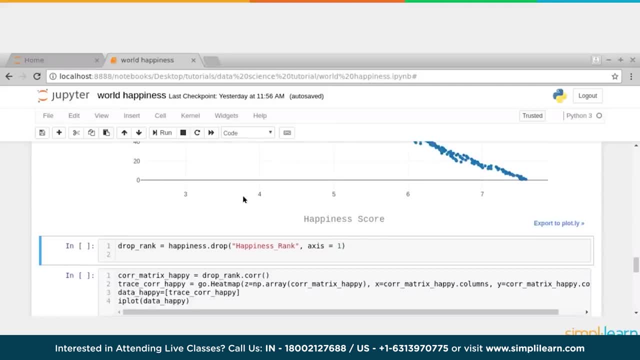 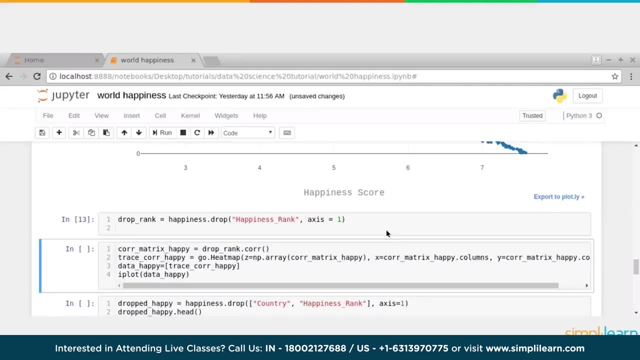 Provide the same information. So there is no, not much of value add. So we'll go ahead and drop the happiness rank as well from our columns. So that's what we're doing here And now we can do. the creation of the correlation heat map. 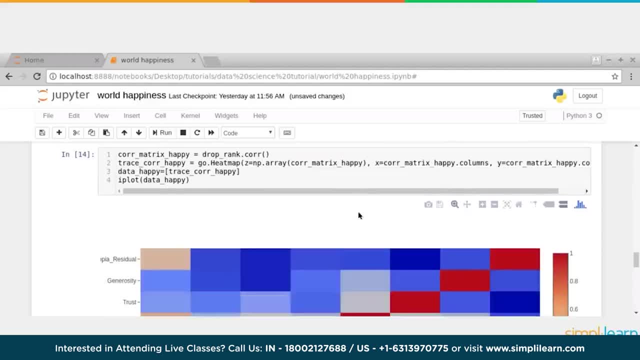 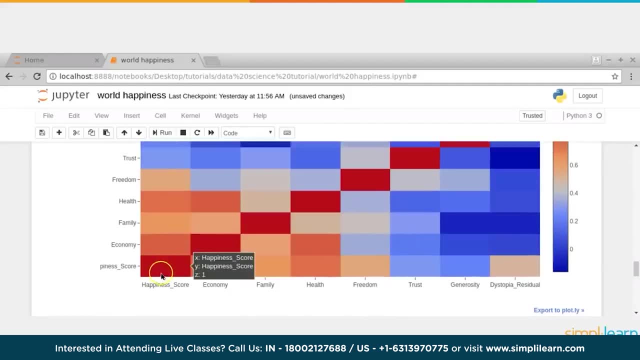 Let us plot the correlation heat map to see how each of these columns is correlated to the others. And we, as we have seen in the slides, this is how it looks. So happiness score is very highly correlated. So this is the legend. we have seen in the slide as well. 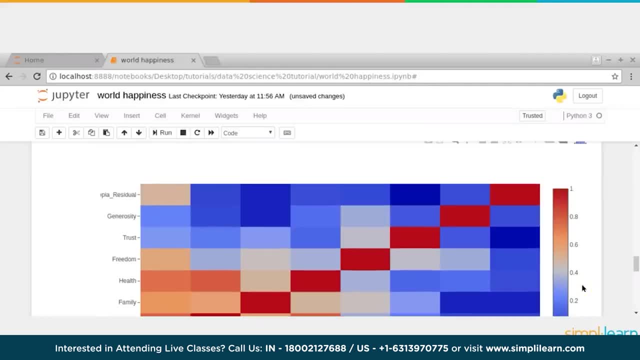 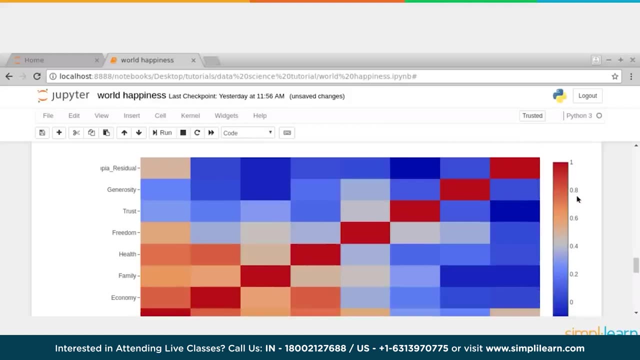 So blue color indicates pretty much zero or very low correlation. Deep red color indicates very high correlation and the value correlation is a numeric value and the value goes from zero to one. If the two items or two features or columns are highly correlated, then there will be 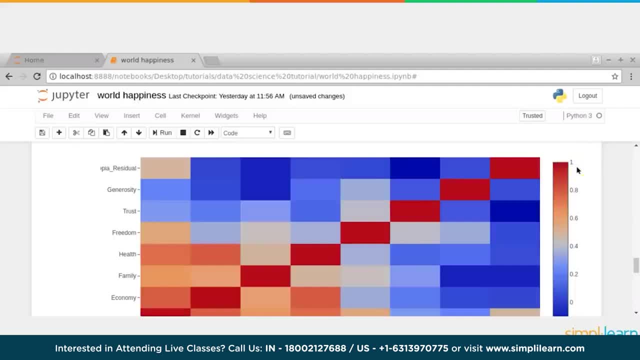 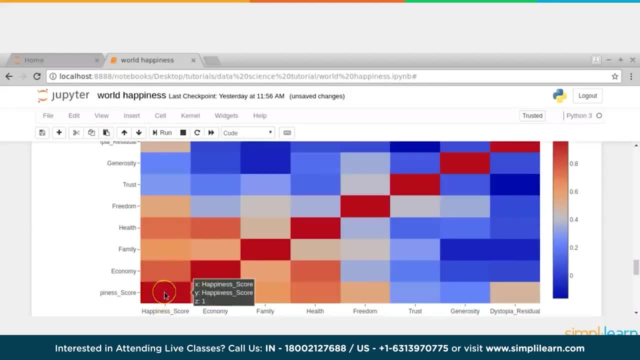 as close to one as possible, and two columns that are not at all correlated will be as close to zero as possible. So that's how it is. For example here- happiness score and happiness score- Every column or every feature will be highly correlated to itself. 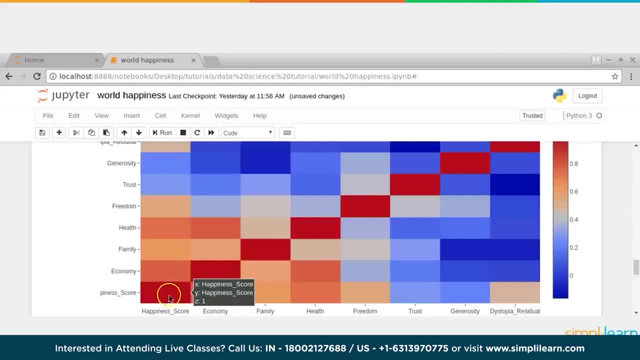 So it is like between them there will be correlation. value will be one, So that's why we see deep red color, But then others are. for example, with higher values are economy and then health and then maybe family and freedom. So these are- generosity and trust- are not very highly correlated to happiness score. 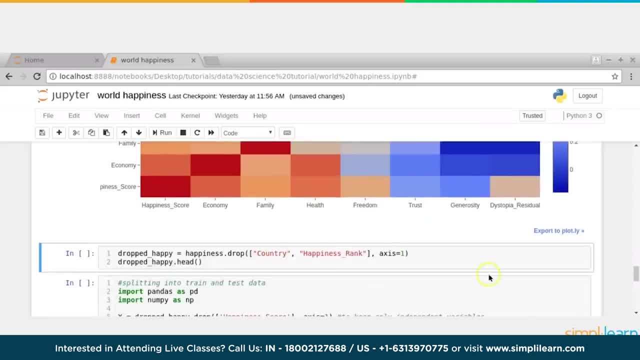 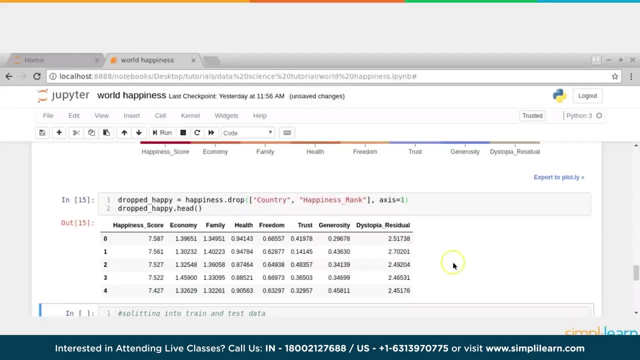 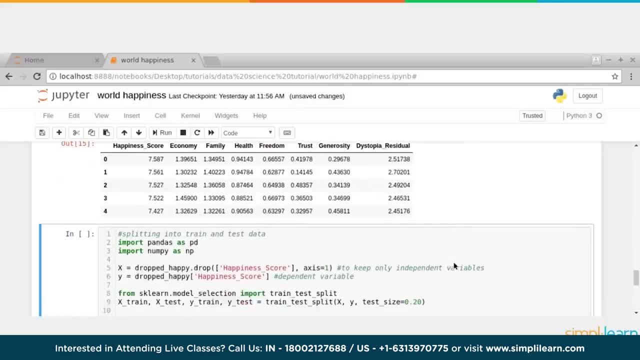 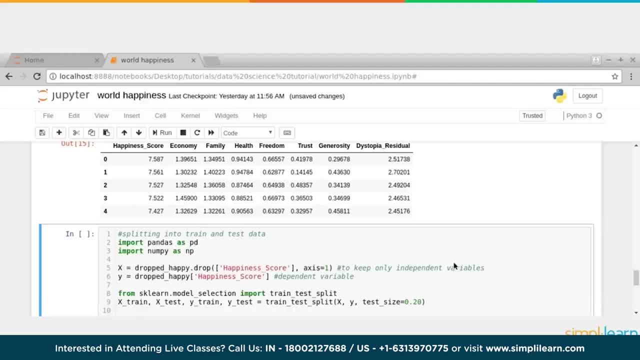 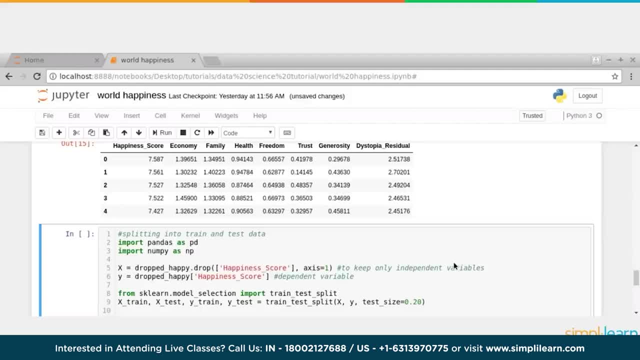 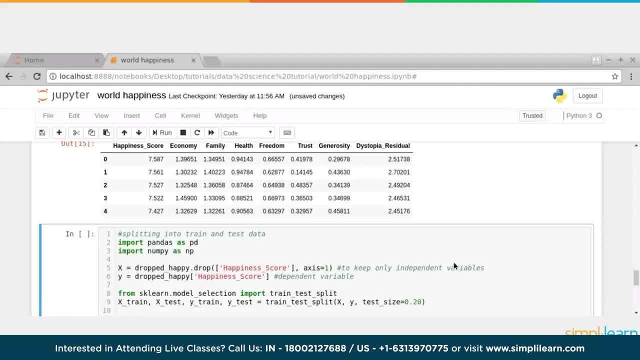 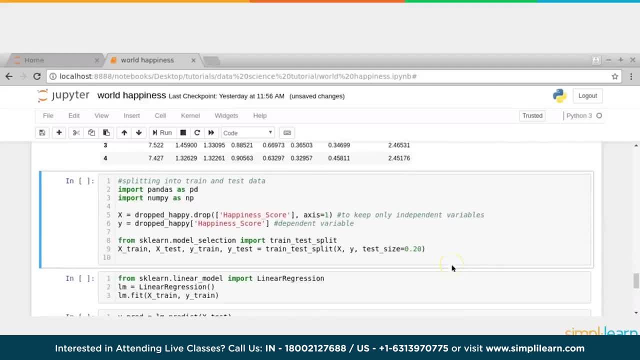 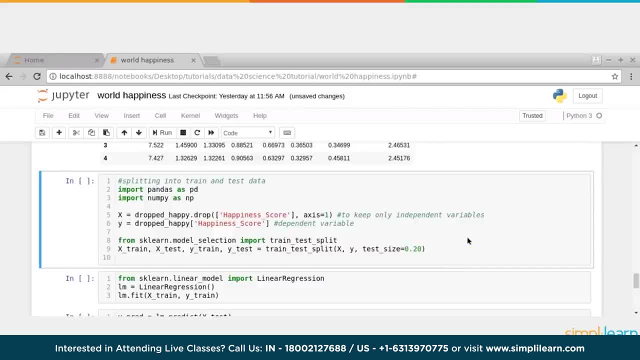 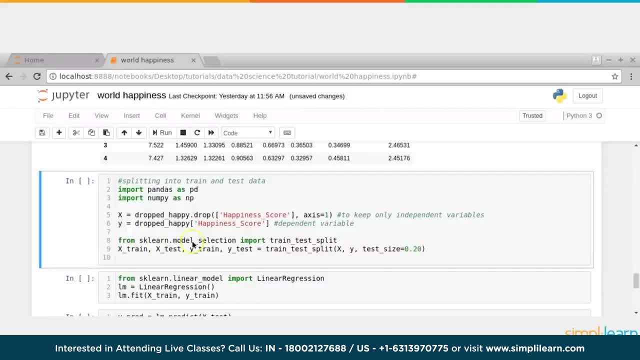 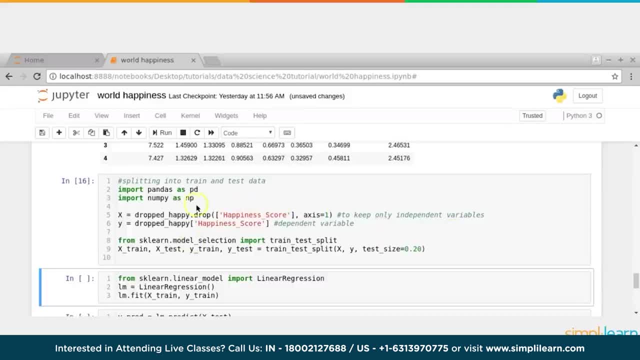 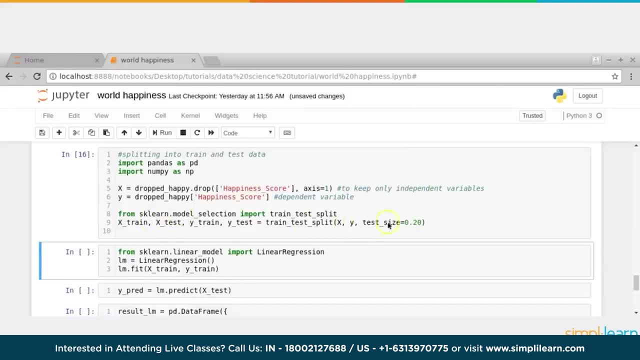 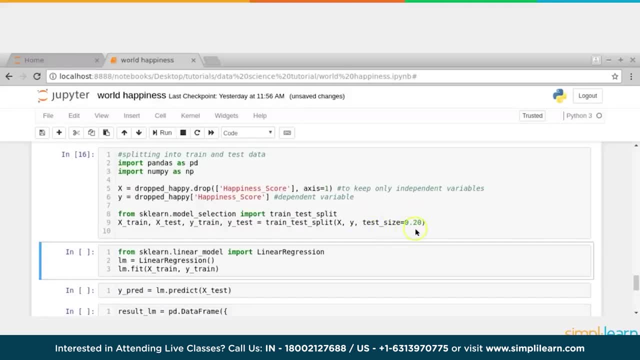 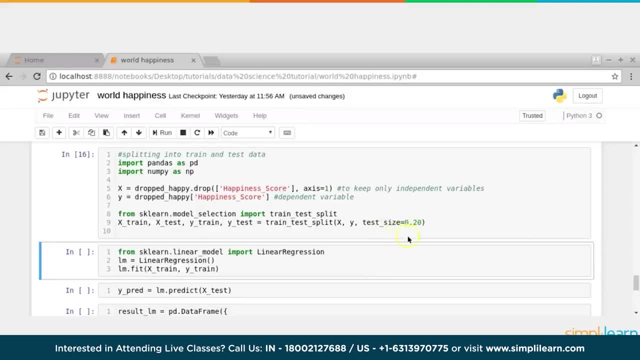 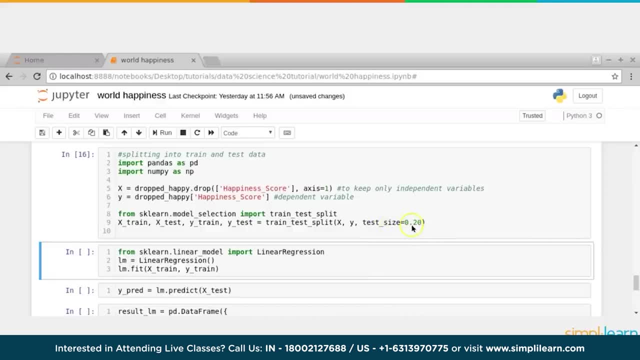 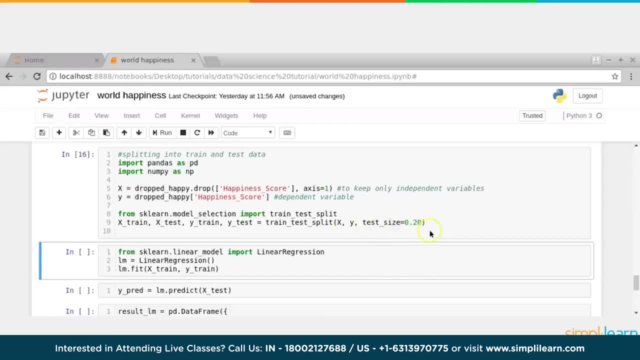 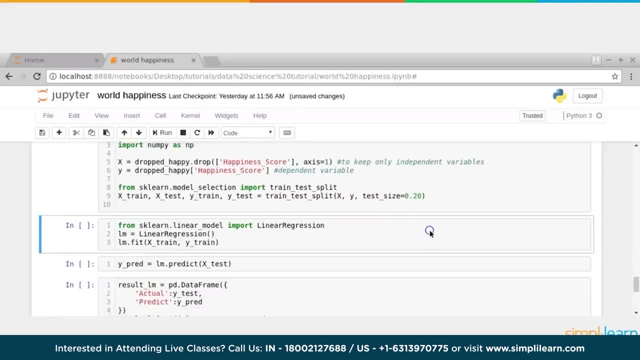 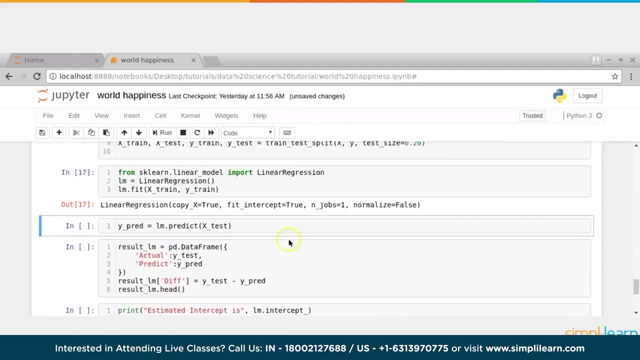 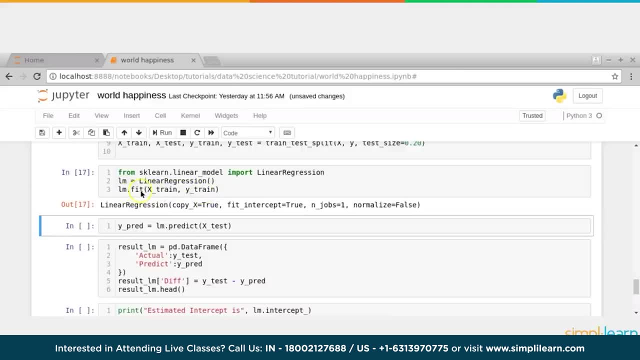 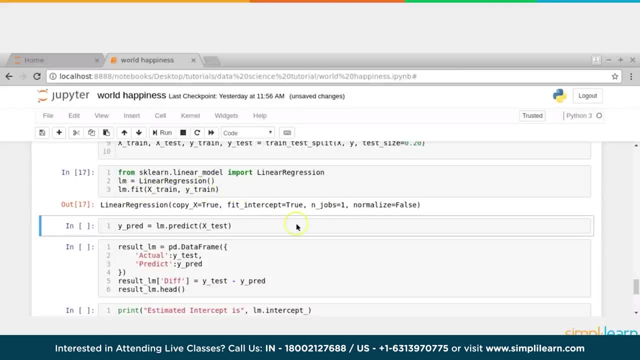 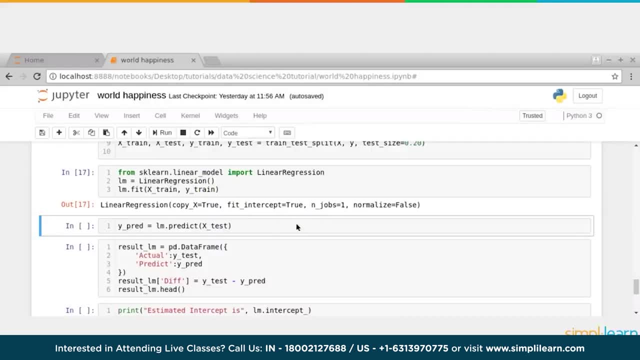 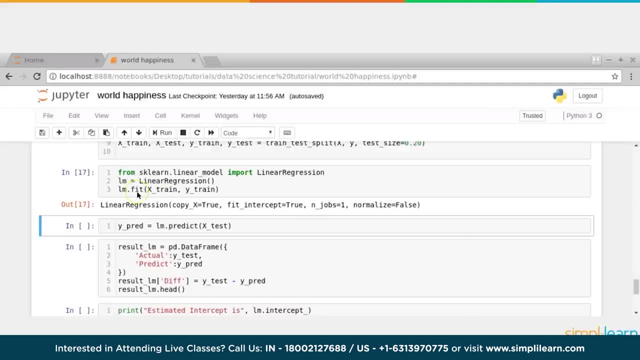 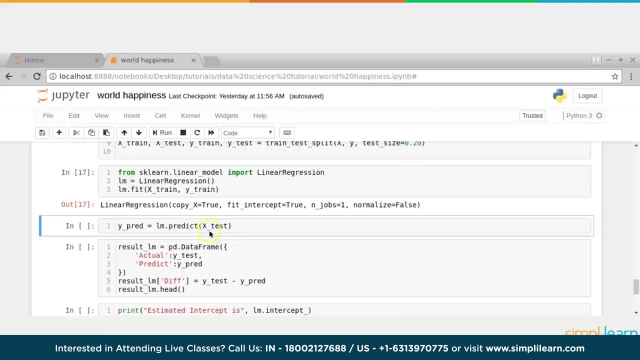 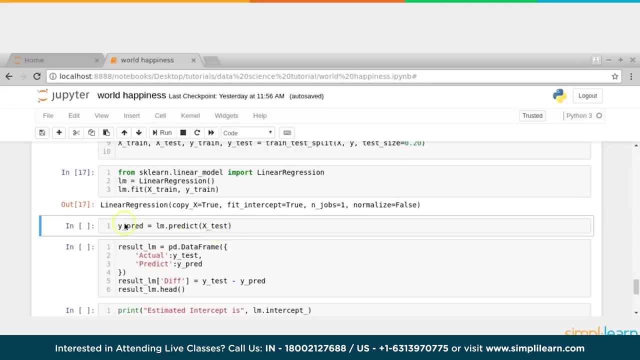 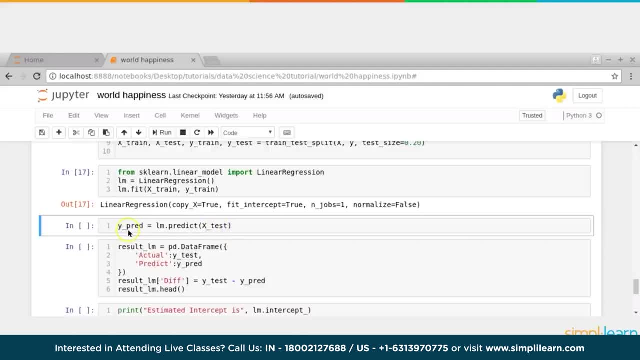 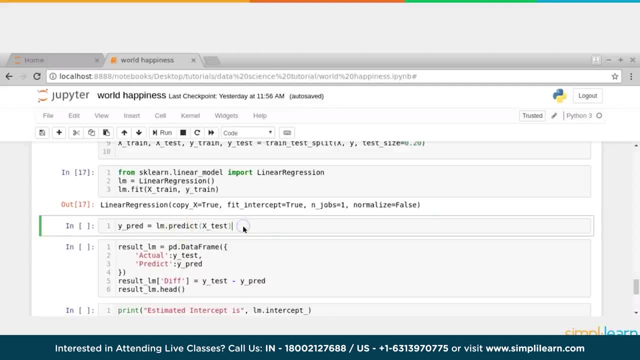 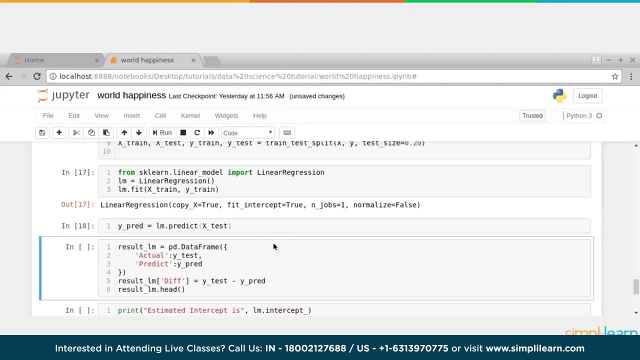 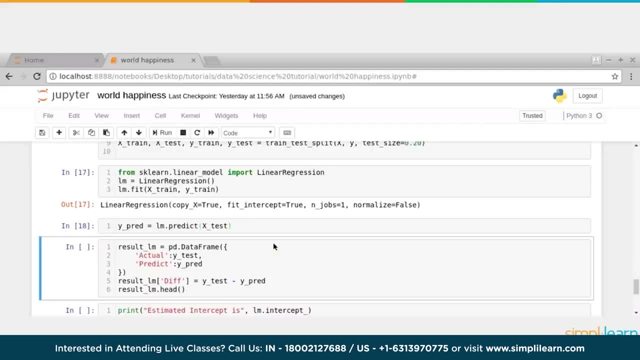 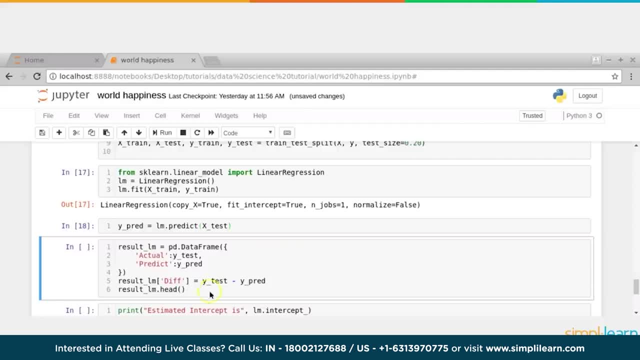 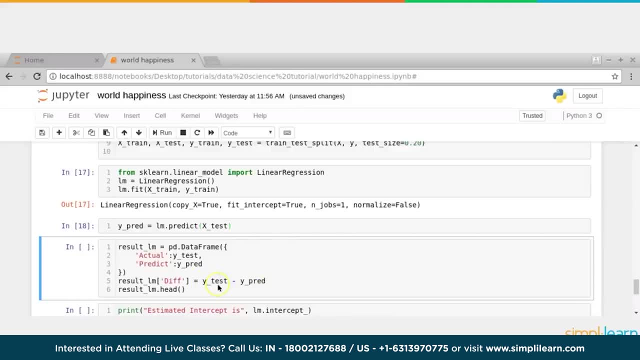 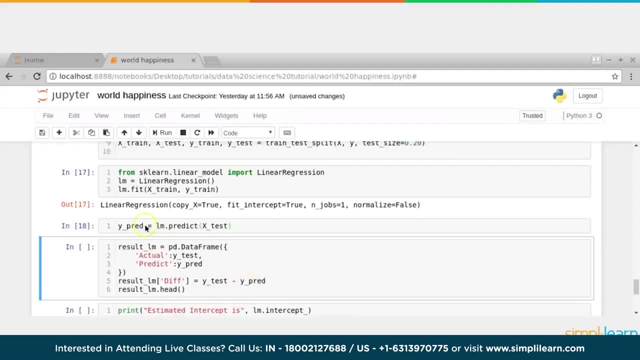 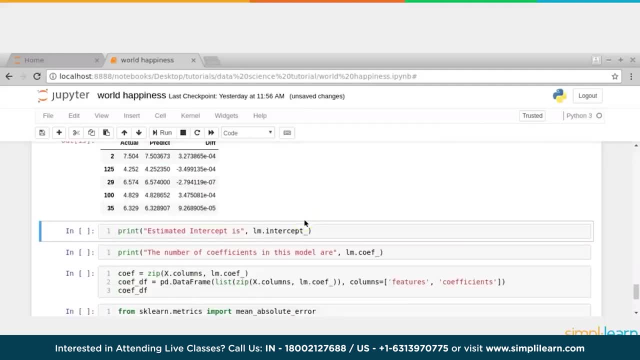 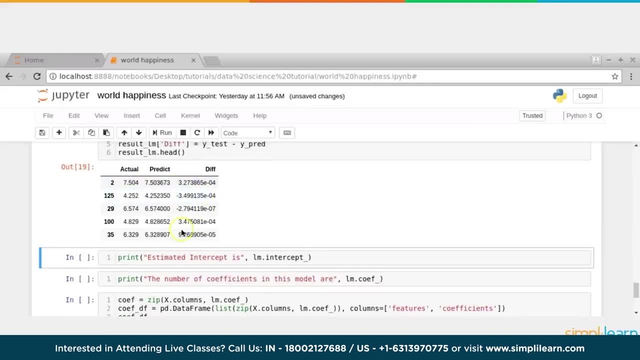 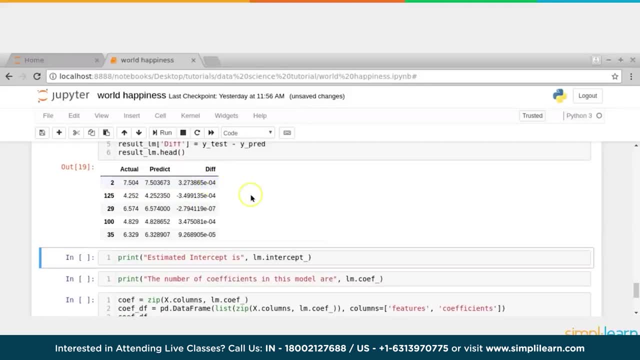 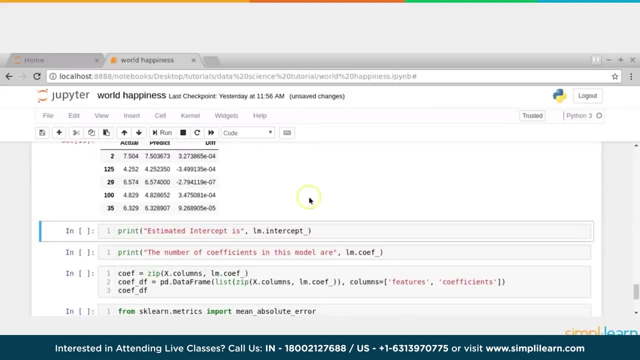 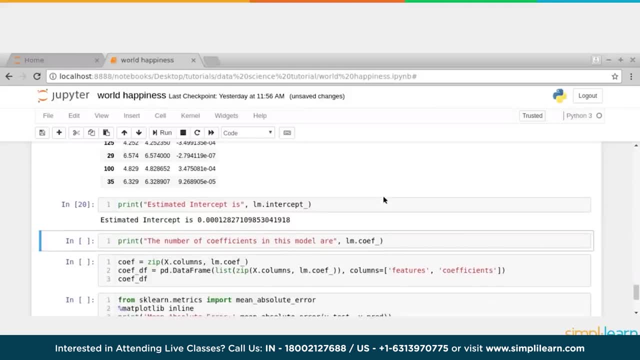 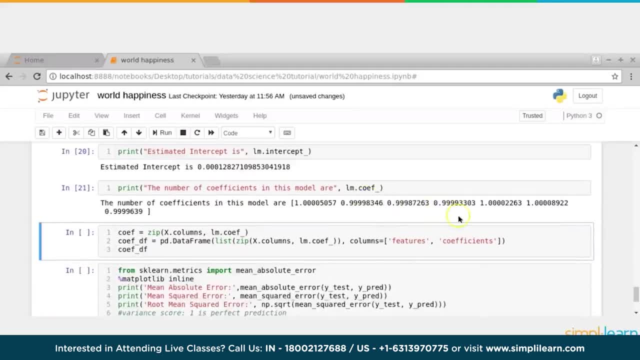 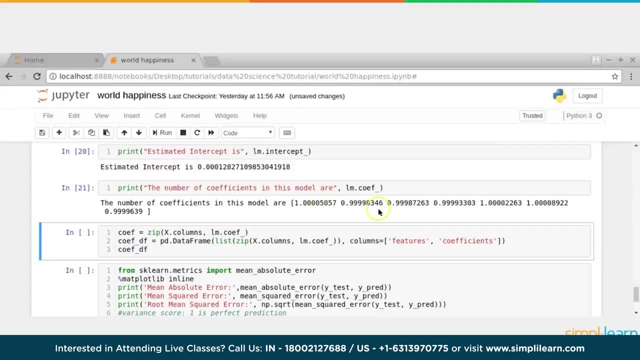 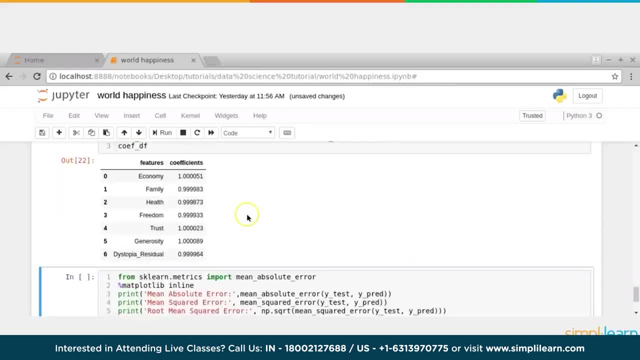 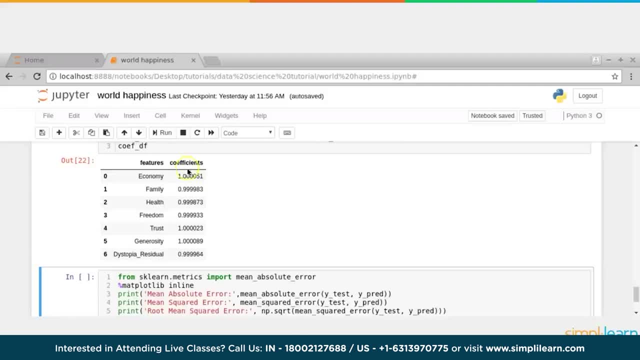 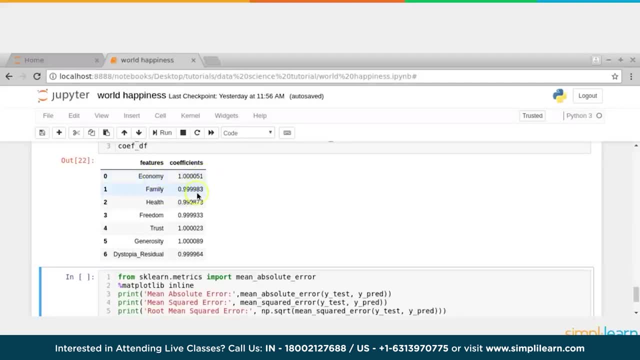 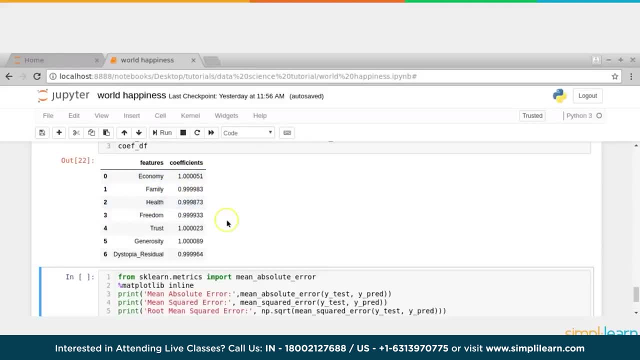 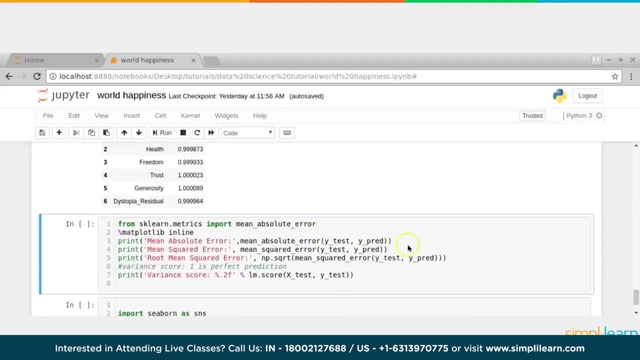 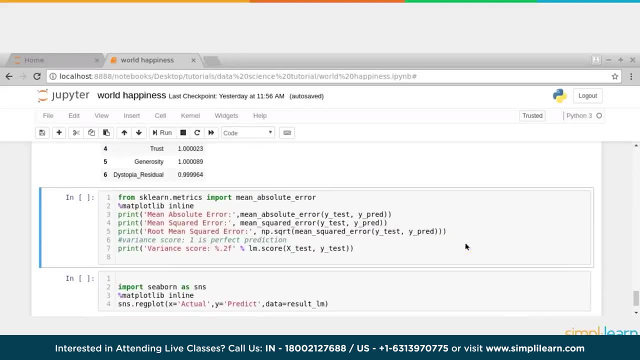 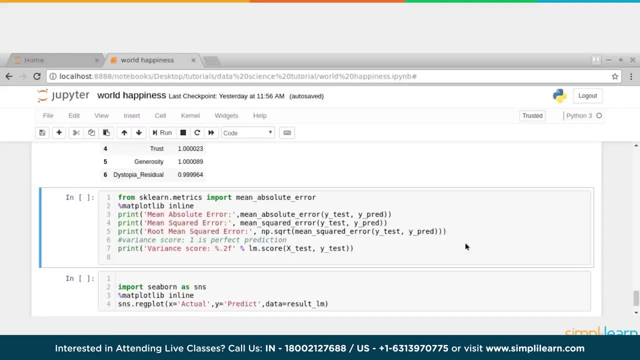 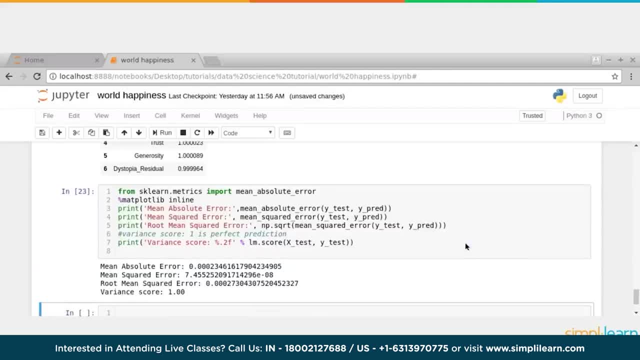 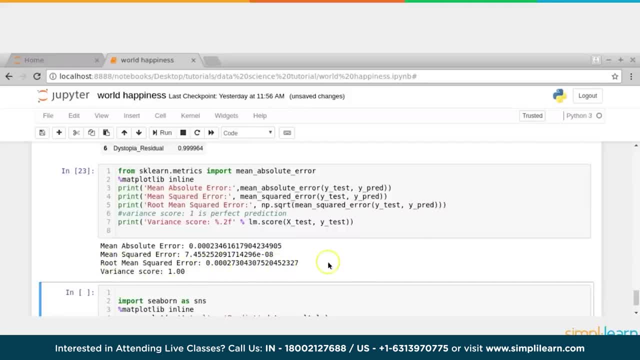 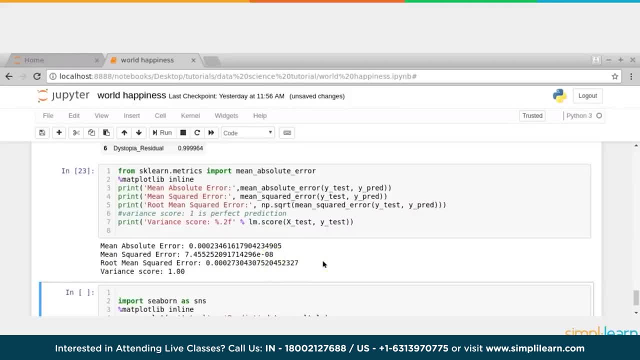 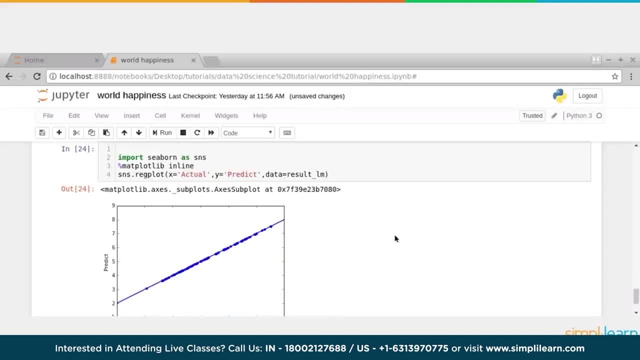 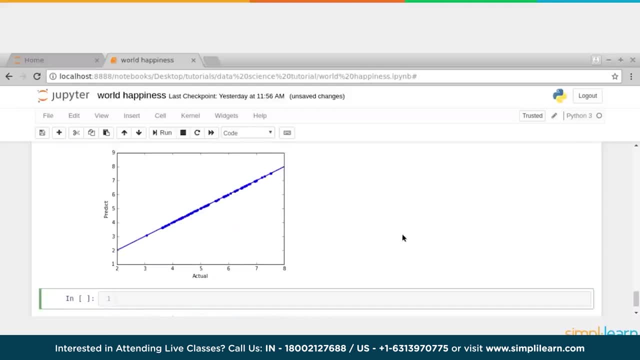 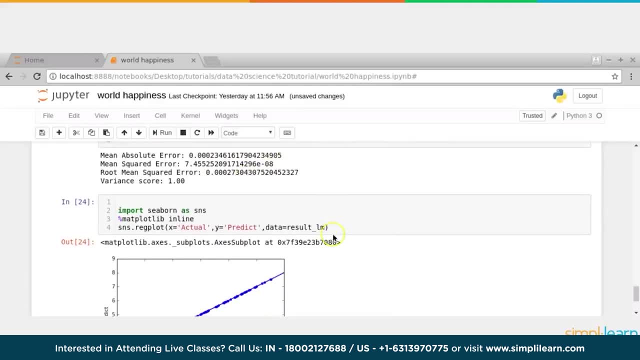 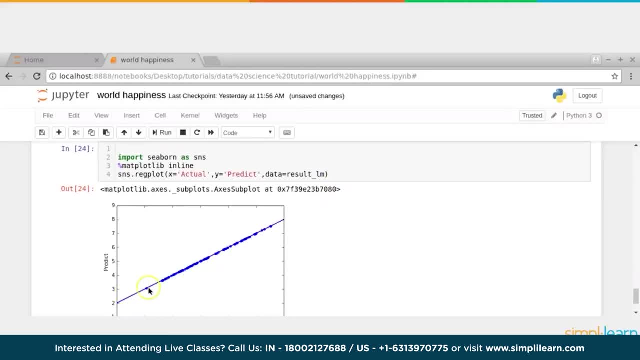 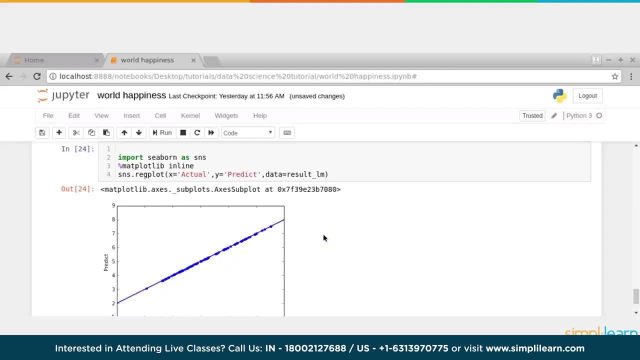 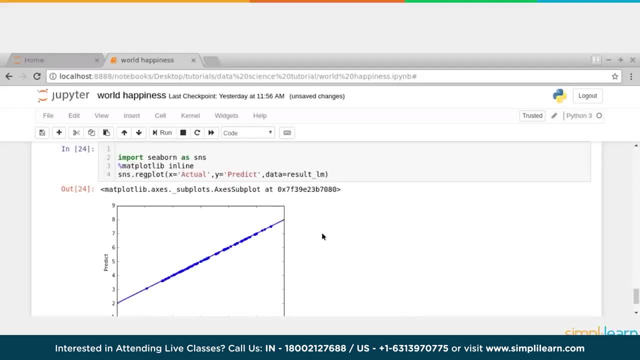 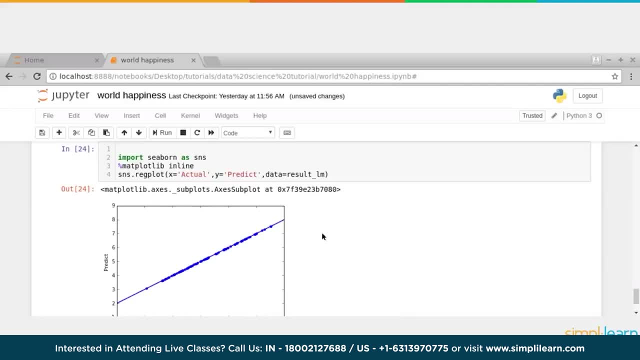 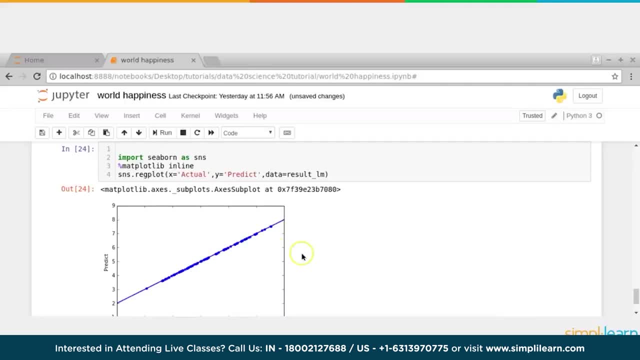 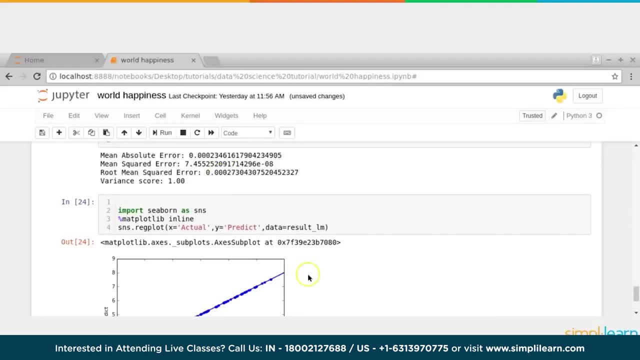 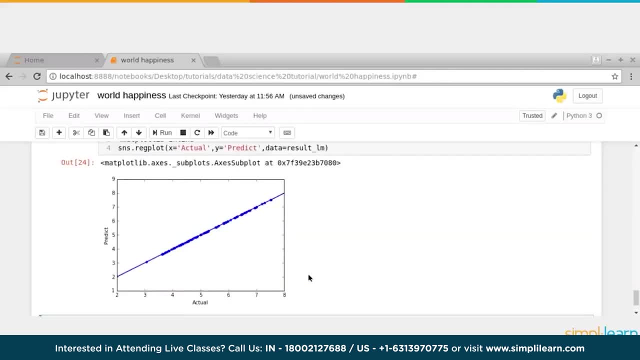 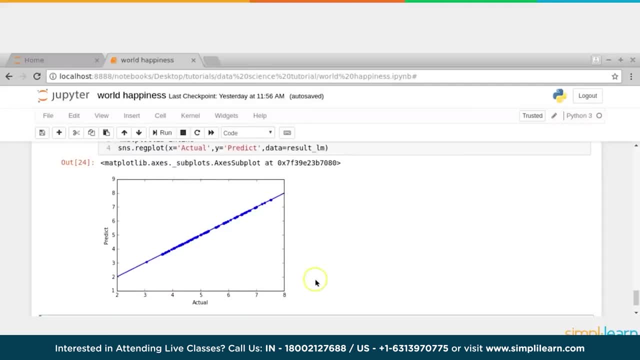 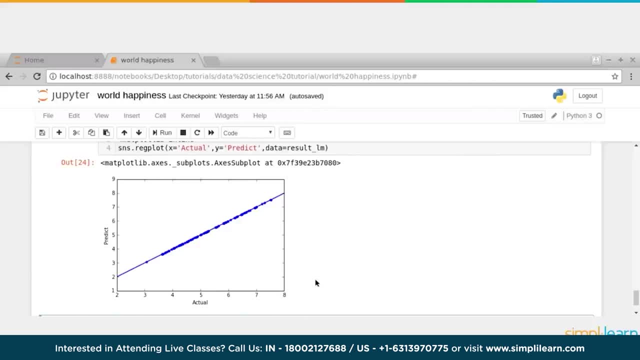 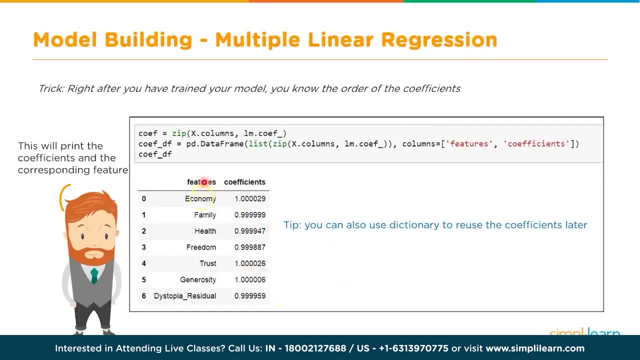 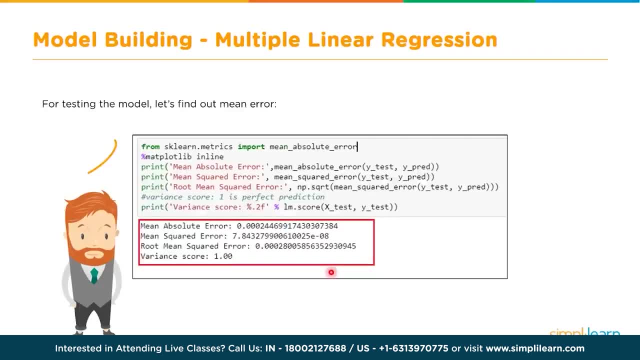 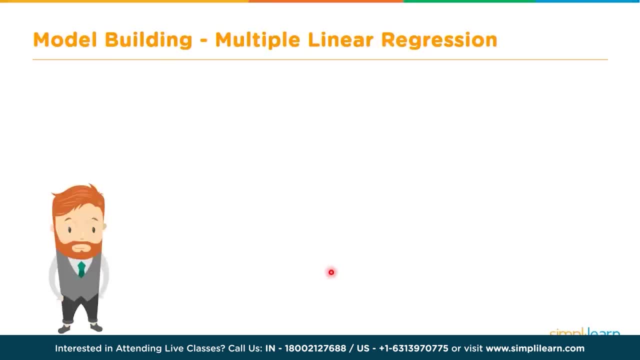 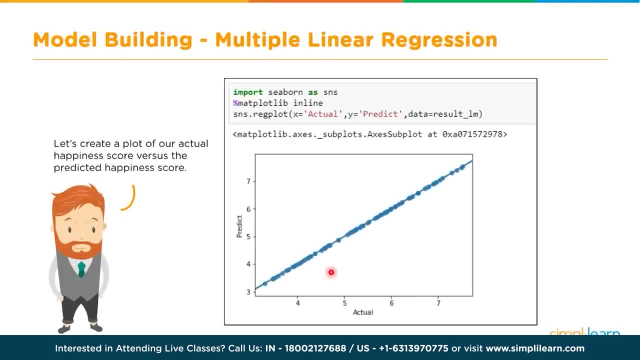 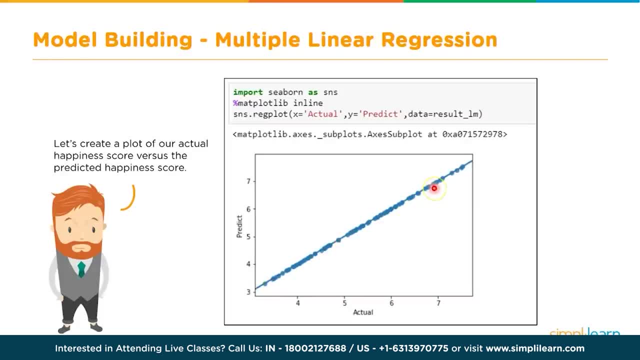 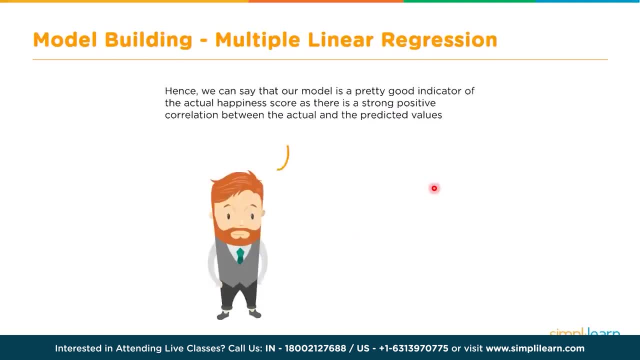 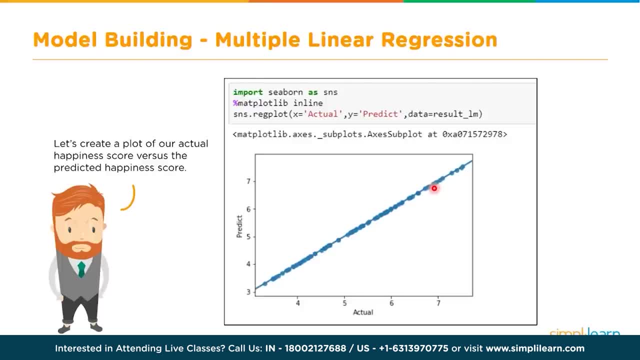 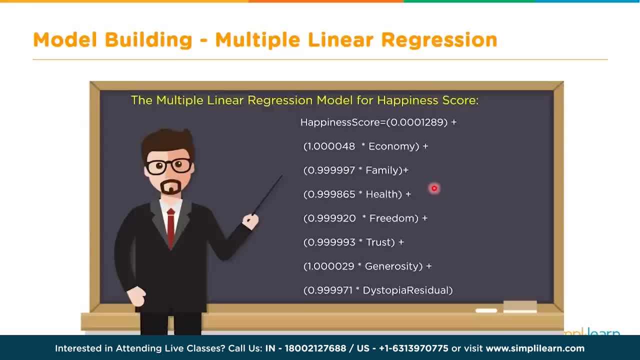 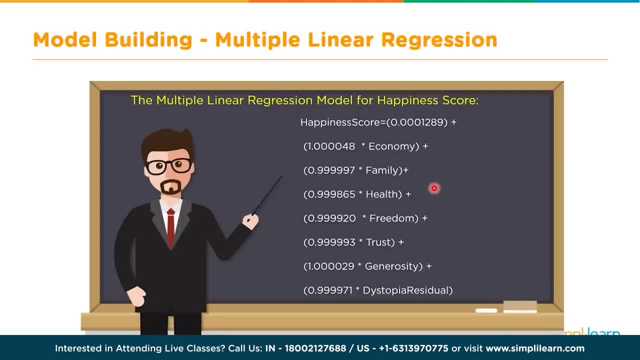 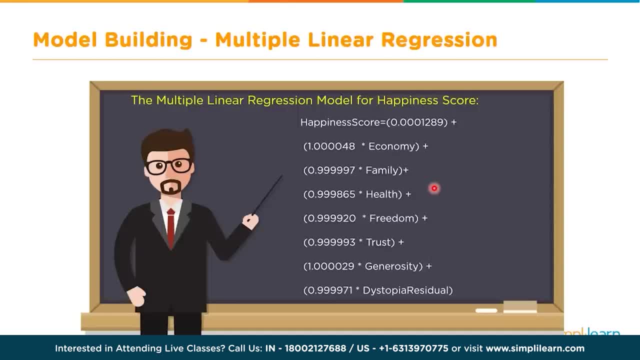 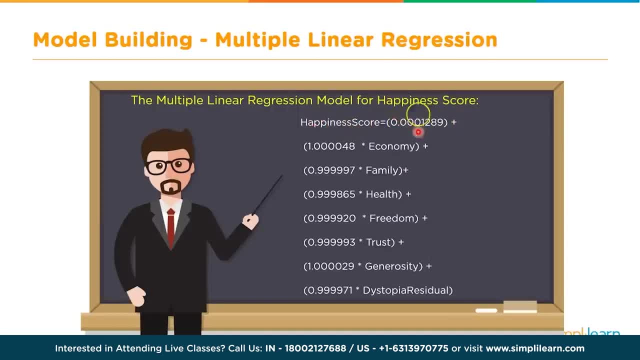 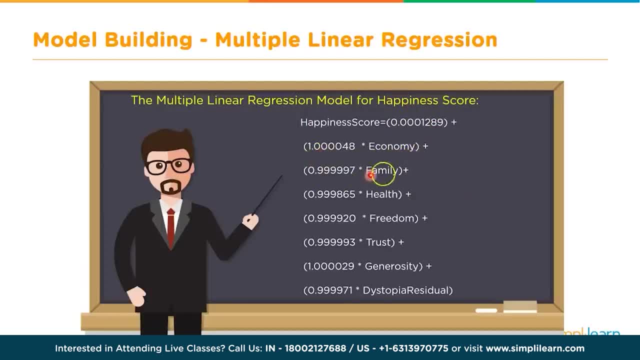 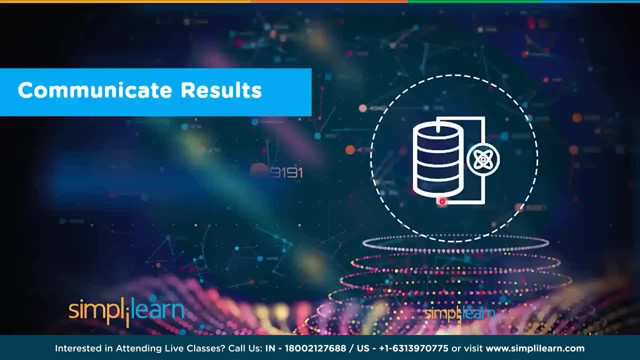 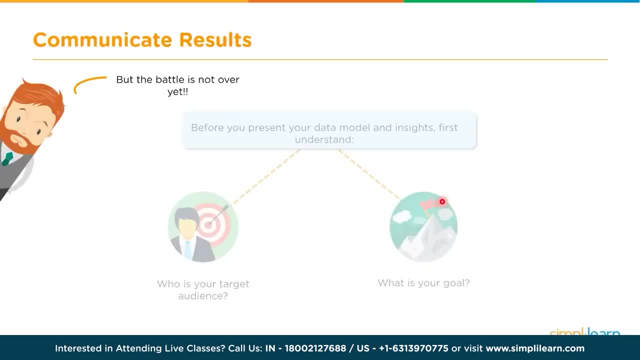 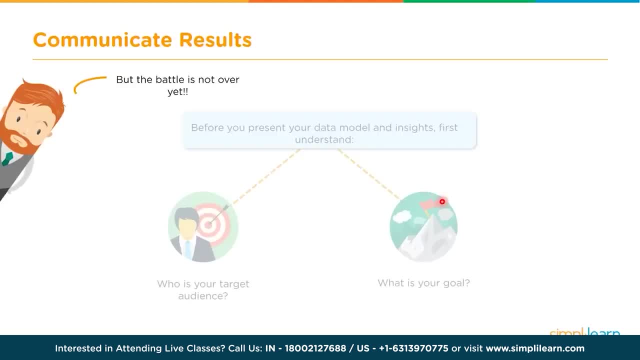 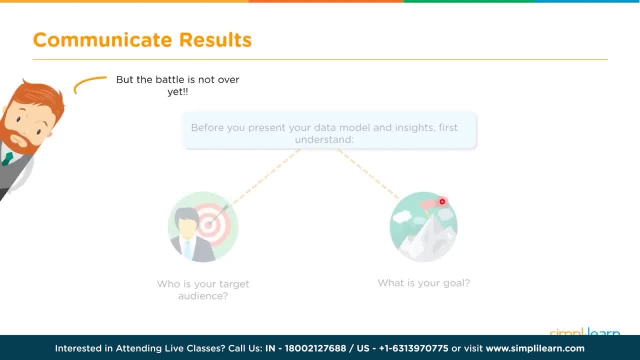 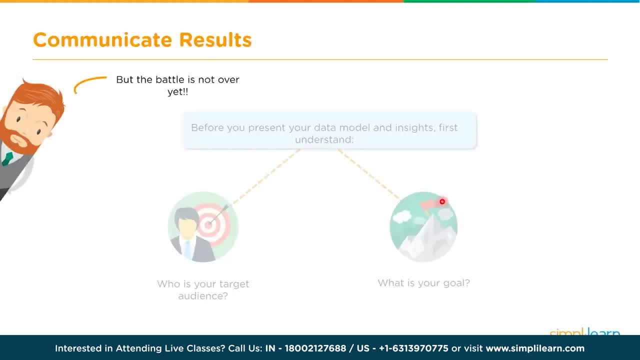 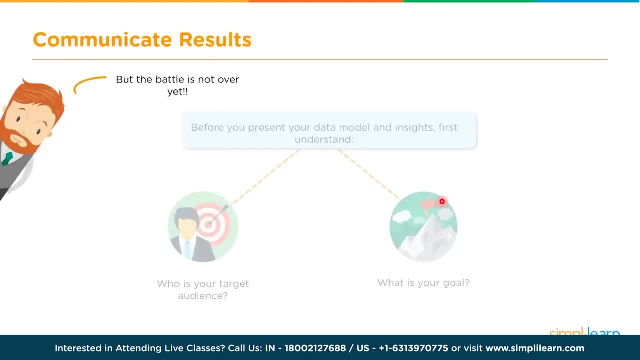 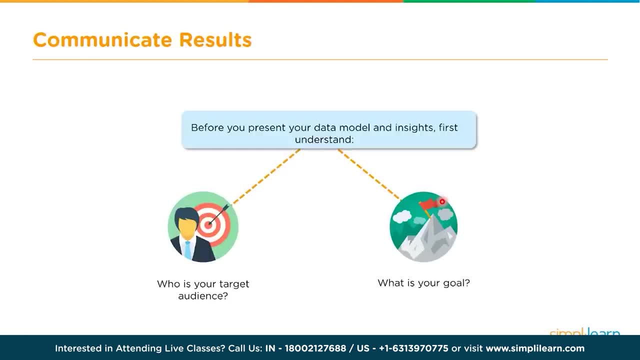 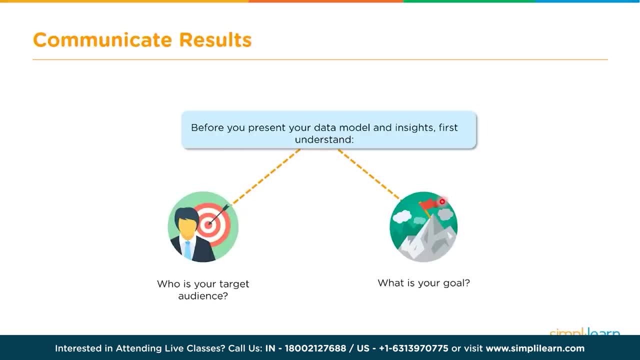 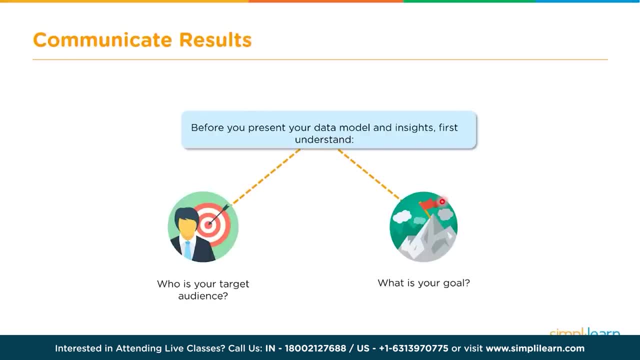 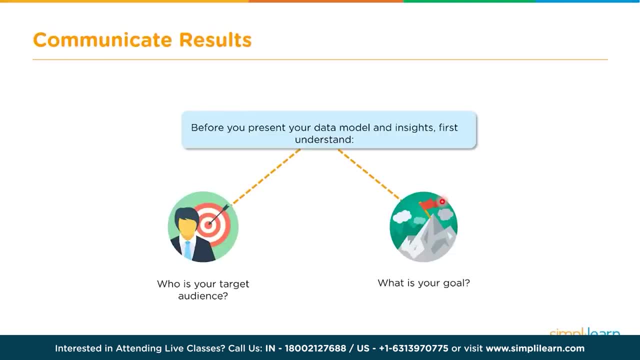 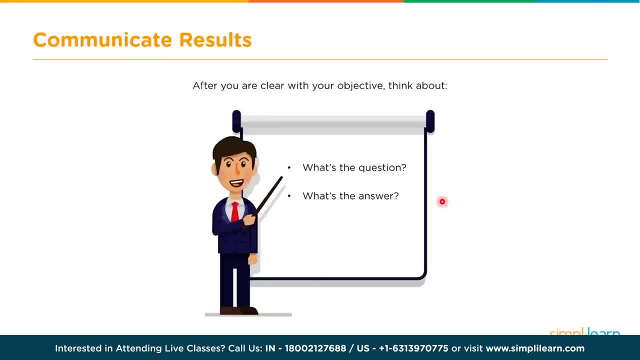 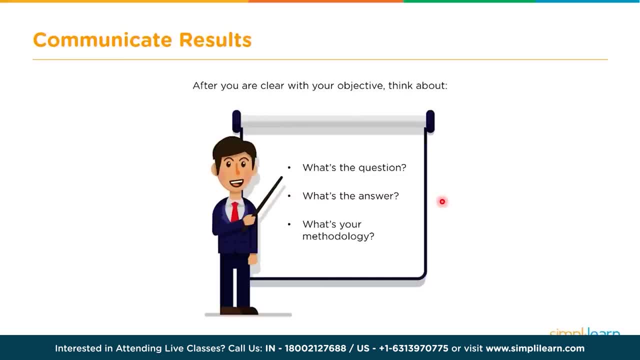 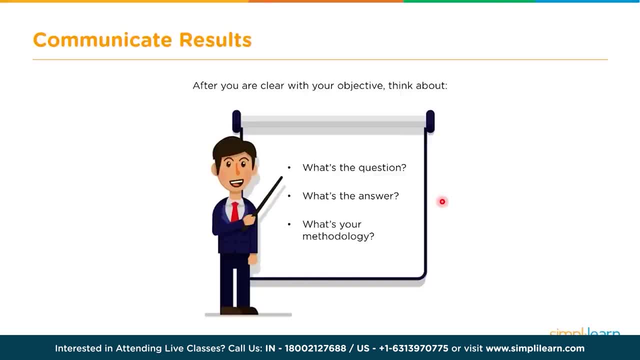 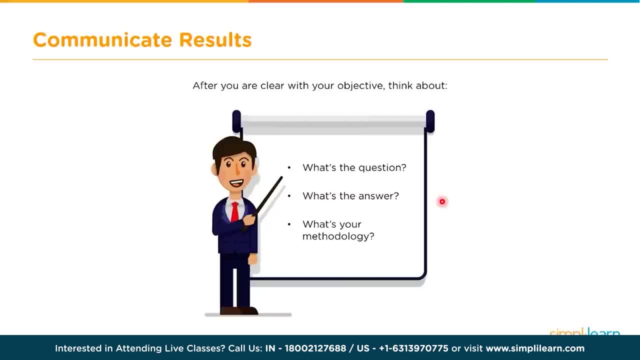 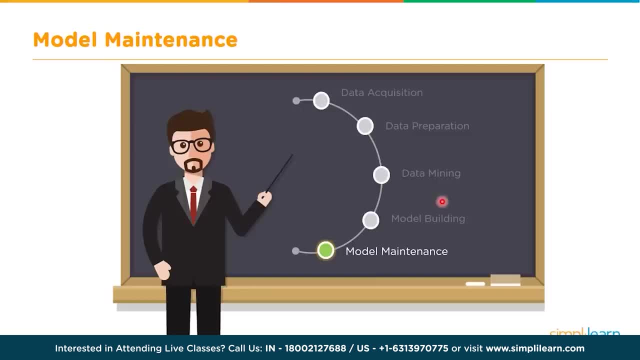 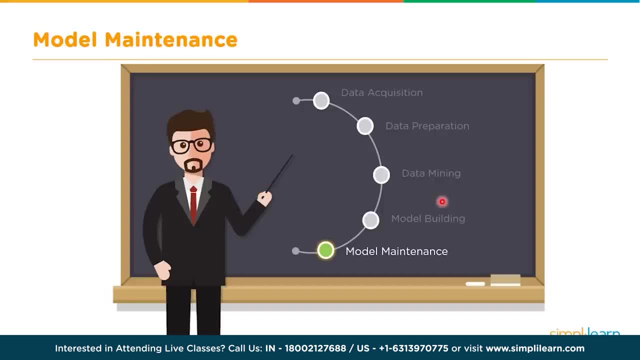 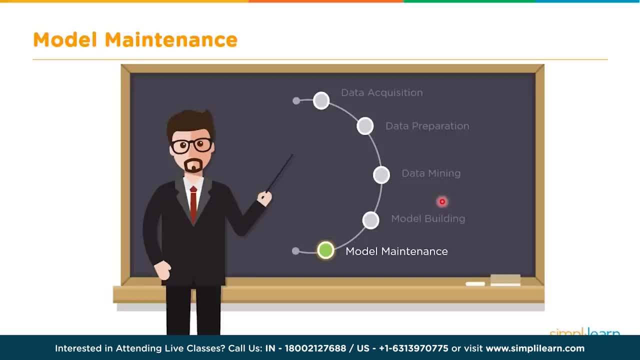 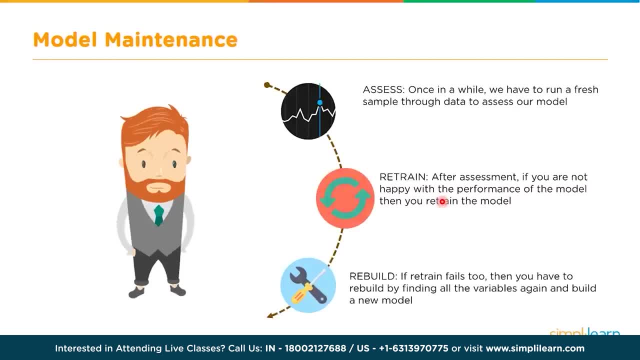 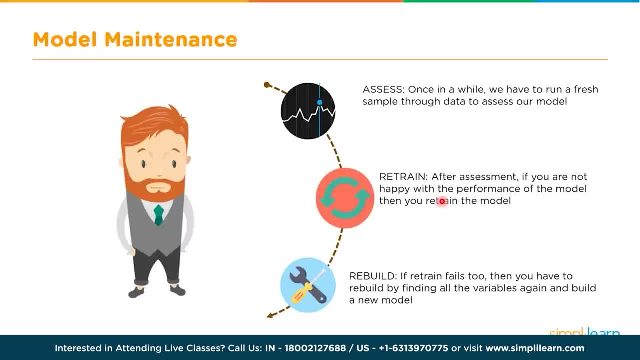 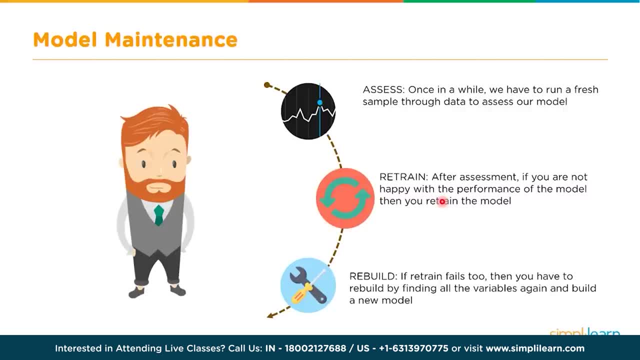 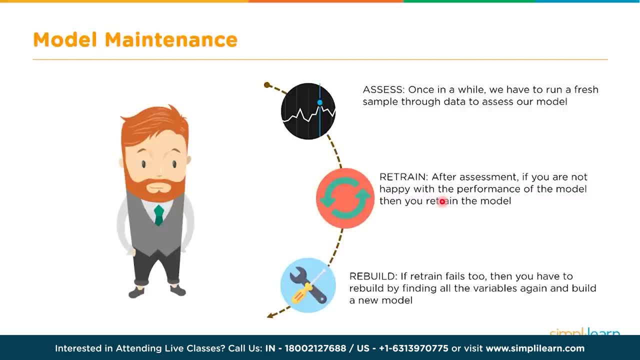 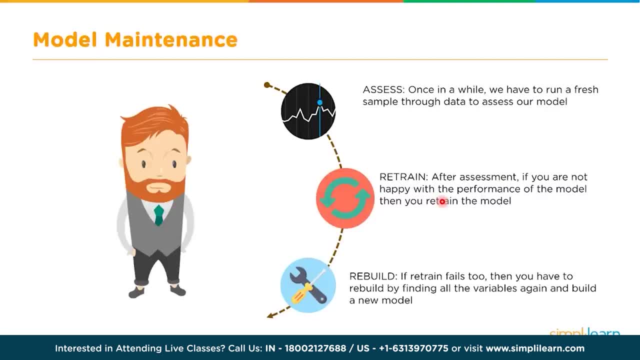 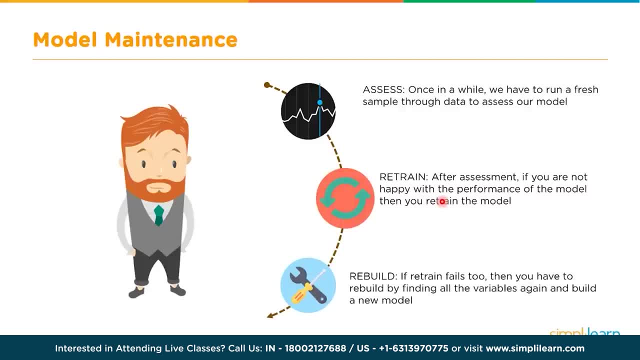 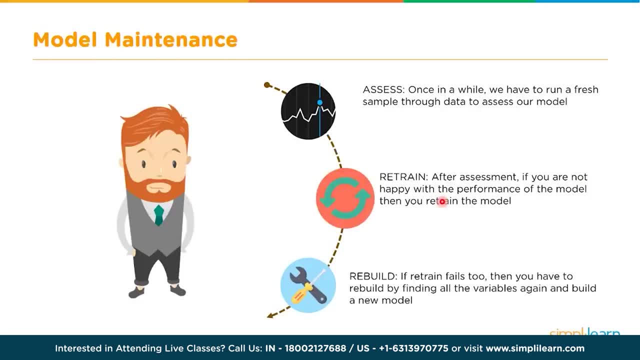 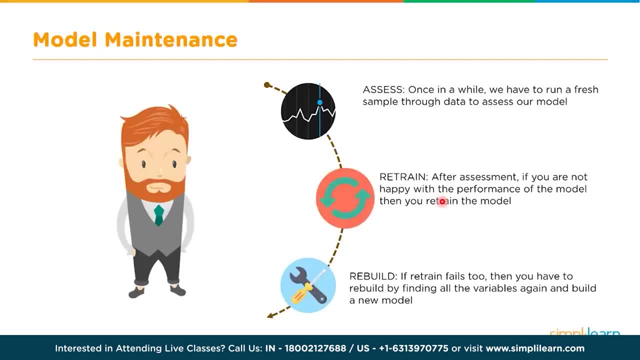 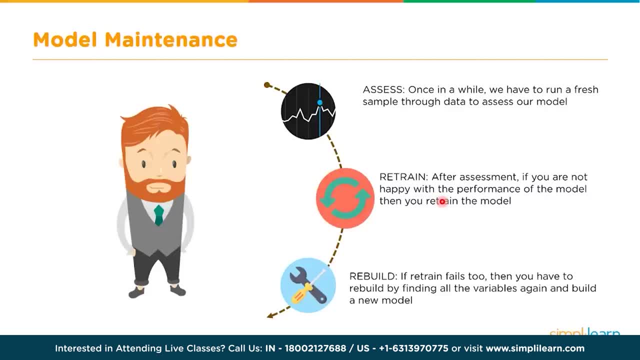 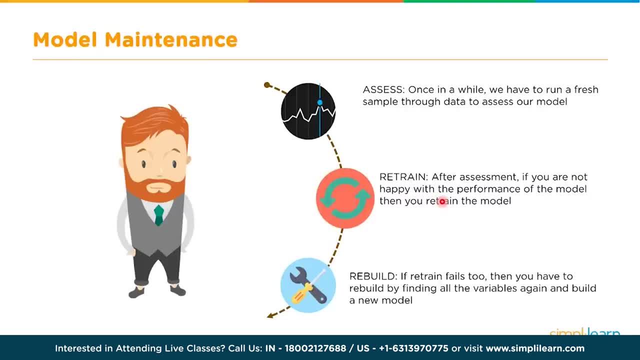 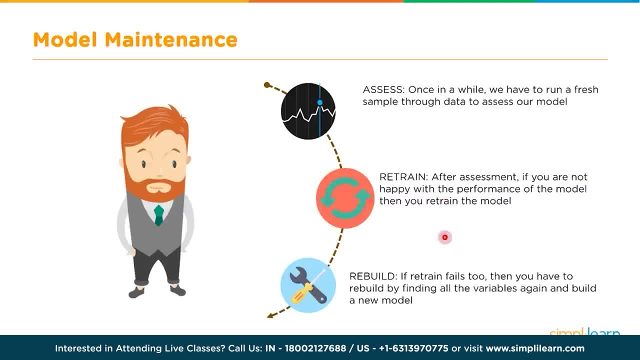 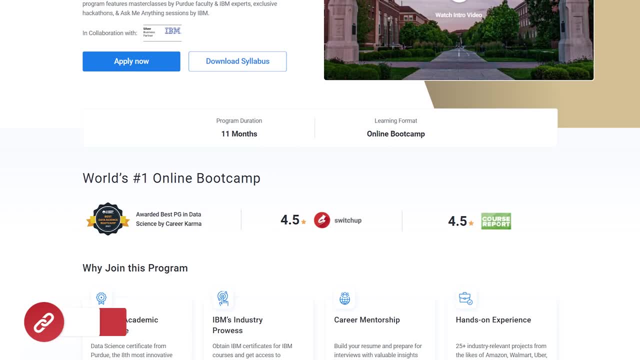 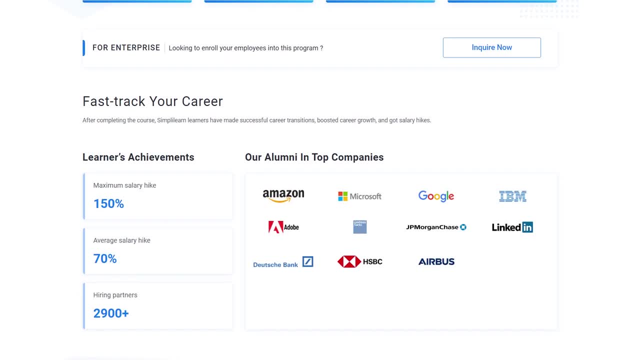 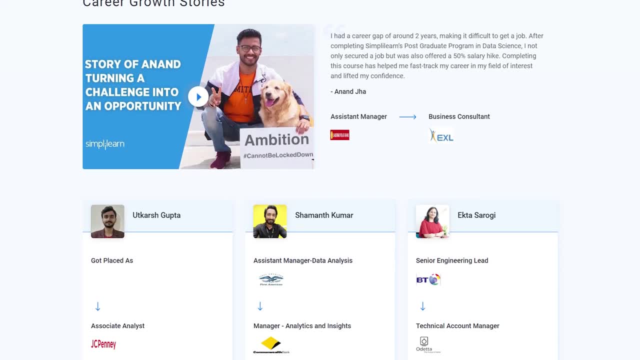 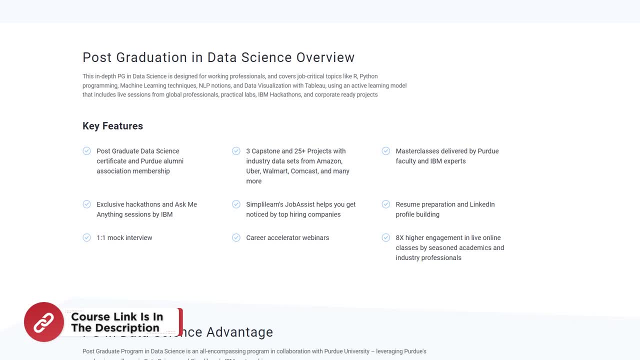 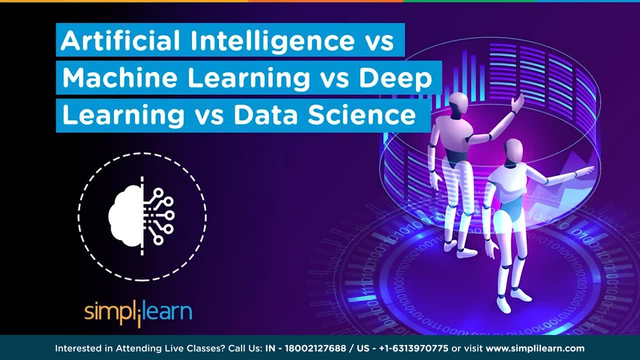 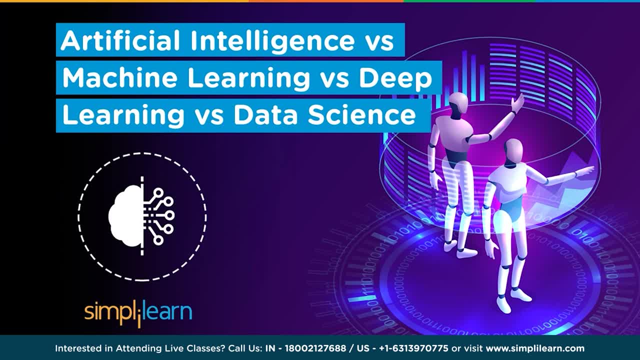 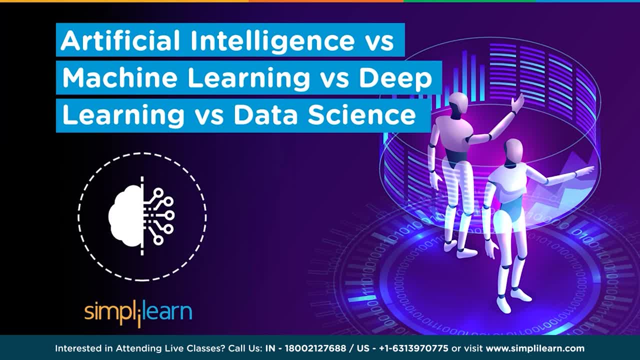 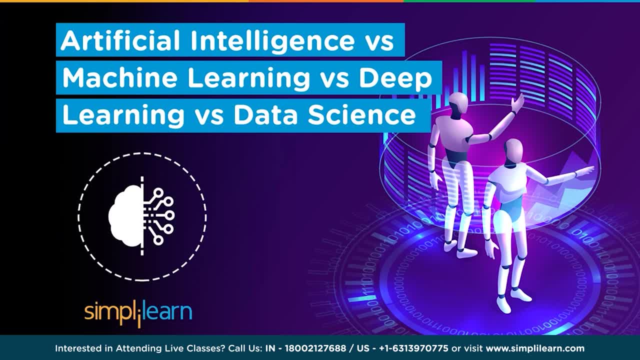 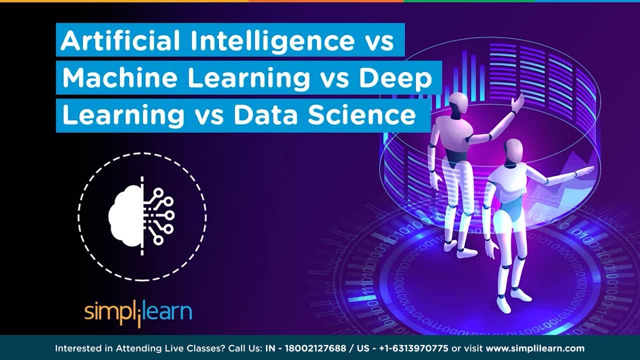 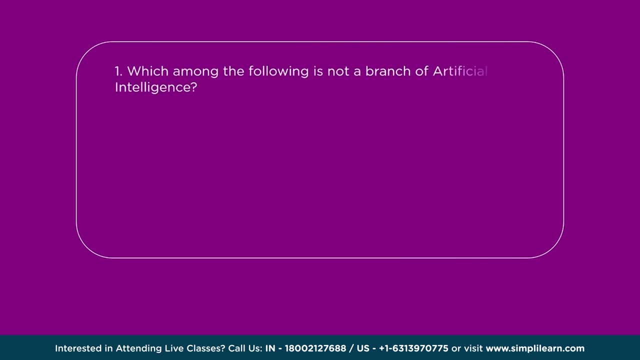 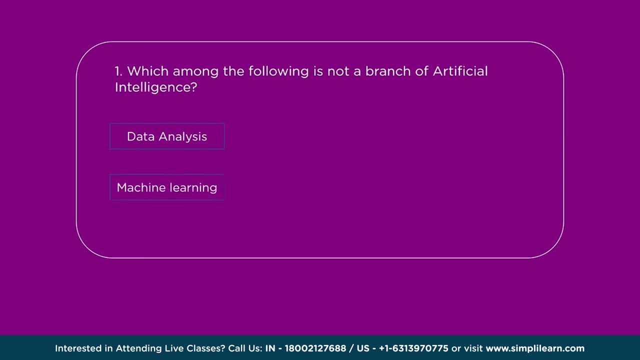 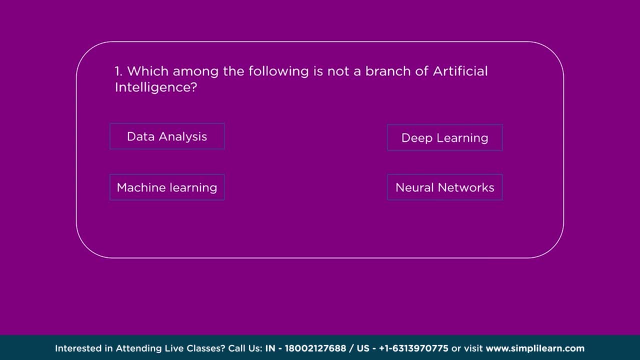 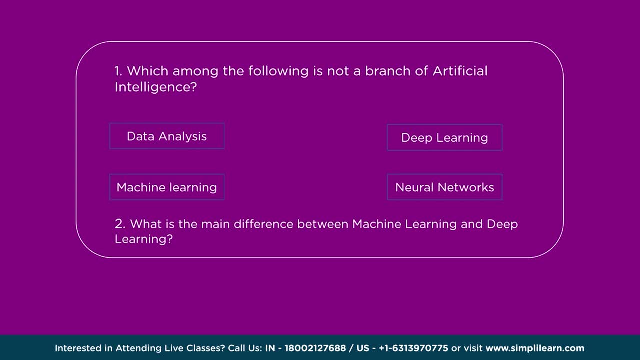 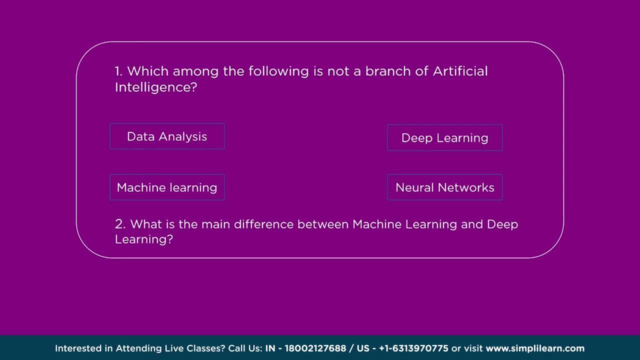 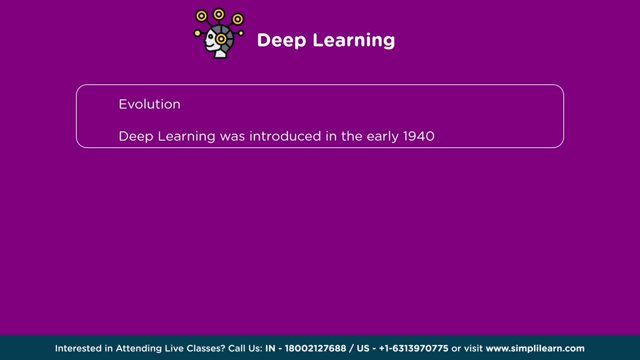 Deep learning did not develop suddenly. It developed slowly and steadily over seven decades. Many theses and discoveries were made on deep learning from the 1940s to 2000.. Thanks to companies like Facebook and Google, the term deep learning has gained popularity. 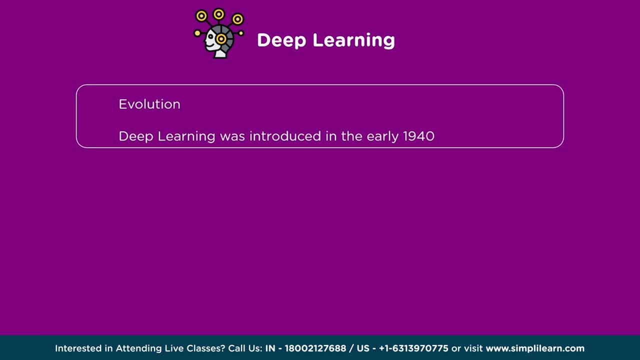 and may give the perception that it is a relatively new concept. Deep learning can be considered as a type of machine learning and artificial intelligence, Or AI, that imitates how humans gain certain types of knowledge. Deep learning includes statistics and predictive modeling. Deep learning makes processes quicker and simpler, which is advantageous to data scientists. 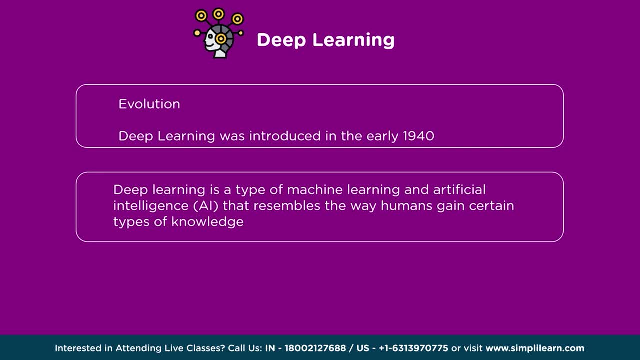 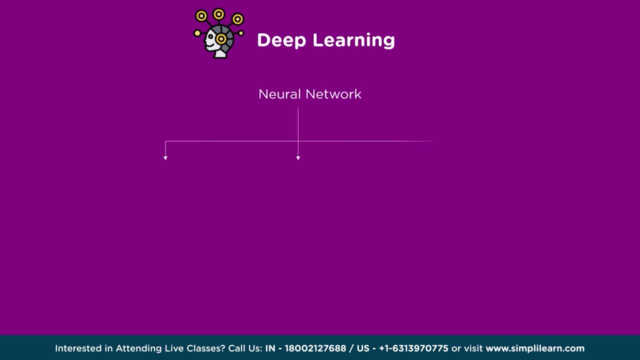 to gather, analyze and interpret massive amounts of data. Having the fundamentals discussed, let's move into the different types of deep learning. Neural networks are the main component of deep learning, But neural networks comprise three main types. They contain artificial neural networks, or ANN, convolution neural networks, or CNN. 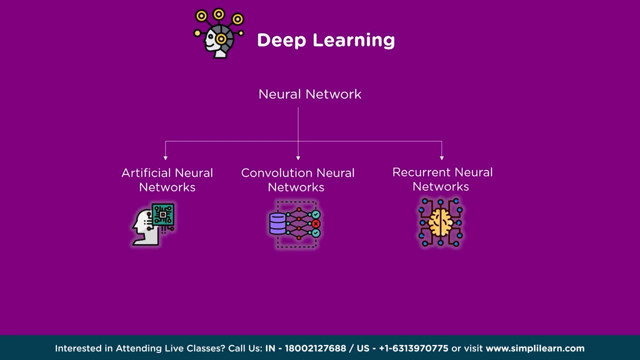 and recurrent neural networks, or RNN. Artificial neural networks are inspired biologically by the animal brain. Convolutional neural networks surpass other neural networks when given inputs such as images, voice or audio. It analyzes images by processing data. Recurrent neural networks uses sequential data or series of data. 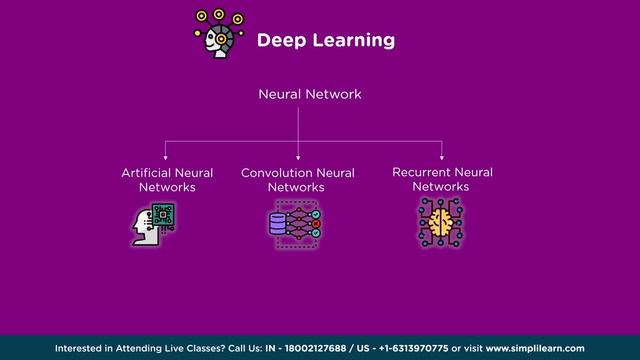 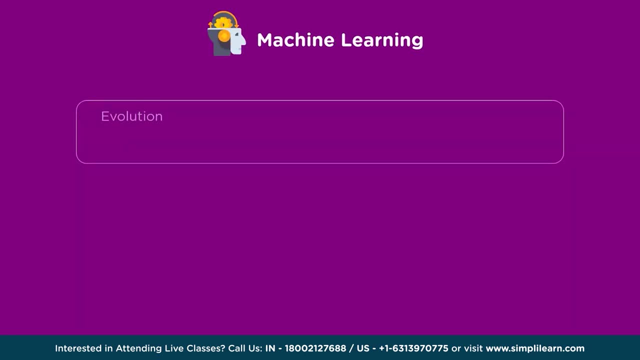 Convolutional neural networks and recurrent neural networks are used in natural language processes, speech recognition, image recognition and many more Machine Learning. The evolution of ML started with the mathematical modeling of neural networks that served as the basis for the invention of machine learning. 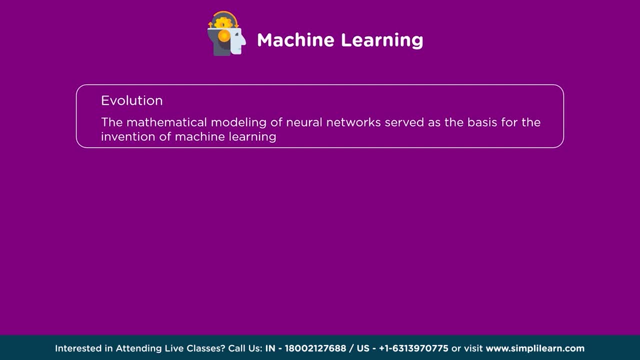 In 1943, neuroscientist Warren McCulloch and logician Walter Pitts attempted to quantitatively map out how humans make decisions and carry out thinking processes. Therefore, the term machine learning is not new. Machine learning is a branch of artificial intelligence and computer science that uses 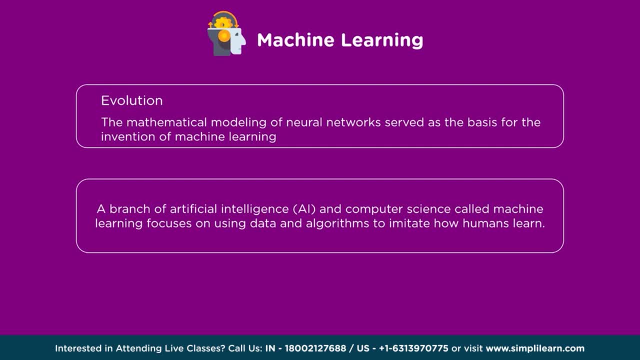 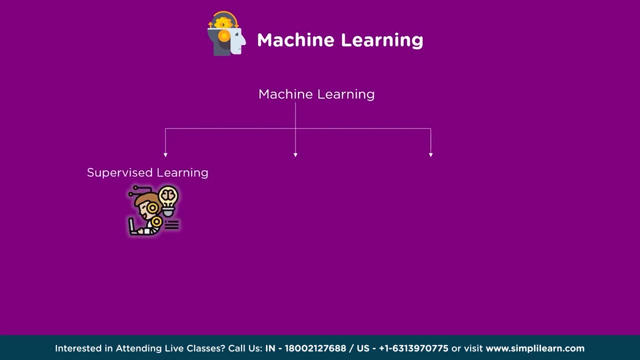 data and algorithms to imitate how humans learn, gradually increasing the system's accuracy. There are three types of machine learning, which include supervised learning. What is supervised learning? Well, here machines are trained using labeled data. Machines predict output based on this data. 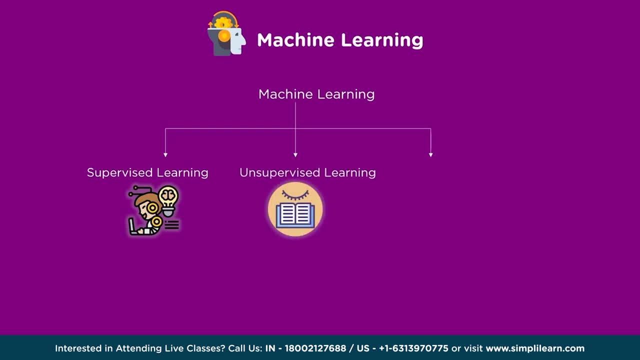 Now coming to unsupervised learning. What is unsupervised learning? Models are not supervised using a training data set. It is comparable to the learning process that occurs in the human brain while learning something new. And the third type of machine learning is reinforcement learning. 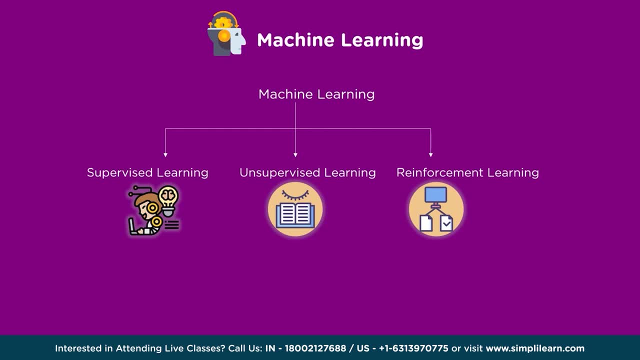 Here the agent learns from feedback. It learns to behave in a given environment based on actions and the result of the action. This feature can be observed in robotics Coming to the evolution of AI. The potential of artificial intelligence wasn't explored until the 1950s. 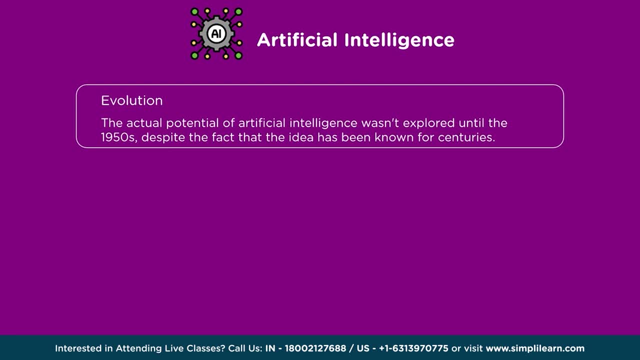 So the idea has been known for centuries. The term artificial intelligence has been around for a decade. Still, it wasn't until British polymath Alan Turing posed the question of why machines couldn't use knowledge like humans do to solve problems and make decisions. 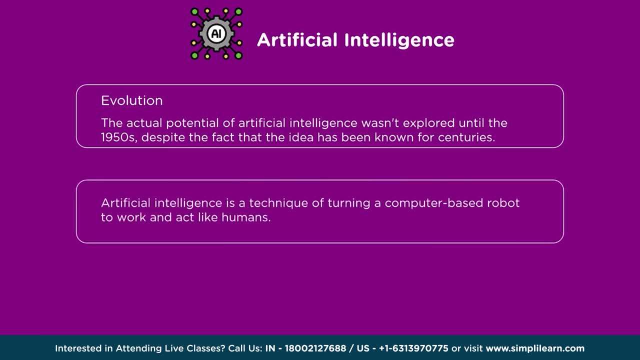 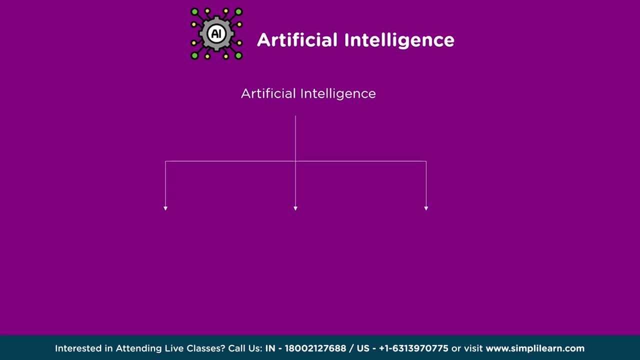 We can define artificial intelligence as a technique of turning a computer-based robot to work and act like humans. Now let's have a glance at the types of artificial intelligence: Weak AI- Weak AI: It performs only specific tasks, like Apple's Siri, Google Assistant and Amazon's Alexa. 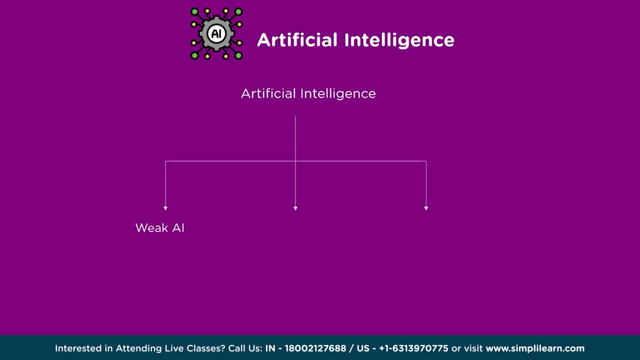 You might have used all of these technologies, but the types I am mentioning after this are under experiment. General AI can also be addressed as artificial general intelligence. It is equivalent to human intelligence. Hence, an AGI system is capable of carrying out any task that a human can. 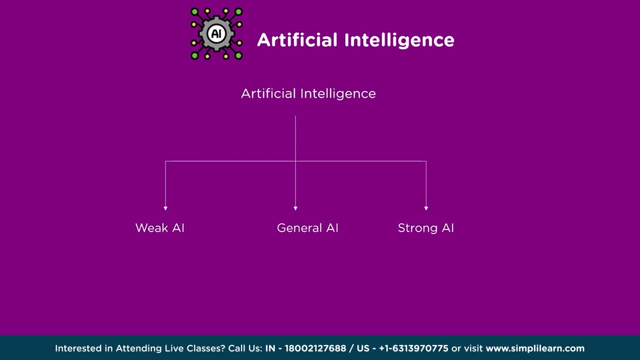 Strong AI aspires to build machines that are indistinguishable from the human mind. Both general and strong AI are hypothetical right now. Rigorous research is going on on this matter. There are many branches of artificial intelligence, which include machine learning, deep learning. 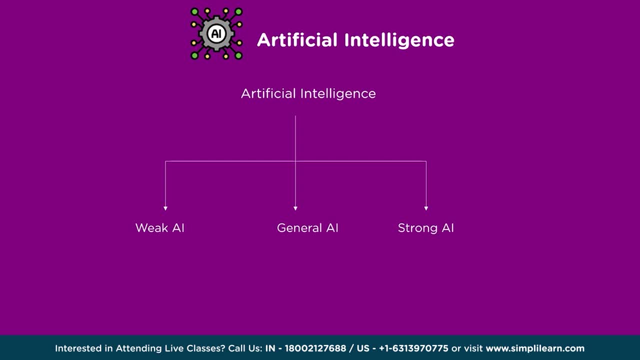 natural language processing, robotics, expert systems and fuzzy logic. Therefore, the correct answer for which is not a branch of artificial intelligence, is option A: data analysis. Now that we have covered deep learning, machine learning and artificial intelligence, we can move on to the final topic: data science. 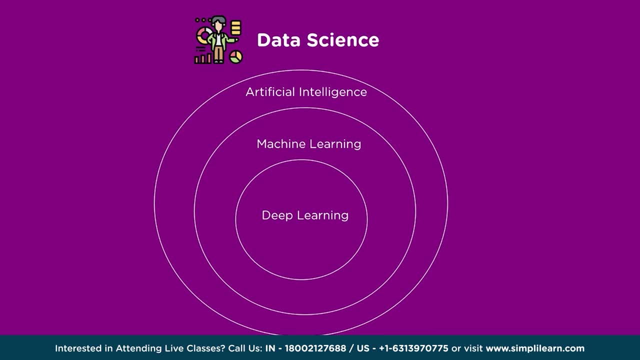 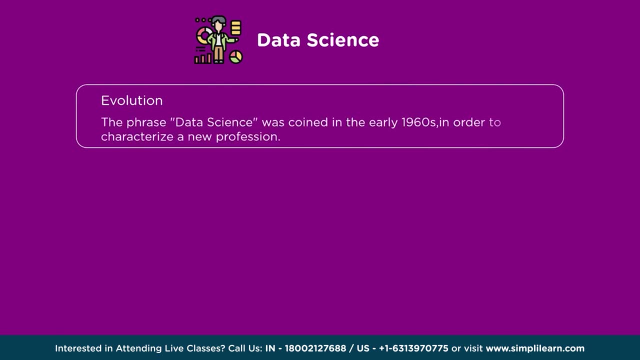 Concepts like deep learning, machine learning and artificial intelligence can be considered a subset of data science. Let us cover the evolution of data science. The phrase data science was coined in the early 1960s to characterize a new profession that would enable the comprehension and analysis of the massive volumes of data being gathered. 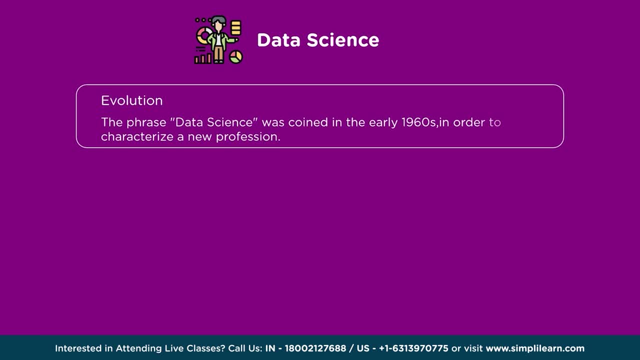 at the time. Since its beginnings, data science has expanded to incorporate ideas and methods from other fields, including artificial intelligence, machine learning, deep learning and so forth. Data science can be defined as the domain of study that handles vast volumes of data. 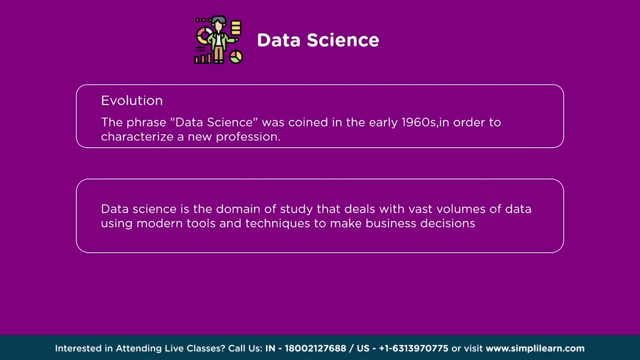 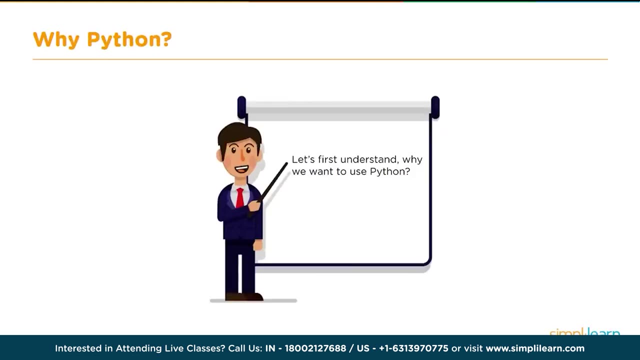 using modern tools and techniques to find unseen patterns, derive meaningful information and make business decisions. Therefore, data science comprises machine learning, artificial intelligence and deep learning. Now let's talk about Python. For doing data science, we need some kind of a programming language. 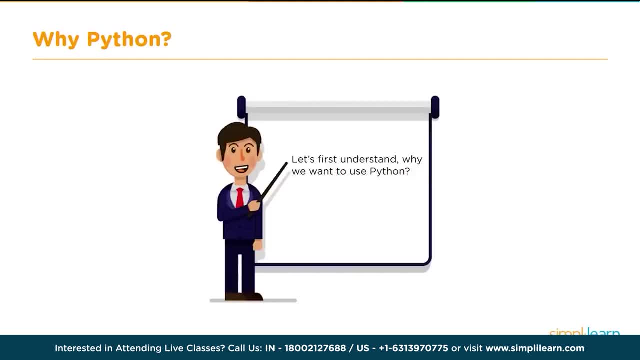 A programming language or a tool and so on. So this session will be about Python. There are other tools, like, for example, R, and we will probably do a separate video on that, But this session is on Python, and you must have already heard. Python is really becoming 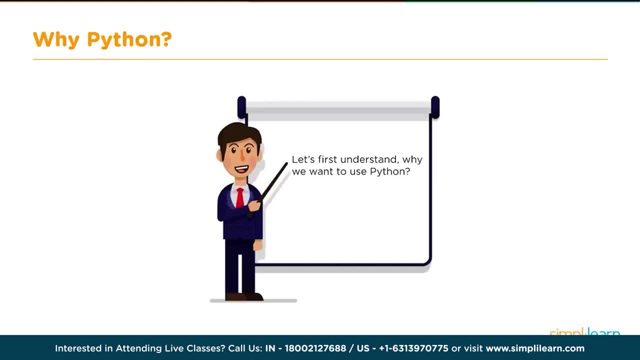 very popular. Everybody is talking about Python, not only data science, in IoT and AI and many other places, So it's a very popular, it's getting very popular. So if you are not yet familiar with Python, this may be a good time to get started with. 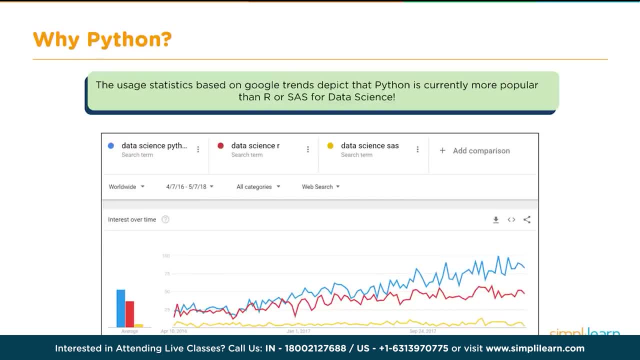 it? Why do we want to use Python? So, basically, Python is used as a programming language, because it is for data science, because it has some rich tools from mathematics and from a statistical perspective it has some rich tools. So that is one of the reasons why we use Python. 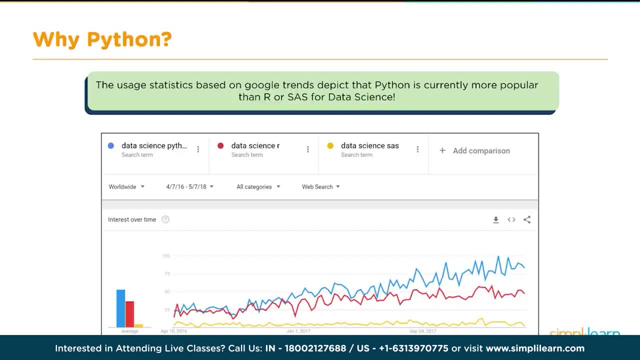 And if you see some of the trends- if you're probably tracking some of the trends- you will see that over the last few years, Python has become programming language of choice, And especially for data science. SAS was earlier One of the most popular tools, but now, increasingly, Python is being used for doing data science. 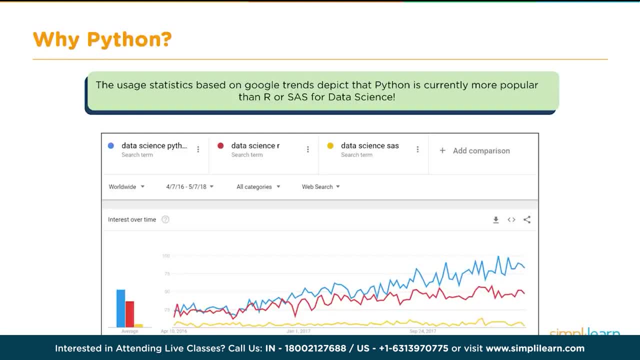 And, of course, as well as R. One of the reasons, of course, is that Python and R are open source compared to SAS, which is a commercial product, So that could definitely be one explanation, But beyond that, I think it is the ease of understanding this language, the ease of using. 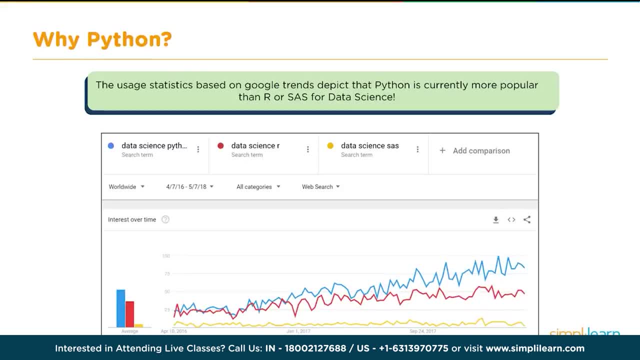 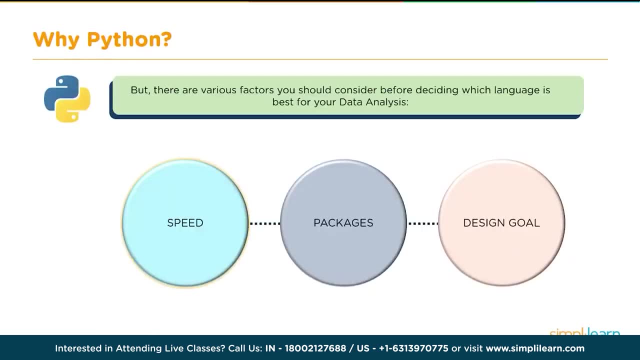 this language, which is also making it very popular, In addition to the availability of fantastic libraries for performing data science. What are the other factors? There are a number of factors. There are speed, then there are availability of number of packages and then, of course, 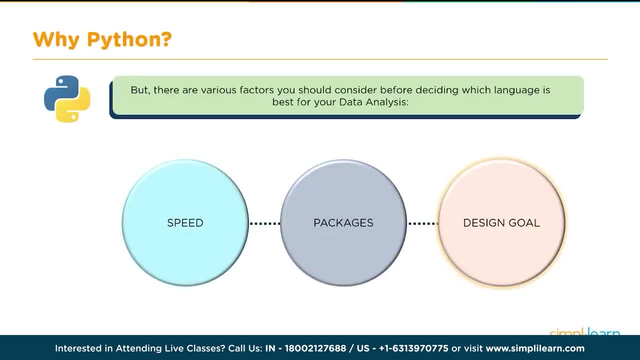 the design goal, All right. So what are each of these design goals? Primarily, the syntax rules in Python are relatively intuitive and easy to understand. thereby it helps in building applications with concise and readable code base. So with a few lines of code you can really achieve a lot of stuff. 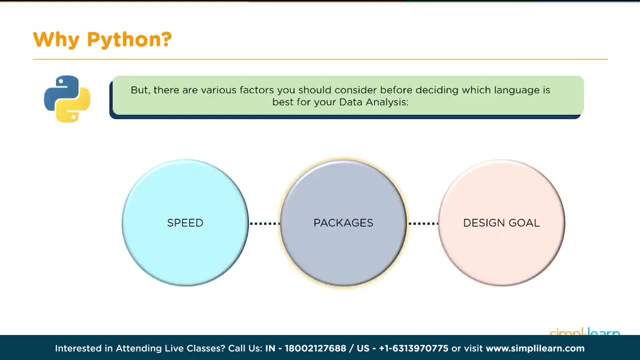 And then there are a lot of packages that are available, that have been developed by other people, Which can be reused, So we don't have to reinvent the wheel. And last but not least, the speed. So Python is a relatively faster language. 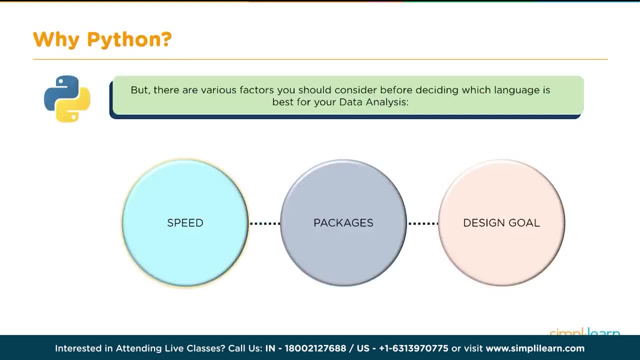 Of course it is not as fast as, let's say, CRC++, but then relatively it is still faster. So these are the three factors which make Python the programming language of choice. So if you want to get started with Python, the first thing obviously is to install Python. 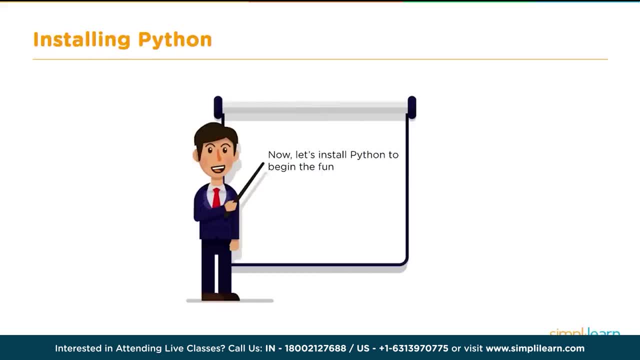 So there is some documentation, there are some steps that you need to follow, So we will try to briefly touch upon this, On that. otherwise, of course, there is a lot of material available on how to install Python and so on. You can always look around. 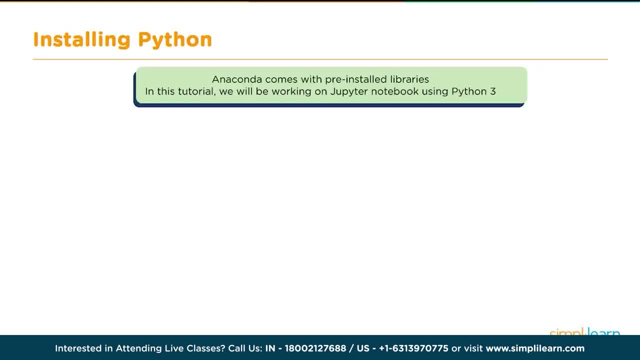 But this is one of the. again, there are different ways in which you can also install Python, So we will use the Anaconda path. There is a packaging tool called Anaconda, So we will use that path. You can also directly install Python. 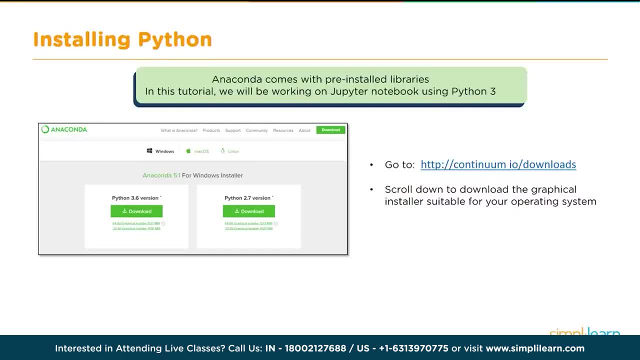 But in our session we will use the Anaconda route. So the first thing you need to do is download Anaconda, And this is the path for that- And once you click on this You will come to a page somewhat like this- and download. 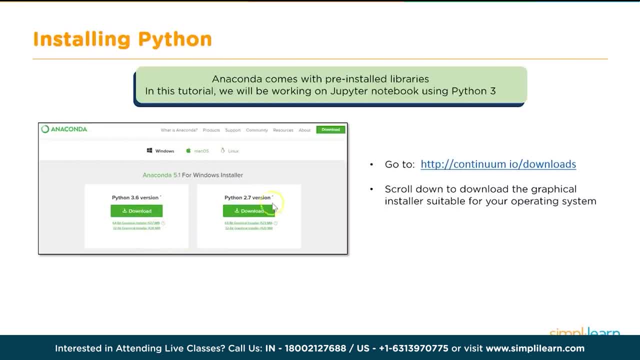 You can do the corresponding download based on whether you have a Windows or Ubuntu. There is also a download possible for a package available for Ubuntu if you are doing something on Ubuntu. So based on which operating system? in fact, this page will automatically detect which. 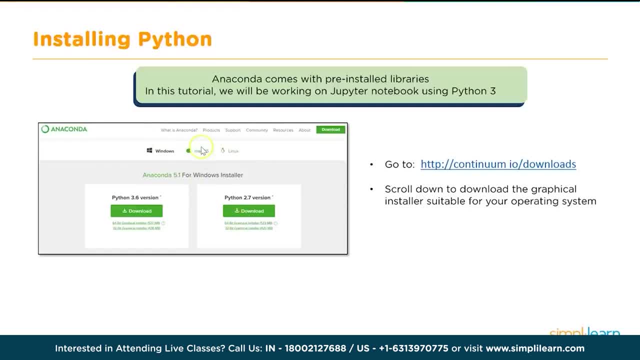 operating system you're having and it will actually suggest So. for example, you see here, if you're running Mac OS, then it will automatically detect that you have Macs And the corresponding installers will be displayed Here. Similarly, if you're on some flavor of Linux, like Ubuntu or any other, then you will get 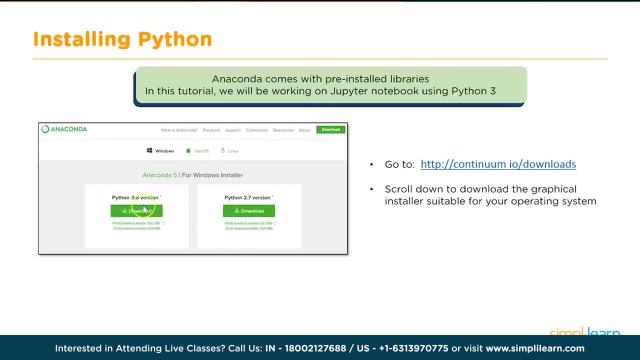 the corresponding download links here And then beyond that, you can also select which version of Python you want to install. Of course, the latest version is in the 3.x range. at the time of recording this, 3.6 is one of the latest versions. 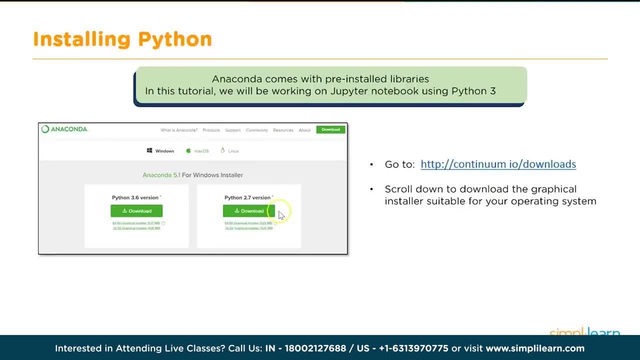 But some of you may want to do or start with the earlier version, which is Python 2.7, 2.x, and you can download that as well. If you don't have anything installed, then my suggestion is start with Python 3.6.. 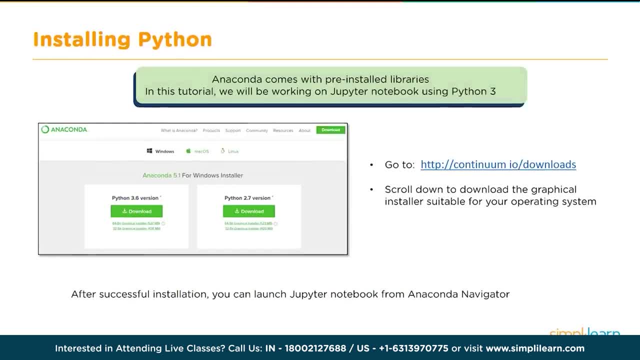 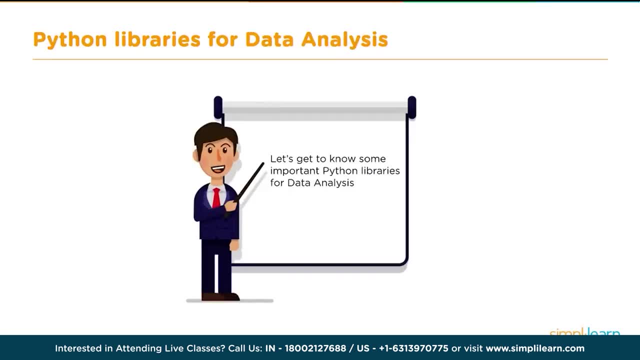 All right. So once you do that, you will be able to install Python and you will be able to run Jupyter notebook. Okay, so, now that you know how to install Python and you have installed Python, let's take a look at what are the various libraries that are available. 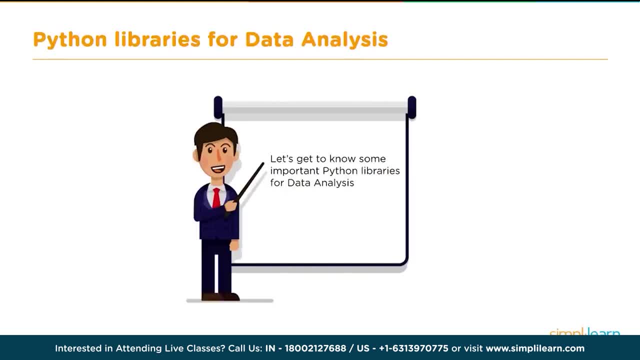 So Python is a very easy language to learn and there are some basic stuff that you can do- For example, adding or printing a hello world statement and so on- without importing any specific libraries. But if you want to perform data analysis, you need to include or import some specific. 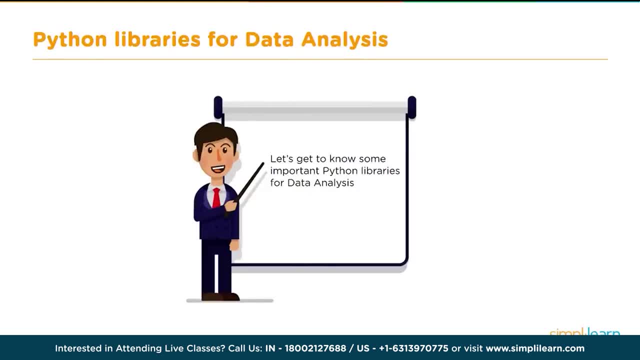 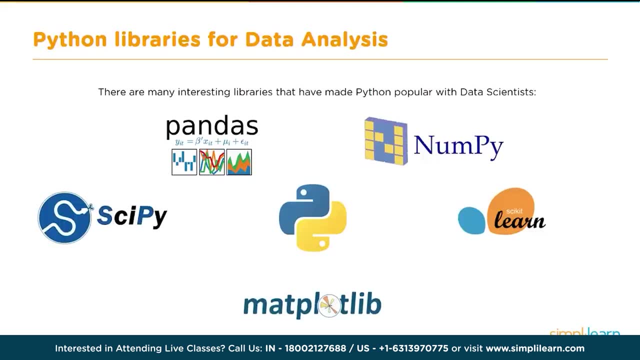 libraries. So we are going to talk about those as we move forward. So pandas, for example, is used for structured data operations. So if you, let's say, are performing something on a CSV file, you import, a CSV file, create. 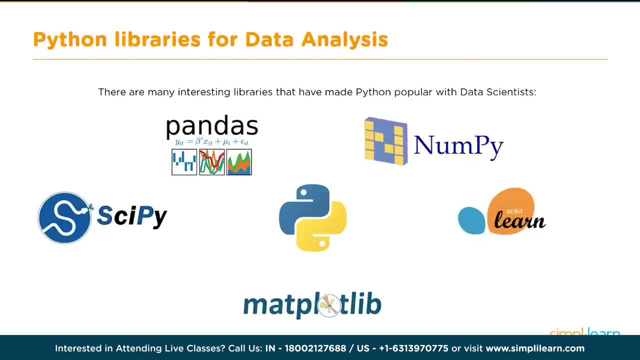 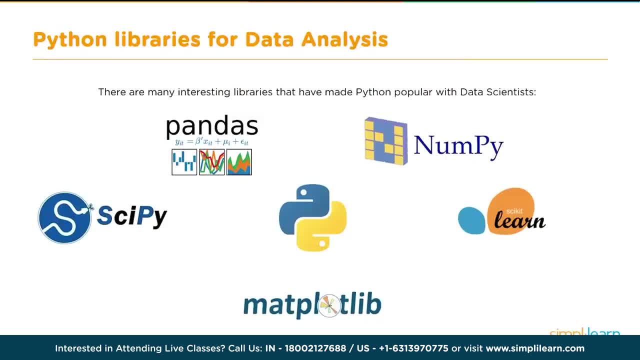 you do any other stuff like, for example, machine learning or so on. So that's pandas SciPy, as the name suggests it is kind of. it provides more scientific capabilities, like for example, it has linear algebra, it has Fourier transform and so on. 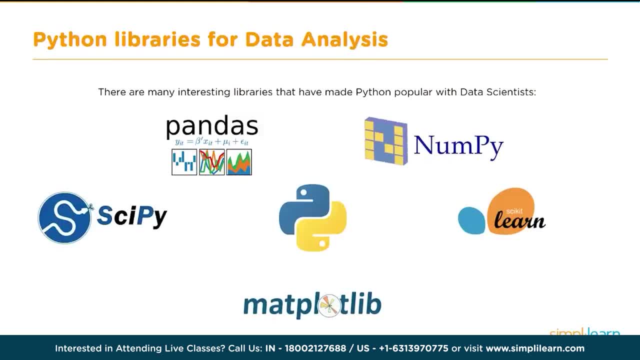 and so forth. Then you have NumPy, which is a very powerful library for performing and dimensional or creating and dimensional errors, And it also has some of the stuff that is there in SciPy, like, for example, linear algebra and Fourier transform and so on and so forth. then you have matplotlib, which is 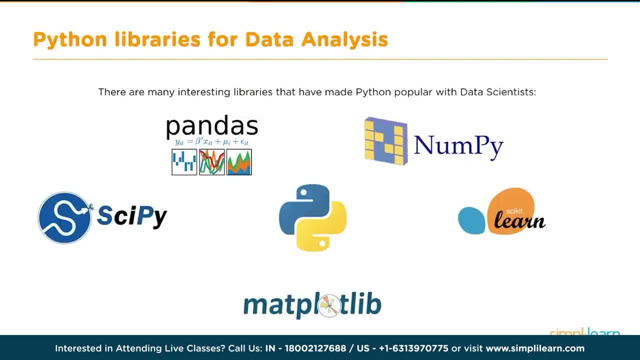 primarily for visualization purpose. it has, again, very powerful features for visualizing your data, for doing the initial what is known as exploratory data analysis, for doing univariate analysis, bivariate analysis. so this is extremely useful for visualizing the data and then scikit-learn. 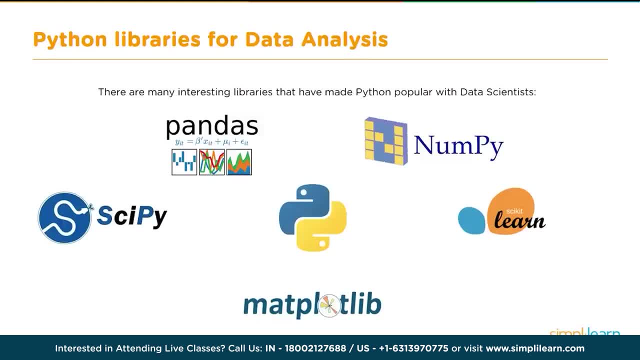 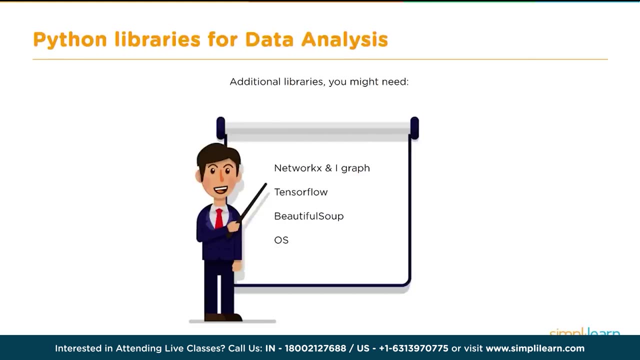 is used for performing all the machine learning activities. if you want to do anything like linear regression, classification or any of this stuff, then the scikit-learn library will be extremely helpful. in addition to that, there are a few other libraries, for example networks and i graph. then, of course, a very important one is tensorflow. so if you are 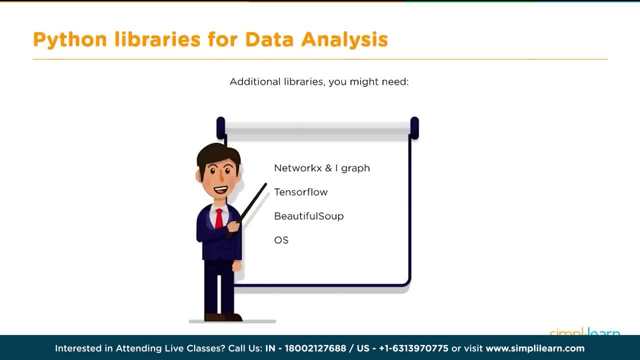 interested in doing some deep learning or ai related stuff, then it would be a good idea to learn about tensorflow, and tensorflow is one of the libraries. there is a separate video on tensorflow, you can look for that, and this is a one of the libraries created by google open source library. so once you are familiar with machine learning, data analysis, 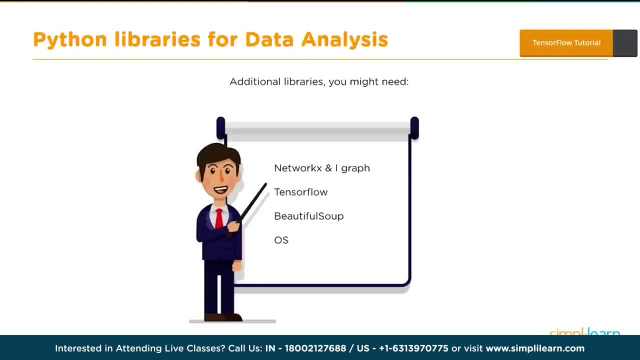 machine learning, then that may be the next step to go to deep learning and ai, so that's where tensorflow will be used. then you have beautiful soup which is primarily used for web scraping, and then you take that data and then analyze and so on. then os library is a very common 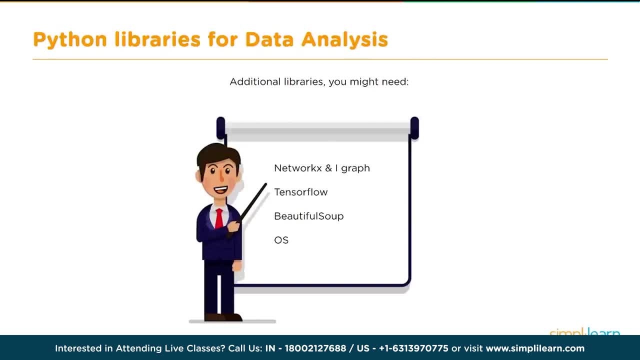 library. as the name suggests, it is for operating system. so if you want to do something on creating directories or folders and things like that, that's when you would use os, all right. so, moving on, let's talk in a little bit more detail about each of these libraries. so psypi. 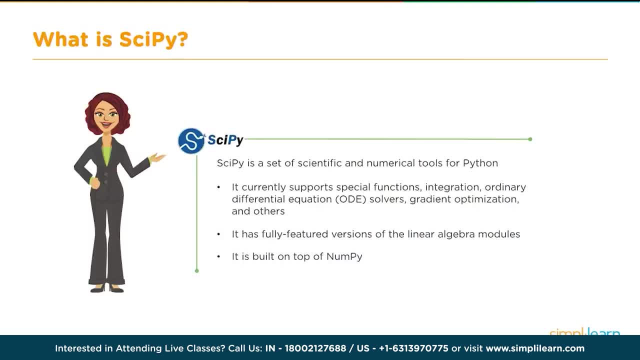 as the name suggests, is a scientific library and it very specifically it has some special functions for integration and for ordinary differential equations. so, as you can see, these are mathematical operations or mathematical functions. so these are readily available in this library and it has linear algebra modules and it is built on top of numpy. so 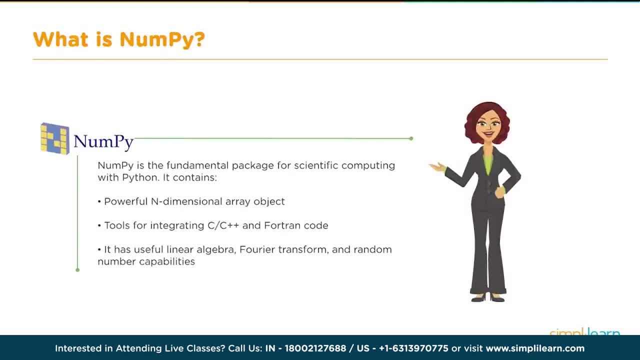 see what is there in numpy. so this is a. again, as the name suggests, that num comes from numbers, so it is a mathematical library, and one of its key features is availability of an n-dimensional array object. that is a very powerful object, and we will see how to use this. and then, of course, you can. 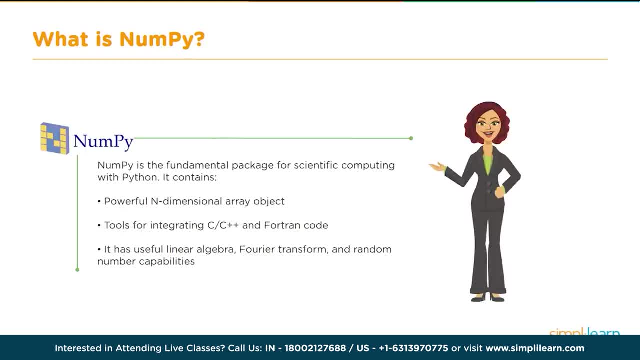 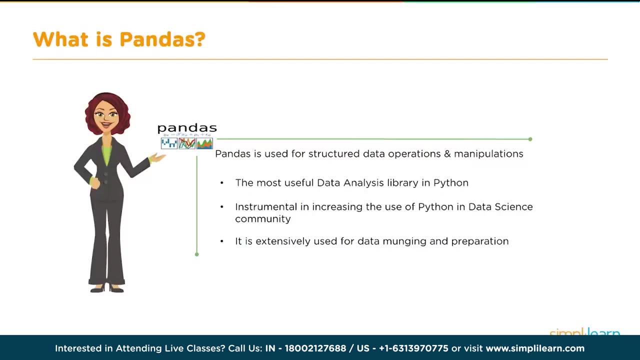 create other, let's say, objects and so on, and it has tools for integrating with c, c plus, plus, and also for trancode, and then it of course also has linear algebra and fourier transformation and so on, all these scientific capabilities. okay, what else? pandas is another very powerful. 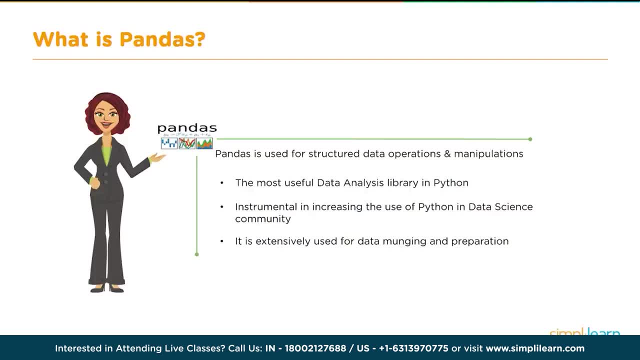 library primarily for data manipulation. so if you are importing any files, you will want to create it like a table. so you will create what is known as data frames. these are very powerful data structures that are used in python programming. so pandas library provides this capability and once you 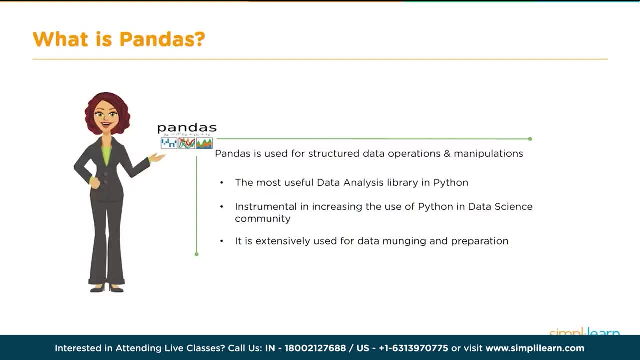 import a data, import the data into data frame, you can pretty much do whatever you're doing, like in a regular database. so people who are coming from a database background or sql background would really like this because it is very they will feel very much at home because it feels like 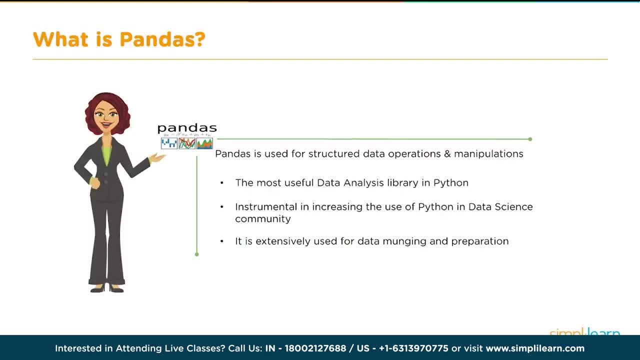 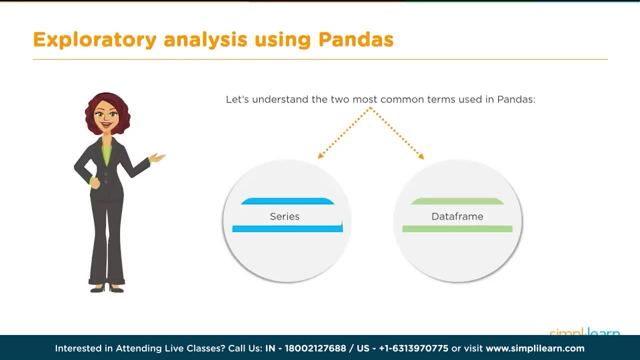 you're using. you're viewing a table or using a table, and you can do a lot of stuff using the pandas library. now there are two important terms or components in pandas: series and the data frame. i was just talking about the data frame, so let's take a look at what are series and 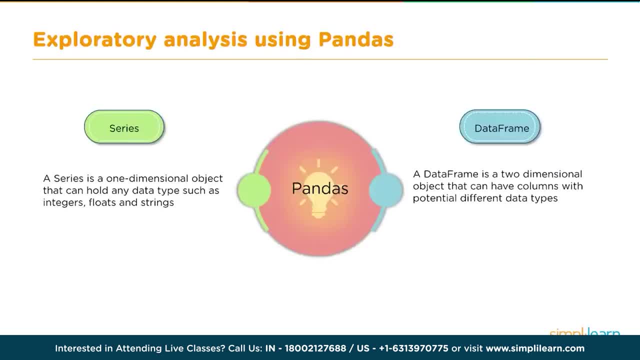 uh, what is a data frame? so within pandas we have series and data frames. so series is primarily- some of you may also be knowing this- as, let's say, an array, so it's a one-dimensional structure, data structure. if you will saying some of the languages, we may call it as an array or 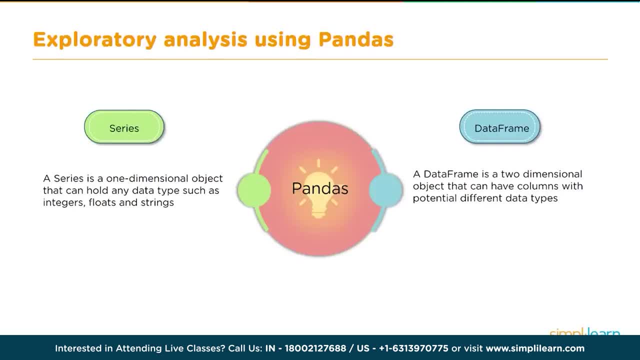 maybe some others, probably an equivalent of a list in r. perhaps i'm not very sure on that aspect, but yes, so this is like a one-dimensional storage of information, so that is what is series, whereas data frame is like a table. so you have a two-dimensional structure: you have rows and you have columns and 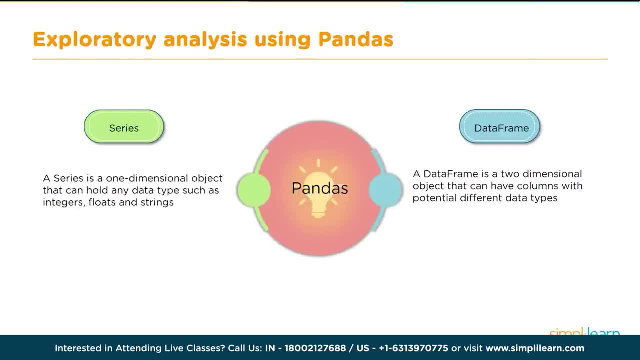 this is very people, as i said, who are familiar with sql and databases will be able to relate to this very quickly. so you have like a table, you have rows and columns and then you can manipulate the data. so if you want to create a series, this is how you would create a code snippet and, as you can, 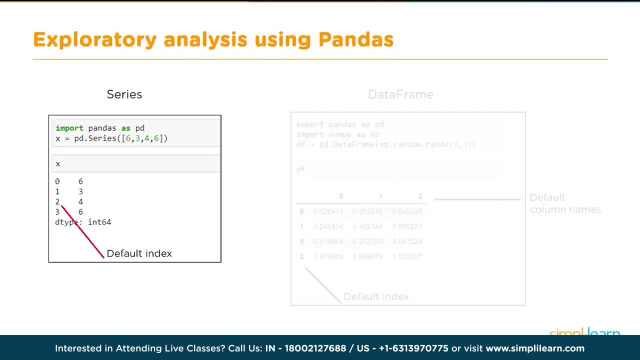 see, the programming in python is very simple. there are no major overheads. you just need to import some libraries, whichever essential, and then start creating objects, so you don't have to do additional declaration of variables and things like that. so that is, i think, one key difference between python and other. 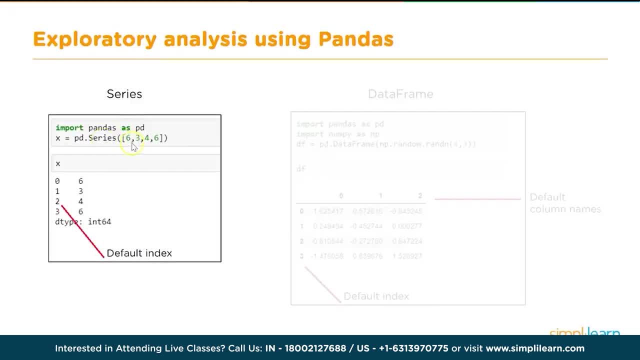 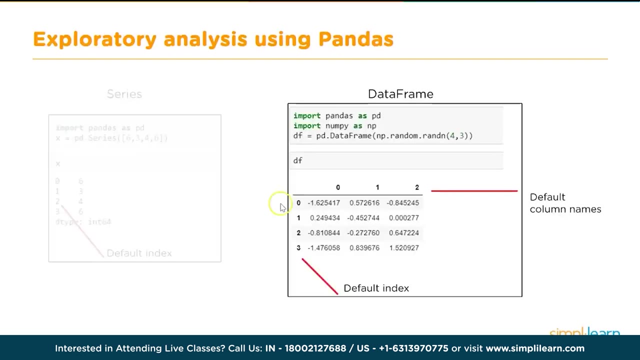 programming languages. and what does this series contain? it has to contain these numbers: six, three, four, six and x is my object consisting of the series. so if you display, if you just say x, it will display the contents of x and you will see here that it creates a default index. then you have 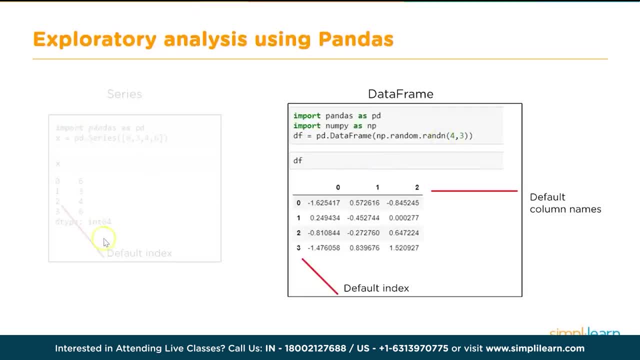 data frame. so if you want to create a data frame, you have to create a data frame, you have to create a data frame. as you can see, the series is like a one dimensional structure. there is just like a row, one row of items, whereas a data frame looks somewhat like this: it is a two-dimensional. 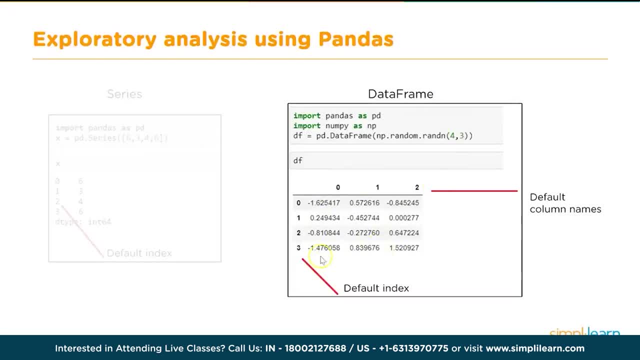 structure, so you have columns in one dimension and then you have rows in the other dimension. how do you create a data frame? you need to create, you need to, rather, import pandas and then you import. in this case, we are basically creating our own data, so that's the reason we are importing. 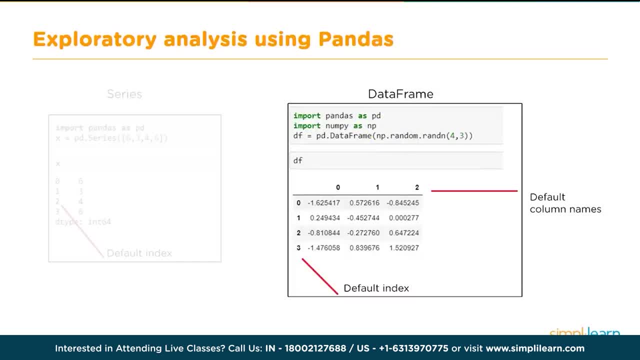 numpy, which is one of the libraries we just referred to a little bit before. so we are using one of the functionalities within numpy to create some random numbers. otherwise this is not really mandatory. you probably will be importing the data from outside- maybe some csv file- and import into the data frame. so that's what we're doing here. so 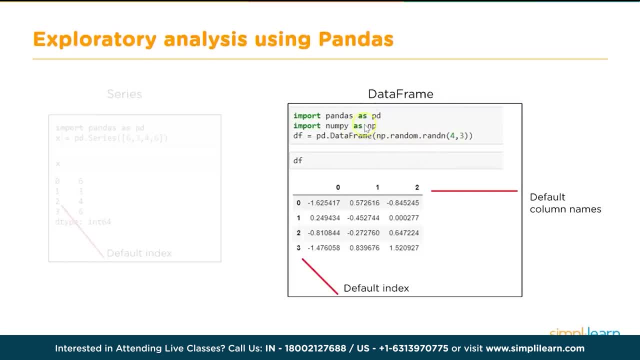 in this case, we are creating our own test data. that's the reason we are importing numpy as np, and then i create a data frame saying pd, dot data frame. so this is the keyword here. similarly, here in this case, while creating series, we said pdcd and then you pass the values. similarly, here you're saying pddata frame. now, in order to create the 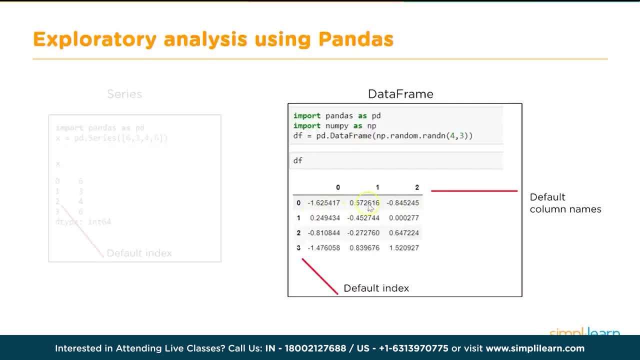 data frame. it needs the values in each of these cells: what are the values in the rows and what are the values in the column, so that in our example, we are providing using this random number generator. so np dot random is like a class or a method that is available in numpy and then you are 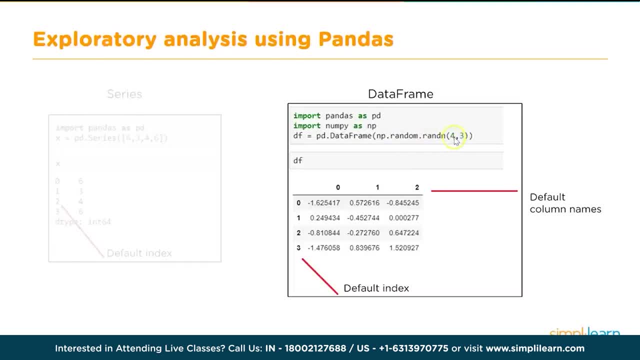 saying: okay, generate some random numbers in the form of a 4 by 3 matrix or 4 by 3 data frame, the number of rows and the 3 here indicates the number of columns. so these are the columns: 0, 1, 2 are the. 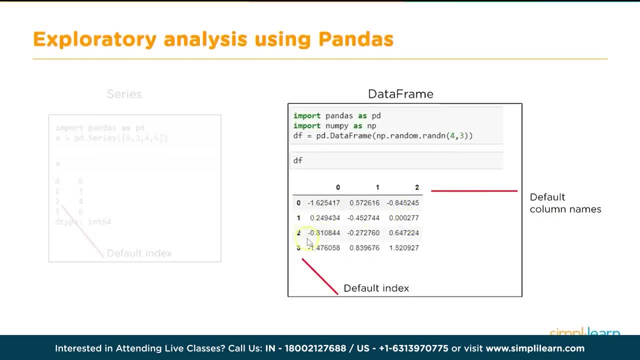 columns and these are the rows here: 0, this is 1, this is 2, this is 3. okay, and once again it will. when you display df, it will give us a default index. there are ways to omit that, but at this point we will just keep it simple. so it will display the default index and then the actual. 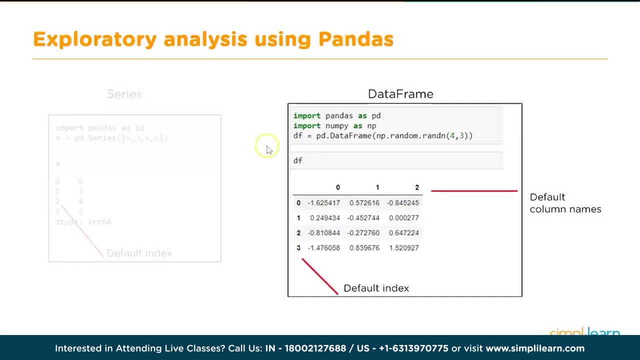 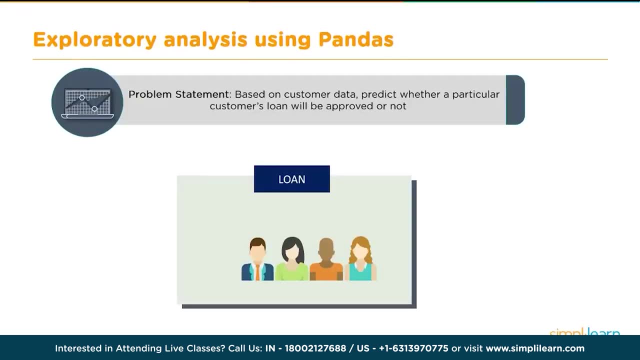 values in each of these rows and columns. so this is the way you can create the data frame. so now that we have learned some of the basics of pandas, let's take a quick look at how we use this in real life. so let's assume we have a situation where we have some customer data and we want to 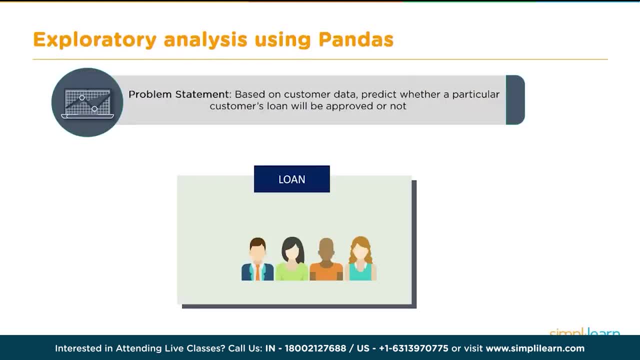 kind of predict whether a customer's loan will be approved or not. so we have some historical data about the loans and about the customers and using that we will try to come up with a way to maybe predict whether loan will be approved or not. so let's see how we can do that. so this is 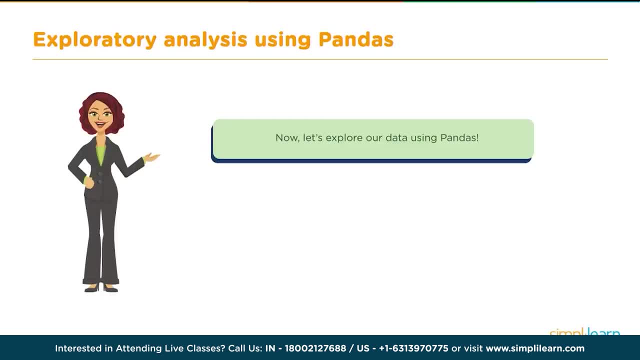 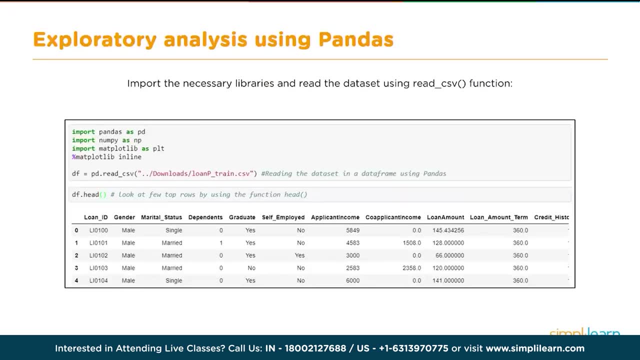 a part of exploratory analysis. so we will first start with exploratory analysis. we will try to see how the data is looking. so what kind of data? so we will, of course, I'll take you into the jupiter notebook and give you a quick live demo, but before that, let's quickly walk through some of the pieces. 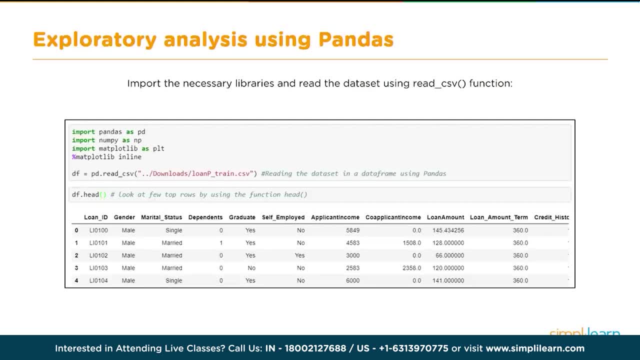 of this program in slides and then I will take you actually into the actual code and do a demo of that. so the python program structure looks somewhat like this. the first step is to import your all the required libraries. now of course it is not necessary that you have to import all. 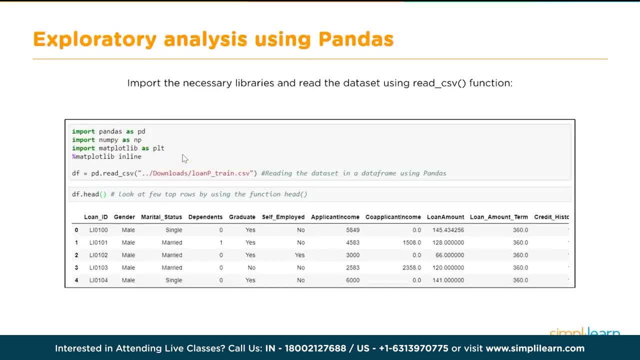 your libraries right at the top of the code, but it is a good practice. so you, if you know you are going to need a certain set of libraries, it may be a good idea to put from a readability perspective. it's a good practice to put all the libraries that you're importing at the beginning of your code. 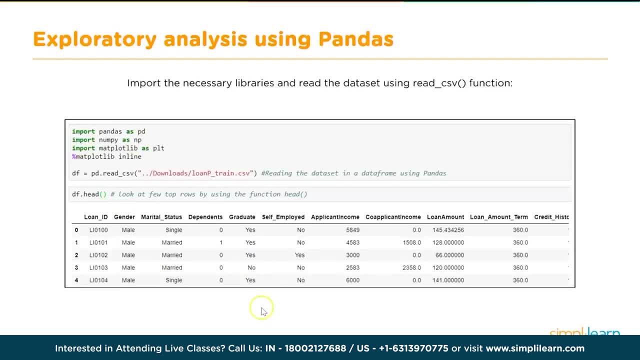 however, it is not mandatory. so in the middle of the code somewhere, if you feel that you need a particular library, you can import that library and then start using it in the middle of the code. so that's also perfectly fine. it will not give any errors or anything. however, as I said, it's not such a good. 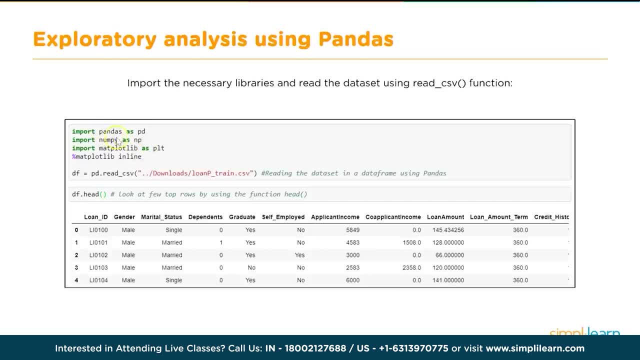 practice. so we will import all the required libraries. in this case, we are importing pandas, numpy and matplotlib and, in addition, if we include this piece of code- percentage matplotlib- inline, what will happen is all the graphs that we are going to create, the visualizations that we are 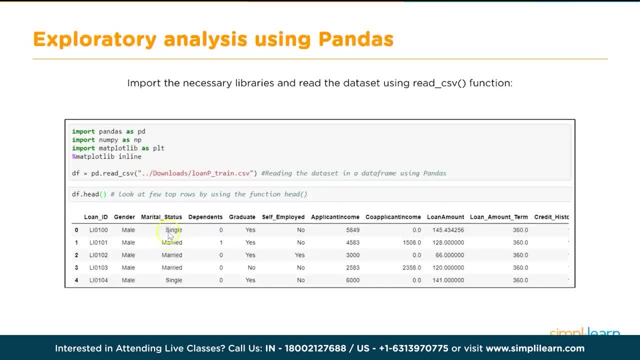 going to create will be created within the notebook. so if you want to have that kind of a provision, you need to have this line. so it's always a good idea when you're starting off. I think it's a good idea to just include this line so that your graphs are shown in line. okay, so these are the four. we will start. 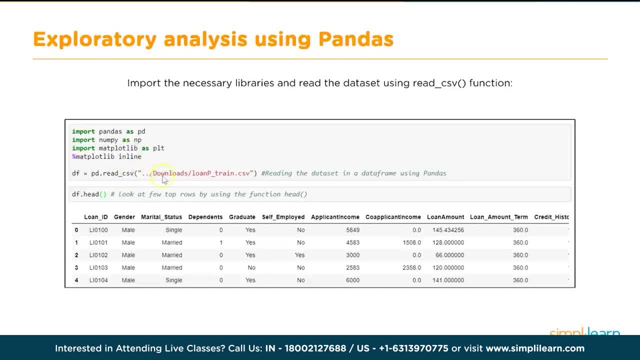 with these four lines of code, then the next step is to import your data. so in our case, there is a training data for loans by the name loan pe, underscore traincsv, and we are reading this data. Unlike the previous example, where we created our data frame with some data that we created ourselves, here we are actually creating a data frame using some external data, and it's the method is very, very straightforward. 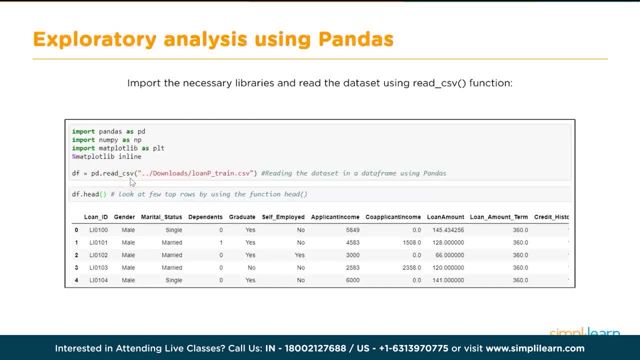 So you use the read underscore CSV method- and it is a very intuitive function name- and you say PD, dot. read underscore CSV and give the path of the file: CSV, file. That's about it, And then that is read into the data frame: DF. This can be any name. We are calling it DF. You can call XYZ anything. There's a name, just name of the object. So head is one of the methods within the data frame and it will give us the first five. So this is just to take a quick look. Now you have imported the data, You want to initially have a quick look how your data is looking, What are the values in some of the columns and so on and so forth. Right, So typically you would do a head DF, dot, head to. 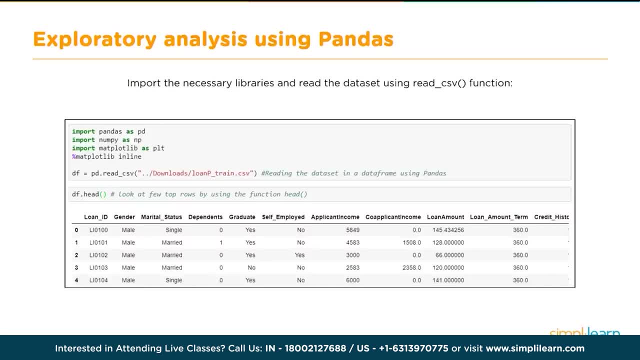 get the sample of, let's say, the first few lines of your data. So that's what has happened here. So it displays the first few lines and then you can see what are the columns within that and what are the values and each of these cells and so on and so forth. You can also, typically you would like to see if there are any null values, or are there any? is the data, for whatever reason, is invalid or looking dirty for whatever reason, some unnecessary character? 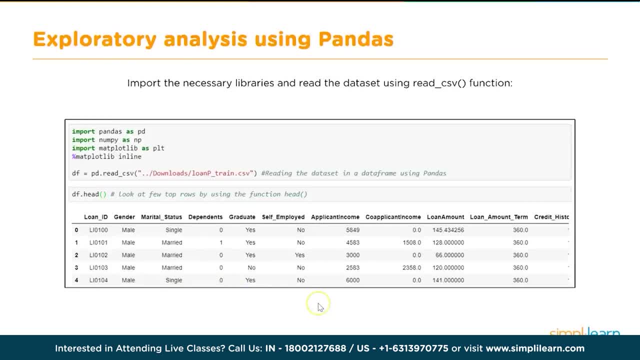 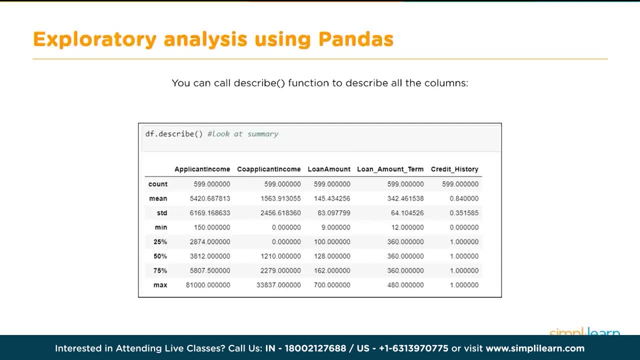 So this will give a quick view of that. So in this case pretty much everything looks okay. Then the next step is to understand the data a little bit overall. for each of the columns, What is the information? So the describe function will basically give us a summary of the data. What else can we do? Pandas also allows us to visualize the 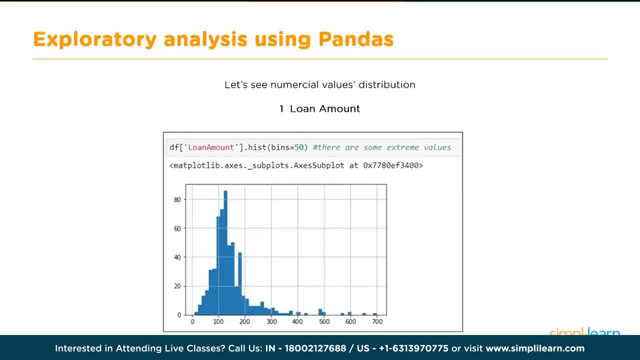 data and this is more like a part of what we call it as univariate analysis. That means each and every column you can take and do some plots and visualization to understand data in each of the columns. So for example, here the loan amount column we can take and then the hist, basically 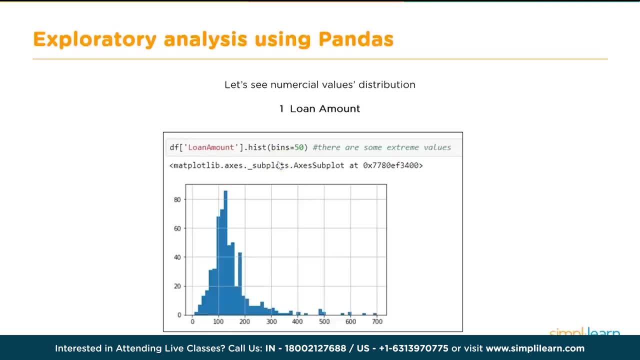 hist method will create a histogram. So you take all the values from one column, which is loan amount, and you create a histogram to see how the data is distributed. So that's what is happening here and, as you can see, there are some extreme values. So this is again to identify. do we have to? 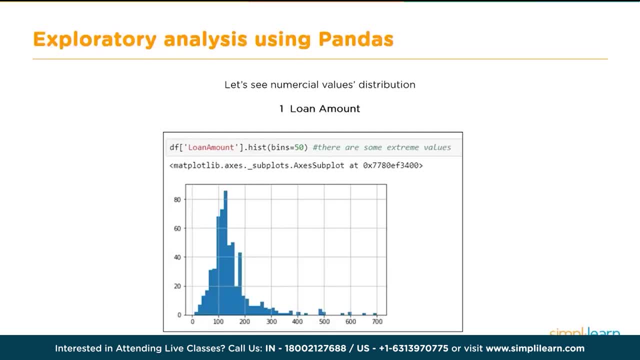 do some data distribution for this column. So that's what I'm seeing here. Let's see how it preparation, because if the data is in a completely haphazard way the analysis may be difficult. so with these are initial or exploratory data analysis is 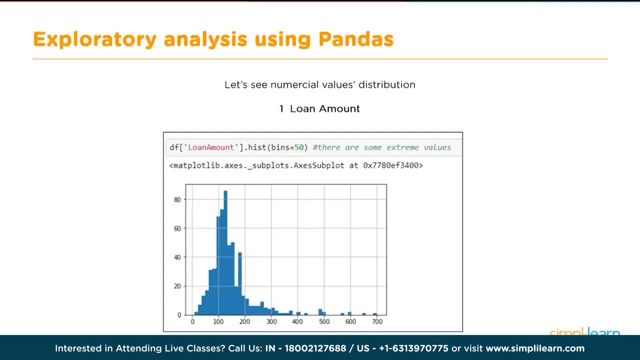 primarily done to understand that and see if we need to do some data preparation before we get into the other steps like machine learning and statistical modeling and so on. so in this case we will see that here. by plotting this histogram we see that there are some extreme values, so there 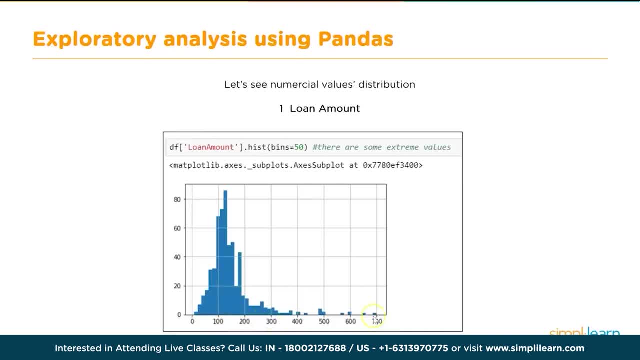 are some values. a lot of it is around hundred range, but there is also something, one or two observations in the 700 range. so it's pretty scattered in that sense, or they are not really scattered, distributedly scattered, but it is randomly scattered, so the range is really huge. so what can we do about this? 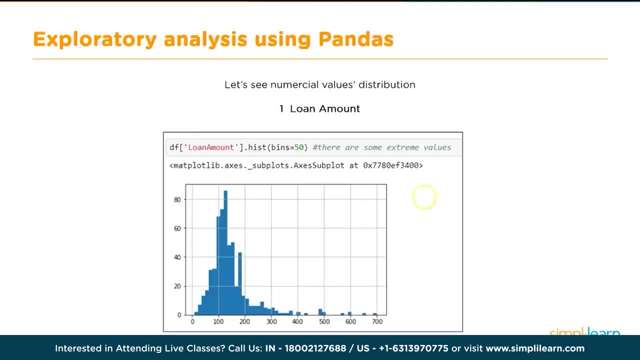 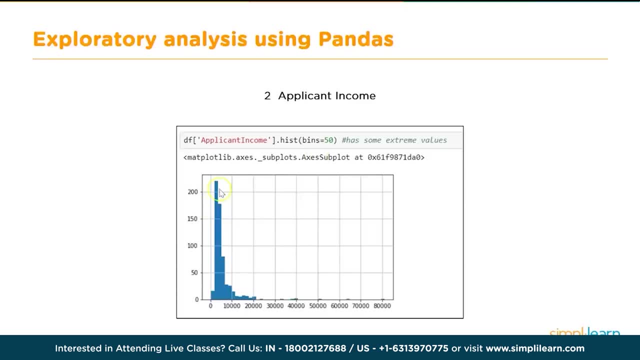 so there are some steps that we need to do- normalization and so on. so we'll see that in a bit. so this is for one of the columns. let's take another column, which is applicant income. similar kind of similar situation. you have most of your observations in this range, but there are also some which are far off. 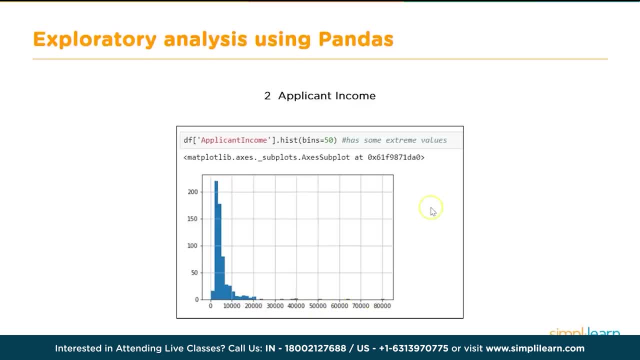 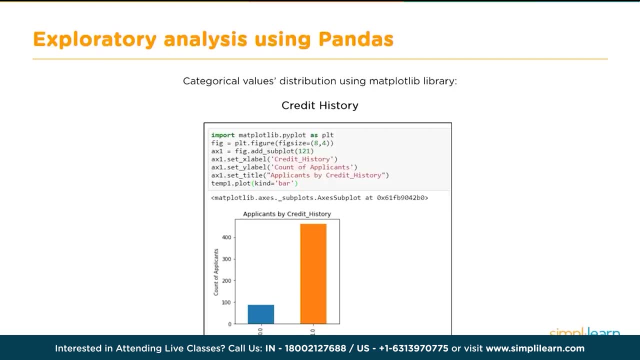 far off from where most of the observations are. so this is also pretty. this also has some extreme values, so we'll have to see what can be done. credit history is the binary value, so some people have a zero value and some will have credit history of one. this is just like a flag. so this, basically, is telling us how many people 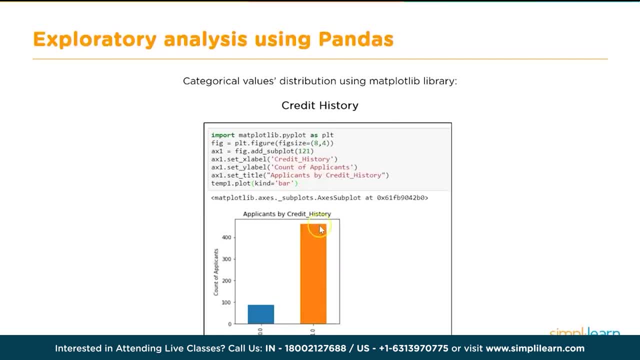 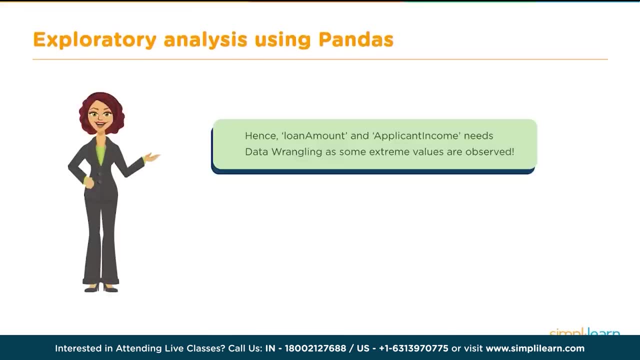 have a one, and how many people have zero? so it looks like majority of them have a value of one and a few- about hundred of them- have a value of zero. okay, what else can we do? so we now understood the value of the value, of the value of the. 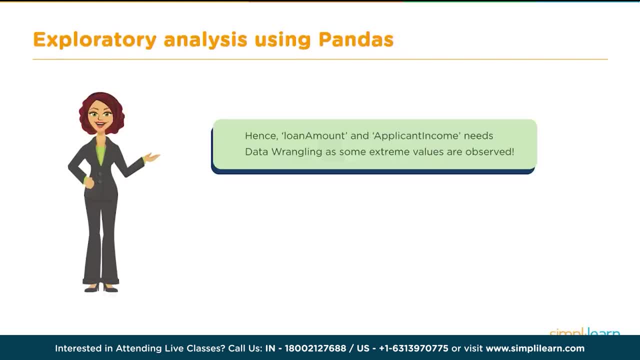 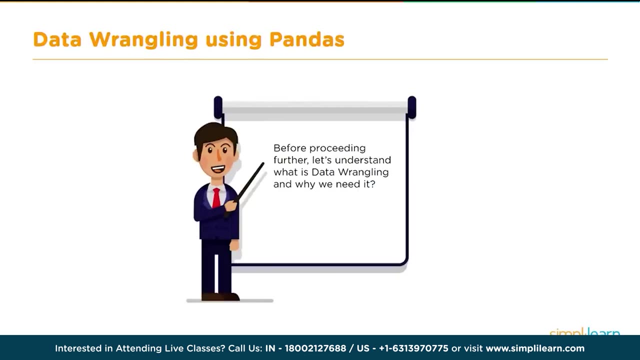 data. so we need to do some data wrangling or data munging and see if we can some bring in some kind of normalization of all this data, and we will kind of try to understand what is data wrangling and before we actually go into it. okay, so data wrangling is nothing but a process of cleaning the 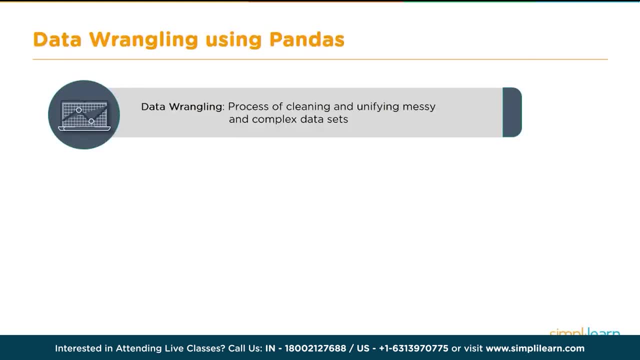 data, if let's say there are, there are multiple things that can happen. in this particular example, there were no missing values, but typically when you get some data, very often it will so happen that a lot of values are missing. either they are null values or there are a lot of zeros. now you cannot use such data as it. 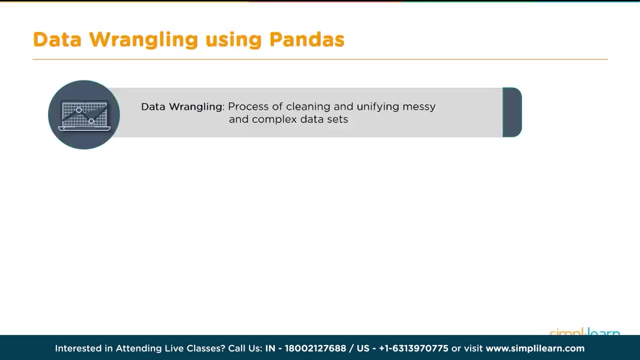 is to perform some, let's say, predictive analysis, or perform some machine learning activities and so on. so that is one part of it. so you need to clean the data. the other is unifying the data. now these ranges of this data are very huge. some of them are going from some columns, are going from zero to one hundred. 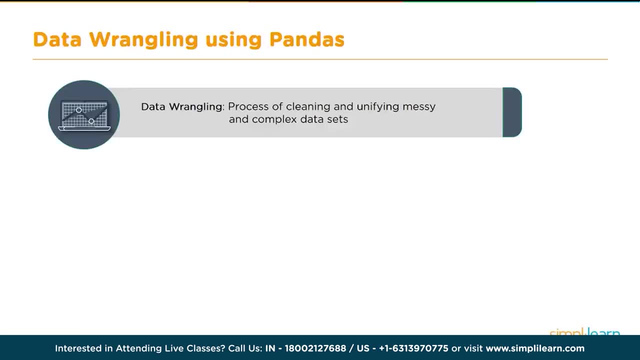 and some columns are just between 10 to 20 and so on. these will affect the accuracy of the analysis, so we need to do some kind of unifying the data and so on. so that is what wrangling data wrangling is all about. so before we 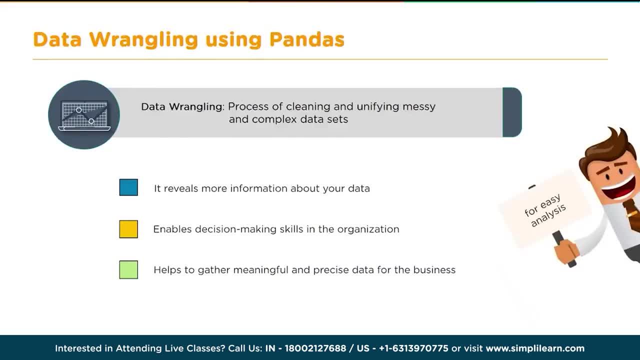 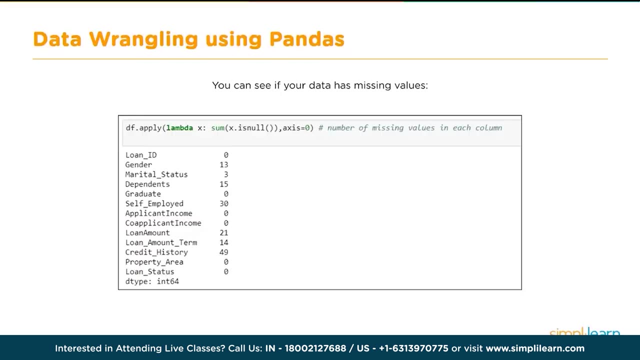 actually perform any analysis. we need to bring the data so to some kind of a shape so that we can perform additional analysis, actual analysis on this, and get some insights. now, how do we deal with missing values is a very common issue when we take data or when we get data from the business. when a data 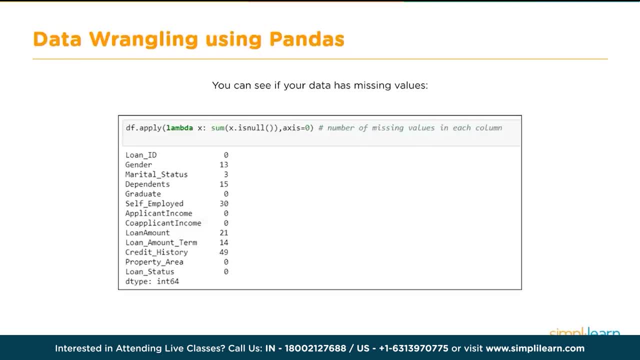 scientist gets the data from the business. so we should never assume that all our data will be clean and all the values filled up and so on, because in real life very often there will be the data will be dirty. so data wrangling is the process where you kind of clean up the data. first of all, identify whether 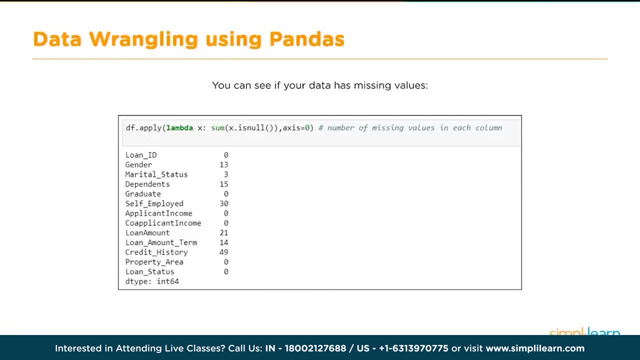 the data is dirty and then clean up. so how do we find some data is missing. so there are a few ways. you can write a small piece of code which will identify if, for a given column, for given row, any of the observations are null. primarily so this line of code, for example, is doing that. 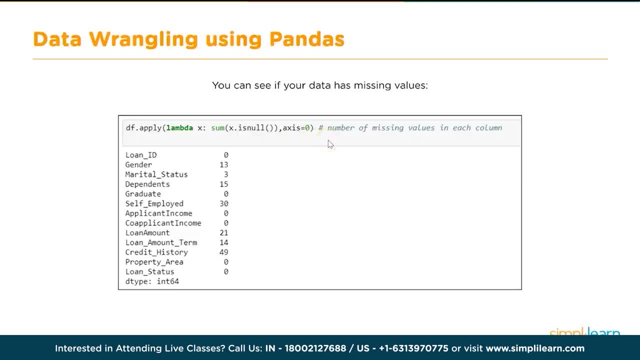 it is trying to identify how many null values or missing values are there for each of the columns. so this is a lambda function and what we are saying is find out if a value is null, and then you add all of them. how many observations are there where this particular column is? 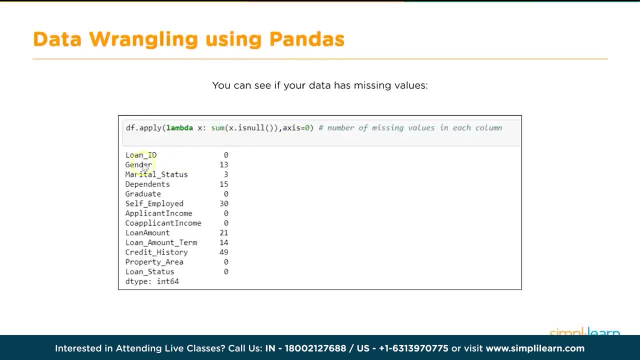 null, so it does that for all the column. so here you will see that for loan ID, obviously it's an ID, so there are no null values or missing values. gender has about 13 observations where the values are missing. similarly, marital status has three, and so on and so forth. so we'll see here, for example, loan amount has 21. 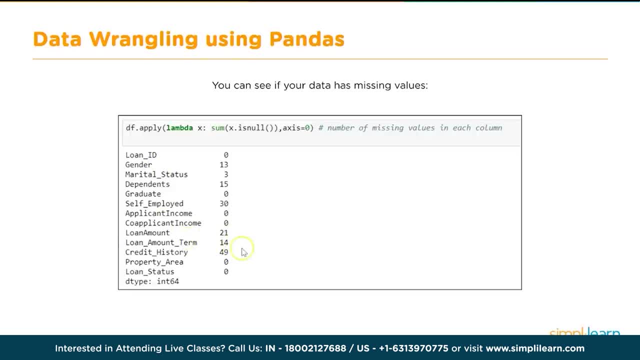 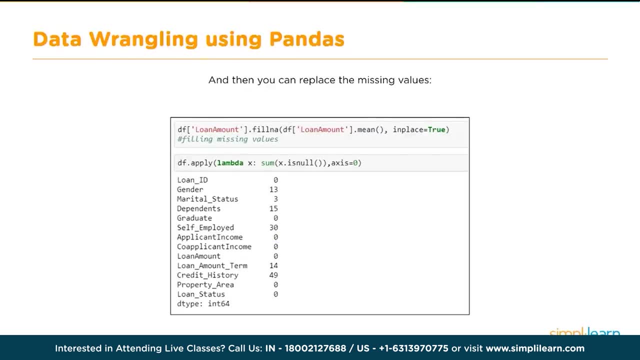 observations where the values are missing. loan amount term has 14 observations, and so on. so we'll see how to handle this. missing values. so there are multiple ways in which you can handle missing values if the number of observations are very small compared to the total number of. 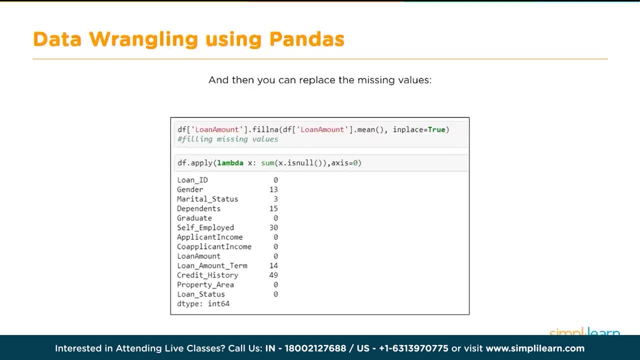 observations. then sometimes one of the easy ways is to completely remove that data. so or delete that record, exclude that record. so that is one way of doing it. so if there are, let's say, a million records and maybe 10 records are having missing values, it may not be worth doing something to fill up those values. it may. 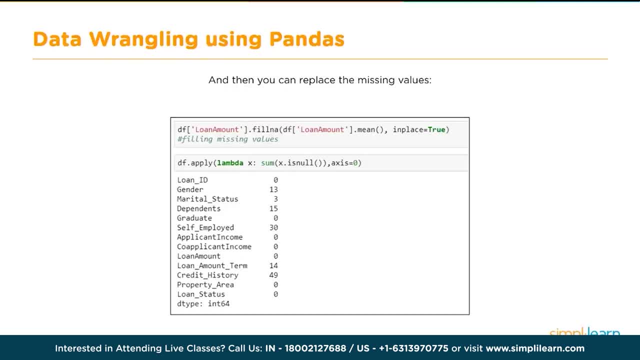 be better off to get rid of those observations, right? so that is the example where the missing values are being filled up and then, while having more values filled up, moving them in to get rid of them. so people often think you just have to spend, you know, 70 000 of inventory. 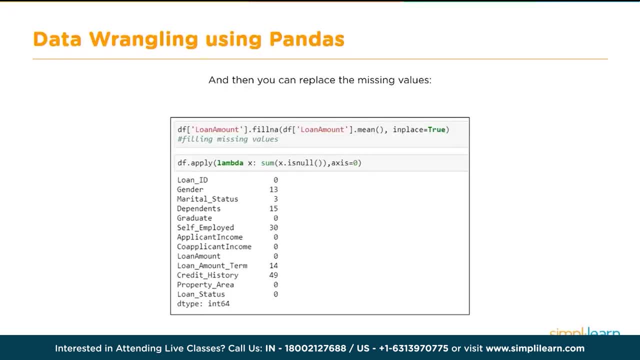 something to fill your ones missing values. so you always want to do is to enter something that are being filled up. so in the same way you entered 200, built them up, you fill up your ones that has too many missing values. as you see, many people don't have that number and my English for gibt zone was: 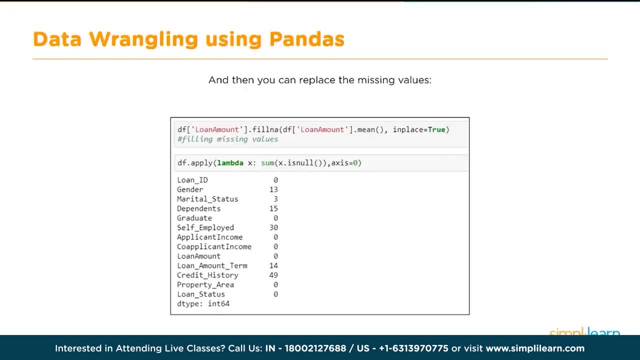 or too low, and it somehow fits within the range of the observations that we are seeing. So this is one technique again there are. it can be case to case and you may have to take a call based on your specific situation, But these are some of the common methods. 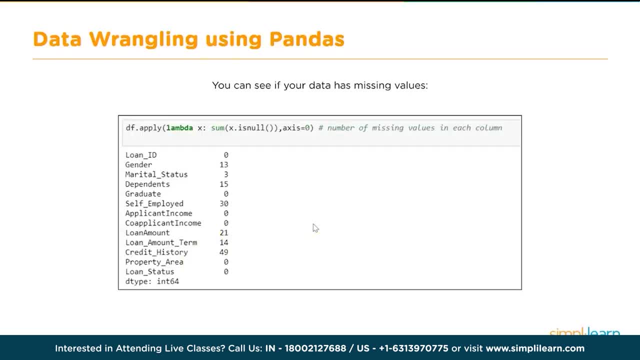 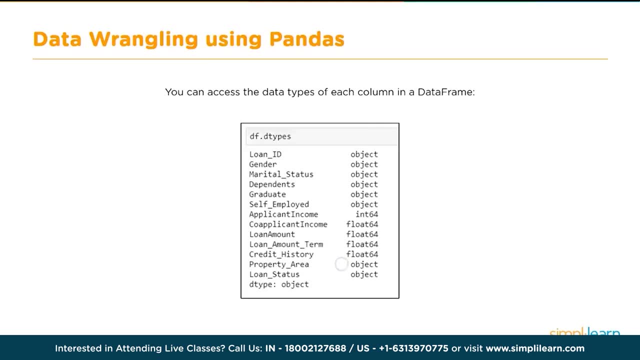 If you see, in the previous case loan amount had 21 and now we went ahead and filled all of those with the mean value. So now there are zero with missing values. So this is one part of a data wrangling activity. What else you can do? 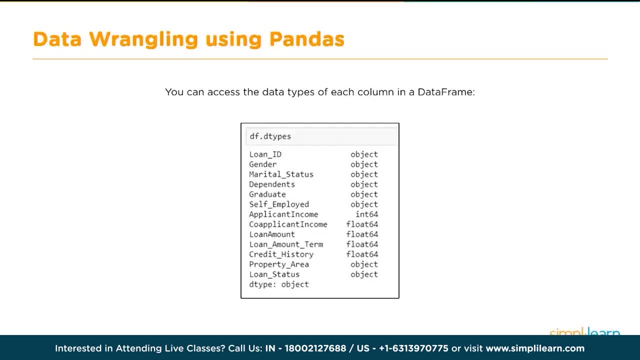 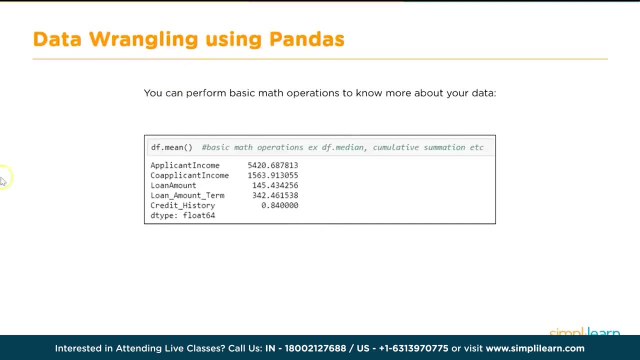 You can also check what are the types of the data. So df, dot, d types will give us what are the various data types. So all right, So you can also perform some basic mathematical observations. we have already seen that mean we found out. 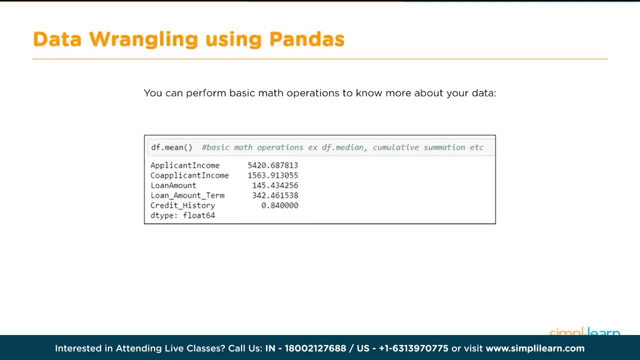 So, similarly, if you do call the mean method for the data frame object, it will actually perform or display or calculate the mean for pretty much all the numerical columns that are available in this right. So for example here applicant income, co-applicant income, and all these are numerical values. 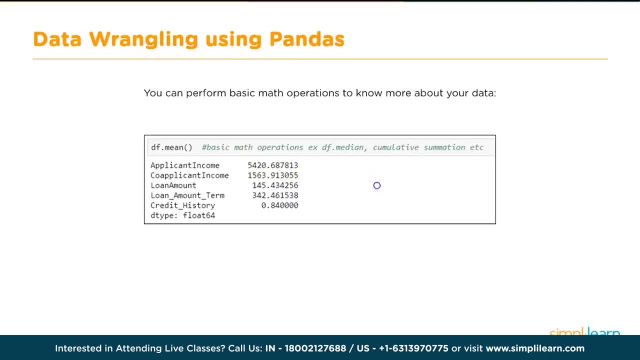 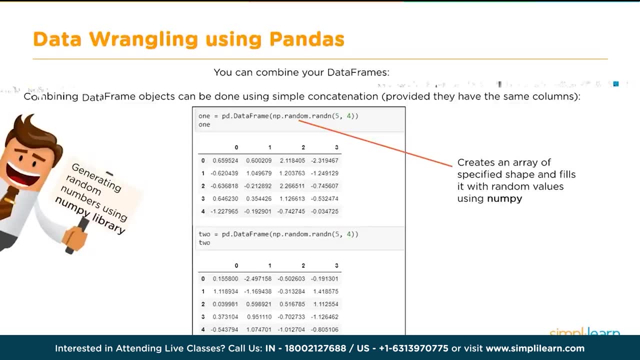 So it will display the mean values of all of those. Now, another thing that you can do is you can actually also combine data frames. So let's say you import data from one CSV file into one data frame and another CSV file into another data frame. 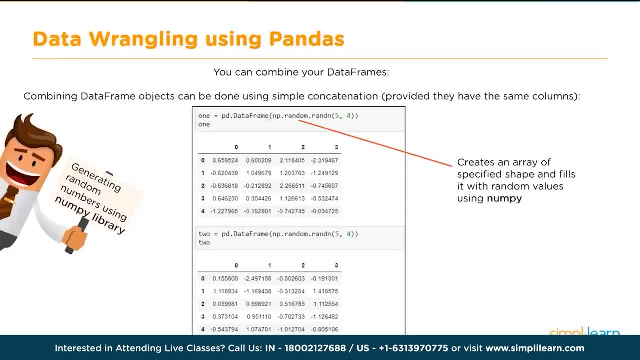 And then you want to merge these because you want to do an analysis on the entire data. Okay, one example could be that you have data in the form of CSV files, one CSV file for each month of the year: January, February, March. 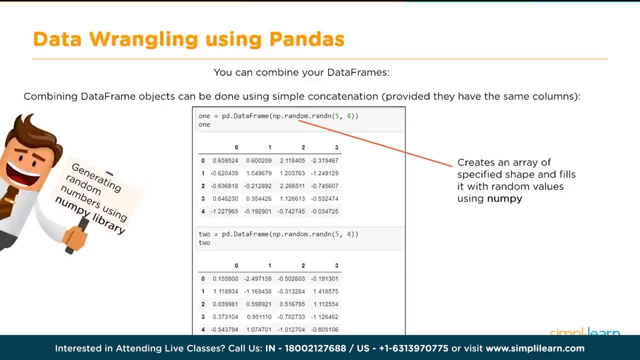 Each of these are in the form of CSV- Okay, They are in a different, So you can import them into, let's say, 12 data frames and then you can merge them together as a single data frame And then you perform your analysis on the entire data frame, or the entire data for the. 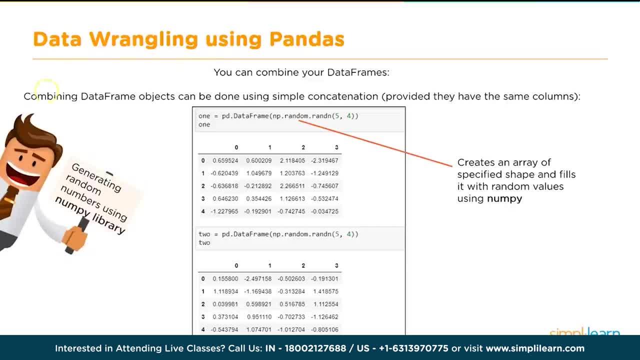 year. So that is one example. So how do we do that? This is how we do again. in this case we are not importing any data, we are just creating some random values or using some random values. So let's assume I have a data frame which is by the name one and I assign some random 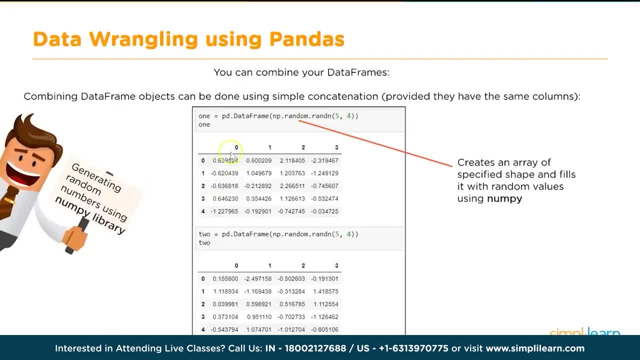 values here, which is a five by four format. So there are five rows and four columns And this is how my data frame one looks. And then I create another data frame, which is data frame two- again random numbers of the format five by four, and I have something like this: 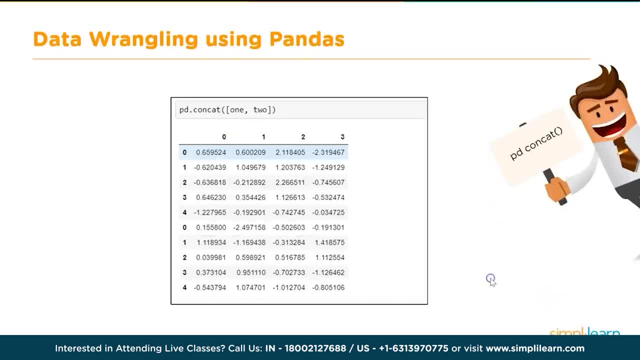 Now I want to combine these two. how do I combine these two? I can use the concatenate or concat method and I can combine these two. So PD, dot, concat and it takes the, the data frames one and two. If you have more or less data frames, you can combine these two. 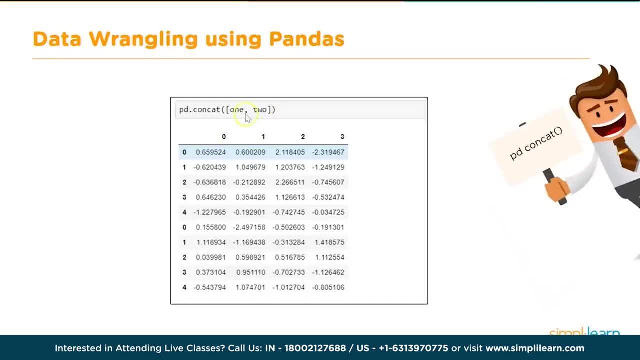 Okay, If you have more of them, you can provide them, and it will just simply add all of them, merge all of them or concatenate, whatever you call, whichever term you call it will. So, of course, we have to make sure that the structure remains the same. 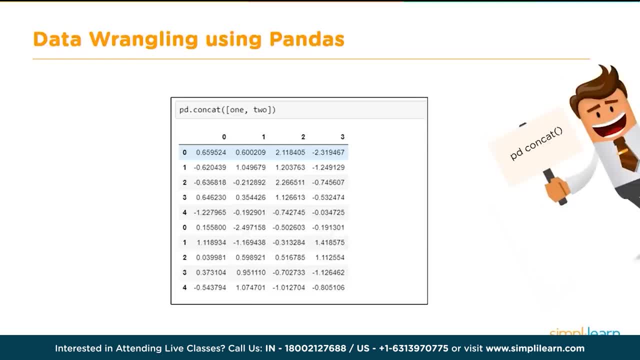 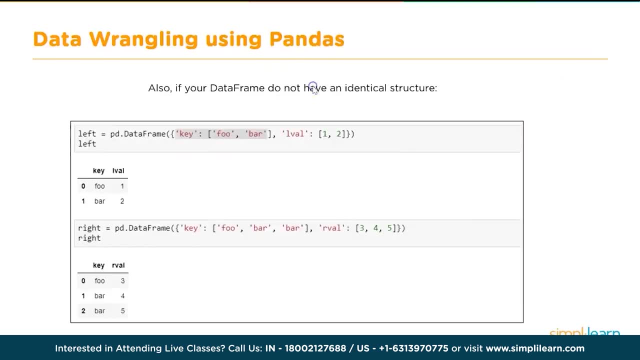 Like I said, this could be, let's say, sales data coming for 12 different months, but each of the files has the same structure. So now you can combine all of them, merge all of them using the concat method. If we have, let's say, structure is not identical, then what will happen? 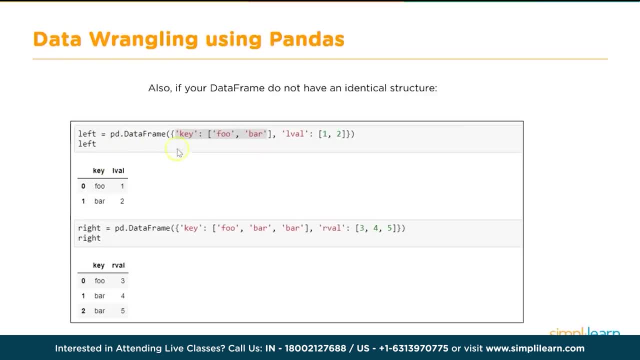 Let's say we have these two data frames: one has a column by the name key and the second column is lval, and a second data frame which has a column by the name key but the second column by the name rval, not lval. 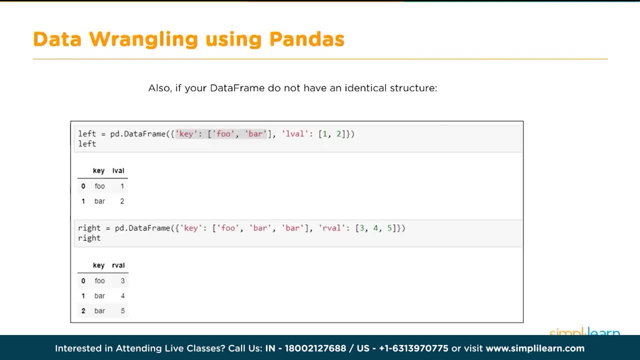 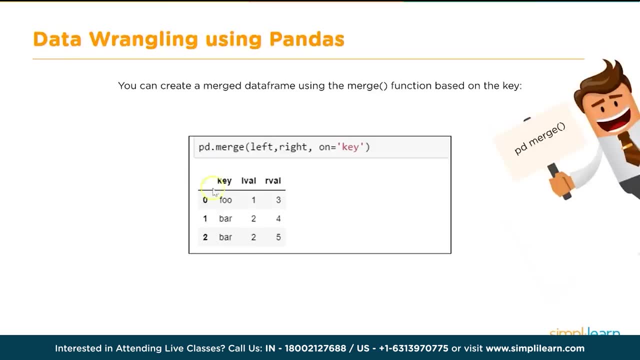 So you see here the structure is not identical, So you can still combine them, but then the way they get combined or merged is somewhat like this: So it takes the key as a common parameter between them. One common column has to be there, otherwise this will not work. 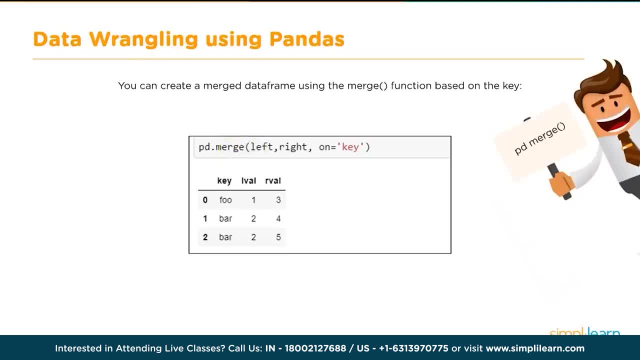 And then we have to use merge instead of concatenate, And when we do a merge then we get. the result will be in this format. What it does is it uses the key as a common thread between them and then it kind of populates. 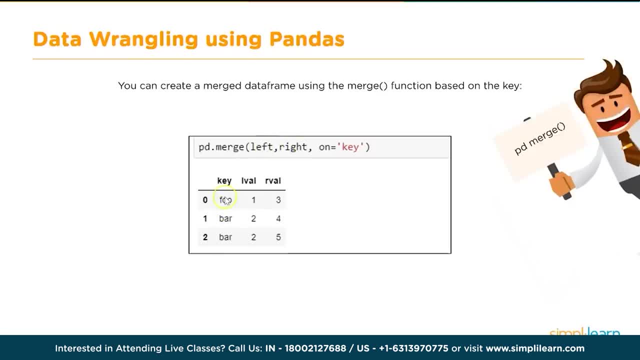 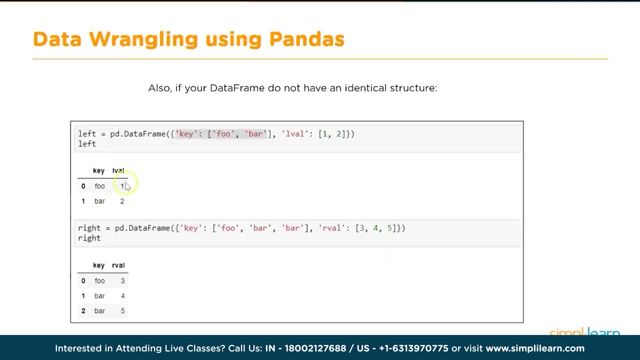 the values accordingly. So, if you see here, the first one had foo and bar for key and then it had l values of one and two, right. So if we go back, foo and bar had one and two l values. That's what we see here, one and two- whereas in the right data frame we had foo, bar and 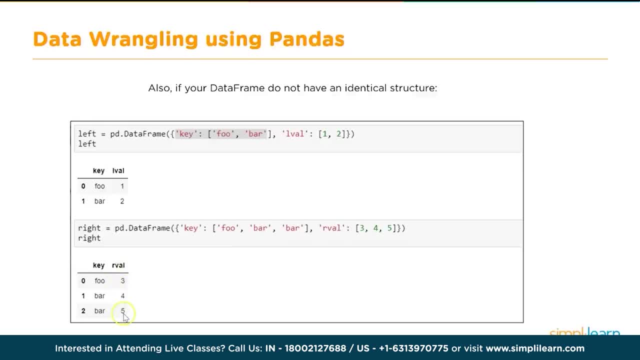 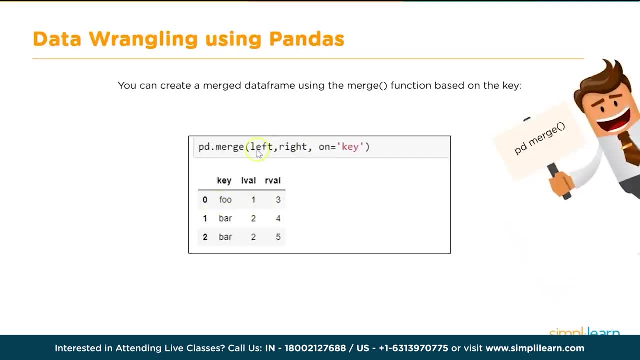 bar as a second time, and then r values are three, four and five. So what it has done for foo, it has put for the existing foo, is already existing because it has come from left. So it will just put the value of rval here, which is three. 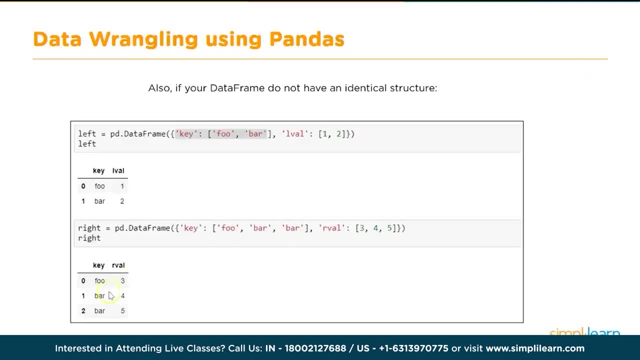 Similarly, it will put four here, because for bar, if you go back for bar, it is the value is four And one more value of bar, it will go and add this five as well. The only thing here is that this one had, for example, left, had only two values and 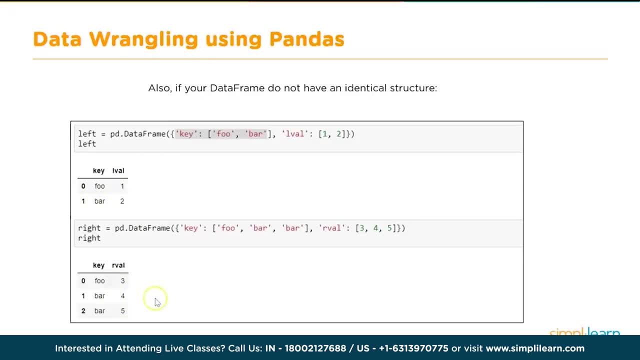 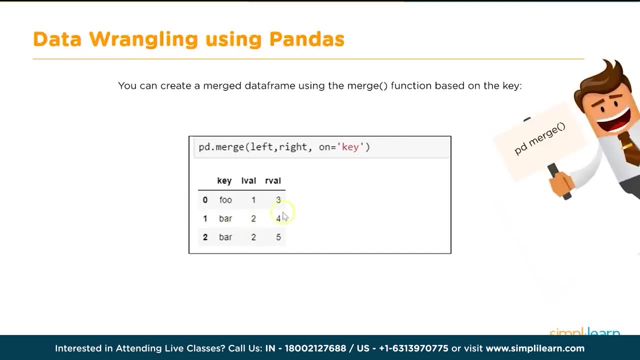 only one value for bar. But since we are appending or merging and there are two key values with the bar, therefore it will kind of repeat the value of lval here. So that's what we are seeing in this case, right? So l value appears twice, the number two appears twice, but that is because r value there. 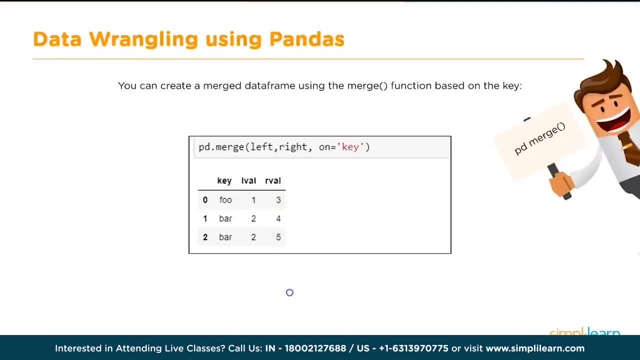 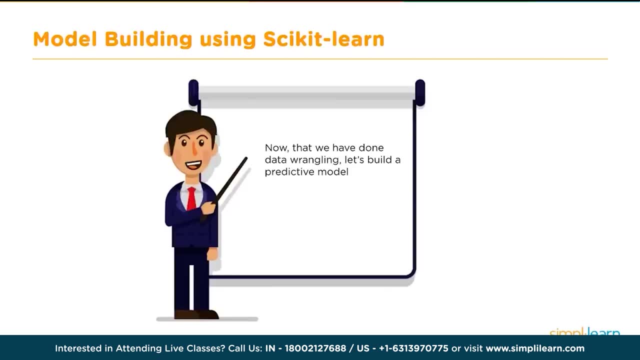 are two of them. Okay, All right. So that is how, when you don't have identical structure, that's how you merge. Now we will talk a little bit about scikit-learn. So scikit-learn is a library which is used for doing machine learning or for performing. 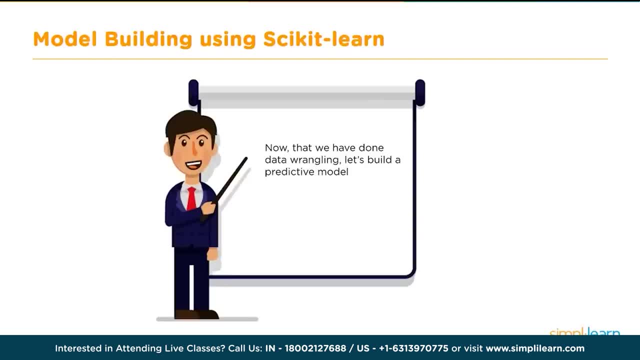 machine learning activities. So if you want to do linear regression, logistic regression and so on, there are easily usable APIs that you can call. and that's the advantage of scikit-learn And it provides a bunch of algorithms. So I think that is the good part about this library. 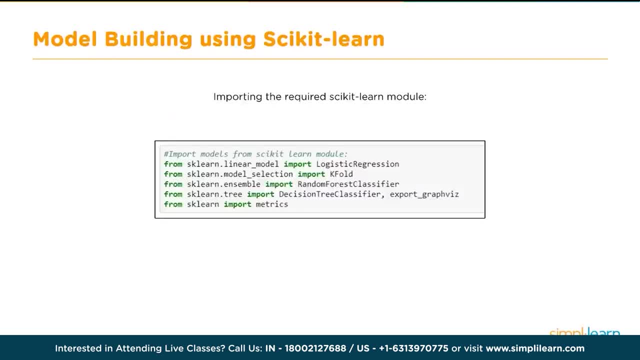 So if you want to use scikit-learn, obviously you need to import these modules, And also there are some sub modules you may have to import based on what you're trying to use, Like, for example, if we know we want to use logistic regression- again, people who are 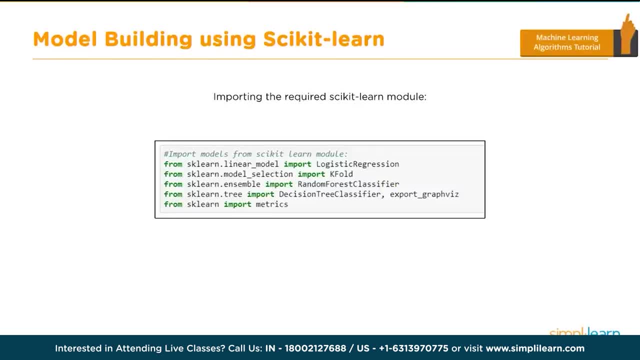 probably not very familiar with machine learning. there is a separate module for machine learning. You may want to take a look at that, but we will just touch upon the basics here. So machine learning has some algorithms like linear regression, logistic regression and random forest classification and so on. 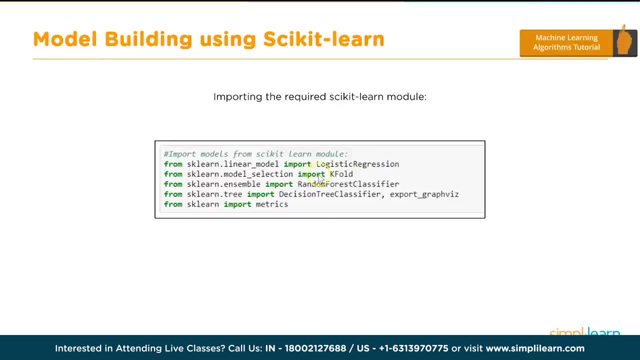 So that is what we are talking about here. So those algorithms are available And, again, if you want to use some of them, you need to import them, and from the scikit-learn library. So scikit-learn is the top level library, which is basically STL, learn right. 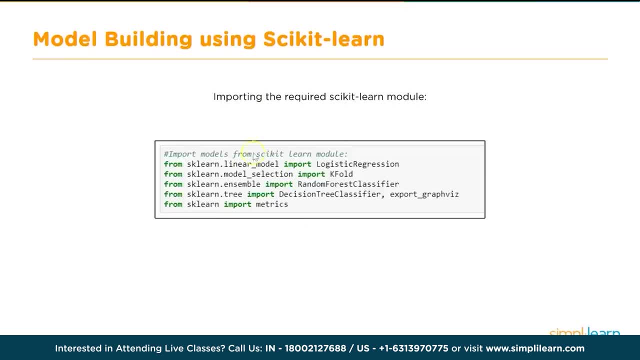 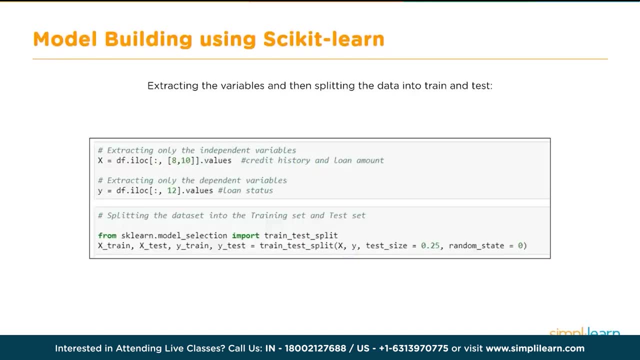 And then it has a kind of sub parts in it. you need to import those based on what exactly you will be. So let's take an example: as we move and we will see that whenever we perform some machine learning activity, those of you who are familiar with machine learning will already know this. 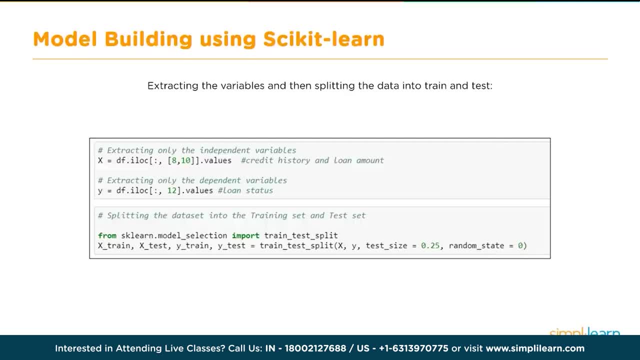 We split our labeled data into two parts: training and test. Now, there are multiple ways of splitting this data. How do we either? some people do it like 50- 50, some people do it 80, 20, which is training is 80 and test it is 20, and so on. 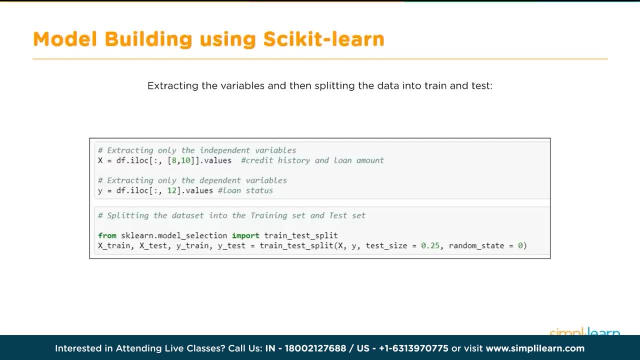 So it is individual preference. There are no hard and fast rules. By and large, we have seen that training data set is larger than the test data set And again, we will probably not go into details of why do we do this at this point. but that's. 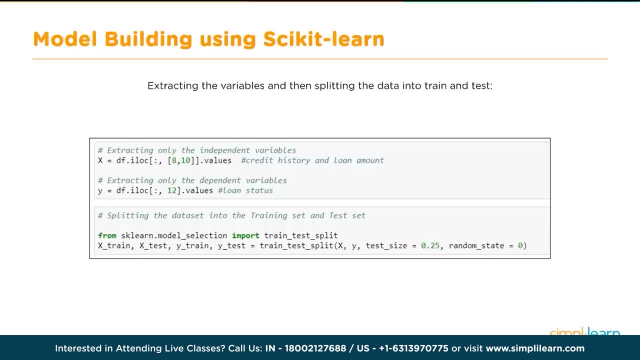 one of the steps in machine learning. So scikit-learn offers a readily available method to do this, which is train test split. All right, So in this example, let's say we are taking the values X and Y are our values. 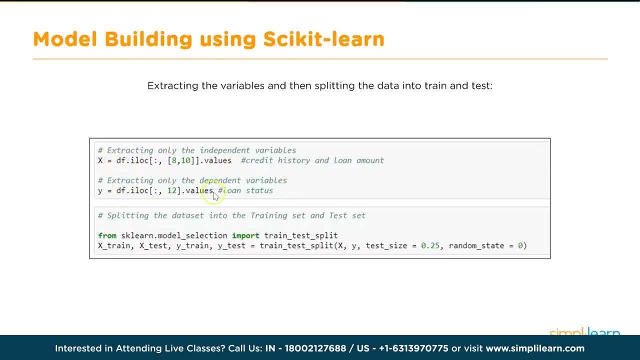 X is the independent variables and Y is our dependent variable And we are using these two. and then I want to split this into train and test data. So what do we do? We import the train test split submodule from within scikit-learn, which is sklearn, right. 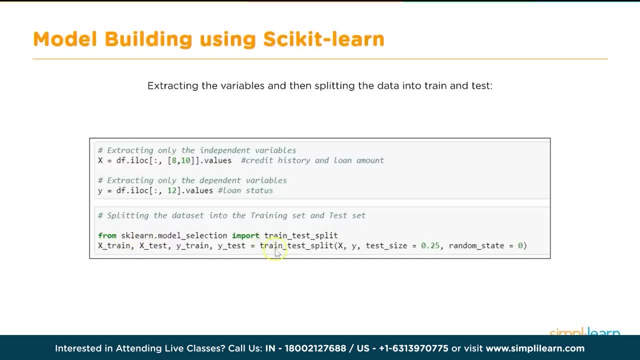 So within that we import train test split and then you call this train test split method or function or whatever you call it, and pass the data. So X is the all the values of the independent variables and Y is our labels. Okay, And then you specify what should be your size of the test data. 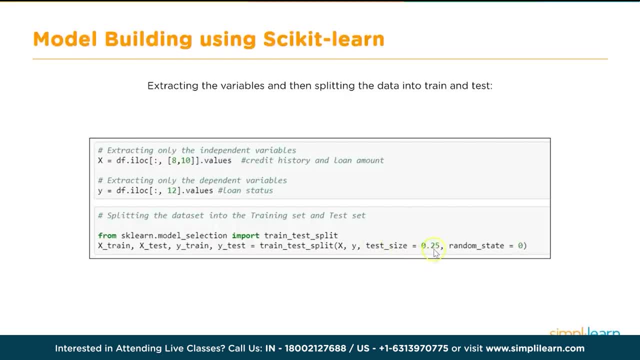 So only one you need to specify. So if you say test size is 0.25, it is understood that train size will be 0.75. So you're telling what should be the ratio of the split. So technically it doesn't nothing prevents you from giving whatever you like here. 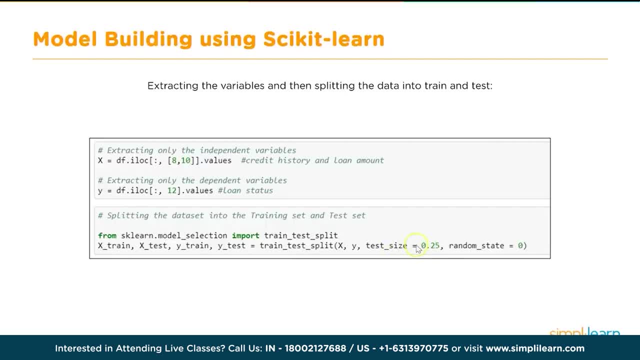 So you can give test as 80 and train as 20.. So whichever way- but then there's normal practices You will have- the training data set would be larger than the test data set. Then typically it would be 80,, 20,, 75,, 25 or 65, 35, something like that. 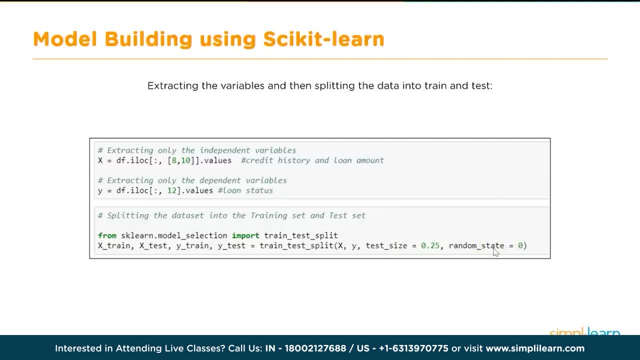 Right, So that is the second parameter. And this is just to say that you know the data has to be randomly split, So it shouldn't be like you take the first 75% and put it in training and then the next 25% and put it in tests, so that so such a thing shouldn't happen. 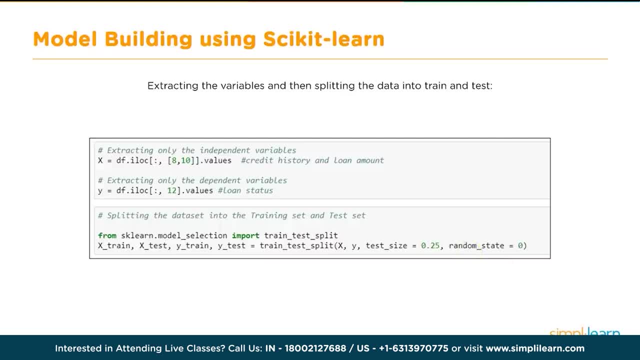 So we first set the state random state, so that the splitting is done in a very random way, So they are randomly picked up the data and then put it into training, Training and test, And then this results in these four data frames, So X- train and X test, and Y- train and Y test. 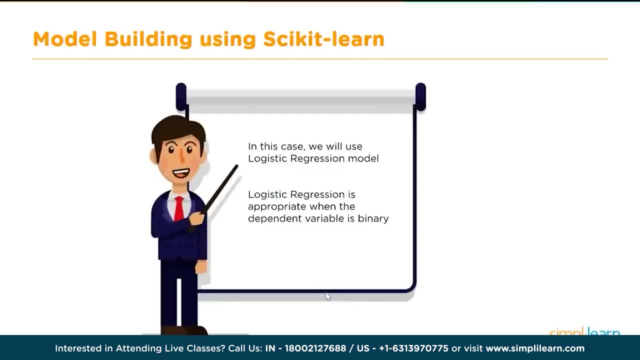 Okay, So that is basically the result. it will. Now that the splitting is done, let's see how to implement or execute logistic regression. So in logistic regression, what we try to do is try to develop a model which will classify the data. 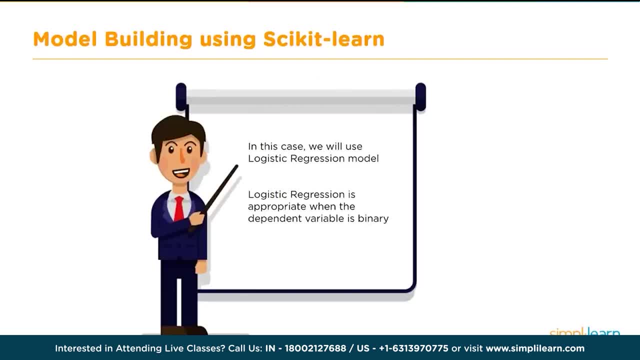 Logistic regression is an algorithm for supervising Or supervised learning, for performing classification. So logistic regression is for classification and usually it is binary classification. So binary classification means there are two classes, So either like a yes, no or, for example, customer will buy or will not buy. 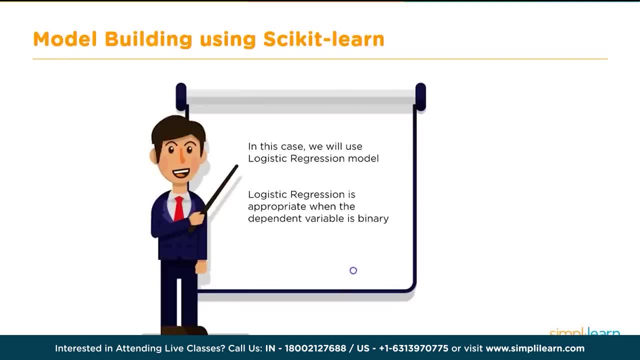 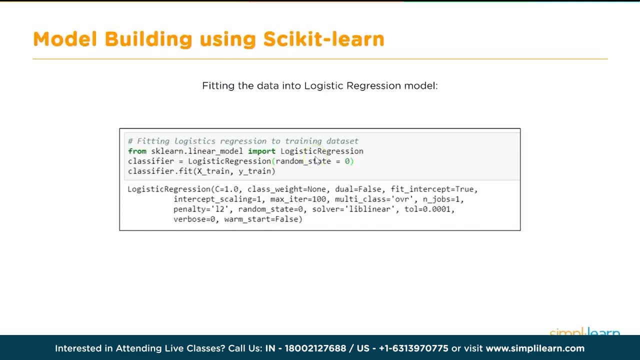 So that is a binary classification. So that's where we use logistic regression. So let's take a look at the code: how to implement something like that using scikit-learn. So the first thing is to import this logistic regression submodule or subclass, whatever. 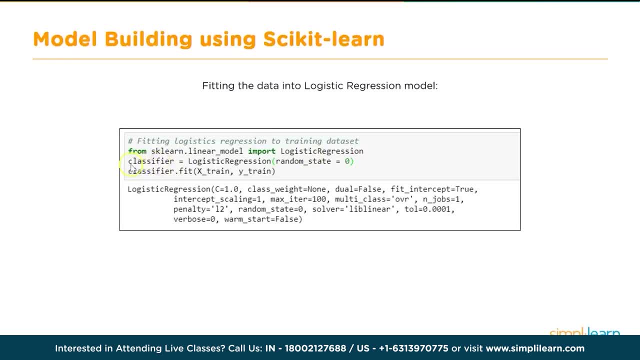 you call it And then create an instance of that. So our object is classifier. So we are creating an object by the name. This is a name. by the way, you can give any name. In our case we are saying classifier. we say classifier is equal to logistic regression. 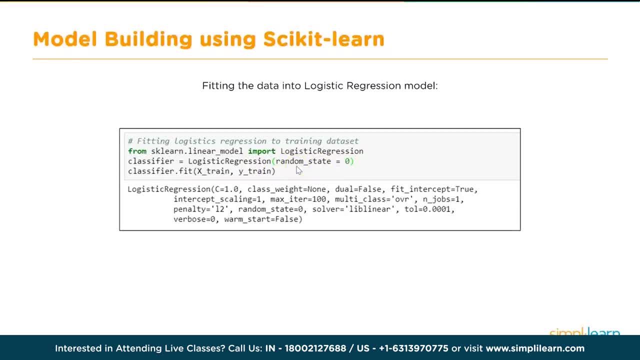 So we are creating an instance of the logistic regression variable or class or whatever. Okay, And you can pass a variable or a parameter rather, which is the random state is equal to zero And once you create the object, which in our case is named classifier, 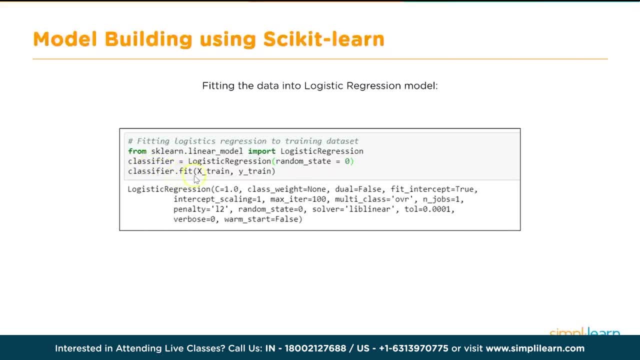 You can then train the object by calling the method fit. So- this is important to note- we don't call any. there is no method like train here, but we call what is known, as there is a method called fit. So you are basically, by calling the fit method, you are training this model. 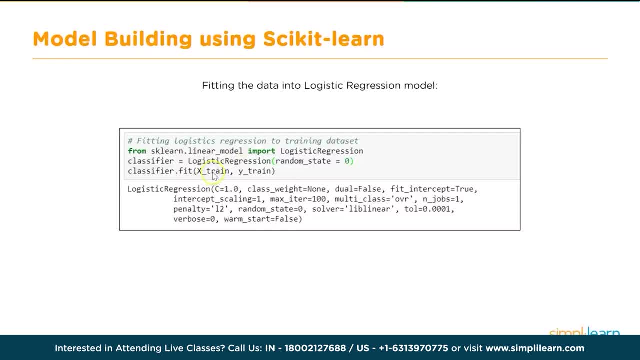 And in order to train the model, you need to pass the training data set. So X underscore train is your independent variables, the set of independent variables, and Y underscore train is your dependent variable Or the label. So you pass both of these and call the fit function or fit method, which will actually 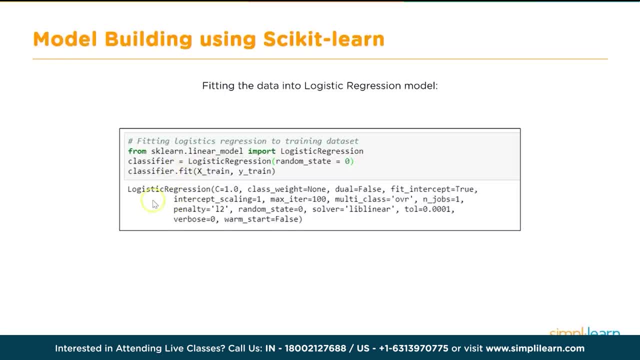 result in the training of this model classifier. Now, this is basically showing what are the possible parameters that can be passed or initiated when we are calling the logistic or the instance of logistic regression. So this is, but you can also look up the help file if you have installed Python. 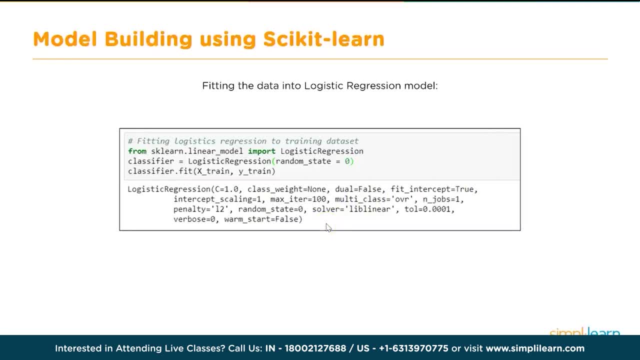 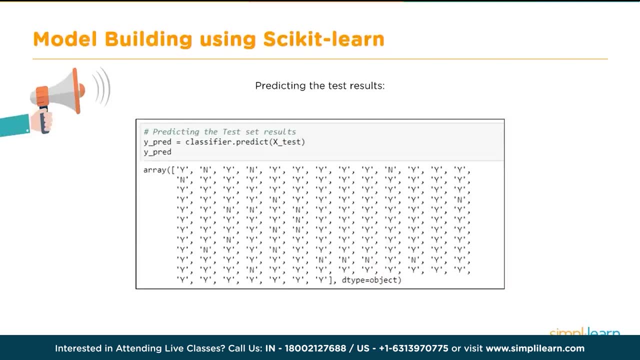 So some of these are very intuitive, but some you may want to take a look at the details of what exactly they do. All right, So moving on. once we train the model by calling fit, then the next step is to test our model. 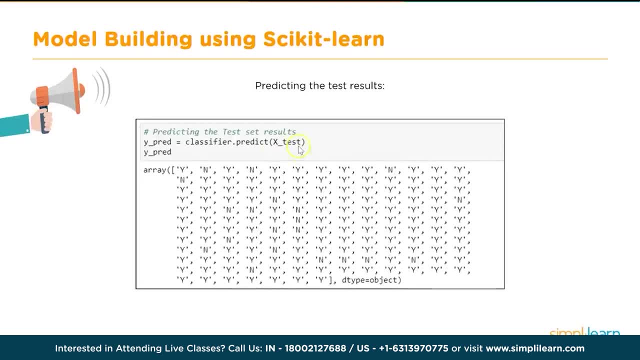 So this is where we will use the test data. You need to pay attention here. Here I am calling. So there are two things. One is, in order to test our data, we have to actually call what is known as the method, known as predict right. 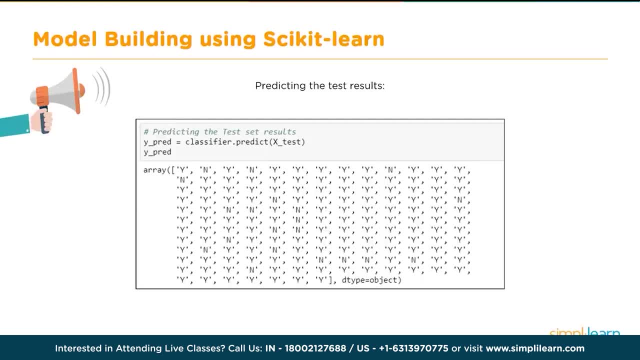 So here, this is where so the training is done. Now is the time for inference, isn't it? So we have the model. Now we want to check whether our model is working correctly, Okay Or not. So what do you do? 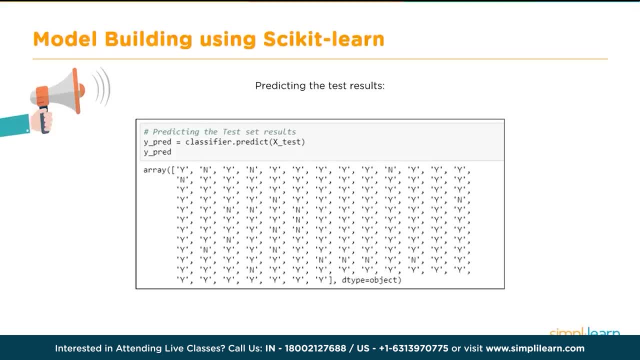 You have your test data, Remember, we split it. 25% of our data was stored here, right? We split it into test and training So that 25% of the data we pass to and call the method predict, so that the model will. 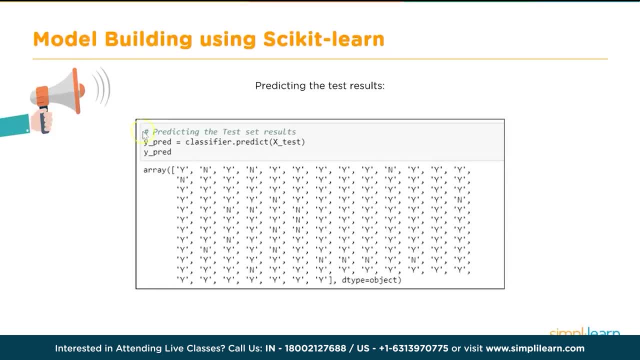 now predict the values for Y, right? So that's why here we are calling it as Y underscore: predict. And if we display here, as I said, this is a logistic regression which is basically binary classification, So it gives us the results like yes or no in this particular case. 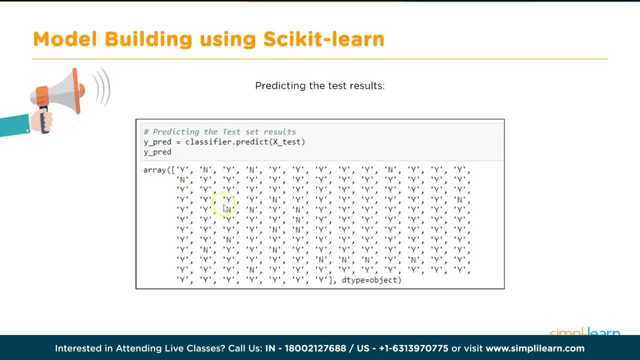 And then you can. so this is what the model has predicted or model has classified now. But we also know we already have the labels for this. So we need to compare with the existing labels, with the known labels, whether this classification is correct or not. 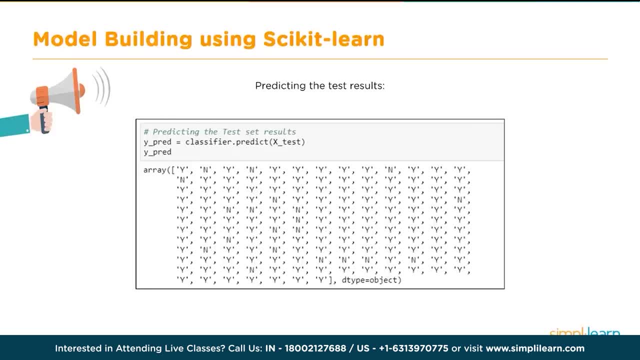 So that is, where is the next step, which is basically calculating the accuracy, and so on, will come into play. Okay, So in this case, the first thing, the most important thing to notice- we do the prediction using predict, And here we are passing X underscore test. 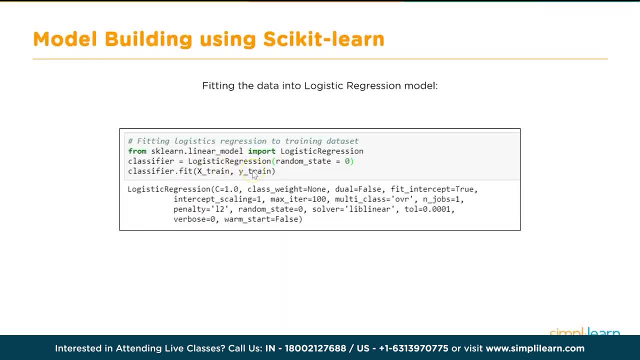 And not train right, In this case we did X and Y train. So again one more point to be noted here: In case of training, we will pass both the independent variables and also the dependent variables, because the system has to, internally, it has to verify. 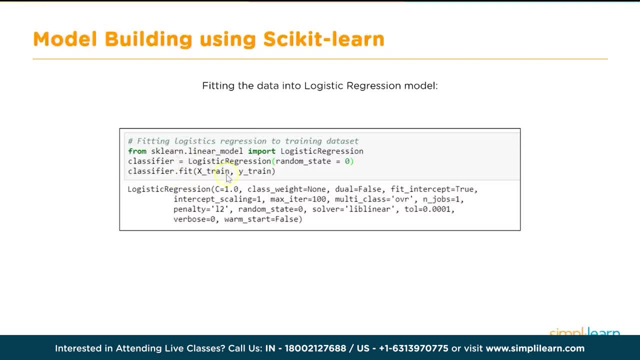 That is what is the training process. So what it will do. it will take the X values. it will try to come up with the Y value and compare with the actual Y value, right? So that is what is the training method. So that's why we have to pass both X as well as Y. 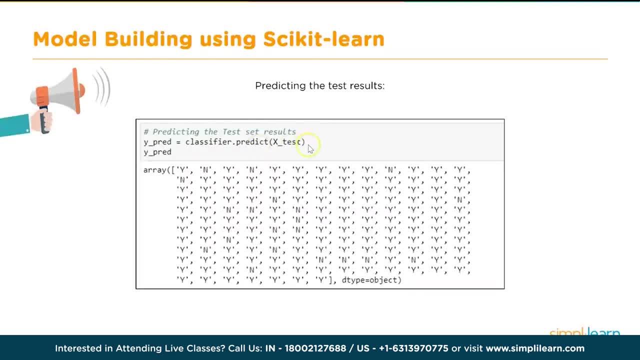 Whereas in case of predict- Okay, In case of predict, we don't pass both. We only pass because we are pretending as if this is the actual data. So in actual data, you will not have the labels, isn't it? So we are just passing the independent variables and the system will then come up with the Y. 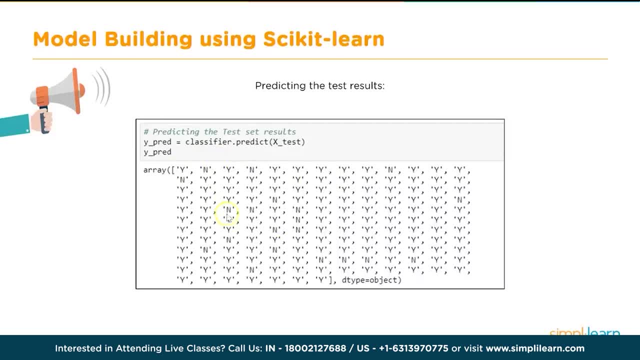 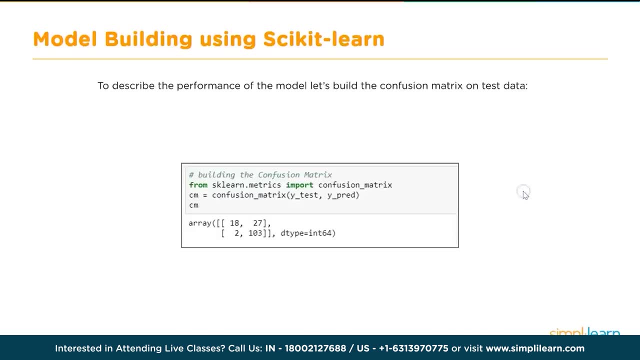 values, which we will then, okay, remember. we also know the actual value, So we will compare this with the actual values and we will find out whether, how accurate the model is. So how do we do that? We use what is known as a confusion matrix. 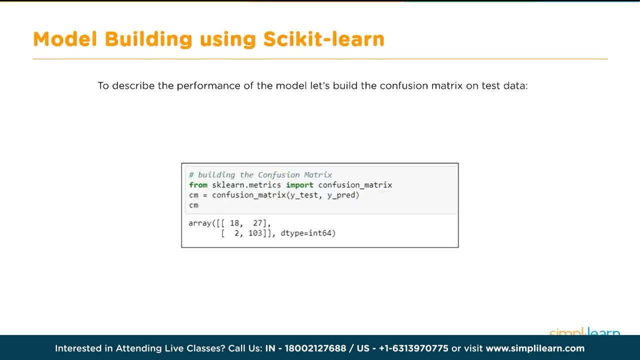 So this is also readily applicable In the Python library. So we import this confusion matrix and some of you who already know machine learning will find this familiar. but those who are new to machine learning, this confusion matrix is nothing but this matrix, this kind of a matrix which basically tells how many of 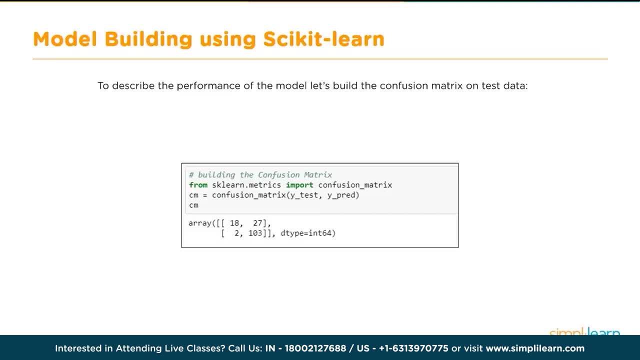 them are correctly predicted and how many of them are incorrectly predicted. So the some of the characteristics. let's quickly spend some time on this confusion matrix itself. This the total numbers out here. These are just the numbers. These are like number of observations. 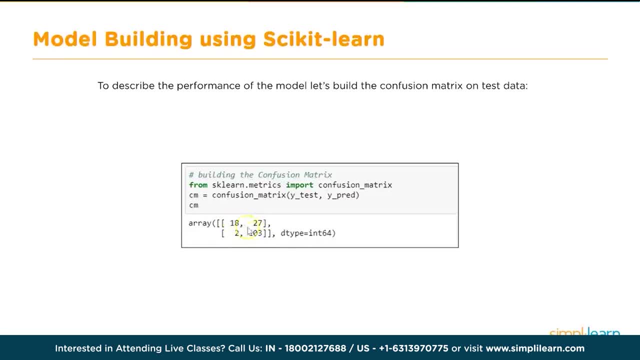 Then the accuracy is considered to be highest. when the the numbers, or the sum of the numbers across the diagonals is maximum, Okay, And the numbers outside of the diagonal should be minimum. So which means that if this model was a hundred percent accurate, then the sum of these two 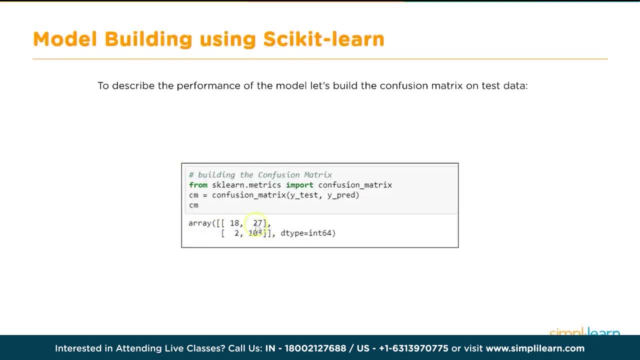 there would have been only numbers in these two along the diagonal, This would have been zero and this would have been zero. Okay, So that is like a hundred percent accurate model. that is very rare, But just that you are aware. So just to give an idea. 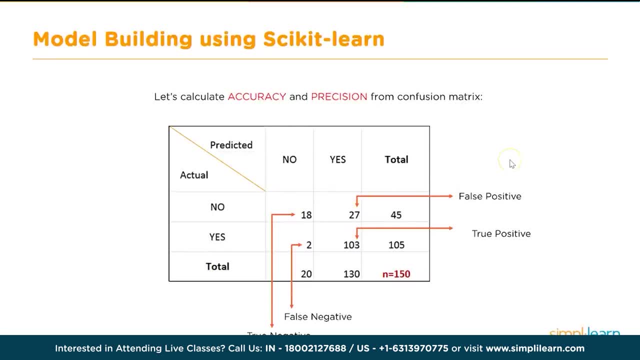 Okay, All right. So once you have the confusion matrix, you then try to calculate the accuracy, which is in a percentage. So there are two things that we can do from a confusion matrix or that we can calculate from a confusion matrix. One is the accuracy and the other is the precision. 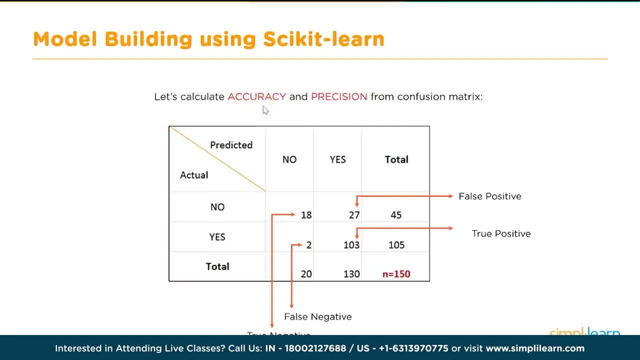 What is the accuracy? Accuracy is basically a measure of how many of the observations have been correctly predicted. Okay, So let's say this is a little bit more detailed view of the confusion matrix. Okay, So let's say this is a little bit more detailed view of the confusion matrix. 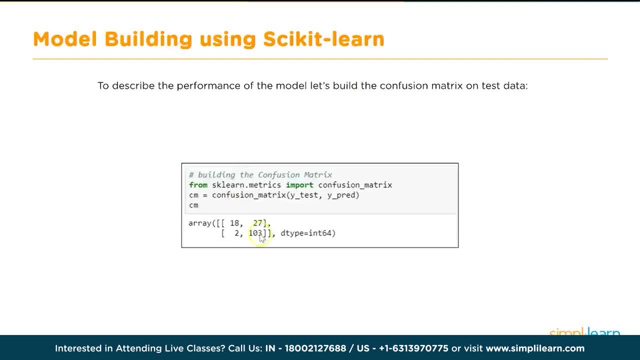 Okay, So let's say this is a little bit more detailed view of the confusion matrix. It looks very similar like as we saw in this case, right? So this is a two by two matrix. That's what we're seeing here: 18, 27, 2, 1,, 0, 3.. 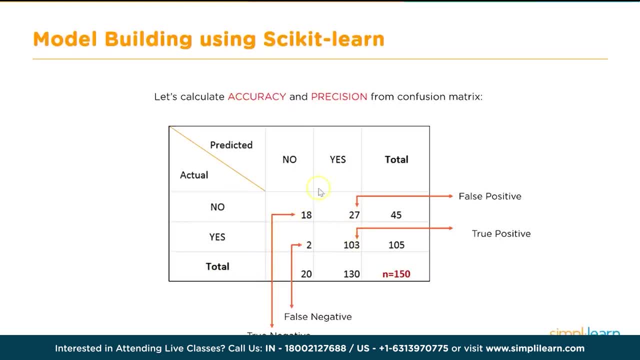 So 18,, 27,, 2,, 1,, 0,, 3.. Now, but what are these values? That is, what is kind of. the labels are shown here in this. So there are altogether 150 observations. So, as I said, the sum of all these four right. 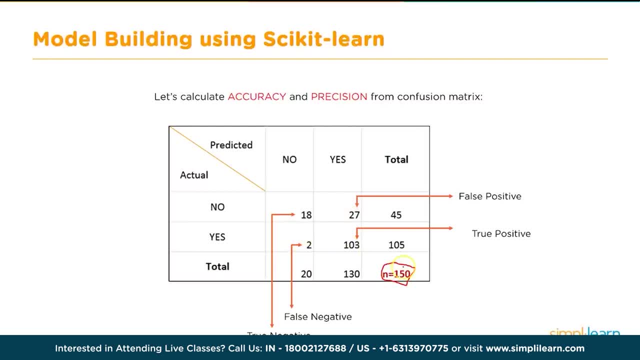 18 plus 27 plus 1,, 0,, 3 plus 2 is equal to 150.. That's the first thing we have to observe. The sum of all these values will be equal to the sum of test observations. number of. 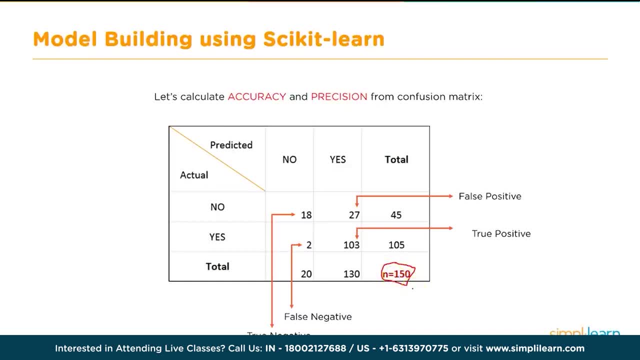 test observations. We have 150 test observations Because, remember we had about 500, we split that into 25, 75. So that is why we have 150 here and I think, 350 in the training data set. Okay, 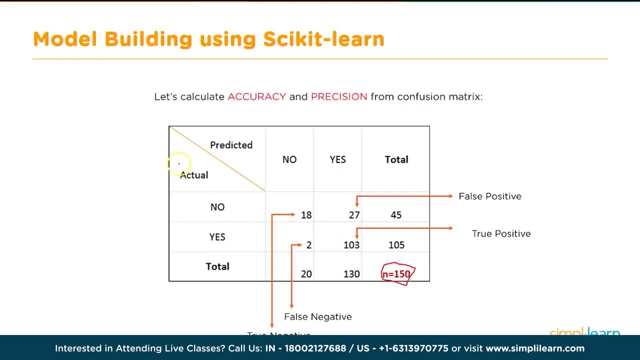 So that we get the numbers correct. So that's the first thing. Now the next thing is: let's take a look at the actual values. This view is the actual view, So there are actually right In the actual data. 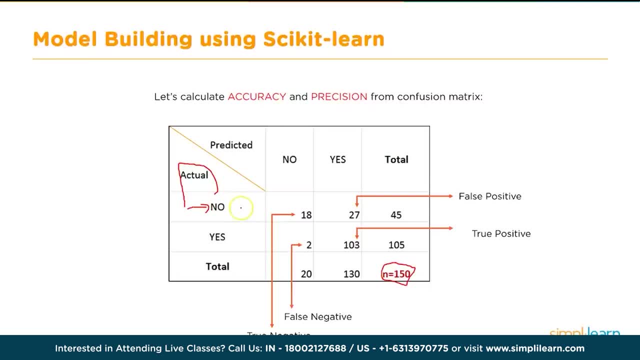 We have labels yes and no. So, as per the actual data, there are 45 observations tagged as no And similarly, there are 105 observations that are tagged as yes or labeled as yes. Okay, Now I know for the first time. when you're seeing this, it may be a little confusing. 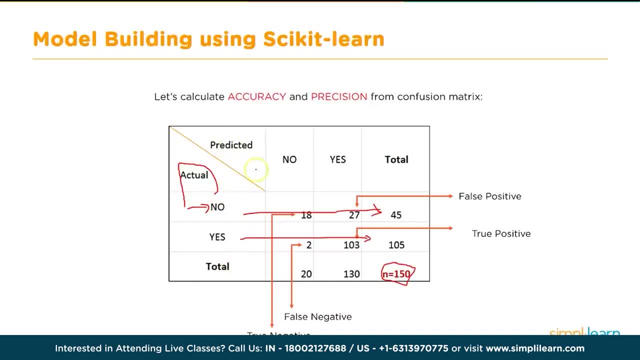 but just stay with me, Okay. So this is the actual part of it, And this side tells us the predicted part of it. So our model has predicted- and it has totally predicted- 20 of them as no right. So that is what this is: totally 20 of them. 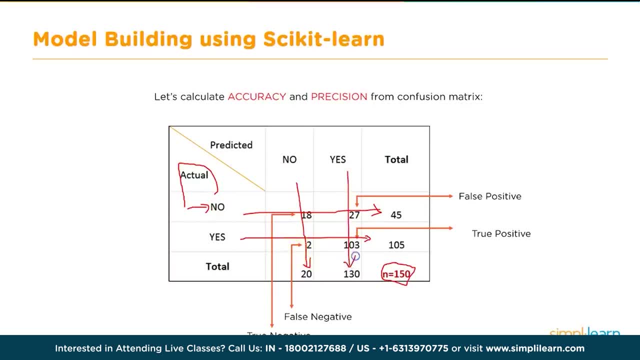 It has predicted as no and it has predicted 130 of them as yes. Okay, I hope this part is clear. So before we go into the middle part, let us first understand what exactly are these numbers So? actually tagged as no, there are 45 total. actually tagged as yes, there are 105, and. 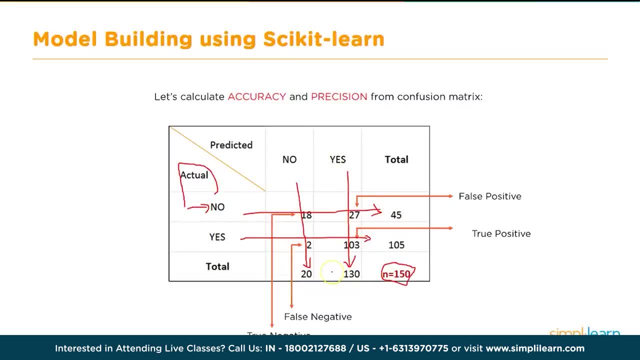 predicted: no, there are 20. predicted as yes, there are 130.. This is the result from our model. Okay, And this is the actual value, which we already know, because this is our label data. That is the first thing. 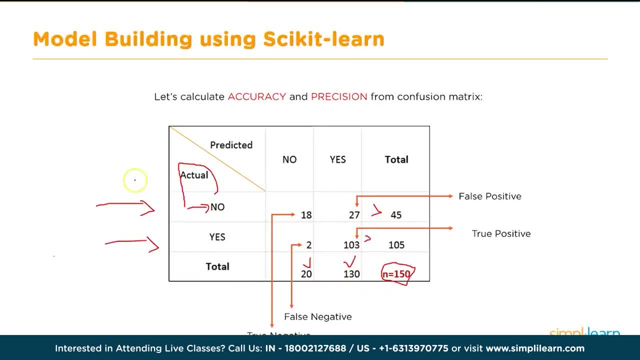 Now, now let us take a look at each of these individually. Okay, Now, what are the options we have? once again, Okay, So now what is happening here? Let us look at these, these values. So this 18 says that these are actually tagged as no and the model is also predicted as: 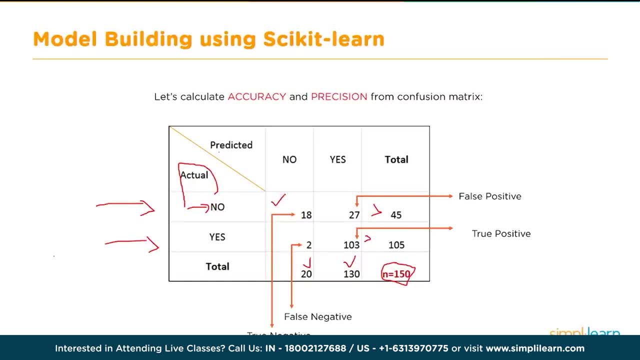 no, which means this is what is known as a true positive right, Or true negative, Sorry Right, Which means that our model, as predicted, is it correctly. It is negative because it says no. So and it has also predicted no. 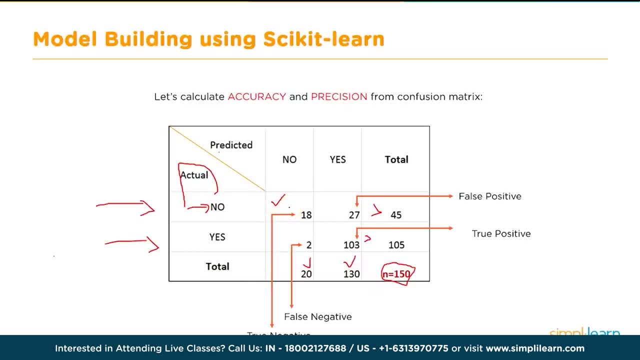 So it is known as what is known as true, negative. Okay, Now let us come to this side of it. That way, we are talking about the diagonal. Remember, I said most of the value should be in the diagonal. Okay, So that means these 18 are correctly tagged, they are labeled as no and our model is predicted. 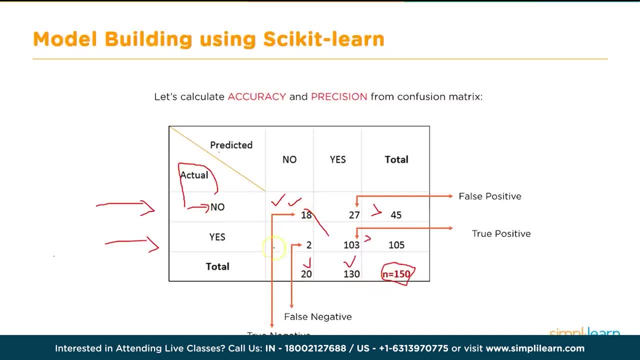 as no, So these are correctly tagged and these are known as true, negative, Okay. Similarly, if we come diagonally down, there are 103 observations which are labeled as yes, actual value is as and our model is also predicted as yes, and these are known. 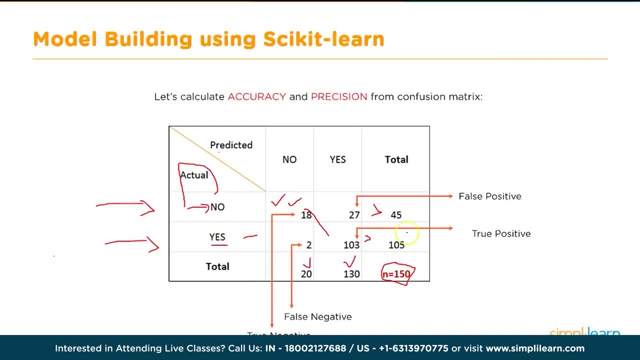 as true, positive values. positive because of this, yes, Okay, Right, So what is important is- this is true, This is also true, So we have to make sure that the maximum number of values are in the true section. Okay, True, positive and true, negative. 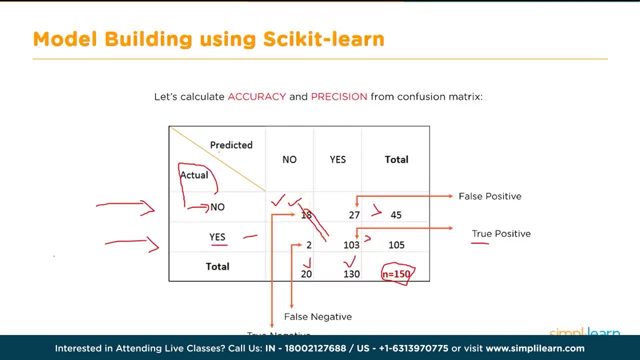 That's the reason I said The sum along the diagonal should be maximum. Now let's see if our model was 100% accurate. This sum, in this case it is only 103 plus 103 plus 18, which is 121.. 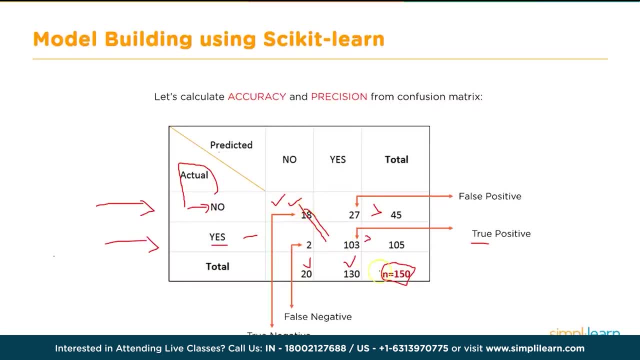 But if our model was accurate, the sum of these two would have been 150.. That means it's a perfect model. Okay, All right, Now what else? Since we covered these two, let's also cover these two. So here, this says that 27 of them were actually labeled. no, but our model is predicted as: 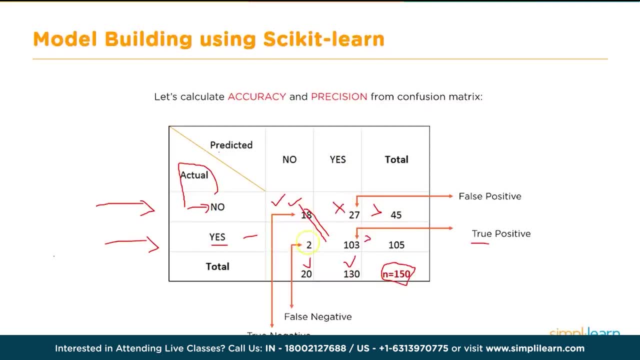 yes, That means this is wrong, Right. Similarly, these are two of them where the actual value is yes, but our model is predicted as no. That means it's a wrong prediction. So you get the point. So, therefore, along the diagonals are the correct values, whereas in other places it. 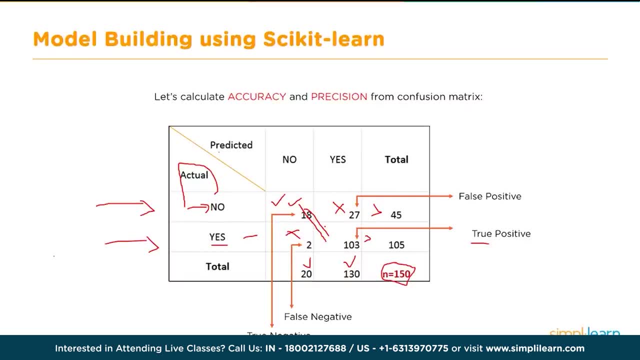 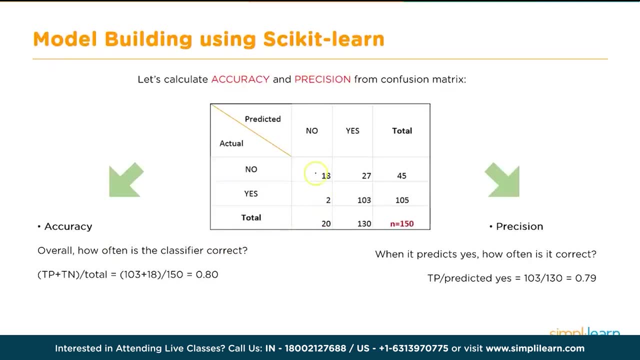 is all wrong values or wrong predictions. Okay, Now how do we calculate accuracy from this information? So the way to calculate accuracy is: so we'd say: okay, there are total observations are 150.. And what are the correctly predicted values? 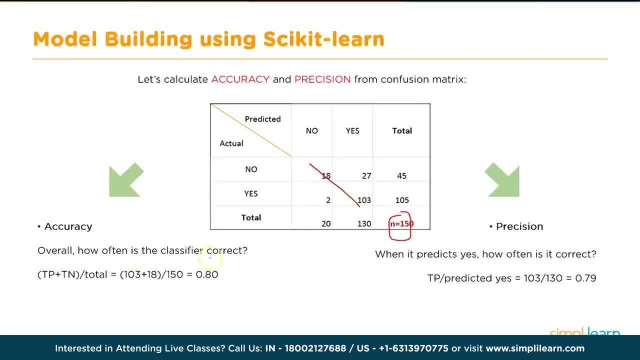 These are the correctly predicted values, which is 18 plus 103.. So this will give us our accuracy. So 103 plus 18, which is 121, divided by our total observations, which is 150, is our accuracy, which is 0.8, or we can say it is 80%. 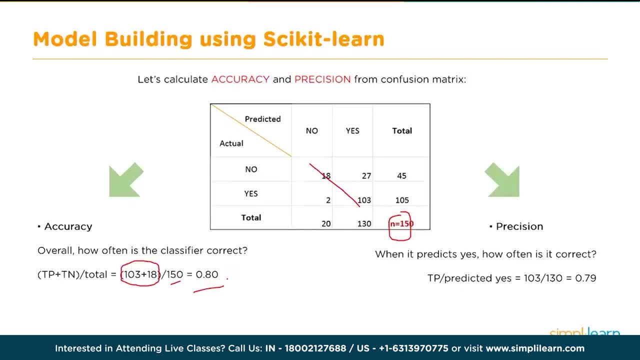 Okay, Now there is another concept called precision. So precision is given by the formula true positives divided by the predicted accuracy. Okay, What do we mean by that? Totally predicted positives? Okay, What do we mean by that? Which are the true positives here? 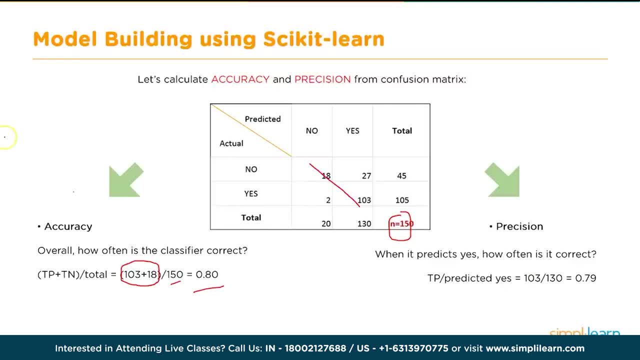 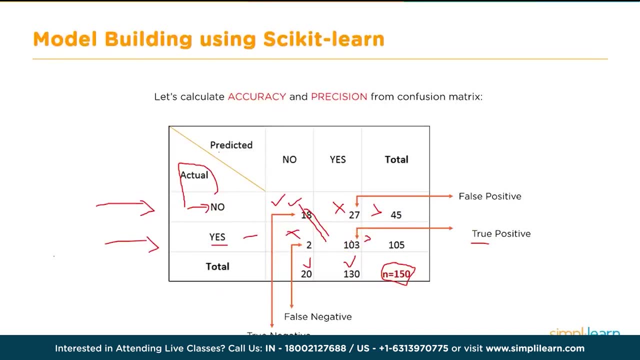 Remember which are the true positives. We just recall, we just talked in the previous slide which are the true positives you see here. So this 103 are the true positives, which means that the value is positive. actual value is positive, predicted value is also positive. 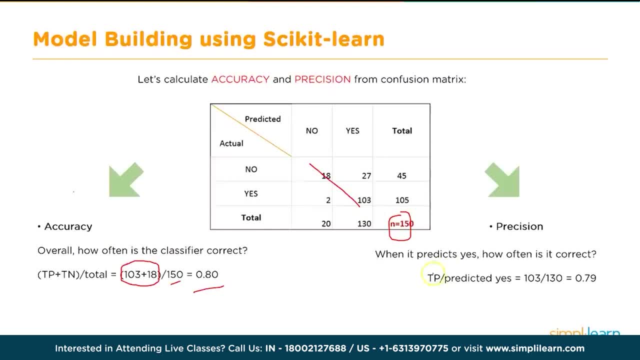 So that's why it's called a true positive. So 103 divided by: so that is our true positive: 103 divided by totally predicted as yes. Now, How many of them have been predicted as yes? You remember, 130 of them have altogether been predicted as yes. 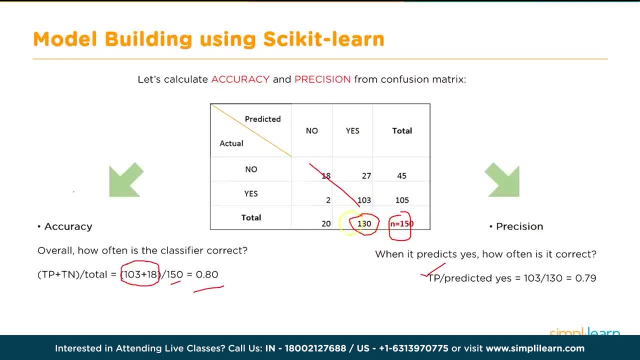 Not that they are correctly predicted- only 103 have been correctly predicted- But 130 of them have been predicted as yes. So precision is basically the ratio of these two out of the totally predicted. how many of them are actually true? That ratio? 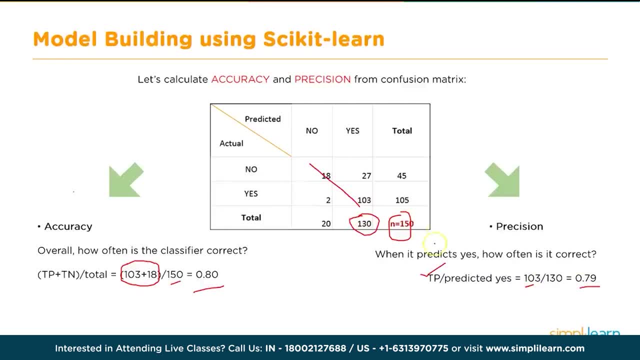 So 103 by 130, which is again about 80%, is the precision. That's how you calculate precision. So this is just a simple formula, Okay, That you need to remember. So accuracy is: you need to take total of true positive and true negative divided by the total. 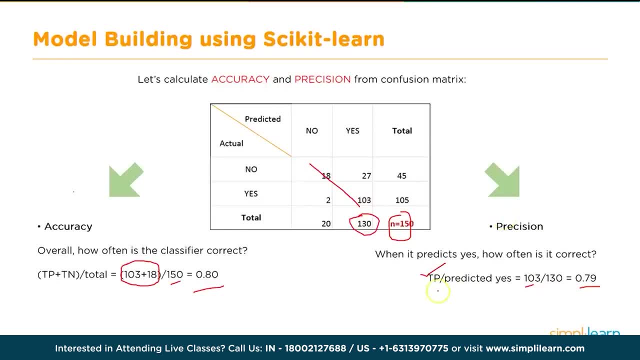 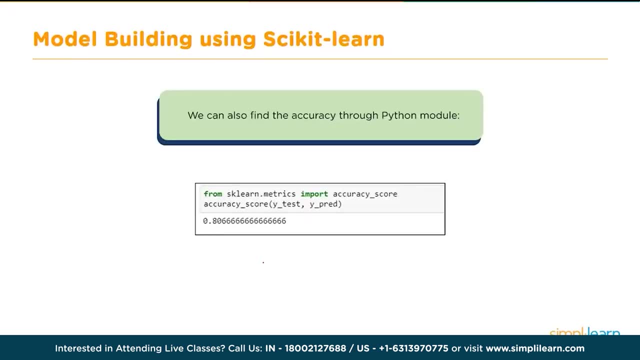 number of observations, whereas precision is true positives divided by the totally predicted positives. Okay, So that is our accuracy and precision. Now, what we did. the accuracy calculation was manual, but we can also use some libraries which are already existing and the functions within that library. 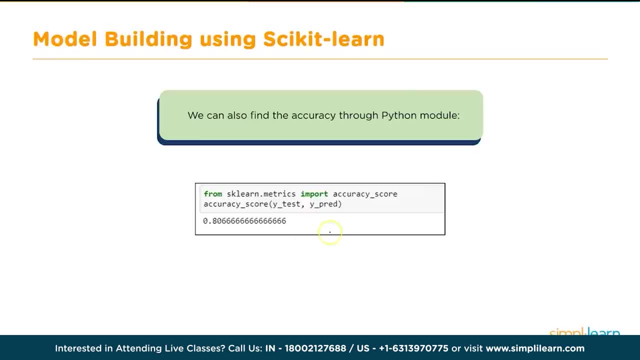 So scikit-learn provides one such method. So, for example, accuracy underscore score, This is one such method. So if you use that and pass your test and predicted values, only the why you need to pass right The dependent variable values. 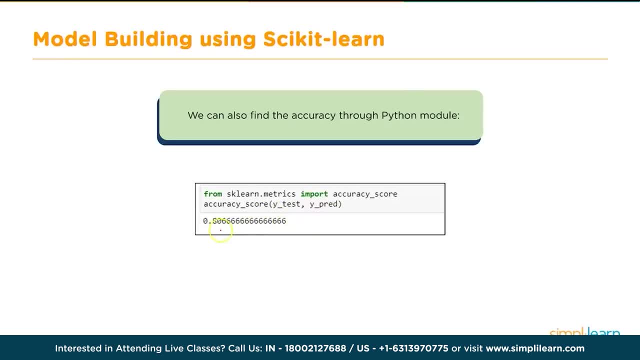 So if you pass that, it will calculate it for you. So in this case again, as you can see, it still calculates the same, which is 80%, which we have seen here as well. Okay, So this can be done using the method. 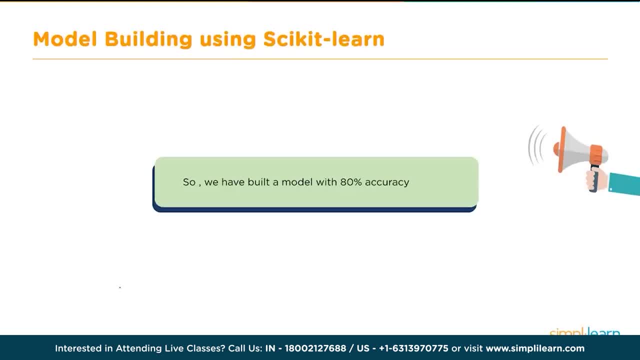 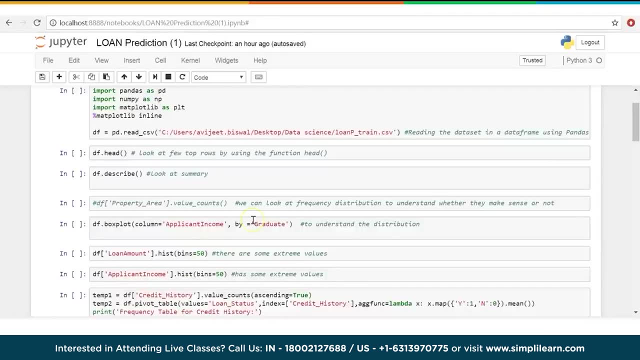 Great. So that's pretty much what we have done here. before we conclude, let me take you into the code. Let me show you how it actually looks. Okay, So this is our code. Let me run it. Okay, One by one. 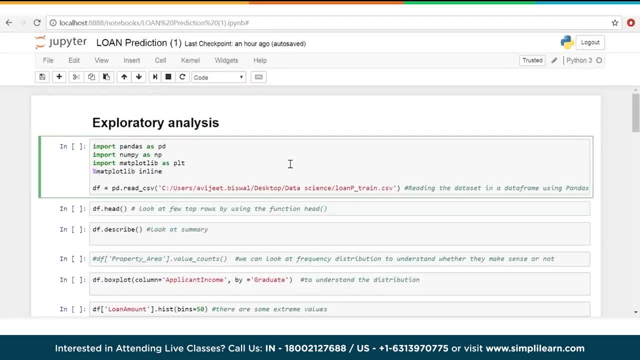 We have already seen most of the steps and slides So I will, but I will run this in the actual Jupyter notebook Some of you, if you're not yet familiar with Jupyter notebook. again, there are other videos we created on how to install Jupyter notebook and how to set up Jupyter notebook and so 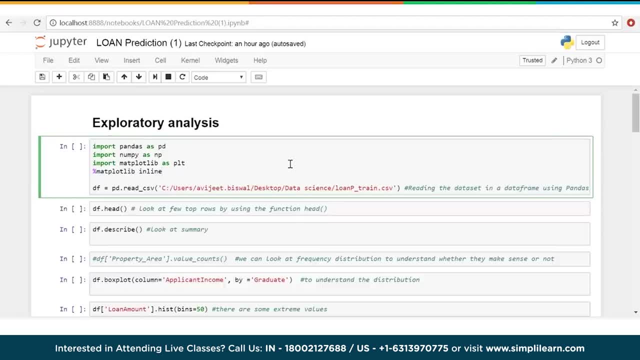 on In this tutorial also we there was one slide on how to install Python and Jupyter notebook. If you have not yet done, please do that, so that then you can actually walk through this code while you're watching this. Okay. 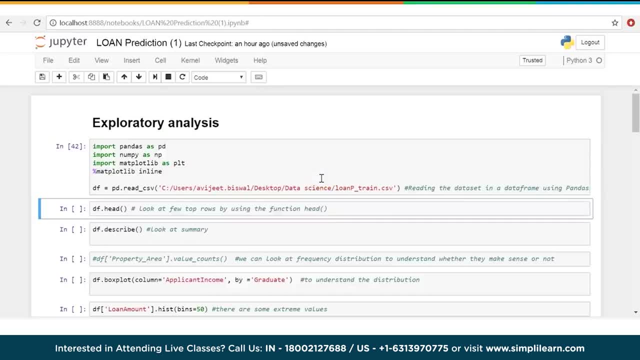 So what are we doing here? We are importing the libraries, required libraries, recall. here we have pandas, we have NumPy and for a visualization we have matplotlib, And this line is basically reading the CSV file. So we have the CSV file locally on our local drive and this is where I'm checking the 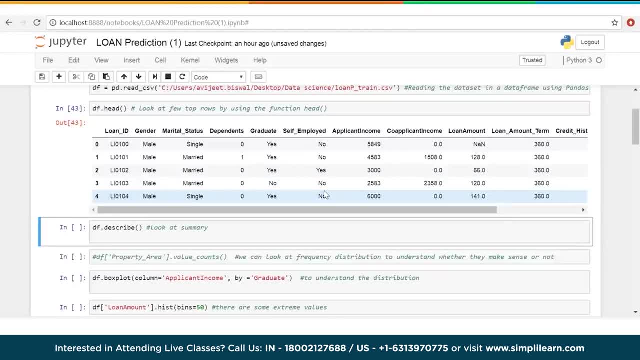 data. So I'm starting with my exploratory analysis how the data is looking. So it looks good. There are no major missing values or anything like that. So it will display all the columns and it will show me the first five rows when I'm 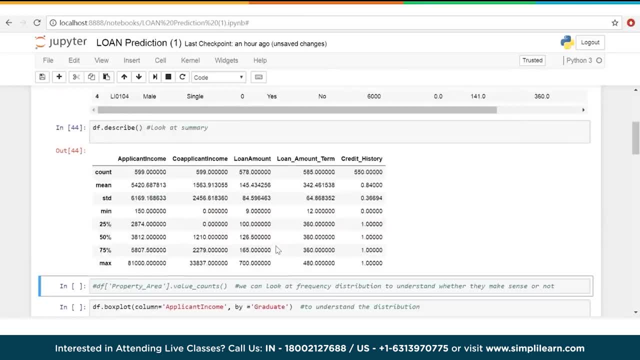 using this head function, And then I want to see a kind of a summary of all the each of the numerical columns. So that's what I'm doing here. So these are the numerical columns and it gives a summary like: how many observations? 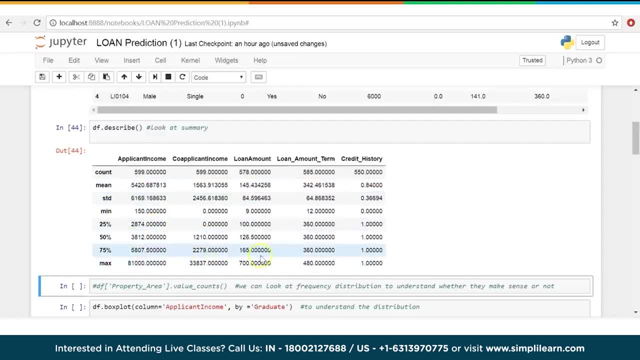 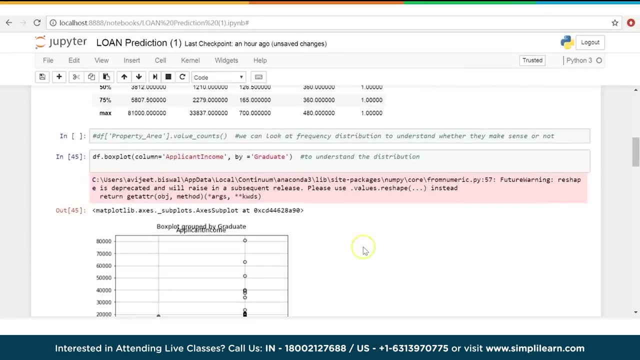 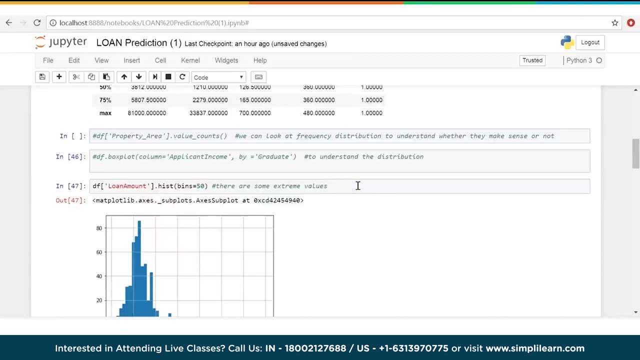 are there. What does it mean? Standard deviation, Minimum, Maximum And so on and so forth for each of them, And then you can do some visualization. So this is the visualization for this. Okay, The next step is to view the data- data visualization- and we will do that using a histogram for. 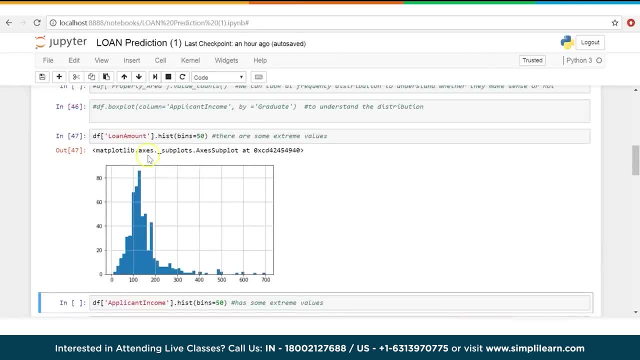 a couple of these columns. So in this case, I'm taking a look at the loan amount And if I create a histogram, it displays the data here in the form of a histogram. One thing that we gather from this- as I mentioned in the slides as well- is that the data that's 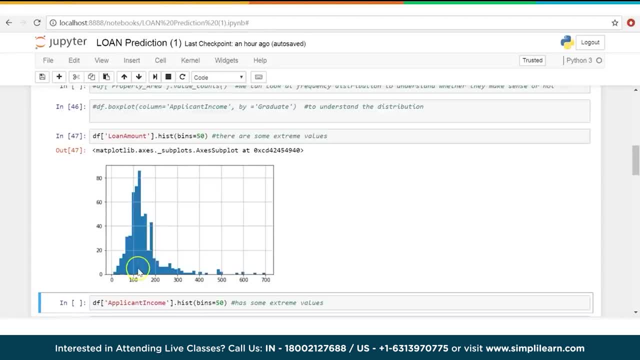 displayed in the form of a histogram. it displays the data that's displayed in the form of a histogram, So we can see in the slides as well as how the data is kind of scattered. So while most of the values are in this range- 0 to 300 range- there are a few extreme values. 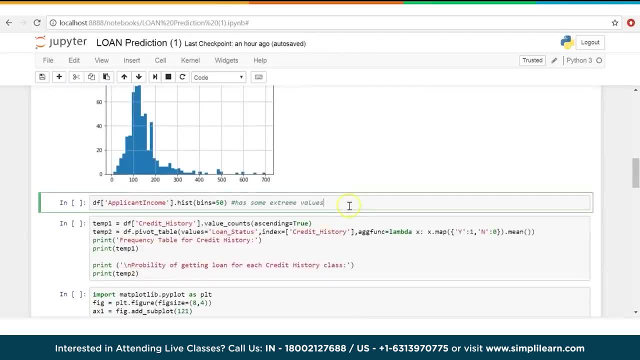 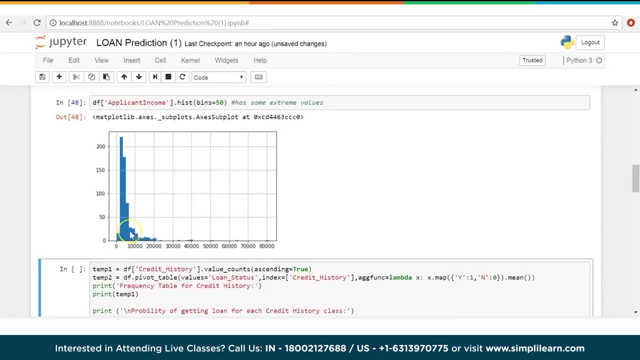 around the 700 range. So that is one information we get from this histogram. Similarly, for the applicant income, if we draw a histogram, something similar, we can see that while most of the values are in this range- 0 to 20,000 range, there are a few. 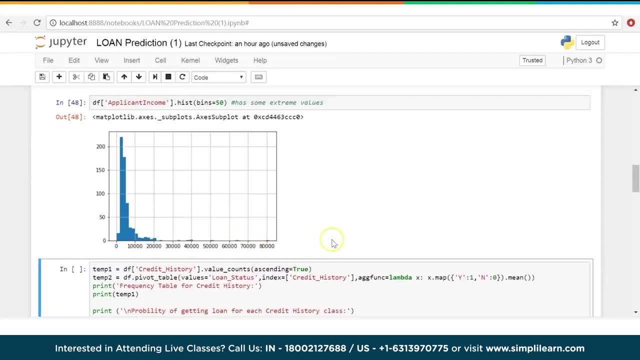 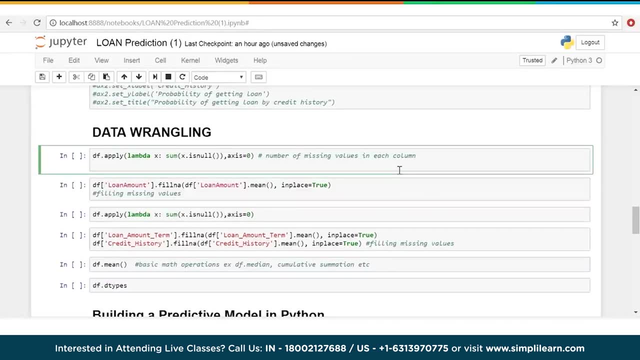 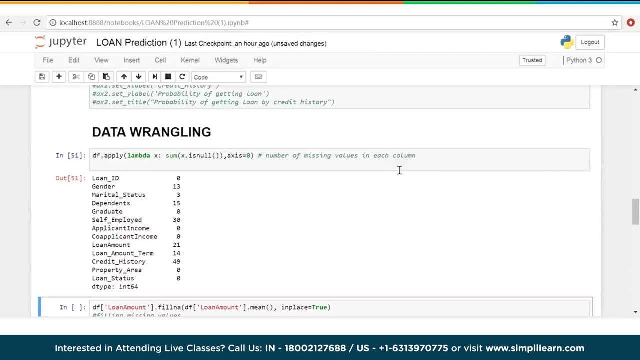 in the range of 80,000 and probably 65,000, and so on. Okay, So the next step is to perform data wrangling, where we will check if any data is missing and how to fill those missing values and so on. So in this case, we will just check for all the columns how many data or how many entries. 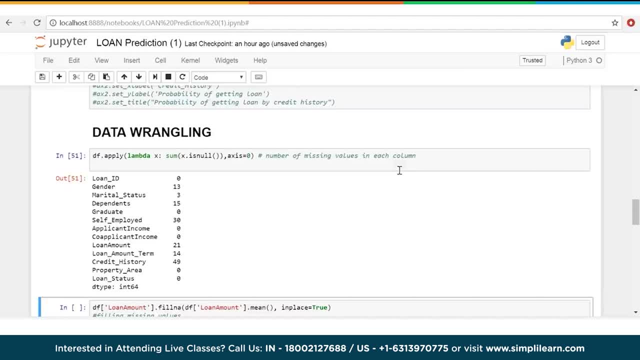 are there with missing values. This is the results. The loan ID has all the columns or all the cells filled. Gender has 13 missing values. Marital status has three missing values, and so on and so forth. Loan amount has 21.. 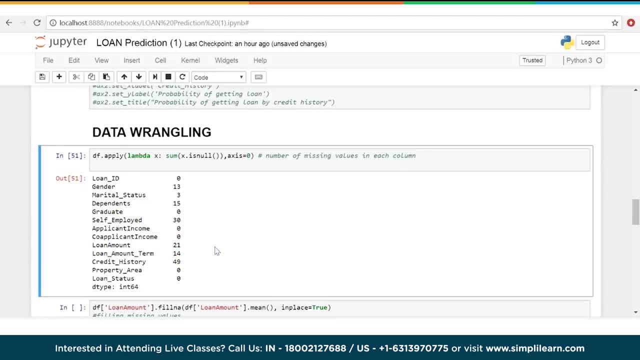 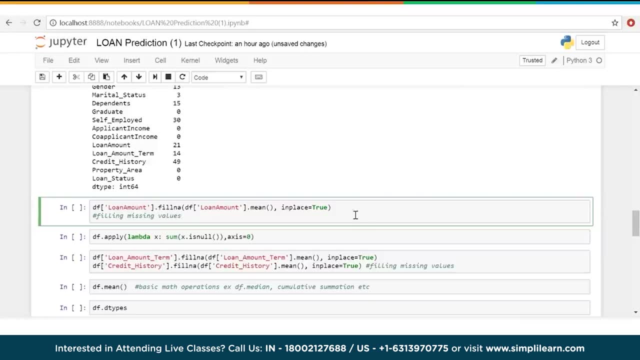 And this is what we are going to show you: How to remove these missing values. So when you have missing values, as I mentioned during the slides, there are a couple of ways of handling that. One is you can completely remove those or you fill in with some meaningful values. 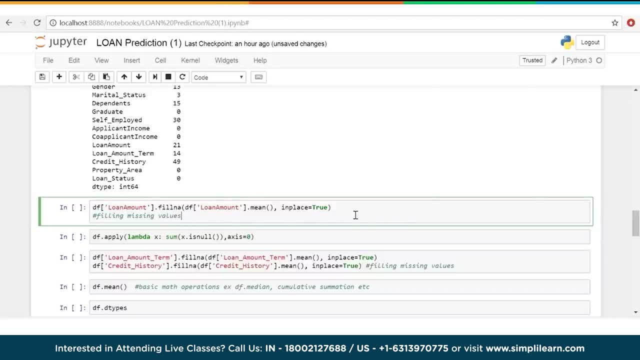 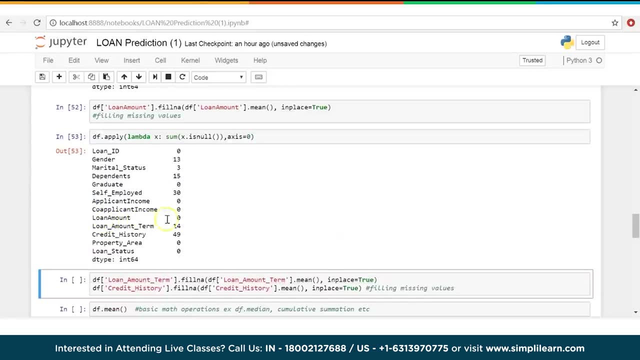 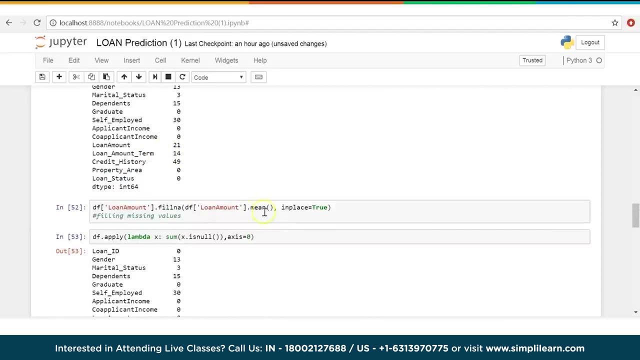 So in this case, we will fill the missing values with the mean value of the loan amount. So let's go ahead and do that. And now, if we check here now, loan amount number of missing values is zero, because what we did was, for all these 21 cells where the values were missing, we filled with the mean. 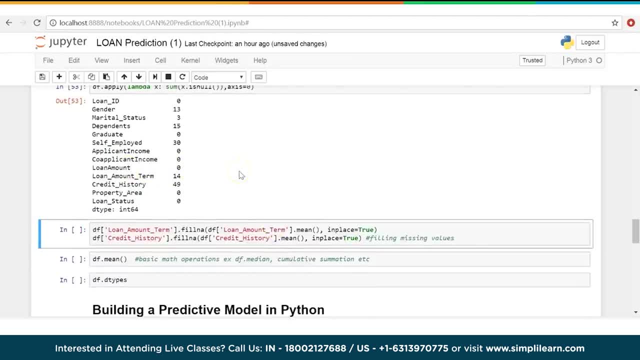 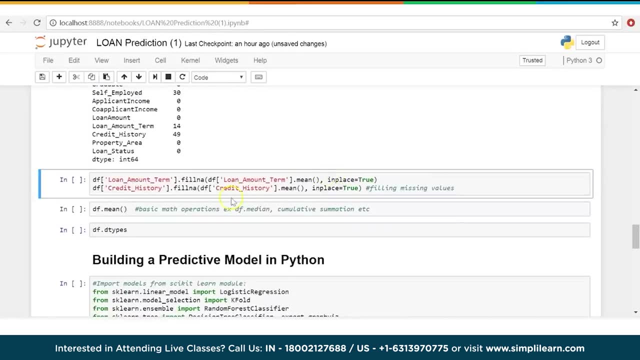 value of the loan amount. So now there are no more missing values for loan amount. We can do this for other columns as well, But this was just one example, So we have shown it here. Okay, so we will run this for credit history and loan amount term as well. 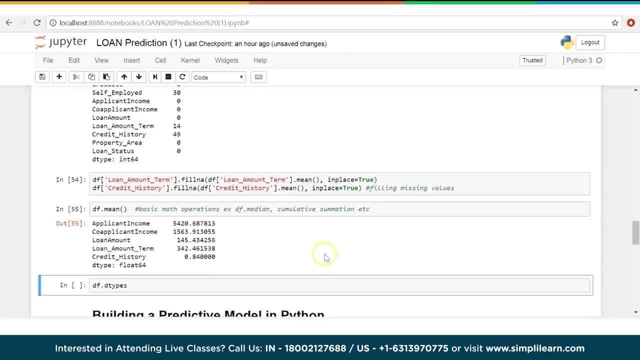 And then if we calculate the mean of pretty much all the numerical columns- that's the method call So dfmean will give us the mean of all the numerical values, And another thing that we can do is we can calculate the mean of all the numerical columns. 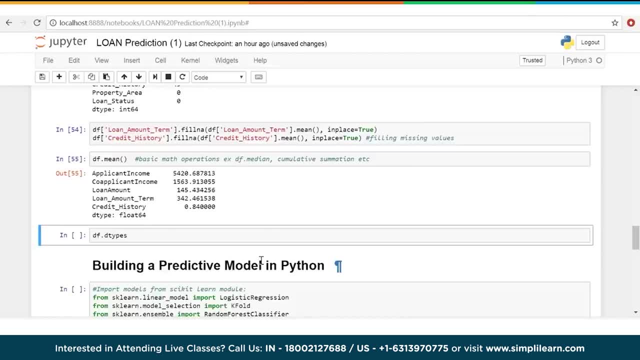 And another thing that we can do is we can calculate the mean of all the numerical columns. So if we want to find out what are the data types of each of these columns, so you can call dfdtypes and get the data types. Of course they may not be that very useful. 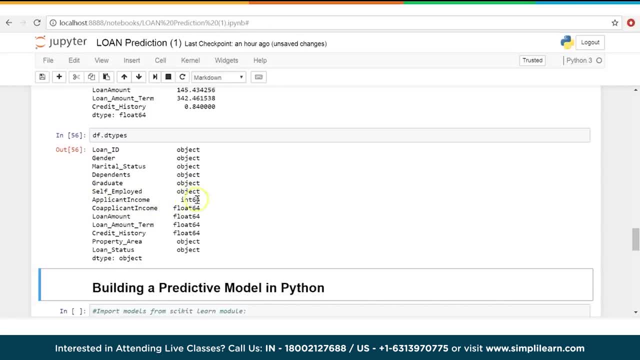 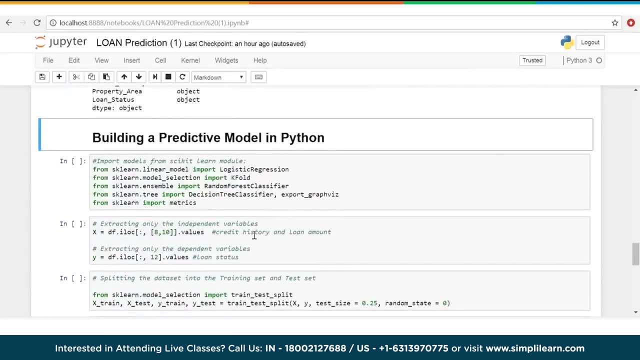 Most of the cases is an object, But for example, this one: it shows as int64, and there are float64 and so on and so forth. Now, in addition to doing the exploratory data analysis, we can do some machine learning activity as well. 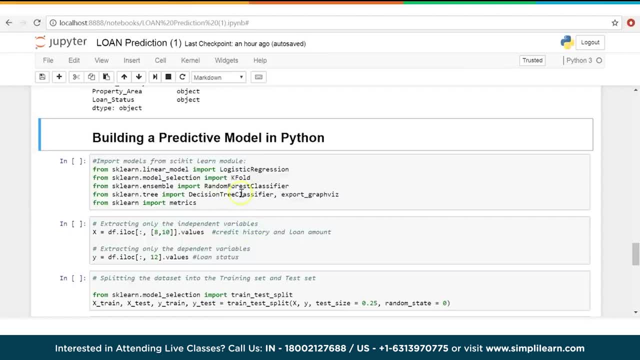 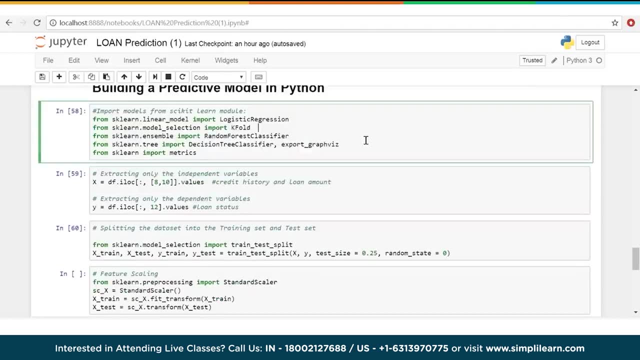 So in this case we are going to do logistic regression. So this is the example that I have shown you in the slides as well. This is the actual code for that. Alright, so the first step here is to import the libraries, And then the next step is to separate the independent variables and the dependent variables. 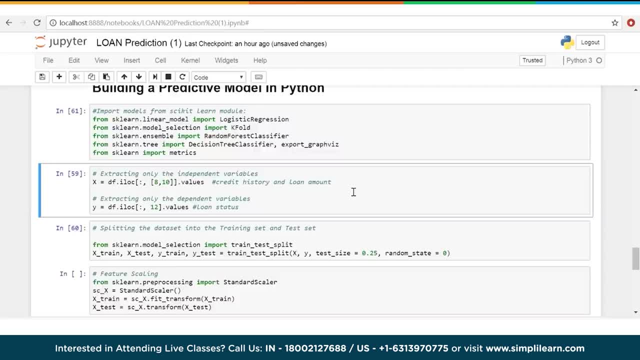 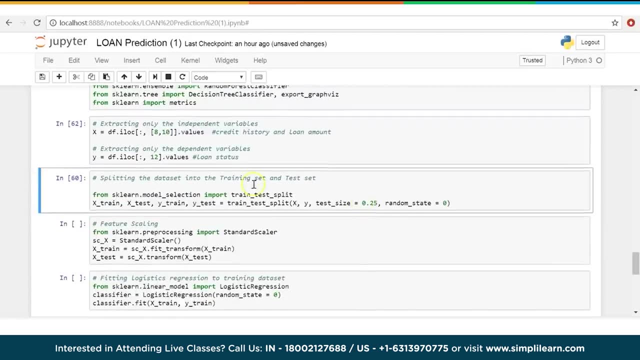 So x is our independent variable and y is our dependent variable. So we separate the data into two parts, and this will be our target as well. right? So that's how we separate it. Now we have to split the data into training and test data sets. 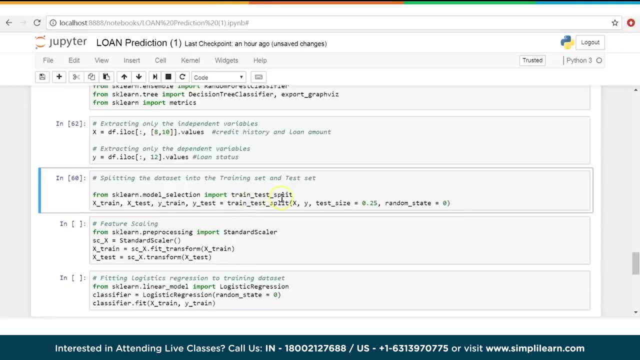 As I mentioned in the during the slides, we use the train test split method And when we call this and pass the independent variables and the dependent variables and we specify the test size to be 0.25, which means the training size will be 0.75, which 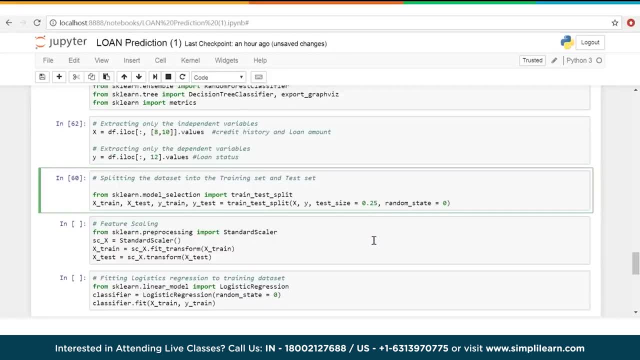 is nothing. but you split the data into training data set, which is 75%, and test data set, in which is 25%. okay, so once you split that, you will have all your independent variables data in x, train, the training data, which is 75% of it. 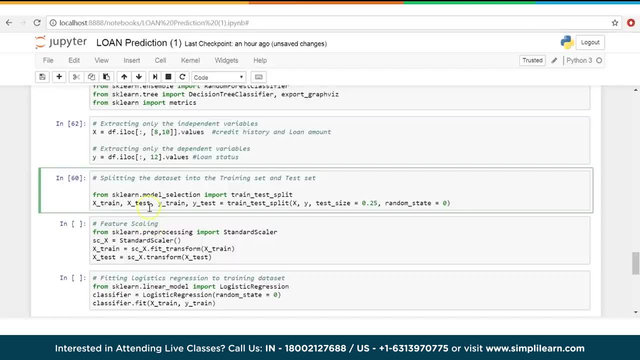 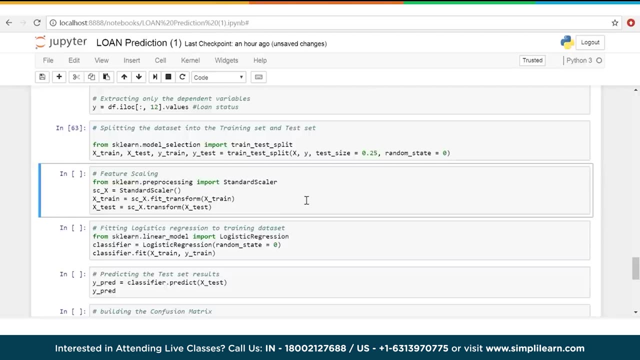 Similarly, independent variables for test will be in x underscore test and dependent variables train will be in y underscore train and dependent variable test will be y underscore test. Once we do this, we have to do a small exercise for scaling. Remember, we had some data which was kind of very scattered. there were some extreme. 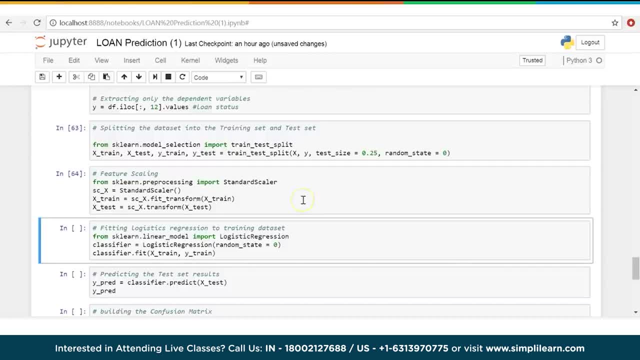 values and so on. So this will take care of that, So that The data is normalized, so that, before we pass to our algorithm, the data is normalized, so that the performance will be much better. The next step is to create the instance of logistic regression object. 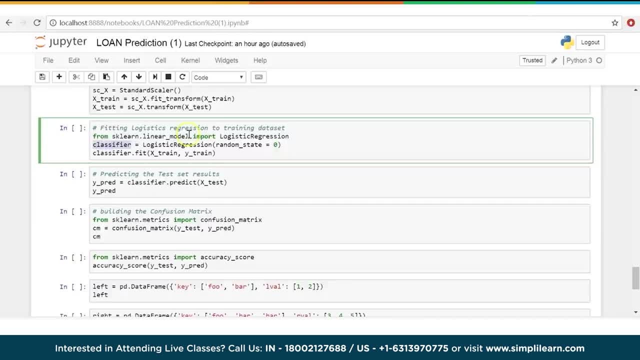 So that's what we are doing here. So classifier is our logistic regression instance. right, classifier is equal to logistic regression. we are saying so one instance of logistic regression is created and then we call the training method. the name of the method actually is fit, but what it is doing is it is taking 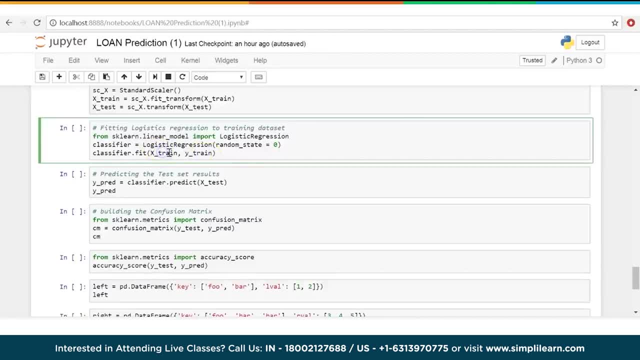 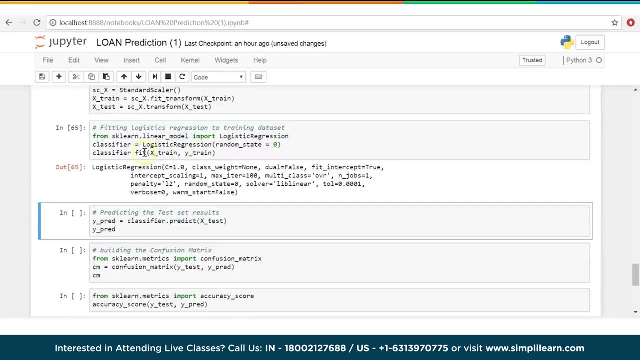 the training data, x is the training data or the independent variables and y is the dependent variables. So we are taking both of these and the model gets trained. So the method for calling the training is fit. okay, so it gives us the output, and then 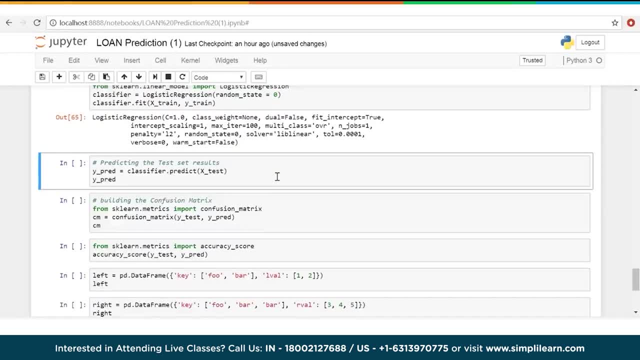 once we are done with the training, we do the testing. and once again, just to recall in the slides, when I was showing you the slides also, I mentioned we don't pass y here. while we are testing, while for training, we do pass y, but right, 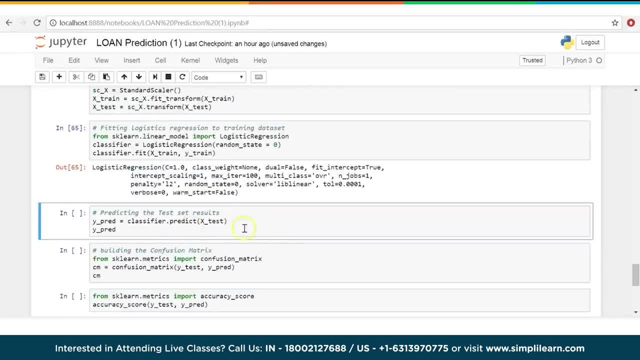 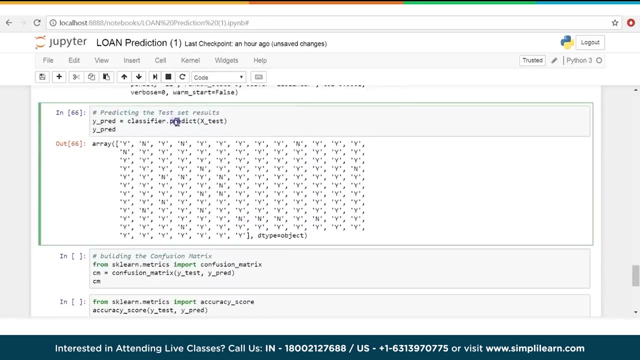 So, for fit, we are passing x and y, but for test we are only passing x, something you need to observe, because y will be calculated by the model and we will then compare that with the known value of y to measure the accuracy. So that's what we will do here, and the method that is called here is predict. 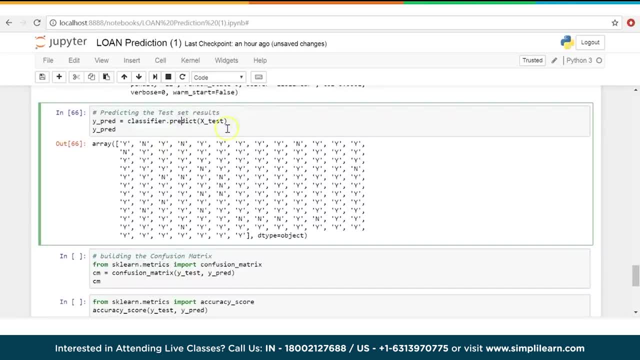 So this will basically create or predict the values of y. Now we have in this case a binary classification, So the outputs are yes or no. Why y indicates yes and n indicates no? So y or n is the output. Now how do we measure the accuracy? 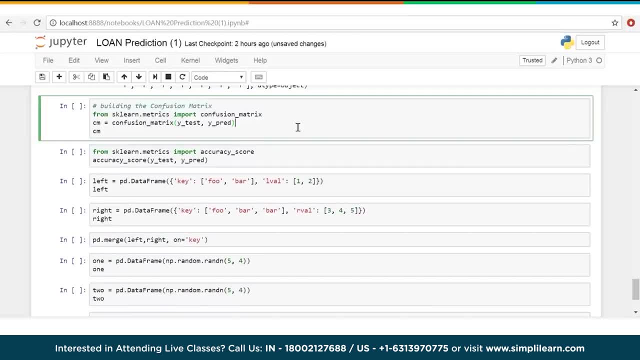 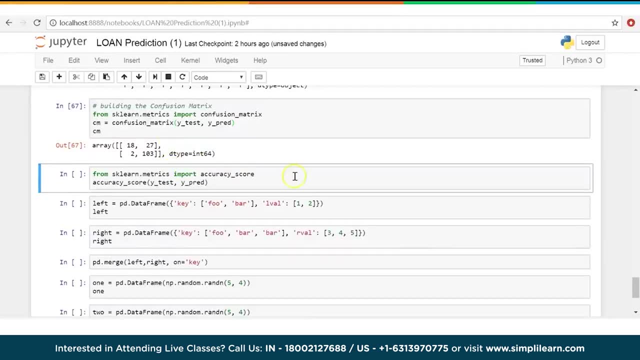 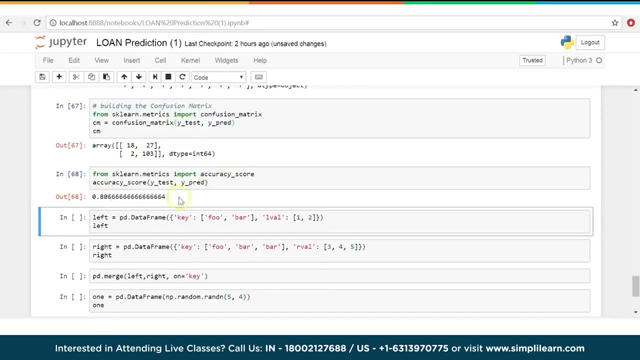 As we have seen earlier, I described how confusion matrix works and how we can use confusion matrix for calculating the accuracy. That's what we are seeing here. So this is the confusion matrix and then you want to do the measure, the accuracy. You can directly use this method and we find that it is 80%. 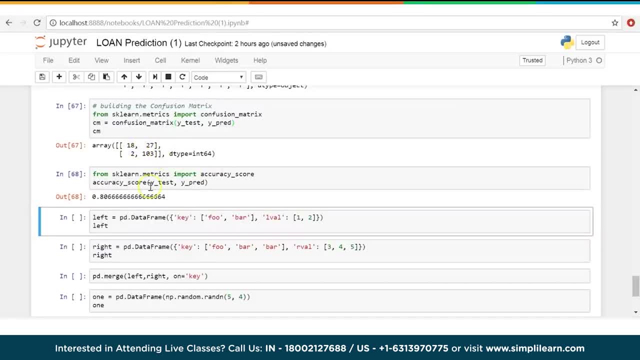 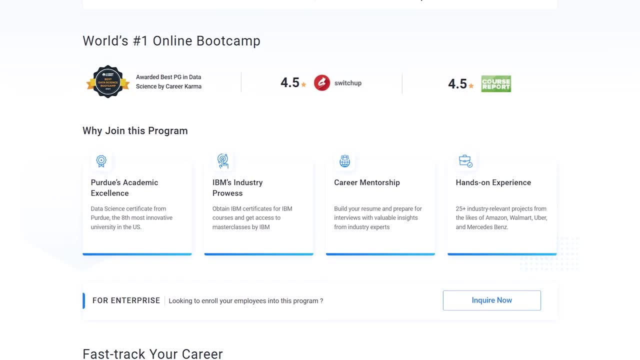 So we in the slides we have seen, when we calculate manually as well, we get an accuracy of 80%. Also, data scientists looking for online training and certification programs from the best universities, or a professional who elicits to switch careers with data science? then try giving Simply. 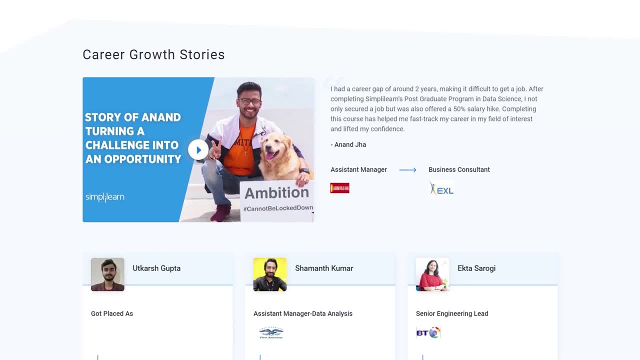 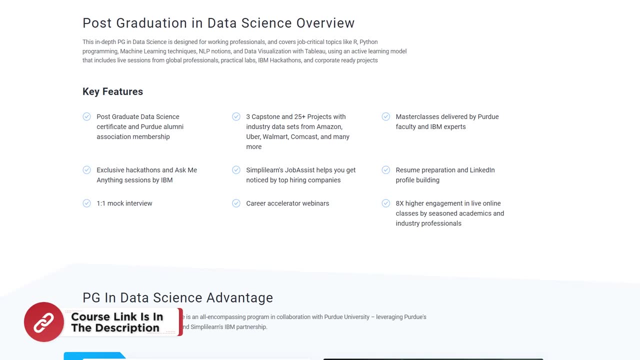 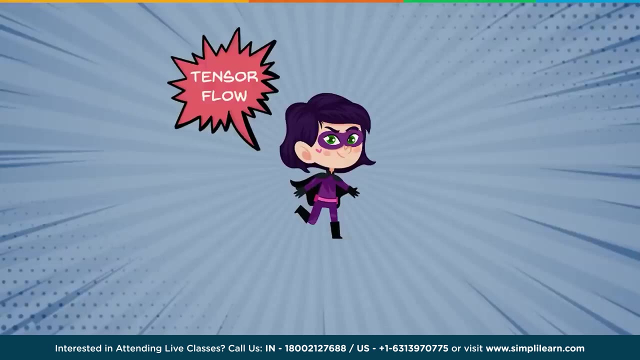 Learn's postgraduate program in data science a shot. The link in the description box below should navigate you to the homepage, where you can find the complete overview of the program being offered. Now over to our training experts. So let's talk about this amazing library, TensorFlow, which is also one of my favorites. 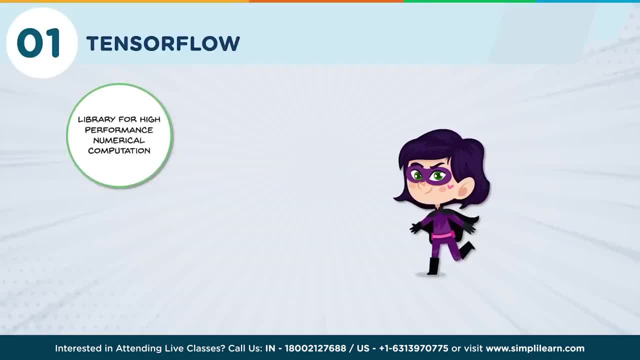 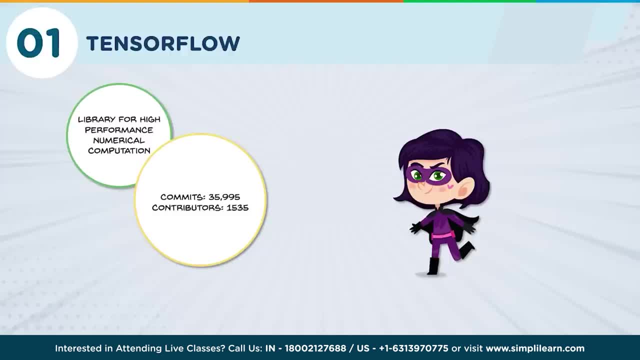 And so TensorFlow is a kind of library, basically for high performance networks. it is a library for those who do nuestros of numerical computations, with around 35,000 GitHub commits and a vibrant community of around 1500 contributors, and it's used across various scientific domains. 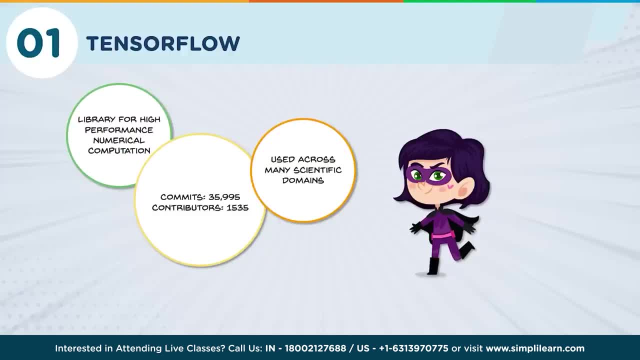 and it's used across various scientific domains. And it's used across various scientific domains. it's basically a framework Where we can define and run computations, which involves sensors and sensors, we can say a partially defined computational objects. again there they will eventually produce. 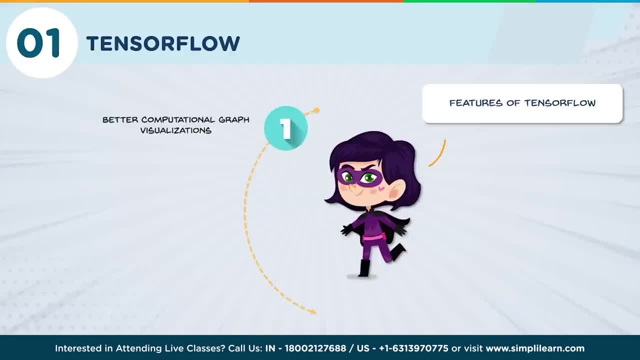 a value. that was about going to TensorFlow. Let's talk about the features of TensorFlow. TensorFlow is majorly used in deep learning. 例到 TensorFlow一定数, TensorFlow enabling spoons and magicians learn. entities can learn and can learn from their owninsiples. 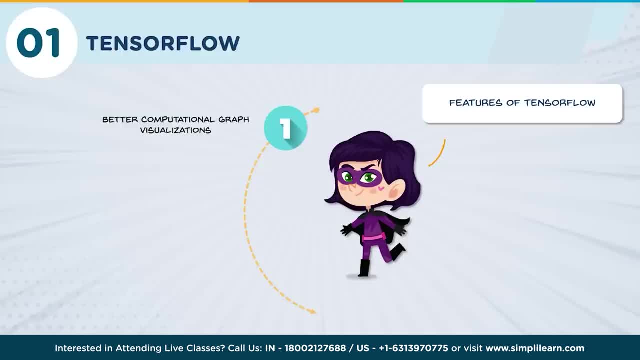 majorly used in deep learning models and neural networks, where we have other libraries like torch and tiano also. but tensorflow has hands-down better computational graphical visualizations when compared to them. also, tensorflow reduces the error largely by 50 to 60 percent in neural machine translations. it's highly parallel in a way where it can train multiple neural networks. 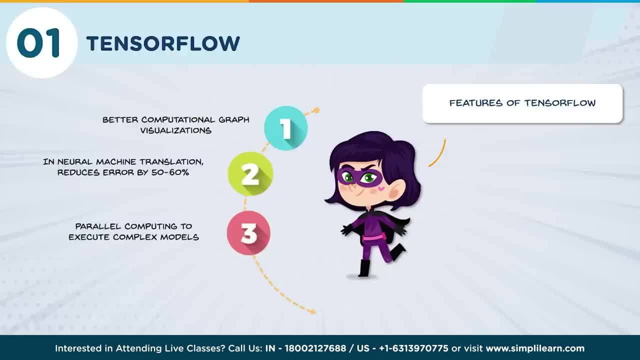 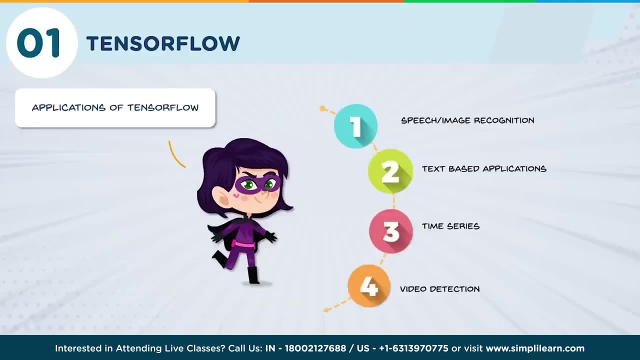 and multiple GPUs for highly efficient and scalable models. this parallel computing feature of tensorflow is also called pipelining. also, tensorflow has the advantage of seamless performance. as it's backed by Google, it has quicker updates, frequent new releases with the latest of features. now let's look at some applications. tensorflow is extensively used in speech and image recognition. 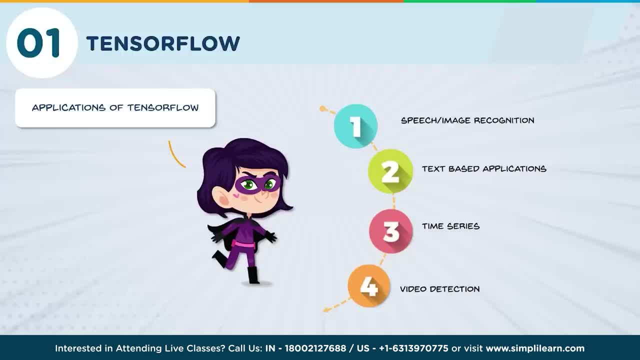 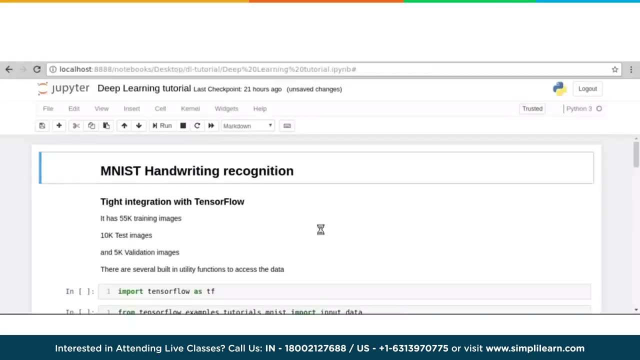 text-based applications, time series, analysis and forecasting and various other applications involving video detection. so favorite thing about tensorflow that it's already popular among the machine learning community and most are open to trying it and some of us are already using it. now let's look at an example of a tensorflow model. in this example we will not dive deep into the explanation. 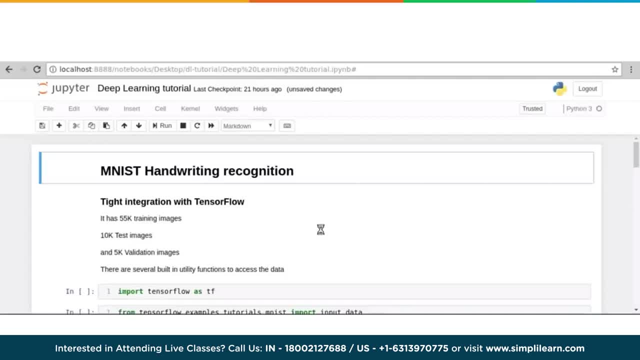 of the model as it is beyond the scope of this video. so here we're using amnes data set, which consists of images of handwritten digits. handwritten digits can be easily recognized by building a simple tensorflow model. let's see how, when we visualize our data using map. 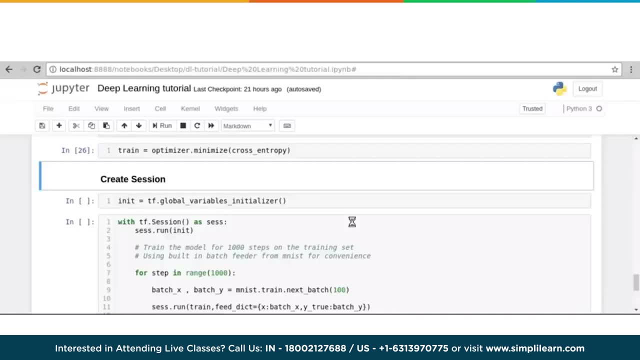 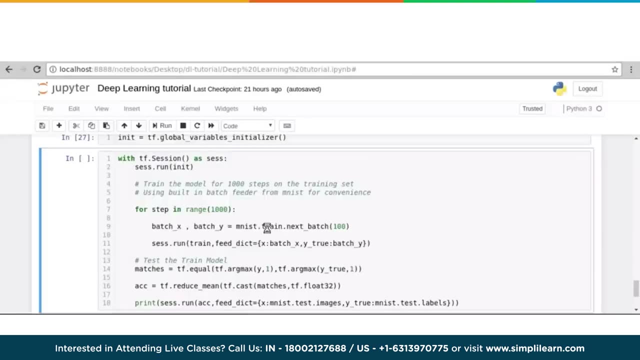 dot web library. the inputs will look something like this: then we create our tensorflow model. to create a basic tensorflow model, we need to initialize the variables and start a session. then, after training the model, we can validate the data and then predict the accuracy. this model has predicted 92 accuracy. let's see, which is pretty well for this model. so that's all for tensorflow. 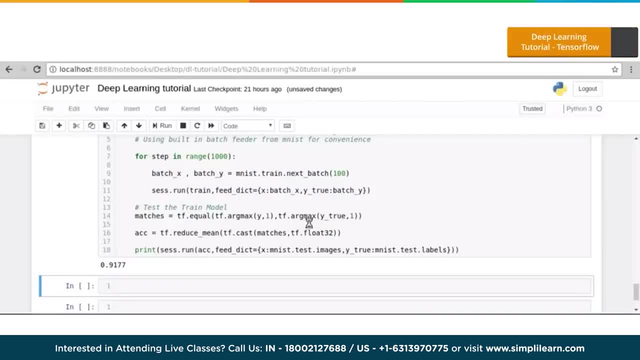 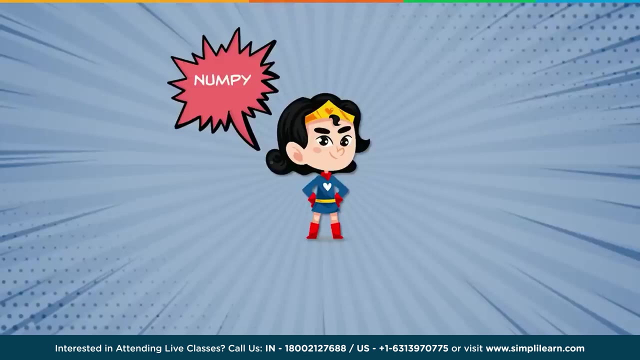 if you need to understand this tutorial in detail, then you can go ahead and watch our deep learning tutorial from simply learn as shown in the right corner. interesting, right? let's move on to the next library. now let's talk about a common, yet a very powerful python library called numpy. numpy is a fundamental package for numerical computation in python. it 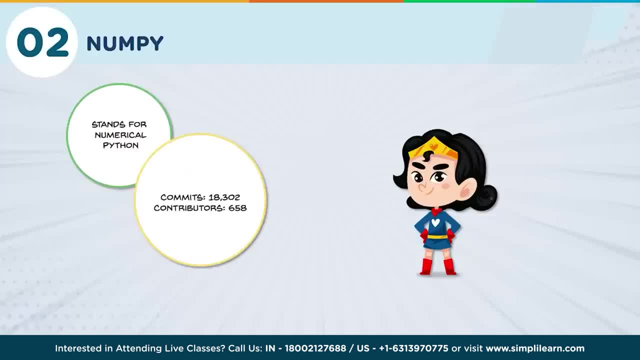 stands for numerical python. as the name suggests, it has around 18 000 comments on GitHub, with an active community of 700 contributors. it's a general purpose array processing package in a way that it provides high performance multi-dimensional objects called arrays and tools for working with them also. 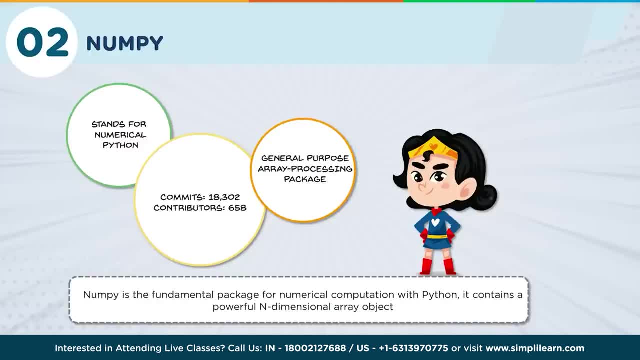 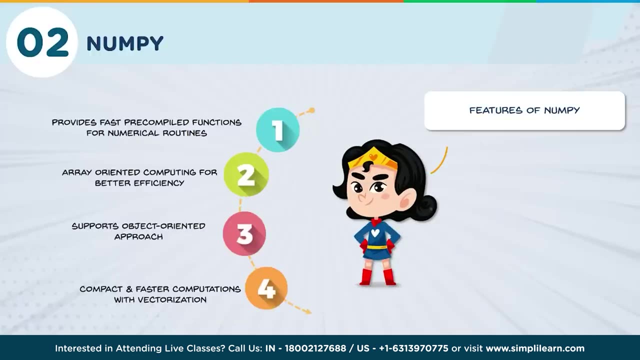 addresses the slowness problem partly by providing these multi-dimensional arrays that we talked about and then functions and operators that operate efficiently on these arrays. interesting right now let's talk about features of numpy. it's very easy to work with large arrays and mattresses using numpy. numpy fully supports object-oriented approach, for example, coming back to nd array, once again it's 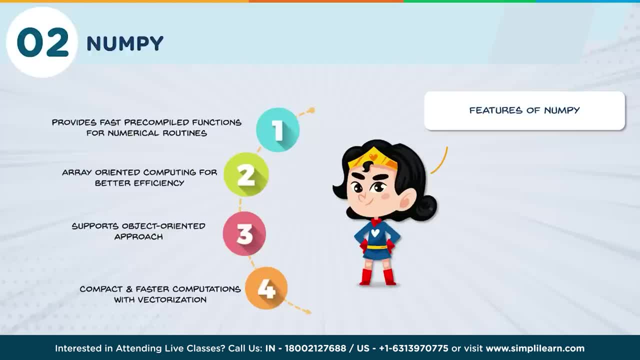 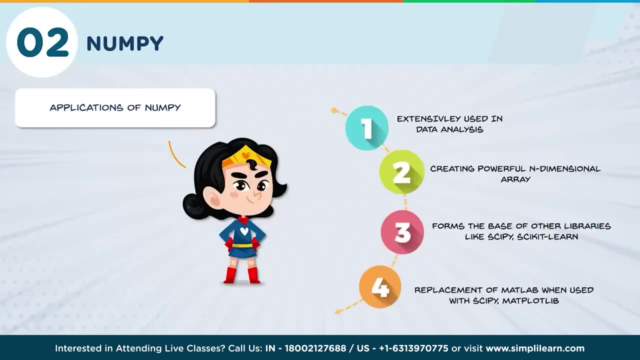 a class possessing numerous methods and attributes. nd array provides for larger and repeated computations. numpy offers vectorization. it's more faster and compact than traditional methods. I always wanted to get rid of loops, and vectorization of numpy clearly helps me with that. now let's talk about the applications of numpy. numpy, along with pandas, is extensively used in data analysis, which 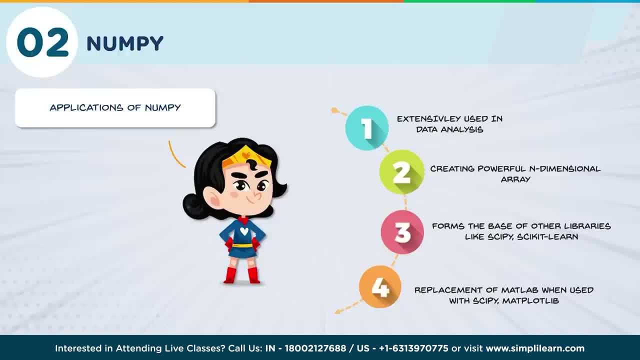 forms the basis of data science. it helps in creating the powerful n-dimensional array. whenever we talk about numpy- the mention of the array- we cannot do it without the mention of the powerful n-dimensional array. also, numpy is extensively used in machine learning. when we are creating machine learning models, as in where it forms the base of other libraries like scipy. 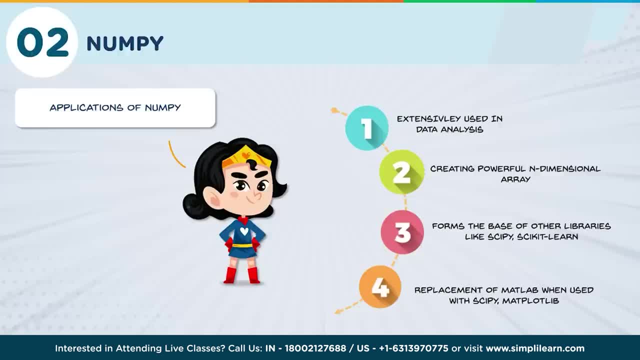 scikit-learn, etc. when you start creating the machine learning models in data science, you will realize that all the models will have their basis numpy or pandas. also, when numpy is used with scipy and matplotlib, it can be used as a replacement of matlab. now let's look at a 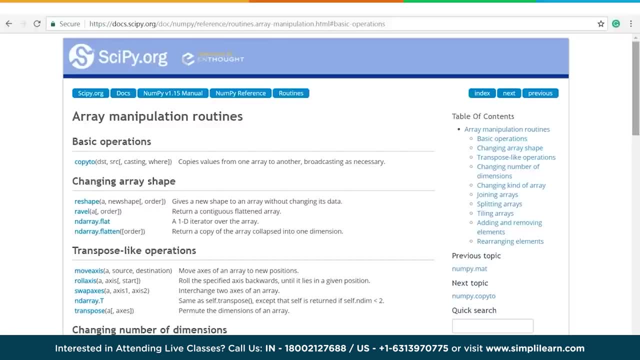 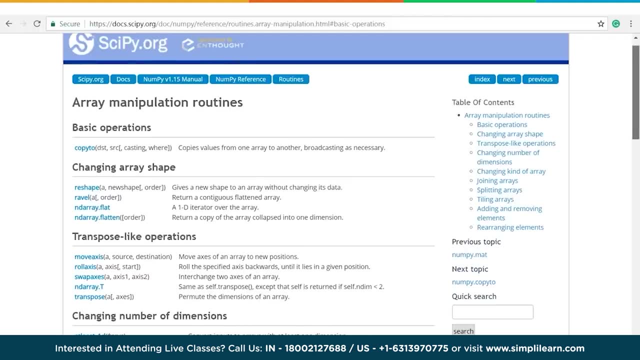 simple example of an array in numpy. as you can see, here there are multiple array manipulation routines, like there are basic examples where you can copy the values from one array to another. we can give a new shape to an array, from maybe one dimensional to we can make it as a two-dimensional. 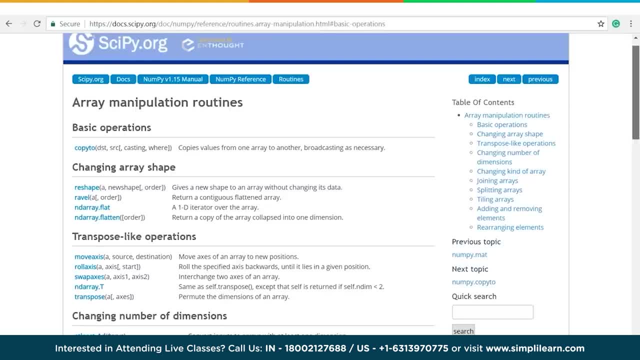 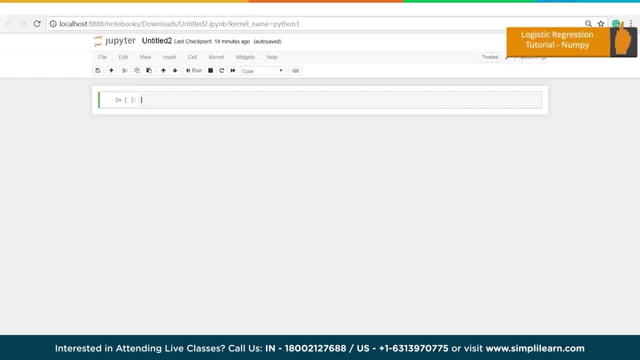 array. we can return a copy of the array collapsed into one dimension. now let's look at an example where this is a jupiter notebook and we will just create a basic array and for detailed explanation of our other videos, which targets on these explanations of each libraries. so first of all, 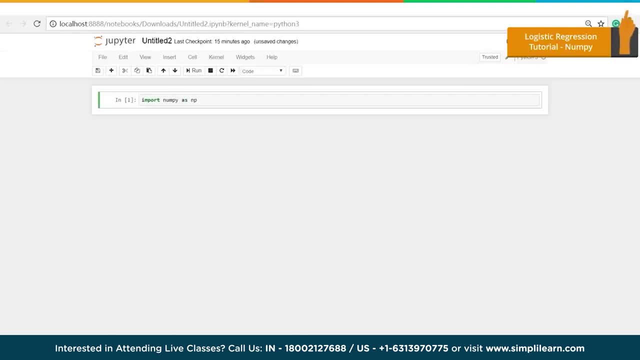 whenever we are using any library in python, we have to import it. so now this np is the alias which we will be using. let's create a simple array. let's look what is the type of this array. so this is an nd array type of array. also, let's look what's the shape of this array. 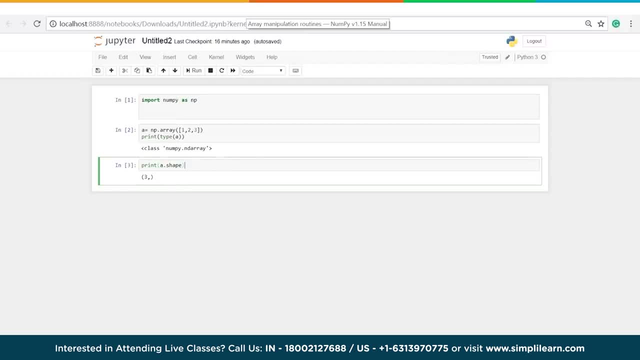 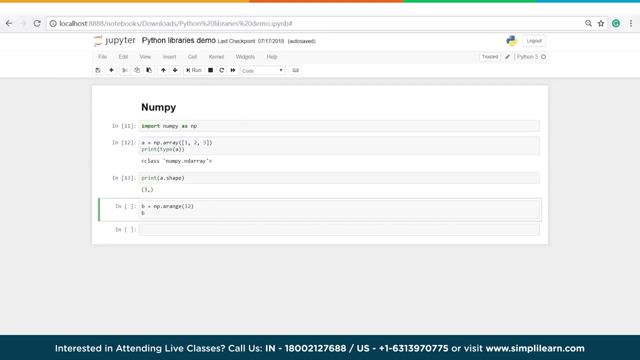 so this is a shape of the array. now, here we saw that we can expand the shape of the array. so this is where you can change the shape of the array using all those functions. now let's create an array using arrange function. so if i give arrange 12, it will give me a 1D array of 12. 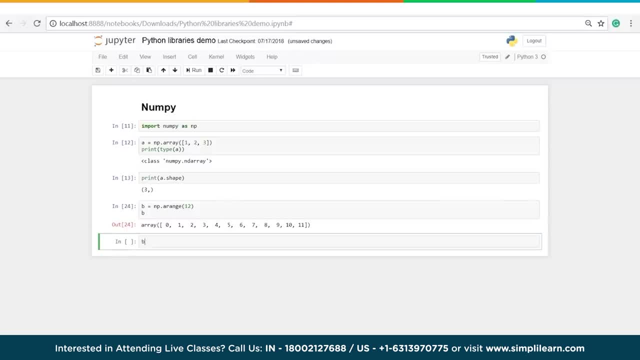 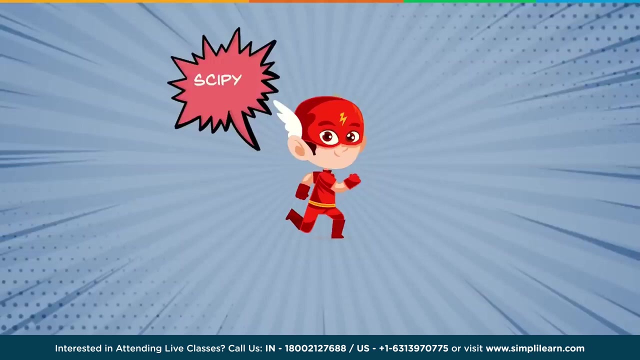 numbers like this. now we can reshape this array to 3 comma 4 or we can write it here for itself. so this is how arranged function and the reshape function works for nonpi. now let's discuss the next library, which is scipy. so this is another free and open source Python library extensively. 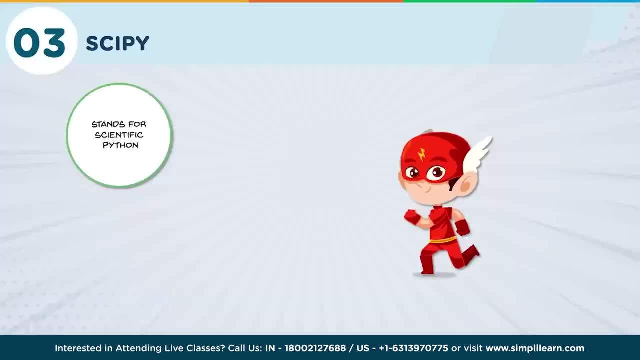 used in data science for high level Comp adaptations. so this library, as the name suggests, transfer scientific python and it has around 19 000 commits on GitHub with an active community of six hundred contributors. it is extensively used for and technical computations also. as it extends numpy, it provides many. 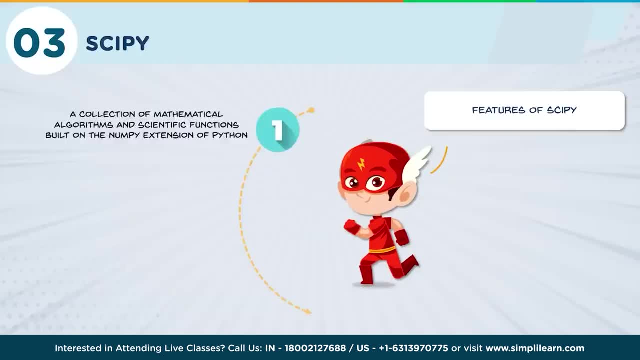 user-friendly and efficient routines for scientific calculations. now let's discuss about some features of sci-fi. so sci-fi has a collection of algorithms and functions which is built on the numpy extension of Python. secondly, it has various high-level commands for data manipulation and visualization, also the 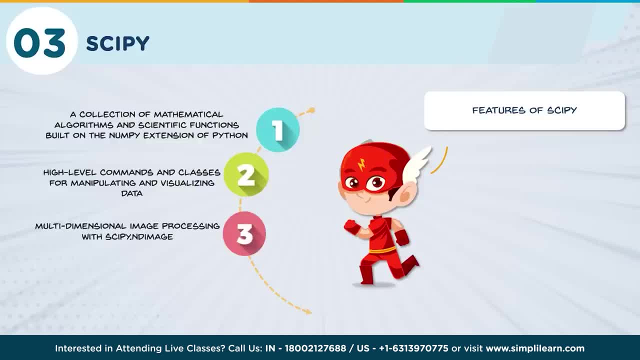 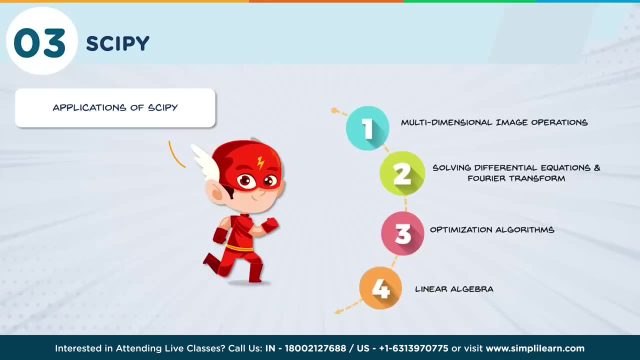 ND image function of sci-fi is very useful in multi-dimensional image processing and it includes built-in functions for solving differential equations, linear algebra and many more. so that was about the features of sci-fi. now let's discuss its applications. so sci-fi is used in multi-dimensional 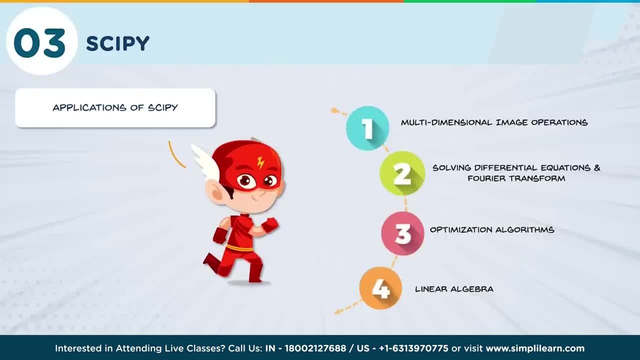 image operations. it has functions to read images from disk into numpy arrays, to write arrays, to discuss images, resize images etc. solving differential equations, Fourier transforms, then optimization algorithms, linear algebra, etc. let's look at a simple example to learn what kind of functions are there in sci-fi. 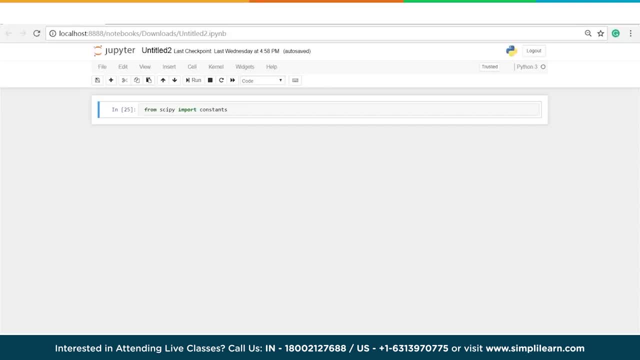 here I'm importing the constants package of sci-fi library, so in this package it has all the constants. so here I am just mentioning C or H or any, and this library already knows what it has to fetch, like speed of light, Planck's constant, etc. so this can be used in further calculations. data analysis is an. 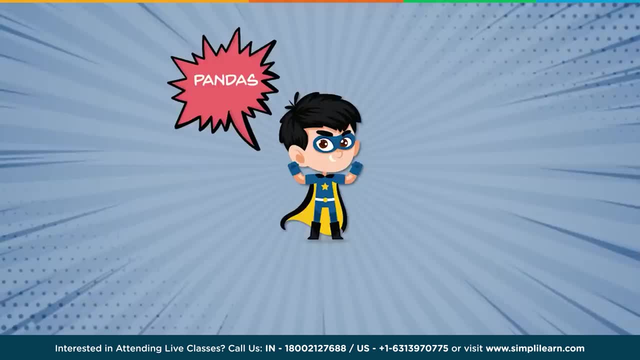 integral part of data science. data scientists spend most of the day in data munching and then cleaning the data also. hence mention of Pandas is a must in data science lifecycle. yes, Pandas is the most popular and widely used Python library for data science, along with numpy and matplotlib- the name itself. 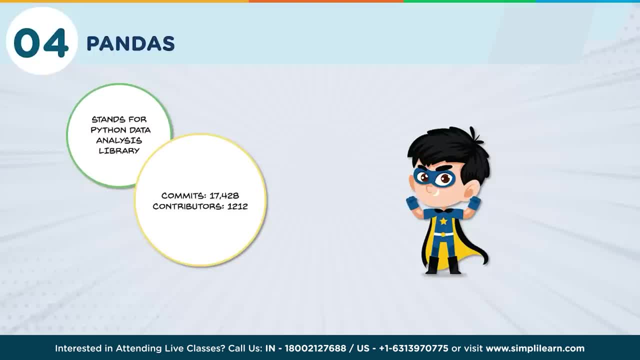 stands for Python data analysis. with around 17,000 commits on github and an active community of 1,200 contributors, it is heavily used for data analysis and cleaning, as it provides fast, flexible data structures like data frames, CVs, which are designed to work with structured data very easily and easily. 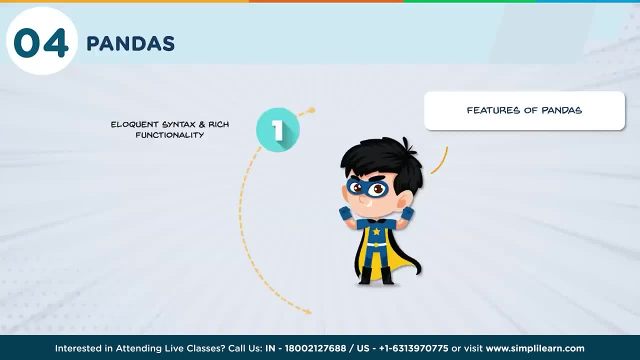 unintudively. now let's talk about some features of Pandas. so Pandas offers this eloquent syntax and rich functionalities. like. there are various methods in Pandas, like drop any, fill any, which gives you the freedom to deal with missing data. also, Pandas provides a powerful apply function which lets you create your own. 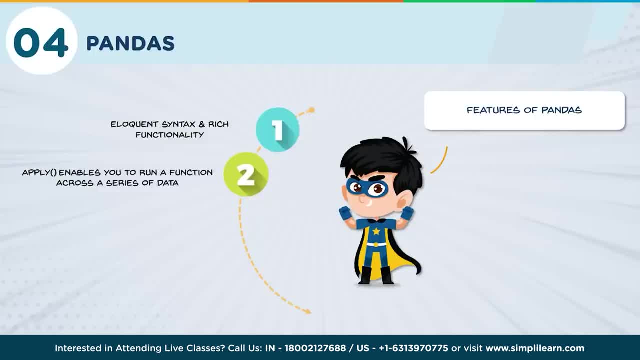 function and run it across a series of data. now forget about writing those four loops while using Pandas- also this library's high level abstraction over low level numpy, which is even in pure C. then it also contains these high level data structures and manipulation tools, which makes it very easy to work with Pandas, like their data. 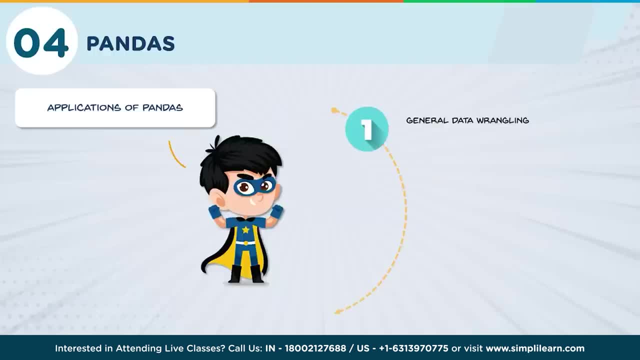 structures and series. now let's discuss the applications of Pandas. so Pandas is extensively used in general data wrangling and data cleaning. then Pandas also finds its usage in ETL jobs for data transformation and data storage, as it has excellent support for loading CSV files into its data frame format. then 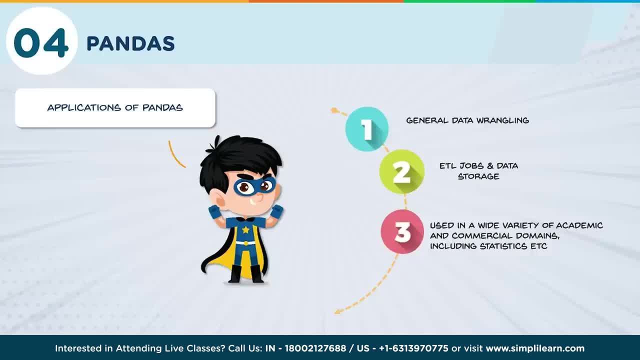 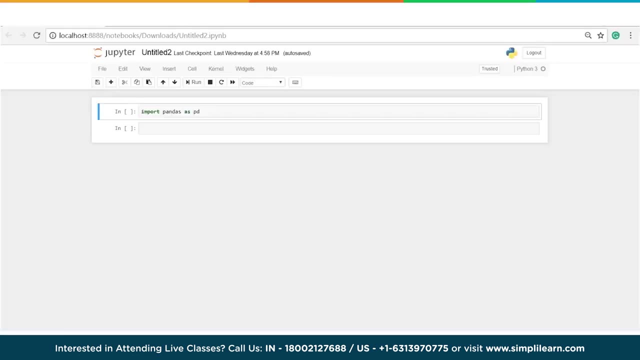 Pandas is used in a variety of academic and commercial domains, including analytics, finance, neuroscience, economics, web analytics, Etc. then Pandas is also very useful in time series specific functionality like date range generation, moving window, linear regression, date shifting, Etc. now let's look at a very 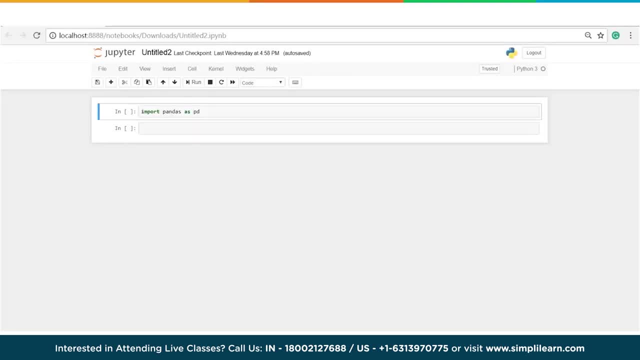 simple example of how to create a data frame. so data frame is a very useful data structure in Pandas and it has very powerful functionalities. so here I'm only enlisting important libraries in data science. you can explore more of our videos to learn about libraries in detail. so let's just go ahead and create a data frame. I'm using Jupiter notebook. 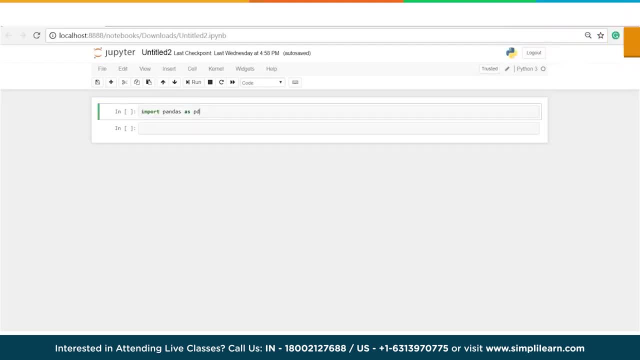 again, and in this before using Pandas- here I'm importing the Pandas library. I can go and run this, so in data frame we can import a file, a CSV file, Excel files. there are many functions doing these things, and we can also create our own data and put it into data frame. so here I am taking. 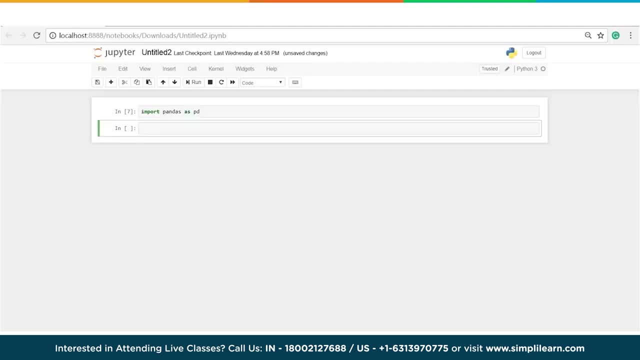 random data and putting in a data frame. also, I'm creating an index and then also giving the column names. so PD is the alias we've given for Pandas: random data of six by four index, which is taking a range of six numbers and column name I'm giving as ABCD. now let's go. 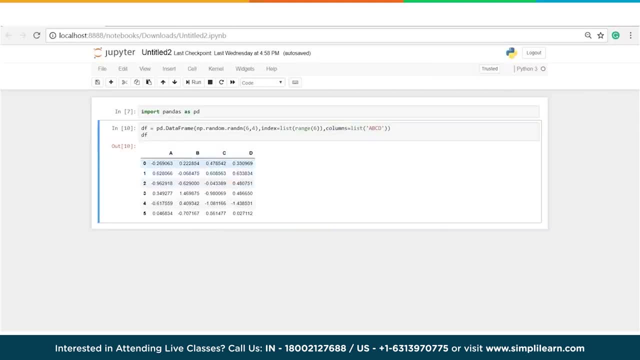 ahead and look at it. so here it has created a data frame with my column. names are ABCD, my list as six, numbers zero to five and a random data of six by four. so data frame is just another table with rows and columns where you can do various functions over it. also, I can go ahead and describe this data. 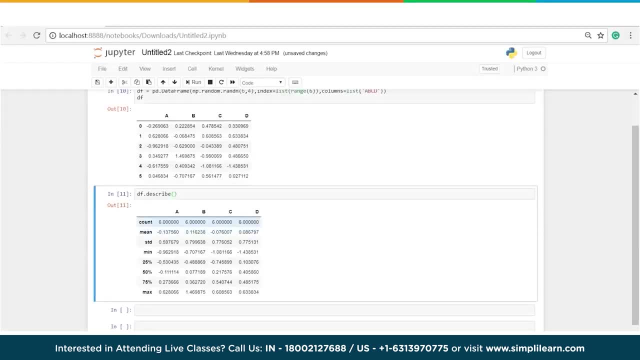 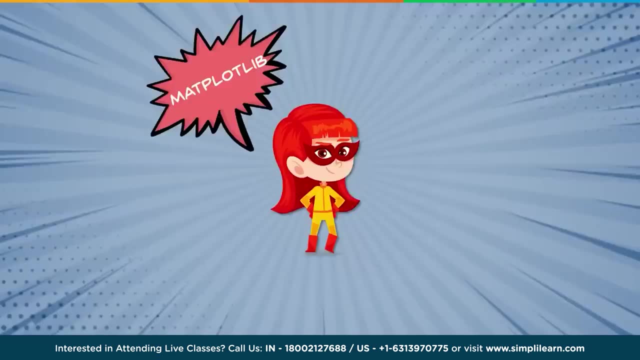 frame to see. so it's giving me all these functionalities where count and mean and standard deviation, Etc. okay, so that was about Pandas. now let's talk about next library and the last one. so matplotlib for me is the most fun library out of all of them. why? because it has such 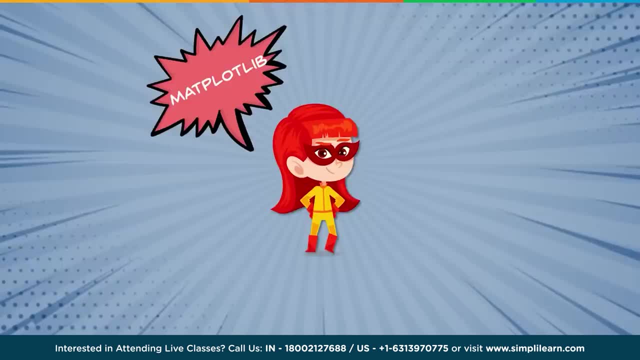 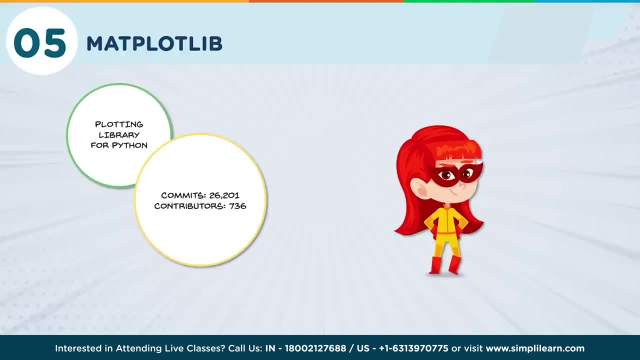 powerful, yet beautiful visualizations we'll see in the coming slides. plot and matplotlib suggests that it's a plotting library for python. it has around 26 000 commits on GitHub and a very vibrant community of 700 contributors and because of such graphs and plots that it produces, it's majorly 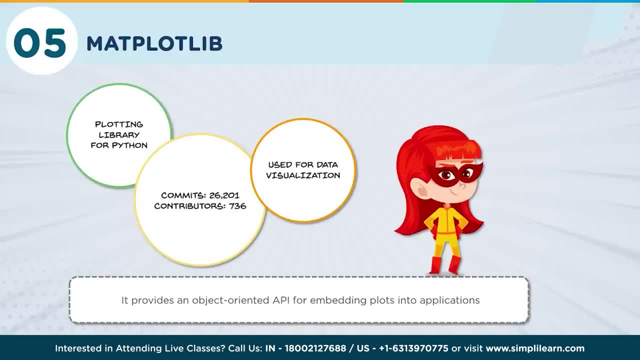 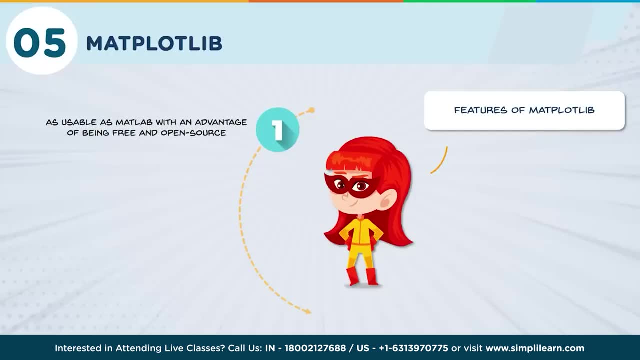 used for data visualization and also because it provides an object-oriented API which can be used to embed those plots into our applications. let's talk about the features of matplotlib. the pi plot module of matplotlib provides matlab like interface, so matplotlib is designed to be as usable as matlab. 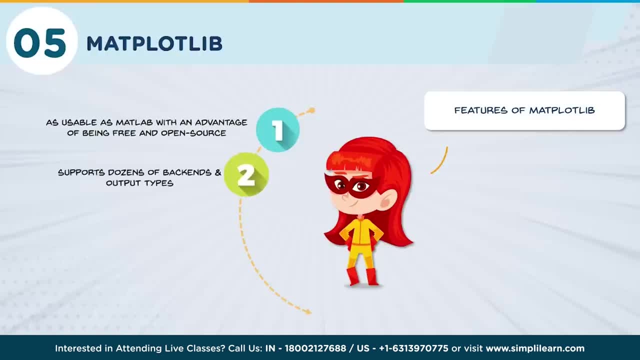 app, with an advantage of being free and open source. Also, it supports dozens of backends and output types, which means you can use it regardless of which operating system you're using or which output format you wish. Pandas itself can be used as wrappers around Matplotlib's. 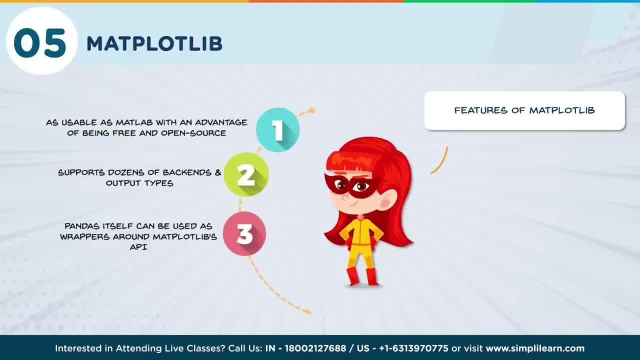 API, so as to drive Matplotlib via cleaner and more modern APIs. Also, when you start using this library, you will realize that it has a very little memory consumption and a very good runtime behavior. Now let's talk about the applications of Matplotlib. 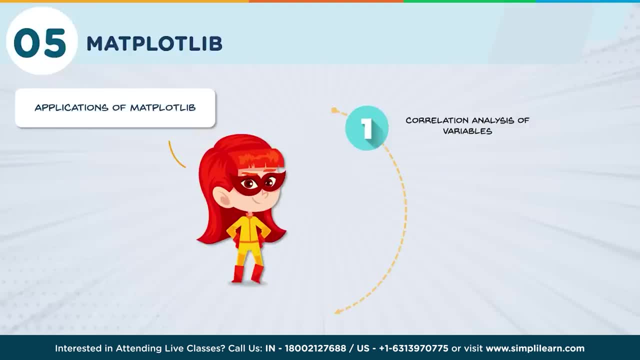 It's important to discover the unknown relationship between the variables in your dataset. so this library helps to visualize the correlation analysis of variables. Also in machine learning we can visualize 95% confidence interval of the model, just to communicate how well our model fits the data. Then Matplotlib finds its application and outlier detection using 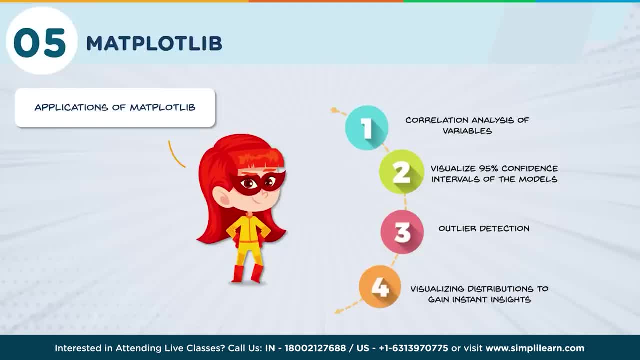 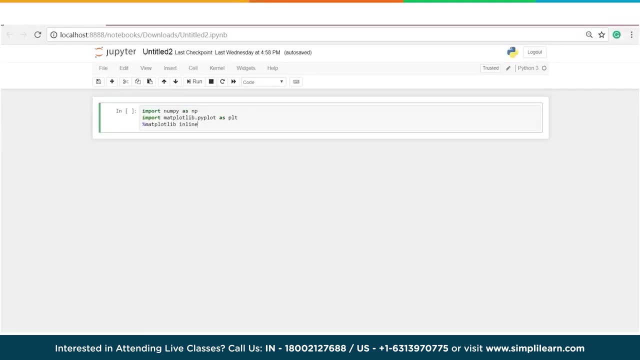 scatterplot, etc. and to visualize the distribution of data to gain instant insights. Now let's make a very simple plot to get a basic idea. I've already imported the libraries here, so this function, matplotlib inline, will help you show the plots in the 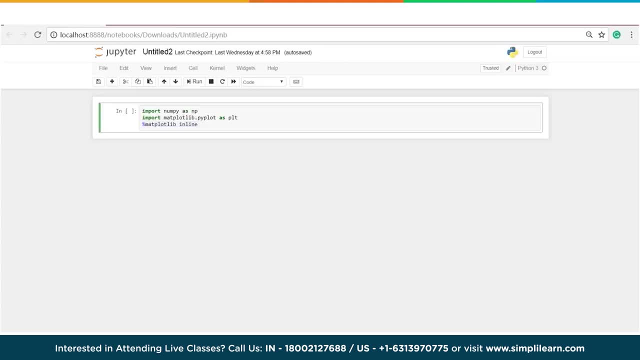 Jupyter notebook. This is also called a magic function. I won't be able to display my plots in the Jupyter notebook if I don't use this function. I'm using this function in numpy to fix random state for reproducibility. Now I'll take my n as 30 and will assign. 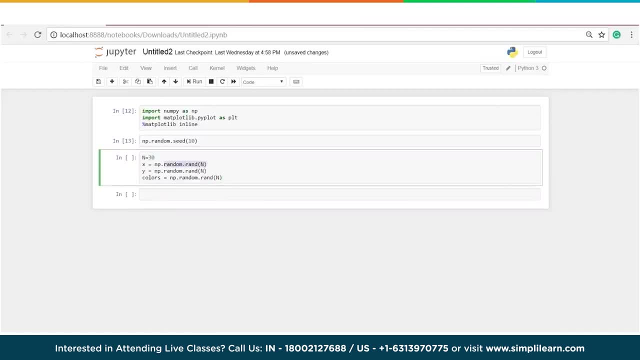 random values to my variables. So this function is generating 30 random numbers. Here I'm trying to create a scatterplot, So I want to decide the area. Let's put this So: this is multiplying 30 with random numbers to the power 2, so that 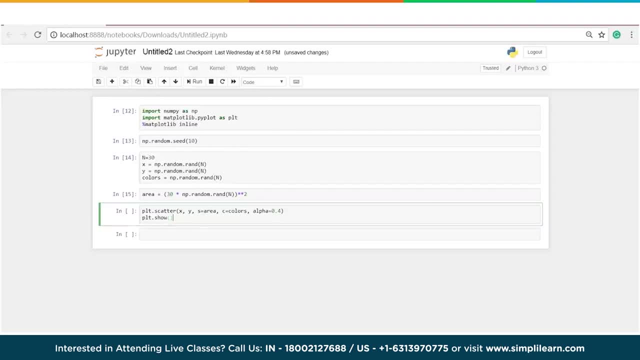 we get the area of the plot which we will see in just a minute. So, using the scatter function and the alias of matplotlib as plt, I've created this. If I don't use this then I have very small circles as my scatterplot. It's colorful, it's nice. 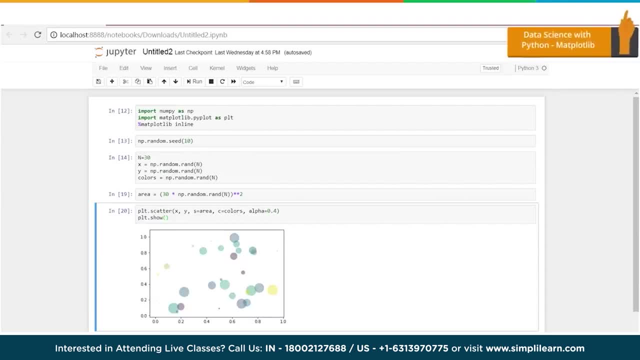 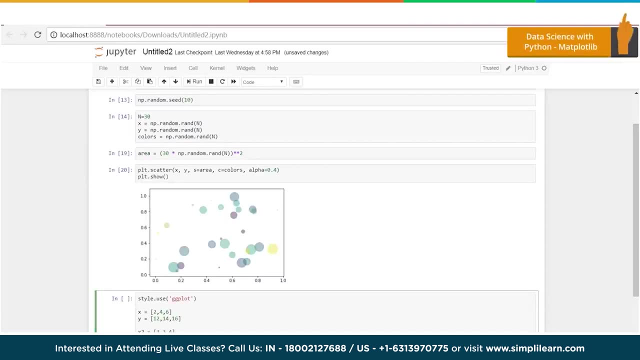 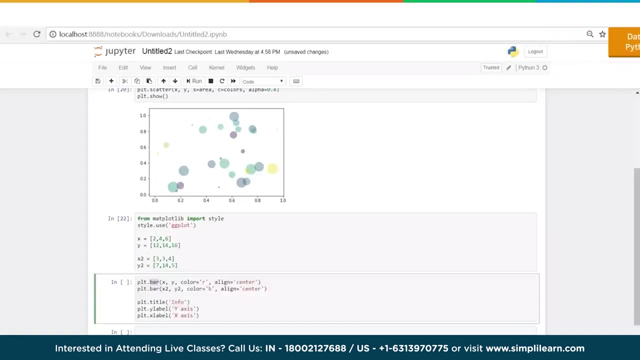 So that's one very easy plot. I suggest that you explore more of matplotlib and I'm sure you will enjoy it. Let's create a histogram. So I'm using my- the style is ggplot- and assigning some values to these variables- any random values. Now we are assigning bars and colors. 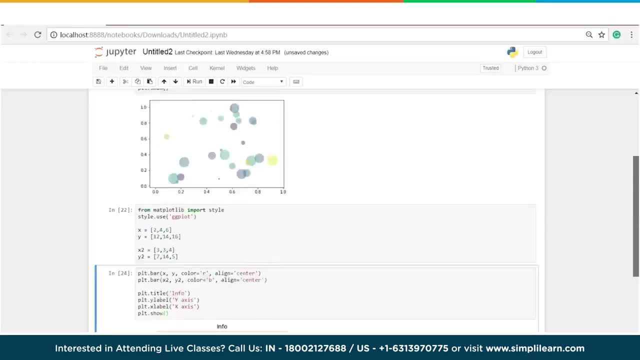 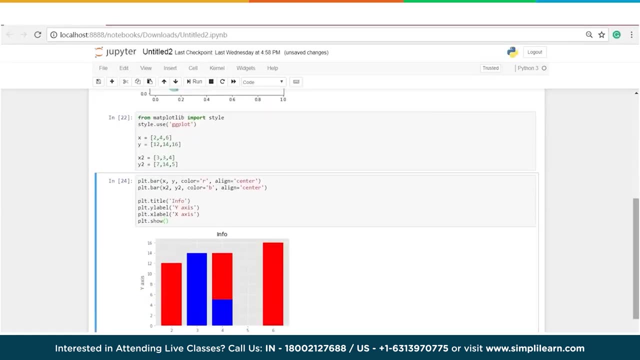 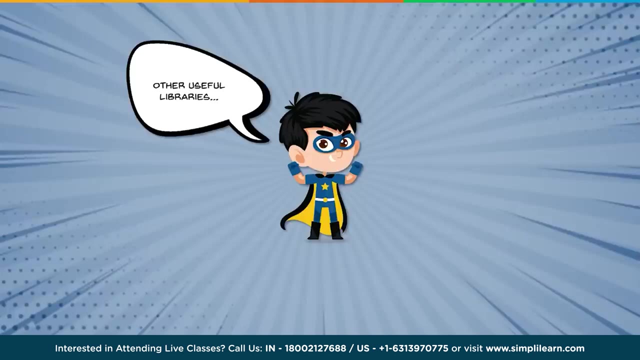 and alignment to the plot, and here we get the graph. So we can create different type of visualizations and plots and then work upon them using matplotlib. And it's just that simple. So that was about the leading Python libraries in the field of data science. But along with these libraries, data scientists are also leveraging the power. 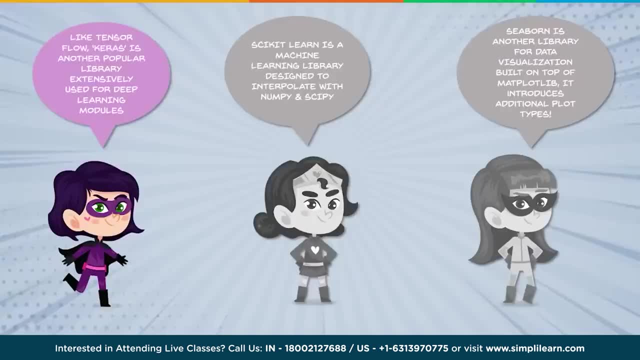 of some other useful libraries. For example, like TensorFlow, Keras is another popular library which is extensively used for deep learning and neural network modules. Keras wraps both TensorFlow and Theano backends, So it is a good option if you don't want to. 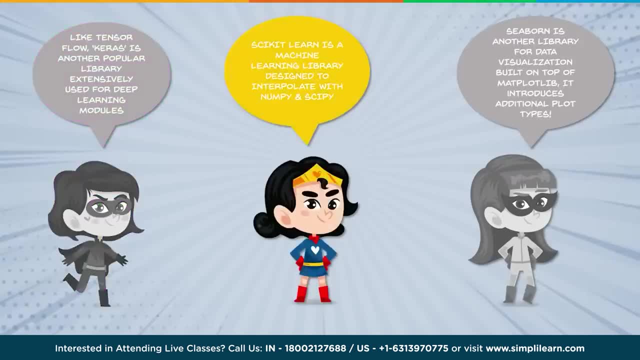 dive into details of TensorFlow. Then scikit-learn is a machine learning library. It provides almost all the machine learning algorithms that you need and it is designed to interpolate with NumPy and SciPy. Then we have Seaborn, which is another library for data visualization. 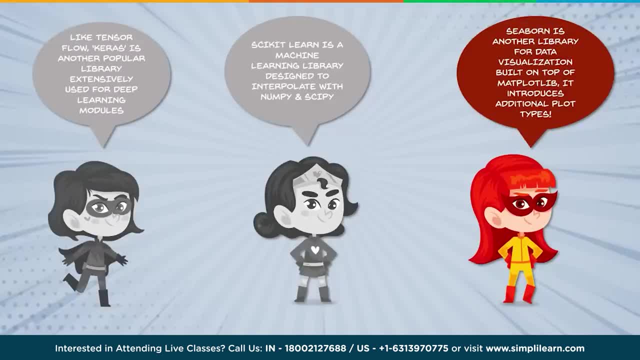 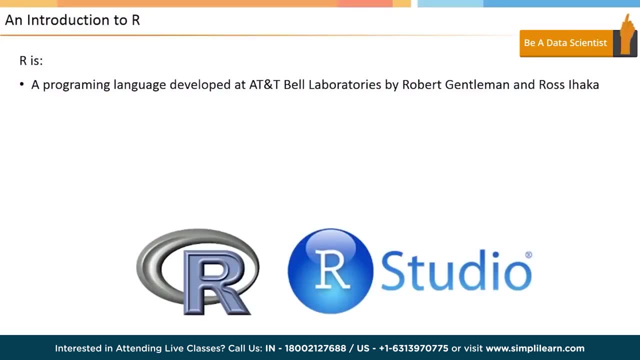 We can say that Seaborn is an enhancement of matplotlib, as it introduces additional plot types. R is a programming language for statistical computing and graphics. It was developed at AT&T Bell Laboratories by Robert Gentleman and Ross Ihaka. It's a GNU project and is 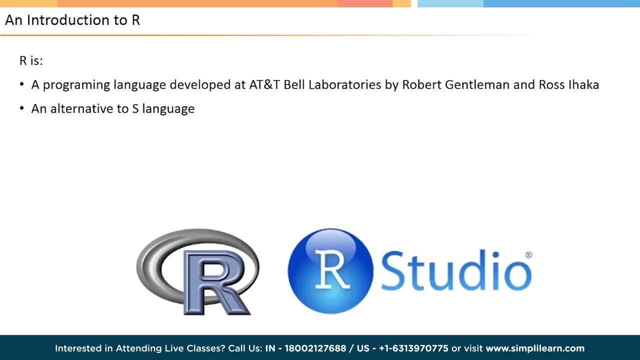 similar to the S language. It is considered as another implementation of S. However, there are a few important differences, but much of the code written for S can be run unchanged in R. R offers various statistical and graphical techniques which make it extensible. R is a free and open source language. The 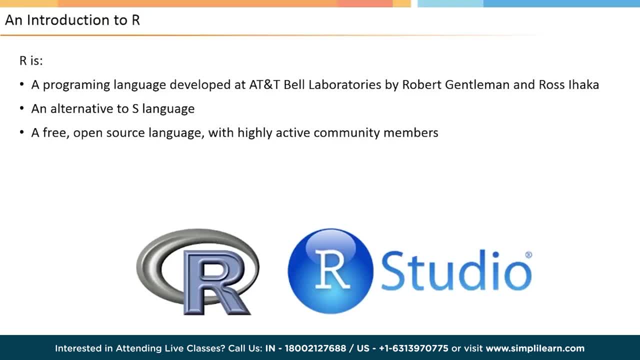 present. R is the result of contributions and collaborations from highly active community members from all over the world. R is capable of compiling and running code on all platforms, such as Linux, MAC and Windows. Due to its underlying philosophy and design, R is useful. 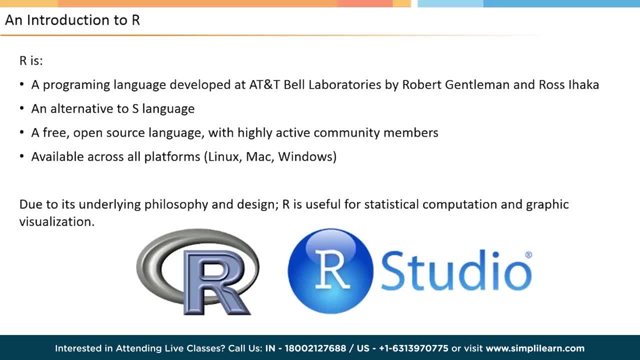 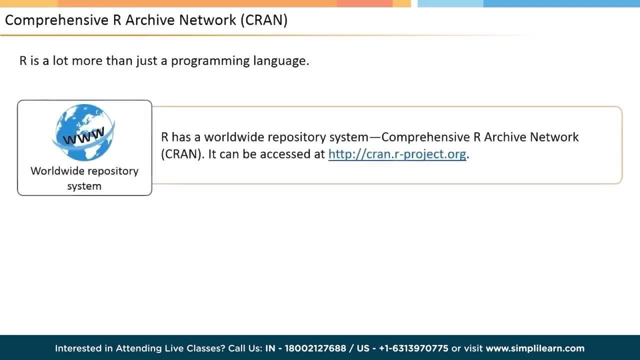 for statistical computation and graphic visualization. R is a lot more than just a programming language. It has a worldwide repository system called Comprehensive R Archive Network, or CRAN, which can be accessed through the given link. CRAN is a network of web servers and FTPs spread across the world. It is an extremely 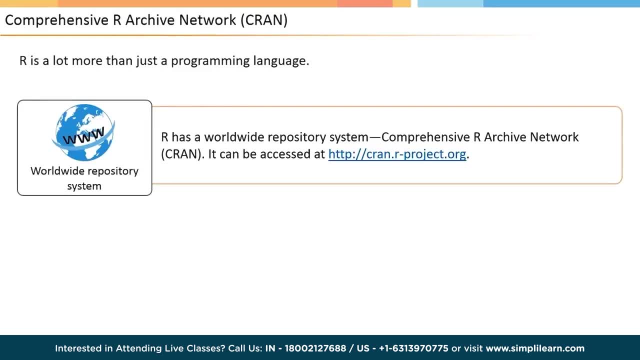 the world. This network stores similar codes and updated documentation of R. As per the data of 2011,, there were more than 3,000 packages hosted on CRAN, while there were many more on other websites as well. At present, the repository includes about 7,429 packages. 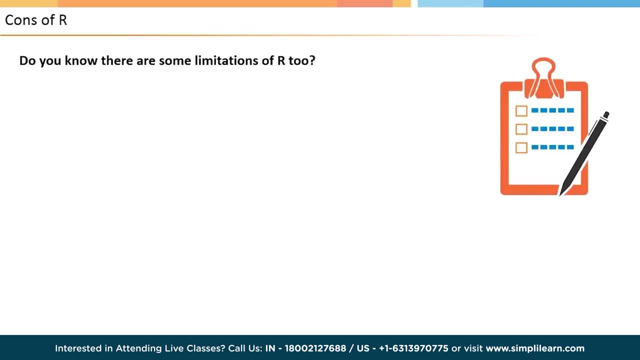 Do you know there are some limitations of R2?? One of the limitations is that it has a steep learning curve. It takes some time for a learner to understand the actual power of R. However, it's much better than other statistical languages. For a novice, it may be difficult to be understood. 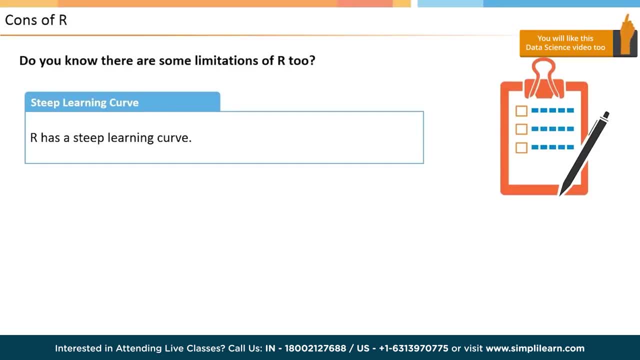 although there are a few easy-to-use GUIs available, but they do not offer the polish of the commercial offerings. Its documentation is sometimes very concise, which makes it less understandable for a non-statistician. However, a few high-standard books are trying to plug in. 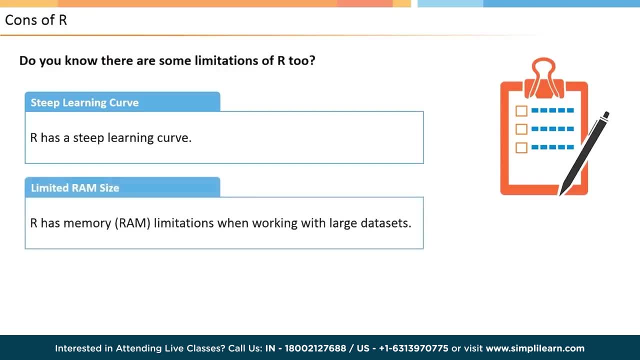 the documentation gaps. In addition, R has memory or RAM limitations. when working with large data sets, Its commands offer less attention to memory management, so they may consume all the available memory quickly. Therefore, when doing data mining, it can be a major restriction. 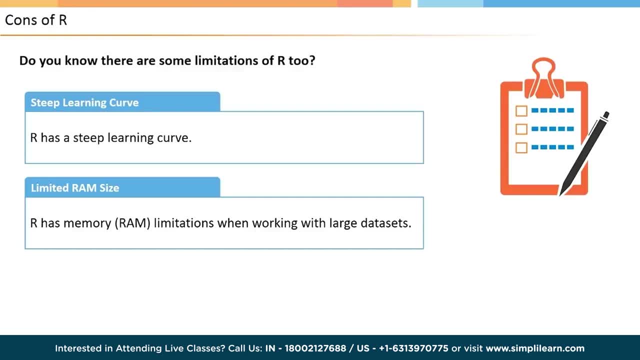 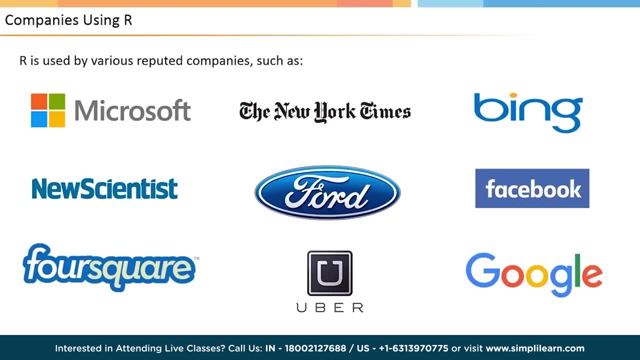 As a solution, one may choose to use 64-bit operating systems over 32-bit ones. Here is a list of various reputed companies that use R for various purposes. Microsoft uses it in video gaming for purposes like Xbox, matchmaking and scientific revenue. Using R developers can perform functions like identifying trouble spots. 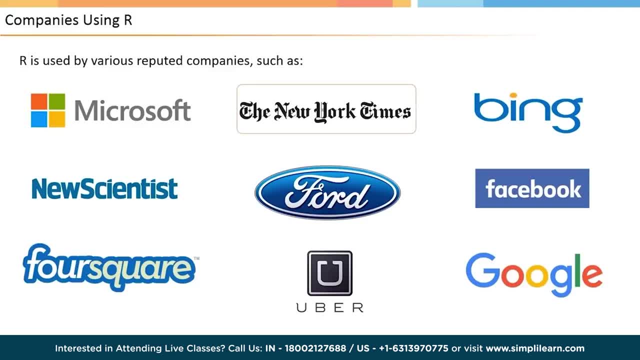 in game levels. The New York Times uses R for purposes like data visualization, data journalism and interactive features like election forecast and dialect quiz. Bing uses this language for social search awareness. The New Scientist magazine is another company that uses R for data visualization and data journalism. 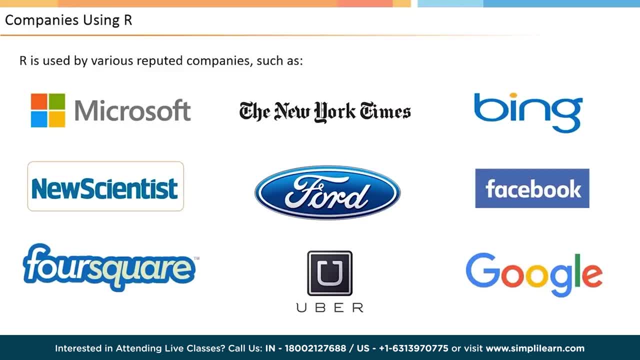 visualization, data journalism and the analysis of news articles. Ford uses R for data-driven decision-making. Facebook also uses it for purposes like experimental analysis, exploratory data analysis, human resources, big data visualization and the analysis of user behavior with respect to. 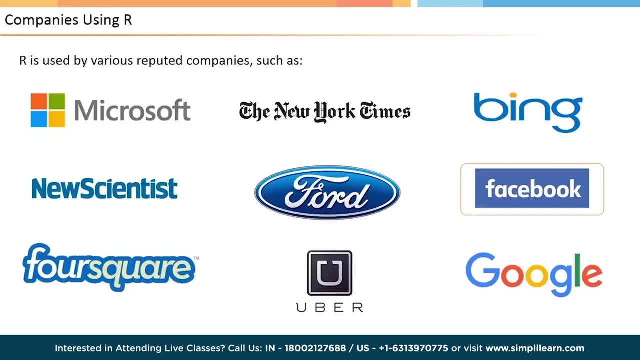 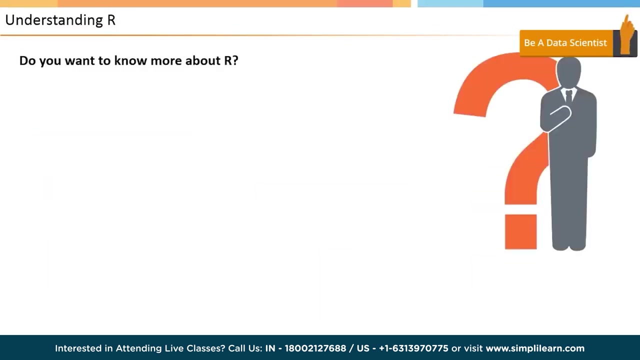 status updates and profile pictures. The famous recommendation engine of Foursquare is backed up by R. Uber uses R for the purpose of statistical analysis. In addition, Google uses it for economic forecasting, advertising effectiveness and big data statistical modeling. Do you want to know more about R? 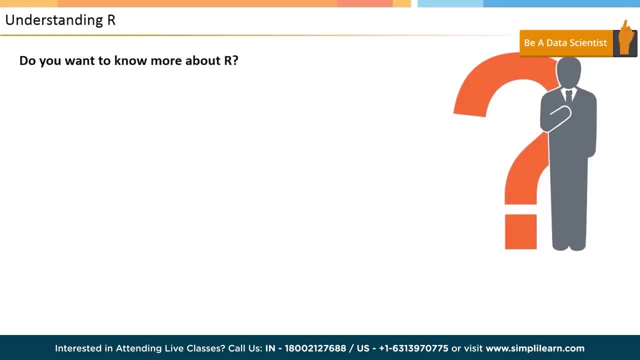 One of the main advantages of R is that users can write their custom functions and own programs with ease. The syntaxes are so easy to learn that even users with no programming experience can use them. R can be used as a powerful environment to do complex analyses on almost each data type. 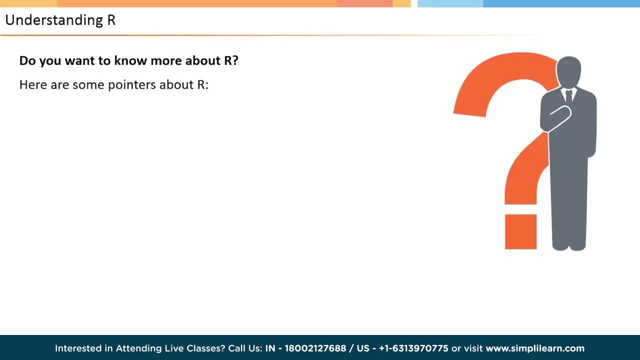 Here are a few more pointers that will help you understand R. R statements or commands can be separated by a semicolon or a new line. The assignment operator used in R is as given, although the equal-to operator also works. All characters after hash are treated as comments. 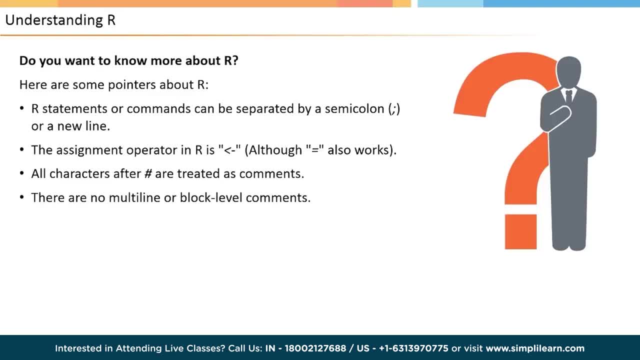 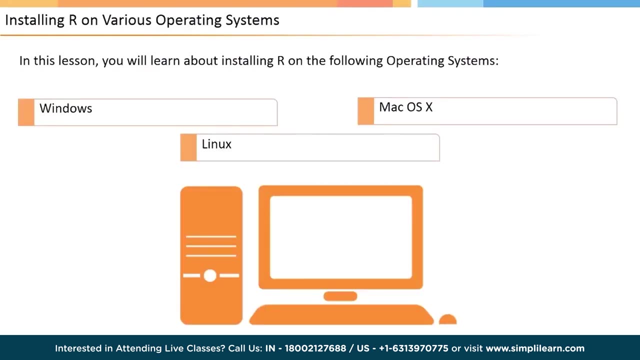 In addition, there are no multi-line or block-level comments. The dollar operator is analogous to a dot operator in other languages. The use of the operator is shown on the screen. In this lesson, you'll learn about installing R on operating systems including Windows, Mac OS X and Linux. 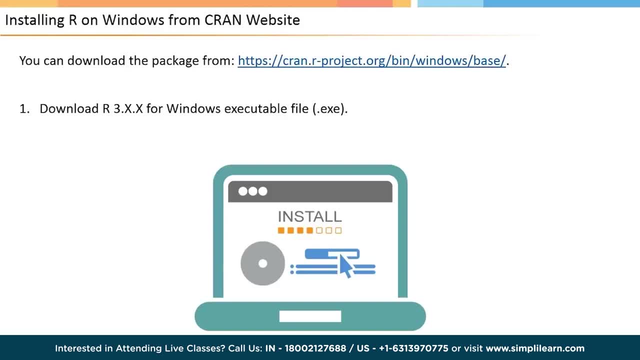 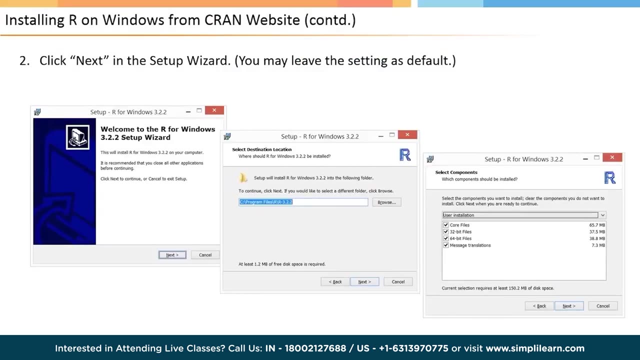 Let's first learn to install R on Windows from CRAN website. For this, you can download the package from the given website. As the first step, you would need to download the given Windows executable from this link. Once the package is downloaded, open the executable and follow the instructions. 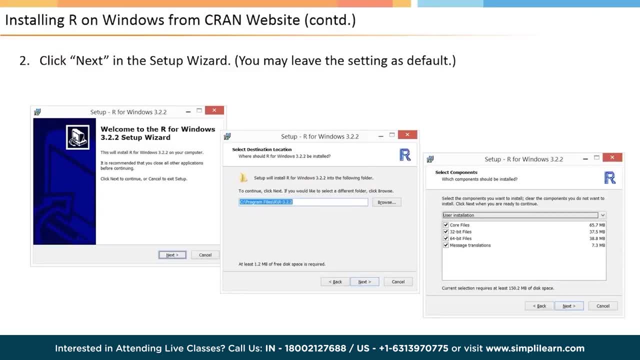 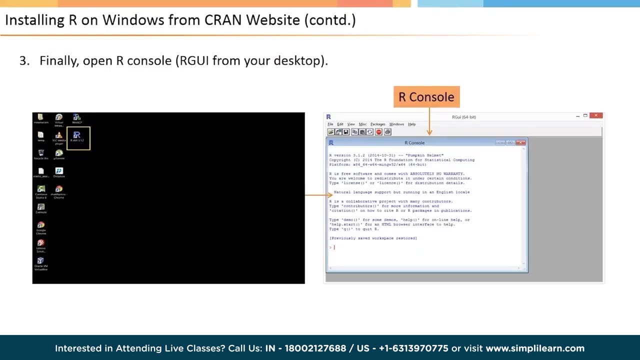 If you are installing R on a 64-bit Windows, the options will include 32 or 64-bit versions of R and the default is to install both. You can choose to leave the settings as default and click Next to proceed. Once you install R successfully, you will see its icon on the desktop. 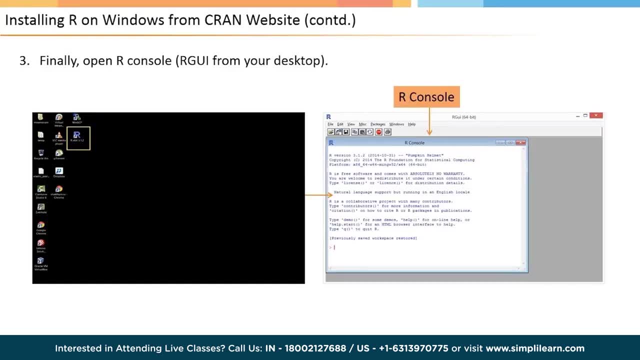 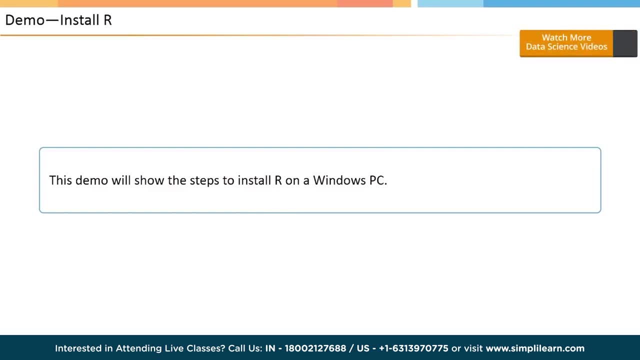 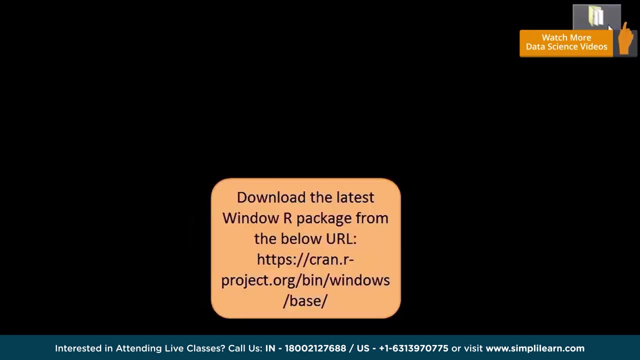 You can start the R console like any other program. This demo will show the steps to install R on a Windows PC. In this demo, you'll learn how to install R on a Windows PC. Download the latest R package from the given URL. 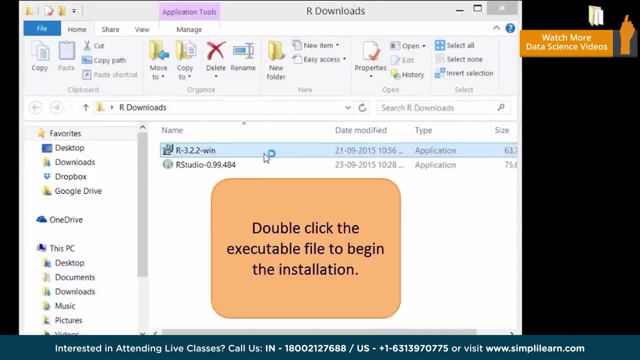 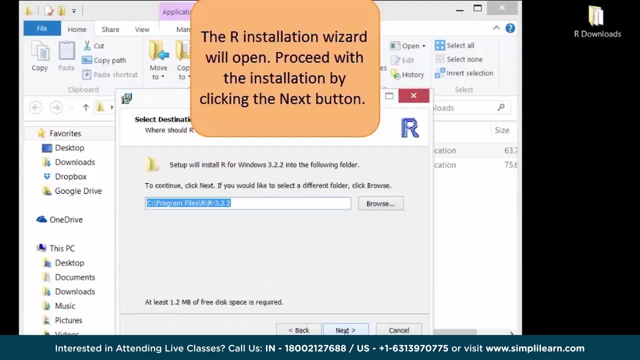 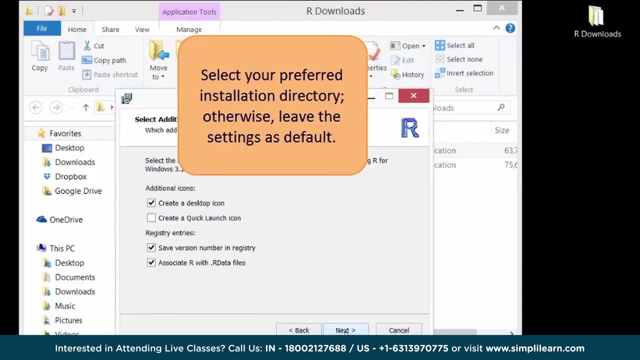 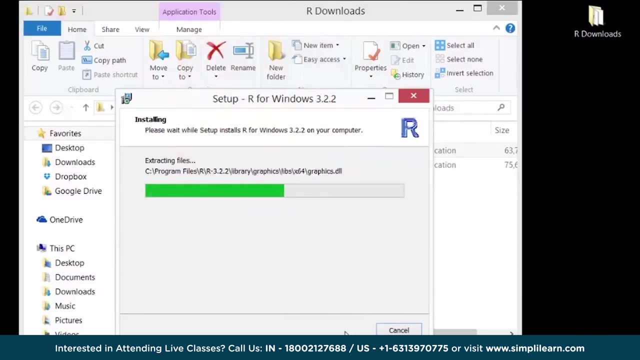 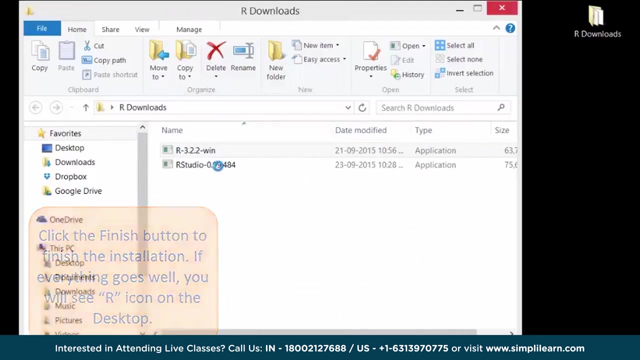 Double-click the executable file to begin the installation. The R installation wizard will open. Proceed with the installation by clicking the Next button. Select your preferred installation directory. Otherwise leave the settings as default. Click the Finish button to finish the installation. If everything goes well, you will see the R icon on the desktop. 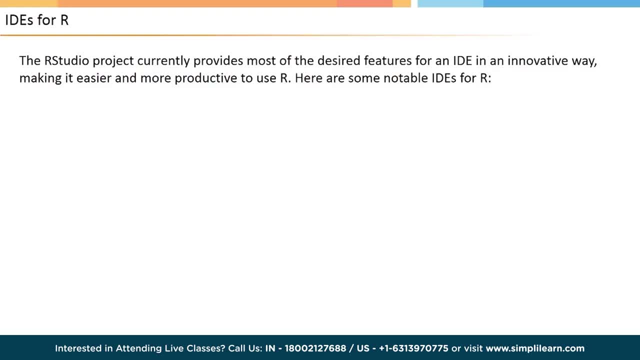 RStudio is an IDE or Integrated Development Environment for R. It's a project that provides most of the desired features for an IDE in an innovative way, which makes it easier and more productive to use. It includes a console and tools for history, plotting, workspace and debugging management. 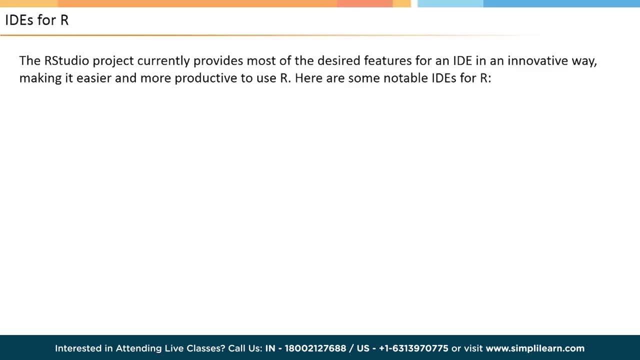 It also includes an editor that highlights the syntaxes, which supports execution of the code directly. Some other notable IDEs are listed in the table shown on the screen, along with the supported platforms. RStudio is available in various commercial and open-source editions. 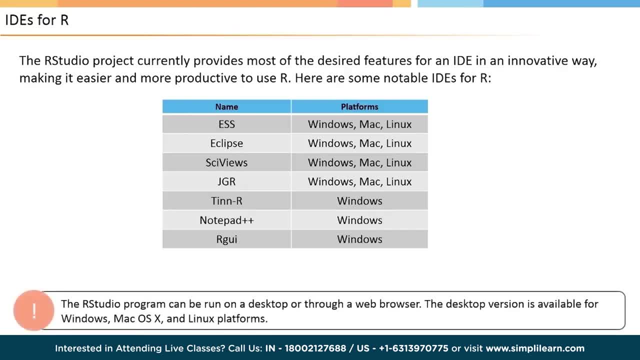 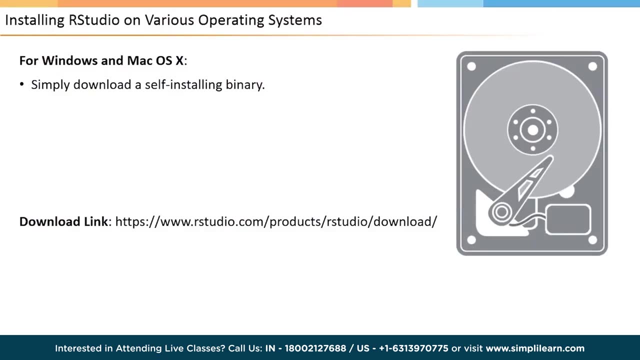 It can be run on a desktop or through a web browser connected to RStudio Server or RStudio Server Pro. The desktop version is available for Windows, Mac OS X and Linux platforms. To install RStudio on a Windows or Mac OS X system, you would need to simply download its self-installing binary. 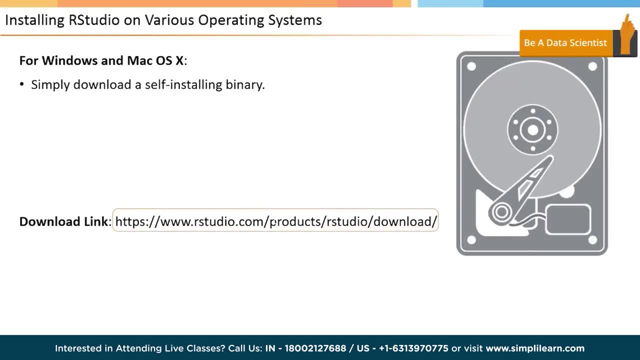 For this, you would need to go to the RStudio official website given on the screen and download the appropriate version for your system. Next, you would need to double-click the downloaded executable file and start the installation process. However, for Linux, the installation process varies. 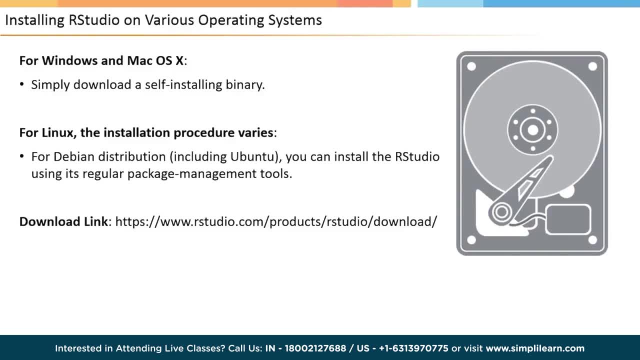 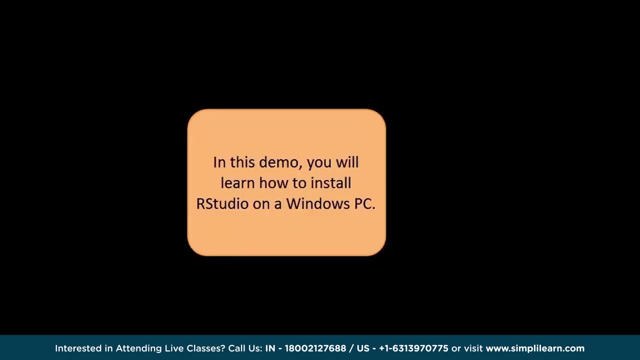 For Debian distribution, including Ubuntu. you can install the RStudio using its regular package management tools. This demo will show the steps to install RStudio on a Windows PC. In this demo, you'll learn how to install RStudio on a Windows PC. 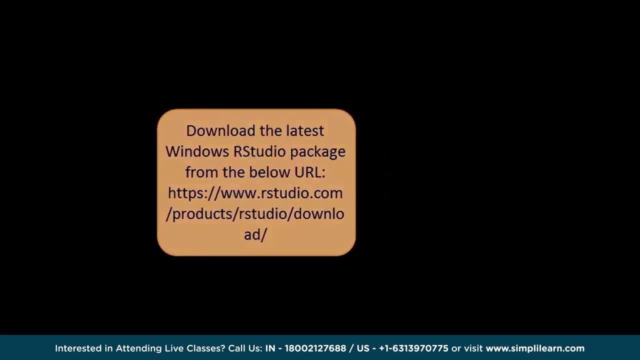 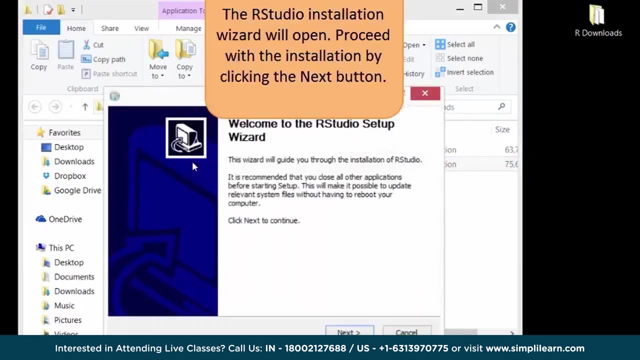 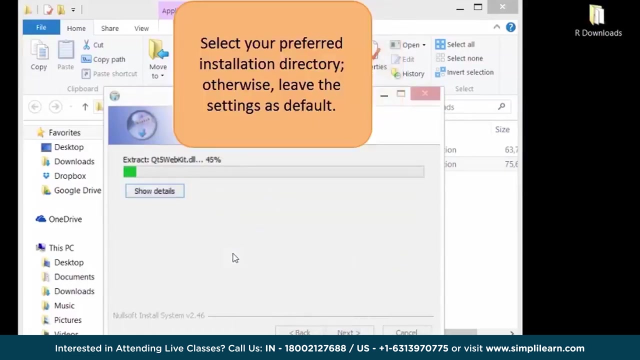 Download the latest Windows RStudio package from the given URL. Double-click the executable file to begin the installation. The RStudio installation wizard will open. Proceed with the installation by clicking the Next button. Select your preferred installation directory. Otherwise, leave the settings as default. 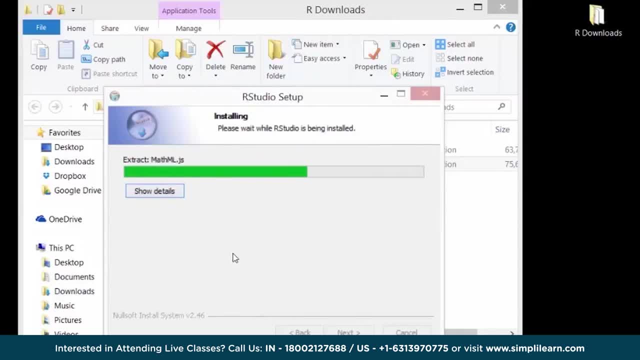 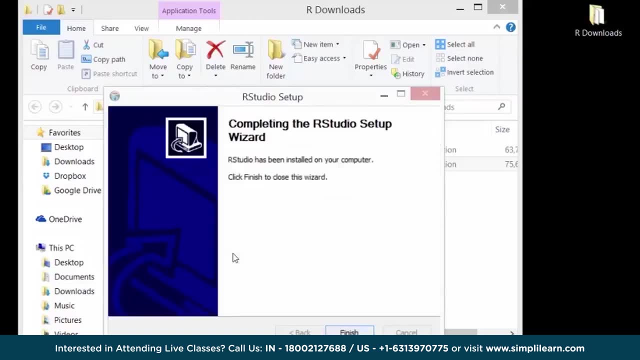 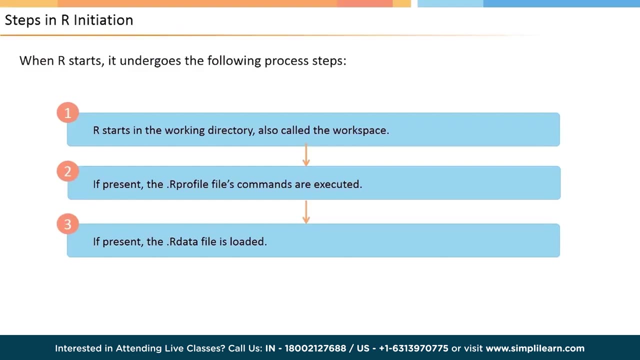 Click the Finish button to finish the installation. When R starts, it undergoes the process steps as shown on the screen. It starts in the working directory, which is also called the workspace. The rprofilefiles commands are executed next, if they are present. 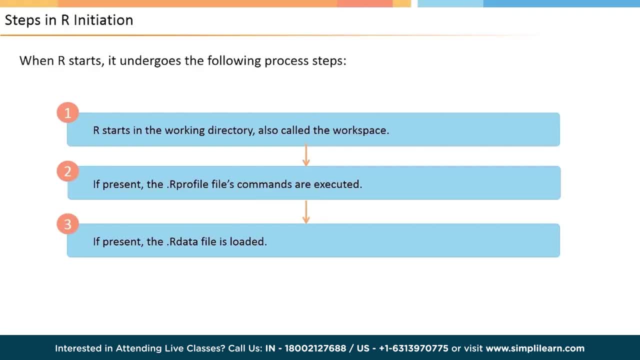 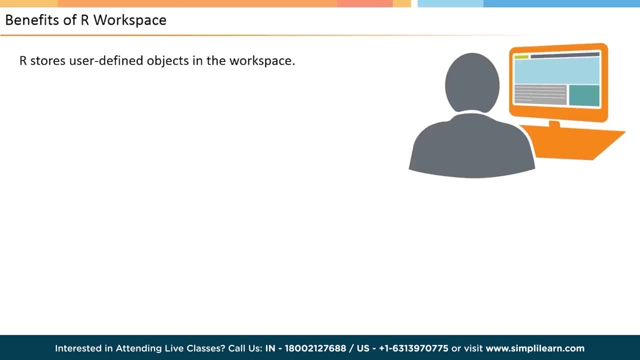 At the end, if present, the rdata file is loaded. The R workspace is the current working environment of R. It includes user-defined objects such as matrices, lists, data frames, functions and vectors. At the end of an R session, you can save a snapshot of the current workspace. 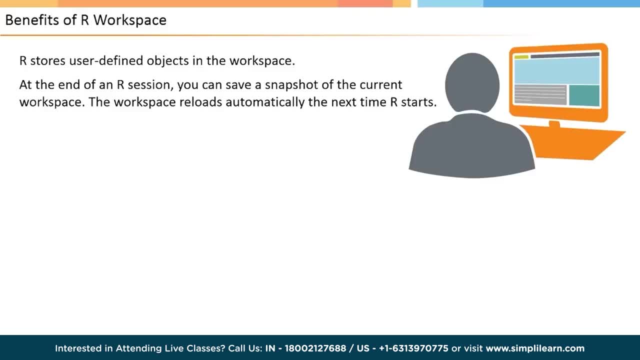 The workspace reloads automatically the next time R starts. In this you can enter commands interactively at the ruser prompt. You can also use up and down arrow keys to browse through your command history. Here are a few examples of such commands. 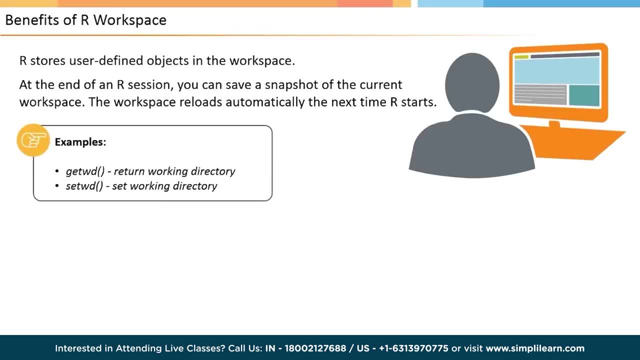 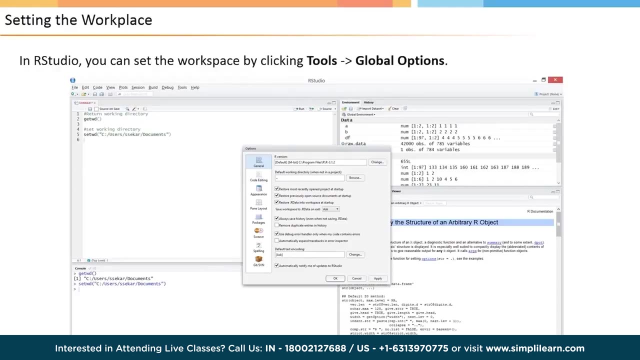 getwd is the command that prints the current working directory and setwd is the command that sets the working directory. To set the workspace in RStudio you can click Tools and then Global Options. as shown on the screen. R has many functions that can be used to perform sophisticated tasks. 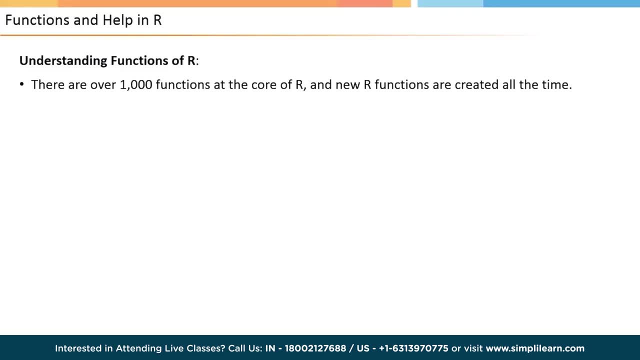 At the core, it has above 1,000 functions. In addition, several new ones are created all the time. Every function of R has its own help page. To access the same, you can type the name of the function in the console, preceded by a question mark. 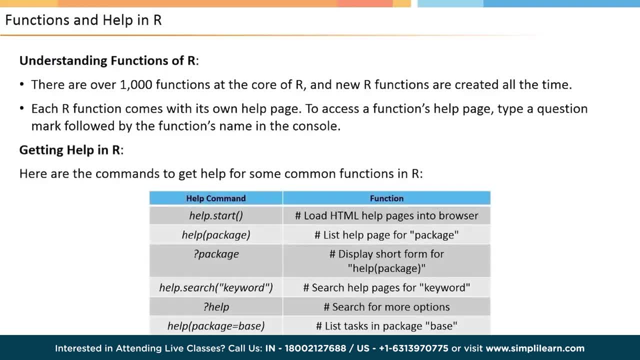 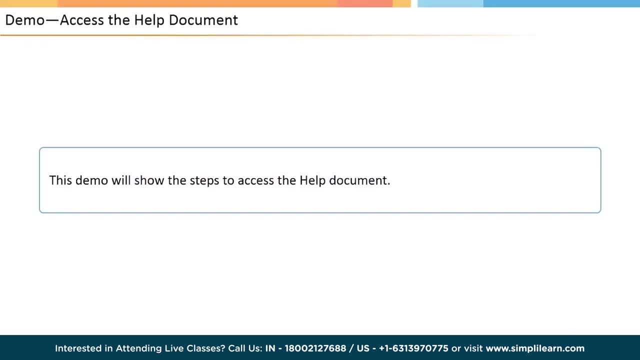 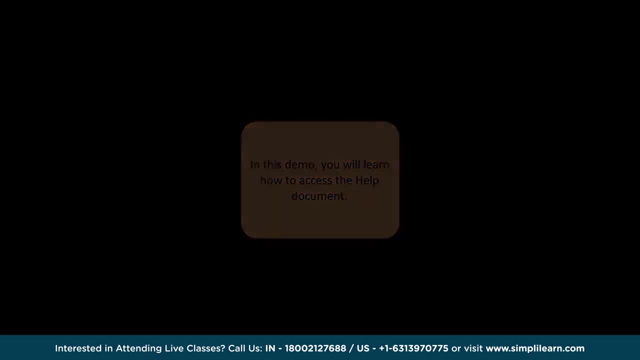 The table given on the screen shows the commands to get help for some common functions in R. This demo will show the steps to access the help document. In this demo you'll learn how to access the help document. To simply load the help document in a browser type: the given command. 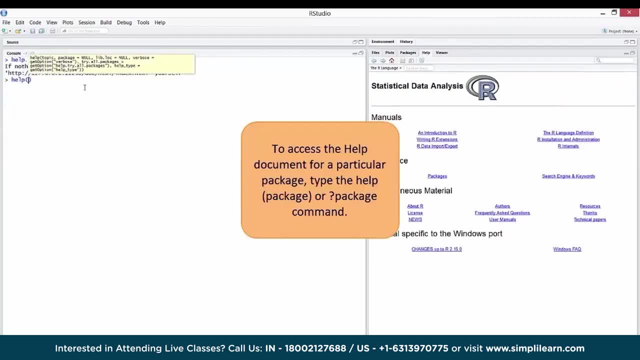 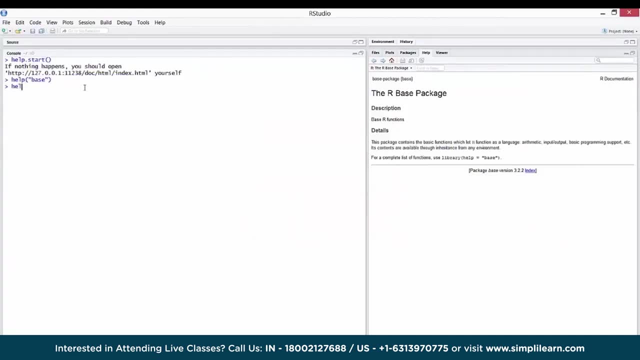 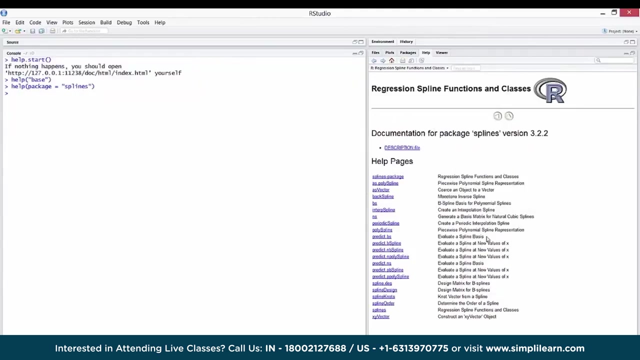 To access the help document for a particular package type: the given commands. To do so you can use a help function. You can also add one management Suture by clicking on it To access the help document by keyword: information in your CIFR type. the command in the console to identify the service. 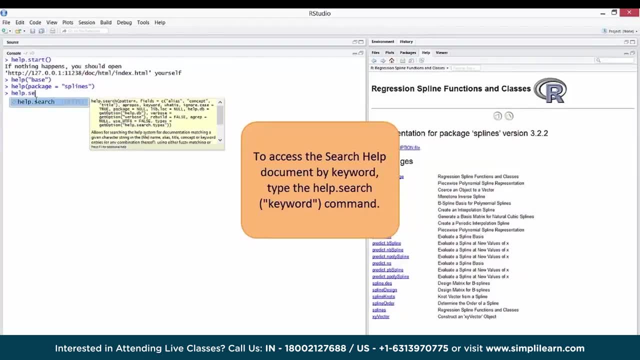 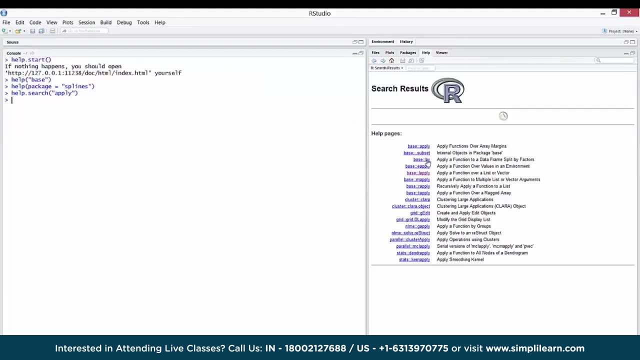 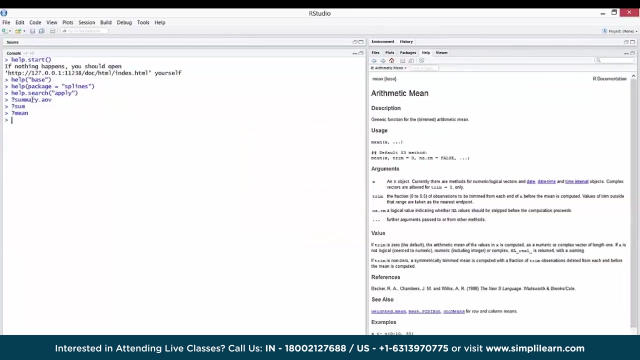 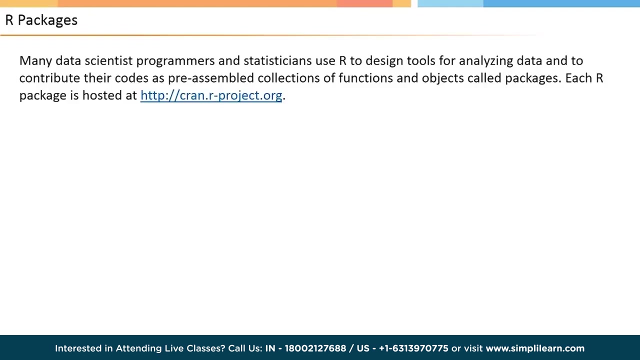 To access the help document by keyword: information type: thecapboard. For more help options, try using the name of functions or package prefixed with a question mark. A few examples are given on the screen. Many data scientist programmers and statisticians use R to design tools for analyzing data. 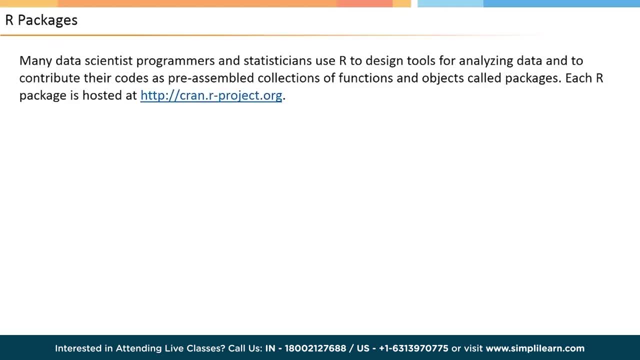 and to contribute their codes as preassembled collections of functions and objects called packages. R packages are defined as the collections of data, R functions and compiled data. These packages are stored in a directory called the library. All these packages are hosted at the given URL. 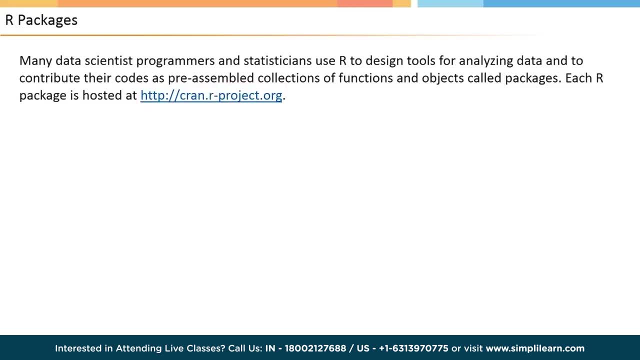 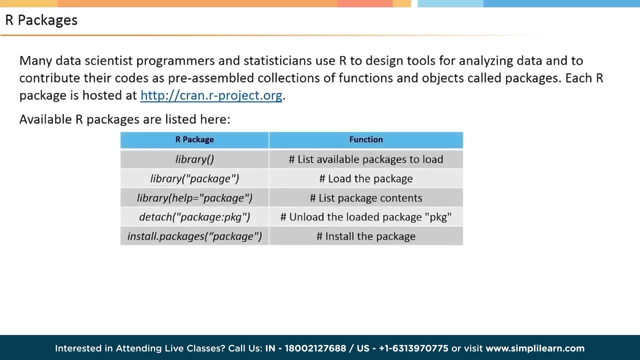 R includes a set of standard packages, while there are a few others that can be downloaded and installed. To use them, you would have to load them into a session. Some of the available R packages and their functions are listed in the given table. 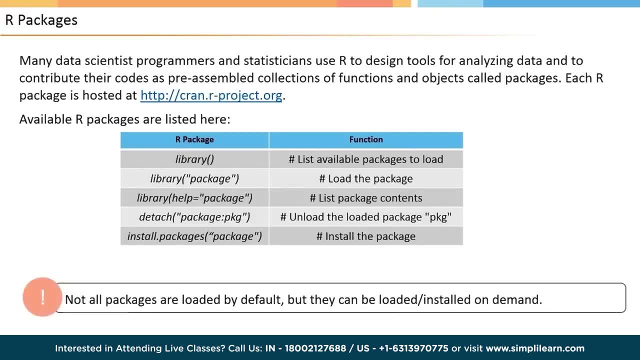 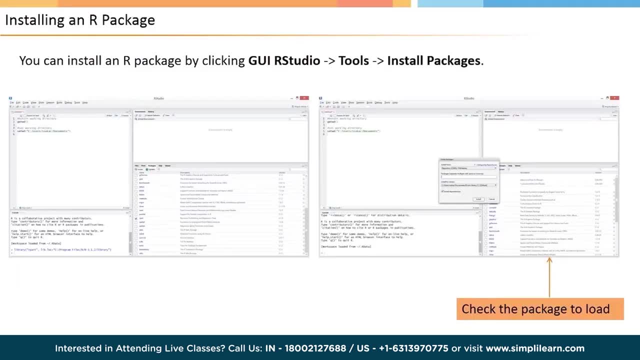 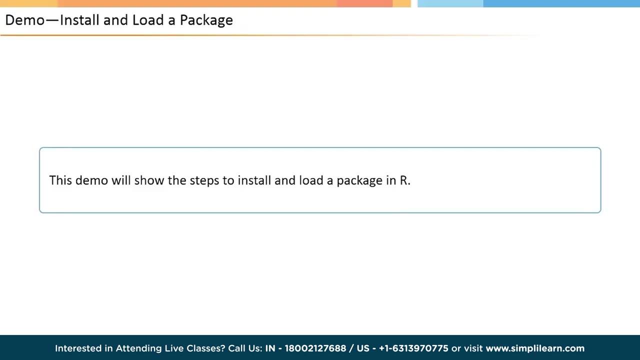 Note that not all packages are loaded by default, But they can be loaded or installed on demand. You can install an R package by clicking GUI R Studio Tools and then Install Packages as shown on the screen. This demo will show the steps to install and load a package in R. 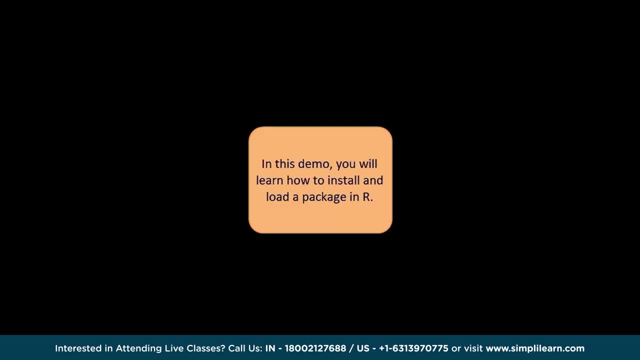 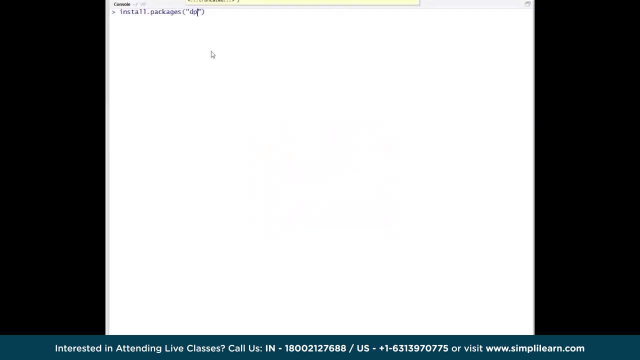 In this demo, you'll learn how to install and load a package in R. To install a package in R type: the given command. To load a package in R type: the given command. To list the contents of a package: type: the given command. 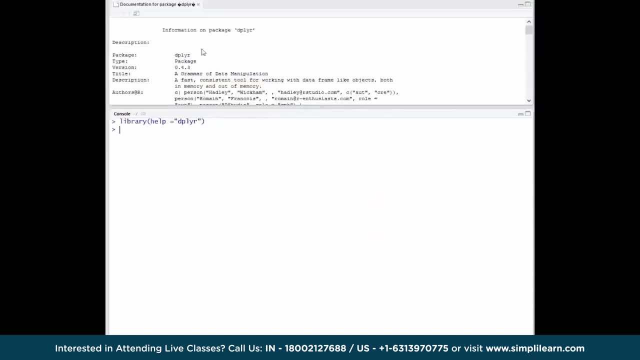 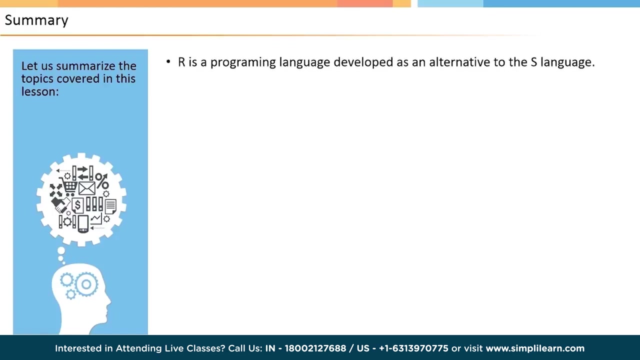 To send and send the package to a destination place: type the given command. To download a package: type the given command. Let's summarize the topics covered in this lesson. R is a programming language developed as an alternative to the S language. R is available across all platforms: Windows, Mac and Linux. 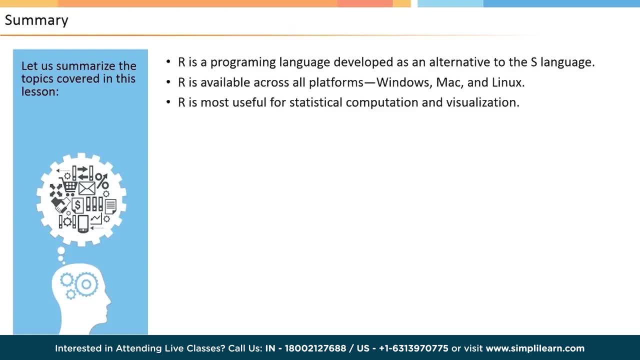 R is most useful for statistical computation and visualization. R has a steep learning curve and its working with large datasets is limited by the RAM size. R can be downloaded from the CRAN website. The RStudio program can run on a desktop or through a web browser. 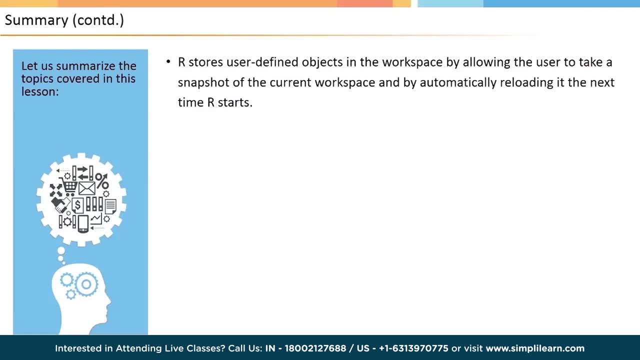 R stores user-defined objects in the workspace by allowing the user to take a snapshot of the current workspace and by automatically reloading it the next time R starts. Each R function comes with its own help page. Not all packages are loaded by default, but can be loaded or installed on demand. 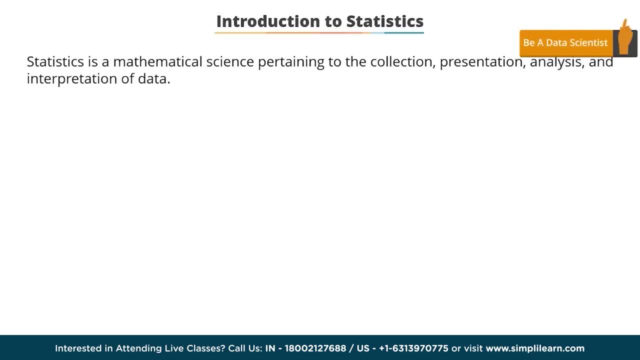 Let's begin this lesson by defining the term statistics. Statistics is a mathematical science. It pertains to the collection, presentation, analysis and interpretation of data. It's widely used to understand the complex problems of the real world and simplify them, to make well-informed decisions. 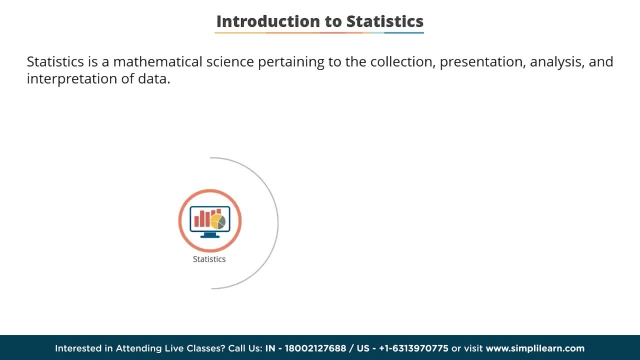 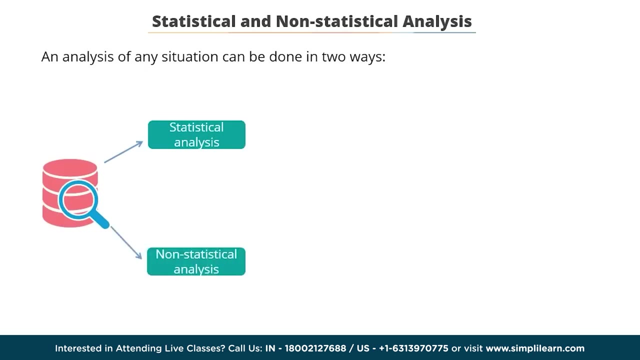 Several statistical principles, functions and algorithms can be used to analyze primary data, build a statistical model and predict the outcomes. An analysis of any situation can be done in two ways: statistical analysis or a non-statistical analysis. Statistical analysis is the science of collecting, exploring and presenting large amounts of data. 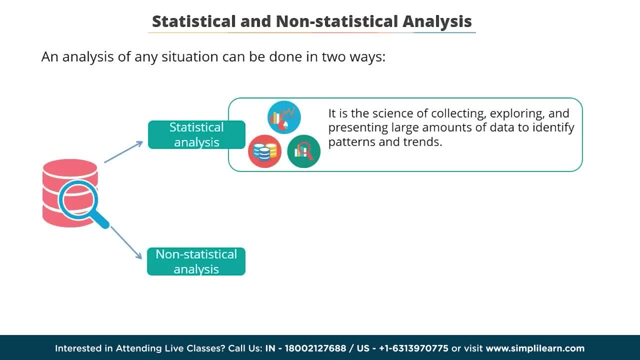 to identify the patterns and trends. Statistical analysis is also called quantitative analysis. Non-statistical analysis provides generic information and includes text, sound still images and moving images. Non-statistical analysis is also called qualitative analysis, Although both forms of analysis provide results. 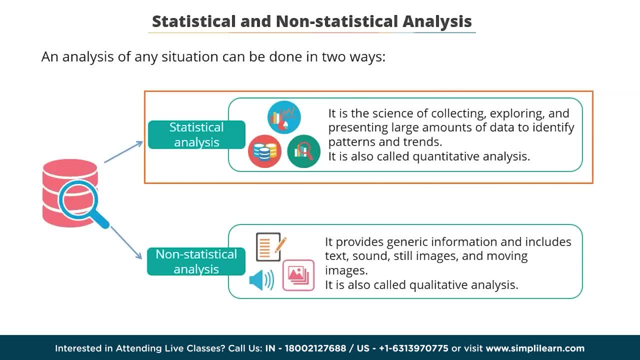 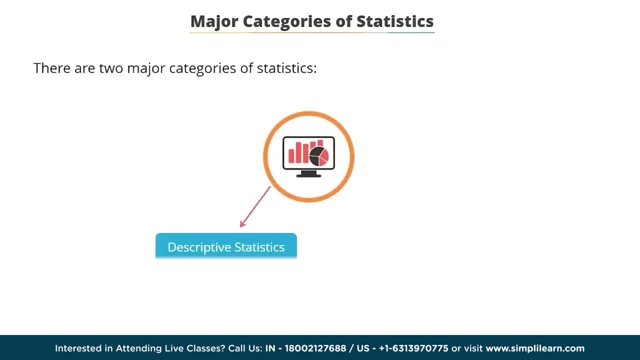 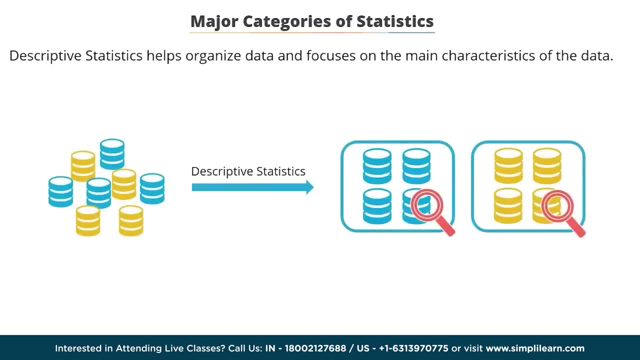 statistical analysis is also called quantitative analysis. Statistical analysis gives more insight and a clearer picture, a feature that makes it vital for businesses. There are two major categories of statistics: descriptive statistics and inferential statistics. Descriptive statistics helps organize data and focuses on the main characteristics of the data. 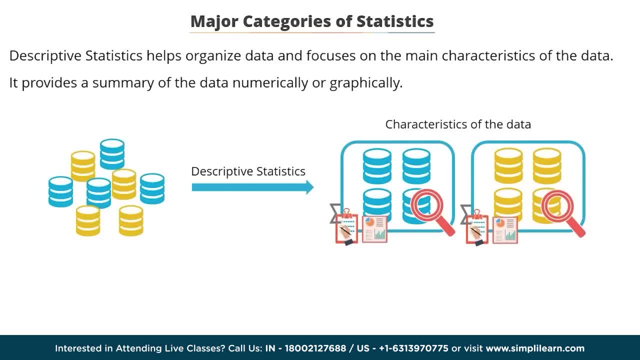 It provides a summary of the data, numerically or graphically. Numerical measures, such as average mode, standard deviation or SD, and correlation are used to describe the data. It is a source of information and a data source to describe the features of a data set. 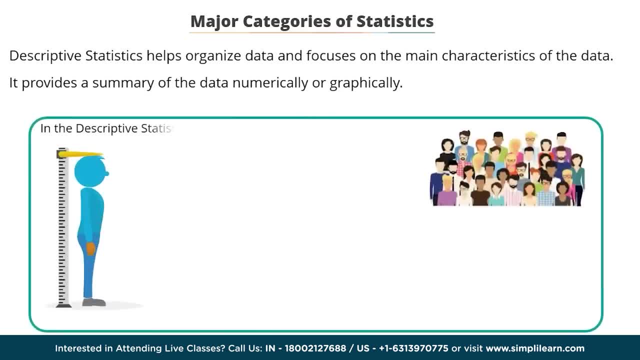 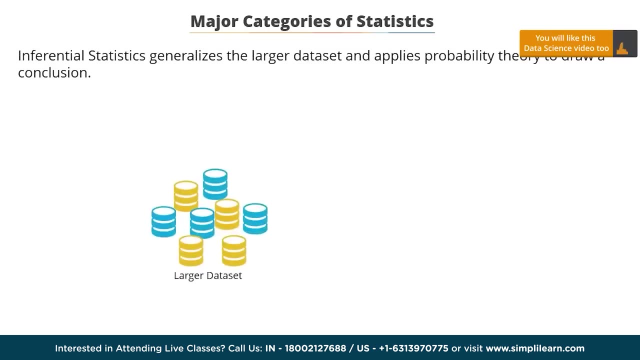 Suppose you want to study the height of students in a classroom. In the descriptive statistics you would record the height of every person in the classroom and then find out the maximum height, minimum height and average height of the population. Inferential statistics generalizes the larger data set. 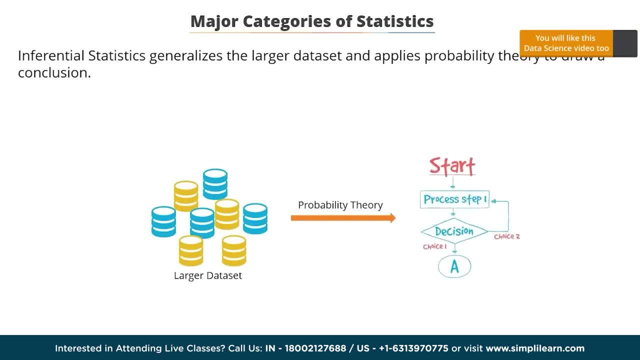 and applies probability theory. to draw a conclusion, It allows you to infer population parameters based on the sample statistics and to model relationships with the data sets. the data modeling allows you to develop mathematical equations which describe the interrelationships between two or more variables. consider the same example. 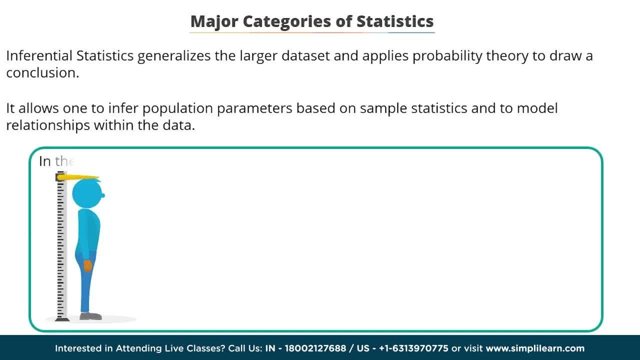 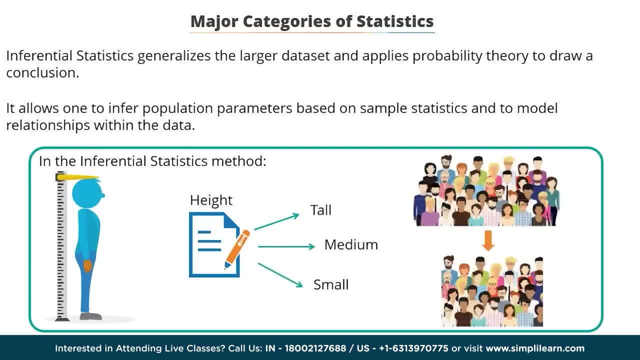 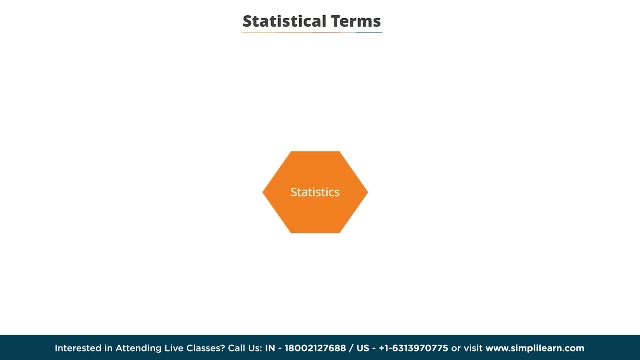 of calculating the height of students in the classroom. in inferential statistics you would categorize height as tall, medium and small and then take only a small sample from the population to study the height of students in the classroom. the field of statistics touches our lives in many ways, from the 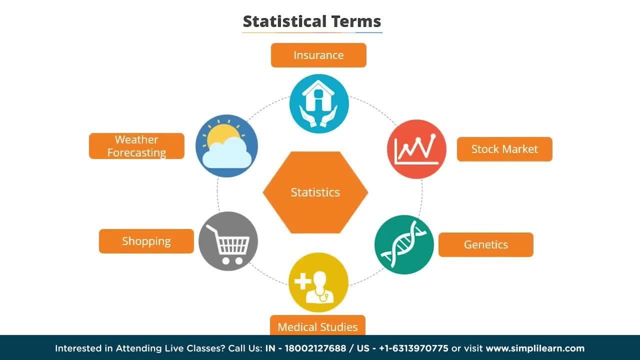 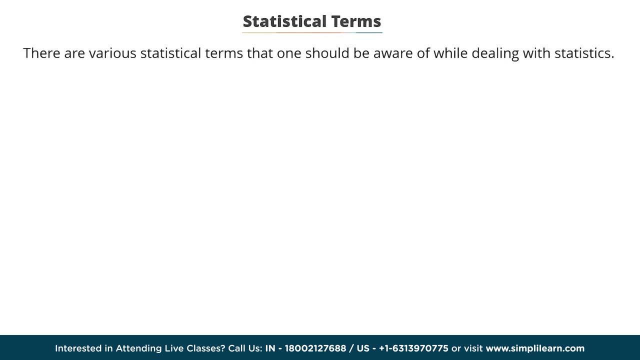 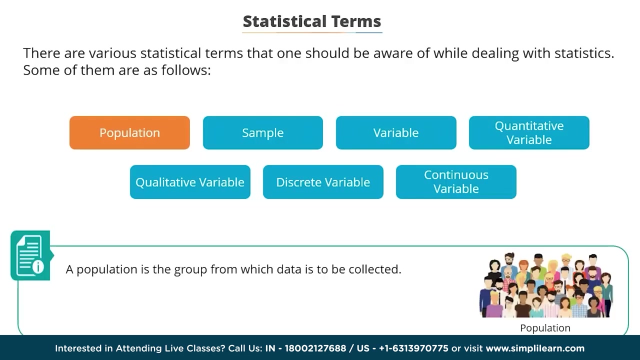 daily routines in our homes to the business of making the greatest cities run. the effect of statistics are everywhere. there are various statistical terms that one should be aware of while dealing with statistics: population, sample variable, quantitative variable, qualitative variable, discrete variable, continuous variable. a population is the group from which data 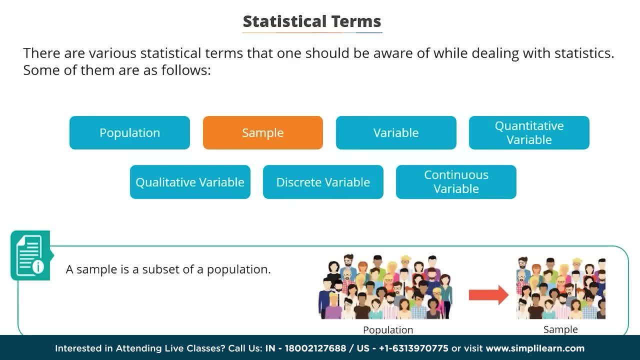 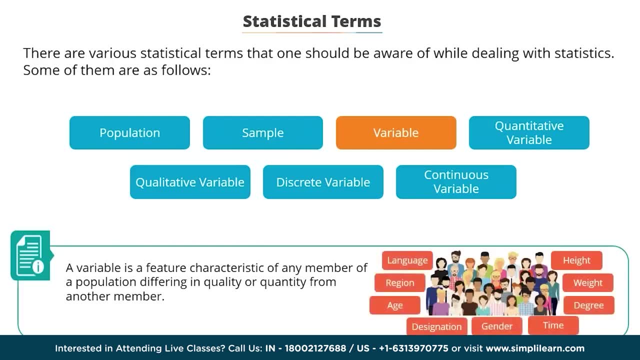 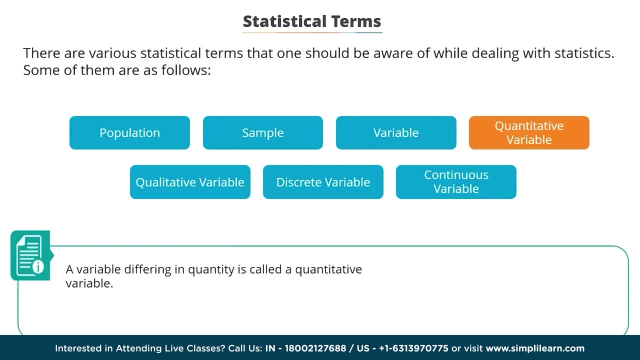 is to be collected. a sample is a subset of a population. A variable is a feature that is characteristic of any member of the population differing in quality or quantity from another member. A variable differing in quantity is called a quantitative variable. for example, the weight of a person, number of people in a car. 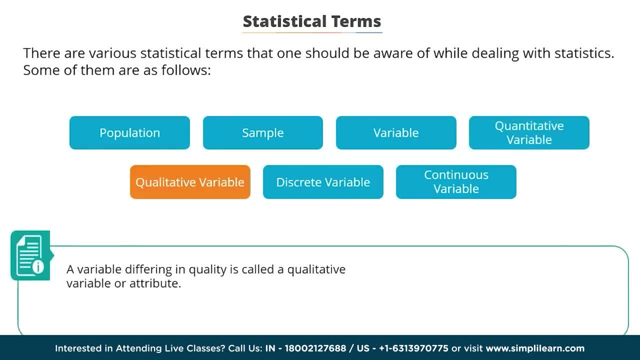 A variable differing in quality is called a qualitative variable or attribute, for example, color, the degree of damage of a car in an accident. A discrete variable is one which no value can be assumed between the two given values, for example the number of children in a family. 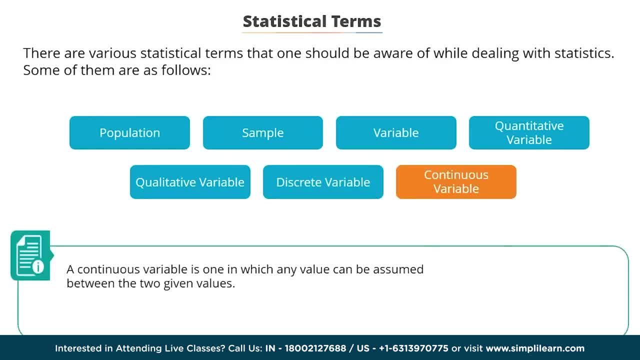 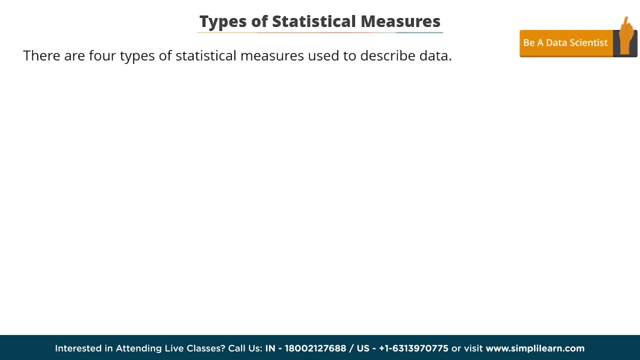 A continuous variable is one in which any value can be assumed between the two given values, for example the time taken for a 100-meter run. Typically, there are four types of statistical measures used to describe the data. They are measures of frequency. 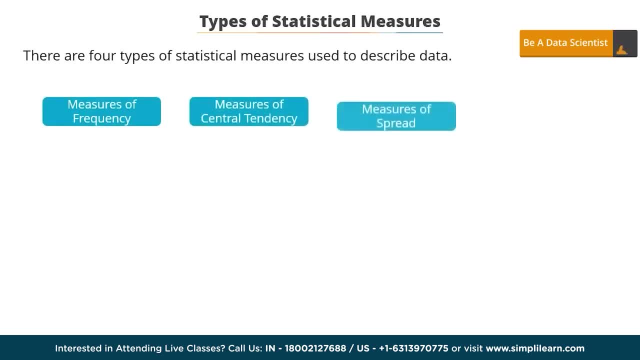 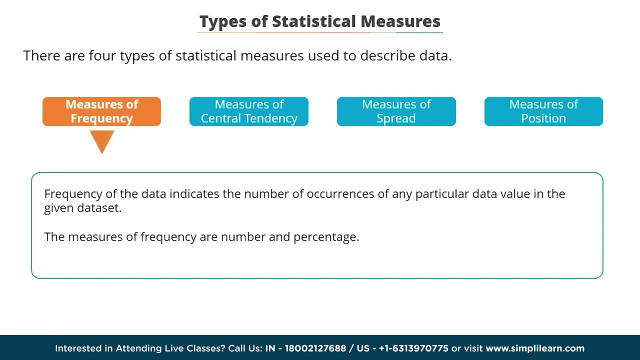 measures of central temperature, measures of tendency, measures of spread, measures of position. Let's learn each in detail. Frequency of the data indicates the number of times a particular data value occurs in the given data set. The measures of frequency are number and percentage. 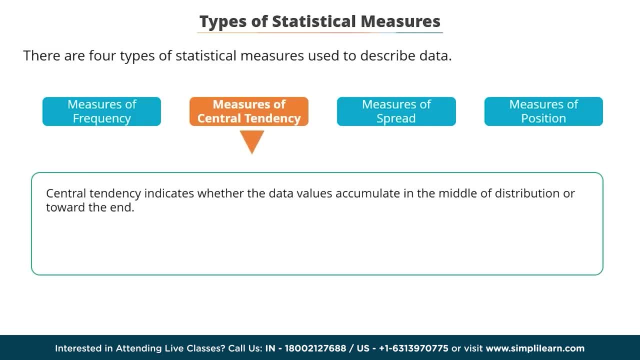 Central tendency indicates whether the data values tend to accumulate in the middle of the distribution or toward the end. The measures of central tendency are mean, median and mode. Spread describes how similar or varied the set of observed values are for a particular variable. 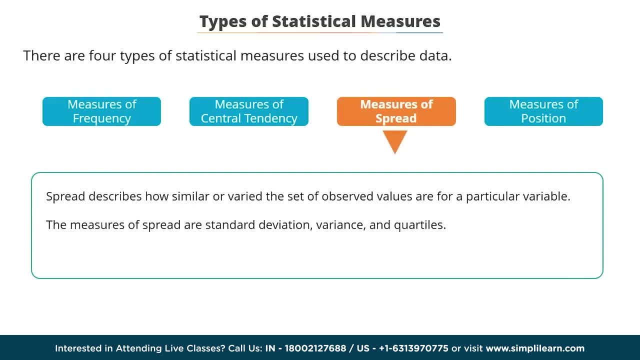 The measures of spread are standard, deviation, variance and quartiles. The measures of spread are also called measures of dispersion. Position identifies the exact location of a particular data value in the given data set. The measures of position are percentiles, quartiles and standard scores. 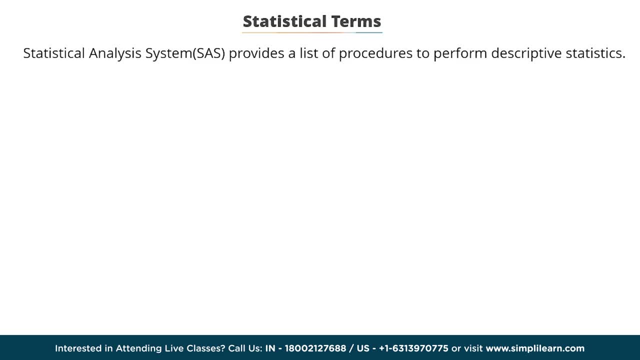 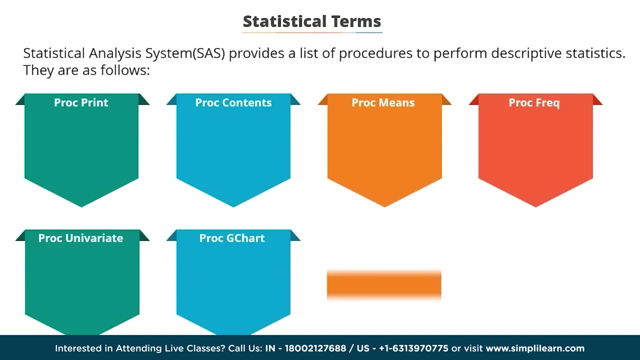 Statistical Analysis System, or SAS, provides a list of procedures to perform descriptive statistics. They are as follows: PROC PRINT. PROC CONTENTS, PROC MEANS. PROC FREQUENCY, PROC UNIVARIATE. PROC GCHART. PROC BOXPLOT. PROC GPLOT. PROC PRINT. 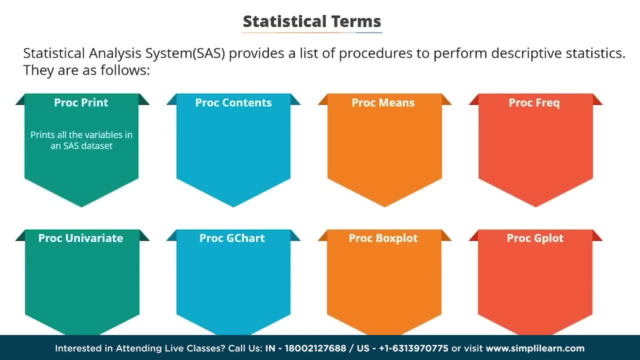 It prints all the variables in a SAS data set: PROC CONTENTS. It describes the structure of a data set: PROC MEANS. It provides data summarization tools to compute descriptive statistics for variables across all observations and within the groups of observations: PROC FREQUENCY. 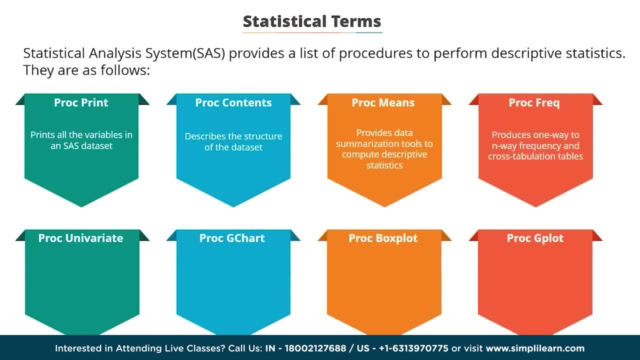 It produces one-way to n-way frequency and cross-tabulation tables. Frequencies can also be an output of a SAS data set, PROC UNIVARIATE. It goes beyond what PROC MEANS does and is useful in conducting some basic statistical analyses and includes high-resolution graphical features. 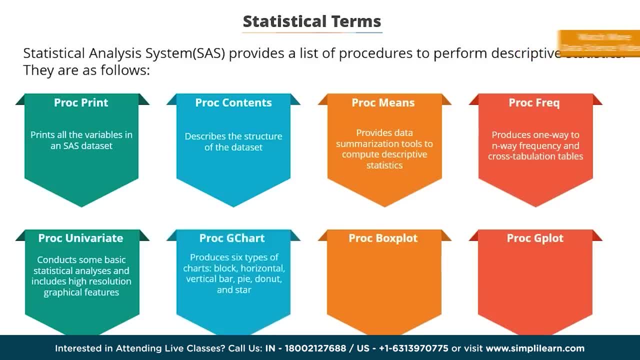 PROC GCHART. The GCHART procedure produces six types of charts: block charts, horizontal vertical bar charts, pie doughnut charts and star charts. These charts graphically represent the value of a statistic calculated for one or more variables in an input SAS data set. 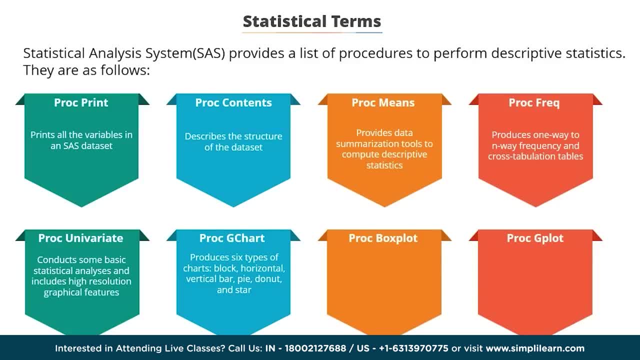 The charted variables can be either numeric or character. PROC BOXPLOT. The boxplot procedure creates side-by-side box-and-whisker plots of measurements organized in groups. A box-and-whisker plot displays the mean quartiles and minimum and maximum observations for a group. 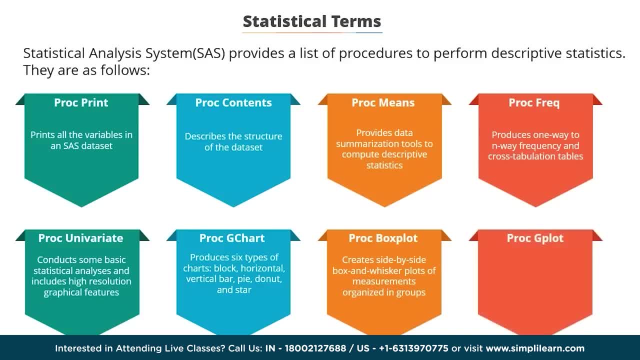 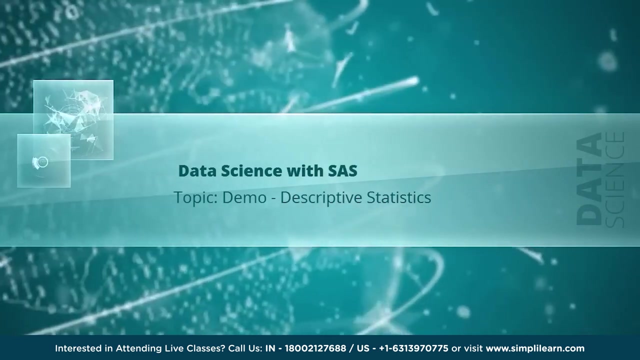 PROC GPLOT. GPLOT procedure creates two-dimensional graphs including simple scatterplots, overlay plots in which multiple sets of data points are displayed on one set of axes, plots against a second vertical axis, bubble plots and logarithmic plots. In this demo, you'll learn how to use descriptive statistics to analyze the mean from the electronic data set. 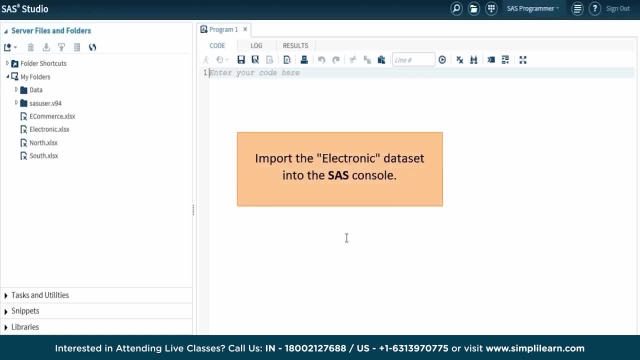 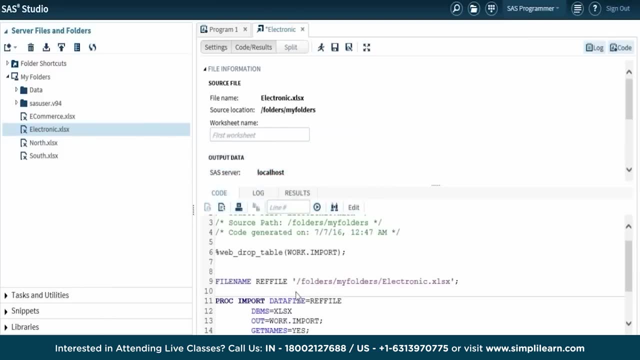 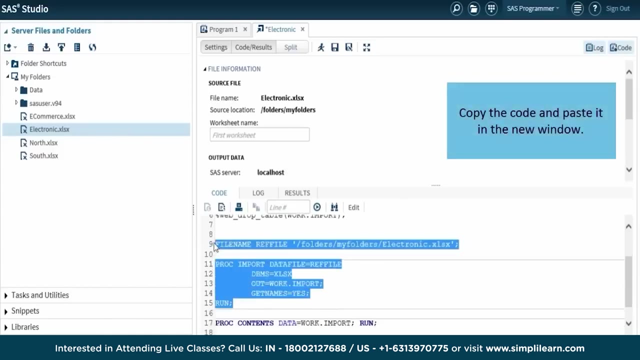 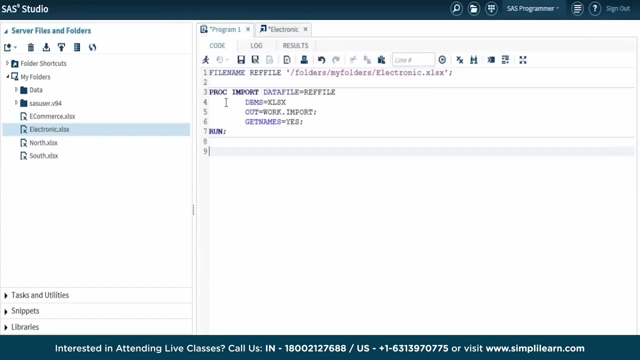 Let's import the electronic data set into the SAS console. In the left plane, right-click the electronic xlsx data set and click Import Data. The code to import the data generates automatically. Copy the code and paste it in the new window. The PROC MEANS procedure is used to analyze the mean of the imported data set. 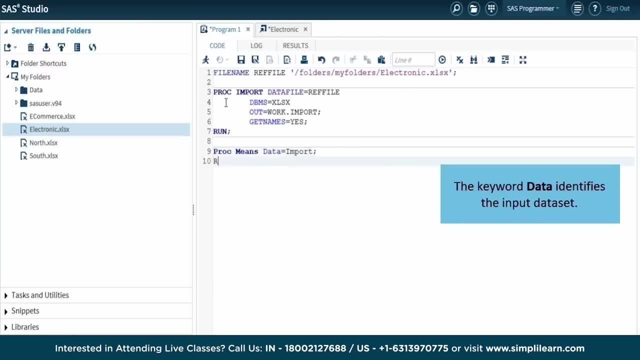 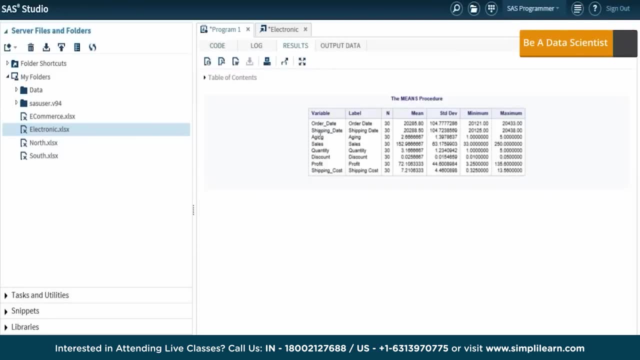 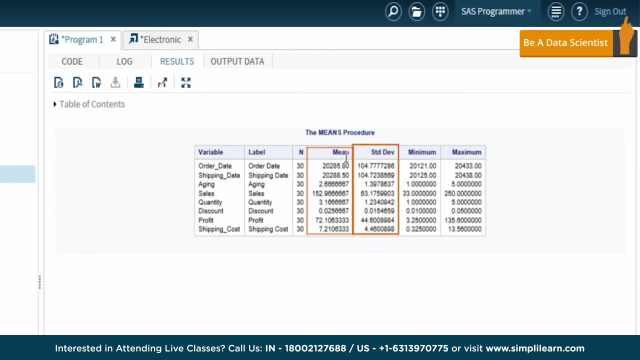 The keyword DATA identifies the input data set. In this demo, the input data set is electronic. The output obtained is shown on the screen. Note that the number of observations mean standard deviation and maximum and minimum values of the electronic data set are obtained. 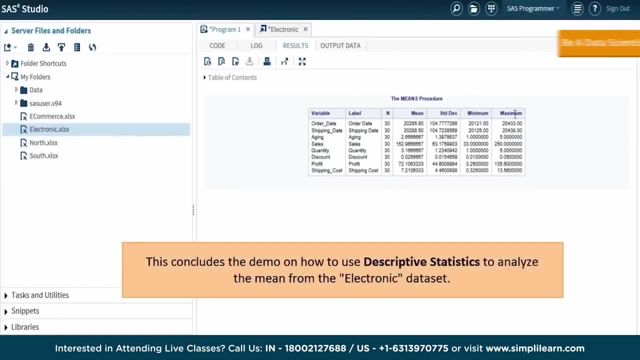 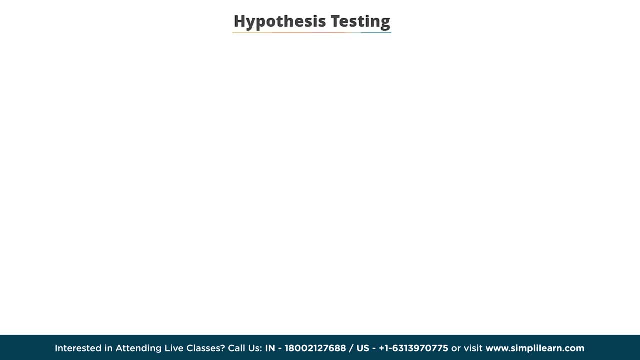 This concludes the demo on how to use descriptive statistics to analyze the mean from the electronic data set. So far you have learned about descriptive statistics. Let's now learn about inferential statistics. Hypothesis testing is an inferential statistical technique to determine whether there is enough evidence in a data sample. 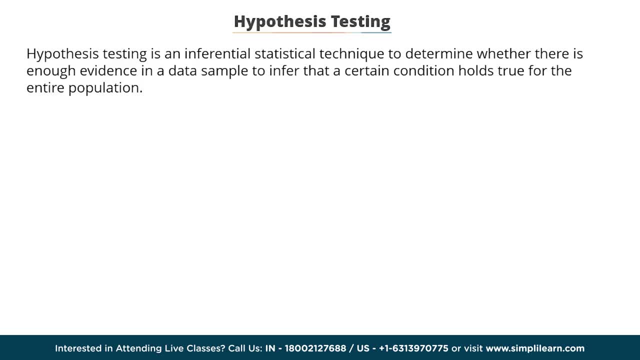 to infer that a certain condition holds true for the entire population. To understand the characteristics of the general population, we take a random sample and analyze the properties of the sample. We then test whether or not the identified conclusions correctly represent the population as a whole. 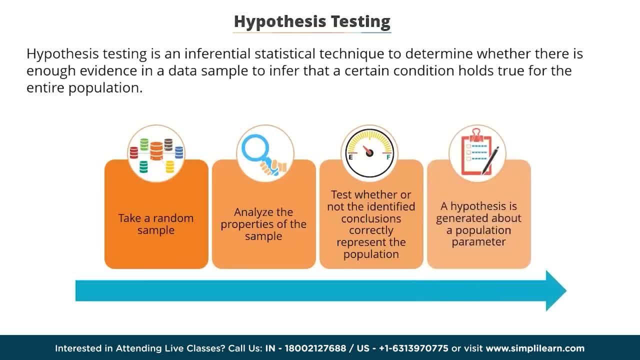 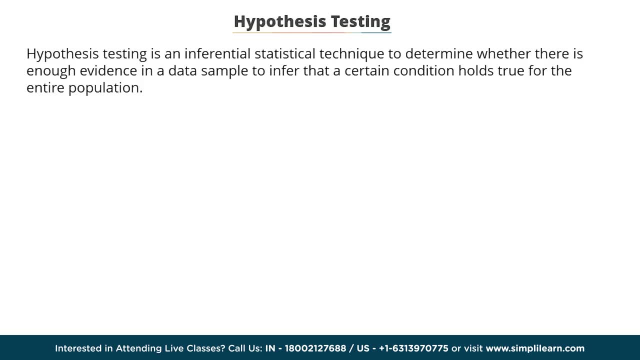 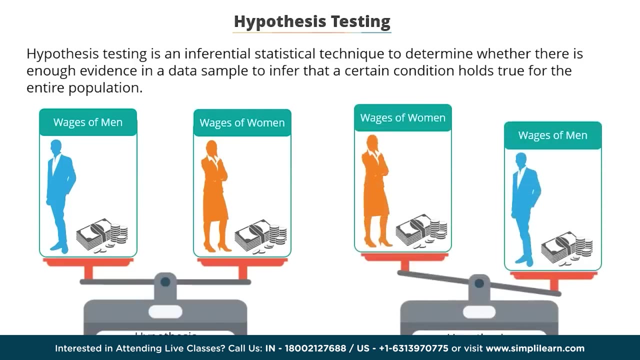 The population of hypothesis testing is to choose between two competing hypotheses about the value of a population parameter. For example, one hypothesis might claim that the wages of men and women are equal, while the other might claim that women make more than men. Hypothesis testing is formulated in terms of two hypotheses. 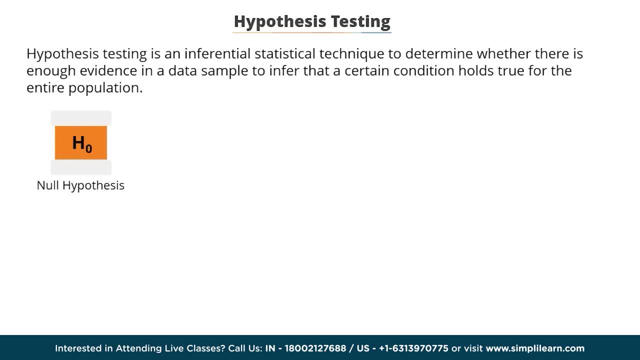 Null hypothesis, which is referred to as H. null Alternative hypothesis, which is referred to as H1.. The null hypothesis is assumed to be true unless there is strong evidence to the contrary. The alternative hypothesis is assumed to be true when the null hypothesis is proven false. 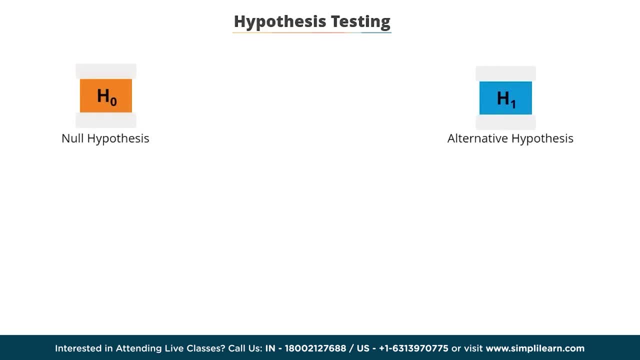 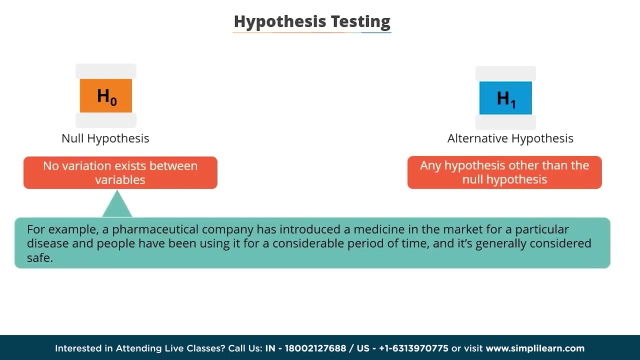 Let's understand the null hypothesis and alternative hypothesis using a general example. Null hypothesis attempts to show that no variation exists between variables, and alternative hypothesis is any hypothesis other than the null. For example, say, a pharmaceutical company has introduced a medicine in the market for a particular disease. 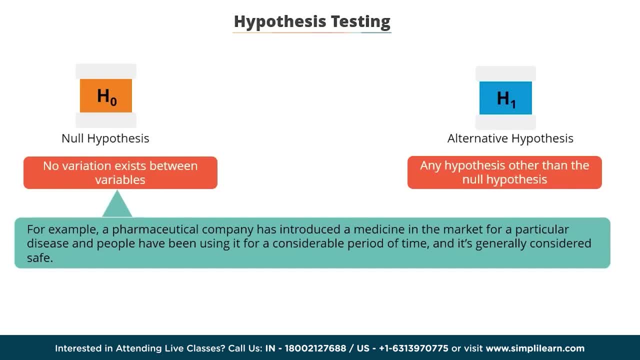 and people have been using it for a considerable period of time and it's generally considered safe. If the medicine is proved to be safe, then it is referred to as null hypothesis. To reject null hypothesis, we should prove that the medicine is unsafe. 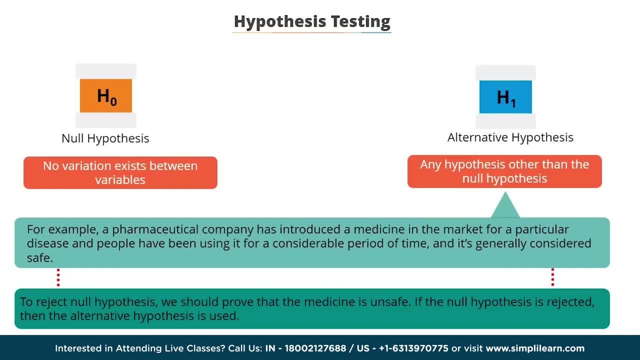 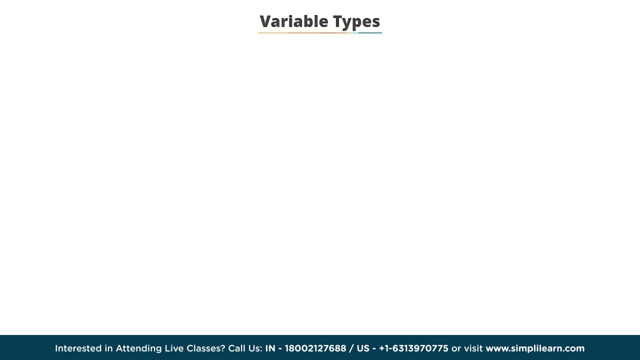 If the null hypothesis is rejected, then the alternative hypothesis is used. Before you perform any statistical tests with variables, it's significant to recognize the nature of the variables involved. Based on the nature of the variables, it's classified into four types. They are categorical or nominal variables. 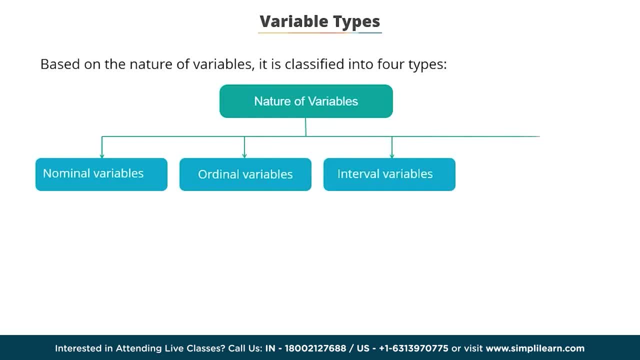 ordinal variables, interval variables and ratio variables. Nominal variables are ones which have two or more categories and it's impossible to order the values. Examples of nominal variables include gender and blood group. Ordinal variables have values ordered logically. However, the relative distance between two data values is not clear. 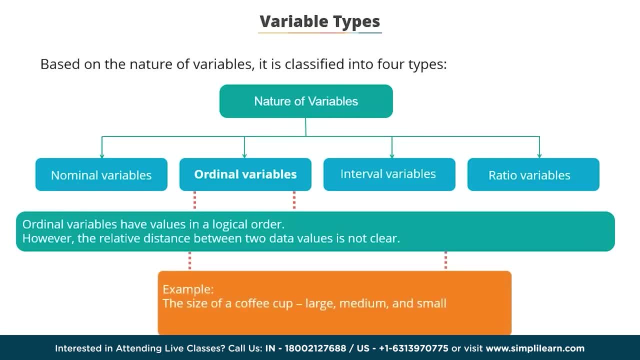 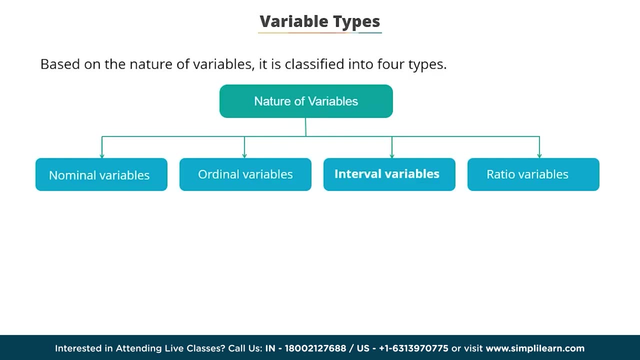 Examples of ordinal variables include considering the size of a coffee cup and considering the ratings of a product. Interval variables are similar to ordinal variables except that the values are measured in a way where their differences are meaningful, With an interval scale equal differences between scale values do have equal quantitative meaning. 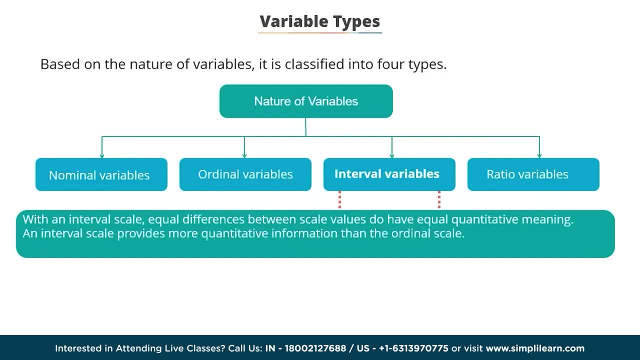 For this reason, an interval scale provides more quantitative information than the ordinal scale. The interval scale does not have a true zero point. A true zero point means that a value of zero on the scale represents zero quantity of the construct being assessed. Examples of interval variables include the Fahrenheit scale. 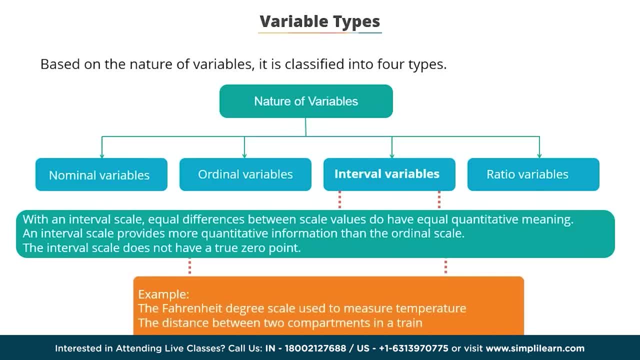 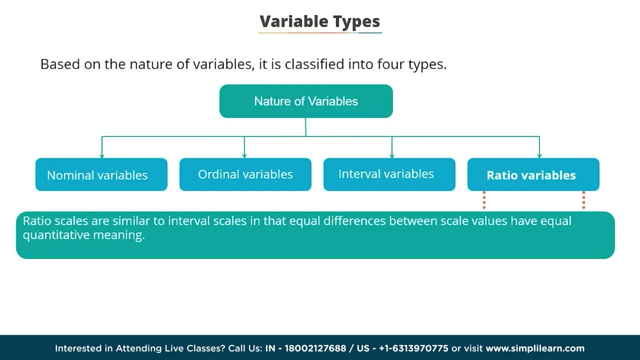 used to measure temperature and distance between two compartments in a train. Ratio scales are similar to interval scales in that equal differences between scale values have equal quantitative meaning. However, ratio scales also have a true zero point, which give them an additional property. For example, the system of inches used with a common ruler. 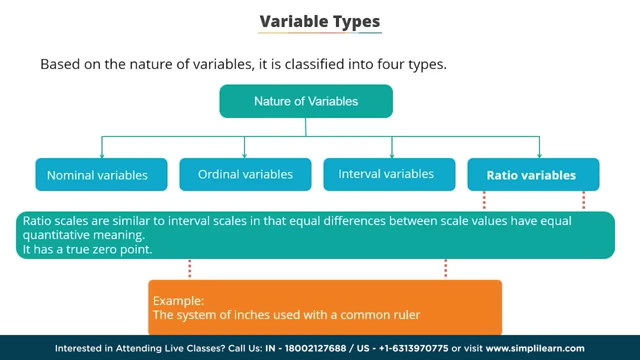 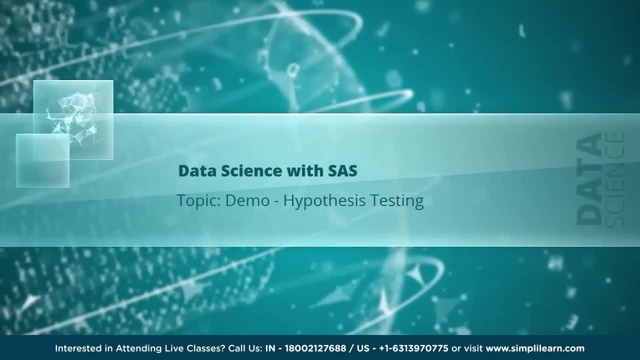 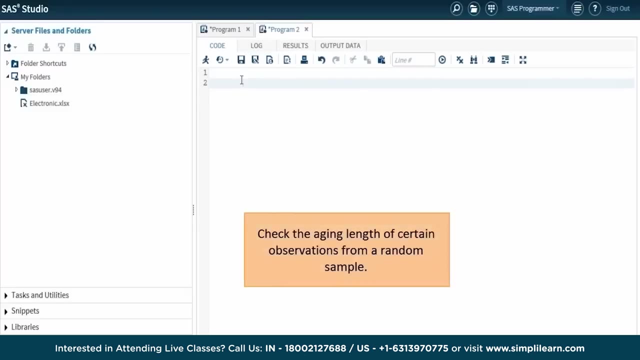 is an example of a ratio scale. There is a true zero point, because zero inches does in fact indicate a complete absence of length. In this demo, you'll learn how to perform the hypothesis testing using SAS. In this example, let's check against the length of certain observations. 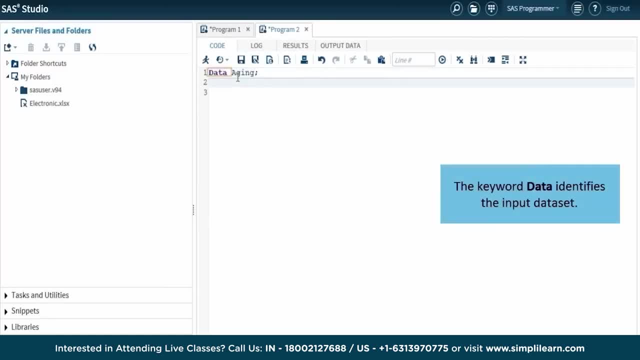 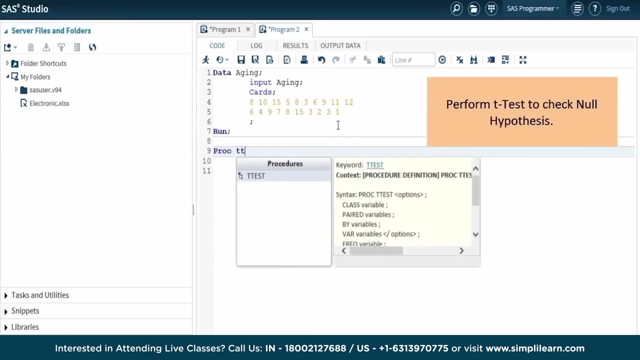 from a random sample. The keyword data identifies the input dataset. The input statement is used to declare the aging variable and cards to read data into SAS. Let's perform a t-test to check the null hypothesis. Let's assume that the null hypothesis to be that. 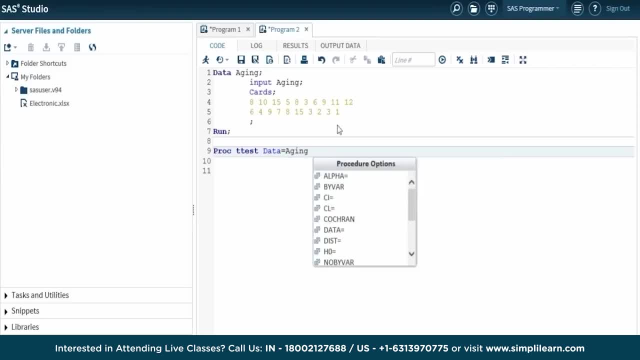 the mean days to deliver a product is 6 days, So null hypothesis equals 6.. Alpha value is the probability of making an error, which is 5% standard, and hence alpha equals 0.05.. The variable statement names the variable to be used in the analysis. 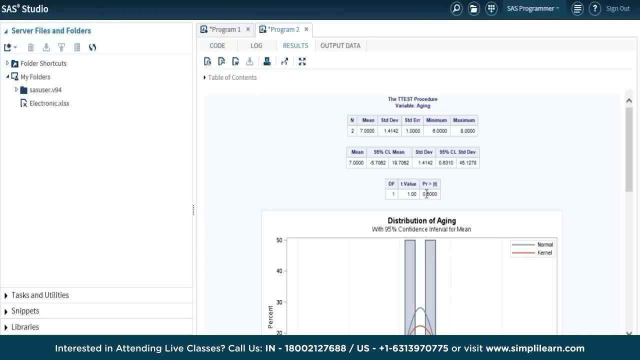 The output is shown on the screen. Note that the p-value is greater than the alpha value, which is 0.05.. Therefore, we fail to reject the null hypothesis. This concludes the demo on how to perform the hypothesis testing using SAS. 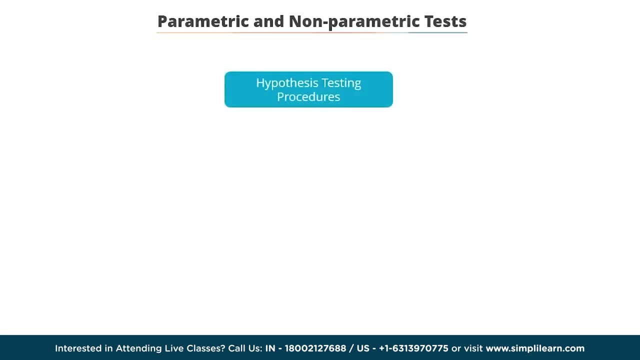 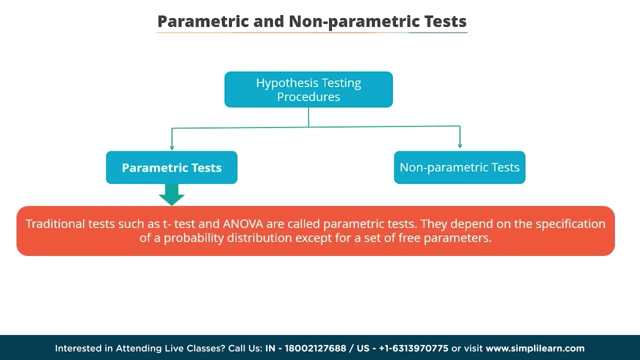 Let's now learn about hypothesis testing procedures. There are two types of hypothesis testing procedures. They are parametric tests and nonparametric tests. In statistical inference or hypothesis testing, the traditional tests, such as t-test and ANOVA, are called parametric tests. 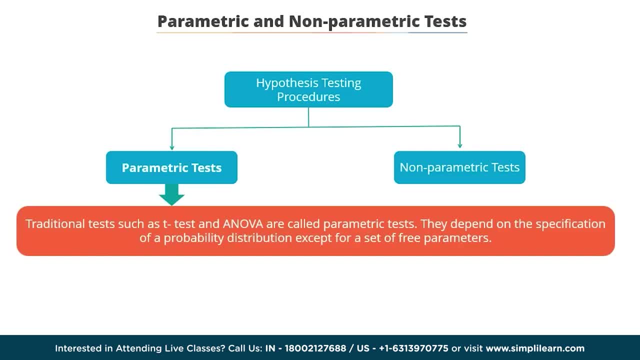 They depend on the specification of a probability distribution, except for a set of free parameters. In simple words, you can say that if the population information is known completely by its parameter, then it is called a parametric test. If the population or parameter information is not known, 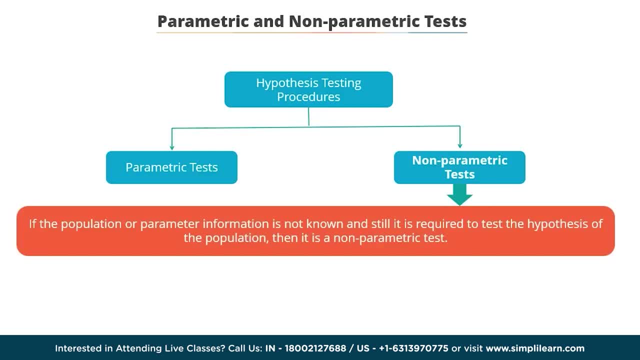 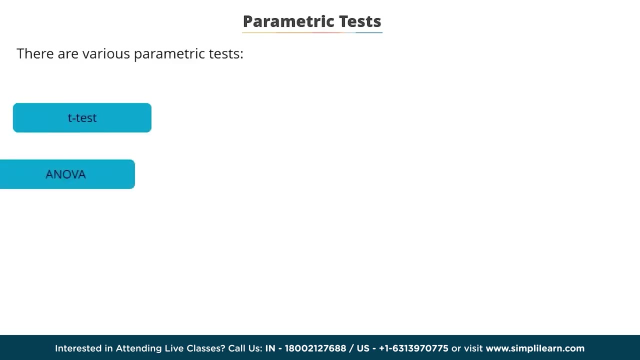 and you are still required to test the hypothesis of the population, then it's called a nonparametric test. Nonparametric tests do not require any strict distributional assumptions. There are various parametric tests. they are as follows: t-test, ANOVA, chi-squared linear regression. 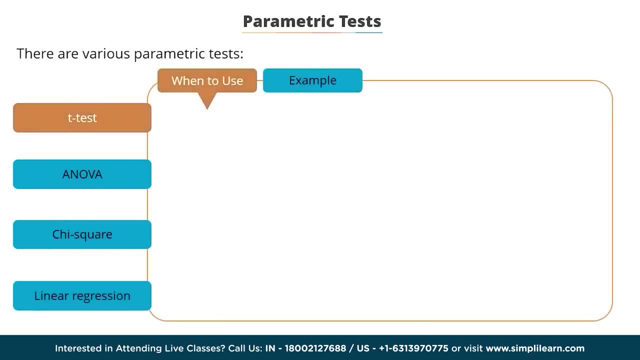 Let's understand them in detail. t-test: A t-test determines if two sets of data are significantly different from each other. The t-test is used in the following situations: To test if the mean is significantly different than a hypothesized value. To test if the mean for two independent groups is significantly different. 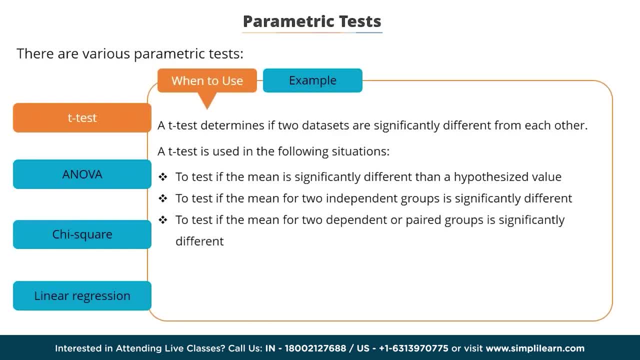 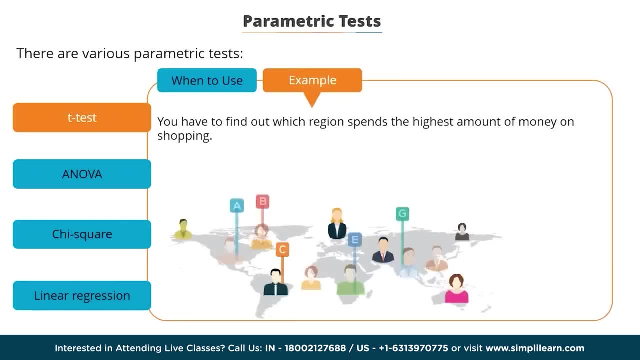 To test if the mean for two dependent or paired groups is significantly different. For example, let's say you have to find out which region spends the highest amount of money on shopping. It's impractical to ask everyone in the different regions about their shopping expenditure. 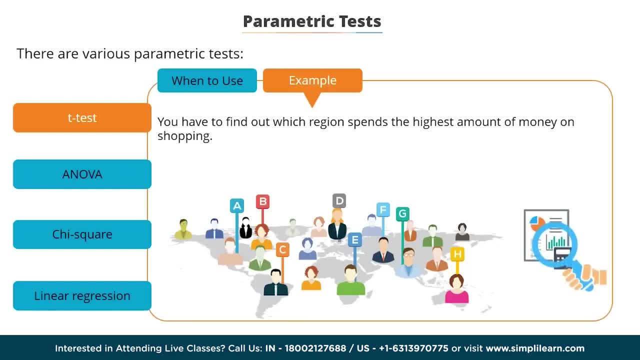 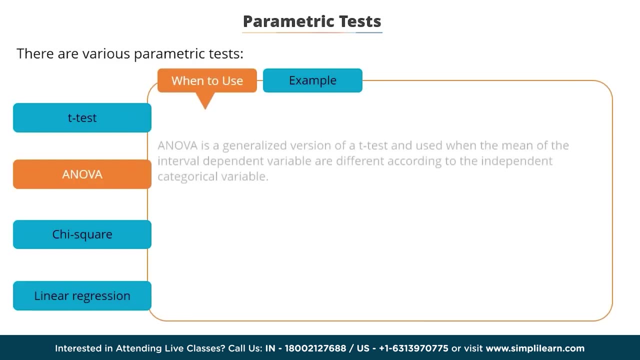 In this case, you can calculate the highest shopping expenditure by collecting sample observations from each region. With the help of the t-test, you can check if the difference between the regions are significant or a statistical fluke. ANOVA- ANOVA is a generalized version of the t-test. 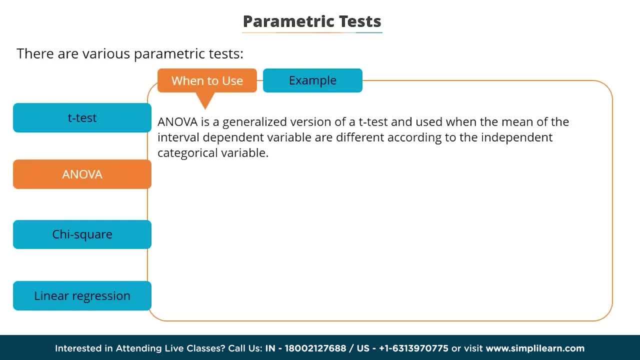 and used when the mean of the interval dependent variable is different to the categorical independent variable. When we want to check variance between two or more groups, we apply the ANOVA test, For example. let's look at the same example of the t-test example. 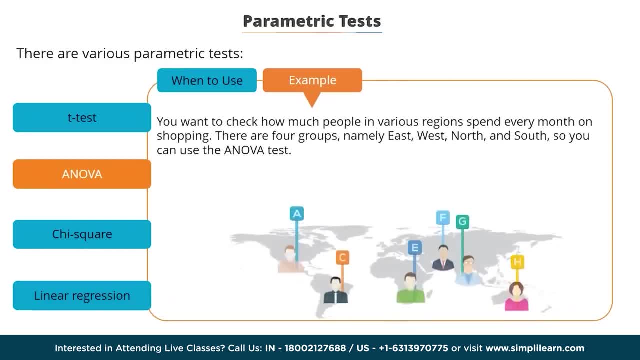 Now you want to check how much people in various regions spend every month on shopping. In this case, there are four groups, namely East, West, North and South. With the help of the ANOVA test, you can check if the difference between the regions is significant. 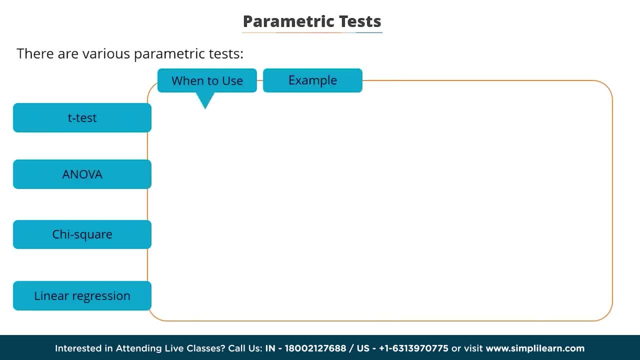 or a statistical fluke, CHI-SQUARE. CHI-SQUARE is a statistical test used to compare observed data with data you would expect to obtain according to a specific hypothesis. Let's understand the CHI-SQUARE test through an example. You have a data set of male shoppers and female shoppers. 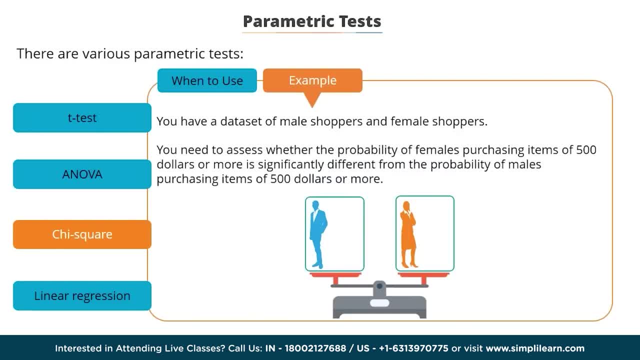 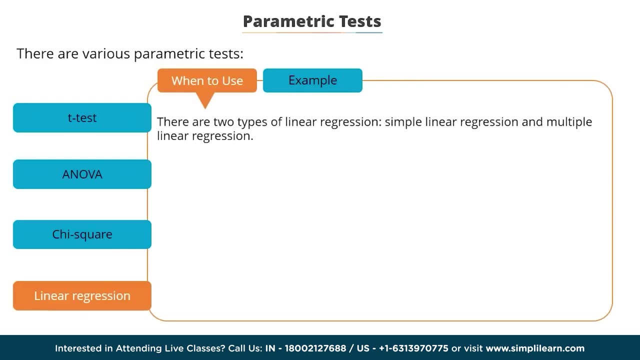 Let's say you need to assess whether the probability of females purchasing items of $500 or more is significantly different from the probability of males purchasing items of $500 or more. LINEAR REGRESSION: There are two types of linear regression: simple linear regression and multiple linear regression. 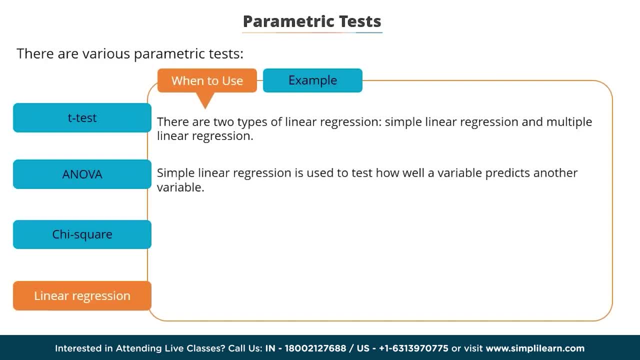 Simple linear regression is used when one wants to test how well a variable predicts another variable. Multiple linear regression allows one to test how well multiple variables or independent variables predict a variable of interest. When using multiple linear regression, we additionally assume the predictor variables are independent. 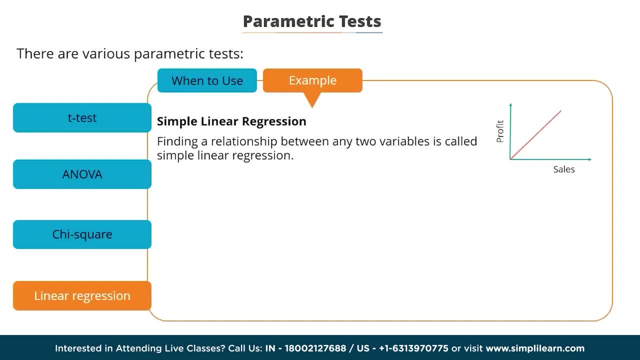 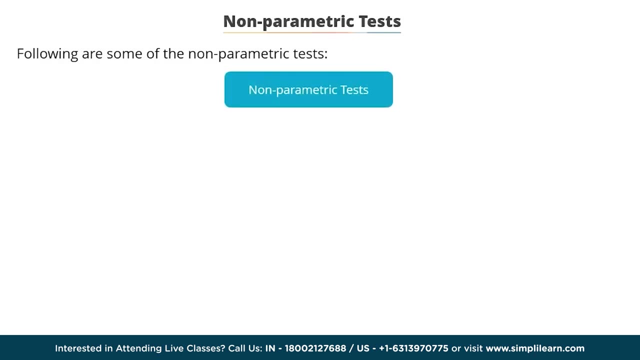 For example, finding a relationship between any two variables, say sales and profit, is called simple linear regression. Finding a relationship between any three variables, say sales, cost and telemarketing, is called multiple linear regression. Some of the nonparametric tests are: Wilcoxon rank sum test. 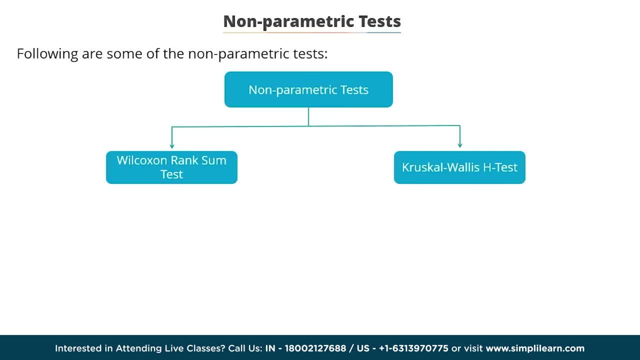 and Quesco-Wallis H test. Wilcoxon rank sum test. The Wilcoxon signed rank test is a nonparametric statistical hypothesis test used to compare two related samples or matched samples to assess whether or not their population mean ranks differ. 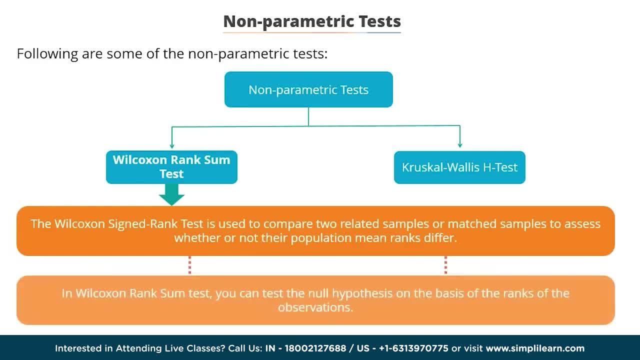 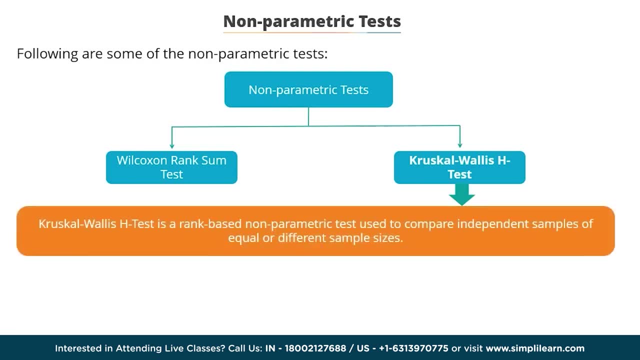 In Wilcoxon rank sum test, you can test the null hypothesis on the basis of the ranks of the observations. Quesco-Wallis H test. Quesco-Wallis H test is a rank-based nonparametric test used to compare independent samples of equal or different sample sizes. 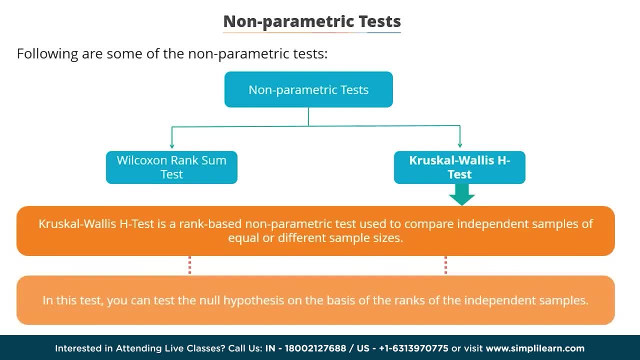 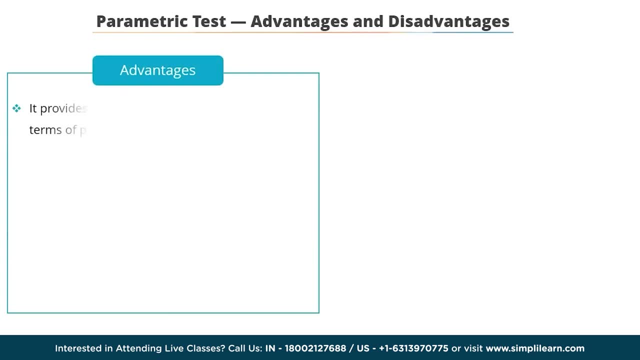 In this test, you can test the null hypothesis on the basis of the ranks of the independent samples. The advantages of parametric tests are as follows: Provide information about the population in terms of parameters and confidence intervals, Easier to use in modeling analyzing. 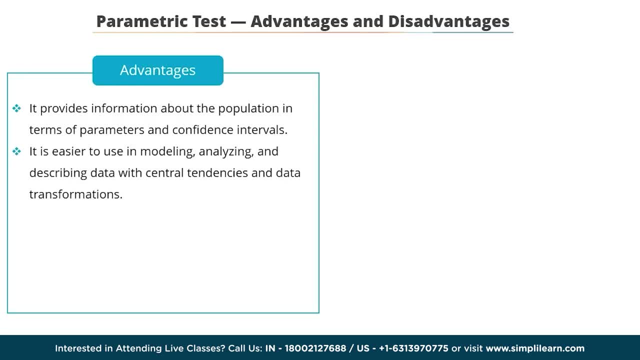 and for describing data with central tendencies and data transformations. Express the relationship between two or more variables. Don't need to convert data into rank order to test. The disadvantages of parametric tests are as follows: Only support normally distributed data. only applicable on variables, not attributes. 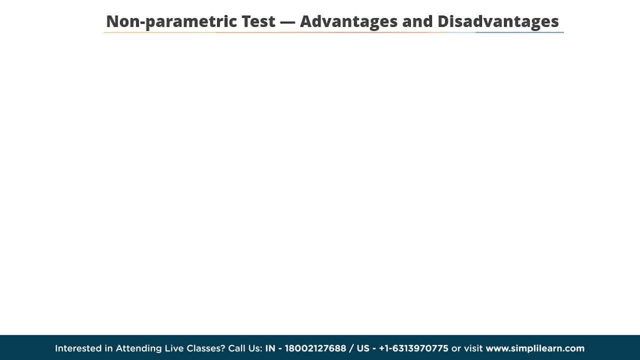 Let's now list the advantages and disadvantages of nonparametric tests. The advantages of nonparametric tests are as follows: Simple and easy to understand. Do not involve population parameters and sampling theory. Make fewer assumptions. Provide results similar to parametric procedures. 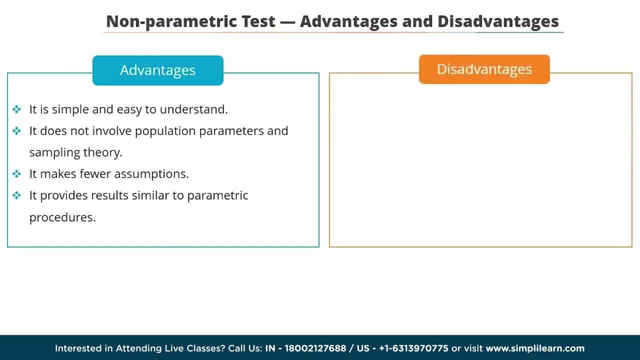 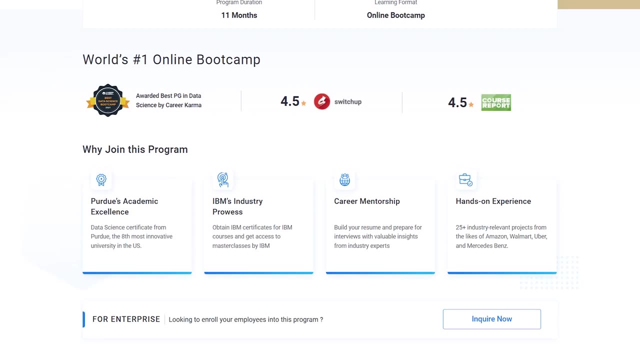 The disadvantages of nonparametric tests are as follows: Not as efficient as parametric tests. Difficult to perform operations on large samples manually. Also, data scientists looking for online training and certification programs from the best universities. or a professional who elicits to switch careers with data science. 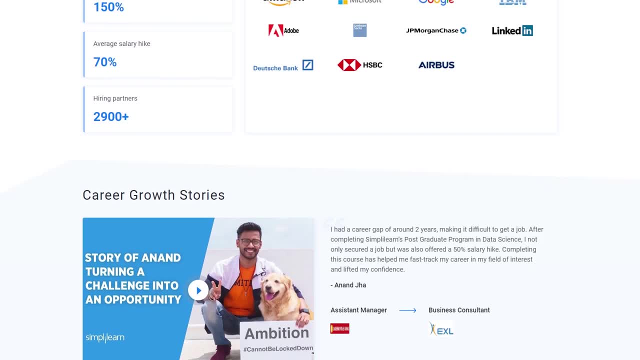 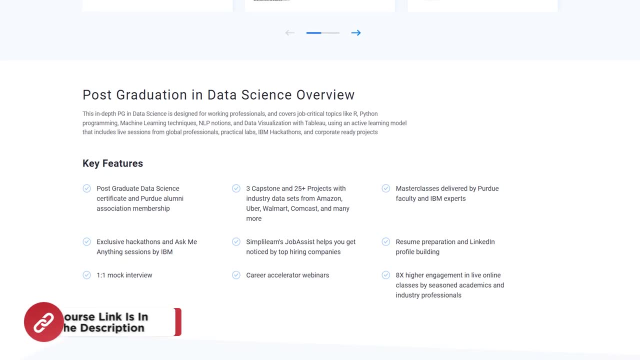 then try giving Simply Learn's postgraduate program in data science a shot. The link in the description box below should navigate to the homepage where you can find the complete overview of the program being offered. Now over to our training experts. So now let's dive into the definition. 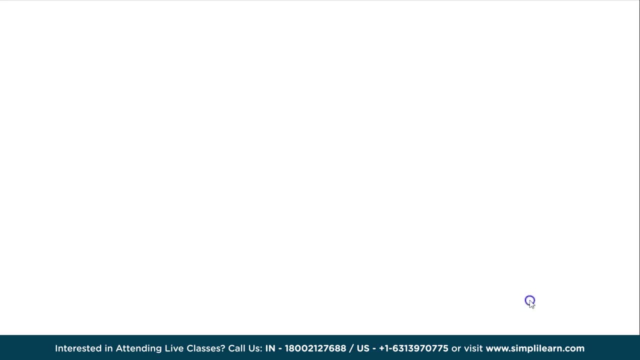 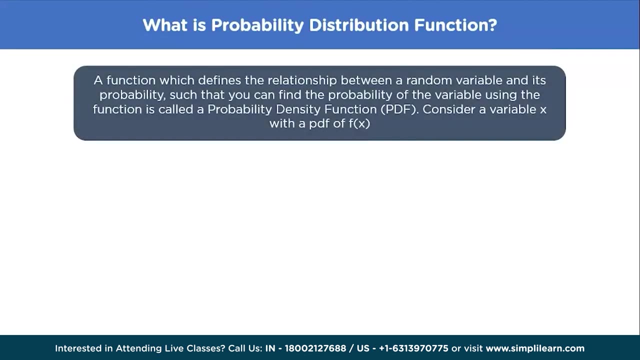 of the probability distribution function. What is probability distribution function? A function which defines the relationship between a random variable and its probability, such that you can find the probability of the variable using the function is called a probability density function. In simple words, probability density is the relationship 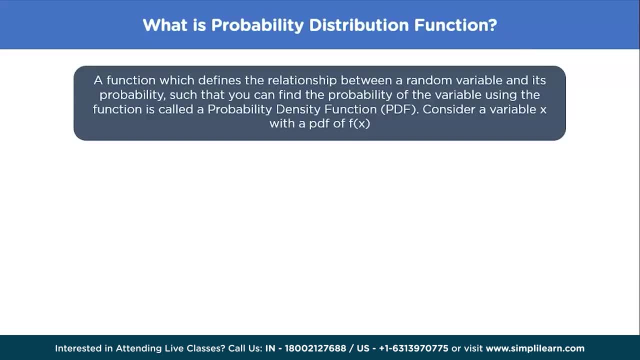 between an observation and the probability. Some outcomes of a random variable will have low probability density and other outcomes will have a very high probability density. Basically, the probability of a variable x happening or occurring will vary and it can sometimes take on a lower value. 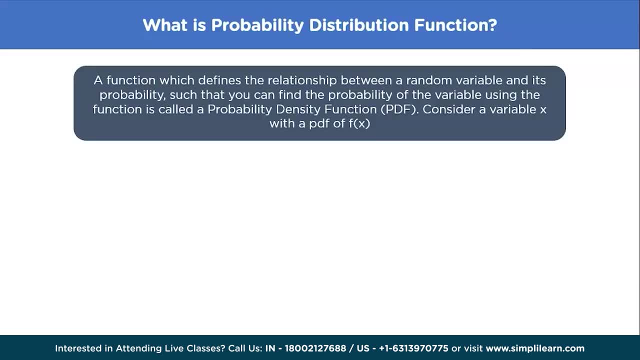 or it can take on a way higher value. The overall shape of the probability density is referred to as probability distribution, and the calculation of probabilities for specific outcomes of a random variable is performed by a probability density function, or PDF for short. Now consider a variable x with a PDF of f of x. 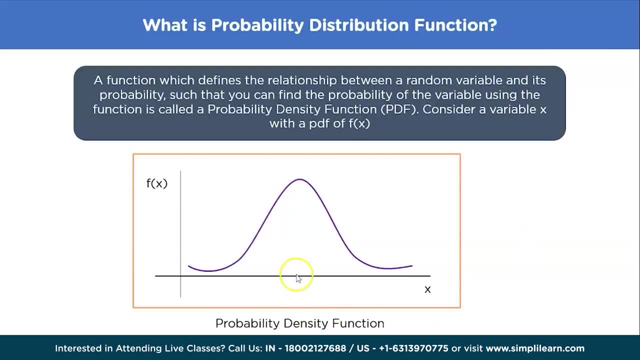 This is what your probability density function will look like. There might be a point where the probability of x occurring is very high. Hence your probability distribution function, or f of x will also be very high. At other points, the distribution or the probability of x 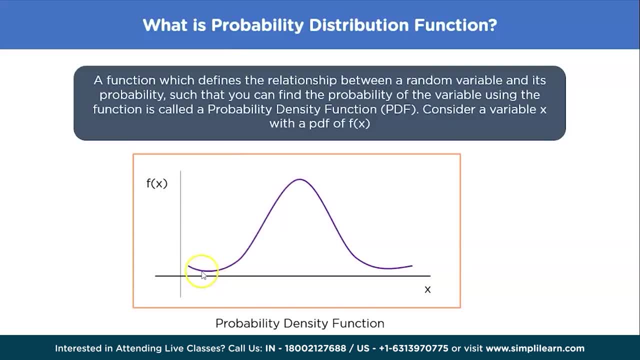 happening or occurring is going to be very low. Hence your f of x is also going to have a very small value. Basically, given the random sample of a variable, we might want to know things like the shape of the probability distribution. This here is something called a normal distribution. 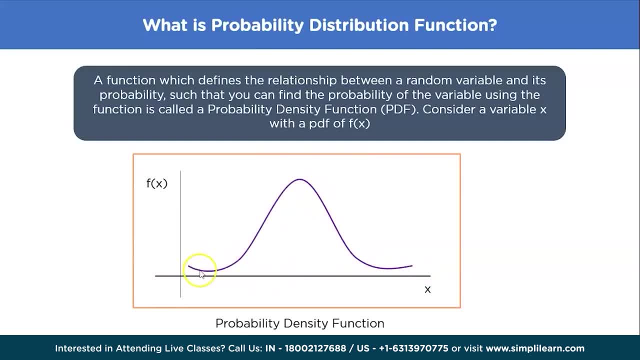 where your probability distribution function takes on a bell shape. However, this is not the probability density function. that might always occur. There are different probability distribution functions and all of their graphs look very different from each other. Knowing the probability distribution for a random variable can help you calculate. 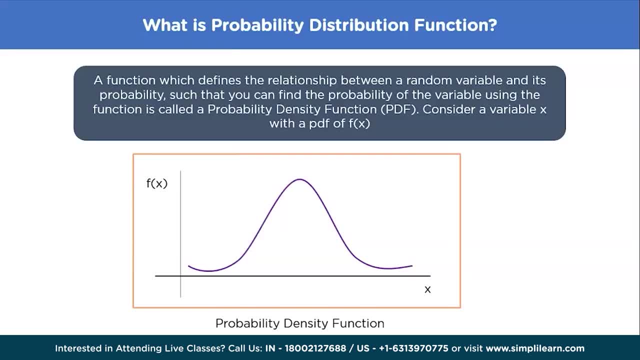 movements of the distribution, like the mean and variance. But it can also be useful for other more general considerations, like determining whether an observation is unlikely or very unlikely and might be an outlier or an anomaly Like. consider this graph itself In this graph: 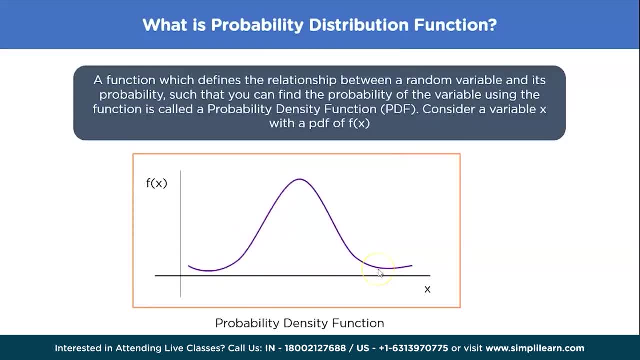 these points over here, which have very less probability distribution, are outliers, which means that the chance of them occurring is very low, And basically this is not something that you are going to see in your regular scenario for your variable x. Now let's consider two points, a and b. 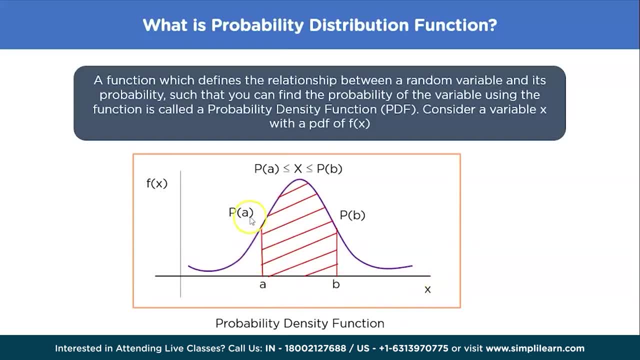 which are values that our variable x can take. p of a and p of p just represent the probability of a and the probability of b, Which can be found out by drawing a straight line and coinciding it with our graphs. The area under the graph: 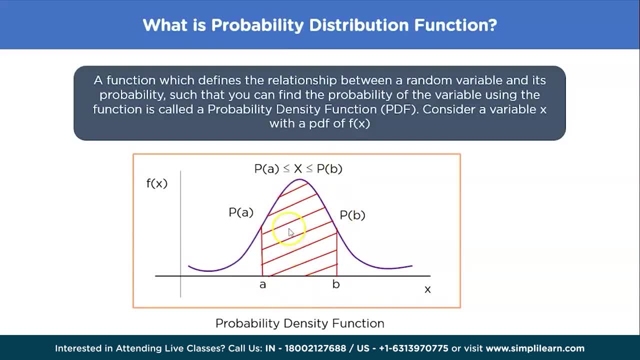 over here, which is going to give you your probability of this region occurring, can be written as probability of a less than equal to x- which is the probability that we are searching for here- less than equal to probability of b. What does this mean exactly? This means that this area. 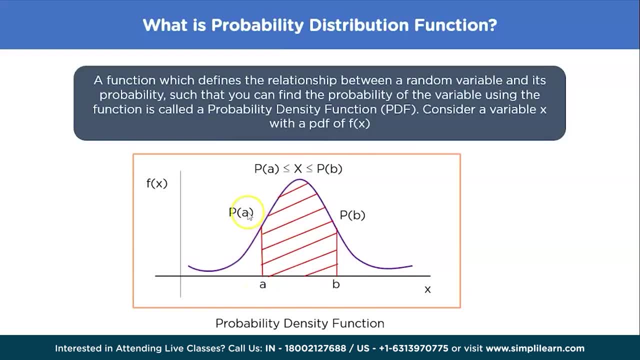 is always going to be greater than or equal to the probability of a, but less than or equal to the probability of b. This gives us the narrow region of the probability which is present over here, And doing this we can find the probability of occurrence. 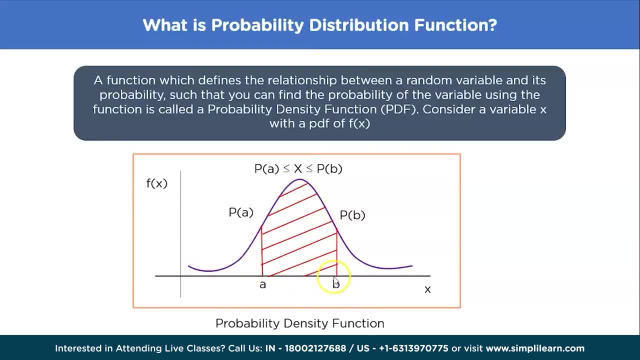 for any value of x. Suppose you want to find the probability of b happening For a probability distribution function. the probability of b happening is not simply this point here, But the entire area of the graph which is taking place before this point itself. 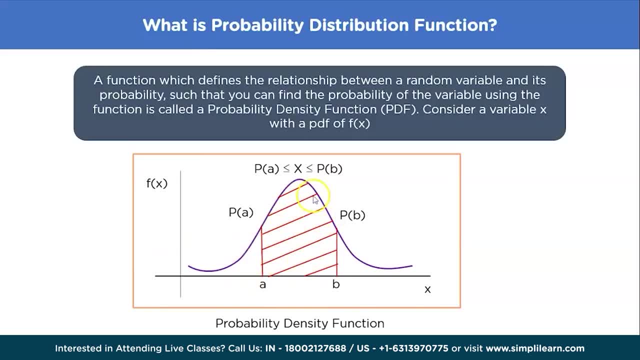 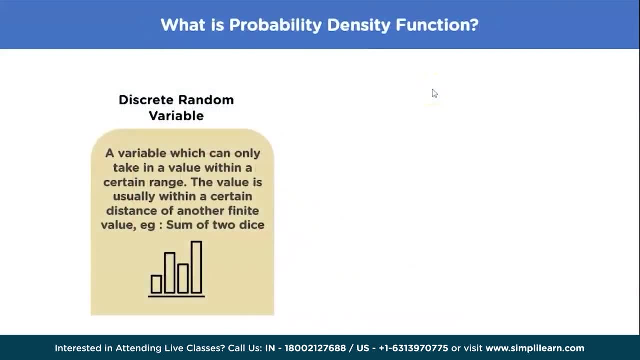 So if you want to find the probability between these regions, you are going to have to find the entire area and not simply the probability at one point. Now, so far, we have been talking about different types of variables, which is discrete, random variables and continuous variables. 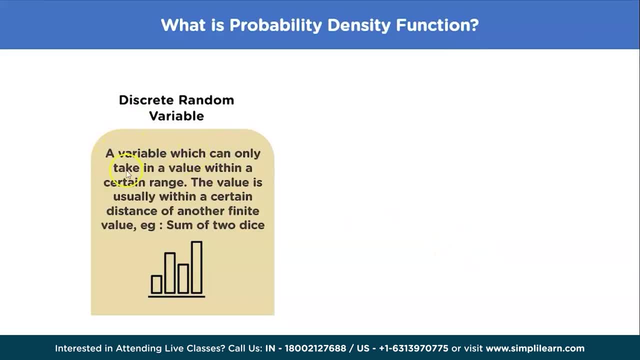 What exactly do these mean? A variable which can only take a value within a certain range is called a discrete, random variable. The value is usually within a certain distance of another finite value. An example of this would be the sum of two dices. 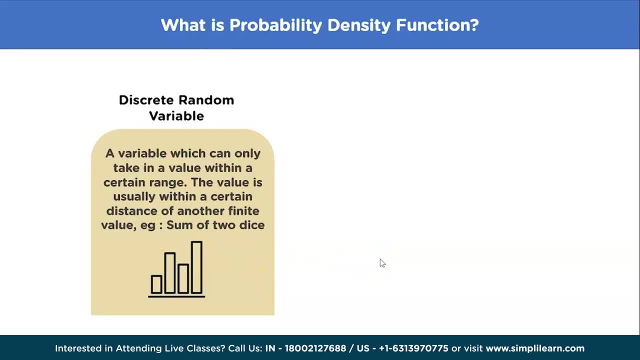 Basically, values which are well defined are called discrete values, And a variable which has well defined values will be called a discrete random variable. This variable can only take values which fall within a certain set of values. Let's say, you roll a dice. 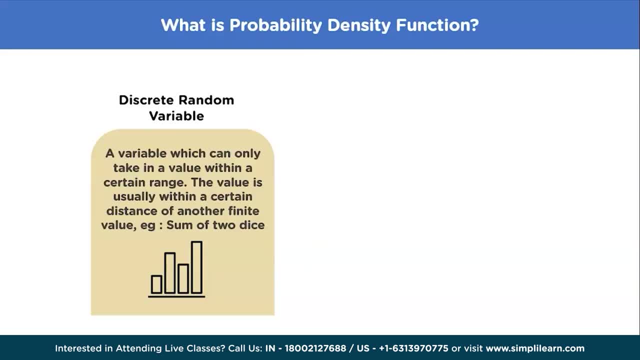 The dice can only give you specific outcomes, which range from 1 to 6.. This is what you would call a discrete output. On the other hand, a continuous random variable can take on infinite different values within a range of values, For example, the height of a student. 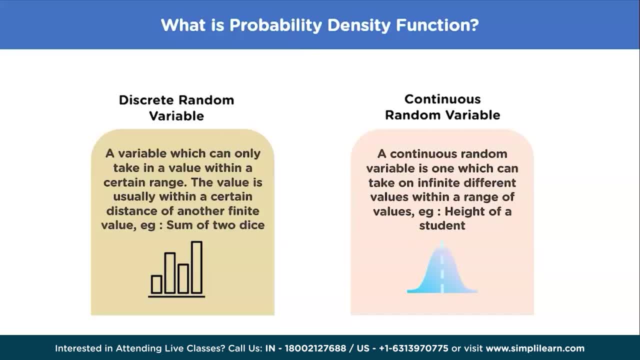 The height of a student is not fixed. Even if the height is 1.7 meters, in reality the height can be 1.77 or 1.765 or 1.789.. The exact height is very hard to determine because it's not easy for us to find the precise. 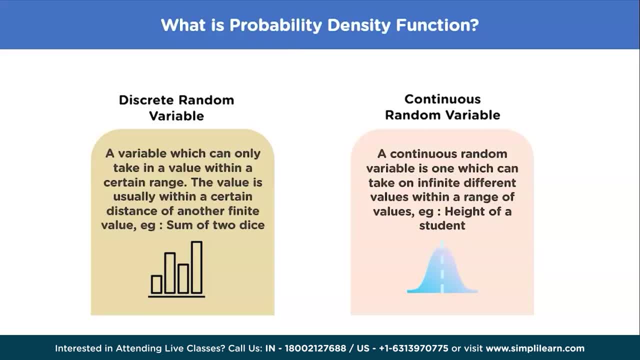 value of the height of a student. So basically, the height can take on an infinite different range of values. When we're trying to define the values that a continuous random variable can take, we usually say it in the form of a range of values. 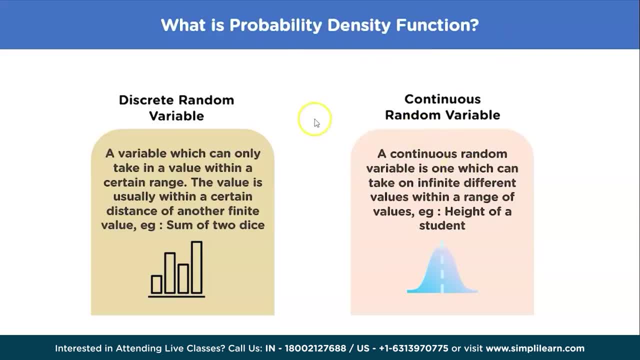 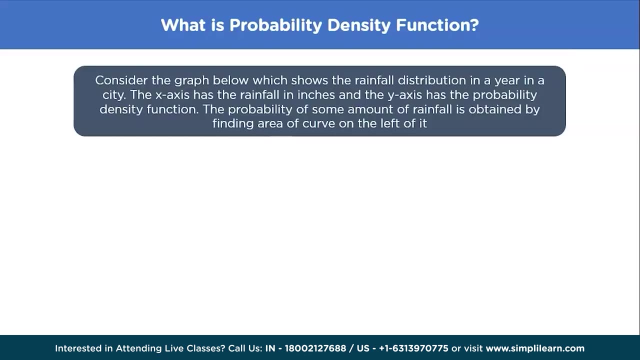 which means that the value can fall in that range and can take on any value in that range. It's not like a discrete, random variable where you can define definitive values. Now let's understand a probability density function with the help of a graph. Consider the graph below. 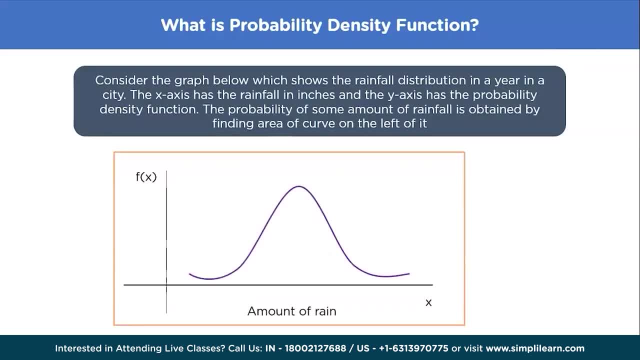 which shows the rainfall distribution in an year in a city. The x-axis has the rainfall in inches, or the amount of rain that we're getting, and the y-axis has the probability density function of getting that amount of rain, The probability of some amount of rainfall. 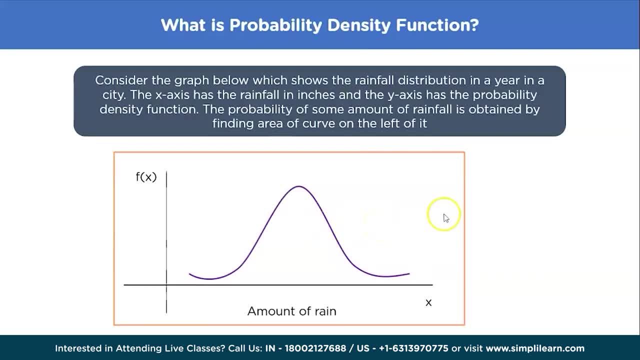 is obtained by finding the area of the curve to the left of it. So let's say we have a point 3.. If we want to find the probability of 3 inches of rainfall occurring, we would have to find the area of the curve. 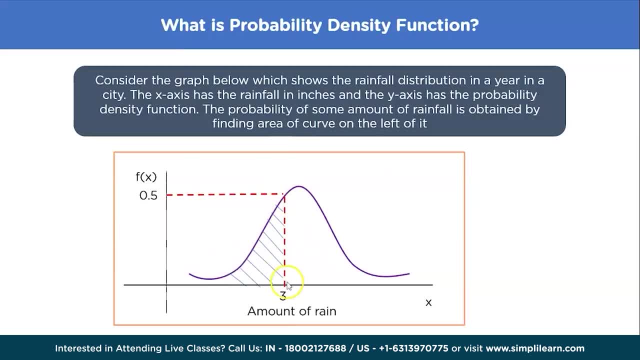 which falls to the left of 3.. When we draw a line from 3 which intercepts the graph, and further extend it onto the y-axis, we get a value of 0.5.. Simply put, this means that the probability of 3 inches of rainfall occurring 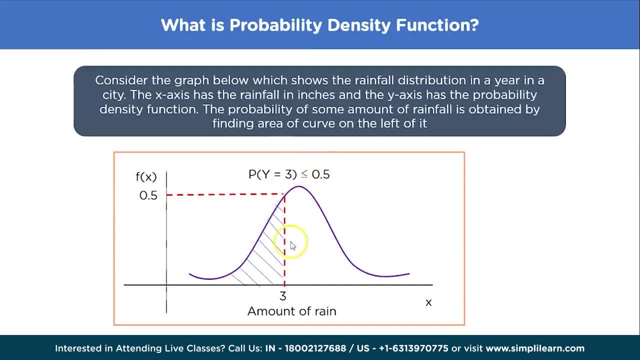 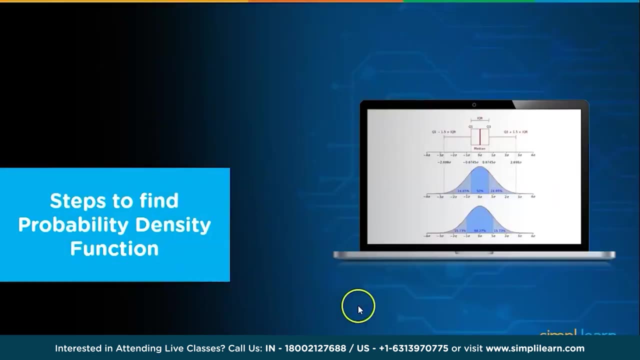 is going to be lesser than or equal to 0.5.. The exact probability can be found out by finding the area of the curve which falls to the left of 3.. How do we find the probability distribution function? The first step is to summarize your density. 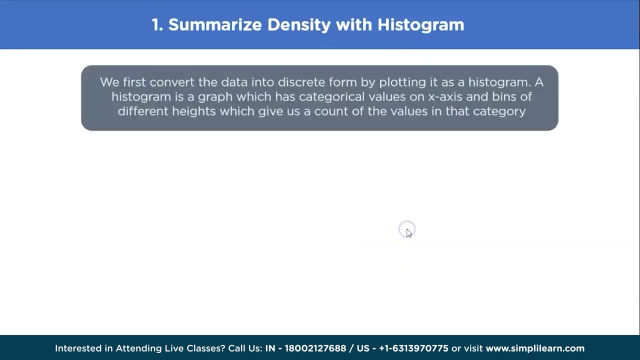 with the help of a histogram. The first step in a density estimation is to create a histogram of the observations in the random sample. Now, what is a histogram? A histogram is a plot which involves first grouping the observation into bins and counting the number of events. 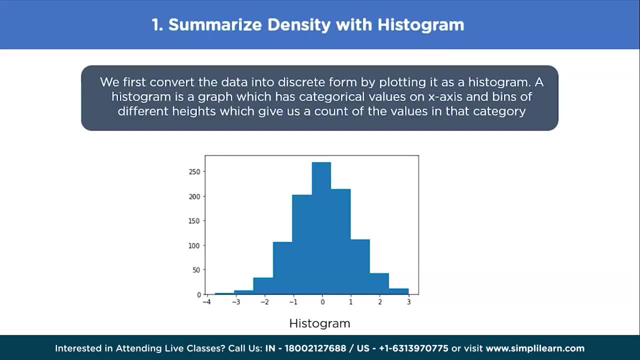 that fall in each bin. The counts of frequency of observation in each bins are then plotted as a bar graph, with the bins on the x-axis and the frequency on the y-axis. The choice of the number of bins is important as it controls the coarseness of the distribution. 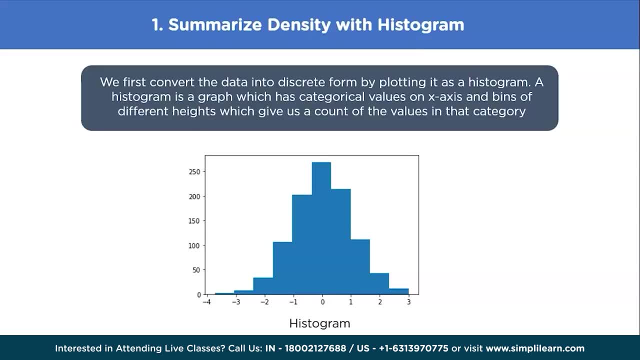 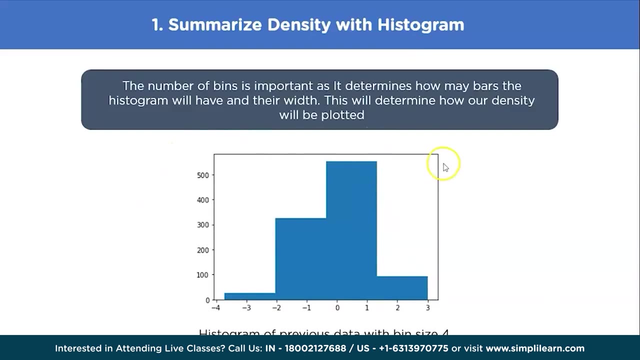 and, in turn, how well the density of the observation is plotted. It is a good idea to experiment with different bin sizes for a given data sample to get multiple perspectives or views on the same data. At the same time, the number of bins is important. 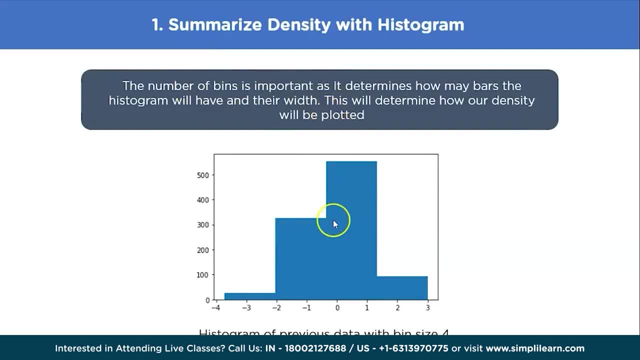 as it determines how many bars the histogram will have and their widths. This will change not only the shape of the graph, but also how the graph is read. This will also determine how our density is plotted. Now let's see how we can summarize our density with histograms using Python. 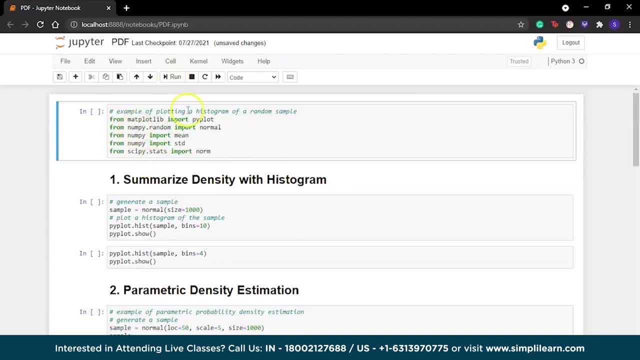 First, let's import all of our necessary modules which we are going to require. We are going to require matplotlib to plot graphs. We are going to need the normal random function so that we can get a normal distribution. We are going to import mean and standard deviation from numpy. 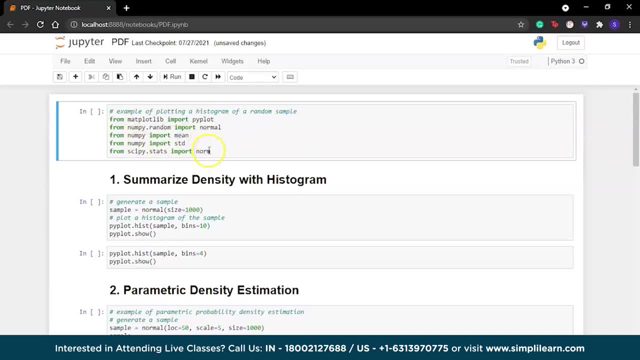 to use on our graphs. We are also going to normalize our data, so we are going to import the norm function from scipy. We finished importing all of our necessary modules. Now let's generate a sample which has a size of 1000, and it is going to be a normal distribution. 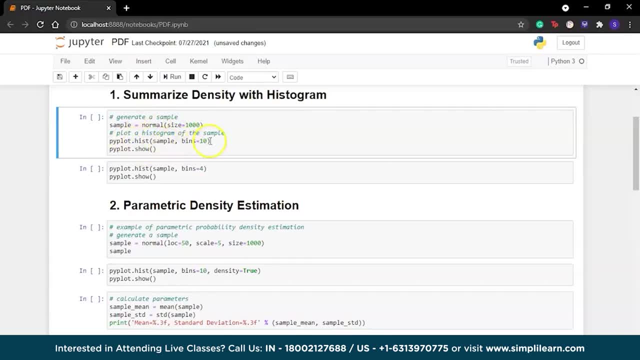 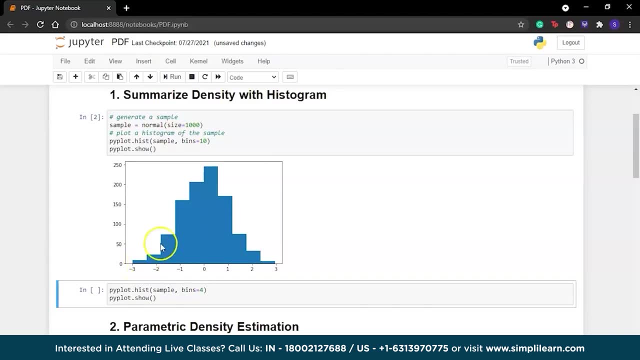 We are going to also plot this with the help of a histogram in bins of 10.. As you can see here, you get a normal distribution which is nothing but a almost bell shaped curve, and we have 10 bins here which are centered at 0. 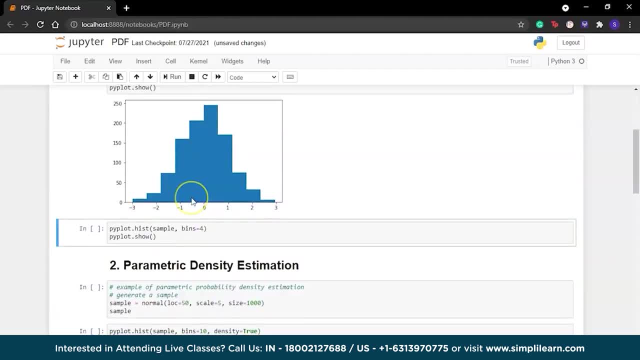 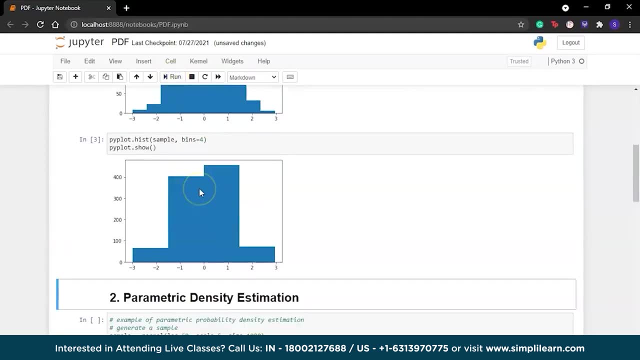 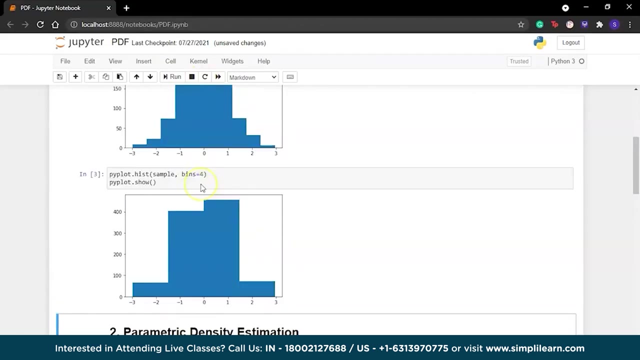 and which extend from minus 3 to 3.. How will our graph look if we change the number of bins, though? Let's run it and see. So you still have a normal distribution, but it is not as well defined Because of how less the number of bins are. 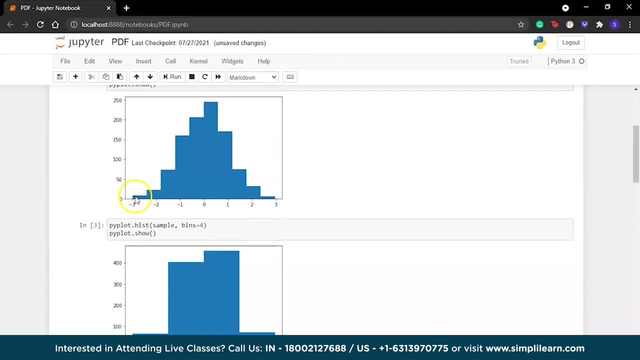 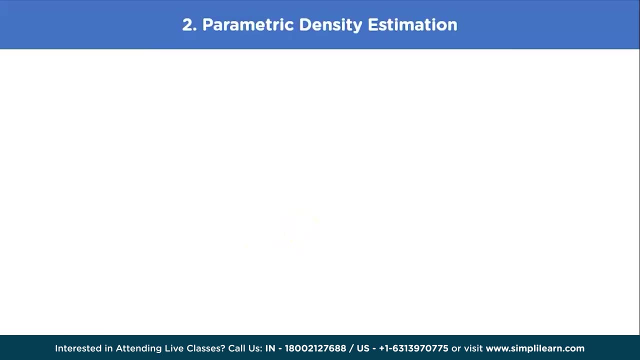 you lose a majority of the data which will contribute to your normal distribution. It doesn't look like a proper normal distribution, but looks more like discrete data at this point. Now let's take a look at the next step of finding our probability distribution function. 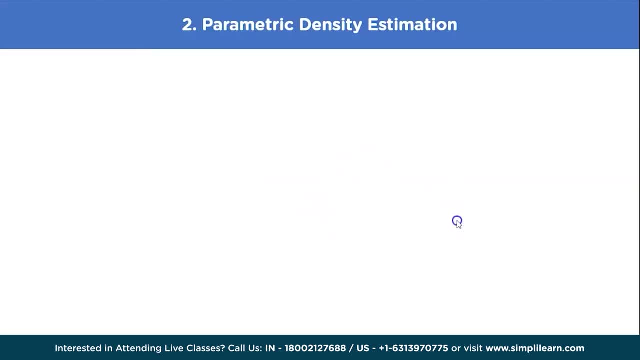 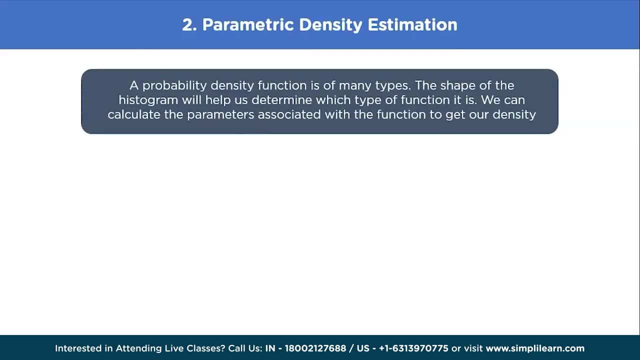 The next step is called parametric density estimation. What exactly is parametric density estimation? The probability density function is of many types. The shape of your histogram will help you determine what type of a function it is. We can also calculate the parameters associated with the function. 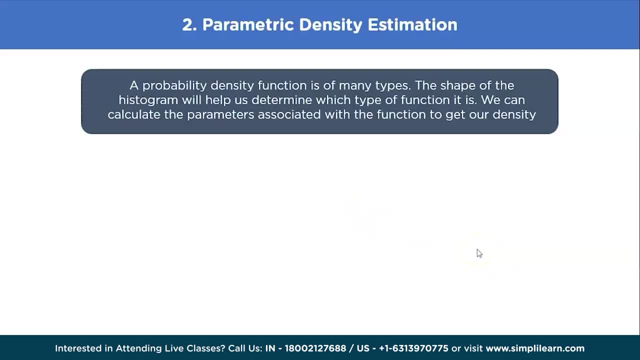 to get our density. Now, different probability distribution functions will have different graphs, which will have different shapes and which will also have different parameters, like mean, standard deviation, etc. associated with them. Using these parameters, we can find important points of our data. Hence it is very important for us. 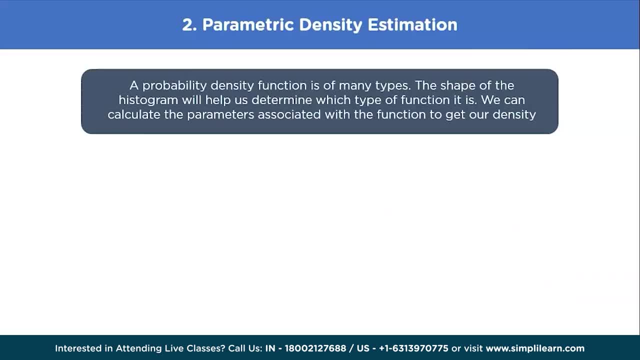 to recognize what type of a distribution it is. Common distributions will occur again and again in different and sometimes unexpected domains. Getting familiar with common probability distributions will help you identify a distribution from a histogram and, once identified, you can attempt to estimate the density of the random. 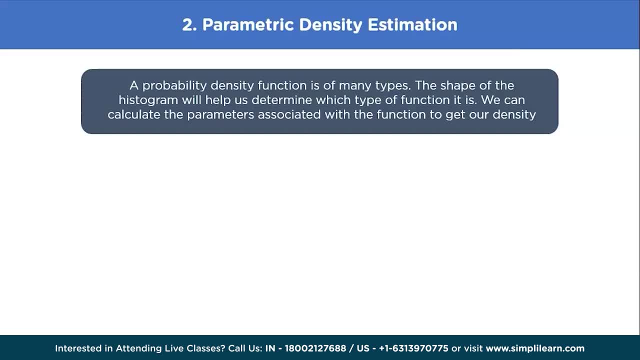 variable with the chosen probability distribution. This can be achieved by estimating the parameters of the distribution from a random sample of data. Now, an example of this would be a normal distribution which has two main parameters: the mean and standard deviation. Given these two parameters, we will now 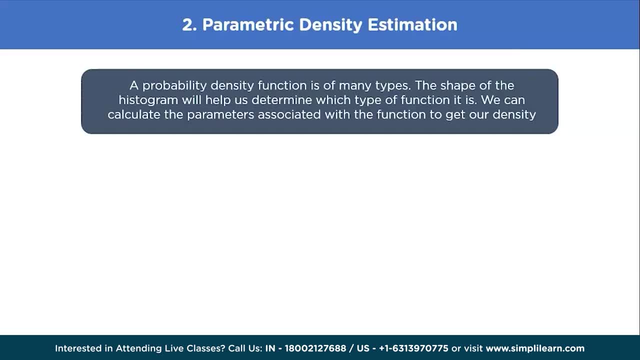 know the probability distribution function. These parameters can be estimated from data by calculating the sample mean and sample standard deviation. This entire process is known as parametric density estimation and it includes identifying your probability distribution function and getting the parameters which are associated with it. 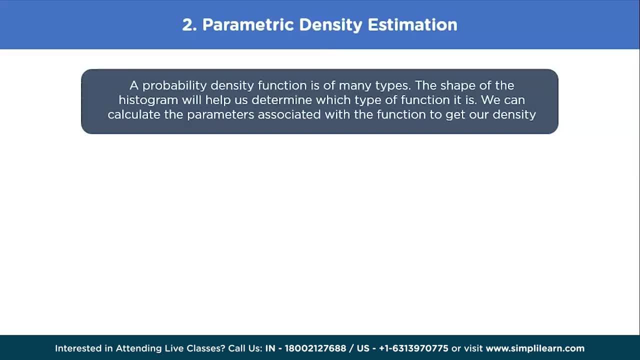 Now, once we have estimated the density, we can check if it's a good fit. This can be done in three different ways. One is plotting the density of the function and comparing the shape to the histogram. The next is sampling the density function and comparing 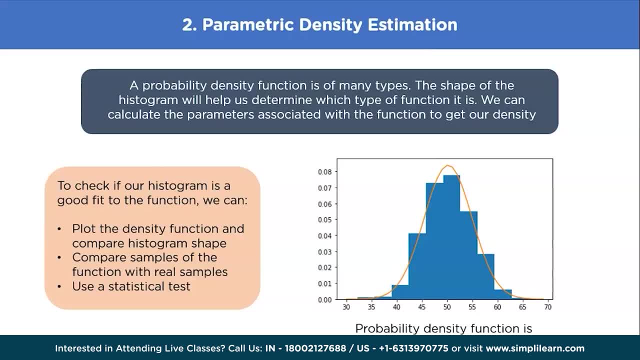 the generated sample to the real sample, and the last one is using a statistical test to confirm if the data fits the distribution Now over here, as you can see, all we've done is taken our data and plotted the density function on top of our histogram, and we've 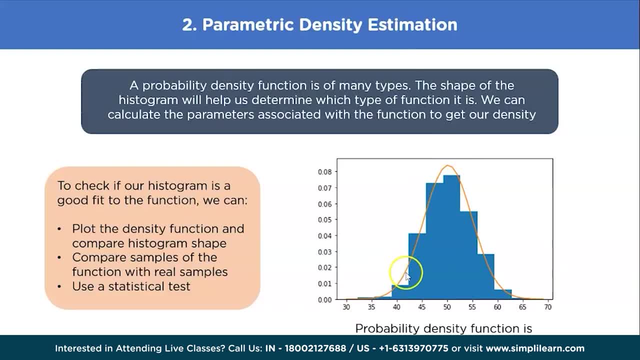 compared the shape, So the distribution, so the density function that we're actually considering here is a normal distribution, and from this graph we can see that it's almost an exact fit to our histogram. Now let's see how we can perform parametric density estimation. 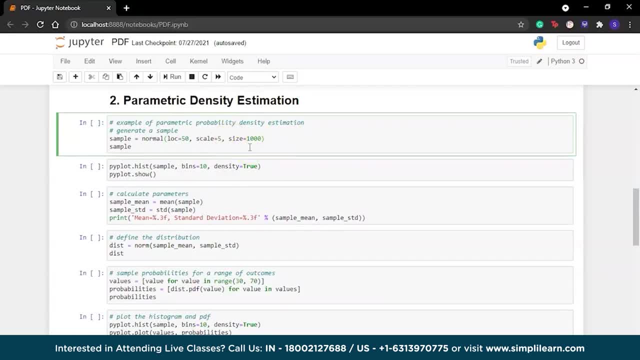 using Python. To begin with, let's generate a random sample of using observations from a normal distribution with a mean of 50, which is determined by the LOC parameter, and a standard deviation of 5, which is determined by the scale parameter. Now just to show you what. 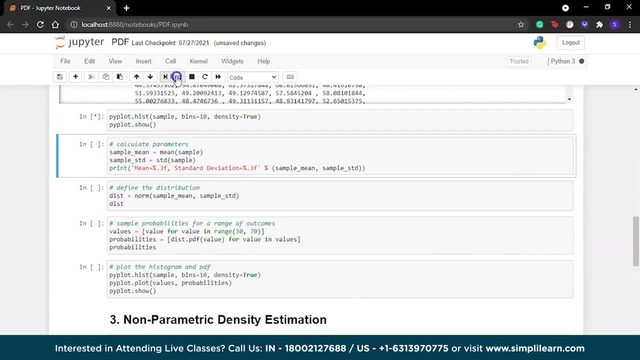 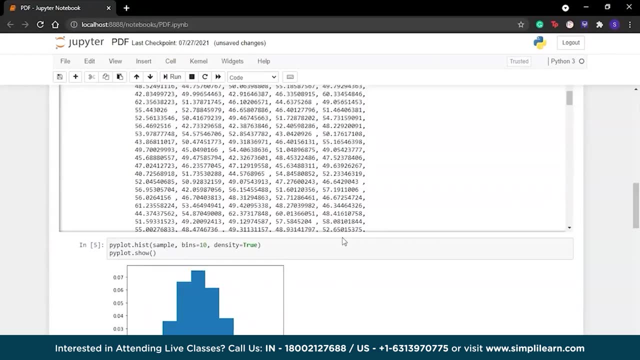 the distribution looks like. we're gonna plot it in the form of a histogram. So this is what the histogram looks like, But this is just to give you a basic idea of our data and what it looks like once plotted. But let's assume that we don't know. 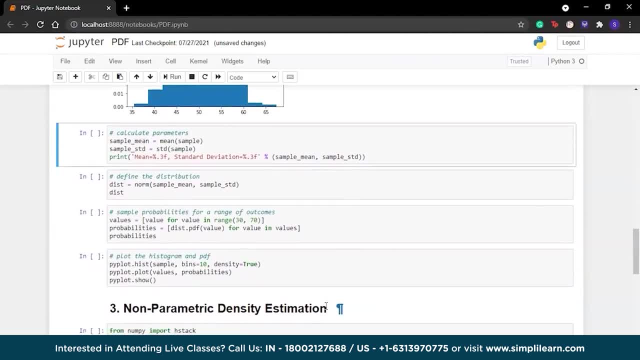 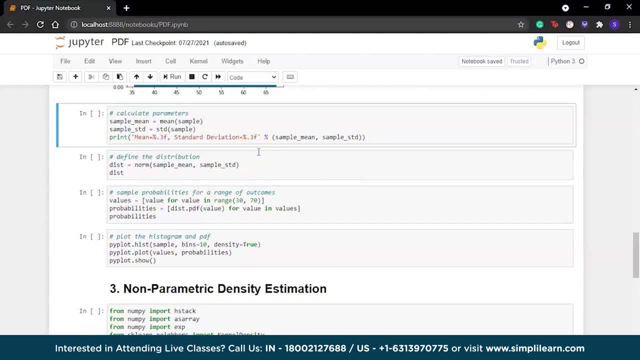 the probability distribution and we don't know what it looks like as a histogram, and we don't know that it's normal. So now, if we just assume that it's normal, we can calculate the parameters of the distribution, specifically the mean and the standard deviation. 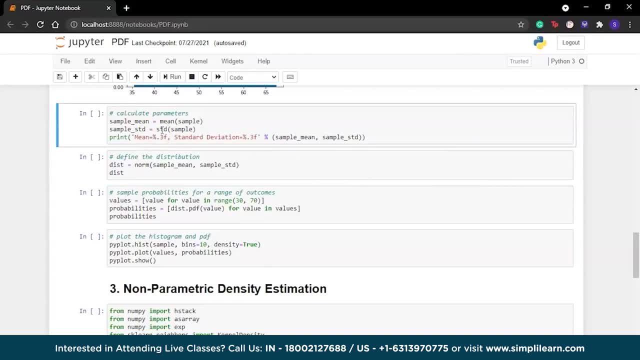 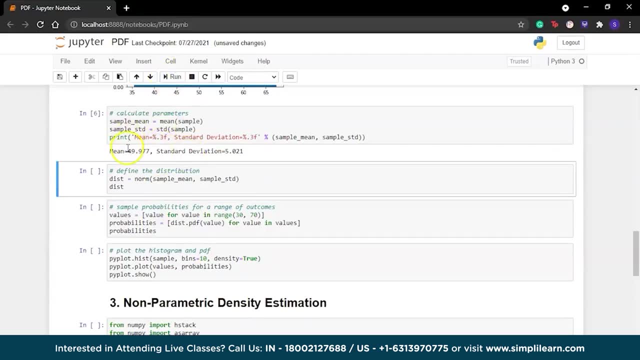 We would not expect the mean and standard deviation to be 50 and 5 exactly, given the small sample size and the noise in the sampling data. So because of this noise and the small sample size, we have a mean of almost 50 and a standard deviation. 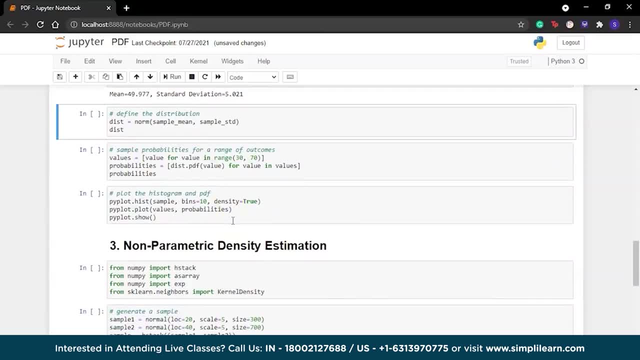 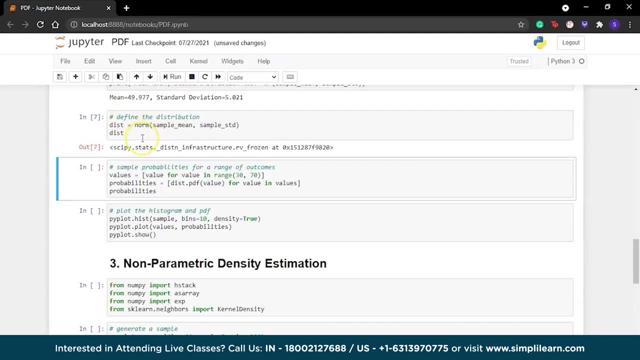 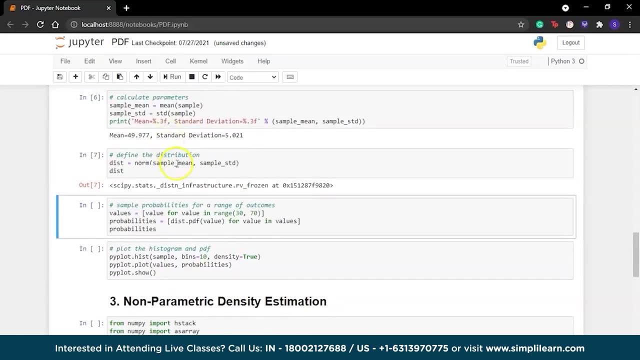 of a little more than 5.. Now let's define the distribution as normal. So now, using this, we've defined a normal distribution, We've used the norm method of the sci-fi library and we're doing this with the mean and the standard deviation that. 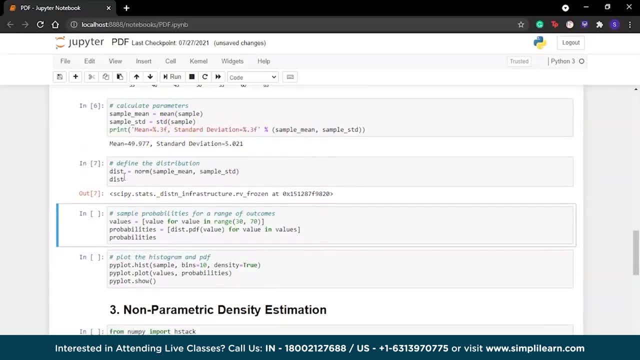 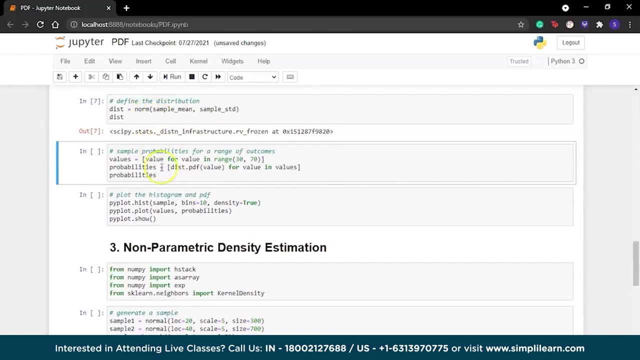 we've obtained from our samples. So up until now we're just assuming that it's a normal distribution and because of that, the parameters that we've calculated is the mean and standard deviation, And using the calculated mean and standard deviation we've gotten a normal distribution. 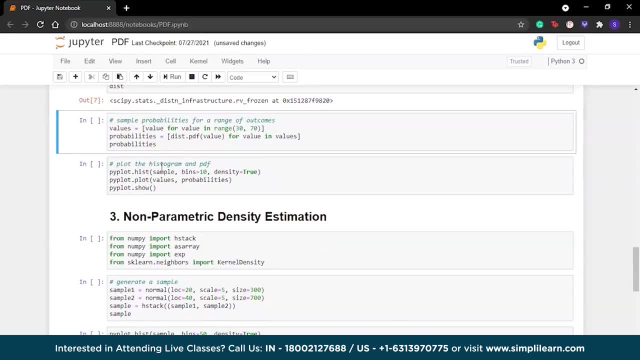 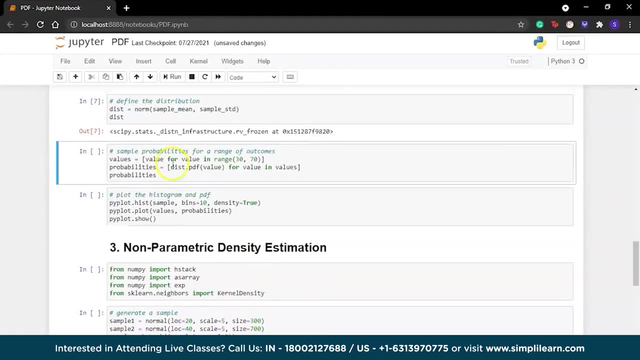 And up until now again, keep in mind we do not know for certain that it is a normal distribution. So far, all we have is this data, So the next thing that we're gonna do is fit the distribution with these parameters and then sample the probabilities for a 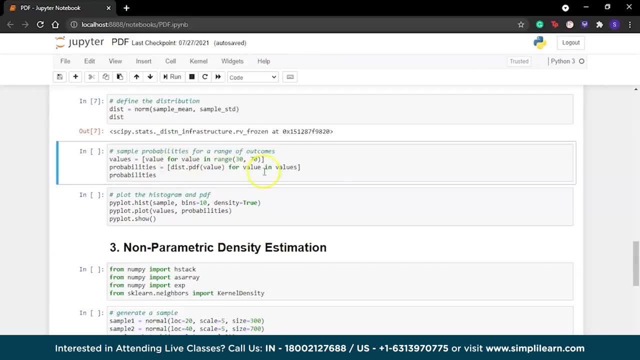 distribution for a range of values in our domain, which in this case is 30 and 70.. So all we're doing is we're calculating probabilities for a range of outcomes and in this case we've taken 30 and 70 as our domain. 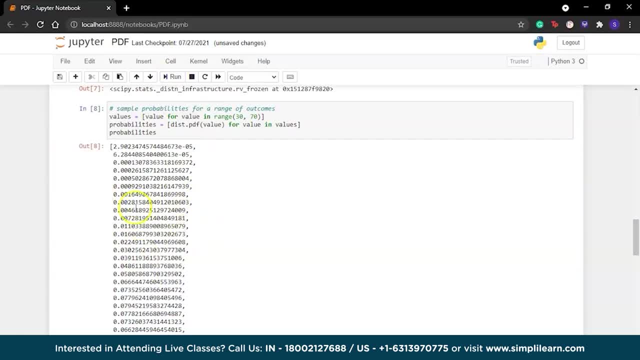 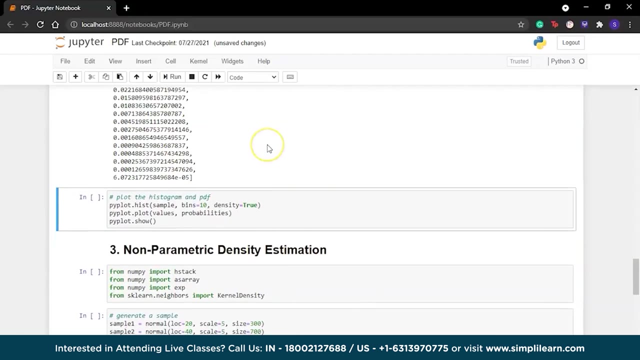 So these are the probability distribution values for the normal distribution that we've defined over here, and this is gonna- this is basically gonna- give you the outline of your normal distribution. These are the points at which your normal distribution will be plotted. Now, what we're basically gonna do is we're gonna: 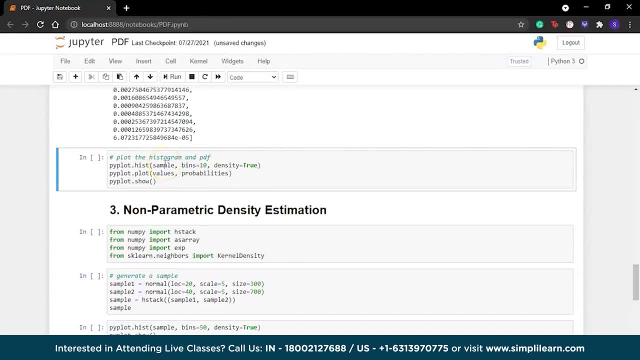 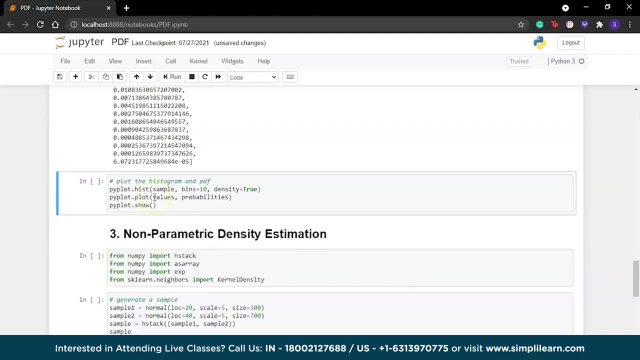 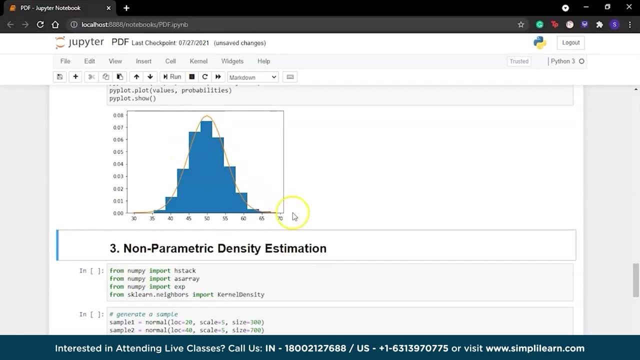 plot our histograms using the samples that we've already generated, along with the values and probabilities of the normal function that we defined over here. So, as you can see, it's an almost a complete fit. The normal distribution that we have here is made using the mean and the standard deviation. 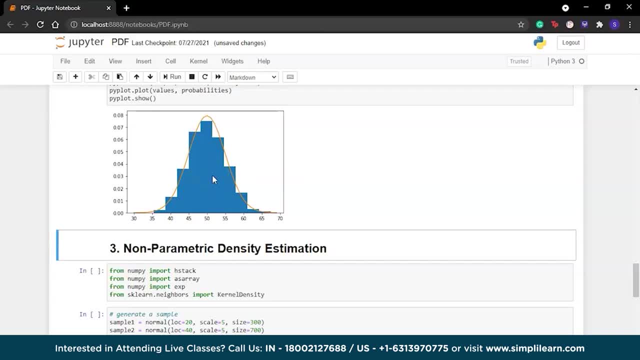 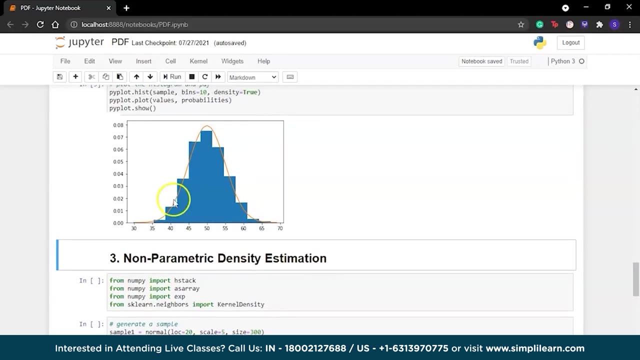 of our actual samples. The reason we took mean and standard deviation was because we assumed it was a normal distribution and the parameters associated with the normal distribution are mean and standard deviation. Using the mean and standard deviation, we got the normal distribution. We calculated probabilities. 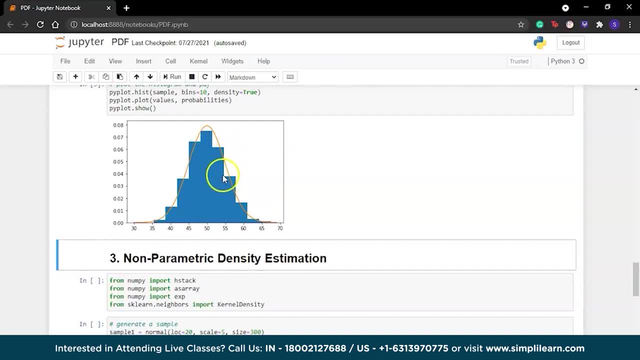 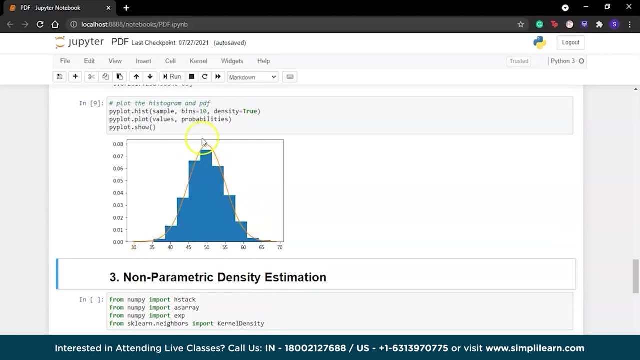 for this normal distribution using a random domain of 30 and 70, and we plotted the probabilities and the values on top of our histogram to see if the normal distribution was a fit to our histogram. If it was not a fit, you would have to go and do. 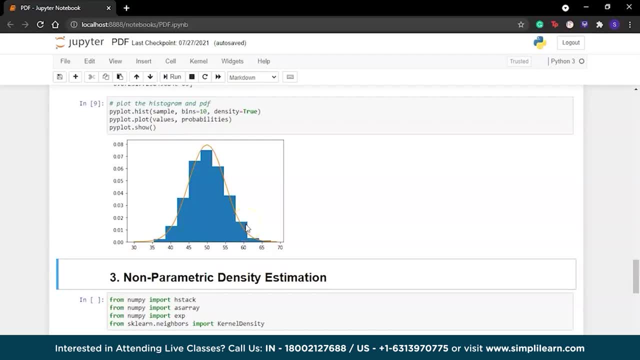 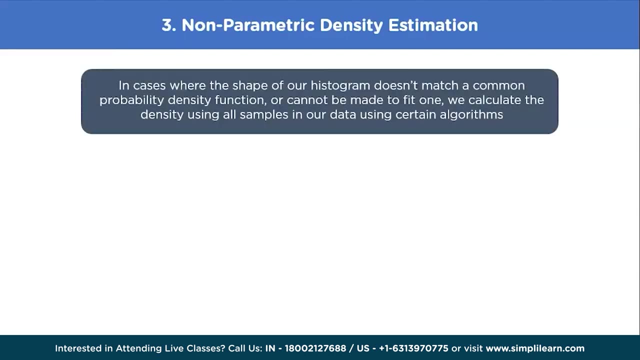 the same procedure with other common probability density functions until you found a function which was a proper fit to your histogram. Now let's move on to the final step, which is used in the calculation of our PDF. This final step is called non-parametric density estimation and 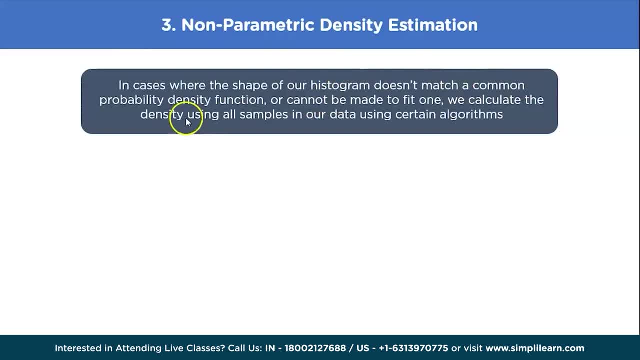 it's only used when the shape of our histogram doesn't match a common probability density function or it cannot be made to fit one. In this case, we will calculate the density using all samples in our data. using certain algorithms, This is only done when a data sample does not resemble. 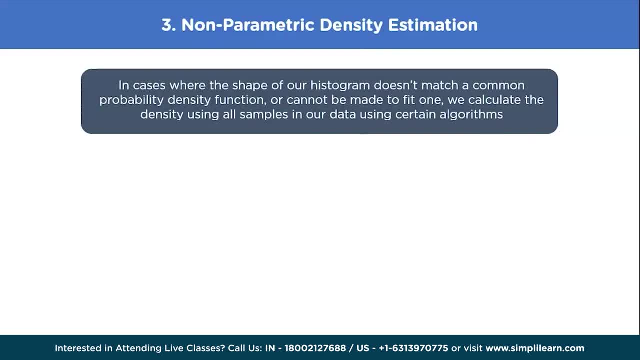 a common probability distribution or it cannot be easily made to fit the distribution. This is often the case when the data has two peaks- this is also called a bimodal distribution- or it has many peaks, which is also called a multimodal distribution, In this case, the parametric density. 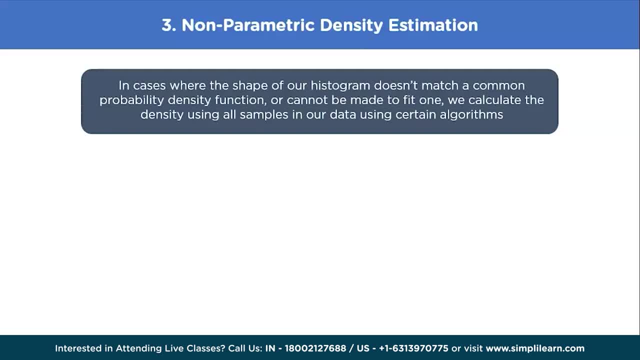 estimation will not be feasible and alternative methods can be used that do not use a common distribution. Instead, you will use an algorithm which is used to approximate the probability distribution of the data without a predefined distribution, which is also referred to as a non-parametric method, because we are 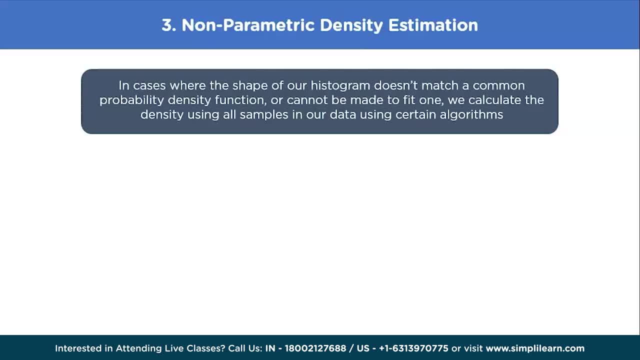 not using any predefined parameters. The distribution method will still have parameters, but these are not controllable in the same way as a simple probability distribution. For example, a non-parametric method might estimate the density using all observations in a random sample, in effect making all observations. 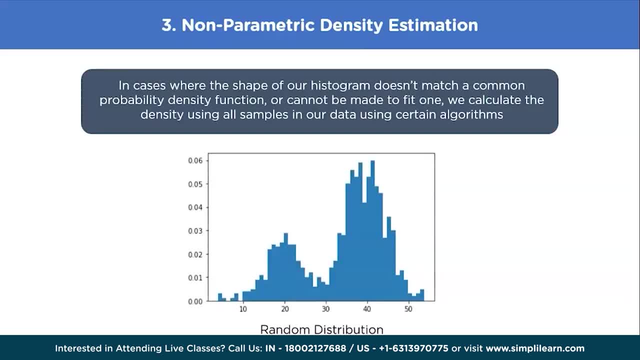 in the sample parameters. Now consider this graph, which has two peaks. This is not a normal distribution or any other sort of distribution that we are familiar with, So for this we are not going to use a parametric estimation method, but which is going to calculate? 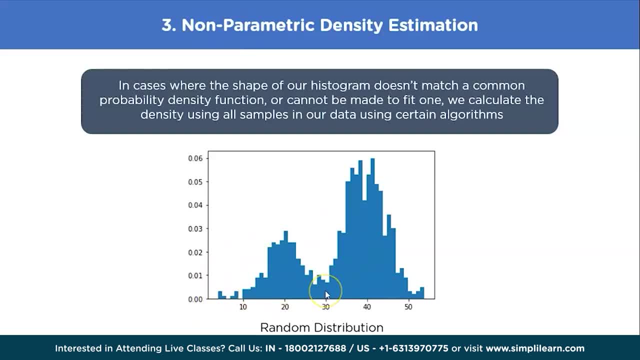 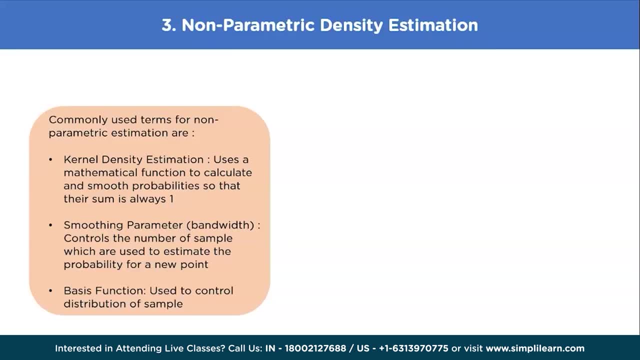 the parameters for every single sample point in this. Perhaps the most common non-parametric approach for estimating the probability density function of a continuous random variable is called kernel smoothing or kernel density estimation, or KDE for short. Kernel density estimation is a non-parametric method for using a 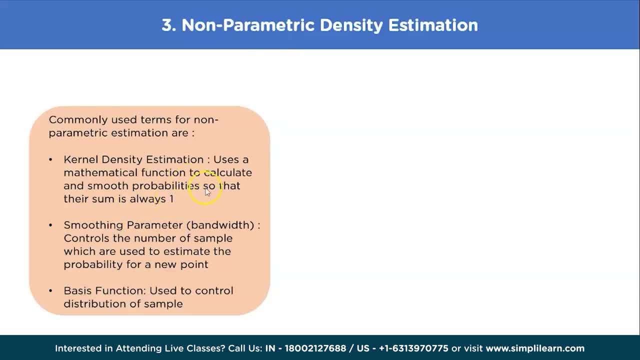 data set to estimate probabilities for new points. It uses a mathematical function and smoothing probabilities, so the sum of the resultant probabilities is always 1.. Now, in this case, a kernel is a mathematical function that returns a probability for a given value of a random variable. 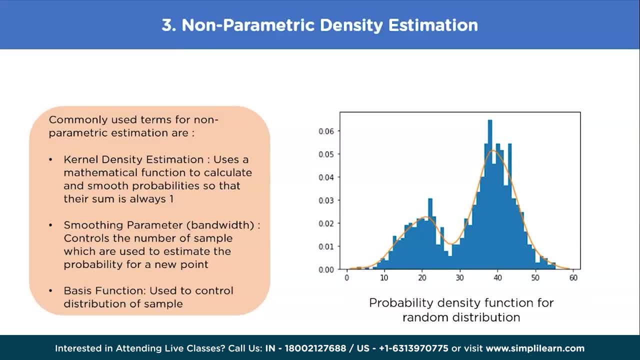 The kernel effectively smooths or interpolates the probabilities across the range of outcomes for a random variable, such that the sum of probabilities always equals 1, a requirement of well-behaved probabilities. You also have a parameter called the smoothing parameter, which controls the scope or the window of 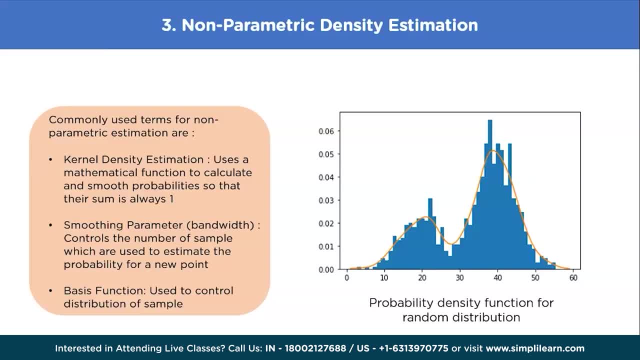 observations from the data samples. that contributes to estimating the probability for a given sample. As such, the kernel density estimation is sometimes referred to as your Parzen-Rosenbald window. Now, at the end, you also have a basis function, which is a function which is chosen to control the 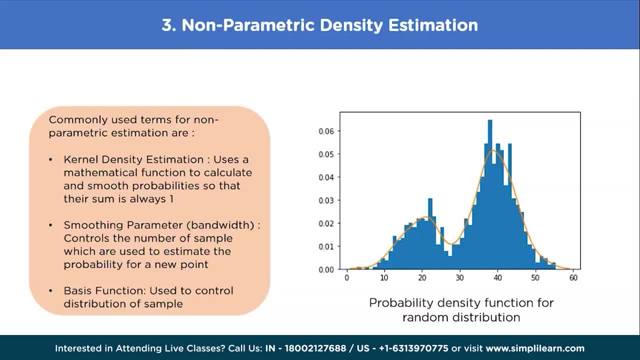 distribution of samples in the data set towards estimating the probability of a new point. This is only done to make sure that you are not learning from a lot of noise and that you are not using a lot of the outliers. Again, let's see how. 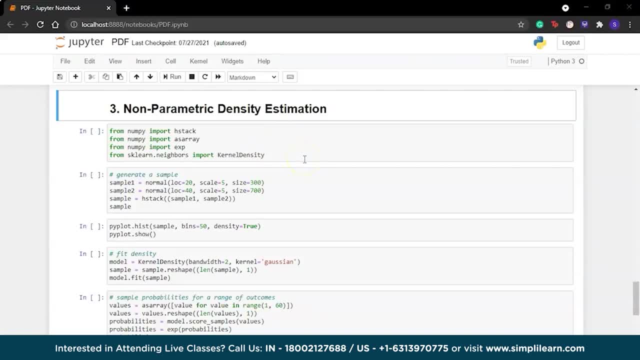 we can perform non-parametric density estimation with the help of Python. So first we will start by importing all the necessary modules, along with the kernel density estimation, which can be imported from sklearn. Now let's create a bimodule distribution by combining two different samples. 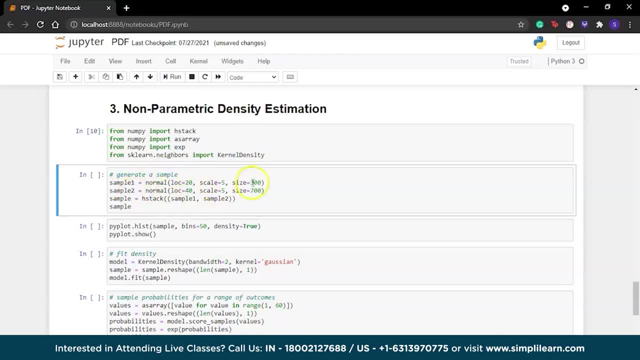 sample 1 and sample 2.. Sample 1 has 300 examples, with a mean of 20 and a standard deviation of 5, while sample 2 has 700 examples, with a mean of 40 and a standard deviation of 5.. We are then going to use HStack. 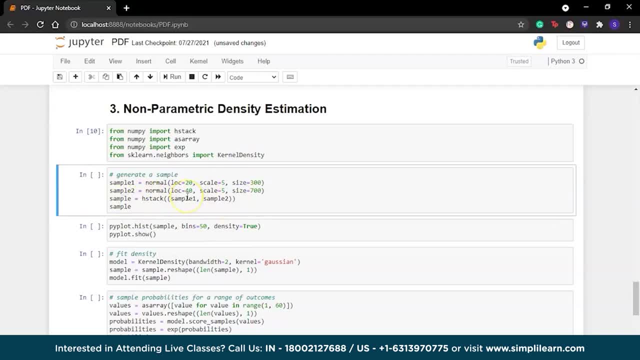 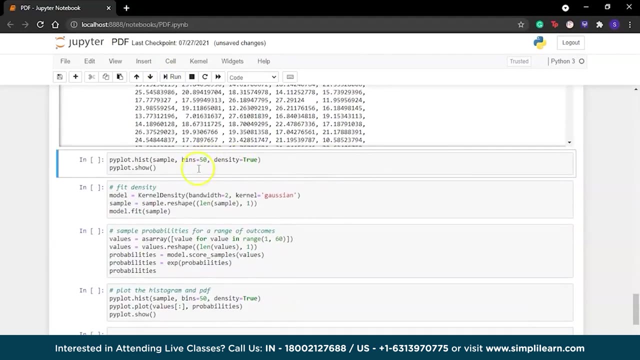 to merge both of them together to get a final sample. The means that we have chosen, which is 20 and 40, are chosen close together to ensure that the distributions overlap in the combined sample. So this is what our distribution is. Let's just 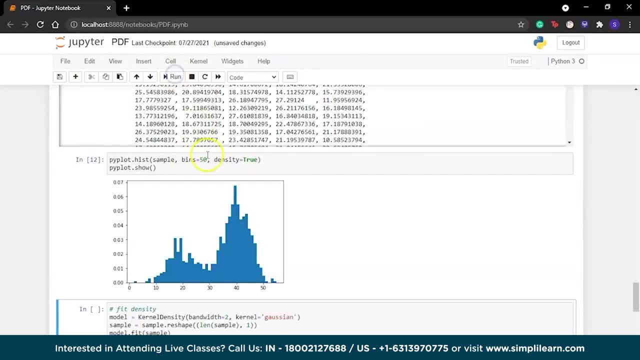 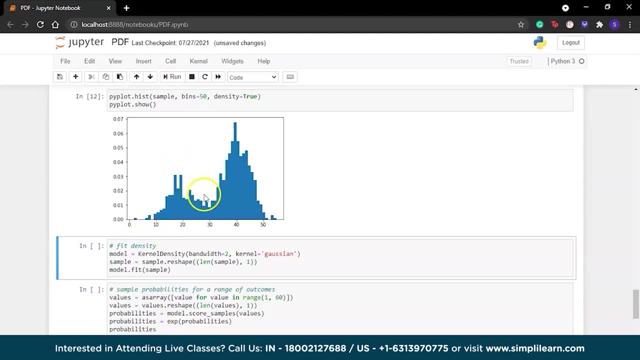 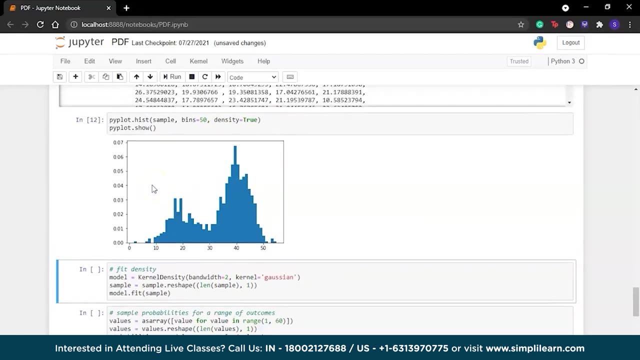 plot it so you get a basic idea of what our graph looks like. So this is what our graph looks like. Now we already know that none of the various different probability distribution functions fit these graphs, So now we are going to perform non-parametric estimations. 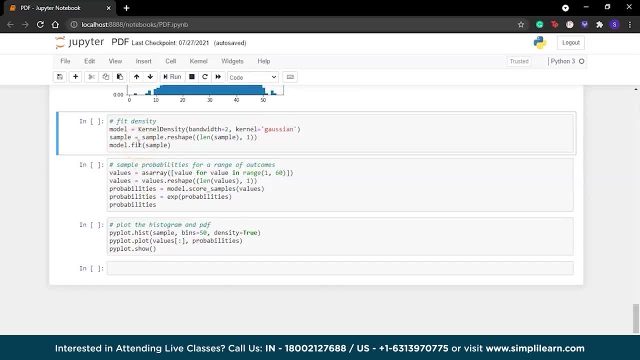 To perform non-parametric estimations, we are going to use the scikit-learn machine learning library, which provides the kernel density class that implements kernel density estimation. First, the class is constructed with the desired bandwidth or window size of 2.. And your basis function. 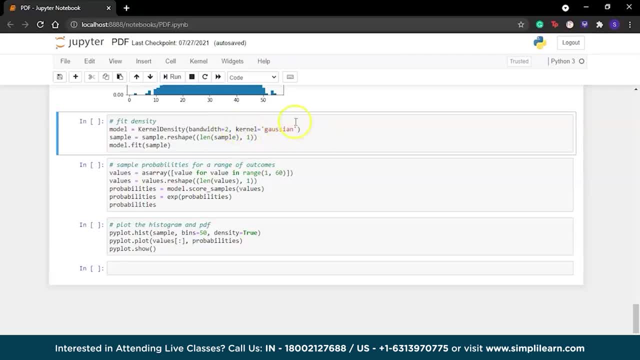 which, in this case, is a Gaussian function. It's a good idea to at least test different configurations to your data, and in this case we are only going to try a bandwidth of 2 and a Gaussian kernel, But usually there are multiple different kernels that you can. 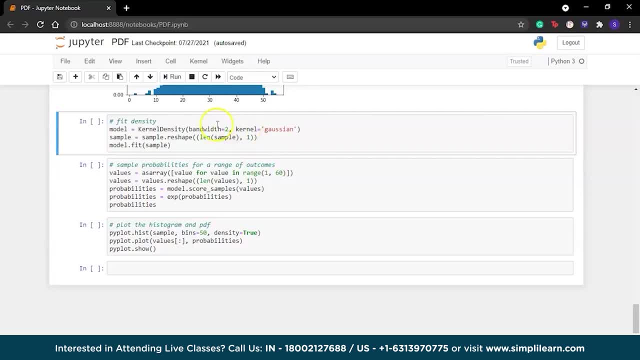 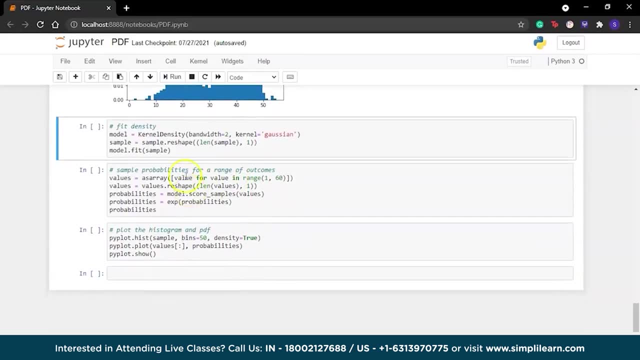 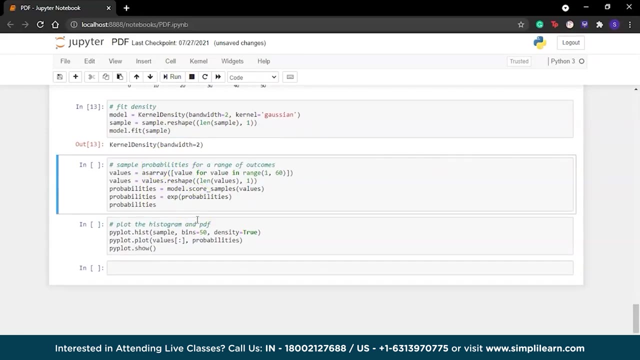 play around with, and you can also tweak your bandwidth to exactly fit the distribution that you have. Now let's run this. So now we have gotten our kernel density estimation. Now we can evaluate how well the density estimates matches our data by calculating probabilities for a range of observations. 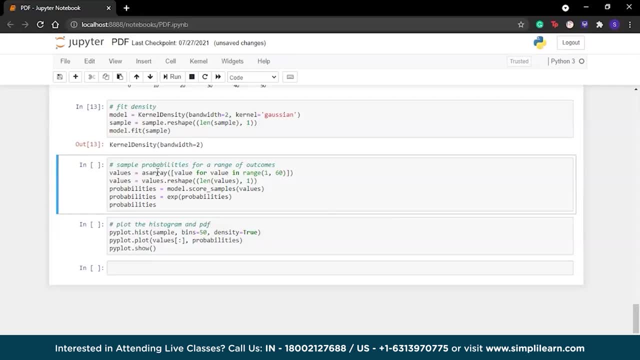 and comparing shapes to the histogram, Just like we did for the parametric case before. So again, we are going to just calculate different probabilities using the kernel density function And we are just going to plot it on top of our histogram to see how well 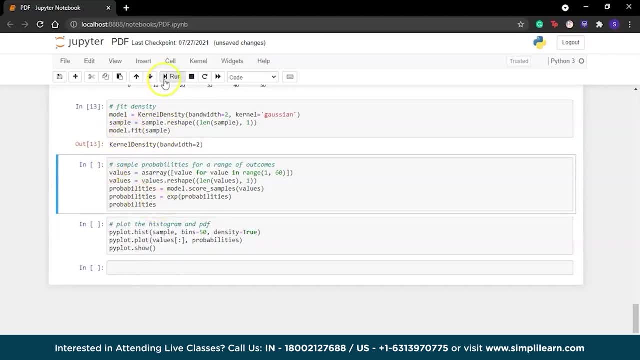 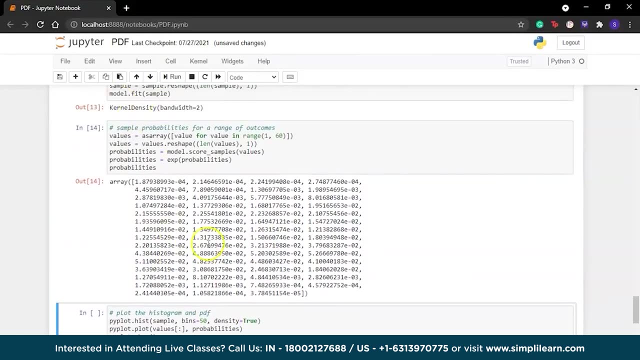 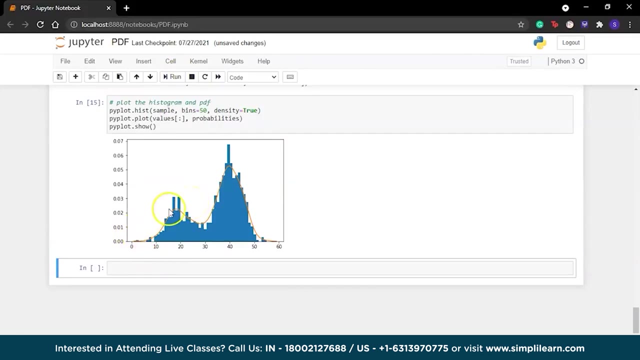 the kernel density function is estimating for our data. So these are the probabilities that we have gotten finally with the kernel density estimation And now we are going to plot it on top of our histogram. As you can see, it's almost a complete fit. It's just left out. 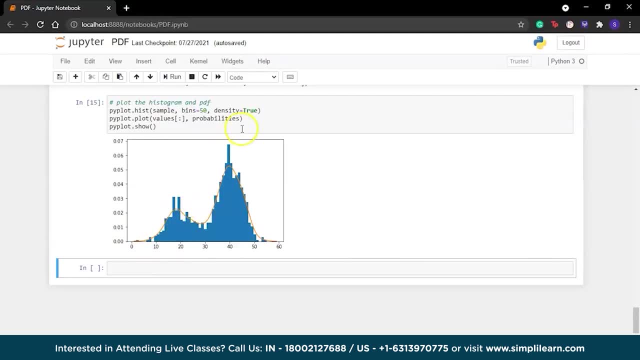 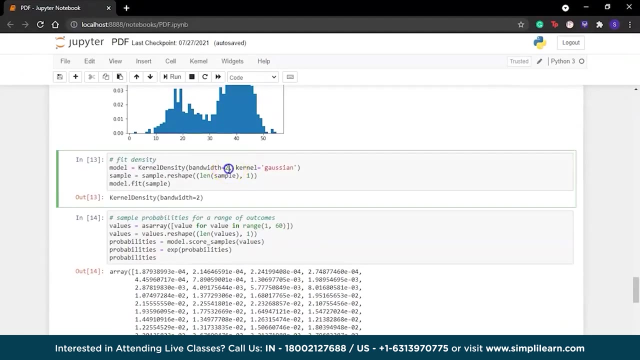 some of these outlier values, which again are ranging very high, But overall we have a pretty good fit. The only problem is it's not very smooth and you can again try tweaking the bandwidth to different values. So let's just, in this case, try tweaking it to 3. 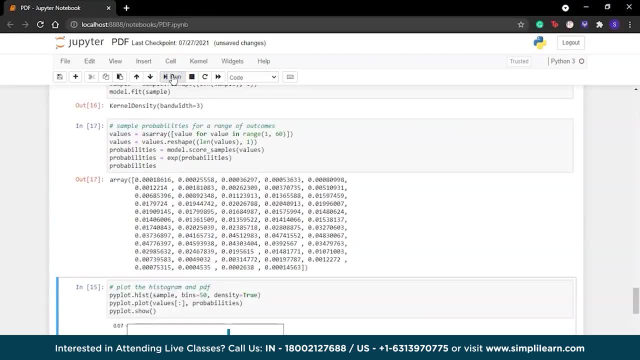 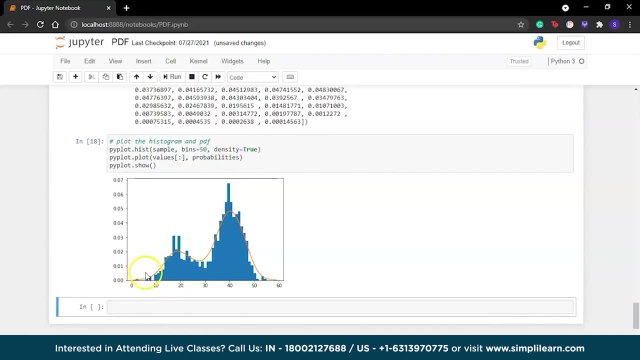 and see how well it runs. So now we have gotten new probabilities and let's run it on top of our bandwidth. So, again using a bandwidth of 3, you can see that we are fitting our data even better and we are again ignoring a lot. 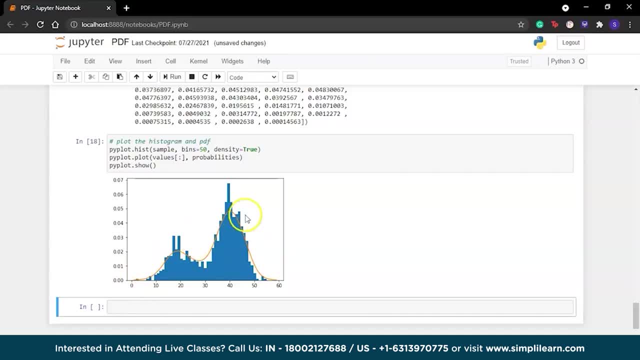 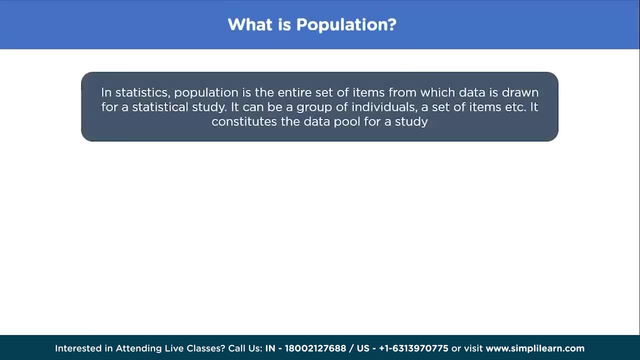 of the outliers which are out there, So this is going to give us a better estimation. So what is a population? In statistics, population is the entire set of items from which data is drawn for a statistical study. It can be a group of individuals, a set of items. 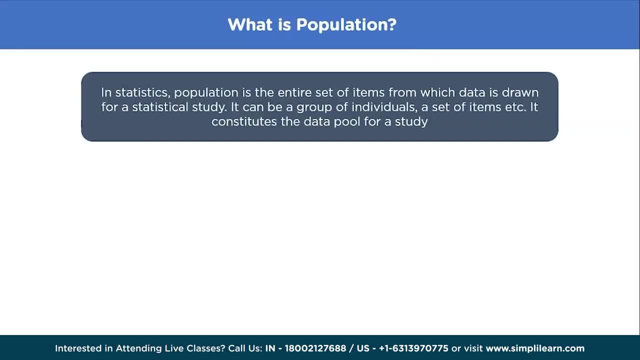 etc. It constitutes the data pool for a study In general. a population is the entire group that you want to draw conclusions about You. usually, when we talk about population, you think about the people living in an area at a time, But in research, a population doesn't always. 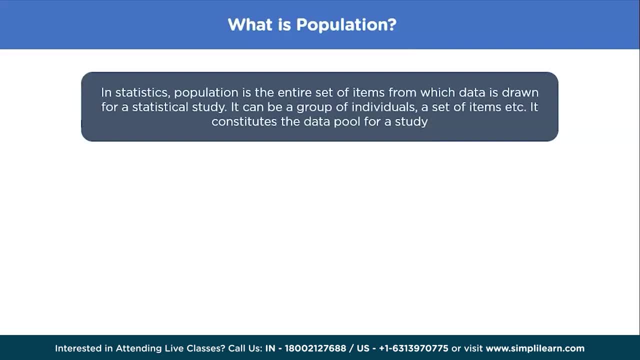 refer to people. It can mean a group containing elements of anything you want to study, such as objects, events, organizations, countries, species, organisms, etc. For example, all undergraduate students in the Netherlands or say: you would like to know whether there is an association. 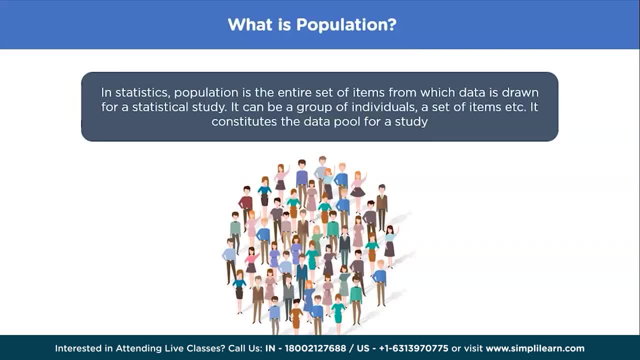 between job performance and the amount of home working hours per week in the specific case of Belgian data scientists. In this case, the population may be Belgian data scientists. However, if the scope of the study is more narrow, then the population will be more specific and include only. 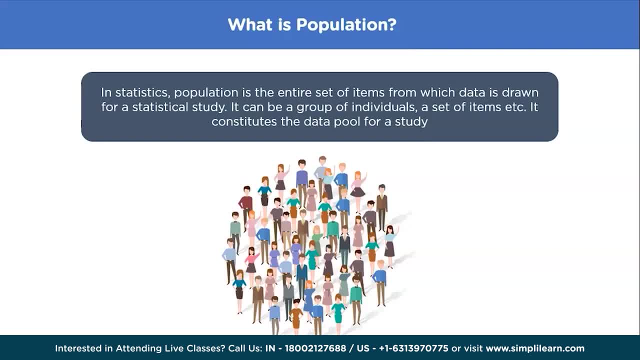 workers who meet that certain criteria. The point is that the population should only include people to whom the results will apply, Since, in this case and many others, it is impossible to observe the entire statistical population due to time constraints, constraints on geographical accessibility and constraints on the 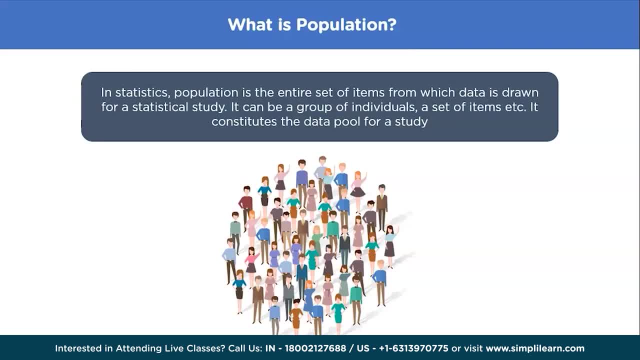 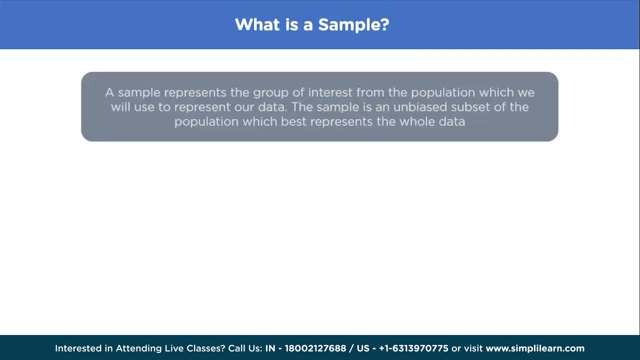 researcher's resources. a researcher would instead absorb the statistical sample from the population in order to attempt to learn something about the population as a whole. This brings us to the topic: What is a sample? A sample represents the group of interest from the population which. 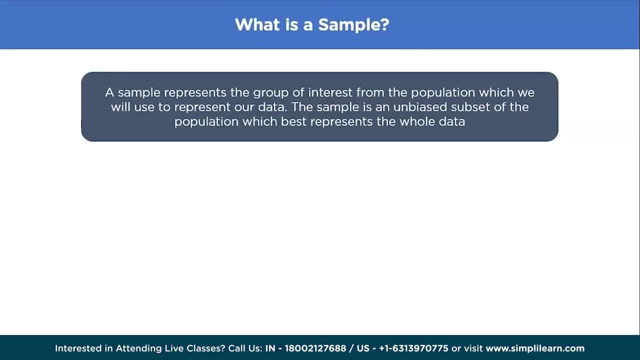 we will use to represent our data. The sample is an unbiased set of the population which best represents the whole data. A sample consists of some observations drawn from the population, So a part or a subset of the population. The sample is the group of elements. who actually 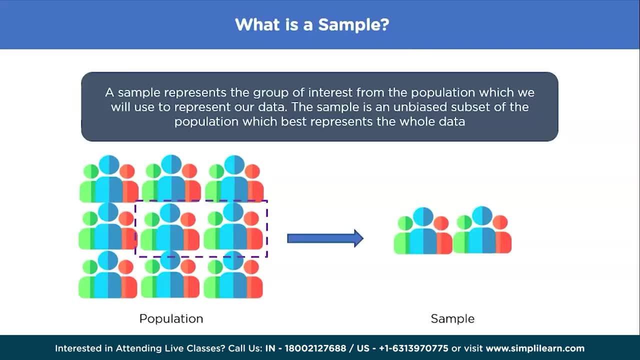 participated in the study. The size of the sample is always less than the total size of the population. Typically, the population is very large, making a census or a complete enumeration of all values in the population Impractical or impossible. The sample represents: 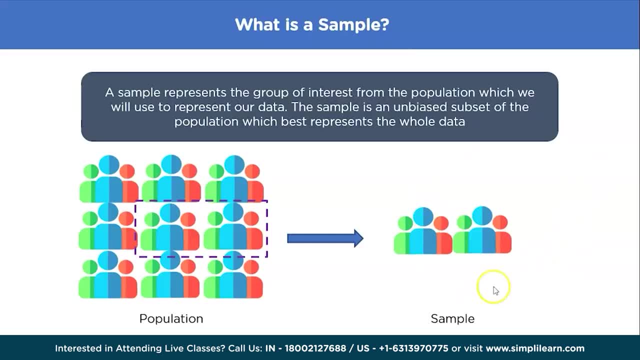 a subset of manageable size Samples are collected and statistics are calculated from the sample so that one can make interferences or extrapolations from the sample to the population. This process of collecting information from a sample is referred to as sampling. Say you are testing? 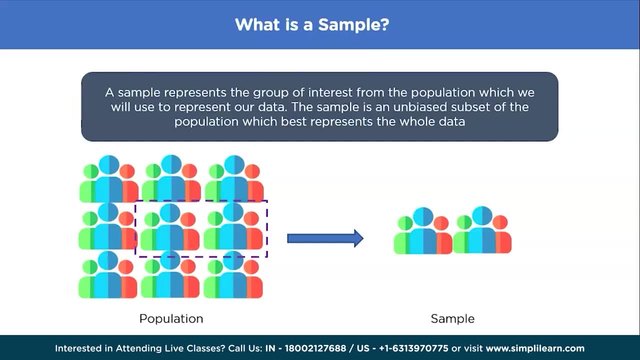 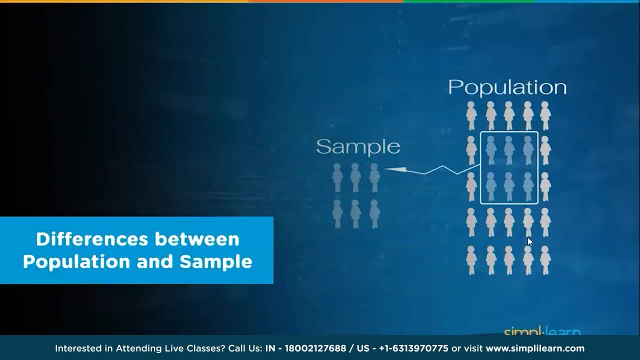 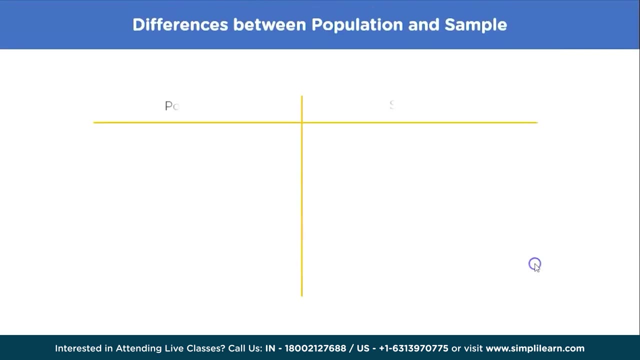 the effects of a new fertilizer on crop yield. All the crop fields represent your population, Whereas the 10 crop fields you tested correspond to your sample. Now let's look at the differences between population and samples with the help of some examples. The first example would be that 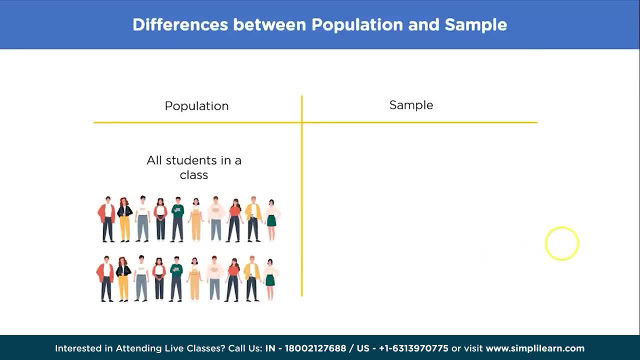 all students in a class would constitute the population of that class. A sample would be only the top 10 students within the same class. The sample is a small subset of the population. in this case, Advertisements for IT jobs in India would mean the complete. 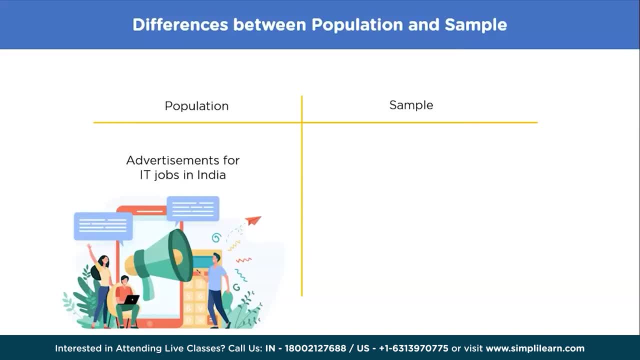 search results that pops up when you search IT jobs in India. A sample of that would be the top 50 advertisements for the same jobs. Another example is all countries of the world. This represents a population of all the countries. A sample would be: 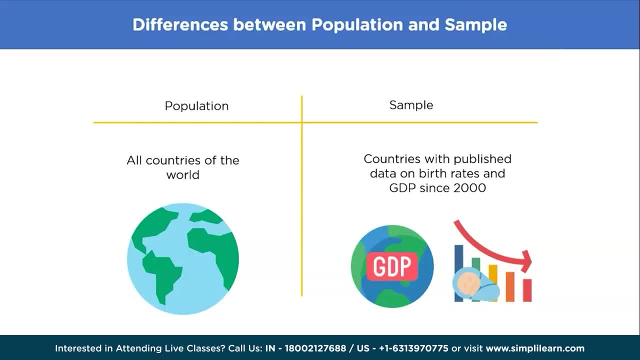 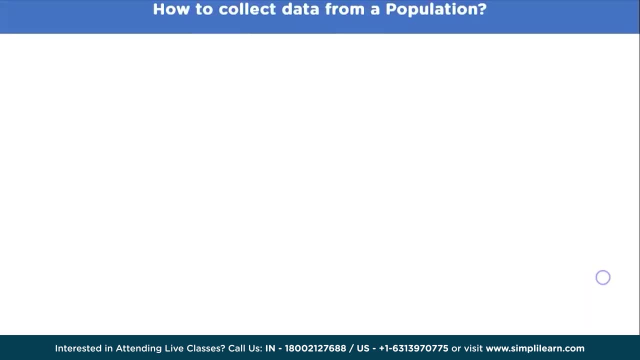 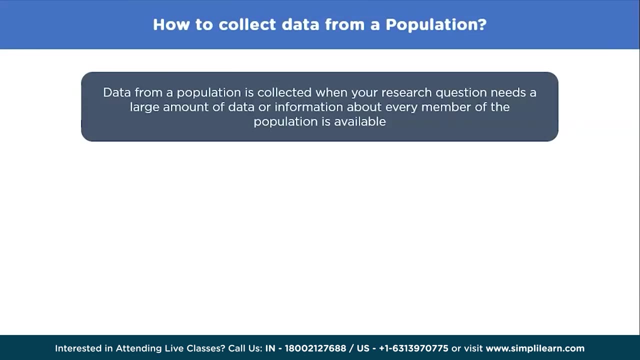 countries with published data on birth rates and GDP since 2000s. Next, let's look at how to collect data from a population. Data from a population is collected when your research question needs a large amount of data or information about every member of the. 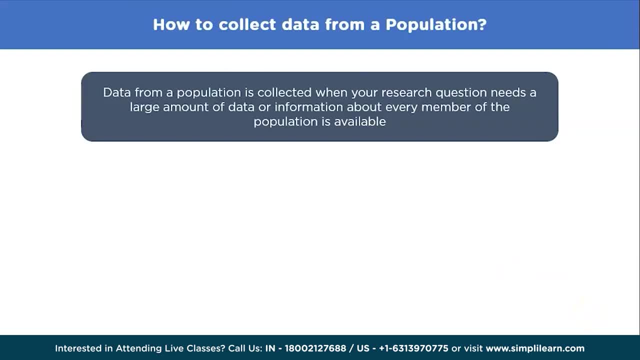 population is available. Populations are used when your research question requires or when you have access to data from every member of the population. Usually, it's only straightforward to collect data from a whole population when it is small, accessible and cooperative. Population data is used when the data 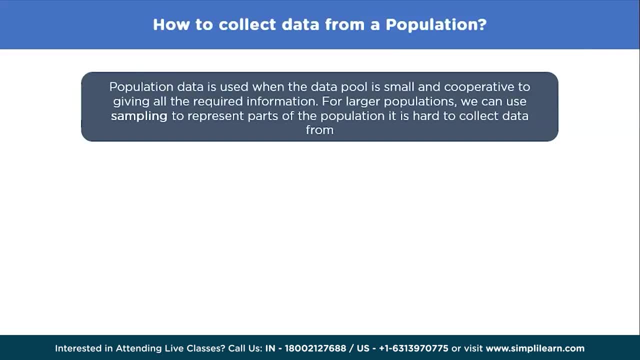 pool is small and cooperative to giving all of the required data. For larger populations, we can use sampling to represent part of the population. It is hard to collect data from. For example, a high school administrator wants to analyze the final exam scores of 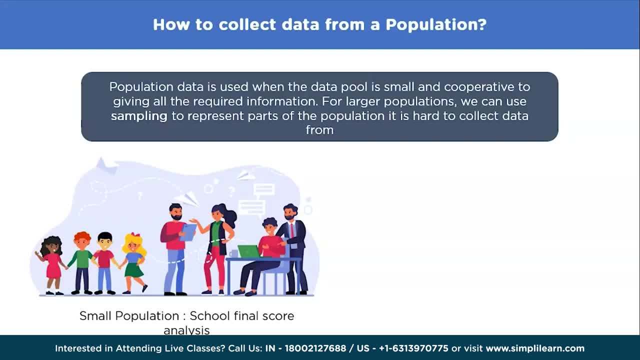 all graduating seniors to see if there is a trend. Since they are only interested in applying the findings to the graduating seniors in this high school, they can use their whole population data set. For larger and more dispersed populations, it is often difficult or impossible to collect data. 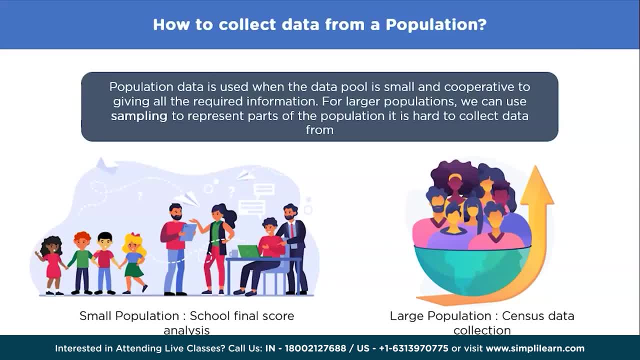 from every individual. For example, every 10 years, the federal US government aims to count every person living in the country using the US Census. This data is used to distribute funding across the nation. However, historically, marginalized and low-income groups have been difficult. 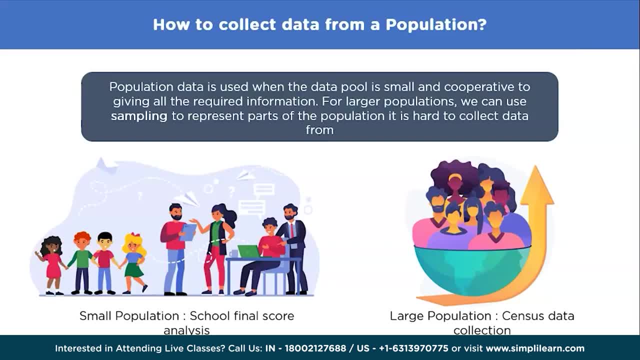 to contact, locate and encourage participation from. Because of non-responses, the population count is incomplete and biased towards some groups, which results in disproportionate fundings across the country. In cases like this, sampling can be used to make more precise interferences about the population. 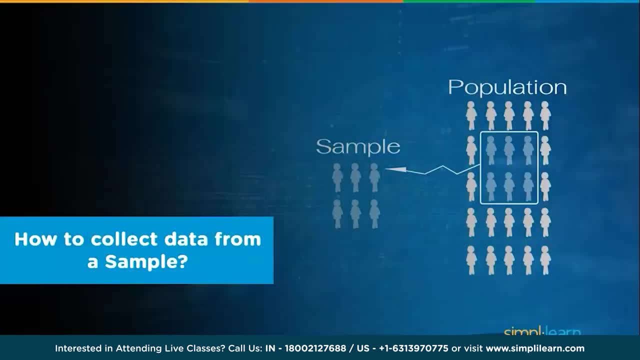 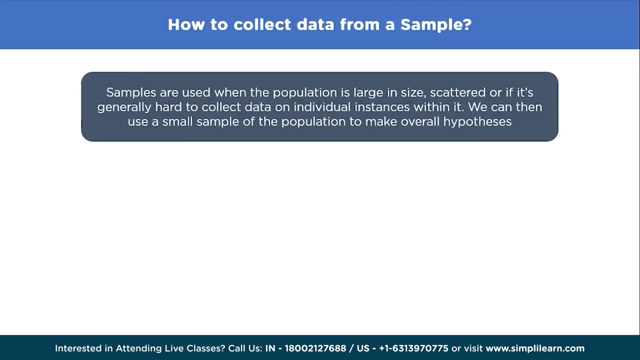 And for that we can collect data from a sample. How do we go about collecting data from a sample? Samples are used when the population is large in size, scattered, or it is generally hard to collect data on individual instances in it. We can use a small sample. 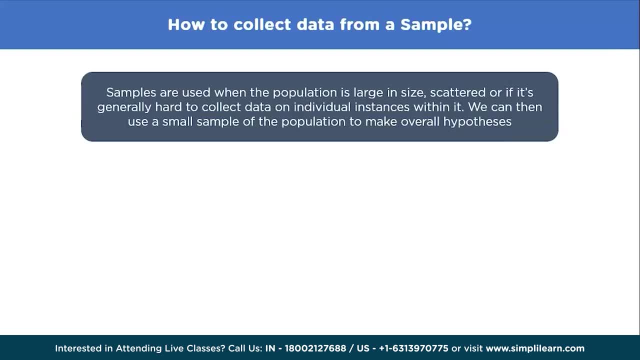 of the population to make overall hypotheses. When your population is too large in size, geographically dispersed or difficult to contact, it is necessary to use a sample. With statistical analysis, you can use sample data to make estimates or test hypotheses about population data. 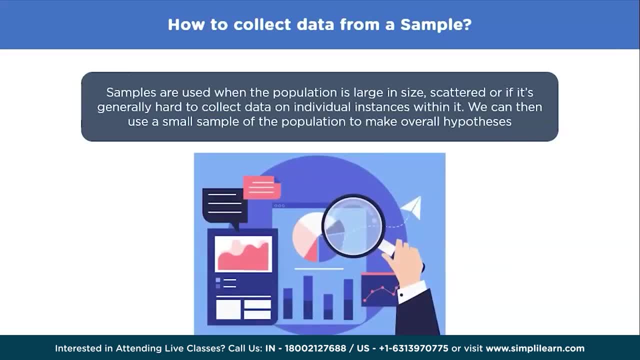 For example, you want to study political attitudes in young people. Your population is the 3,000 undergrads in the Netherlands. Because this is not practical to collect data from all of them, you use a sample of 300 undergraduate volunteers from three Dutch. 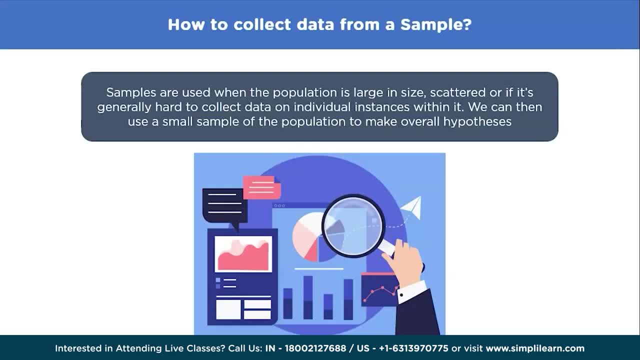 universities. This is the group who will complete your online study. Ideally, a sample should be randomly selected and representative of the population. Using probability sampling methods such as simple random sampling or stratified sampling reduces the risk of sampling bias and enhances both. 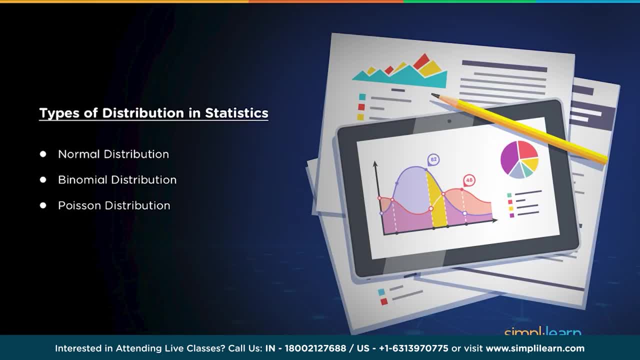 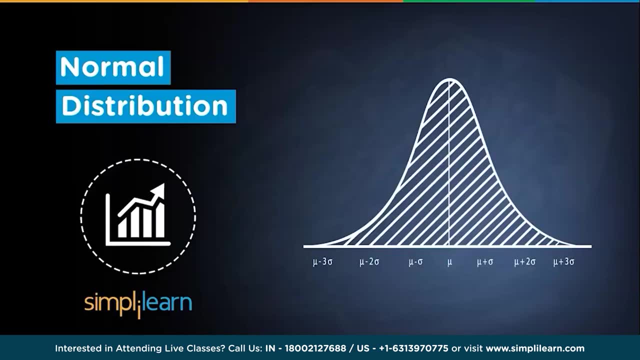 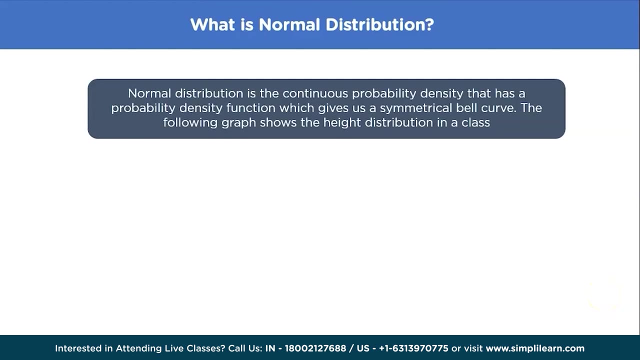 internal and external validity. We will discuss the three main types of probability distribution, that is, normal, binomial and Poisson distribution. So let's move ahead. So what is normal distribution? Normal distribution is a continuous probability density that has a probability. 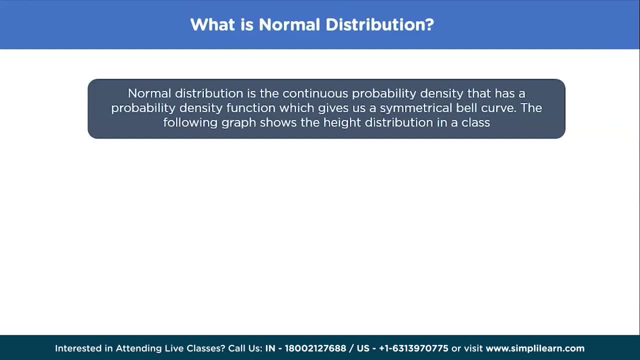 density function, which gives us a symmetrical bell curve. Now data can be distributed or spread out in different ways, But there are many cases where the data tends to be around a central value, with no bias to the left or right, which means that it doesn't. 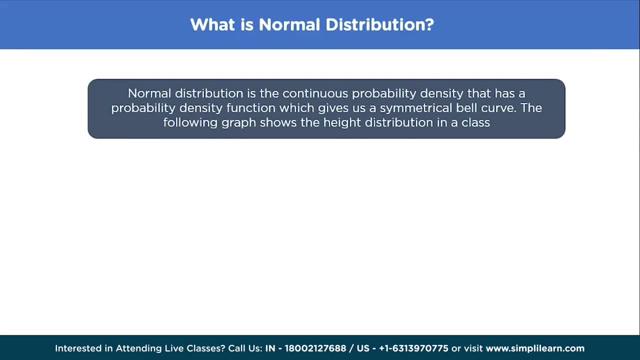 show any particular spikes towards the left or the right, And it gets close to a normal distribution. Half of the data will fall on the left of the mean and the other half will fall on the right. Now let's take a look at a 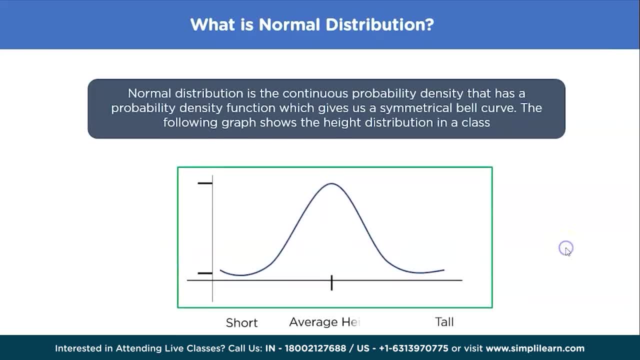 graph which shows the height distribution in a class. As you can see, the average height is in the middle and the data to the left of the average height represents the short people and the data to the right of it represents the taller people. The y-axis shows us the 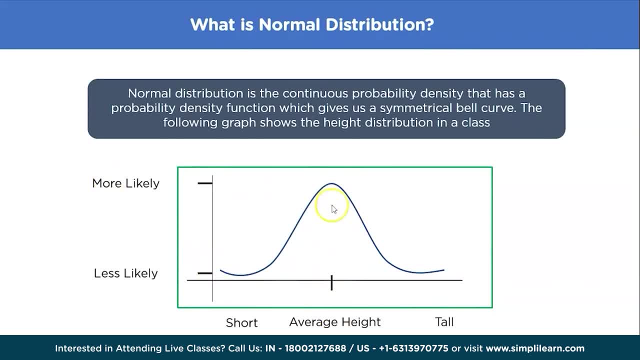 likelihood of any of these heights occurring. The average height has the most distribution or it has the most number of cases in the class, And as the height decreases or increases, the number of people who have that height also decreases. This kind of a distribution. 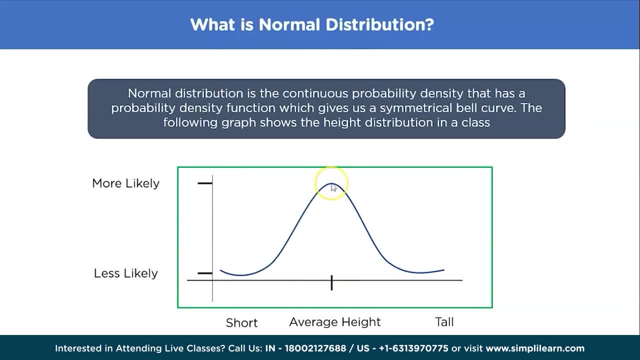 is called a normal distribution, where the average or the mean is always the highest point and any other point after that or before that is significantly lower. The resulting data gives us a bell curve and, as you can see, there is no abrupt bias or spike in the data. 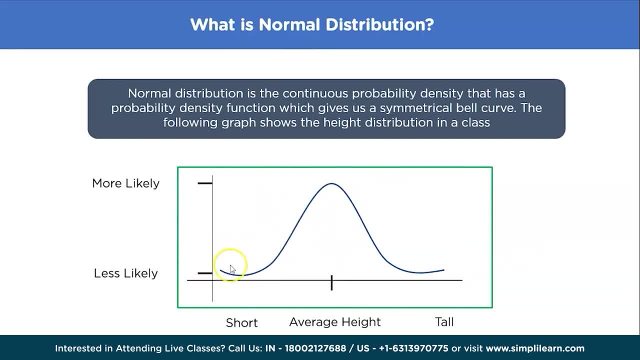 anywhere except for the average height. So this kind of a curve is called a bell curve, and it's usually seen in a normal distribution. The reason we call this a normal distribution is because the data is normally distributed with the average being the highest and 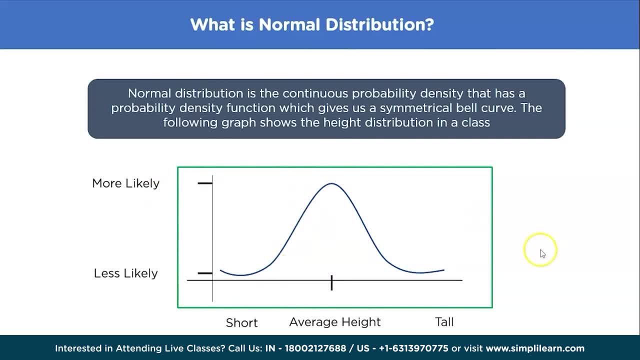 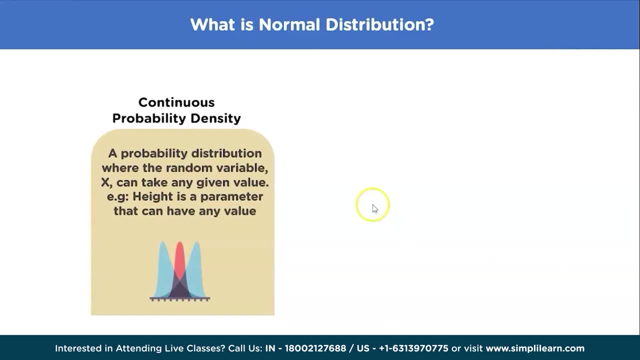 all the other data points having a lower likelihood. Now we came across two terms which are associated with normal distribution: continuous probability density and probability density function. What is continuous probability density? Continuous probability density is a probability distribution where the random variable x can take any given 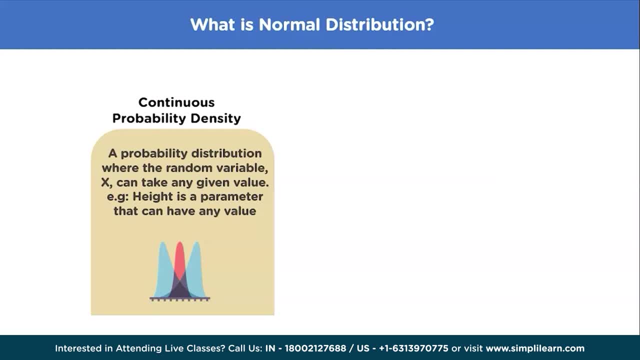 value because there are infinite values that x could assume. the probability of x taking on any specific value 0.. For example, let's say you have a continuous probability density for men's height. What is the probability that a man will have the exact height? 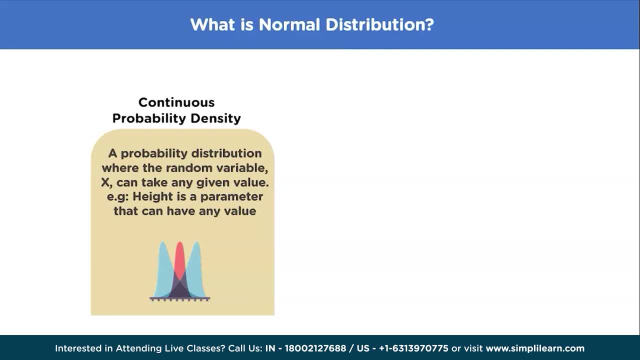 of 70 inches. It is impossible to find this out because the probability of one man measuring exactly 70 inches is very low. It is more probable that he will measure around 70.1 inches or maybe 69.97 inches, and it doesn't stop there. 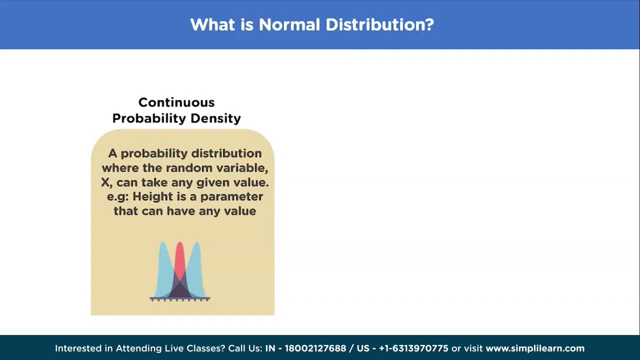 The fact is that it is impossible to exactly measure any variable that is on a continuous scale and because of this it is impossible to figure out the probability of one exact measurement which is occurring in a continuous probability density. Next we have the probability density function. 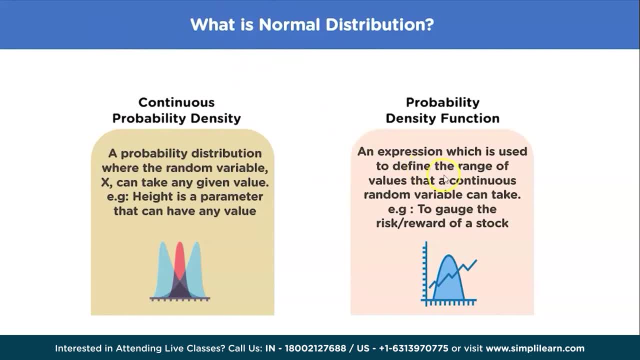 It is nothing but a function or an expression which is used to define the range of values that a continuous random variable can take. An example of this would be to gauge the risk and reward of a stock. A probability density function is a statistical measure which is used to gauge the 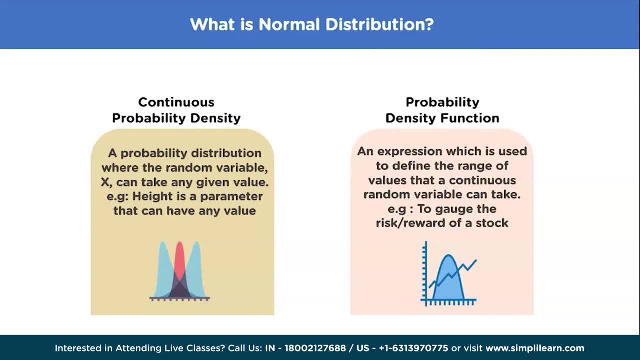 likelihood of a discrete value. A discrete variable can be measured exactly, while a continuous variable can have infinite values. However, for both continuous as well as discrete variables, we can define a function which gives us the range of values within which these variables will fall. 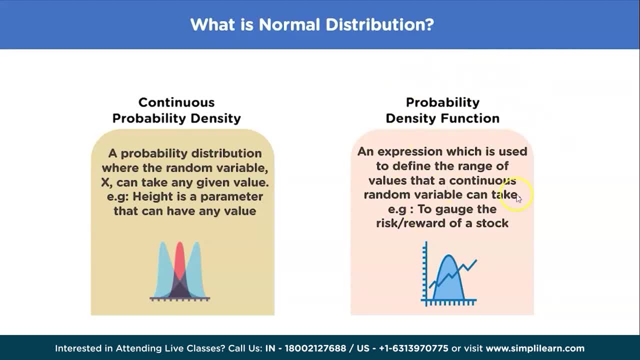 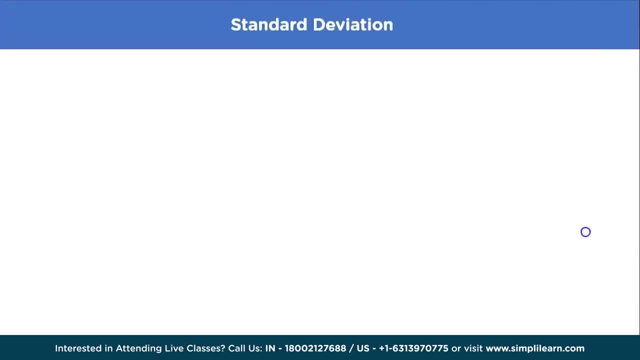 and that function is known as the probability density function. Now let's take a look at standard deviation. What is standard deviation? Standard deviation is used to measure how the values in your data differ from one another, or how spread out your data is A standard deviation. 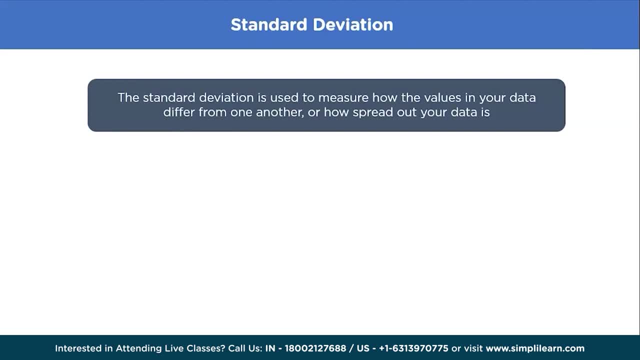 is a statistic that measures dispersion of a data set relative to its mean. The standard deviation is calculated as the square root of variance by determining each data point's deviation relative to the mean. If the data points are further from the mean, that means that there is a higher deviation. 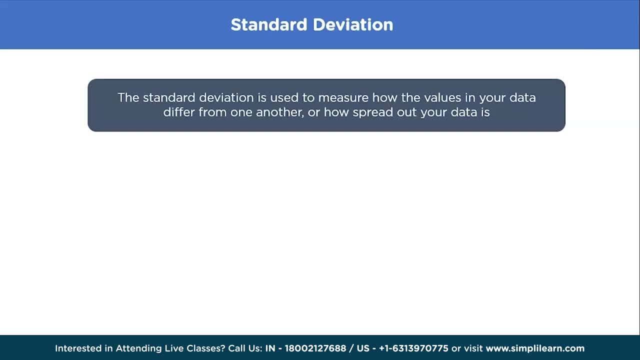 within the data set, and then the data is said to be more spread out. This leads to a higher standard deviation too. Let's take an example of income in rural and urban areas. In rural areas, let's say, such as farming areas, the income doesn't differ that much. 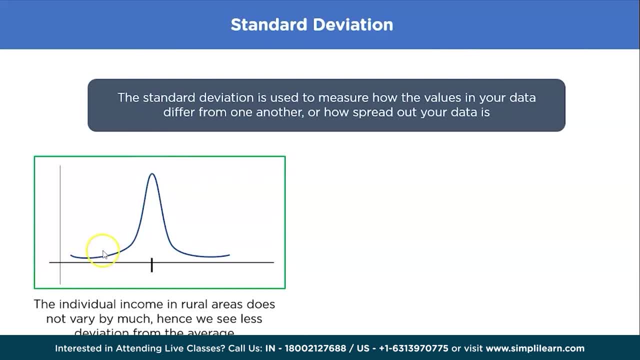 More or less everyone earns the same. Because of this, our bell curve has a very low standard deviation and it has a very narrow peak. However, in urban areas, the wealth distribution is very uneven. Some people can have very high incomes and can be earning a lot. 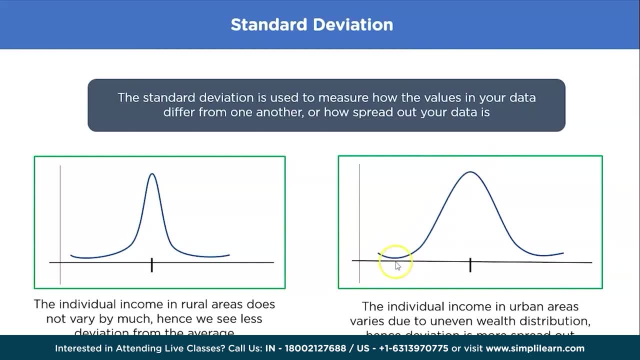 while other people can have very low incomes. Furthermore, the data distribution between these two income points is going to be more spread out because there are a lot more people living there who work in various fields and who have various incomes. Because of this, our standard deviation is more spread out. 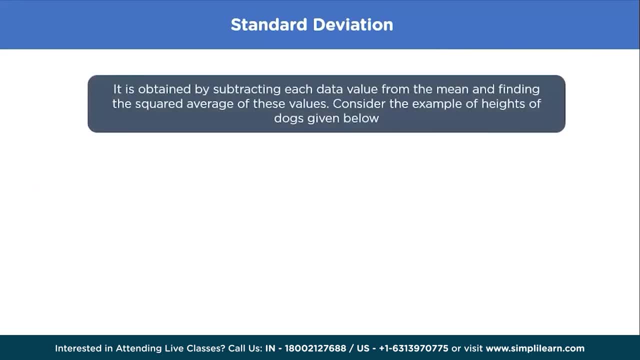 and our bell curve will also have a wider peak. Now, how can we find the standard deviation? Standard deviation is obtained by subtracting each data value from the mean and finding the squared average of these values. Let's look at how we can do this. 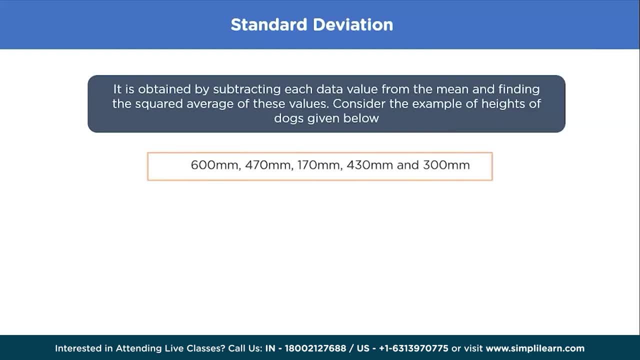 with the help of an example. These values correspond to the height of various dogs. We can find the mean by finding the average of all these values, which is nothing but adding all the values and dividing it by the total number of values, The mean that we get. 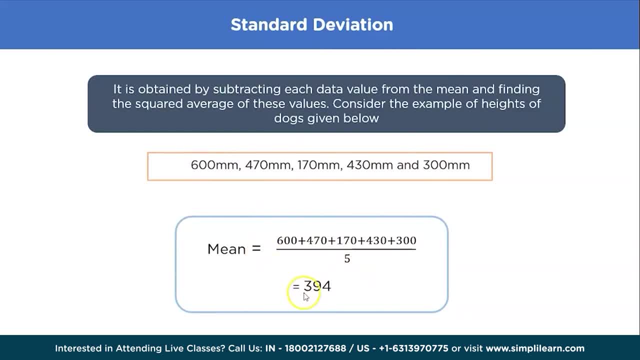 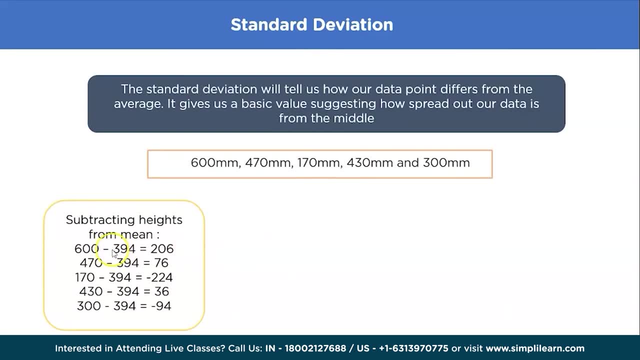 is 394.. This means that the average height of a dog is 394 mm. To find the standard deviation, first we need to subtract the height from the mean. This will tell us how far from the mean our data points actually are. Next we will square up. 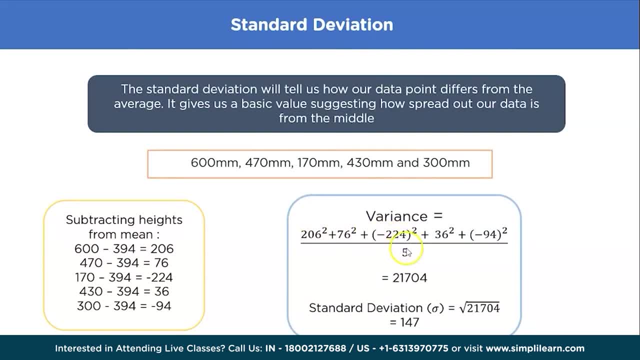 all of these differences and add them up and again, divide it by the total number of values that we have. This is called the variance. The variance that we get in this case is 21704.. Finally, when we find the square root of this value, we will get the standard deviation. 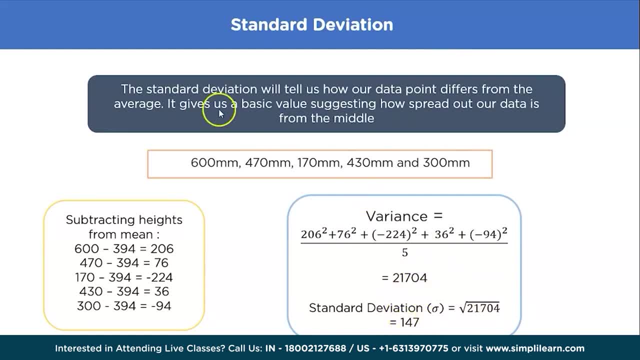 The standard deviation here is 147.. The standard deviation will tell us how our data points differ from the average And it gives us a basic value suggesting how spread out our data is: from the very middle or from the mean. So when we plot these values, 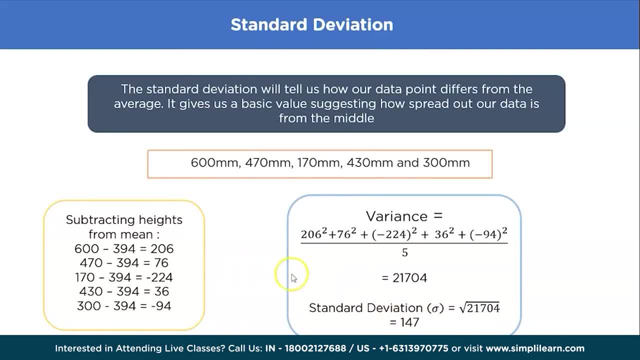 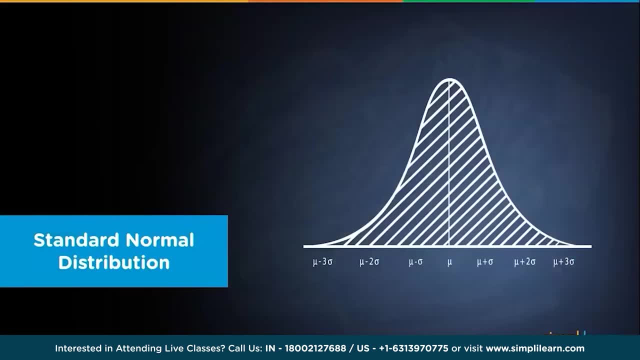 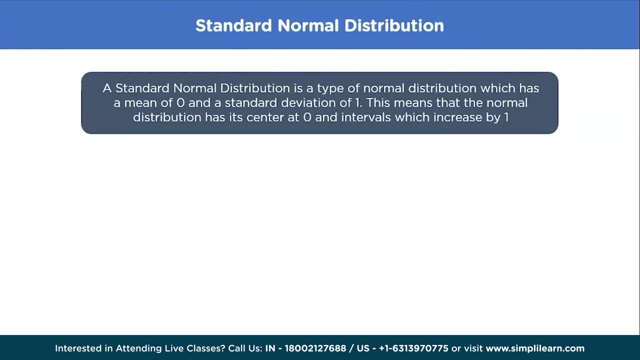 this value, 147 will mean that a curve will have a width of 147 points around the mean. Now, what is the standard normal distribution? The standard normal distribution is a type of normal distribution that has a mean of 0 and a standard deviation of 1.. 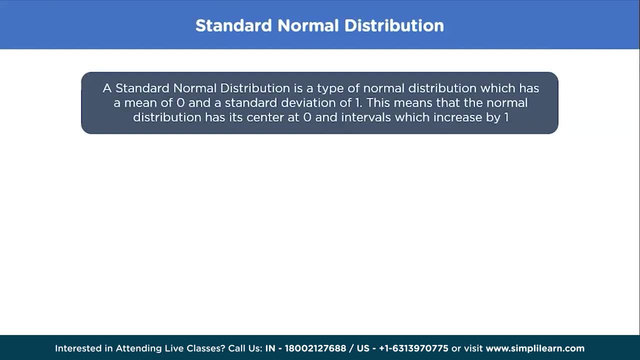 This means that the normal distribution has its center at 0 and it has intervals which increase by 1.. All normal distributions, like the standard normal distribution, are unimodal and symmetrically distributed with a bell shaped curve. However, a normal distribution can take on. 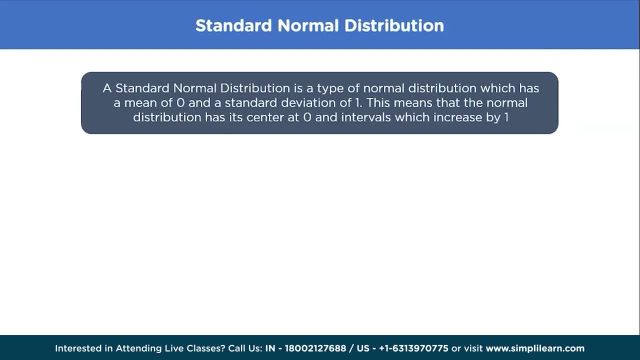 any value as its mean and standard deviation. In the standard normal distribution, however, the mean and standard deviation are always fixed. When you standardize a normal distribution, the mean becomes 0 and the standard deviation becomes 1.. This allows you to easily calculate. 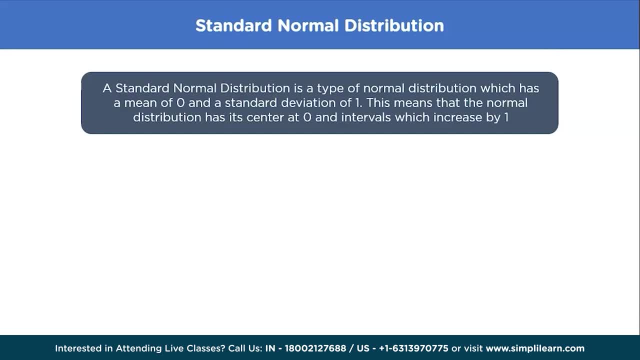 the probability of certain values occurring in your distribution, or to compare data sets with different mean and standard deviations. The curve shows a standard normal distribution. As you can see again, the data is centered at 0.. This does not mean that the data necessarily starts at 0.. 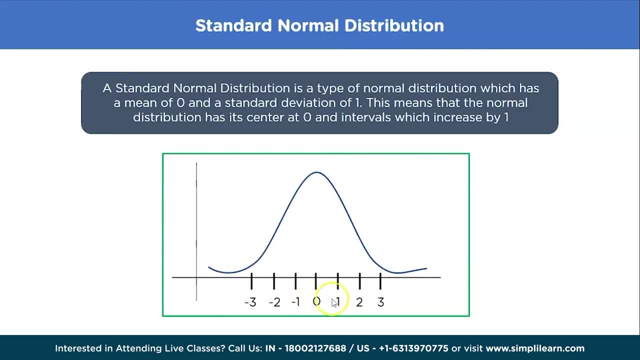 This means that after standardizing, this point is where our mean will lie. In a standard normal distribution, the standard deviation is 1.. So all the data points will increase or decrease in steps of 1.. Let's better understand a standard normal distribution with the help. 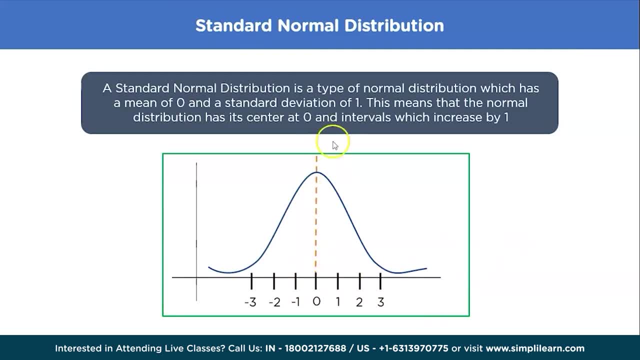 of an example. Again, as you can see, the data is centered around 0,, which is nothing but the mean. Let's again consider the weights of students in class 8th. The average weight here is around 50 kgs and the data 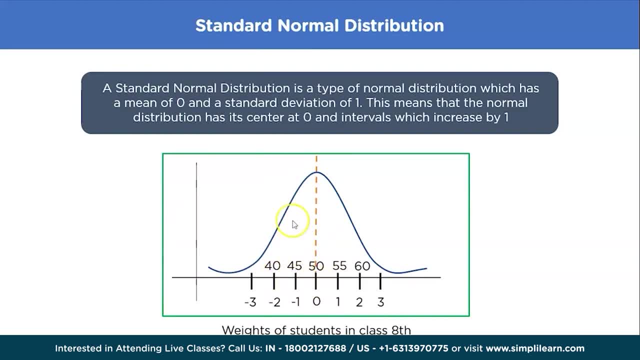 increases and decreases in steps of 5. The data over here in this curve is evenly distributed along these steps. This is what a standard, normal distribution will look like. We already know that the mean of our data is 50 and because the data is increasing and decreasing, 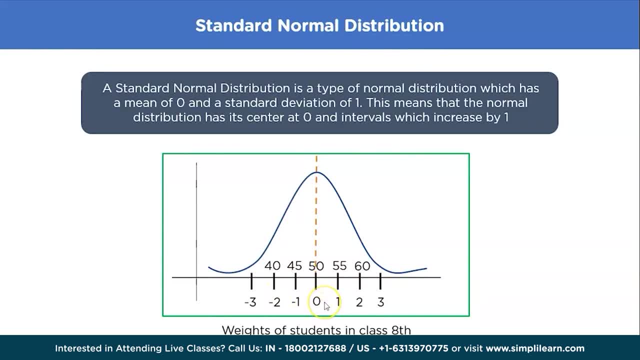 in equal steps. we can just standardize it and take it to mean that the data is increasing and decreasing in steps of 1.. This is what a standard, normal distribution looks like, and when you have a data which looks like this, you can always standardize it and convert it into. 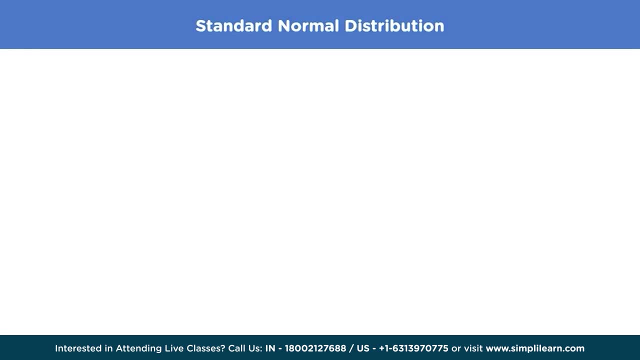 a standard normal distribution. Now, standard normal distribution has a couple of properties which makes calculation comparatively easy. The first one is that 68% of the values fall within the first standard deviation, which means that 68% of all data values on this curve will fall. 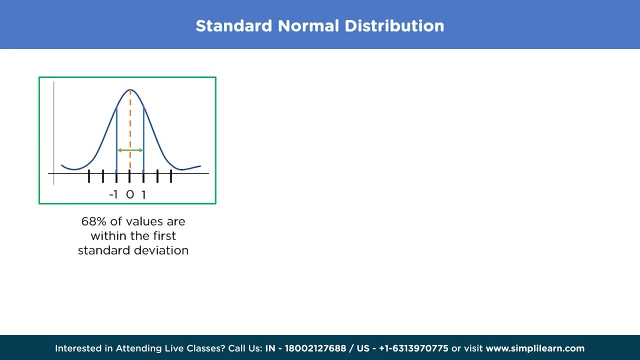 between the range of or the first interval ranging from to 1.. The second property is that 95% of the rest of the values are within the second standard deviation, or from the second negative point to the second positive point And finally 99.7%. 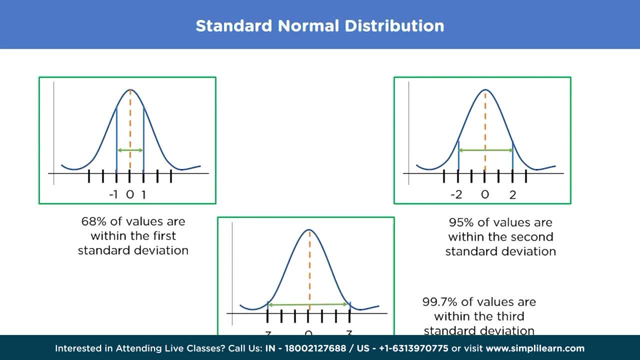 of the values fall within the third standard deviation or from the third negative point to the third positive point. This makes calculations on standard normal distribution fairly easy. You can compare scores on different distributions with different means and standard deviations. You can normalize scores for statistical decision making. 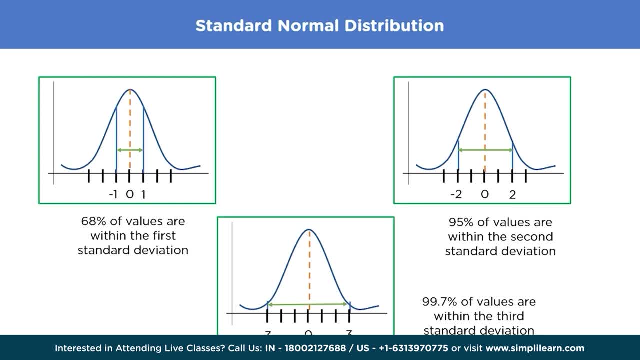 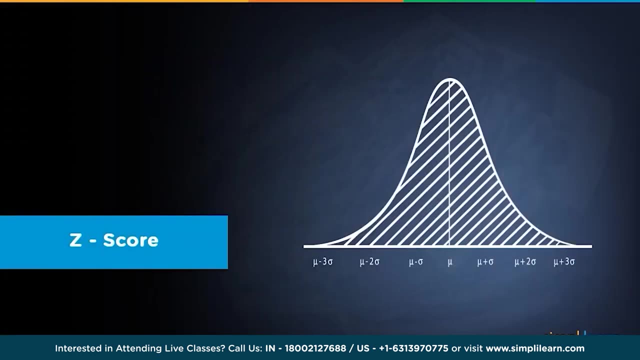 using standard normal distribution. You can find the probability of observations in a distribution which fall above or below a given value. And finally, you can find the probability that a mean significantly differs from a population mean. Now let's take a look at z-score. 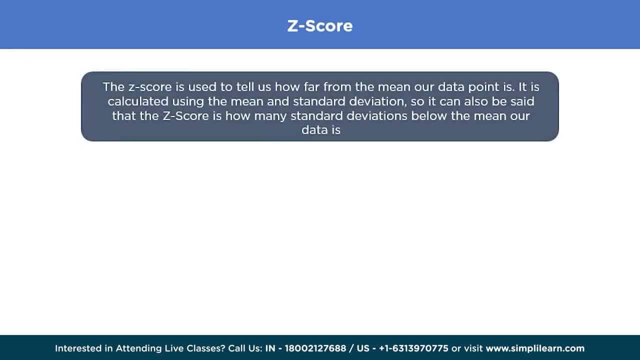 So what is a z-score? A z-score is used to tell us how far from the mean our data point actually is. It is calculated using the mean and standard deviation, so it can be said that the z-score is how many standard deviations below the mean. 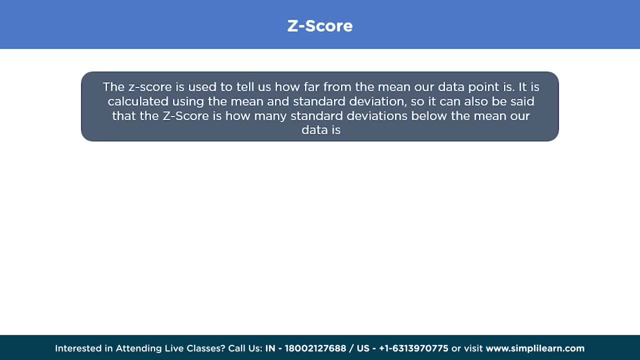 our data is. Basically, by using the z-score, we can get an approximate location of where our data point lies on the graph with regards to the mean. Now, the z-score is given by subtracting the data point from the mean and dividing it by standard deviation. 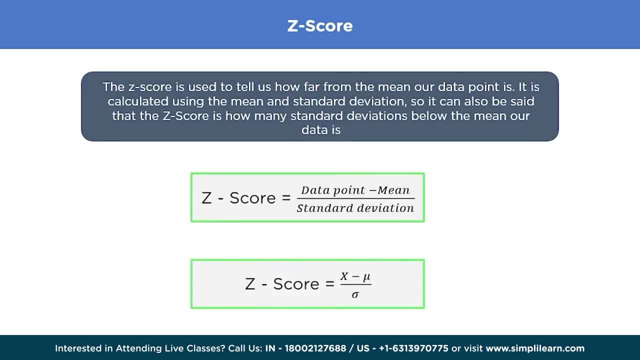 This can also be written as x minus mu divided by sigma. Now any normal distribution can be standardized by converting its values into z-scores. The z-score will tell you how many standard deviations from the mean each values lie While data points are referred. 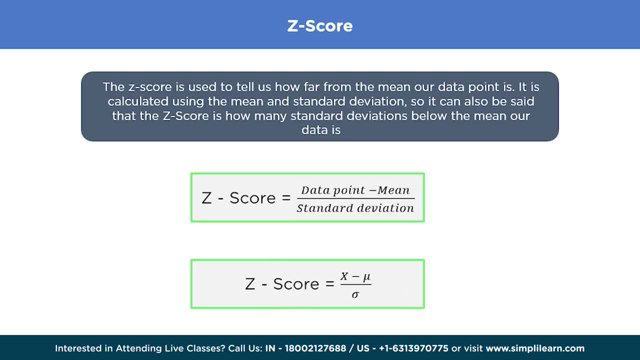 to as x. in a normal distribution they are called z or z-scores. in the z-distribution A z-score is the standard score that will tell you how many standard deviations away from the mean an individual point will lie. A positive z-score will mean that 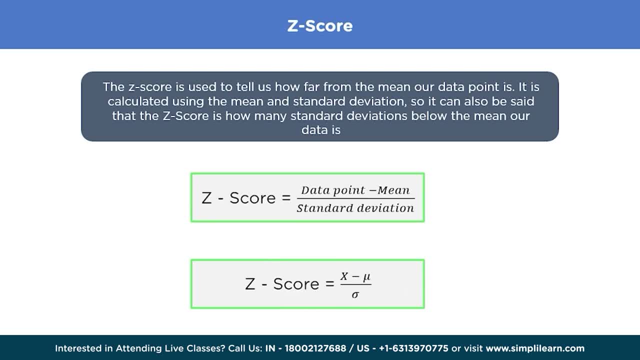 your x value is greater than the mean and a negative z-score will mean that your x value is less than the mean. A z-score of 0 will mean that your x value is equal to the mean And again, to standardize a value from a normal distribution. 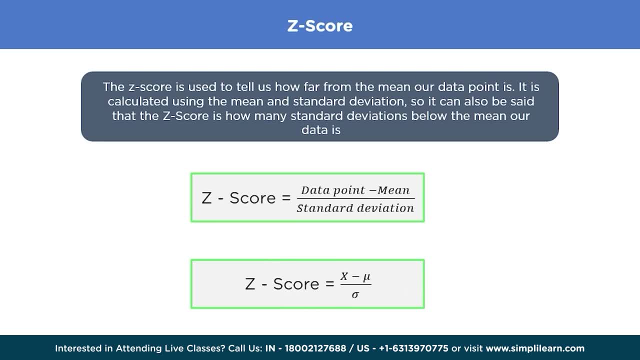 all we have to do is convert it to a z-score by subtracting the mean from our individual value and dividing it by the standard deviation. Now let's see how we can find the z-score from data points with the help of a solved example. 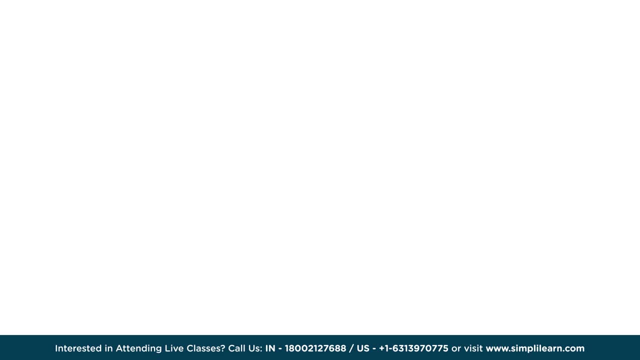 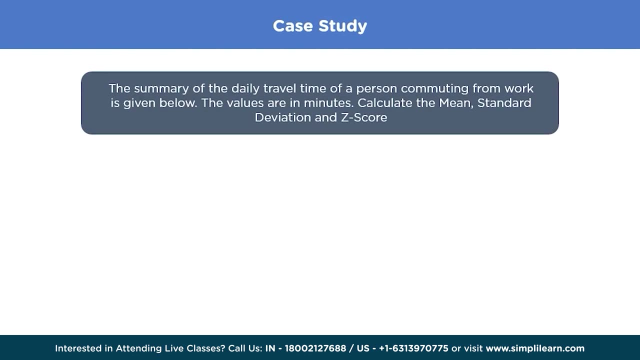 Let's do a case study. In this case study, we'll be taking the summary of daily travel time of a person who's commuting to and from work. All these values are in minutes And using these values we have to calculate the mean, the standard deviation. 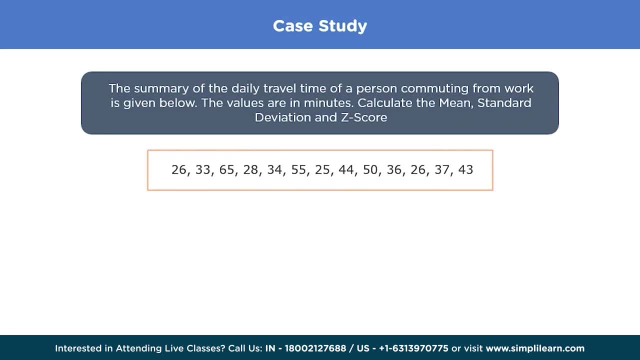 and the z-score. These values are as shown. As we can see, there are 13 values in total. Let's start by finding the mean. The mean is the average and it can be gotten by adding all of these values and dividing it by. 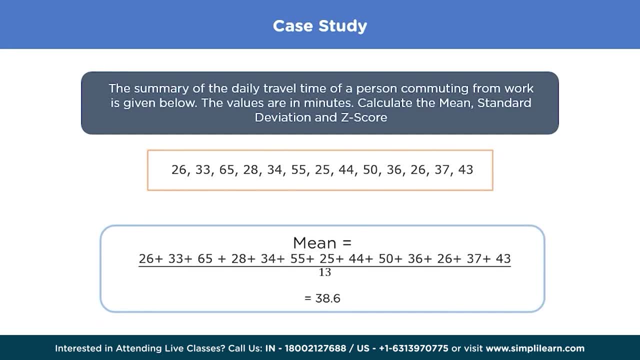 the total number of values, This gives us a value of 38.6.. The mean tells us the average of all our data points, which means, on an average, he travels for 38.6 minutes to reach work. Next let's subtract the individual. 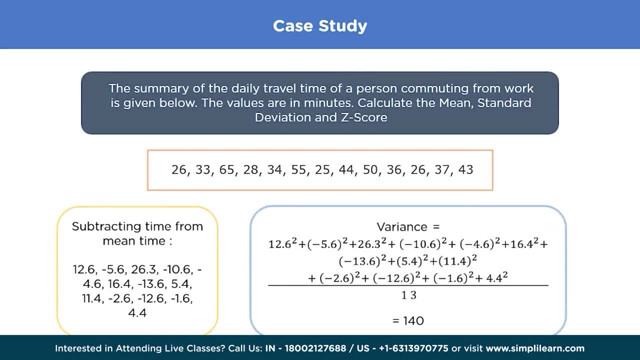 values from our mean and calculate the variance and standard deviation. The values on the left give us the values that we get after subtracting it from the mean, and the variance can be calculated by squaring all of these values, adding up all of the squared. 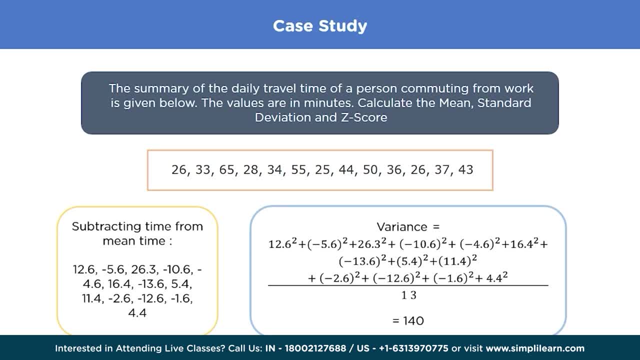 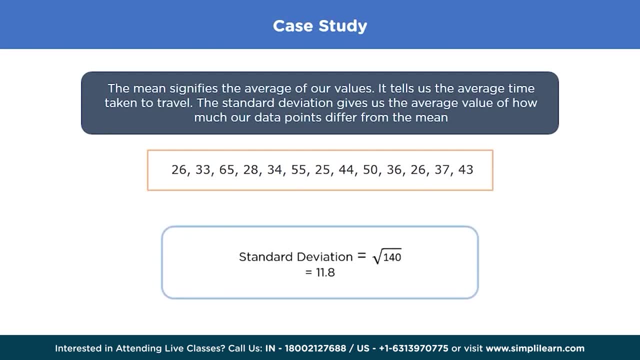 values and dividing it by the total number of values, At the end of the day we get a variance of 140.. To calculate the standard deviation, all we have to do is take a square root of the variance, which gives us a value of 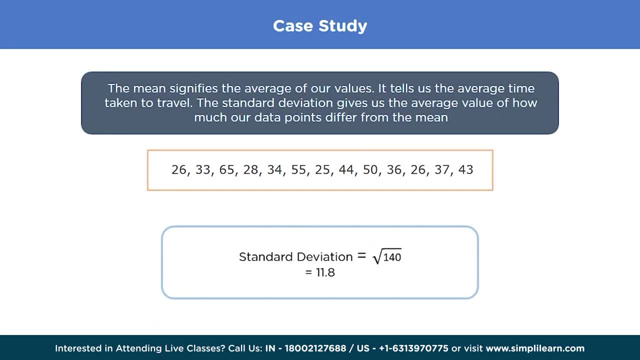 11.8.. Now the mean signifies the average of our values, and we already know this. It gives us the average time which is taken to travel, but the standard deviation will tell us the average value of how much our data points differ from the mean. 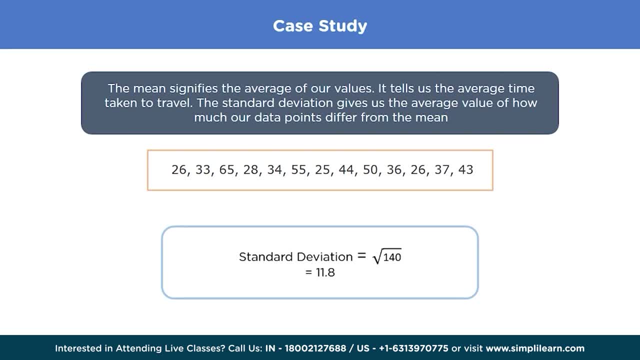 It gives us the deviation within our own data and it tells us how far away, on an average, a point is from the mean. Now the value that we get is 11.8, which means that, on an average, a single data point is around 11.8. 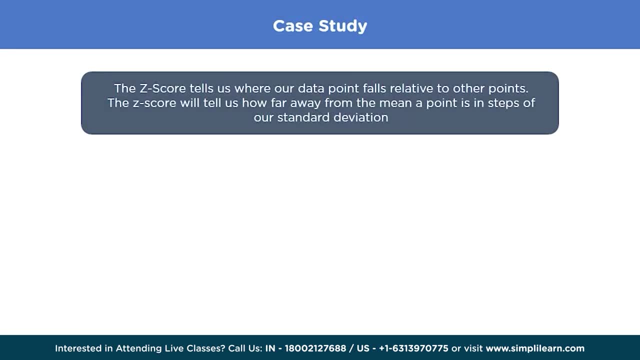 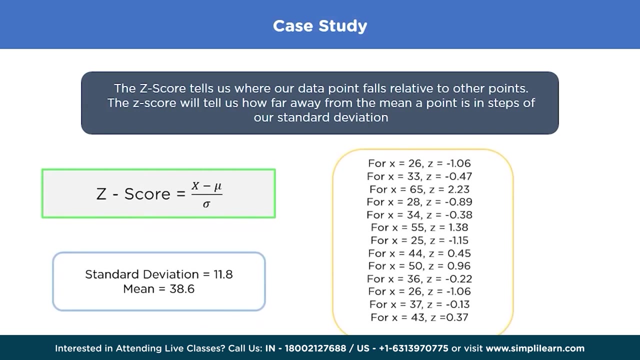 data points away from the mean. Now let's calculate the z-score. The z-score is given by subtracting individual data points from the mean and dividing it by the standard deviation. We know that we have a standard deviation of 11.8. 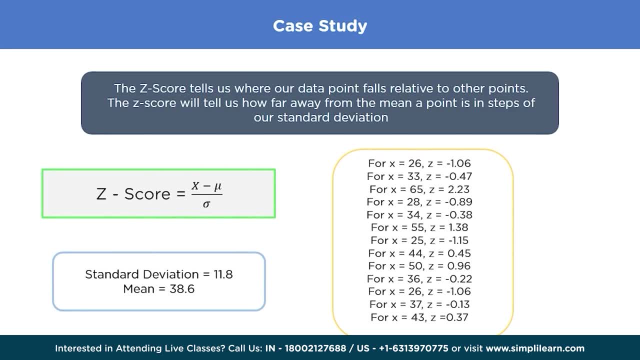 and a mean of 38.6.. Using these values, we can calculate the z-scores for individual x-values. Now we know that a negative z-score means that our x-value is lower than our mean, But what does the number 1.06? 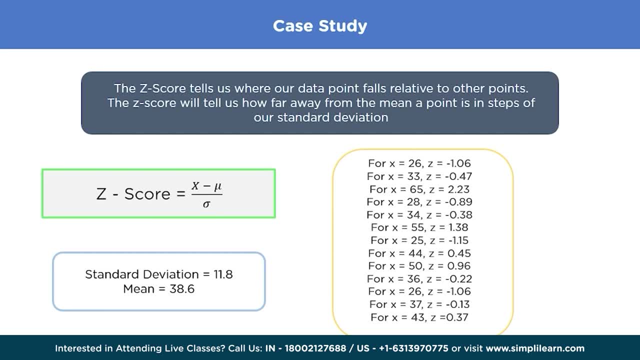 mean. This means that the z-score for 26 is 1.06 standard deviation less than the mean. The negative symbol here means that our x-value is less than the mean. And by how? less? 1.06 times the standard deviation. 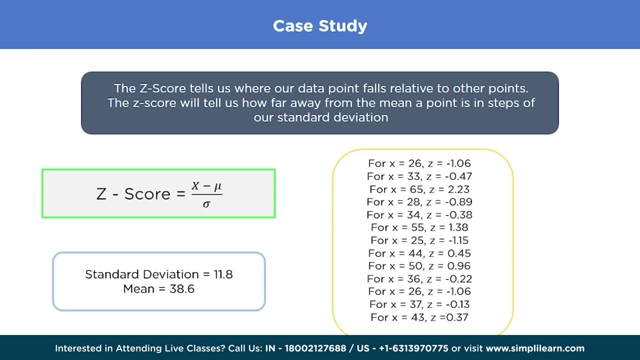 Now we know that the negative value of a z-score means that our x-value is less than our mean. But what does the number 1.06 mean? This means that the z-score is 1.06 times the standard deviation less than the mean. 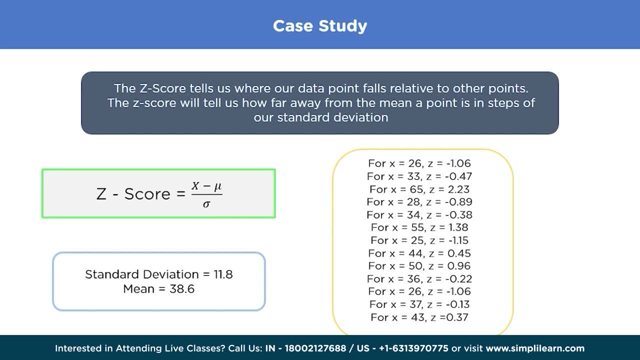 The same thing can be said for the z-score of 33.. It is 0.47 times the standard deviation, less than the mean. The z-score of 65 is 2.23 times the standard deviation, more than the mean. That means it has to be added to the mean. 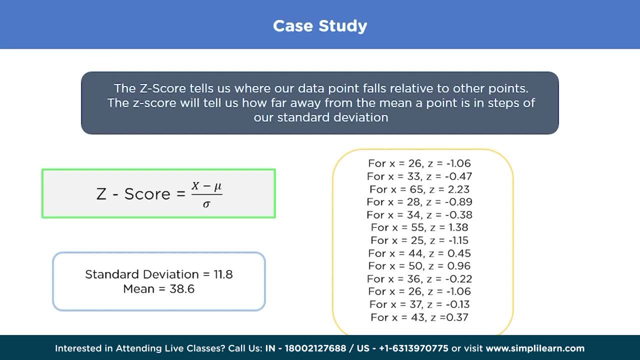 The reason that we know it's more than the mean is because this has a positive value. So this means that, using z-scores, we can know where our data points fall relative to other points on the graph. The z-score will tell us how far away from the 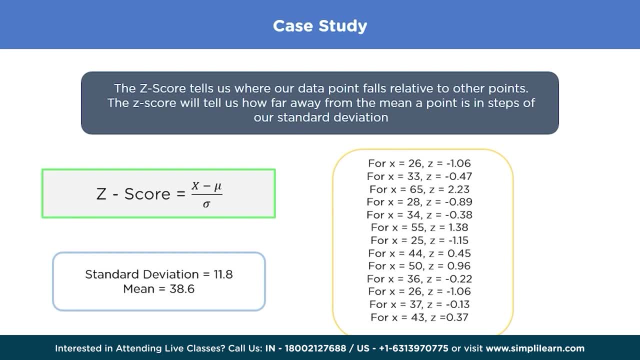 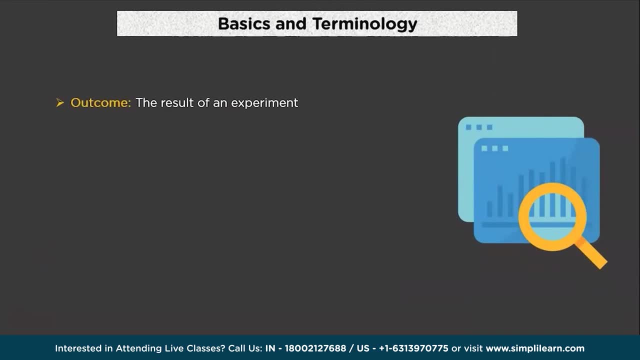 mean a point is in steps of our standard deviation Basics and terminology. The first one is outcome. Whenever we do an experiment, like flipping a coin or rolling a dice, we get an outcome. For example, if we flip a coin, we get an outcome. 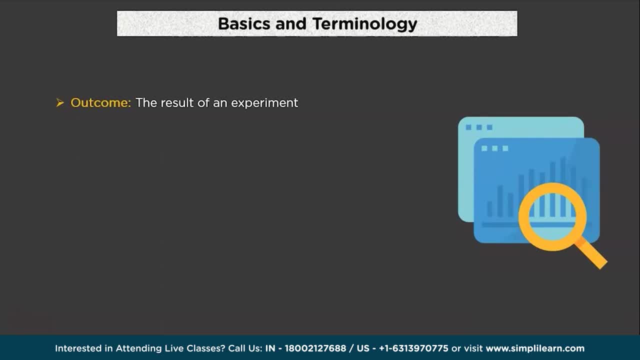 of heads or tails, And if we roll a die, we get an outcome of 1,, 2,, 3,, 4,, 5 or 6. Random experiment: A random experiment is any well defined procedure that produces an observable outcome that could not be perfectly predicted in advance. 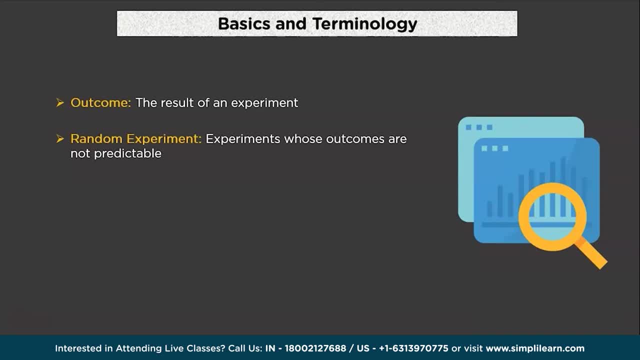 A random experiment must be well defined to eliminate any vagueness or surprise. It must produce a definite, observable outcome so that you know what happened after the random experiment is run. Random events: Consider a simple example. Let us say that we toss a coin up in the air. 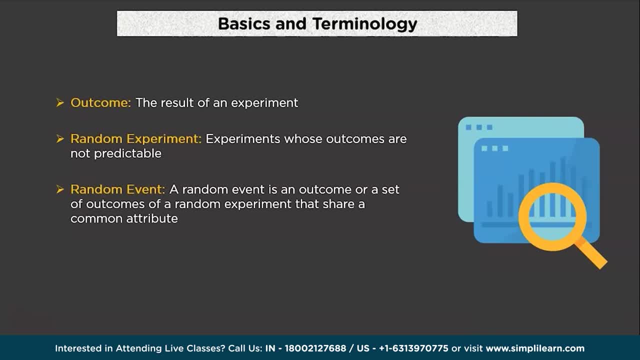 What can happen when it gets back? It either gives a head or a tail. These two are known as outcome, and the occurrence of an outcome is an event. Thus, the event is the outcome of some phenomenon. The last one is sample space. 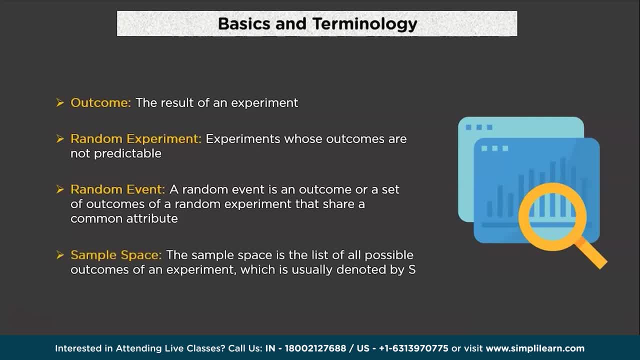 A sample space is a collection or a set of possible outcomes of a random experiment. The sample space is represented using the symbol S. The subset of all possible outcomes of an experiment is called events, and a sample space may contain a number of outcomes. that depends on the experiment. 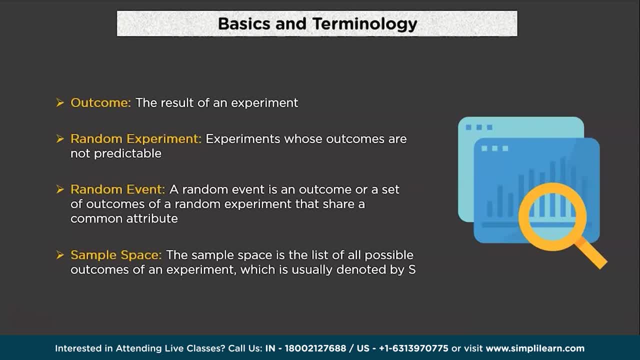 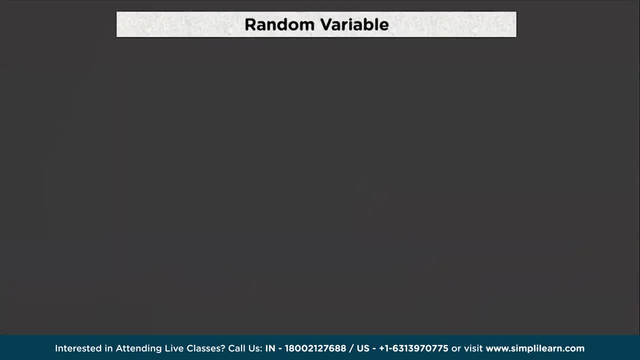 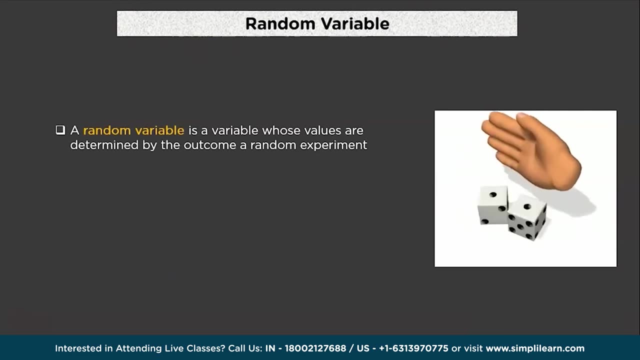 If it contains a finite number of outcomes, then it is known as a discrete or finite sample spaces. Now let's discuss what is random variable. A random variable is a numerical description of the outcome of a statistical experiment. A random variable that may assume: 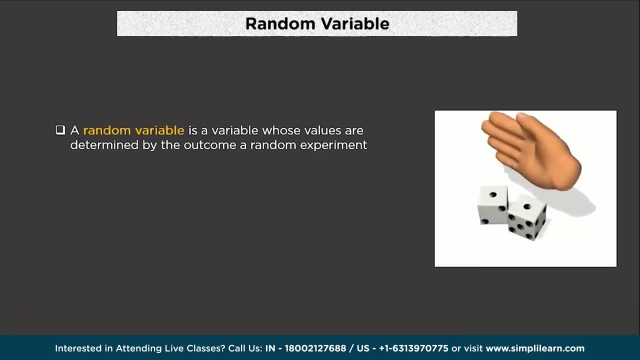 only a finite number of values is said to be discrete, One that may assume any value in some interval on the real number line is said to be continuous. Let's see an example. Let X be a random variable defined as the sum of numbers when two dices are. 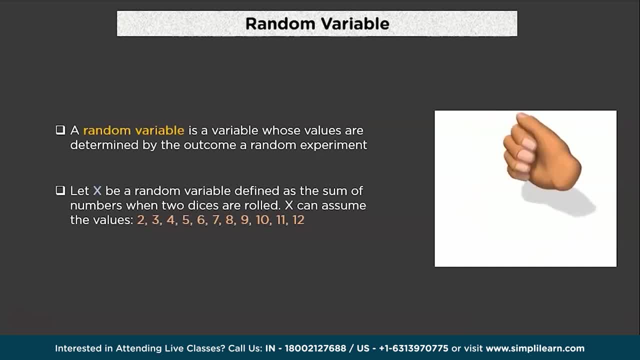 rolled X can assume the values 2,, 3,, 4,, 5,, 6,, 7,, 8,, 9,, 10,, 11, and 12.. Notice: there is no 1 here, because the sum 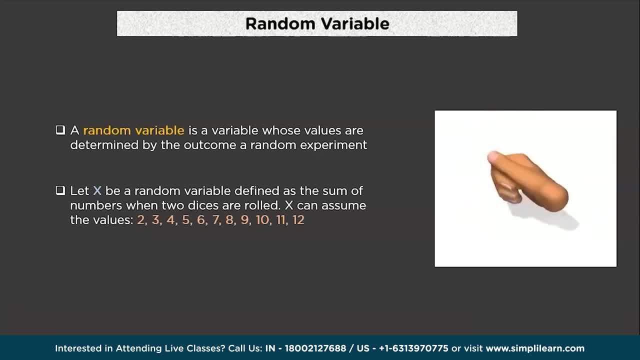 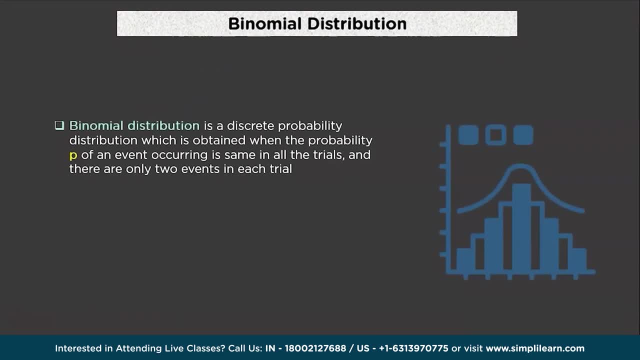 on the two dice can never be 1.. Now that we know the basics, let's move on to binomial distribution. The binomial distribution is used when there are exactly two mutually exclusive outcomes of a trial. These outcomes are appropriately labeled: success and failure. 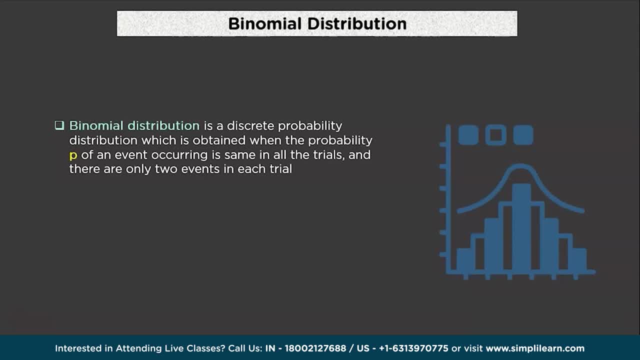 The binomial distribution is used to obtain the probability of observing X successes in n number of trials, with the probability of success on a single trial denoted by P. The binomial distribution assumes that P is fixed for all the trials. Here is a real-life example. 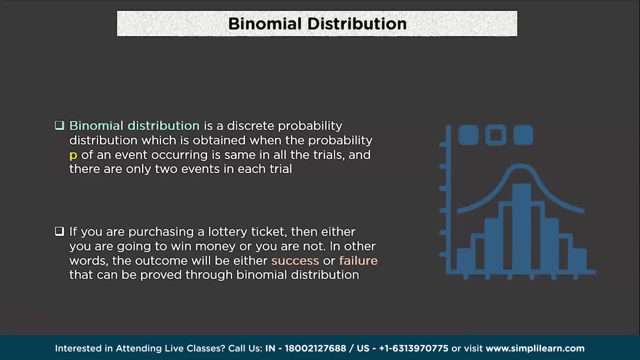 of a binomial distribution. Suppose you purchase a lottery ticket, Then either you are going to win the lottery or not. In other words, the outcome will be either success or failure. that can be proved through binomial distribution. There are four important conditions that needs to be fulfilled. 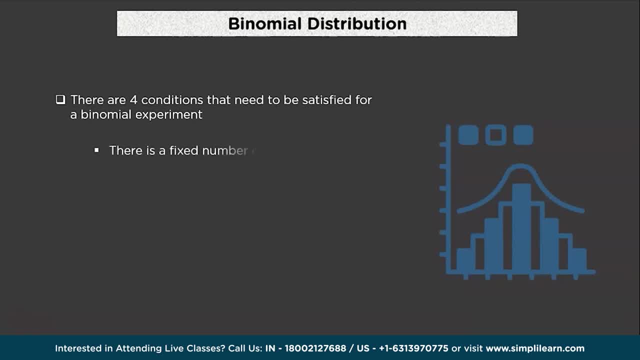 for an experiment to be a binomial experiment, The first one is there should be a fixed number of n trials carried out. The outcome of a given trial is only two. that is, either a success or a failure. The probability of success remains constant from. 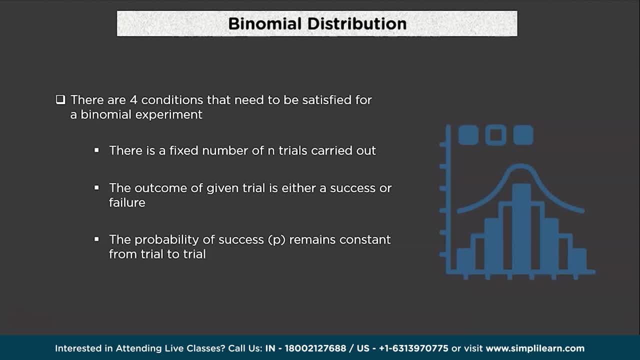 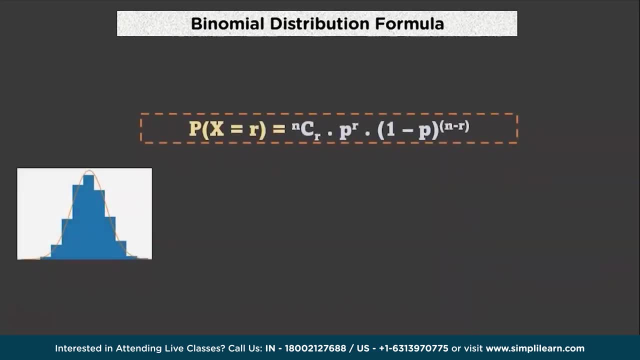 trial to trial. It does not change from one trial to another And the trials are independent. The outcome of a trial is not affected by the outcome of any other trial. To calculate the binomial coefficient, we use the formula, which is nCr into P to the power. 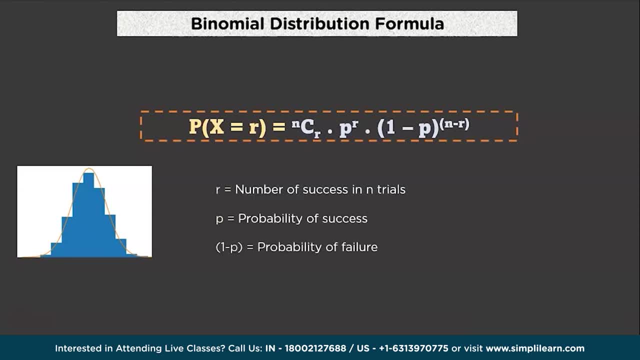 R into 1-P to the power n-R, where R is the number of success in n number of trials and P is the probability of success. 1-P denotes the probability of a failure. Now let's use this formula to solve an example. 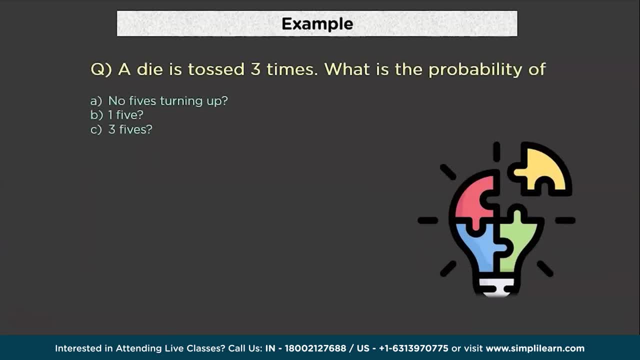 Suppose a die is tossed three times, What is the probability of no-five turning up, one-five and three-fives turning up? To calculate the no-five turning up here, R is equal to zero and n is equal to three, Substituting. 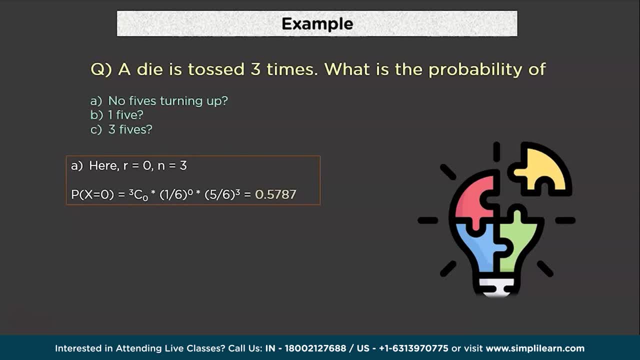 the value. in the formula we have 3-3-0 into 1-6 to the power 0, into 5-6 to the power 3, where 1-6 is the probability of success and 5-6 is the probability of failure. 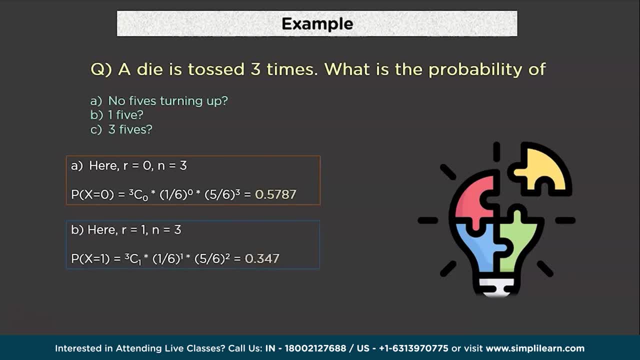 Calculating this equation, we will get the value to be 0.5787.. In a similar manner, to calculate the probability of one-five turning up, we will replace R with 1 and n will be 3.. So P will be equal to. 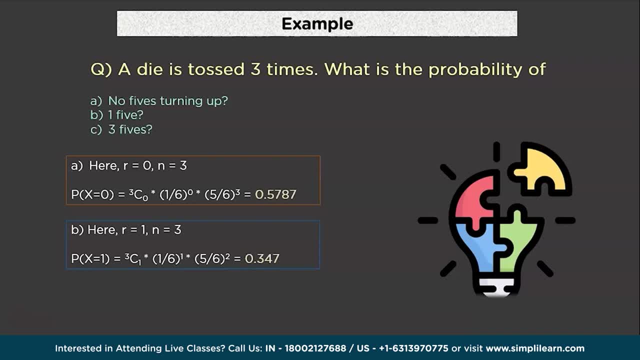 3C1 into 1-6, to the power 1, into 5-6, to the power 2, which will come out to be 0.347.. And for three-five turning up, we substitute R equal to 3 and the formula will remain the same. 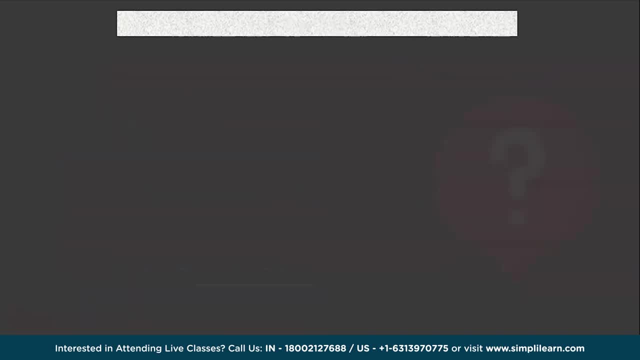 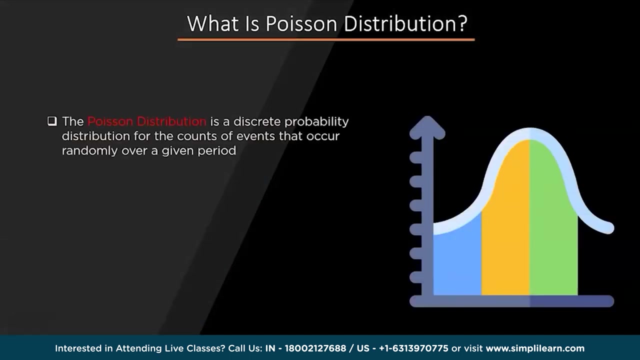 and we will get the value to be 0.0046.. Now that we are done with the concepts of animal probability distribution, here is a problem for you to solve. Post your answers in the comment section and let us know A Poisson. 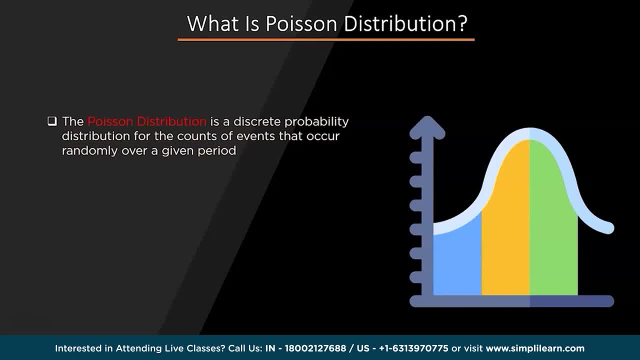 distribution is a probability distribution used in statistics to show how many times an event is likely to happen over a given period of time. To put it another way, it's a count distribution. Poisson distributions are frequently used to comprehend independent events at a constant rate over a given. 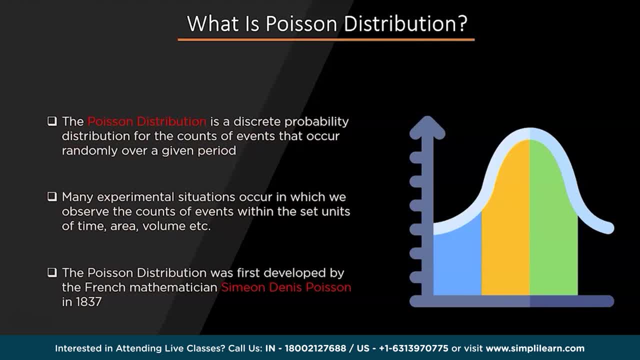 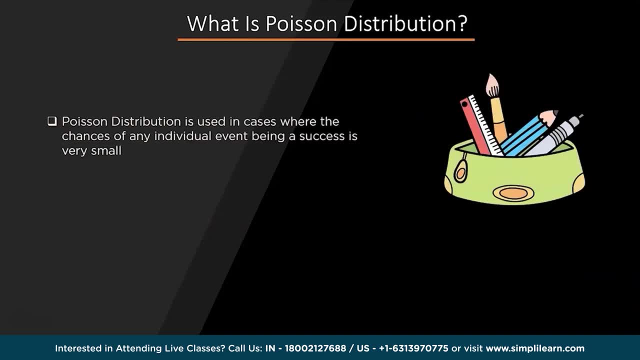 interval of time. The Poisson distribution was developed by French mathematician Simon-Denis Poisson in 1837.. A Poisson distribution is used in cases where the chances of any individual event being a success is very small. The number of defective pencils. 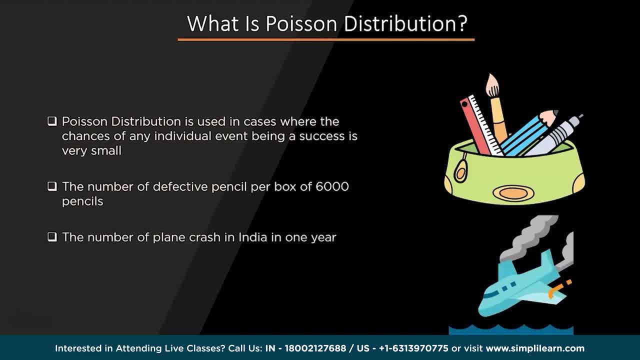 per box of a 6000 pencil, the number of plane crashes in India in one year or the number of printing mistakes in each page of a book. All of these examples can have use of Poisson distribution. The Poisson distribution can be used to calculate. 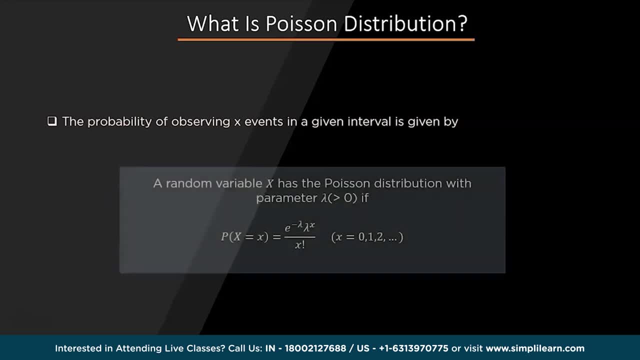 how likely it is that something will happen. x number of times. A random variable, x has a Poisson distribution with parameter lambda and the formula for that is: e to the power minus lambda into lambda to the power x divided by x factorial, Where x can be the number of times. 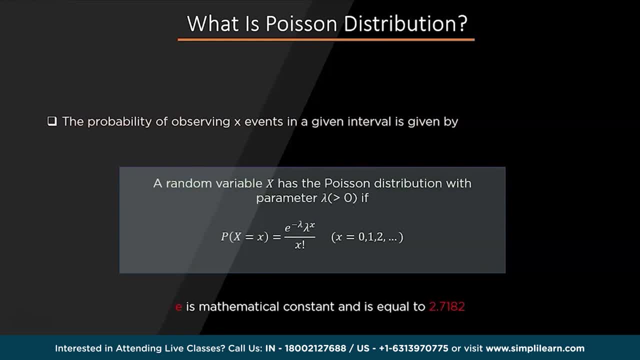 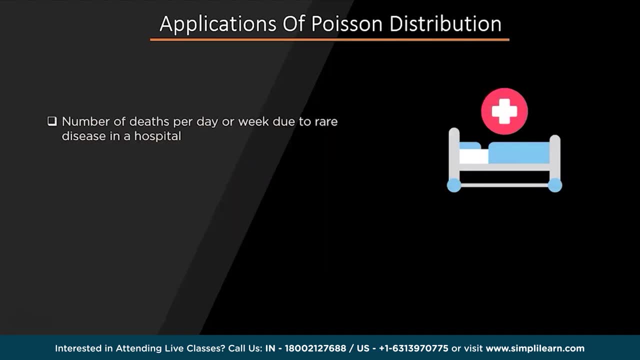 the event is happening. The value of e is taken as 2.7182.. Let's discuss some application of Poisson distribution. If you want to calculate the number of deaths per day or week due to rare disease in a hospital, you can use the Poisson distribution. 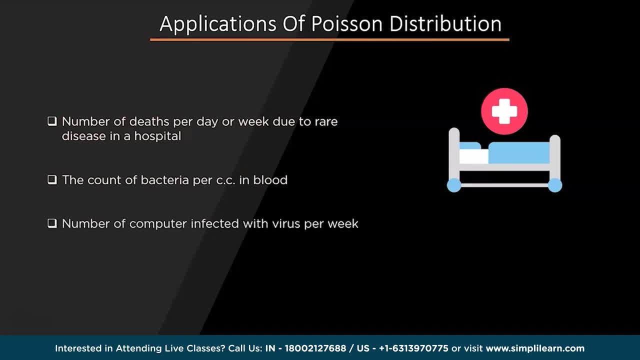 In a similar manner, the count of bacteria per cc in blood or the number of computers infected with virus per week, The number of mishandled baggage per 1000 passengers can also have an application for Poisson distribution. Let's discuss one example. 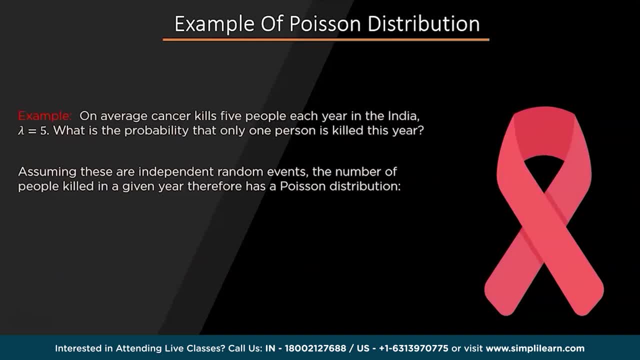 to see how we can calculate the Poisson distribution. Suppose, on an average, a cancer kills 5 people each year in India. What is the probability that one person is killed this year? We'll assume all these events are independent, random events. 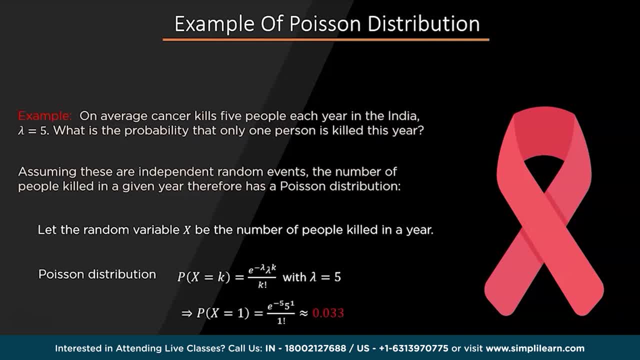 So by the formula we have, x is equal to 1 because we have to calculate the probability of one person that is killed this year. So p will be equal to e, to the power minus 5 into 5, to the power 1 divided by 1 factorial. 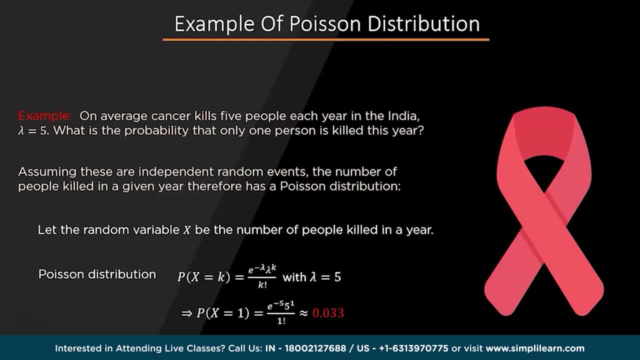 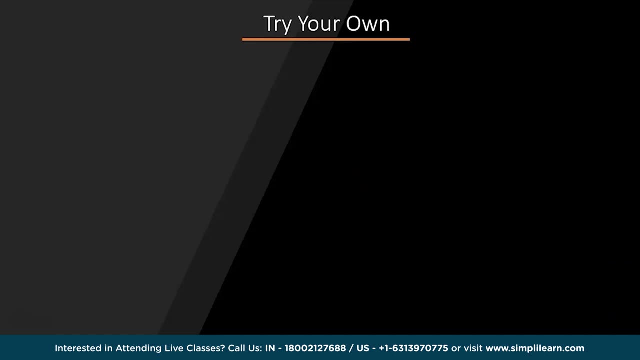 which will come out to be 0.033, which will be near to 3.3%. So the probability that only one person is killed this year due to cancer is 3.3%. Now we have one question for you. Do try to answer in the comment section. 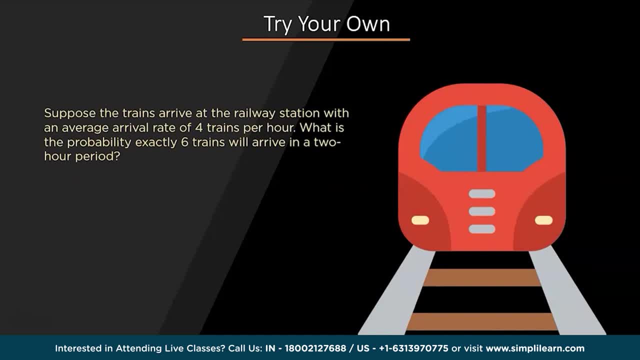 Suppose the trains arrive at a railway station with an average arrival rate of 4 trains per hour, What is the probability exactly 6 trains will arrive in a 2 hour period. And here are your options. Please do let us know your answers in the comment section. 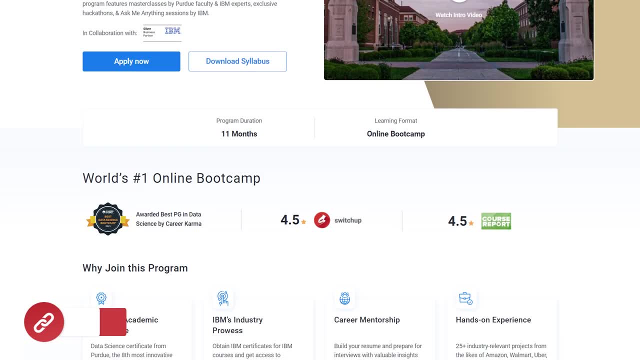 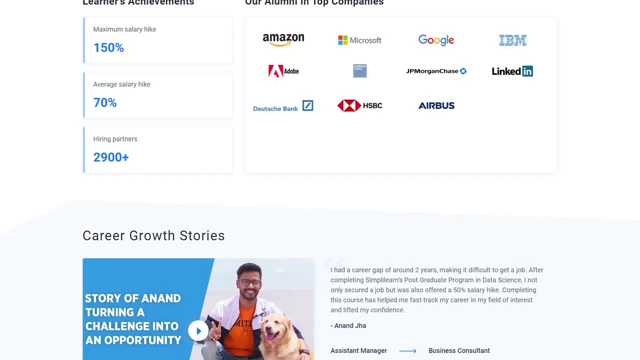 Also data scientists looking for online training and certification programs from the best universities, or a professional who elicits to switch careers with data science? then try giving Simply Learn's post graduate program in data science a shot. The link in the description box below should navigate you to the home page. 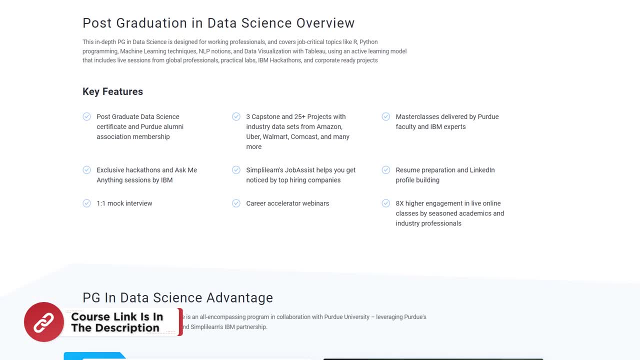 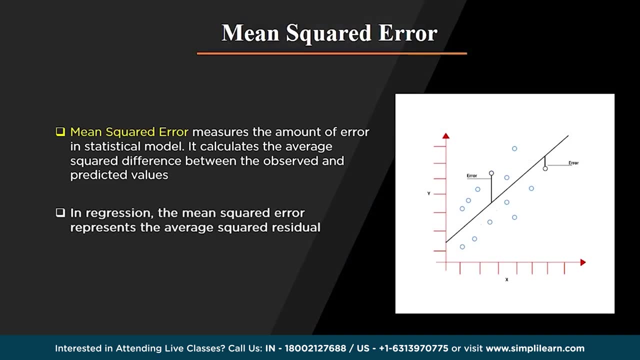 where you can find the complete overview of the program being offered. Now over to our training experts. Let's start by defining what is mean squared error. Mean squared error measures the amount of error in a statistical model. It calculates the average squared difference between the observed and predicted. 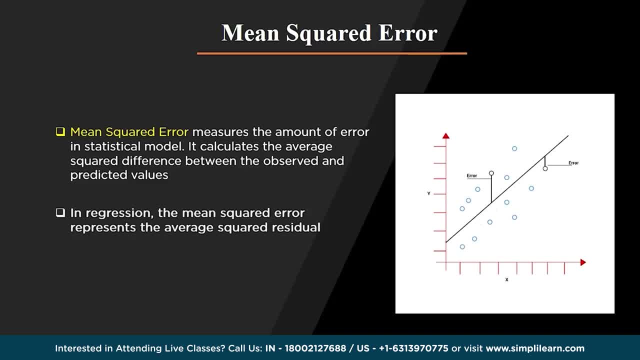 values In regression line. the mean squared error represents the average squared residual. As you can see in the graph, as the data points fall closer to the regression line, the model has less error, decreasing the mean squared error. A model with less error produces more precise. 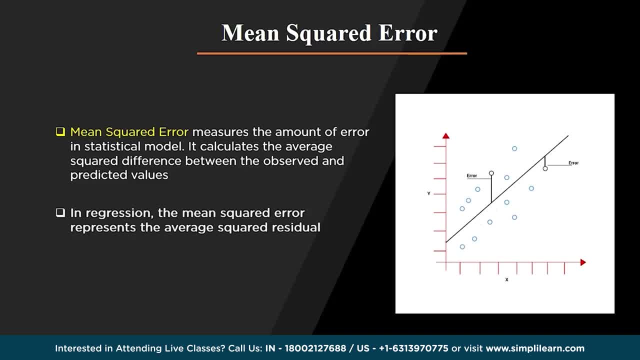 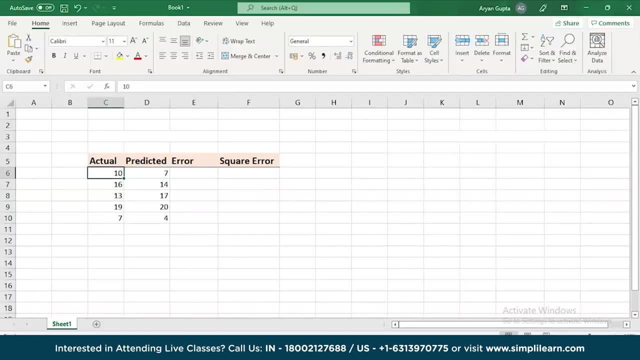 predictions. Now let's jump to our excel workbook and discuss it with an example. Here we have a small table with the actual and predicted values. We'll start by finding the error between the actual and predicted value, which will be the difference between the actual minus predicted values. 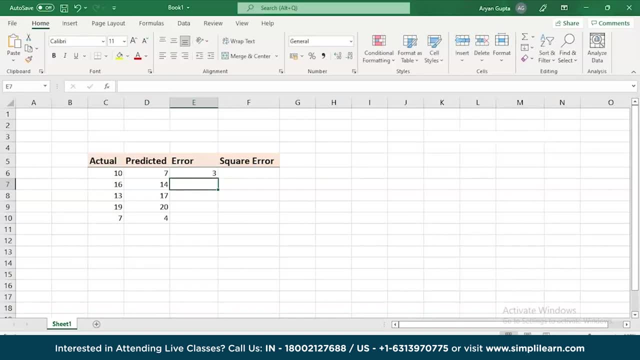 So here 10 minus 7 will become 3,, 16 minus 14 will become 2,, 13 minus 17 will become minus 4.. 19 minus 20 becomes minus 1, and 7 minus 4 becomes 3.. Now 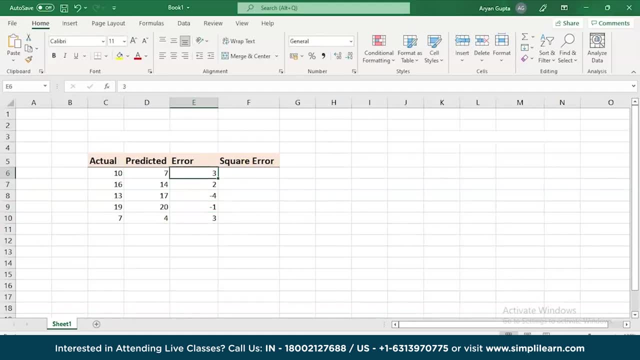 just calculate the total of the errors. While calculating the total, we'll treat this negative value as a positive value. So here the total of the errors will become 3 plus 2,, 5 plus 4,, 9,, 10 and 13.. 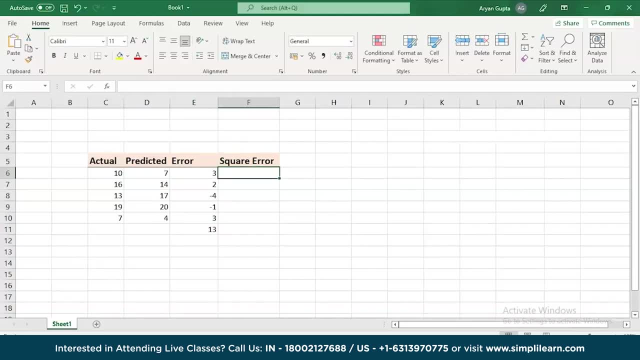 Then we'll calculate the square of the errors. So here, 3 square will become 9,, 2 square will become 4,, 4 square will become 16,, 1 square will become 1 and 3 square again is 9.. 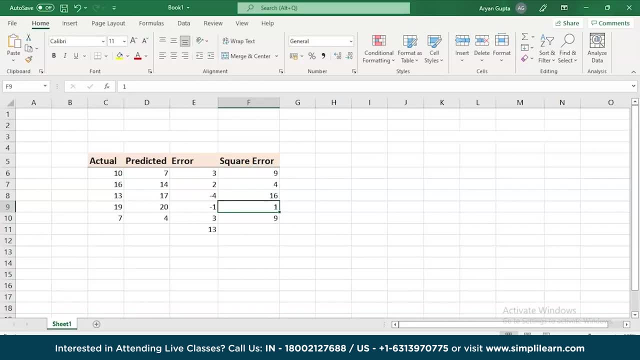 And we'll do the total of the square errors. So this will become 9 plus 4,, 13,, 13 plus 1,, 14,, 14 plus 16,, 30 and 39.. To find the MAC. 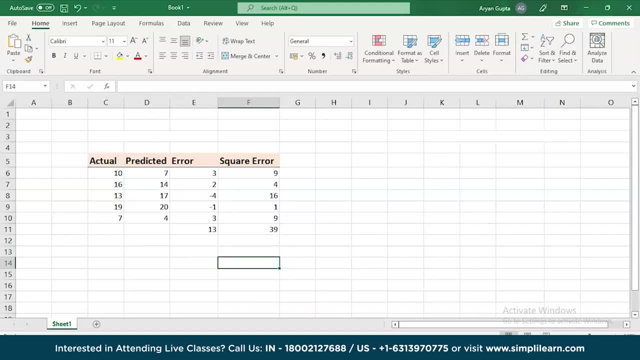 that is the mean squared error. we'll divide the total of the square error values with the total number of records. So here MAC will be equal to 39 divided by, and we have the total number of records, that is 5, which will be 7.8.. 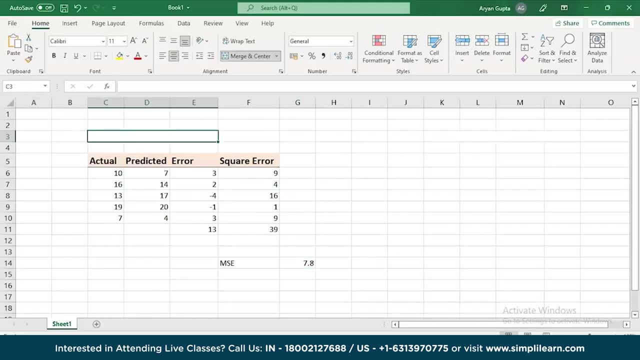 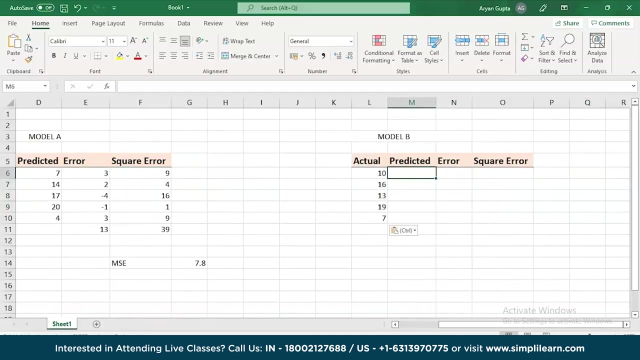 Let's name this as model A. Now, for the comparison purpose, we'll create another model, that is model B. We'll have all the columns here And we'll keep the actual values here same. We'll just change the predicted values. 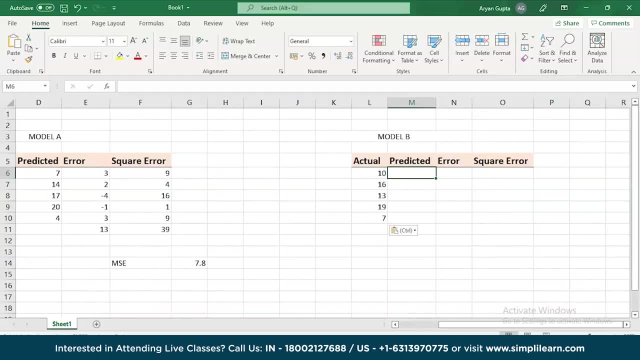 So let's take some random values. We'll keep this as 13,. we'll take this as 20,. we'll take this as 12,, 13 and 3.. Now, to calculate the error, we'll subtract the predicted values from the actual values. 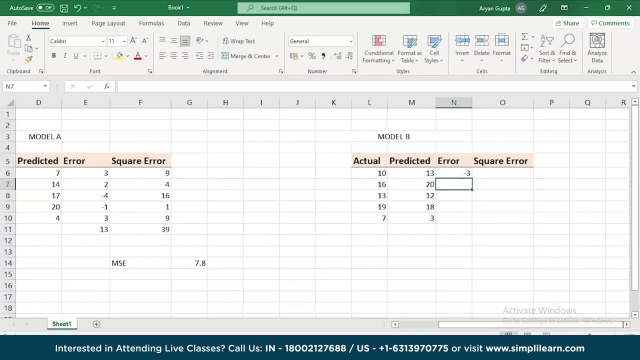 So 10 minus 13 will become minus 3,, 16 minus 20 will become minus 4,, this will become 1,, this will be 1, and this will be 4.. Now to calculate the square error. 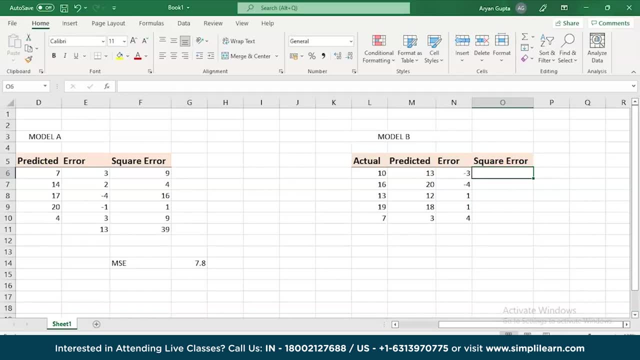 we'll just square the error values. So this will be 9,, this will be 16,, this will be 1,, this will be 1, and this will be 16.. The total of all the square values will come out to be 43.. 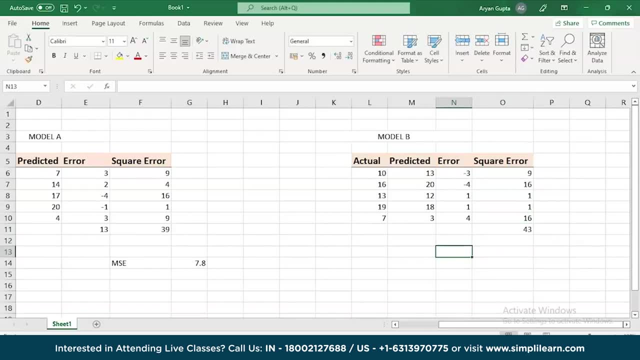 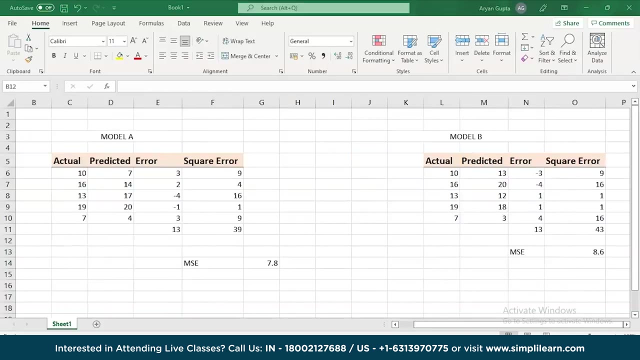 Now to calculate the MSE again, we'll divide the total square values with the total number of records. So here this will be equal to 43 divided by 5, which will come out to be 6.. If you observe here: 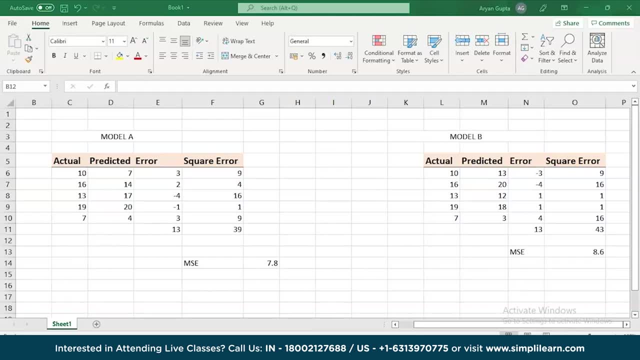 the total of the errors in both Model A and Model B is same, that is, 13.. So which model to prefer? Since the MSE of Model A is lesser than Model B, we'll prefer Model A Because we are okay with a model. 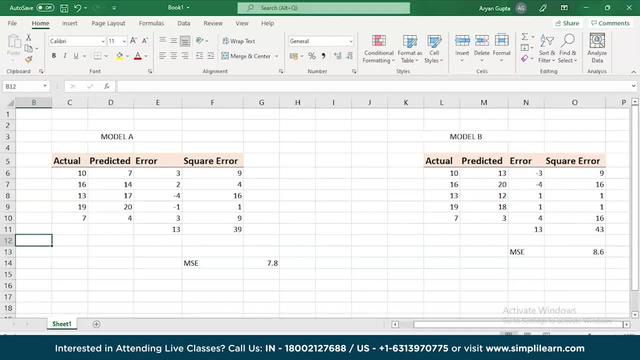 that has small, small errors. But in Model B there are some significantly large errors. Suppose in this case 16 minus 20 minus 4 minus 3 and this here 4.. So we do not want a model where 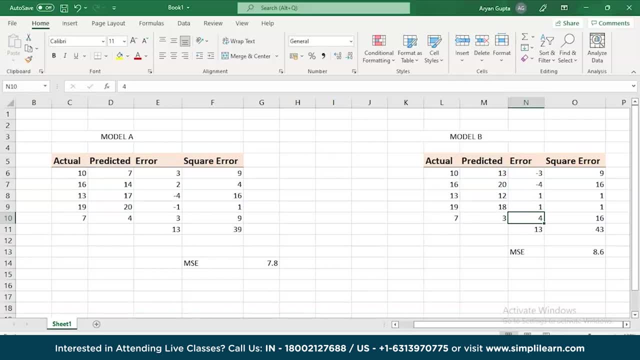 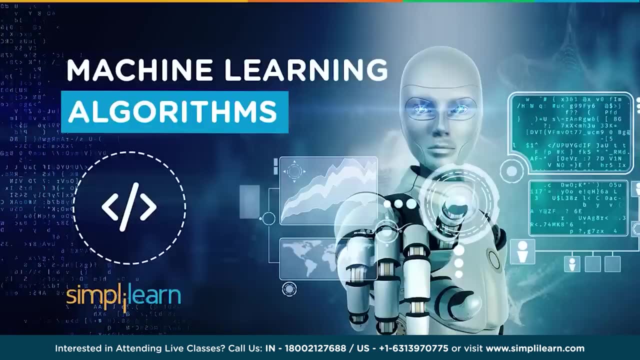 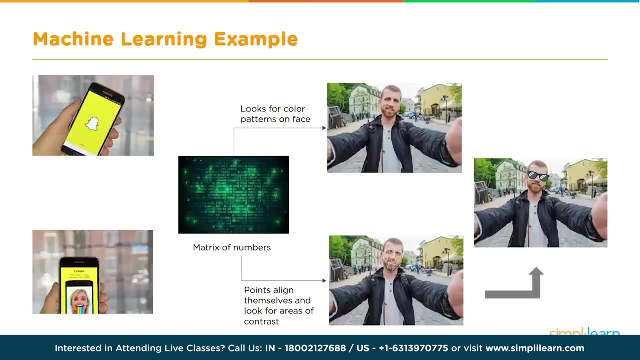 the errors- large errors specifically- are more frequent. We can have a model with the small errors. that will be okay, So we'll prefer Model A over Model B. Most of you must be using Snapchat to apply filters on your photos, But do you know how Snapchat? 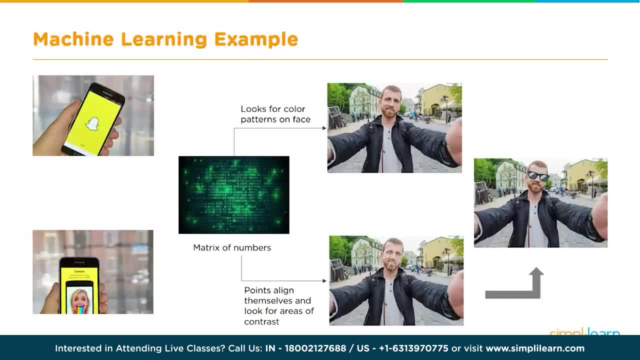 recognizes your photo on the screen and puts filters on it. Even if there are multiple faces on the photo, it applies filters in appropriate position. Snapchat actually does this using a technique called facial recognition, which in turn uses machine learning, The machine learning algorithm. 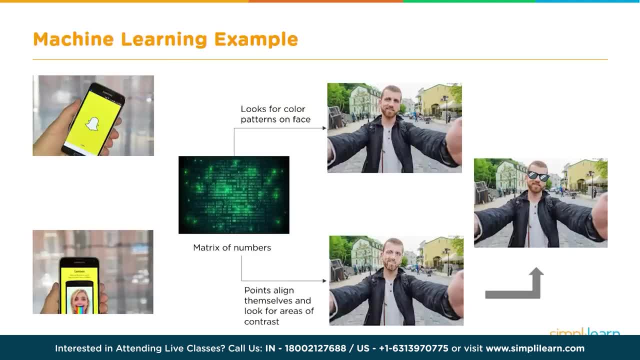 detects the features on your face, like the nose, the eyes, and it knows where exactly your eyes are, where exactly your nose is, and accordingly it applies the filters. We will take a few more examples as we move along and try to understand how machine learning algorithms can be. 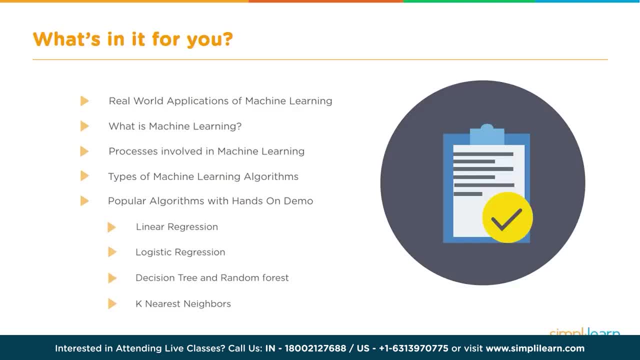 applied to solve some of our real-life problems. So what will you learn from this video? We will talk about some real-world applications of machine learning. We will also see and understand what exactly is machine learning and how it works. We will also see the process involved. 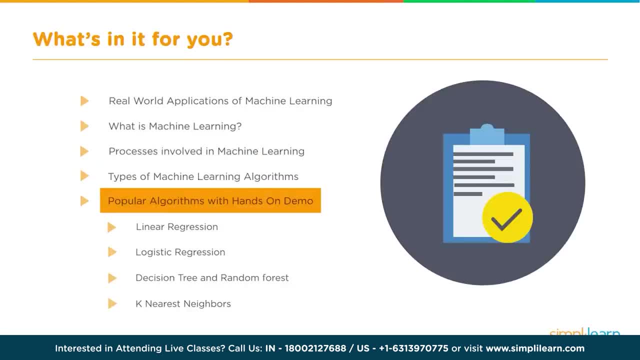 in machine learning, the types of machine learning algorithms, and we will also see a few hands-on, including some code, Python code of the following algorithms: linear regression, logistic regression, decision tree and random forest and k-nearest neighbors. Okay, so let's get started. 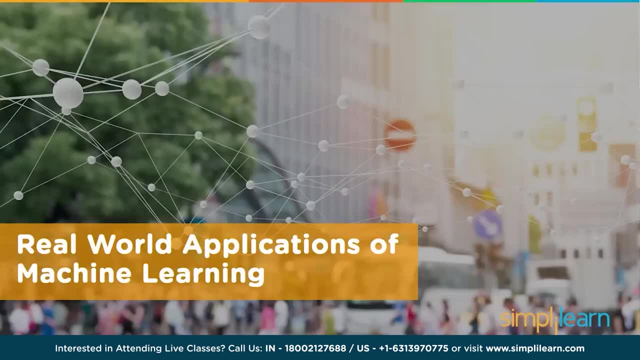 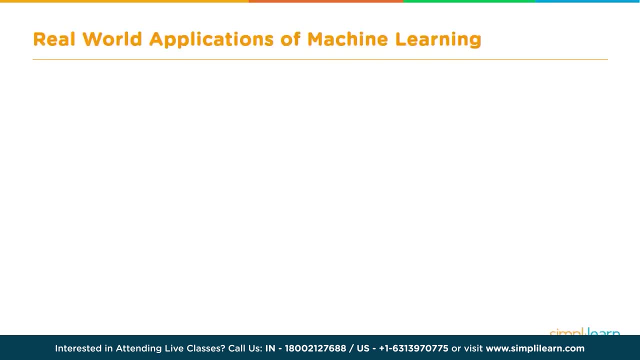 Let's consider some of the real-world applications of machine learning. It's no longer just a buzzword. Machine learning is being used in a variety of industries to solve a variety of problems. Facial recognition is one of them. It's becoming very popular these days. 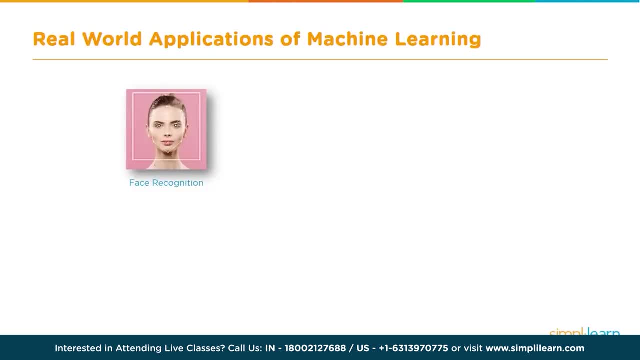 for security, for police, for solving crime- a lot of areas. Facial recognition is being used. Voice recognition is another area. It's becoming very common these days. Some of you must be using Siri. That's an example of machine learning and voice recognition. 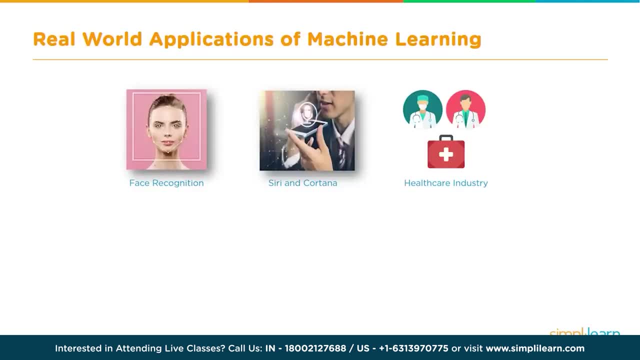 Healthcare industry is another big area where machine learning is adopted in a very big way. As you all may be aware, diagnostics needs analysis of images, let's say like x-ray or MRI, and increasingly, because of the shortage of doctors, machine learning and artificial intelligence is being used to help. 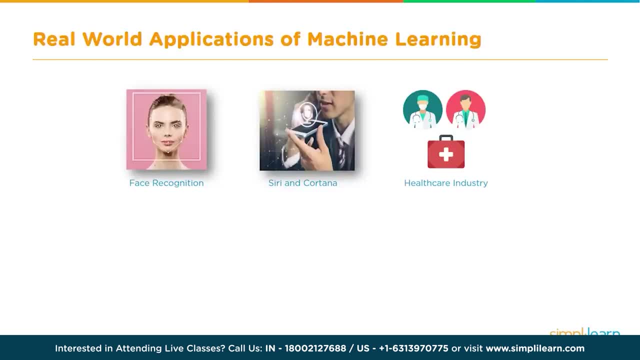 and support doctors in analyzing these images and identifying the advent of any diseases. Weather forecast is another area and in fact Netflix has actually come up with a very interesting use case. You all must be aware of the House of Cards show on Netflix, So they did an analysis. 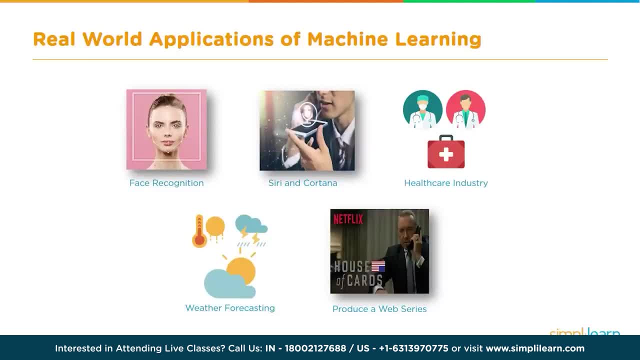 on their customer behavior. They got data of their 30 million customers- Information about where they pause, where they fast forward a video- and they used this information. They provided this information to their playwrights and told them that this is what we want. 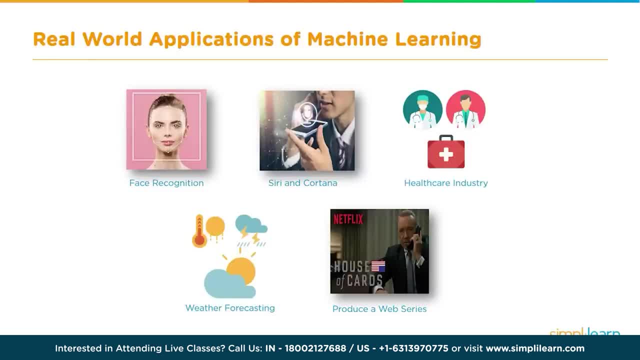 This is what our audience is looking for, These are the areas that interest them and these are the areas where they get bored, And the playwrights wrote the scripts accordingly. This is really, really interesting and it actually brings a new era. So what is machine learning? 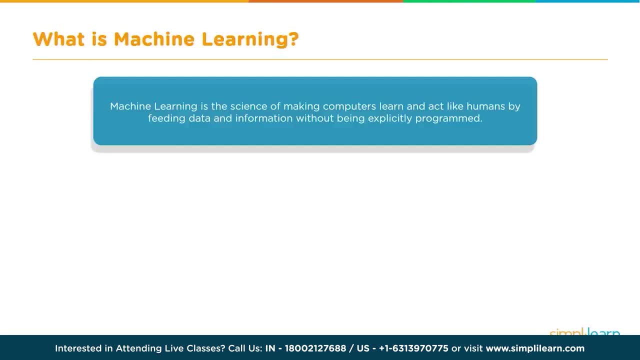 Machine learning is a science of making computers learn and act like humans. So here, when we say computers, very often what comes to our mind is writing a piece of code or program and telling the computer step by step what to do. But in machine learning we don't do that. The system, 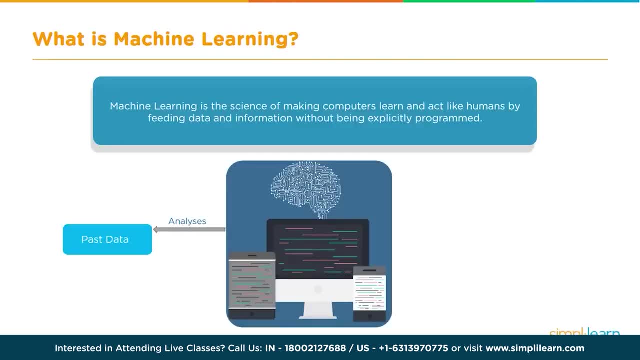 learns on its own. We just provide past data, historical data, what we call as labeled data, And the system learns during the process, what is known as training process. We tell the system whether the outcomes are right or wrong, and that feedback is taken by the system and it. 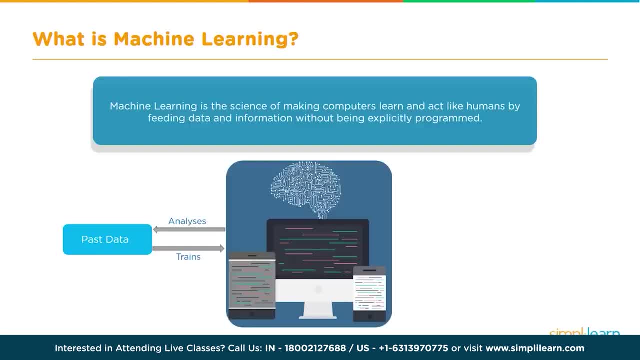 corrects itself, and that's how it learns till it gives the correct output for most of the cases. Obviously, it won't be 100% correct, but the aim is to get as accurate as possible. So let's take you through, step by step, process of machine learning. 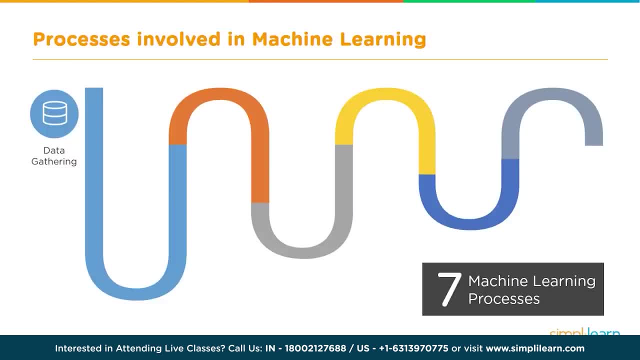 The first step in machine learning is data gathering. Machine learning needs a lot of past data, especially- we will see a little later- supervised learning. We will see what that is in a little while, But that's the most common form of learning. So the 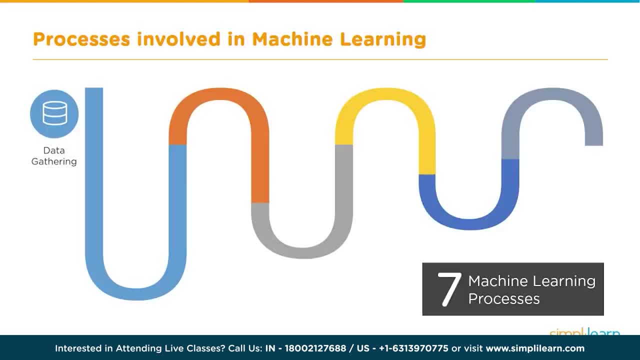 first step there is data gathering. You need to have sufficient historical data. Then the second step is pre-processing of this data so that this can be used for the machine learning process. The raw data cannot be used directly, so it needs to be pre-processed. 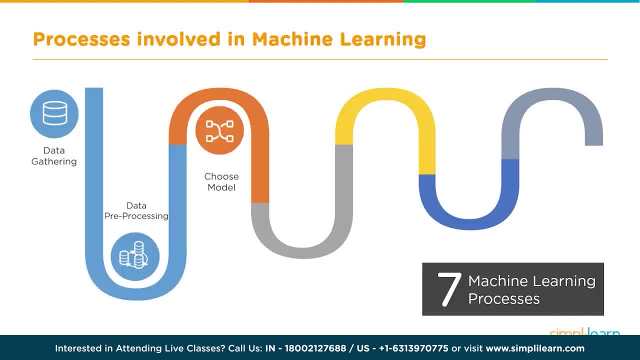 before it is fed into the machine learning system. The next step is to choose a model. So what kind of algorithm and what kind of model within that algorithm are we going to use? And then we need to train this model. So before training the model, it's just 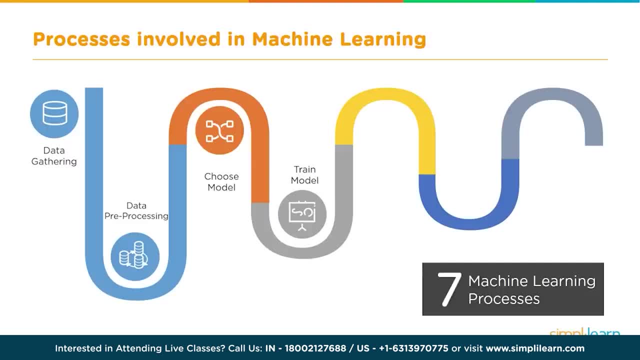 like a blank model and after training it becomes a trained model. And once we train the model, we need to also test it to make sure it is predicting correctly. It's working fine, with minimum errors, And subsequently it will be deployed and once again it may have to be. 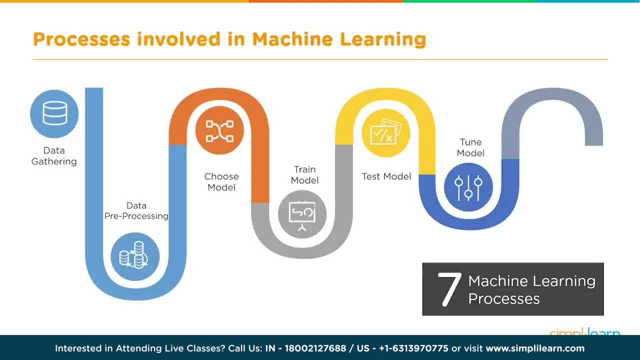 tuned from time to time, or fine tuned from time to time to improve the accuracy, and so on and so forth. After training the model, we have to test the model, And during testing we may have to- we may find out that the accuracy is not good enough. 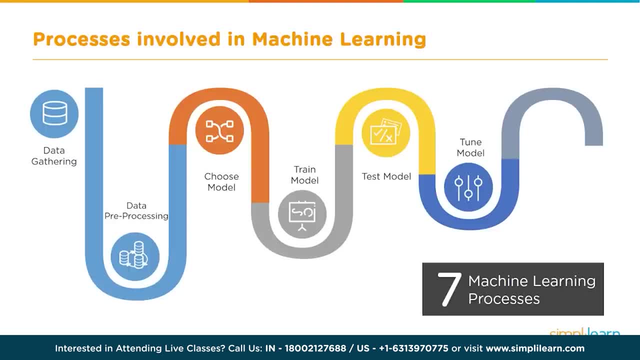 so we may have to tune the model, We may change some parameters and run through this process once again, Perform the training once again, So it can be an iterative process, And once the model is ready, then we deploy it to do the predictions. What are the? 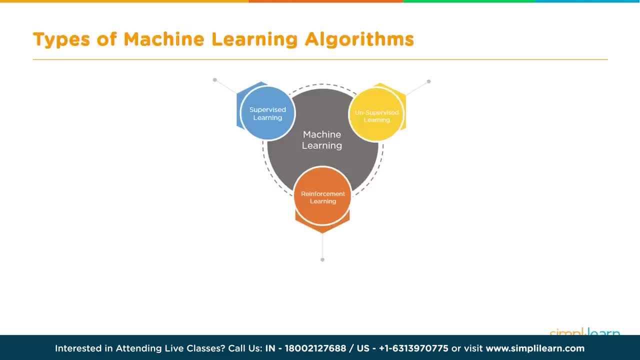 different types of machine learning algorithms. Machine learning algorithms are broadly classified into three types: The supervised learning, unsupervised learning and reinforcement learning. Supervised learning, in turn, consists of techniques like regression and classification, and unsupervised learning, we use techniques like association and clustering. 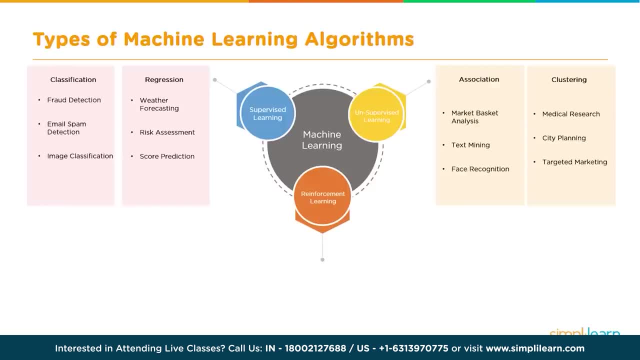 And reinforcement learning is a recently developed technique and it is very popular in gaming. Some of you must have heard about AlphaGo, So this was developed using reinforcement learning. Primary difference between supervised learning and unsupervised learning: Supervised learning is used when we have historical data. 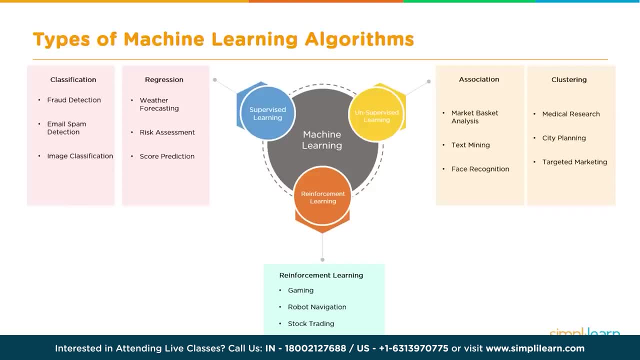 and we have labeled data, which means that we know how the data is classified. so we know the classes if we are doing classification, or we know the values when we are doing regression. So if we have historical data with these values, which are known as labels, then we use. 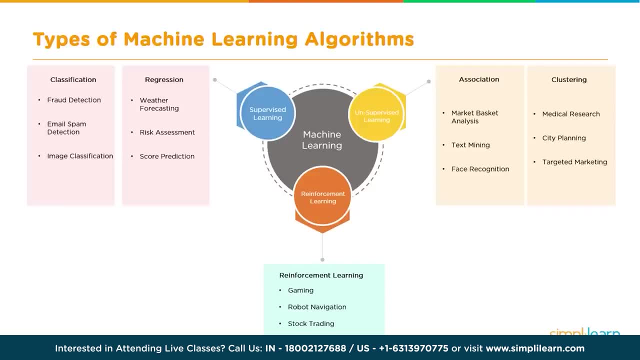 supervised learning. In case of unsupervised learning, we do not have past labeled data, Historical labeled data, So we use techniques like association and clustering to maybe form clusters or new classes maybe, and then we move from there. In case of reinforcement learning, the system learns pretty much. 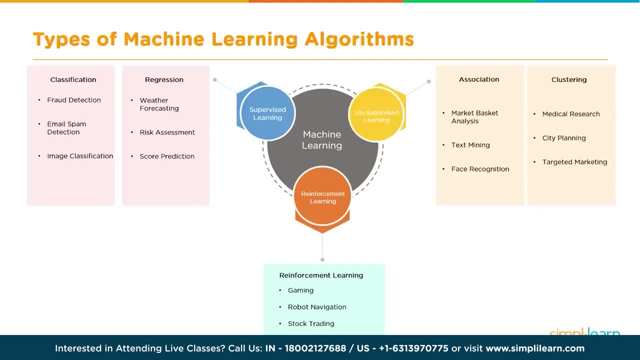 from scratch. There is an agent and there is an environment. The agent is given a certain target and it is rewarded when it is moving towards that target and it is penalized if it is moving in a direction which is not achieving that target. So it is more like a carrot and stick. 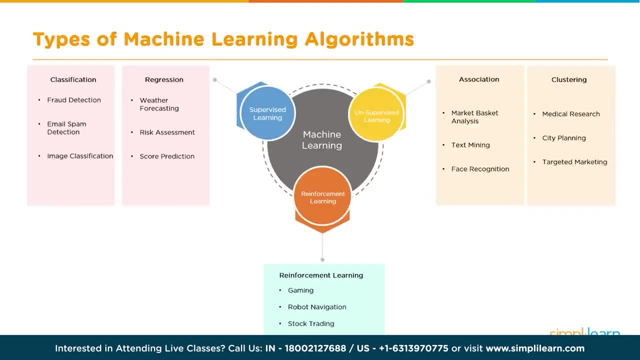 model. So what is the difference between these three types of algorithms? Supervised algorithms or supervised learning algorithms are used when you have a specific target value that you would like to predict. The target could be categorical, having two or more possible outcomes, or classes, if you will, That is. 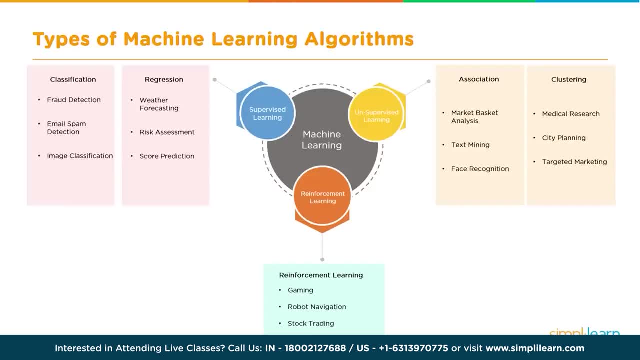 what is classification, or the target could be a value which can be measured, and that's where we use regression, like, for example, weather forecasting. you want to find the temperature, Whereas in classification you want to find out whether this is a fraud or not a fraud, or if it is email spam. 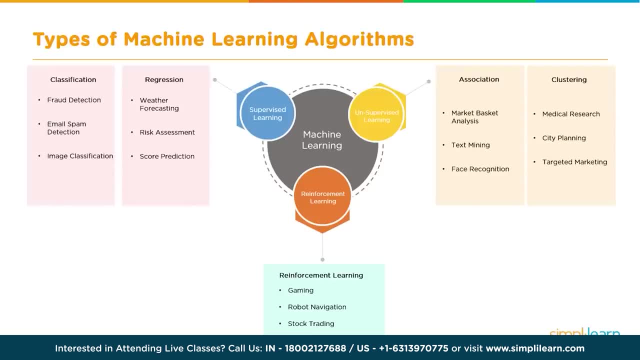 whether it is spam or not spam. So that is a classification example. So if you know- or this is known as labeled information- If you have the labeled information, then you use supervised learning. In case of unsupervised learning, we have input data, but 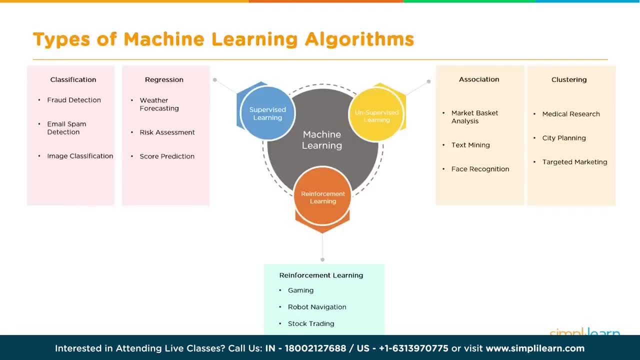 we don't have the labels or what the output is supposed to be. So that is when we use unsupervised learning techniques like clustering and association and we try to analyze the data. In case of reinforcement learning, it allows the agent to automatically determine the ideal behavior within a specific 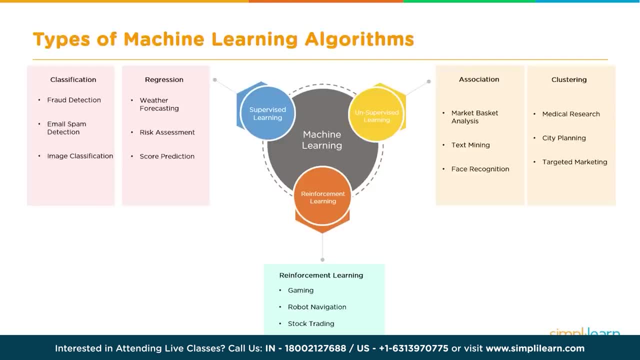 context and it has to do this to maximize the performance, like, for example, playing a game. So the agent is told that you need to score the maximum score possible without losing lives. So that is a target that is given to the agent and it is allowed to learn. 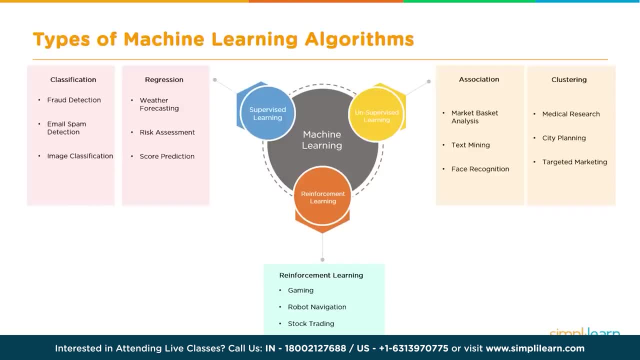 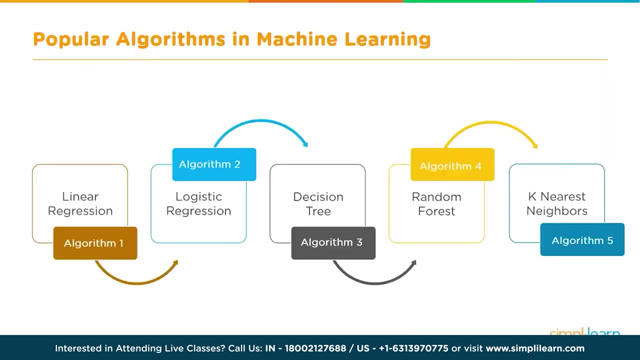 from scratch. play the game itself multiple times and slowly it will learn the behavior which will increase the score and keep the lives to the maximum. That's an example of reinforcement learning. So we will discuss about some of the most popular algorithms in machine learning, A few of them. 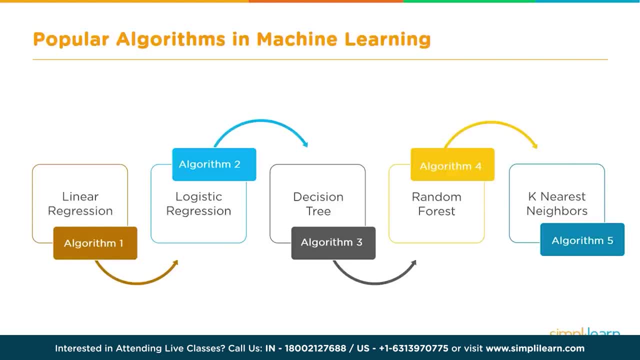 are listed here. This is by no means an exhaustive list. There are really a lot of algorithms available out there, But these are some of the most common ones. What are these algorithms? Linear regression, logistic regression, decision tree, random forest and k- nearest neighbors. 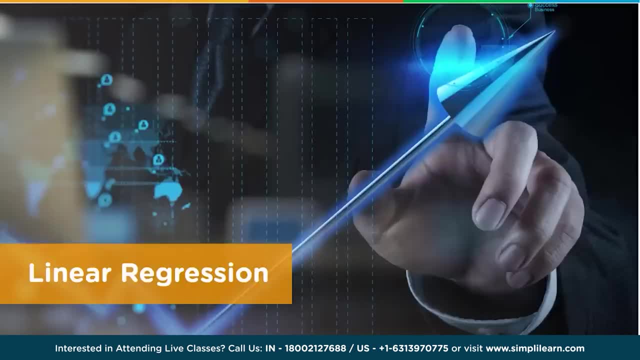 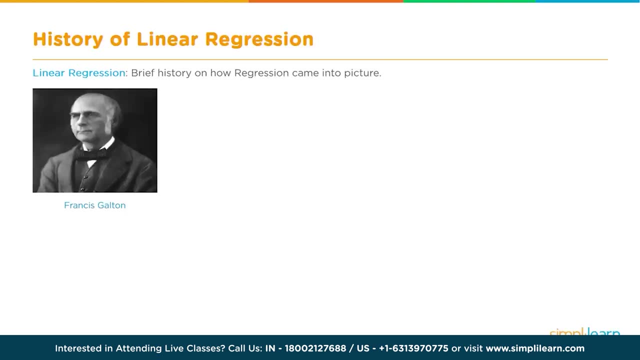 So let's look at each of these in detail. Linear regression: A little history about linear regression. Sir Francis Galton is credited with the discovery of the linear regression model. So what he did was he started studying the heights of father and son to. 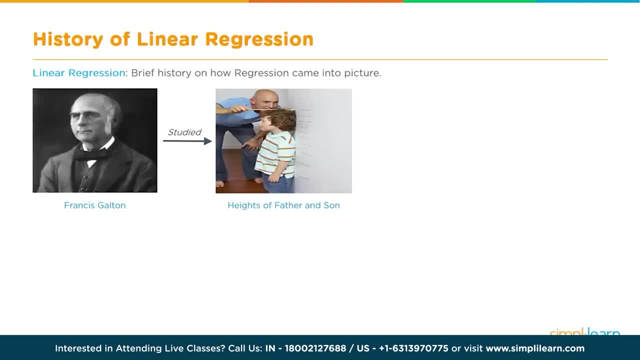 predict the son's height or the child's height even before he or she is born. So he collected enough data of the heights of father and the respective sons. He plotted this data on the x and y axis and he drew a line in such a way. 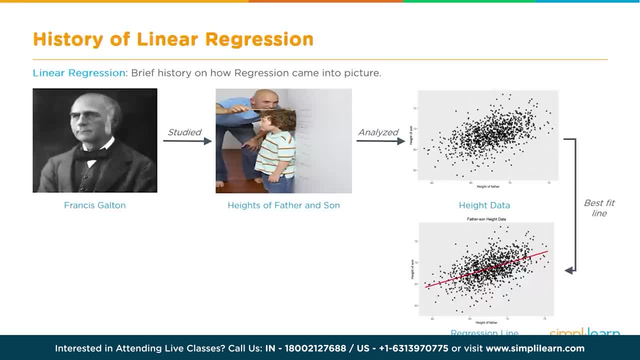 that the distance of these points from the line was the least, Which is now what we call it as mean square error. So at that time this term was probably not there, But that's what he did, And then he was able to use this line to predict. 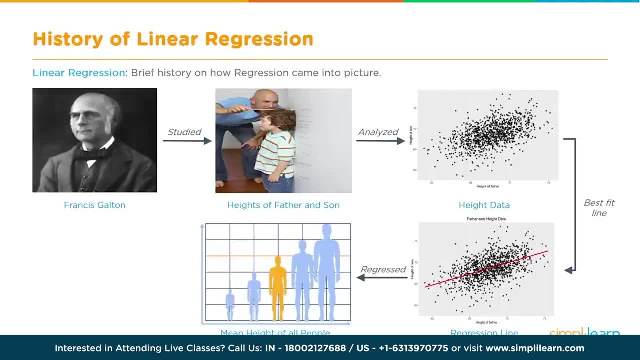 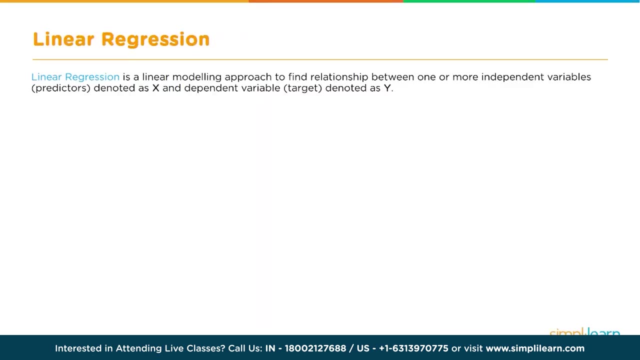 the height of the child which was yet to be born, based on the height of the father. So that was the very beginning, or very initial phase of linear regression algorithm. So that was a little bit of history. But what is linear regression? So linear regression is: 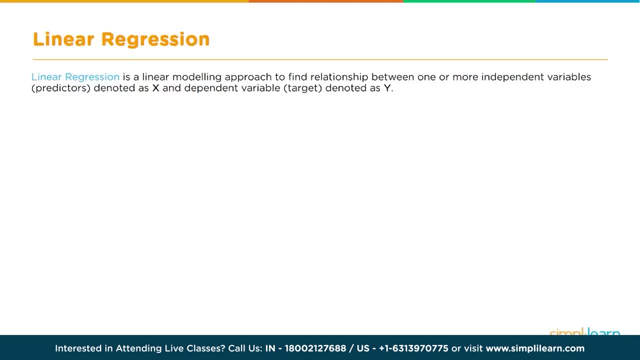 a way of modeling a linear model, creating a linear model to find the relationship between one or more independent variables, denoted by x, and a dependent variable which is also known as the target and denoted as y. A few examples are shown here. Let's say we: 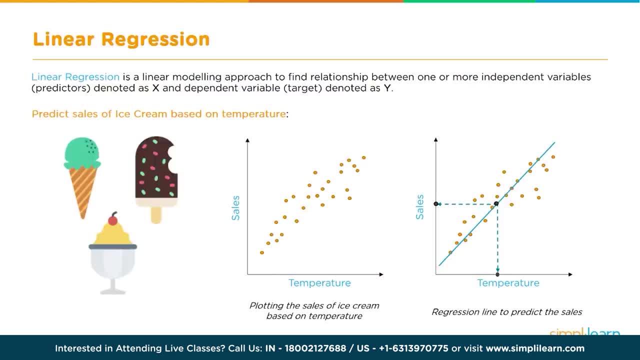 are going to plot the sales of ice cream and the temperature, So temperature on the x axis and the sales on the y axis, and this is how the data would look. And if we draw a line in such a way that the distance of each of these points 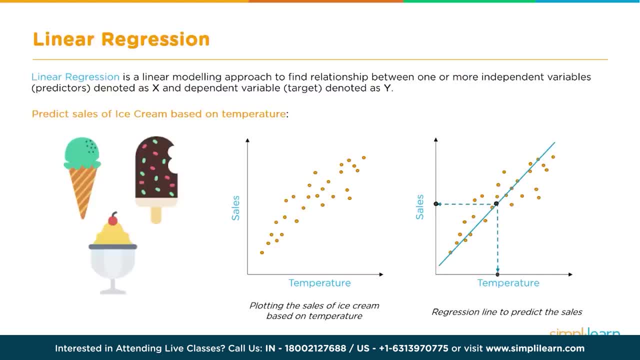 from this line is minimum. that is known as a regression line or the best fit line. So regression is all about finding this line And it is called linear regression because it is a straight line, linear, and the equation doesn't have any non-linear component, which 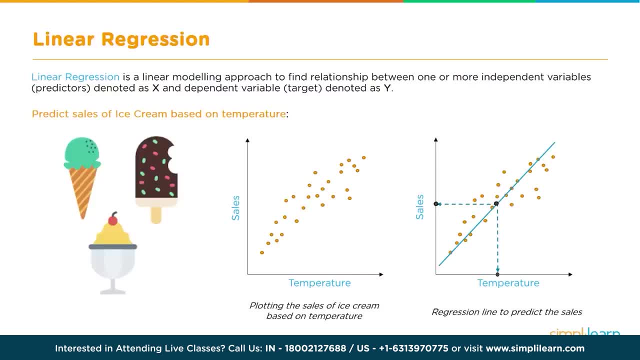 means we do not have x to the power of 2 or 3 or any of this. So this is simple linear regression. and simple linear regression is when there is only one independent variable, So there is only one x. So that is simple linear. 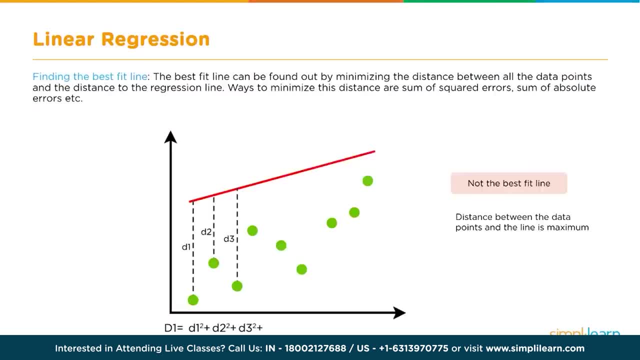 regression. So let's see how this is actually done. So linear regression is all about finding the best fit line, And the way it is done is in a recursive manner. So first a random line is drawn and the distance is calculated from this line of all the points. 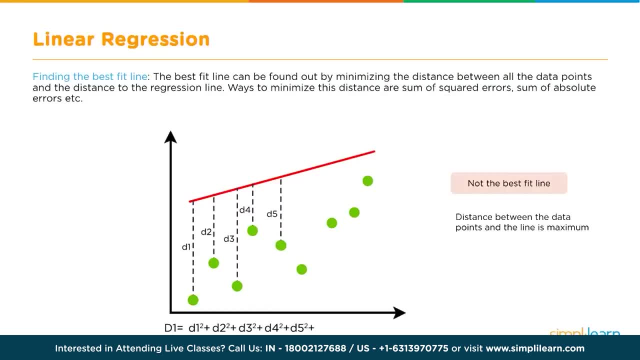 as you can see in this example, And that distance is known as the error, and to ensure that there are no negative values, this is squared, So we actually take the square of the distance of the point from the line and add it up and we make sure that. 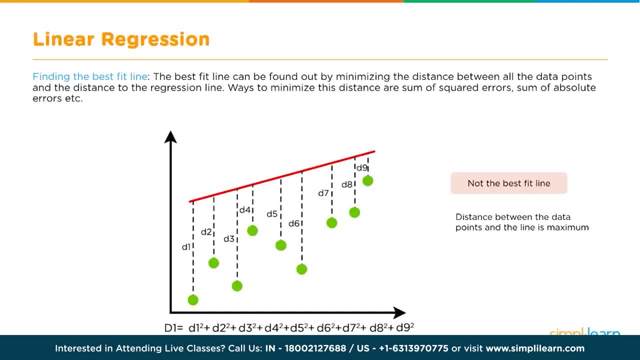 at the end, this sum, which is known as the sum of squared errors, is the minimum. So, as you can see, this is where we start, and then we keep changing the line in such a way and calculate the distance once again, the sum of the squares once again. and here again you will. 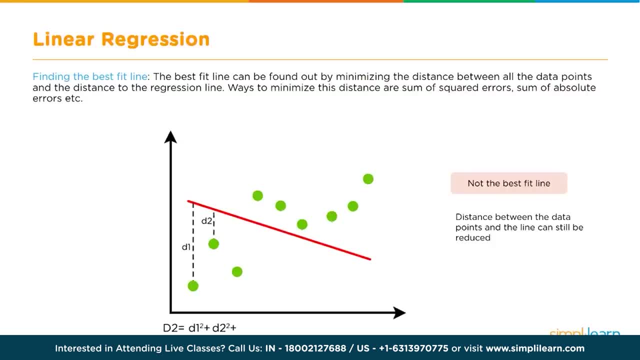 see that this is probably not minimum and we keep changing this, unless until we get a line where this value is minimum. So here we find that the sum of the squares of the distance, which is also the sum of squared errors, capital D, denoted by capital D, is minimum. 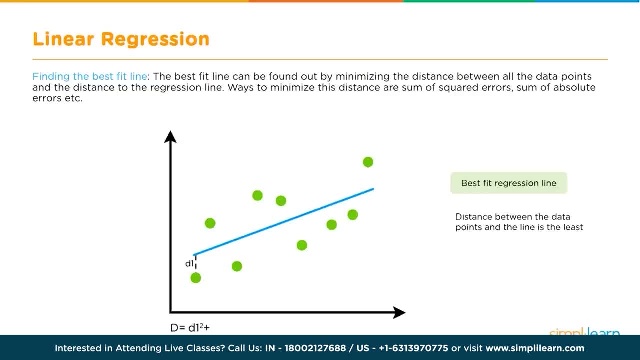 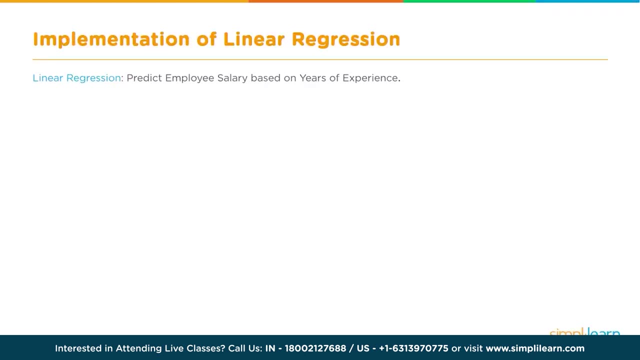 So now we found the best fit regression line. So this is a recursive process, it's an iterative process and this is what behind the scenes, this is what happens when we try to do linear regression. Now we'll take an example of linear regression and we will actually demonstrate. 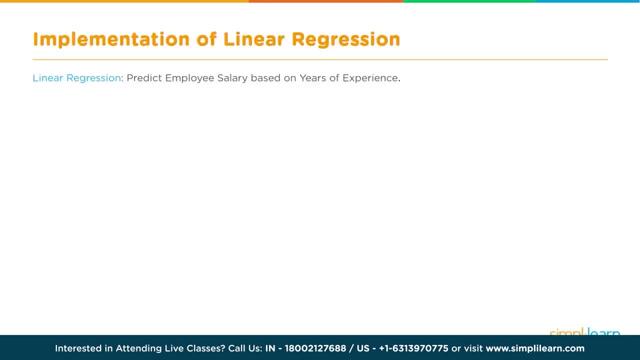 this using Python and we will be using Jupyter Notebook for this. In case you are familiar with Jupyter Notebook, I think that would be very helpful and if you need the data set, please put a comment under this video so that we can provide you with the data set Before. 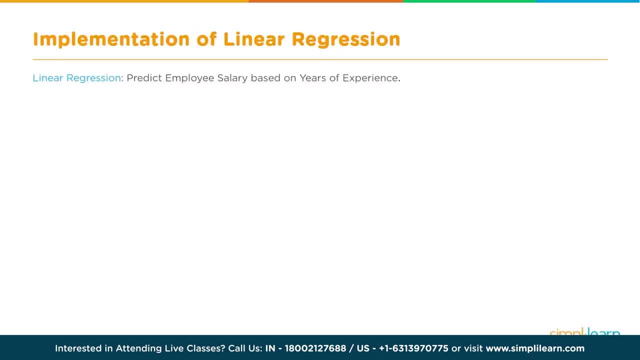 we go there. just let's try to understand what this example is all about. Let's say there is a new joining joining the company and we want to determine what should be the pay or the salary for this new joining and for that we already have the labeled. 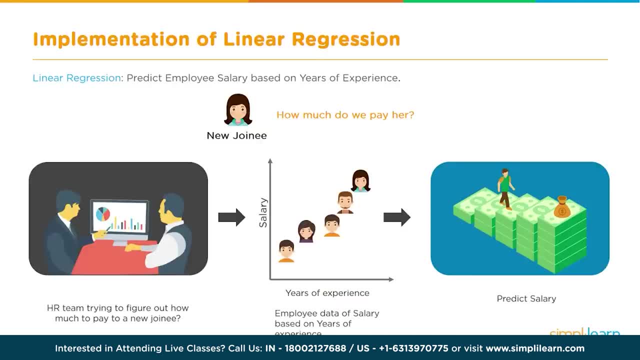 data, which is the details of our employees, based on their years of experience and their salaries. and for the new joining, we have the experience and we need to determine what should be the salary. So let's take a look at the demo So before we go into the Jupyter. 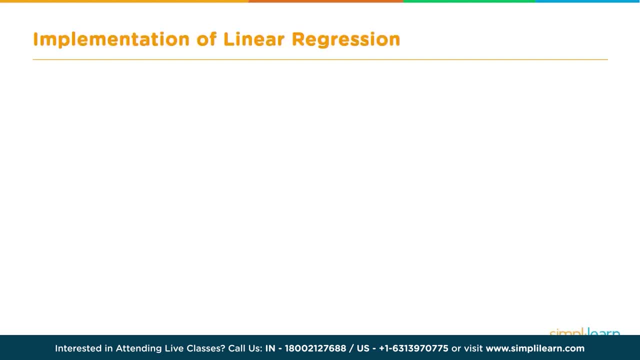 Notebook. let's quickly review the code: what the code is doing. The first section is about importing the libraries. Some of you who are familiar with Python will already be knowing this. You don't have to go into details. and then we import the data set and then we visualize. 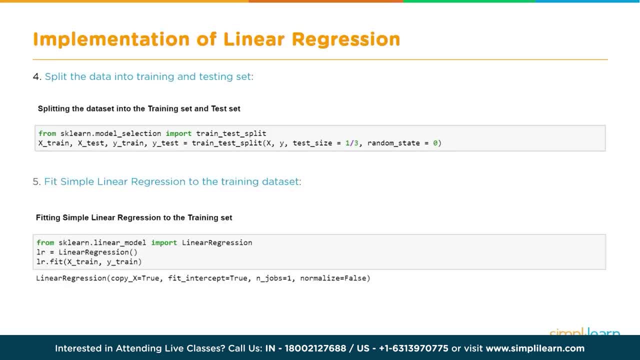 the data, just to get a quick idea about how the data is looking, and then we split the data into training and test data sets. This is a common procedure in machine learning process- any machine learning process- and the overall training and test process. we do with two different. 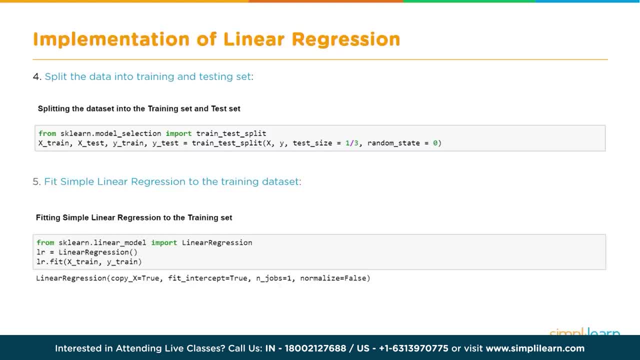 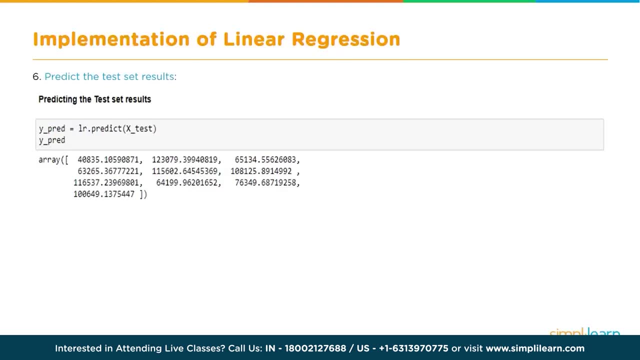 data sets. So that's what we are doing here, And then we build or train our model, the linear regression model, and then we do the testing and we find out what is the errors and visualize our results. and this is how the test results look and this is how 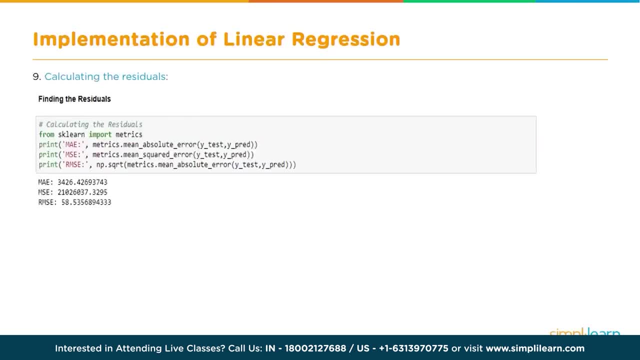 the training result looks And then we calculate the residuals. Residuals are nothing but the errors. There are couple of ways of measuring the accuracy, but the root mean square error is the most common one, RMSE, and in this case we got root mean. 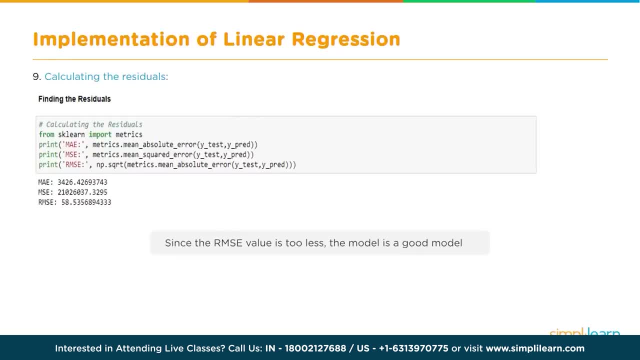 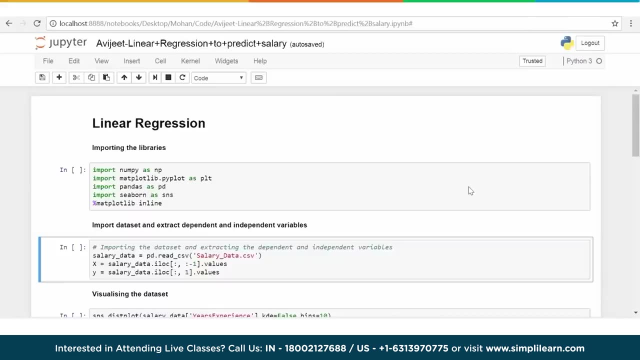 square error of 58, which is pretty good and that's our best fit. Alright, so now let's go into Jupyter Notebook and take a look at by running it live. Okay, so this is our code for the linear regression demo and this is how. 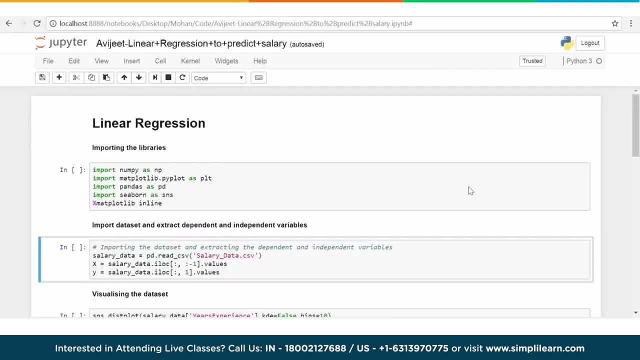 the Jupyter Notebook looks and this code in the Jupyter Notebook looks. I will walk you through the code pretty much line by line and let's see how this works. the linear regression. So the first part is pretty much a standard template in pretty much all our 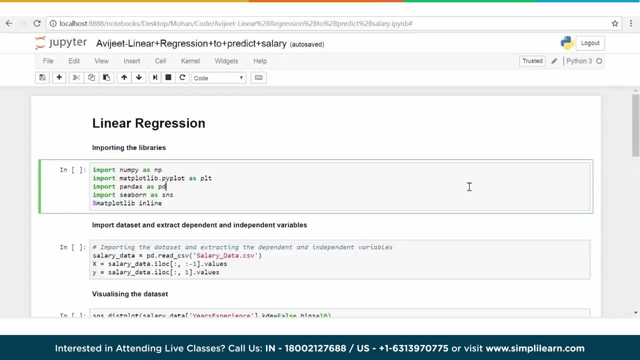 code we will see. This is importing the required libraries. so numpy is a library, matplotlib is a library, pandas and so on. So these libraries are required. each of these libraries have a different purpose, so some of them are required for manipulating your data, some for 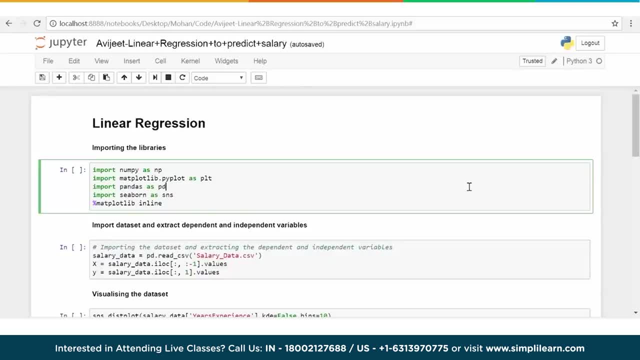 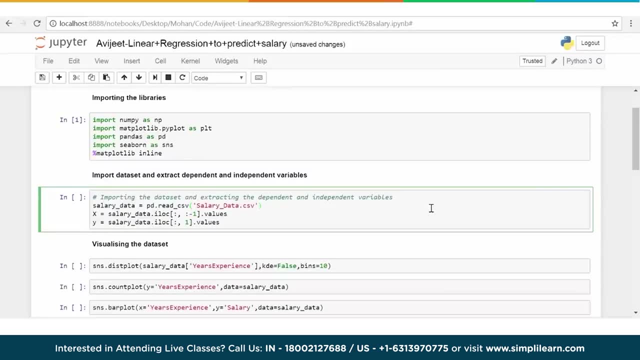 plotting, as the name suggests, matplotlib, and so on and so forth. Okay, so let's go ahead and import all these libraries and then we will import our data. So, in this example, what we are trying to do, the use case in this particular example is: we have some. 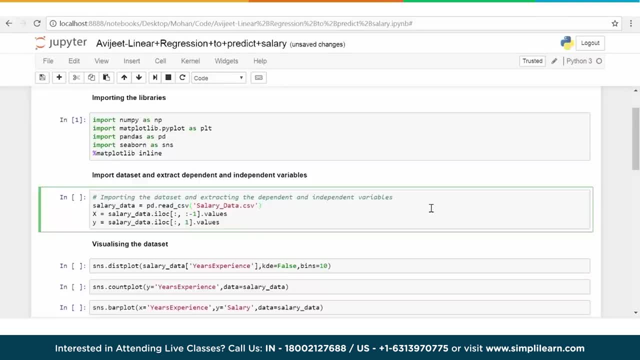 historical value of salary data, and now we want to build a model so that we can predict the salary for new employee, a person who is joining new, and we will use the same, the characteristics that were available to us or the features that were available to us, and we will try. 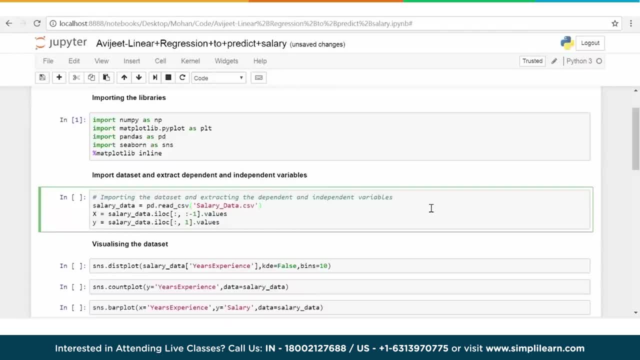 to predict what will be this salary of this new person. Okay, so that's the kind of the use case. So let's go ahead and load the data and let me introduce a cell and see how the data looks. So, salary underscore data. So we have basically two. 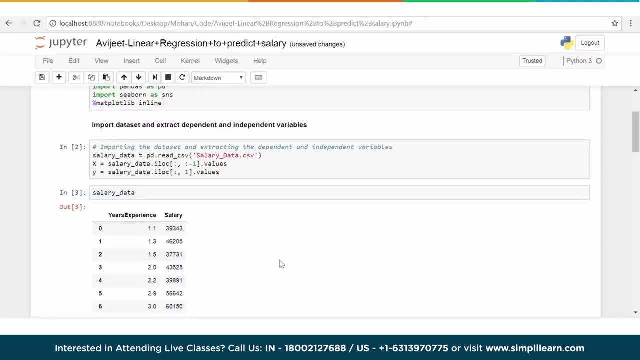 features right. so it's pretty much like a simple linear regression we are trying to do So. we have years of experience and salary and in this case what we are trying to do is this is our predictor. so years of experience is our predictor and we are trying to predict. 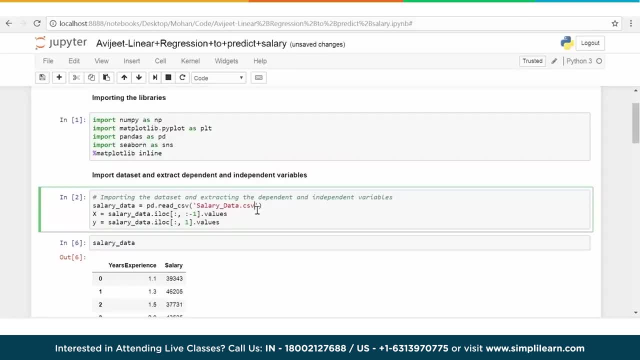 what the salary would be. So once again, so x is what is known as the predictor and y is the target. So number of years of experience we are taking as input and we will try to find what will be the salary of this person based on that. Okay so, 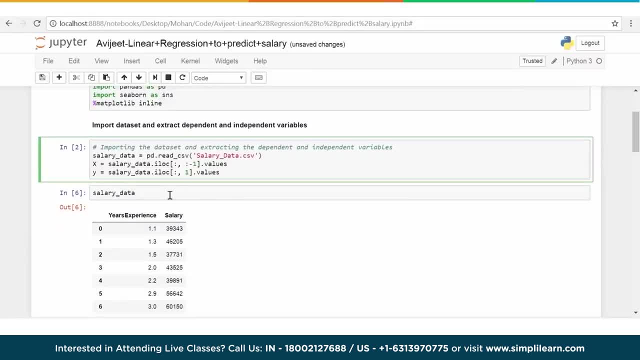 that's what we are going to do. So I have shown what is how the overall- how the data has been imported- looks. Now let's take a quick look at these extracted values or extracted columns as well. So let me put in x here and see how it looks. So this: 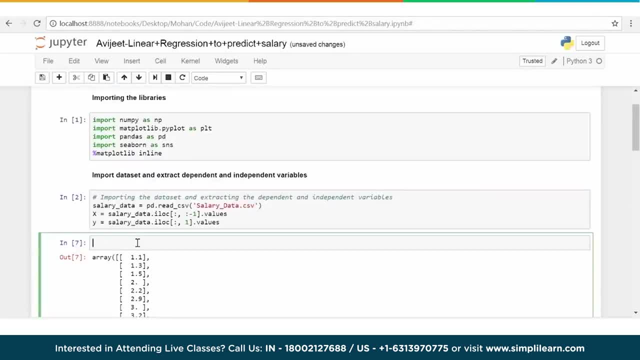 is basically one column and same way. if we put y here, we will see what exactly. I'm sorry this has to be in small, lower case. So this is the salary information. Okay, so this is how our data is, and then we can do a little bit of plotting of the. 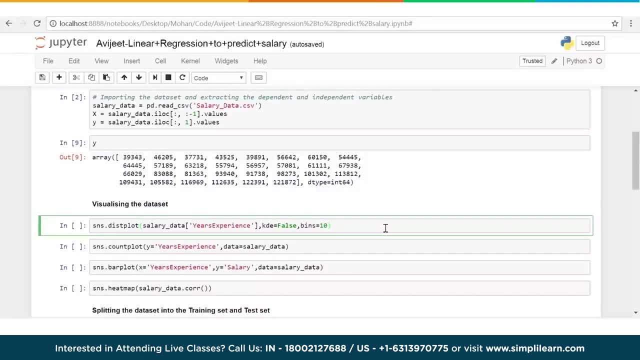 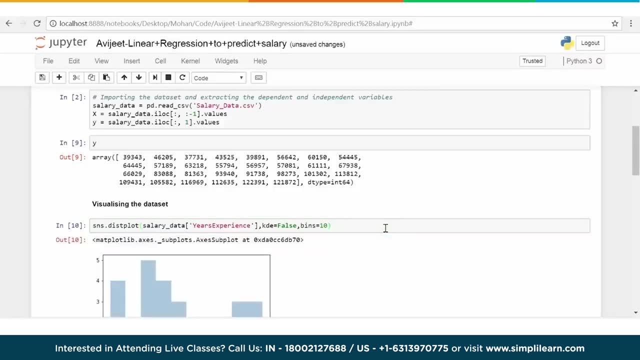 data, to play around a little bit, because we imported the data. typically we want to do some exploratory analysis: how they compare with each other and so on and so forth, How they are correlated. So let's draw a quick plot, a bar plot, and see. 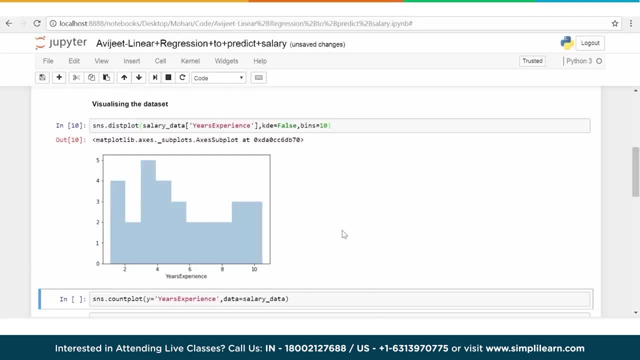 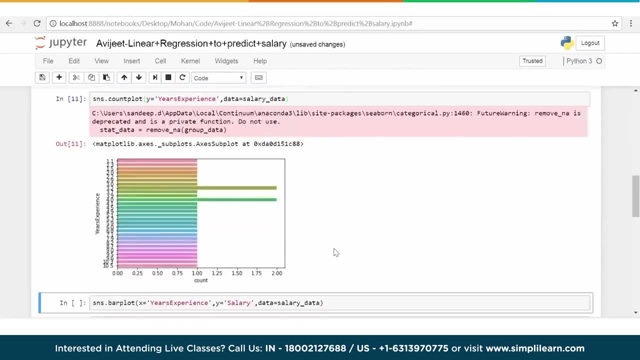 how the years of experience are being seen here, Right, so this is how the bar plot looks. Similarly, let's do one more, which is basically more like this is horizontal bar plot. Okay, so how many people and with what experience, and so on and so forth. So what this shows 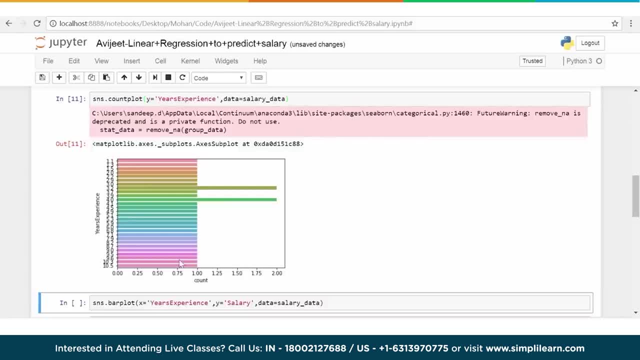 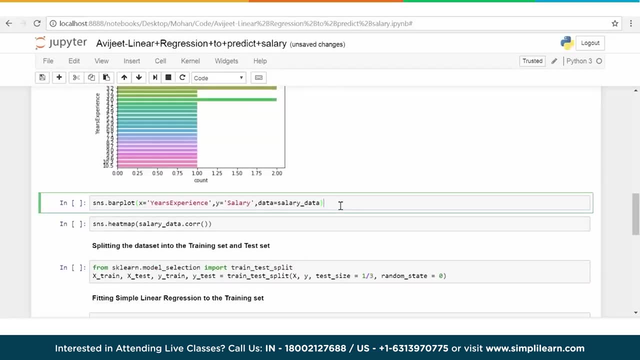 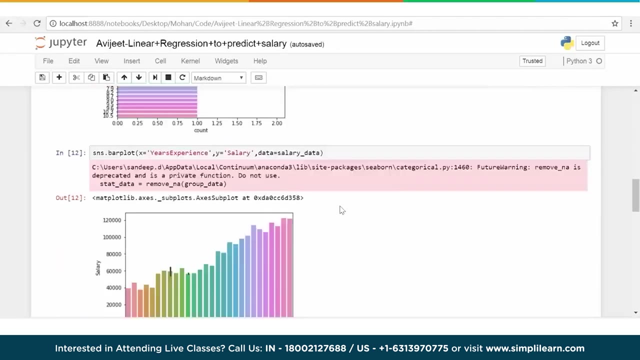 is the count, how many records are there with a given experience, and things like that? Okay, so this is another way of visualizing the data, and this is a third view, and this is one more view, and then we can do a quick heat map. So there is only one. 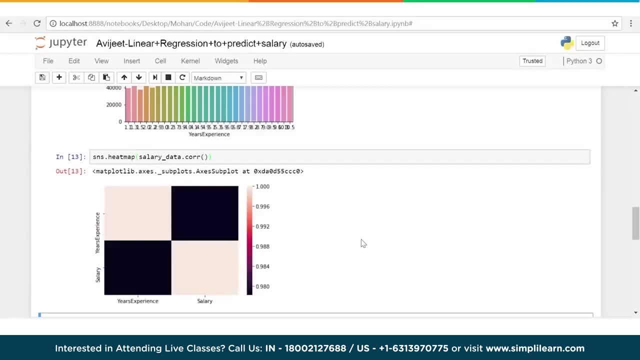 or actually there are only two variables. so there is not a lot of plotting that we can do Or not a lot of visualization that we can do, since there are only two variables, But nevertheless, whatever is possible we can do a quick to get a quick idea about how the data 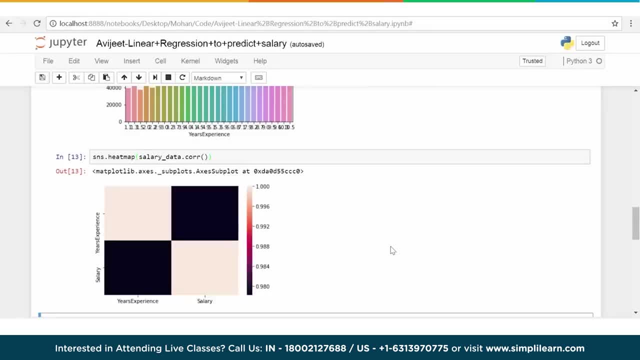 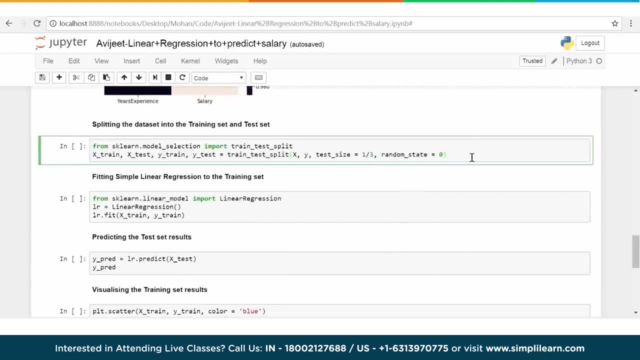 is looking and how the variables are related to each other. Is there a correlation, and things like that? Alright, so once we are done with that, this is the most important part of our demo here, which is, basically: this is the beginning of our training process. So the first thing, 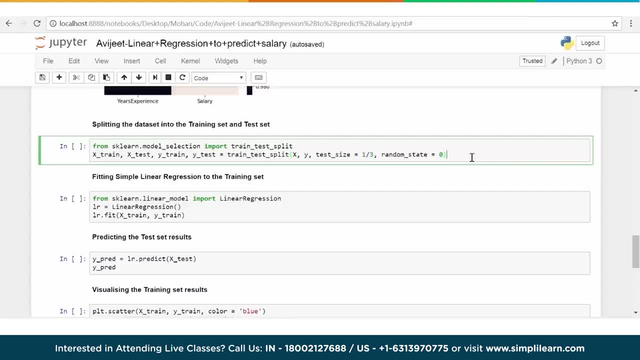 before we start the model building and model training process is to split the data into training and test data sets. Okay now, whenever we do any machine learning exercise, especially supervised learning, we never use the entire label data for training purpose. The reason being, then: we will not. 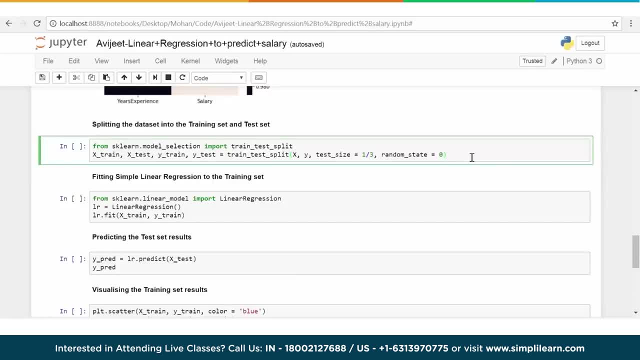 be able to correctly evaluate how well the training has happened. Okay, so what we do is we split the data, we take a portion of the data- we call that as the training data set- and we set aside some portion of the data- we call that as a test data set. We use 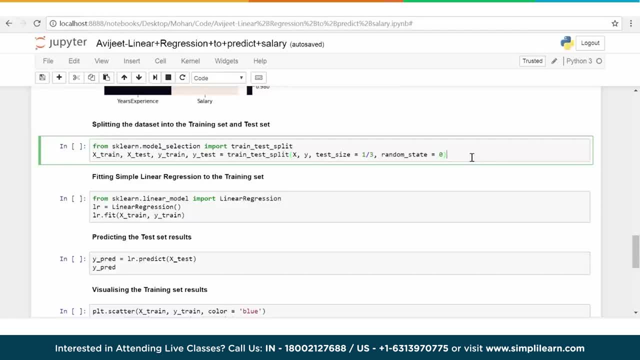 the training data set to actually perform the training, to train our model. and once that is done, we use the test data set to check how well the model has been trained, How accurately it is able to predict. Okay, now the reason is with our test data set also. 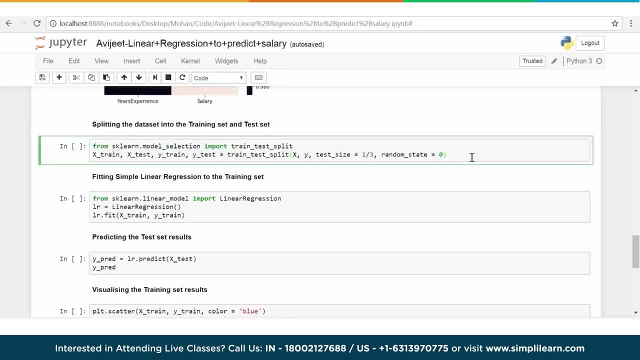 since that is also labeled, we allow the model to predict the values and we compare it with the labeled information to see whether it has predicted correctly or not. Okay, so that is the reason in all machine learning activities. whenever we perform machine learning, we especially training of. 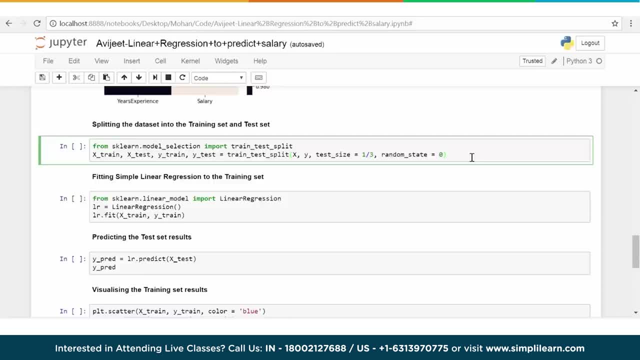 a model. we split this data into training and test data set, and that is what we are going to do here Now. there is no need to write any separate code for that. There is a readily available function for that: train underscore, test underscore split. So that is what we are going to use. 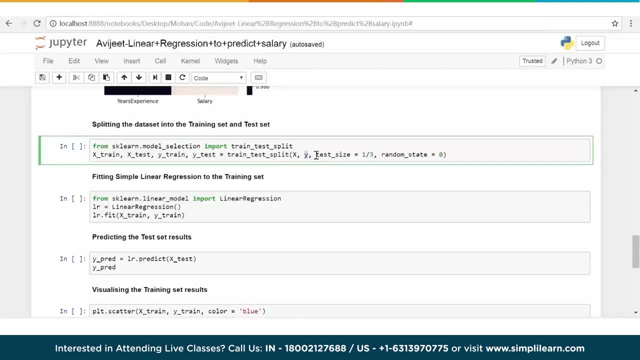 here It takes the data set- x and y is the data set- and in addition it takes a parameter which tells how the data has to be split. So for example, here it says test size is equal to 1 by 3. that means it is 33 percent right. 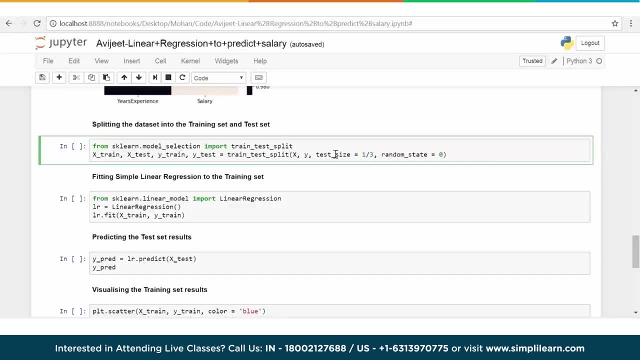 33.33 percent, So one third of the data you want to set aside for test. Now there are no hard and fast rules as to what should be the split of test and training data set. It is a matter of individual preferences. Some people would. 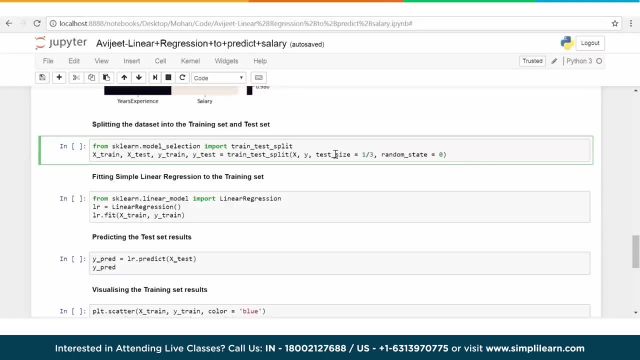 like to have 50, 50, some people would prefer 80, 20 and so on and so forth. So it is completely up to the individuals to decide on that. So, in this particular case, what we are doing is we are setting aside one third of 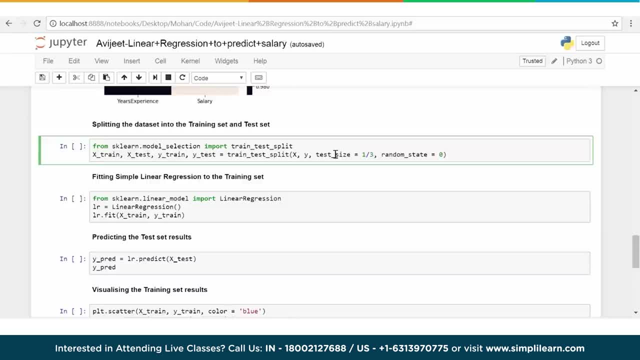 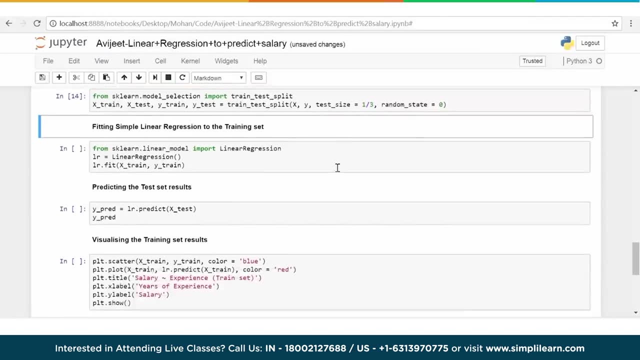 the data set for testing purpose and two thirds of the data set for training purpose. So that is exactly what we are doing here Now. the next step is to create an instance of linear regression. So linear regression model is readily available. So we create an instance of the linear. 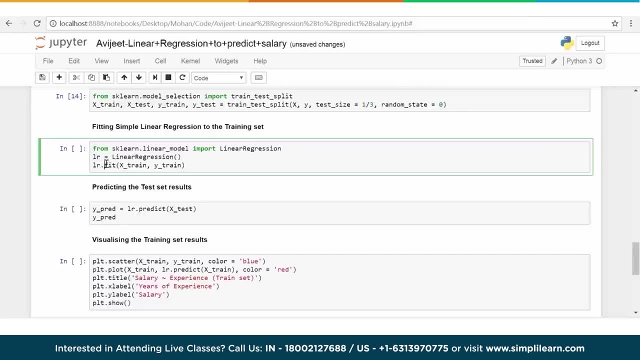 regression model and give it a name like LR, and then we call the fit method of the linear regression model. Now this fit method is common across all the algorithms, So any algorithm you use if you want to start the training process, you call the fit method. Okay, and 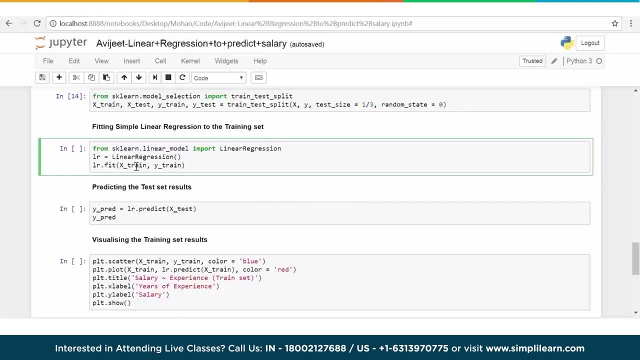 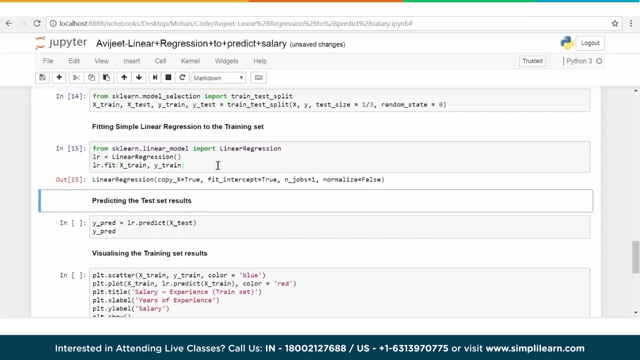 then we pass the training data set. Now training data set, we send the predictor, as I was saying, or the independent variable and also the dependent variable. We pass both of them, Okay, and the system will basically learn based on this. So now the training has happened. Training is completed. 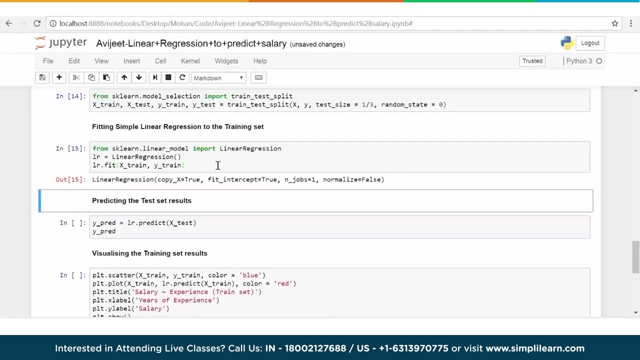 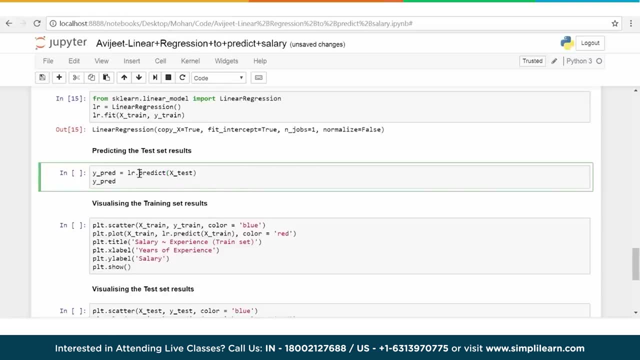 and now we need to see whether it is predicting correctly or not. We need to test it right. So for testing we have another method called predict. Again, this is common across all algorithms. Any algorithm you use, you will have this predict method for testing. 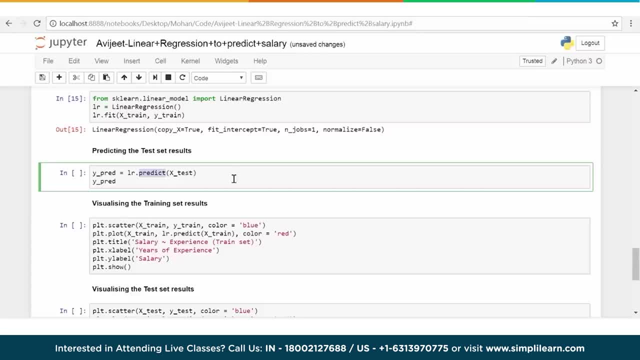 your model, Okay, or for actually predicting the values, whether during testing or when you actually deploy the model. Okay. now here, predict will take only one parameter, which is the independent variables. Right, the reason being the dependent variable is what it will predict, Right, so y underscore. 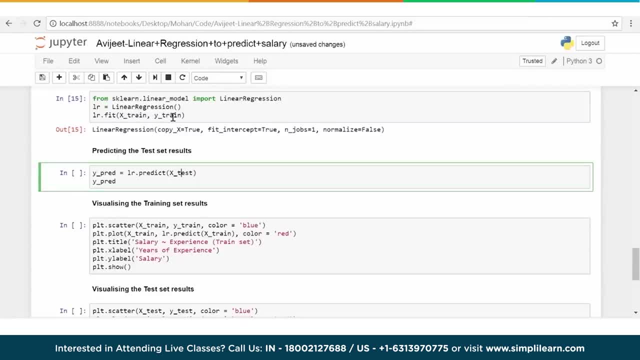 test we don't have to pass, whereas here, y underscore train, we passed for training purpose, But y underscore test we do not pass, because that is what the model will predict. So we don't have to pass that. And then the model will predict: and that is what. 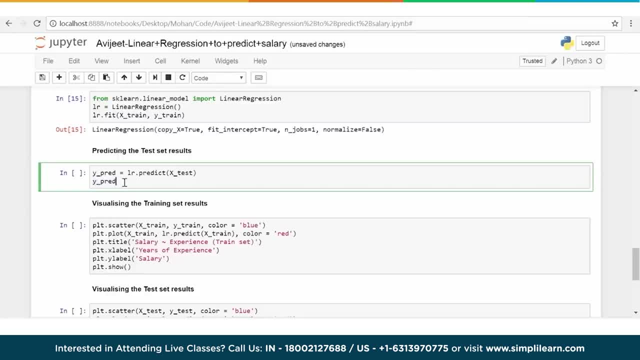 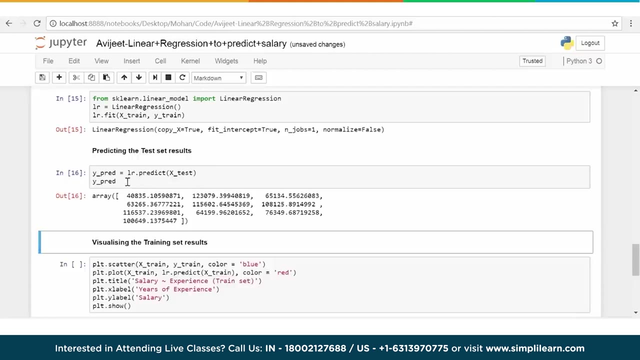 we call it as y underscore pred, But we will use y underscore test to compare with what the model has predicted, and thereby we can determine how accurate the model is. Okay, so let me go ahead and run this code. So it has done with the testing or with the prediction. 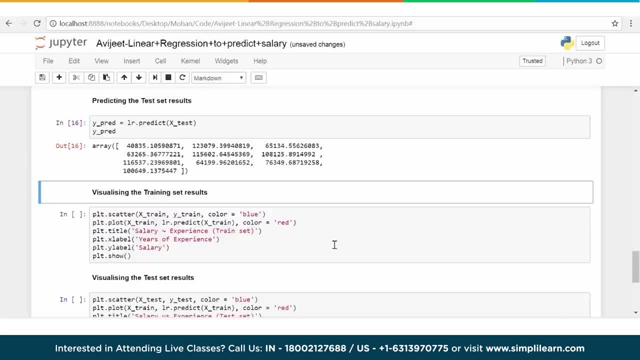 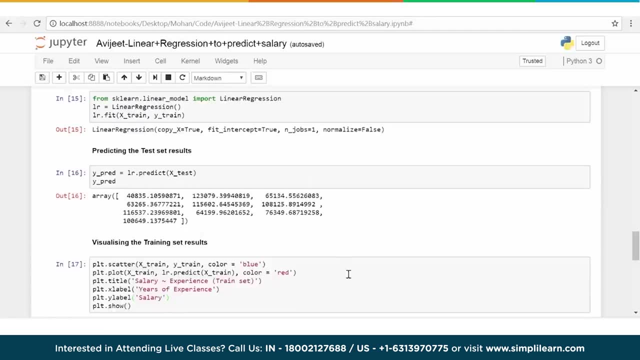 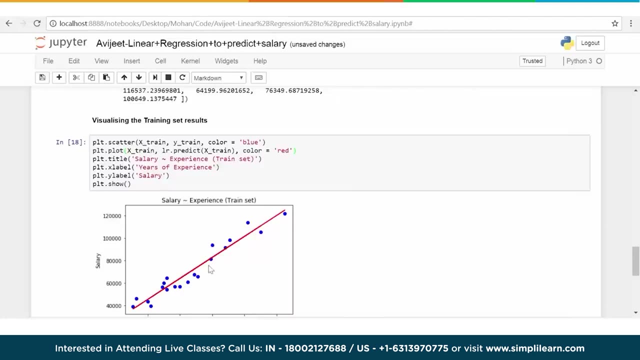 of the values. So these are the predicted values and now we can visualize. we can generate some plots to visualize this information. So let's plot this training set, results, information and see how it looks. So what we are doing here is, basically, we have the. 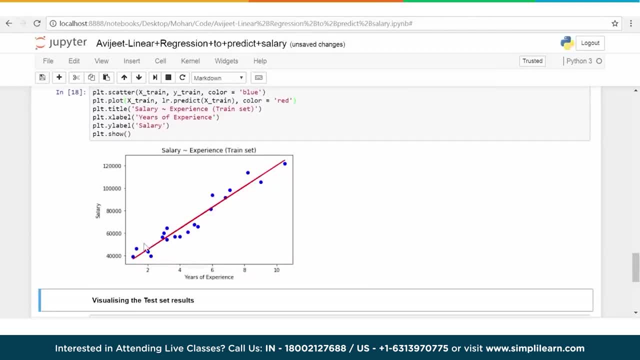 training data set plotted The salary versus the years of experience. Right, this is the training data, the dots basically. And then this line is what our model has, So this is the best fit. So linear regression: what is linear regression process? 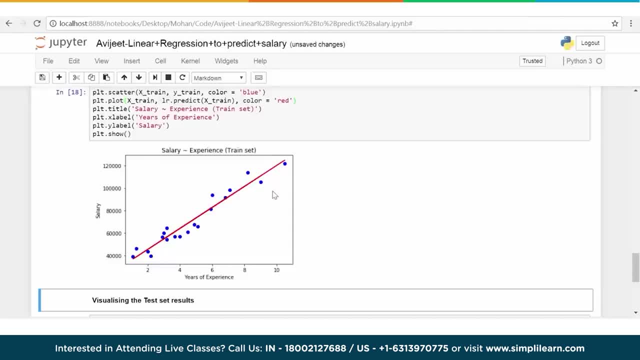 We find a equation of a line which is the best fit. So our model- this is the equation, or this is the line that our model has kind of come up with saying that this is the best fit model. Okay. so, as you can see, intuitively it feels okay because 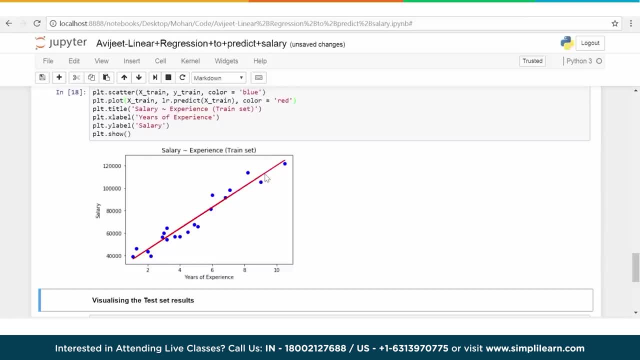 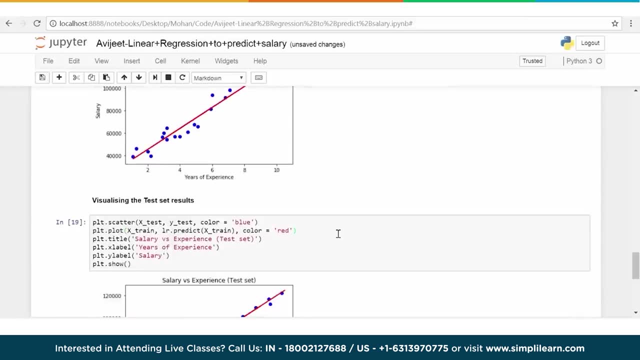 it is passing through pretty much the middle of our data set. Okay, so this is for the training part. Now we do the same for our test as well and see how it is doing, or how it looks Here also, it looks pretty good because the line passes. 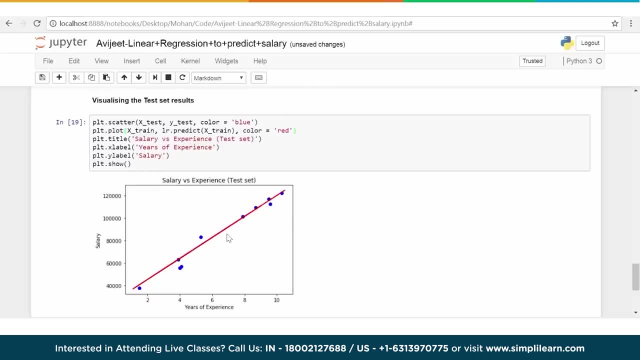 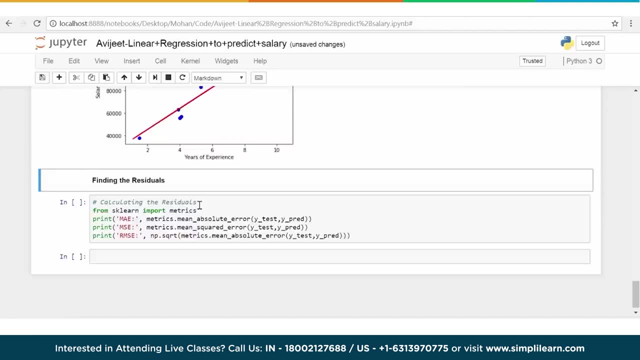 pretty much in the middle of the overall data set. That's what we are trying to do here. Alright, and then how do we measure the accuracy? So these residuals are nothing but the errors. The term residuals is nothing but the errors we have seen in the 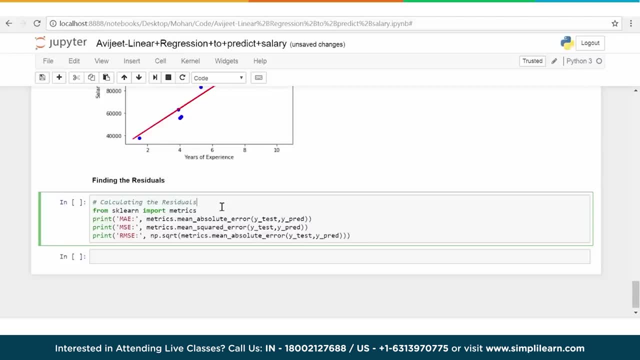 slides as well. So we calculate the accuracy of our model by calculating the various residuals. We have like mean square error. then we have the mean absolute error and then we have the root mean square error. They are pretty much. they are very closely related. 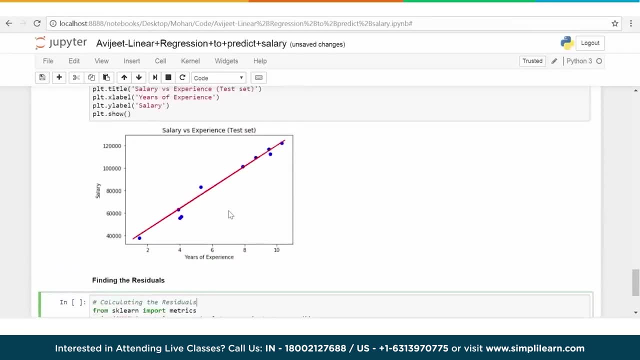 this is nothing but the error and the actual value. So, for example, let me explain with this particular line: So what our model says is: if the value of the years of experience- so let me take this point- maybe If the value of the years of experience. 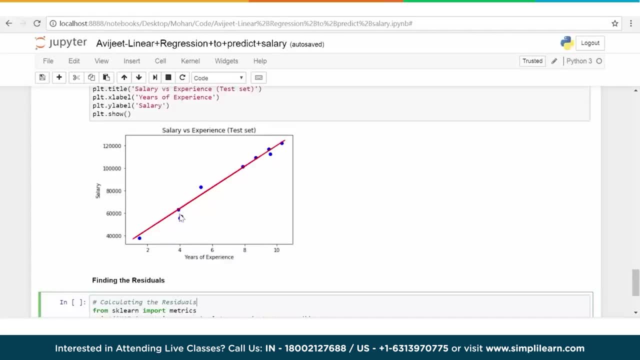 is 4, then the salary will be, according to our data, that salary probably should be. what is this? maybe around 58000, and there are, of course, 3 points, 3 data points pretty much around this 4 years experience. One maybe around 58. 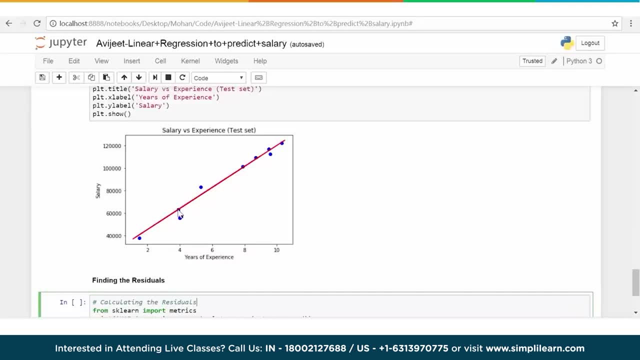 or in fact, 2 of them are around 58 and there is one more which is probably 60. Now these are the 3 data points, whereas our model predicts that if the years of experience is 4, then the salary should be 60000. let's say: 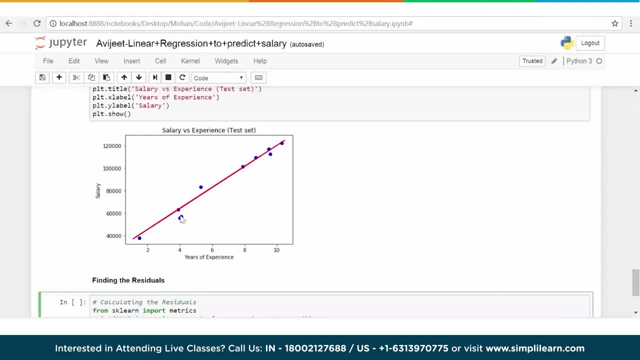 Let's assume this goes to 60000.. Which means that one of the data points is very accurately predicted by our model, but there are 2 of them which are off. So there is an error for these 2 values. and what is that error? The error is nothing but the. 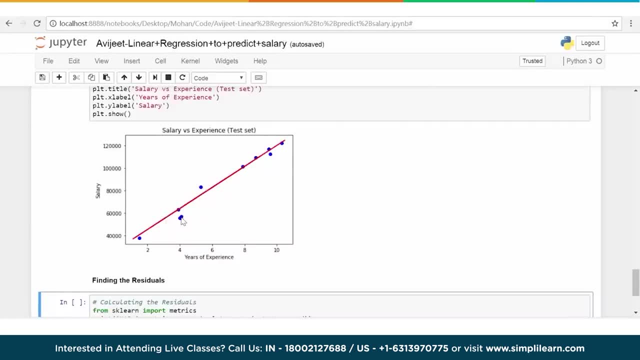 distance of this point from this line, The distance of this point, of each of these data points, from the line, is the error. So that's basically for each of the values, it will correct, it will calculate, rather, and instead of taking the absolute value, we kind of take. 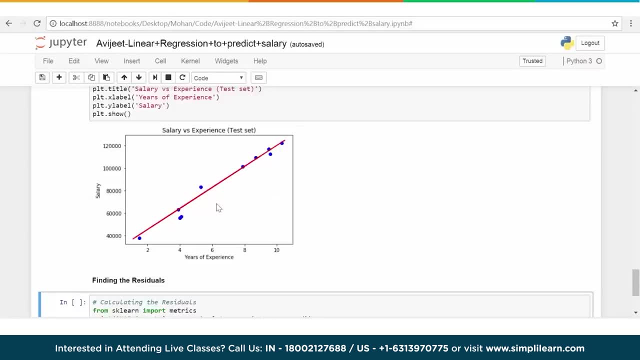 the square of that. So, because the value can be positive or negative. So, in order to avoid a cancellation- so there are some positive values, there are some negative values and they get cancelled out- What we do is we take a square of that. So that is basically. 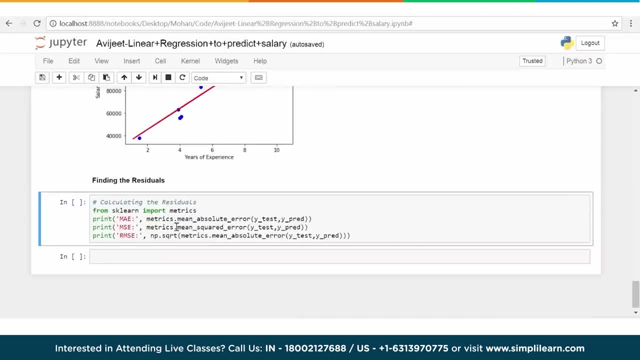 what is the root mean square or the mean square error. And then if we take a square root of that, it becomes root mean square error. So this was explained, probably in the slides as well. So that is what we will calculate here and we print it. 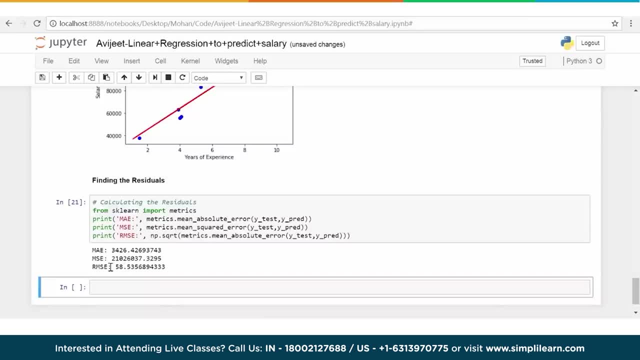 okay. And these values- the root mean square error, the mean square error and the mean absolute error. the lower these values are, the better, So the accuracy is higher if these values are lower, So in a way it is inversely proportional, Okay. 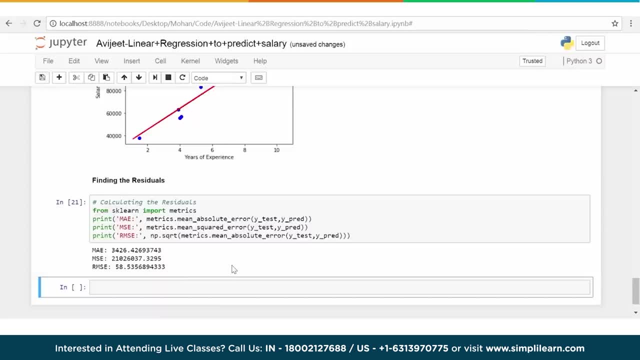 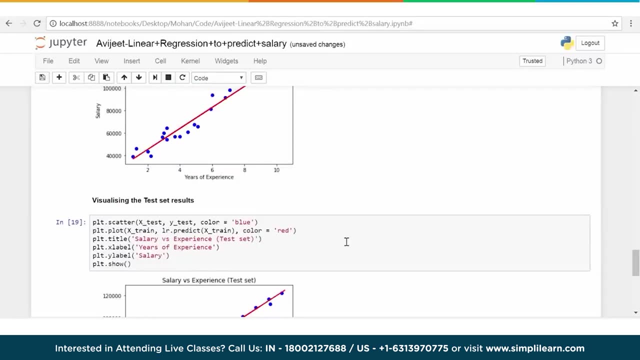 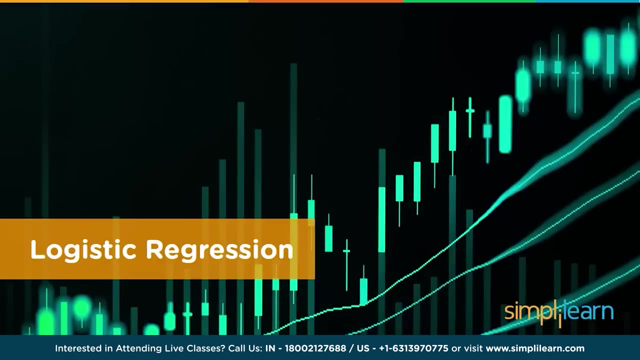 So that's the way we measure the accuracy of our linear regression model. Alright, so that brings us to the end of this demo and we will continue with the other demos. Alright, now that we have seen linear regression, let's take a look at our next machine. 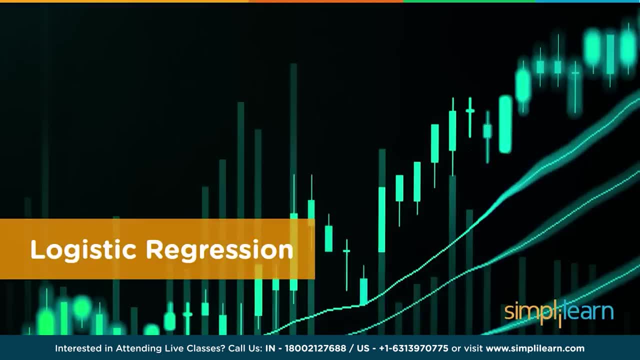 learning algorithm, which is logistic regression. Now, what's interesting about this algorithm is that, while it says regression, the name has regression in it, but keep in mind, this is not used for regression, but this algorithm is used for classification. Now, many people get confused By this name, so you need 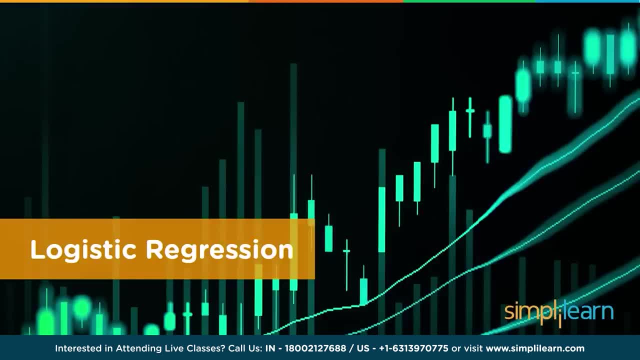 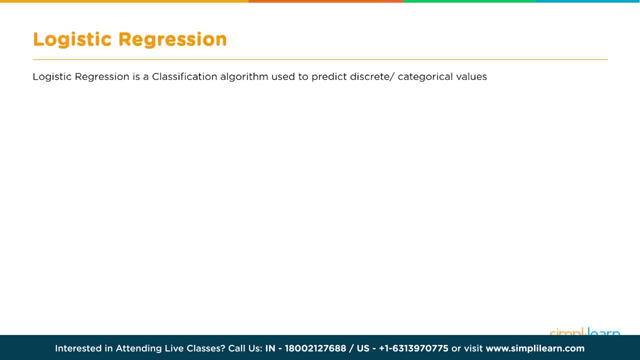 to be aware of it. Linear regression is used to solve regression problems where we are trying to predict a value, whereas logistic regression is used to solve a classification problem. So we are trying to find, for example, whether a person will repay the loan or not, or whether we want. 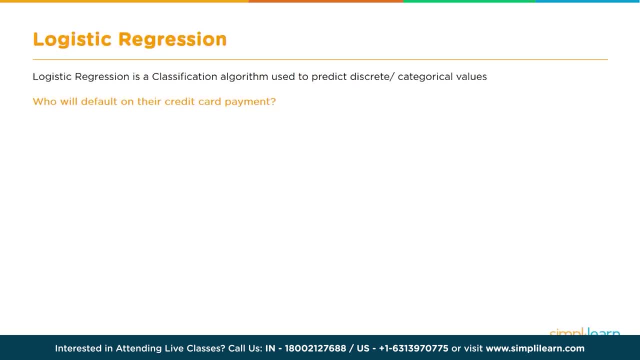 to find whether this image is of a cat or a dog. So this is a classification problem, Okay, So just that you should be aware of the name. So in this slide we are talking about whether a person, credit card user or credit card holder- will default. 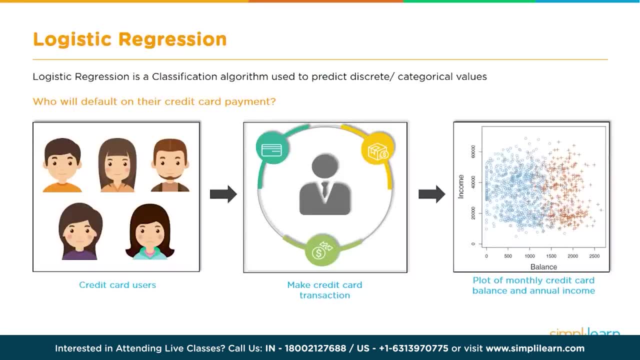 on the payment So we can create a profile. We have historical data and of people- their income and their credit card balance, and we have examples of people who have defaulted and people who have not defaulted and based on that, we let the system learn to predict. 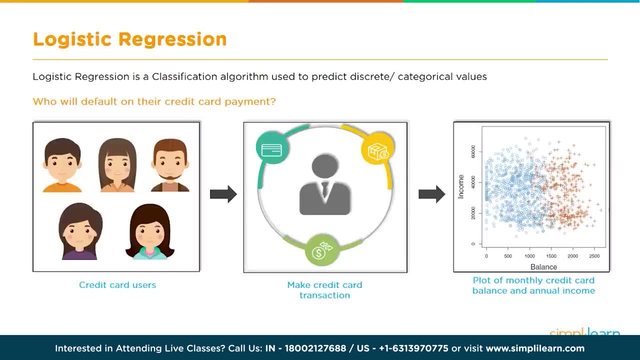 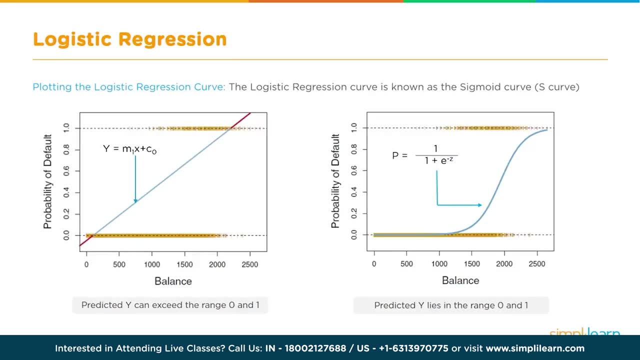 this particular value, whether the person will default on the payment or not. Now how does the logistic regression work If we try to draw a straight line to determine the probability? So we are trying to predict whether this person will default or not. Okay, 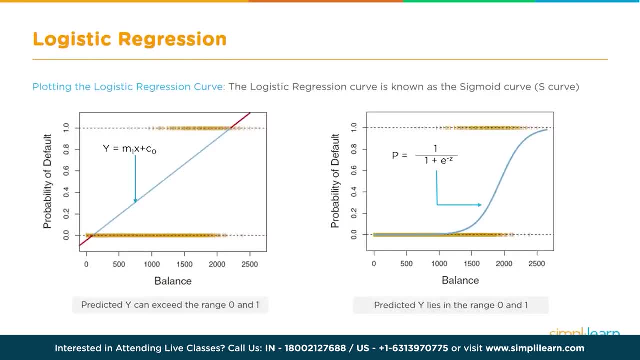 So if we draw a straight line, then the predicted value can exceed 0 and 1, which is not a good idea. So the probability is calculated between 0 and 1 using what is known as a sigmoid curve, So it is not a straight line. 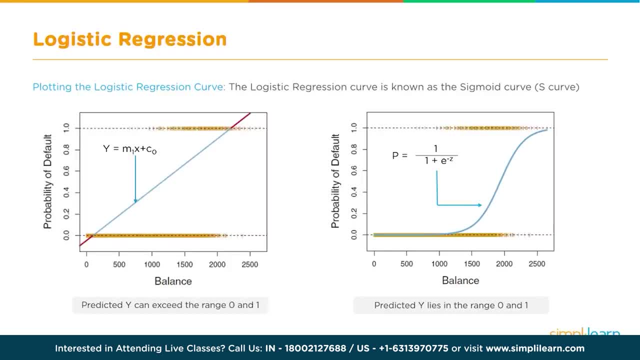 but we use a different formula, a different mechanism to find the probability and find the value between 0 and 1, and the formula for that is: p is equal to 1 by 1 plus e to the power of minus z. Here z is actually the linear. 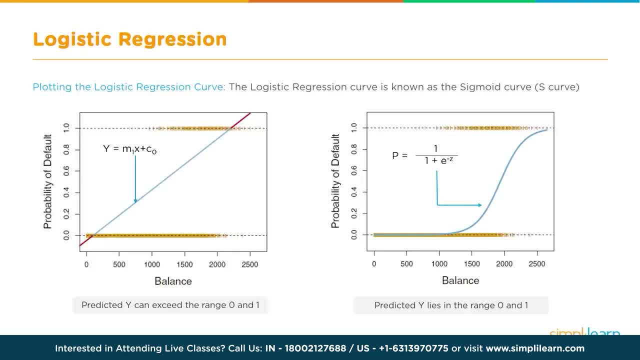 equation that we used in figure 1, which is m1x plus c0. So this is fed to p and the value is calculated between 0 and 1 and we will see, actually automatically, we will see here that if z is negative and much, much higher, a very high, 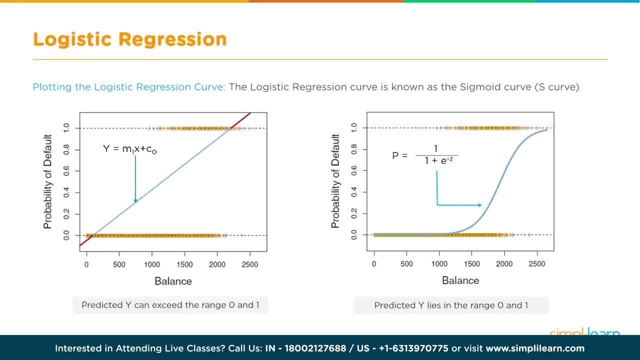 value it will. the equation will be 1 by 1 plus 0, which is equal to 1.. So we will see here that if the value of z is positive- and it is some high number- then the value of p can at the most be equal to. 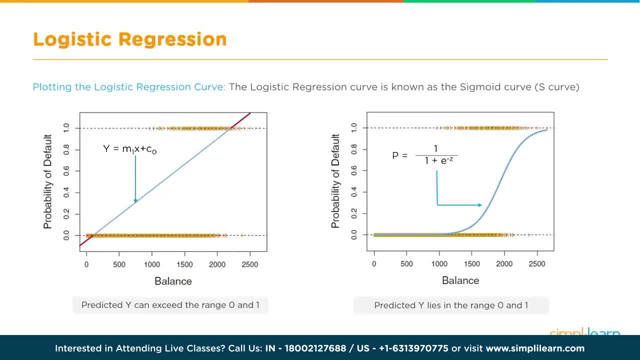 1, because this portion here is 1 by a very high number, Let's say infinity. So 1 by infinity is 0, so this whole thing becomes 1 by 1, so that is equal to 1.. p is equal to 1.. So that is where. 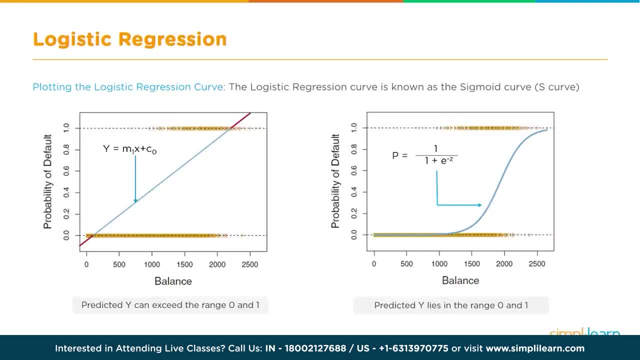 the maximum value it can achieve is 1.. Similarly, if the value is negative, if the z value is negative or negative and very high value, then this will become very high and therefore the denominator will become infinity. So 1 by infinity is 0 and therefore p is equal to 0.. 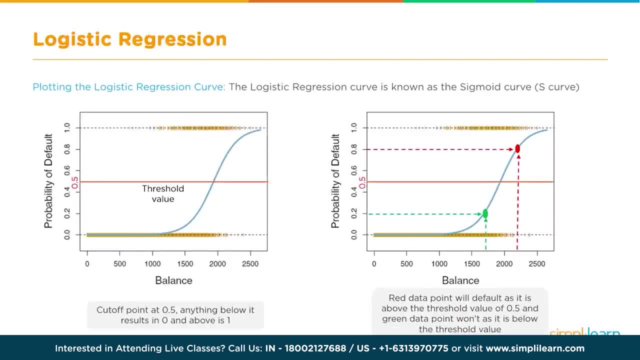 So that's the way the sigmoid function works. This is how the graph looks, and there has to be a threshold value which is, like in this case, 0.5.. So if the value is greater than 0.5, we consider the output as 1, whereas 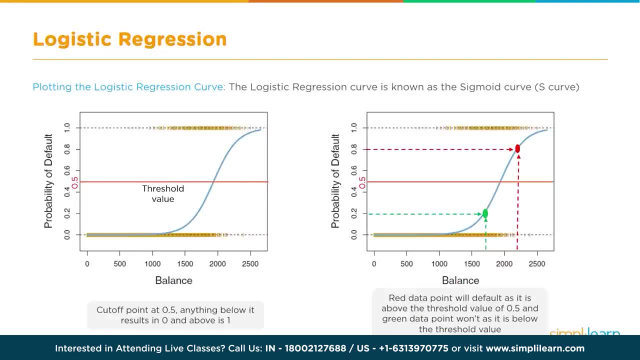 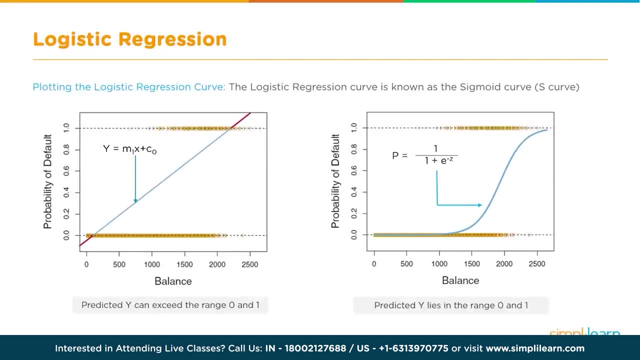 if the value is less than 0.5, we consider the value as 0, because- remember, let me go back- in this case it doesn't exactly give us a 1 or a 0. So we need to keep that in mind. It doesn't. 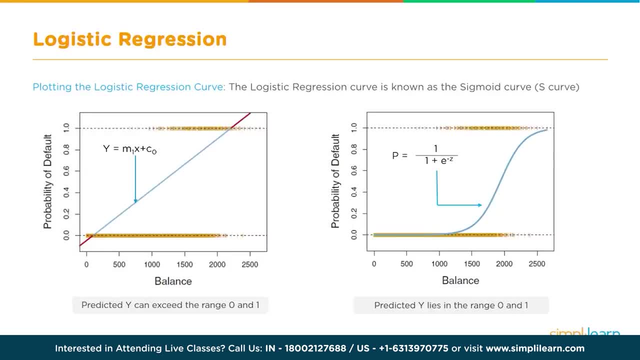 give us exactly a 1 or a 0. It will give a value between 0 and 1, irrespective of what the value of z is. It will give us a value between 0 and 1.. It's like the probability between 0. 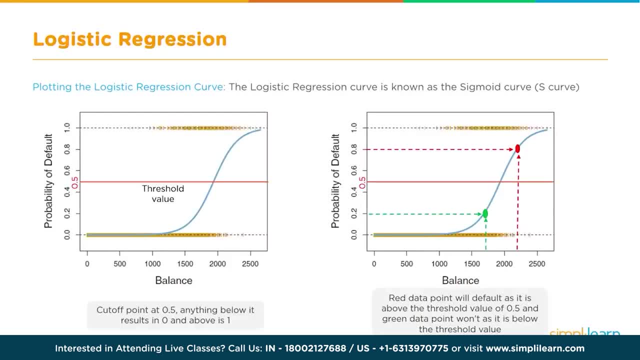 and 1.. Now we have to have a threshold and then, based on what the value is, If the value is greater than 0.5, then we say, okay, this probability is 1, and if the value is less than 0.5, the probability. 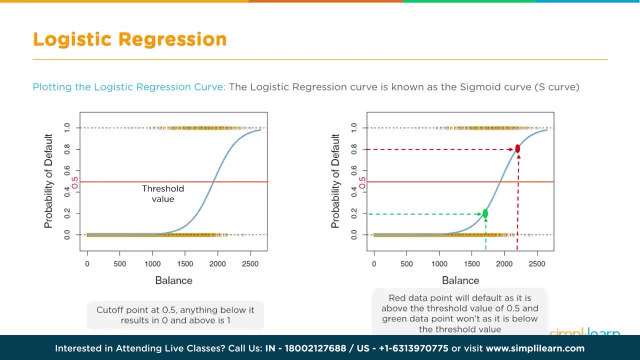 is 0.. So we decide that based on the cutoff or a threshold value. So, for example, we continue on that: If a person having a balance of- maybe this is 1750, then the probability that he will repay the loan is 0.2. 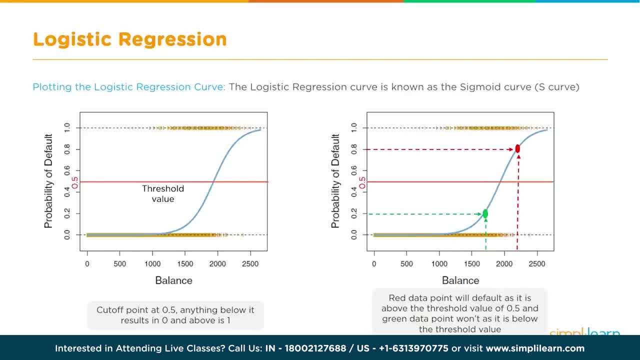 which means which is less than 0.5, the threshold value which we have set, that means the probability is 0, which means the person will not repay, Whereas if the balance is somewhere in the range of 2250 maybe, which is this red dot. 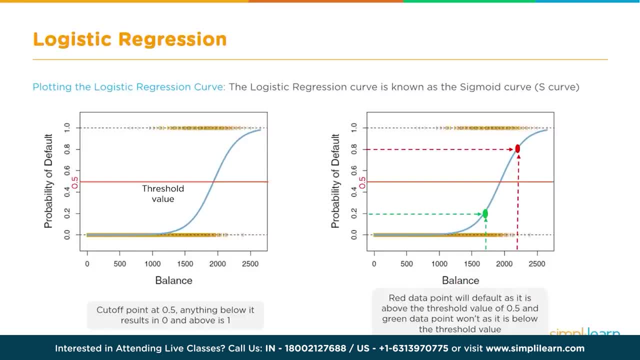 then the sigmoid function calculates the probability of default as 0.8, which means the output is 1, which means the person will default on payment. So that is how the logistic regression works. So in this case it says that, okay, this person will default. It is classified. 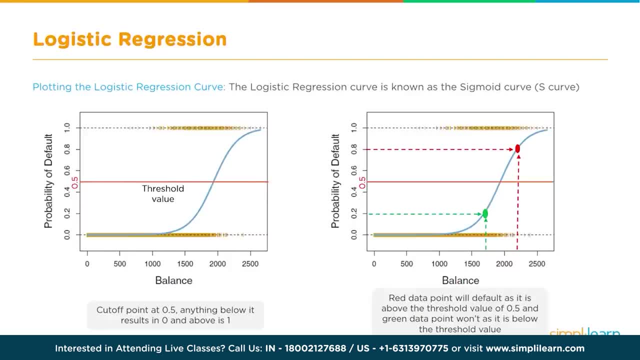 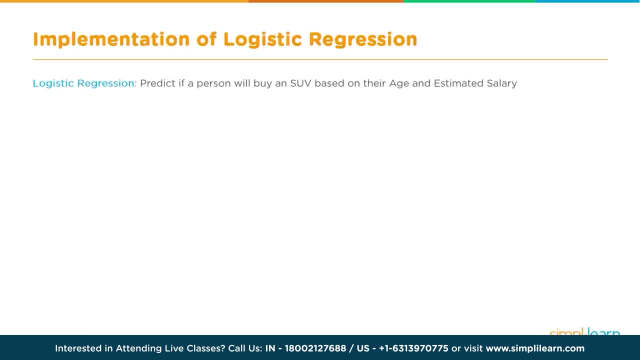 as a defaulter In this case, the second one, and in the first case it is a non-defaulter. So these are the two different classes of these two different cases. So let's move on and see how logistic regression is implemented. So this is another example. 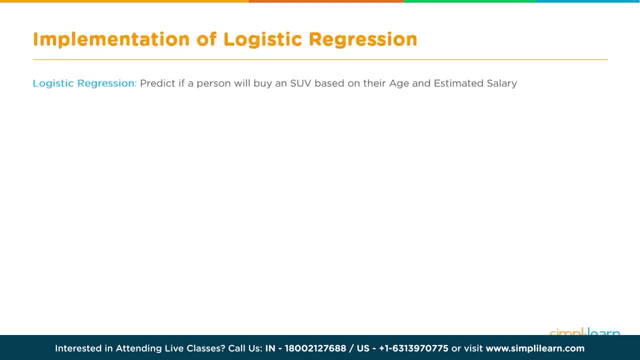 of logistic regression. Can we predict whether a person is going to buy an SUV based on their age and their estimated salary? So these are our two inputs and based on that can we predict whether this person will buy an SUV or not. So this is a logistic. 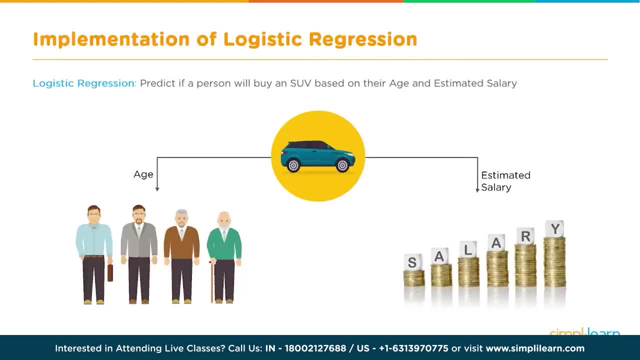 regression problem And we are going to demonstrate this using Python Curd and in Jupyter Notebook. And before going into Jupyter Notebook, let's take a look at how we go about solving this problem and how the code looks. So this is the implementation of logistic. 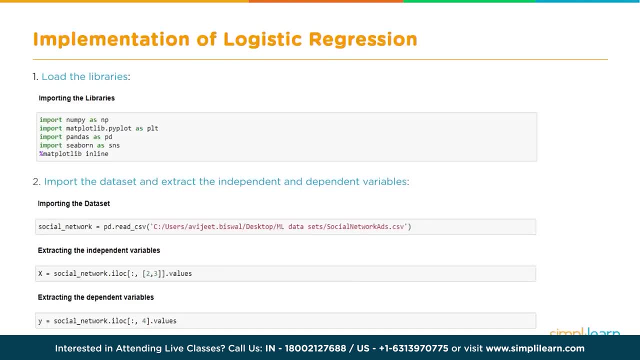 regression. This is the code, the Python code. I just take you very briefly at a high level, what each parts are. So first section, of course, is importing the libraries, and then we import the data set and within this data set, we just take for performing or for training our 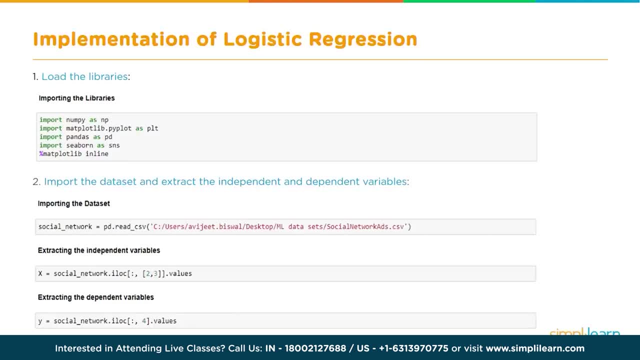 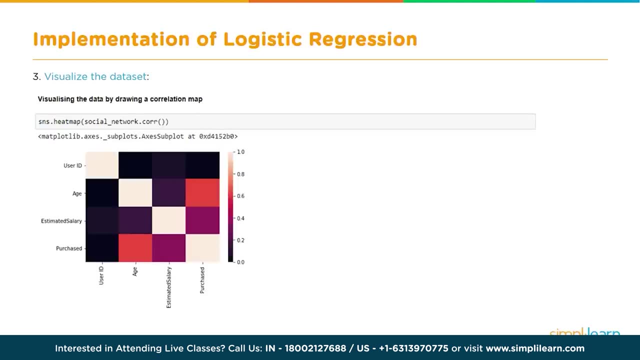 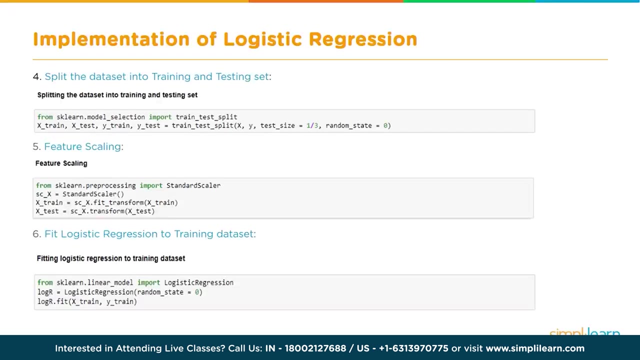 model. we only take the independent variables into one, create one vector and then we extract the labels separately and then we visualize our data. this is how the data looks and then we split the data into training and test set, like we did in linear regression, and we do some feature scaling as. 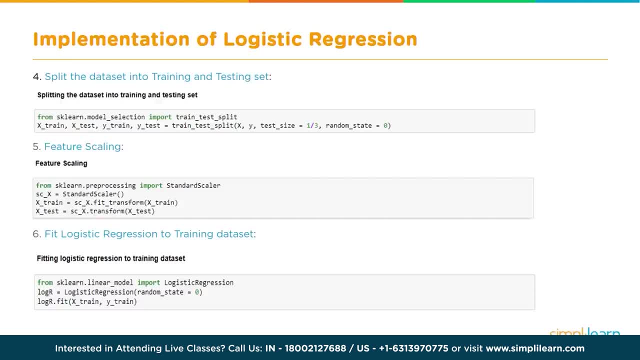 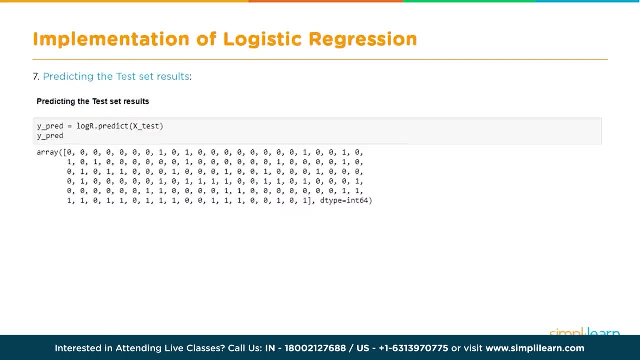 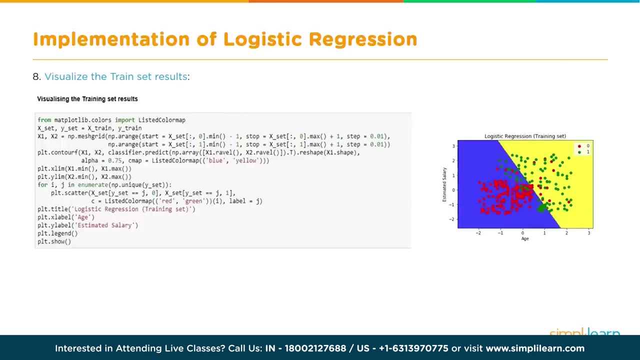 well, which improves the performance of our model. and then we train and test the model. so these are the test results and we visualize the test results. so this is the visualization of the trained results. they look pretty good. the classification: they are reasonably accurately classified: the red dots and the green 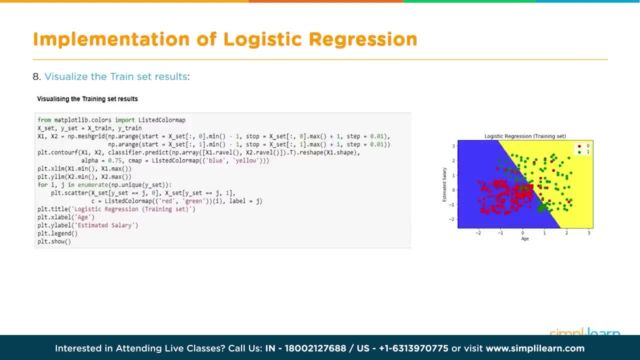 dots and there are a few, of course, miscalculations or misclassifications, but by and large it looks pretty good. and this is the visualization of the test results. again looks pretty good. and then we evaluate our model and this is what we'll be doing in the 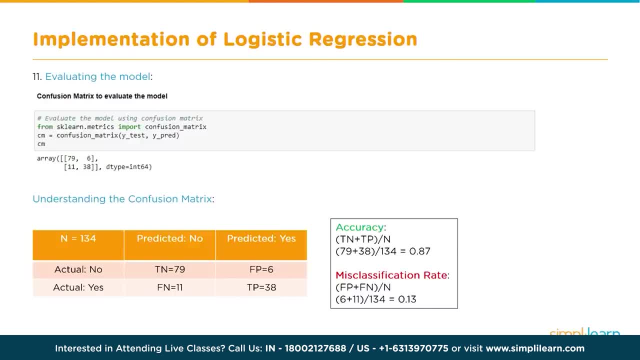 code as well, and for this we use what is known as confusion matrix. now let's try to understand what this confusion matrix is. i know the name itself is confusing, but actually it is very simple. now, once we predict these values and compare with the actual values, we 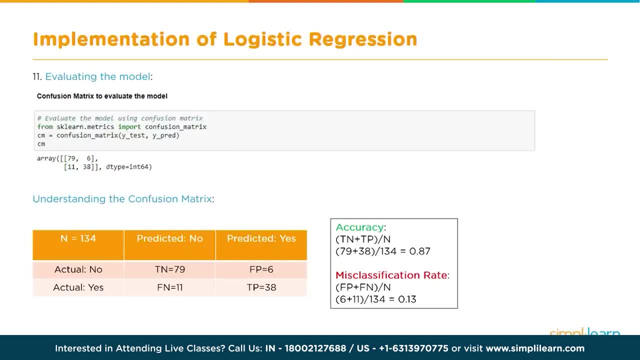 can create or represent the results in the form of a matrix. so we have altogether 34 observations and, if we put it in a tabular form, the predicted values and the actual values. first of all, in order to identify whether our model is more accurate or less accurate. 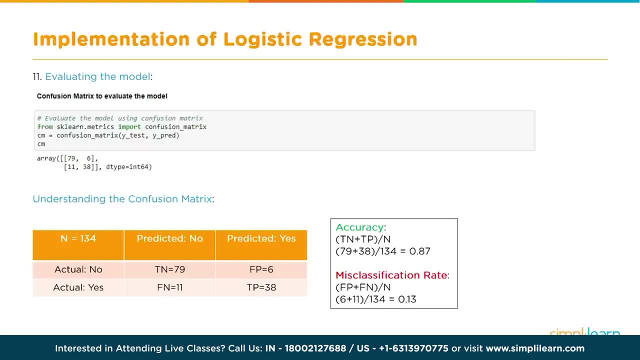 the criteria is that the values along the diagonal should be maximum. so, for example, this is 79 and this is 38. the sum of these should be maximum. so what do we mean by that? that means that if we have a perfect model, then this sum will be equal to 134. 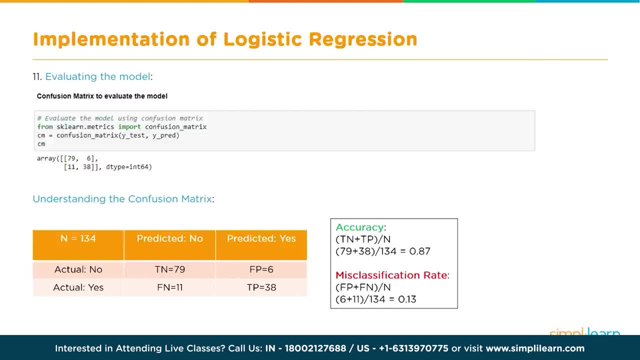 and the values here will be zero. so that is an ideal, perfect, logistic regression model. that is of course very rare, but that is the a. the sum of these numbers are the maximum. numbers should be in the diagonal, and in the other cells there should be as less as possible. 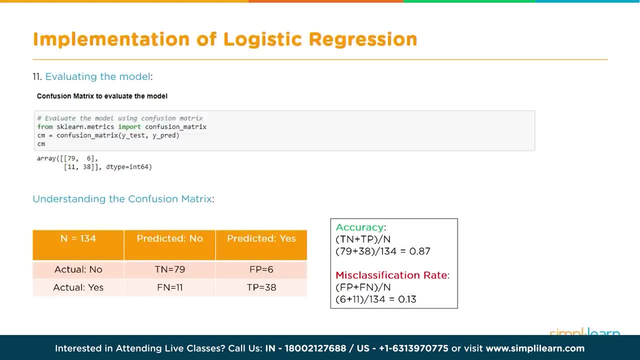 okay. so here we see, in this case that it is 79 plus 38, and so that is equal to 117. so 117 of them have been correctly predicted, which gives us an accuracy of 87 percent. so out of 134, 117 have been correctly predicted, and 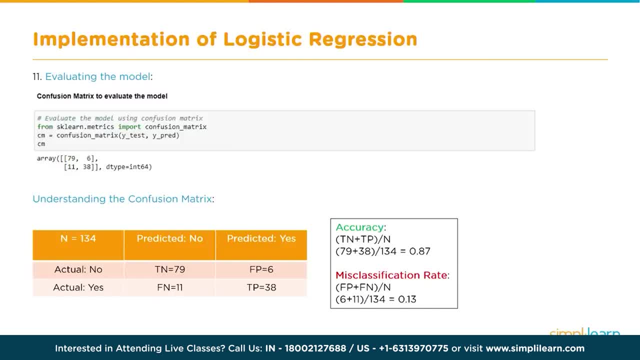 the 6 plus 11. 17 of them have been incorrectly, so this is 6 plus 11. 17 of them have been misclassified, so which is, uh, about 0.13 percent, so we have an accuracy of 87 percent. okay, so i hope the 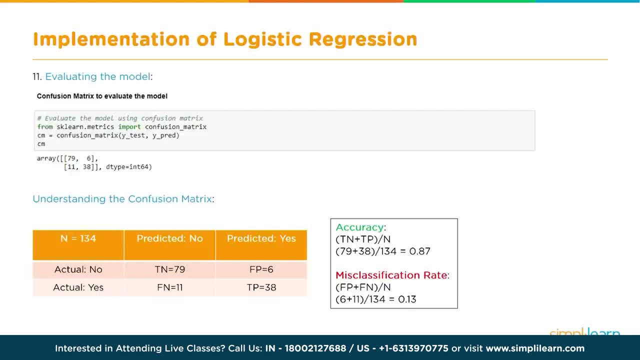 way we calculate or we'll do it in a way. we find accuracy from confusion matrix. i hope it is clear. by the way, once again a quick reminder: if you need this data set to perform this on your own, please put a comment and under this video and we will send you. 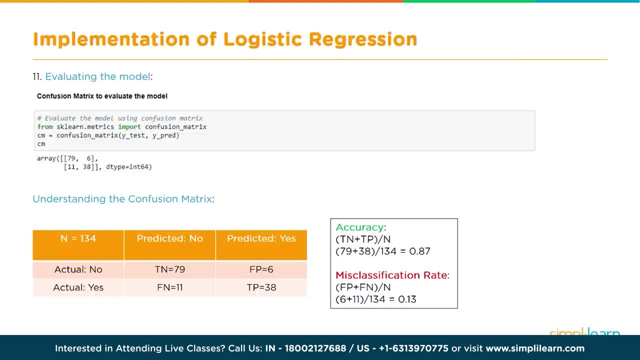 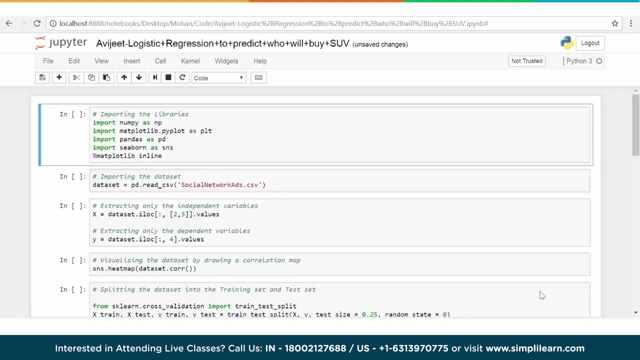 the data set. all right, so let's go and check in python notebook how exactly this is done. all right, so this is the demo of logistic regression, and here what we're doing is we've taken an example of a data set and a scenario where we will predict whether a person is going. 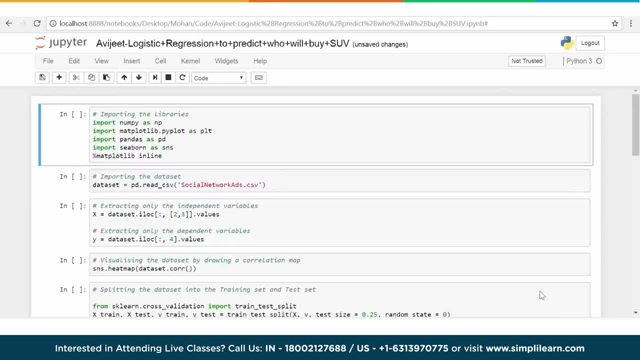 to buy an suv or not, and we will use logistic regression for this, and the parameters we will take are, for example, the person's age, his salary and a few other parameters. we will see very quickly what those are. okay, so the first step: we import the required. 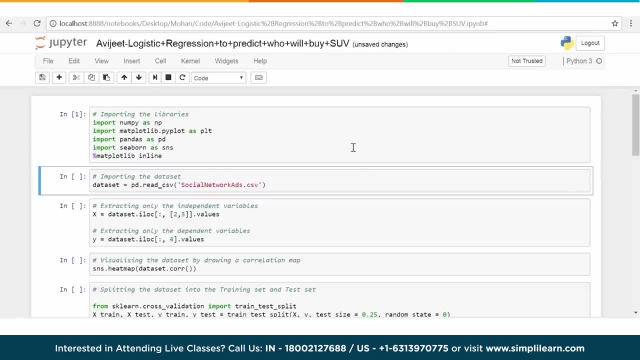 libraries. so that's what we are doing in this particular cell, like, for example, numpy, matplotlib, pandas, so for performing any preparation of the data before we actually launch into the learning process and then we load the data. so let me just introduce one more cell and see how the data looks. so why don't? 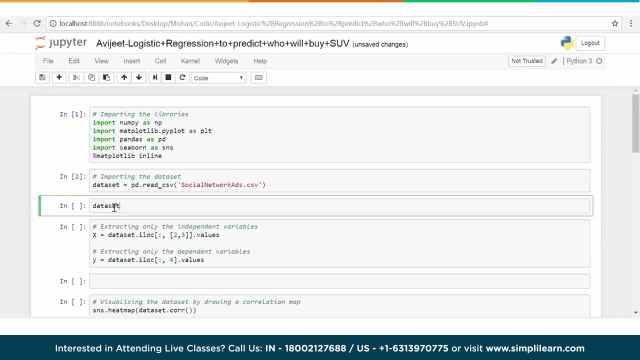 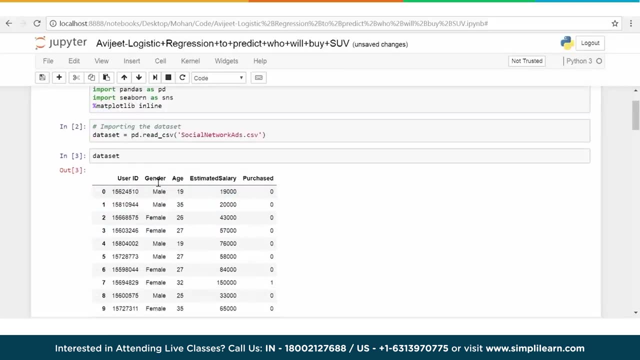 we do that here, and if i say data set and then if i run this, this is how our data looks. so these are the parameters, or the features, as we call it in machine learning language. we have gender, age and estimated salary. user id is also there, but 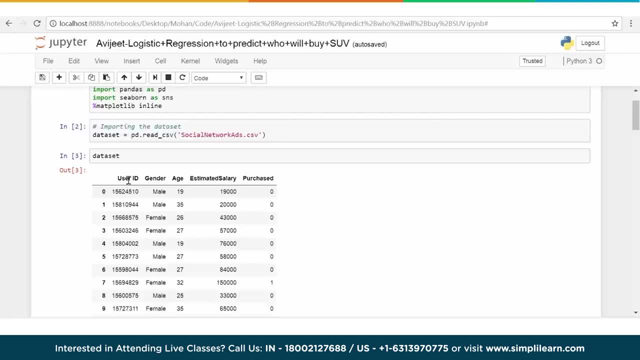 it's not really a feature, it will probably not contribute, so we will not be using this. we will primarily be using these three columns, and in technical terms these columns are known as predictors. and then we have the labeled value. this is known as our target and in this is the labeled 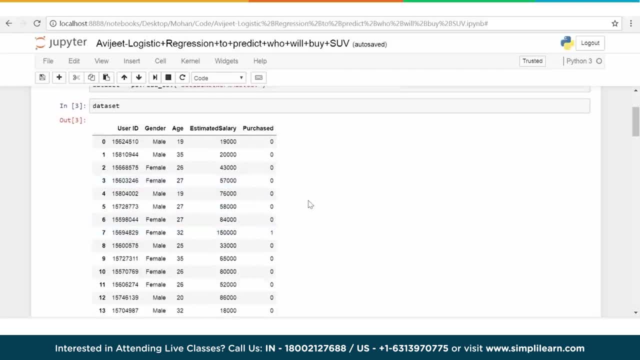 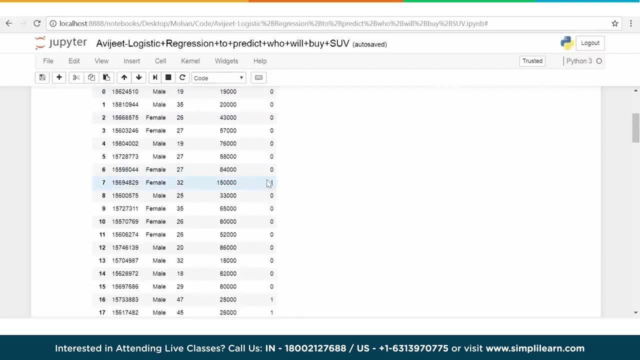 value, so it has zero or one. so we are basically performing a binary classification- zero or one- whether the person will purchase or not purchase. zero means he will not purchase, one means he will purchase. okay, and the. the other way of also looking at it is from a more from a mathematical way of 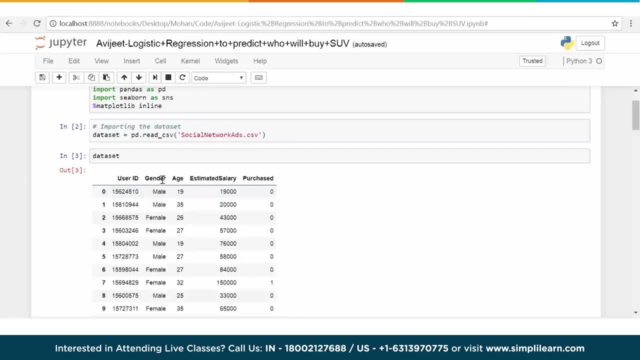 looking at it from a mathematical perspective, these are our independent variables. gender, age and estimated salary are our independent variables and purchased is our dependent variables. so in our equation, like, y is equal to something, something 1x plus m2x and so on, this is our y. 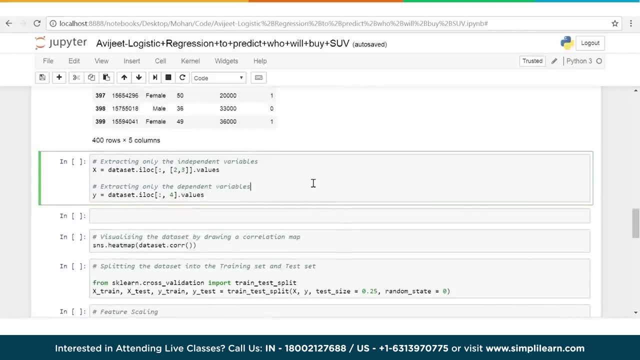 okay, all right. so now let's move forward. what we will do next is to extract this, the, or separate out the independent variables and the dependent variables. how do we do that? so we load them into x, capital, x and y, and what we are doing here is we are 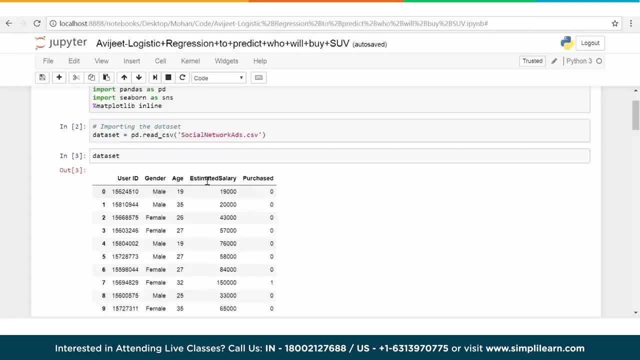 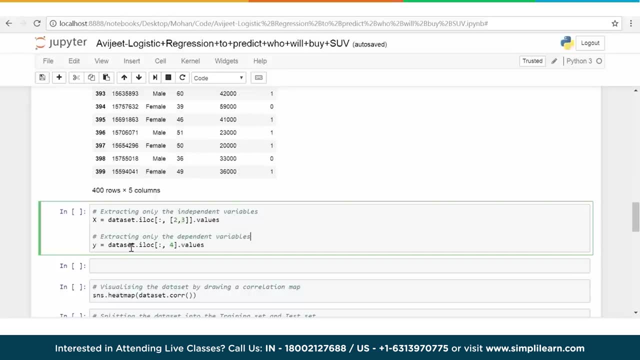 taking the second and the third column. we are taking these three right. so gender, age and estimated salary. so that is what we are taking here: two up to three, and then y is basically the last column, which is the fourth column. so let's go ahead and extract. 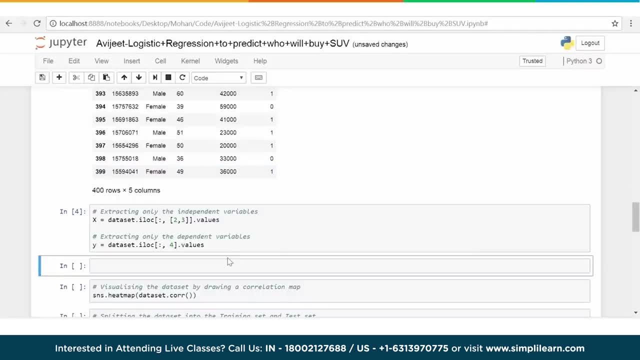 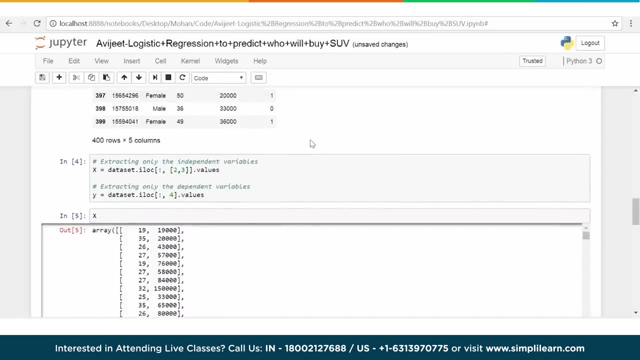 that? and, once again, why don't we take a look at how the data is looking? so let me just print x. so we only- yeah, we are basically taking two and three. so what is two and three? two and three is our age and our estimated salary. yeah, that's. 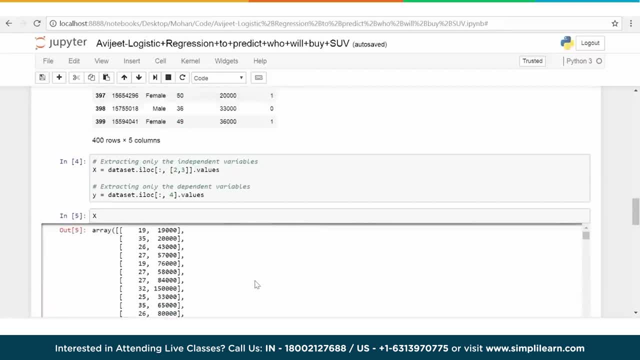 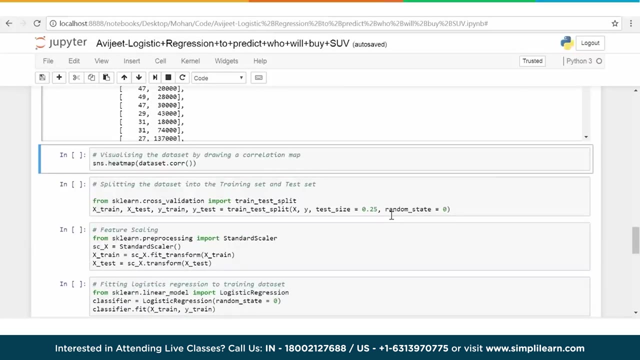 right, so these are the only two independent variables, and our dependent variable is obviously the last one, whether the person will buy or not. okay, so we have the data loaded now. let's now that we have the data in python, let's take a quick look at how. 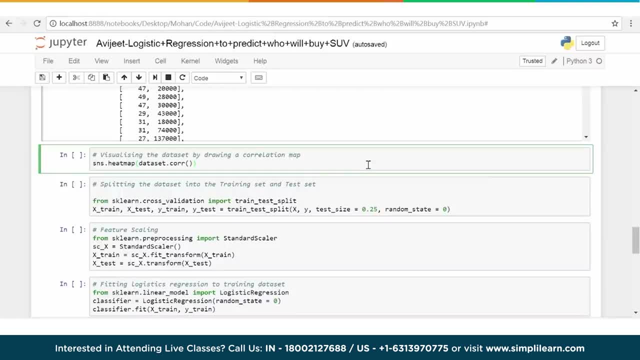 the data looks. so, in terms of visualization, let's visualise the data and perform a little bit of what is known as exploratory analysis, right? so, as a data scientist, whenever you get new data, you just play around and see how the data is looking before you actually launch into. 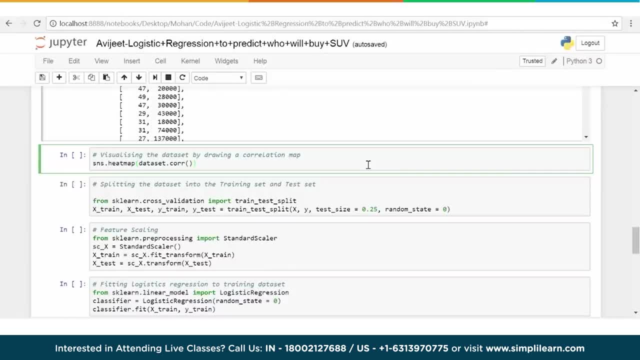 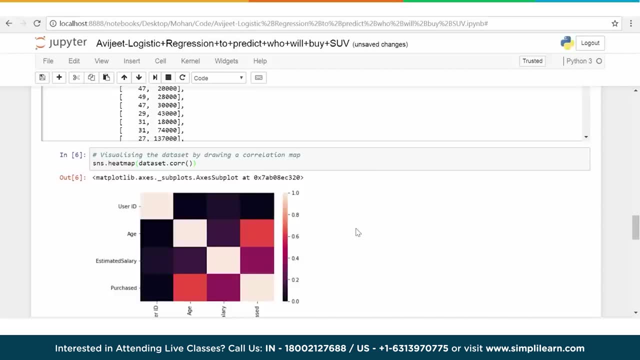 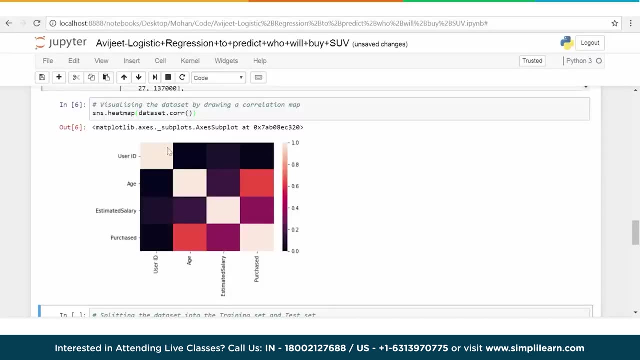 the actual training or the modeling part of it. so let's run a small heat map and see how the data looks. so we have just passed the entire data set here and this is how the heat map looks: how, how they are related, how the various what you call uh features are. 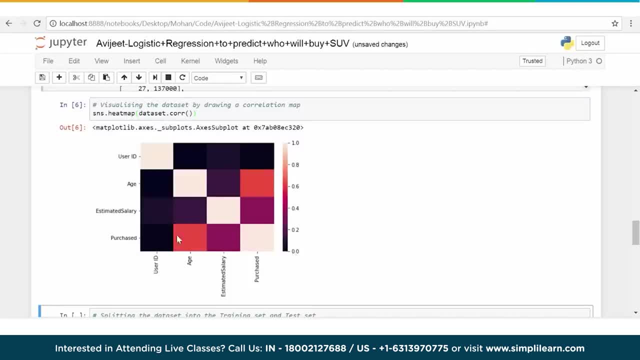 related to each other and this is a scale. here, very dark means basically there is a pretty much no, no correlation. this is, in a way, to measure the correlation as well- and light means there is a very high correlation. so, as you can see, a value or a feature will have very high. 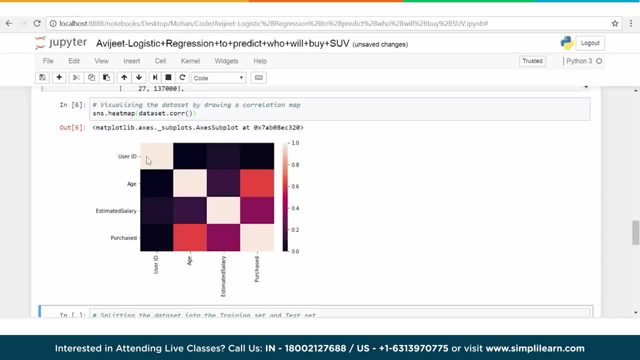 correlation of one to itself. so the user id- and this is user id- it has a very high correlation to itself. similarly purchased and purchased it has. so the diagonal will be very high. so that is really not relevant. but then the other values is what we have to see. For example, there is a correlation of 0.6 in this. 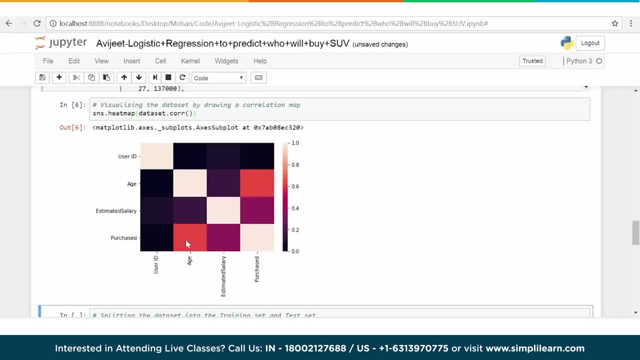 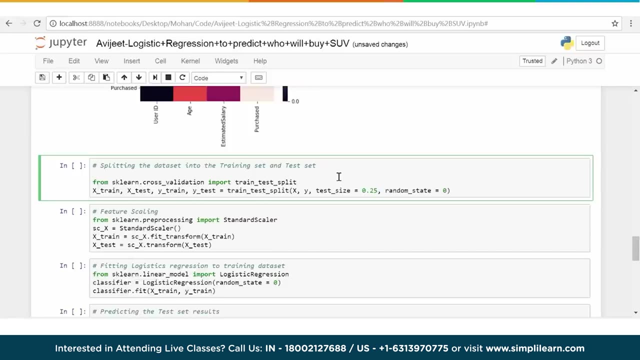 area, which is basically, if you take age and purchased right, whether the person has purchased and the age. So that's, that's a quick look at exploring the data. So that's all we are doing here. Here's where the actual, the crux of this code is. So, from here on, what we do is the first. 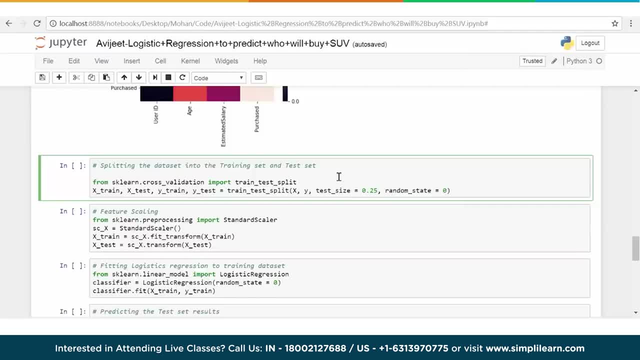 step before we start the training process is split our data into train and test, training data set and test data set. So whenever we perform any machine learning activity, we have, let's say, our label data. we never pass the entire data to the model, Because when we are, then when we are. 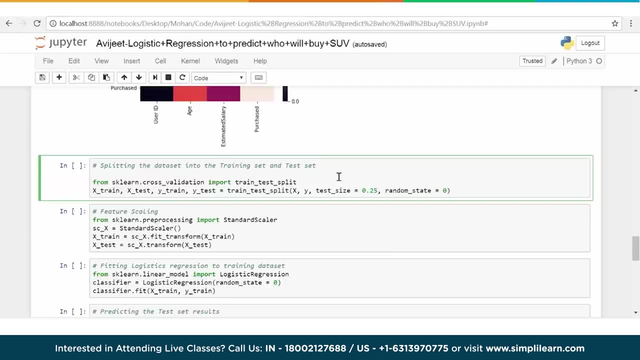 measuring the accuracy, whether the model is performing well or not. we will not be able to do that if we use up the entire data for training purpose, So we split the data into what is known as a training data set. We train the model with the training data set And 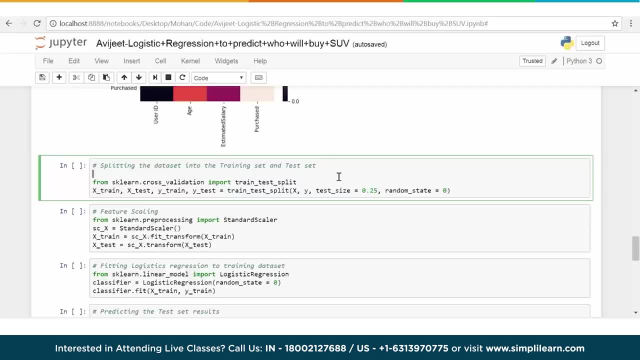 then this test data set, which is kept separately, which the model has not yet seen. We use that to check whether it is able to identify, perform the predictions correctly or not. Okay, That will give us a higher accuracy or or a better estimate of how the model is doing. All right, So this is a 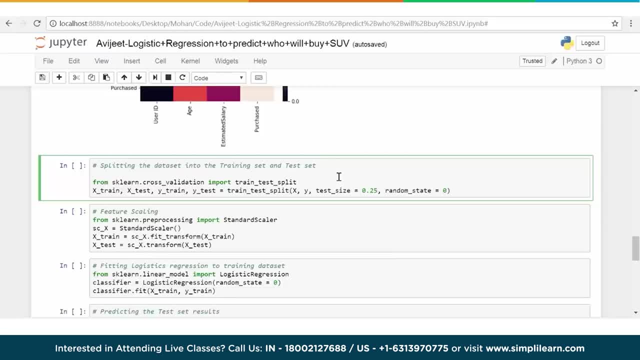 very common practice in machine learning. So whenever we have, whenever we perform training of the model, we split the data into training. Now, how do we do this? We don't have to write any special code. There is already a method available. 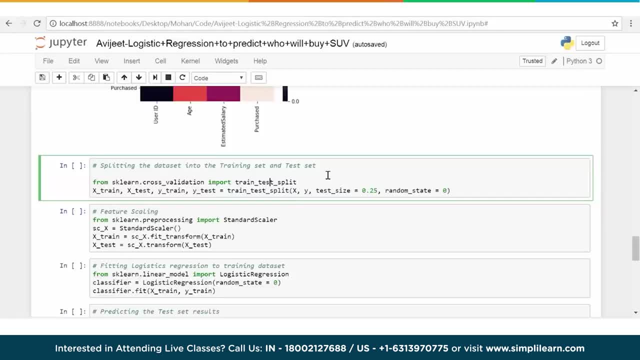 which is train, underscore, test, underscore split, And we just call this method. Only thing is it takes these parameters and we have to specify especially this parameter which tells the, the method, how the data should be split. Now, when we are splitting the data into training and 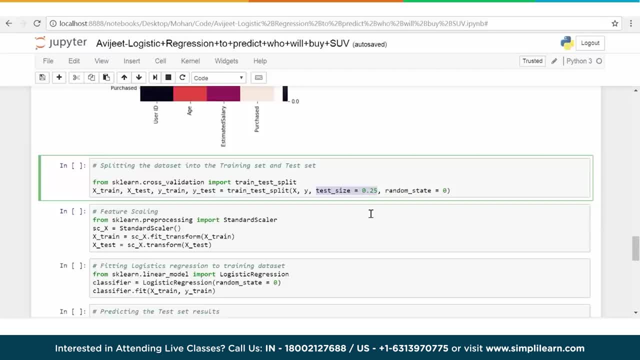 test. there are no hard and fast rules how we split this data. Some people prefer 50, 50. Some people prefer 80, 20, and so on and so forth. So that is flexible And it could be to some extent. 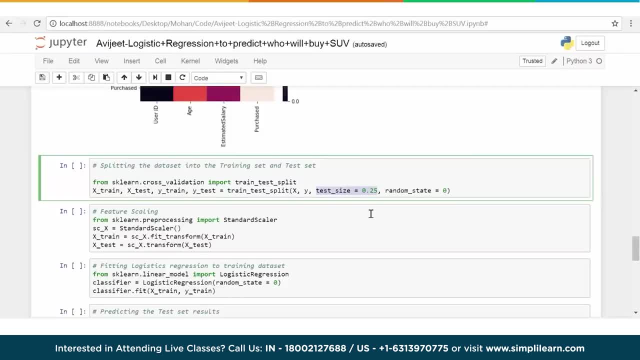 individual preferences. So in our case, we are splitting this data into 75, 25, which means 75% of the data will we will use for training, 25% we'll use for test. So that is what we are specifying. 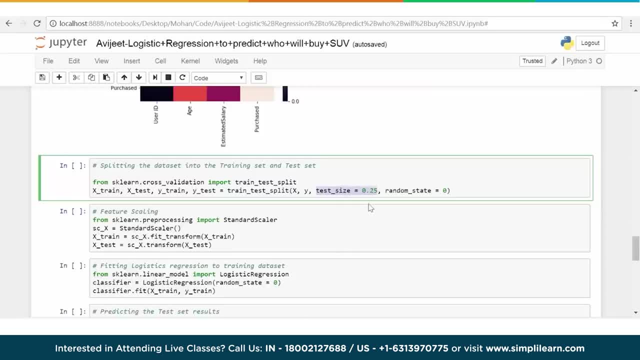 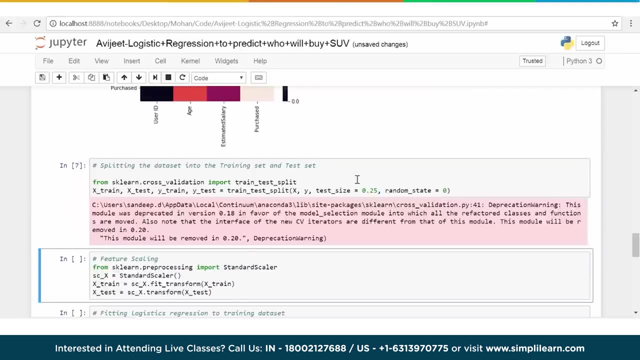 here. as a parameter, We say, test underscore size is equal to 0.25.. That means put or keep uh, 25% of the data set aside, 25% of the data as test data And therefore the remaining 75% will be used for training. All right, So let's move on. I execute this, Then we perform. 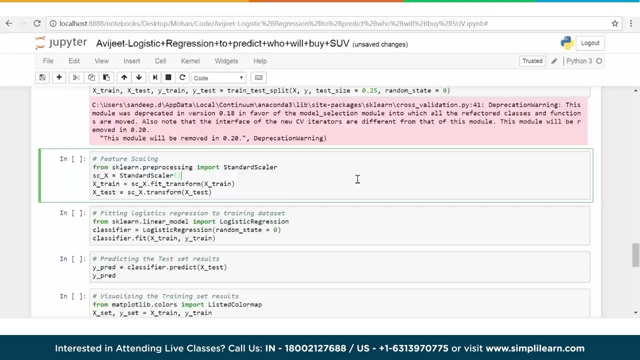 what is known as feature scaling. So what is feature scaling? Usually, what happens is, uh, the, the values that we have in the data. sometimes they can be, uh, some numbers will be very large, Some will be very small, So th? th, there is a huge variation. So, in order to, if we have that, 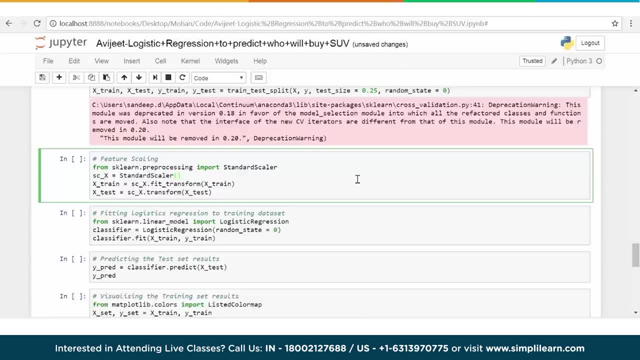 and if we use that as it is, the accuracy of our model will come down. So we have to somehow normalize these values. So that is what scaling does, feature scaling does. And, uh, again, we don't have to write any special code for this There. 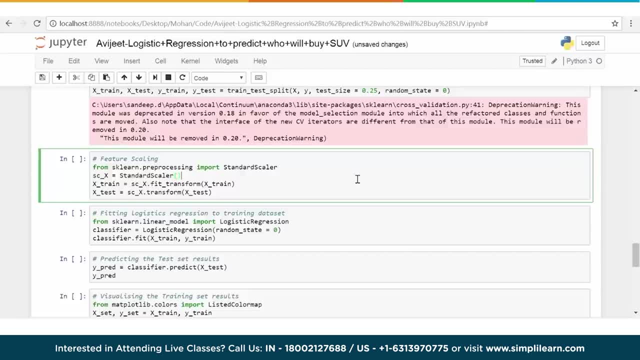 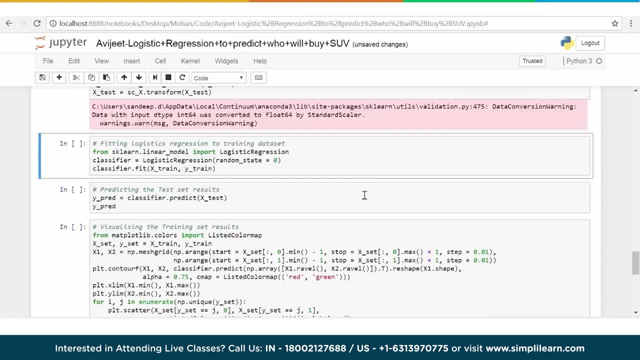 is a standard method, uh available or standard class available, called a standard scaler. So we just create an instance of that and pass our data for scaling purpose. Okay, So let's go ahead and do that now. So this is all. what we have done is more like a data preparation. So we, we chose. 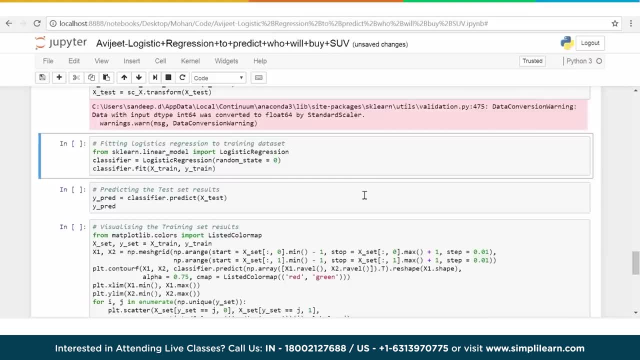 what are the parameters, what features we want? We did the feature scaling and we split the data. Now everything is ready. Next is to to start the actual training process. So this is the most crucial part of the code. So here, as we said, we will use the logistic regression model. 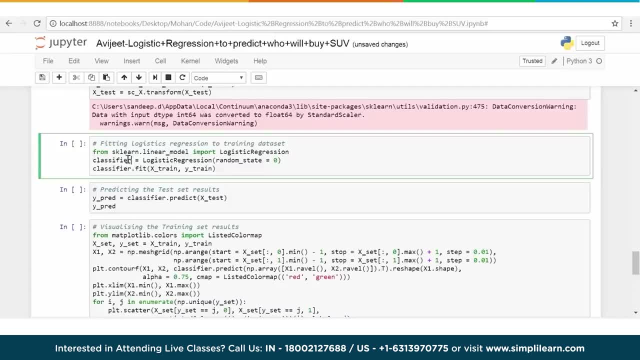 So we have to create, we create an instance of regression model. So I call that as classifier. You can give any name and um, we just do some kind of a initialization. random value initialization- so we call this as a random state or we assign it as a random state- is equal to zero And we 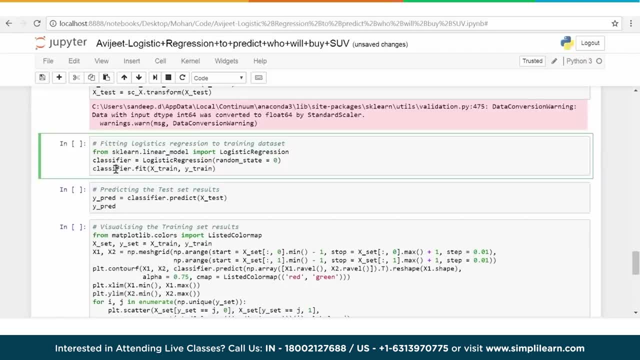 we have an instance of the logistic regression model and we use that model, the fit method. So any, uh, any algorithm that we have when we want to perform the training, um, we have to use the fit method. Okay, We call the fit method. Now let's say: 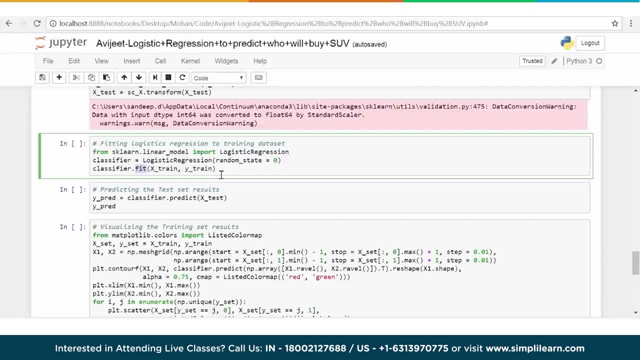 instead of logistic regression we are using k uh, k nearest neighbors algorithm. you will have k nearest neighbor, dot fit or linear regression. linear regression, dot fit, right. So that is where that is the way it works And we pass the training data set, the x. 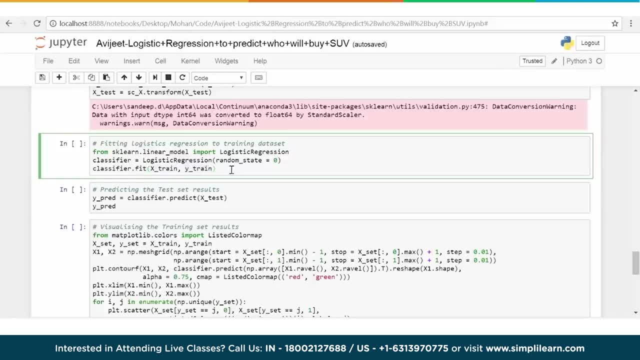 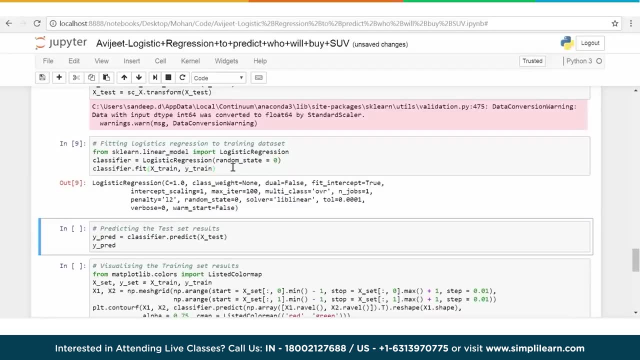 is the independent variables and y are the labels, So we pass both of them for the training purpose. So once the training is done, we get the results of: or the model is trained. okay, the model is trained Now. the next step is to test the model, how well the model is performing. This is where 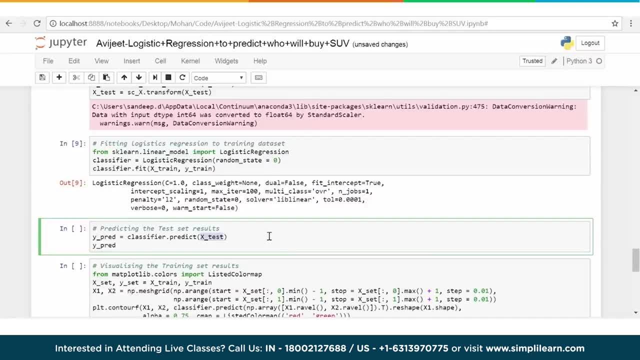 we use the test data set, we pass the test test data set, And here there is a another method that we have to use that is known as a predict method. So again, this is a predict method is common across all algorithms that we have. So any algorithm we have, we have to call the predict. 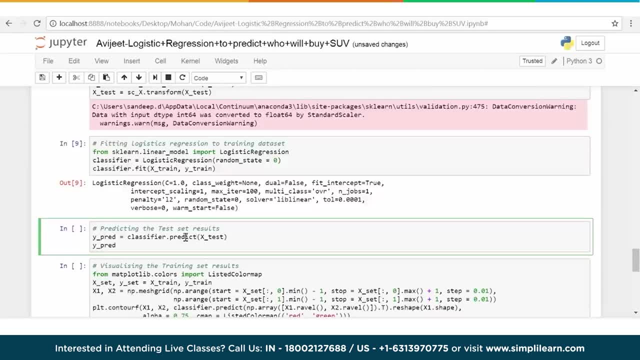 method for performing the test or even when we deploy it. when new data comes in, we are trying to predict for new data set. we always use predict. okay, so fit is only for the for training. okay, then predict is used for testing and for the actual performance of the prediction. 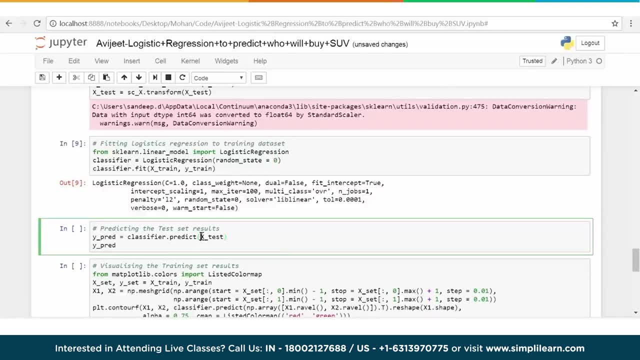 Now, one thing we need to observe here again is we only pass the x part of it and not the y part of it. So this can always, sometimes this can lead to confusion in when we are calling fit, we are passing x and y. when we are calling predict, we are only calling x. The reason is: 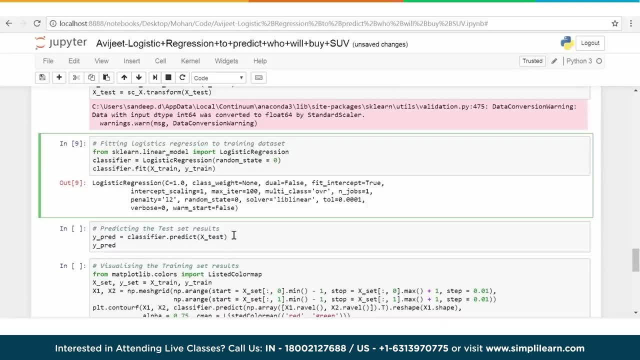 the y part. That is what the model will predict, So you don't have to pass the y part, right? So y is what the model will predict for us, So you don't pass here. we had to pass it because the model has to learn from the existing values, So that's why we had to pass label as well. 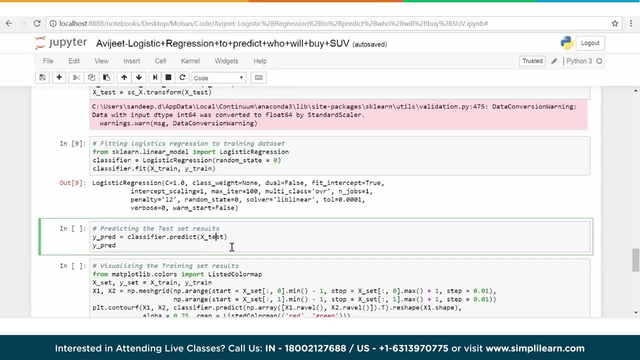 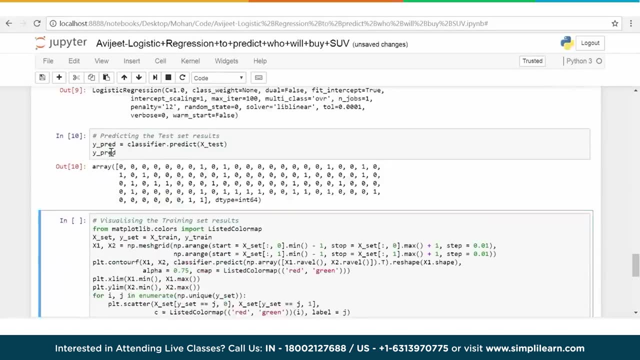 But when we are testing it, the model will calculate this, And that's the reason we do not pass the y value. Okay, so now when we run predict, it will calculate those values or find those values, and it will put it in y. 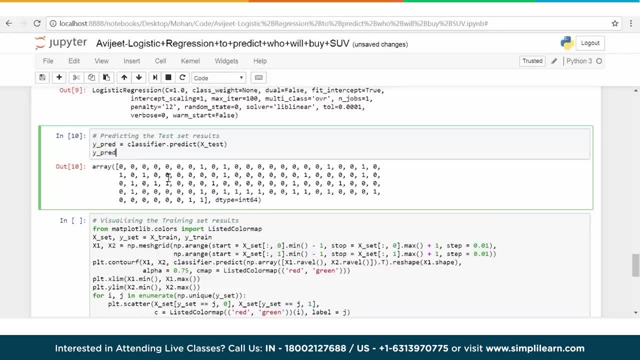 And that is what is being displayed here And, as you can see, the values can be either a zero or one, which means the person will buy the SUV, which means which is one, which is which is a value of one, or zero means the person will not buy the SUV. Okay, now, 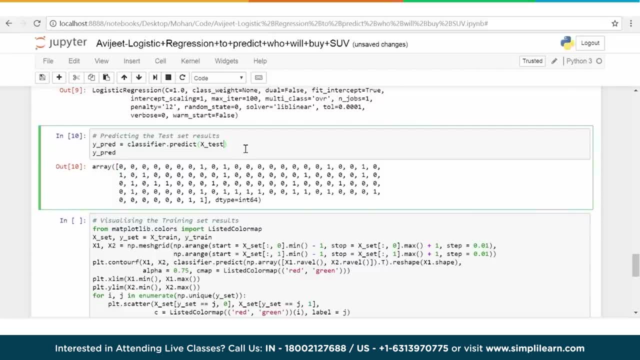 one more thing we need to remember is, while we have not passed the y values or the labels to the system, but we have these labels available with us. right, y underscore predict, So y underscore test is available with us. that is what we have to use to find out how accurate. 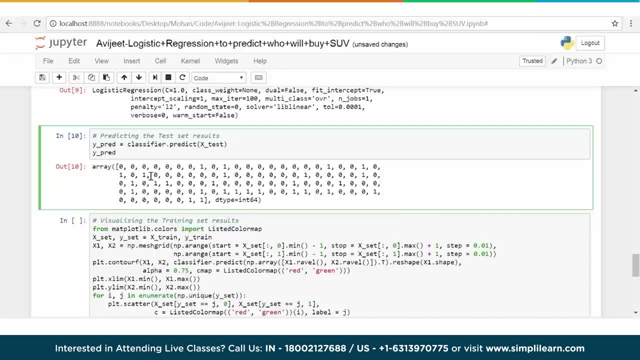 the system is So. it has given us the results. Now we will compare these results, which the system has predicted, with the actual values that we have, which is available in y underscore test. So we will see how well, how that is done, how that accuracy is calculated in a. 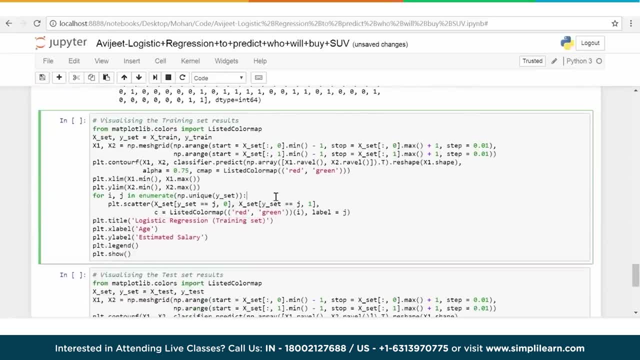 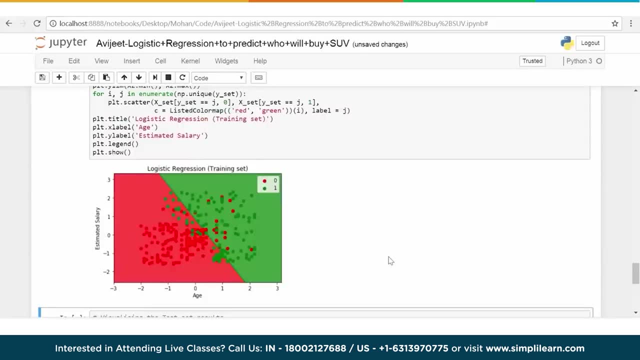 little bit. Okay, now that the training is completed, we can go ahead and do some visualization of the training results. So let me execute this code and take a look In a form of a plot. So this is how the classification is done. So these are like the class this: 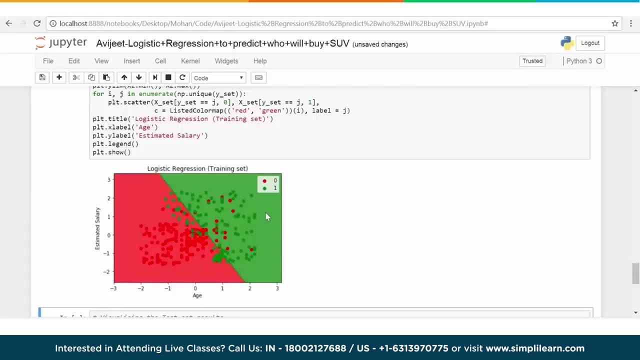 is like the class boundary: the green color belongs to the class one and red color belongs to class zero, And these dots indicate it has been misclassified. So some of them have been misclassified. So that's what we are seeing: some red dots in the green area and 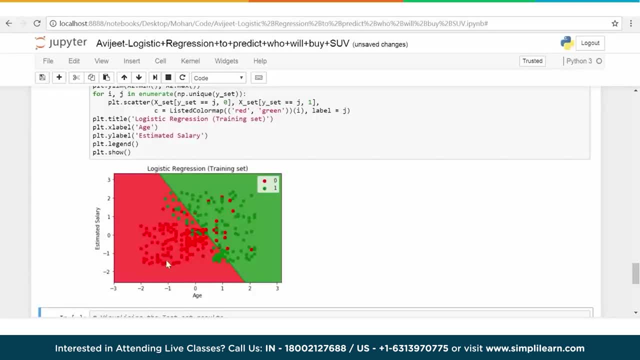 some green dots in the red area right, Whereas, if you probably it's not very clear, but you can see here that there are also red dots in the red area and the green dots in the green area. So those are the data points which are correctly predicted And these in the opposite locations. 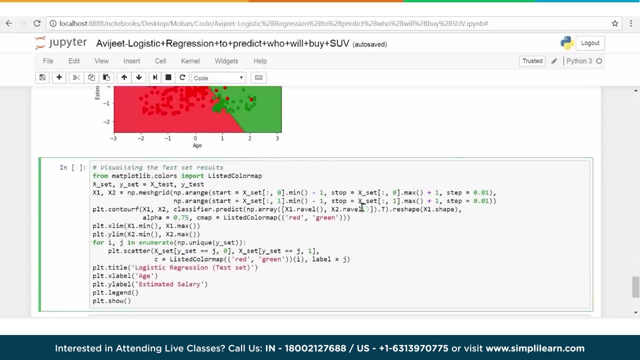 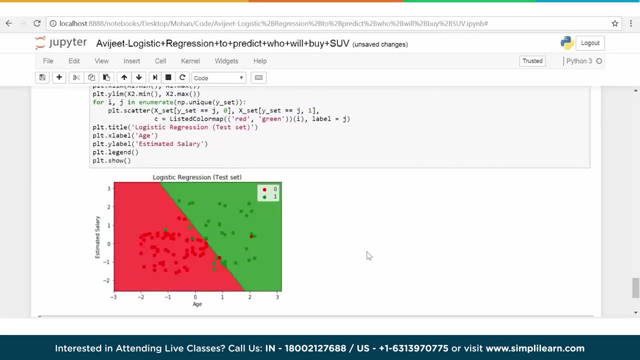 are the ones that have been misclassified. rather Same for test as well. So test data set also. if we visualize, we plot, we will see something similar, But this also gives a at a high level. whether is that a major in a major way? are there major misclassifications? 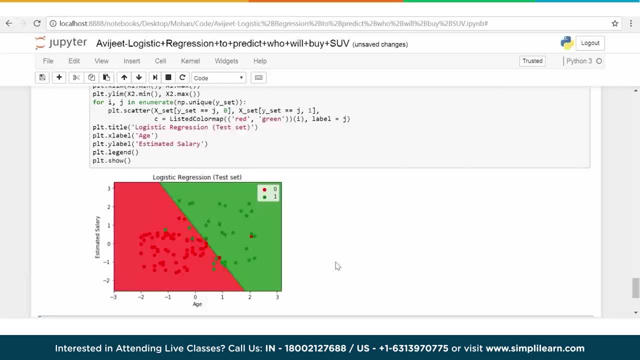 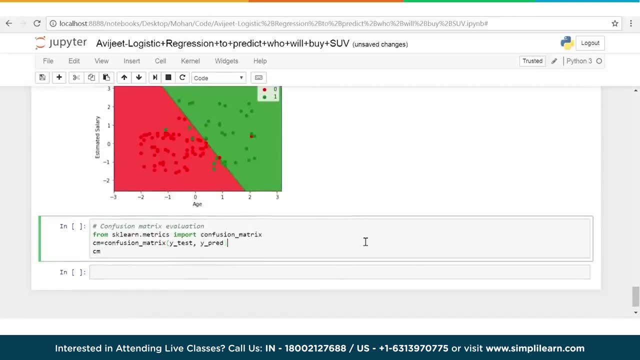 Or there are particular things, or are there mixed misclassifications. So in the case of a test like this, it's a very simple thing. There are so many more things to be analyzed. So the first thing we do is we get the data points and we get the piece of information and we get the values. 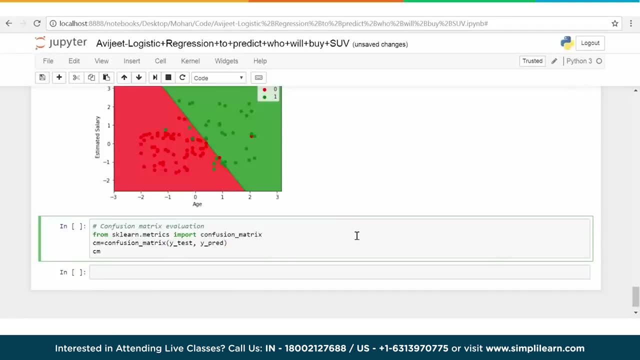 for each of the test as well. So we get the value for the test. So from here we have the values for each of the test. So, for example, if this is the number of tests and we have the number of tests in this particular test, we get the. 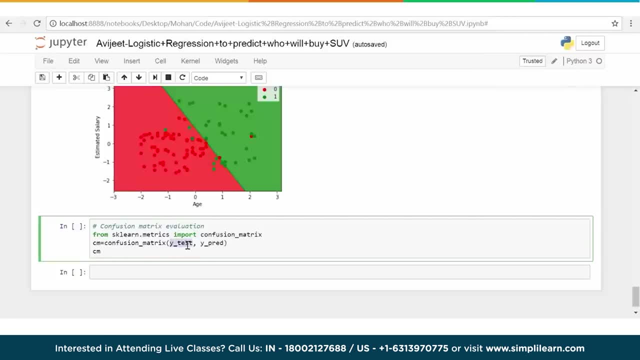 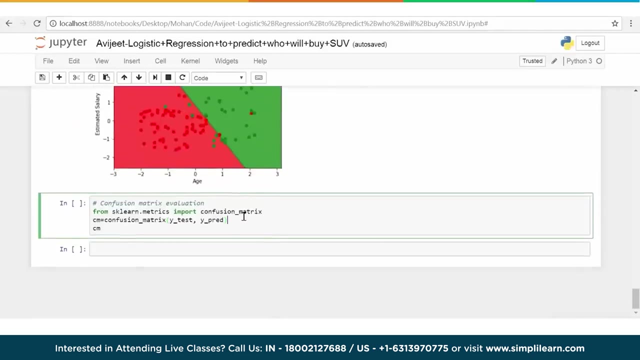 number of tests, labeled value or label data set and this is what is predicted by our model. okay, y underscore pred is predicted. are the predictions. these are the values of here we saw this is y underscore pred. okay, so we we pass these two parameters and we create a matrix, and this matrix is known as. 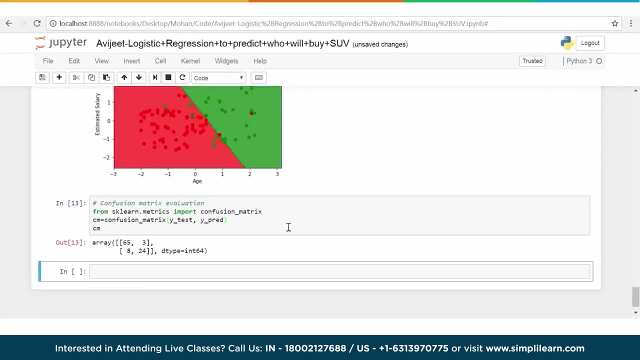 confusion matrix. now, what is the significance of this? first thing is that the total number of values here is equal to the number of data sets in your test data. okay, so let's go ahead, and in the next cell, let me just add up these values: so 65 plus 3 plus 8 plus 24, so how many? 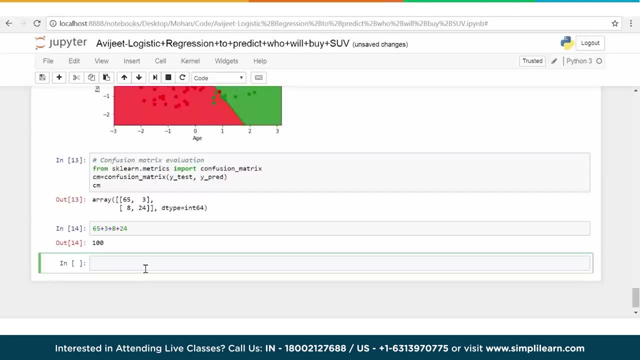 are there. there are 100 in number, so there are totally 100 observations in your test data set. that is the first point. then the second point is the number in the diagonals right, the total value in the diag diagonals. if that is a high that indicates a higher accuracy, the higher that number is, the 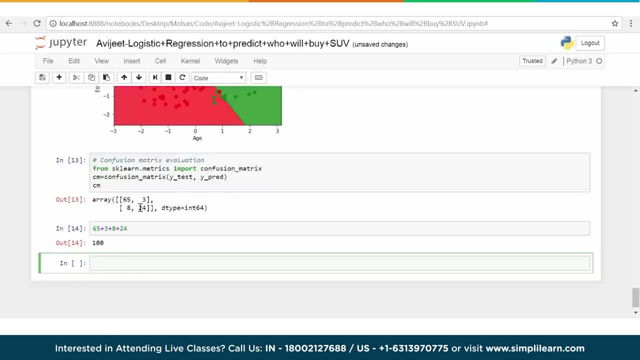 total in the diagonal, the higher the accuracy. okay, and if we have quite a few numbers non-diagonal locations, that means accuracy is not very high. so here looks like the accuracy is pretty good. now we can actually quantify the accuracy by using these numbers. so what we do is the sum along the 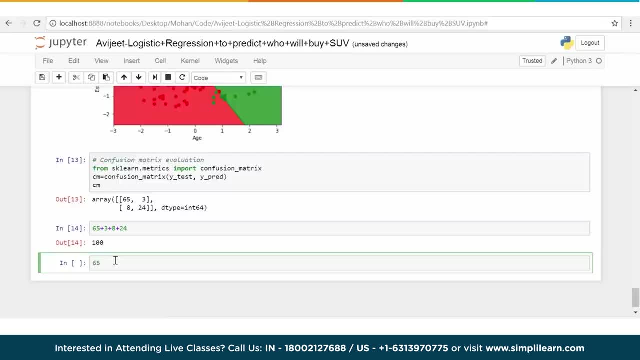 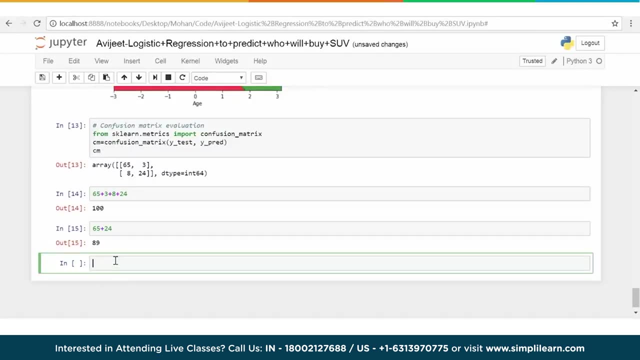 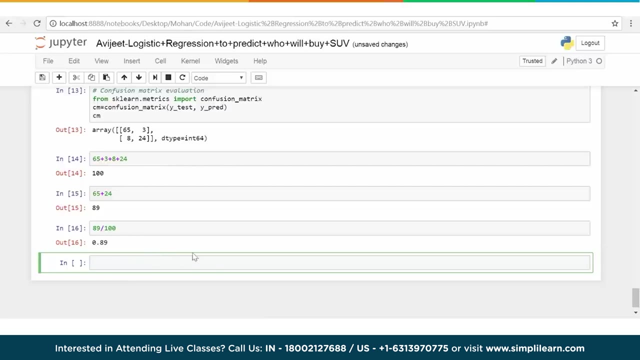 diagonal. we have to take and divide that by the total observation. so 65 plus 24 is what we have along the diagonal and we have 100 observations. so 89 by 100 is our percentage. so we got about 90 percent accuracy for this particular model. okay, so that brings us to the end of this demo. 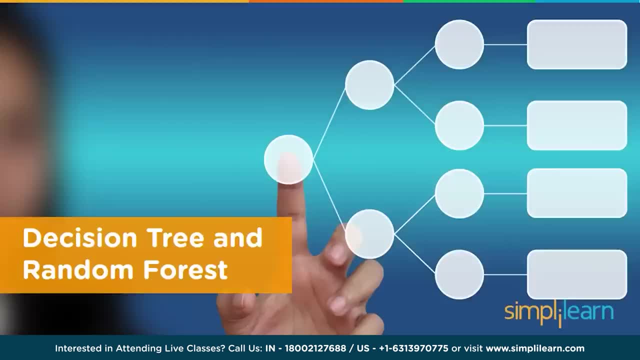 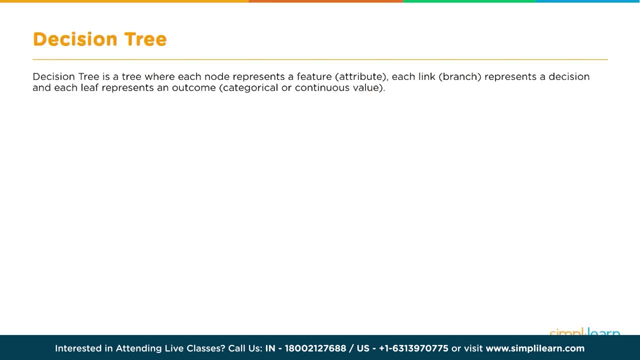 and we will move on to the next demo. all right, so the next algorithm is decision tree algorithm and random forest. they are being taken together because they are very closely related. so what is a decision tree? decision tree is another algorithm and, unlike logistic regression, which is only used for binary classification, decision tree can be used for 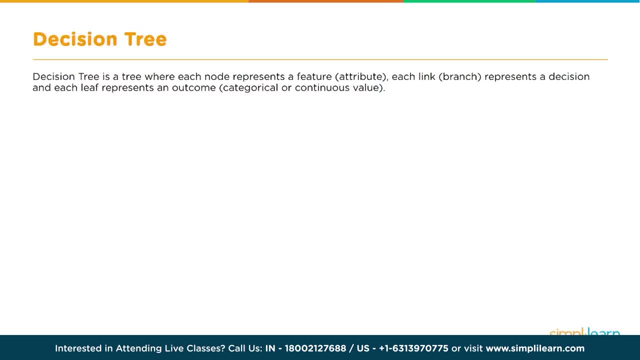 classification as well as regression, even though it is more popular for classification, and it can be used to classify multiple classes as well, not just binary classification. so how does decision tree work? one of the good things about decision trees is that it is easy to represent and show. 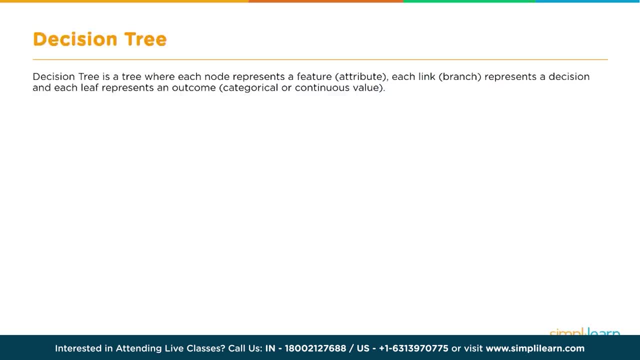 how exactly it works and therefore it is very easy to understand as well. now let's take an example. let's say a person receives a job offer and he needs to decide whether to accept the job offer or not. so we will use decision tree to come to the decision to accept or not to accept. so this: 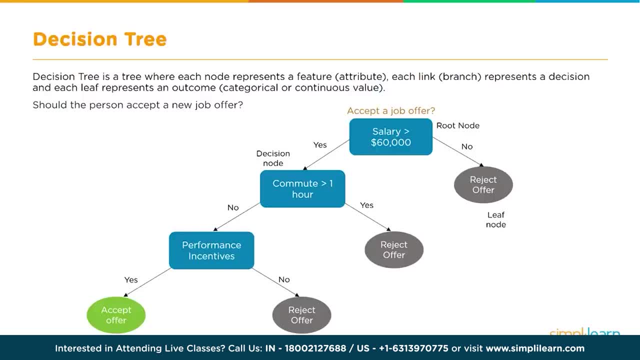 is how, first of all, a decision tree looks. it is actually an inverted tree. it is an inverted tree, so the root is at the top, okay so, and that is known as the root node. the node where the tree starts is known as the root node. and then we have some inner nodes, or decision nodes, and we have the 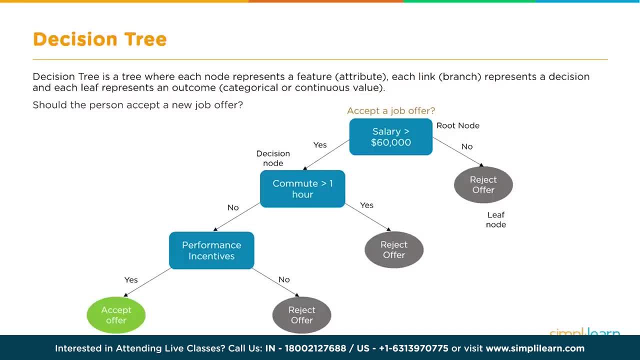 nodes where we have a decision, either positive or negative. these are known as leaf nodes or terminal nodes. okay, so we have the root node and we have leaf nodes or terminal nodes. there can be multiple of them and in between we have decision nodes or internal nodes. there are different terms used so need not be hung up. 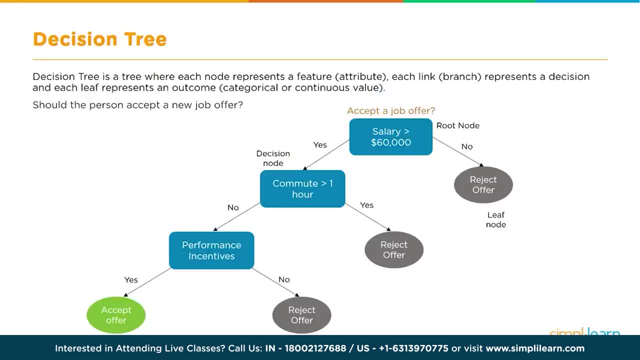 by the exact terminology. now, let's say, we have to use this decision tree to find out whether this person will accept the job offer or not. so first thing he considers is the salary. is the salary greater than 60 000? if no, it's a clear decision: the offer will be rejected. so we reach. 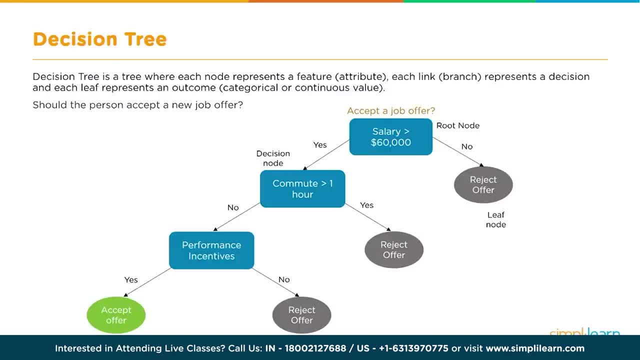 a decision. therefore, this is a leaf node. now, if the salary is greater than 60 000, it is not a clear-cut decision because there are probably other factors based on which the decision needs to be made. for example, what is the commute time? if the commute time is greater than one hour, then the is rejected, okay. so even though the salary 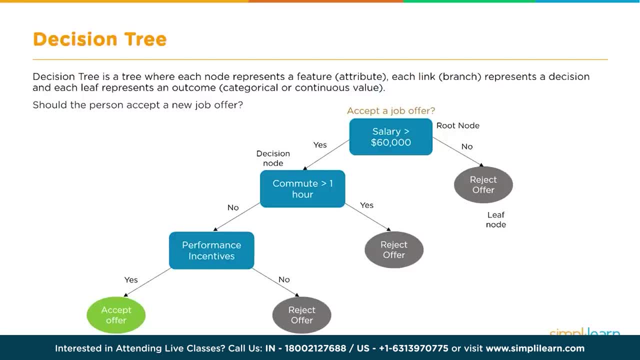 is greater than 60 000. so this is again a leaf node. if the commute time is less than one hour, still it is not a confirmed decision because there are still a few other factors, for example performance incentives. are there sufficient performance incentives as a part of this offer? 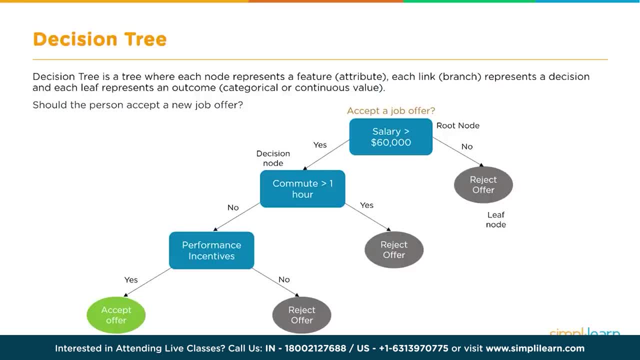 if no, then again the offer is rejected, and this is another leaf node. if yes, if there are sufficient performance incentives, then the offer is accepted. so this is another leaf node. by the way, keep in mind that these are all the leaf nodes. this is a leaf node. this is a leaf node. this is a leaf node. 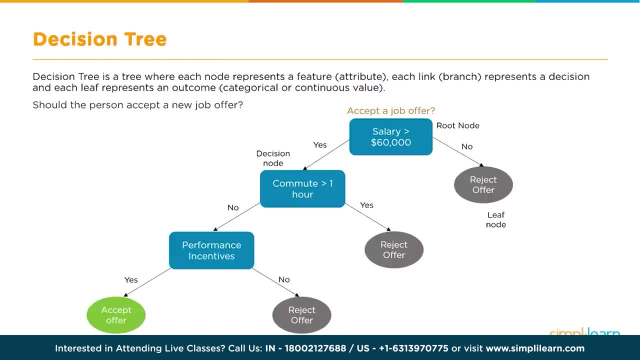 there's a leaf node, and they of course belong to different categories. in this case it is still a binary classification, so this belongs to one class, which is accept offer, and these leaf nodes belong to a different class, which is reject offer. so let's take an example and see how. 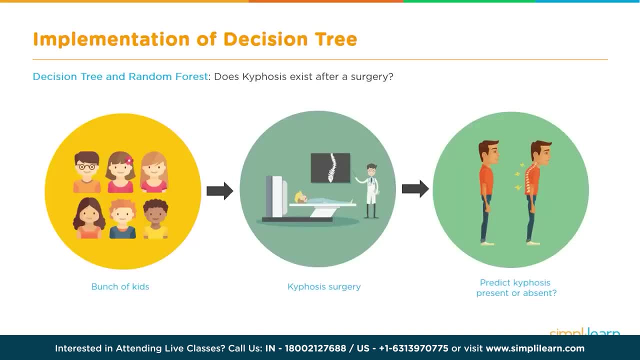 we can solve this problem using decision tree. let's say, we have to implement a classification algorithm for kyphosis patient and the problem is a bunch of kids have been have undergone a kyphosis surgery and we need to predict whether kyphosis is present in them or not. and how can we do this? 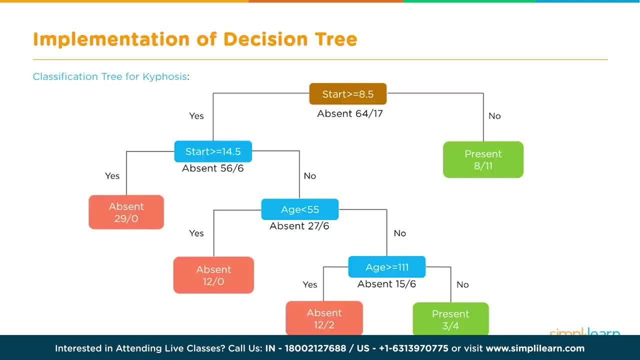 using decision tree algorithm. so this is how the classification tree for kyphosis looks. so it starts with: if the age is greater than 8.5. so this is how the decision tree looks. so the first criteria is the vertebra, the number on which the surgery has been performed, if it is. 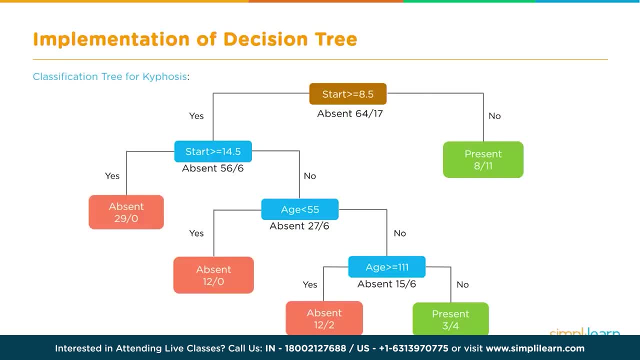 greater than 8.5, then we need to perform further analysis and look at other criteria. if it is less than 8.5, it is clear that kyphosis is present, and if it is greater than 8.5, then we check whether the vertebra operated upon is greater than 14.5 or not. if it is greater than 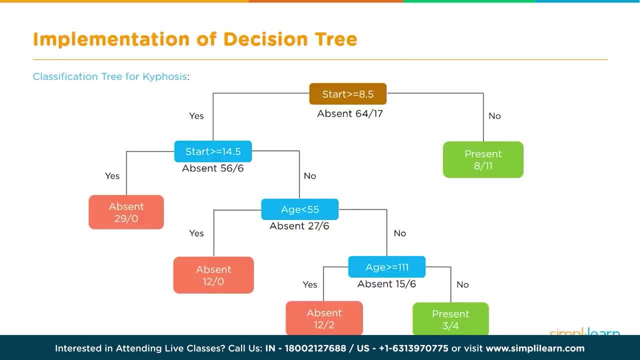 14.5, then kyphosis is absent. if not, then the next criteria is the age. if the person's age is less than 55 years, then kyphosis is absent, but if it is greater than 55 years, then a further analysis is required to see if the person's age is greater than 111 years, which is of course almost impossible. 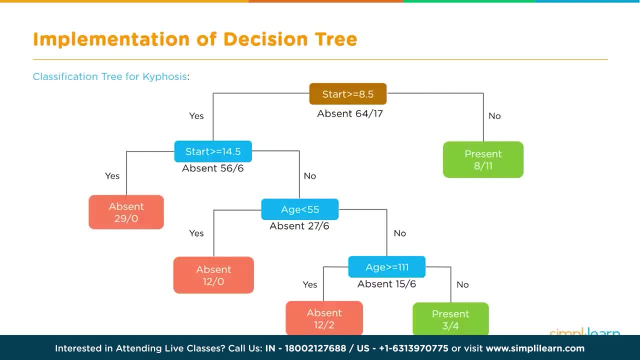 but yes. so if if no, then there is no kyphosis. then we check if the age is greater than 111 years, which means the person is between 55 and 111 years. if the person is between 55 and 111 years, that is this path. that means kyphosis is present, otherwise it is absent. so this is very easy to understand. 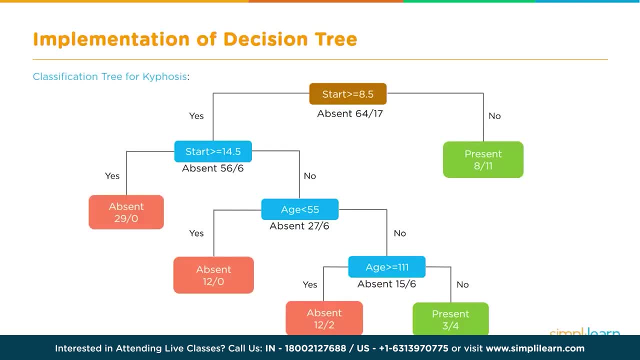 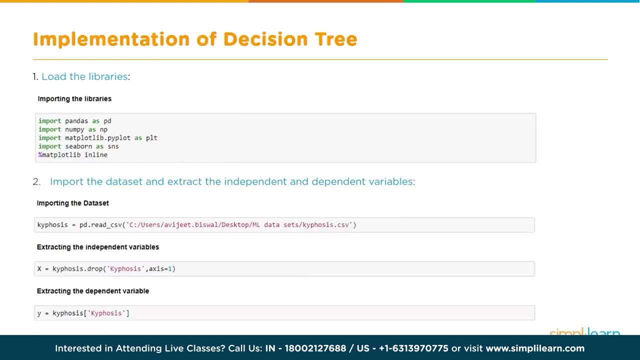 decision tree. and now what we are going to do is we are going to implement this in python in our jupiter notebook and, uh, we have a data set that is available for this and, once again, if anyone wants this data set, please put a comment under this video and we will be more than happy to share the data set with you. 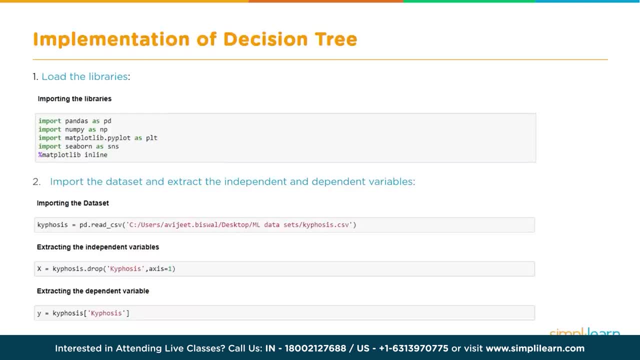 before we go into the jupiter notebook, let's take a look at what the code is doing. what are the various sections of the code? so first one, of course, is loading the libraries, as usual. then we import the data and then extract the independent variables and then separate the labels. 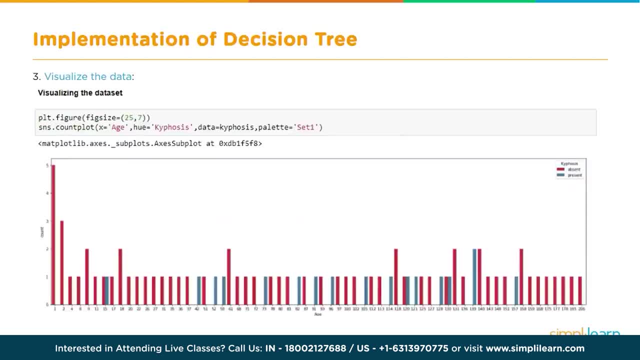 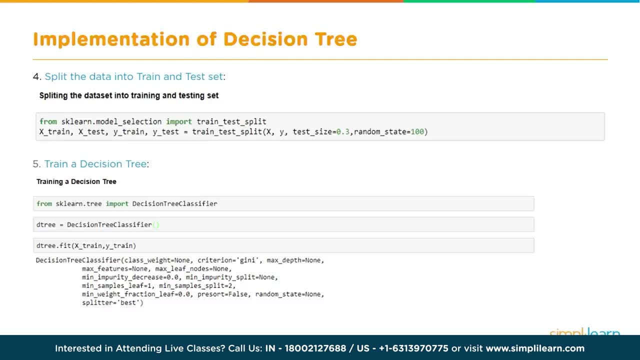 which is the dependent variable, and then we visualize the data- this is how it looks- and then we, as usual, split the data into training and test data sets and then perform the training of the decision tree, and then we test that model with our test data. and then, since this, 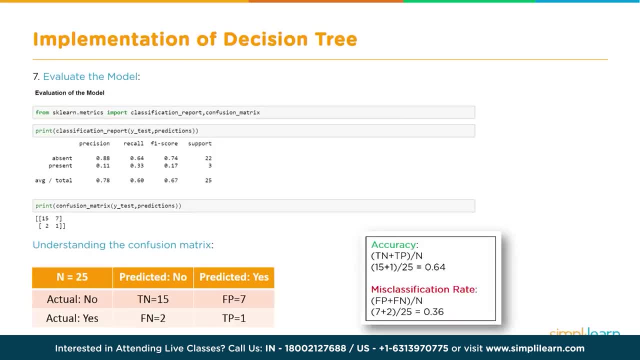 is a classification problem. we evaluate this model using the confusion matrix. remember we talked about this in the previous example as well. so this is the confusion matrix for this particular problem, and here you can see that 16 plus 3, 19 of them have been correctly predicted. 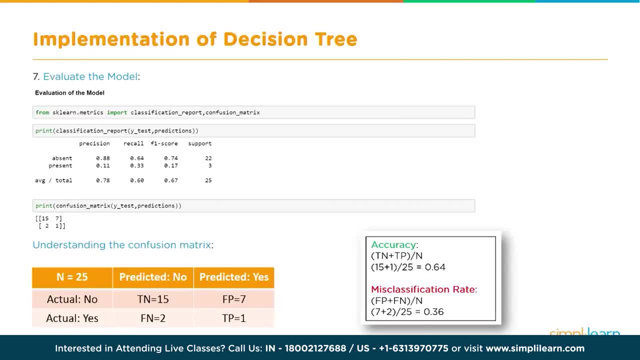 25, which gives us a 64 accuracy. and this 4 plus 2, 6 of them have been misclassified. just to recap once again, how do we determine from the confusion matrix whether this is accurate or not? the numbers in this diagonal should be maximum. so here we see that, out of 25, n is equal to 25, which is the total. 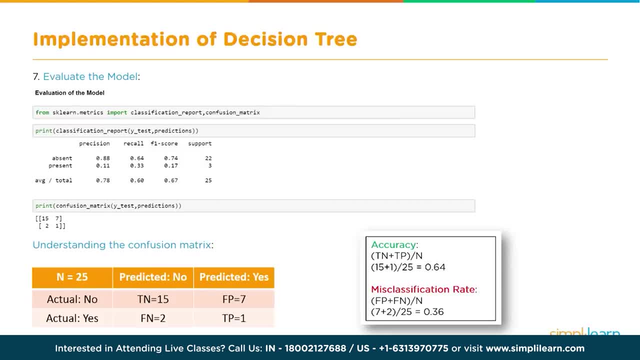 number of observations out of 25. in this case, in this diagonal, we have 16 plus 3, 19 of the values we feel there is good accuracy, which is 64 percent. they have been correctly classified. 64 percent of the observations have been correctly classified by this model, whereas 24 percent have. 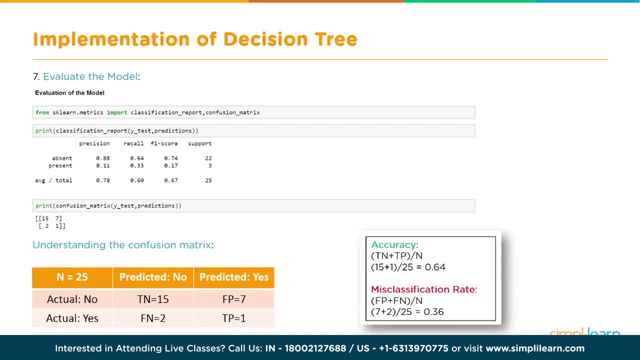 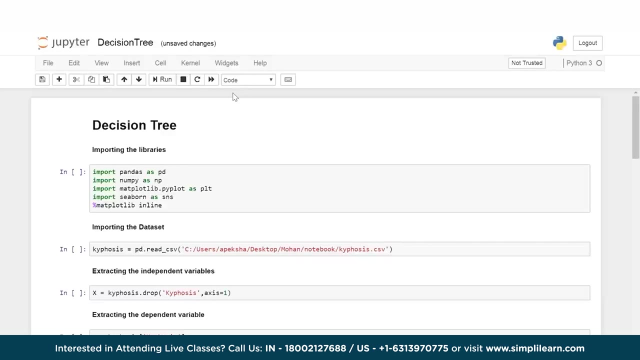 been misclassified- which consists of this 4 plus this 2.. so that's how we use the confusion matrix to determine the accuracy of our decision tree model. so let's go into the jupiter notebook and take a look and run the code and see how it looks. so this is our python notebook for decision tree. 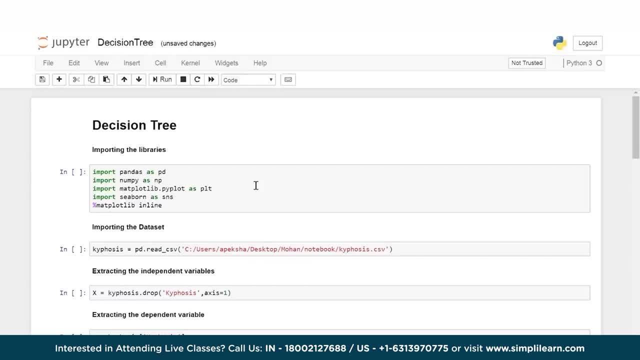 and i will take you through the code, not line by line, of course, but we will see the blocks, as always. the first block is to import the required libraries, like pandas and numpy and so on, and then we import the data. for this we are using kyphosis dot csv file- and then we extract the independent. 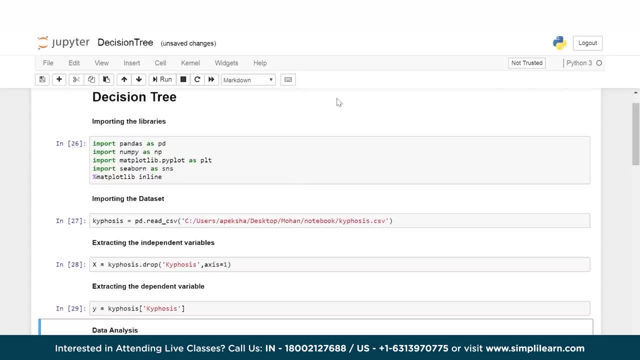 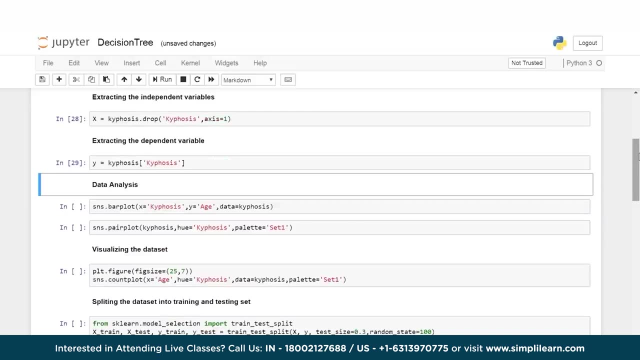 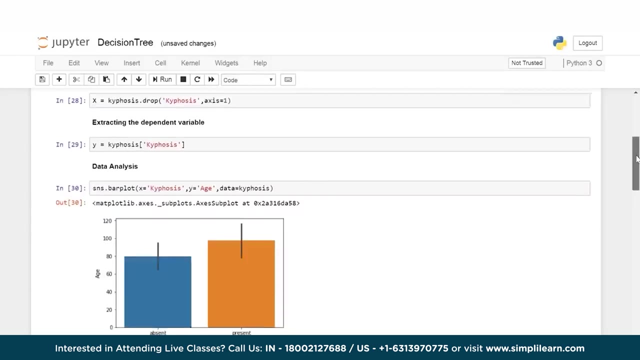 variables and then the dependent variable. dependent variable is the target, which is our classification, and also we call it as the label data, whether it is whether this person, individual, has kyphosis or not, and then we will run a little bit of initial exploratory analysis on the data, so, as a data, 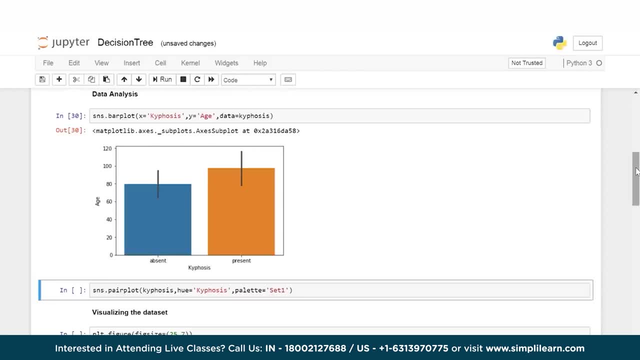 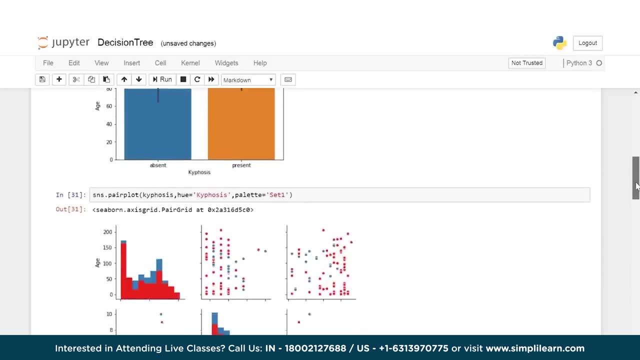 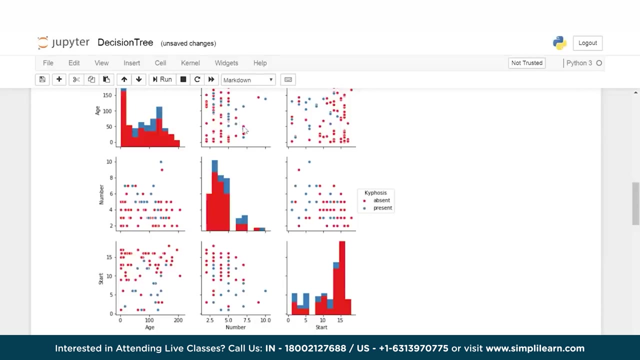 scientist. whenever you get new data, you do that. so we plot age against whether the person has kyphosis or not, and then we plot the various parameters against each other. so, for example, this is like age versus the number and, by the way, the data. how does the data look? let's take a look at the data this has. 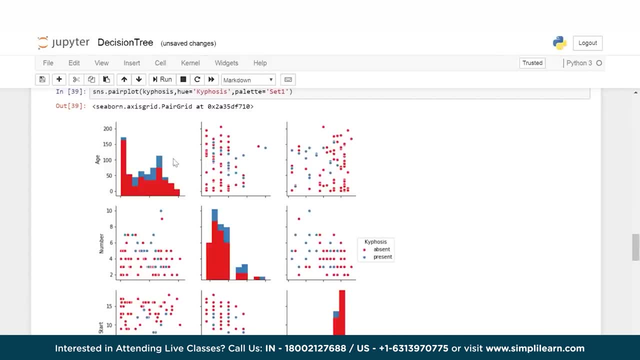 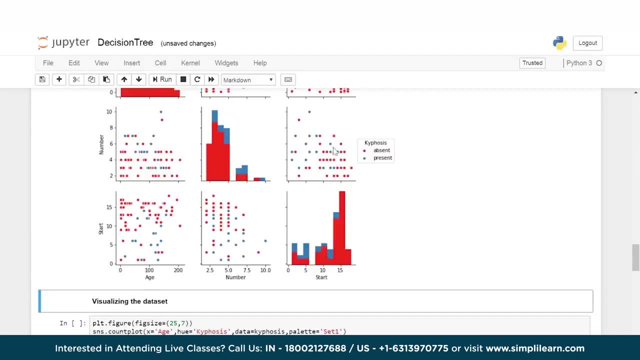 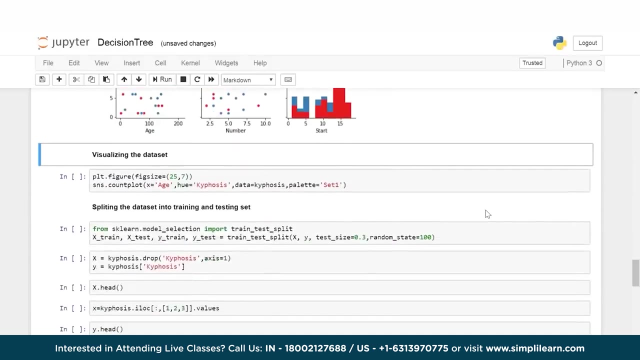 primarily three columns, one attribute against the other. so for example, this is age versus the number, the number versus the start, and so on and so forth. so this is just to give get a quick idea about the overall, how the overall data looks, so we can do a few more visualizations, like with respect to the 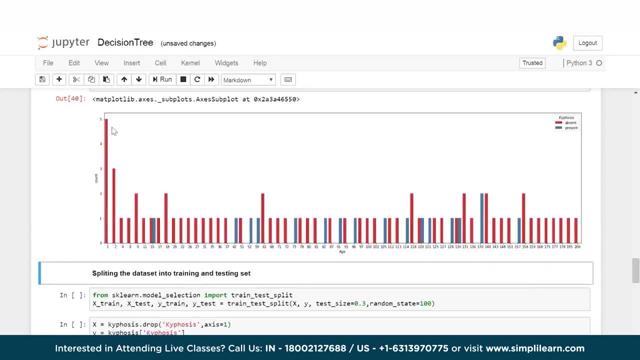 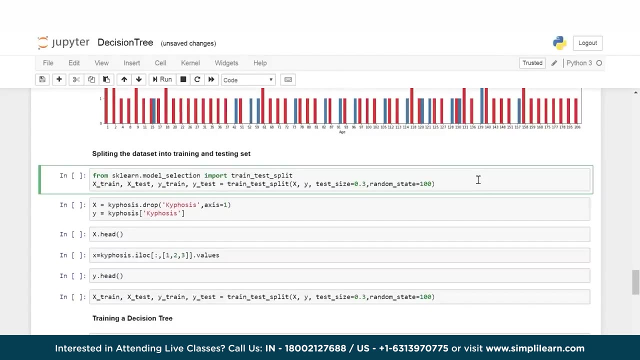 respect to the age and the count, the number of vertebrae that have been operated upon, and the red color indicates kyphosis is absent and the blue color indicates kyphosis is present. so this is another view, and so on. so we can basically do as much of exploratory analysis we can and then 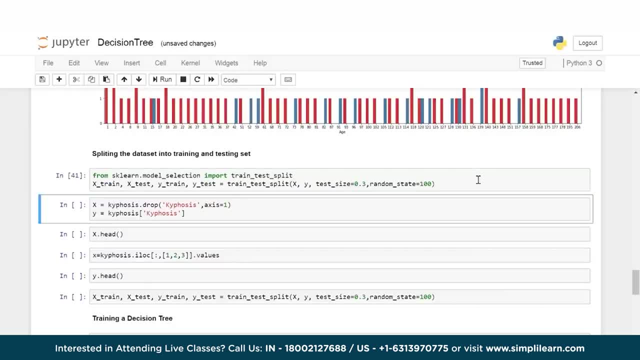 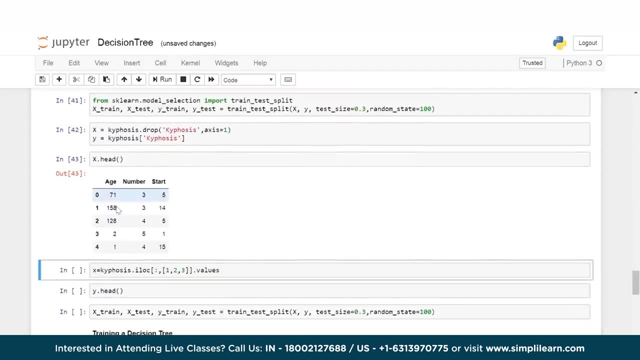 we start training our model. so this is where we split the data into training and test data set, like in all other machine learning examples earlier also, and we can visualize the data or just quick take a quick look at how the data looks. just the first four or five entries here. if we do, 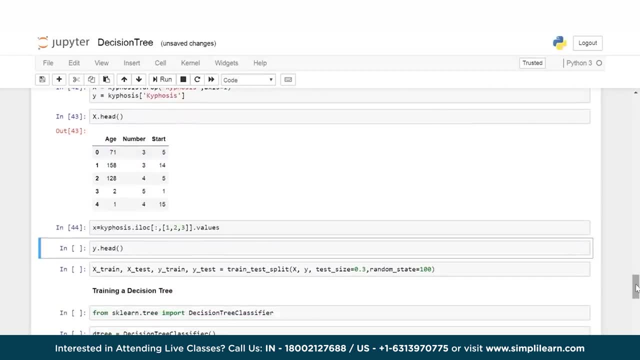 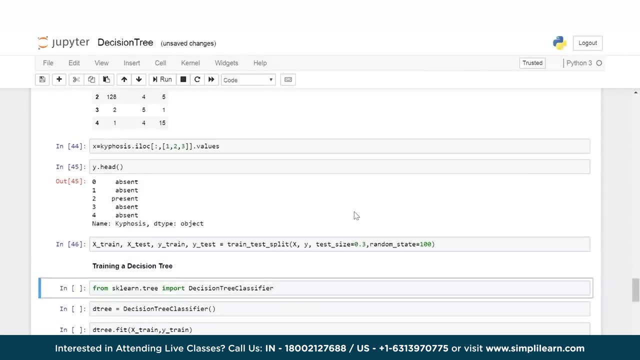 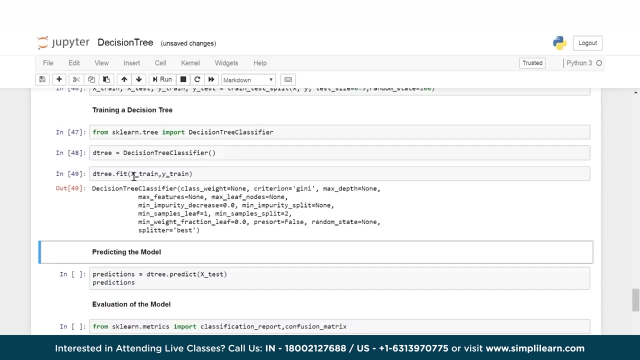 the head. that's what the head function does- and similarly y as well. we can take a look at how the target is looking and then we can get into the training of the decision tree. so we train our model with the training data set using this fit method and then we test whether the model is working fine or not using the test data set. 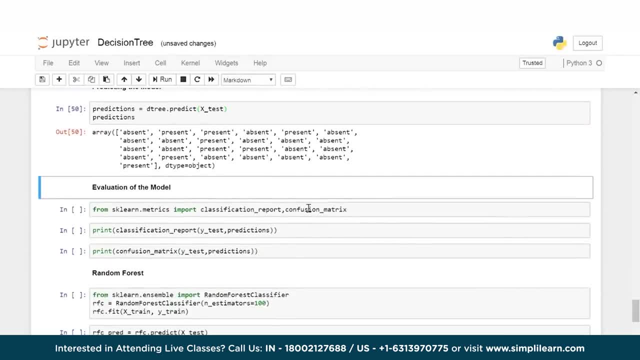 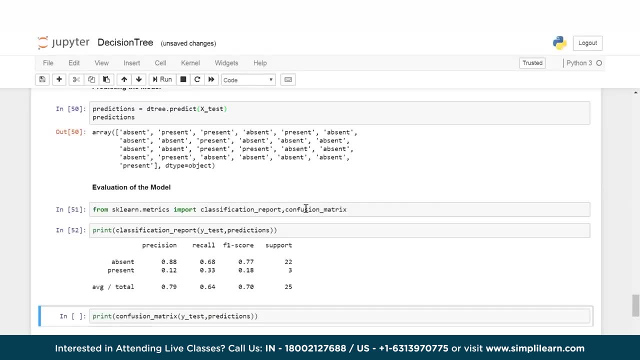 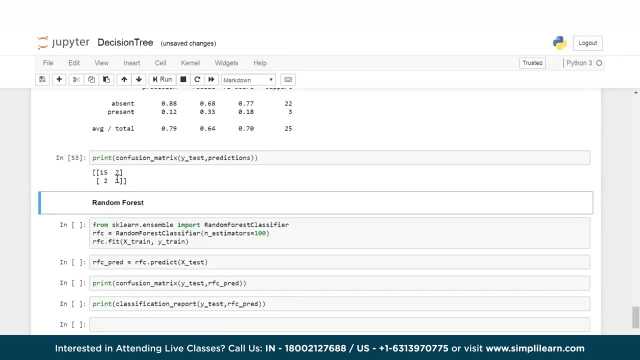 and this is the result of our test data. and then we evaluate the model, and for evaluating we use the confusion matrix. so just let's take a quick look at the confusion matrix and see what is the accuracy. so we get about 16 right. as i mentioned, the diagonal values is what matters, so we have 16. 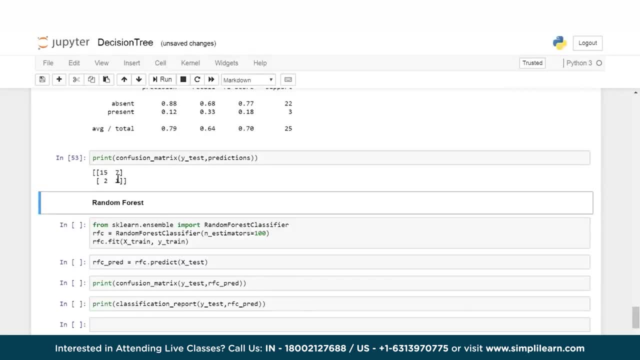 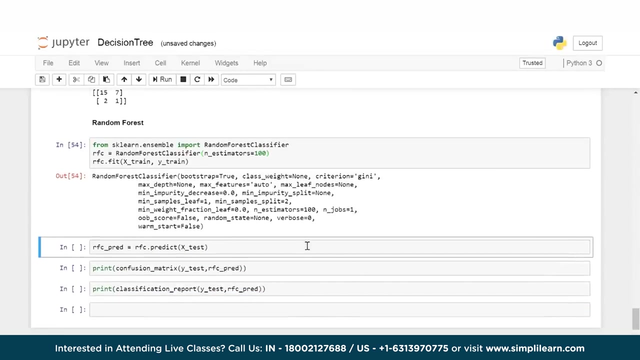 and i'm correctly identified out of 25. so that gives us about 62, i think 70, accuracy. so that is using a decision tree. now, instead of decision tree, let's check what happens if we use random forest. so we use- let's say, our forest consists of 100 trees- and we do the same, we train our model and 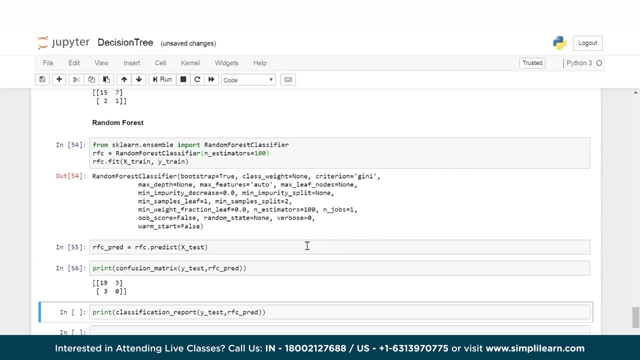 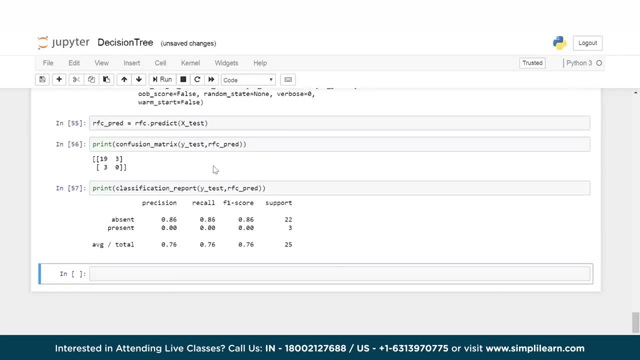 then, with the test data set, we try to test the model and here we that we get 19 of them out of 25 correct, so that is a much better accuracy. so this is about 76 percent. so 19 out of 25 is 76 percent accuracy and we saw in by using the decision tree. we got only 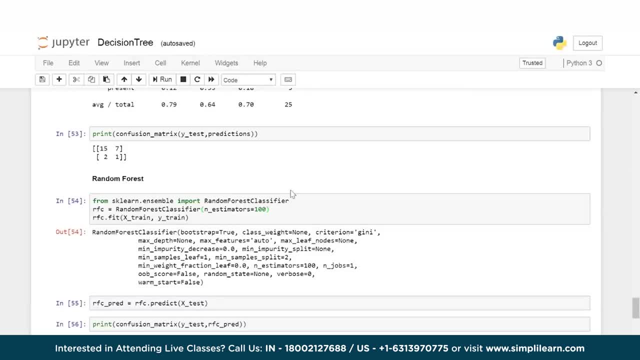 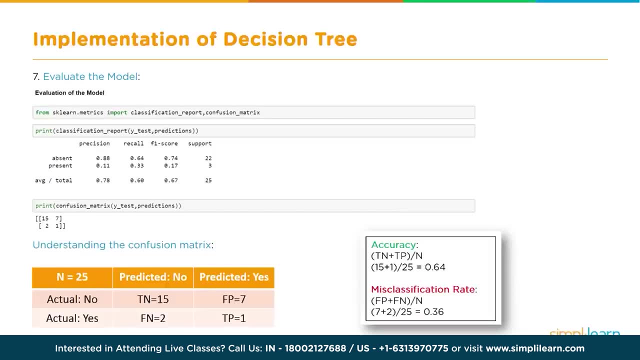 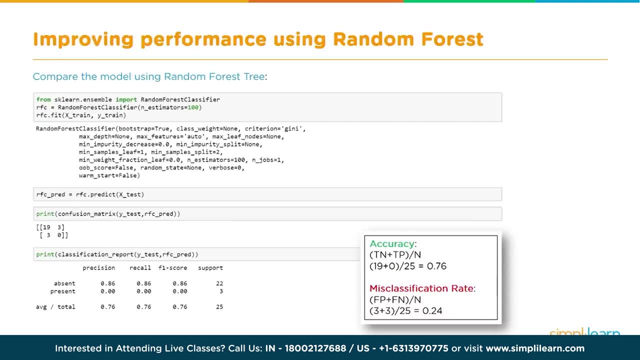 64, that is, 16 by 25 was only 64. so this is a quick demo of implementation of decision tree. so once we evaluate the model, the next thing we can do is what happens if you want to improve the performance. so that's where random forest comes into play. so in instead of using 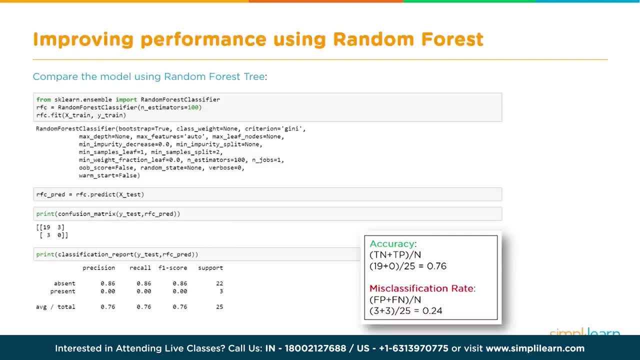 a decision tree. what happens if we use a random forest? and what is the random forest? it's very similar to decision tree. only thing is that instead of using one tree, we use a number of trees. that's why it's called a forest. so we use multiple trees and we take like a average or a vote. 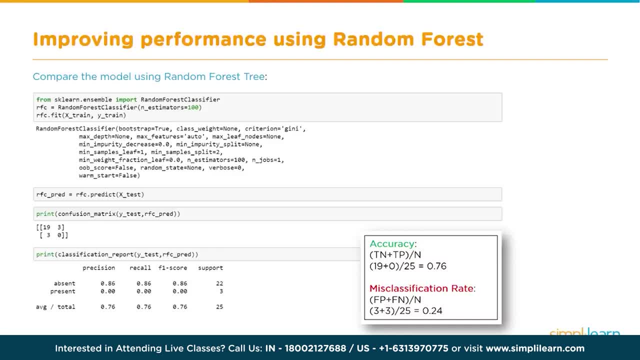 of all the trees for each observation and we finally calculate or we finally classify each observation based on that. So in this case it helps in improving the accuracy. So, as we have seen here, if we take a decision tree, the accuracy now comes to 76%, right In the previous case. 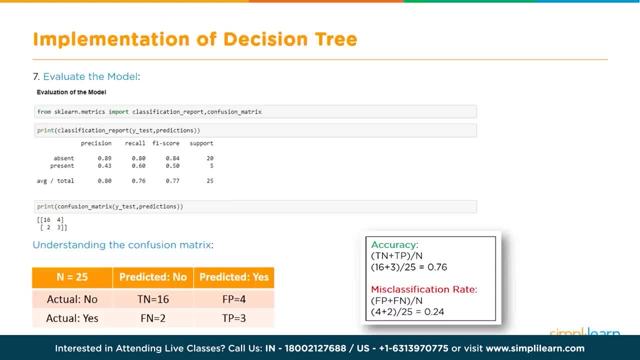 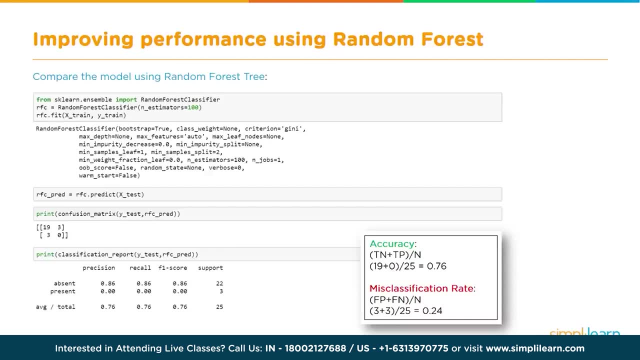 it was only 64% Using just the decision tree. now, when we use random forest, the performance has improved to a good extent and it has become 76%. So random forest usually helps in increasing the accuracy when we are using decision trees as our algorithm. Okay, the last algorithm is the. 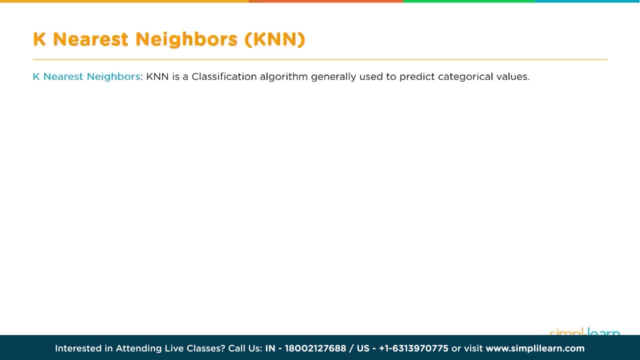 k-nearest neighbors algorithm. This is again a classification algorithm and it is actually very simple and straightforward, very easy to understand as well In this case. let's say, we have historical data of heights and weights And we also have the labels. So if the height and weight is in this range, these are cats and 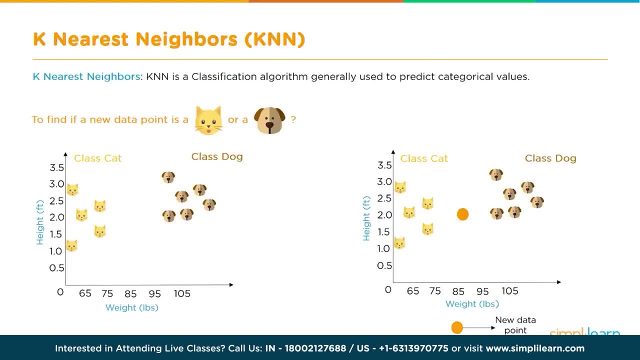 if the heights and weights are in this range, these are dogs. So this is one class and this is another class. And now if we get a new point or new data set and we find that for this particular animal, the height and weight, if we plot, it is here. So how do we determine whether it belongs? 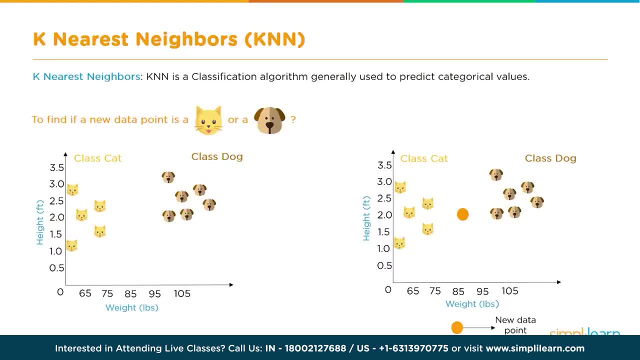 to the cat class or the dog class. That is where the k here comes into play. So when we are using this algorithm we need to specify what should be the value of k. So let's say we say we determine that the value. 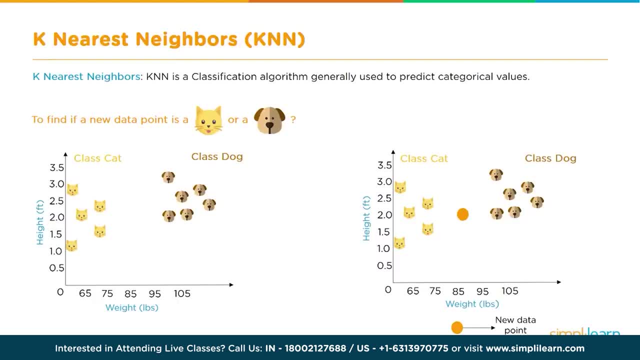 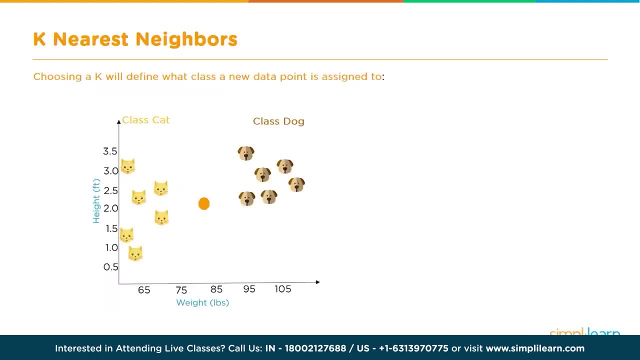 of k is three. So what we will do is we will find out the nearest objects, nearest three objects to this data point that we have. So let's go to the next slide here. Okay, And we define k as three. 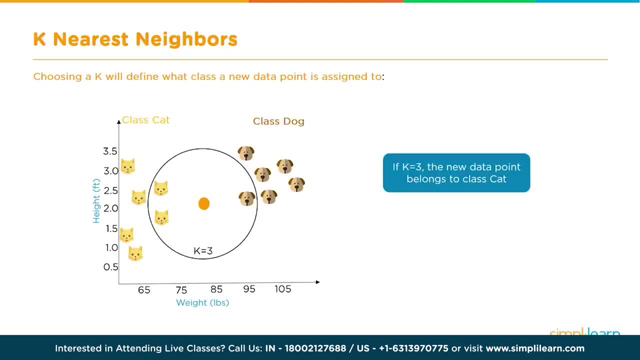 So what happens? We find the nearest three objects to this data point and then we find out what is the maximum number of items, which class the maximum number of items belong to? So in this case, there are two cats and there is one dog. Therefore, we determine that this 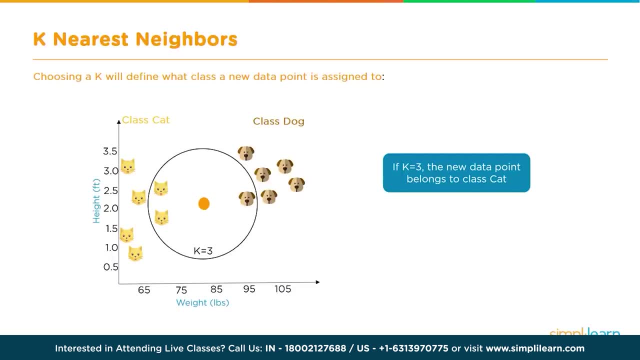 new data point belongs to the cat class. Now what happens if we say k is equal to seven? In that case, these are the seven data points which are nearest to this new data point. And now you see that, instead of cats, dogs are more So, which means that now the point: or this data or 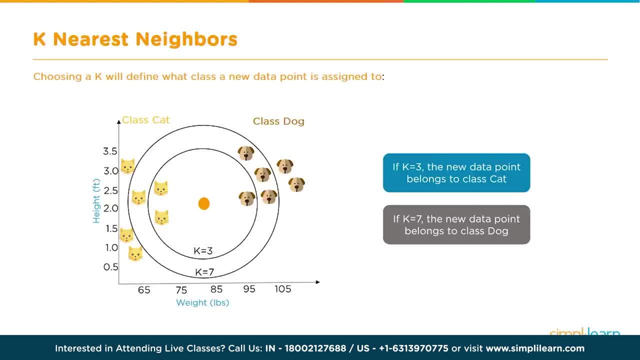 this new creature belongs to the class dog. So this is while this is a slight drawback, but by trial and error it's not a drawback. So this is a slight drawback, but by trial and error we should be able to find out the right value of k And once we use that, that's how we train the. 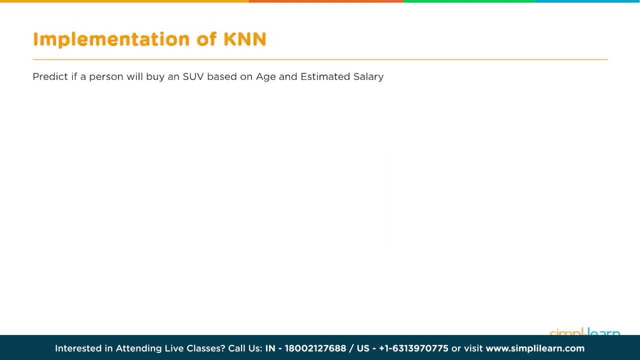 model. Now let's use k nearest neighbors and take an example to solve one of our previous problems that we did using logistic regression: whether a person is going to buy an SUV or not, based on the age and estimated salary. So before we go into Jupyter Notebook, let's again take a quick. 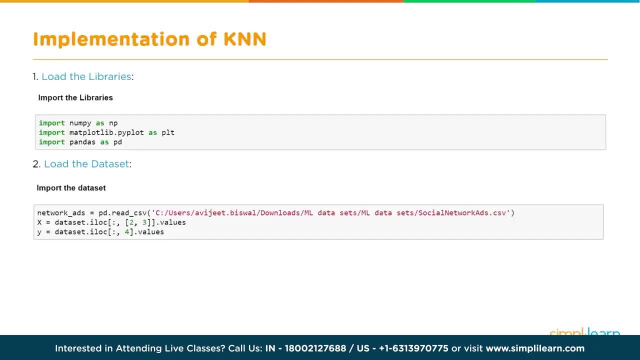 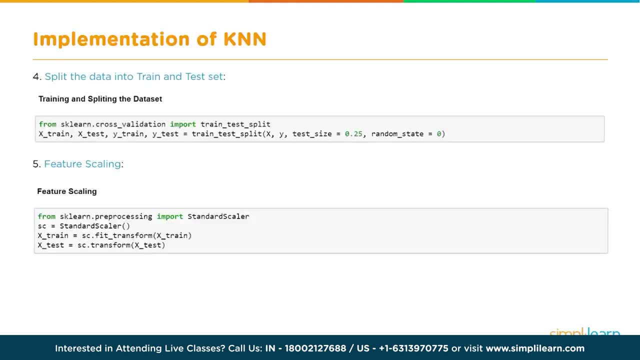 look at the core. So what are the various sections in the core? As always, we import the libraries, we load the data set, we visualize the data, we split the data into training and test data set. we do some feature scaling and then we train our model and then we test our. 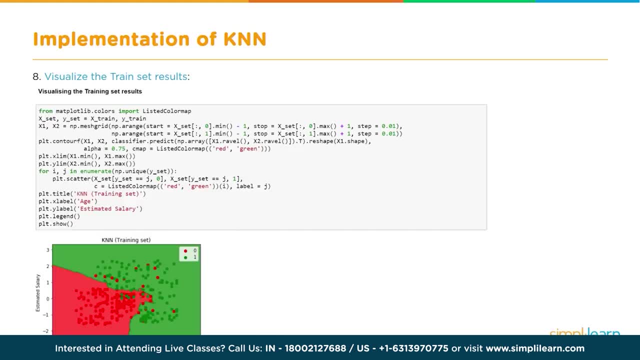 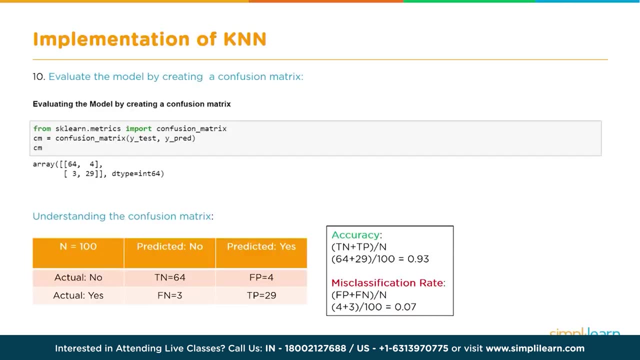 model. we visualize the training set results and then we visualize our test results And both of these seem to be looking pretty good, And then we evaluate our model using the confusion matrix. So remember, whenever we use a classification algorithm, the way to evaluate our model, to find 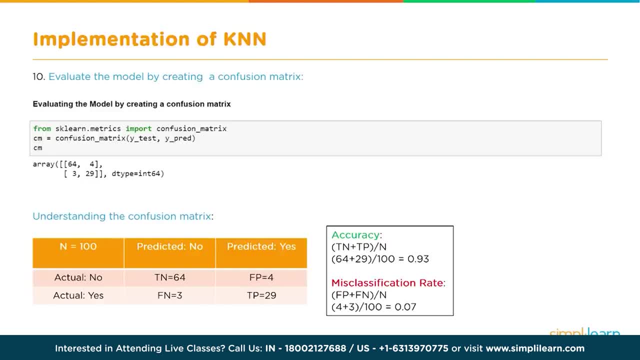 accuracy of our model is the confusion matrix. We have seen in logistic regression, we have seen in decision tree and now in KNN as well. So in this case, once again, the total number of observations is 100. And we see that along the diagonal, which is the number we need to consider. 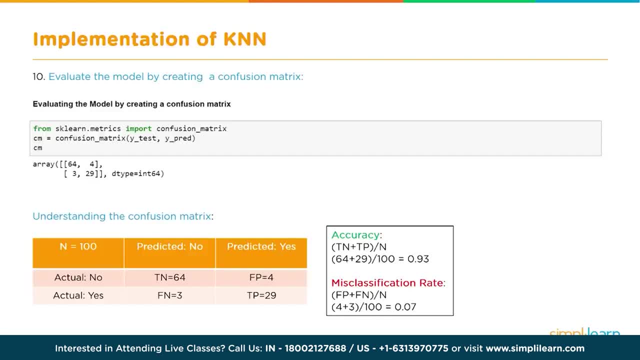 there are 93 values, which means we achieve 93% accuracy, And a few of them, that is, only seven of them, are misclassified. So this is a pretty good accuracy Compared to our previous example. So let's go and check how this looks in Jupyter Notebook. 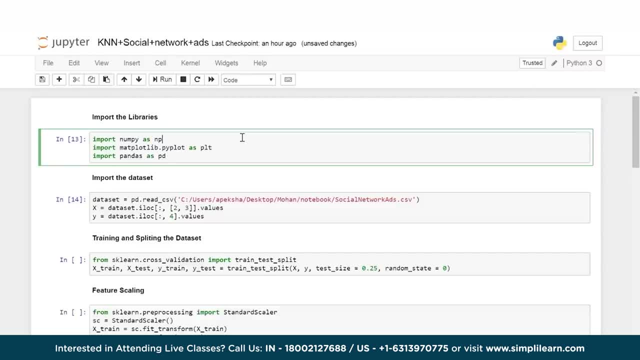 So this is my Python notebook for k-nearest neighbor implementation And I will quickly walk you through this code. The first block is, as usual, we are importing the various libraries like NumPy, pandas and matplotlib, And then we load the data set And we split the data into training and 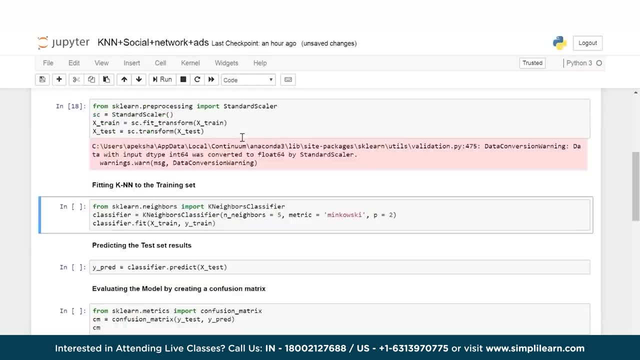 test, And then we load the data set And we split the data into training and test, And then we load the data set. And then we load the data set And then we do feature scaling And then we start training our model. And here we are specifying k as five. Okay, And now the data. 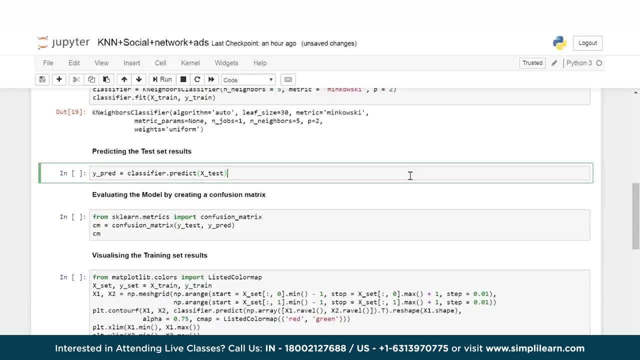 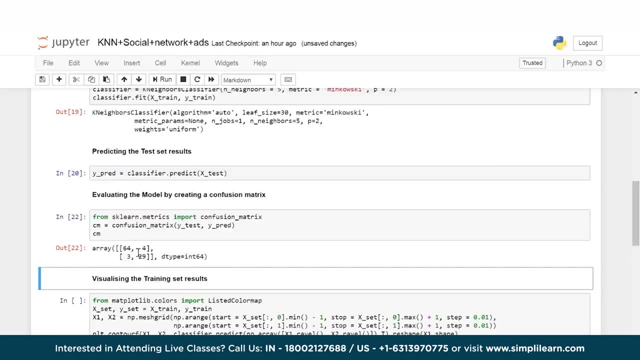 set is trained. Now we go and test it with our test data set. Then we evaluate the model. And here we get that. as you can see in the diagonal, there are 73 entries, So total is 73.. And here we get that. as you can see in the diagonal, there are 73 entries, So total is 73.. 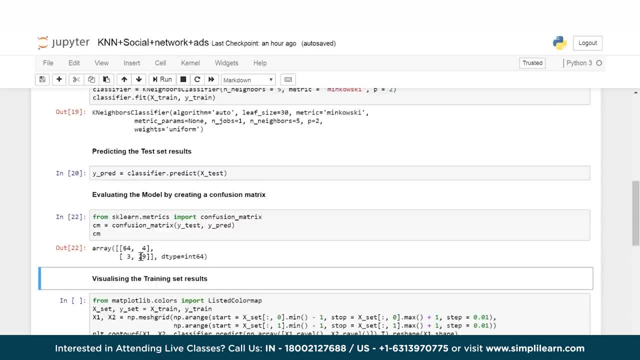 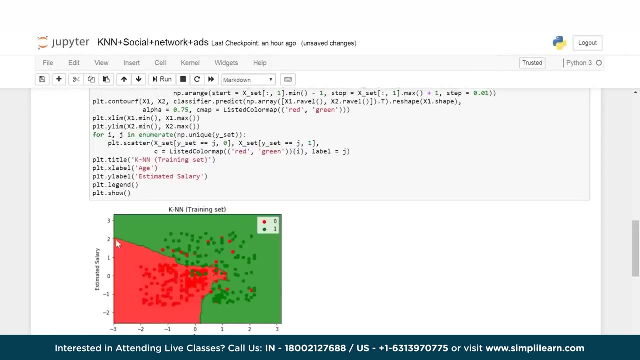 Which means out of total of 80, 73 have been classified correctly, which is about 90% accuracy we are getting, And seven of them have been misclassified. We can now visualize the training results. So these are the zeros and these are the ones. 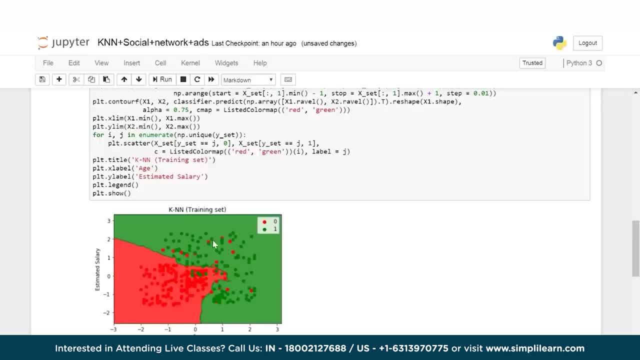 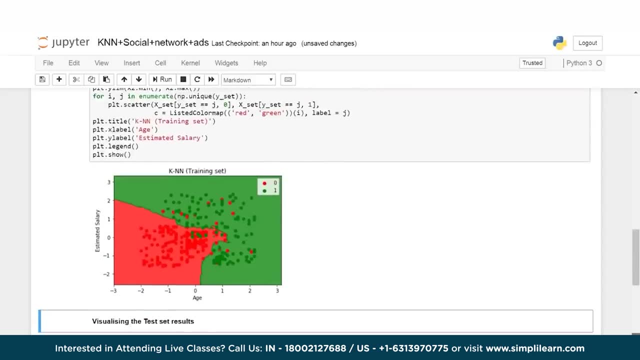 This is the training set. So there are a few, as you can see, misclassifications: The green ones in the red area and the red ones in the green area. These are the misclassified values And same way we can check the. 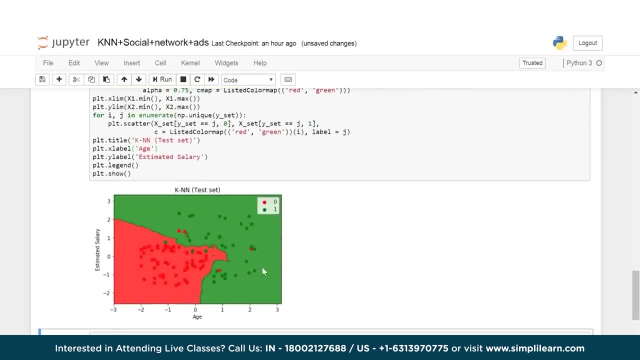 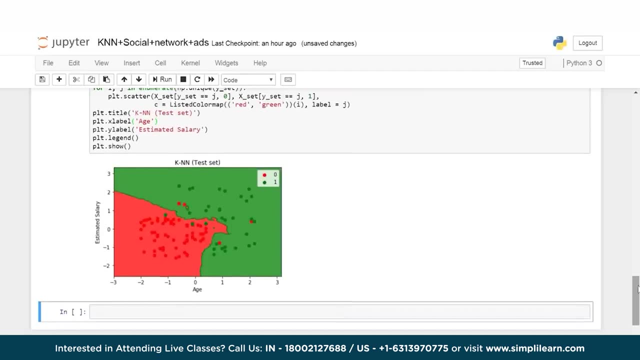 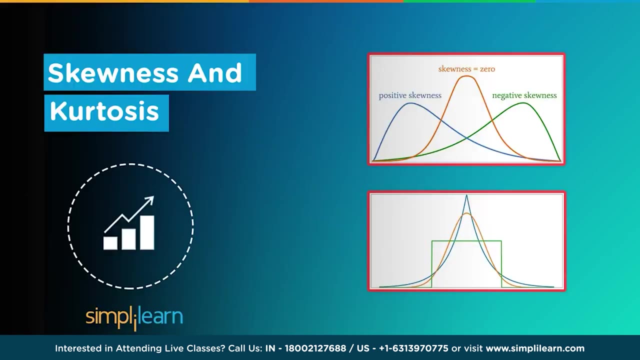 visualize the results of the test data set as well. And here again we see there are a few little bit of misclassification. And that brings us to the end of this Python notebook demo for KNN classification. As you know, in today's world, data is becoming increasingly. 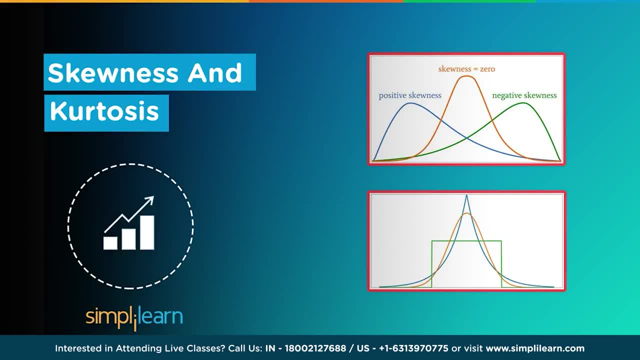 important. Entire professions are dedicated to studying, understanding and manipulating the data. Hence it is important to know about the different types of data and their associated properties. So in this session we will discuss how to calculate the distortion in the normal curve. 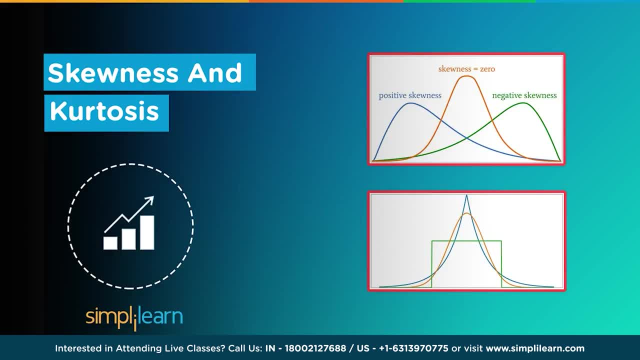 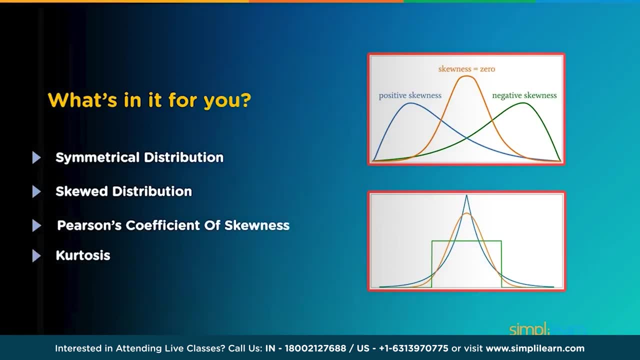 using skewness and kurtosis. So let's get started. We will start this tutorial by understanding symmetrical distribution. Then we'll move on to discuss skewed distribution and Pearson's coefficient of skewness. Finally, we will discuss kurtosis. 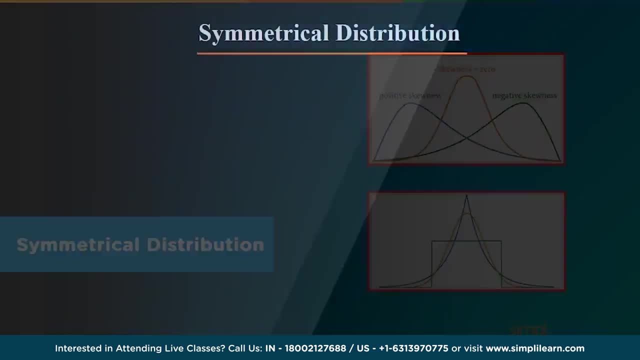 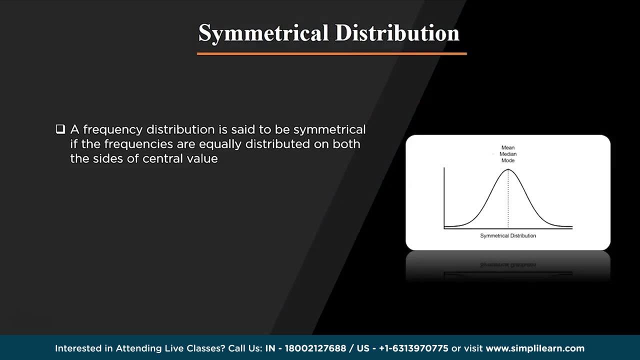 Let's get started. Symmetrical distribution. A distribution is said to be symmetrical distribution when it is equally distributed on both the sides of the mean value. The distribution shape can either be a bell shape or U-shaped. In symmetrical distribution, the values of mean, median and mode are all equal. 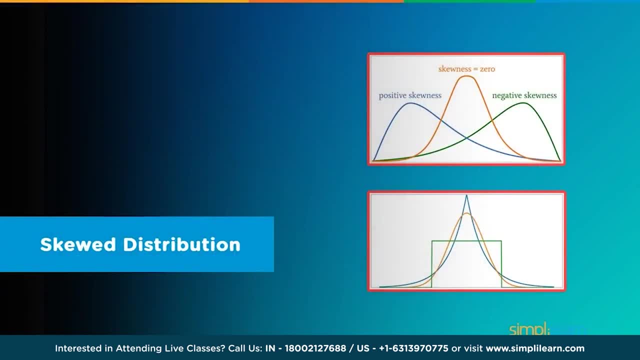 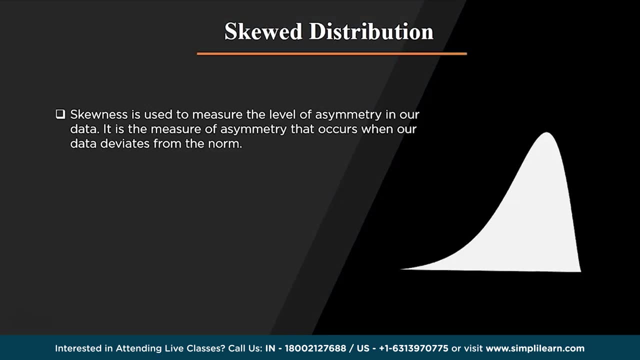 as you can see in the graph, Skewed distribution. Skewness is used to measure the level of asymmetry in our graph. Skewed distribution is used to measure the level of asymmetry in our graph. It is the measure of asymmetry that occurs when our data deviates from the norm. 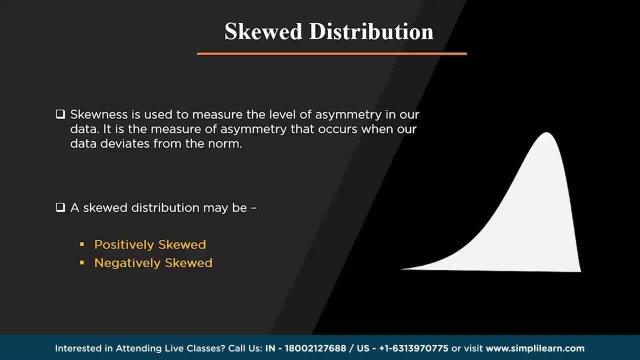 Sometimes the normal distribution tends to be tilted more on one side. This is because the probability of data being more or less than the mean is higher and hence makes the distribution asymmetrical. This also means that the data is not equally distributed. The skewness can be of 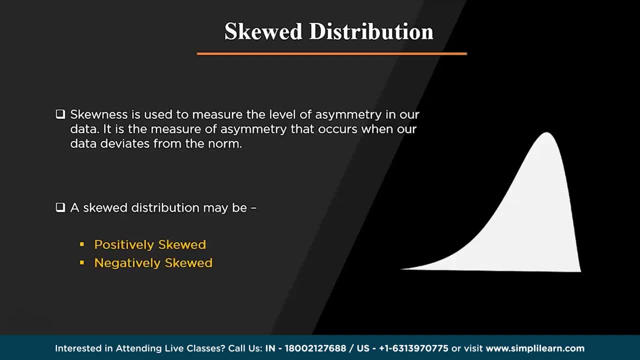 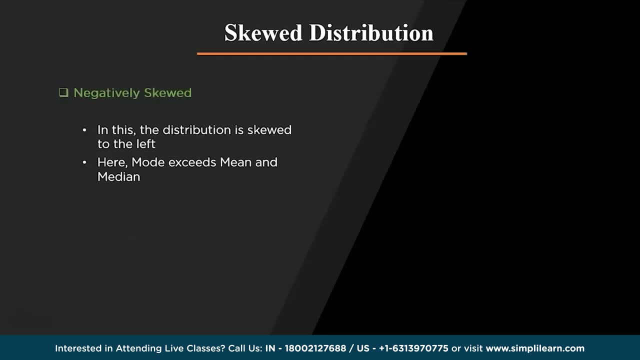 two types: Positively skewed and negatively skewed. Let's discuss them separately. Negatively skewed: In a negatively skewed distribution, the data points are more concentrated towards the right hand side of the distribution, As you can see in the graph. this makes the mean median and mode. 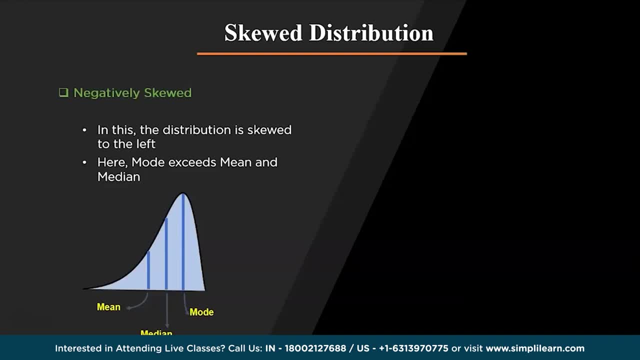 bend towards the right Hence. these values are always negative. In this distribution mode is greater than median, and median is greater than mean. Now let's move on to positively skewed distribution. In a distribution that is positively skewed, the values are more concentrated towards. 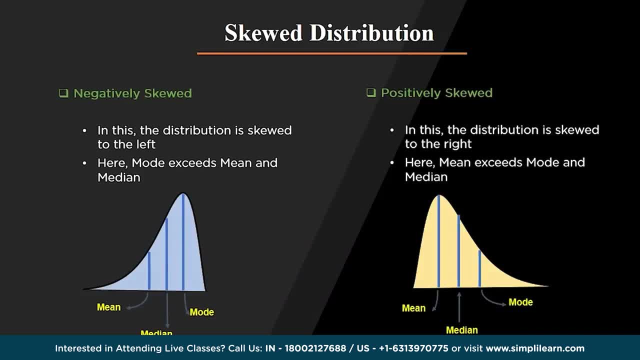 the right side and the left tail is spread out, as you can see in the graph. Hence the statistical results are bent towards the left hand side. Therefore, the mean, median and mode are always positive In this distribution, mean is greater than median and median is greater than mode. 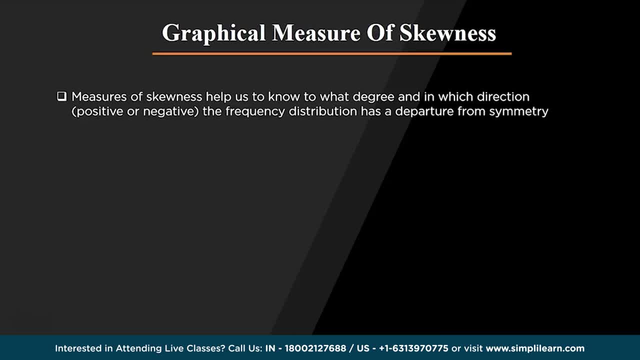 The measure of skewness always helps us to know to what degree and in which direction- positive or negative- the frequency distribution has a departure from symmetry. Positive or negative skewness can be detected graphically, depending on whether the right tail or the left tail is longer, but we don't get the idea of the magnitude. 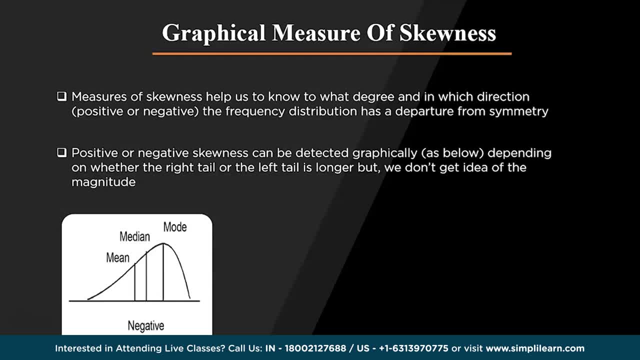 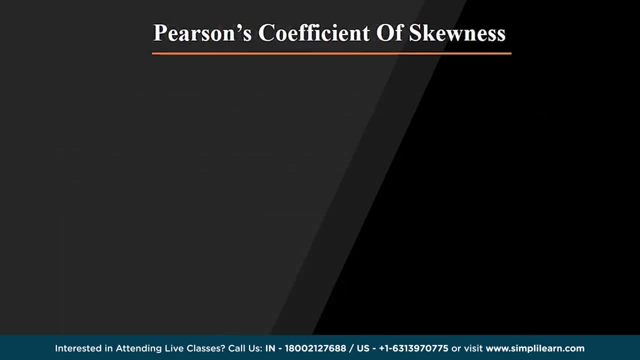 In a negatively skewed symmetry, the values are always negative. This is the symmetrical distribution, and in a positively skewed, the values are always positive. Now let's discuss PSU's coefficient of skewness. The median is always the middle value, and the mean and the mode are the extremes. 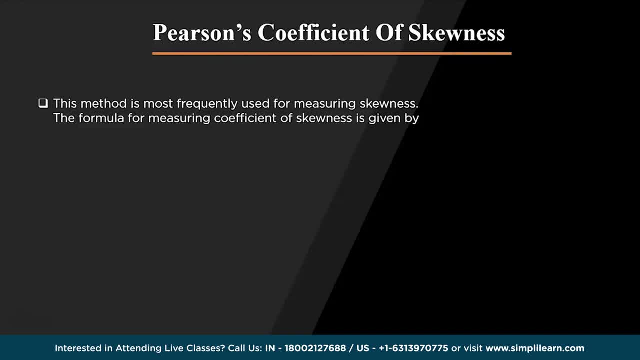 So we can derive the formula to capture the horizontal distance between the mean and the mode using the PSU's post-procedure. So the formula to calculate the PSU's coefficient is mean- mode divided by the standard deviation. The division by the standard deviation will help you to scale down the difference between. 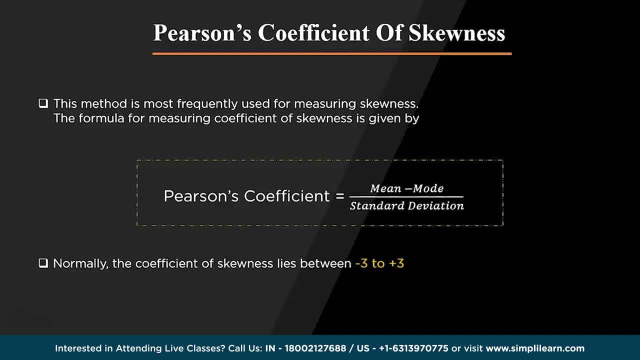 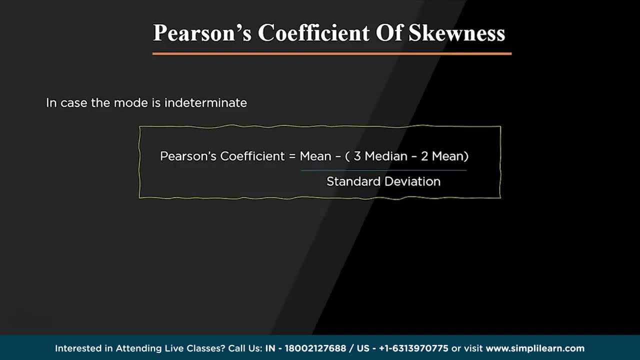 mode and the mean. This will scale down their values in the range of. In case where the mode is indeterminate, we can calculate the PSU's coefficient by mean- mean divided by the standard deviation. the value of coefficient is between and .5 and .7, the value will be minus 0.5.. 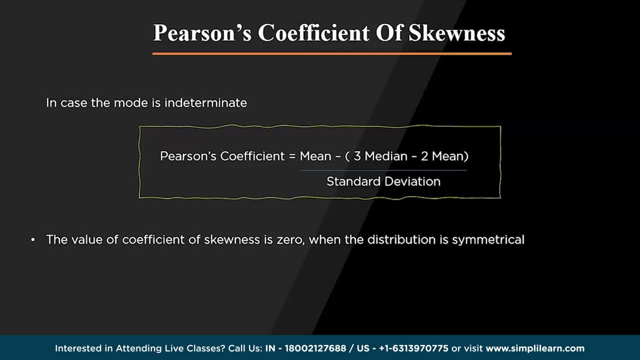 0.5, the distribution of the value is always symmetrical. If the value of coefficient is 0,, then the distribution is symmetrical. If the value of coefficient is positive, then the distribution is positively skewed, and if the coefficient is negative, then the distribution 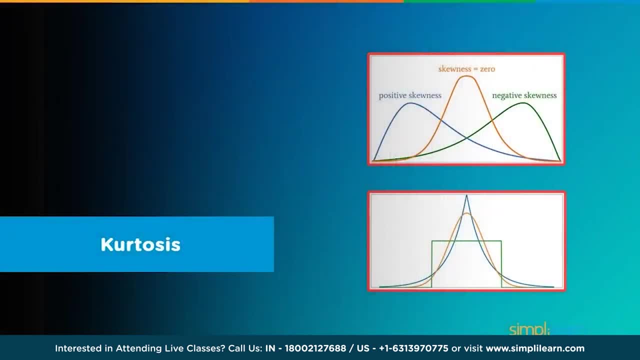 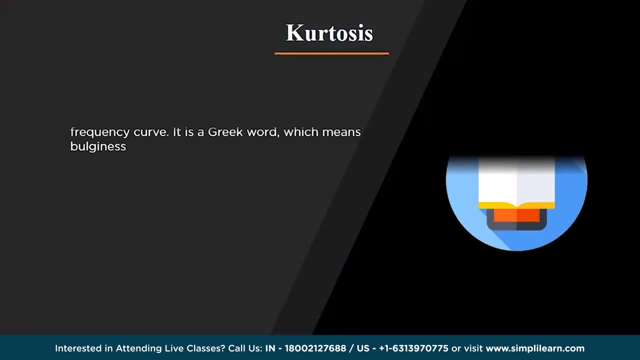 will be negatively skewed. Now that we have discussed the symmetrical and skewed distribution, let's move on to understand what is kurtosis. Kurtosis is used to find the presence of outliers in our data. It gives us the total degree of outliers present. The data can be heavily 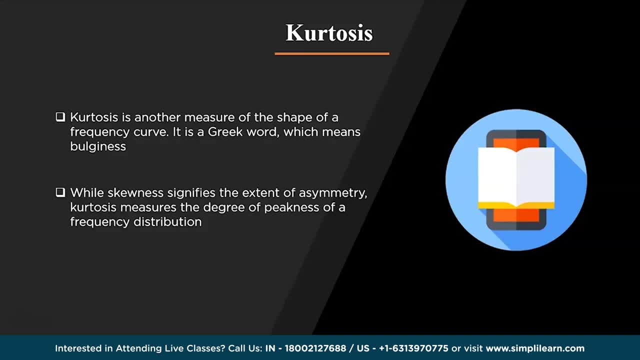 tailed and the peak can be flatter, almost like punching your distribution or squishing it. While skewness signifies the extent of the symmetry, kurtosis measures the degree of peakness of a frequency distribution When the peak of the curve becomes relatively high. 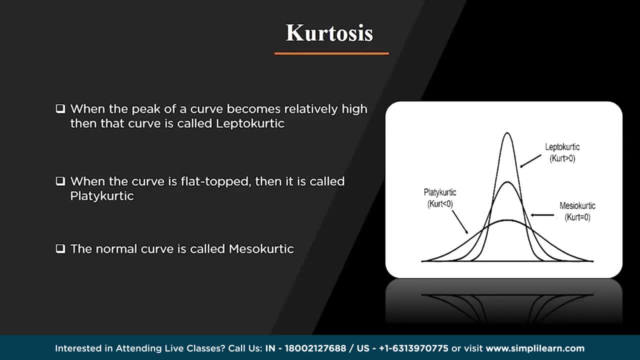 then the curve is called leptokurtic, and when the curve is flat it is called platokurtic. When the curve is similar to the normal curve, it is called mesokurtic. The expected value of kurtosis is 3.. This is observed in a symmetrical distribution. A kurtosis greater than 3 will 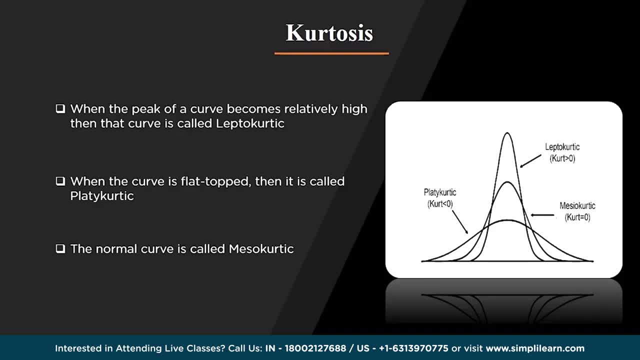 indicate positive kurtosis. Further, a kurtosis less than 3 will mean a negative kurtosis. The range of value for a negative kurtosis is from minus 2 to infinity. The greater the value of kurtosis, the higher is the peak, as you can see from the graph. 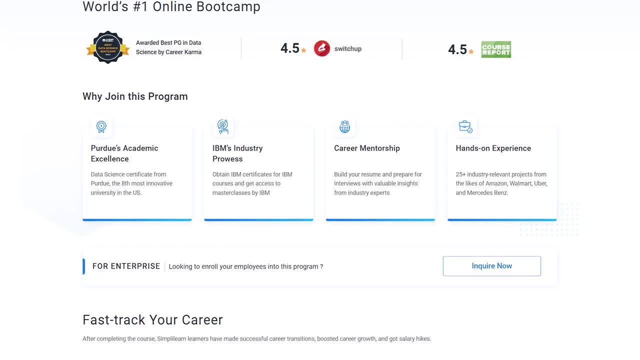 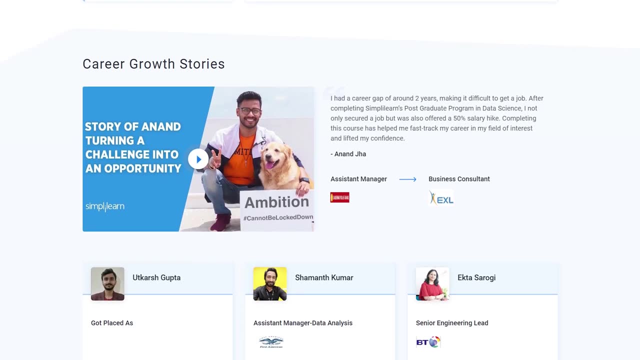 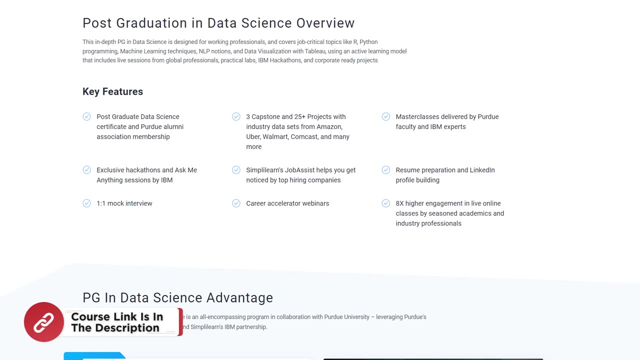 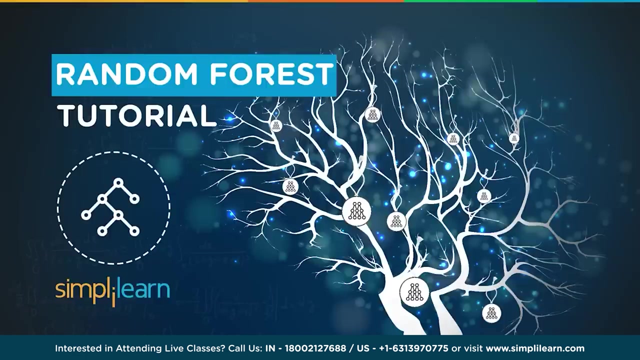 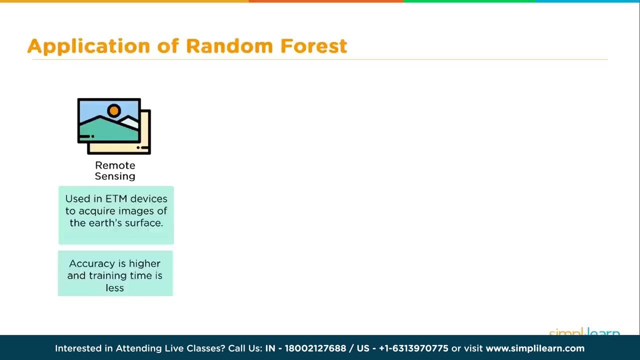 Let's take a look at random forest, one of the many powerful tools in the machine learning library. Before we dive into the topic, let's start by looking at a few of the uses for our random forest Currently. today it is used in remote sensing. For example, they are used in the ETM devices. 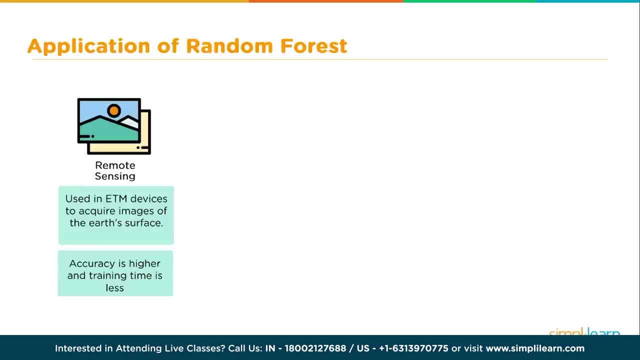 If you are a space buff. that is the enhanced thermatic mapper they use on satellites which see far outside the human spectrum for looking at land masses And they acquire images of the earth's surface. The accuracy is higher and training time is less than many other machine learning tools out there. Also, object detection multi-class. 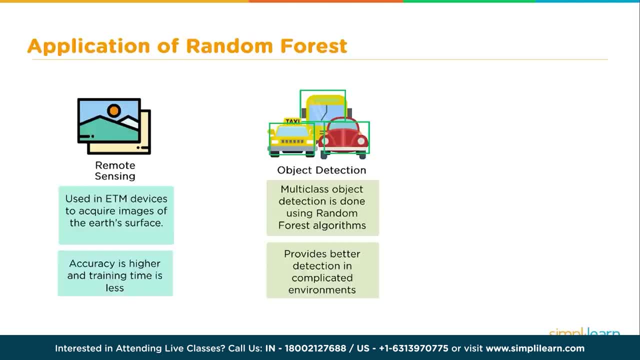 object detection is done using random forest augmentation. This is done using random forest augmentation algorithms. A good example is traffic, where you try to sort out the different cars, buses and things, And it provides a better detection in complicated environments. And then we have another example: connect. Let's take a little closer look at connect. 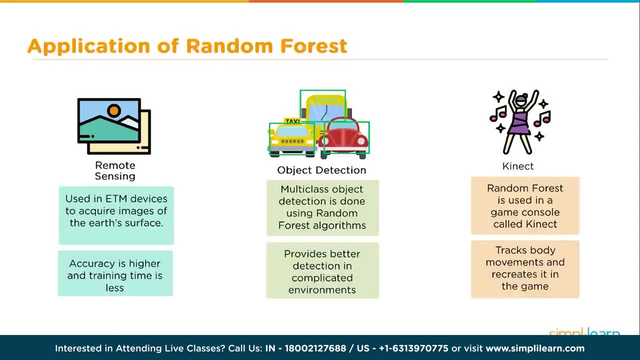 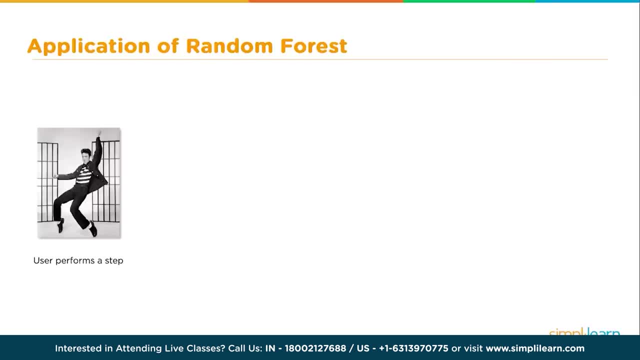 Connect uses the random forest as part of the game console. What it does is it tracks the body movements and it recreates it in the game. Let's see what that looks like. We have a user who performs a step, In this case it. 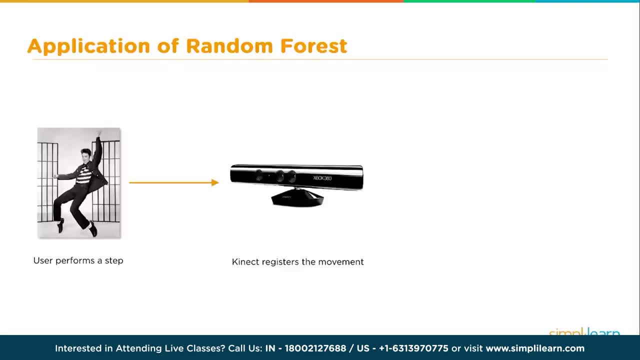 looks like Elvis Presley going up. We have a user who performs a step- In this case it looks like Elvis Presley going up. That is then recorded so that connect registers the movement and then it marks the user based on accuracy. 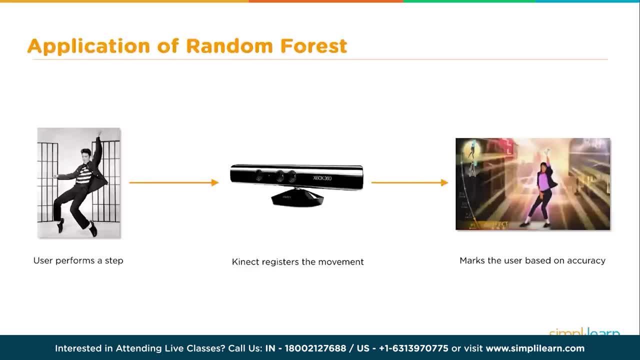 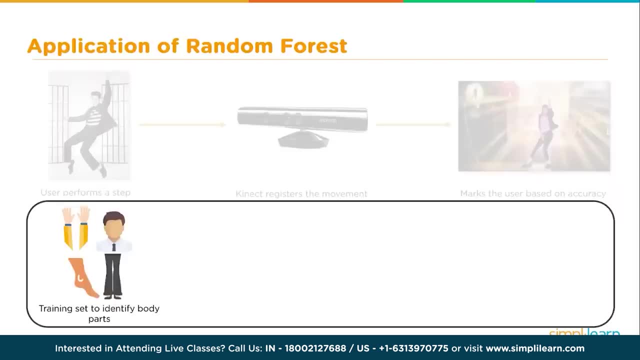 It looks like we have Prince going on. this one from Elvis Presley to Prince. That's great, So it marks the user based on the accuracy. If we look at that a little closer, we have a training set to identify body parts. Where are the hands? Where are the feet? What's? 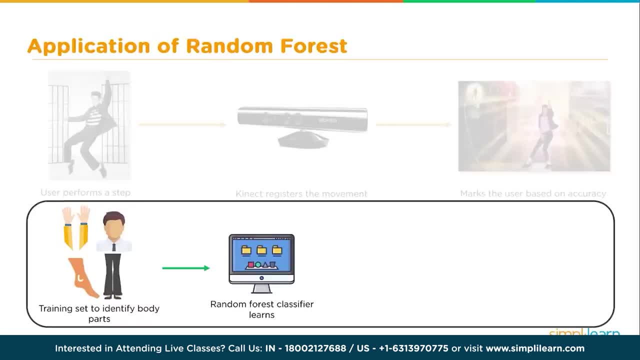 going on with the body. That then goes into a random forest classifier that learns from it. Once we've trained the classifier, it then identifies the body parts while the person's dancing. It's able to represent that in a computer format and then, based on that, it scores the game. 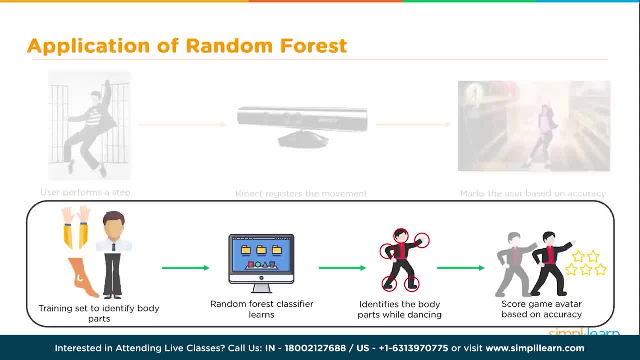 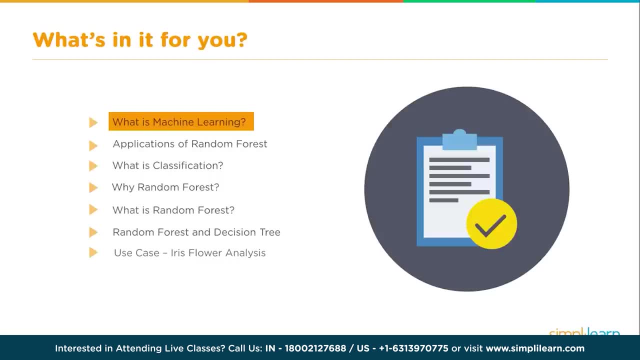 and how accurate you are as being Elvis Presley or Prince, and you're dancing. Let's take an overview of what we're going to cover today. What's in it for you? What we're going to start with is: what is machine learning? 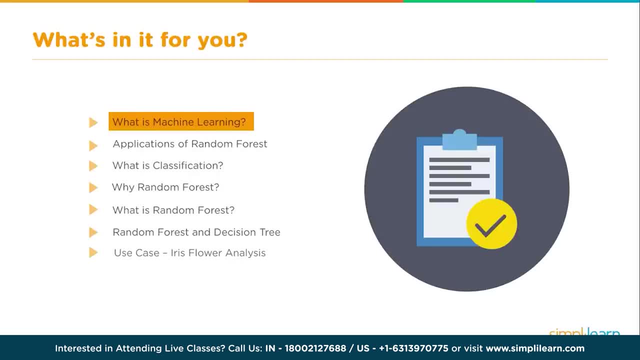 We're not going to go into detail on that. We're going to specifically look at how the random forest fits in the machine learning hierarchy. Then we're going to look at some applications of random forest. What is classification? which is its primary use? 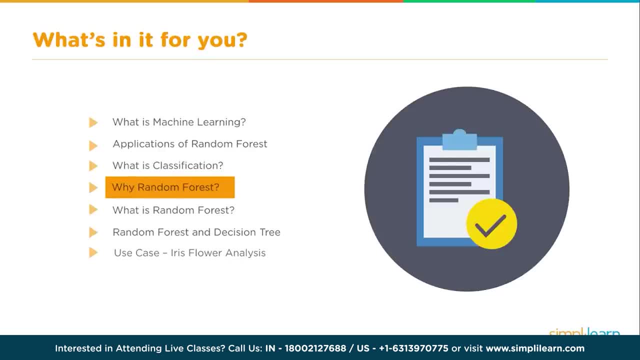 Why use random forest? What's the benefits of it? How does it actually come together? What is random forest? Then we'll get into random forest and the decision tree. That's the final step in how it works. Finally, we'll get some Python code in there and we'll use the case the iris flower analysis. 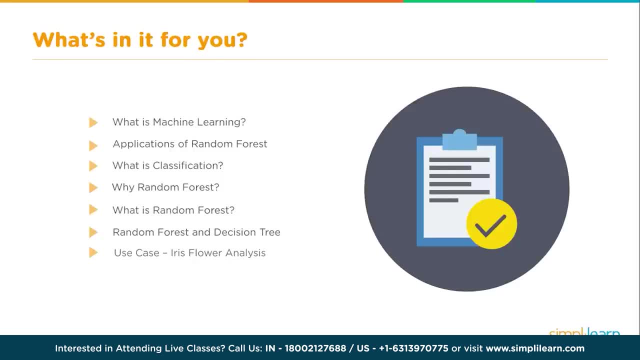 Now if you don't know what any of these terms mean or where we're going with this, don't worry. We're going to cover all the basics and have you up and running and even have you doing some basic script in Python by the end. 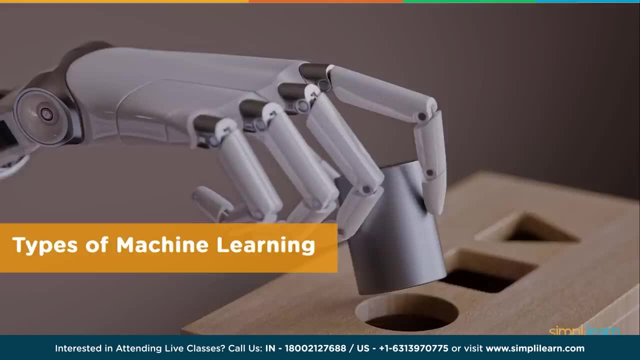 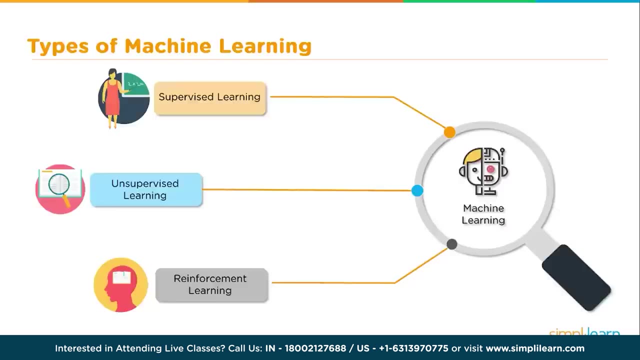 Let's take a closer look at types of machine learning. Specifically, we're going to look at where the decision tree fits in with the different machine learning packages out there. We'll start with the basic types of machine learning. There's supervised learning, where you have lots of data and you're able to train your models. 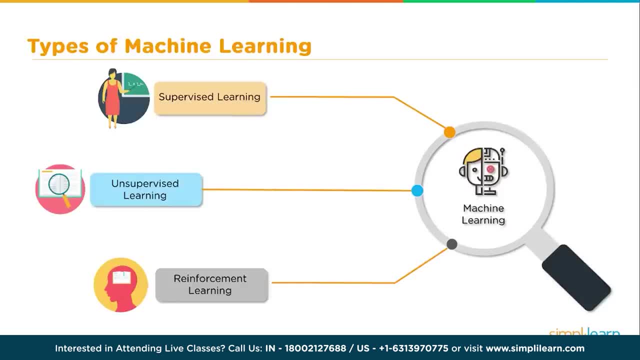 There's unsupervised learning, where it has to look at the data and then divide it based on its own algorithms without having any training. And then there's reinforcement learning, where you get a plus or negative if you have the answer correct. 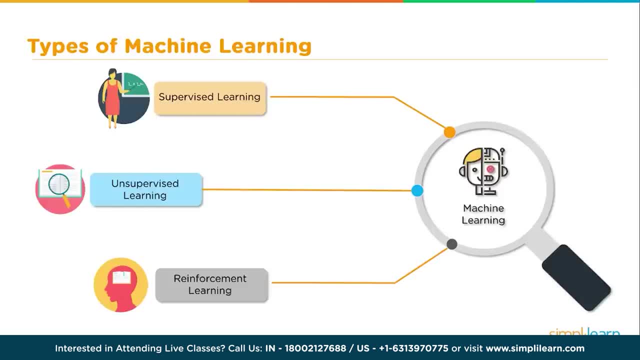 This particular tool belongs to the supervised learning. Let's take a closer look at that, what that means in supervised learning. Supervised learning falls into two groups: classification and regression. We'll talk about regression a little later and how that differs. This particular format goes underneath classification. 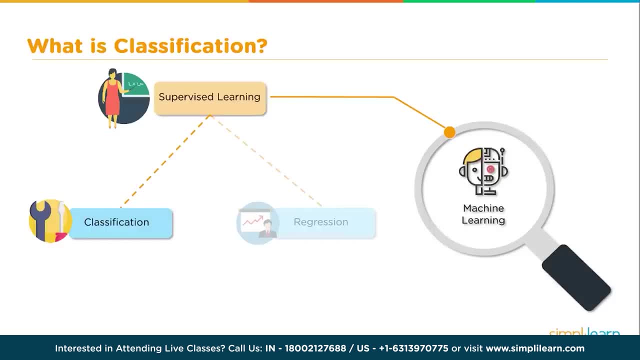 So we're looking at supervised learning and classification in the machine learning tools. Classification is a kind of problem where the outputs are categorical in nature, like yes or no, true or false or zero or one. In that particular framework there's the KNN, where the NN stands for nearest neighbor. 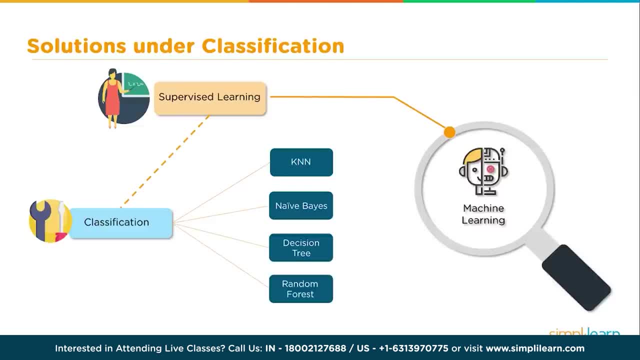 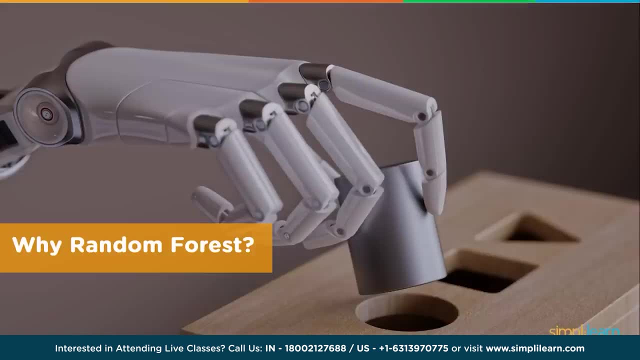 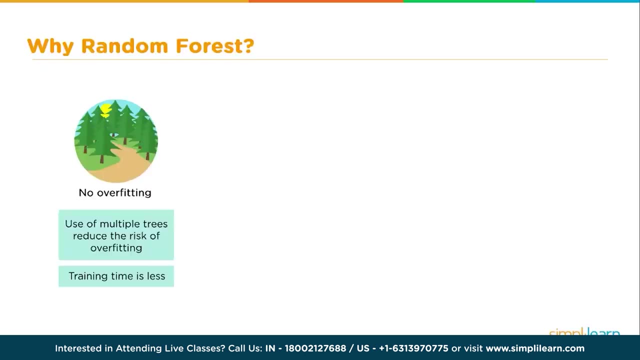 NAVBase, the decision tree, which is part of the random forest that we're studying today. So why random forest? It's always important to understand why we use this tool over the other ones. What are the benefits, here And so with the random forest? the first one is there's no overfitting. 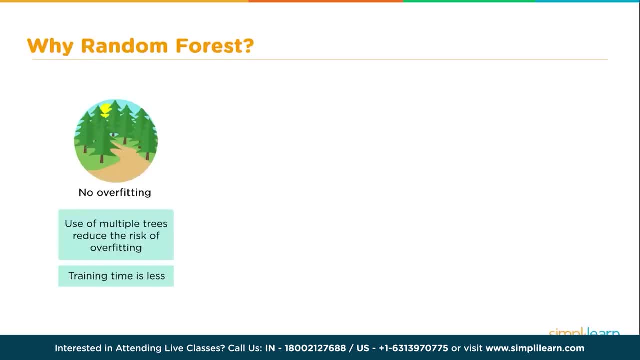 If you use of multiple trees, reduce the risk of overfitting. Training time is less. Overfitting means that we have fit the data so close to what we have as our sample that we pick up on all the weird parts And instead of predicting the overall data. 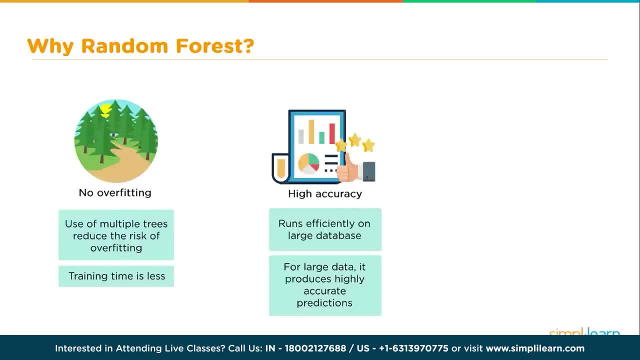 you're predicting the weird stuff which you don't want. High accuracy Runs efficiently in large database For large data. it produces highly accurate data. In today's world of big data, this is really important And this is probably where it really shines. 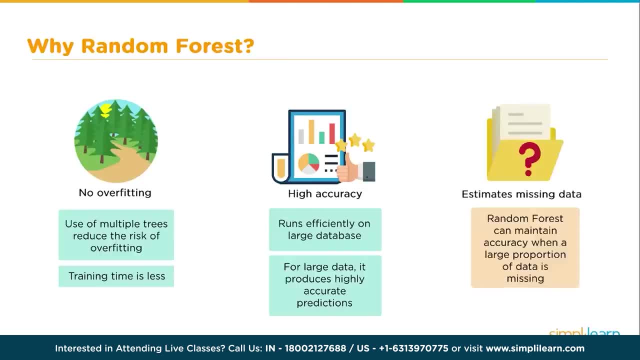 This is where why random forest really comes in. It estimates missing data. Data in today's world is very messy, So when you have a random forest, it can maintain the accuracy when a large proportion of the data is missing. What that means is if you have data that comes in from five or six different areas. 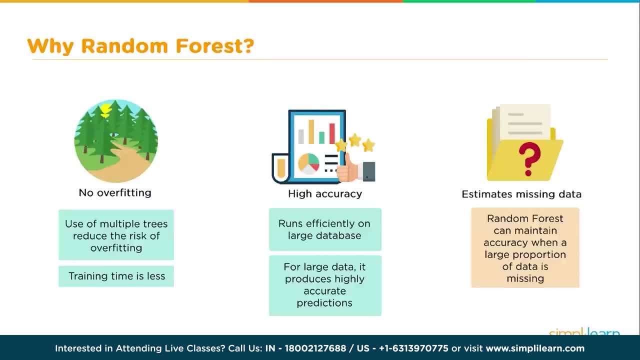 and maybe they took one set of statistics in one area and they took a slightly different set of statistics in the other. So they have some of the same shared data, But one is missing: the number of children in the house. if you're doing something over demographics, 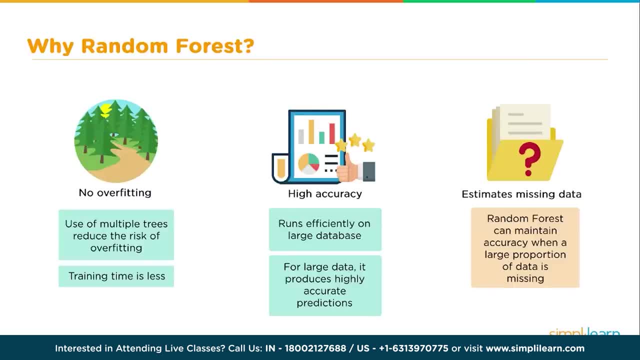 And the other one is missing- the size of the house. It will look at both of those separately and build two different trees, And then it can do a very good job of guessing which one fits better. even though it's missing that data, Let us dig deep into the theory of exactly how it works. 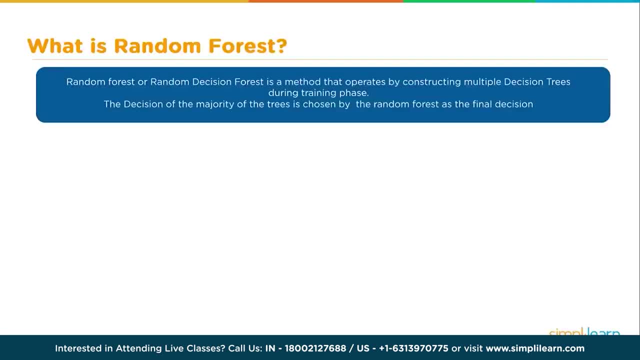 And let's look at what is a random forest. A random forest or a random decision forest is a method that operates by constructing multiple decision trees. The decision of the majority of the trees is chosen by the random forest as the final decision. 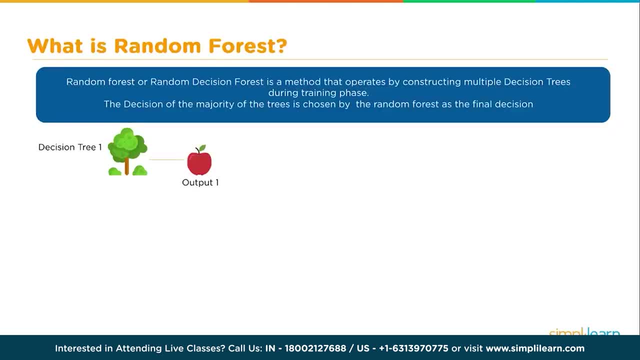 And we have some nice graphics here. We have a decision tree, And they actually use a real tree to denote the decision tree, which I love, And, given a random, some kind of picture of a fruit, this decision tree decides that the output is: it's an apple. 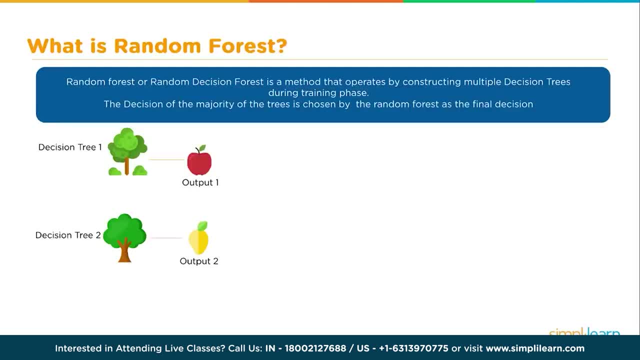 And we have a decision tree two, where we have that picture of the fruit, goes in And this one decides that it's a lemon, And the decision tree tree gets another image and it decides it's an apple. And then this all comes together in what they call the random forest. 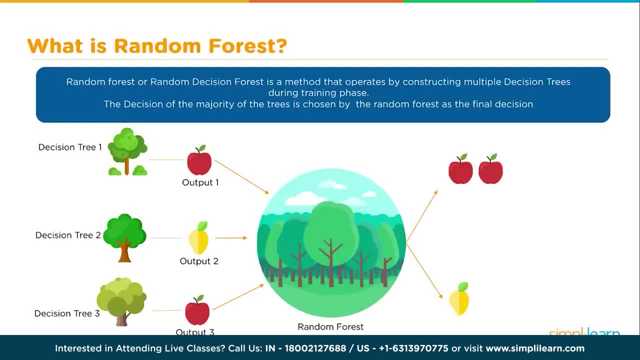 And this random forest then looks at it and says: OK, I got two votes for apple, one vote for lemon. The majority is apples, so the final decision is apples. To understand how the random forest works, we first need to dig a little deeper. 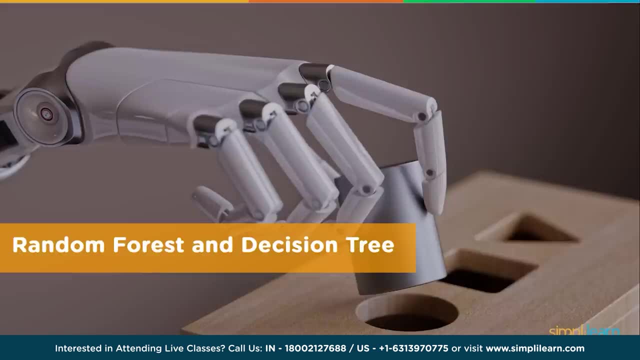 and take a look at the random forest and the actual decision tree and how it builds that decision tree, And looking closer at how the individual decision trees work. we'll go ahead and continue to use the fruit example, since we're talking about trees and forests. 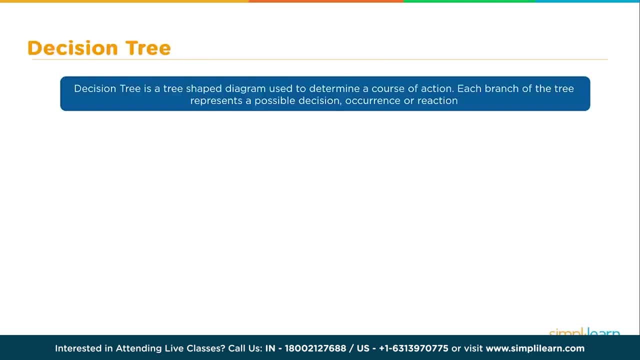 A decision tree is a tree shaped diagram used to determine a course of action. Each branch of the tree represents a possible decision occurrence or reaction. So in here we have a bowl of fruit And if you look at that, it looks like they switched from lemons to oranges. 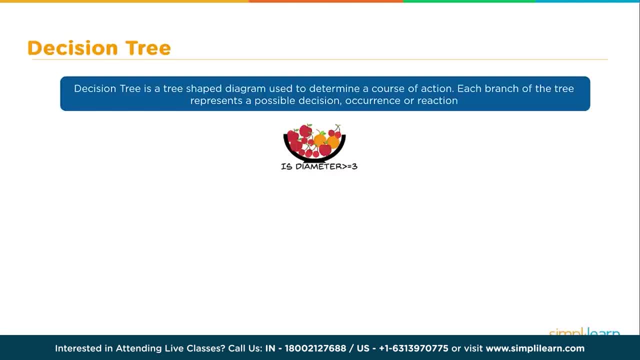 We have oranges, cherries and apples, And the first decision of the decision tree might be is the diameter greater than or equal to three, And if it says false, it knows that they're cherries, because everything else is bigger than that. 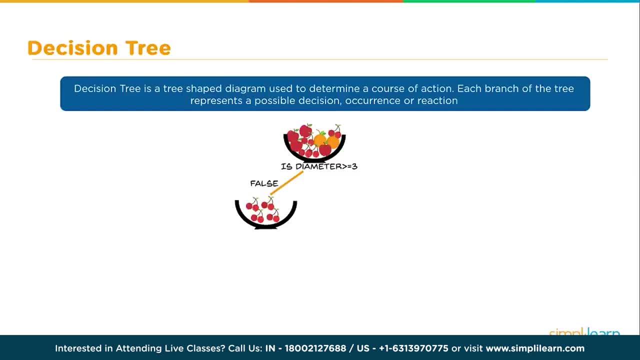 So all the cherries fall into that decision. So we have all that data, we're training, We can look at that. We know that that's what's going to come up. Is the color orange? Well, it goes. hmm, orange or red? 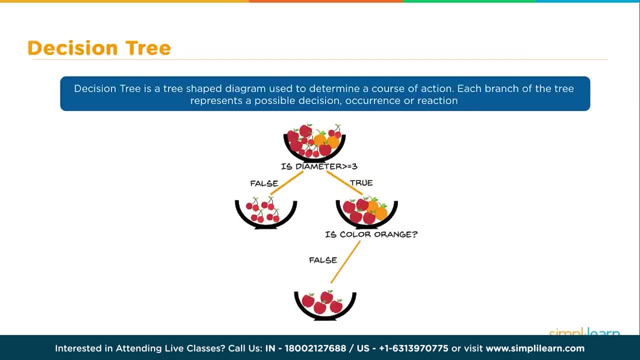 Well, if it's true, then it comes out as the orange, And if it's false, that leaves apples. So in this example, it sorts out the fruit in the bowl or the images of the fruit: A decision tree. these are very important terms. 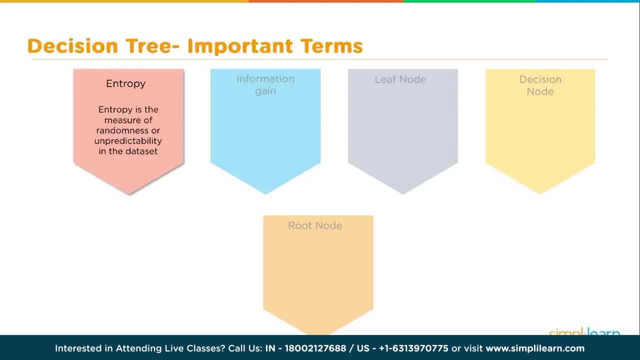 to know, because these are very central to understanding the decision tree and when working with them. The first is entropy. Everything on the decision tree and how it makes a decision is based on entropy. Entropy is a measure of randomness or unpredictability in the data set. 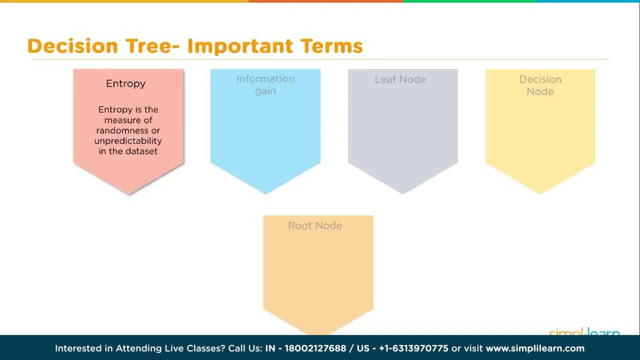 Then they also have information gain: the leaf node, the decision node and the root node. We'll cover these other four terms as we go down the tree, But let's start with entropy. So, starting with entropy, We have here a high amount of randomness. 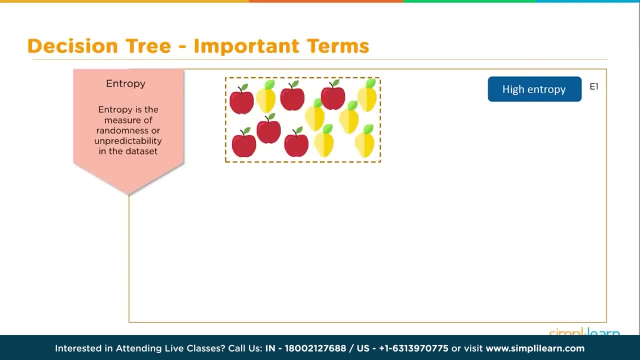 What that means is that, whatever is coming out of this decision, if it was going to guess based on this data, it wouldn't be able to tell you whether it's a lemon or an apple. It would just say it's a fruit. So the first thing we want to do is we want to split this apart. 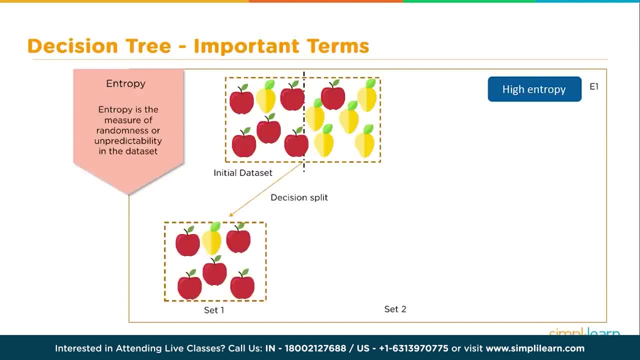 And we take the initial data set and we're going to create a data set one and a data set two. We just split it in two And if you look at these new data sets after splitting them, The entropy of each of those sets is much less. 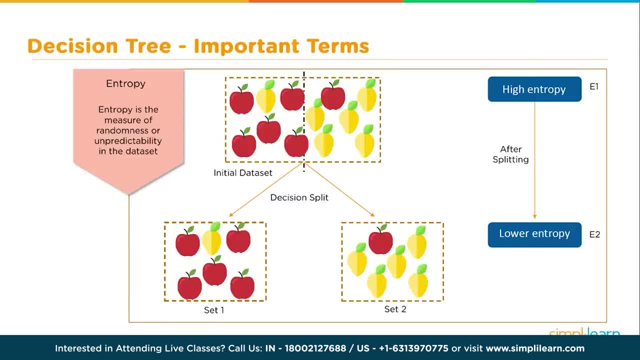 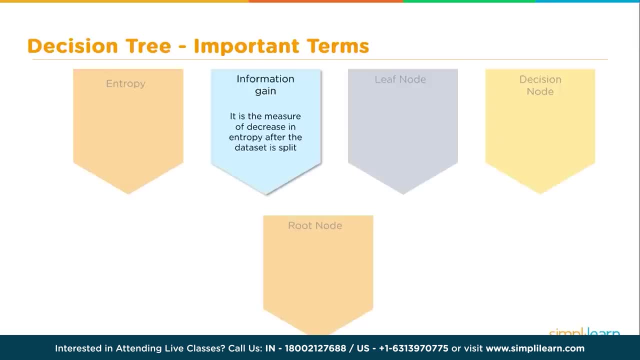 So for the first one, whatever comes in there, it's going to sort that data and it's going to say, okay, if this data goes this direction, it's probably an apple, And if it goes into the other direction, it's probably a lemon. 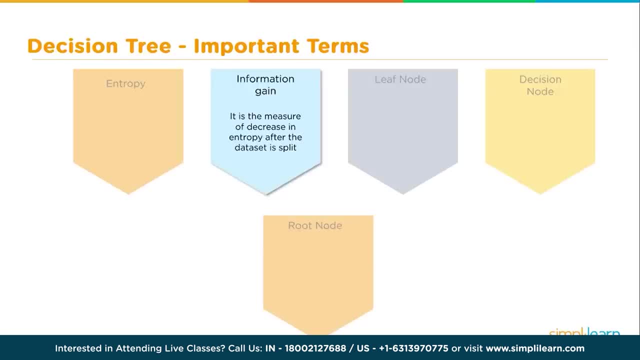 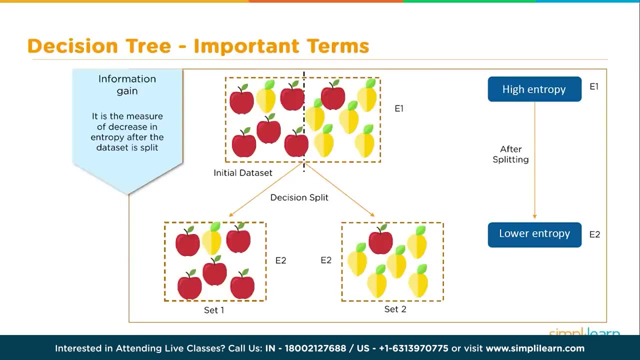 So that brings us up to information gain. It is the measure of decrease in the entropy after the data set is split. What that means in here is that we've gone from one set which has a very high entropy to two lower sets of entropy. 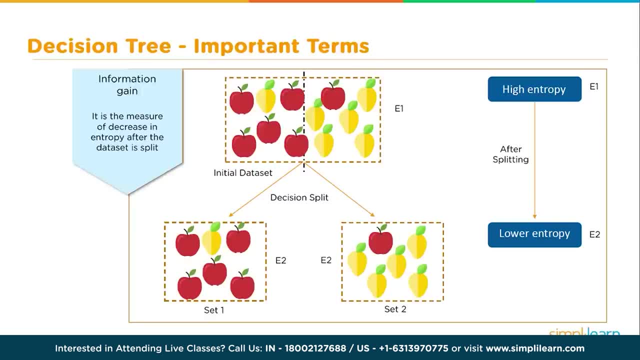 And we've added in the values. We've added in the values of E1 for the first one and E2 for the second, two which are much lower, And so that information gain is increased greatly in this example, And so you can find that the information gain simply equals decision E1 minus E2.. 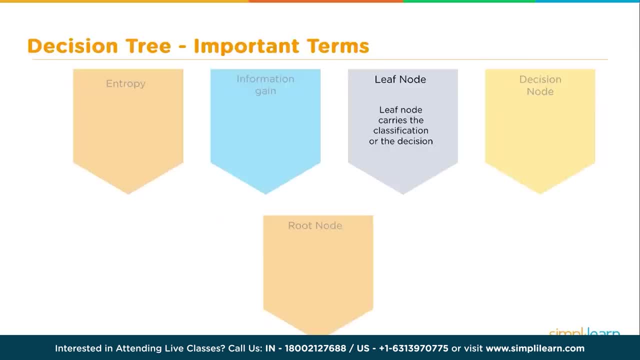 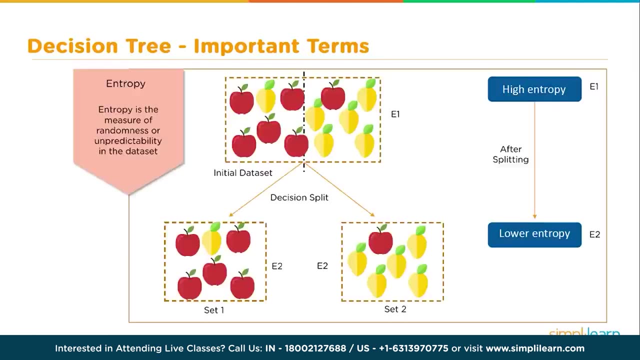 As we're going down our list of definitions, we'll look at the leaf node And the leaf node carries the classification or the decision. So we look down here to the leaf node, We finally get to our decision. So our set 1 or our set 2.. 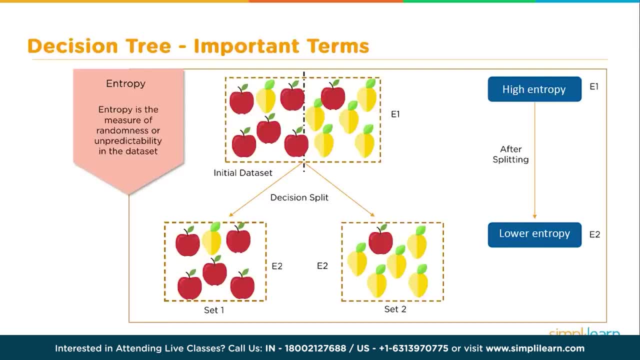 When it comes down there and it says, OK, this object's gone into set 1, if it's gone into set 1, it's going to be split by some means And we'll either end up with apples on the leaf node or a lemon on the leaf node. 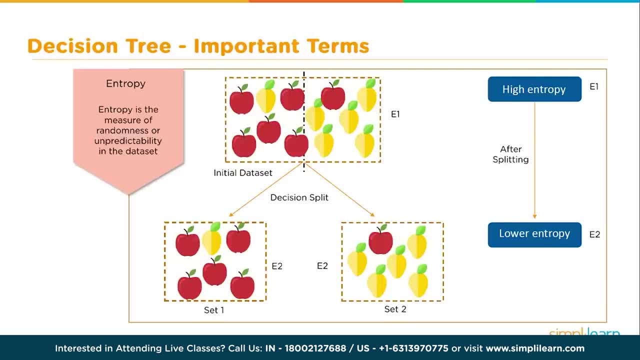 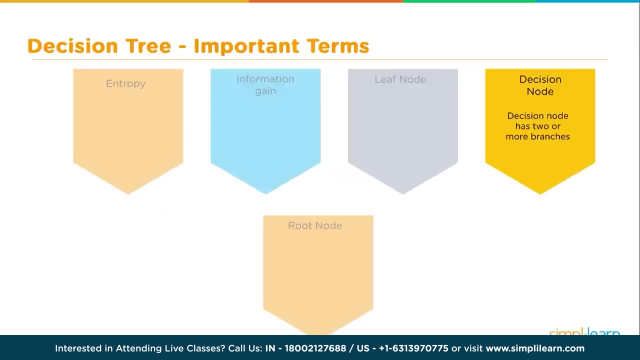 And on the right it'll either be an apple or lemons. Those leaf nodes are those final decisions or classifications. That's the definition of leaf node in here. If we're going to have a final leaf where we make the decision, we should have a name. 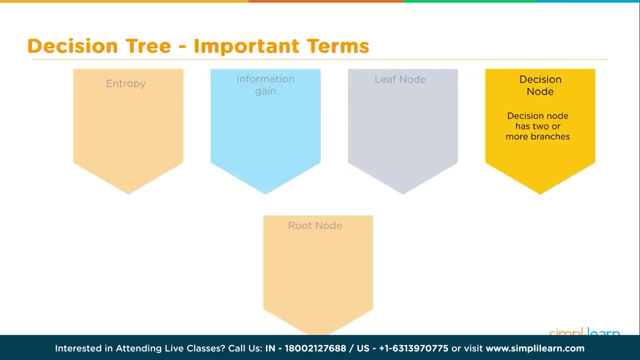 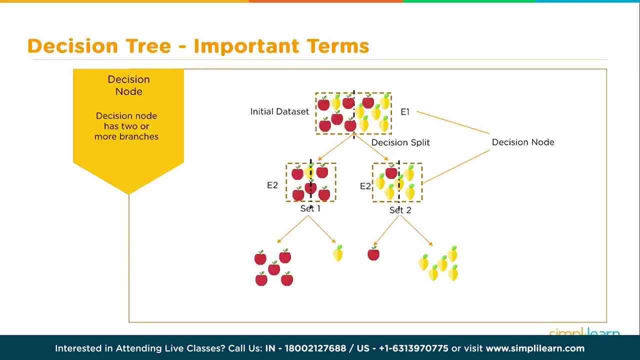 for the nodes above it And they call those decision nodes A decision node. decision node has two or more branches And you can see here where we have the five apples and one lemon and in the other case the five lemons and one apple. they have to make a choice of which tree it goes down based. 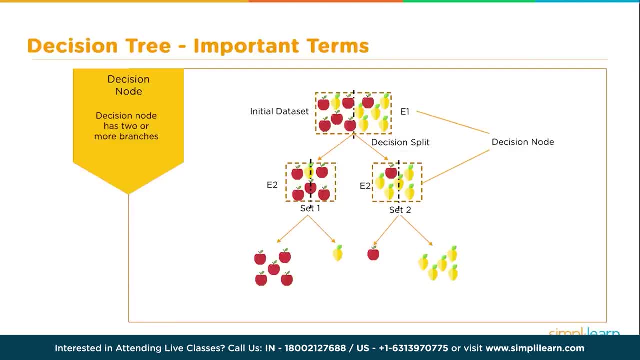 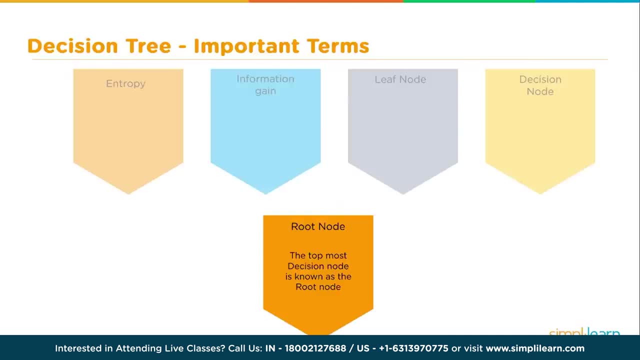 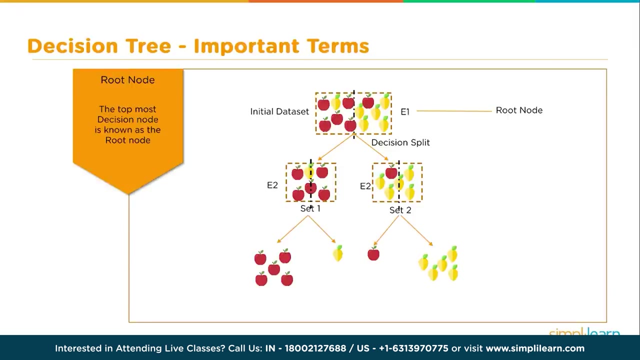 on some kind of measurement or information given to the tree. And that brings us to our last definition, the root node. the top, most decision node is known as the root. the root node: This is where you have all of your data and you have your first decision it has to make, or the first split in information. 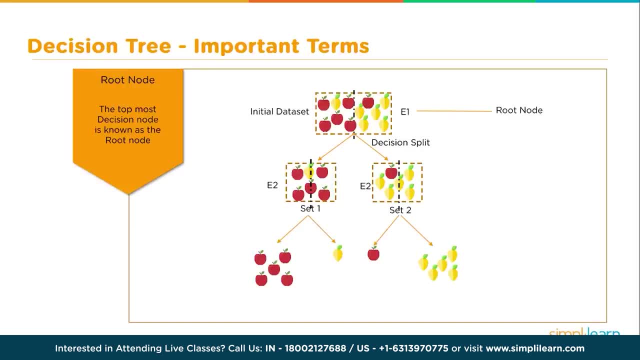 So far we've looked at a very general image, with the fruit being split. Let's look and see exactly what that means to split the data and how do we make those decisions on there. Let's go in there and find out. how does a decision tree work? 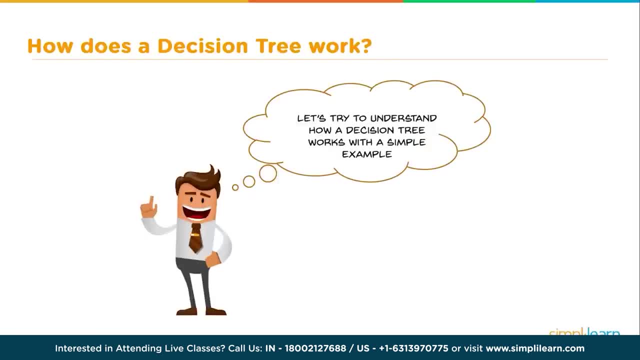 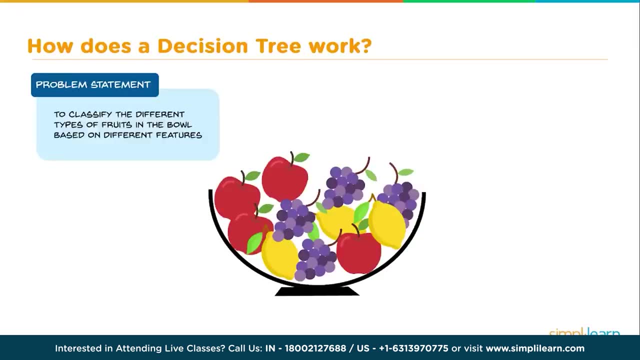 So let's try to understand this and let's use a simple example and we'll stay with the fruit. We have a bowl of fruit and so let's create a problem statement and the problem is we want to classify the different types of fruits in the bowl based on different features. 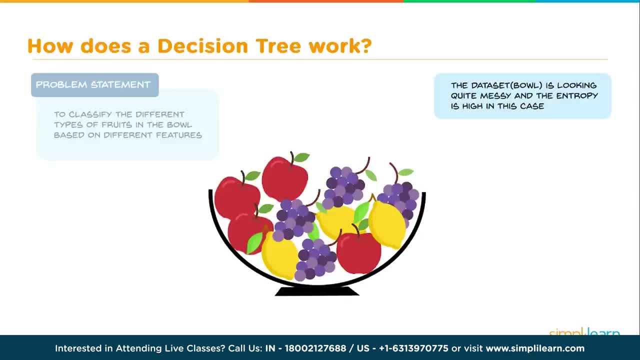 The data set in the bowl is looking quite messy, and the entropy is high in this case. So if this bowl was our decision maker, it wouldn't know what choice to make. It has so many choices. Which one do you pick? Apple, grapes or lemons, And so we look in. here We're going to start with a training set. 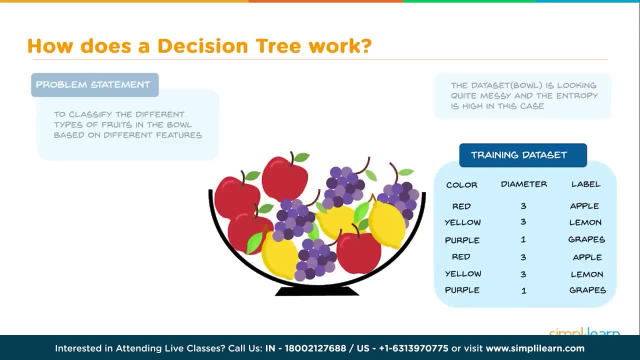 so this is our data, that we're training our data with, and we have a number of options here We have the color and under the color we have red, yellow purple. We have a diameter 3, 3, 1, 3, 3, 1 and we have a label. 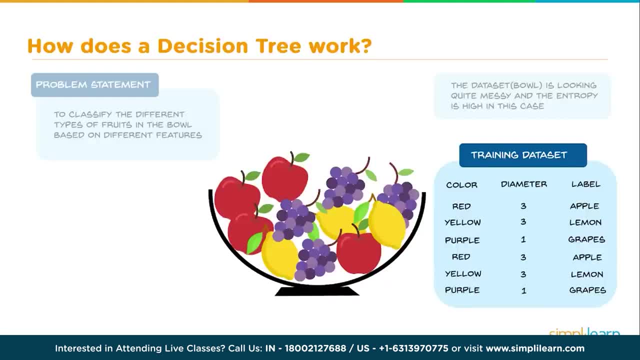 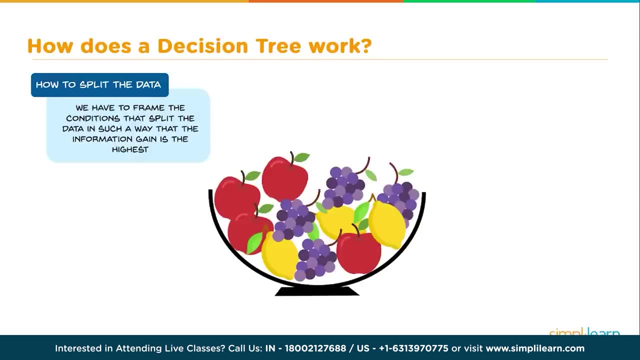 apple lemon grapes. apple lemon grapes. And how do we split the data? We have to frame the conditions to split the data in such a way that the information gain is the highest. It's very key to note that we're looking for the best gain. 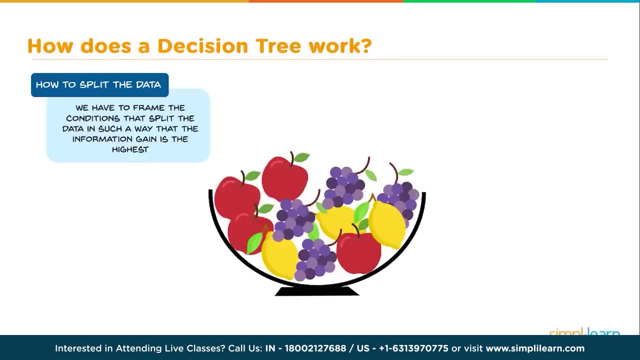 We don't want to just start sorting out the smallest piece in there. We want to split it the biggest way we can, And so we measure this decrease in entropy. that's what they call it entropy. there's our entropy after splitting, And now we'll try to choose a condition that gives us the 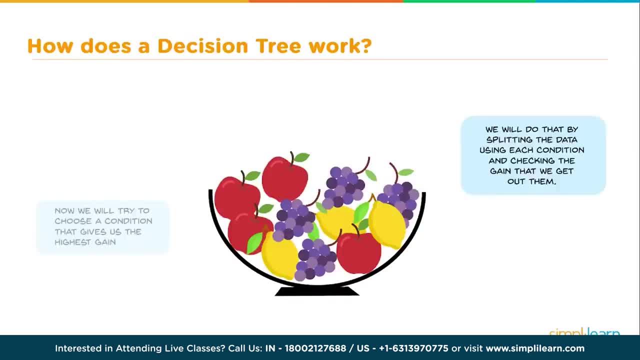 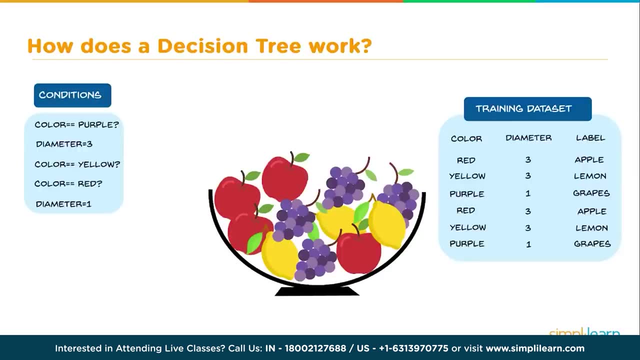 highest gain. We will do that by splitting the data, using each condition and checking the gain that we get out of them. The conditions that give us the highest gain will be used to make the first split. So let's take a look at these different conditions. We have color. we have 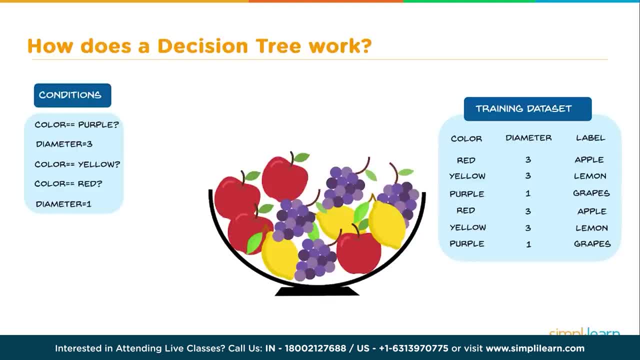 diameter. and if we look underneath that, we have a couple different values. We have: diameter equals 3,. color equals yellow, red, diameter equals 1.. And when we look at that, you'll see over here we have 1,, 2,, 3,, 4, 3's. 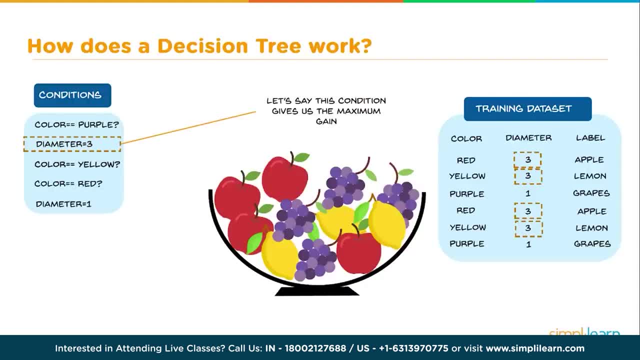 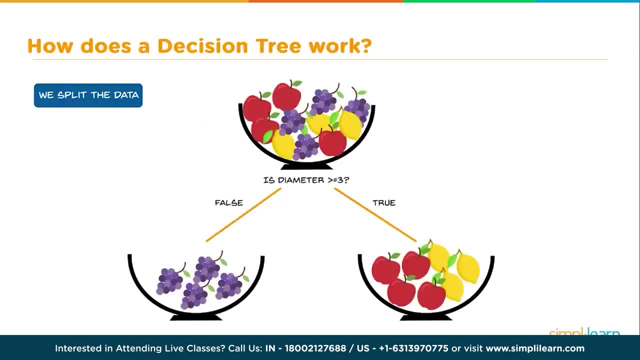 That's a pretty hard selection. So let's say the condition gives us the maximum gain of 3. So we have the most pieces fall into that range. So our first split from our decision node is we split the data based on the diameter. 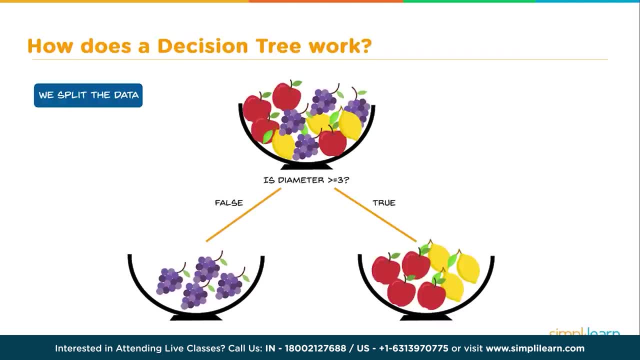 Is it greater than or equal to 3?? If it's not, that's false- it goes into the great bowl. If it's true, it goes into a bowl full of lemon and apples. The entropy after splitting has decreased considerably, So now we can make two decisions. If you look at it, there's very much. 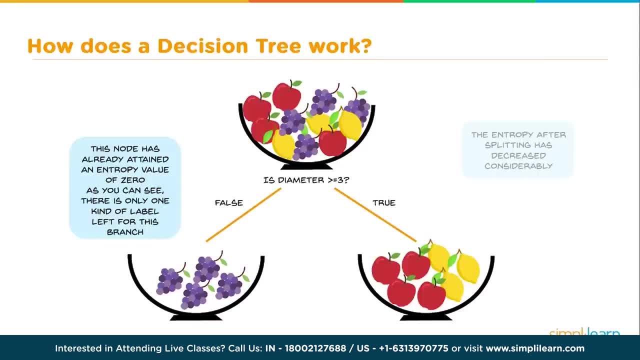 less chaos going on there. This node has already attained an entropy value of zero. as you can see, There's only one kind of label left for this branch, So no further splitting is required for this node. However, this node on the right still requires a split to decrease the entropy further. 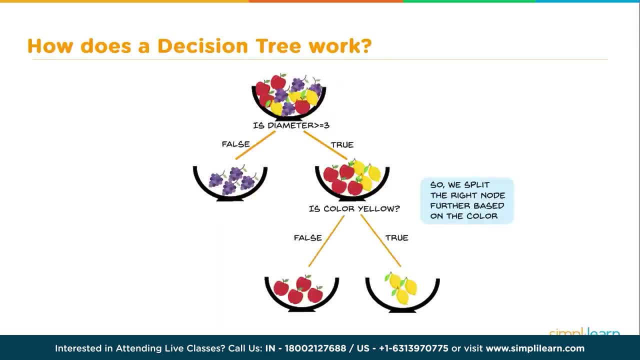 So we split the right node further based on color. If you look at this, if I split it on color, that pretty much cuts it right down the middle. It's the only thing we have left in our choices of color and diameter too. 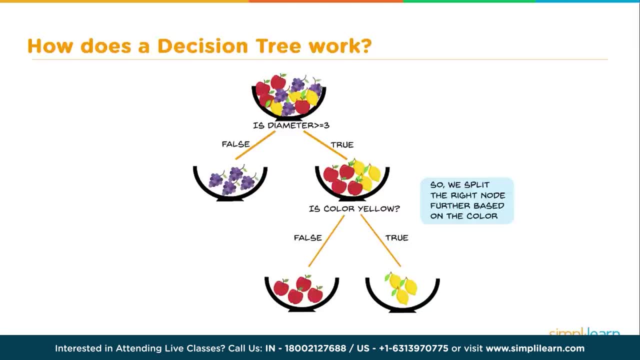 And if the color is yellow, it's going to go to the right bowl, And if it's false, it's going to go to the left bowl. So the entropy in this case is now zero. So now we have three bowls with zero entropy. There's only one type of data in. 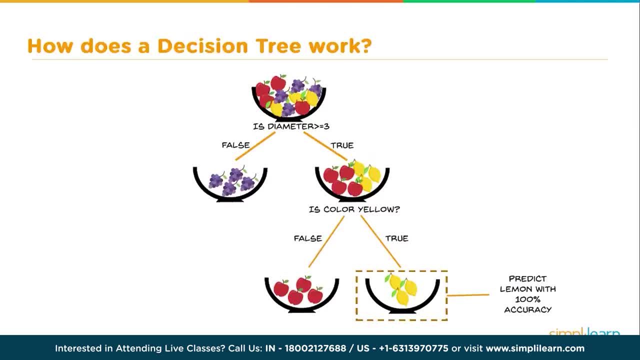 each one of those bowls. So we can predict a lemon with a hundred percent accuracy And we can predict the apple also with a hundred percent accuracy, Along with our grapes up there. So we've looked at kind of a basic tree in our forest. 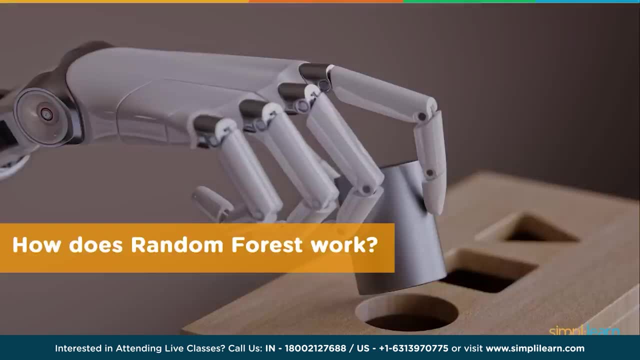 But what we really want to know is: how does a random forest work as a whole? So to begin our random forest classifier, let's say we already have built three trees And we're going to start with the first tree that looks like this: 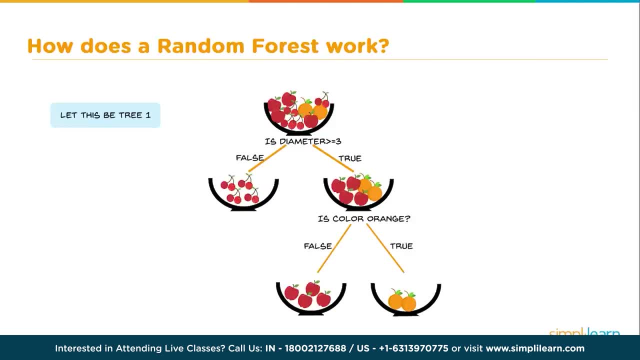 Just like we did in the example, this tree looks at the diameter. If it's greater than or equal to three, it's true. otherwise it's false. So one side goes to the other side and the other side goes to the other side. 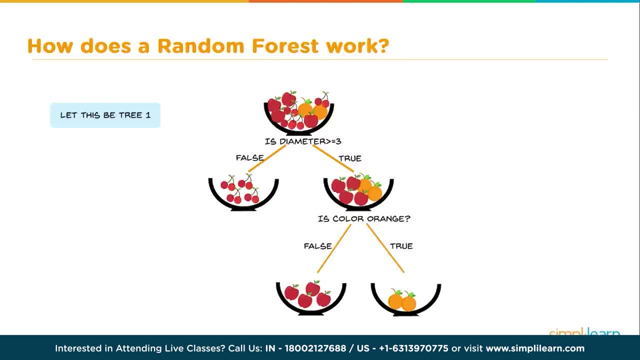 So one side goes to the other side and the other side goes to the other side. One side goes to the smaller diameter, one side goes to the larger diameter, And if the color is orange, it's going to go to the right. true, We're using oranges now instead of lemons. 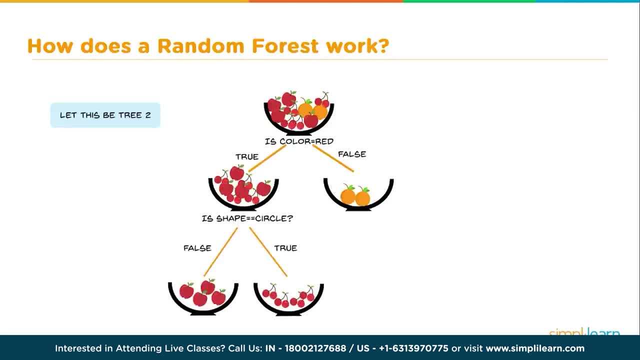 And if it's red it's going to go to the left. false. We build a second tree, very similar, but it's split differently. Instead of the first one being split by diameter, this one when they created it. if you look at that first bowl, it has a lot of 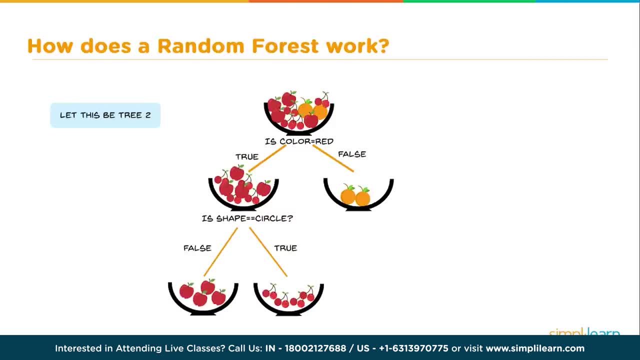 red objects. So, it says, is the color red? Because that's going to bring our entropy down the fastest. And so, of course, if it's true, it goes to the left, If it's false, it goes to the right. And then it looks at the shape. 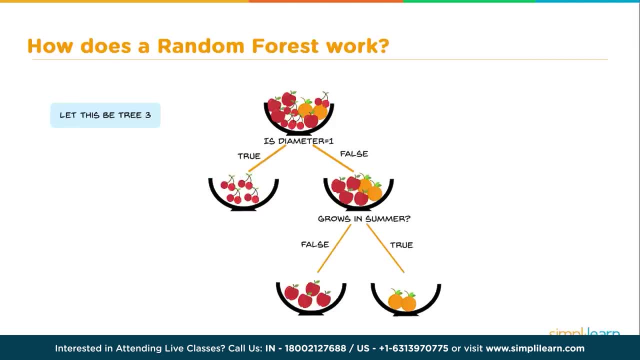 false or true, and so on and so on. And tree three is the diameter equal to one, And it came up with this because there's a lot of cherries in this bowl, So that would be the biggest split on. there is the diameter equal to one. 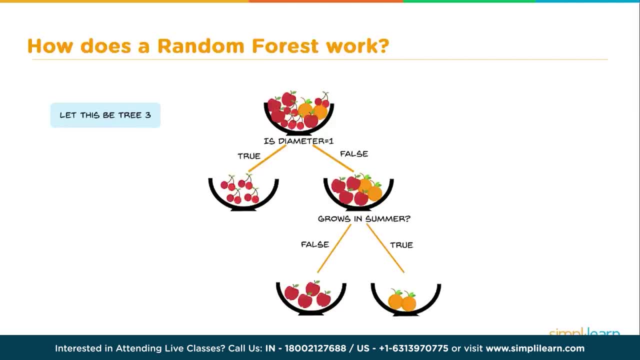 That's going to drop the entropy the quickest. And, as you can see, it splits it into true. if it goes false- and they've added another category: does it grow in the summer? And if it's false, it goes off to the left. If it's true, it goes off to the right. 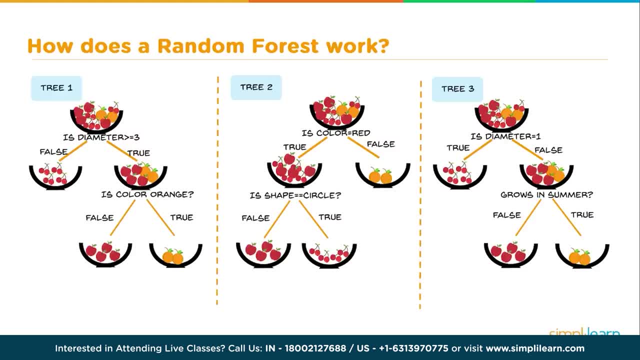 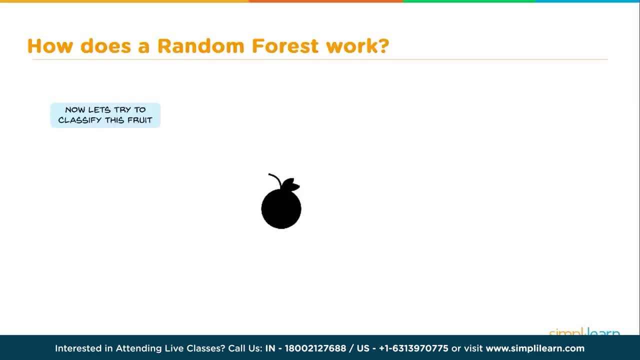 Let's go ahead and bring these three trees so you can see them all in one image. So this would be three completely different trees categorizing a fruit, And let's take a fruit. Now let's try this And this fruit. if you look at it, we've blackened it out. 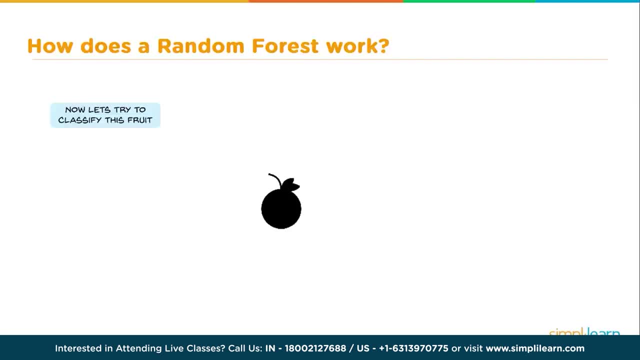 You can't see the color on it, so it's missing data. Remember, one of the things we talked about earlier Is that a random forest works really good if you're missing data, if you're missing pieces. So this fruit has an image, but maybe the person had a black and white. 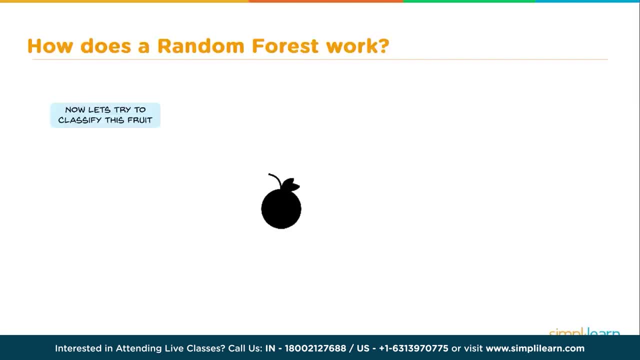 camera. when they took the picture- And we're going to take a look at this and it's going to have- they put the color in there. so ignore the color down there. But the diameter equals three. We find out it grows in the summer- equals yes. 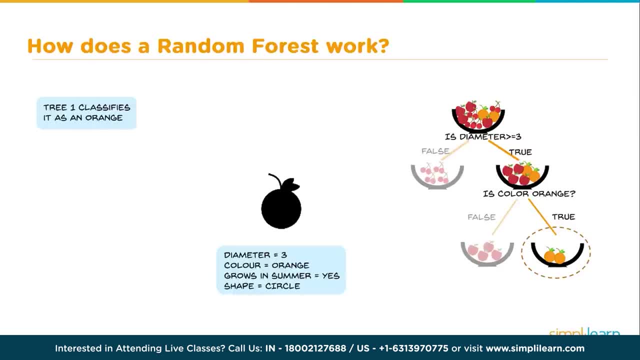 And the shape is a circle, And if you go to the right you can look at what one of the decision trees did. This is the third one. Is the diameter greater than or equal to three? Is the color orange? Well, it doesn't really know on this one, but if you look at the value, it'd say true and it'd go to the right. 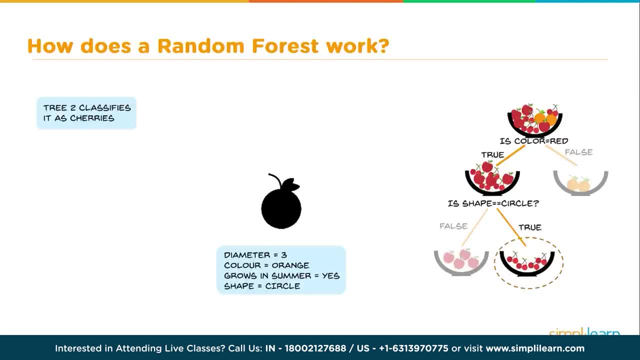 Tree. two classifies it as cherries. Is the color equal- red. Is the shape: a circle? True, it is a circle. So this would look at it and say, oh, that's a cherry. And then we go to the other classifier and it says: is the diameter equal one? 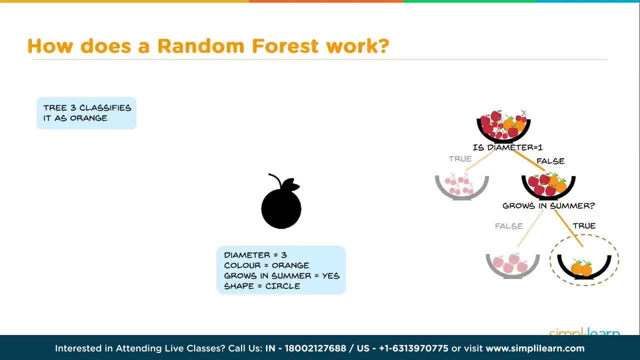 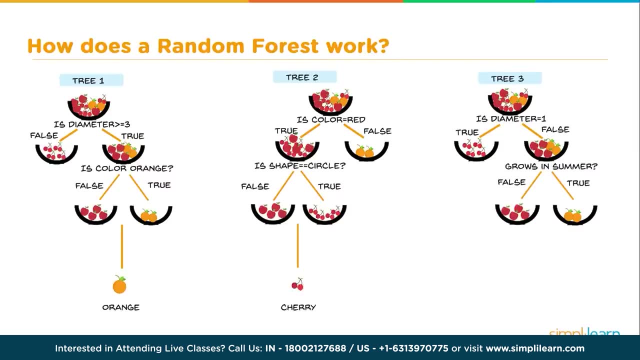 Well, that's false. Does it grow in the summer? True, So it goes down and looks at it as oranges. So how does this random forest work? The first one says it's an orange, The second one said it was a cherry. 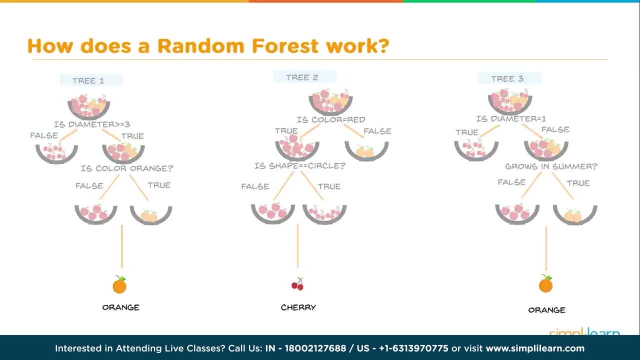 And the third one says: hmm, it's an orange. And you can guess that if you have two oranges and one says it's a cherry, when you add that all together it's a cherry. And you can guess that if you have two oranges and one says it's a cherry, when you add that all together it's a cherry. 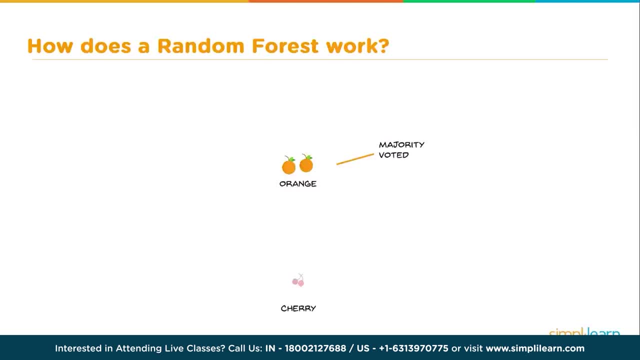 And you can guess that if you have two oranges and one says it's a cherry, when you add that all together it's a cherry, The majority of the vote says orange. So the answer is: it's classified as an orange, even though we didn't know the color and we're missing data on it. 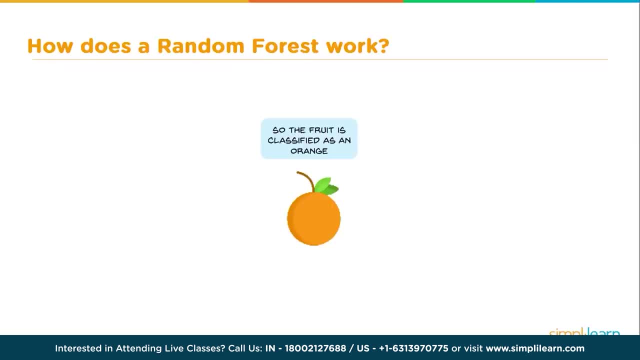 So the answer is it's classified as an orange, even though we didn't know the color and we're missing data on it. I don't know about you, but I'm getting tired of fruit, So let's switch. and I did promise you we'd start looking at a case example and get into some Python coding. 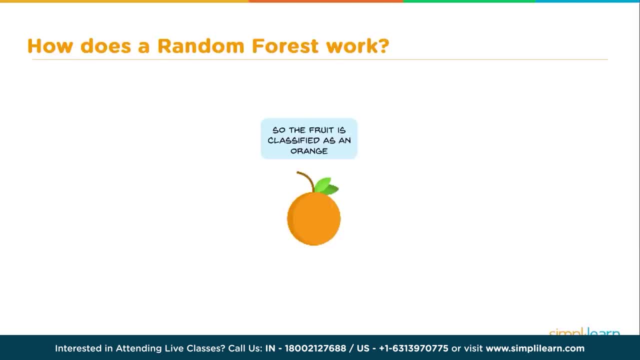 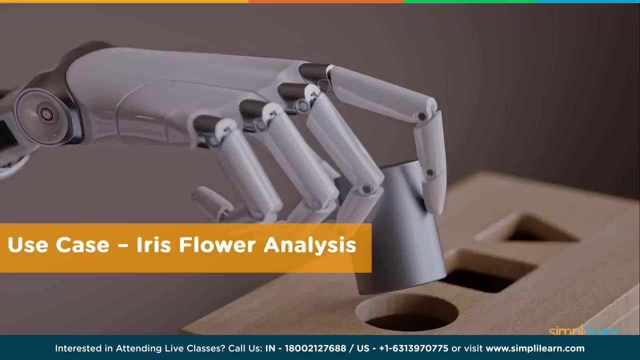 So let's switch, and I did promise you we'd start looking at a case example and get into some Python coding. Today we're going to use the case the iris flower analysis. Ooh, this is the exciting part, as we roll up our sleeves and actually look at some Python coding. 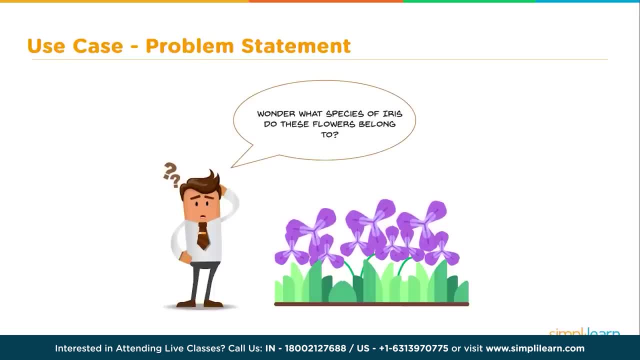 Before we start the Python coding, we need to go ahead and create a problem statement, Wonder: what species of iris do these flowers belong to? Let's try to predict the species of the flowers using machine learning in Python. Let's see how it can be done. 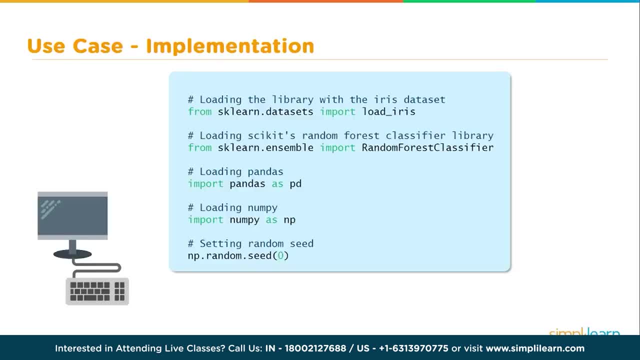 So here we begin to go ahead and implement our Python code, And you'll find that the first half of our implementation is all about organizing and exploring the data coming in. Let's go ahead and take this first step, which is loading the different modules into Python. 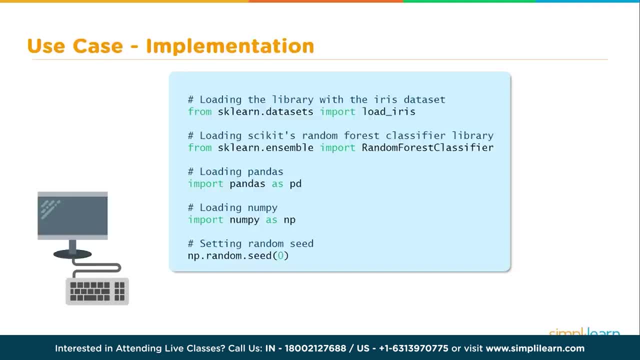 And let's go ahead and put that in our favorite editor. whatever your favorite editor is, In this case I'm going to be using the Anaconda Jupyter Notebook, which is one of my favorites. Certainly there's Notepad++ and Eclipse and dozens of others, or just even using the Python terminal window. 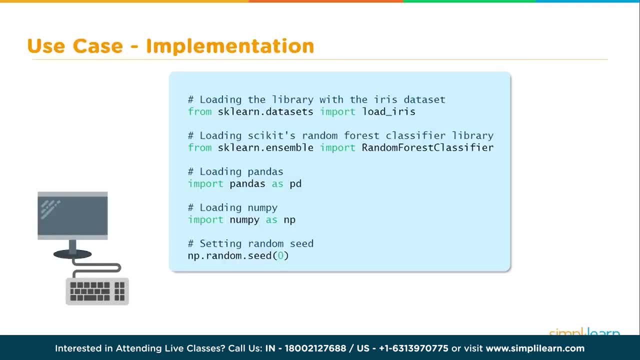 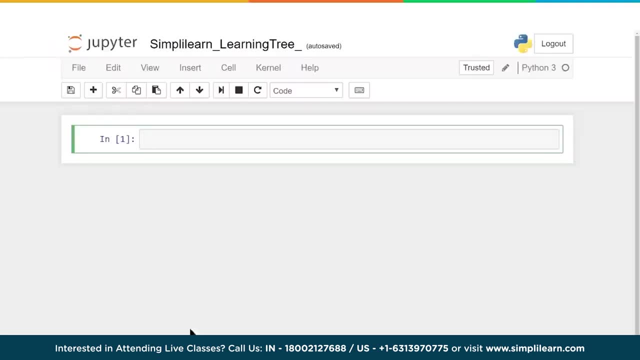 Any of those will work just fine to go ahead and explore this Python coding. So here we go. Let's go ahead and flip over to our Jupyter Notebook, And I've already opened up a new page for Python 3 code And I'm just going to paste this right in there. 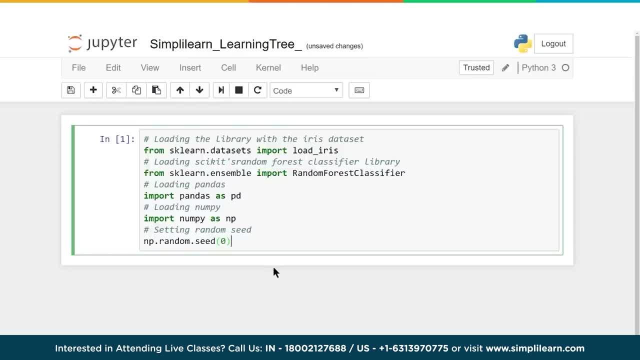 And let's take a look and see what we're bringing into our Python. The first thing we're going to do is, from the sklearndatasets, import load iris. Now, this isn't the actual data. This is just the module that allows us to bring in the data, the load iris. 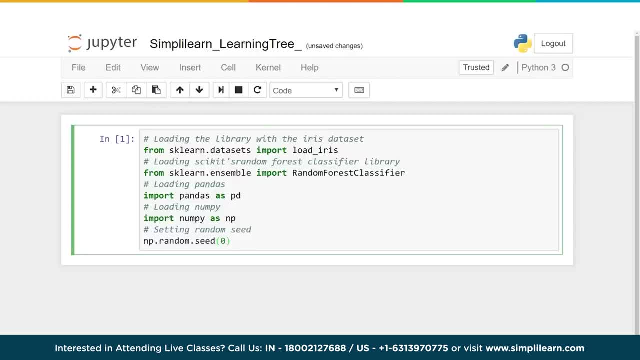 And the iris is so popular- it's been around since 1936 when Ronald Fisher published a paper on it- And they're measuring the different parts of the flower And, based on those measurements, predicting what kind of flower it is. And then, if we're going to do a random forest classifier, we need to go ahead and import a random forest classifier from the sklearn module. 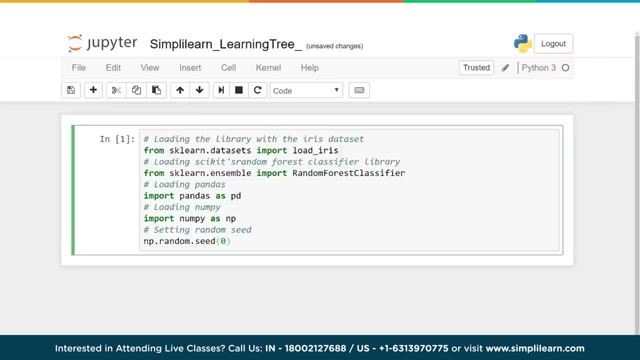 So sklearnensemble, import random forest classifier. And then we want to bring in two more modules, And these are probably the most commonly used modules in Python and data science with any of the other modules that we bring in- And one is going to be pandas- 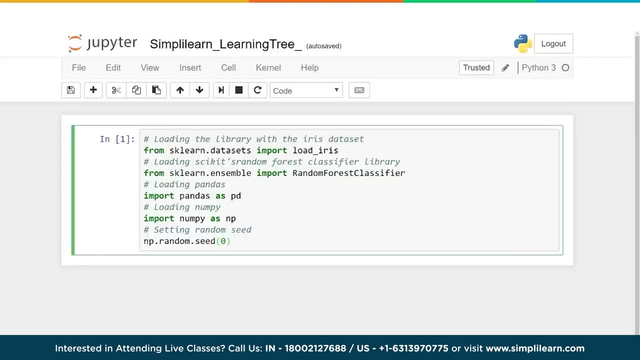 We're going to import pandas as pd. pd is a common term used for pandas And pandas is basically: It creates a data format for us where, when you create a pandas data frame, it looks like an XScale spreadsheet, And you'll see that in a minute when we start digging deeper into the code. 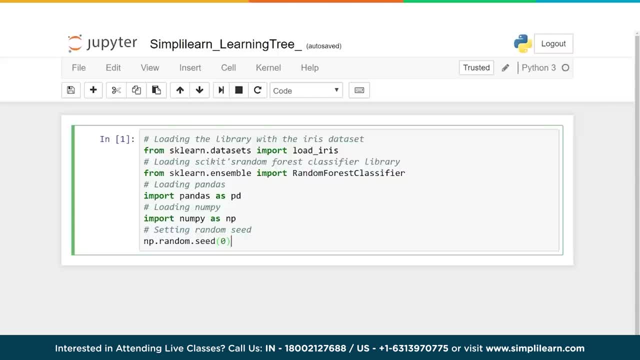 Pandas is just wonderful because it plays nice with all the other modules in there. And then we have numpy, which is our numbers Python, And the numbers Python allows us to do different mathematical sets on here. We'll see right off the bat. 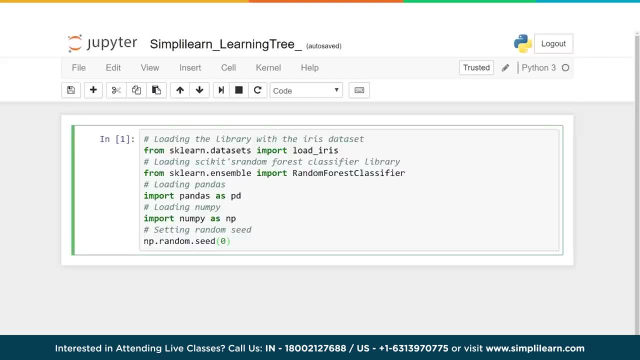 We're going to take our np and we're going to go ahead and seed. the randomness with it was zero. So np random seed is seeding. that is zero. This code doesn't actually show anything. We're going to go ahead and run it because I need to make sure I have all those loaded. 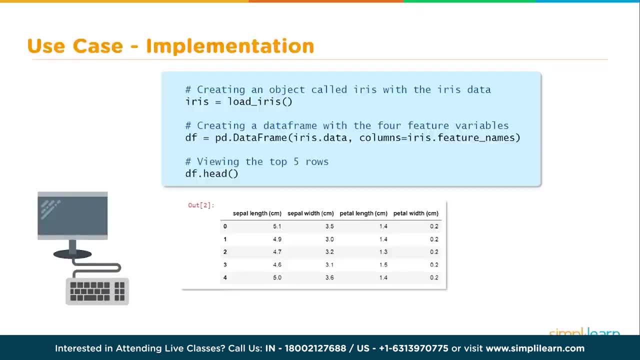 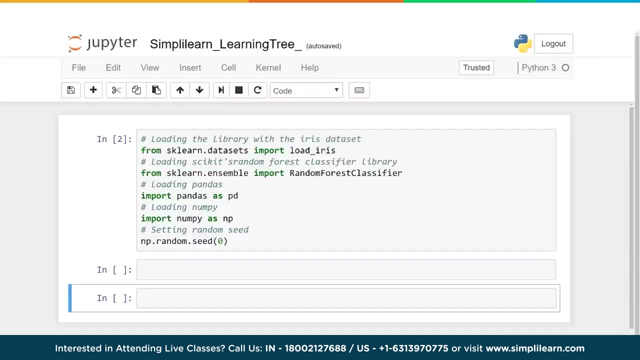 And then let's take a look at the next module on here. The next six slides, including this one, are all about exploring the data. Remember, I told you half of this is about looking at the data and getting it all set. So let's go ahead and take this code right here, the script, and let's get that over into our Jupyter notebook. 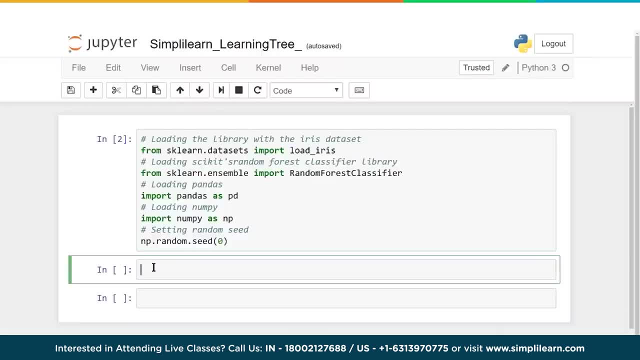 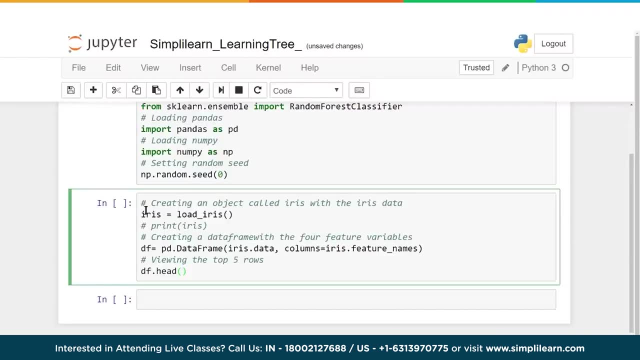 And here we go. We've gone ahead and run the imports And I'm going to paste the code down here And let's take a look and see what's going on. The first thing we're doing is we're actually loading the iris data. 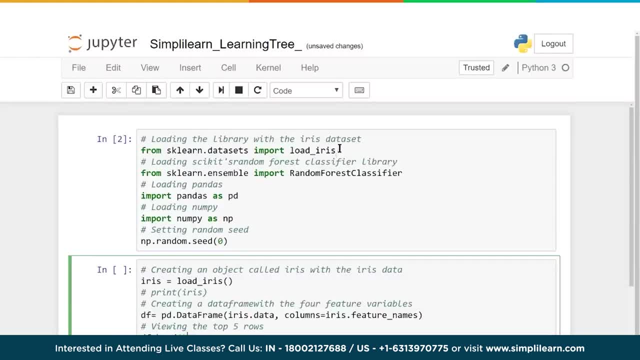 And, if you remember, up here we loaded the module that tells it how to get the iris data. Now we're actually assigning that data to the variable iris And then we're going to go ahead and use the df to define data frame And that's going to equal pd. 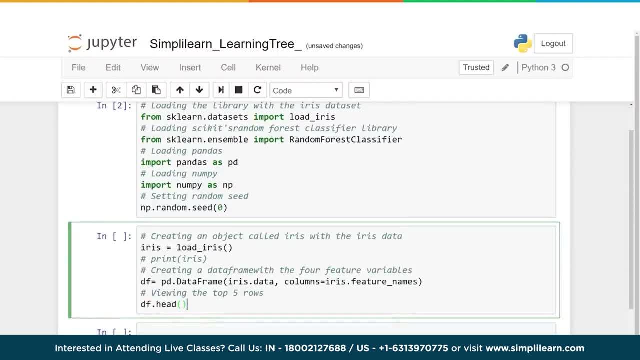 And, if you remember, that's pandas as pd. So that's our pandas And panda data frame. And then we're looking at iris data and columns equals iris feature names, And we're going to do the df head And let's run this so you can understand what's going on here. 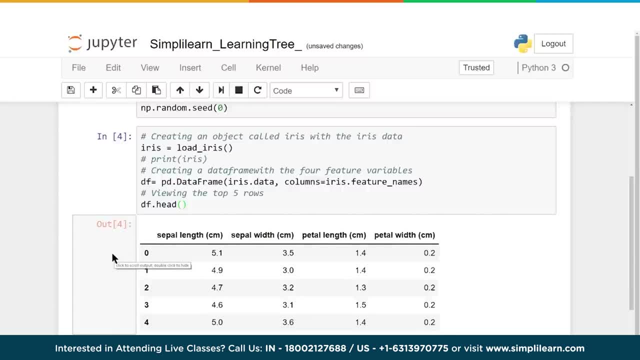 The first thing you want to notice is that our df has created what looks like an Excel spreadsheet, And in this Excel spreadsheet we have set the columns. So up on the top you can see the four different columns, And then we have the data irisdata down below. 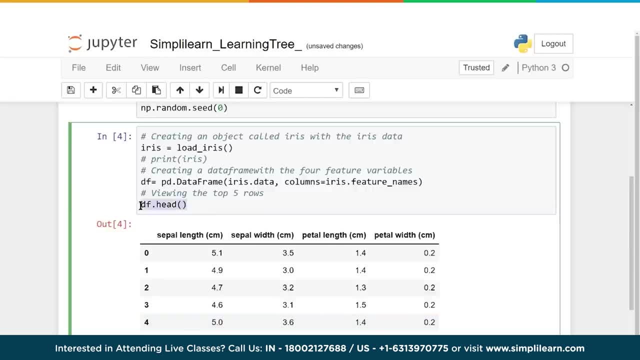 It's a little confusing Without knowing where this data is coming from. we're going to go ahead and set the columns, So let's look at the bigger picture And I'm going to go print. I'm just going to change this for a moment. 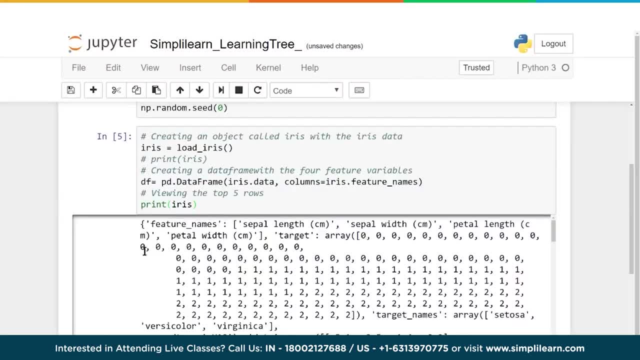 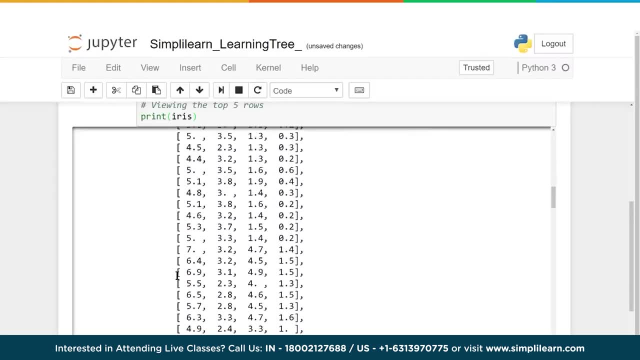 And we're going to print all of iris and see what that looks like. So when I print all of iris I get this long list of information And you can scroll through here and see all the different titles on there. What's important to notice is that, first off, there's brackets at the beginning. 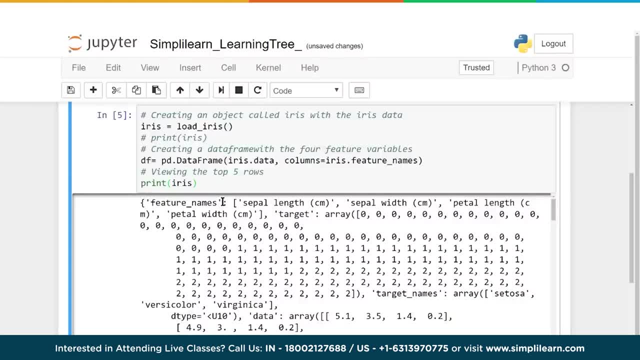 So this is a Python dictionary, And in a Python dictionary you'll have a key Or a label And this label pulls up whatever information comes after it. So feature names which we actually used over here under columns, is equal to an array of sepal length, sepal width. petal length, petal width. 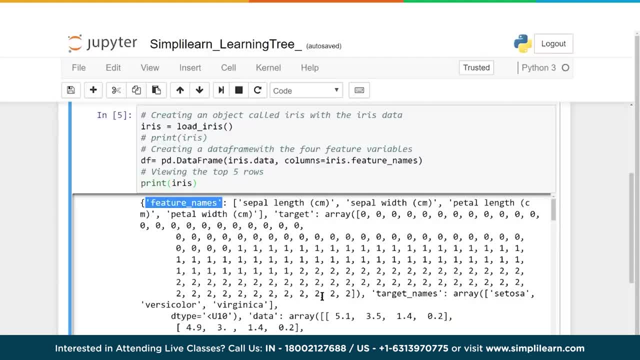 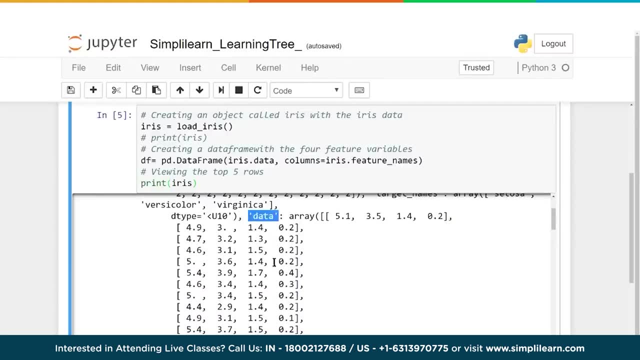 These are the different names they have for the four different columns And if you scroll down far enough, you'll also see data down here. Oh goodness, it came up right towards the top And data is equal to the different data we're looking at. 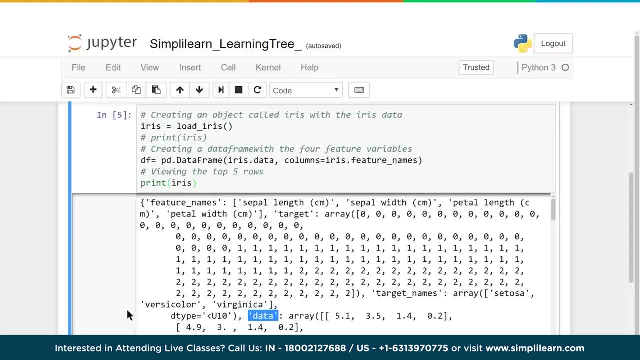 Now there's a lot of other things in here, like target- We're going to be pulling that up in a minute- And there's also the names, the target names, which is further down, And we'll show you that also in a minute. 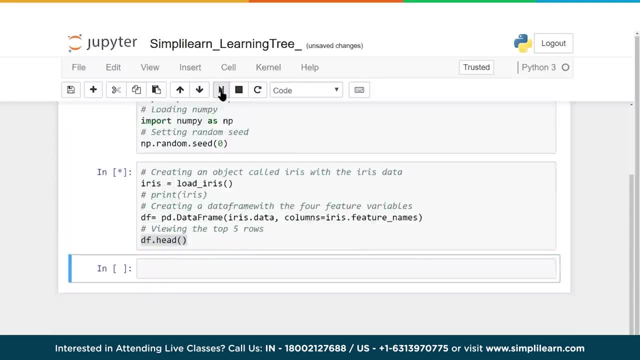 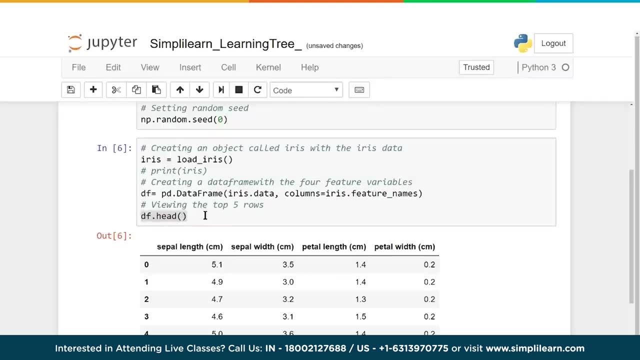 Let's go ahead and set that back to the head. And this is one of the neat features of pandas and panda data frames Is, when you do dfhead or the panda data framehead, it'll print the first five lines of the data set in there. 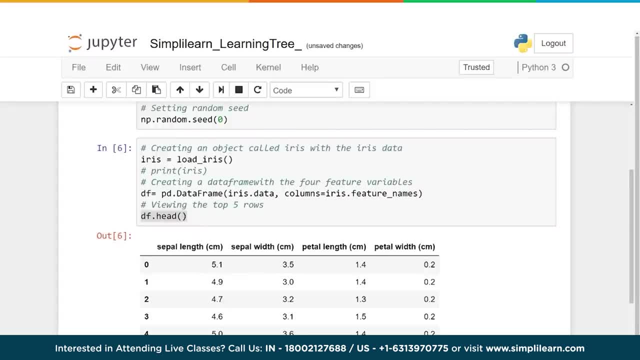 Along with the headers, if you have them. In this case we have the column headers set to iris features And in here you'll see that we have 0,, 1,, 2, 3, 4.. In Python, most arrays always start at 0. 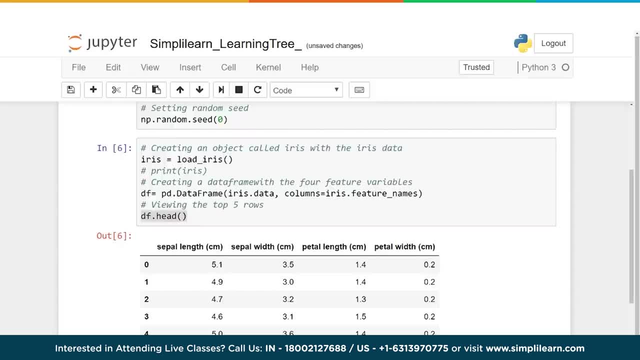 So when you look at the first five, it's going to be 0,, 1,, 2, 3, 4,, not 1, 2,, 3,, 4, 5.. So now we've got our iris data imported into a data frame. 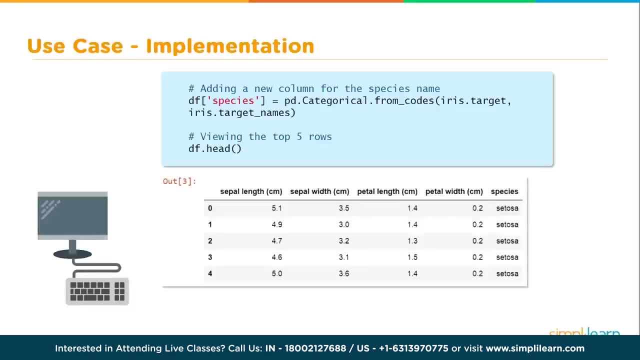 Let's take a look at the next piece of code in here, And so in this section here of the code, we're going to take a look at the target And let's go ahead and get this into our notebook, this piece of code. 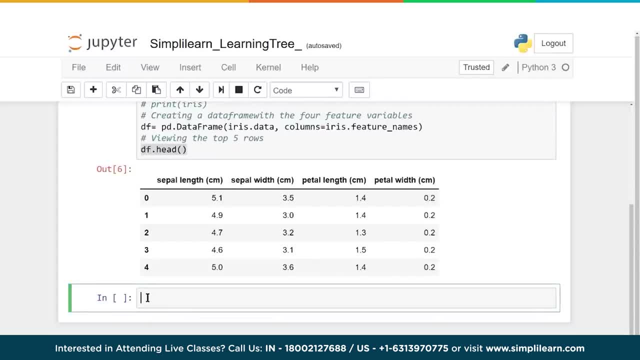 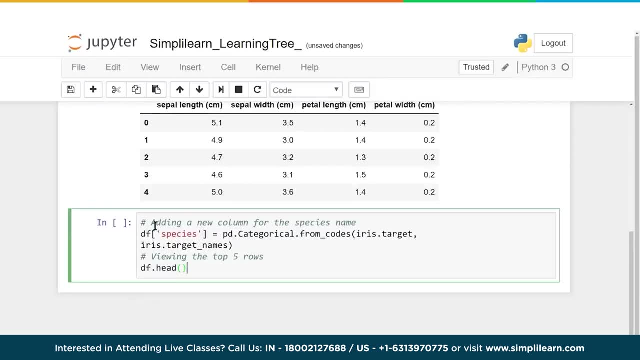 So we can discuss it a little bit more in detail. So here we are in our Jupyter notebook. I'm going to put the code in here And before I run it I want to look at a couple of things going on. So we have dfspecies. 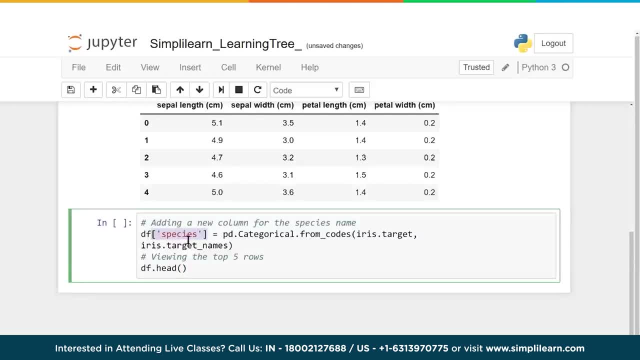 And this is interesting because right here you'll see where I have dfspecies in brackets, which is the key code for creating another column, And here we have iristarget. Now these are both in the pandas setup on here, So in pandas we can do either one. 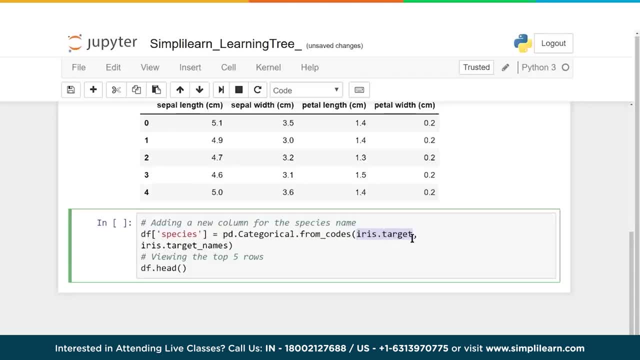 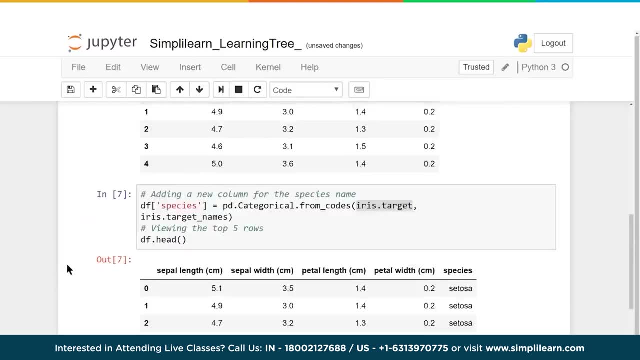 I could have just as easily done iris And then, in brackets, target. depending on what I'm working on, Both are acceptable. Let's go ahead and run this code and see how this changes. And what we've done is we've added the target from the iris data set as another column on. 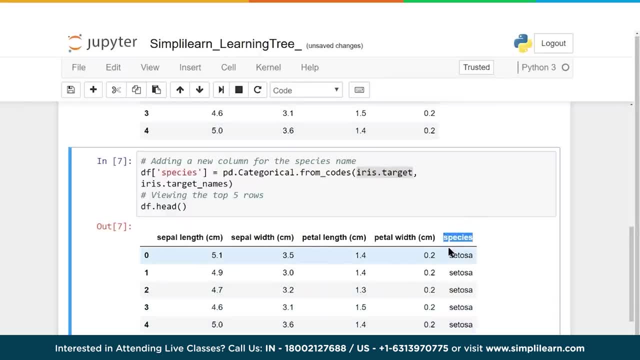 the end. Now, what species is? this is what we're trying to predict. So we have our data, which tells us the answer for all these different pieces, And then we've added a column with the answer. That way, when we do our final setup, we'll have the ability to program. 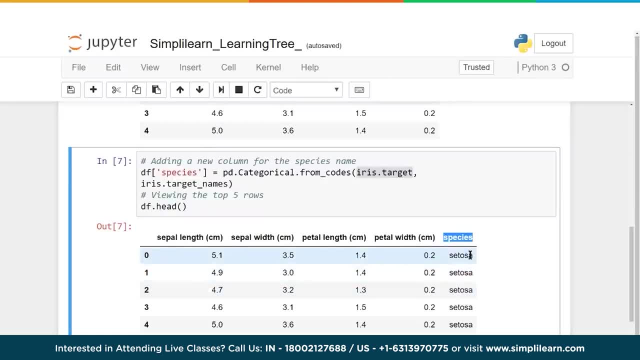 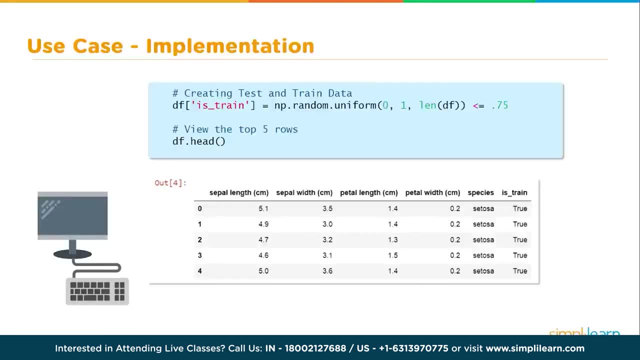 Our, our neural network, to look for these, this different data, and know what a setosa is, or a vericolor, which we'll see in just a minute- or virginica. Those are the three that are in there, And now we're going to add one more column. 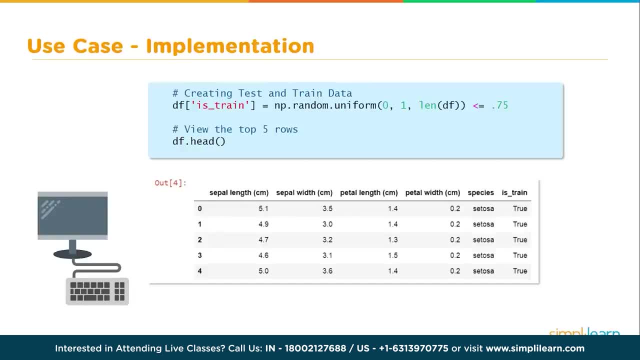 I know we're organizing all this data over and over again. It's kind of fun. There's a lot of ways to organize it. What's nice about putting everything onto one data frame is I can then do a printout and it shows me exactly what I'm looking at and I'll show you that where you. where that's. 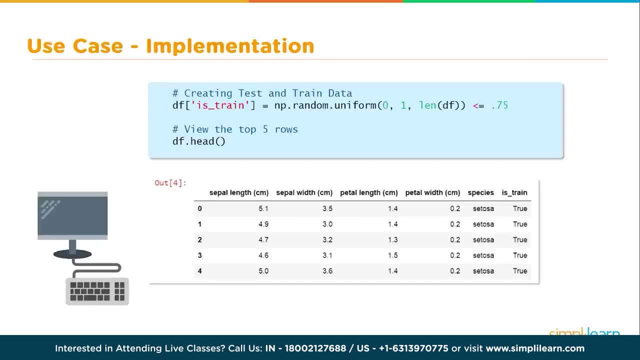 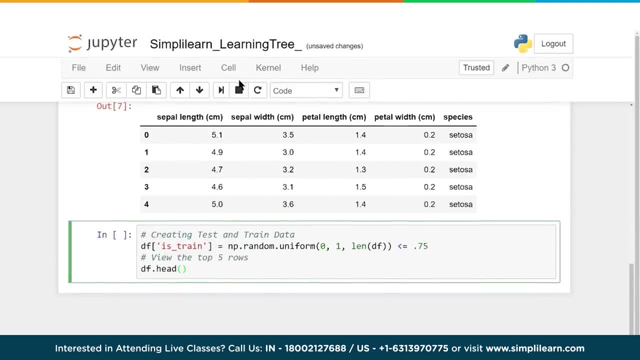 different, And then after that and do it slightly differently. But let's go ahead and put this into our script up to that now, And here we go, We're going to put that down here and we're going to run that, And let's talk a little bit about what we're doing. 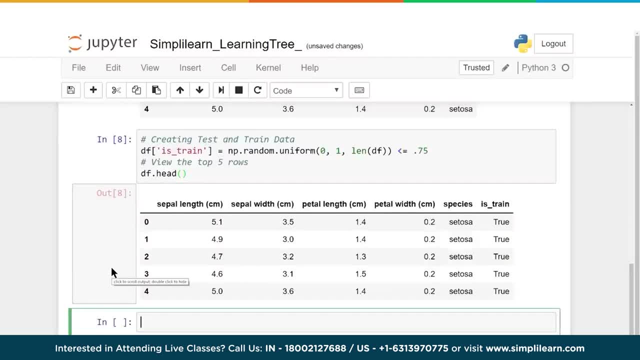 Now we're exploring data and one of the challenges is knowing how good your model is. Did your model work? And to do this, we need to split the data, and we split it into two different parts. They usually call it the training and the testing. 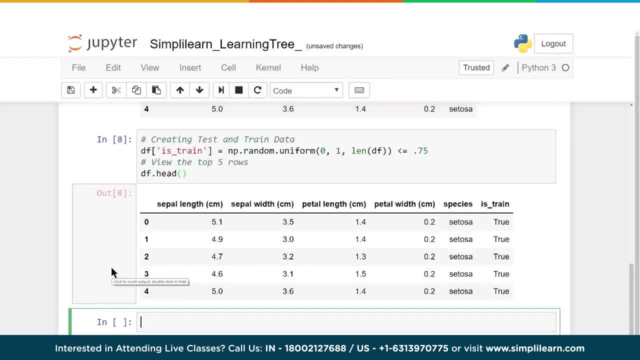 And so in here We're going to go ahead and put that in our database so you can see it clearly, And we've set it DF and remember you can put brackets. This is creating another column is trained, So we're going to use part of it for training and this equals NP. 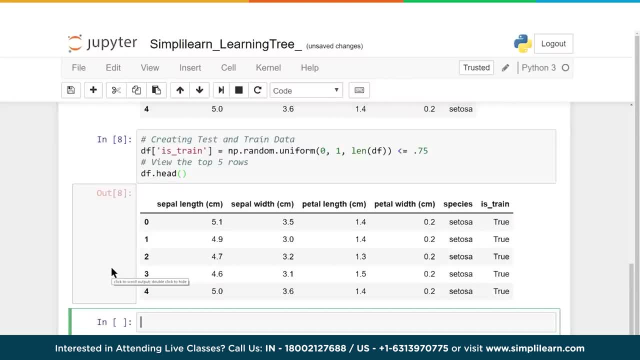 Remember that stands for numpy dot, random dot, uniform. So we're generating a random number between zero and one and we're going to do it for each of the rows. That's where the length DF comes from. So each row gets a generated number and if it's less than point seven, five it's true. 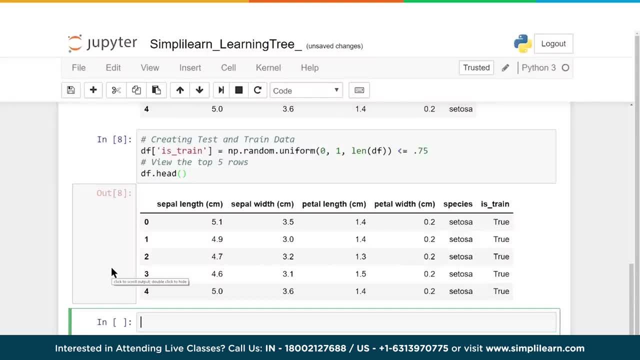 And if it's greater than point seven five, it's false. This means we're going to take 75% of the data roughly, because there's a randomness involved and we're going to use that to train it, and then the other 25% we're going to hold. 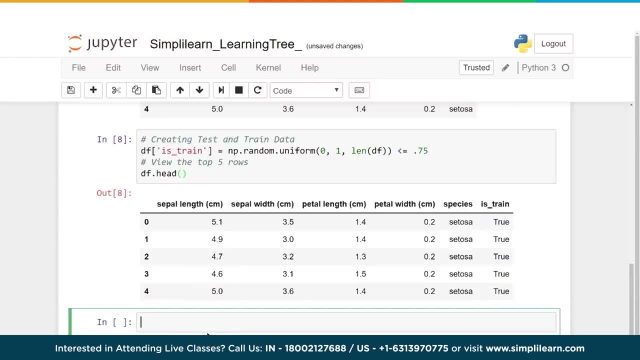 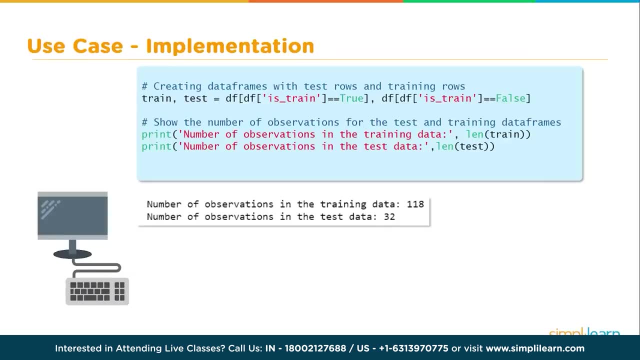 off to the side and use that to test it later on. So let's flip back out over and see what the next step is. So, now that we've labeled our database for which is training and which is testing, let's go ahead and sort that into two different variables. 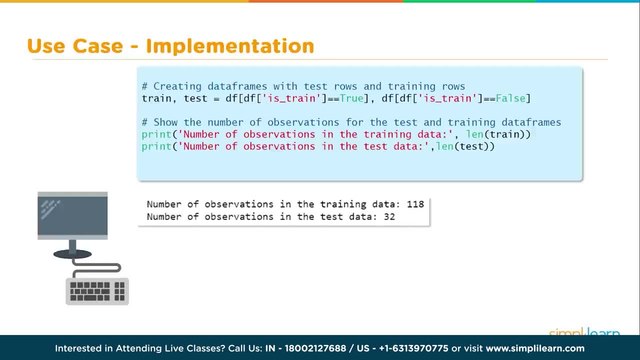 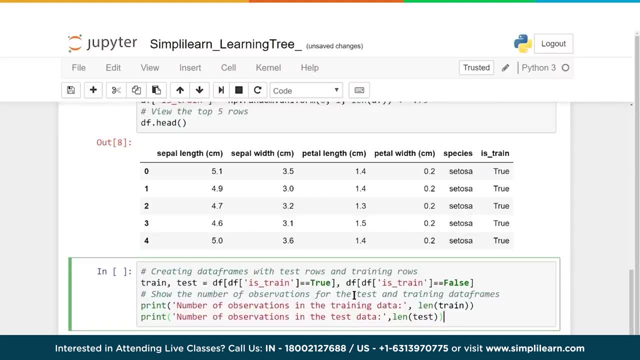 Train and test, And let's take this code And let's bring it into our project. Here we go, Let's paste it on down here, And before I run this, let's just take a quick look at what's going on here. 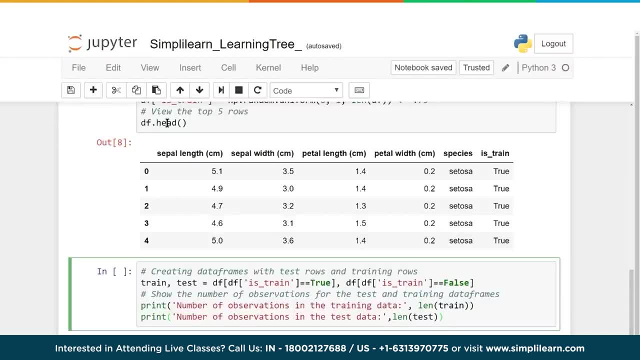 Is we have up above we created- remember there's our def dot head which prints the first five rows, And we've added a column is train at the end, And so we're going to take that and we're going to create two variables. 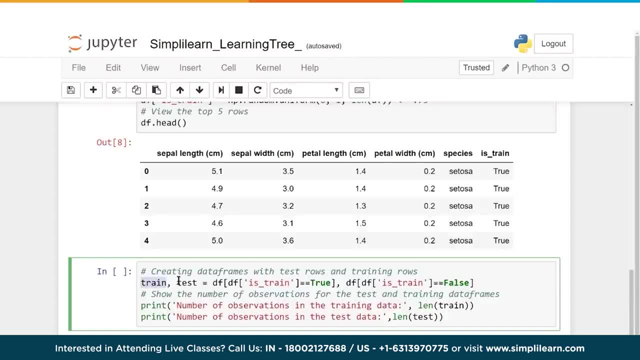 We're going to create two new data frames, One's called train, One's called test, 75% in train, 25% in test- And then to sort that out, we're going to do that by doing df, our main original data. 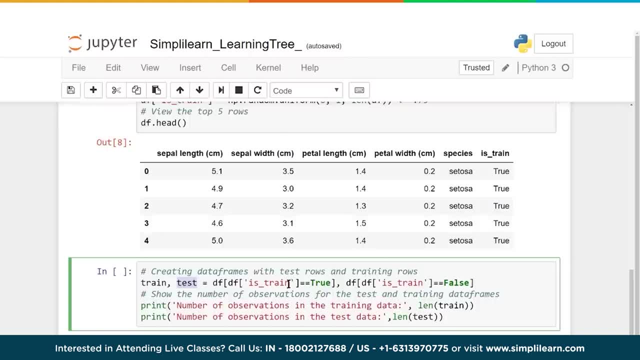 frame with the iris data in it, And if df is train equals true, that's going to go in the train, And if df is train equals false, it goes in the test, And so when I run this, we're going to print out the number in each one. 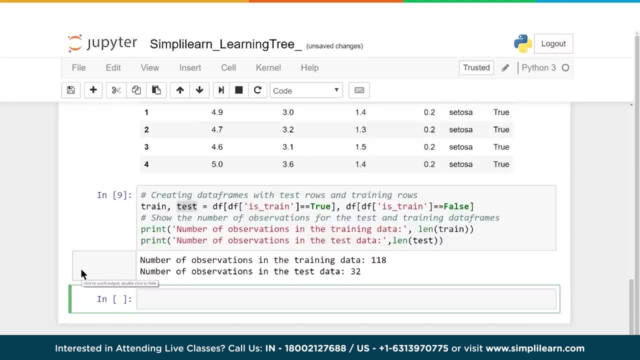 Let's see what that looks like And you'll see that it puts 118 in the training module And it puts 32 in the testing module, Which lets us know that there was 118. So we can see that there's 150 lines of data in here. 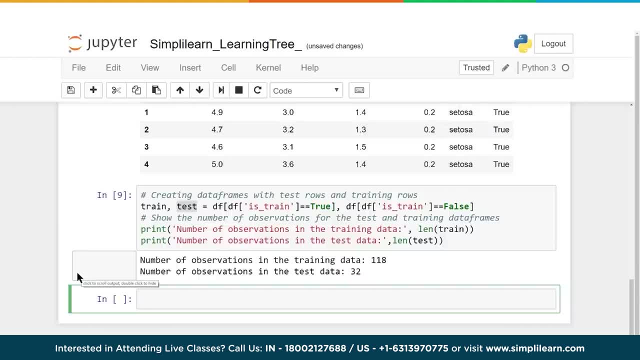 So if you went and looked at the original data, you could see that there's 150 lines And that's roughly 75% in one and 25% for us to test our model on afterward. So let's jump back to our code and see where this goes. 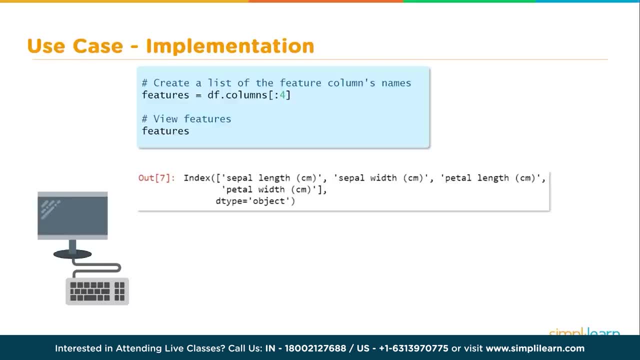 In the next two steps, we want to do one more thing with our data, And that's make it readable to humans. I don't know about you, but I hate looking at zeros and ones, So let's start with the features And let's go ahead. 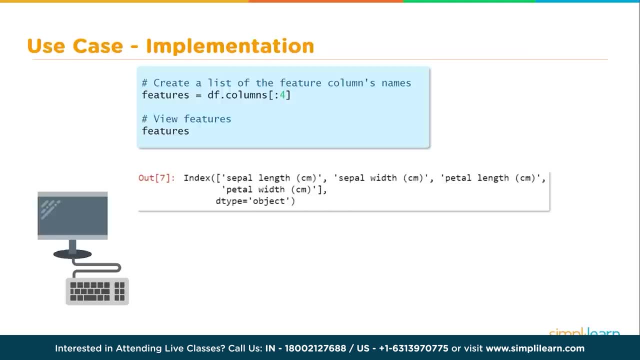 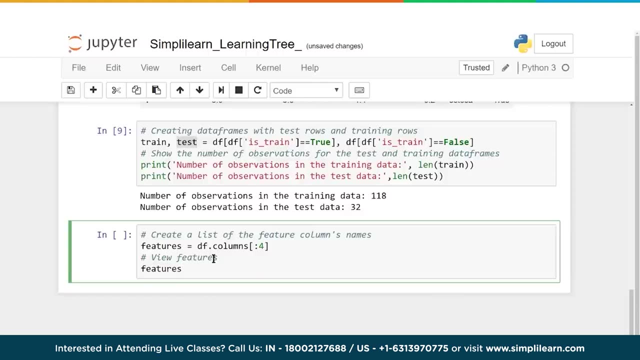 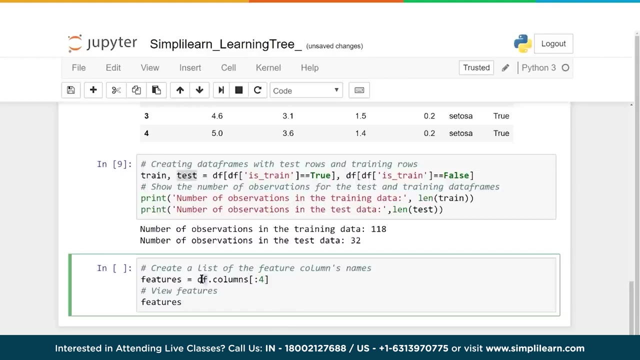 And Make those and make those readable to humans And let's put that in our code. Let's see, here we go, paste it in And you'll see, here we've done a couple very basic things. We know that the columns in our data frame- again this is a panda thing- the DF columns. 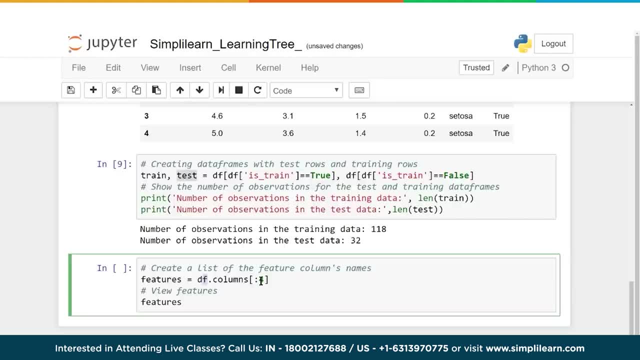 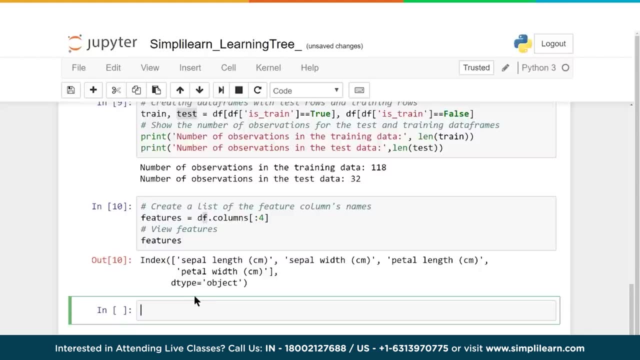 And we know the first four of them- 0,, 1,, 2,, 3, that would be the first four- are going to be the features or the titles of those columns, And so when I run this, You'll see down here that it creates an index: SEPA length, SEPA width, petal length and petal width. 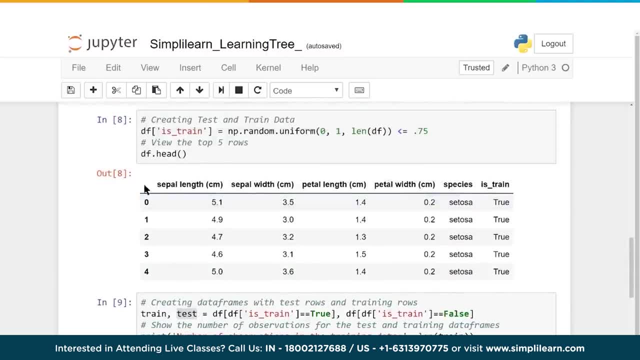 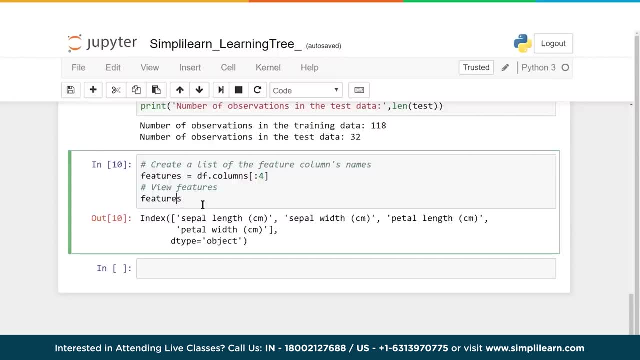 And this should be familiar, because if you look up here, here's our column titles going across, and here's the first four. One thing I want you to notice here is that when you're in a command line- whether it's Jupyter Notebook, or you're running command line in the terminal window. 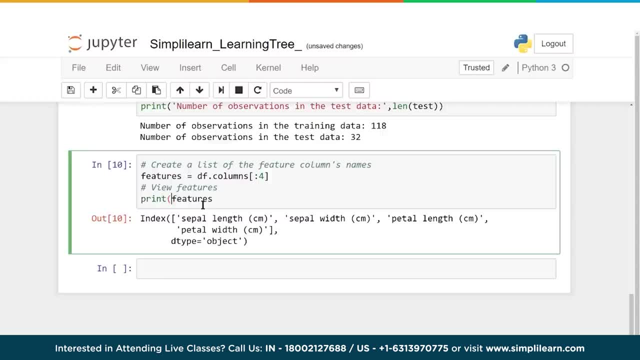 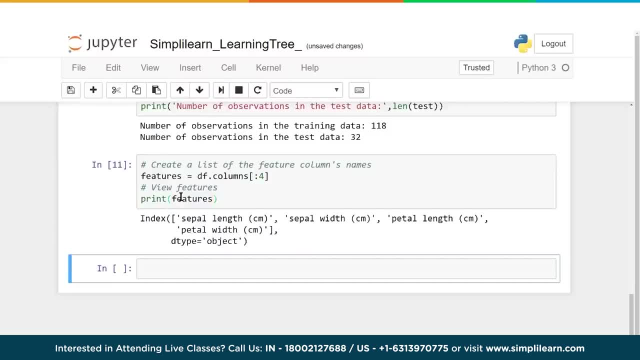 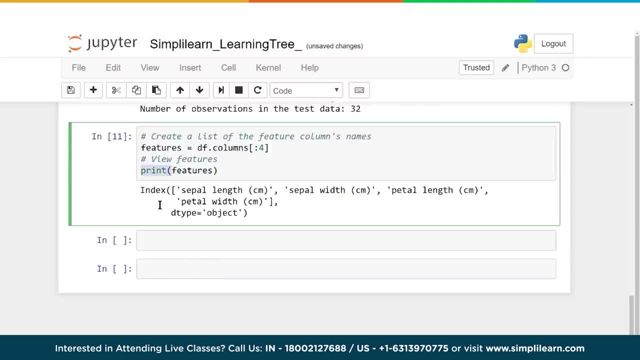 But for this. when I run it, you'll see it gives me the same thing. But for this we want to go ahead and we'll just leave it as features, because it doesn't really matter. And this is one of the fun thing about Jupyter Notebooks is I'm just building the code as we go. 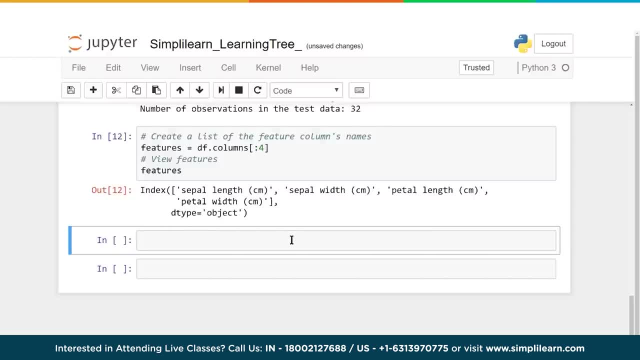 And then we need to go ahead and create the labels for the other part, And then we need to go ahead and create the labels for the other part. So let's take a look and see what that. So let's take a look and see what that. 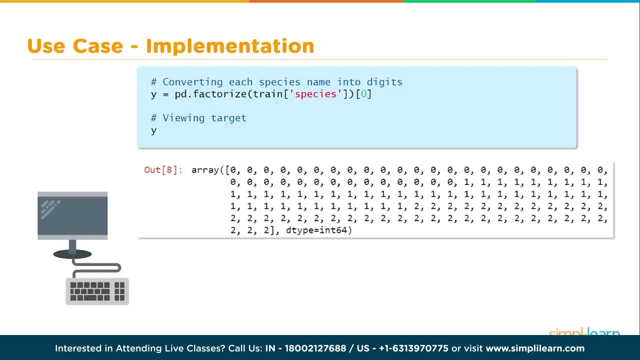 before we actually start running the training. and the testing is we're going to go ahead and convert the species on here into something the computer understands. So let's put this code into our script and see where that takes us All. right, here we go. 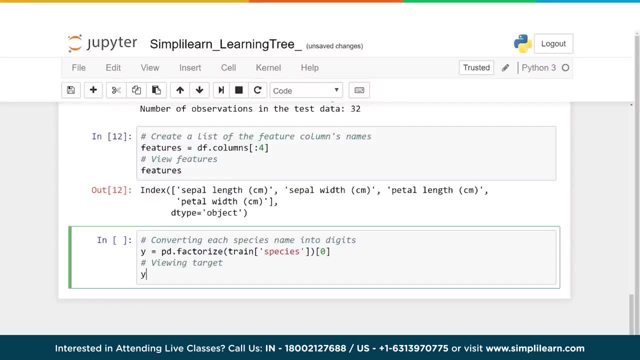 We've set y equal to pdfactorize train species of 0.. So let's break this down just a little bit. We have our pandas right here, pd And pdfactorize what's factorize doing. I'm going to come back to that in just a second. 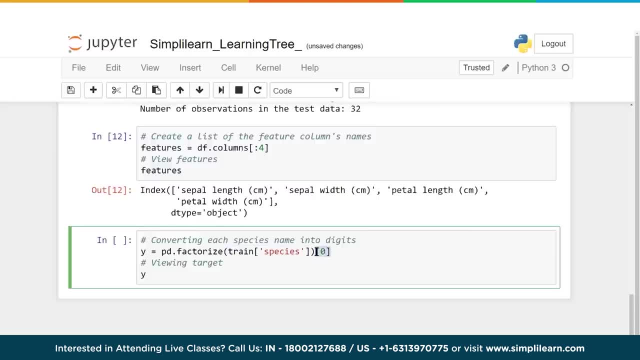 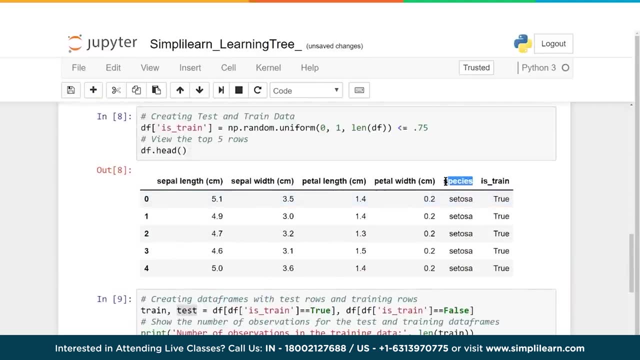 Let's look at what train species is and why. we're looking at the group 0 on there And let's go up here and here is our species. Remember this: We created this whole column here for species And then it has setosa setosa, setosa, setosa. 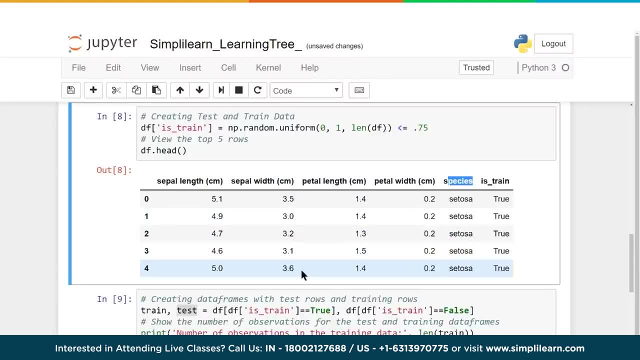 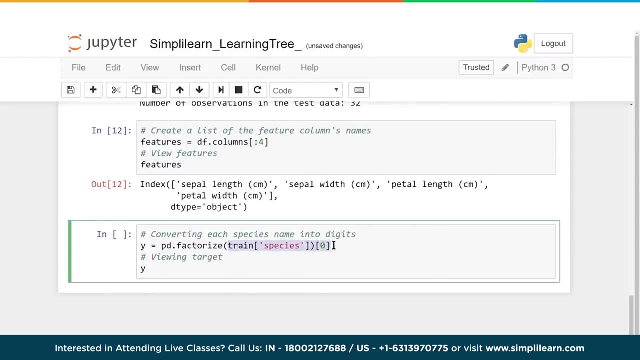 And if you scroll down enough, you'd also see virginica and vericolor. We need to convert that into something the computer understand: 0s and 1s, So the train species of 0, because this is in the format of an array of arrays. 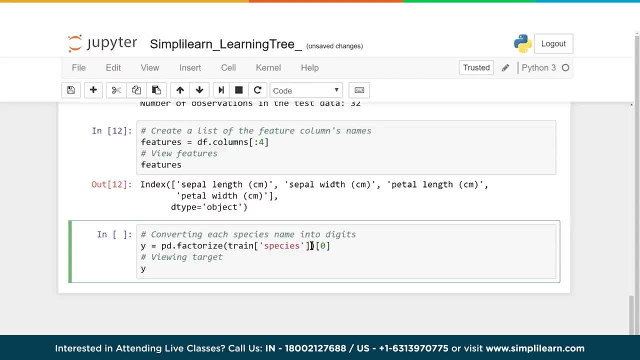 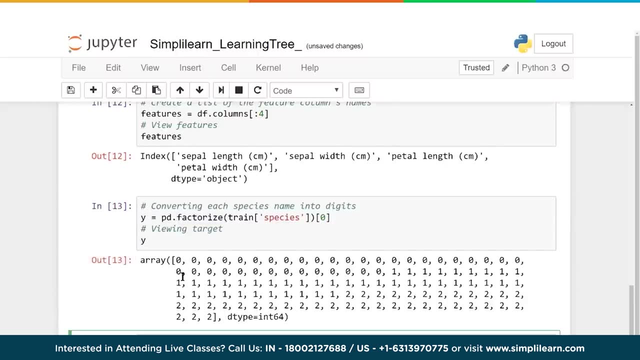 so you have to have the 0 on the end, And then species is just that column. Factorize goes in there and looks at the fact that there's only three of them. So when I run this, you'll see that y generates an array. 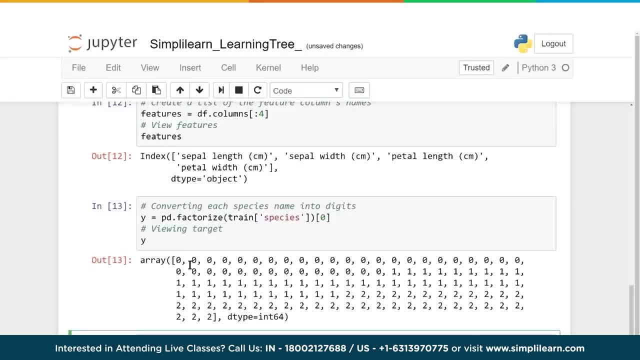 that's equal to. in this case it's a training set and it's 0s, 1s and 2s representing the three different kinds of flowers We have. so now we have something the computer understands and we have a nice table that we can read and understand. 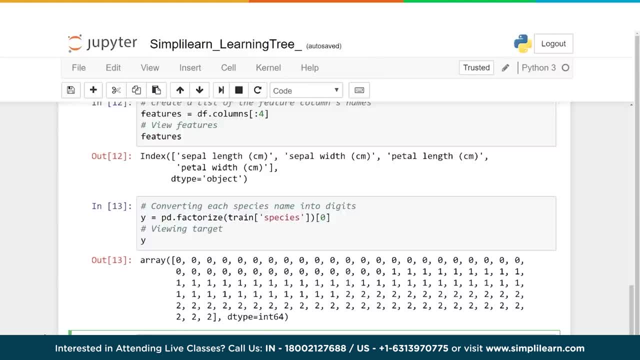 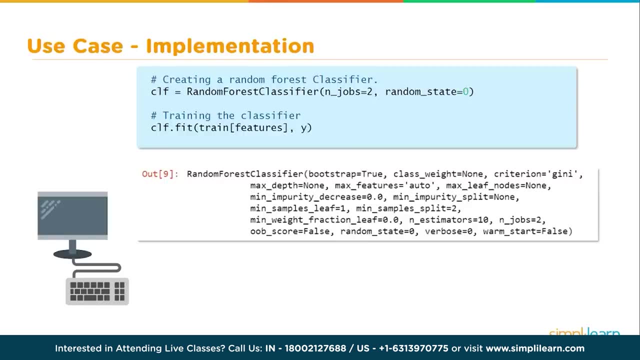 And now, finally, we get to actually start doing the predicting. So here we go. We have two lines of code. Oh, my goodness, That was a lot of work to get to two lines of code, but there is a lot in these two lines of code. 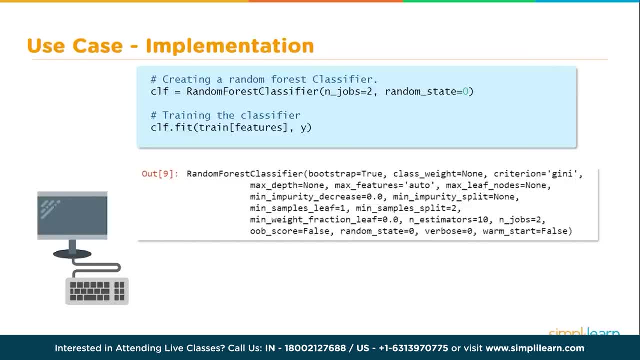 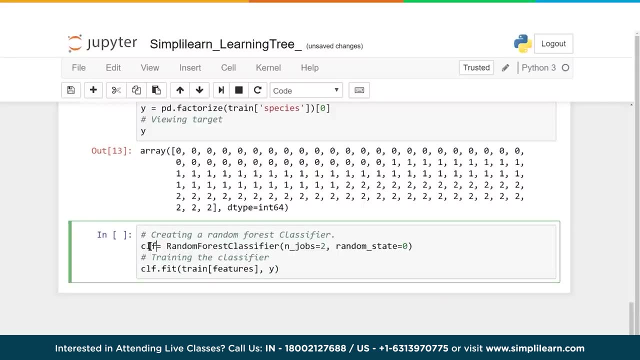 So let's take a look and see what's going on here and put this into our full script that we're running. Let's paste this in here and let's take a look and see what this is We have. we're creating a variable clf. 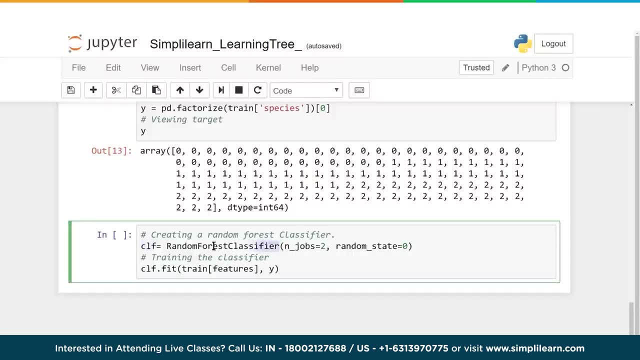 and we're going to set this equal to the random forest classifier And we're passing two variables in here and there's a lot of variables you can play with. As far as these two are concerned, they're very standard njobs. all that does is to prioritize it. 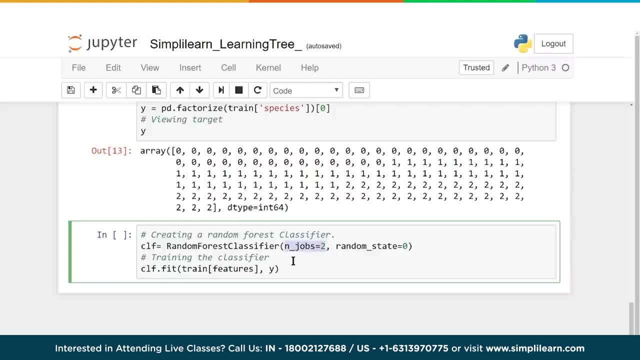 Not something to really worry about. Usually, when you're doing this on your own computer, you do njobs equals 2.. If you're working in a larger or big data and you need to prioritize it differently, this is what that number does. is it changes your priority? 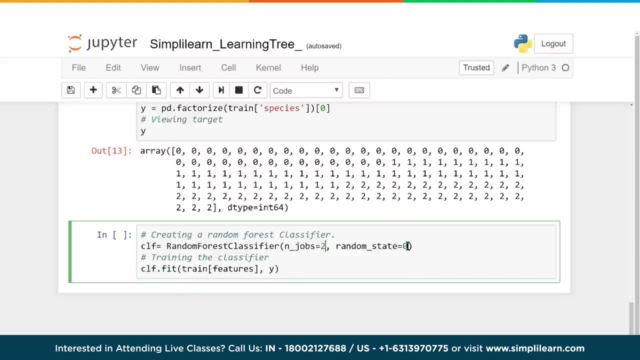 And how it's going to run across the system and things like that, And then the random state is just how it starts. Zero is fine for here, But let's go ahead and run this. We also have clffit train features y. 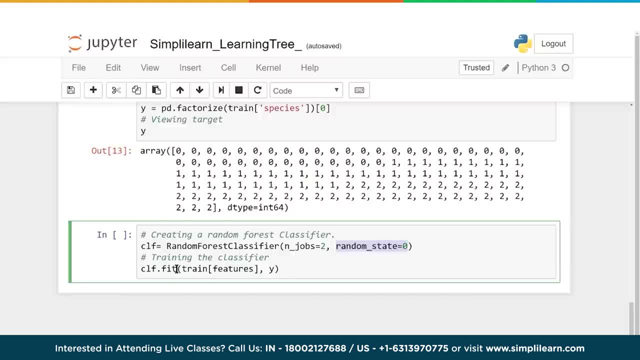 And before we run it, let's talk about this a little bit more clffit. So we're fitting, we're training it. We are actually creating our random forest classifier right here. This is the code that does everything, And we're going to take our training set. 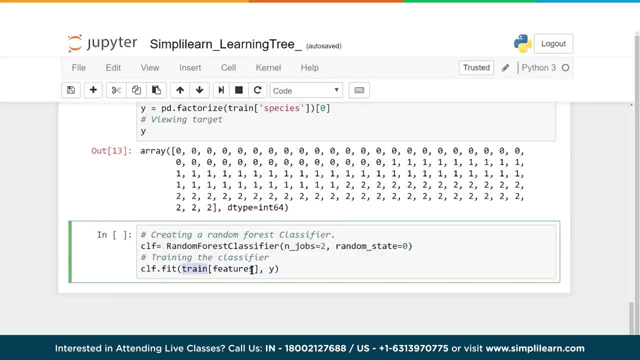 Remember, we kept our test off to the side And we're going to take our training set with the features, And then we're going to go ahead and put that in. And here's our target, the y. So the y is 0,, 1, and 2, that we just created. 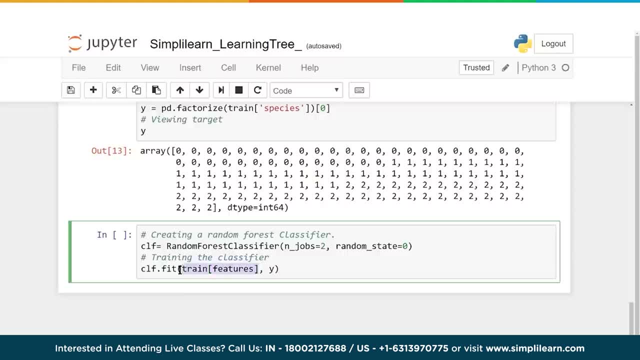 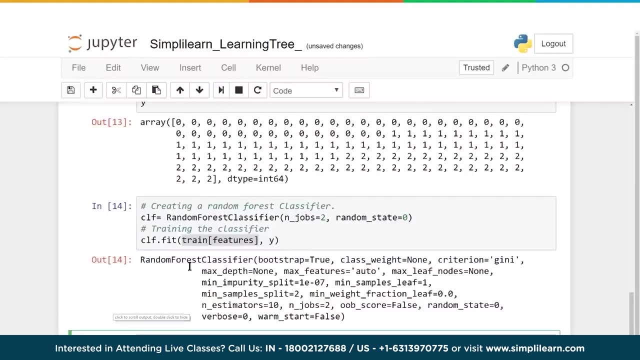 And the features, is the actual data going in that we put into the training set And let's go ahead and run that. And this is kind of an interesting thing because it printed out the random forest classifier and everything around it, And so when you're running this in your terminal window, 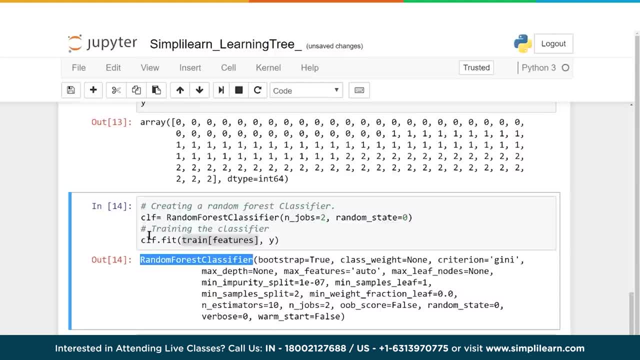 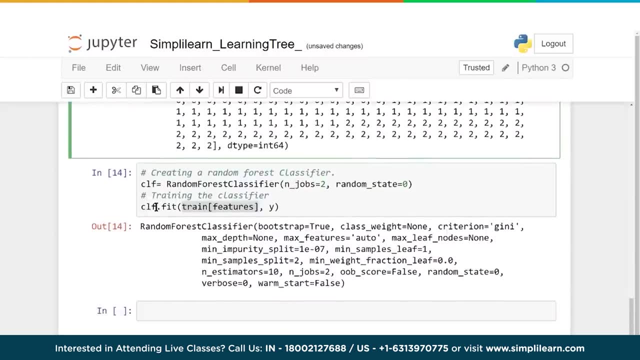 or in a script like this. this automatically treats this, just like when we were up here and I typed in y and it printed out y instead of print y. This does the same thing: It treats this as a variable and prints it out. 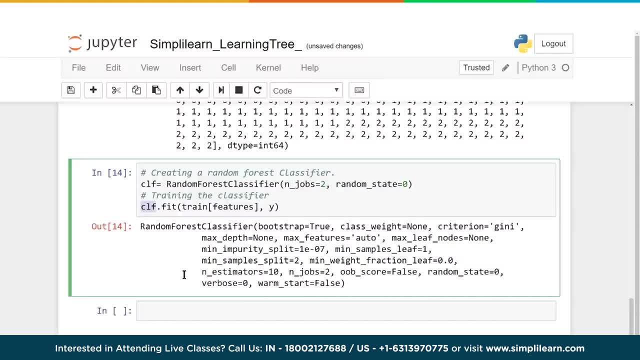 But if you were actually running your code, that wouldn't be the case. And what it's printed out is. it shows us all the different variables we can change And if we go down here, you can actually see in jobs equals 2.. 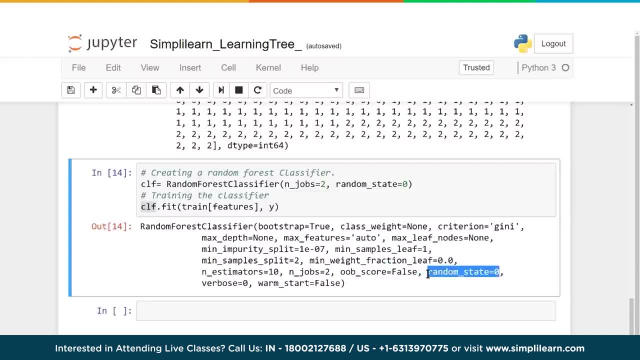 You can see, the random state equals 0.. Those are the two that we sent in there. You would really have to dig deep to find out all these different meanings of all these different settings on here. Some of them are self-explanatory. 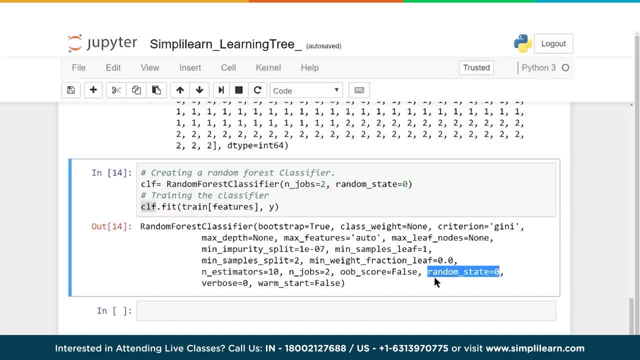 if you kind of think about it a little bit like max features is auto, So all the features that we're putting in there is just going to automatically take all four of them. Whatever we send it, it'll take. Some of them might have so many features. 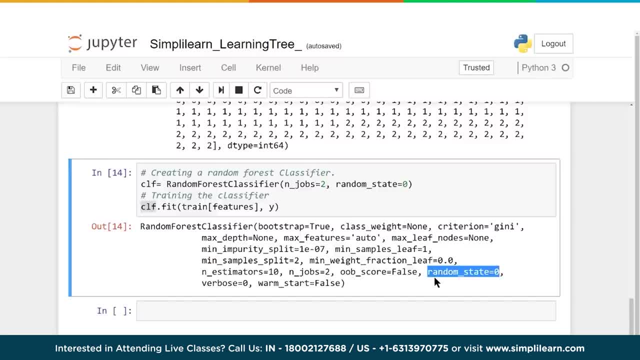 because you're processing words. there might be like 1.4 million features in there because you're doing legal documents and that's how many different words are in there. At that point, you probably want to limit the maximum features that you're going to process. 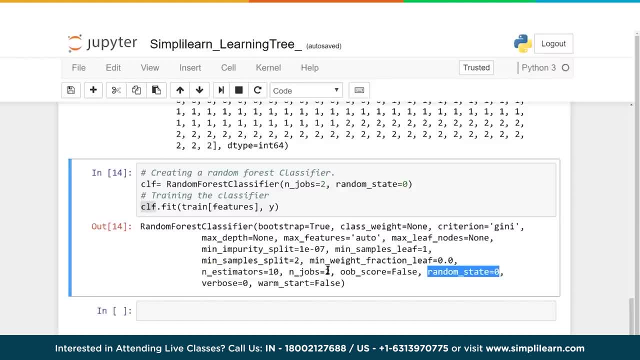 And leaf nodes. that's the end nodes. Remember we had the fruit and we're talking about the leaf nodes. Like I said, there's a lot in this. We're looking at a lot of stuff here, So you might have in this case, 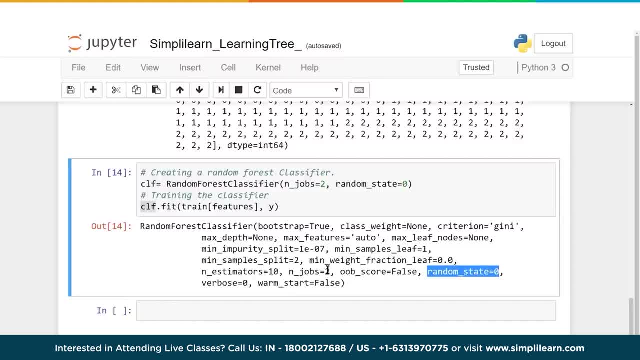 there's probably only, I think, three leaf nodes, maybe four. You might have thousands of leaf nodes, at which point you do need to put a cap on that and say, okay, you can only go so far, and then we're going to use all of our resources. 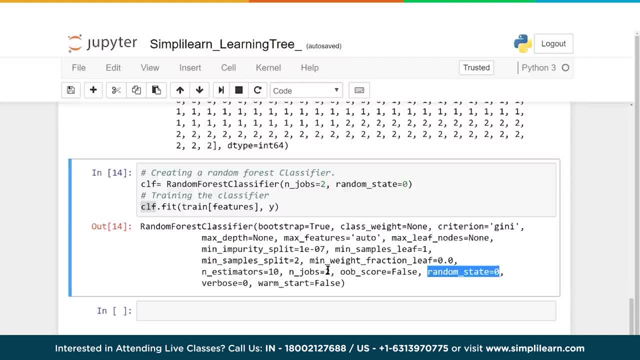 on processing this, And that really is what most of these are about is limiting the process and making sure we don't overwhelm a system. And there's some other settings in here. Again, we're not going to go over all of them. 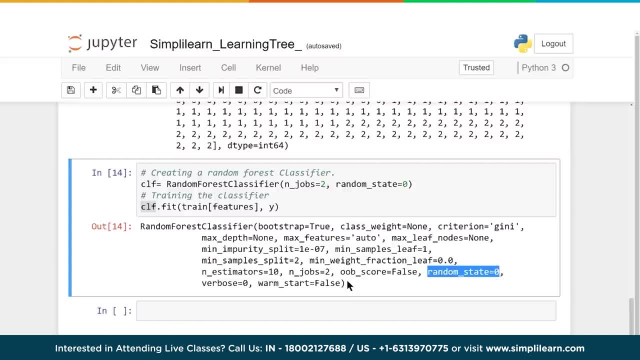 Warm start equals false. Warm start is if you're programming it one piece at a time externally, Since we're not, we're not going to have, we're not going to continually detrain this particular learning tree And again, like I said, there's a lot of things in here. 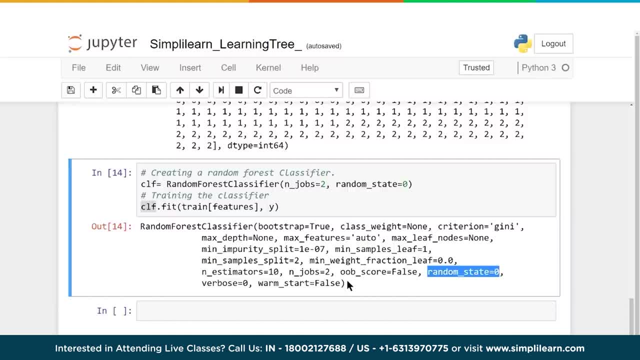 that you'll want to look up more detail from the sklearn, And if you're digging in deep and you're looking for a major project on here. For today, though, all we need to do is fit or train our features and our target Y. 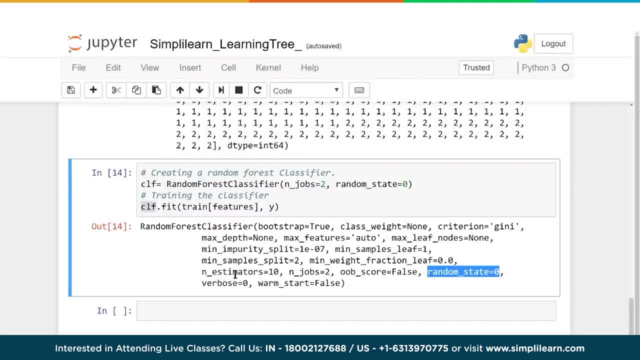 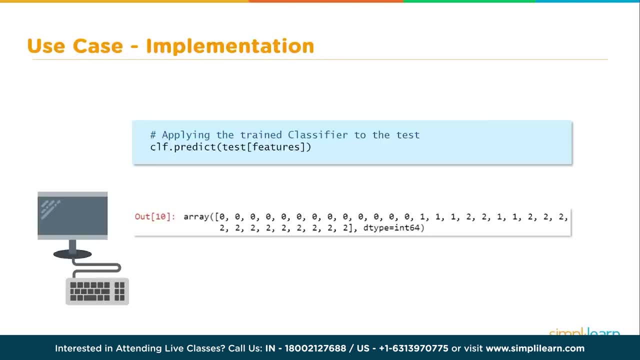 So now we have our training model. What's next? If we're going to create a model, we now need to test it. Remember, we set aside the test feature- test group- 25% of the data. So let's go ahead and take this code. 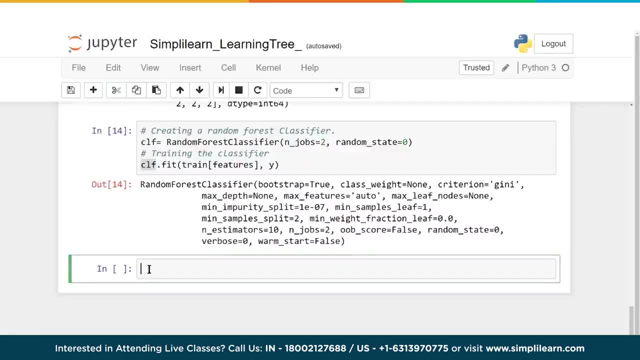 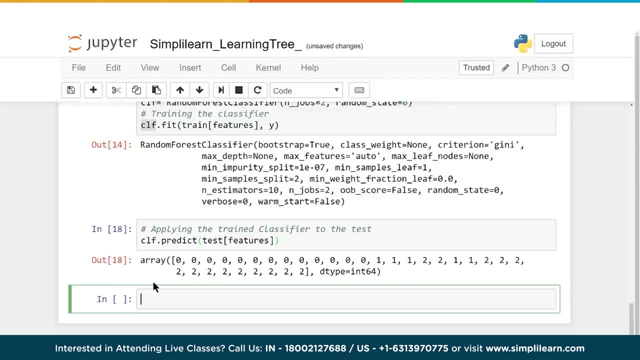 and let's put it into our script and see what that looks like. Okay, here we go And we're going to run this And it's going to come out with a bunch of zeros, ones and twos, which represents the three type of flowers. 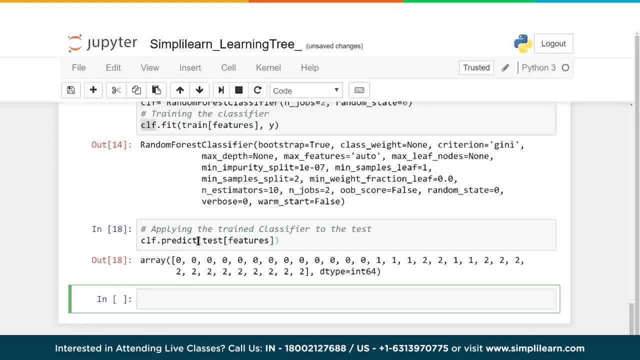 the setosa, the virginica and the versicolor, And what we're putting into our predict is the test features, And I always kind of like to know what it is I am looking at. So, real quick, we're going to do test features. 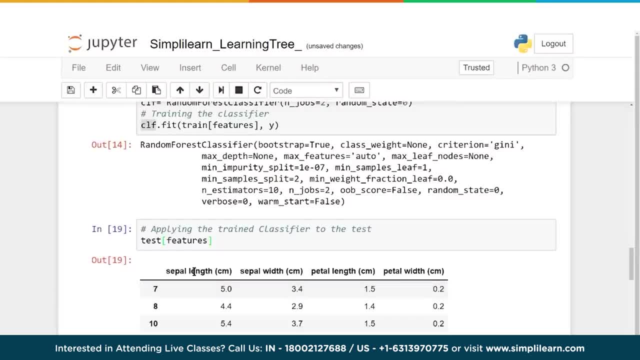 And remember, features is an array of sepal length, sepal width, petal length, petal width. So when we put it in this way, it actually loads all these different columns that we loaded into features. So if we did just features, 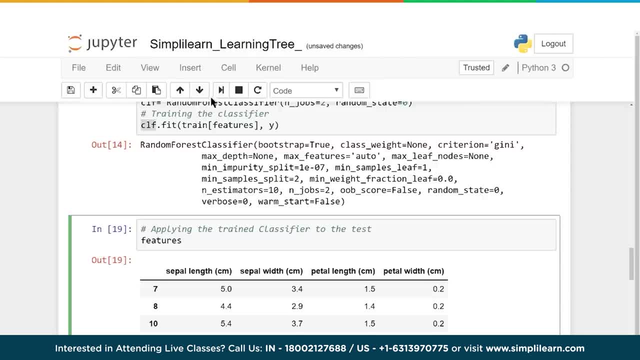 let me just do features in here, see what features looks like. This is just playing with Panda's data frames. You'll see that it's an index. So when you put an index in like this into test features, into test, it then takes those columns. 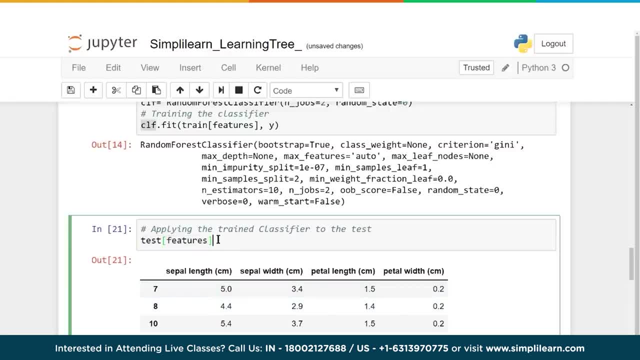 and creates a Panda data frame from those columns And in this case we're going to go ahead and put those into our predict. So we're going to put each one of these lines of data- the 5.0,, 3.4,, 1.5, 0.2,. 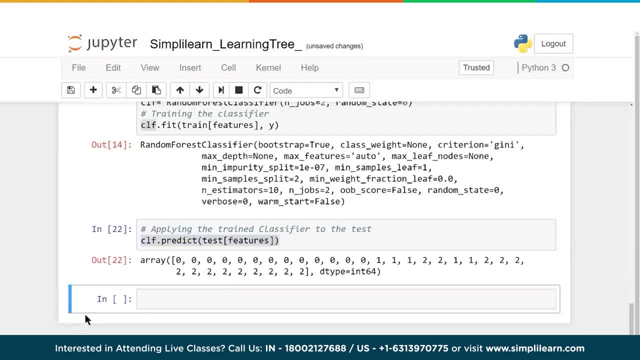 and we're going to put those in and we're going to predict what our new forest classifier is going to come up with. And this is what it predicts. It predicts 0, 0, 0, 1, 2, 1, 1, 2, 2, 2.. 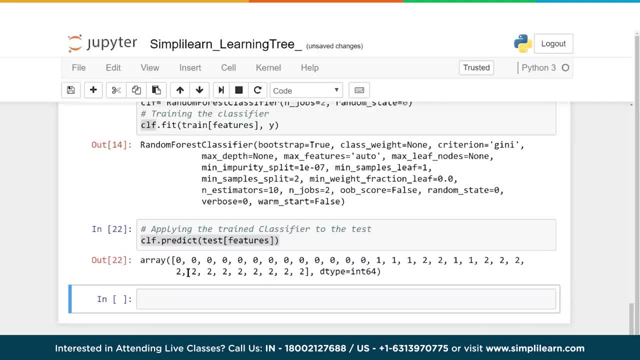 And again, this is the flower type: setosa, virginica and versicolor. So now that we've taken our test features, let's explore that, Let's see exactly what that data means to us. So the first thing we can do with our predicts: 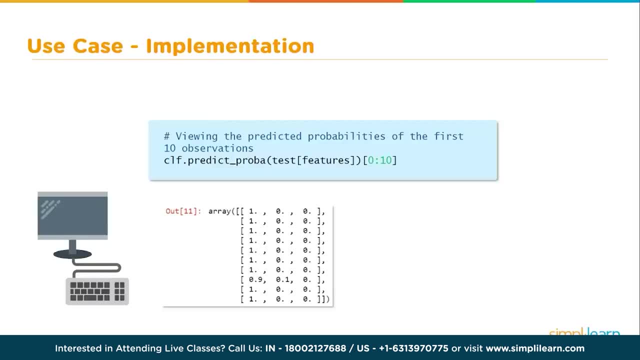 is, we can actually generate a different prediction model. When I say different, we're going to view it differently. It's not that the data itself is different. So let's take this next piece of code and put it into our script. So we're pasting it in here. 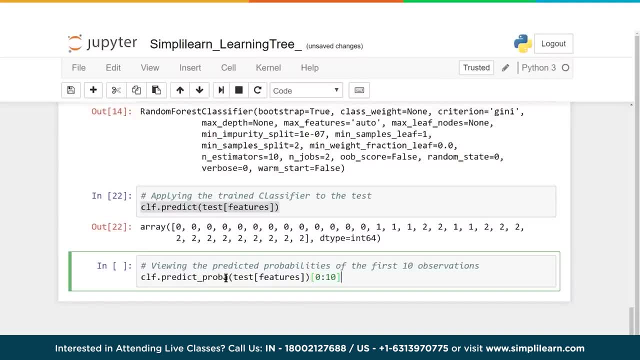 And you'll see that we're doing a predict and we've added underscore proba for probability. So there's our clfpredict probability. So we're running it just like we ran it up here, but this time, with this, we're going to get a slightly different result. 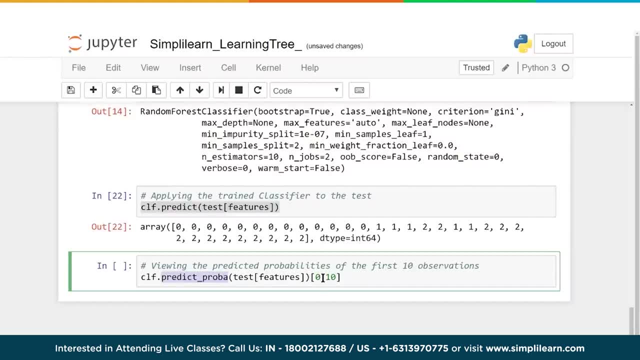 And we're only going to look at the first 10.. So you'll see down here, instead of looking at all of them, which was what? 27,? you'll see right down here that this generates a much larger field on the probability. 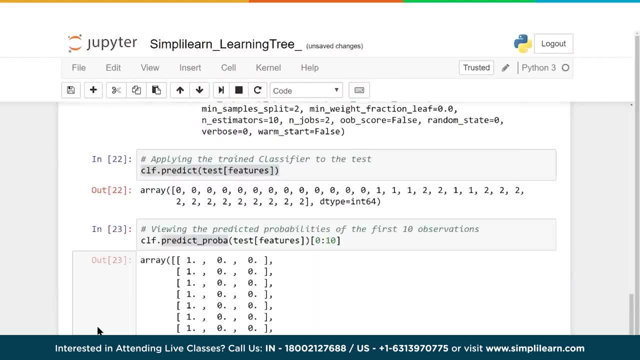 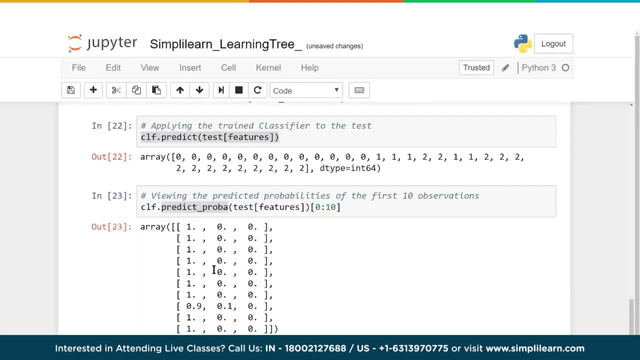 And let's take a look and see what that looks like and what that means. So when we do the predict, the predict underscore proba for probability, it generates three numbers. So we had three leaf nodes at the end And if you remember from all the theory we did, 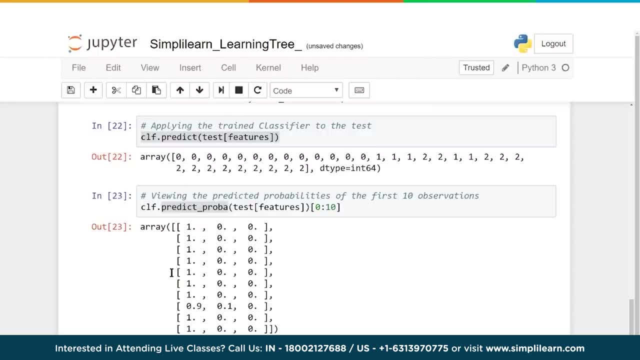 this is the predictors. The first one is predicting a 1 for setosa, It predicts a 0 for virginica, And it predicts a 0 for versicolor, And so on, and so on, and so on. You know what? I'm going to change this just a little bit. 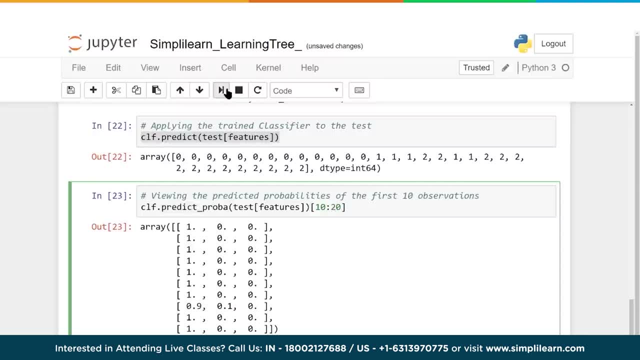 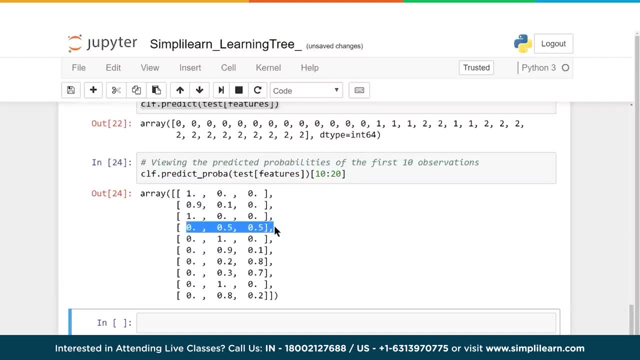 Let's look at 10 to 20, as we can, And we start to get in a little different of data And you'll see right down here it gets to this one, this line right here, And this line has 0,. 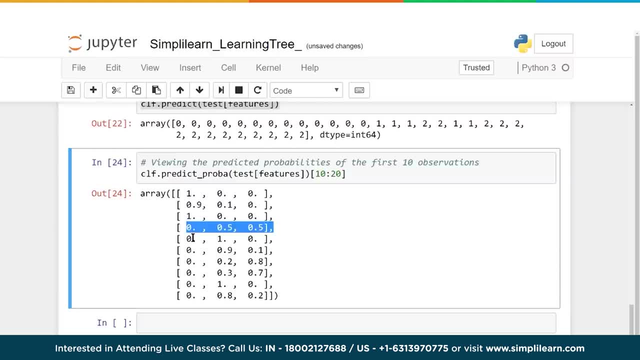 0.5, 0.5. And so if we're going to vote and we have two equal votes, it's going to go with the first one. So it says setosa gets 0 votes, virginica gets 0.5 votes. 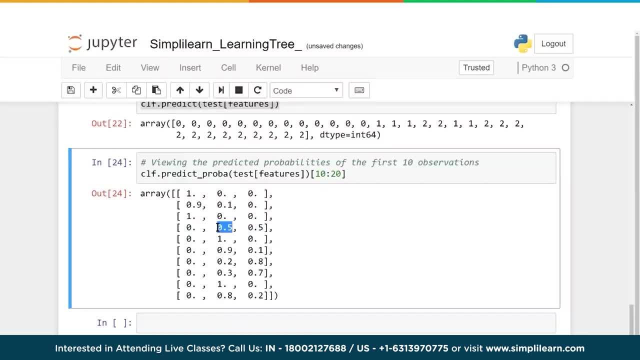 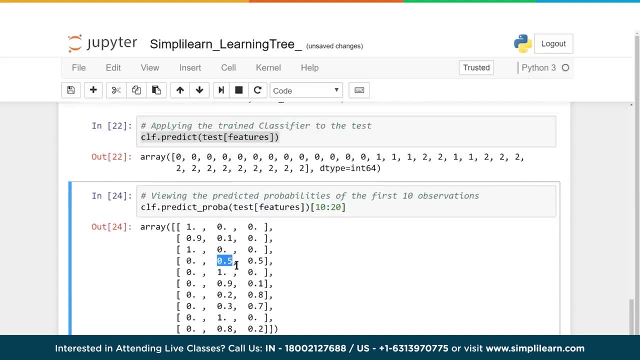 versicolor gets 0.5 votes, But let's just go with the virginica, since these two are equal, And so on and so on. down the list You can see how they vary on here. So now we've looked at both. how to do a basic. 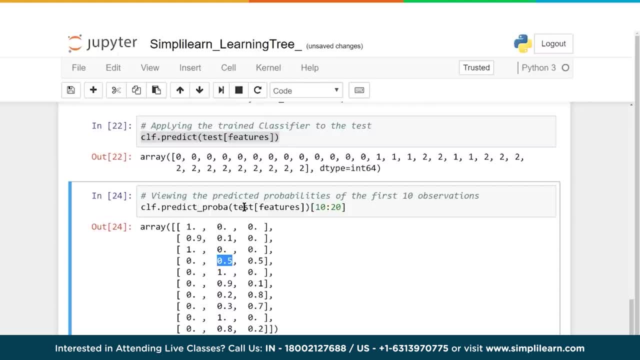 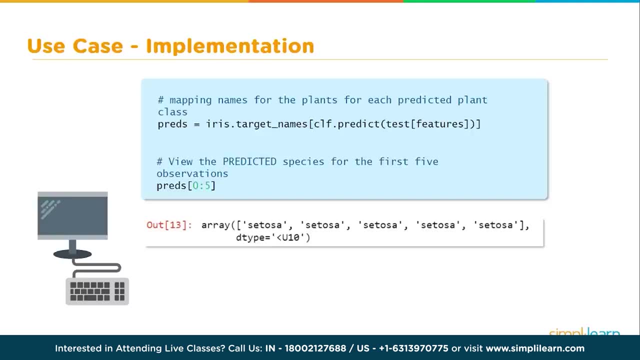 predict of the features and we've looked at the predict probability. Let's see what's next on here. So now we want to go ahead and start mapping names for the plants. We want to attach names so that it makes a little more sense for us. 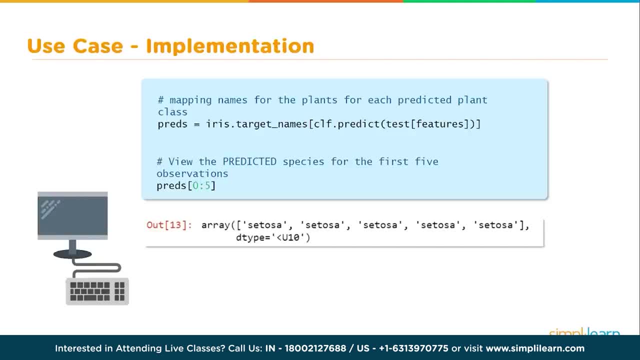 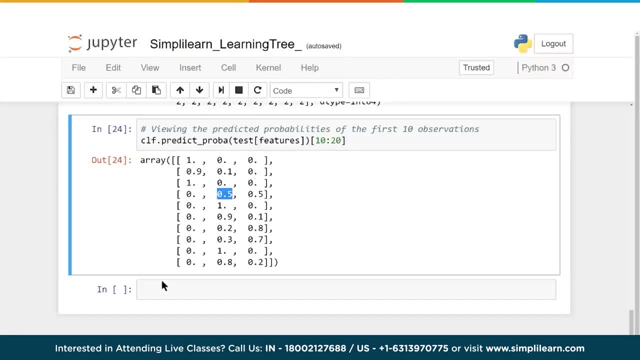 And that's what we're going to do in these next two steps. We're going to start by setting up our predictions and mapping them to the names. So let's see what that looks like And let's go ahead and paste that code in here and run it. 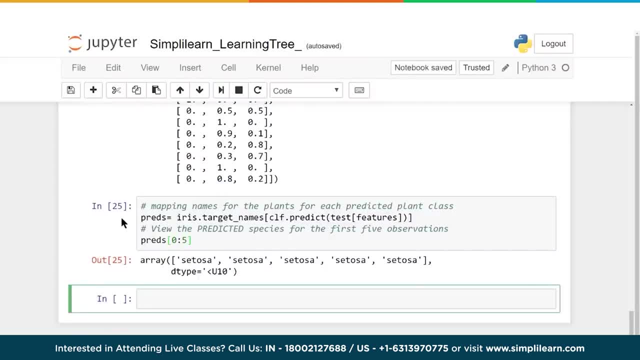 And this goes along with the next piece of code, So we'll skip through this quickly and then come back to it a little bit. So here's iristargetNames, And if you remember correctly, this was the names that we've been talking about this whole time. 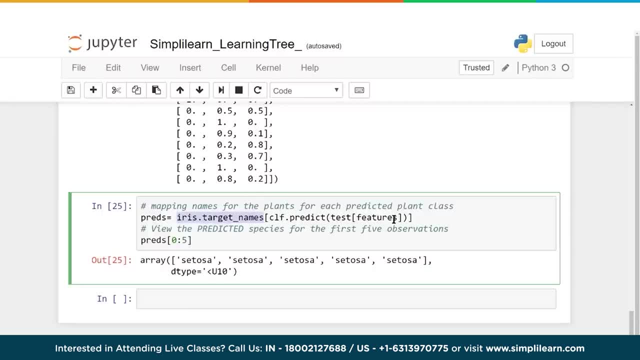 The setosa virginica versicolor. And then we're going to go ahead and do the prediction again. We could have just set a variable equal to this instead of re-running it each time, But we're going to go ahead and run it again. 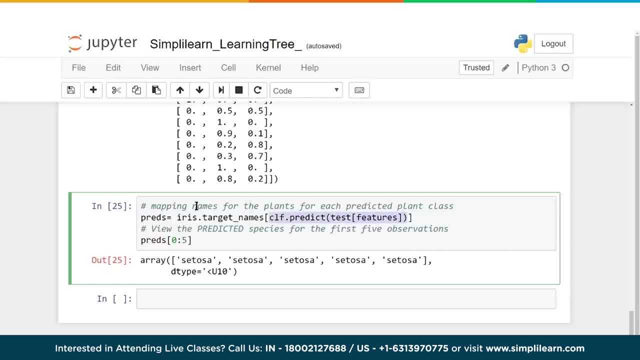 Remember that returns the zeros, the ones and the twos, And then we're going to set that equal to predictions. So this time we're actually putting it in a variable And when I run this it distributes and it comes out as an array. 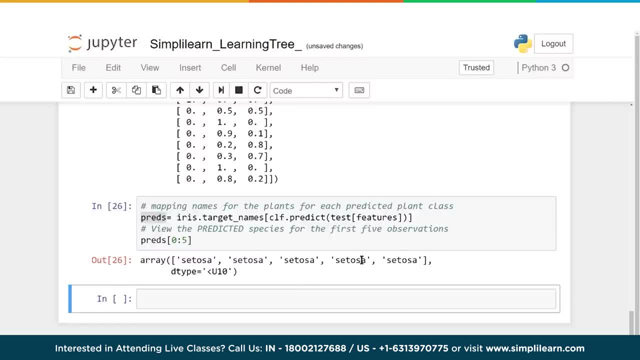 And the array is: setosa, setosa, setosa, setosa, setosa. We're only looking at the first five. We could actually do. let's do the first 25, just so we can see a little bit more on there. 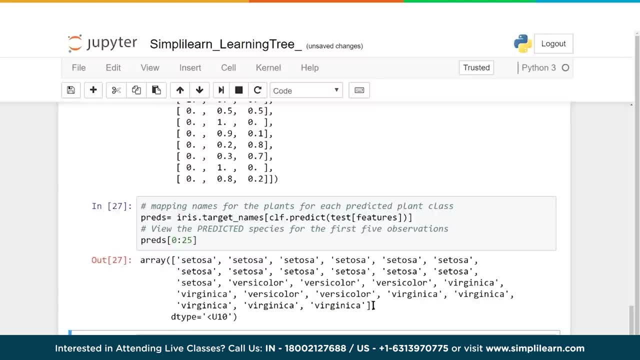 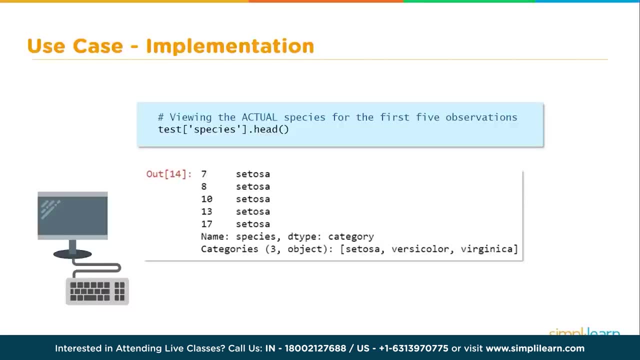 And you'll see that it starts mapping it to all the different flower types- The versicolor and the virginica in there, And let's see how this goes with the next one. So let's take a look at the top part of our species. 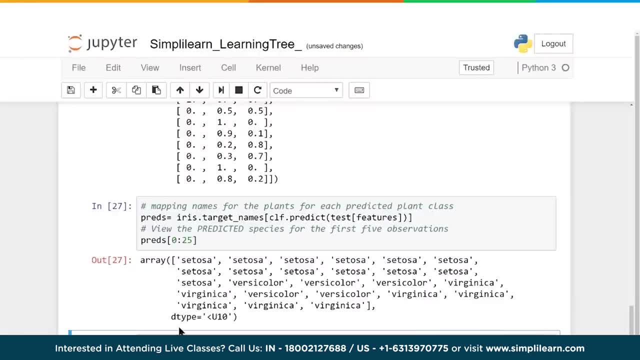 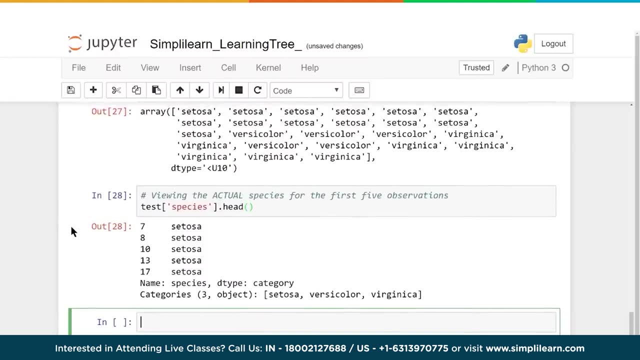 in here And we'll take this code and put it in our script And let's put that down here and paste it. There we go And we'll go ahead and run it. And let's talk about both these sections of code here. 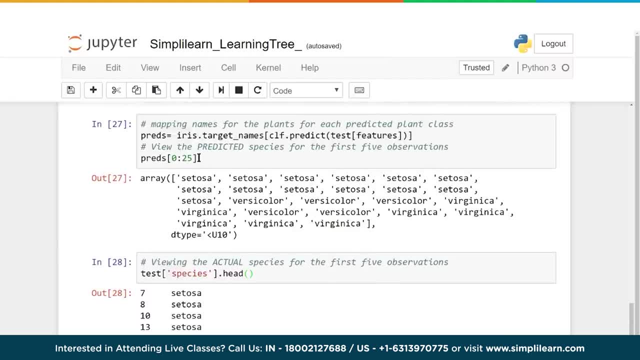 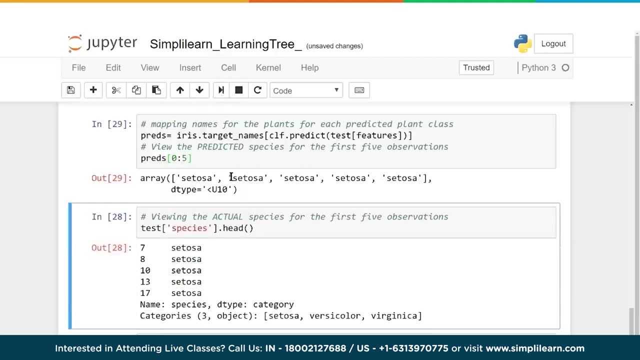 And how they go together. The first one is our predictions, And I went ahead and did predictions through 25.. Let's just do 5. And so we have setosa, setosa, setosa, setosa. That's what we're predicting from. 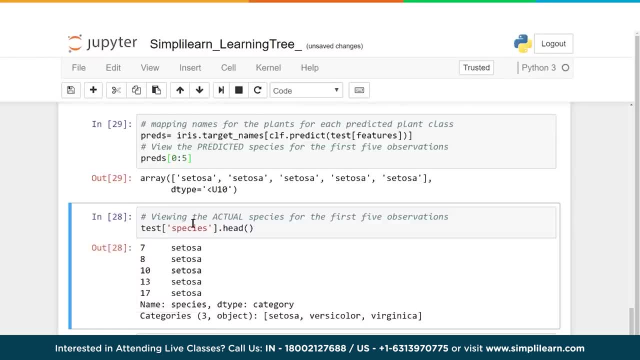 our test model. And then we come down here and we look at test species. I remember I could have just done testspecieshead And you'll see, it says setosa setosa, setosa, setosa And they match. So the first one is what our 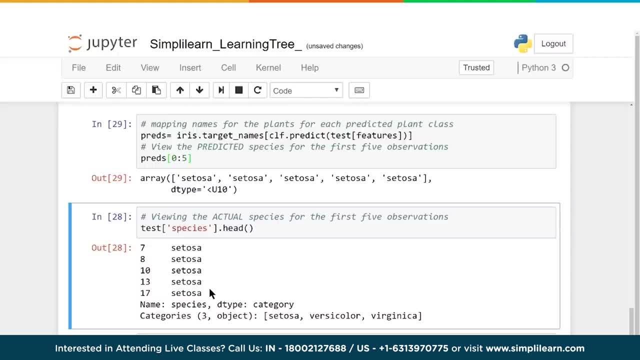 forest is doing, And the second one is what the actual data is. Now we need to combine these so that we can understand what that means. We need to know how good our forest is. So that's where we come up to the next step. 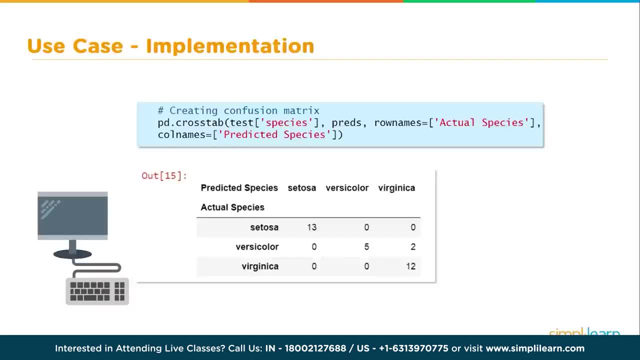 Which is lots of fun. We're going to use a single line of code to combine our predictions and our actuals, So we have a nice chart to look at And let's go ahead and put that in our script In our Jupyter Notebook here. 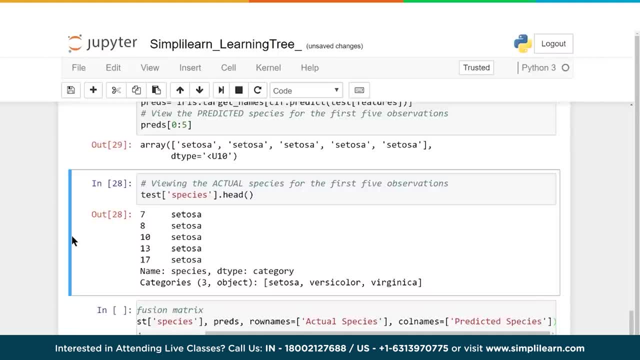 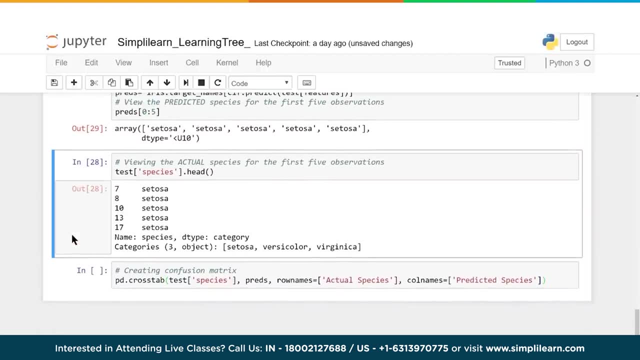 Let's go ahead and paste that in, Because I'm on the Jupyter Notebook. I can do a control minus. You can see the whole line there. There we go, Resize it And let's take a look and see what's going on here. 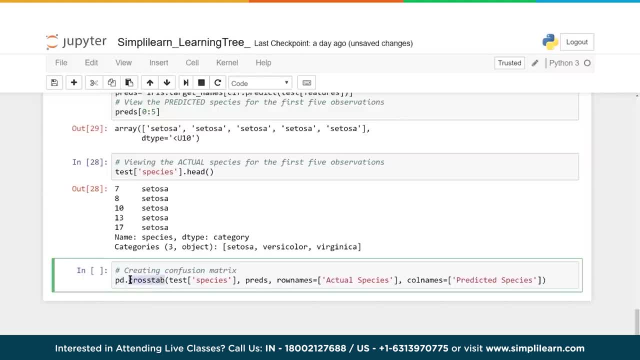 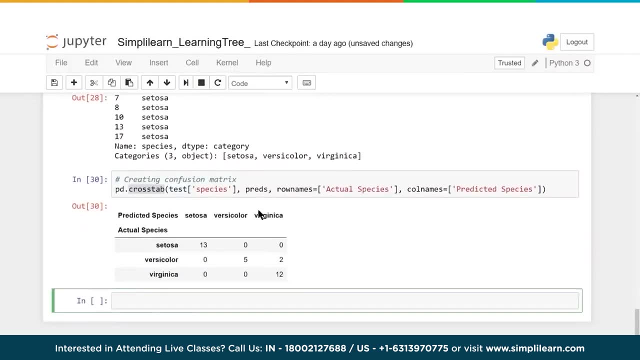 So we're doing pandas- Remember, PD stands for pandas- And we're doing a crosstab. This function takes two sets of data and creates a chart out of them. So when I run it you'll get a nice chart down here And we have the predicted species. 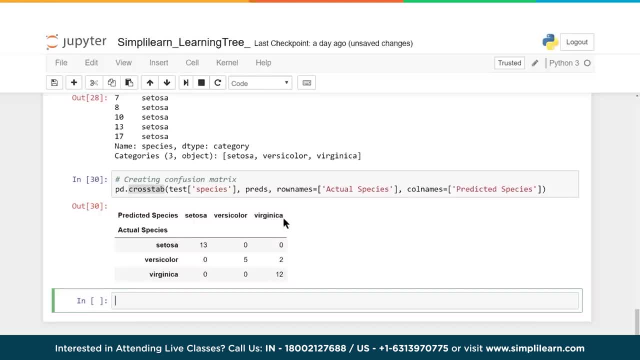 So across the top you'll see the Cetosa versicolor virginica And the actual species, Cetosa versicolor virginica. And so the way to read this chart, and let's go ahead and take a look on how to read this chart here. 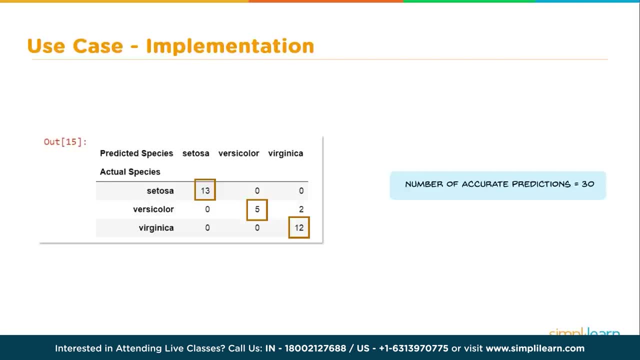 When you read this chart, you have versicolor where they meet. You have versicolor where they meet And you have virginica where they meet And they're meeting where the actual and the predicted agree. So this is the number of accurate predictions. 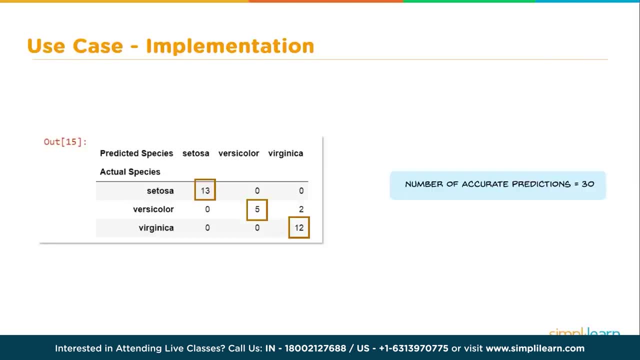 So in this case it equals 30. If you add 13 plus 5 plus 12, you get 30. And then we notice here where it says virginica, but it was supposed to be versicolor. This is inaccurate. So now we have two. 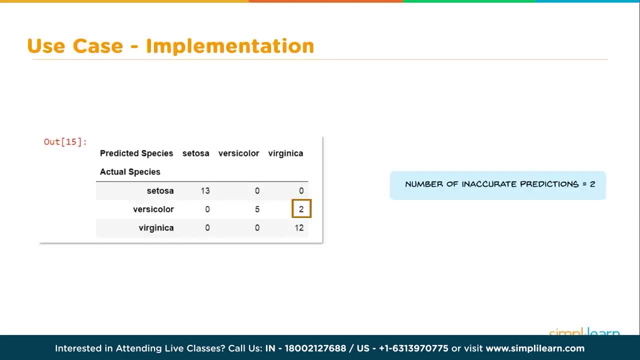 Two inaccurate predictions and 30 accurate predictions. So we'll say that the model accuracy is 93. That's just 30 divided by 32. And if we multiply it by 100, we can say that it is 93% accurate. So we have a 93% accuracy. 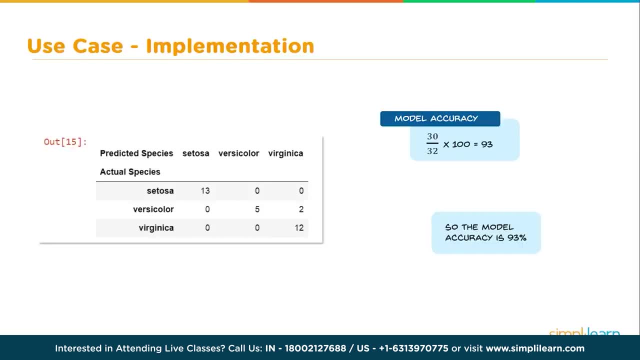 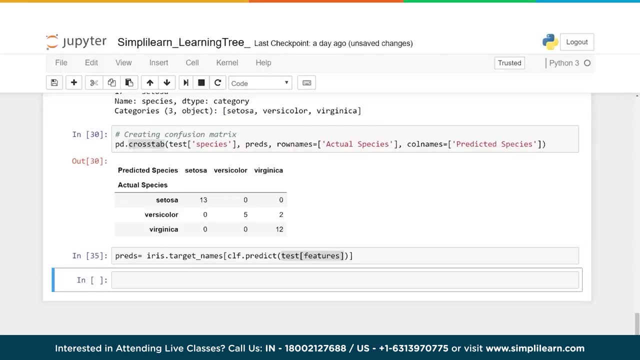 with our model. I did want to add one more quick thing in here on our scripting before we wrap it up. So let's flip back on over to my script In here. we're going to take this line of code from up above. I don't know if you remember it, but 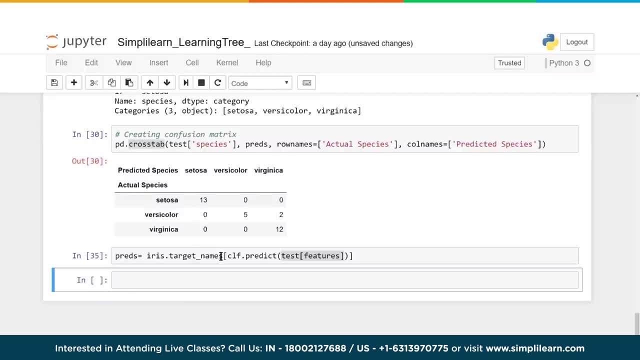 predicts equals the iris dot target underscore names. We're going to map it to the names and we're going to run the prediction and we read it on test features. But you know, we're not just testing it, we want to actually deploy it. So at this point I would go ahead and change this. 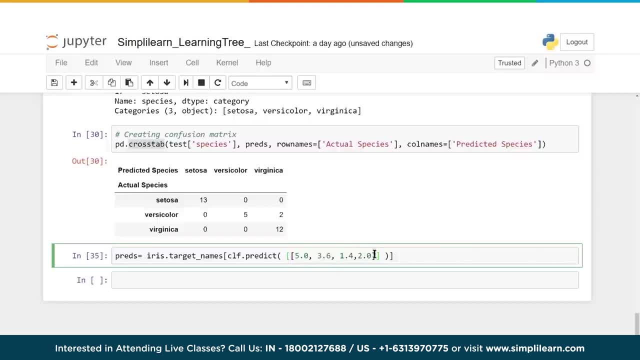 and this is an array of arrays. This is really important when you're running these to know that. So you need the double brackets and that could actually create data. Let's just do two flowers. So maybe I'm processing more data coming in and we'll put two flowers in here. 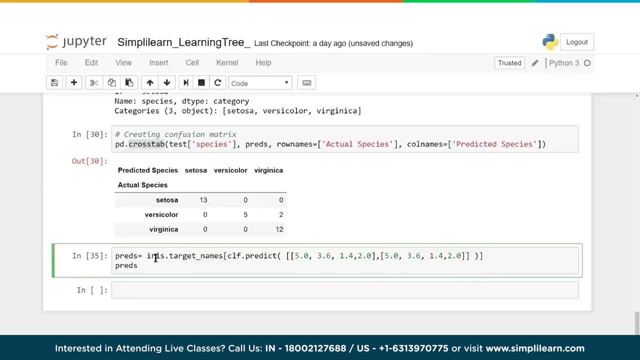 and then I actually want to see what the answer is. So let's go ahead and type in preds and print that out, And when I run this you'll see that I've now predicted two flowers that maybe I measured in my front yard as versicolor and versicolor. 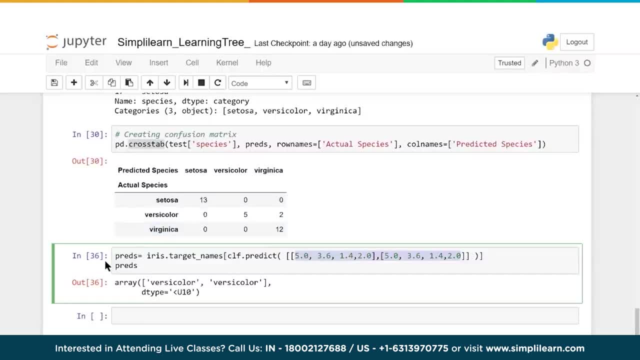 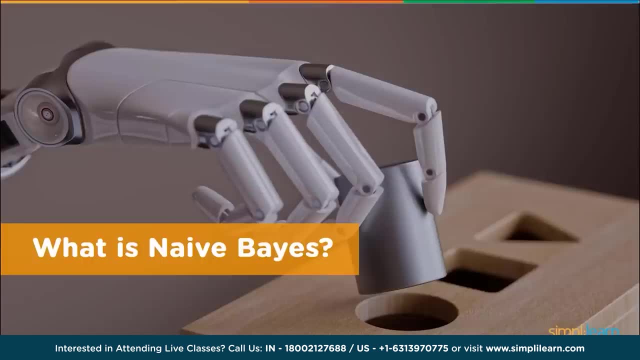 Not surprising, since I put the same data in for each one. This would be the actual end product going out to be used on data that you don't know the answer for What is naive Bayes? Let's start with a basic introduction to the Bayes theorem. 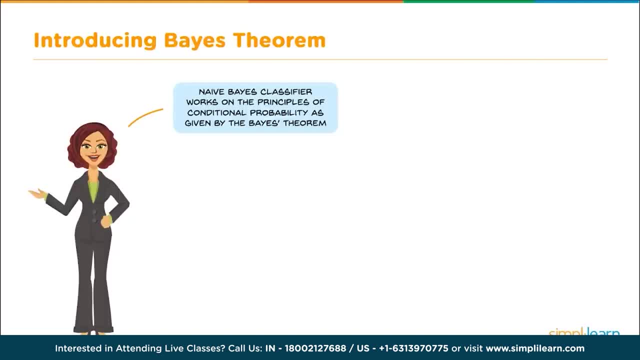 Here we have Thomas Bayes from the 1700s, who first coined this in the western literature. Naive Bayes classifier works on the principle of conditional probability as given by the Bayes theorem. Before we move ahead, let us go through some of the simple concepts and the probability. 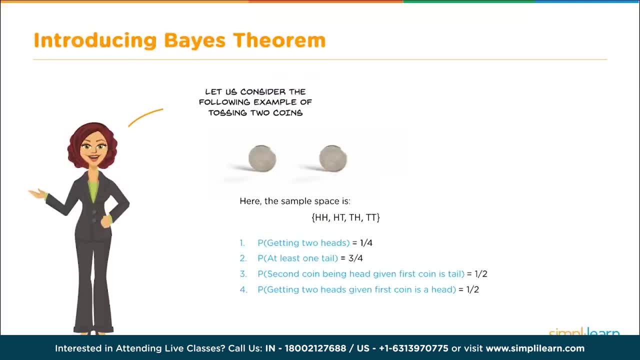 that we will be using. Let us consider the following example of tossing two coins. Here we have two quarters and if we look at all the different possibilities of what they can come up as we get that, they can come up as head heads, come up as head, tell, tell, head and tell, tell. 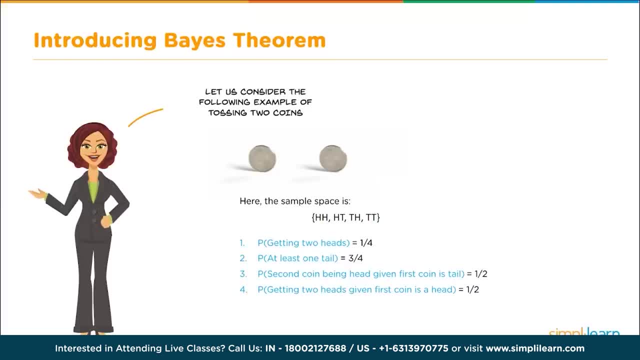 We usually denote probability as a P, a capital P. So the probability of getting two heads equals one fourth. You can see on our data set we have two heads and this occurs once out of the four possibilities, And then the probability of at least one tell. 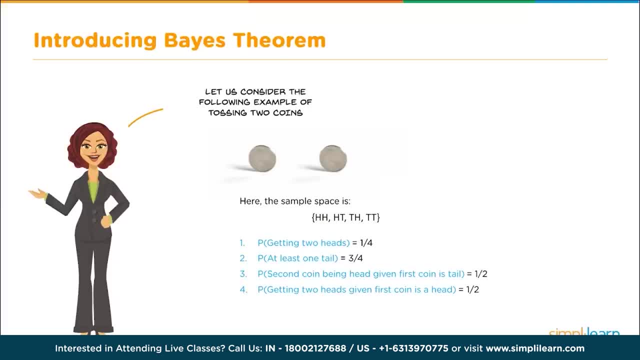 occurs three quarters of the time. You'll see, on three of the coin tosses we have tells in them and out of four that's three fourths. And then the probability of the second coin being head, given the first coin is tell is one half and the probability 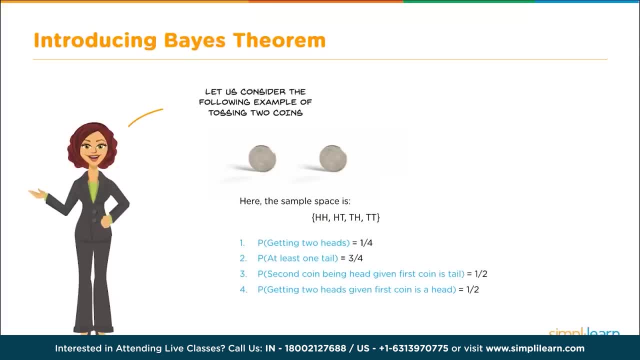 of getting two heads, given the first coin is one half. We'll demonstrate that in just a minute and show you how that math works. Now, when we're doing it with two coins, it's easy to see, but when you have something more complex, you can see where these formulas 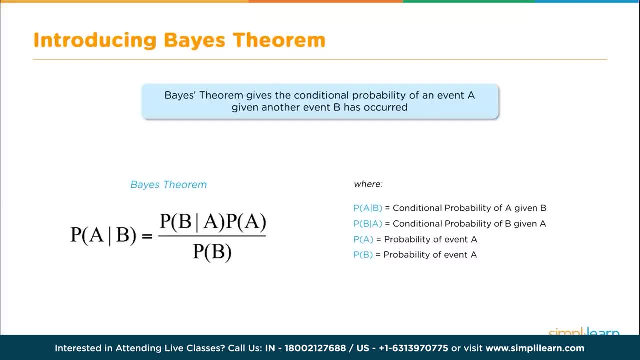 really come in and work. So the Bayes Theorem gives us the conditional probability of an event A given another event B has occurred. In this case, the first coin toss will be B and the second coin toss A. This can be confusing, because we've actually 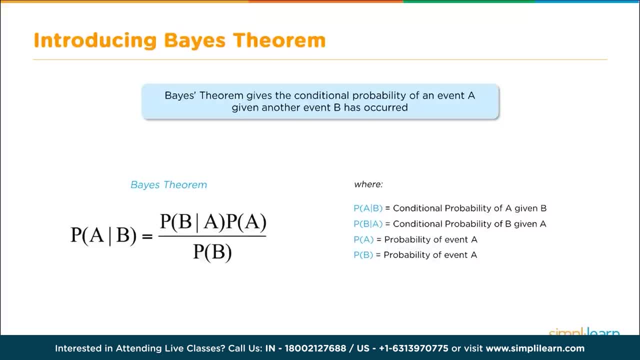 reversed the order of them and go from B to A instead of A to B. It's a lot when you work in probabilities. The reason is we're looking for event A. we want to know what that is, so we're going to label that A, since that's our focus. 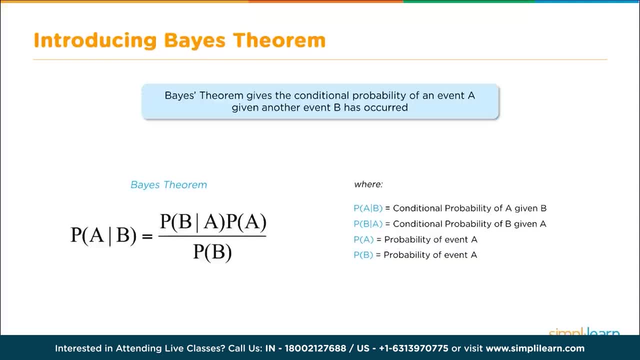 And then, given another event, B has occurred. In the Bayes Theorem, as you can see on the left, the probability of A occurring, given B has occurred, equals the probability of B occurring, given A has occurred, times the probability of A over the probability of B. 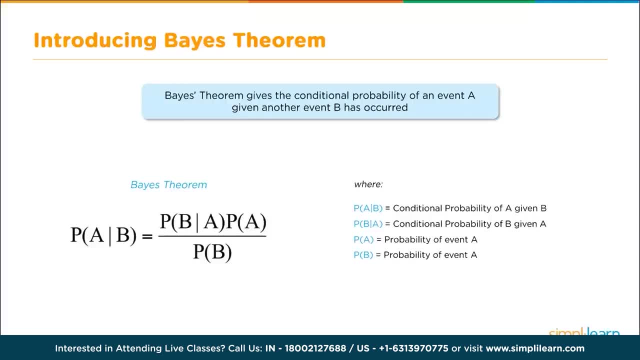 This simple formula can be moved around just like any algebra formula And we could do: the probability of A given B times the probability of B equals the probability of B given A times the probability of A. You can easily move that around and multiply it and divide it out. 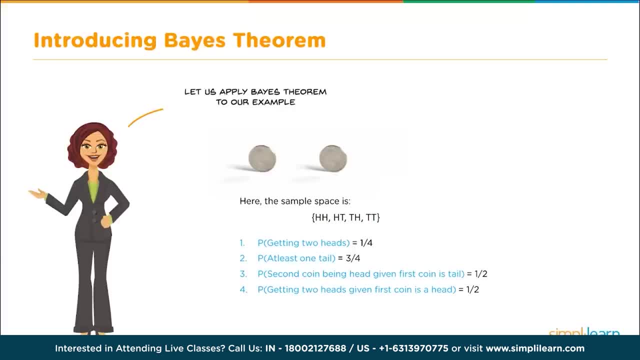 Let us apply Bayes Theorem to our example. Here we have our two quarters and we'll notice that the first two probabilities of getting two heads and at least one tail we compute directly off the data. So you can easily see that we have one example. 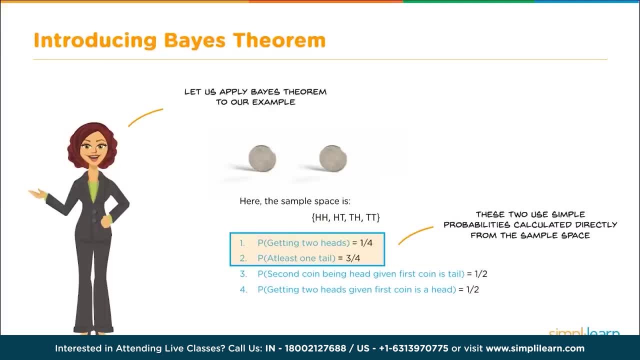 out of four and we have three with tails in them, giving us three quarters or three fourths- 75%. The second condition, the second set, three and four. we're going to explore a little bit more in detail Now. we stick to a simple example with two coins. 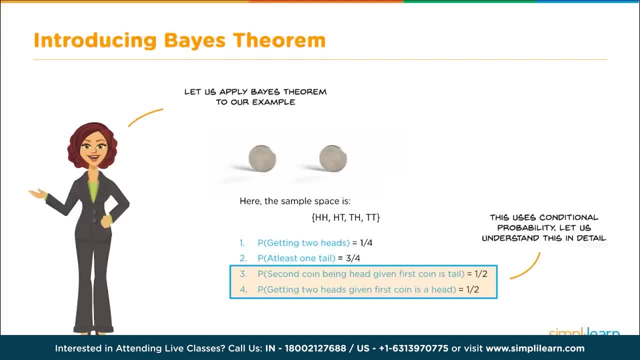 because you can easily understand the math. The probability of throwing a tail doesn't matter what comes before it, and the same with the heads. So it's still going to be 50% or one half. But when that probability gets more complicated, let's say you have a D6 dice. 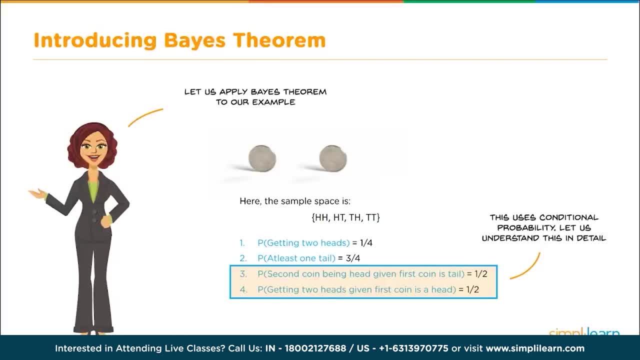 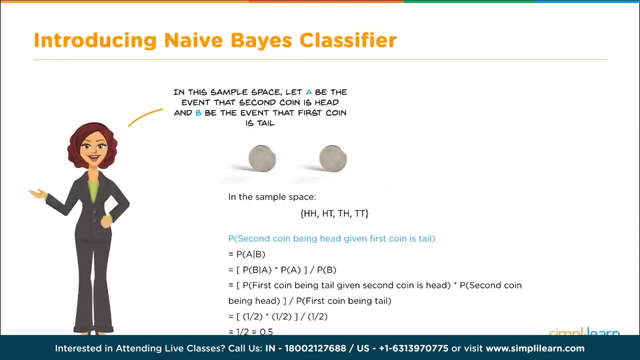 or some other instance, then this formula really comes in handy. But let's stick to the simple example for now. Let A be the event that the second coin is head and B be the event that the first coin is tails. Again, we reversed it because we want to know what the second event is going to be. 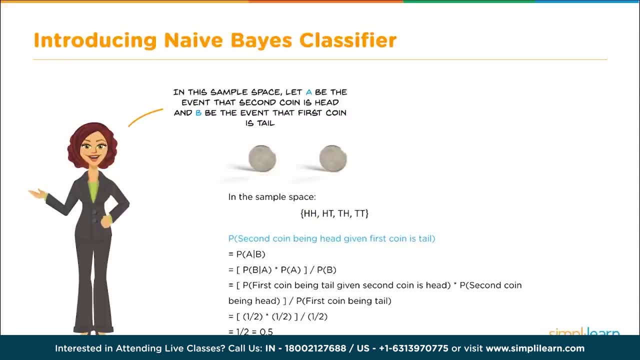 So we're going to be focusing on A And we write that out as the probability of A given B And we know this from our formula, that that equals the probability of B given A times the probability of A over the probability of B. And when we plug that in, 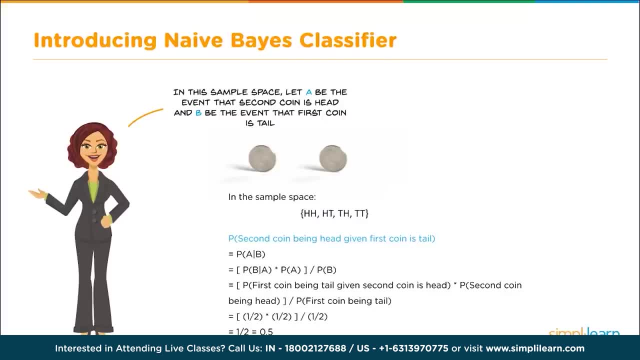 we plug in the probability of the first coin being tails, given the second coin is heads, and the probability of the second coin being heads over the probability of the first coin being tails. When we plug that data in and we have the probability of the first coin being tails. 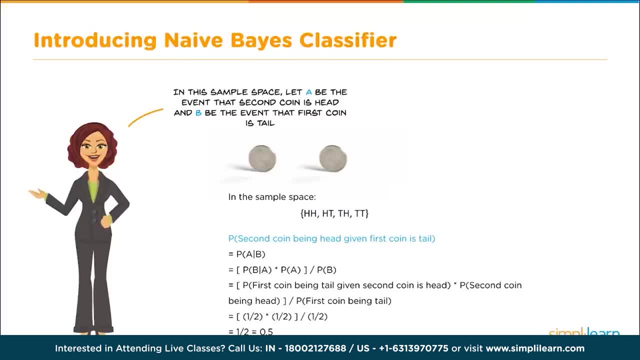 given the second coin is heads times the probability of the second coin being heads over the probability of the first coin being tails. You can see it's a simple formula to calculate. We have one half times one, half over one half, or one half equals .5. 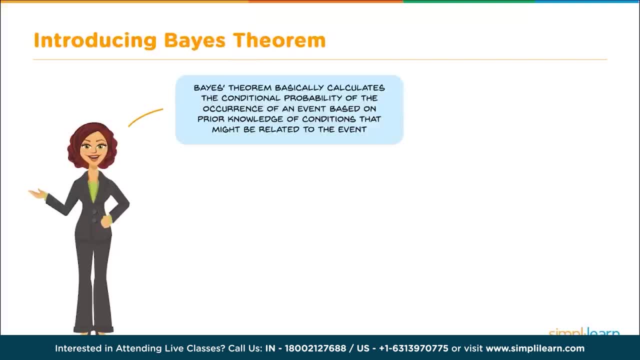 or one fourth. So the Bayes Theorem basically calculates the conditional probability of the occurrence of an event based on prior knowledge of conditional probability and the conditions that might be related to the event. We will explore this in detail when we take up an example of online shopping. 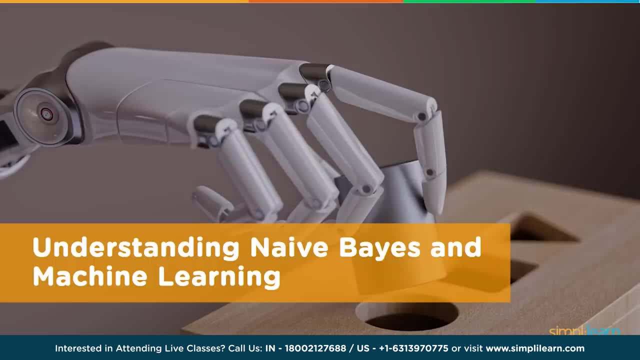 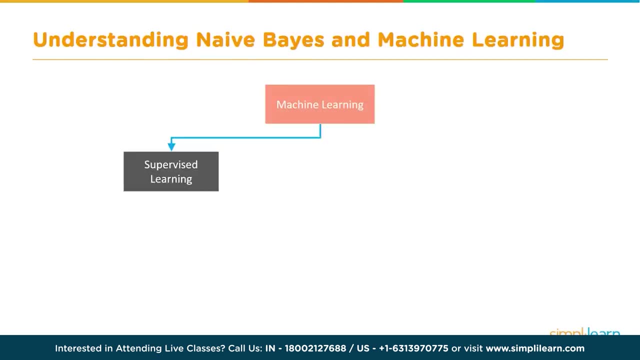 further in this tutorial Understanding naive Bayes and machine learning. Like with any of our other machine learning tools, it's important to understand where the naive Bayes fits in the hierarchy. So under the machine learning, we have supervised learning and there is other things like unsupervised learning. 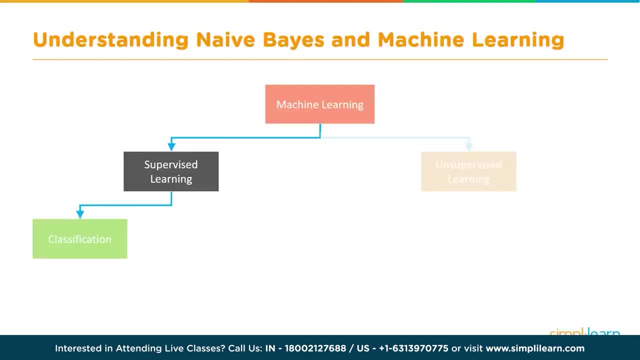 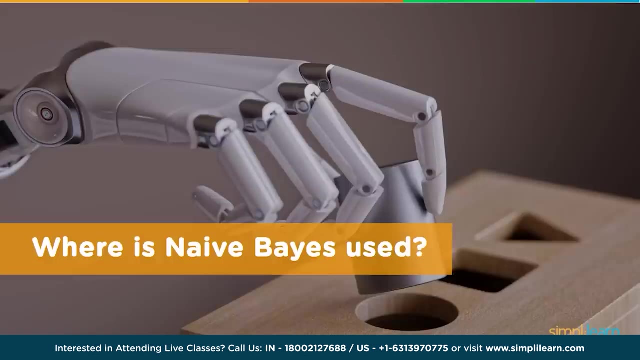 there's also reward system. this falls under the supervised learning, and then under the supervised learning there's classification, there's also regression, and then under classification is your naive Bayes. Let's go ahead and glance into where is naive Bayes used? Let's look at some of the used scenarios for it. 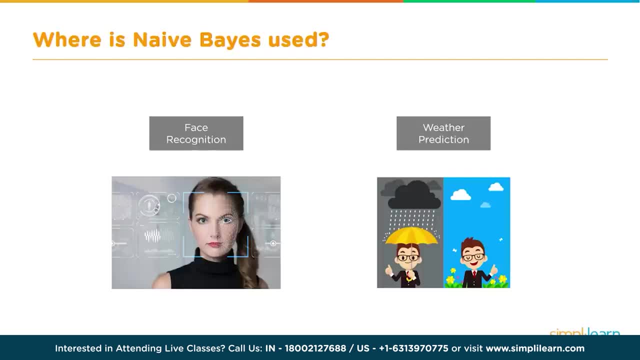 As a classifier. we use it in face recognition- is this Cindy, or is it not Cindy? or whoever? or it might be used to identify parts of the face that they then feed into another part of the face recognition program. This is the eye, this is the nose, this is the mouth. 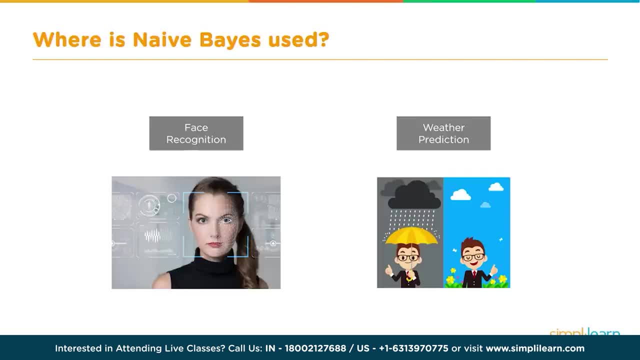 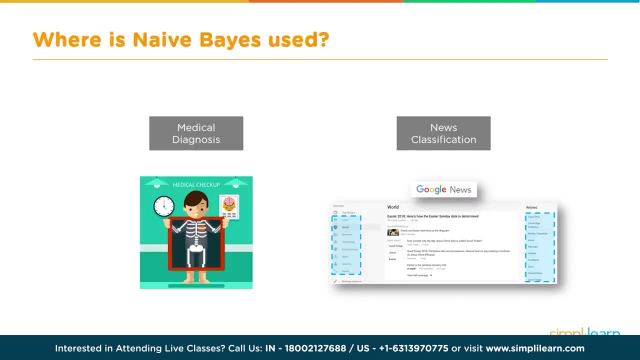 Weather prediction- is it going to be rainy or sunny? Medical recognition: news prediction. political diagnosis: we might diagnose somebody as either as high risk or not as high risk for cancer or heart disease or other ailments, and news classification when you look at the Google news, 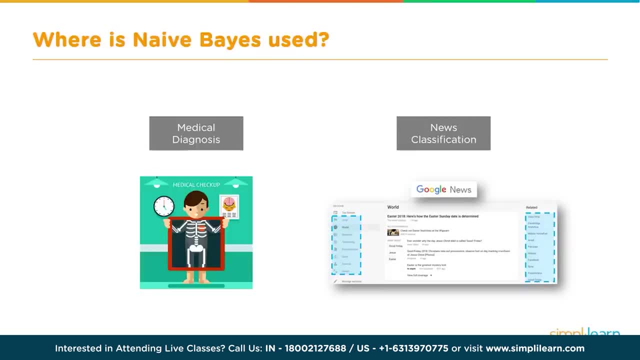 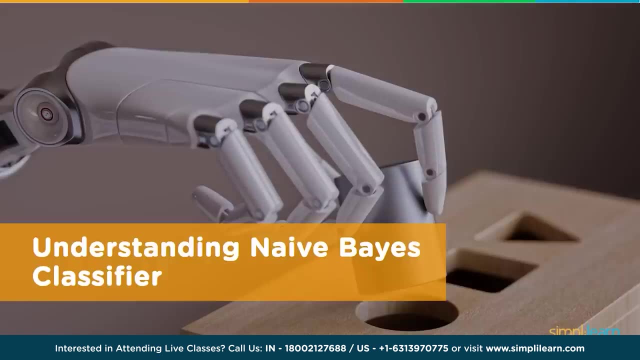 and it says: well, is this political or is this world news, or a lot of that is all done with the naive Bayes Understanding naive Bayes classifier. Now we already went through a basic understanding with the coins and the two heads and two tells, and head, tell, tell, heads, etc. 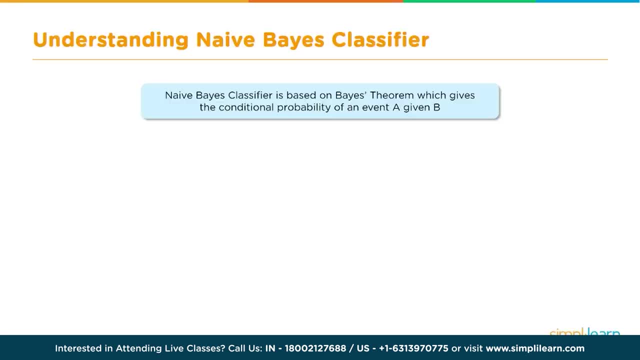 We're going to do just a quick review on that and remind you that the naive Bayes classifier is based on the Bayes theorem, which gives a conditional probability of event A given event B, and that's where the probability of A given B equals the probability of B. 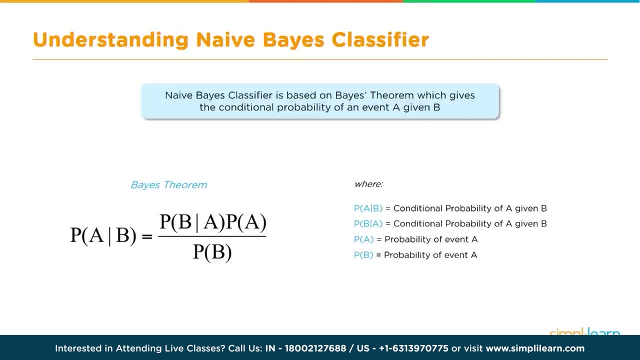 given A times probability of A over probability of B. Remember, this is an algebraic function so we can move these different entities around. We can multiply by the probability of B, so it goes to the left hand side, and then we can divide by the probability of A. 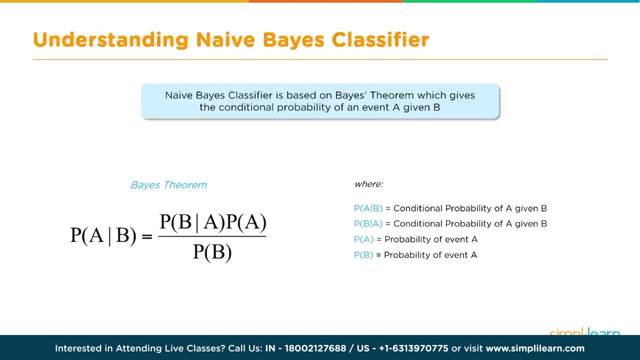 given B and just as easily come up with a new formula for the probability of B. To me, staring at these algebraic functions kind of gives me a slight headache. It's a lot better to see if we can actually understand how this data fits together in a table. And let's go ahead. 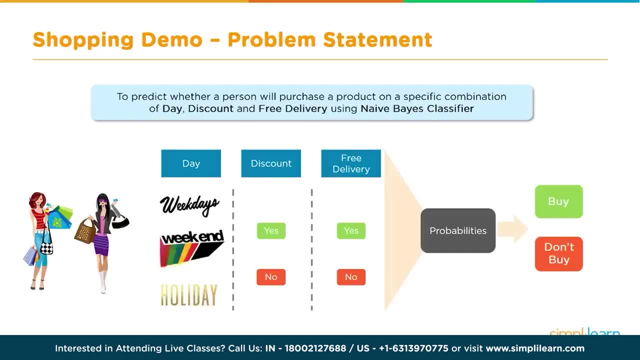 and start applying it to some actual data so you can see what that looks like. So we're going to start with the shopping demo problem statement and remember we're going to solve this first in table form so you can see what the math looks like, and then we're going to solve it. 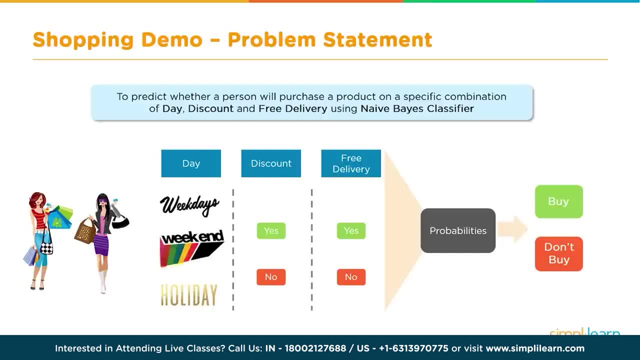 in Python And in here we want to predict whether the person will purchase a product. are they going to buy or don't buy? Very important: if you're running a business, you want to know how to maximize your profits or at least maximize the purchase of the people. 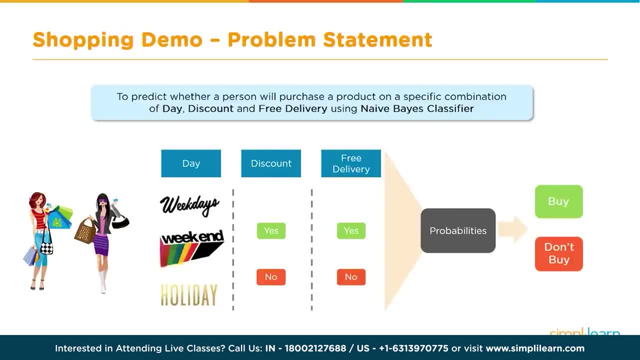 coming into your store And we're going to look at a specific combination of different variables. In this case we're going to look at the day, the discount and the free delivery And you can see here under the day. we want to know whether it's on the weekday. 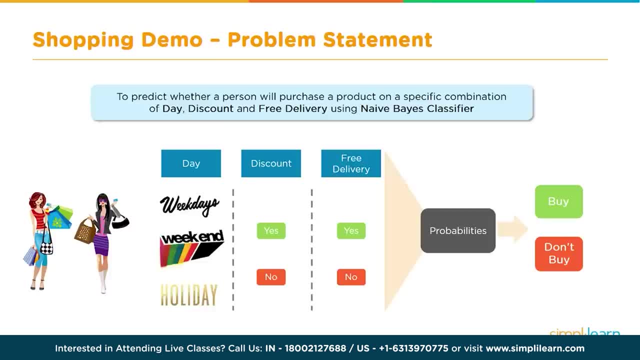 you know somebody's working. they come in after work or maybe they don't work Weekend. you can see the bright colors coming down there celebrating not being in work or holiday. And did we offer a discount that day, Yes or no? Did we offer free delivery? 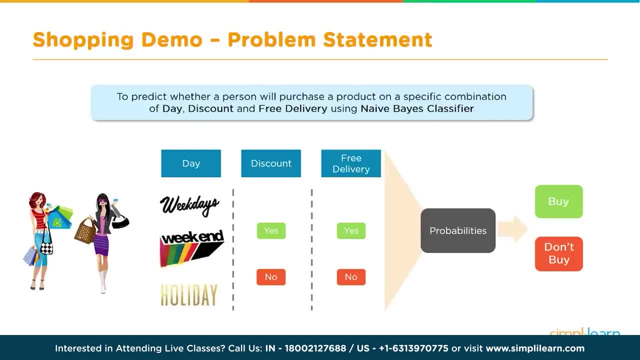 That day Yes or no, And from this we want to know whether the person's going to buy based on these traits, so we can maximize them and find out the best system for getting somebody to come in and purchase our goods and products from our store Now. 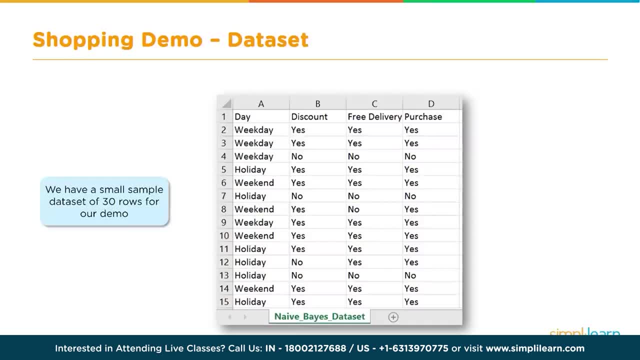 having a nice visual is great, but we do need to dig into the data. So let's go ahead and take a look at the data set. We have a small sample data set of 30 rows. we're showing you the first 15 of those. 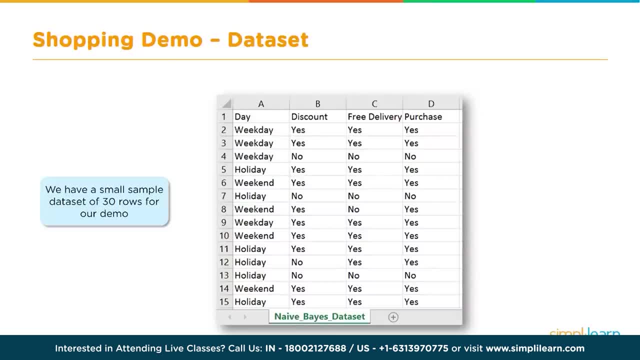 rows for this demo. Now the actual data file you can request, just type in below under the comments on the YouTube video and we'll send you some more information and send you that file. As you can see here, the file is very simple: columns and rows. We have the day. 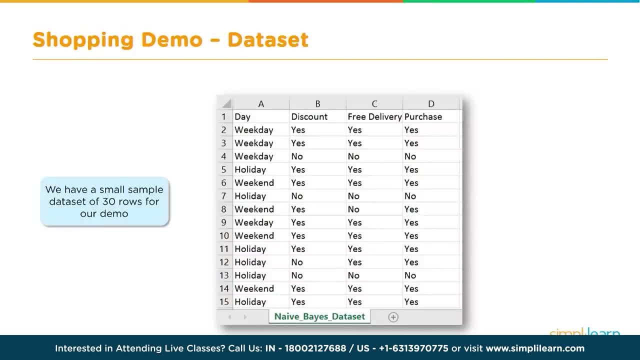 the discount, the free delivery, and did the person purchase or not? And then we have under the day whether it was a weekday, a holiday, was it the weekend? This is a pretty simple set of data and long before computers, people used to look at this data. 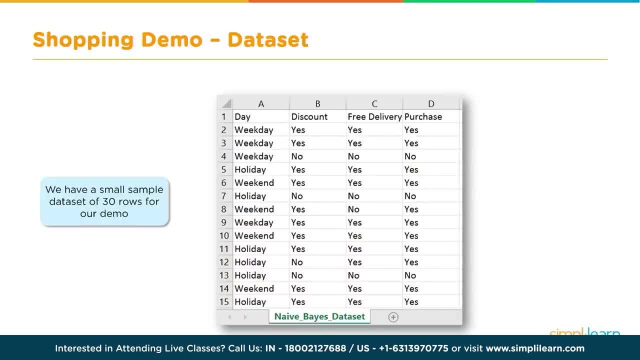 and calculate this all by hand. So let's go ahead and walk through this and see what that looks like when we put that into tables. Also note: in today's world we're not usually looking at three different variables in 30 rows Nowadays, because we're able to collect data so much we're. 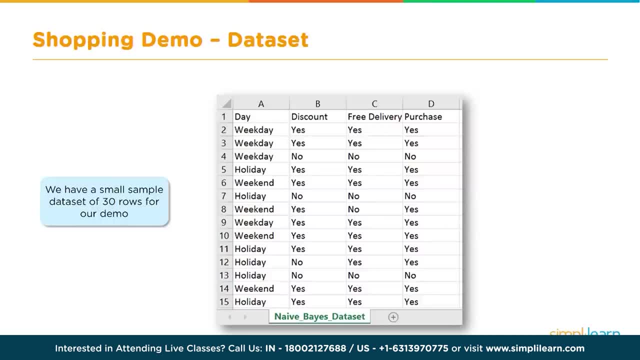 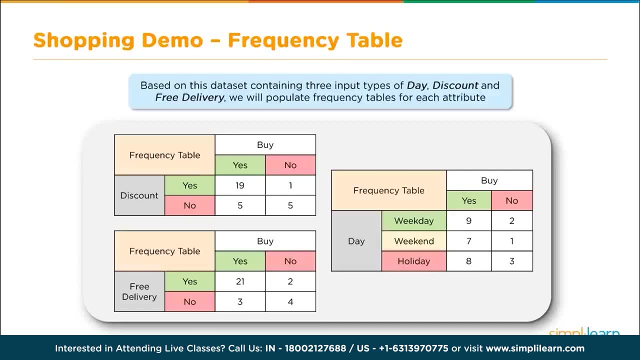 usually looking at 27,- 30 variables across hundreds of rows. The first thing we want to do is we're going to take this data and, based on the data set containing our three inputs- day discount and free delivery- we're going to go ahead and 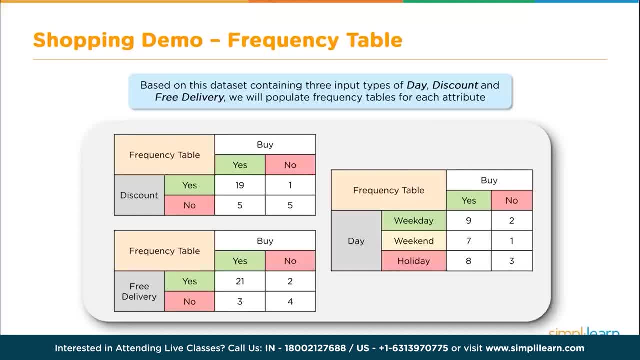 populate that to frequency tables for each attribute. So we want to know if they had a discount. how many people buy and did not buy? did they have a discount, yes or no? Do we have a free delivery, yes or no? On those days, how many people made a purchase? 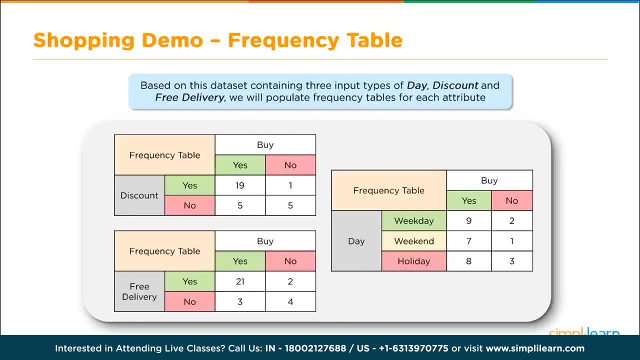 and how many people didn't. And the same with the three days of the week. Was it a weekday, a weekend, a holiday? And did they buy, yes or no? As we dig in deeper to this table for our Bayes Theorem, let 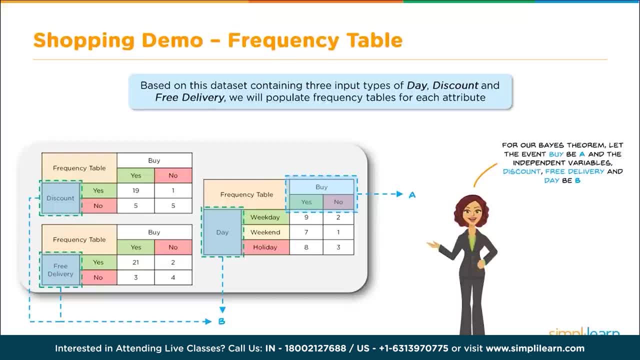 the event buy be A. Now remember when we looked at the coins I said we really want to know what the outcome is- Did the person buy or not? And that's usually event A is what you're looking for And the independent variables discount, free delivery. 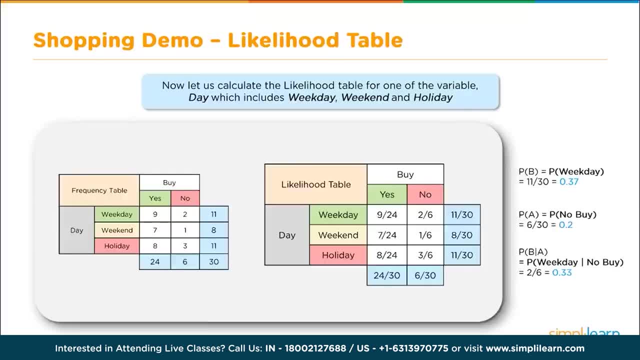 and day be B, So we'll call that probability of B. Now let us calculate the likelihood table for one of the variables. Let's start with day, which includes weekday, weekend and holiday, And let us start by summing all of our rows. So 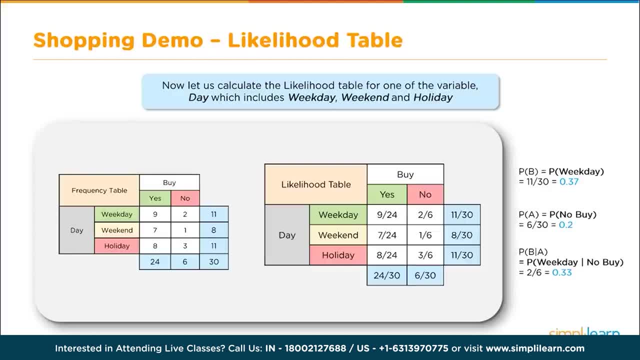 we have the weekday row, and out of the weekdays there's 9 plus 2, so it's 11 weekdays. There's 8 weekend days and 11 holidays. That's a lot of holidays. And then we want to sum up the total number. 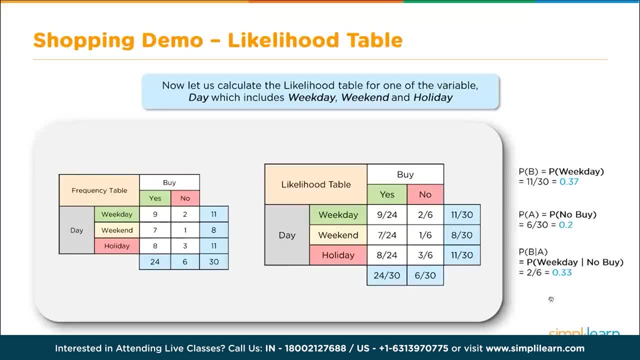 of days, So we're looking at a total of 30 days. Let's start pulling some information from our chart and see where that takes us, And when we fill in the chart on the right, you can see that 9 out of 24. 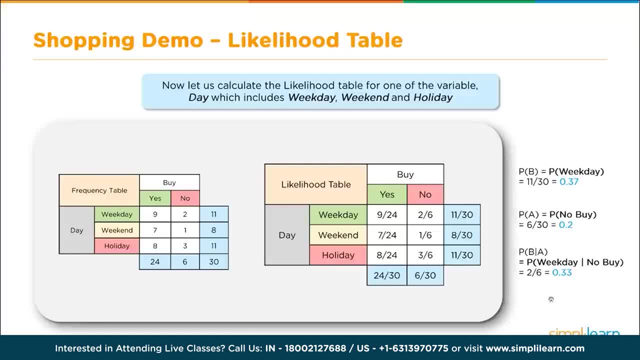 purchases are made on the weekday, 7 out of 24 purchases on the weekend and 8 out of 24 purchases on a holiday, And out of all the people who come in, 24 out of 30 purchase. You can also see how many people do not. 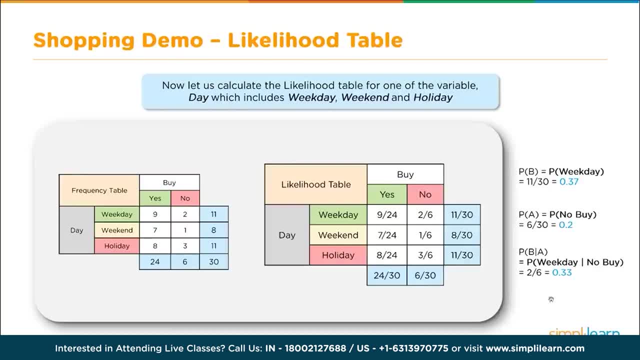 purchase On the weekday, it's 2 out of 6 didn't purchase, and so on, and so on. We can also look at the totals and you'll see. on the right we put together some of the formulas. The probability of making a purchase on the weekend comes. 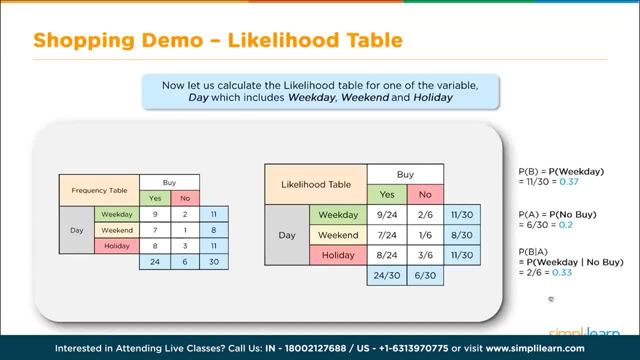 out 11 out of 30.. So out of the 30 people who came into the store throughout the weekend, weekday and holiday, 11 of those purchases were made on the weekday, And then you can also see the probability of them not making a purchase. And this is done for. 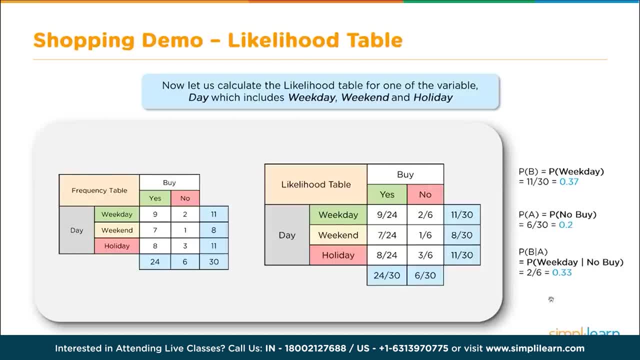 it doesn't matter which day of the week. So we call that probability of no buy would be 6 over 30 or 0.2.. So there's a 20% chance that they're not going to make a purchase no matter what day. 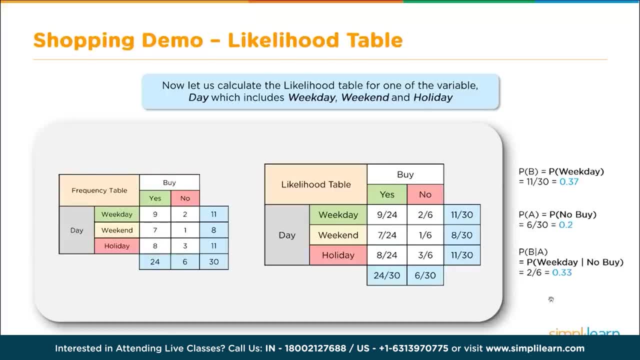 of the week it is And finally, we look at the probability of B of A. In this case we're going to look at the probability of the weekday and not buying. Two of the no buys were done on the weekend out of the six people who did not. 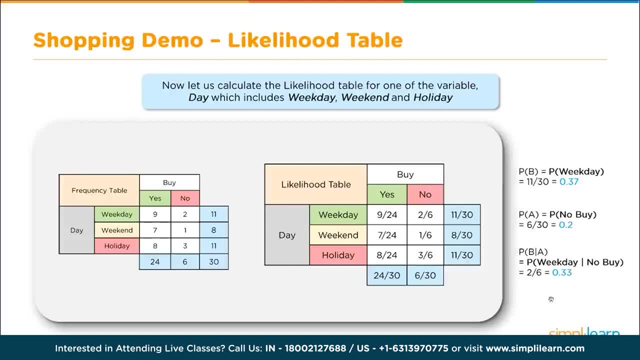 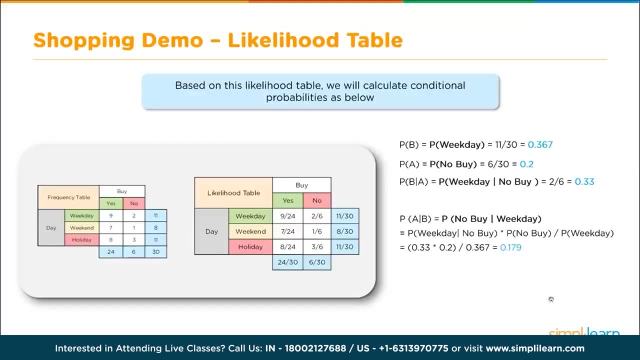 make purchases. So when we look at that probability of the weekday without a purchase is going to be 0.33 or 33%, Let's take a look at this, at different probabilities, and, based on this likelihood table, let's go ahead and calculate. 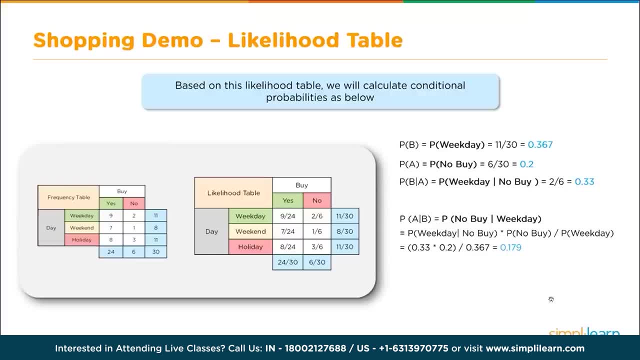 conditional probabilities as below The first three we just did. the probability of making a purchase on the weekday is 11 out of 30, or roughly 36, or 37%, 0.367.. The probability of not making a purchase at all doesn't matter. 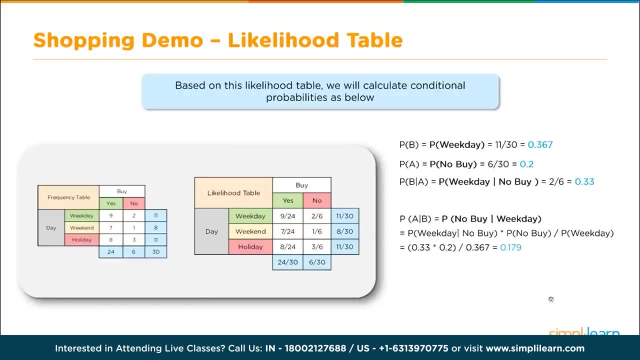 what day of the week is roughly 0.2 or 20%, And the probability of a weekday no purchase is roughly 2 out of 6.. So 2 out of 6 of our no purchases were made on the weekday. And then, finally, we take 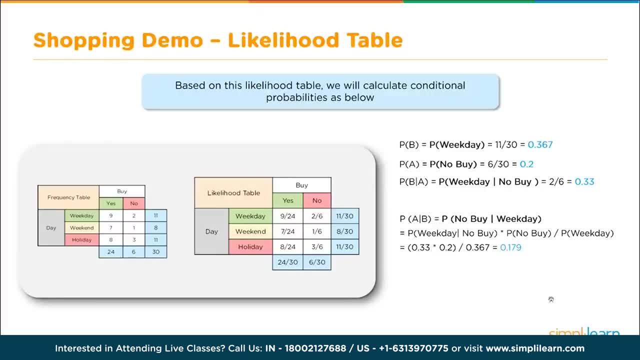 our P. If you look, we've kept the symbols up there. We've got probability of B, probability of A, probability of B if A. We should remember that the probability of A if B is equal to the first, one times the probability of. 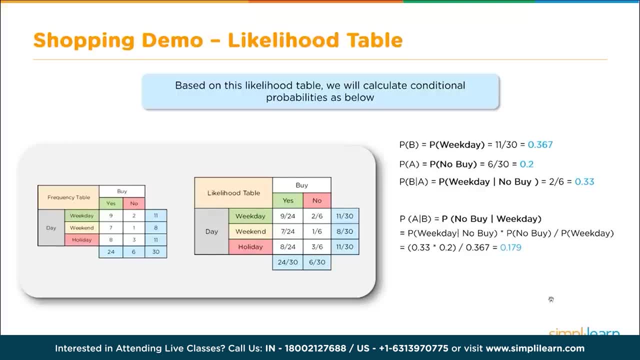 no buys over the probability of the weekday, So we could calculate it both off the table we created. we can also calculate this by the formula and we get the 0.367, which equals 0.33 times 0.2, over 0.367, which equals: 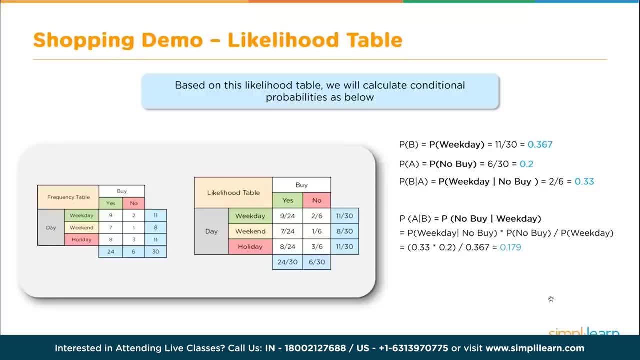 0.179, or roughly 17 to 18%, And that would be the probability of no purchase done on the weekday. This is important because we can look at this and say, as the probability of buying on the weekday is more than the probability of not, 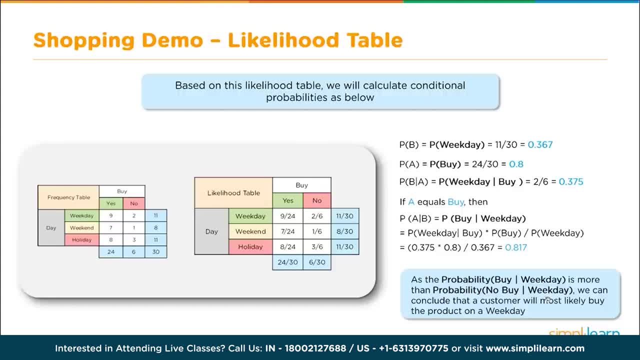 buying on the weekday, we can conclude that customers will most likely buy the product on a weekday. Now we've kept our chart simple and we're only looking at one aspect, So you should be able to look at the table and come up with the same. 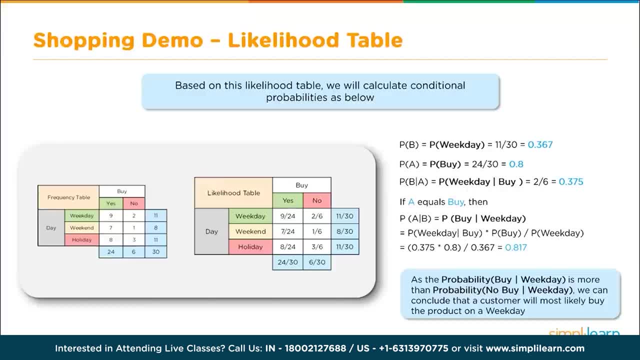 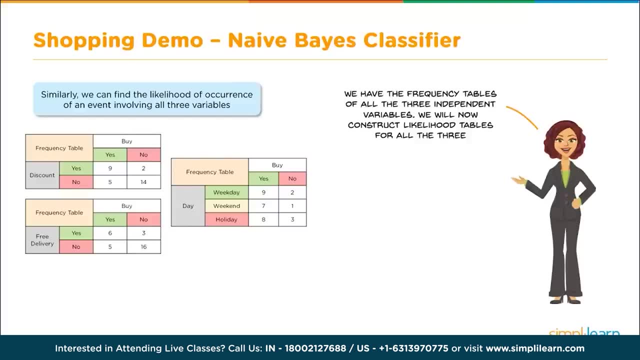 information or the same conclusion. That should be kind of intuitive at this point. Next, we can take the same setup. We have the frequency tables of all three independent variables. Now we can construct the likelihood tables for all three of the variables we're working with. We can take our 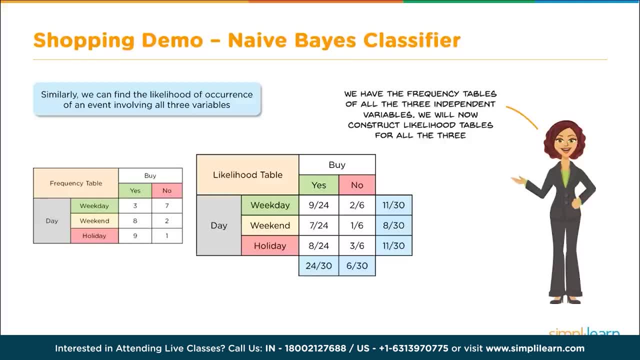 table and we can say, like we did before: we have weekday, weekend and holiday. We filled in this table And then we can come in and also do that. for the discount- Yes or no, Did they buy, Yes or no? And we fill in that. 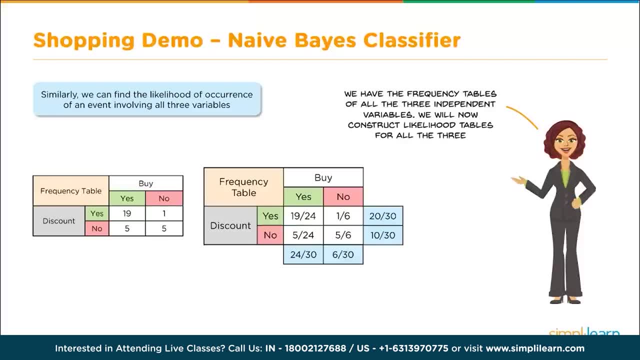 full table. So now we have our probabilities for a discount and whether the discount leads to a purchase or not, And the probability for free delivery. Does that lead to a purchase or not? And this is where it starts getting really exciting. Let us use these three likelihood tables. 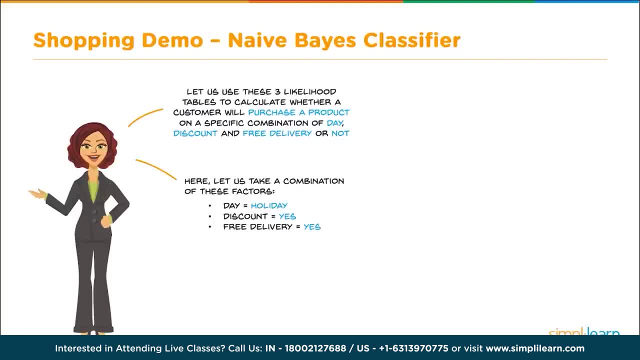 to calculate whether a customer will purchase a product on a specific combination of day discount and free delivery or not purchase. Here let us take a combination of these factors: Day equals- holiday. Discount equals yes. Free delivery equals- yes. Let's dig deeper into. 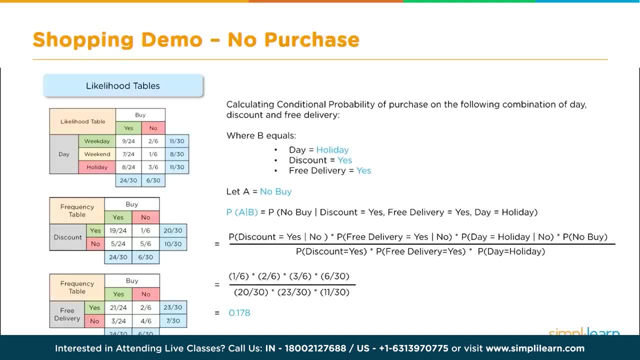 the math and actually see what this looks like, And we're going to start with looking for the probability of them not purchasing on the following combinations of days. We're actually looking for the probability of A equal- no buy, no purchase- And our probability of B we're going to set equal. 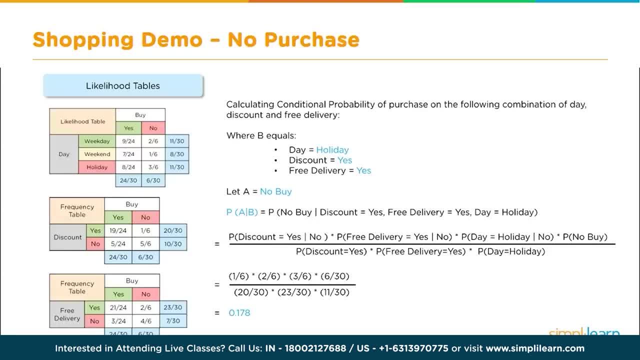 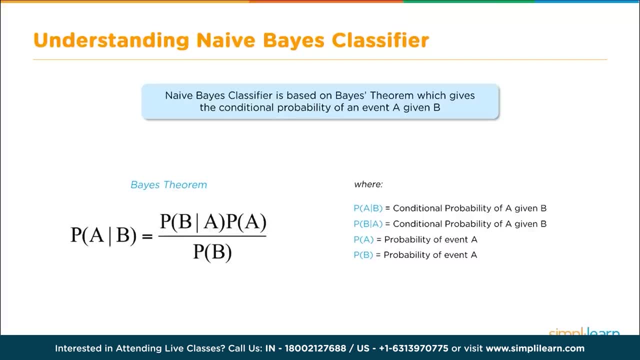 to. is it a holiday? Did they get a discount? Yes, And was it a free delivery? Yes. Before we go further, let's look at the original equation: The probability of A if B equals the probability of B, given the condition. 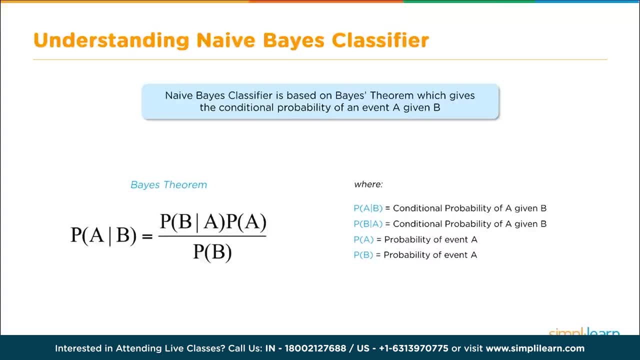 A and the probability times, the probability of A over the probability of B occurring. Now this is basic algebra, so we can multiply this information together. So when you see the probability of A given B, in this case the condition is B, C and D. 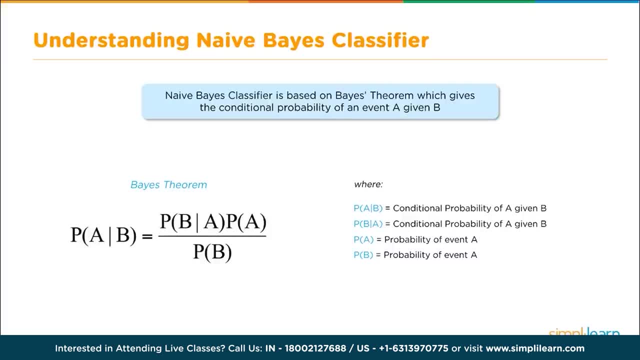 Or the three different variables we're looking at, And when you see the probability of B, that would be the conditions- we're actually going to multiply those three separate conditions out, Probability of. you'll see that in just a second in the formula times, the full probability. 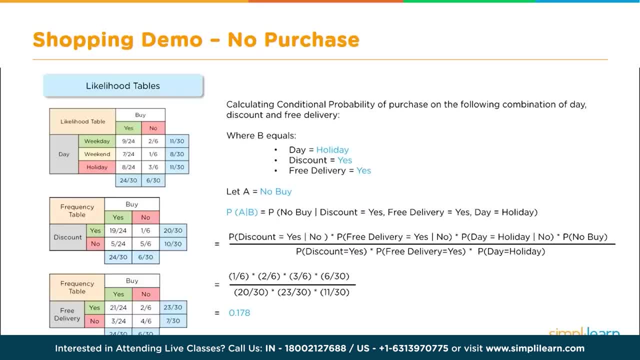 of A over the full probability of B. So here we are back to this and we're going to have let A equal no purchase and we're looking for the probability of B on the condition A, where A sets for three different things. Remember that equals the probability of. 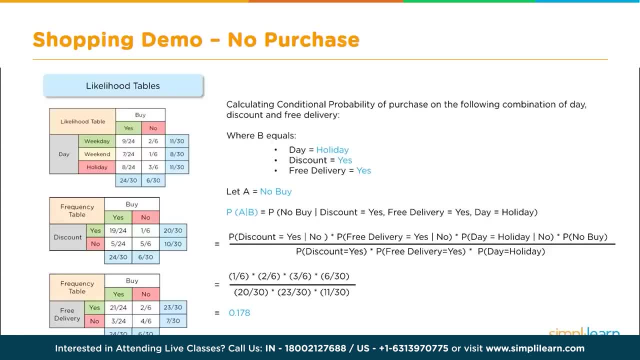 A, given the condition B, And in this case we just multiply those three different variables together. So we have the probability of the discount times, the probability of free delivery times, the probability is the day equal a holiday. Those are our three variables of the probability of A if B. 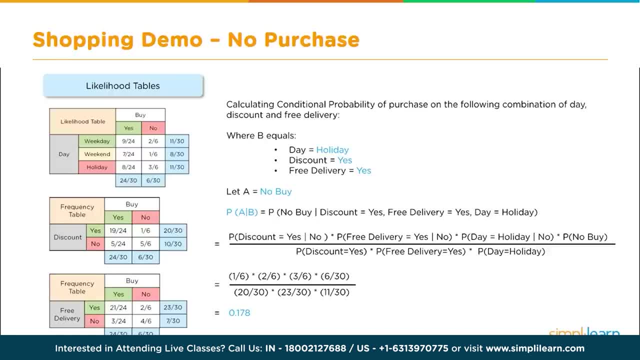 And then that is going to be multiplied by the probability of them not making a purchase. And then we want to divide that by the total probabilities and they're multiplied together. So we have the probability of a discount, the probability of a free delivery and the probability 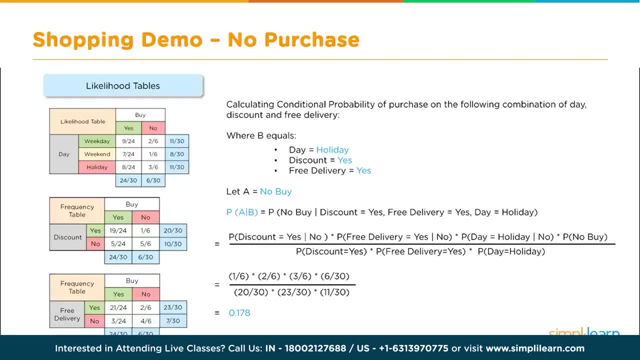 of it being on a holiday. When we plug those numbers in, we see that one out of six were no purchase on a discounted day, two out of six were a no purchase on a free delivery day and three out of six were a no purchase. 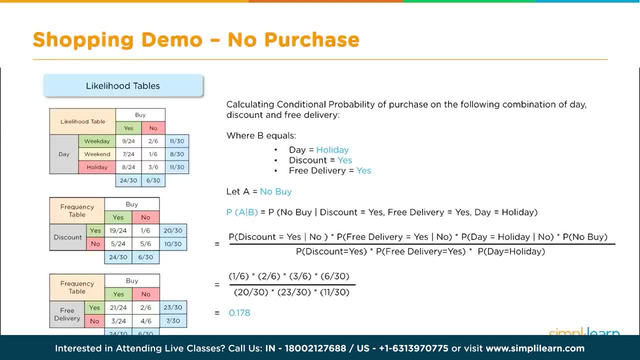 on a holiday. Those are our three probabilities of A if B multiplied out. And then that has to be multiplied by the probability of a no purchase. And remember, the probability of a no buy is across all the data. So that's where we get the six out of thirty. 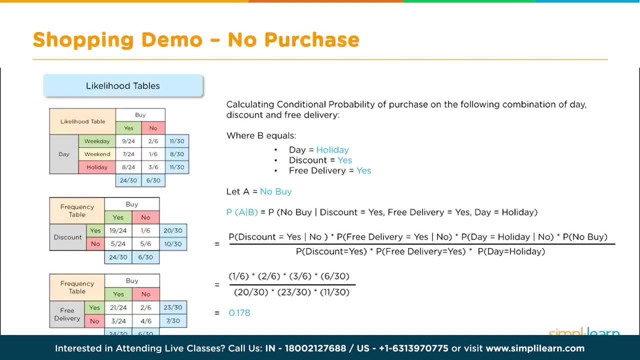 We divide that out by the probability of each category over the total number. So we get the twenty out of thirty had a discount, twenty-three out of thirty had a yes for free delivery and eleven out of thirty were on a holiday. We plug all those numbers in. 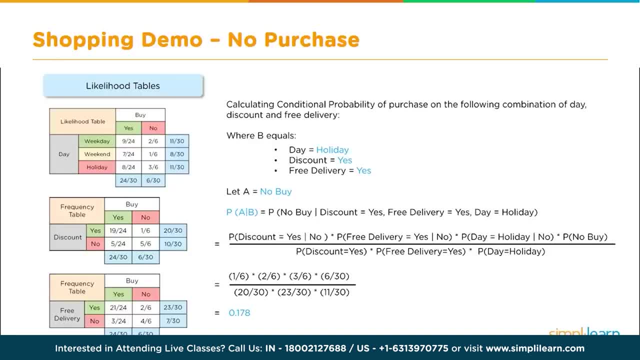 we get .178.. So in our probability math we have a .178. if it's a no buy for a holiday, a discount and a free delivery, Let's turn that around and see what that looks like if we have a purchase. 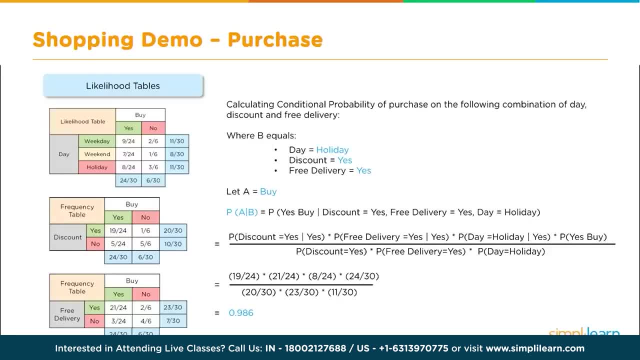 I promise this is the last page of math before we dig into the Python script. So here we're, calculating the probability of the purchase using the same math we did to find out if they didn't buy. Now we want to know if they did buy. 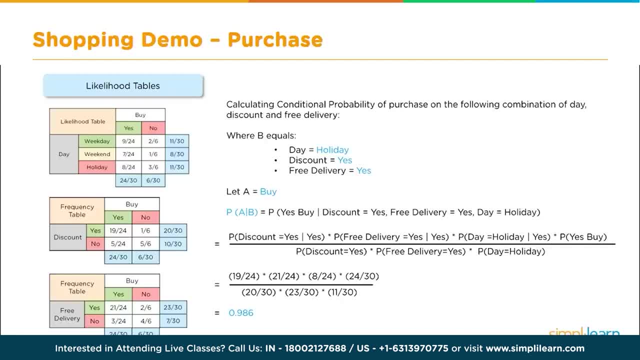 And again we're going to go by the day: equals a holiday discount equals yes, free delivery equals yes, and let A equal buy. Now, right about now, you might be asking: why are we doing both calculations? Why would we want to know the? 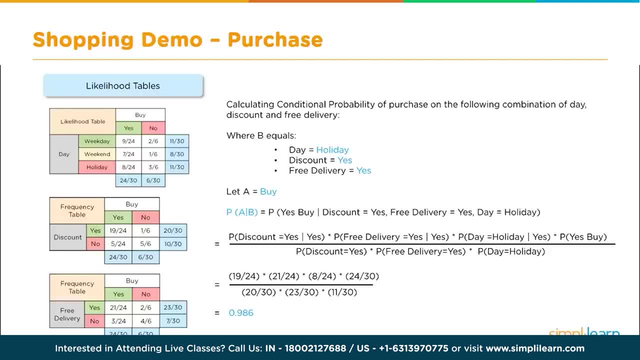 no buys and buys for the same data going in. Well, we're going to show you that in just a moment. we're going to have both of those pieces of information so that we can figure it out as a percentage as opposed to a probability. 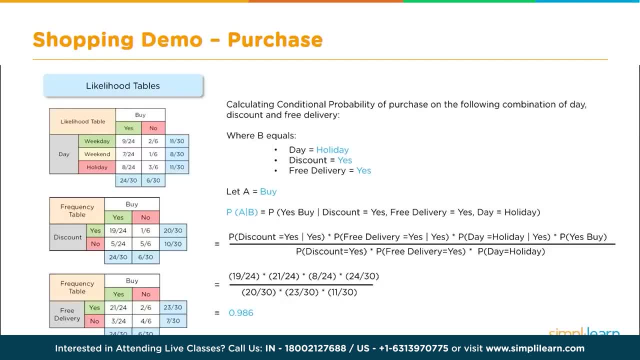 equation And we'll get to that normalization here in just a moment. Let's go ahead and walk through this calculation And, as you can see here, the probability of A on the condition of B, B being all three categories- Did we have. 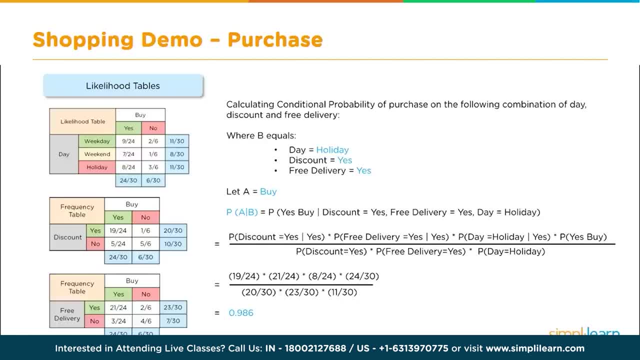 a discount with a purchase, Did we have a free delivery with a purchase? And is a day equal to holiday. And when we plug this all into that formula and multiply it all out, we get our probability of a discount, probability of a free delivery probability. 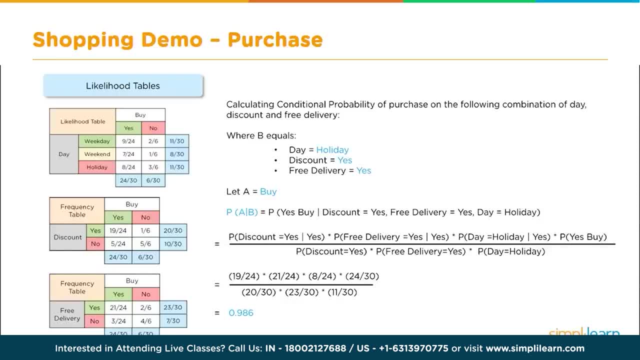 of the day being a holiday times, the overall probability of it being a purchase divided by again multiplying the three variables out: the full probability of there being a discount, the full probability of being a free delivery and the full probability of there being a day equal holiday. 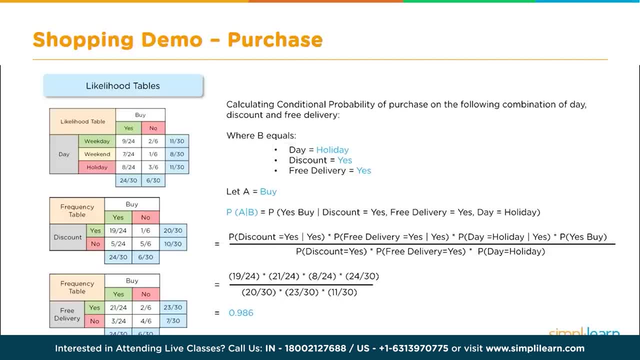 And that's where we get this: 19 over 24 times 21 over 24, times, 8 over 24, times the P of A 24 over 30 divided by the probability of the discount, the free delivery times the day, or 20 over 30,, 23 over 30. 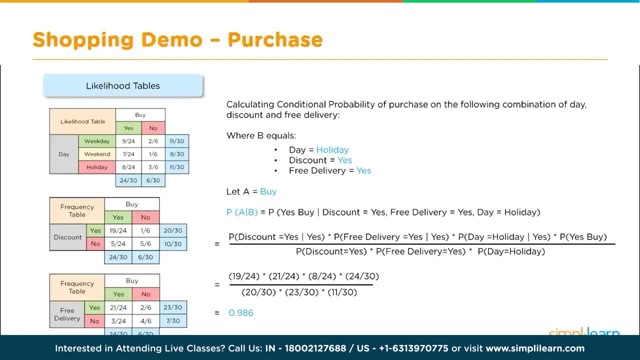 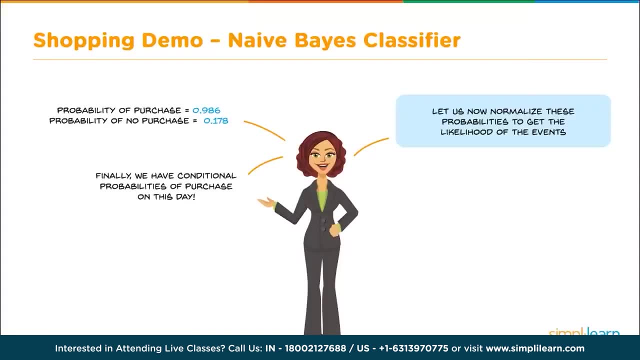 times 11 over 30, and that gives us our .986.. So what are we going to do with these two pieces of data we just generated? Well, let's go ahead and go over them. We have a probability of purchase equals .986. 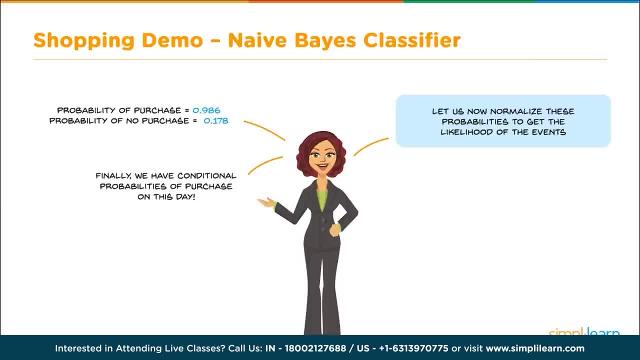 We have a probability of no purchase equals .178. So, finally, we have a conditional probabilities of purchase on this day. Let us take that we're going to normalize it and we're going to take these probabilities and turn them into percentages. This is simply done by taking the 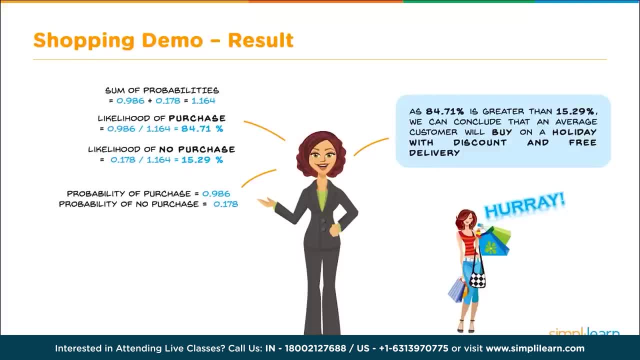 sum of probabilities which equals .986 plus .178, and that equals the 1.164.. If we divide each probability by the sum, we get the percentage, And so the likelihood of a purchase is 84.71% and the likelihood of 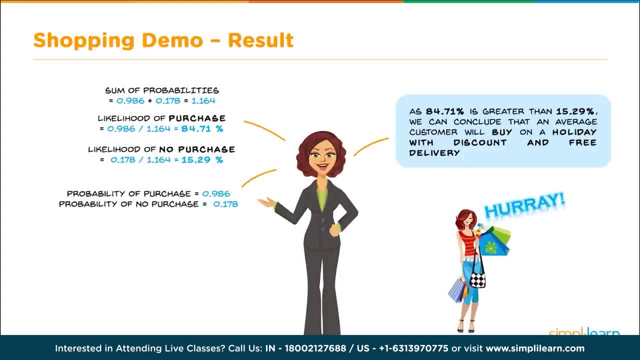 no purchase is 15.29%, given these three different variables. So if it's on a holiday, if it's a discount and has free delivery, then there's an 84.71% chance that the customer is going to come in and make a purchase. 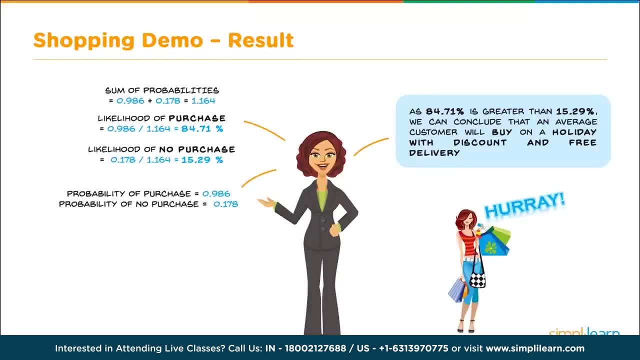 Hooray, They purchased our stuff. We're making money. If you're owning a shop, that is the bottom line- is you want to make some money so that you can keep your shop open and have a living? Now, I promised you that we were going. 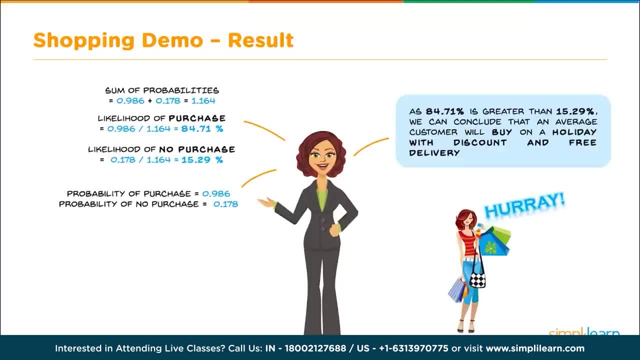 to be finishing up the math here with a few pages. So we're going to move on and we're going to do two steps. The first step is: I want you to understand why you want to use the naive Bayes. What are the advantages of naive Bayes? 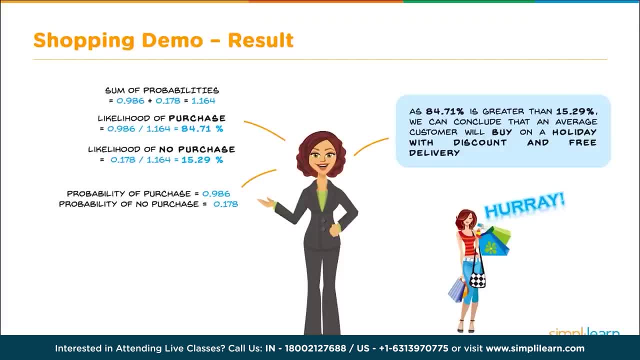 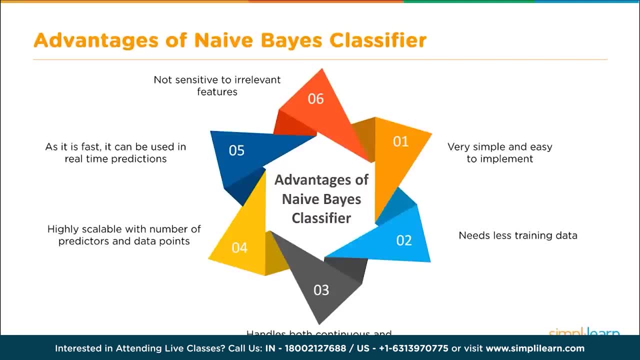 And then once we understand those advantages, we'll just look at that briefly. then we're going to dive in and do some Python coding. Advantages of naive Bayes classifier. So let's take a look at the six advantages of the naive Bayes classifier and we're. 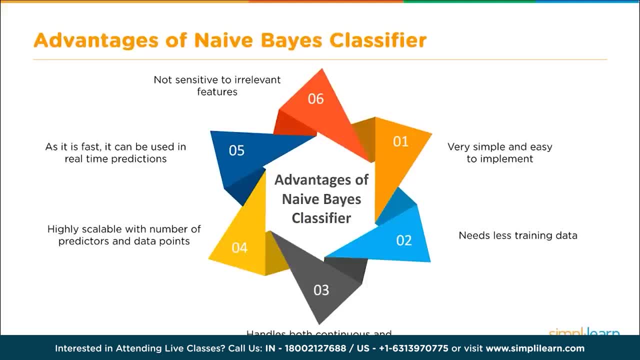 going to walk around this lovely wheel. It looks like an origami folded paper. The first one is very simple and easy to implement. Certainly you could walk through the tables and do this by hand. You've got to be a little careful because the notations 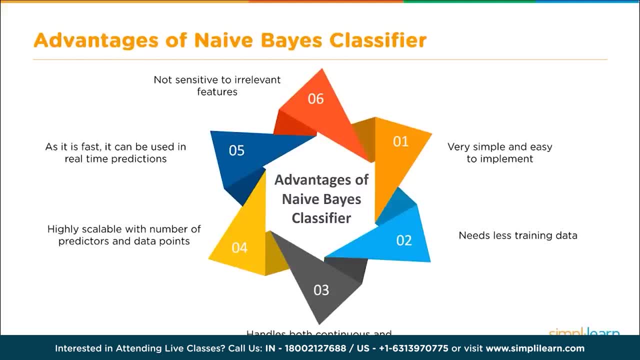 can get confusing. You have all these different probabilities and I certainly mess those up as I put them on. you know, is it on the top or the bottom? You've got to really pay close attention to that When you put it into Python. 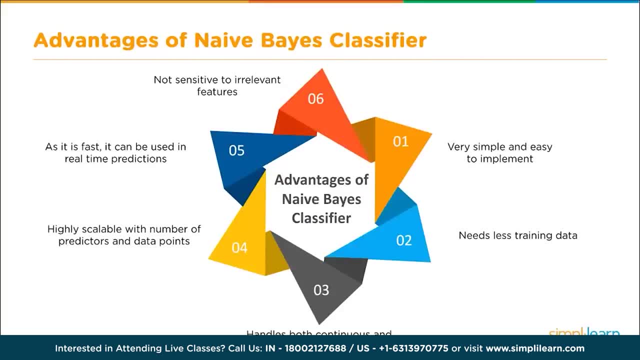 it's really nice because you don't have to worry about any of that. You let the Python handle that, the Python module. But, understanding it, you can put it on a table and you can easily see how it works. and it's a simple algebraic function. 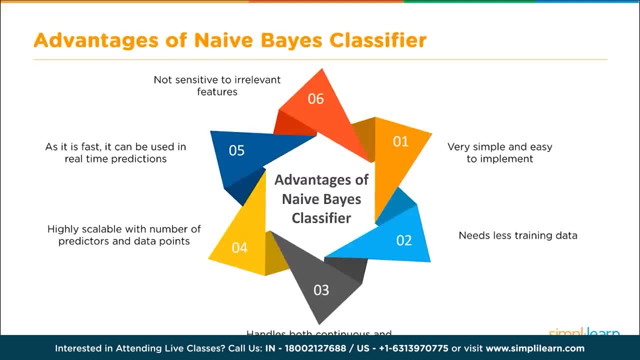 It needs less training data, so if you have smaller amounts of data, this is a great powerful tool for that Handles both continuous and discrete data. It's highly scalable with number of predictors and data points, So, as you can see, you just keep multiplying. 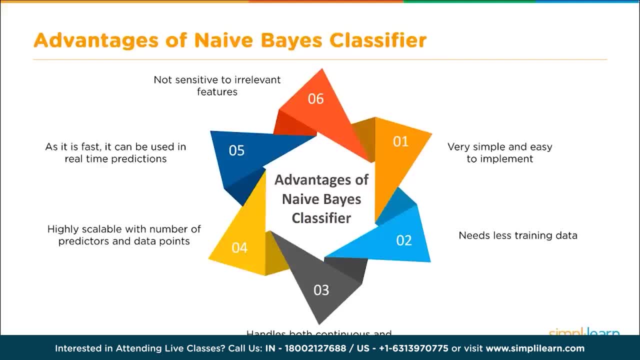 different probabilities in there and you can cover not just three different variables or sets. you can now expand this to even more categories. Number five: it's fast. It can be used in real time predictions. This is so important. This is why it's used in a lot. 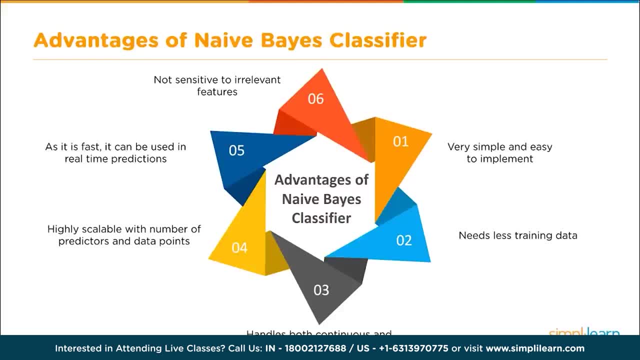 of our predictions on online shopping carts, referrals, spam filters- is because there's no time delay, as it has to go through and figure out a neural network or one of the other mini setups where you're doing classification, And certainly there's a lot of other tools out there in the machine learning. 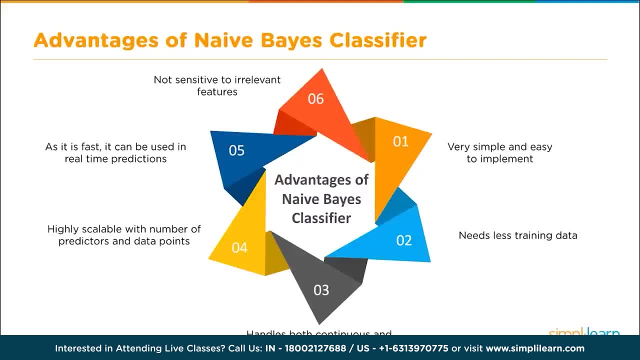 that can handle these, but most of them are not as fast as the Naive Bayes. And then, finally, it's not sensitive to irrelevant features. So it picks up on your different probabilities and if you're short on data on one probability, you can kind of 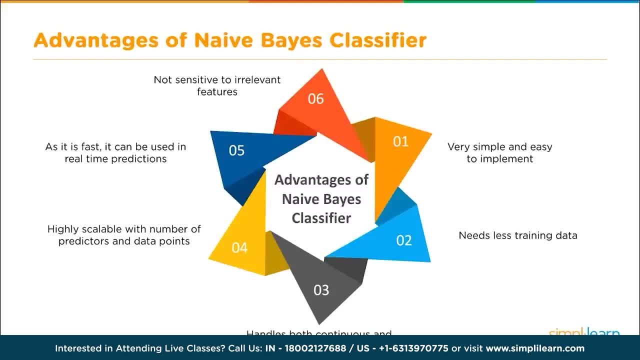 automatically adjust for that. Those formulas are very automatic and so you can still get a very solid predictability, even if you're missing data or you have overlapping data for two completely different areas. We see that a lot in doing census and studying of people and habits. 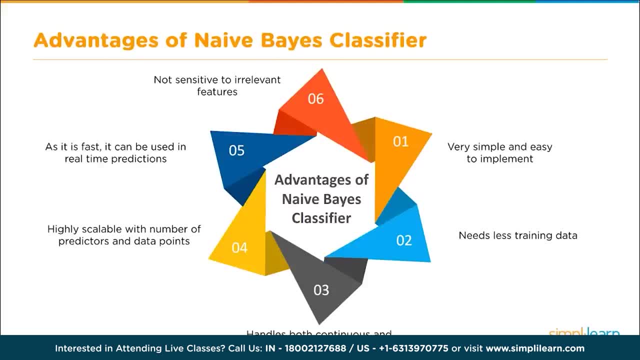 Where they might have one study that covers one aspect, another one that overlaps, and because the two overlap, they can then predict the unknowns for the group that they haven't done the second study on, or vice versa. So it's very powerful. 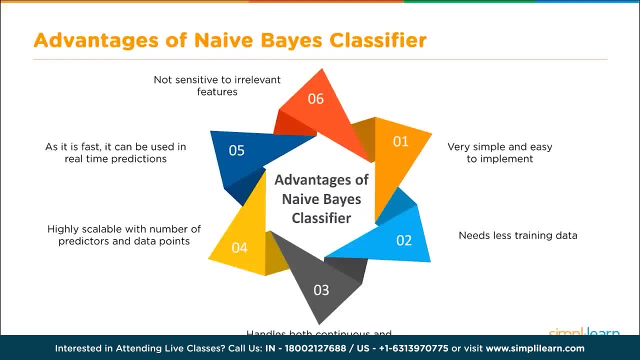 in that it is not sensitive to the irrelevant features and, in fact, you can use it to help predict features that aren't even in there. So now we're down to my favorite part: We're going to roll up our sleeves and do some actual 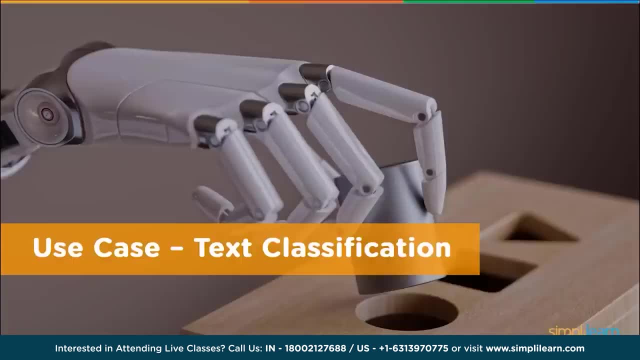 programming. We're going to do the use case text classification Now. I would challenge you to go back and send us a note on the notes below underneath the video and request the data for the shopping cart So you can plug that into Python. 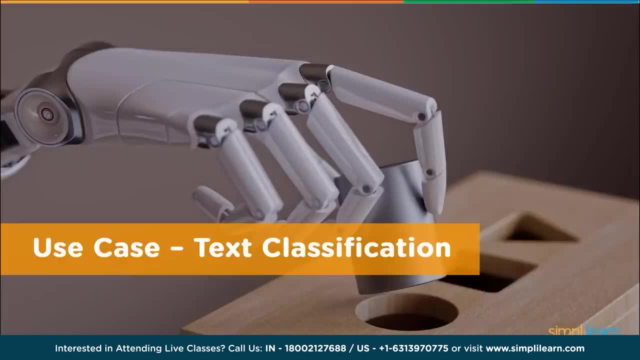 code and do that on your own time so you can walk through it, since we walked through all the information on it. But we're going to do a Python code doing text classification- very popular for doing the naive bays- So we're going to. 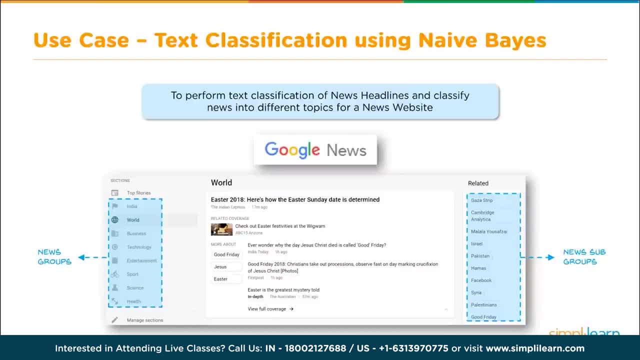 use our new tool to perform a text classification of news headlines and classify news into different topics for a news website. As you can see here we have a nice image of the Google News and then related on the right subgroups. I'm not. 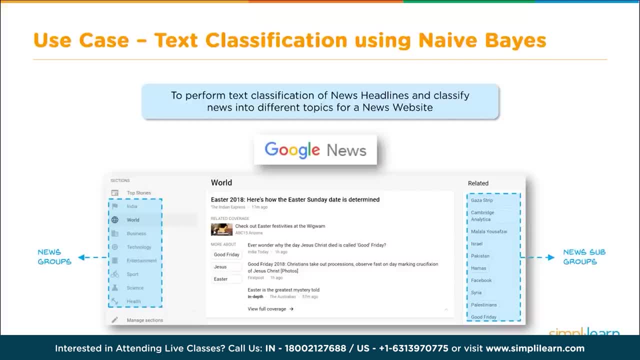 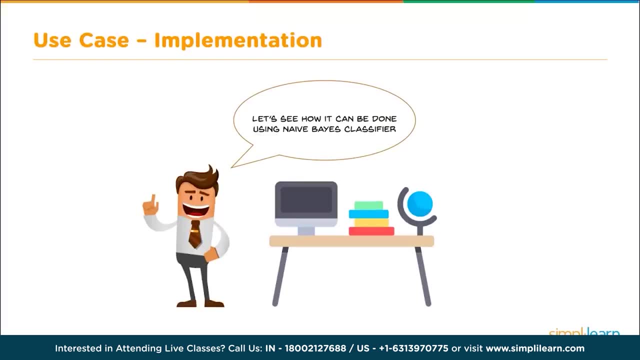 sure where they actually pulled the actual data we're going to use from. It's one of the standard sets, But certainly this can be used on any of our news headlines and classification. So let's see how it can be done using the naive bays classifier. 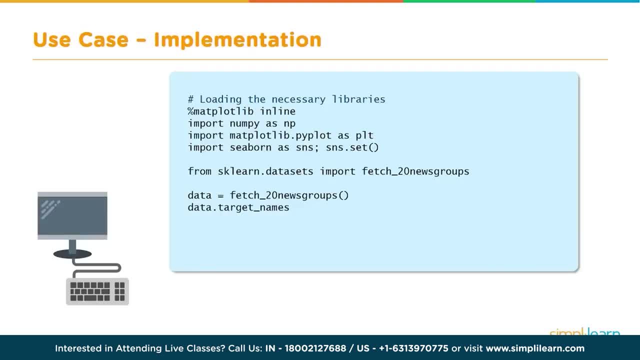 Now we're at my favorite part. We're actually going to write some Python script, Roll up our sleeves And we're going to start by doing our imports. These are very basic imports, including our news group, And we'll take a quick glance. 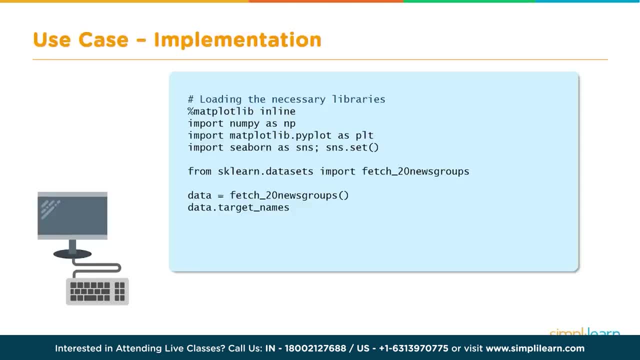 at the target names, Then we're going to go ahead and start training our data set and putting it together. We'll put together a nice graph, because it's always good to have a graph to show what's going on. And once we've trained it and we've shown you a graph of what's going, 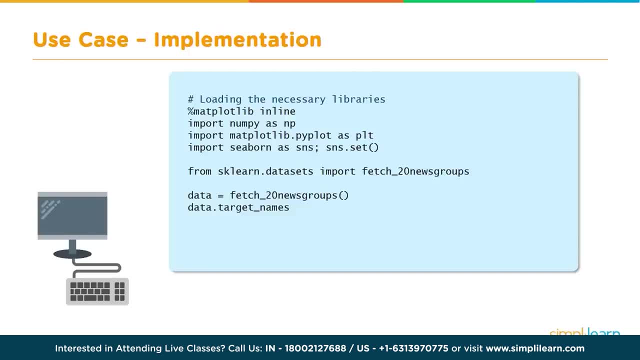 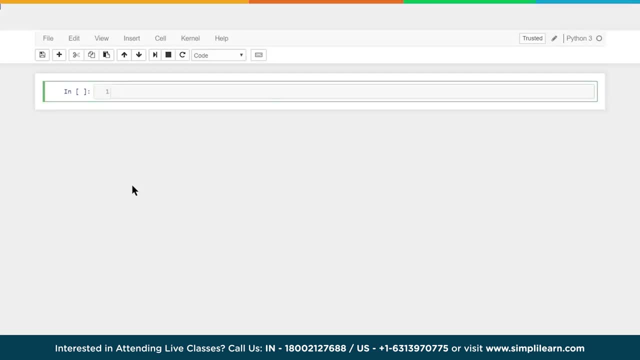 on. then we're going to explore how to use it and see what that looks like. Now I'm going to open up my favorite editor or inline editor for Python. You don't have to use this. You can use whatever your editor that you like, whatever interface. 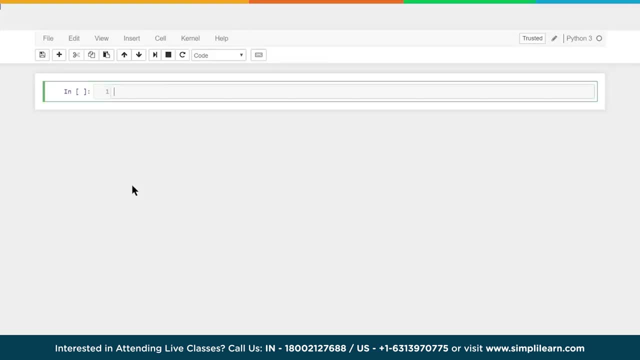 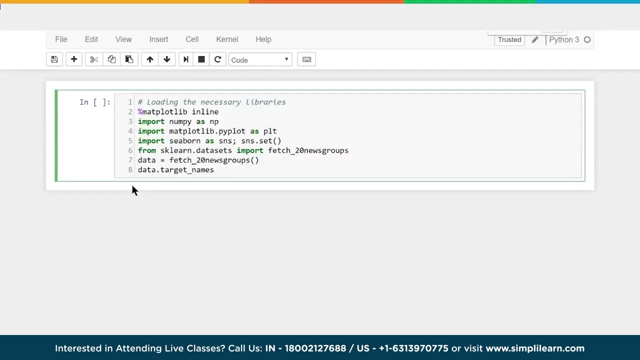 IDE you want. This just happens to be the Anaconda Jupyter notebook And I'm going to paste that first piece of code in here so we can walk through it. Let's make it a little bigger on the screen so you have a nice view of what's going. 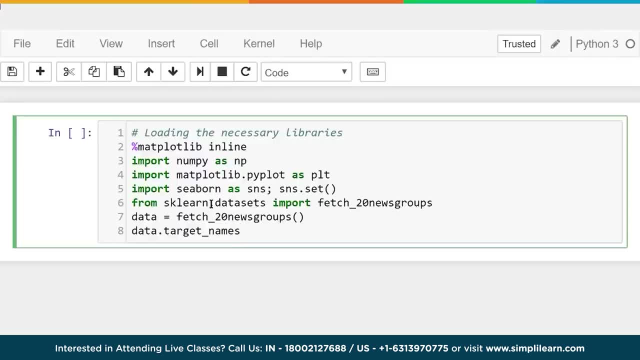 on, And we're using Python 3, in this case 3.5.. So this would work in any of your 3x. If you have it set up correctly, it should also work in a lot of the 2x You just 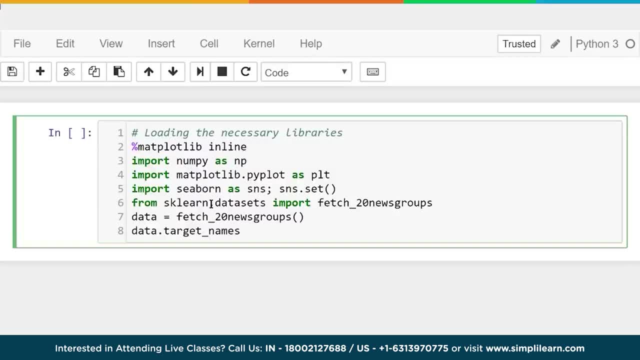 have to make sure all of the versions of the modules match your Python version, And in here you'll notice. the first line is your percentage matplot library inline. Now three of these lines of code are all about plotting the graph. This one lets the 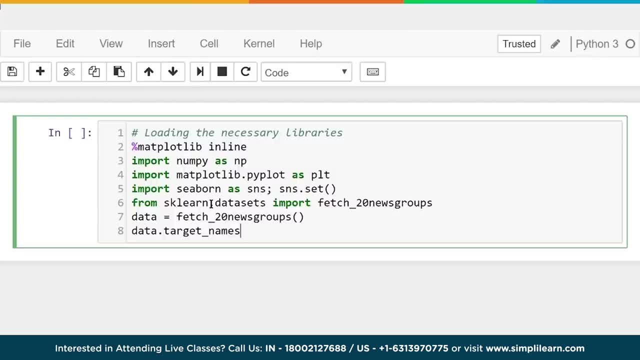 notebook notes- and this is an inline setup- that we want the graphs to show up on this page. Without it, in a notebook like this, which is an explorer interface, it won't show up. Now, a lot of IDEs don't require that. A lot of them like 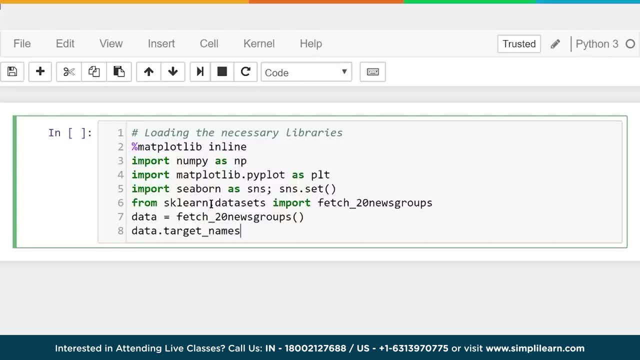 if I'm working on one of my other setups. it just has a popup and the graph pops up on there. So you have that setup also. But for this we want the matplot library inline, And then we're going to import numpy as. 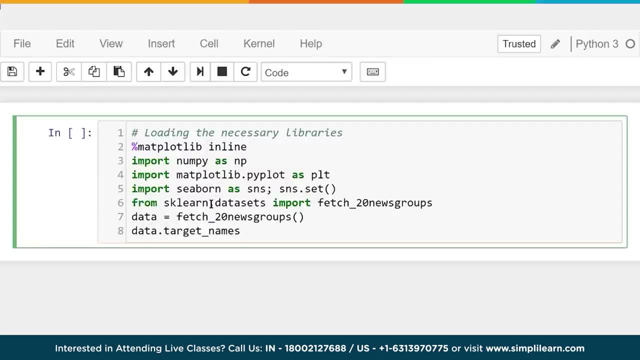 np, that's number Python, which has a lot of different formulas in it that we use for both of our sklearn module And we also use it for any of the upper math functions in Python And it's very common to see that as np, numpy as np. 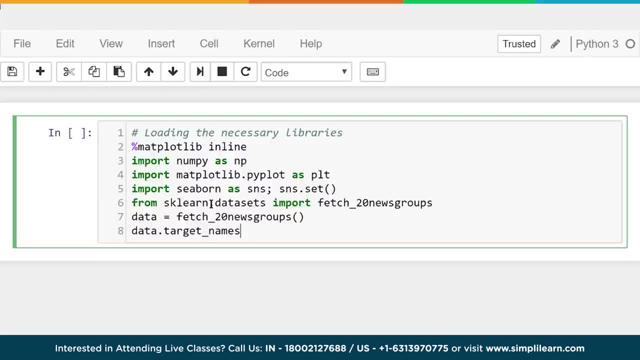 The next two lines are all about our graphing. Remember, I said three of these were about graphing. Well, we need our matplot, librarypyplot, as plt, And you'll see that plt is a very common setup, as is the sns and just like the np. 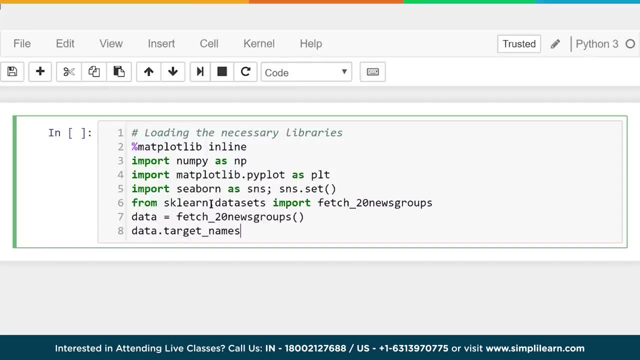 And we're going to import seaborn as sns And we're going to do the snsset Now. seaborn sits on top of pyplot and it just makes a really nice heatmap. It's really good for heatmaps And if you're not familiar with heatmaps, that just means 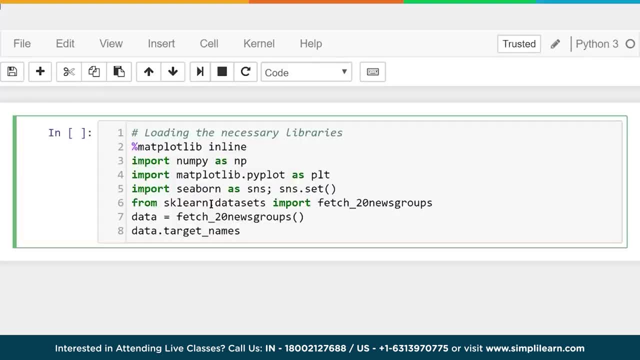 we give it a color scale. The term comes from the brighter red, it is the hotter. it is in some form of data And you can set it to whatever you want And we'll see that later on. So you'll see that, those three lines of code. 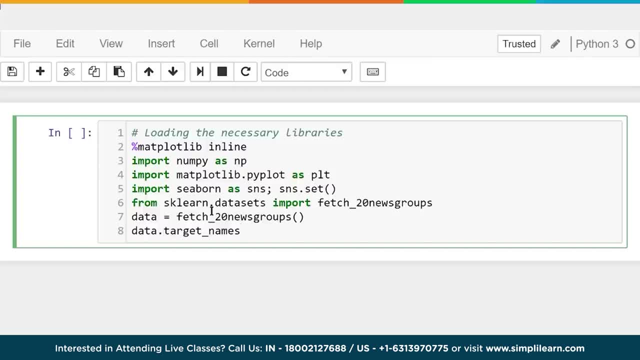 here are just importing the graph function so we can graph it, And as a data scientist you always want to graph your data and have some kind of visual. It's really hard just to shove numbers in front of people and they look at it and it doesn't mean anything. 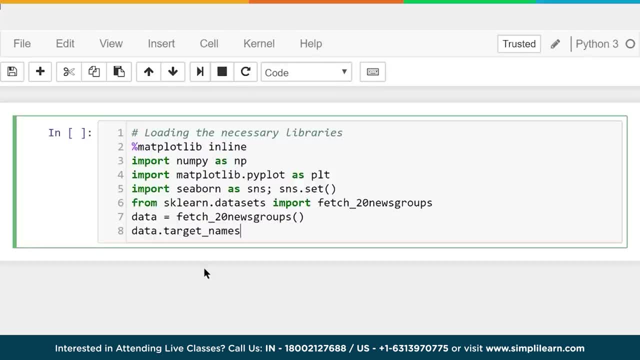 And then from the sklearndatasets we're going to import the fetch20newsgroups- Very common one for analyzing, tokenizing words and setting them up and exploring how the words work. and how do you categorize different things when you're dealing with documents. 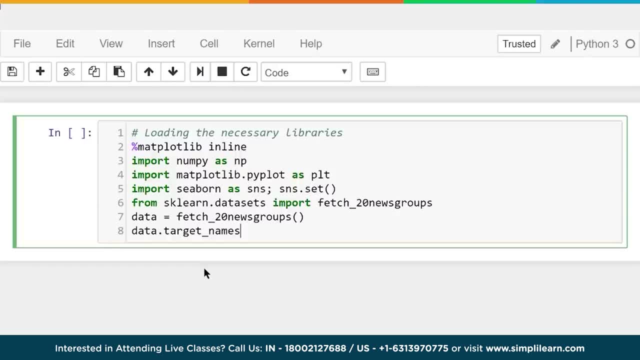 And then we set our data equal to fetch20newsgroups, So our data variable will have the data in it And we're going to go ahead and just print the target names- DatatargetNames- And let's see what that looks like. 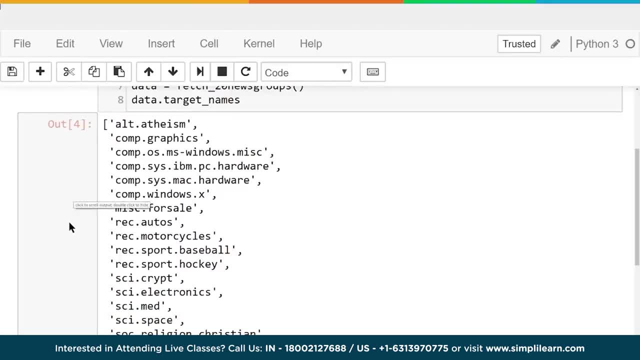 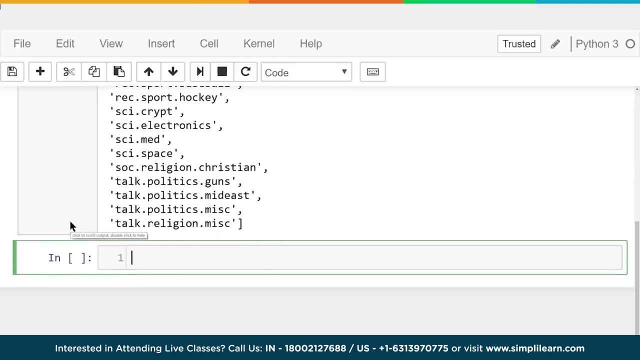 And you'll see, here we have alt atheism, compgraphics, composmswindowsmiscellaneous, and it goes all the way down to talkpoliticsmiscellaneous, talkreligionmiscellaneous. These are the categories they've already assigned to this newsgroup. 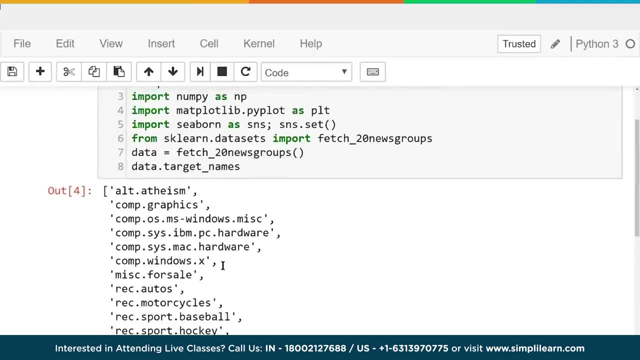 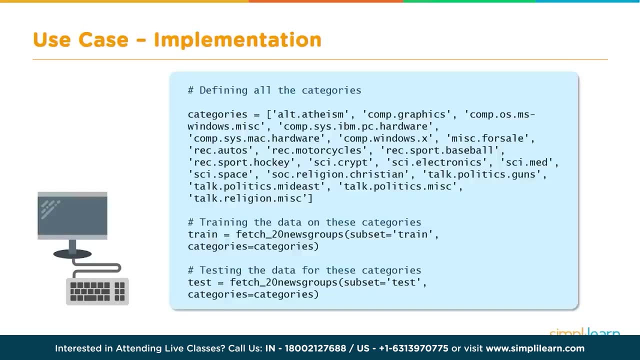 And it's called fetch20 because you'll see, there's- I believe there's- 20 different topics in here, or 20 different categories as we scroll down. Now we've gone through the 20 different categories and we're going to go ahead and start defining all the 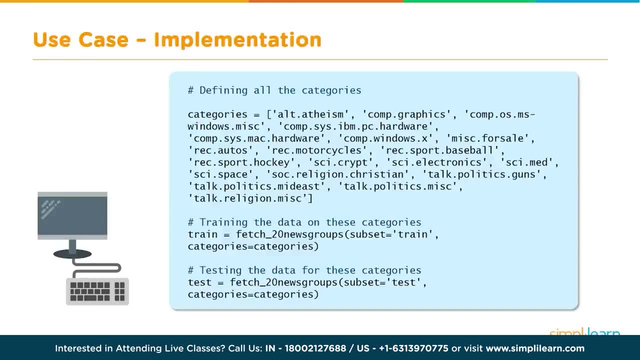 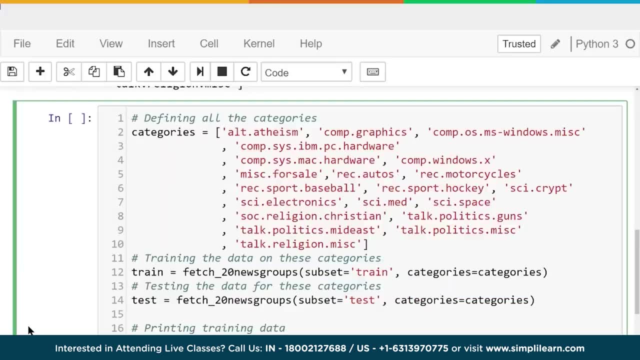 categories and set up our data. So we're actually going to go ahead and get the data all set up and take a look at our data And let's move this over to our Jupyter Notebook And let's see what this code does. 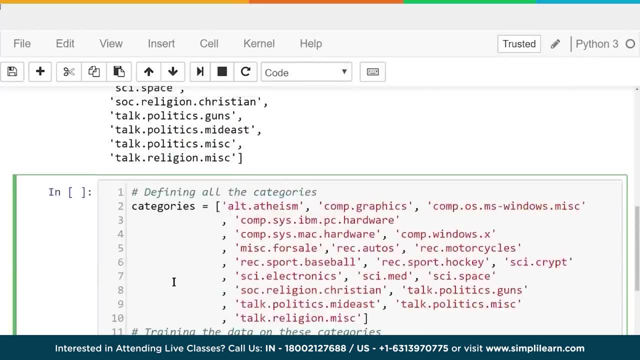 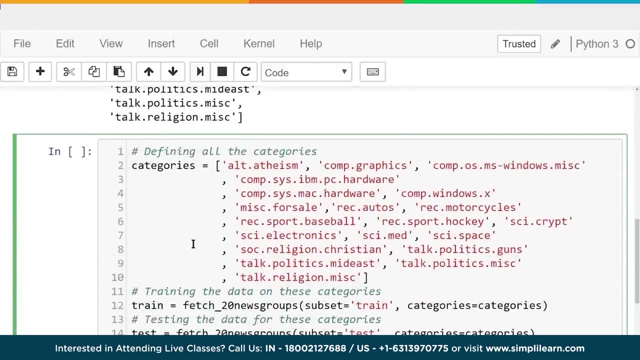 First we're going to set our categories. Now, if you noticed up here, I could have just as easily set this equal to datatargetNames, because it's the same thing. But we want to kind of spell it out for you so you can see the different categories. 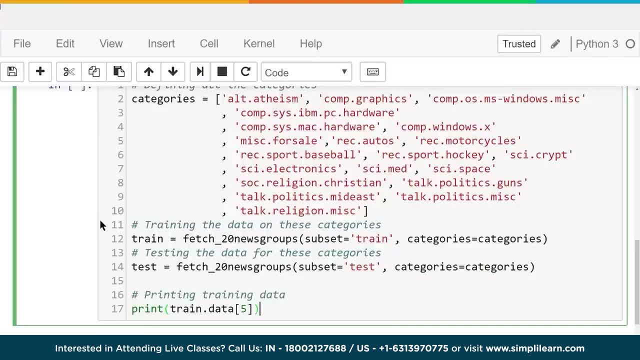 It kind of makes it more visual so you can see what your data is looking like in the background. Once we've created the categories, we're going to open up a train set, So this training set of data is going to go into fetch20newsgroups. 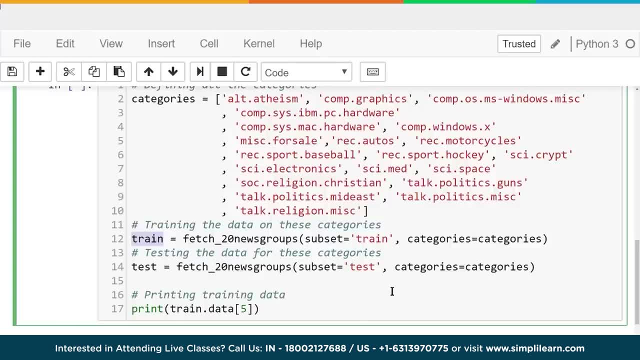 and it's a subset in there called train and categories equals categories. So we're pulling out those categories that match And then if you have a train set, you should also have the testing set. We have test equals fetch20newsgroups subset equals test and categories. 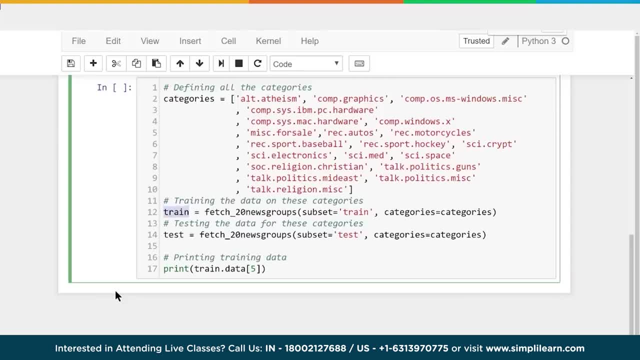 equals categories. Let's go down one side so it all fits on my screen. There we go, And just so we can really see what's going on. let's see what happens when we print out one part of that data. So it creates train and under train. 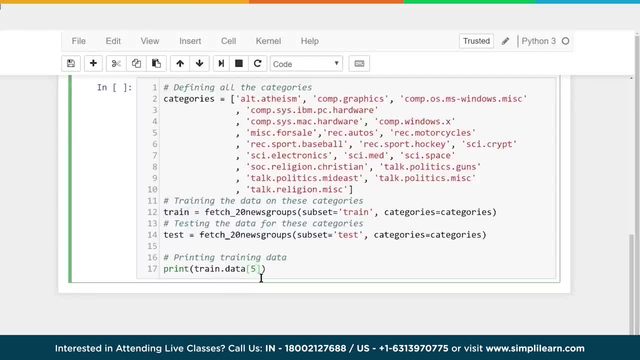 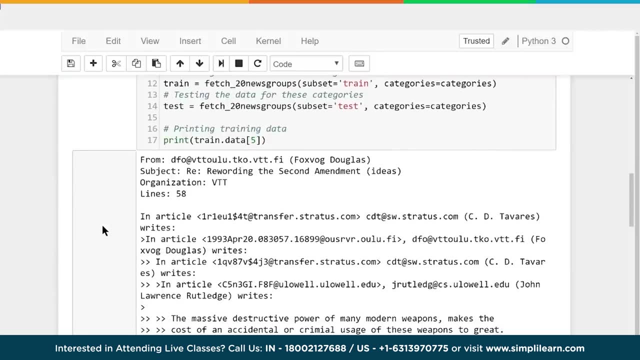 it creates traindata and we're just going to look at data piece number 5. And let's go ahead and run that and see what that looks like. And you can see, when I print traindata number 5 under train, it prints out one of the articles. This is article. 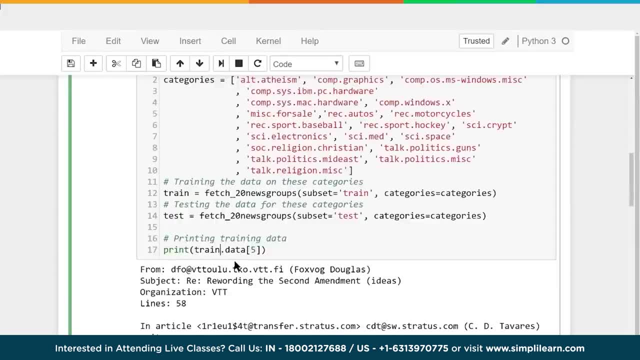 number 5.. You can go through and read it on there And we can also go in here and change this to test, which should look identical because it's splitting the data up into different groups. Train and test And we'll see test number. 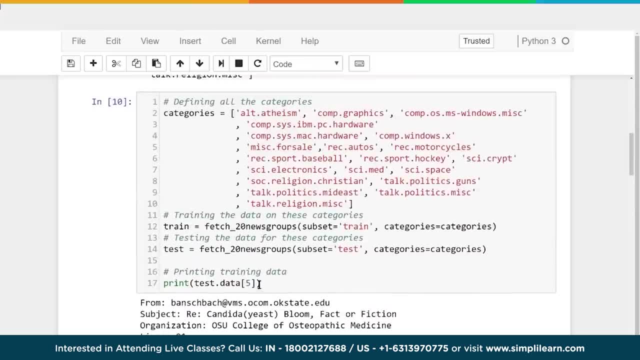 5 is a different article but it's another article in here And maybe you're curious and you want to see just how many articles are in here. We could do length of train dot data and if we run that you'll see that the training data has. 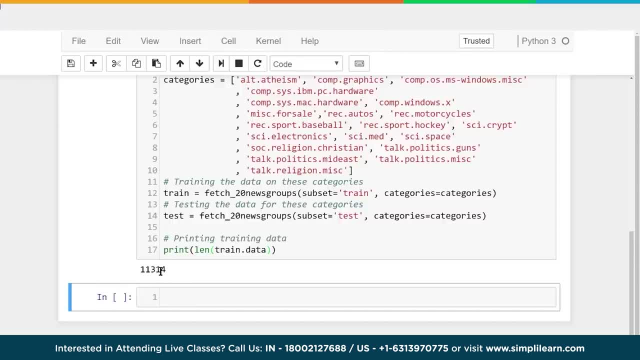 11,314 articles, So we're not going to go through all those articles. That's a lot of articles, But we can look at one of them just so you can see what kind of information is coming out of it and what we're looking at. And we'll just look at. 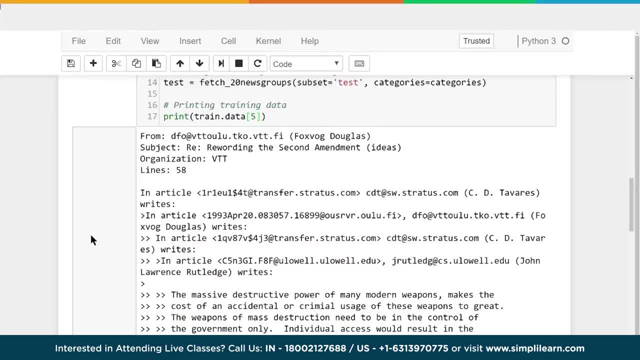 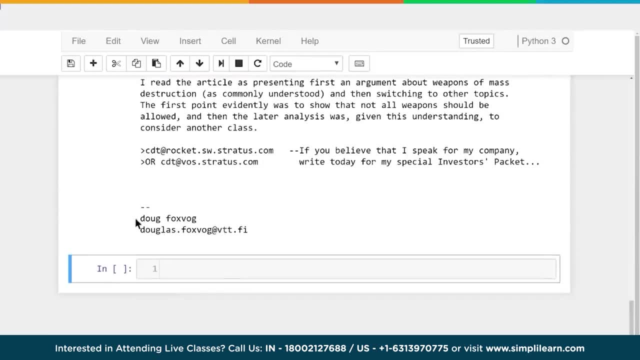 number 5 for today And here we have it, rewording the second amendment. IDs VTT, line 58, lines 58 in article, etc. And you can scroll all the way down and see all the different parts to there. Now we've looked at it and that's pretty complicated when you 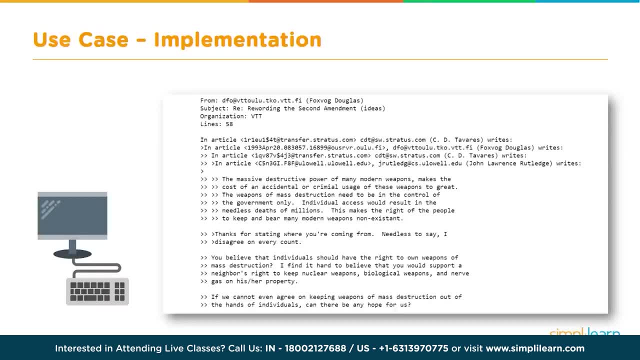 look at one of these articles to try to figure out. how do you weight this? If you look down here, we have different words and maybe the word from- Well from- is probably in all the articles, so it's not going to have a lot of meaning as far as trying. 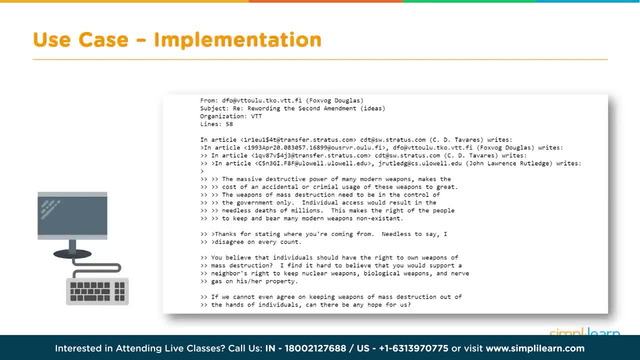 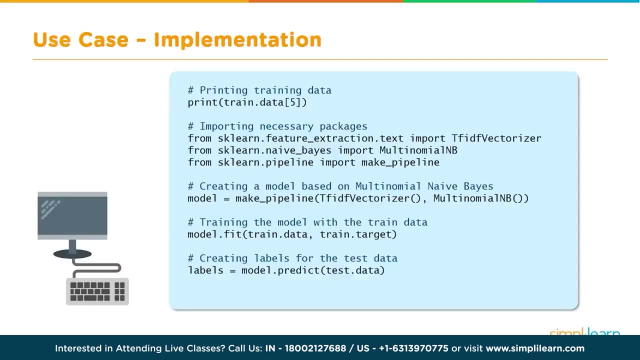 to figure out whether this article fits one of the categories or not. So trying to figure out which category it fits in based on these words is where the challenge comes in. Now that we've viewed our data, we're going to dive in and do the actual predictions. 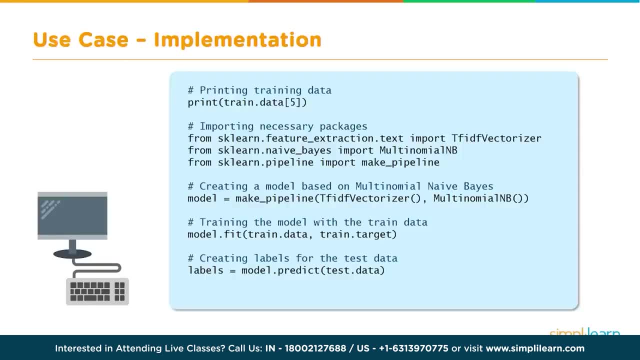 This is the actual naive base And we're going to throw another model at you or another module at you here in just a second. We can't go into too much detail, but it deals specifically working with words and text and what they call tokenizing those words. 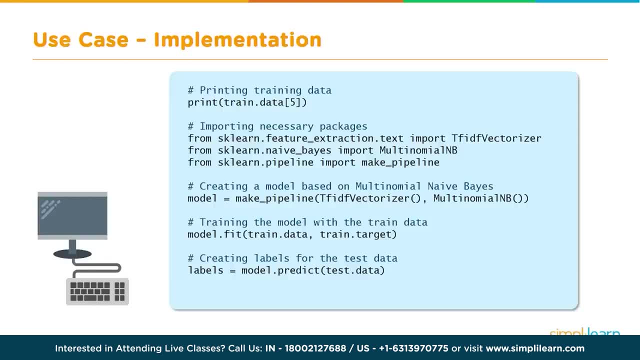 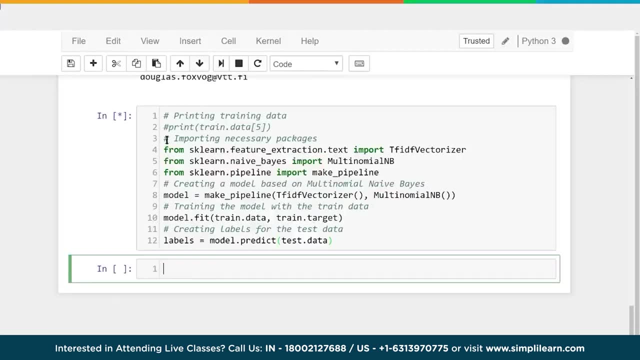 So let's take this code and let's skip on over to our Jupyter notebook and walk through it, And here we are in our Jupyter notebook. Let's paste that in there and I can run this code right off the bat. It's not actually going to display anything yet. 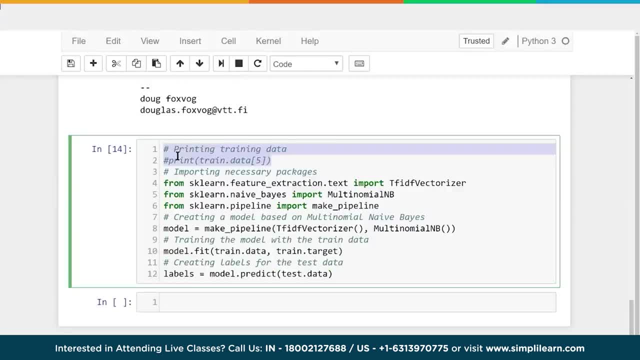 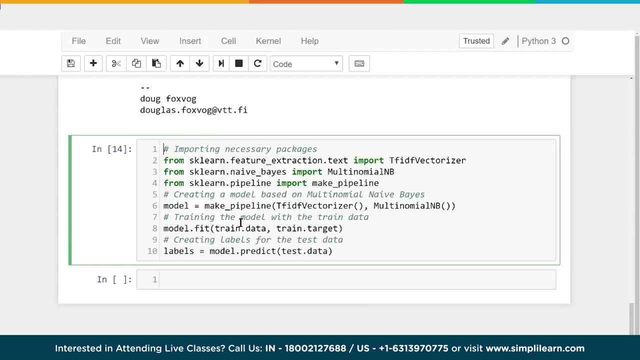 But it has a lot going on in here. So at the top we have the print module from the earlier one. I didn't know why that was in there. So we're going to start by importing our necessary packages And from the sklearn features, extraction dot text. 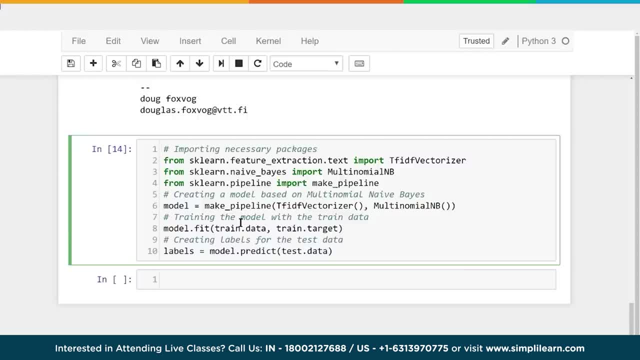 we're going to import tf idf vectorizer. I told you we were going to throw a module at you. We can't go too much into the math behind this or how it works. You can look it up, The notation for the math. 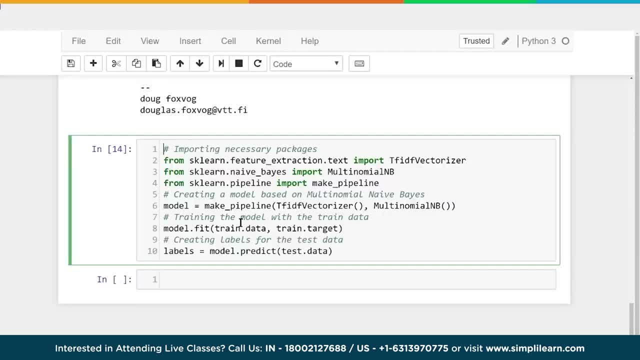 is usually tf, dot, idf, And that's just a way of weighing the words, And it weighs the words based on how many times they're used in a document, How many times or how many documents they're used in, And it's a well used formula. It's been around for a 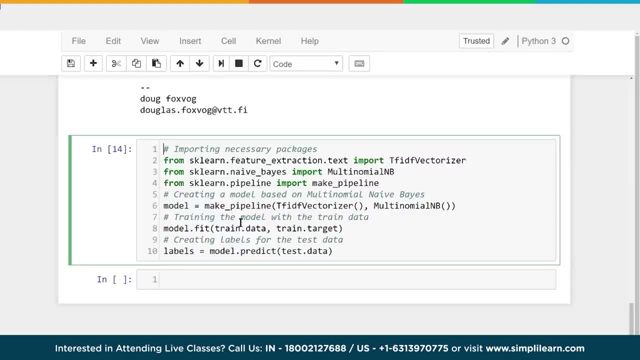 while It's a little confusing to put this in here, But let's let it know that it just goes in there and weights the different words in the document for us. That way we don't have to wait And if you put a weight on it, If you remember. 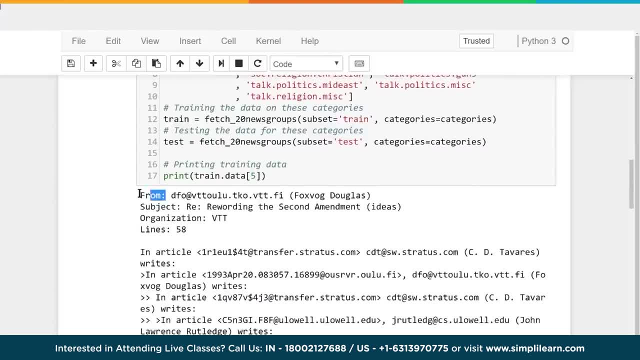 I was talking about that up here earlier. If these are all emails, they probably all have the word from in them. From probably has a very low weight. It has very little value telling you what this document's about. Same with words like in in article. 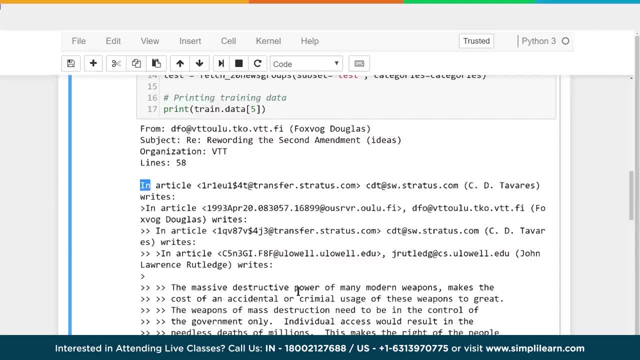 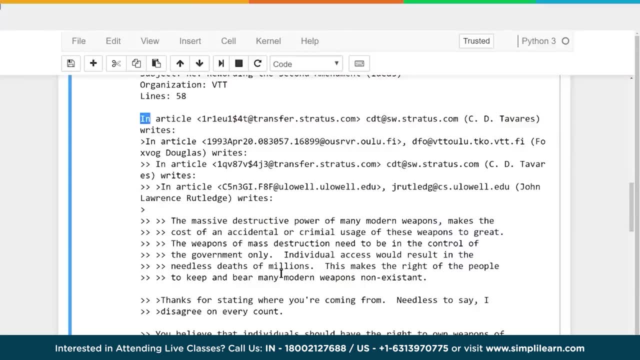 in articles in cost of un, maybe, cost, might, or where words like criminal weapons, destruction. These might have a heavier weight because they describe a little bit more what the article's doing. Well, how do you figure out all those weights? 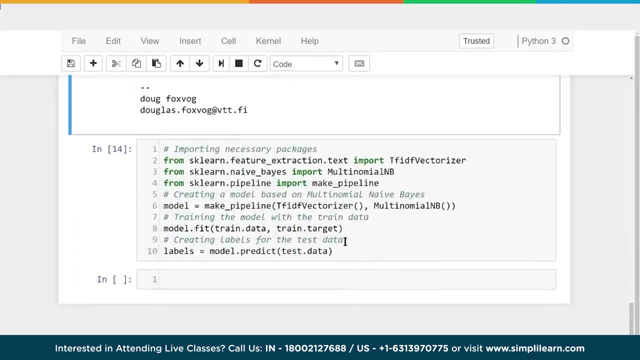 in the different articles. That's what this module does, That's what the tf idf vectorizer is going to do for us, And then we're going to import our sklearnnaivebase and that's our multinomial in b: Multinomial. 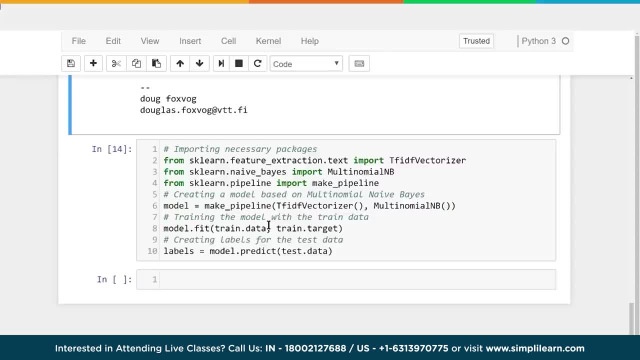 naive base. Pretty easy to understand that where that comes from. And then, finally, we have the sklearn pipeline, import make pipeline. Now, the make pipeline is just a cool piece of code because we're going to take the information we get from the tf idf vectorizer. 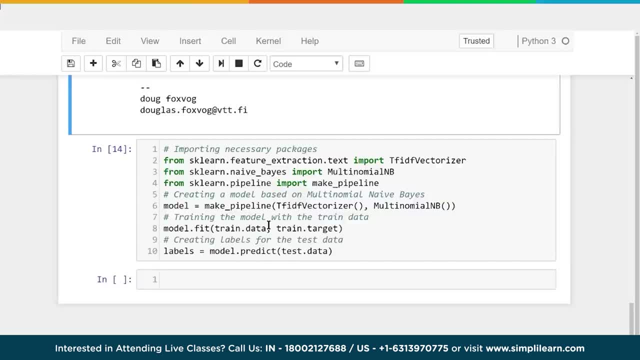 and we're going to pump that into the multinomial in b. So a pipeline is just a way of organizing how things flow. It's used commonly. you probably already guessed what it is if you've done any businesses. they talk about the cells pipeline. if you're on. 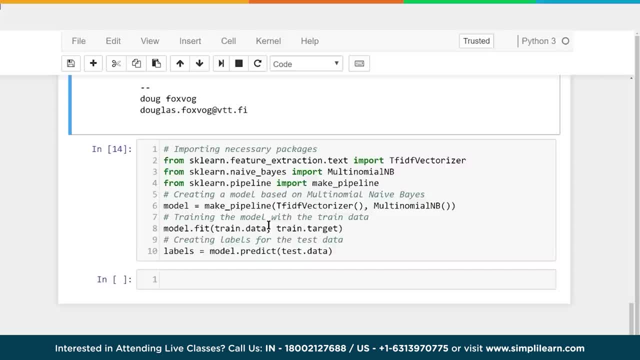 a work crew or a project manager. you have your pipeline of information that's going through or your projects and what has to be done, in what order. That's all this pipeline is. We're going to take the tf id vectorizer and then we're going to push. 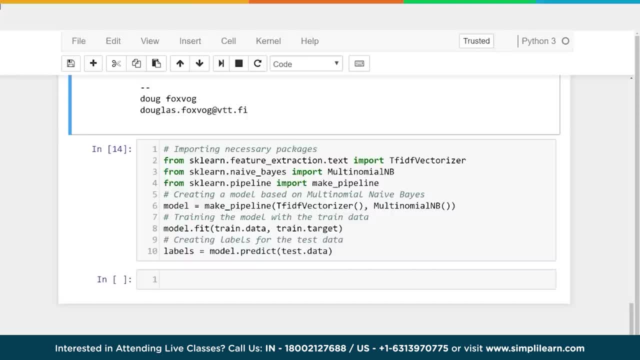 that into the multinomial in b. Now we've designated that as the variable model. We have our pipeline model and we're going to take that model. and this is just so elegant. this is done in just a couple lines of code: modelfit, and we're going to. 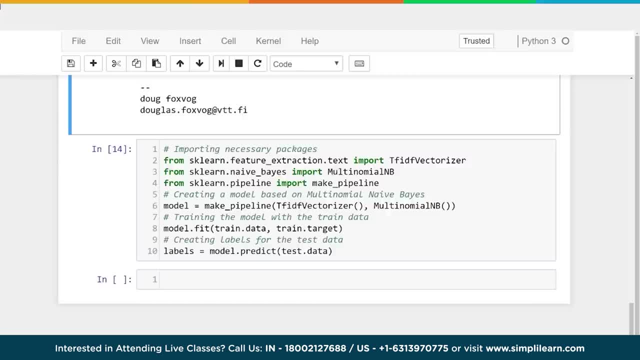 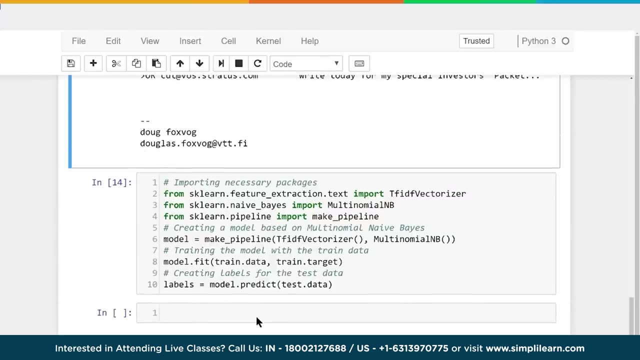 fit the data and first the train data and then the train target. Now the train data has the different articles in it- you can see the one we were just looking at- and the traintarget is what category they already categorized that particular article as And what's happening here. 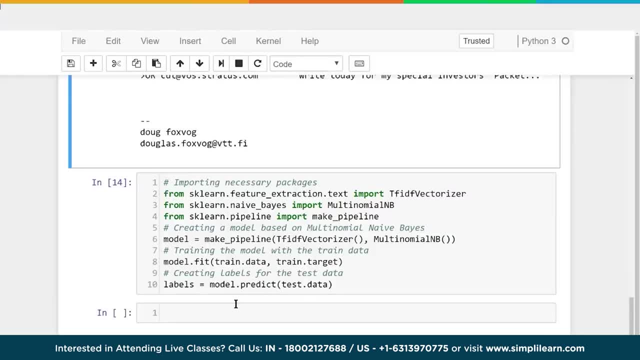 is the train data is going into the tf id vectorizer, so when you have one of these articles that goes in there, it weights all the words in there. So there's the thousands of words with different weights on them. I remember once running a model on this and I 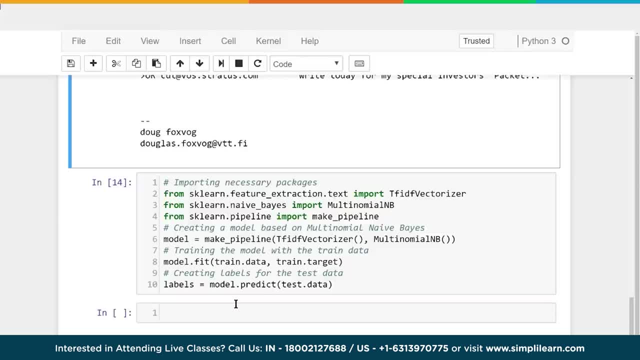 literally had 2.4 million tokens go into this. So when you're dealing with large document bases, you can have a huge number of different words. It then takes those words, gives them a weight and then, based on that weight, based on the words and the weights it then puts, 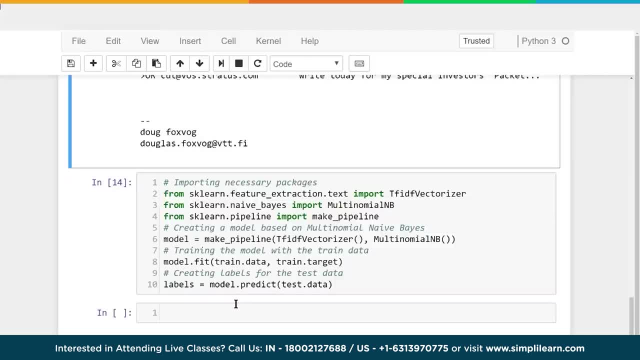 that into the multinomial in b, And once we go into our naive base we want to put the train target in there. So the train data that's been mapped to the tf id vectorizer is now going through the multinomial in b, and then we're telling it: well, these are the answers. 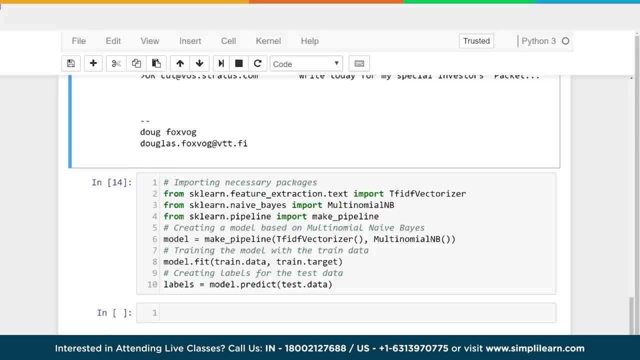 These are the answers to the different documents. So this document that has all these words, with these different weights from the first part, is going to be, whatever category it comes out of- Maybe it's the talk show or the article on religion- miscellaneous, Once we fit that. 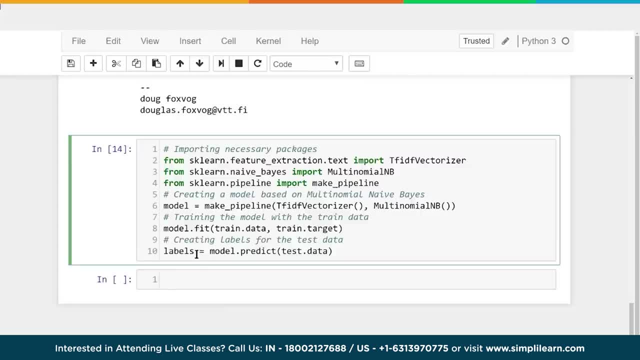 model. we can then take labels and we're going to set that equal to modelpredict. Most of the sklearn use the term predict to let us know that we've now trained the model and now we want to get some answers And we're going to put our 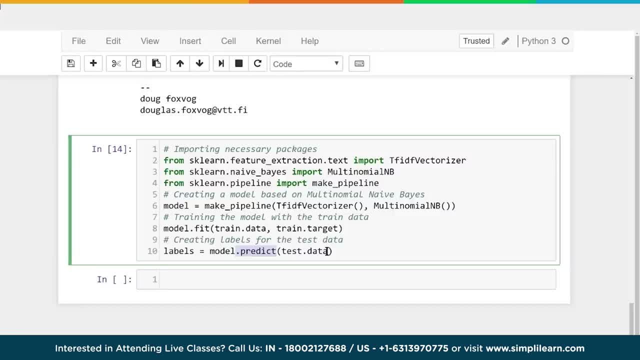 test data in there, because our test data is the stuff we held off to the side, We didn't train it on there and we don't know what's going to come up out of it, and we just want to find out how good our labels are. Do they match what they should be? 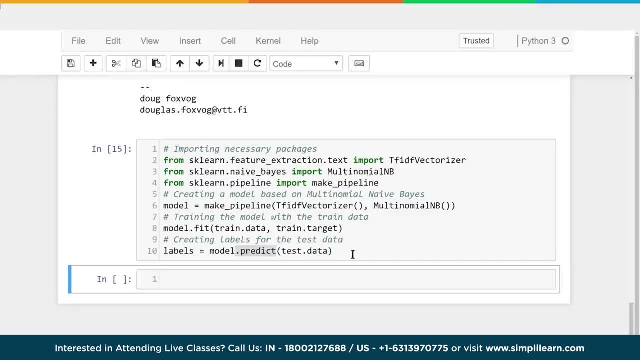 Now, I've already run this through. There's no actual output to it to show. This is just setting it all up. This is just training our model, creating the labels so we can see how good it is, and then we move on to the next step, to find out what happens. 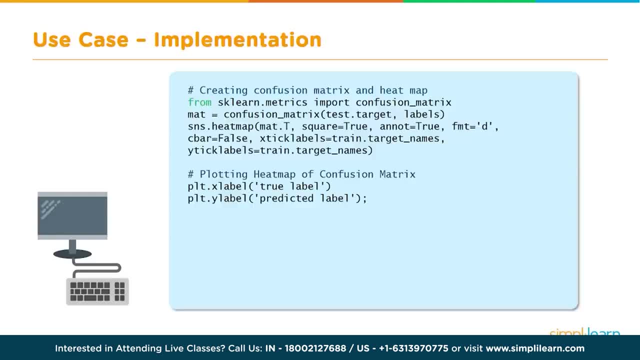 To do this, we're going to go ahead and create a confusion matrix and a heat map. So the confusion matrix, which is confusing just by its very name, is basically going to ask: how confused is our answer? Did it get it correct or did it? 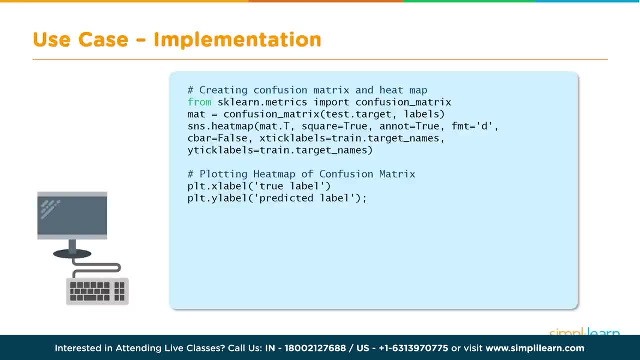 miss some things in there or have some missed labels, And then we're going to put that on a heat map so we'll have some nice colors to look at to see how that plots out. Let's go ahead and take this code and see how. 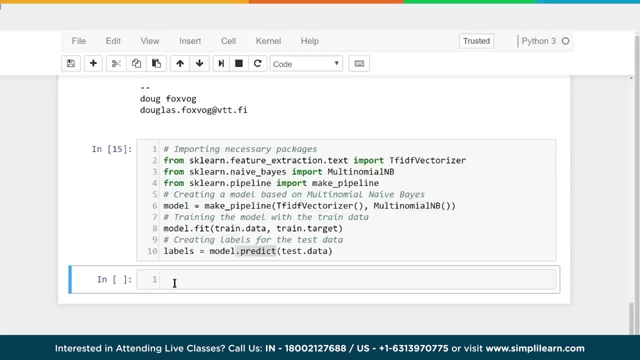 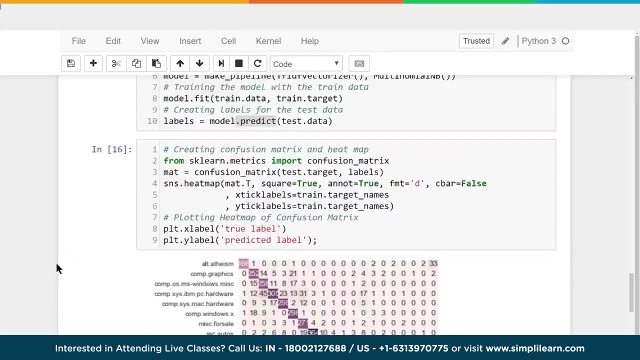 that. take a walk through it and see what that looks like. So back to our Jupyter notebook. I'm going to put the code in there and let's go ahead and run that code. Take it just a moment and remember we had the inline. that way my graph shows up. 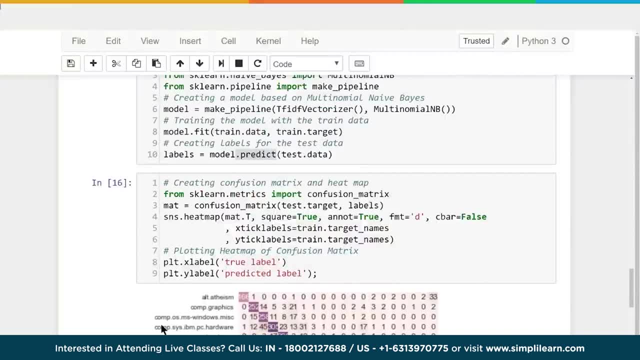 on the inline here And let's walk through the code and then we'll look at this and see what that means. So let me make it a little bit bigger. There we go. No reason not to use the whole screen Too big. 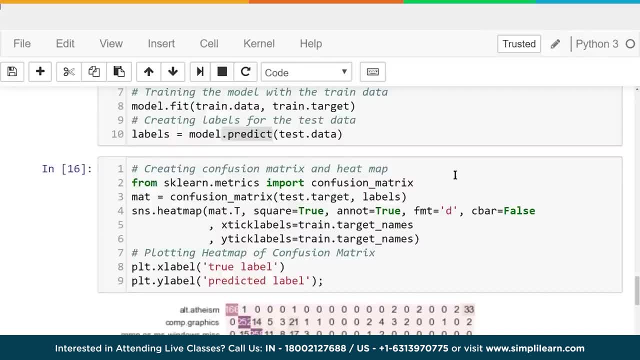 So we have here from sklearnmetrics import confusion matrix And that's just going to generate a set of data that says the prediction was as such- the actual truth was either agreed with it or it was something different- And it's going to add up those numbers so we can take a look and just see how. 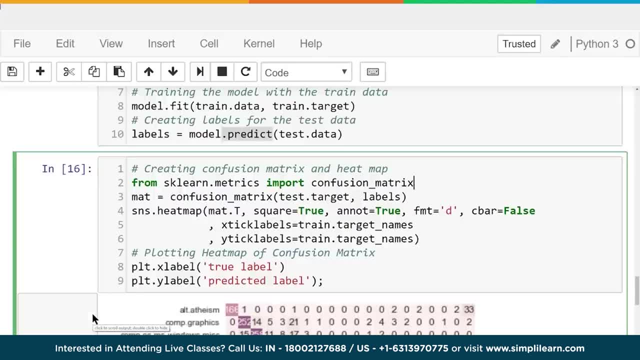 well, it worked And we're going to set a variable mat equal to confusion matrix. We have our test target, our test data. that was not part of the training- Very important in data science. we always keep our test data separate, Otherwise it's. 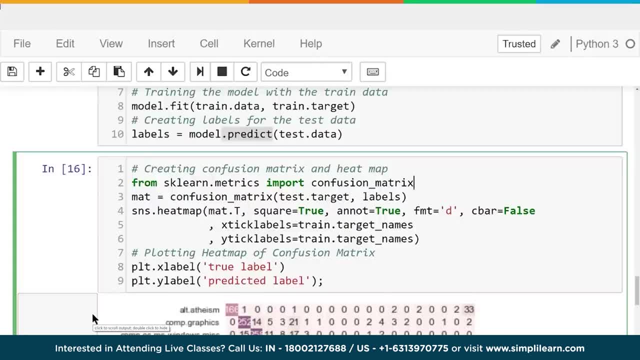 not a valid model if we can't properly test it with new data. And this is the labels we created from that test data. These are the ones that we predict it's going to be. So we go in and we create our snheatmap. The 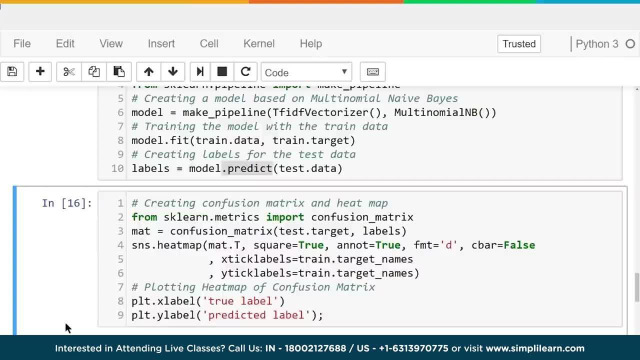 sns is our seaborn, which sits on top of the piplot. So we create a sns heatmap. We take our confusion matrix and it's going to be matt, and then we have other variables that go into the sns heatmap. We're not going to go into detail. 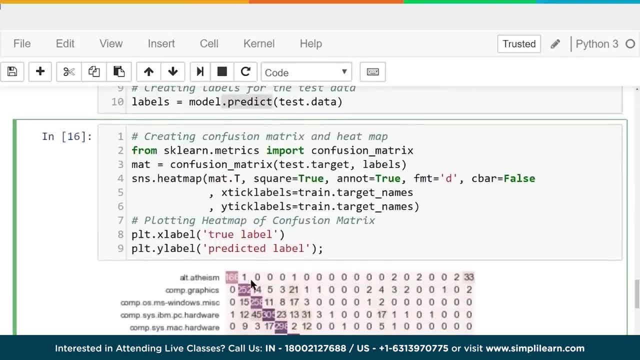 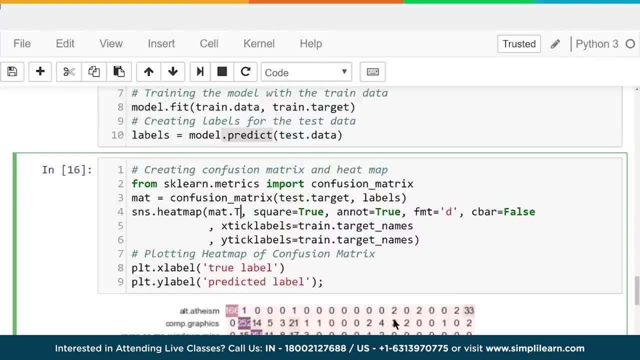 what all the variables mean. The annotation equals true. That's what tells it to put the numbers here. So you have the 166,, the 1, the 0001,. format d and cbar equals false. have to do with the format. 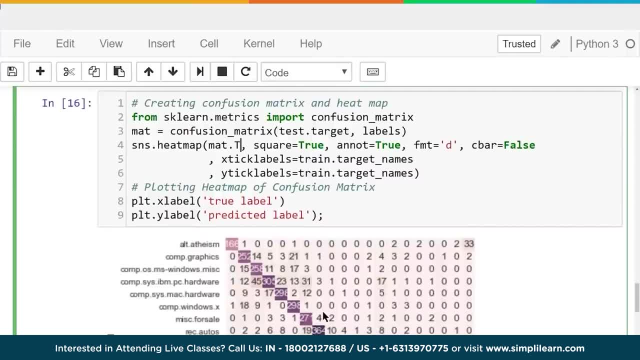 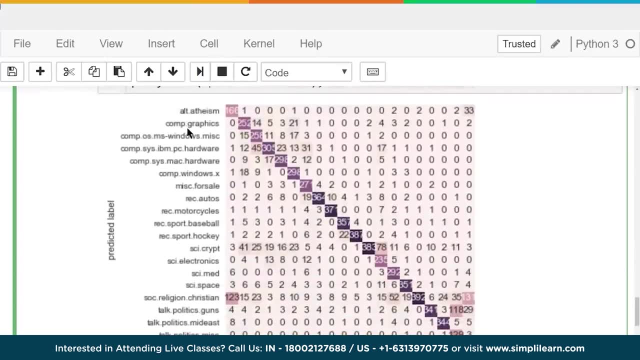 If you take those out, you'll see that some things disappear. And then the xtick labels and the ytick labels. those are our target names And you can see right here. that's the alt atheism. comp graphics, comp os, ms, windowsmiscellaneous. 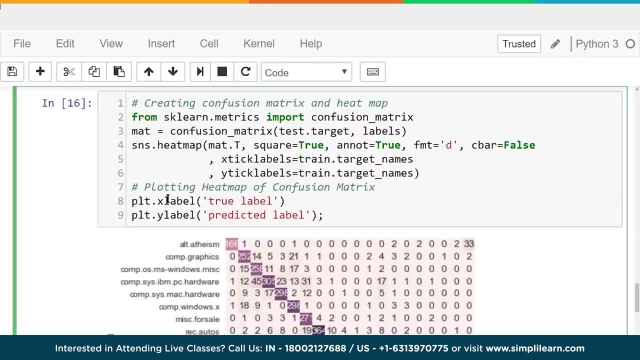 And then, finally, we have our pltxlabel. Remember the sns or the seaborn sits on top of our matplot library, our plt. And so we want to just tell it: xlabel equals, true is true, The labels are true. and then the ylabel is prediction label. 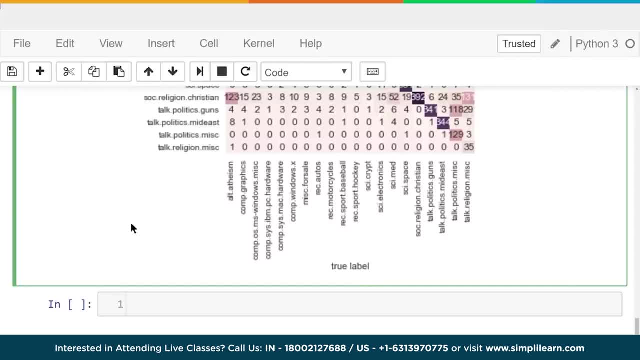 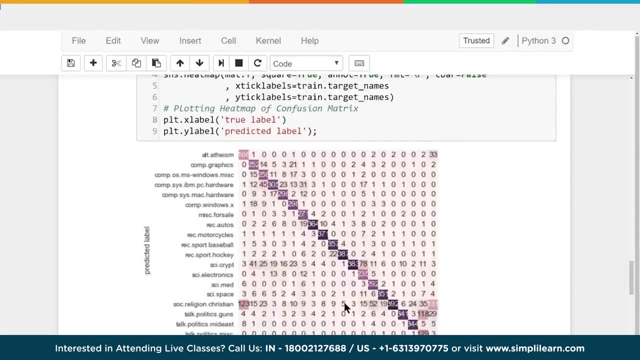 So when we say a true, this is what it actually is and the prediction is what we predicted. And let's look at this graph, because that's probably a little confusing the way we rattled through it, And what I'm going to do is I'm going to go ahead. 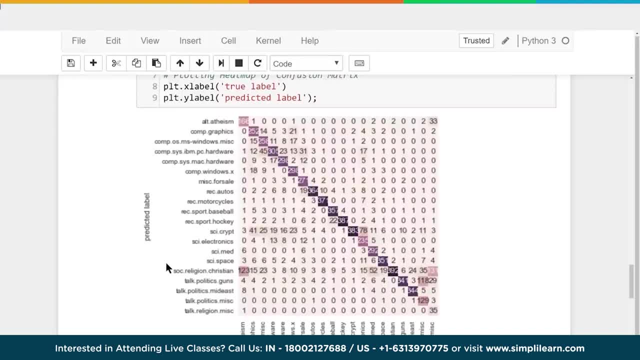 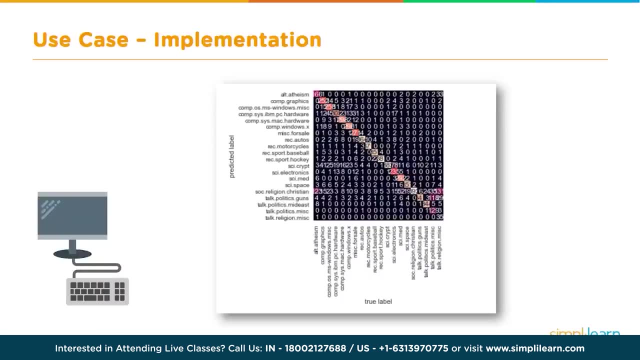 and flip back to the slides, because they have a black background they put in there. that helps it shine a little bit better so you can see the graph a little bit easier. So in reading this graph, what we want to look at is how the color scheme has come out, And you'll see. 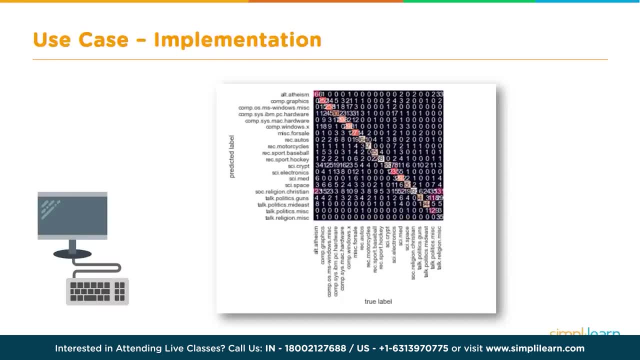 a line right down the middle, diagonally from upper left to bottom right. What that is is, if you look at the labels, we have our predicted label on the left and our true label on the right. Those are the numbers where the prediction and the true come together, And this is what we want to. 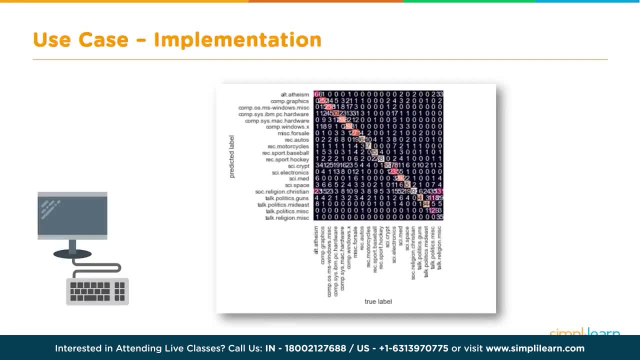 see is we want to see those lit up. That's what that heat map does, As you can see that it did a good job of finding those data And you'll notice that there's a couple of red spots on there where it missed. It's a little confused. 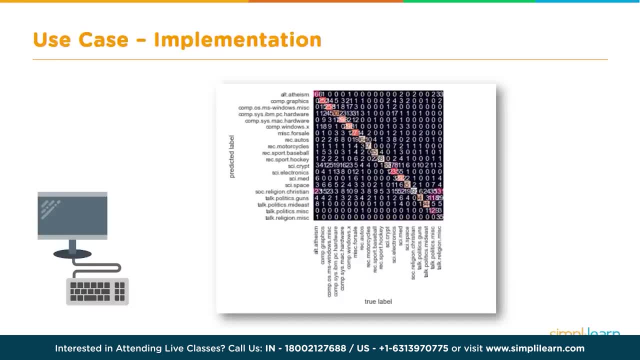 when we talk about talk religion- miscellaneous versus talk politics, miscellaneous Social religion, Christian versus alt atheism. It mislabeled some of those And those are very similar topics so you could understand why it might mislabel them, But overall it did a pretty good job. 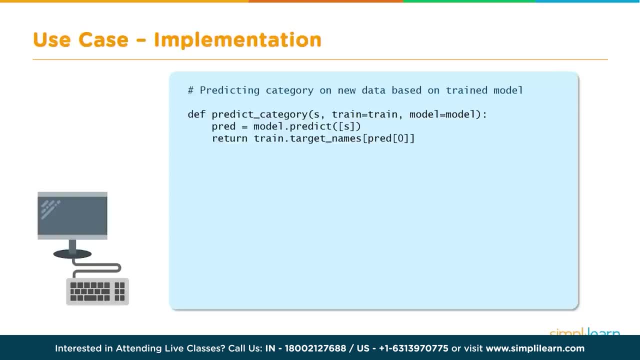 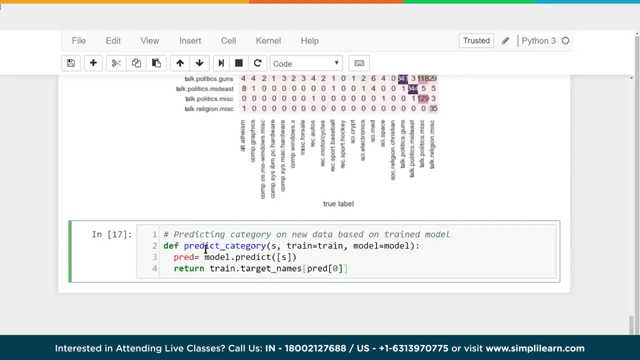 If we're going to create these models, we want to go ahead and be able to use them. So let's see what that looks like. To do this, let's go ahead and create a definition, a function to run, And we're going to call this function. let me just expand. 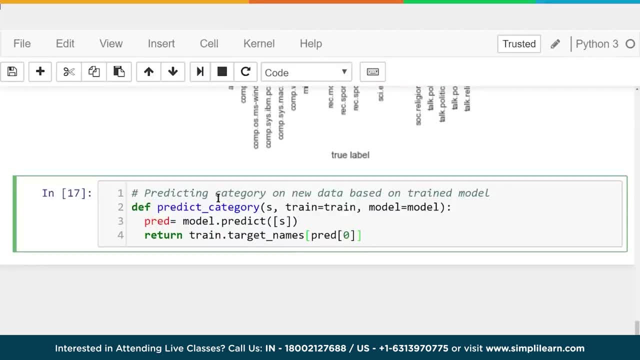 it just a notch here. There we go. I like mine in big letters. Predict categories. We want to predict the category. We're going to send it s a string And then we're sending it. train equals train. We have our training model And then we had our pipeline. 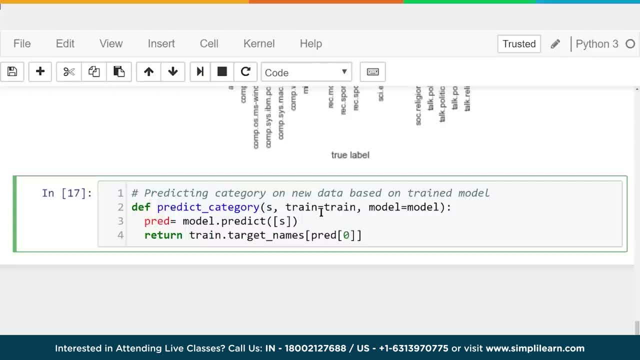 Model equals model. This way, we don't have to resend these variables each time. The definition knows that because I said train equals train and I put the equal for model And then we're going to set the prediction equal to the model. dot predict s. So it's going to send whatever. 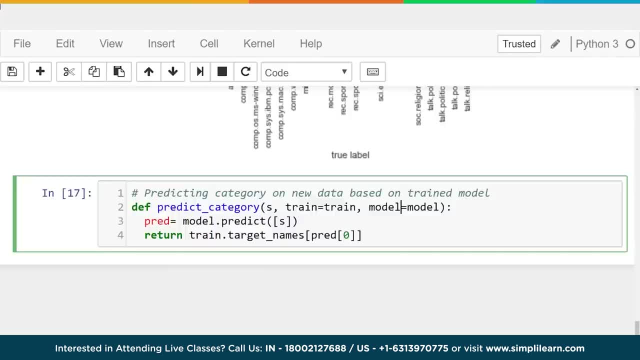 string we send to it. It's going to push that string through the pipeline, the model pipeline It's going to go through and tokenize it and put it through the tf, idf. Convert that into numbers and weights for all the different documents and words. 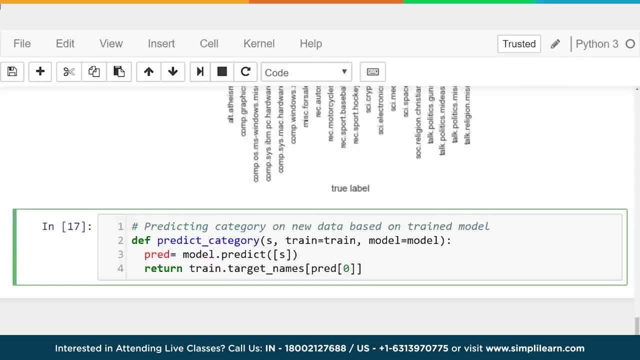 And then it'll put that through our naive bays And from it we'll go ahead and get our prediction. We're going to predict what value it is And so we're going to return train dot target names, predict of zero, And remember that the 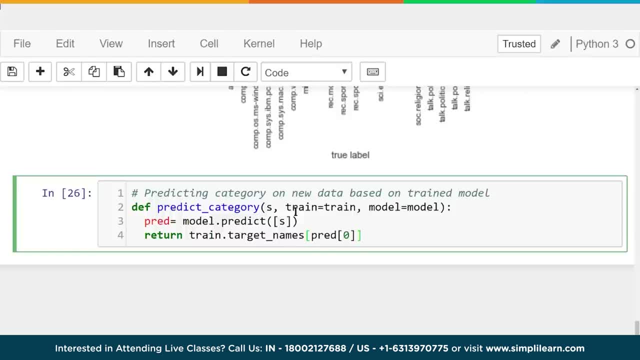 train dot target names. that's just categories. I could have just as easily put categories in there. dot predict of zero. So we're taking the prediction, which is a number, and we're converting it to an actual category. We're converting it from. 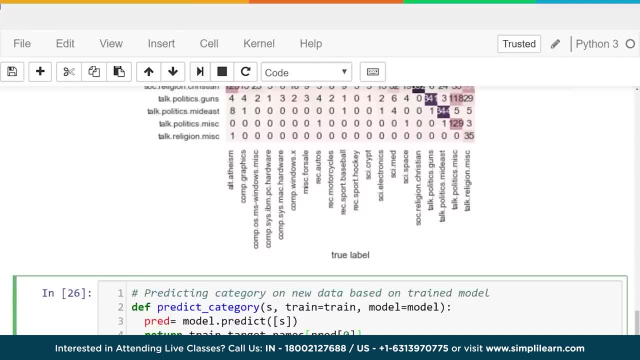 I don't know what the actual numbers are, but let's say zero equals alt atheism, So we're going to convert that zero to the word, Or one. maybe it equals comp graphics, So we're going to convert number one into comp graphics. That's all that is. 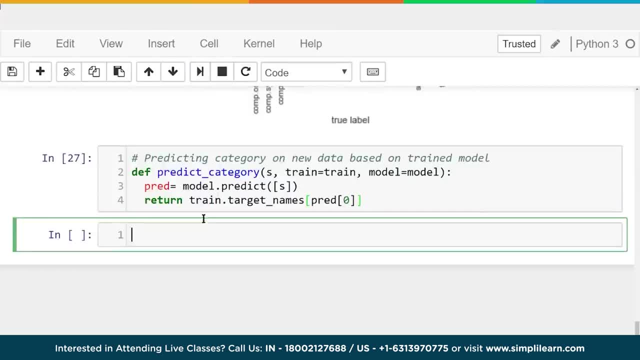 And then we got to go ahead and we need to go ahead and run this. So I load that up And then, once I run that, we can start doing some predictions. So let's go ahead and type in predict category And let's just do. 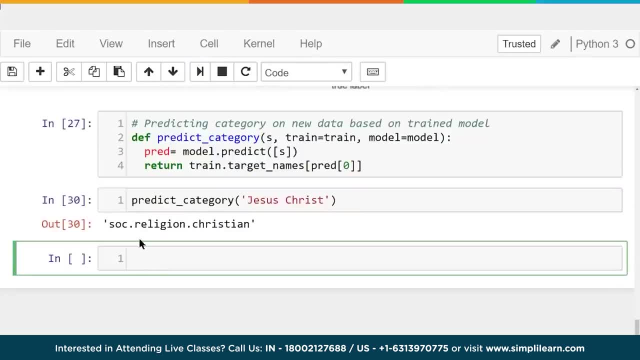 predict category Jesus Christ, And it comes back and says it's social religion, Christian. That's pretty good. Now note I didn't put print on this. One of the nice things about the Jupyter notebook editor and a lot of inline editors is if 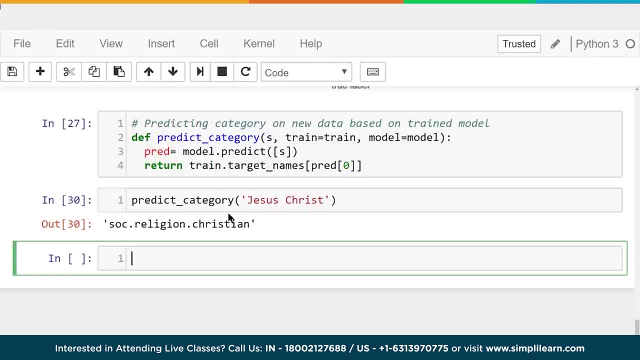 you just put the name of the variable out. it's returning the variable train dot target underscore names. It'll automatically print that for you In your own ID. you might have to put in print. Let's see where else we can take this. 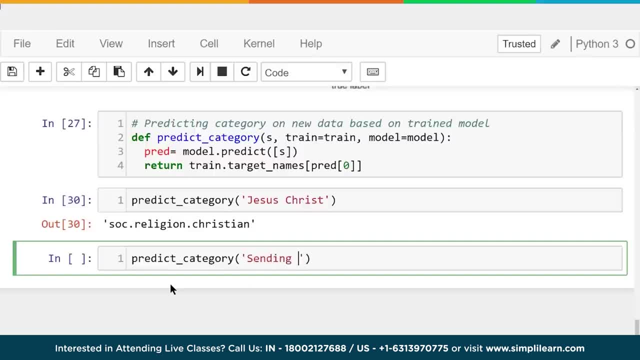 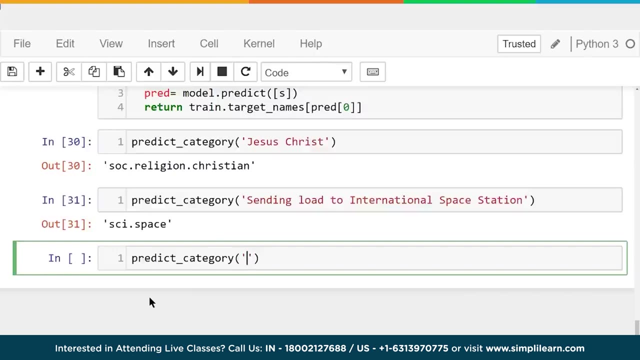 And maybe you're a space science buff. So how about sending load to international space station? And if we run that, we get science space. Or maybe you're a automobile buff, And let's do. they were going to tell me Audi is better than BMW, but I'm going to do. 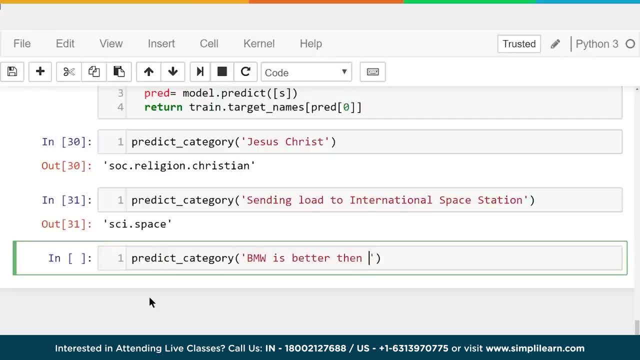 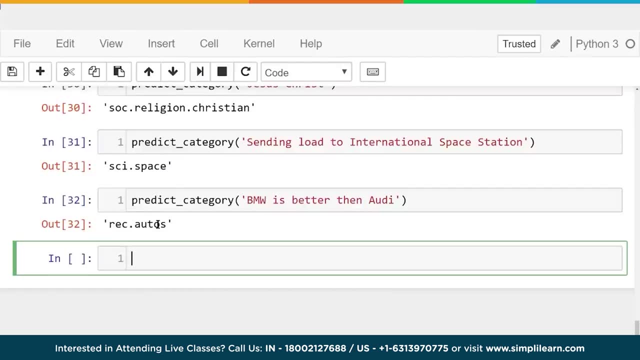 BMW is better than an Audi. So maybe you're a car buff And we run that and you'll see. it says foundational. I'm assuming that's what REC stands for Autos. So I did a pretty good job labeling that one. 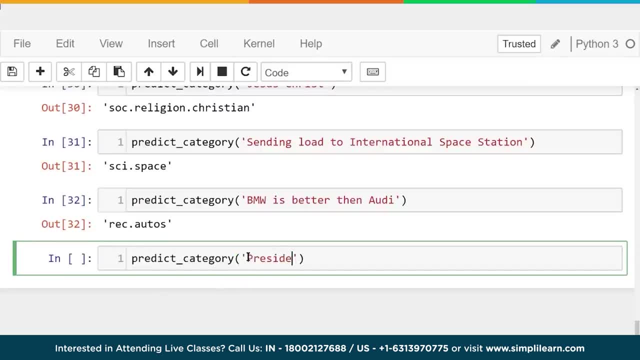 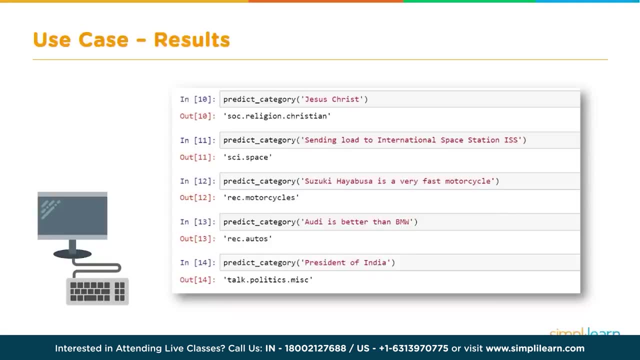 How about if we have something like a caption running through there, President of India, And if we run that it comes up and says: talk politics miscellaneous. So when we take our definition or our function and we run all these things through, kudos. 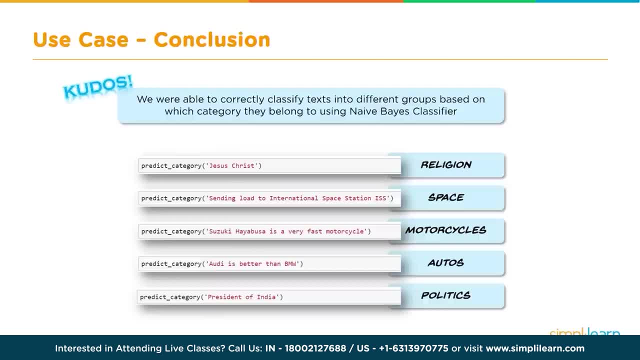 We made it. We were able to correctly classify texts into different groups based on which category they belong to, using the Naive Bayes class classifier. Now we did throw in the pipeline the TF-IDF vectorizer. we threw in the graphs, Those are all. 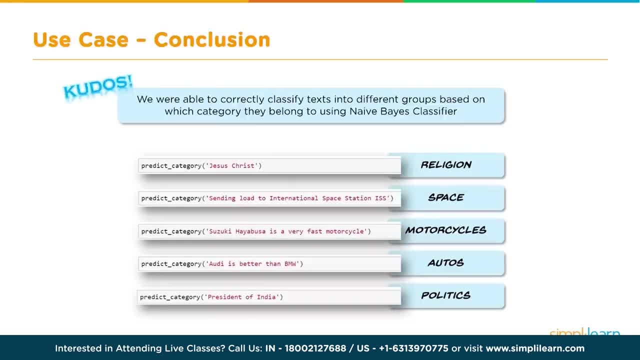 things that you don't necessarily have to know to understand the Naive Bayes setup or classifier, But they're important to know. One of the main uses for the Naive Bayes is with the TF- IDF tokenizer or vectorizer, where it tokenizes a word and has 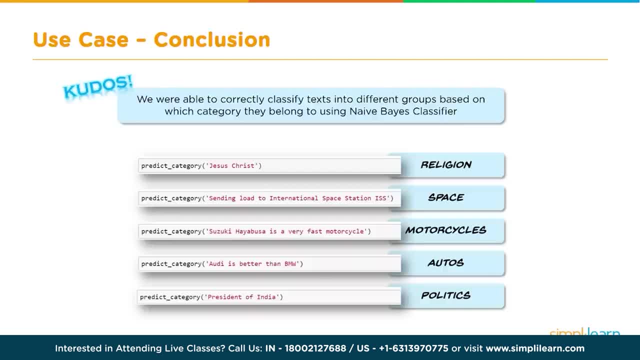 labels And we use the pipeline because you need to push all that data through and it makes it really easy and fast. You don't have to know those to understand Naive Bayes, but they certainly help for understanding the industry and data science And we can see. 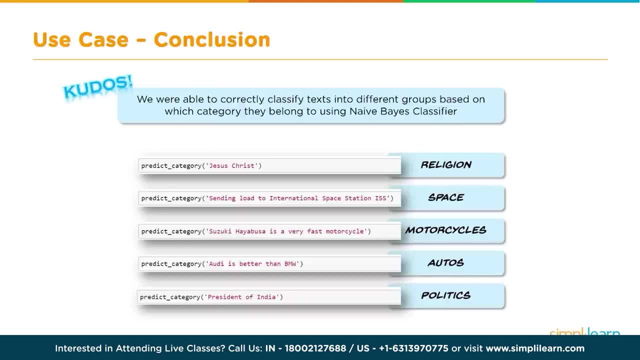 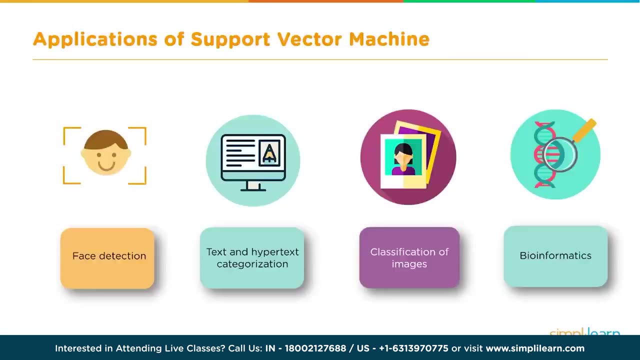 our categorizer, our Naive Bayes classifier. We were able to predict the category- religion, space, motorcycles, autos, politics- and properly classify all these different things. we pushed into our prediction and our trained model. Before we dive into the SVM, let's take a look at 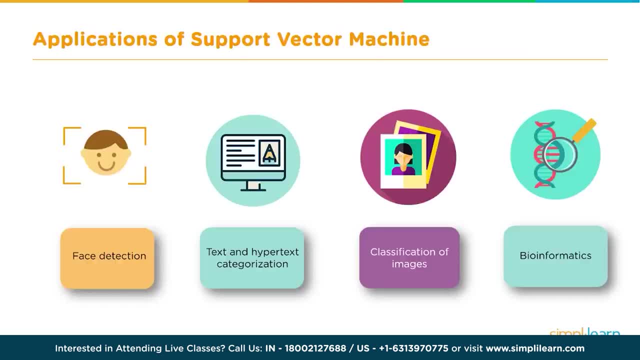 applications of the support vector machine, At least some general ones that are commonly used with it: Face detection, text and hypertext categorization, classification of images and bioinformatics. These are only but a few of those that are used with this SVM. 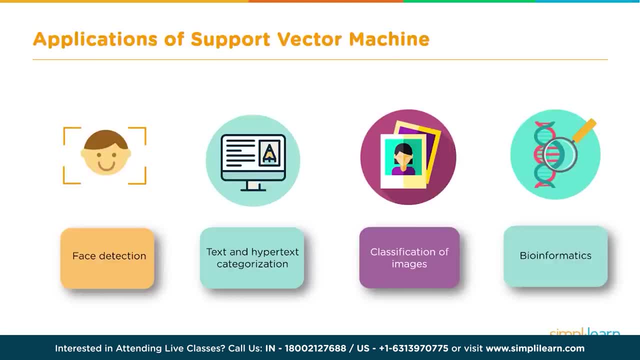 As we go through this lesson, see if you can figure out what other ones you can apply it to, And also what you would want to use some other tools for. What's in it for you? Today we're going to cover about six different sections. 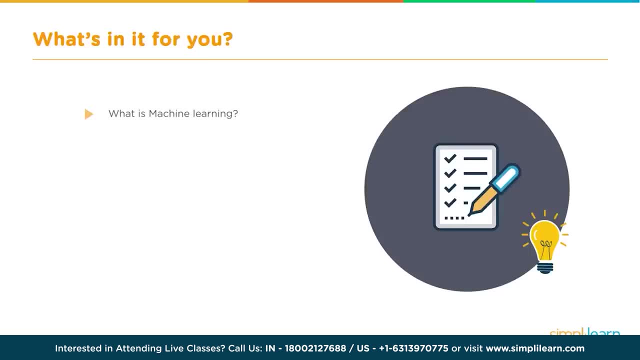 We're going to start with what is machine learning, So we can see where the vector machine fits in. Why the support vector machine, What is a support vector machine? And understanding the support vector machine, Once we go through an understanding of how it works and what it looks like. 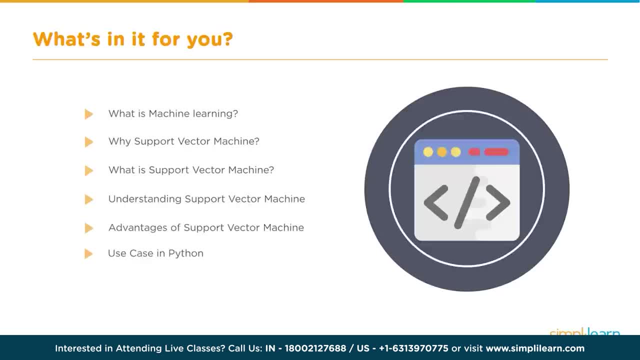 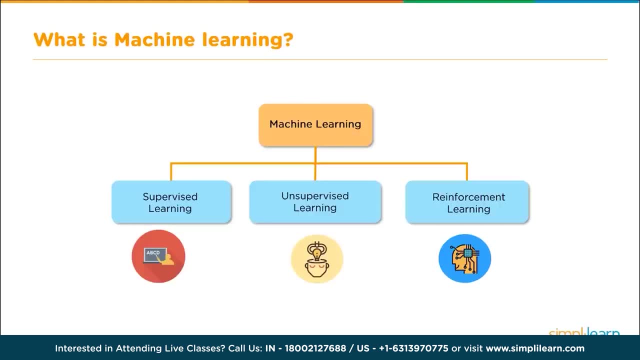 we're going to look at the advantages of support vector machine and finally dive in to a use case in Python where we'll write some script on it. Let's start with what is machine learning and even more specific, where does the support vector machine algorithm fit in The biggest split? 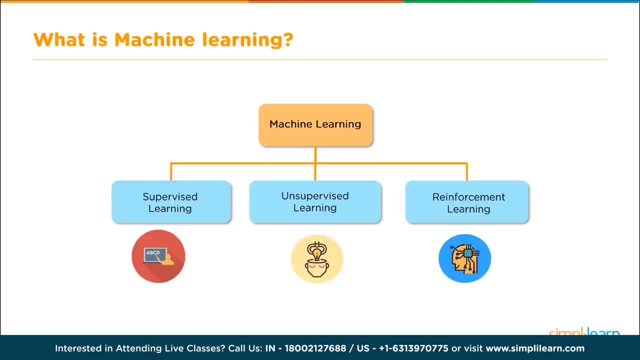 in machine learning is between the three categories: supervised learning, where we have data and we can train it. unsupervised learning, where we're just guessing at what we can make sense of the data. and reinforcement learning, where we reinforce a good or bad behavior. Since the 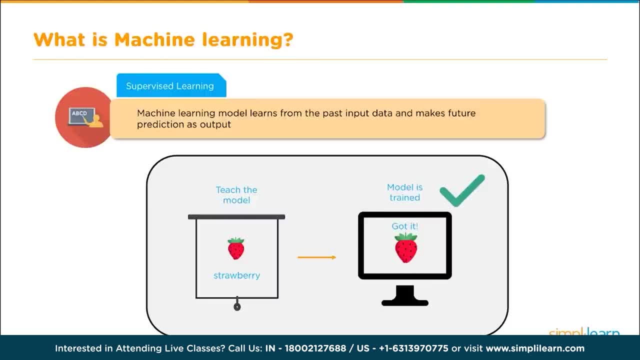 SVM is specific to supervised learning. machine learning model learns from the past input data and makes future predictions as output. So we teach the model, we teach it what a strawberry is and once the model is trained, it can identify a strawberry. That's what's. 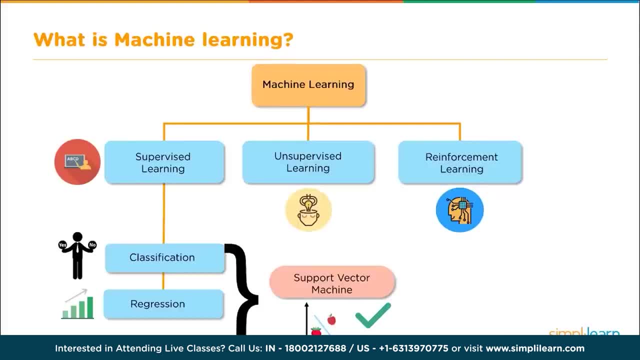 meant by supervised learning. In the larger picture of the machine learning model and under supervised learning, you can see that the support vector fits in under classification, deciding what yes and no is, And there is also a regression version, but it is primarily used for classification. Let's take a detour. 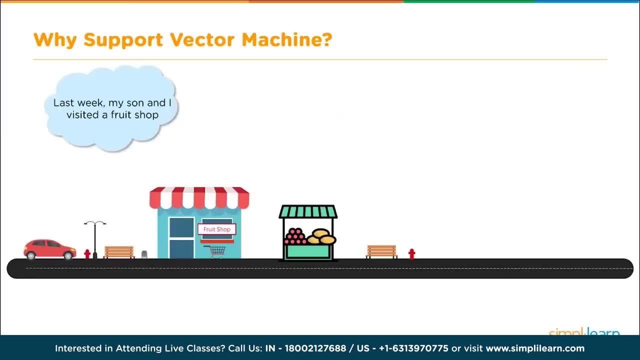 and see if we can connect this to the human experience and find out why support vector machine. So in this example, last week my son and I visited a fruit shop. Dad, is that an apple or a strawberry? So the question comes up: what fruit did I just pick up? 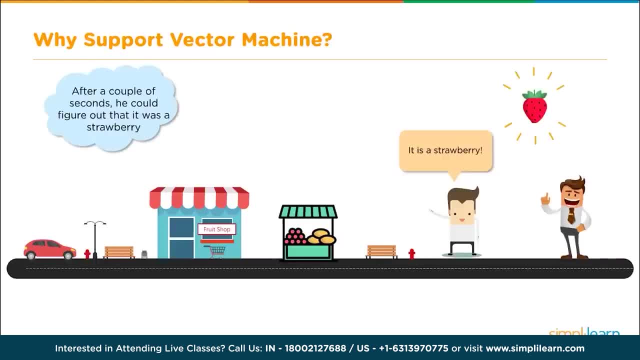 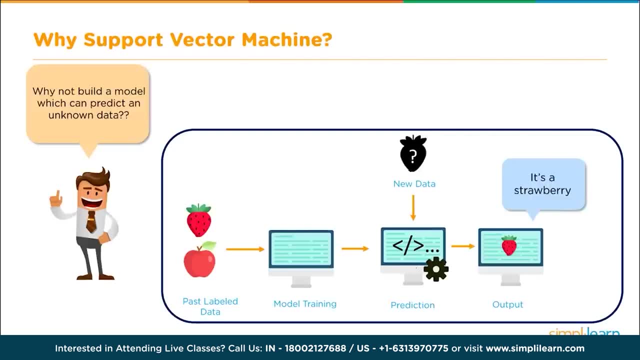 from the fruit stand. After a couple of seconds, you can figure out that it was a strawberry. So let's take this model a step further and let's- why not? build a model which can predict an unknown data, And in this we're going to be looking. 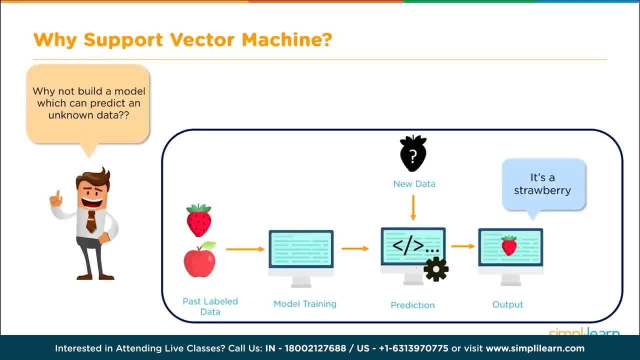 at some sweet strawberries or crispy apples. We want it to be able to label those two and decide what the fruit is, And we do that by having data already put in. So we already have a bunch of strawberries we know are strawberries and they're already. 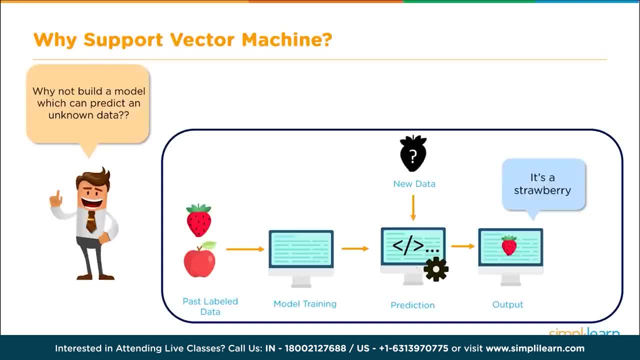 labeled as such. We already have a bunch of apples we know are apples and are labeled as such. Then, once we train our model, that model then can be given the new data, and the new data is this image In this case, you can: 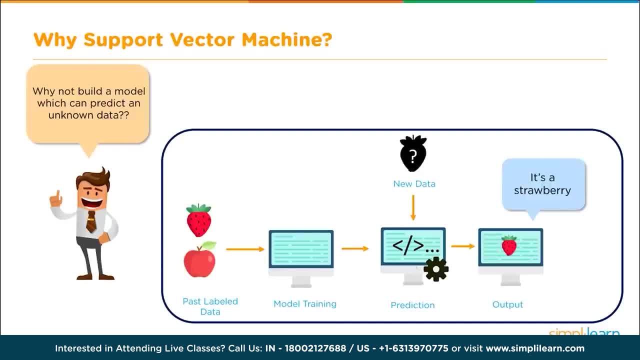 see a question mark on it and it comes through and goes. it's a strawberry. In this case, we're using the support vector machine model. SVM is a supervised learning method that looks at data and sorts it into one of two categories, And in this case we're sorting the strawberry. 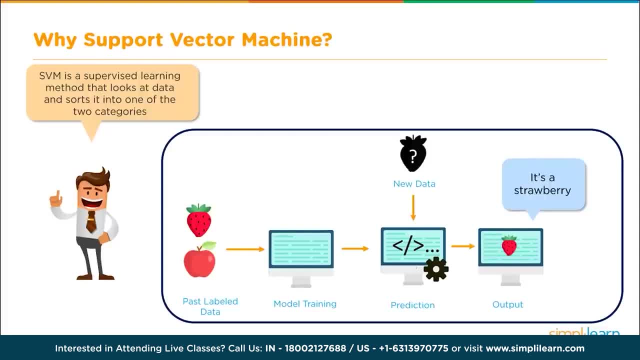 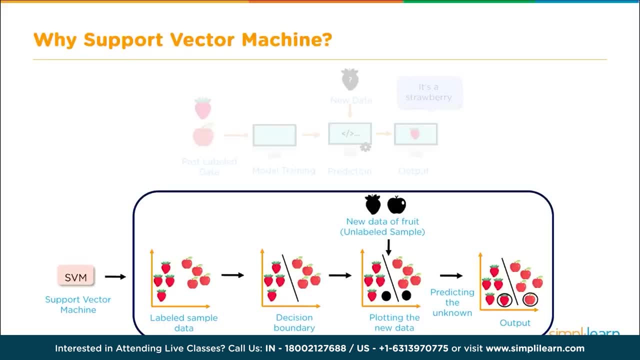 into the strawberry side. At this point you should be asking the question: how does the prediction work? Before we dig into an example with numbers, let's apply this to our fruit scenario. We have our support vector machine. We've taken it and we've taken. 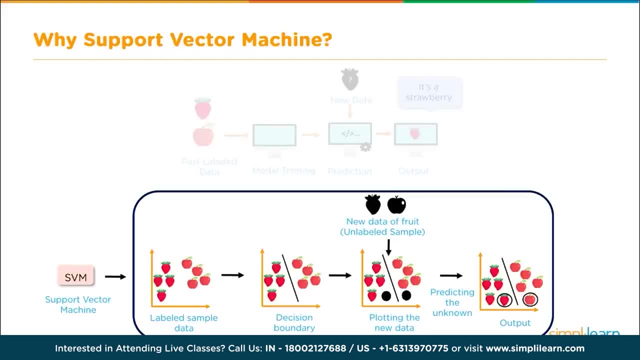 labeled. sample of data- strawberries and apples- and we draw on a line down the middle between the two groups. This split now allows us to take new data, in this case an apple and a strawberry, and place them in the appropriate group, based on which. 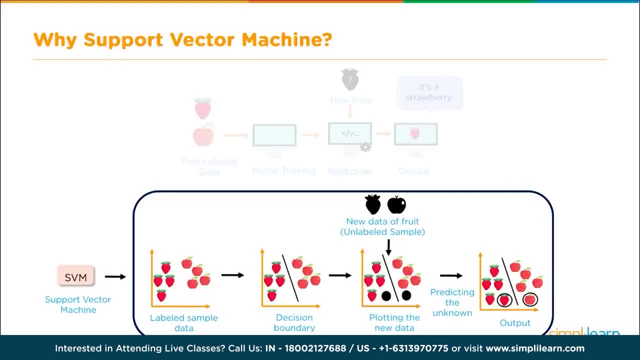 side of the line they fall. in That way, we can predict the unknown. As colorful and tasty as the fruit example is, let's take a look at another example. with some numbers involved, We can take a closer look at how the math works. 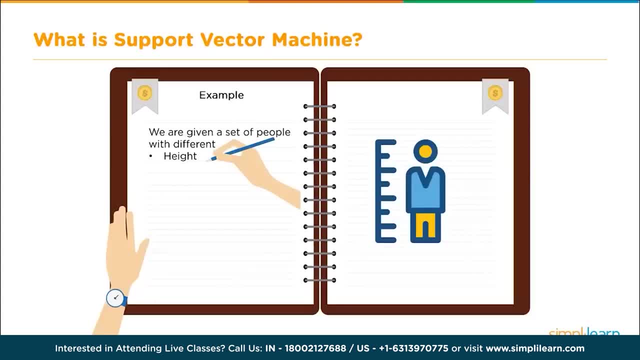 In this example, we're going to be classifying men and women. We're going to start with a set of people with a different height and a different weight. To make this work, we'll have to have a sample data set of female. We have their 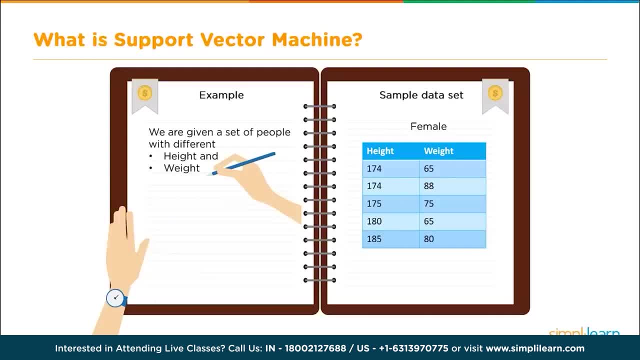 height and weight: 174,, 65,, 174,, 88, and so on. We'll need a sample data set of the male. They have a height 179,, 90,, 180 to 80, and so on. 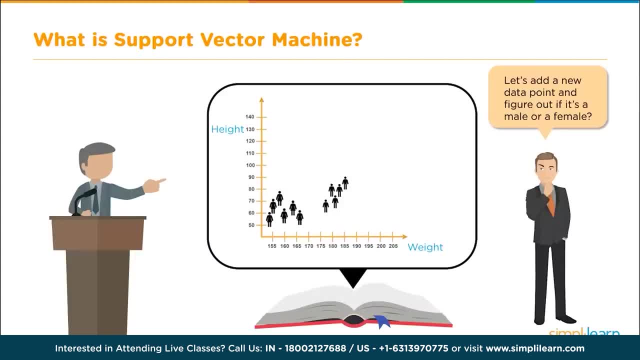 Let's go ahead and put this on a graph so we have a nice visual. You can see here we have two groups based on the height versus the weight. On the left side we're going to have the women On the right side. 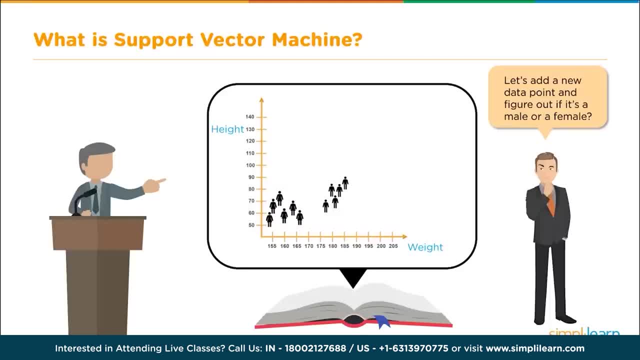 we're going to have the men. If we're going to create a classifier, let's add a new data point and figure out if it's male or female. Before we can do that, we need to split our data first. We can split our data by choosing: 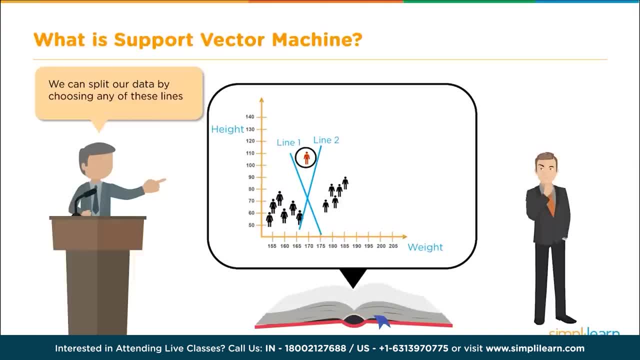 any of these lines. In this case we draw in two lines through the data in the middle that separates the men from the women. But to predict the gender of a new data point, we should split the data in the best possible way. We say the best possible way. 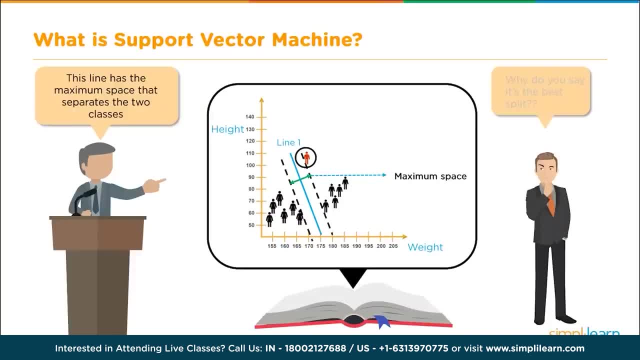 because this line has a maximum space that separates the two classes. Here you can see, there's a clear split between the two different classes. In this one there's not so much a clear split. This doesn't have the maximum space that separates the two. That is why this line. 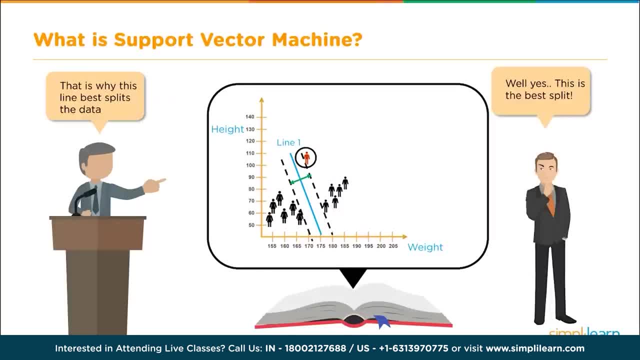 best splits the data. We don't want to just do this by eyeballing it. Before we go further, we need to add some technical terms to this. We can also say that the distance between the points in the line should be as far as possible In technical terms. 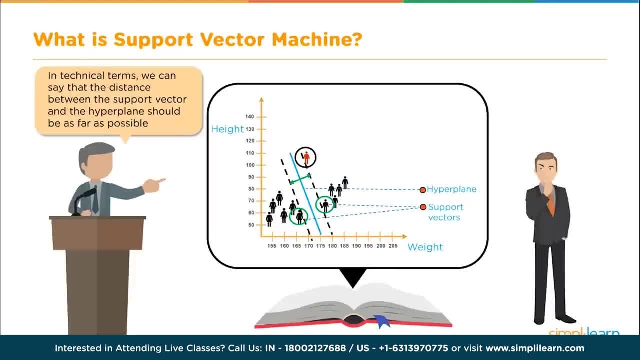 we can say the distance between the support vector and the hyperplane should be as far as possible. This is where the support vectors are the extreme points in the data set. If you look at this data set, they have circled two points which seem to be: 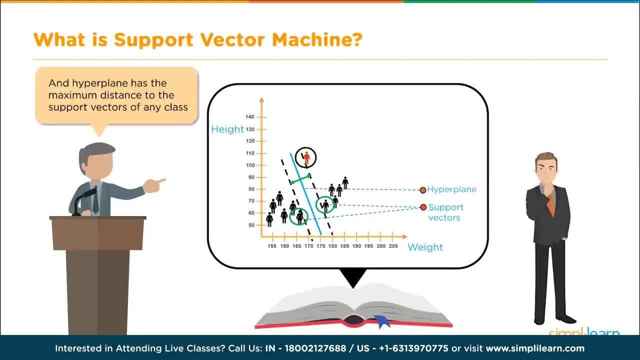 right on the outskirts of the women and one on the outskirts of the men. Hyperplane has a maximum distance to the support vectors of any class. You'll see the line down the middle. We call this the hyperplane because when you're dealing with multiple dimensions, 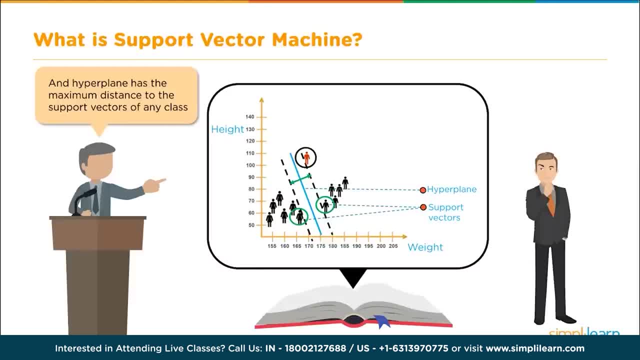 it's really not just a line but a plane of intersections. You can see here where the support vectors have been drawn in dashed lines. The math behind this is very simple. We take D plus the shortest distance to the closest positive point, which would be on the men's side. 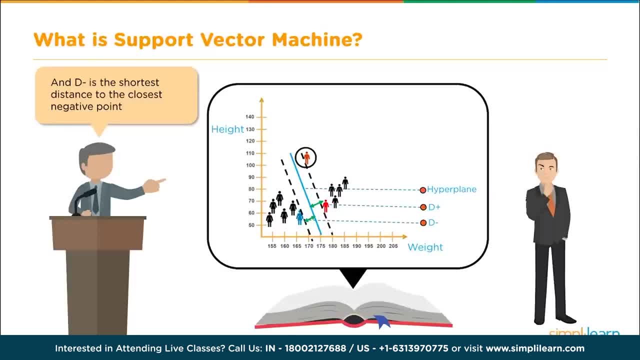 and D minus is the shortest distance to the closest negative point, which is on the women's side. The sum of D plus and D minus is called the distance margin, or the distance between the two support vectors that are shown in the dashed lines. 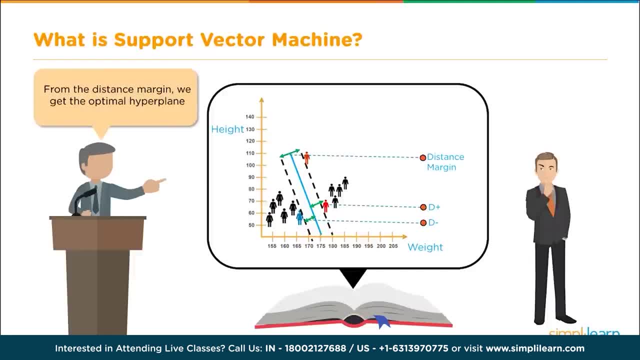 Then, by finding the largest distance margin, we can get the optimal hyperplane. Once we've created an optimal hyperplane, we can easily see which side the new data fits in. Based on the hyperplane, we can say the new data point. 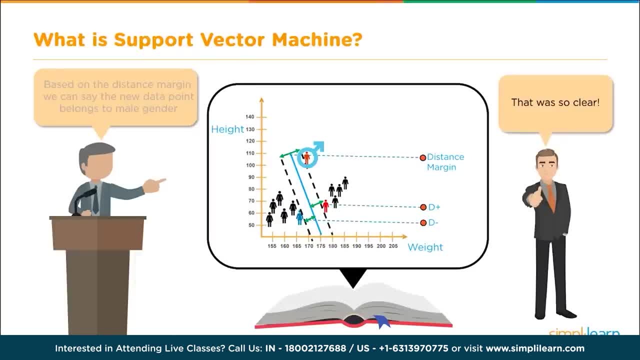 belongs to the male gender. We can also compare how that works on a visual level. As a data scientist, you should also be asking what happens if the hyperplane is not optimal. If we select a hyperplane having low margin, then there is a high chance of misclassification. 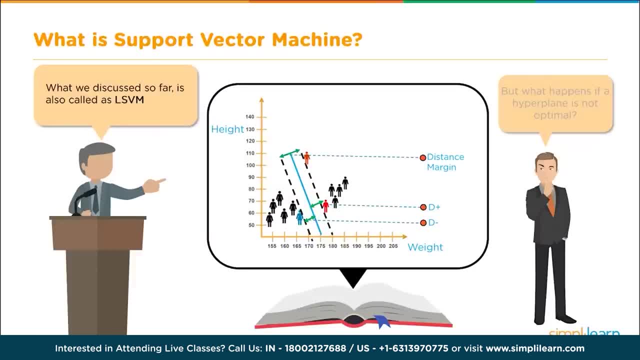 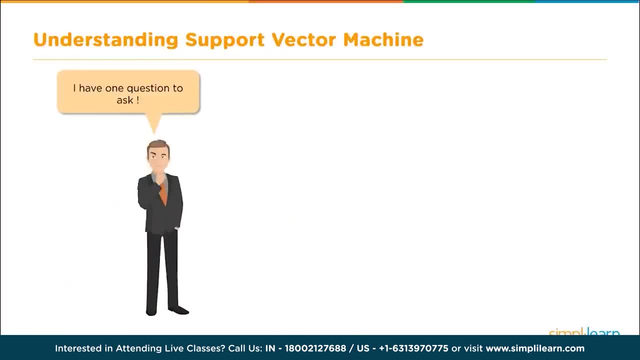 This particular SVM model, the one we discussed so far, is also called or referred to as the LSVM. So far, so clear. but a question should be coming up. We have our sample data set, but instead of looking like this, what if it looked like this? 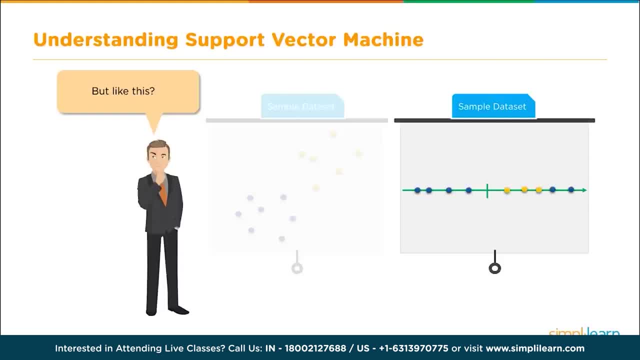 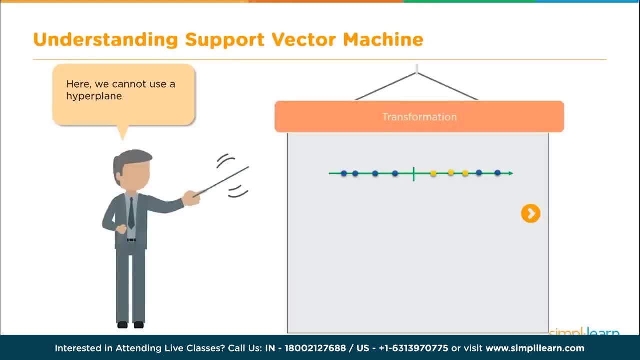 with two sets of data, but one of them occurs in the middle of another set. You can see here where we have the blue and the yellow and then blue again on the other side of our data line. In this data set we can't use a hyperplane. 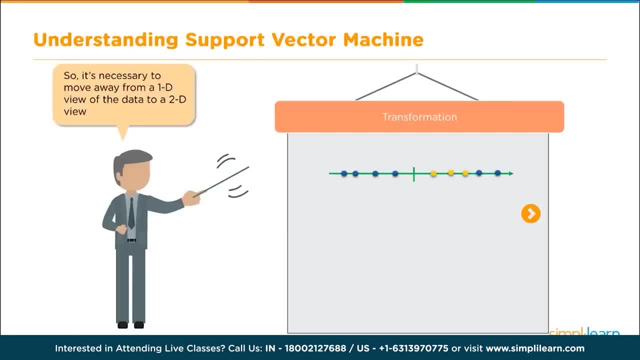 So when you see data like this, it's necessary to move away from a 1D view of the data to a two-dimensional view of the data, And for the transformation we use what's called a kernel function. The kernel function will take the 1D. 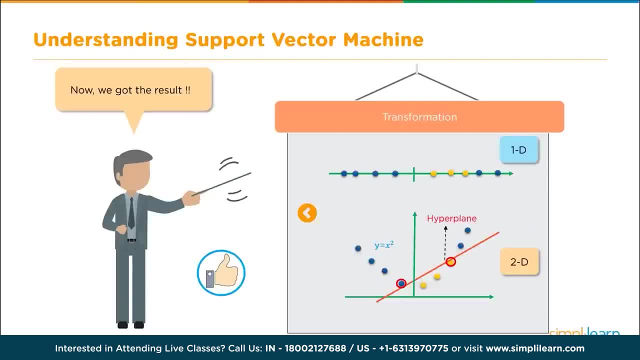 input and transfer it to a two-dimensional output. In this picture here, the 1D, when transferred to a two-dimensional, makes it very easy to draw a line between the two data sets. What if we make it even more complicated? How do we perform an SVM? 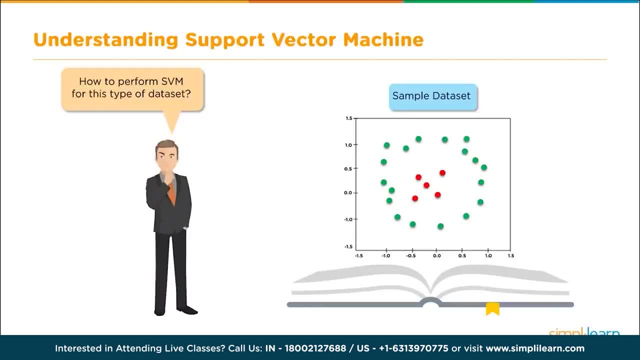 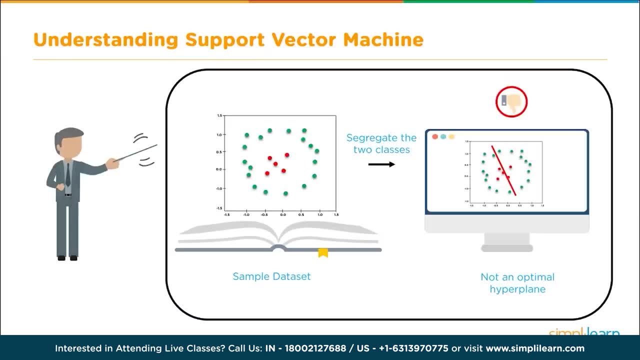 for this type of data set. Here you can see we have a two-dimensional data set where the data is in the middle surrounded by the green data on the outside. In this case, we're going to segregate the two classes. We have our sample data set. 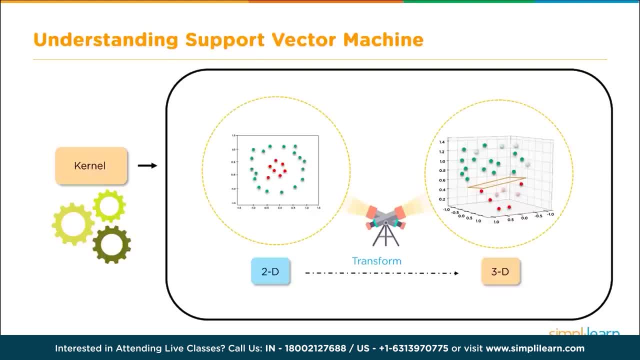 and if you draw a line through, it's obviously not an optimal hyperplane in there. It's a 2D to a 3D array And when you translate it into a three-dimensional array using the kernel, you can see where you can. 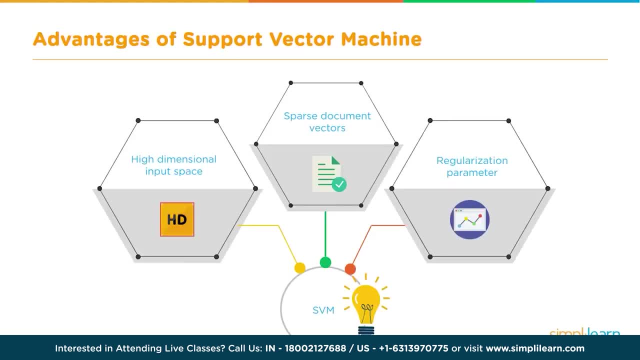 place a hyperplane right through it and easily split the data. Before we start looking at a programming example and dive into the script, let's look at the advantage of the support vector machine. We'll start with high-dimensional input space, or sometimes referred to. 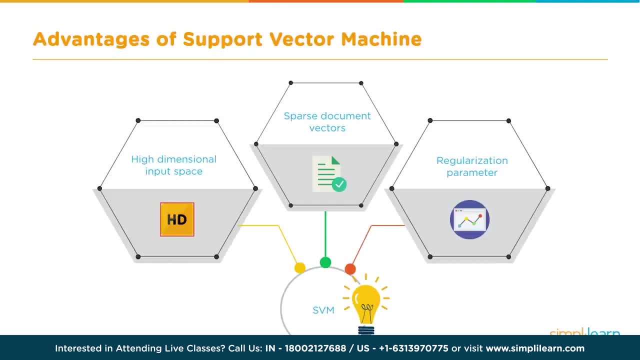 as the curse of dimensionality. We looked at earlier one dimension, two dimension, three dimension. When you get to a thousand dimensions a lot of problems start occurring with most algorithms that have to be adjusted for. The SVM automatically does that in high-dimensional space. One of the 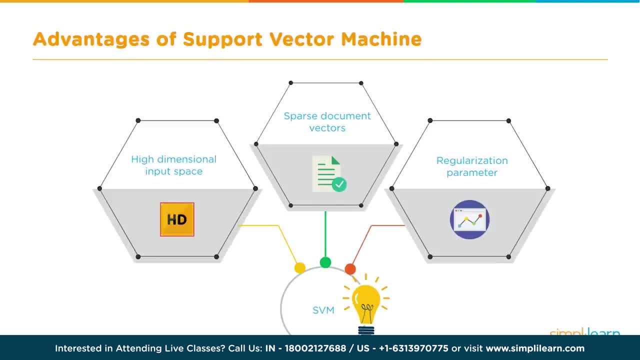 high-dimensional space. one high-dimensional space that we work on is sparse document vectors. This is where we tokenize the words in documents so we can run our machine learning algorithms over them. I've seen ones get as high as 2.4 million different tokens. 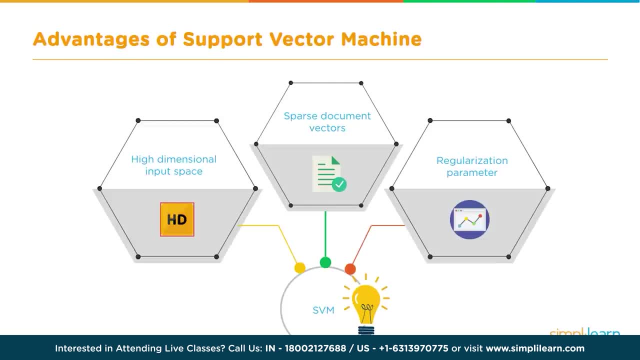 That's a lot of vectors to look at. And finally, we have regularization parameter. The regularization parameter, or lambda, is a parameter that helps figure out whether we're going to have bias or overfitting of the data, Whether it's going to be overfitted to a very 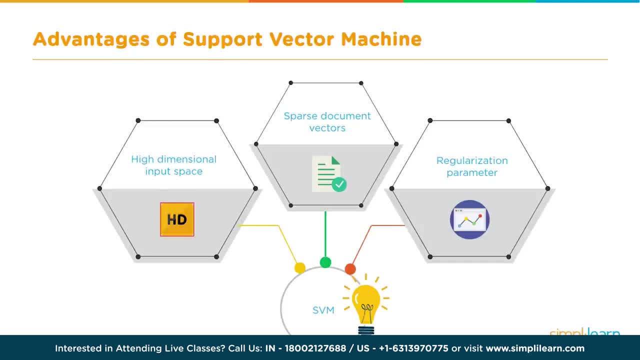 specific instance or it's going to be biased to a high or low value. With the SVM, it naturally avoids the overfitting and bias problems that we see in many other algorithms. These three advantages of the support vector machine make it a very powerful tool. 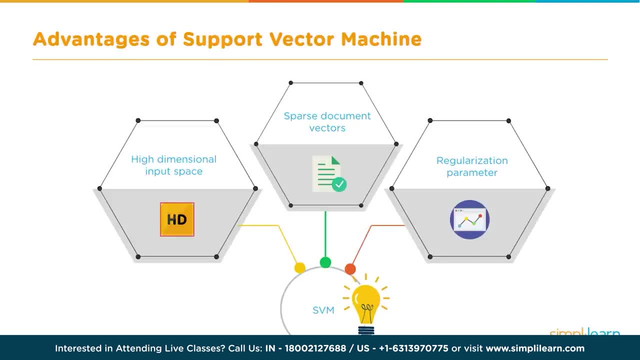 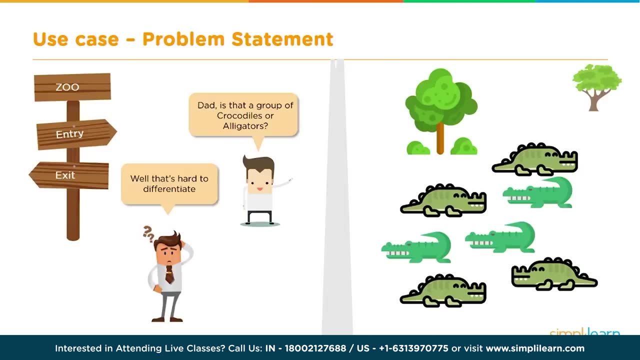 to add to your repertoire of machine learning tools. Now, we did promise you a use case study. We're actually going to dive into some Python programming. We're going to go into a problem statement and start off with the zoo. For example, we have family members. 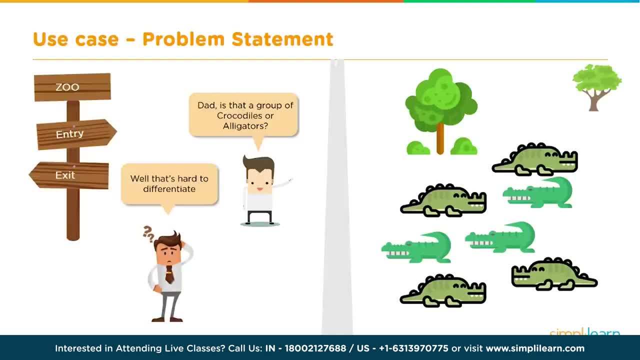 going to the zoo and we have the young child going. Dad, is that a group of crocodiles or alligators? Well, that's hard to differentiate, And zoos are a great place to start looking at science and understanding how things work, especially. 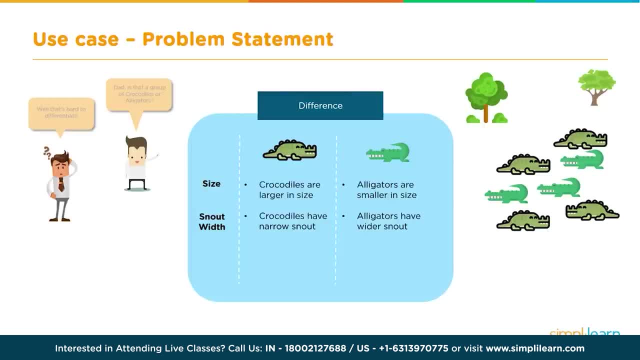 as a young child, And so we can see the parents sitting here thinking, well, what is the difference between a crocodile and an alligator? Well, one, crocodiles are larger in size. alligators are smaller in size. snout width. the crocodiles have a narrow. 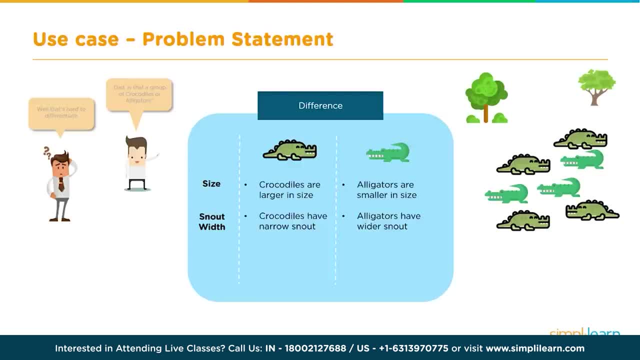 snout and alligators have a wider snout. And of course, in the modern day and age, the father is sitting here thinking how can I turn this into a lesson for my son? And he goes: let a support vector machine. 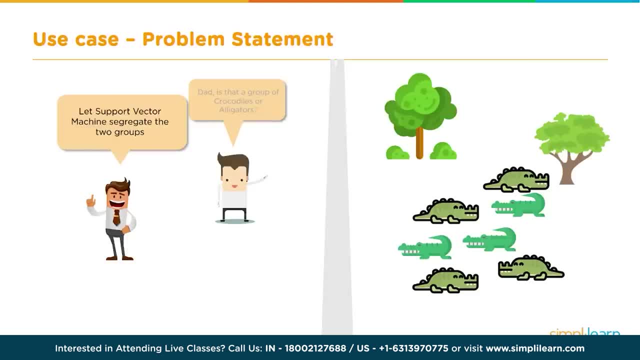 segregate the two groups. I don't know if my dad ever told me that, but that would be funny. Now, in this example, we're not going to use actual measurements and data. We're just using that for imagery, And that's very common in a lot of machine. 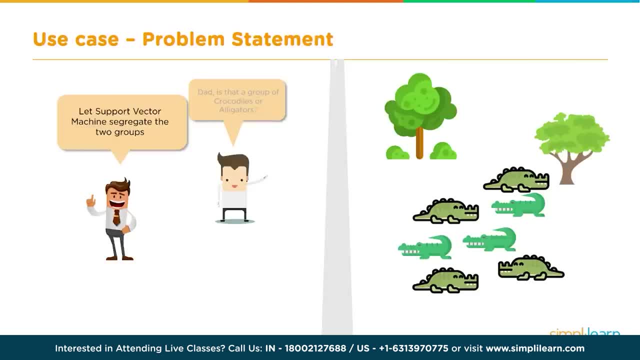 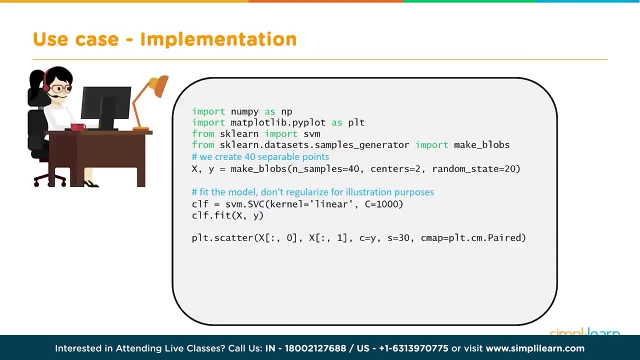 learning algorithms and setting them up. But let's roll up our sleeves- and we'll talk about that more in just a moment- as we break into our Python script. So here we arrive, in our actual coding, And I'm going to move this into a 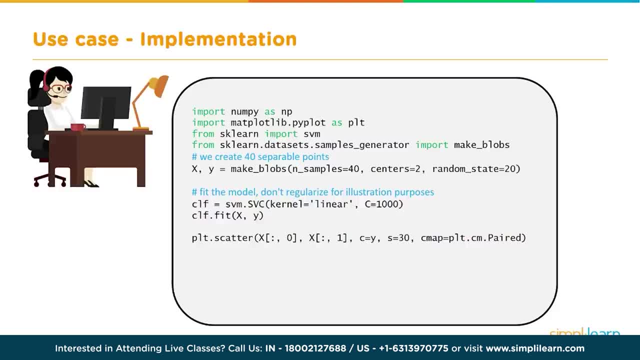 Python editor in just a moment. But let's talk a little bit about what we're going to cover First. we're going to cover in the code the setup, how to actually create our SVM, And you're going to find that there's only two lines of code that. 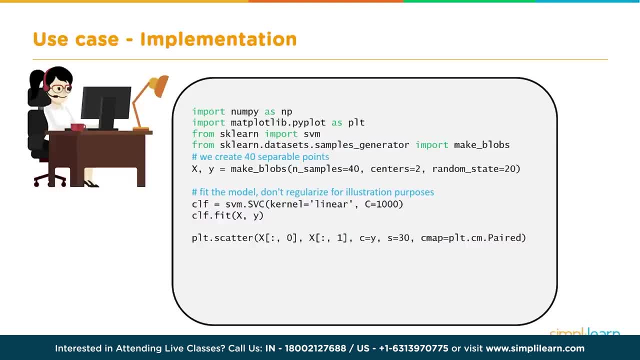 actually create it and the rest of it is done so quick and fast that it's all here in the first page And we'll show you what that looks like as far as our data, because we're going to create some data I talked about. 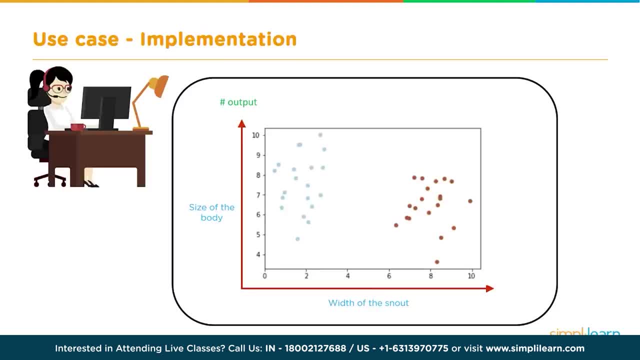 creating data just a minute ago, And so we'll get into the creating data here and you'll see this nice correction of our two blobs And we'll go through that in just a second. And then the second part is: we're going to take this and we're going to bump it up a notch. 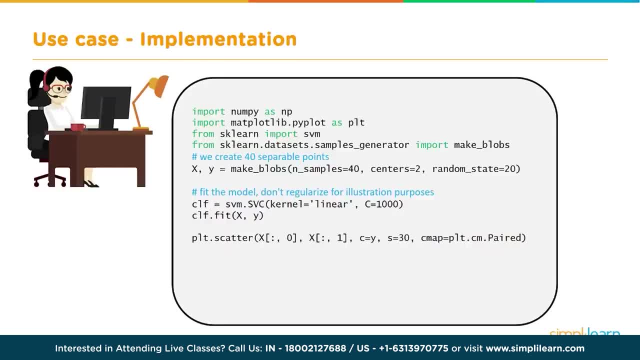 We're going to show you what it looks like behind the scenes, But let's start with actually creating our setup. I like to use the Anaconda Jupyter notebook because it's very easy to use, But you can use any of your favorite Python. 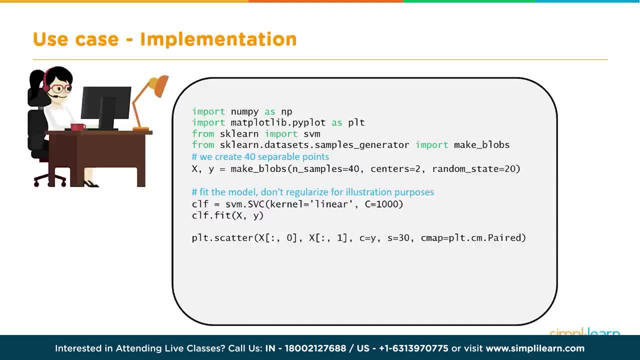 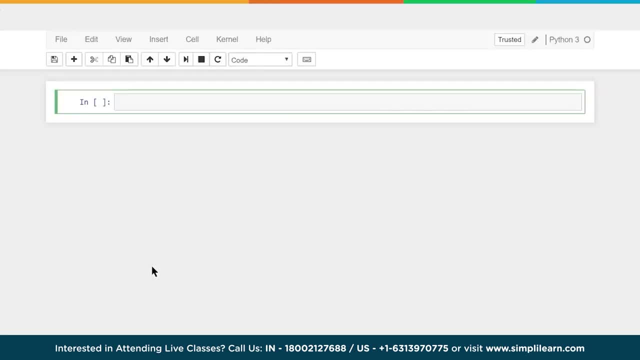 editors or setups and go in there, But let's go ahead and switch over there and see what that looks like. So here we are in the Anaconda Python notebook or Anaconda Jupyter notebook with Python. We're using Python 3.. 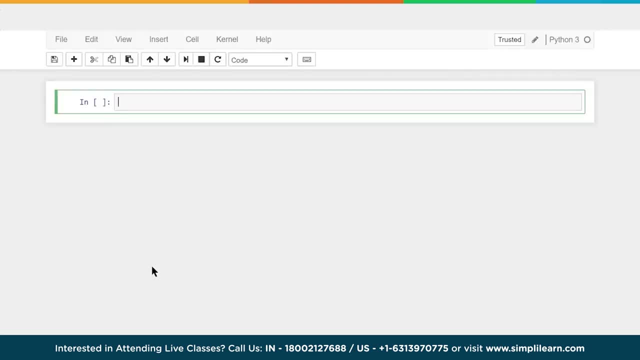 I believe this is 3.5, but it should work in any of your 3x versions. You'd have to look at the sklearn and make sure. if you're using a 2x version or an earlier version, Let's go ahead and put our code in there. 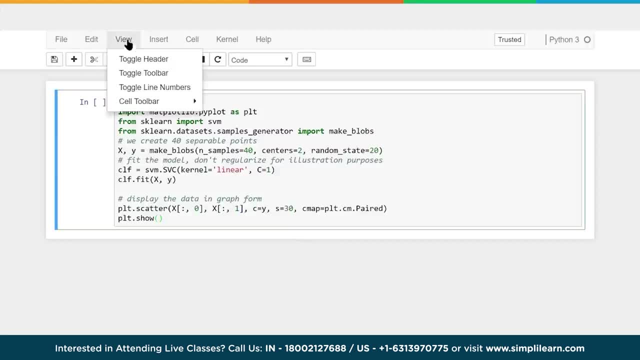 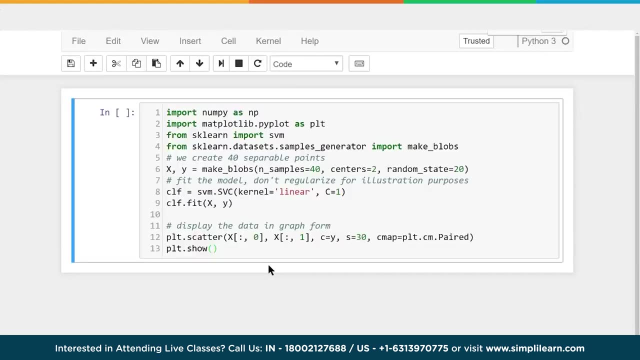 One of the things I like about the Jupyter notebook is I can go up to view and I'm going to go ahead and toggle the line numbers on to make it a little bit easier to talk about, And we can even increase the size, because this is edited in. in this case I'm using 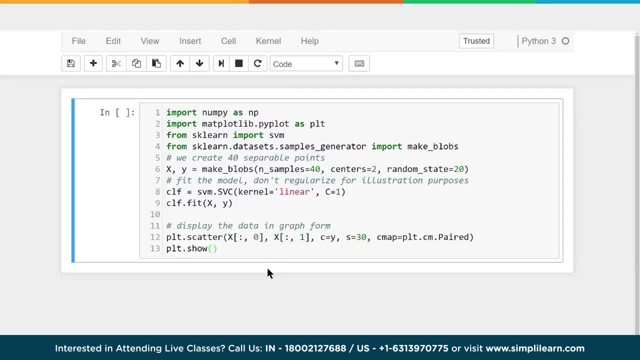 Google Chrome Explorer and that's how it opens up for the editor. Like I said, any editor will work. Now the first step is going to be our imports, And we're going to import 4 different parts. The first two I want you to look at are line 1. 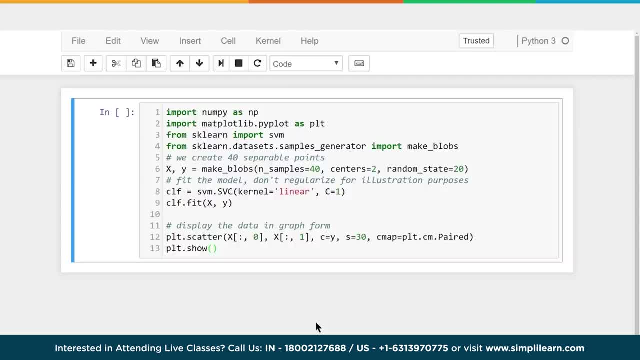 and line 2 are numpy as np and matplotlibrarypyplot as plt. Now, these are very standardized imports when you're doing work. The first one is the numbers Python. We need that because part of the platform we're using uses that for the numpy array, And I'll talk 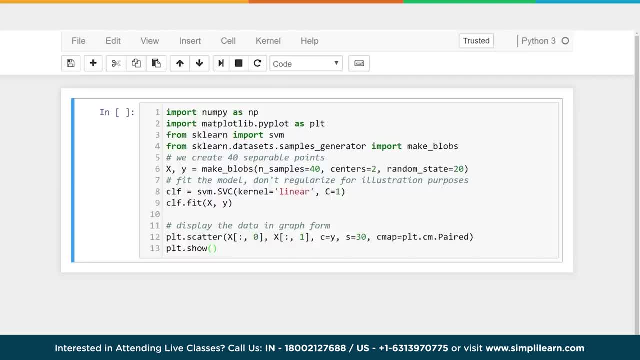 about that in a minute so you can understand why we want to use a numpy array versus a standard Python array. And normally it's pretty standard setup to use np for numpy. The matplotlibrary is how we're going to view our data. So this has you do need the. 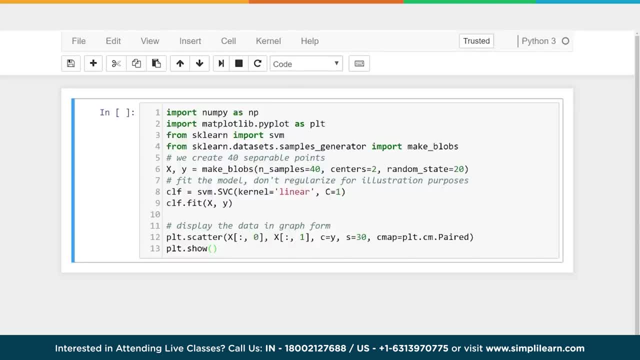 np for the sklearn module. But the matplotlibrary is purely for our use, for visualization, And so you really don't need that for the SVM. But we're going to put it there so you have a nice visual aid and we can show you what it looks like. That's really important. 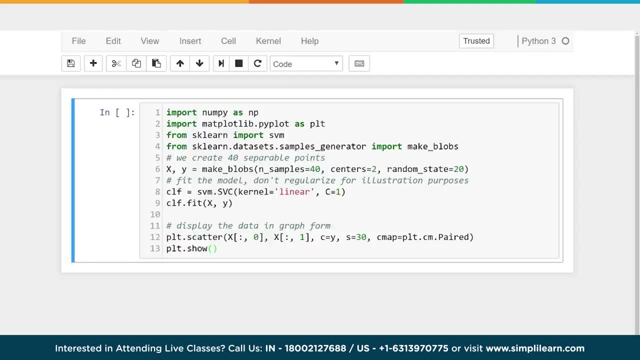 at the end, when you finish everything, So you have a nice display for everybody to look at. And then, finally, we're going to- I'm going to jump one ahead- to line number 4.. That's the sklearndatasetssamplesgenerator. That's the sklearndatasetssamplesgenerator. 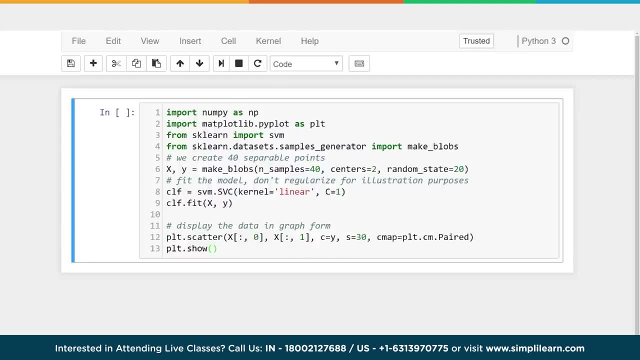 import makeblobs And I told you that we were going to make up data And this is a tool that's in the sklearn to make up data. I personally don't want to go to the zoo, get in trouble for jumping over the fence and probably get eaten by. 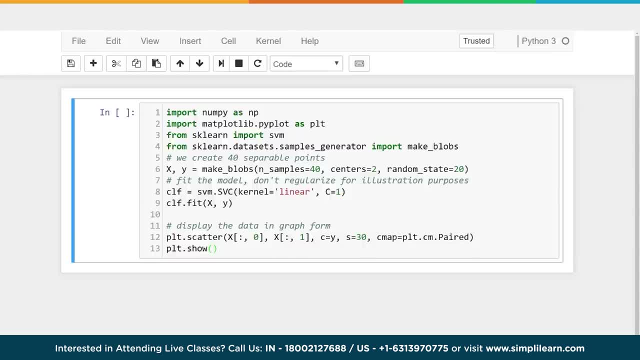 the crocodiles or alligators, as I work on measuring their snouts and width and length. Instead, we're just going to make up some data, And that's what that makeblobs is. It's a wonderful tool if you're ready to test your. 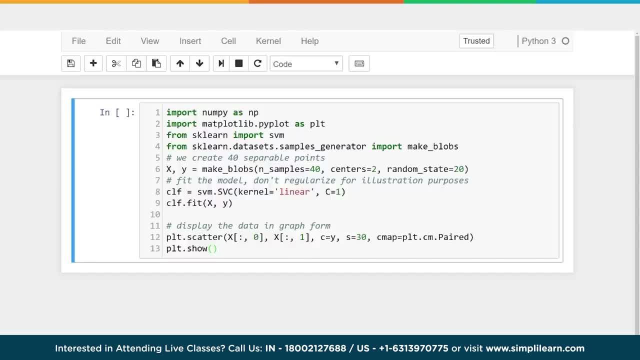 setup and you're not sure about what data you're going to put in there. You can create this blob and it makes it real easy to use. And finally we have our actual SVM, The sklearn import SVM, on line 3.. So that covers all our imports. 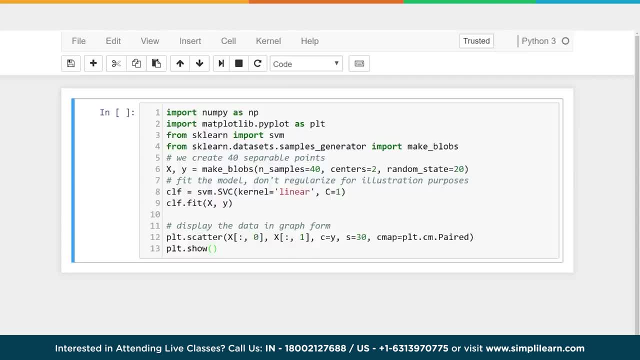 We're going to create- remember, I used the makeblobs to create data- and we're going to create a capital X and a lowercase Y equals makeblobs in samples, equals 40.. So we're going to make 40 lines of data. 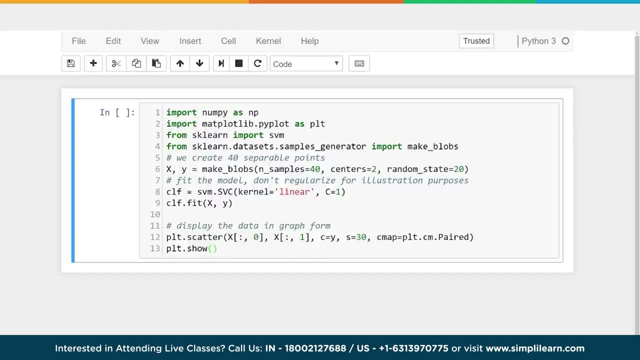 It's going to have two centers with a random state equals 20.. So each group is going to have 20 different pieces of data in it, And the way that looks is that we'll have under X an XY plane. So I'll have two numbers under X and 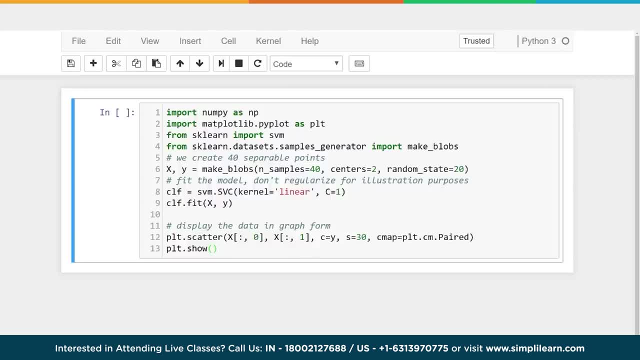 Y will be 0 or 1.. That's the two different centers. So we have yes or no, in this case alligator or crocodile. That's what that represents. And then I told you that the actual sklearn, or the SVM, is in two lines of code And we see. 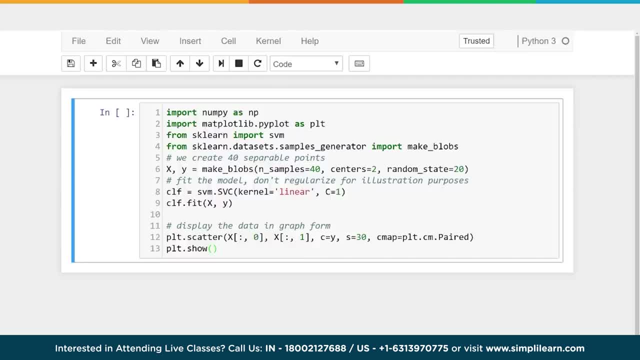 it right here, with clf equals svm, dot, svc, kernel equals linear And I set c equal to 1.. Although, in this example, since we are not regularizing the data, since we want it to be very clear and easy to see, I went ahead. you can set it. 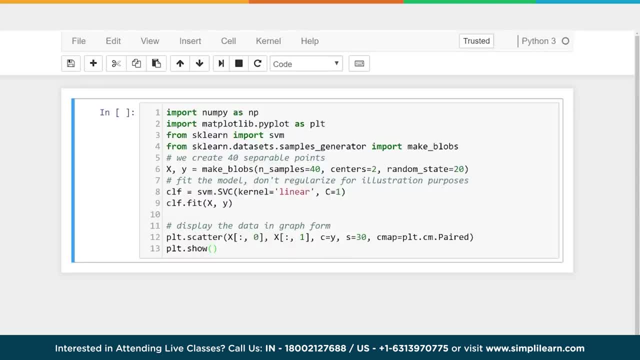 to 1000 a lot of times when you're not doing that. But for this thing- linear because it's a very simple linear example. We only have the two dimensions and it'll be a nice linear hyper plane. It'll be a nice linear line instead of a full. 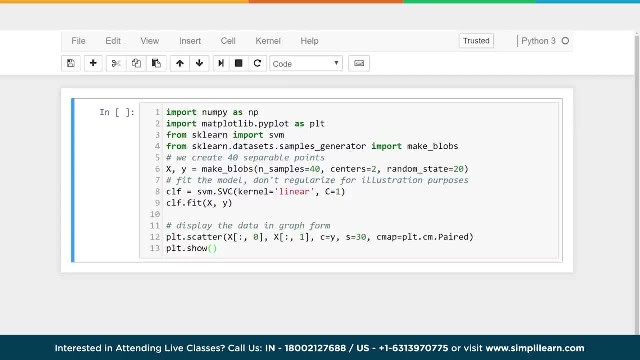 plane. So we're not dealing with a huge amount of data, And then all we have to do is do clf, dot fit X, comma Y, And that's it. Clf has been created, And then we're going to go ahead and display it And I'm going to. 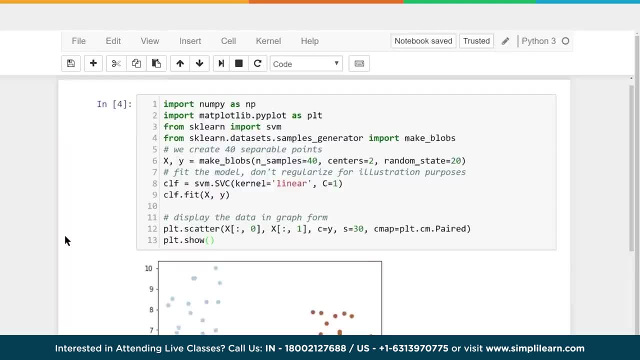 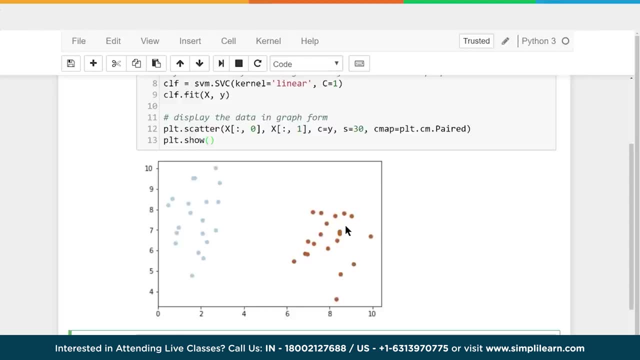 talk about this display here in just a second, But let me go ahead and run this code- And this is what we've done- is we've created two blobs. You'll see the blue on the side and then kind of an orangish on the other side. That's our two sets of. 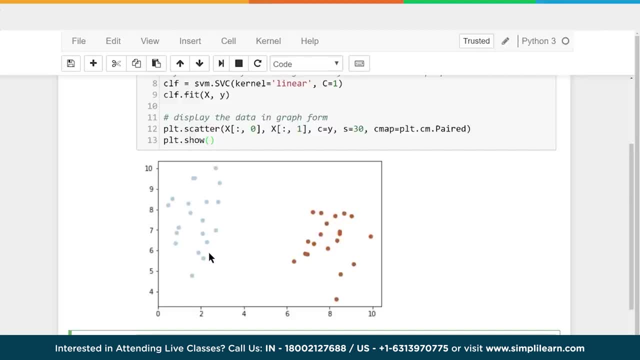 data They represent- one represents crocodiles and one represents alligators- And then we have our measurements. In this case we have like the width and length of the snout, And I did say I was going to come up here and talk. 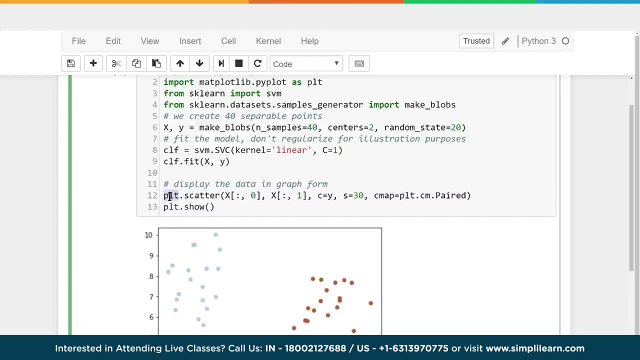 just a little bit about our plot And you'll see plt- That's what we imported. We're going to do a scatter plot. That means we're just putting dots on there. And then look at this notation: I have the capital X and then in: 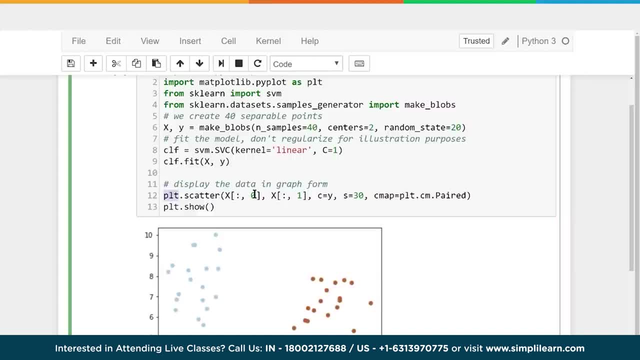 brackets. I have a colon, comma zero. That's from numpy. If you did that in a regular array you'll get an error in a Python array. You have to have that in a numpy array. It turns out that our make blobs returns a numpy. 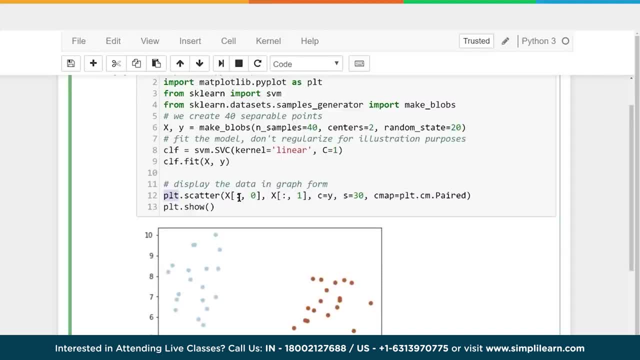 array. And this notation is great because what it means is: the first part is the colon. It means we're going to do all the rows, That's all the data in our blob we created under capital X, And then the second part has a comma. 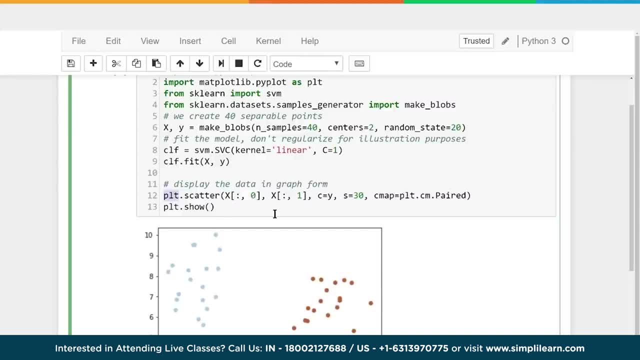 zero. We're only going to take the first value And then, if you notice, we do the same thing, but we're going to take the second value. Remember we always start with zero and then one, So we have column zero and column one. 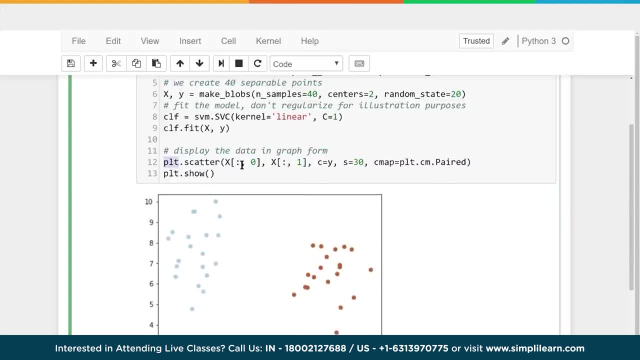 And you can look at this as our XY plots. The first one is the X plot and the second one is the Y plot. So the first one is on the bottom zero, two, four, six, eight and ten, And then the second. 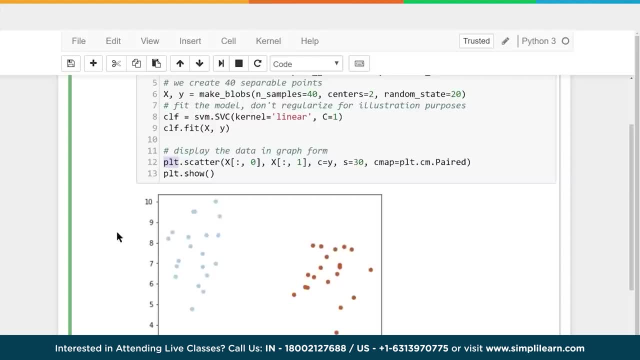 one X of the one is the four, five, six, seven, eight, nine, ten. going up the left hand side S equals thirty, is just the size of the dots, So we can see them. It says real tiny dots. 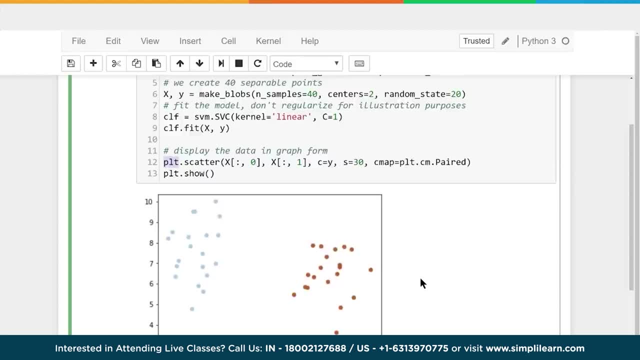 And then CMAP equals PLT, dot, CM, dot paired, And you'll also see the C equals Y. That's the color We're using, two colors, zero one, and that's why we get the nice blue and the two different colors for the alligator. 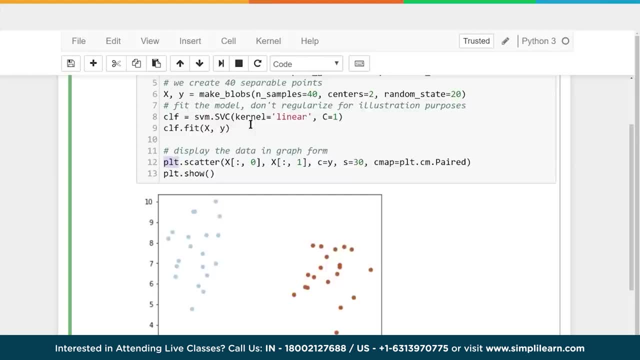 and the crocodile. Now you can see here that we did this. the actual fit was done in two lines of code. A lot of times it'll be a third line where we regularize the data. We set it between like minus one and one And we reshape it. 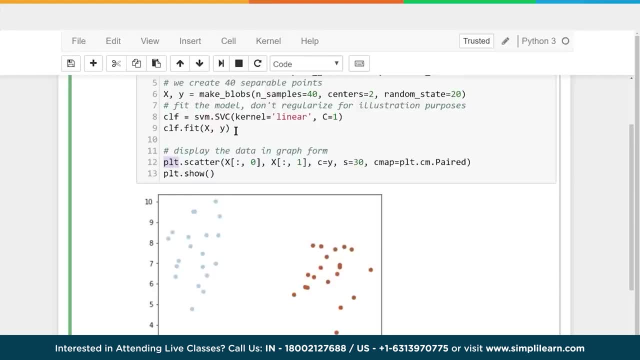 But for this it's not necessary And it's also kind of nice because you can actually see what's going on. And then, if we wanted to, we wanted to actually run a prediction. Let's take a look and see what that looks like. 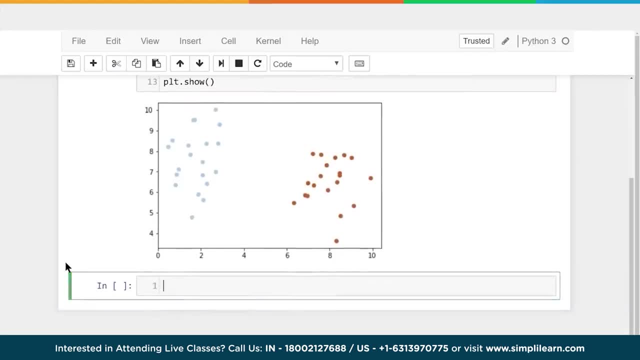 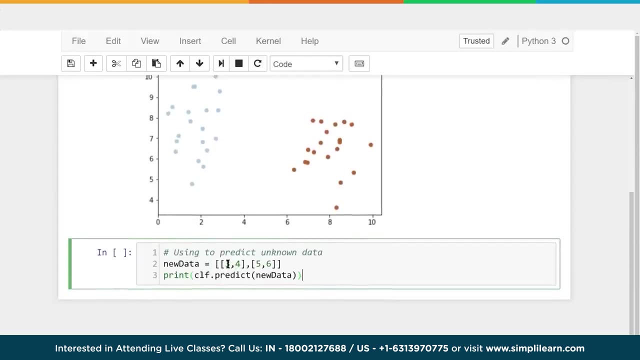 And to predict some new data, and we'll show this again as we get towards the end of digging in deep. You can simply assign your new data. In this case, I am giving it a width and length three, four and a width and length five, six. 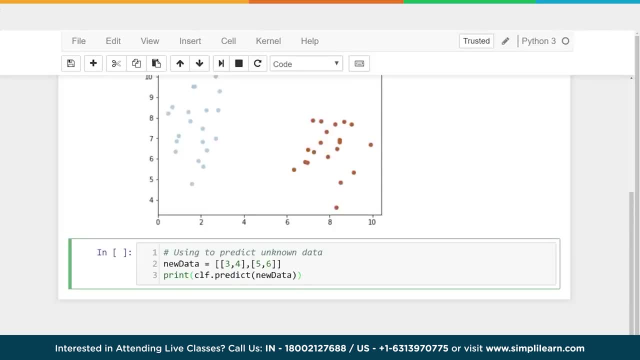 And note that I put the data as a set of brackets and then I have the brackets inside, And the reason I do that is because when we're looking at data, it's designed to process a large amount of data coming in. We don't want to just process one line at a time. 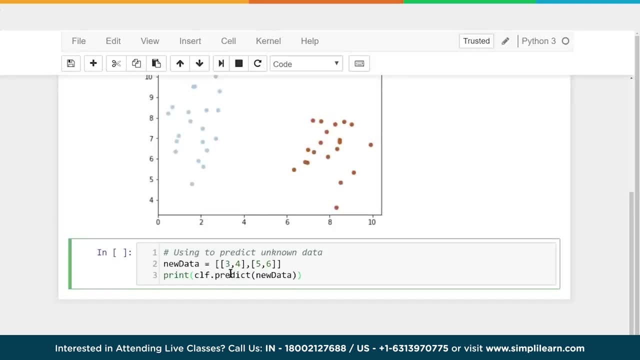 And so in this case I'm processing two lines And then I'm just going to print and you'll see clfpredict new data. So the clf and the predict part is going to give us an answer And let's see what that looks like. 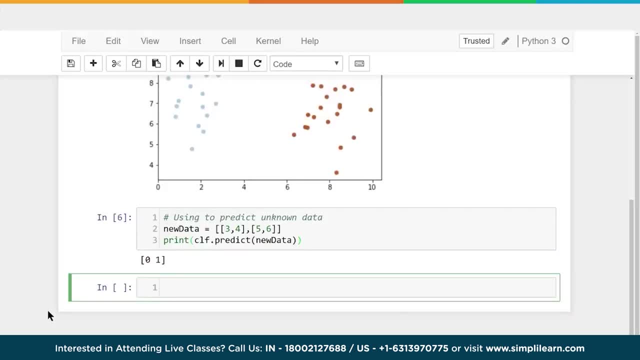 And you'll see zero one. So it predicted the first one. the three, four is going to be on the one side and the five- six is going to be on the other side. So one came out as an alligator and one came out as a crocodile. 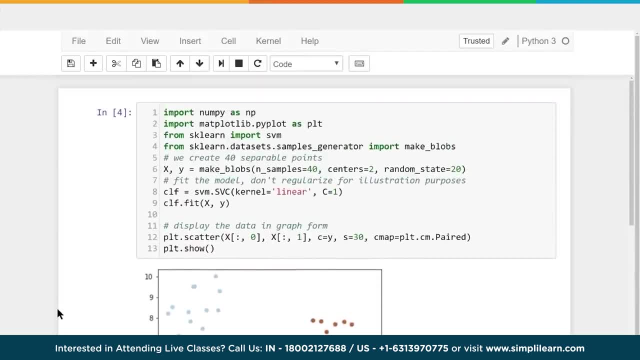 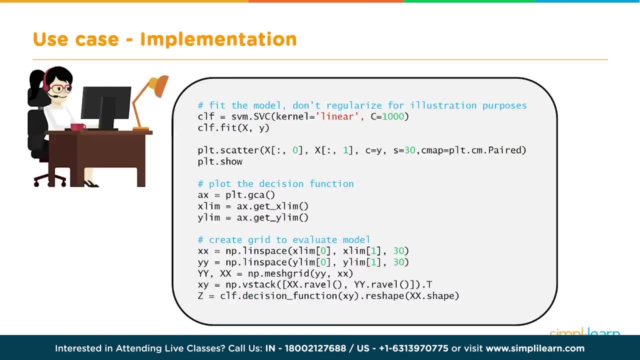 Now, that's a pretty short explanation for this setup, But really we want to dug in and see what is going on behind the scenes And let's see what that looks like. So the next step is to dig in deep and find out what's going on behind the 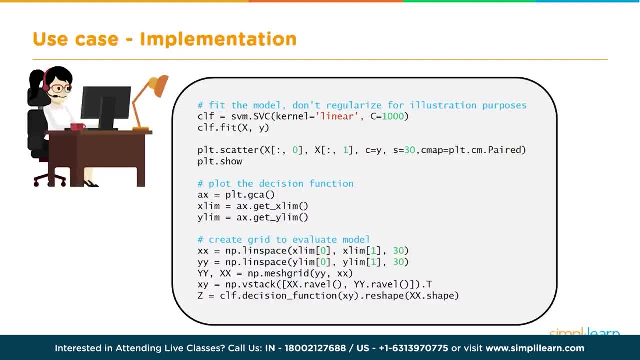 scenes And also put that in a nice pretty graph. We're going to spend more work on this than we did actually generating the original model, And you'll see here that we go through a few steps and I'll move this over to our editor in just. 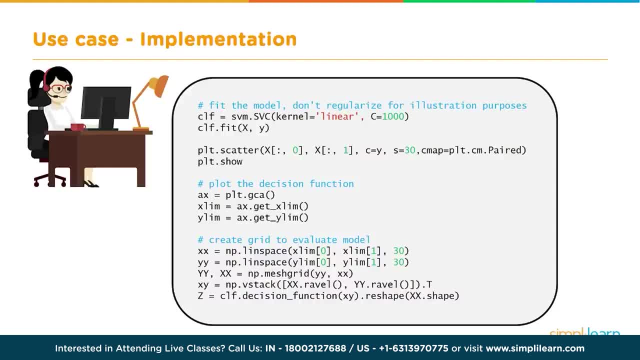 a second. We come in, we create our original data. It's exactly identical to the first part and I'll explain why we redid that and show you how not to redo that. And then we're going to go in there and add in those lines. 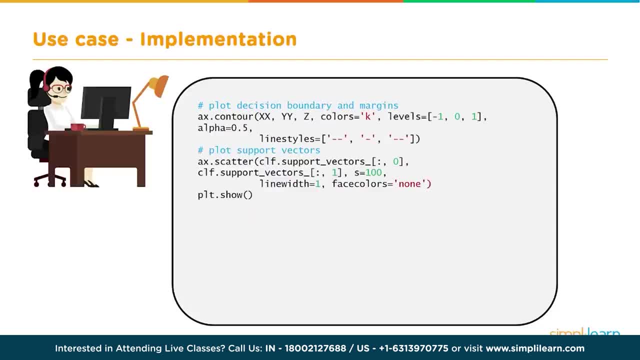 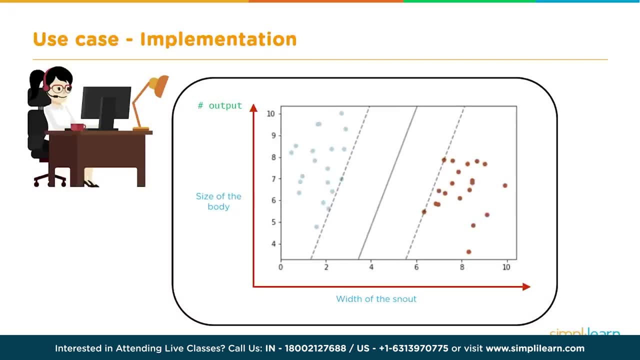 We're going to see what those lines look like and how to set those up And finally, we're going to plot all that on here and show it And you'll get a nice graph with the what we saw earlier when we were going through the theory behind this, where it 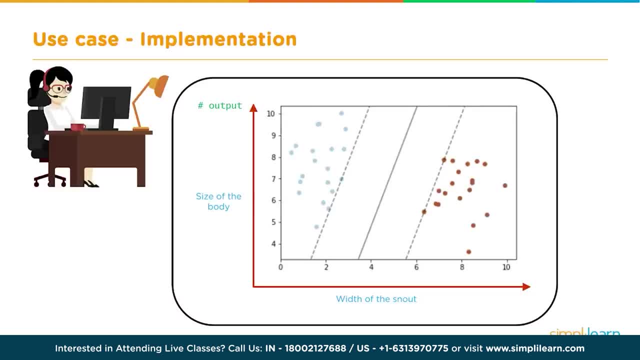 shows the support vectors and the hyperplane And those are done where you can see the support vectors as the dashed lines and the solid line which is the hyperplane. Let's get that into our Jupiter notebook Before I scroll down to a new line. 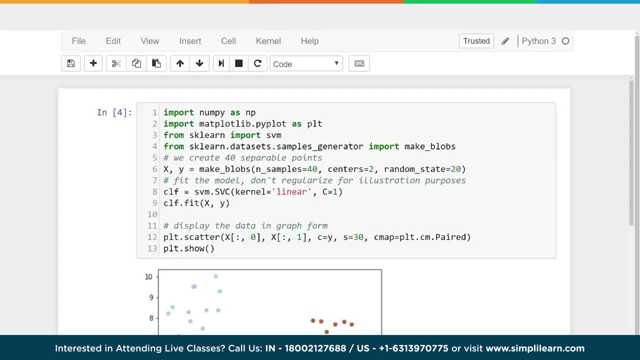 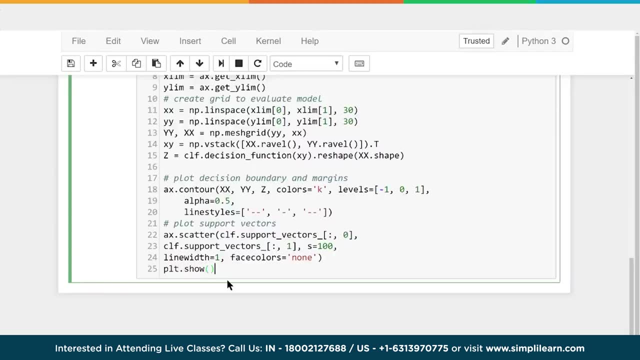 I want you to notice line 13.. It has plot show And we're going to talk about that here. in just a second Let's scroll down to a new line down here and I'm going to paste that code in And you'll see that the plot show has moved. 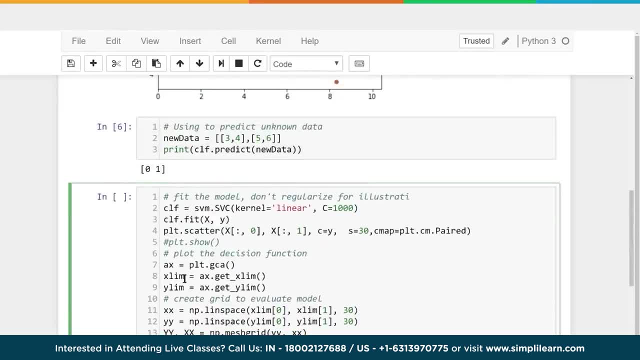 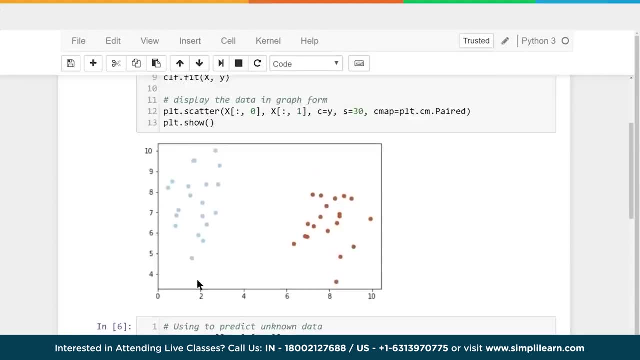 down below. Let's scroll up a little bit and if you look at the top here of our new section, 1,, 2,, 3 and 4 is the same code we had before. Let's go back up here and take a look at that. 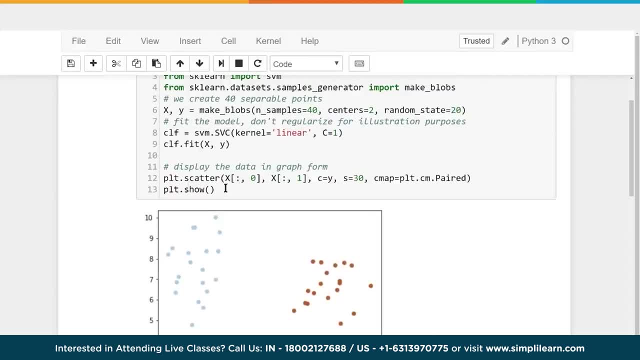 We're going to fit the values in our SVM and then we're going to plot scatter it and then we're going to do a plot show. So you should be asking: why are we redoing the same code? Well, when you do the plot show, 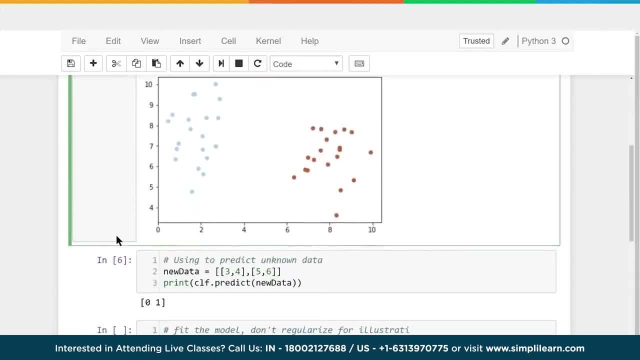 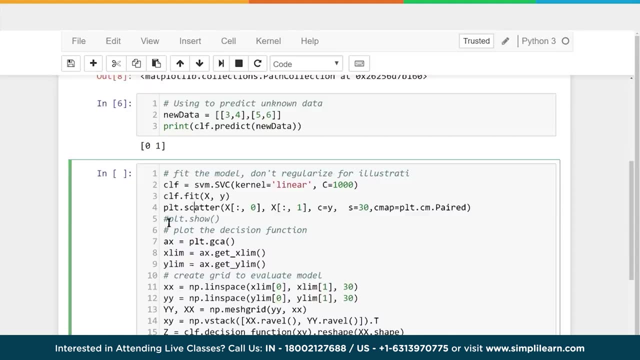 that blanks out what's in the plot. So once I've done this plot show, I have to reload that data. Now we could do this simply by removing it up here, re-running it and then coming down here, and then we wouldn't have to re-run these first four lines of code. 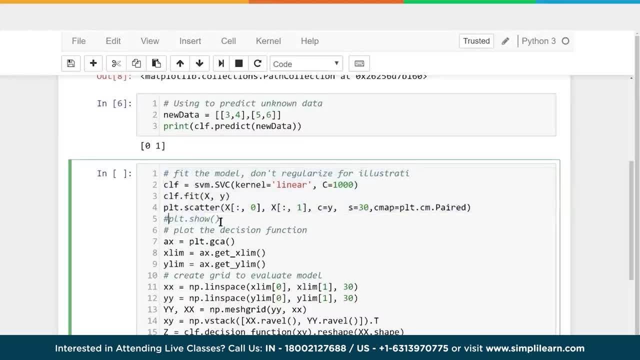 Now in this it doesn't matter too much and you'll see the plot show is down here and then removed right there on line 5.. I'll go ahead and just delete that out of there, because we don't want to blank out our screen. We want to move on to the. 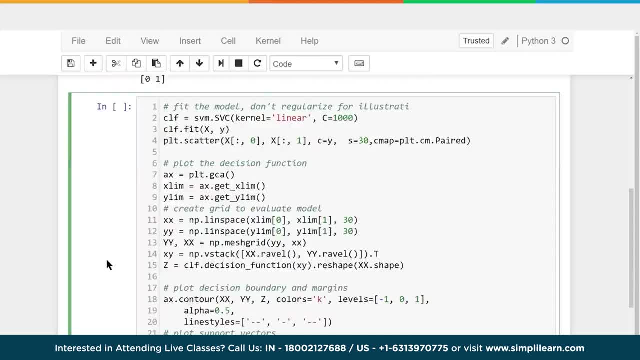 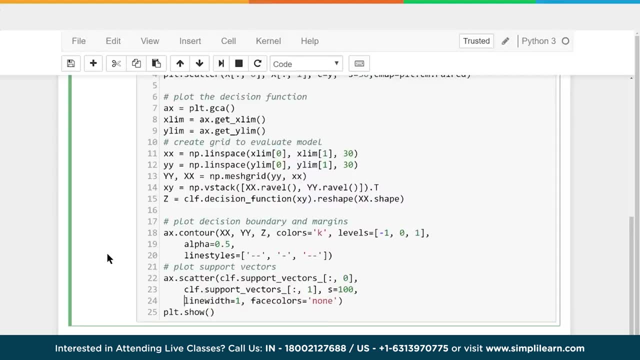 next setup, So we can go ahead and just skip the first four lines, because we did that before. And let's take a look at the AX equals PLT dot GCA. Now, right now, we're actually spending a lot of time just graphing. That's all we're doing here. 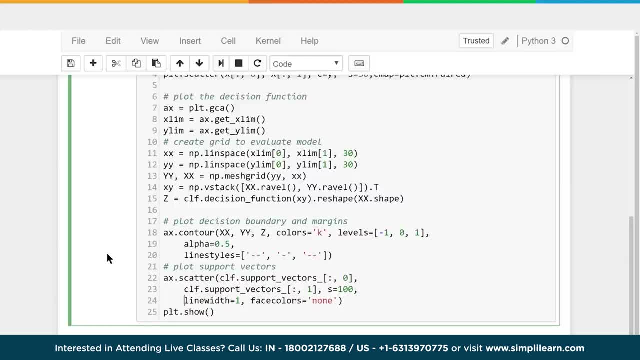 Okay, so this is how we display a nice graph with our results and our data. AX is a very standard used variable. when you're talking about PLT and it's just setting it to that axis, the last axis in the PLT, It can get very confusing. 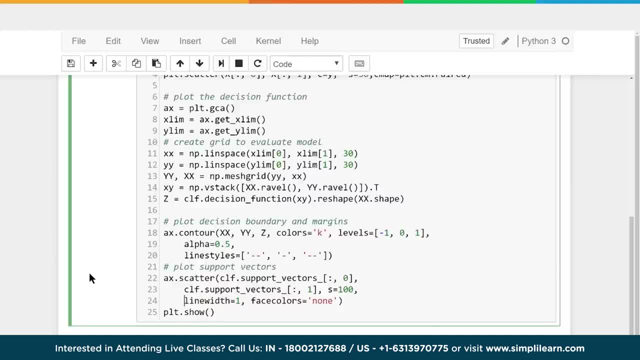 if you're working with many different layers of data on the same graph, and this makes it very easy to reference the AX. So this reference is looking at the PLT that we created and we already mapped out our two blobs on, And then we want to know the limits. 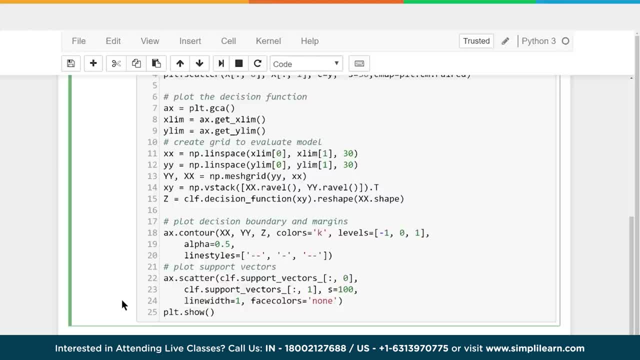 So we want to know how big the graph is. We can find out the X limit and the Y limit simply with the get X limit and get Y limit commands, which is part of our metplot library, And then we're going to create a grid. 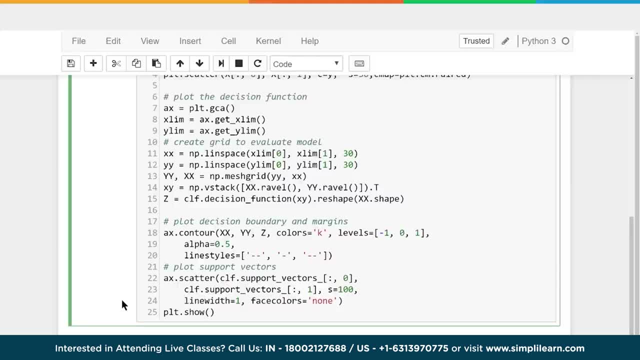 and you'll see down. here we have: we've set the variable XX equal to NP, dot line space, X limit 0, X limit 1, comma 30, and we've done the same thing for the Y space. and then we're going to go in here and we create a mesh. 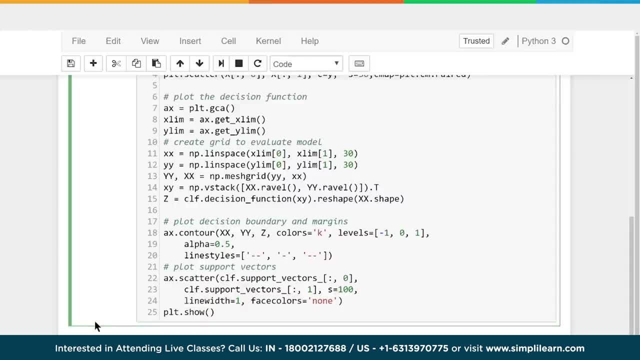 grid and this is a numpy command. so we're back to our numbers, Python. Let's go through what these numpy commands mean. with the line space and the mesh grid, We've taken XX, small s. XX equals NP line space and we have our X limit 0. 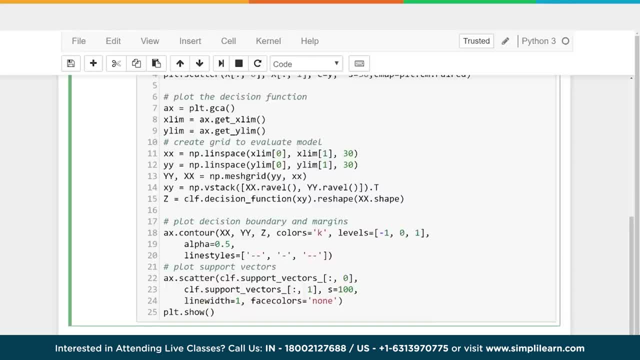 and our X limit 1, and we're going to create 30 points on it, And we're going to do the same thing for the Y axes. Now, this has nothing to do with our evaluation. It's all we're doing is we're creating a grid. 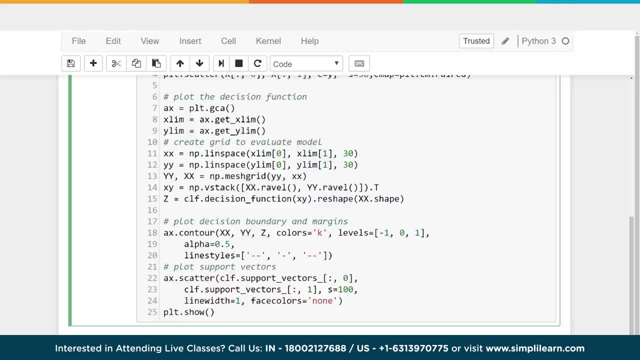 of data, And so we're creating a set of points between 0 and the X limit. We're creating 30 points and the same thing with the Y, and then the mesh grid loops those all together so it forms a nice grid. So if we were 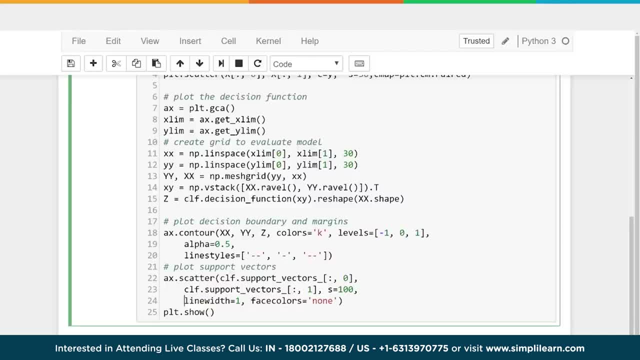 going to do this, say between the limit 0 and 10 and do 10 points. we would have a 0011, 01, 02,, 03, 04 to 10, and so on. You can just imagine a point at each. 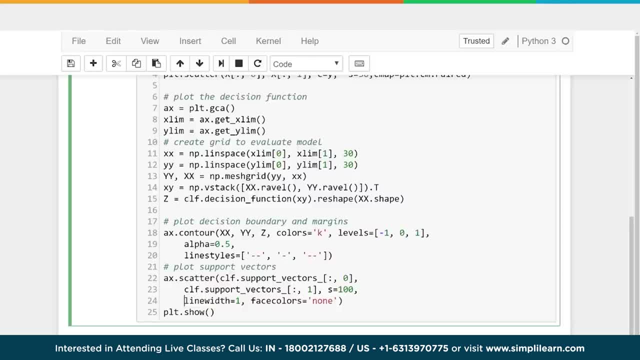 corner of one of those boxes And the mesh grid combines them all. so we take the YY and the XX, we created and creates the full grid And we've set that grid into the YY coordinates and the XX coordinates. Now, remember we're working with Numbi and Python. 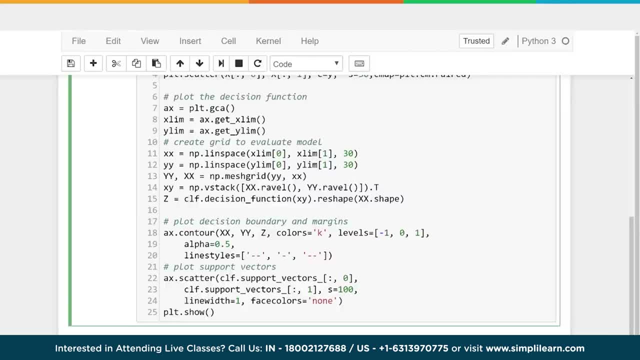 we like to separate those We like to have, instead of it being X comma 1, X comma Y, and then X2 comma Y2, and in the next set of data it would be a column of X's and a column of Y's, And that's. 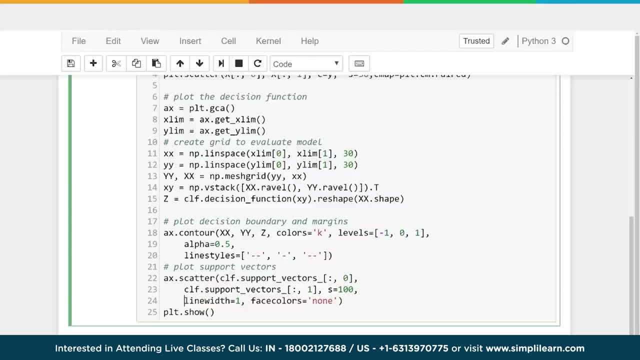 what we have here is we have a column of Y's, and we put it as a capital YY, and a column of X's, capital XX, with all those different points being listed, And finally we get down to the Numbi VStack, Just as. 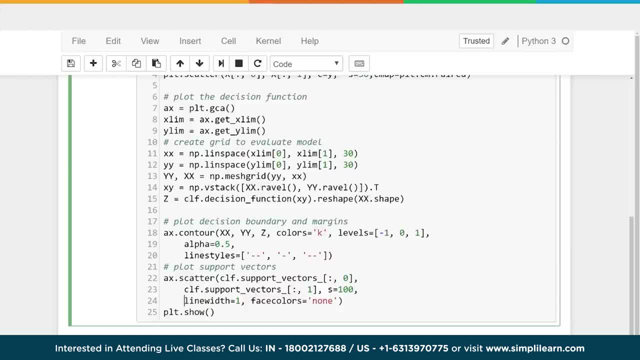 we created those in the mesh grid. we're now going to put them all into one array, XY array. Now that we've created the stack of data points, we're going to do something interesting here. We're going to create a value, Z, and the Z equals. 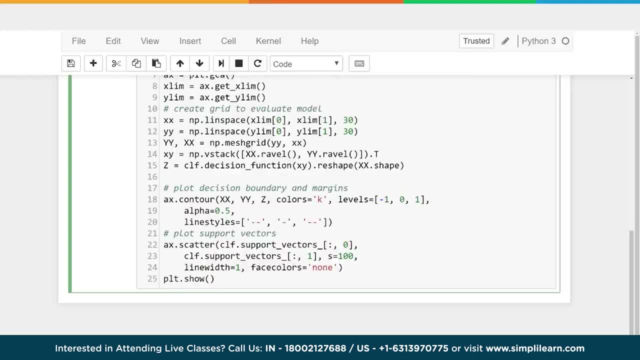 the CLF. that's our support vector machine. we created and we've already trained And we have a dot decision function and we're going to put the XY in there. So here we have all this data. we're going to put that XY in there. 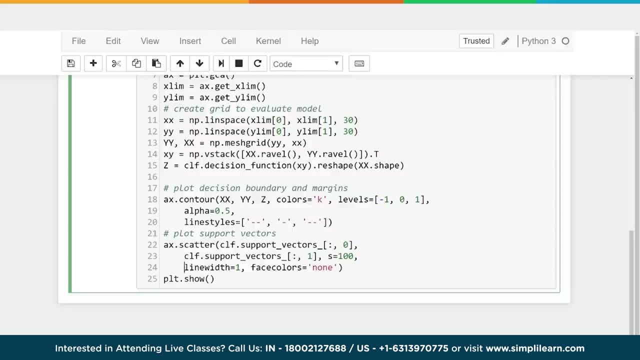 that data and we're going to reshape it And you'll see that we have the XX dot shape in here. This literally takes the XX, resets it up connected to the Y and the Z value, lets us know whether it is the left hand side. it's going to generate three different. 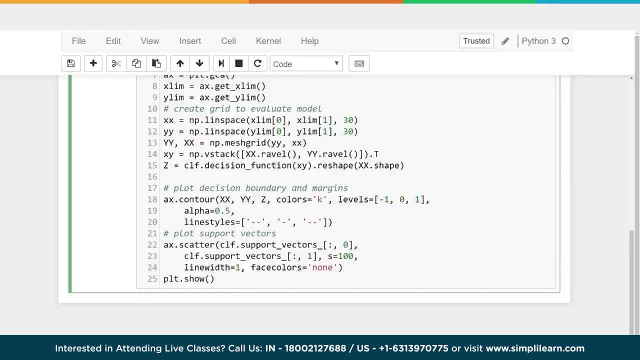 values. the Z value does, And it'll tell us whether that data is a support vector to the left, the hyperplane in the middle or the support vector to the right. So it generates three different values for each of those points, And those points have been reshaped. 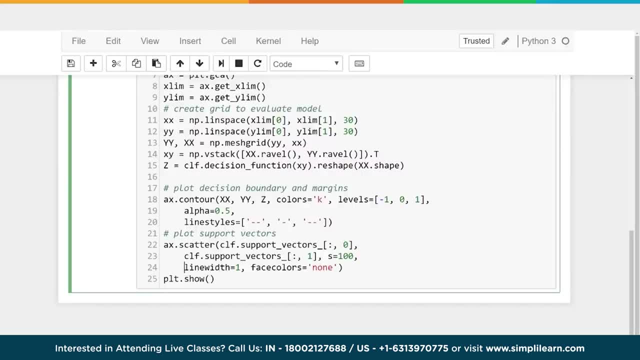 so that they're right on the line, on those three different lines. So we've set all of our data up, we've labeled it to three different areas and we've reshaped it and we've just taken 30 points in each direction. If you do the math, you have. 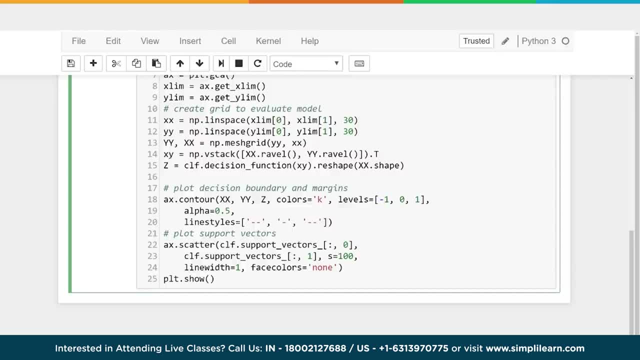 30 times 30, so that's 900 points of data, and we've separated it between the three lines and reshaped it to fit those three lines. We can then go back to our map plot library where we've created the AX and we're going to create a contour. 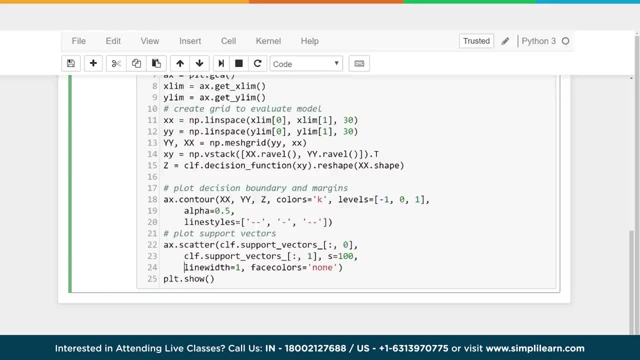 And you'll see here we have contour, capital XX, capital YY. these have been reshaped to fit those lines. Z is the labels. So now we have the three different points with the labels in there and we can set the colors. equals K, And I told you we had three different. 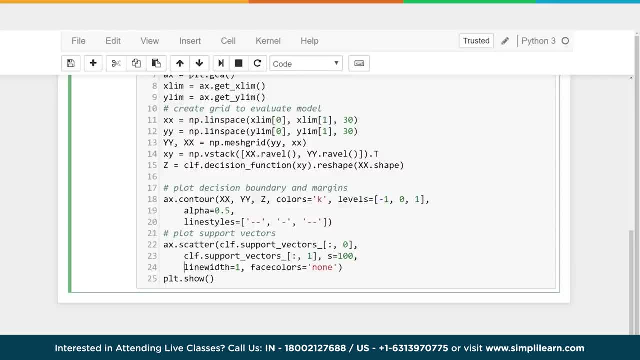 labels. but we have three levels of data. The alpha just makes it kind of see through, So it's only .5 of the value in there. So when we graph it the data will show up from behind it wherever the lines go. And finally the line styles. 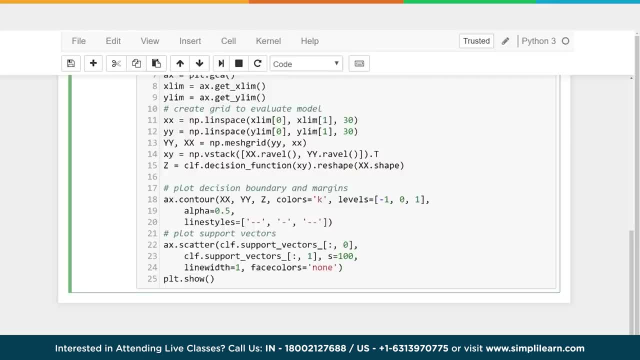 This is where we set the two support vectors to be dash, dash lines, and then a single one is just a straight line. That's what all that setup does. And then, finally, we take our AX dot scatter. We're going to go ahead and plot. 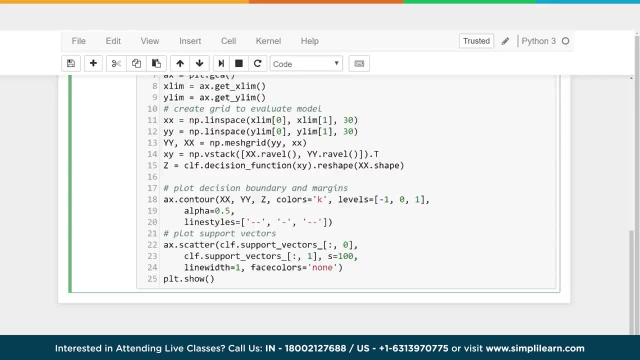 the support vectors, but we've programmed it in there so that they look nice like the dash dash line and the dash line on that grid. And you can see here when we do the CLF dot support vectors. we are looking at column 0 and column 1. 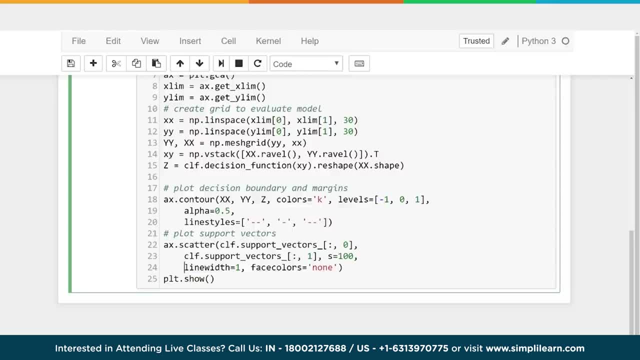 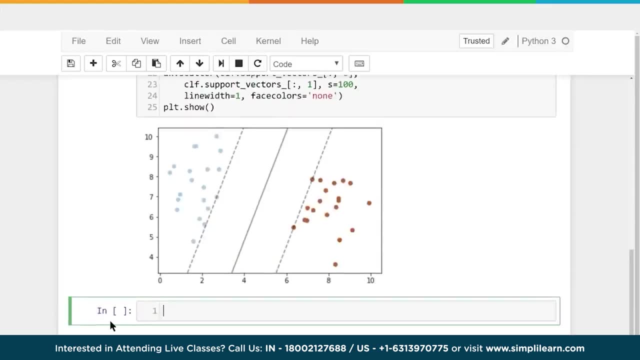 and then again we have: the S equals 100, so we're going to make them larger, and the line width equals 1. face colors equals none. Let's take a look and see what that looks like when we show it And you can see when we get down to our end result. 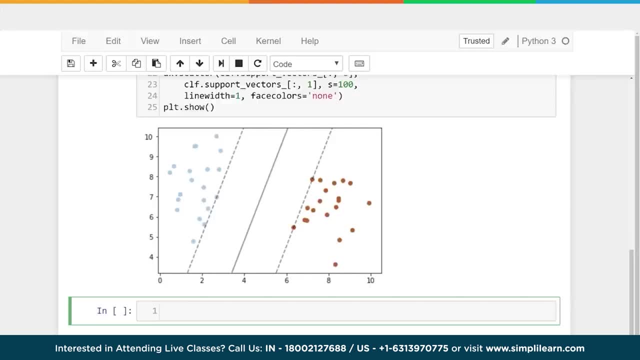 it creates a really nice graph. We have our two support vectors and dash lines, and they have the near data. so you can see those two points, or in this case the four points where those lines nicely cleave the data, and then you have your hyperplane. 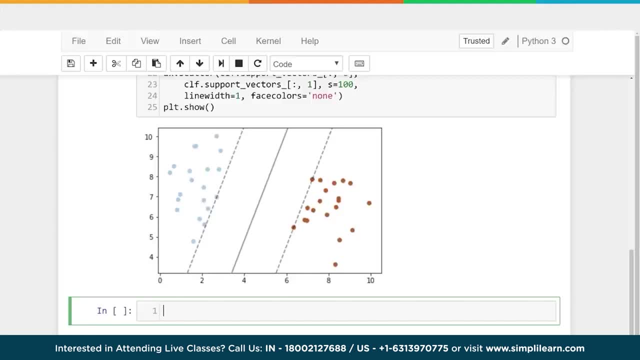 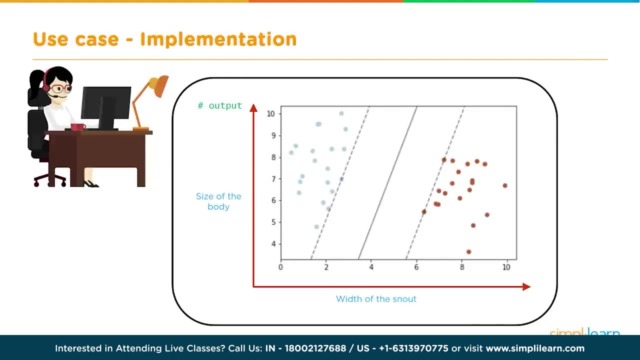 down the middle, which is as far from the two different points as possible, creating the maximum distance. So you can see that we have our nice output for the size of the body and the width of the snout, and we've easily separated the two groups of crocodile and alligator. 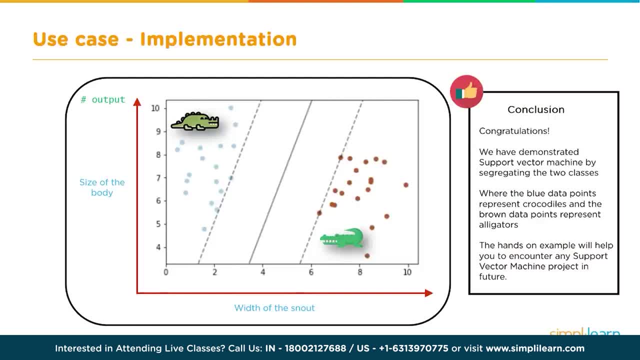 Congratulations, You've done it, We've made it. Of course, these are pretend data for our crocodiles and alligators, but this hands on example will help you to encounter any support vector machine projects in the future and you can see how easy they are to set up. 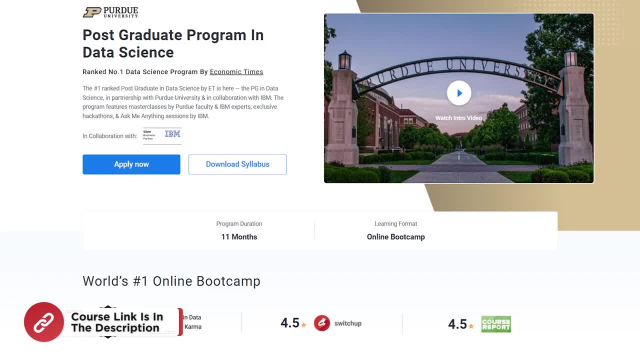 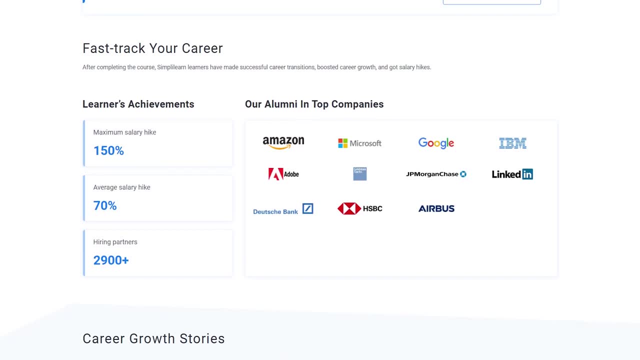 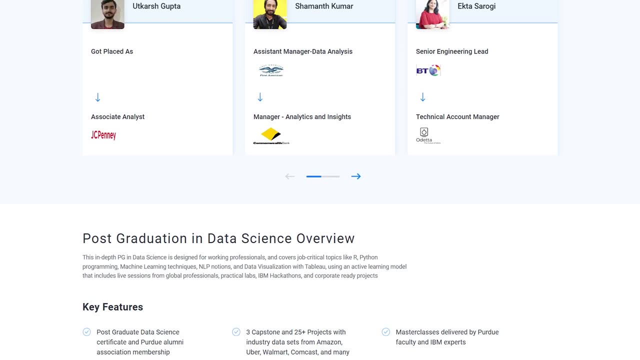 and look at in depth. Try giving Simply Learn's post graduate program in data science a shot. The link in the description box below should navigate you to the home page, where you can find the complete overview of the program being offered. Now over to our training. 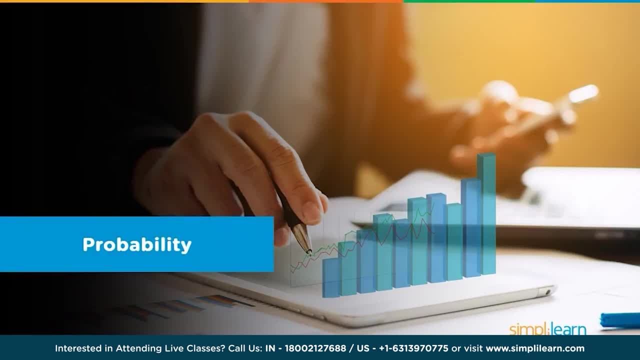 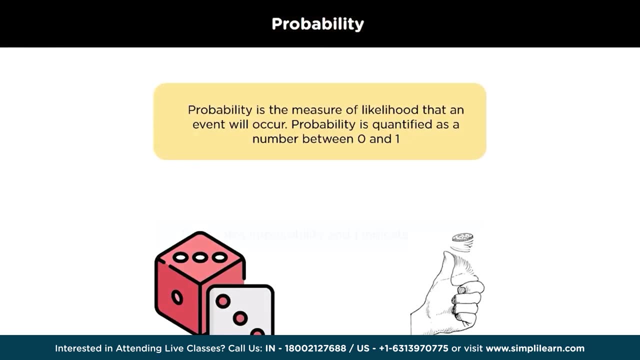 experts. Let's get started. What is probability? Probability is the branch of mathematics concerning numerical descriptions of how likely an event is to occur, or how likely it is that a proposition is true. The probability of an event is a number between 0 and 1.. 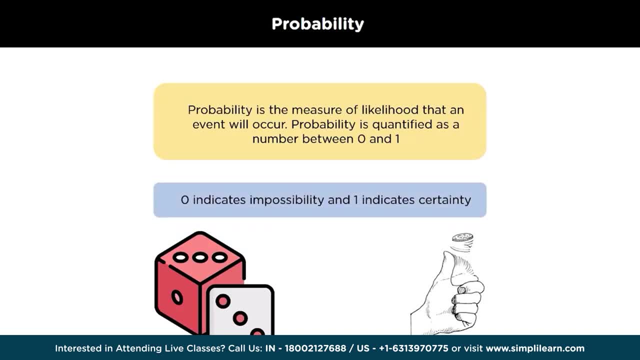 Where, roughly speaking, 0 indicates the impossibility of the event and 1 indicates certainty. The higher the probability of an event, the more likely is that the event will occur. Let's look at an example. A simple example is the tossing of a fair. 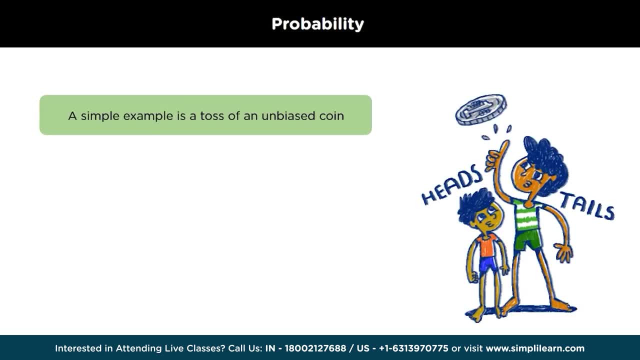 unbiased coin. Since the coin is fair, the outcome- that is, heads and tails- are both equally probable. The probability of heads equals the probability of tails, and since no other outcomes are possible, the probability of either heads or tails can be set to be 1 by 2, which is also 50%. 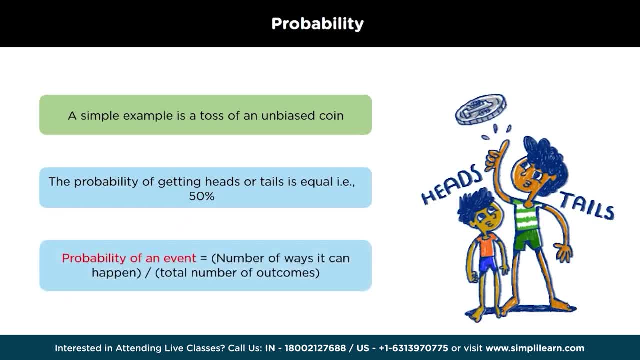 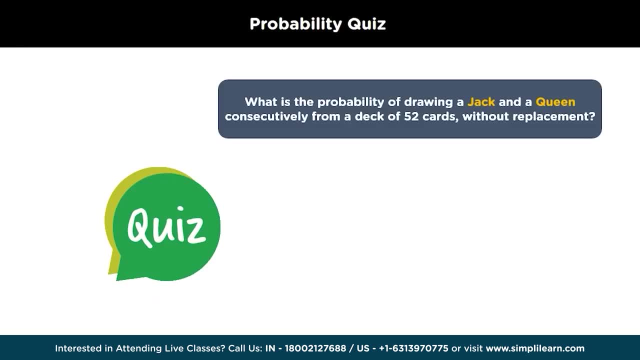 The probability of an event can be calculated by number of ways it can happen, divided by the total number of outcomes. Now that we know about the probability, let's see if you can answer this question: What is the probability of drawing a jack and a queen consecutively? 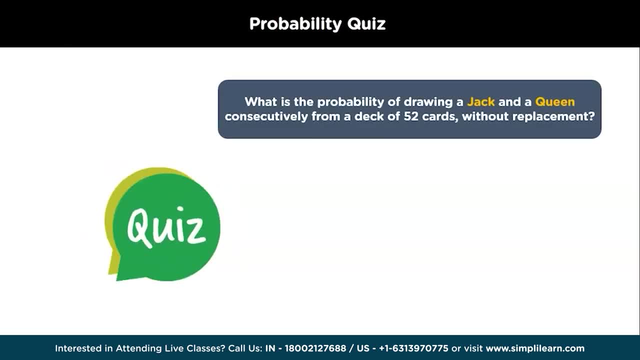 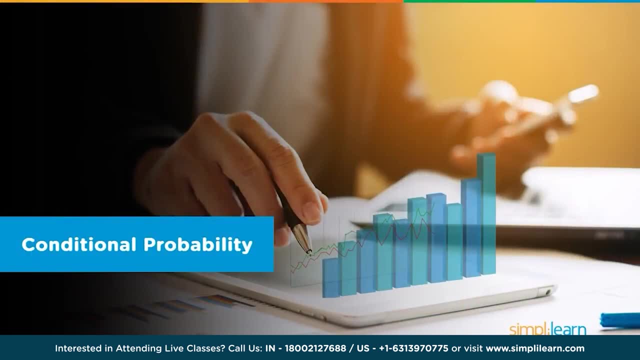 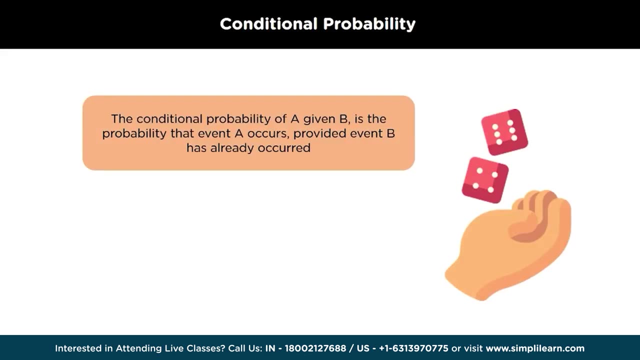 from a deck of 52 cards without replacement. Here are your options. Post your answers in the comment section and let us know. Now let's move on to conditional probability. Let A and B be the two events associated with a random experiment. Then the probability of A's occurrence. 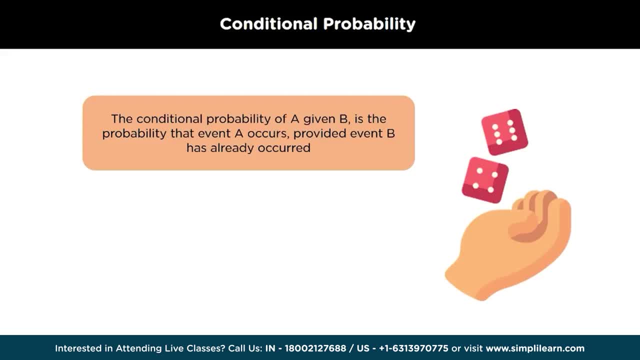 under the condition that B has already occurred and probability of B is not equal to 0, is called the conditional probability. It is denoted by PA slash B. Thus we can say that PA slash B is equal to PA intersection B divided by P of B. 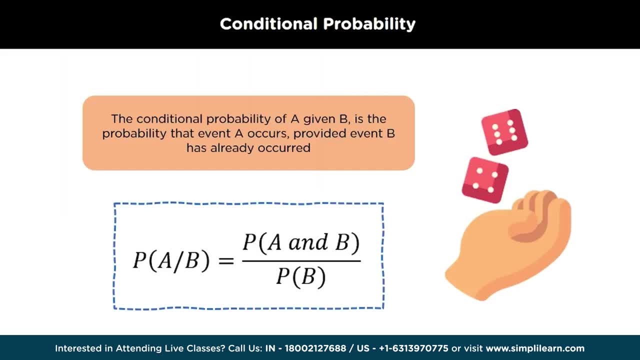 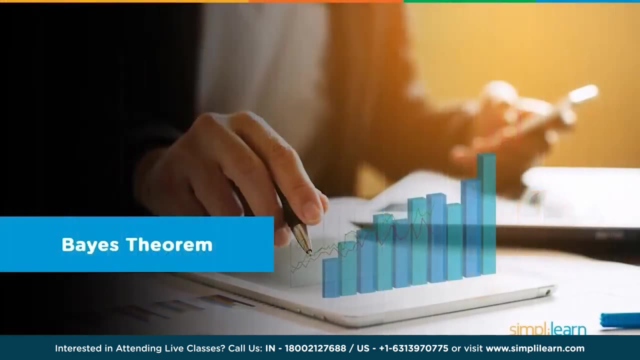 where PA slash, B is the probability of occurrence of A, given that B has already occurred, and PB is the probability of occurrence of B. To know more about conditional probability, you can check our previous video, which is specifically on conditional probability. Now let's move on to 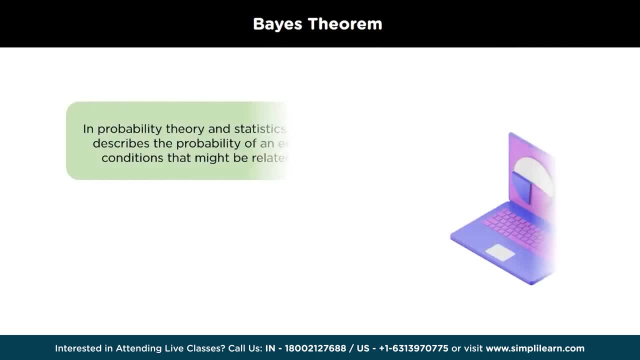 Bayes theorem. The Bayes theorem is the mathematical formula for calculating conditional probability in probability and statistics. In other words, it is used to figure out how likely an event is associated on its proximity to another. Bayes law or Bayes rule are the other names of this theorem. 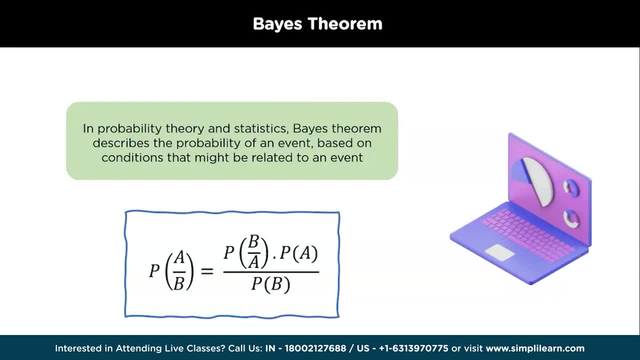 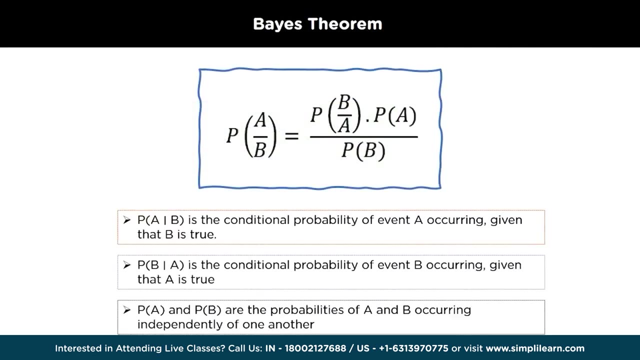 The formula for the Bayes theorem can be written in a variety of ways. The most common version is: PA slash B is equal to P of B, slash A into P of A divided by P of B, where PA slash B is the conditional probability of event A occurring. 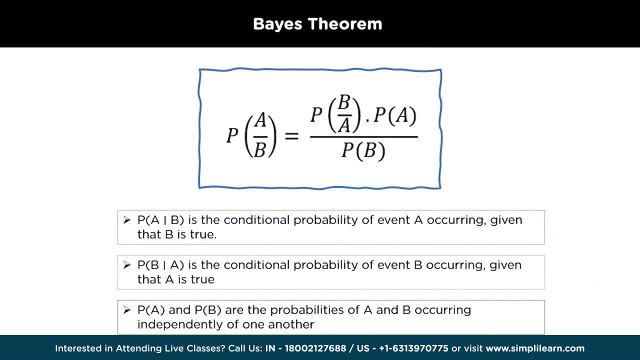 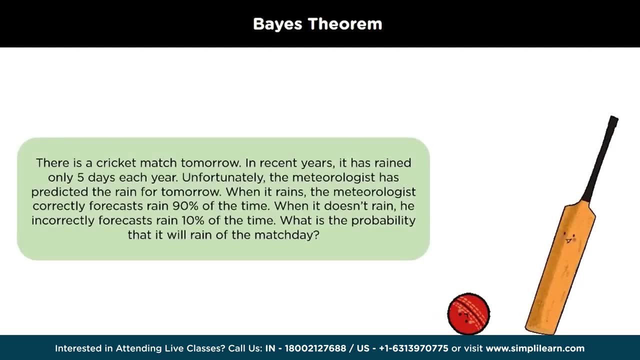 given that B is true and PA and P of B, are the probabilities of A and B occurring independently of one another? Let's solve a problem using the Bayes theorem. to understand it better: There is a cricket match tomorrow, and in recent years it has rained only. 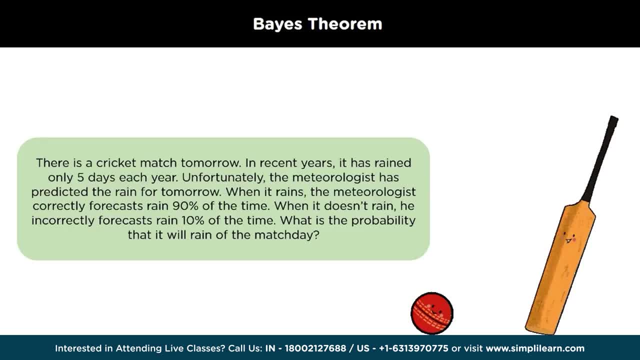 5 days each year. Unfortunately, the meteorologist has predicted the rain for tomorrow. Now, when it rains, the meteorologist correctly forecasts rain 90% of the time, and when it doesn't rain, he incorrectly forecasts rain 10% of the time. 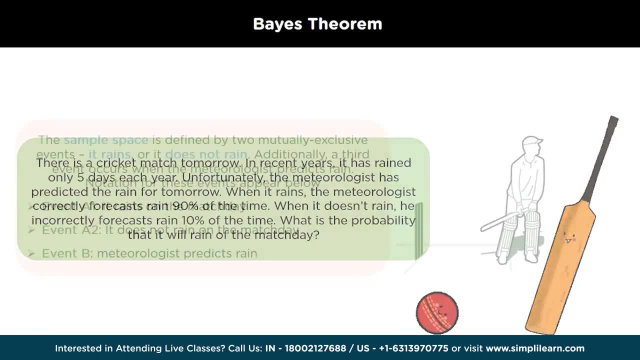 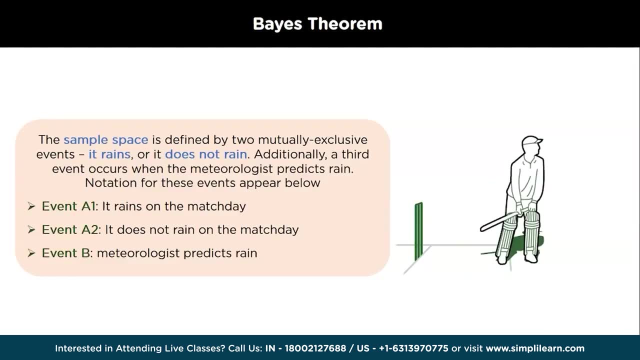 Let's calculate what is the probability that it will rain on the match day. So the two sample spaces here are the events that it rains and it does not rain. Additionally, a third event is also there: that meteorologist predicts the rain. So the notation for these events: 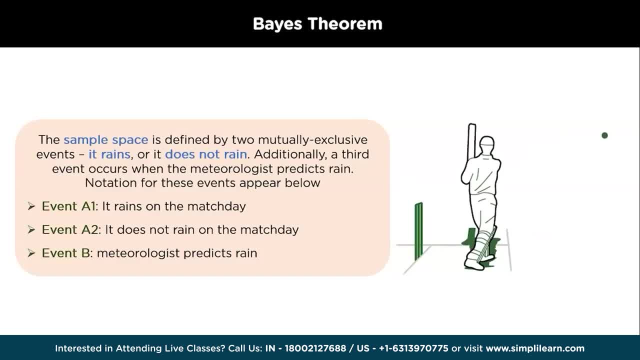 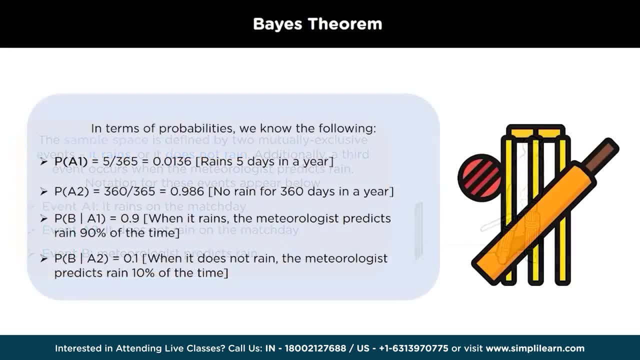 appear below: Event A1 is equal to it rains on the match day, event A2 that it does not rain on the match day. and event B is the meteorologist predicting the rain. Now, in terms of probability, we know the following: Probability of A1. 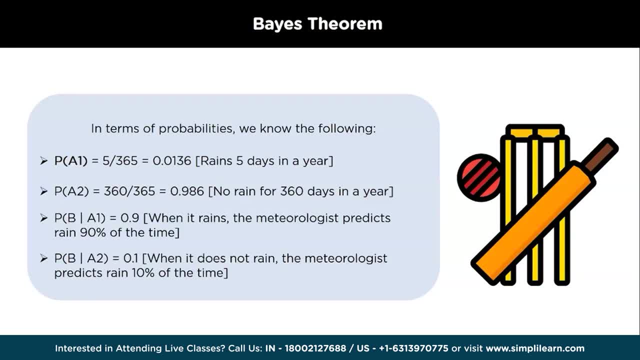 is 5 by 365, that it rains 5 days in a year, which will come out to be 0.0136.. PA2 is 360 by 365. that is no days for 360 days in a year, which will come out to be. 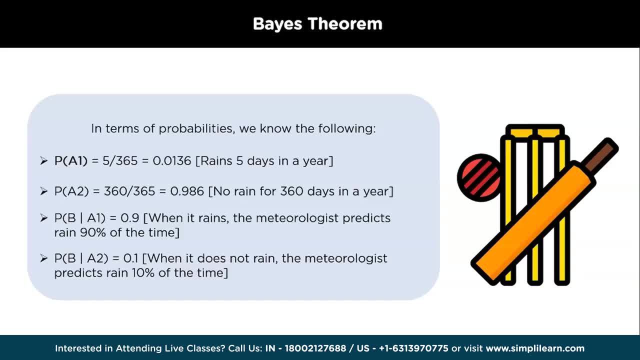 0.986.. PB slash A1 is 0.9.. This signifies when it rains, the meteorologist predicts the rain 90% of the time. In a similar manner, PBYA2 is 0.1. that it does. 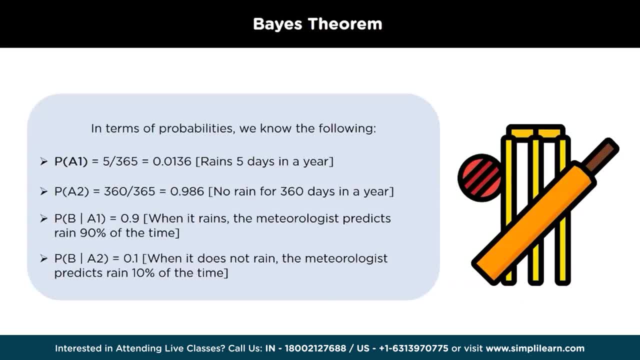 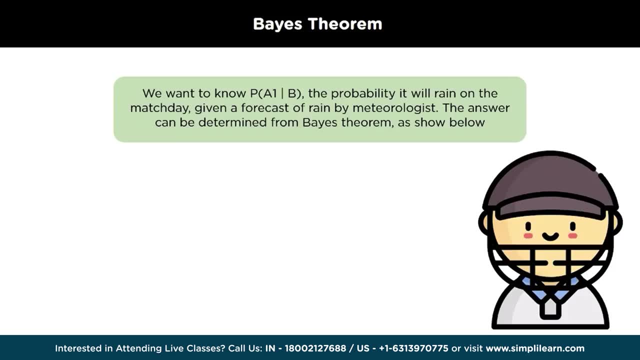 not rain. the meteorologist predicts the rain 10% of the time. Combining all this we can calculate PA1 slash B. that is the probability it will rain on the given match day. given a forecast of rain by meteorologist, The answer can be determined. 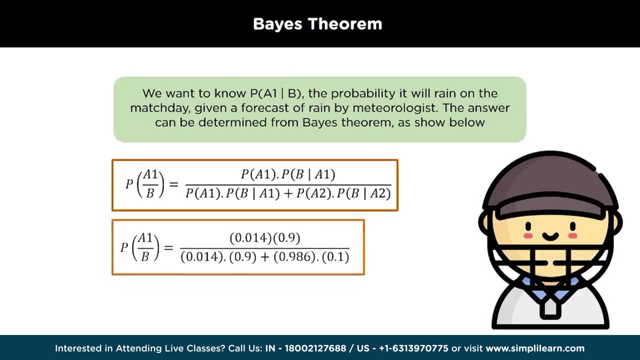 using the Bayes theorem as shown below. So here is the formula of the Bayes theorem and, putting all the values that we have calculated in the previous slide, the probability that it will rain on the match day, given a forecast of the rain by meteorologist. 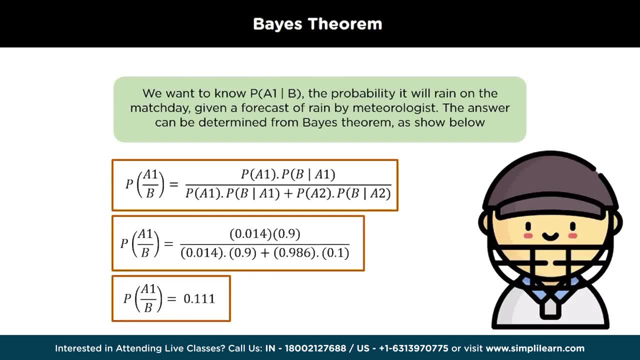 will come out to be 0.111, which will be equal to 11.11%. So there is an 11% chance that it will rain on the match day, given that the meteorologist has predicted the rain. I hope this example is clear to you. So what is? 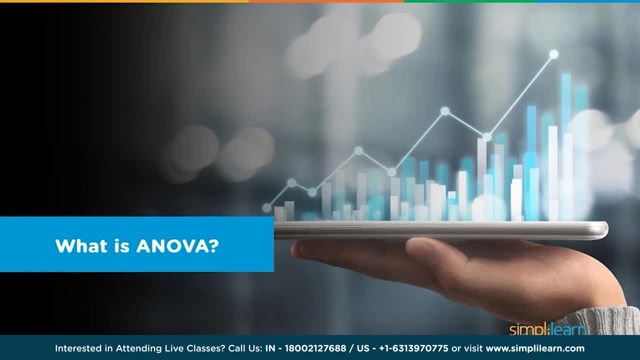 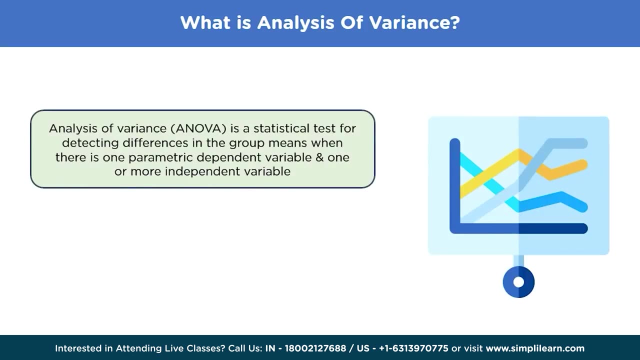 analysis of variance. ANOVA is to test the differences among the means of the population by examining the amount of variation within each sample relative to the amount of variation between the samples. This technique was invented by R A Fisher and is thus often referred to as 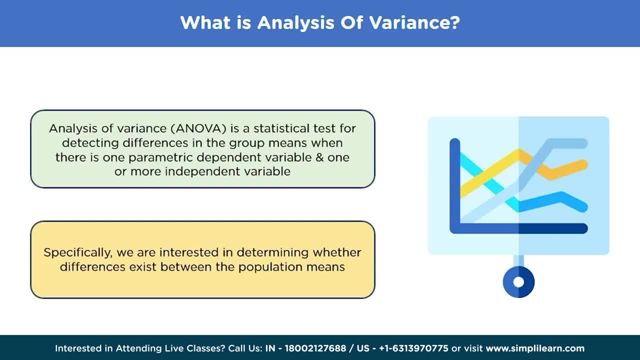 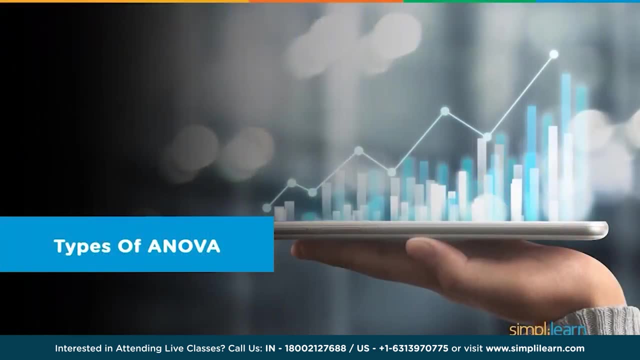 Fisher's ANOVA Analyzing the variance tests the hypothesis that the means of two or more populations are equal. In a regression study, analysts used the ANOVA test to determine the impact of independent variables on the dependent variable. So what are its types? 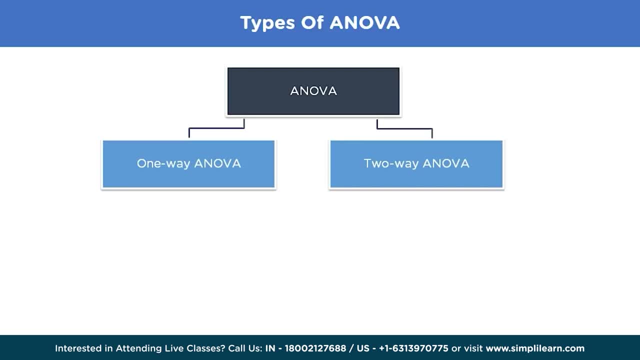 There are basically two types of ANOVA, which is a one-way ANOVA and a two-way ANOVA. When we are comparing more than three groups based on one factor variable, then it is said to be a one-way analysis of variance. 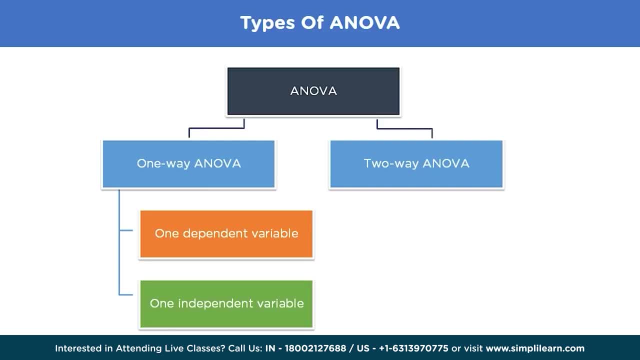 For example, if we want to compare whether or not mean output of three workers is the same, based on the working hours of the three workers, we will use a one-way ANOVA. Now let's move on to two-way ANOVA. 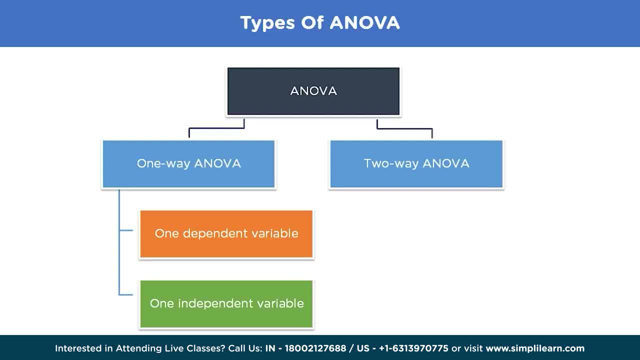 When factor variables are more than two, then it is said to be a two-way analysis of variance. For example, based on working conditions and working hours, we can compare whether or not the mean output of three workers is the same. Now let's 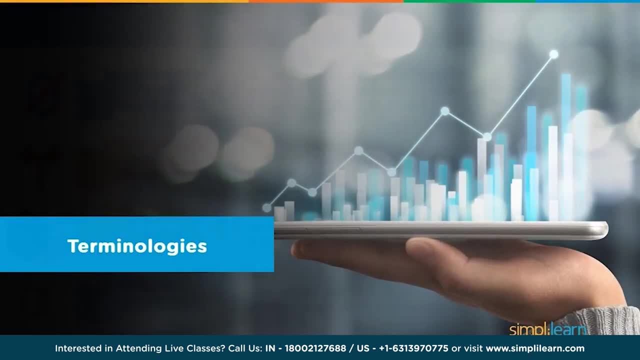 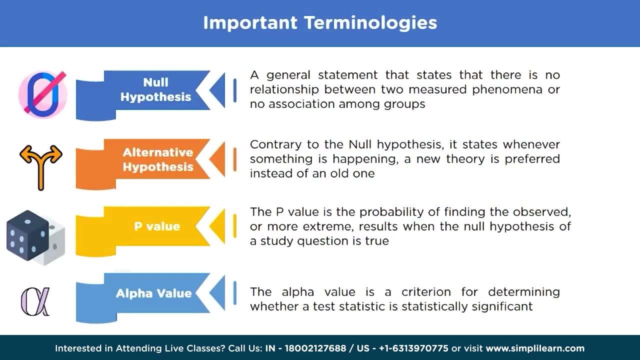 discuss some key terminologies used in ANOVA. We will start with the null hypothesis. The null hypothesis is the assumption that an event will not occur. A null hypothesis has no bearing on the study's outcome unless it is rejected. Alternative hypothesis: The alternative hypothesis. 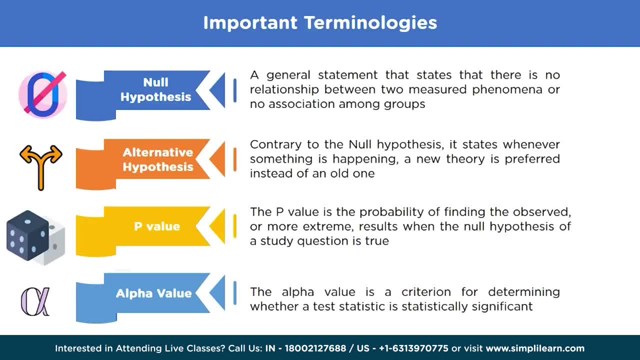 is the logical opposite of the null hypothesis. The acceptance of the alternative hypothesis follows the rejection of the null hypothesis. H1 is the symbol for it, P-value. In statistics, the P-value, also called probability value, is the probability measure of finding. 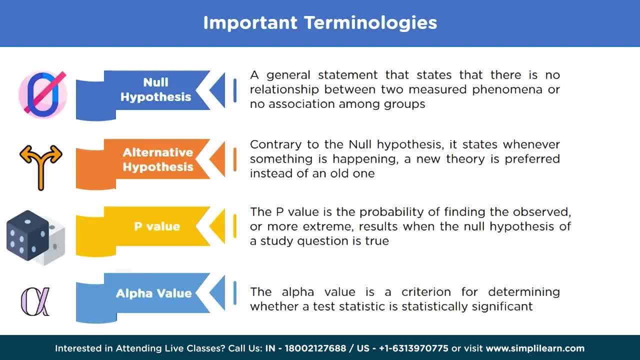 observed, or more extreme results when the null hypothesis of a given statistical test is true. The P-value is the primary value used to quantify the statistical significance of the result of a hypothesis test. Now let's move on to alpha-value. The alpha-value is the criteria for determining. 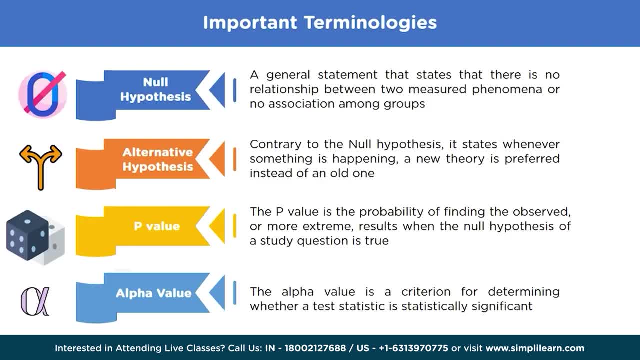 whether a test's statistics is statistically significant or not. This test provides the P-value, which is the probability of observing results as extreme as those in the data, assuming the results are truly due to chance alone- An alpha-value of 5% or lower. 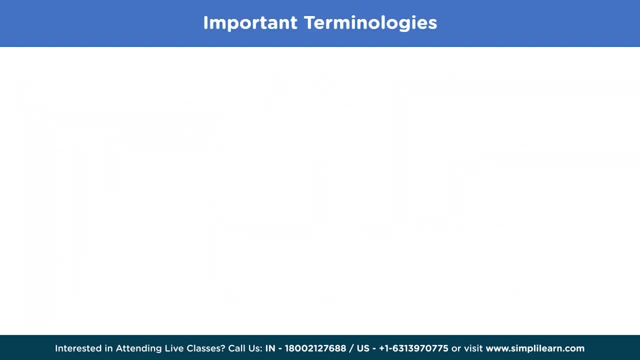 is often considered to be statistically significant. Now let's try to understand these terminologies by taking an example. Let's assume that a new drug is developed with the goal of lowering the blood pressure more than the existing drug. So in this case, a null hypothesis. 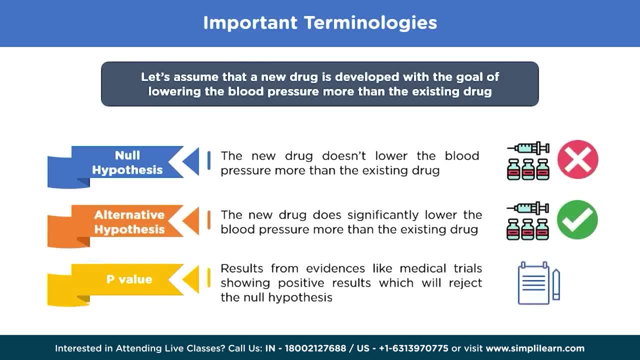 will be that a new drug doesn't lower the blood pressure more than the existing drug. The alternative hypothesis will be that a new drug does significantly lower the blood pressure more than the existing drug And the P-value will be the results from evidence like medical trials showing the positive results. 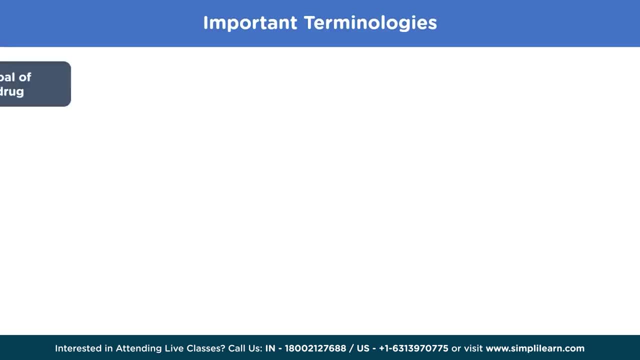 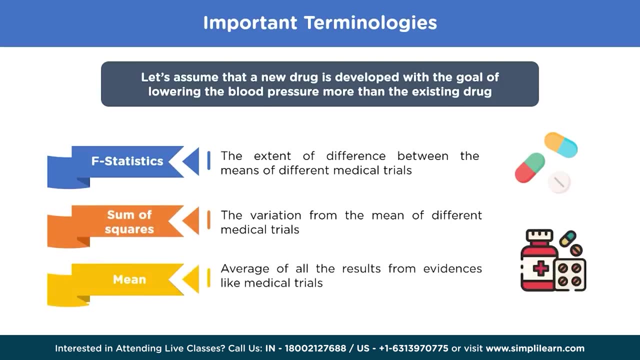 which will reject the null hypothesis. The S-statistic will be the extent of difference between the means of different medical trials. The sum of squares will be the variation from the mean of different medical trials, And the mean will be the average of all the results. 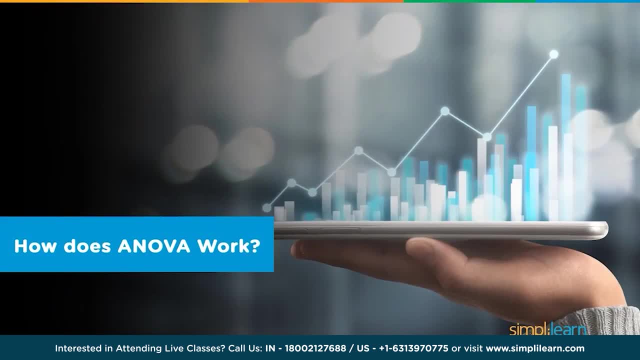 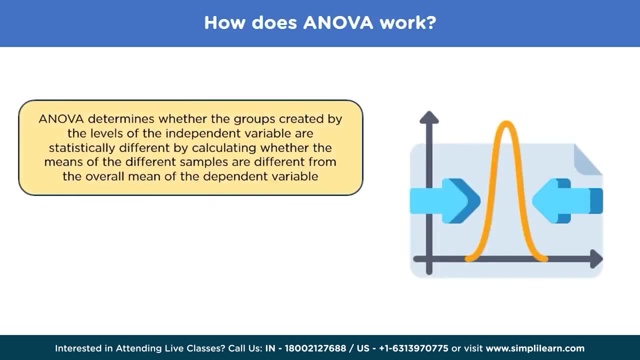 from evidence, like medical trials. Now let's understand the co-concept between how the ANOVA works. The one-way ANOVA compares the means between the groups you are interested in and determines whether any of those means are statistically significant or different from each other. 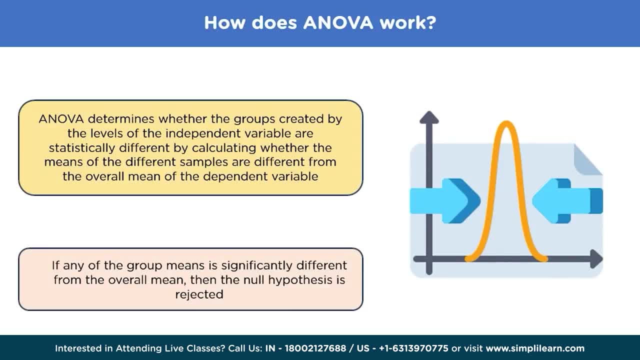 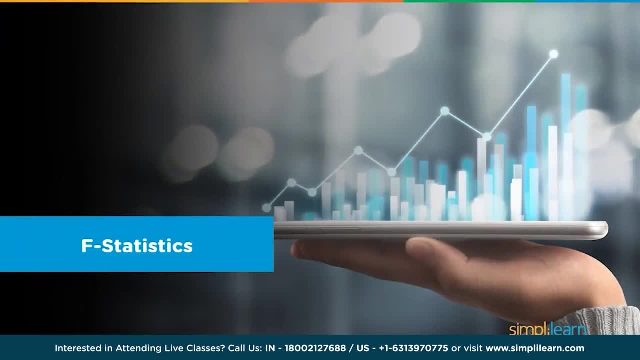 Specifically, it tests the null hypothesis. If any of the group means is significantly different from the overall mean, then the null hypothesis in this case will be rejected. Now let's discuss the term F-statistics, which is very much used in the analysis of variance. 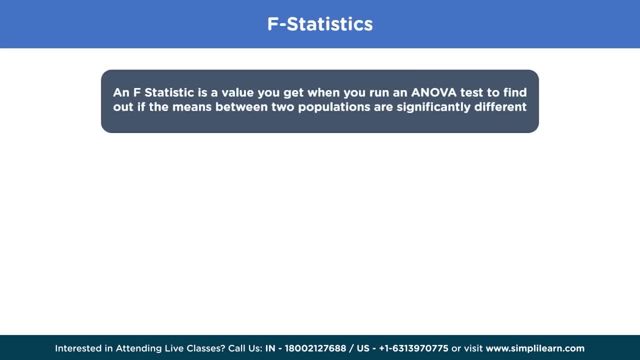 F-statistics, or F-ratio, is a statistical measure that tells us about the extent of difference between the means of different samples. Lower the F-ratio, the closer are the samples to the means. If there are three different data sets, then this part will be the 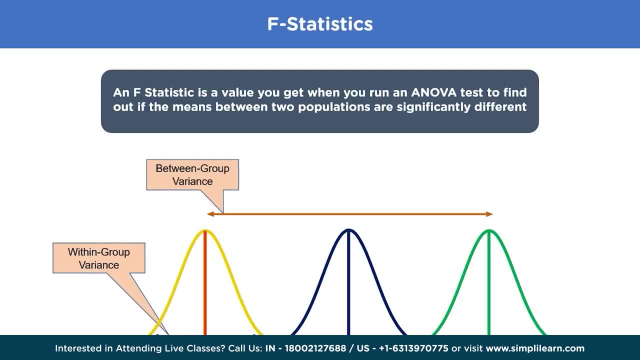 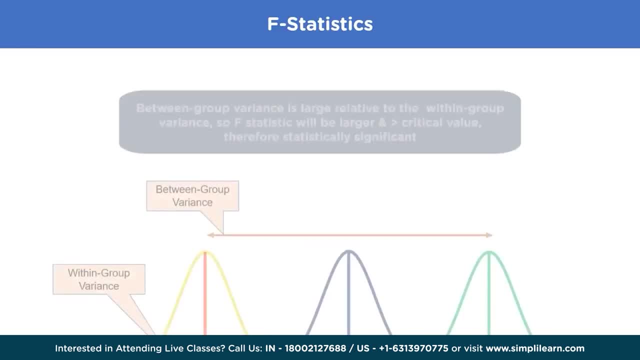 within-group variance, that is, the variance between the samples. This line will be the variance between the means of the different samples, which is also called between-group variance. If the between-group variance is large relative to the within-group variance, the F-statistic will be comparatively. 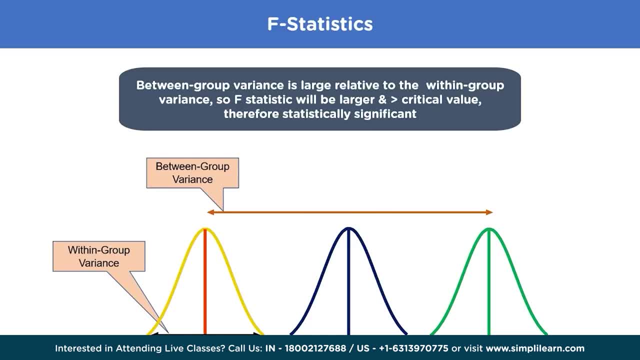 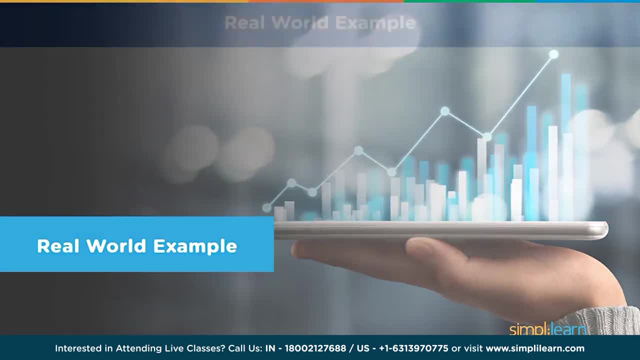 large to the critical value and therefore will be statistically significant. Now that we have covered almost all the theory regarding the ANOVA, let's try to understand how this is used. as a real-world example, Suppose you are a marketing manager of the product company. Your team has 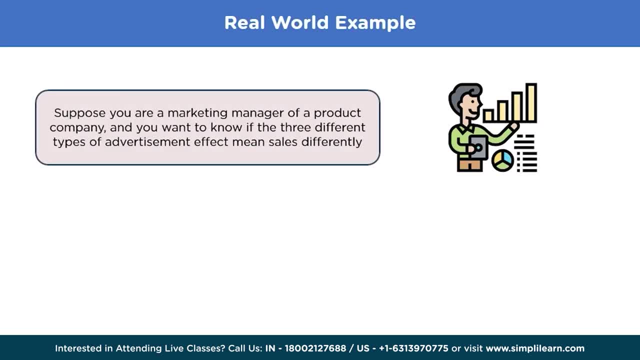 recently launched three new advertisements and you want to know if the three different types of advertisements affect means sales differently. So how can you do that? You will use each type of advertisements at 20 different stores for one month and then measure the total sales of each store. 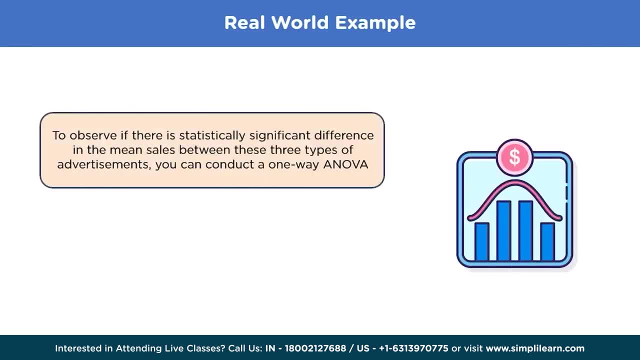 for a month To observe if there is statistically significant differences in the means sales between these three types of advertisements, you will conduct a one-way ANOVA. For calculating the ANOVA, you will use the type of advertisement as a factor and the sales as a response. 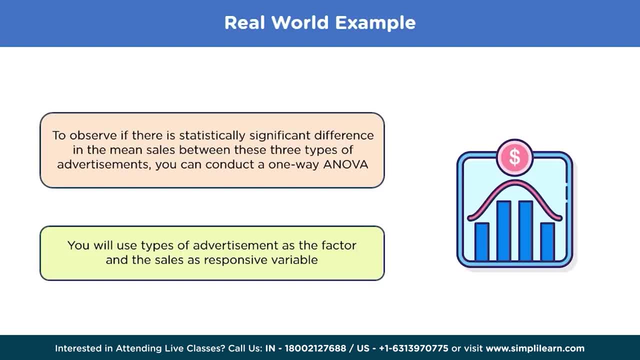 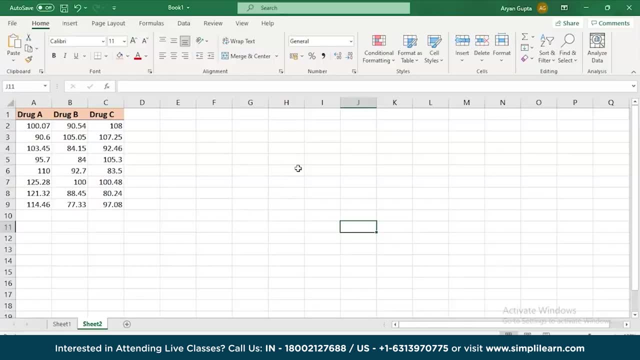 variable. Now that we have covered all the topics in ANOVA and have understood how it is used in a real-world example, let's see how you can run an ANOVA test in Excel. Suppose you are a research scientist and you want to perform clinical trials. 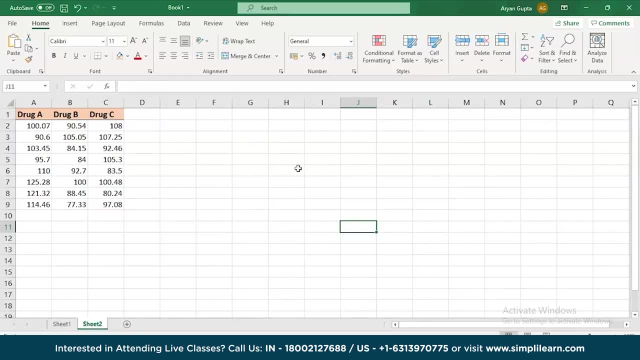 to study the effectiveness of three drugs developed by three healthcare companies to cure a certain disease. The data below represents the time taken to cure the disease for different patients when they consume either drug A, B or C. The time is represented in terms of total hours and minutes. 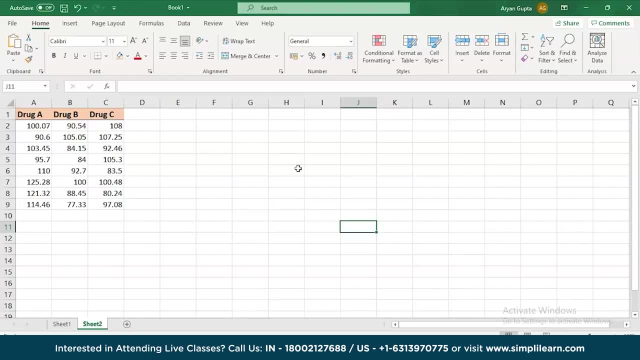 At the 0.05 level of significance. that is the alpha value. we need to test whether the mean time for the three drugs to cure the disease are equal. So how you can do that. We will first move on to the data tab. 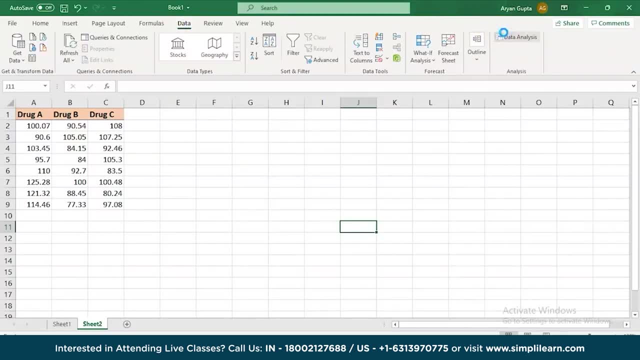 and then click data analysis. We will select the ANOVA single factor and click OK. Now it is asking for an input range. Select the data you have on the table. We have the labels in our first row and the alpha is 0.05.. 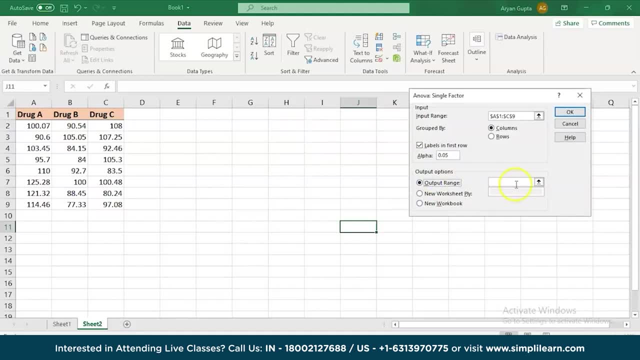 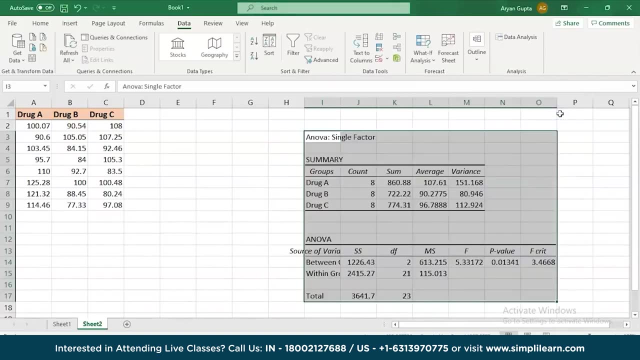 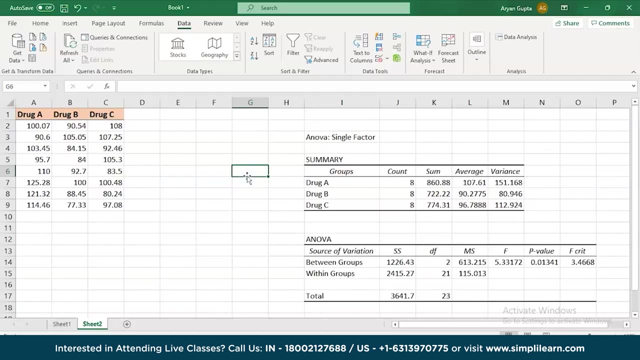 For the output range. we will get the output here on the same page. So we will select some cell in the same page and we will click OK. So you can see we have our analysis of variance table with the summary. Let's understand each term one by one. 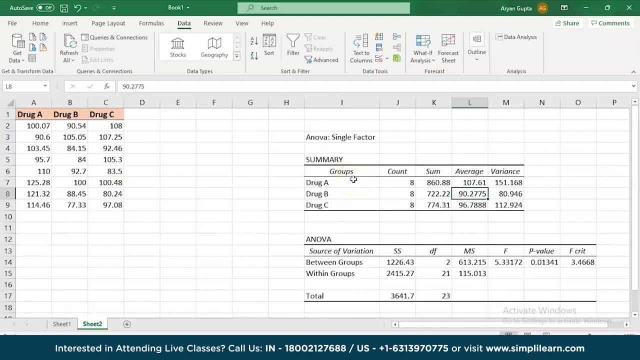 The average time taken to cure the disease after consumption of three drugs are 107,, 90 and 96 hours approximately. The difference between the largest and the smallest mean is 17.47.. Here, one significant observation is that the F value is. 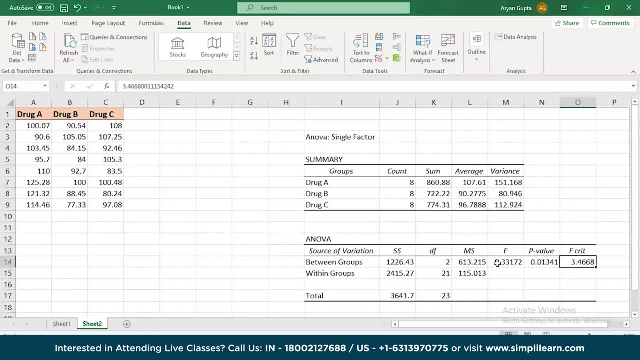 greater than F critical value. So this means we can reject the null hypothesis. It also means that the average time taken to cure the disease is not the same for all the three drugs. Using the paired comparison, we can conclude that the time taken by the drug 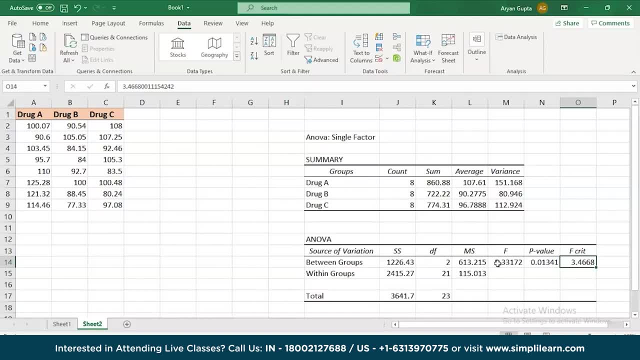 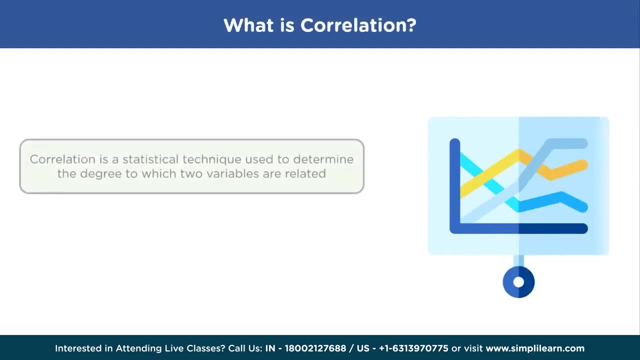 A to cure the disease is more than time taken by drug C and with further is more time taken by drug B to cure the disease. What is correlation? Correlation refers to a statistical relationship between the two entities. It measures the extent to which the two variables 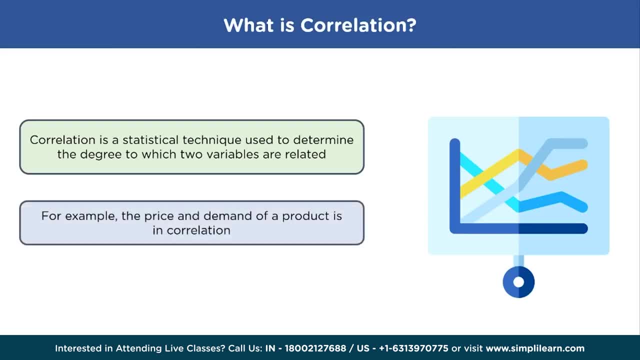 are linearly related. For example, the price and demand of a product is in correlation. They are linearly related. The value of correlation always lies between minus one to plus one. There are mainly two types of correlation. The first one is positive correlation. 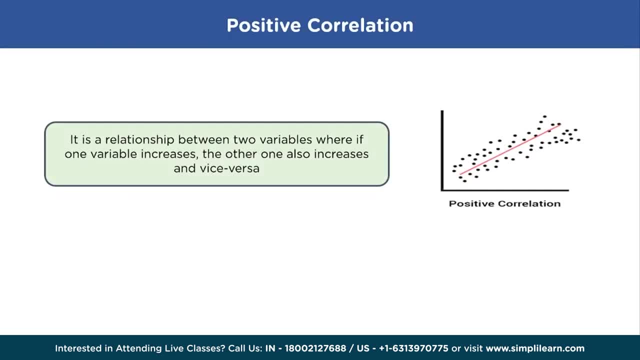 A positive correlation means that the linear relationship is positive and the two variables increases or decreases in the same direction. The number of trees cut down and the probability of erosion are in correlation. When one increases, other also increases, and vice versa. Negative correlation: A negative correlation is just 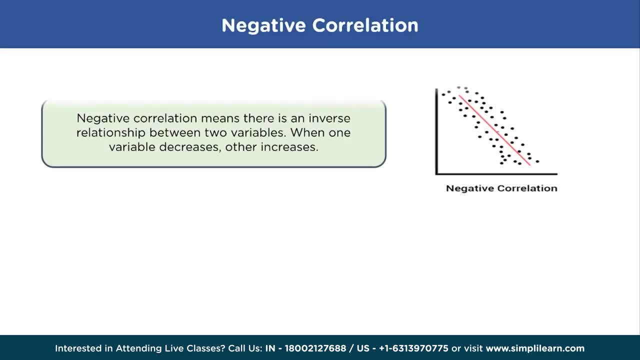 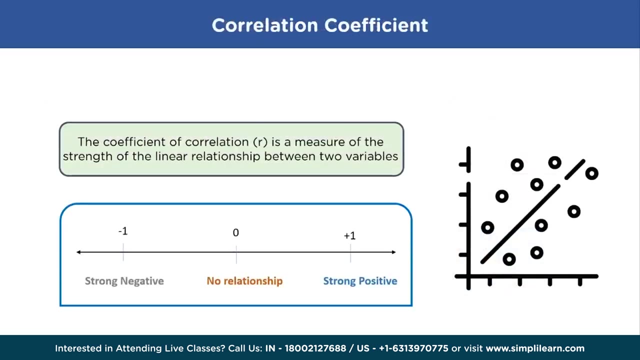 the opposite. The relationship line has a negative slope and the variables change in opposite directions. For example, if you decrease the speed of the car, the time taken to reach the destination increases. This is a negative correlation Correlation coefficient. The correlation coefficient. 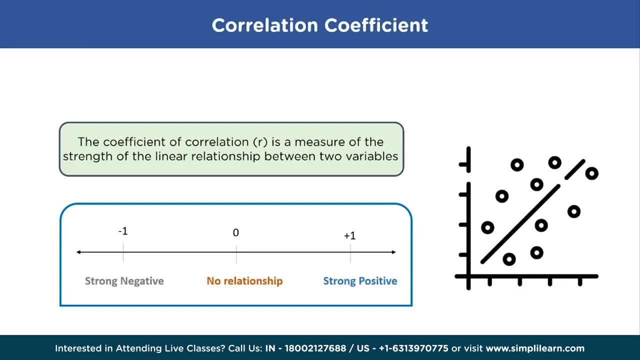 which is denoted by R, gives us the measure of the strength of the linear relationship between the two variables. Correlation coefficient is denoted by the letter R, and it ranges from minus one to plus one. If it is less than zero, it implies that there is a negative correlation. 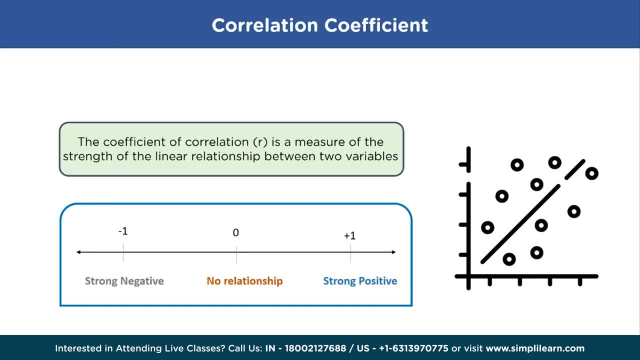 The minus one indicates there is a strong negative correlation between the variables. If R is greater than zero, it implies there is a positive correlation. and plus one is the strongest point of a positive correlation. When R is equal to zero, we can say that there is no correlation. 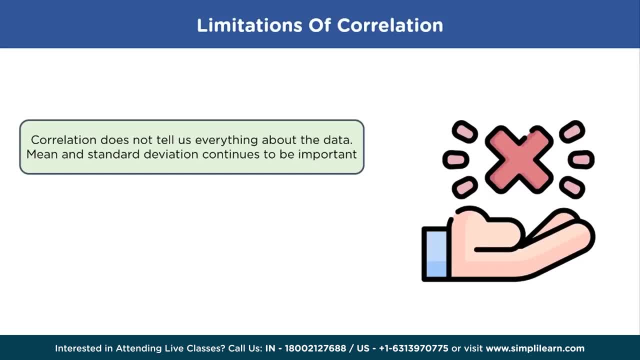 between the variables. There are also some limitations of correlation. Correlation coefficient does not give you every insight on the data. Mean and standard deviation are still the important parameters to get the insight of a data. The second one is the data will not produce a straight line. 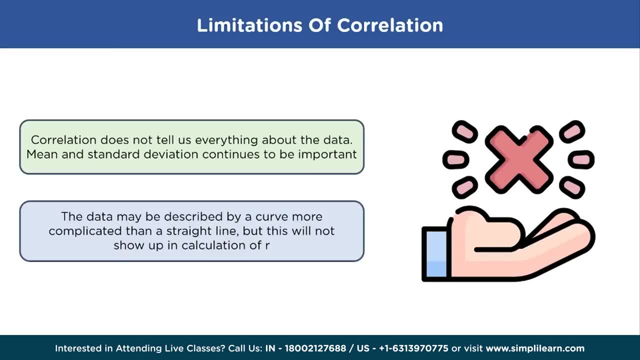 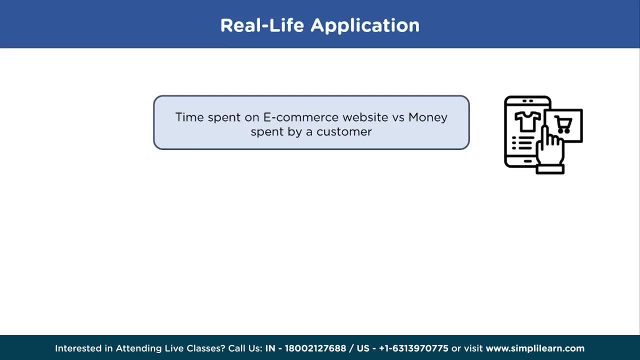 every time and it will be difficult to predict the value of R just with the straight line or the slope of the graph. Now let's see some real-life applications of correlation. If you take any e-commerce company whose website is accessed by millions of users, 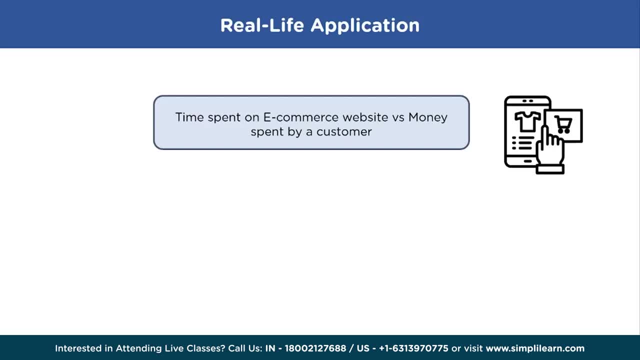 and their time was spent by the customer and the respective money spent by the customer. We can also predict the unique users that visited the website and how it affected the sales in a day. The third application can be the patient blood pressure and the medication used. 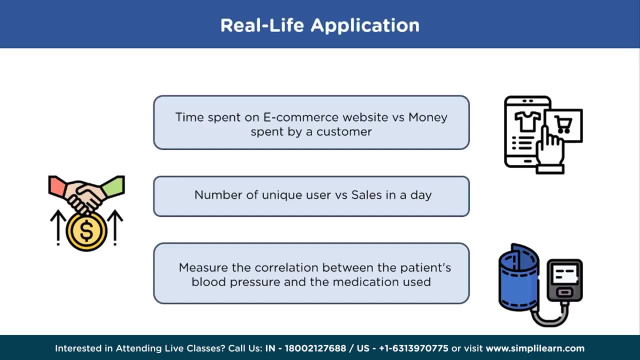 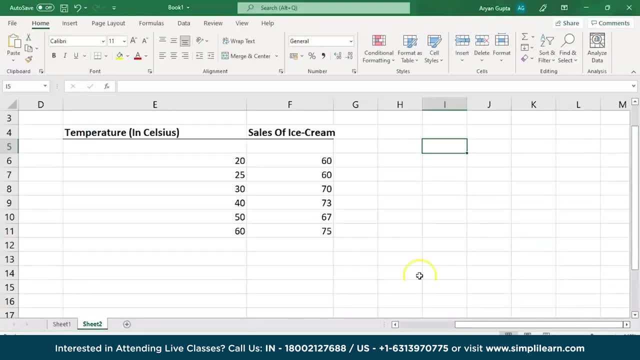 The level of patient blood pressure and the effect of medication on it can be in a correlation. Now let's jump on to Excel workbook to see how you can calculate the correlation coefficient. So here we are on the Excel workbook, If you see. 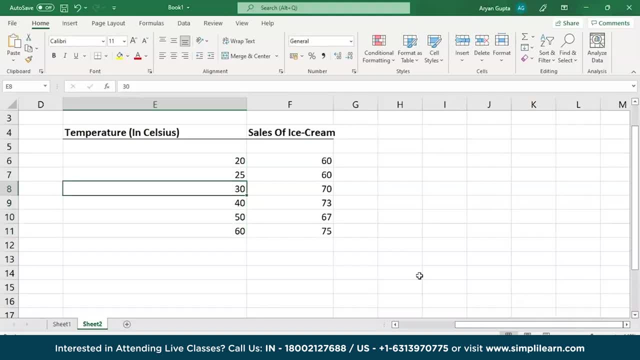 we have the temperature in degree Celsius, such as 20,, 25,, 30,, 40,, 50 and 60, and the corresponding sales of ice cream in the units. To calculate the correlation, we will use the CORREL function. Now we have an array 1 and array 2.. 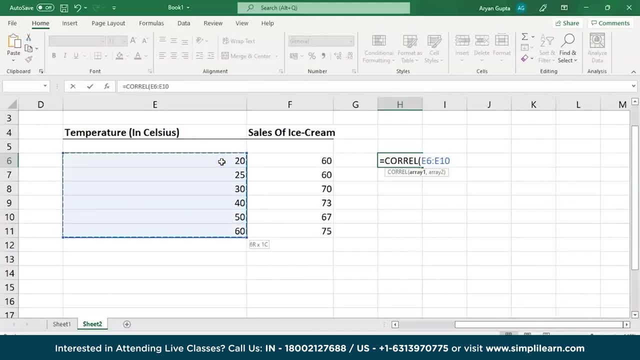 So we will select the array 1, that is, temperature in degree Celsius, and the array 2 will be our sales of ice cream. So you can see, there is a very strong correlation between the temperature of a day and the sales of ice cream unit. 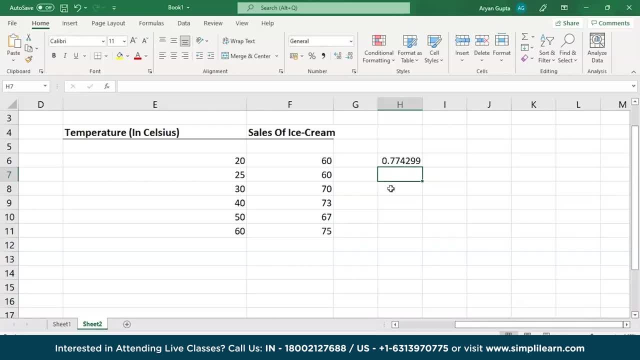 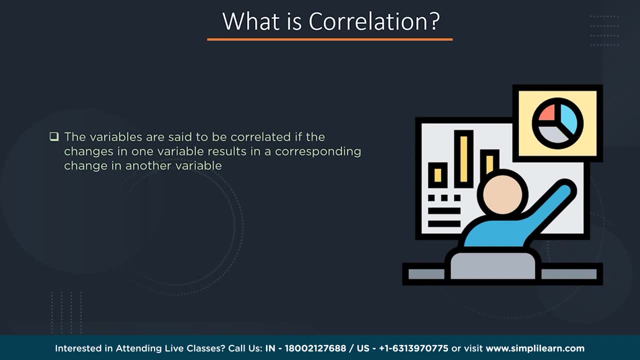 If the sales of ice cream unit increases and if the temperature decreases, the sales of ice cream unit decreases. What is correlation? Correlation refers to the statistical relationship between the two entities. It measures the extent to which two variables are linearly related. 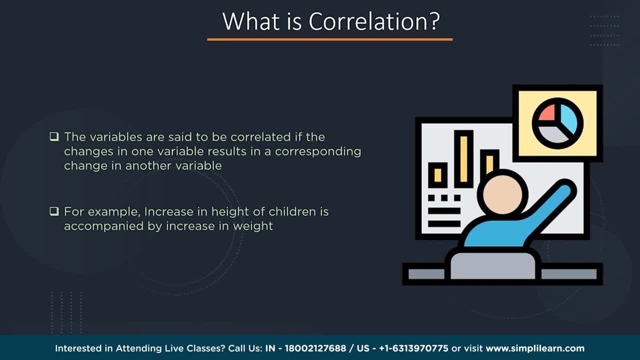 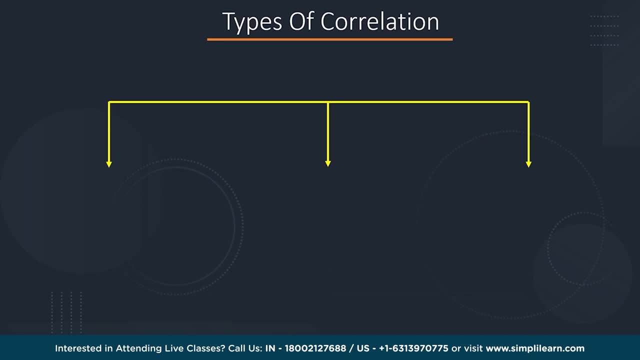 For example, the increase in the height of the children is accompanied often by the increase in weight. The value of the correlation always lies between minus 1 to plus 1.. There are mainly three categories of correlation. The first one is positive correlation and negative correlation. 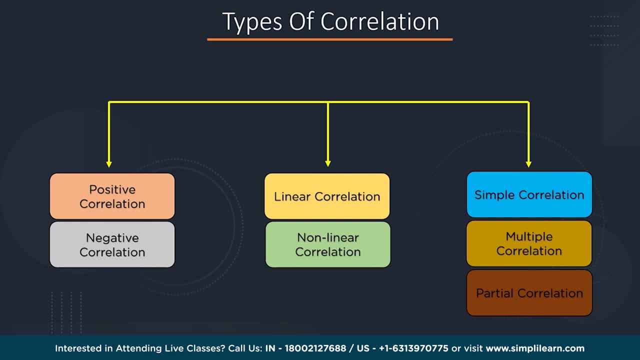 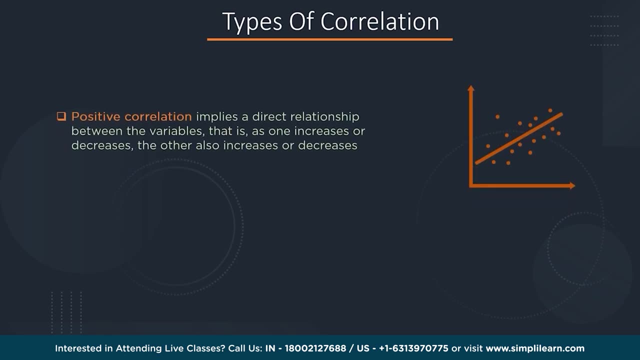 The second one is linear and nonlinear correlation. And the third one is simple, multiple and partial correlation. Let's discuss each of them one by one. Positive correlation: A positive correlation means that a linear relationship is positive And the two variables increases or decreases in the same direction. 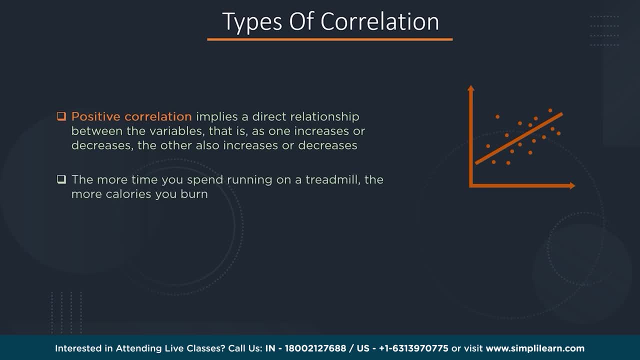 as you can see from the graph, For example, the calories you burn is directly proportional to the amount of time you run on a treadmill. On the other hand, a negative correlation is just the opposite. The relationship line has a negative slope and the variable changes in the opposite direction. 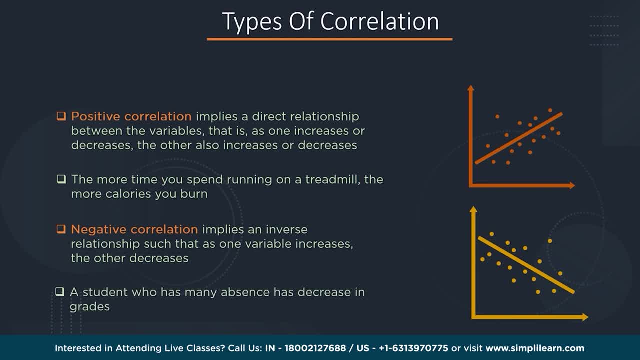 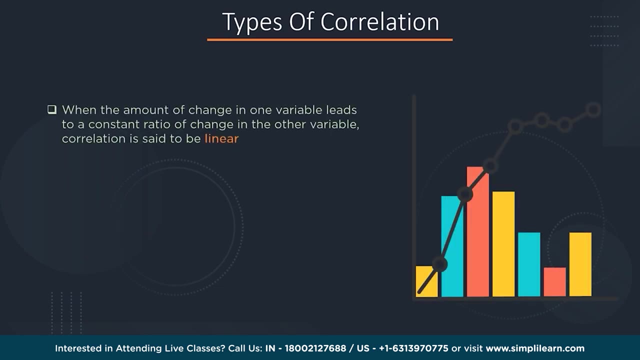 That is, one variable decreases while the other increases. An example can be a student who has many absences has a decrease in grades. Let's now discuss linear and nonlinear correlation. When we change the value of a variable which leads to a constant ratio change. 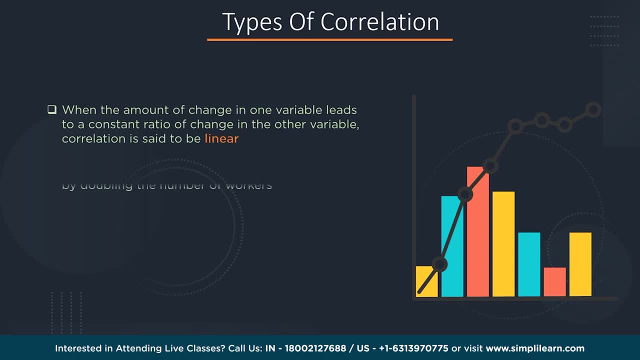 in other variable, then that relation is said to be linear. For example, the factory doubles its output by doubling the number of workers. On the other hand, correlation is said to be nonlinear when the amount of change in one variable is not in constant ratio. 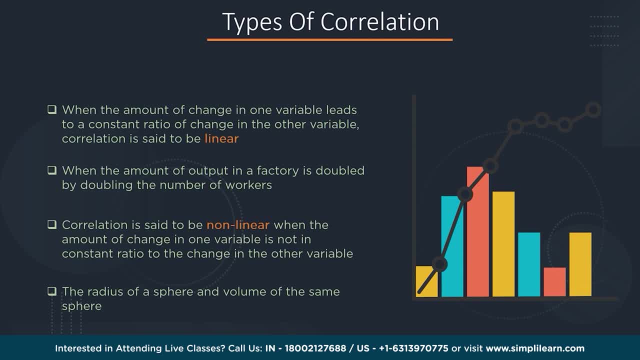 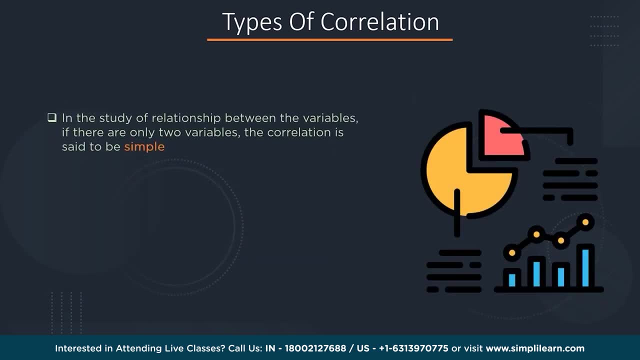 to the change in the other variable. For example, the volume of the same sphere does not happen to be in the same ratio. Now let's discuss simple multiple and partial correlation When studying the relationship between the variables, when only two variables are involved. 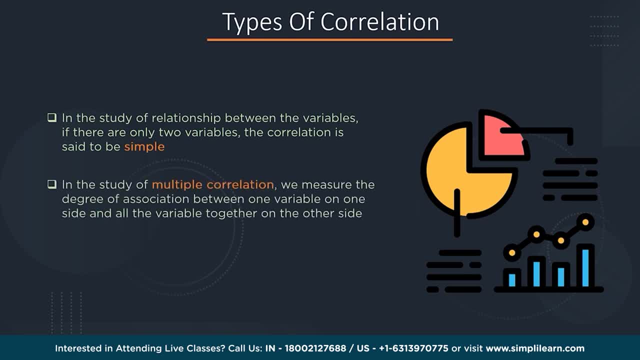 the correlation is said to be simple. In the multiple correlation, we measure the degree of association between one variable on the one side and all the variables together on the other side, And for the partial correlation we study the relationship of one variable with one of the other variables. 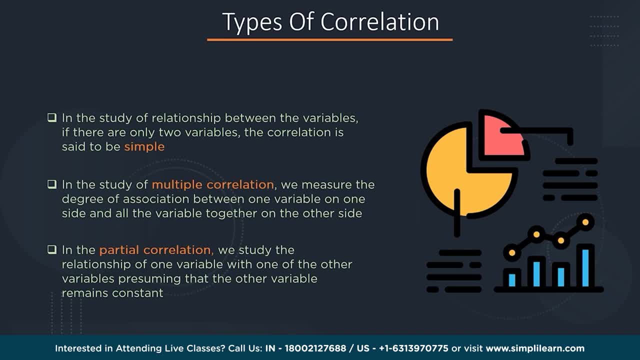 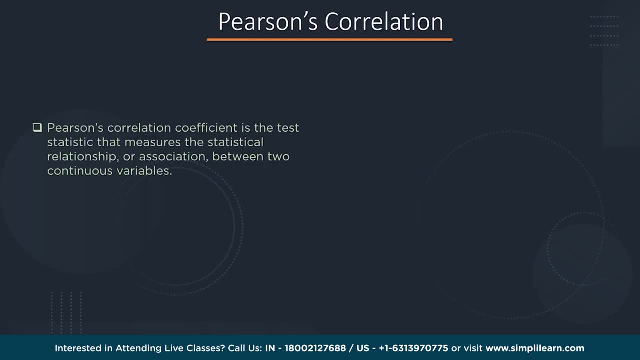 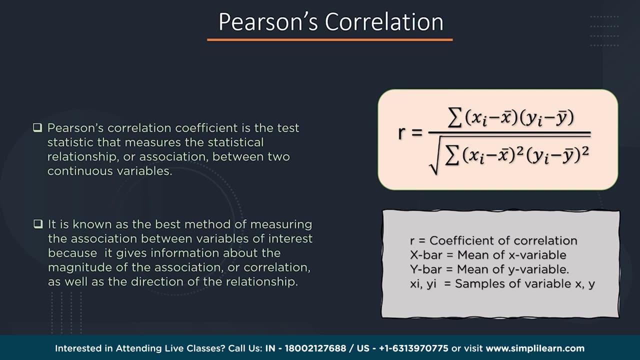 presuming that all the variables remains constant. Now that we know all the types of correlation, let's discuss the two major types to calculate a correlation coefficient. The first one is PSN's correlation. PSN's correlation coefficient is a test statistic that measures 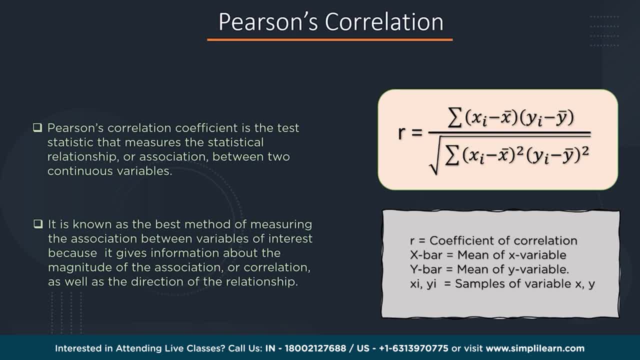 the statistical relationship between the two continuous variables. The PSN's correlation coefficient is often denoted by R, and the formula to calculate the PSN's correlation coefficient is: sigma i minus y bar divided by under root, sigma x- i minus x bar whole square. and y? i minus y bar whole square. 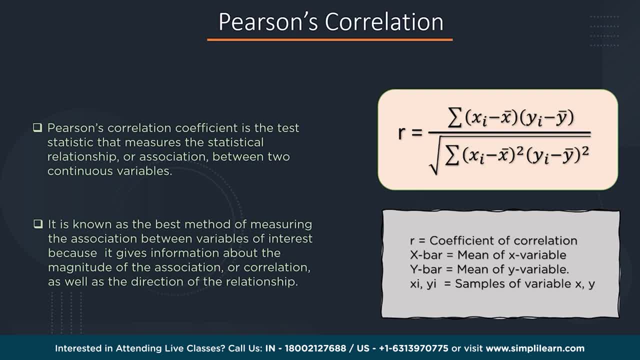 Where R is the coefficient of correlation, x, y is the mean of x variable and y. bar is the mean of y variable and x, i and y. y denotes the samples of variable x and y respectively. The PSN's correlation coefficient is the best method to measure. 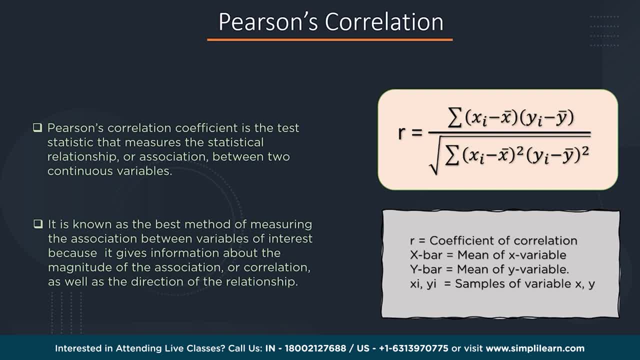 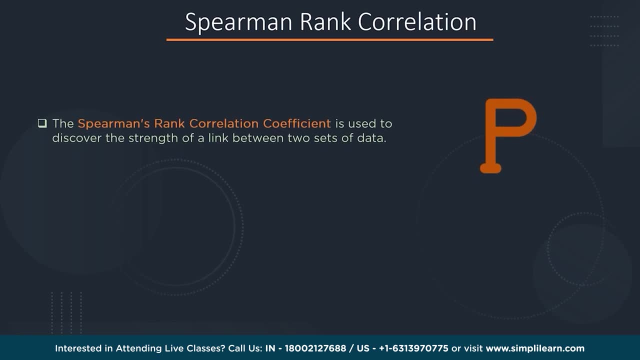 the association between two variables of interest, because it gives information about the magnitude of the association or correlationship, as well as the diagram of the relationship between the two variables. The second best method is PSN's rank correlation. This PSN's rank correlation is used to discover the strength of a link. 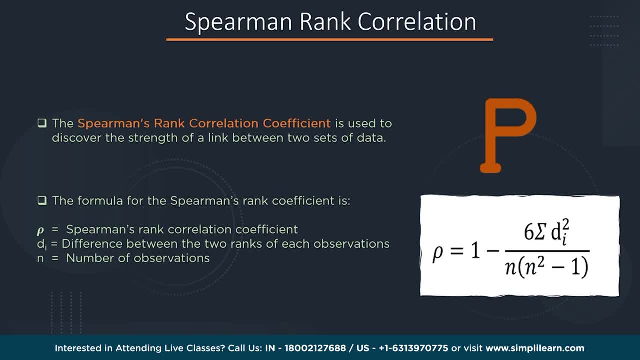 between the two sets of data. The formula to calculate this PSN's rank correlation coefficient is: rho is equal to 1 minus sigma. di whole square divided by n bracket, n square minus 1, where rho is this PSN's rank correlation coefficient. di is the difference between: 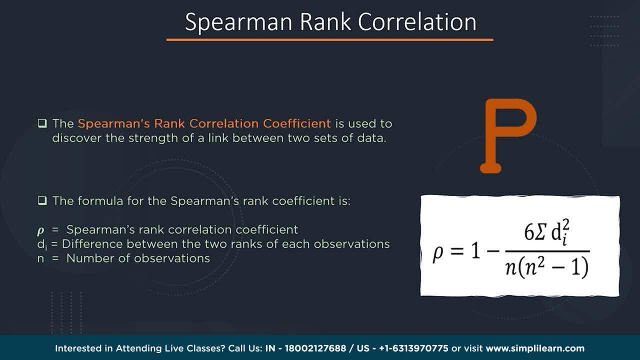 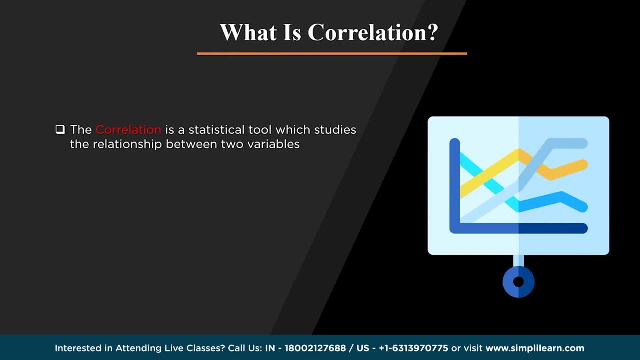 two ranks of each observation, and n is the number of observations. Let's begin. What is correlation? A correlation is a statistical relationship between two entities. It measures the extent to which the two variables are linearly related. In simple words, it is the measurement of strength. 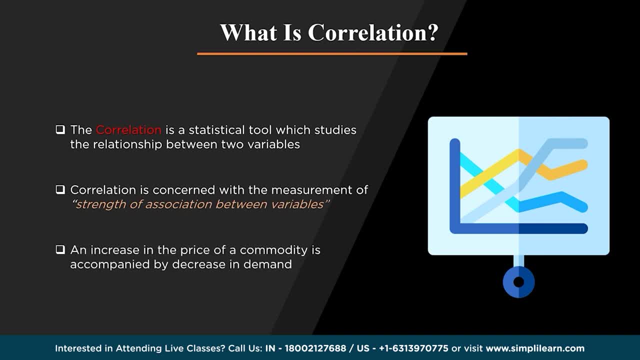 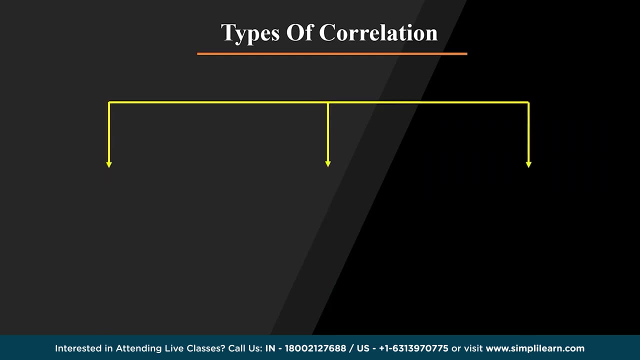 of association between the two variables. For example, an increase in the price of commodity is always accompanied by decrease in demand. The value of the correlation always lies between minus 1 to plus 1.. Types of correlation: There are mainly three categories of correlation. 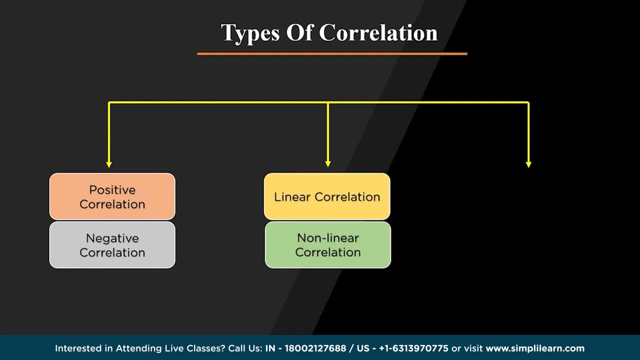 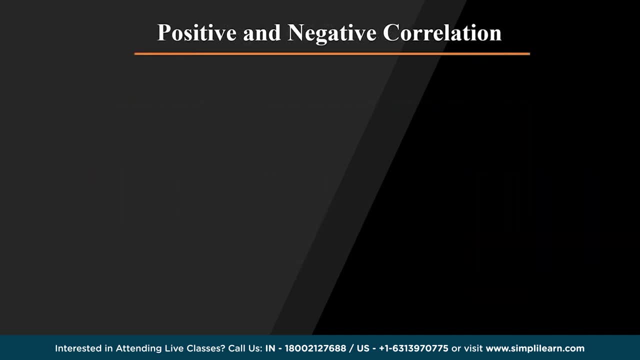 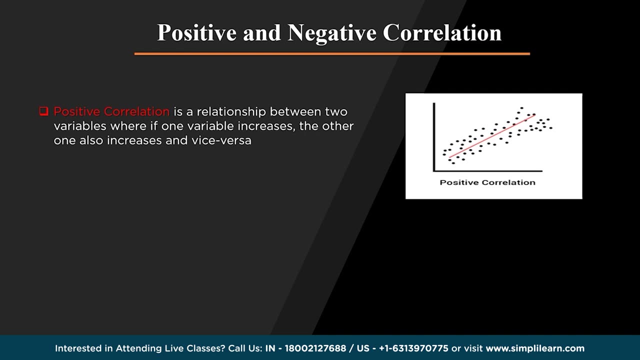 The first one is positive and negative correlation, The second one is linear correlation and non-linear correlation, And the third one is simple, multiple and partial correlation. Let's discuss positive and negative correlation. A positive correlation means that a linear relationship is positive and the two variables increases or decreases. 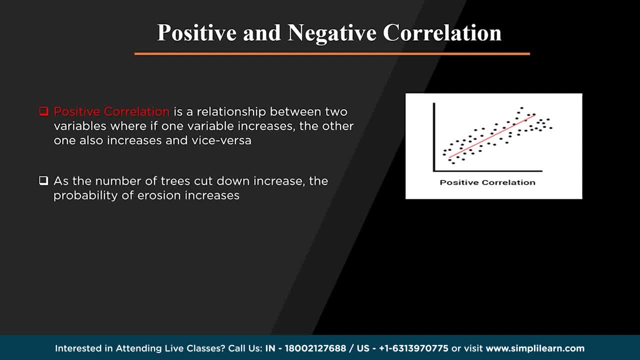 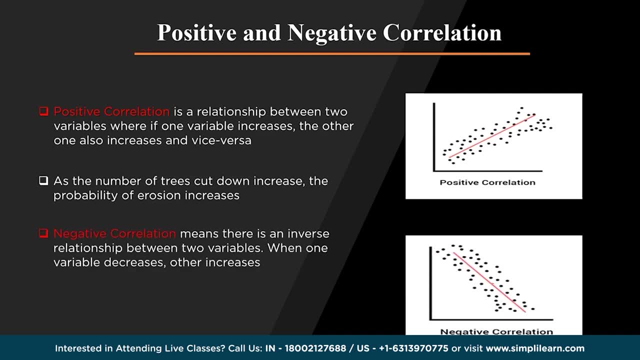 in the same direction, as you can see from the graph. An example can be: as the number of trees cut down increases, the probability of soil erosion also increases In the same manner. a negative correlation is just the opposite. The relationship line has a negative slope. 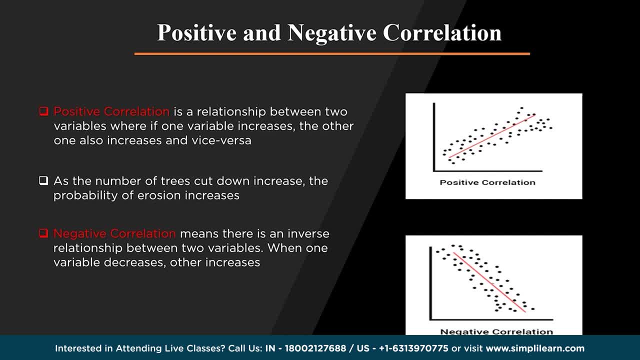 as you can see from the graph, And the variables changes in the opposite direction. That is, one variable decreases while the other increases. To understand this, an example can be: if a car decreases the speed, the time taken to reach the destination increases. 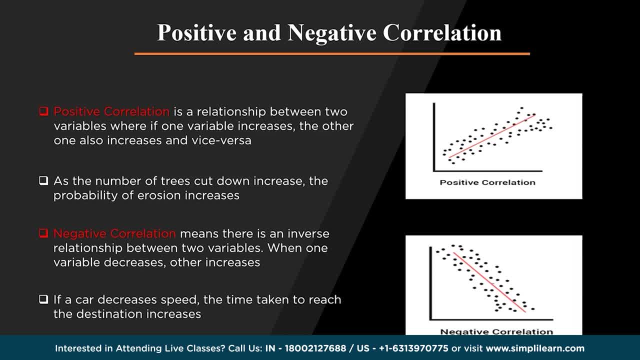 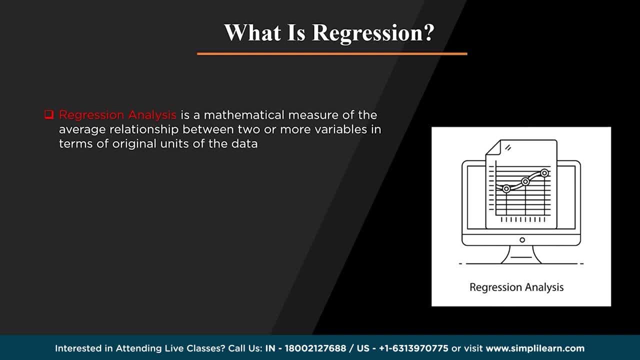 To know more about the types of correlation, you can refer to our previous videos, and you can find the link in our description. Now, what is regression? Regression analysis, like most multivariate statistics, allows you to infer that there is a relationship between two or more variables. 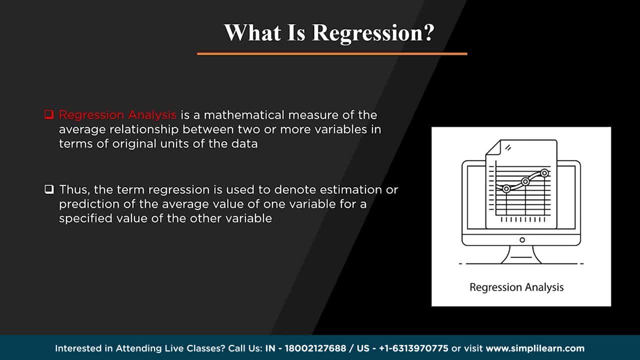 These relationships are seldom exact because there is a variation caused by many variables, not just the variables being studied In regression analysis. there are two types of variables: One is dependent variable and other is independent variable. Let's discuss what the boat variable represents. 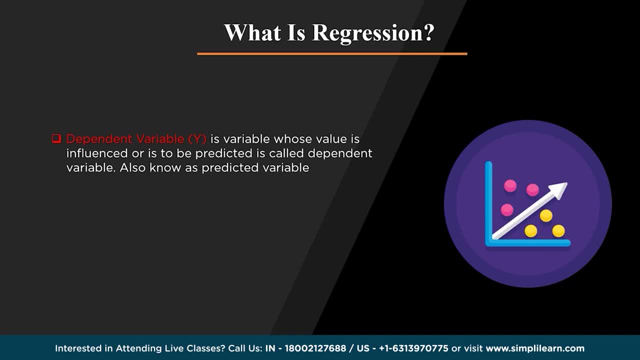 A dependent variable is a variable whose value is influenced or is used to be predicted. The dependent variable is often denoted by y and is also known as a predicted variable, Whereas independent variable, which is denoted by x, is a variable which influences the value. 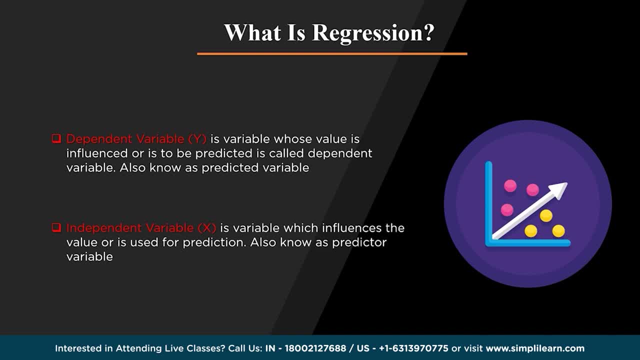 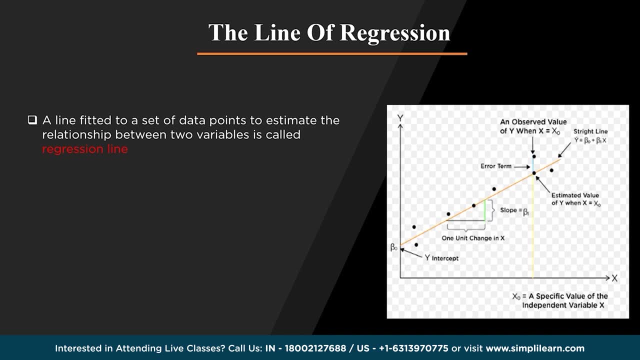 or is used for prediction. The independent variable is also known as a predictive variable. The line of regression. The regression line is a line which is used to describe the behavior of a set of data. In other words, it gives the best trend of the given data. 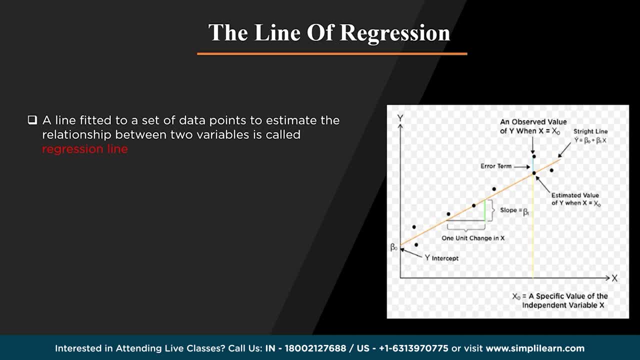 Regression lines are useful in forecasting procedures. The purpose is to describe the interrelationship between the dependent variable and independent variable. The regression equation of y and x describes the change in the value of y for given changes in the value of x and vice versa. 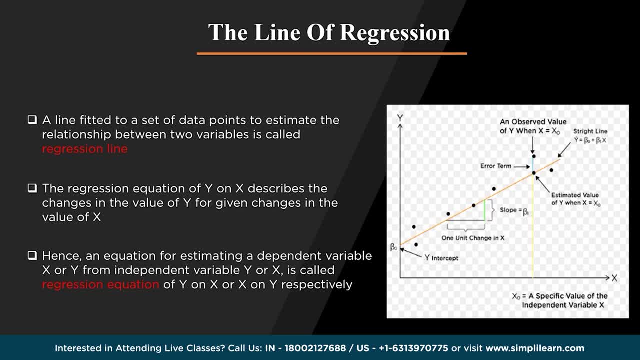 In the regression line equation. x and y are the variables of interest in our data, with y the unknown or dependent variable and x the known or the independent variable. Let's discuss the two key terms in this graph. The first one is slope. The slope is the vertical and horizontal distances. 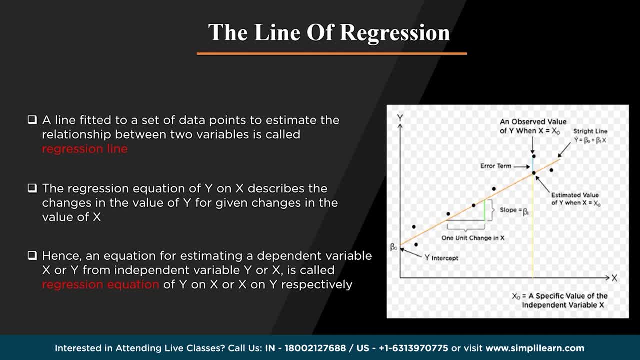 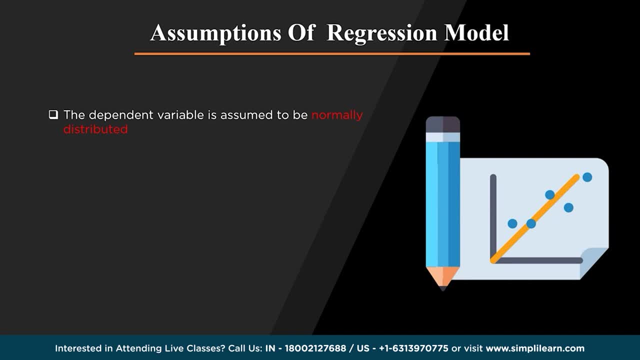 between the two points on a line And you can see y intercept, which is the coordinate of the point at which the curve intersects an axis. There are some assumptions we take to create the regression model. The first one is the dependent variable is assumed to be normally distributed. 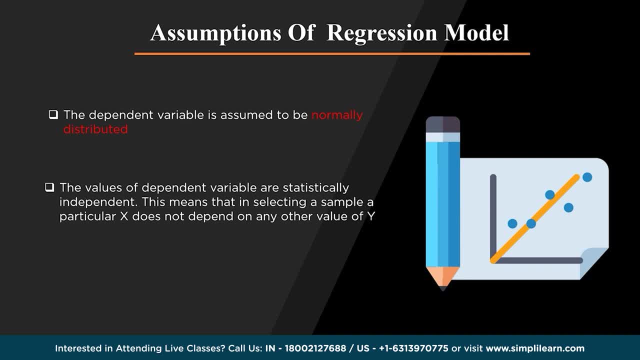 The values of the dependent variable are statistically independent. This means that when we select the sample of a particular x, it does not depend on any other value of y. And the third one is error values. Now let's discuss a simple regression model. A simple regression model is used. 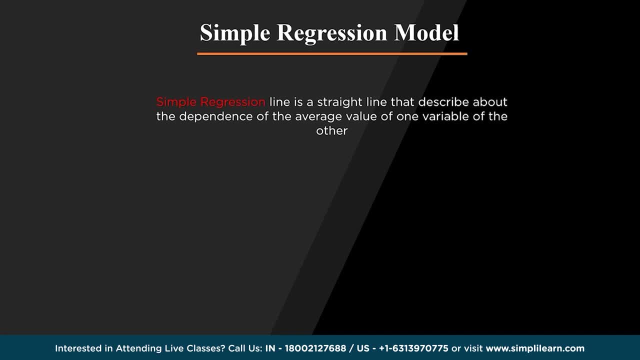 to depict a relationship between variables which are proportional to each other, Meaning the dependent variable increases, decreases with the independent variable. The equation of a simple regression model is: y is equal to b0 plus b1x plus e, where y is dependent variable. 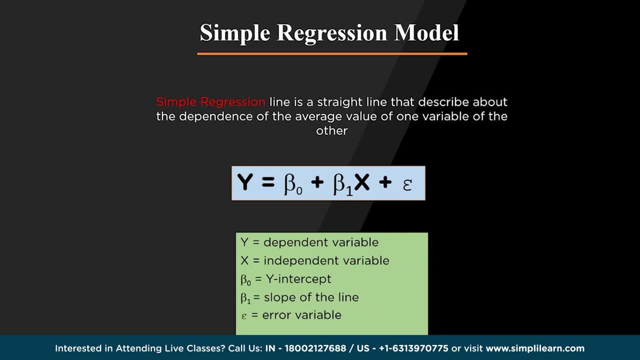 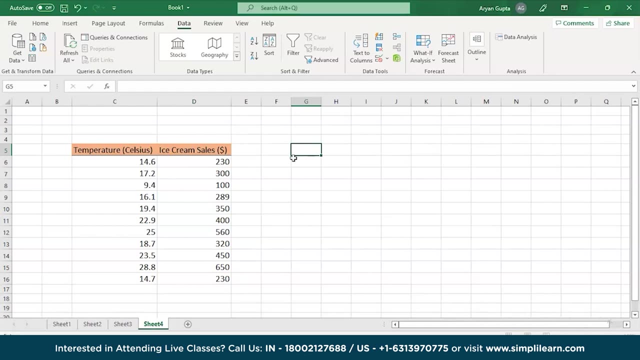 x is independent variable, b0 and b1 represents y, intercept and the slope of the line respectively, and e is the error variable. Now let's move on to Excel to calculate the regression coefficient of a given data. We are on our Excel workbook In front of us. 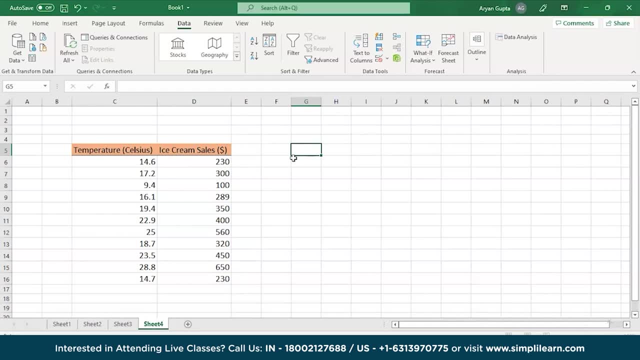 we have the data of temperature of the day and sales of the ice cream on that day. Let's try to understand this regression analysis and summary output using this data. So the first step is to go to the data tab and select data analysis. 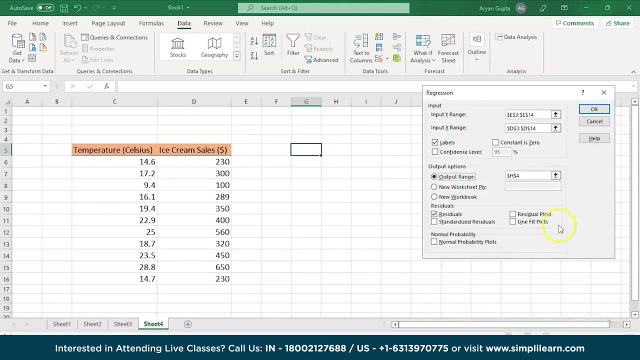 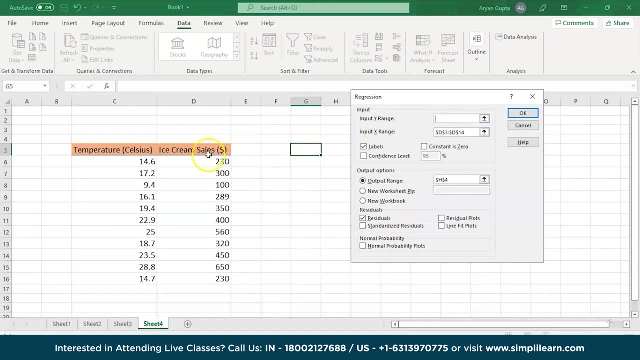 Then select regression and click OK. We'll get this table. Now let's look at the y range as the ice cream sales. This y range is predictable variable, also called as dependent variable. For the input x range, we'll select the temperature. 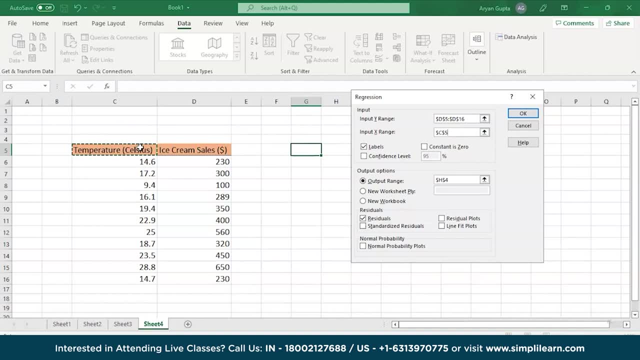 in degree Celsius. This is the explanatory variable, also called as independent variable. One thing you should keep in mind is that the y column must be adjacent to each other. We have the label, so we'll check the label and we'll select the output range. 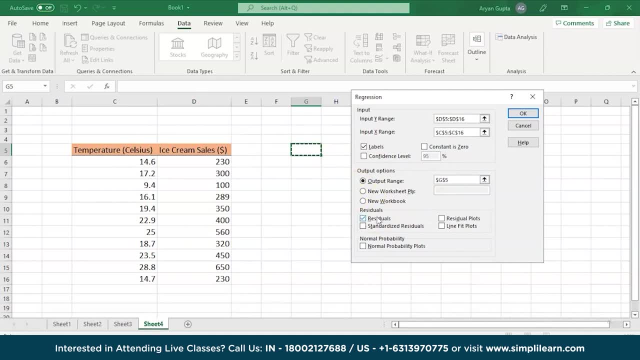 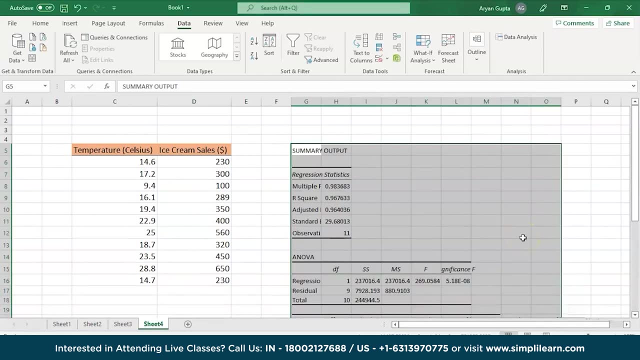 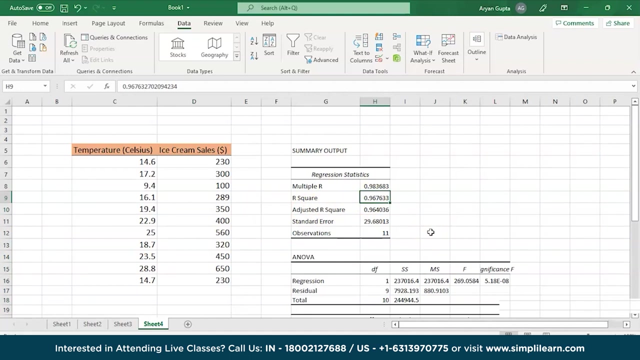 from G5.. Check the residuals and click OK. Excel produces the following output. Let's analyze some key data. We got the r-square value to be 0.9676, which is very good. This shows that the 96% of the variation in ice cream sales. 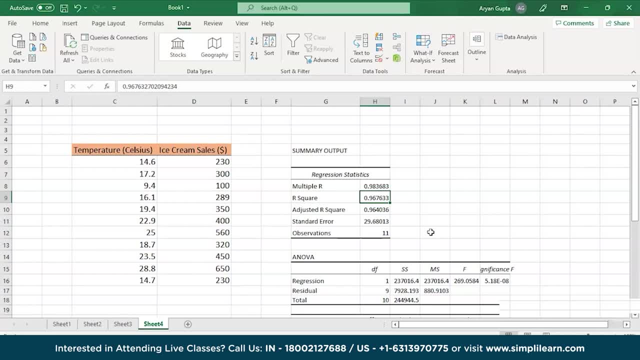 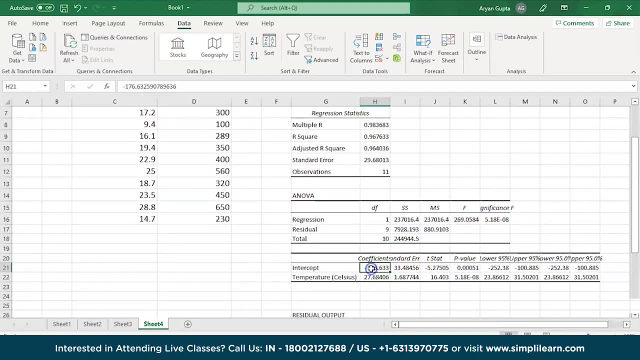 is explained by the temperature of the day. Closer to the 1, the better the regression line fits the data. Now let's move little more and analyze this coefficient. If you look at the coefficient, you'll get the equation of the regression line. 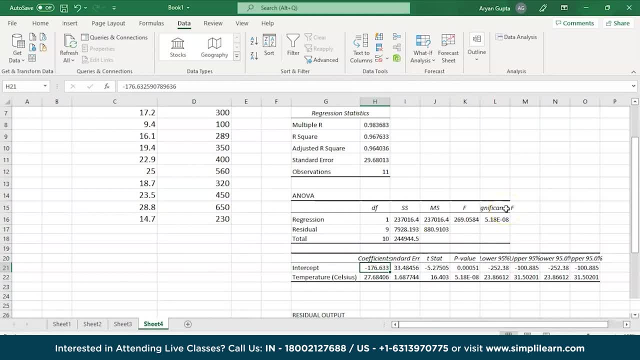 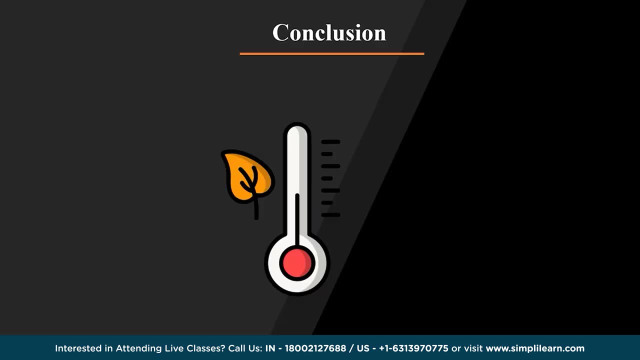 In our case it is minus 26.33 plus 27.68 into temperature of the day. Substituting the temperature of the day for any given day, we can find the sales of the ice cream. With the above discussion we can conclude that there is a big difference. 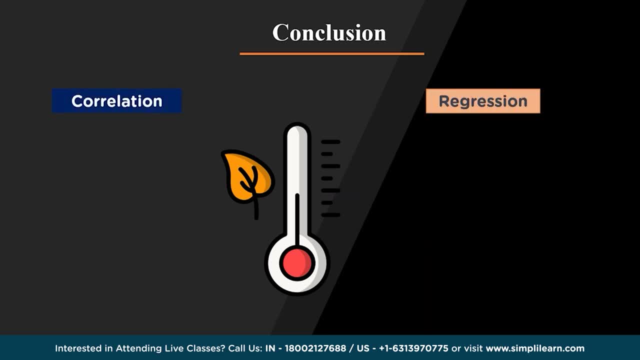 between the correlation and regression, although these are studied together. Correlation is used to study whether the variables under study are correlated, Whereas regression is used to establish the functional relationship between the two variables. The equation of the regression line is of form: y is equal to fx plus c. 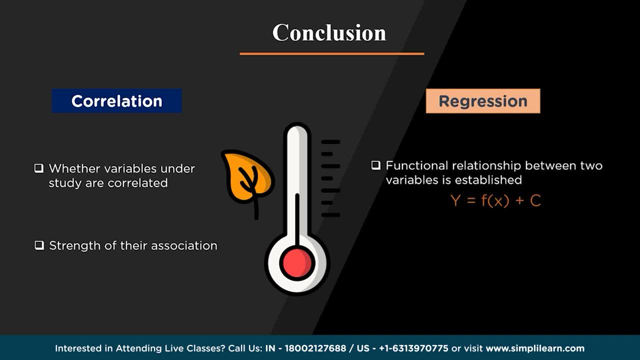 Correlation is used to establish the strength of the association between the two variables that are being studied, Whereas regression is used to make the future predictions on the any given event. Also, data scientist looking for online training and certification programs from the best universities. 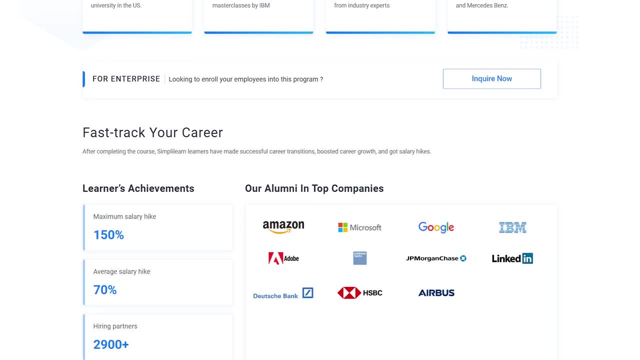 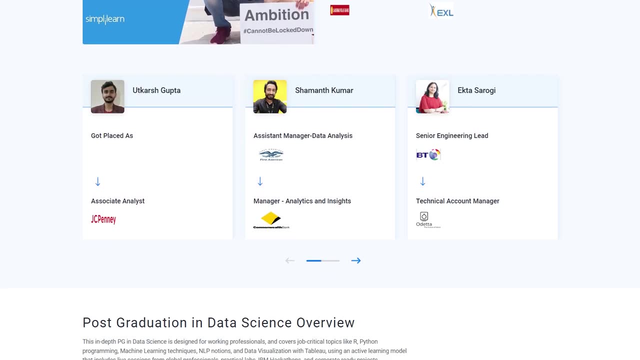 or a professional who elicits to switch careers with data science, try giving SimplyLearn's post graduate program in data science a shot. The link in the description box below should navigate you to the home page, where you can find the complete overview of the program being offered. 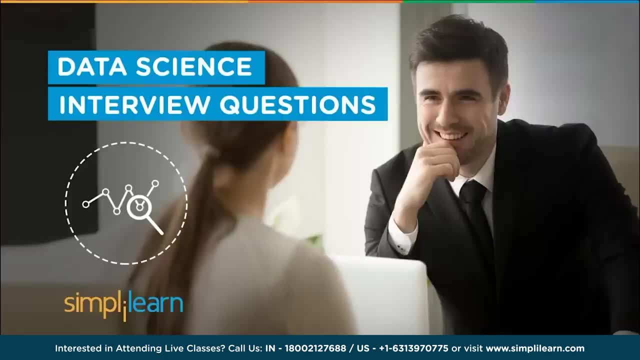 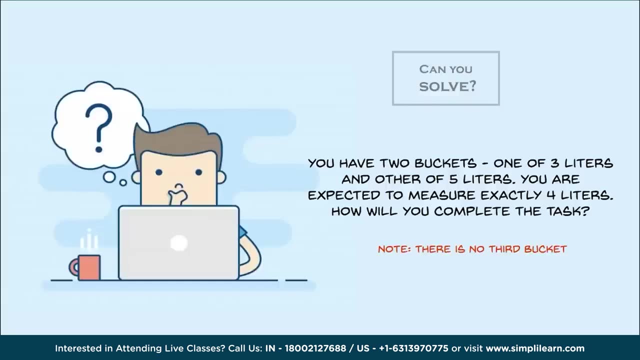 Now over to our training experts: Data science interview questions. My name is Richard Kirschner with the SimplyLearn team. That's wwwsimplylearncom. Get certified, get ahead Before we dive in and start going through the questions one at a time. 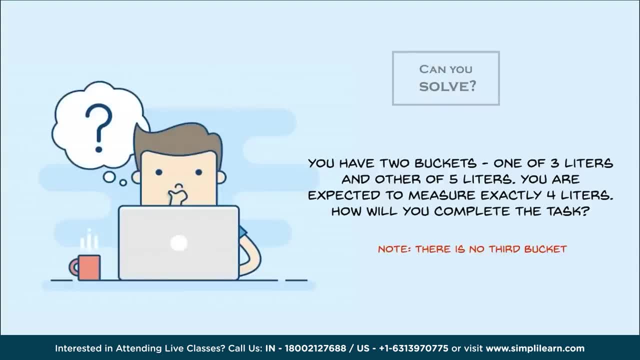 we're going to start with some of the logical kind of concept that enters in a lot of interviews. In this one you have two buckets, One of three liters and the other of five liters. You're expected to measure exactly four liters. How will you complete the task? 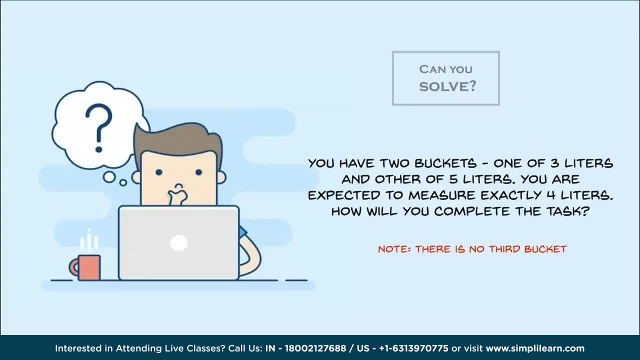 And note you only have the two buckets. You don't have a third bucket or anything like that, Just the two buckets. And the object of the question like this is to see how well you are thinking outside the box. In this case, you're in a larger box. 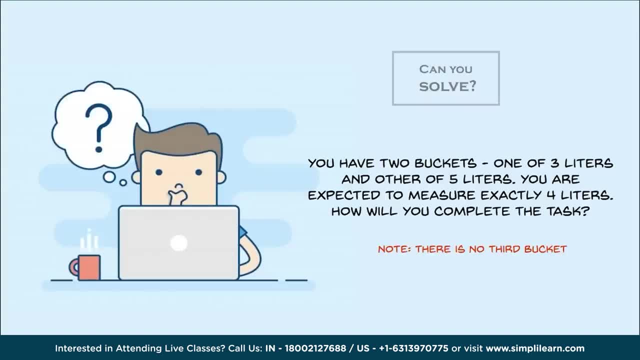 You have two buckets And also the pattern which you go on, And what that means is, if you look at the two buckets- and we'll show you their answer in just a second- you have three liters and a bucket with five liters. 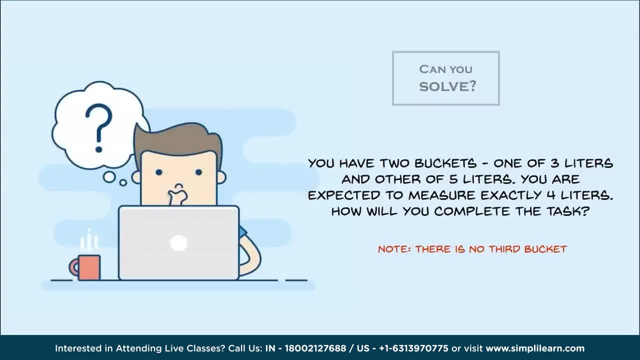 And the first thought is: what happens if you go from left to right? so we have a direction. And what happens if you pour the three liters into the five liter bucket? Well, if you pour the three liters into the five liter bucket, you have an empty bucket of three liters. 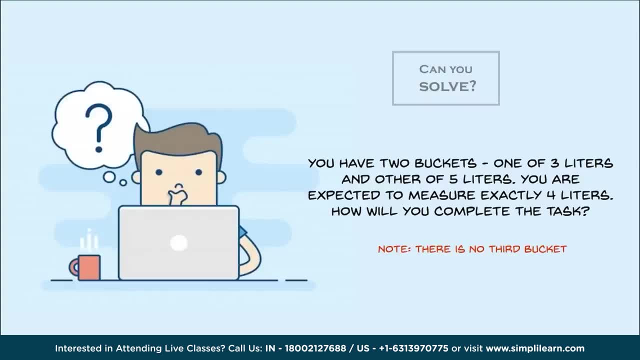 And what's really important here is thinking outside the box. you realize that you have a five liter bucket that has three liters in it and two empty liters, So you have two additional liters you can fill up. If we continue that process, we can pour from the left to right. 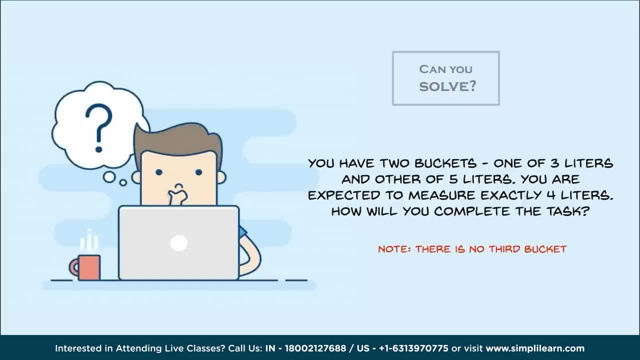 from the small bucket to the large bucket and empty the five liter bucket into additional liters, into the five liter bucket, And three minus two is one And you can keep doing that. You can empty the five liter bucket in pour that one liter in. 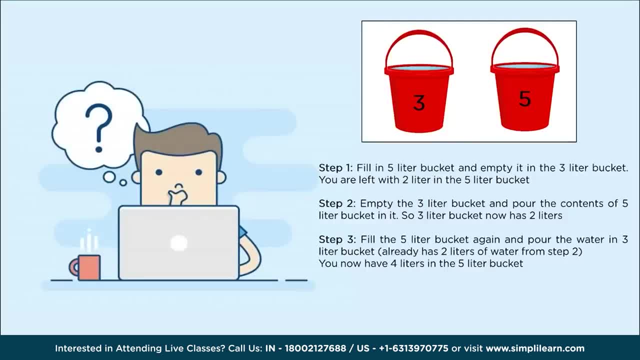 and then you can pour three liters in. What's cool about these questions as you explore them is you realize there's multiple ways usually to solve them. I went from small bucket to big bucket- The Simply Learn team, their solution that they pulled out. 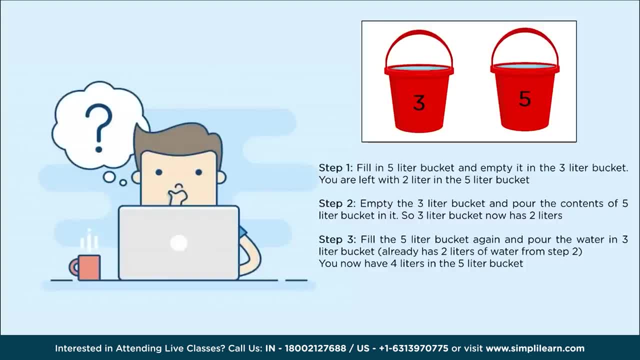 was you fill the five liter bucket and empty it into the three liter bucket. Now you're left with two liters in the five liter bucket. So that's great. You can go from large to small. Remember, we went from small to large, So you can go both either way. 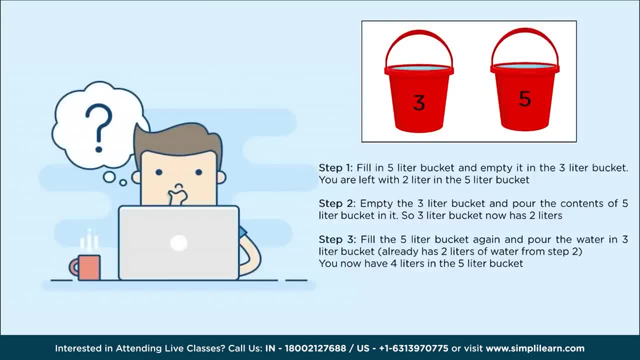 But you have to go one way or the other. it turns out And you can empty the three liter bucket and pour the contents of the five liter bucket in it. So the three liter bucket now has two liters. And if it has two liters, 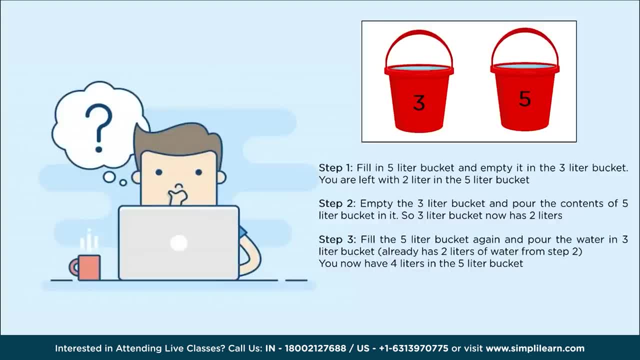 that means it has an empty one liter And by now you probably have guessed that if you have an empty space you can start using that empty space of one liter as a measuring. So we fill the five liter bucket again and we pour the water in the three liter bucket. 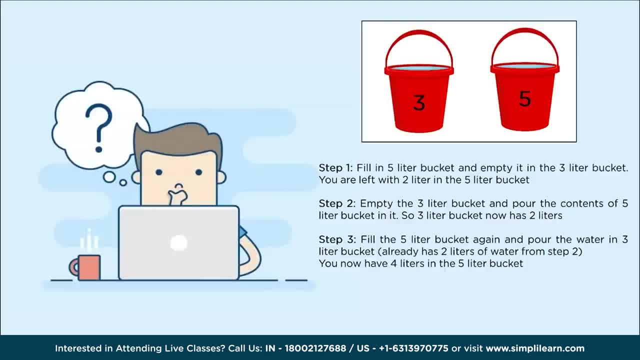 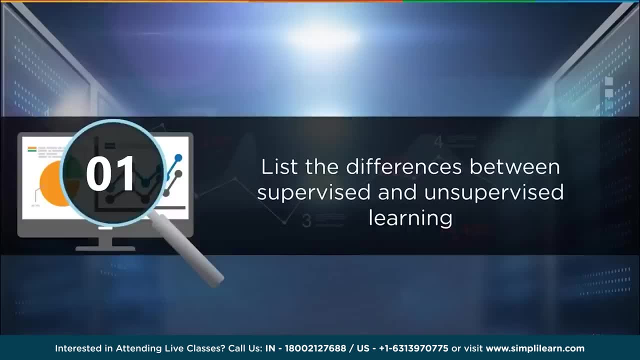 It already has the two liters And this one is four. So interview questions, They break up into all kinds of different patterns. We have logic like this one, which is a lot of fun. We have questions that come up that are more vocabulary. 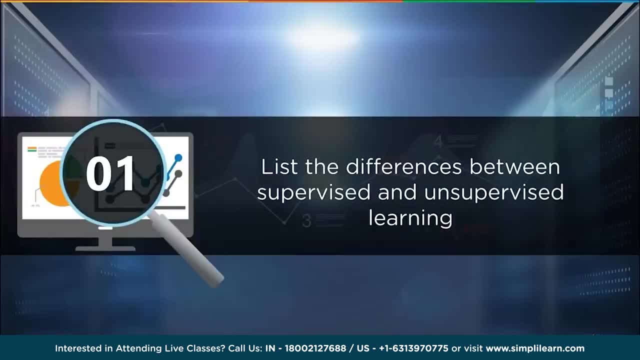 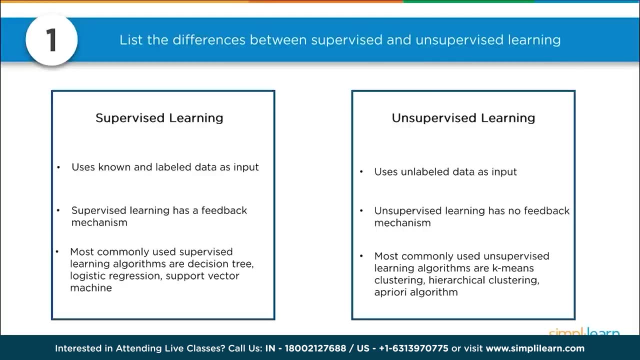 List the difference between supervised and unsupervised learning, Probably one of the fundamental breakdowns in data science. And supervised learning uses known and labeled data as input. Supervised learning has a feedback mechanism. Most commonly used supervised learning algorithms are decision tree logistic regression. 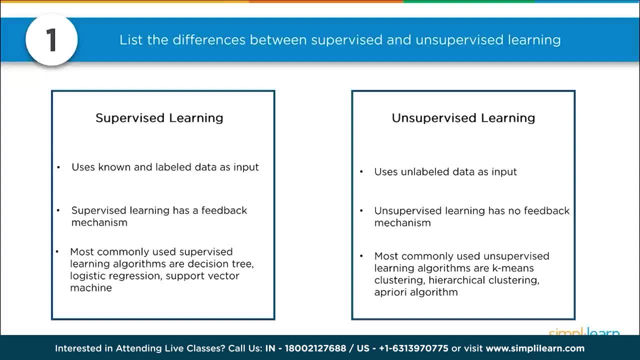 and support vector machine And you should know that those are probably the most common used right now and there certainly are so many coming out. So that's a very evolving thing and be aware of a lot of the different algorithms that are out there outside of the deep learning. 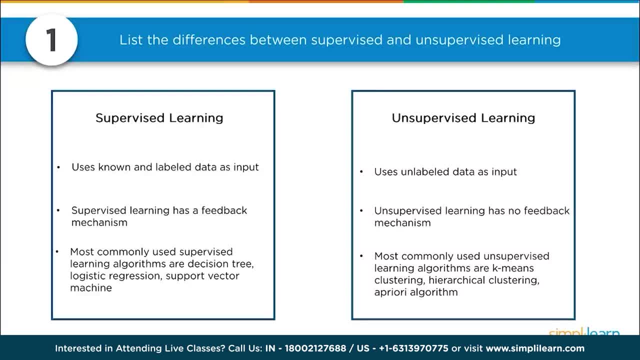 Because a lot of these work faster on raw data and numbers than they do than a deep neural network would. Unsupervised learning uses unlabeled data as input. Unsupervised learning has no feedback mechanism. Most commonly used unsupervised learning algorithms are k-means clustering. 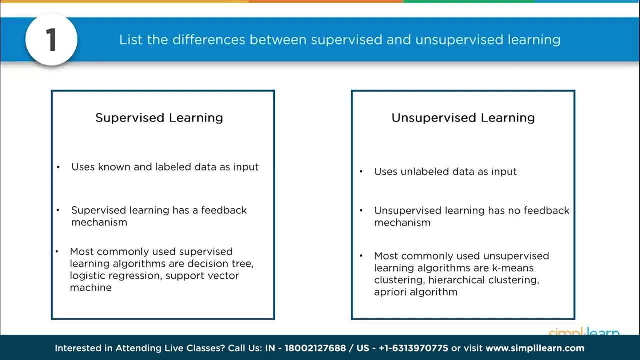 hierarchical clustering and so on, And there certainly are more. I'm going to say k-means definitely is at the top of the list in the hierarchical clustering. Those two are used so many times, So really important to understand what those are and how they're used. 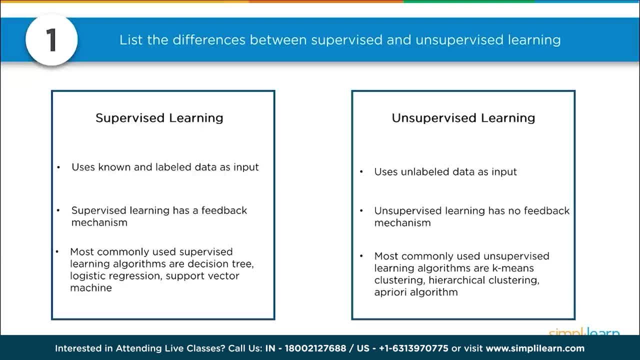 And most important is to understand that supervised learning is: you have your data set, where you have training data and you have all those different pieces moving around, but you're able to train it. You know the answers And, unsupervised, we're just grouping things together. 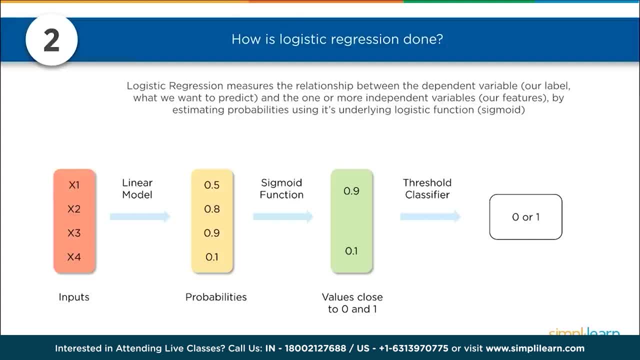 that look like they go together: The relationship between the dependent variable- our label, what we want to predict- and the one or more independent variables- our features, by estimating probability using its underlying logistic function, sigmoid. And whenever I draw these charts, 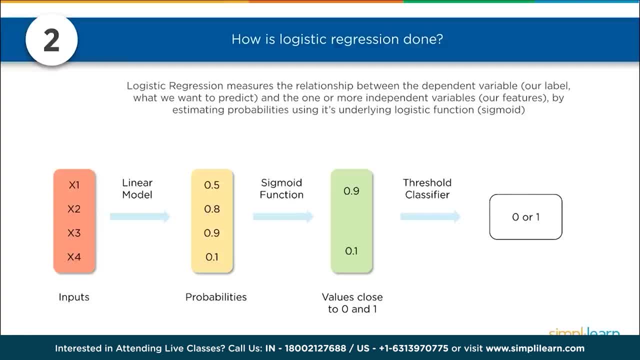 I always end up drawing them. the right hand side first, because you want to know what your output is. What is it you want out of here? And the left hand side: what do you have going in? So you have your in and out. 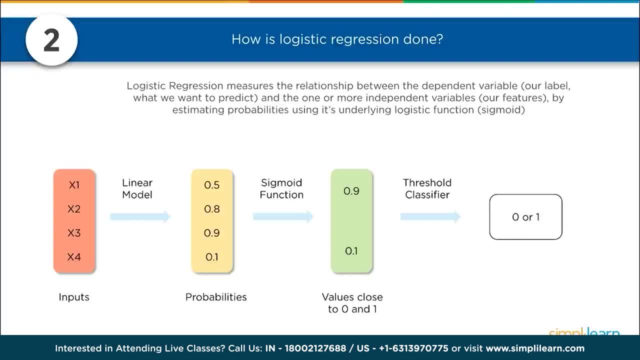 You can see, we have a nice labeled image here to help you remember this. We have our inputs, we have our linear model based on these features coming in The sigmoid function, and it's important to note that the sigmoid function is maybe the most commonly used. 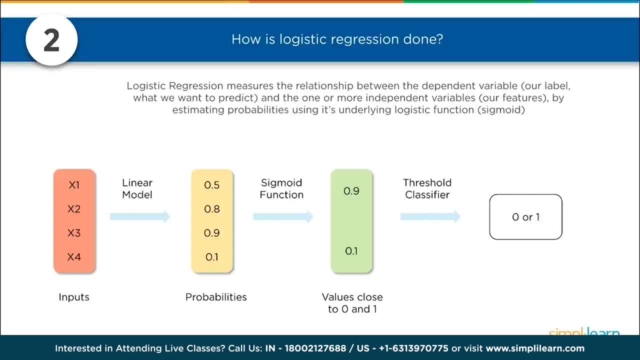 but it's only one of a number of functions that are out there, And the sigmoid function turns our probabilities into a value between 0 and 1, or very close to 0, or very close to 1, between .1 and .009.. 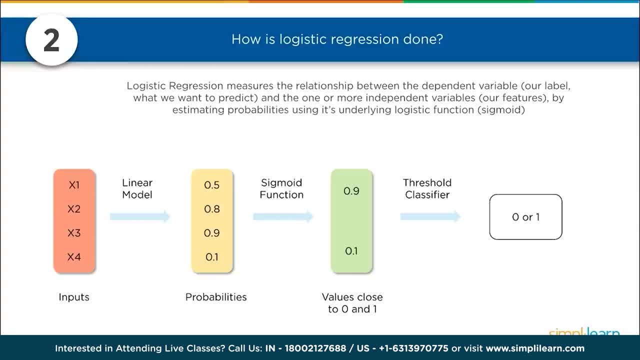 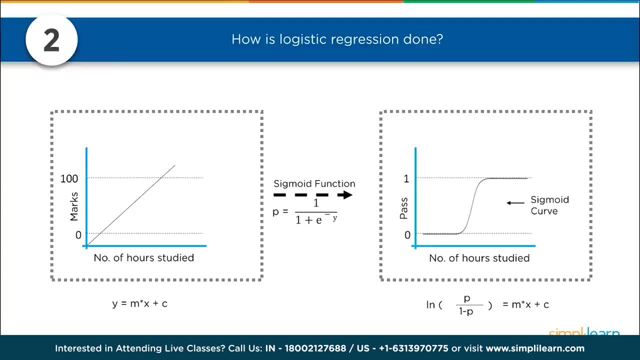 And based on that we generate an answer, in this case a 0 or 1.. How is logistic regression done? So last time we talked about the sigmoid function Generally, depending on what's your interview level of math and what expertise you're going in. 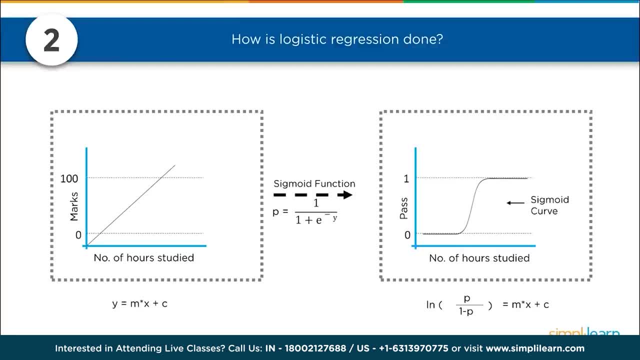 for the market. you'll have to understand that formula of the probability equals 1 over 1, plus e to the negative y, And that's e to the base 2.. So you have your probability function or your sigmoid function, which pushes it. 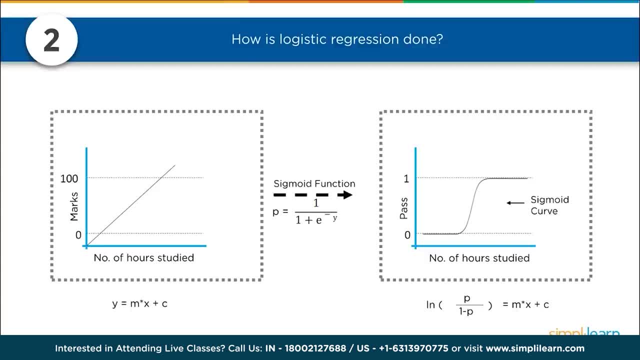 as you can see, we have a nice visual of that. That helps a lot to have that visual. on the sigmoid function, You definitely should know: your y equals m times x plus c, your basic Euclidean geometry of forming a line in the slope plus the intercept, the y intercept. 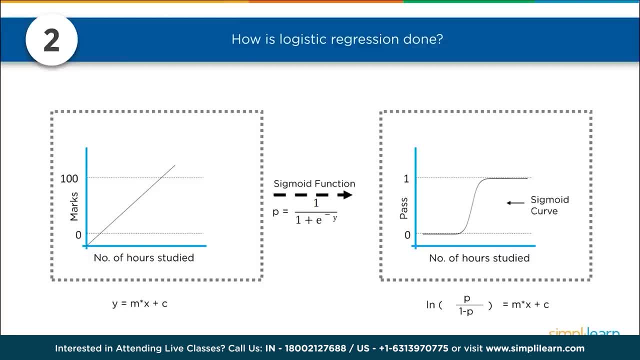 And then you have your natural law and the natural log is to the e as opposed to a base 2 or base 10.. So your natural log to the e of the probability over 1 minus a probability equals your m times x plus c, or your Euclidean line. 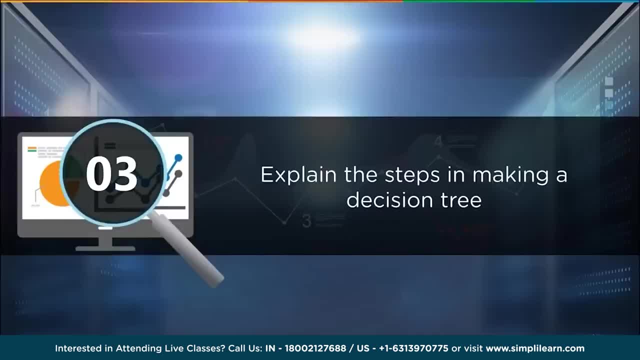 That helps a lot as far as the graphing and understanding the sigmoid function. So we'll just keep pushing on to question number 3.. Explain the steps in making a decision tree. And I noticed last time we brought up the decision tree in the forest. 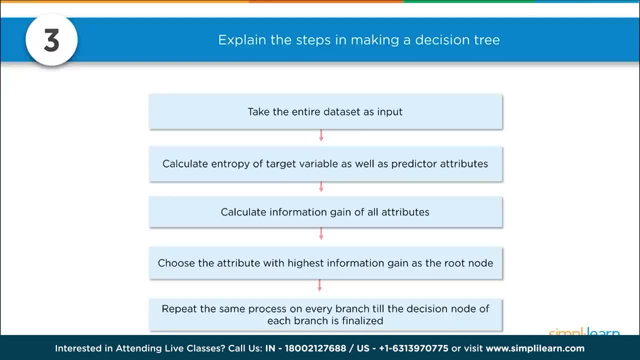 a lot of questions came up. what is the difference? So let's go through that In a decision tree. you're going to take the entire data set as input. You're going to calculate entropy of the target variable as well as the predictor attributes. 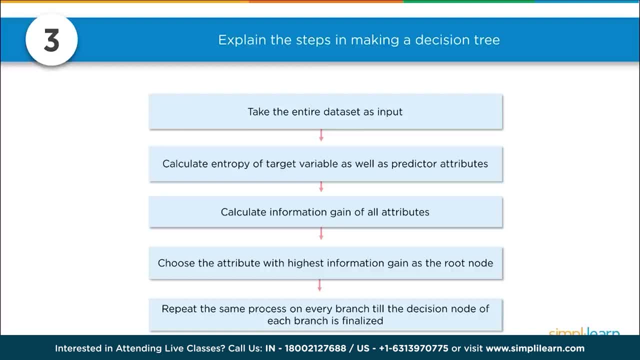 And remember entropy is just how chaotic is it. So if you have, like you know, banana and grapes and oranges, if you're mixing in fruit and that's your data coming in, you have all these different objects that are so separate from each other. 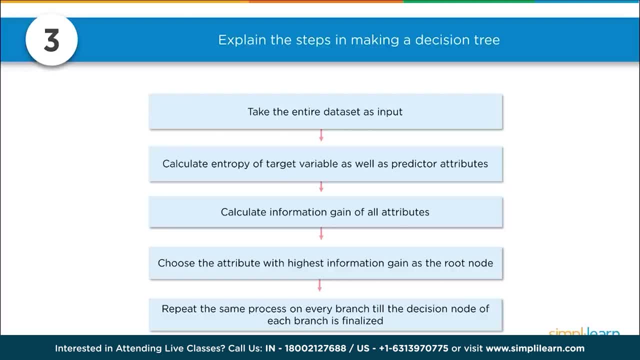 and the more they become uniform, the lower the entropy And we call that information gain. So we gain information on sorting different objects from each other. You have the information gain of all attributes and then you choose the attribute with the highest information gain as the root node. 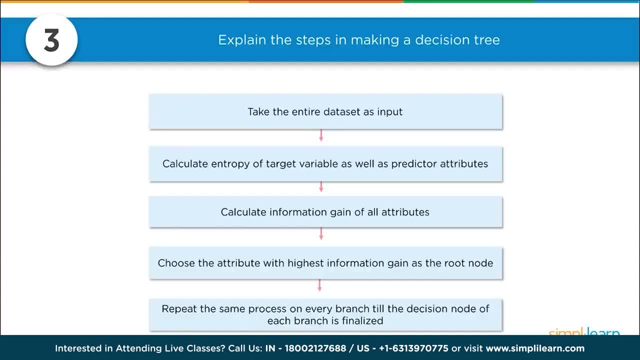 So if you can separate your group and each group, chaos and each group is lowered. whichever split lowers the chaos the most. that's where you split it and that's your root node. At that point, you repeat the same procedure on every branch until the decision node. 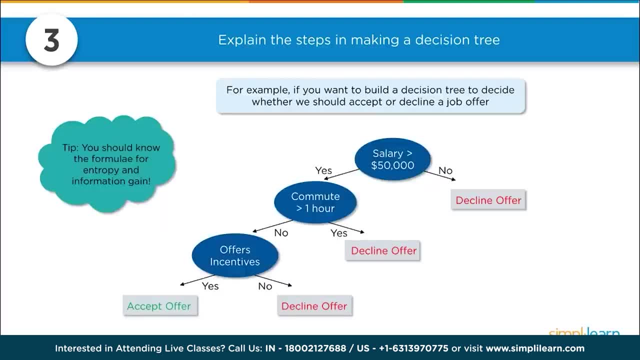 of each branch finalized. So understanding that setup is pretty important. as far as decision trees- and you can see here we have a nice visual to help us decide whether we should accept or decline a job offer. Since these are interview questions, that's a good one to ask. 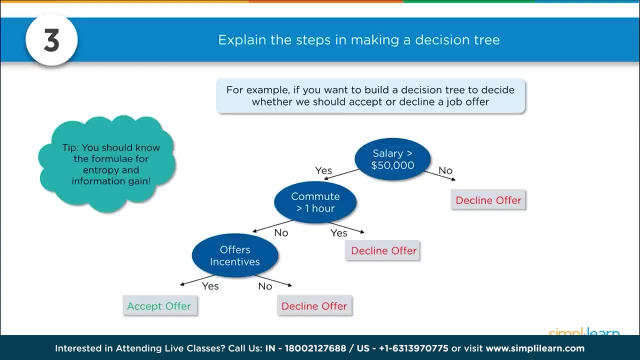 And, just as a tip, you should be pretty aware of the formula for entropy and information gain, So you need to look those up if you don't remember those. And the salary: if it's greater than $50,000, no decline the offer. 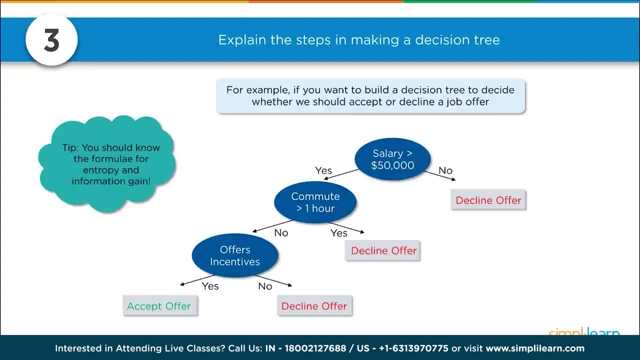 Yes, it's got a good salary. The commute is greater than an hour: Yes, decline the offer. No offers incentives: Yes, accept the offer, No incentives. decline the offer. You also should understand how do you build a random forest model? 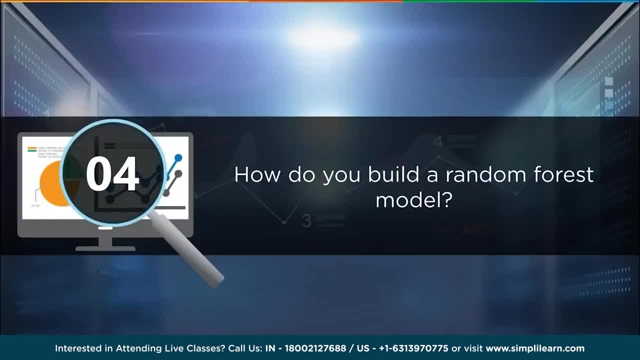 And remember that a random forest is built up of a number of decision trees. So if you split your data up into a lot of different packages and you do a decision tree in each of those different groups of data, the random forest is bringing all those trees together. 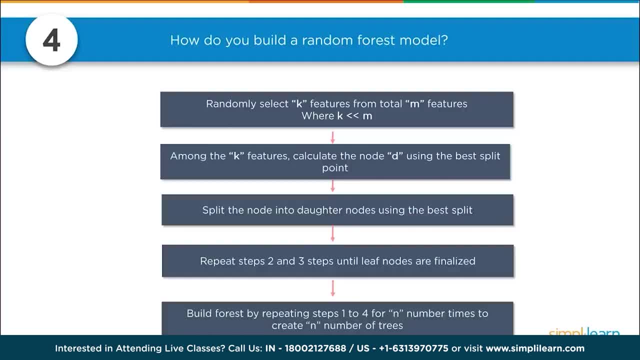 So how do you build a random forest model? Randomly select k features from a total of m features. where k is less than m Among the k features, calculate the node d using the best split point. Split the node into daughter nodes using the best split. 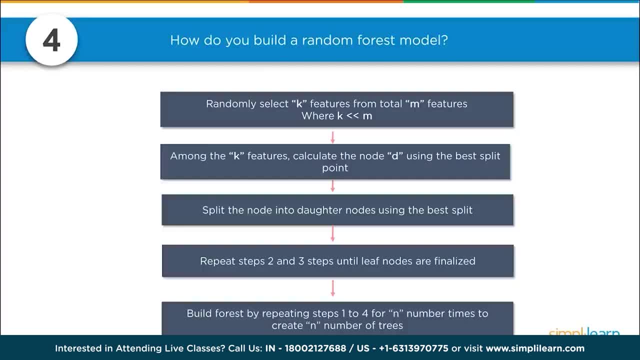 Repeat steps two and three steps until leaf nodes are finalized. Build forests by repeating steps one to four for n number times to create n number of trees. So you can see it's got the same build pattern as the tree, but instead you're building a number of different trees. 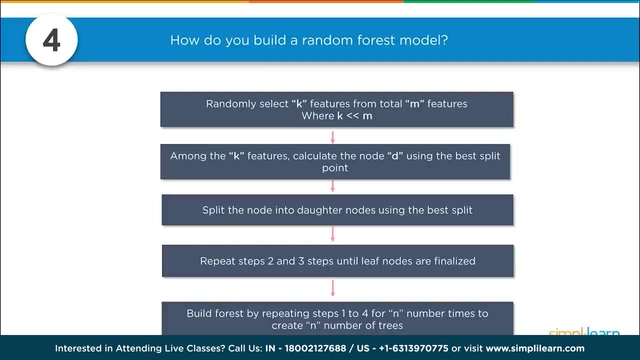 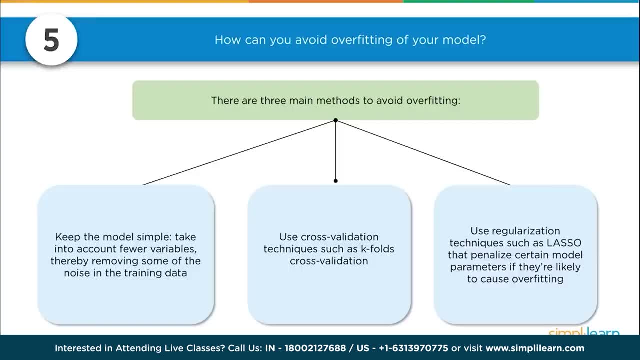 little small trees, so it would all have an n leaf node. Random forest has a vote at the end and whoever gets the most votes wins. That's the answer. This is a very important question in any kind of mathematical, scientific, data science setup in any of them. 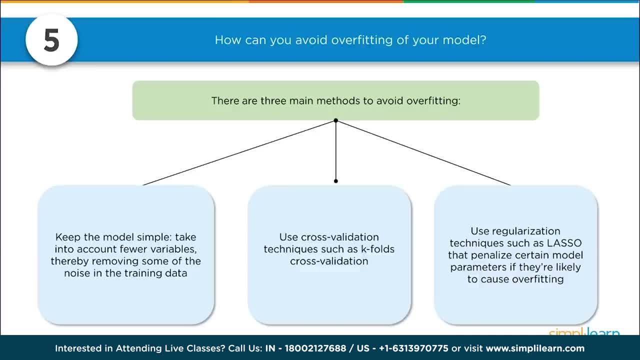 There are three main methods to avoid overfitting, and you should really understand overfitting. Overfitting means that your model is only set for a very small amount of data and ignores the bigger picture. Keep the model simple. Take into account fewer variables. 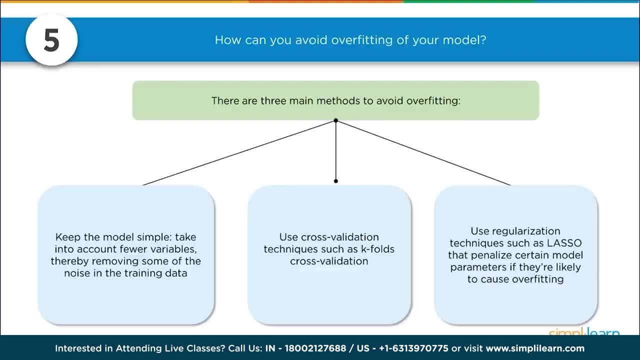 thereby removing some of the noise in the training data. Good advice for any programming at all: Use cross validation techniques such as k-folds cross validation. This is a lasso that penalizes certain model parameters if they're likely to cause overfitting. 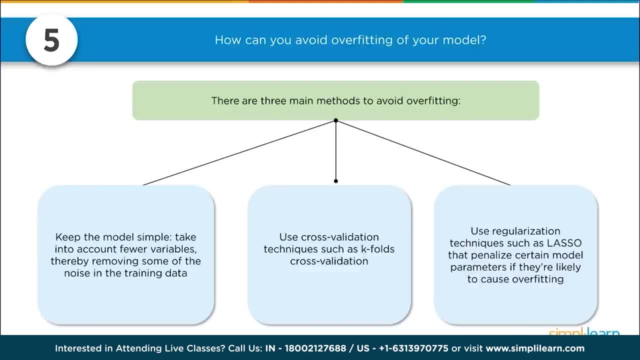 And you should also be well aware that your cross validation techniques- that's like a pre-data or your lasso- and your regularization techniques are usually during the process. So when you're prepping your data, that's when you're going to do a cross validation. 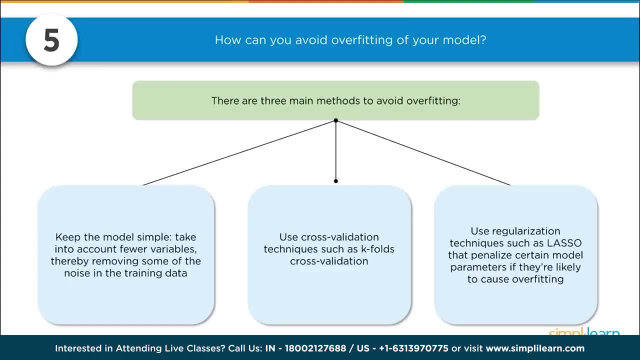 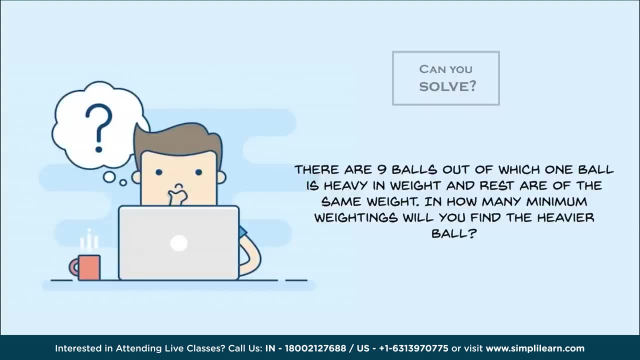 such as splitting your data into three groups and you train it on two groups and test it on one and then switch which two groups. you tested on that kind of thing, So can you solve, oop, another one of these? which two groups are heavy in weight? 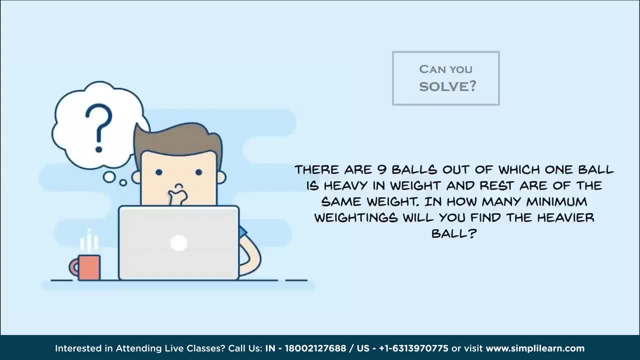 and the rest are of the same weight And how many minimum weighings will you find the heavier ball? And when we say weighing, think of a scale where you can put objects on one side and the other and you can see which side is heavier. 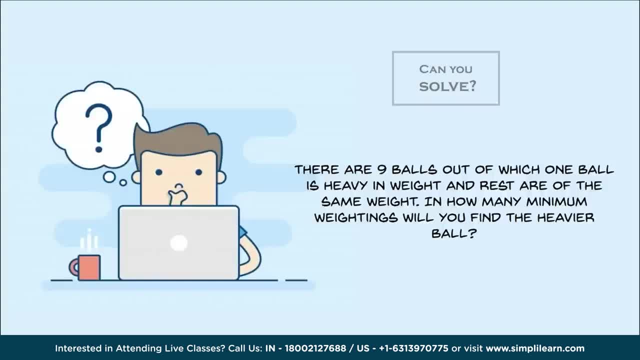 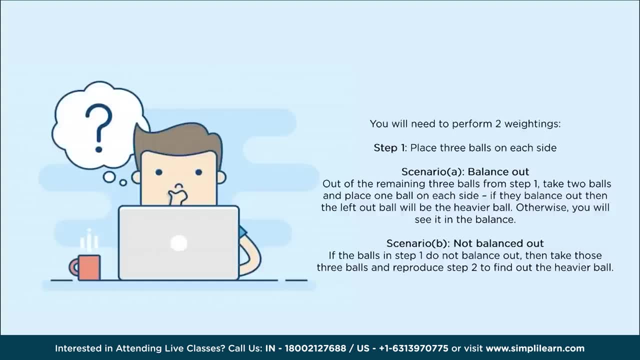 And you want to minimize that. You want to split the balls up in such a way that you're going to do as few measurements as you can. You will need to perform two weighings, So you can get it down to just two weighings. 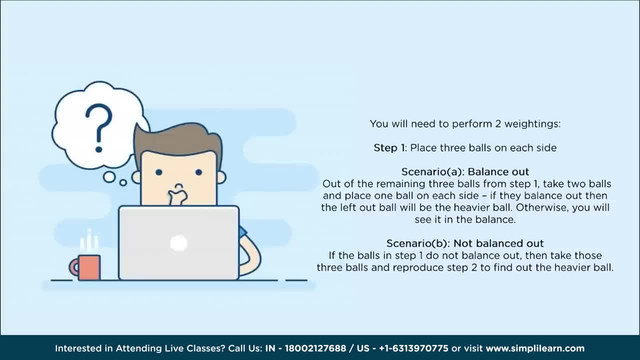 And I always think if there's nine balls, you can just randomly pick six of the balls, and three on one side, three on the other, And if they balance out both sides are equal, then you know the heavy weight isn't in any of those. 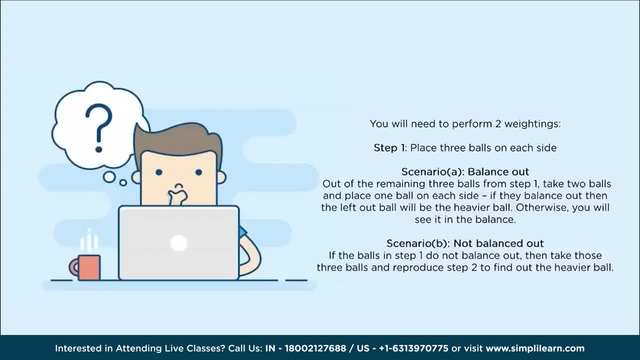 So, out of the remaining three balls from step one, take two balls and place one ball on each side. A little tricky there, because I always want to put all three. I want to put two on one side and one on the other, but no, just randomly pick two of those. 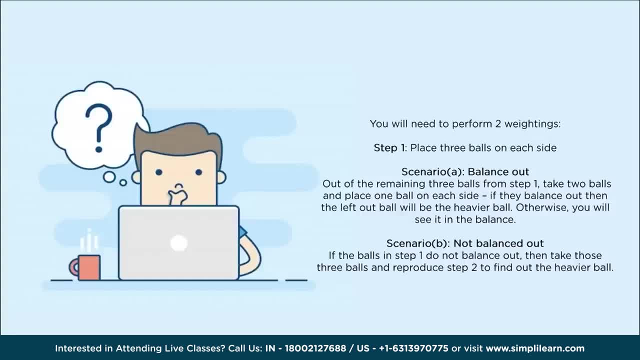 put one on each side. If they balance out, then the left out ball- the one you didn't measure- will be the heavier one. Otherwise, you'll see it in the balance. You'll see which one's heavier and which one's down. Now we go to scenario B. 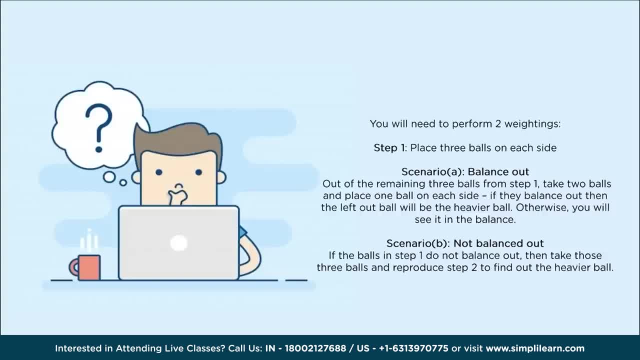 where they did not balance out. So now we know which side has the heavier ball in it, And it's just very similar to what we did before. If the balls in step one do not balance out, then take those three balls that had the heavier side on them. 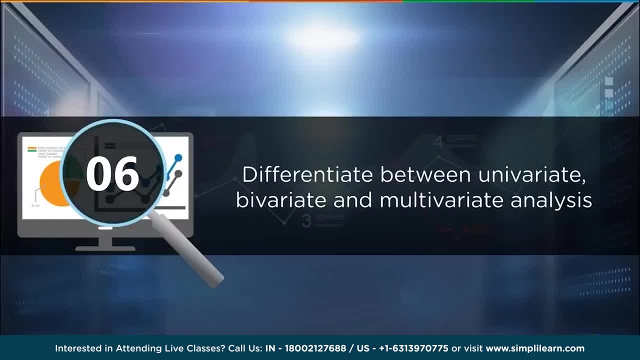 and reproduce. step two, to find out the heavier ball Difference between univariate, bivariate and multivariate analysis. And hopefully, if you know a little Latin, you'll kick in there that you have uni and you have bi and you have multi. 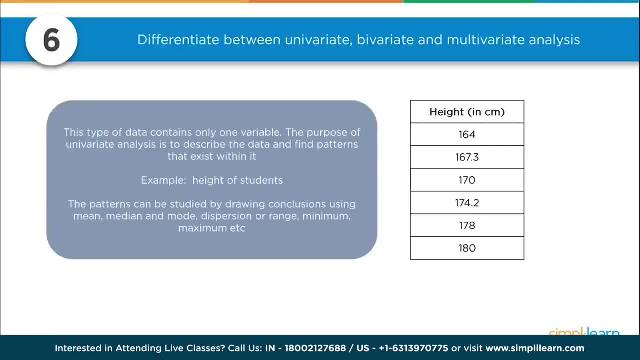 Because the answer is in the words themselves. So the first one: this type of data contains only one variable, So that's the univariate. Purpose of the univariate analysis is to describe the data and find patterns that exist within it. So when you only see one variable coming in, 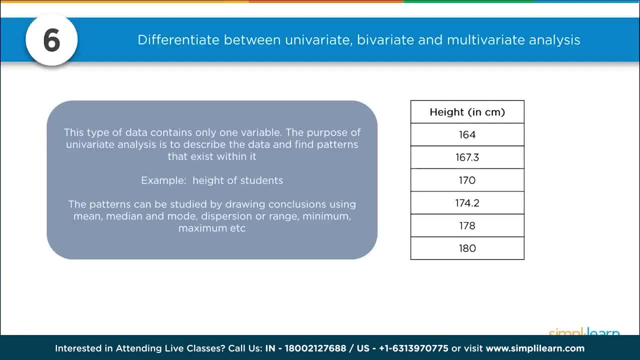 in this case we're using height of students. you're limited as far as what you can do with that data, So you can come up and draw different patterns and conclusions from those patterns using the means, the median, the mode, dispersion range: minimum, maximum. 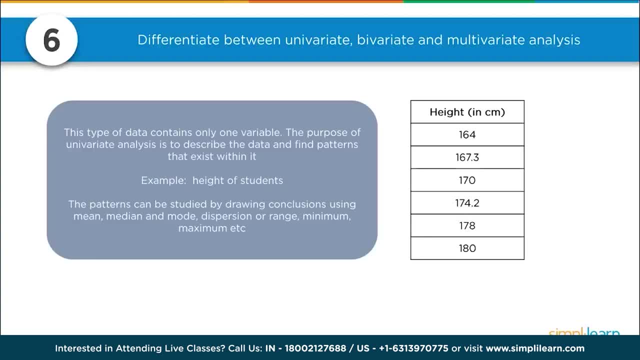 So we're describing the data. So all those words would describe the data and that's about all you can do with data like that. There's no correlation, there's nothing to go beyond that as far as guessing or predicting anything. So we move into. 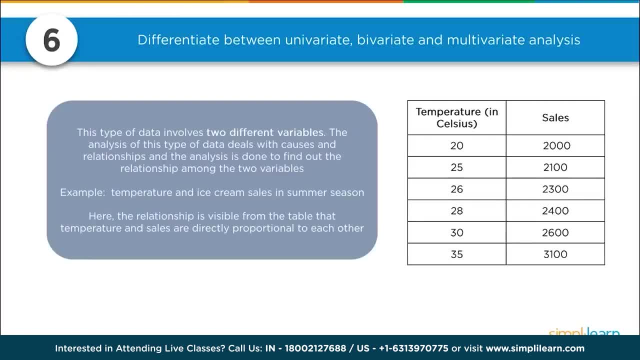 bivariate. You know, uni means one, bi means two. Bivariate. this type of data involves two different variables. The analysis of this type of data deals with causes and relationships, And the analysis is done to find out the relationship among the two variables. 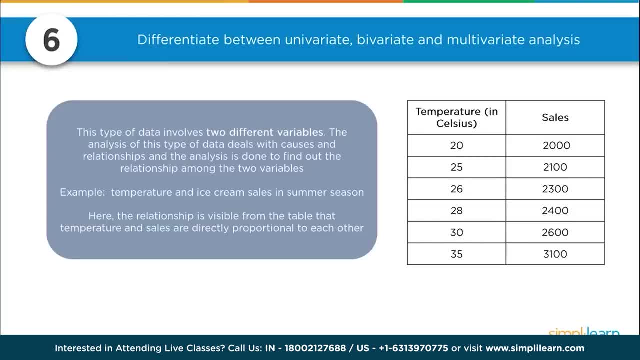 And this is always a favorite one, because everybody loves ice cream in the summer, when it's hot, and very few people go for ice cream in the winter, when it's really cold. So it's easy to see the correlation in the data: The temperature and ice cream sells in summer season. 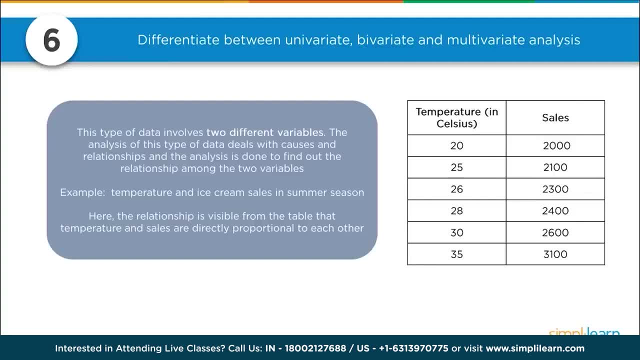 And you can see here where the temperature goes from 20 to 35, and as the temperature goes up so does the sales of ice cream. It goes from 2,000, I'm not sure- 2,000 to what, so I'm guessing it's a very large chain. 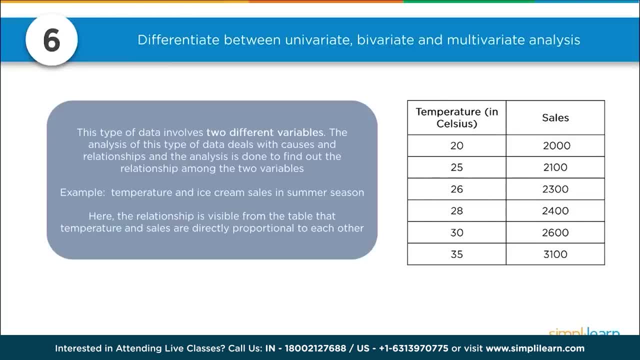 because if they're selling 2,000 ice cream cones and they have a lot of business, good for them. You know a little vendor on the corner selling 2,000 ice cream cones a day and 3,100 the next day. Here the. 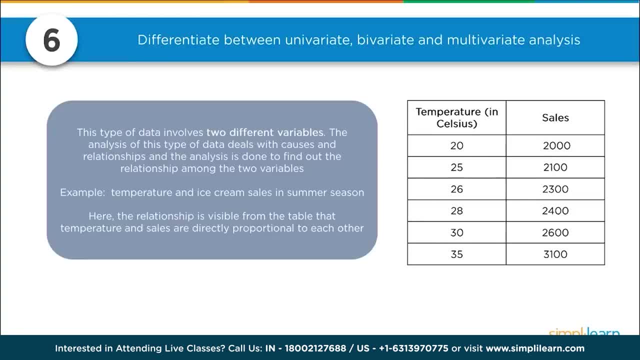 relationship is visible from the table that temperature and sales are directly proportional to each other. So the hotter the temperature, we can predict an increase in sales. So the word prediction should come up. So we have description and prediction When the data involves three. 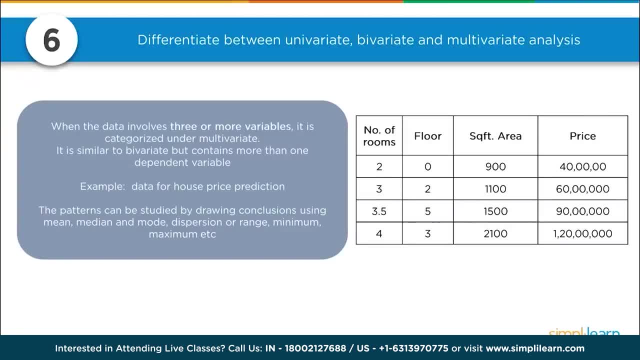 or more variables. it is categorized under multivariate. It is similar to bivariate, but contains more than one dependent variable. In this example, another really common one: the data for house price prediction. the patterns can be studied by drawing conclusions using mean, median and. 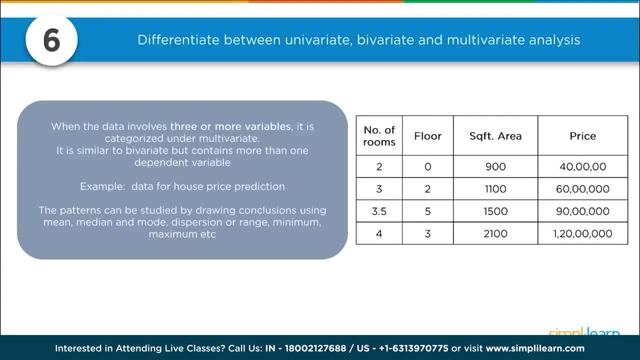 mode, dispersion or range- minimum, maximum, etc. And so you can start describing the data- that's what all that was- and then using that description to guess what the price is going to be. So this is very good if you're in the market and you 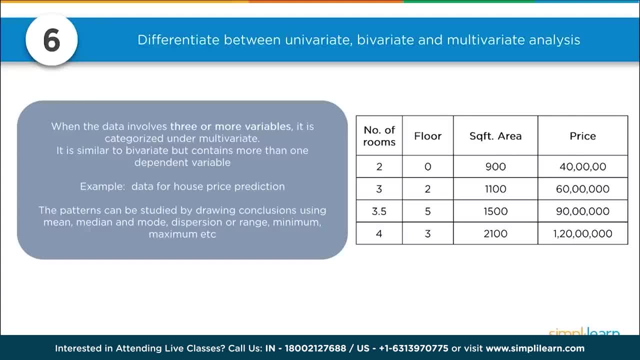 have already looked at the area and you already know that a two bedroom, zero floor, 900 square foot house usually runs about 40,000,. you can guess what the next one that looks similar to it is, And I'll just throw in another word in there I don't see very. 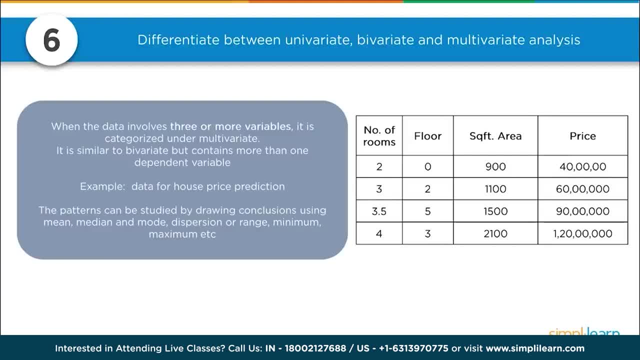 often, unless you're really a hardcore data science. we talked about describing the data, descriptive, we talked about predictive and there's also postscriptive. Postscriptive means we're going to change the variables to try to guess what the outcome is if we change. 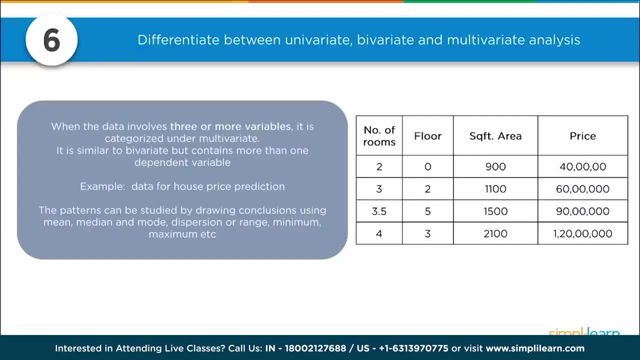 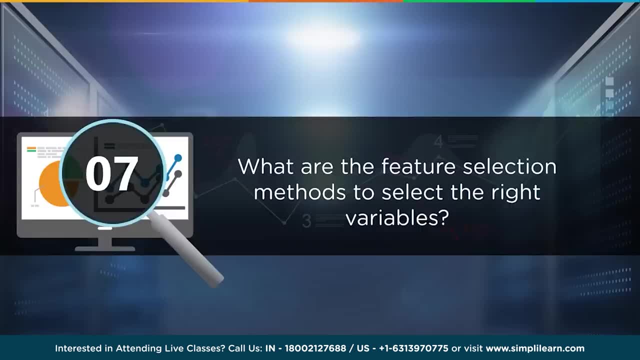 what's going on. So that would be the next step. That usually doesn't show up unless you're dealing with some really hardcore data science groups. What are the feature selection methods to select the right variables? There are two main methods for feature selection. There's: 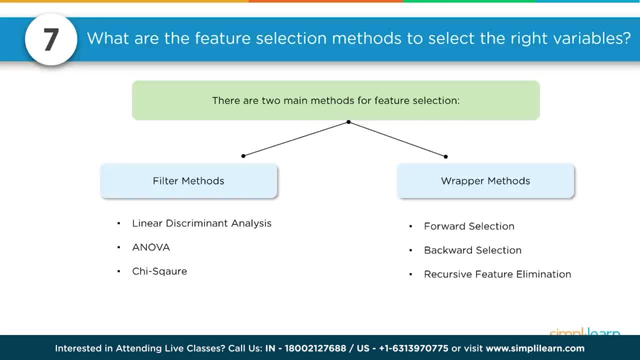 filter methods and wrapper methods And when you're filtering your before we discuss the two methods real quick. the best analogy for selecting features is: bad data in, bad answer out. So when we're limiting or selecting our features, it's all about cleaning up the data coming in. 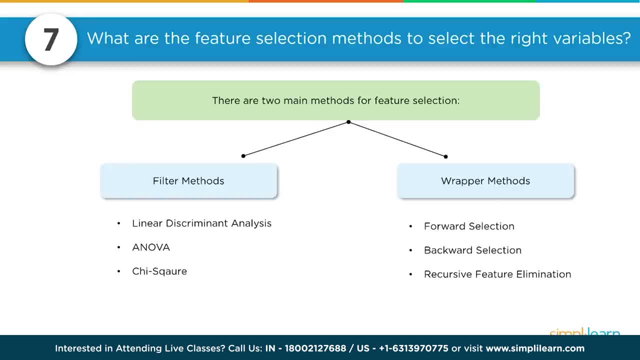 so it's cleaner and is more representative of what we're trying to predict. Filter method: Filter methods as they come in. we have linear discrimination analysis, ANOVA, chi-squared- Chi-squared is probably the most common one- And these are all part of pre-processing. 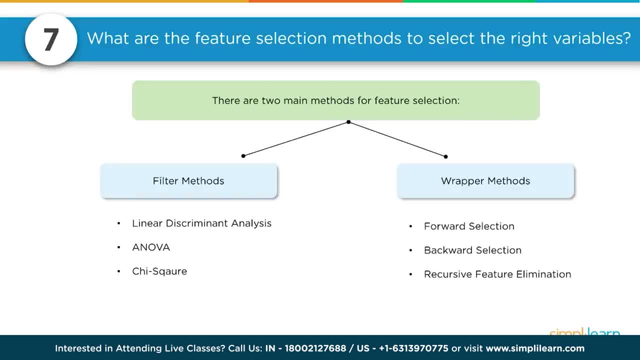 We're taking out all the outliers, all the things that have a difference that is very different from the data. we're looking at the odd ones And sometimes you take the odd ones out and then you analyze them separately to see why they're odd. But remember your. 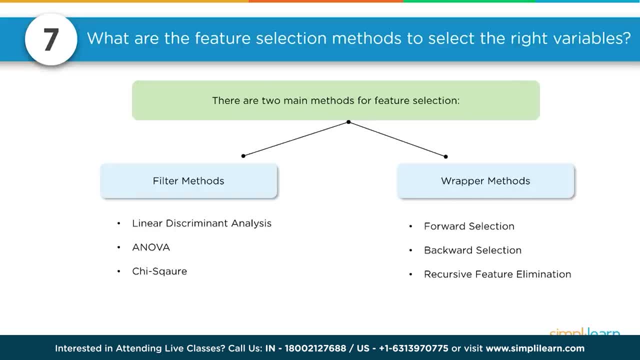 filter methods. you want to pull all that weird stuff out. Wrapper methods, on the other hand, are forward selection, backward selection, recursive feature elimination, And one of the most important things to remember about wrapper methods is they're very labor intensive. 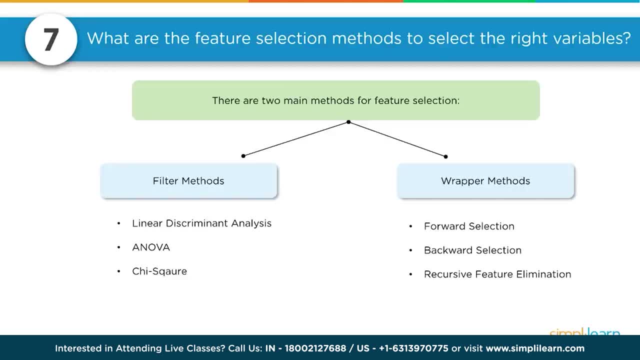 You have to have some pretty high end computers if you're doing a lot of data analysis with the wrapper method And just quickly forward. selection means you have all your different features. They're off to the side and we test just one feature at a time and we keep adding them in. 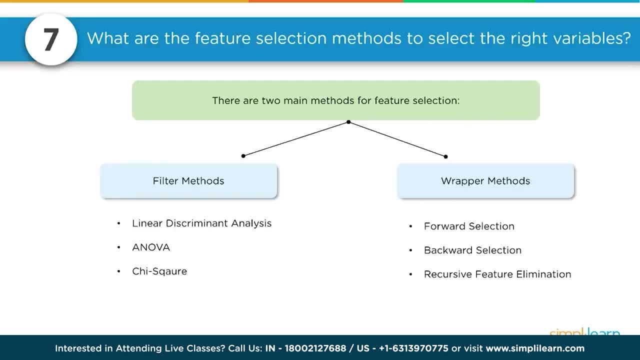 until we get a good fit. Backward is we have all the features and we run a test on that to see how well it does, and then we start removing features to see what works. And recursive, which is the most processing hungry algorithm out there, goes through and just recursively looks through. 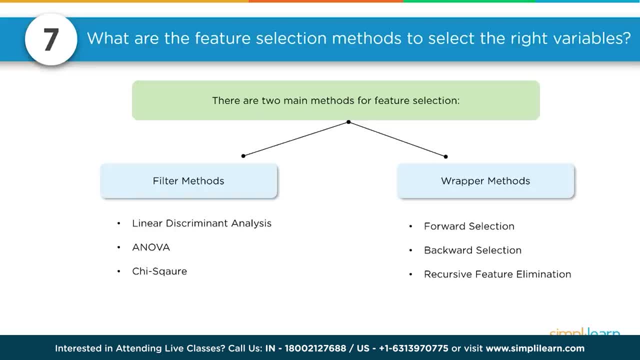 all the different features and how they pair together. But again we have filter method and wrapper method and it's important to understand that we're sorting the data out and finding out which features are going to represent the data the best and which ones are not going to really 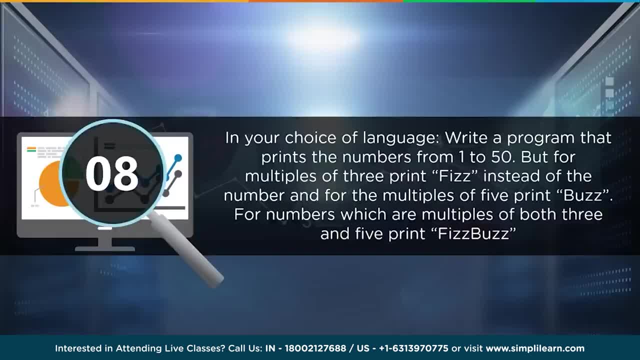 add any value to our models. Alright, let's jump to number eight In your choice of language. write a program that prints the numbers from one to fifty, But for multiples of three, print fizz instead of the number. and for the multiples of five, print. 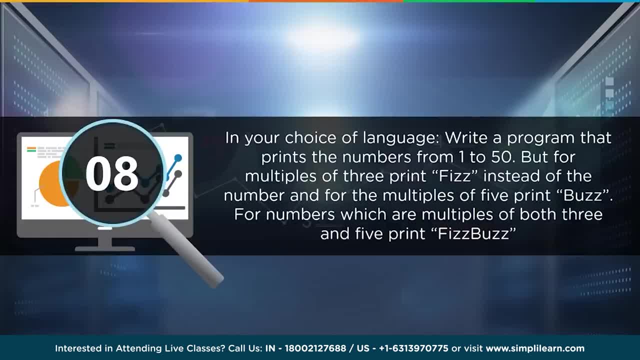 buzz For numbers which are multiples of both three and five print fizz buzz. And this really is testing your knowledge in iterating over data, Very important. My sister, who runs at the university the data science team, is in charge of their department. It's the first question she asks in her. 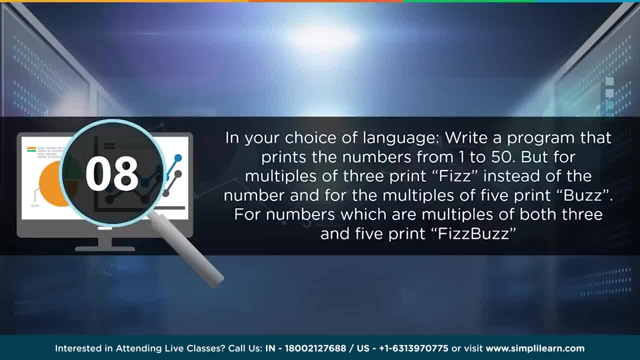 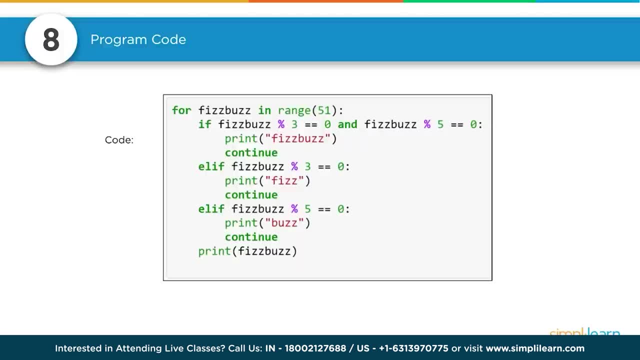 interview of anybody who comes in is: how do they iterate through data? So this question comes up a lot and it's very important you have an understanding. And there's actually a slight error on this code which I'll point out in just a second. The concept: 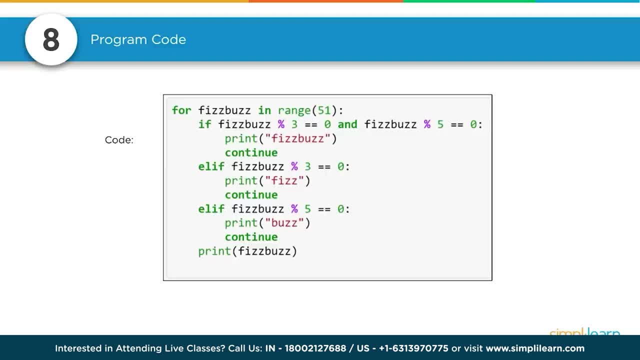 is, we have fizz buzz in range and you have range fifty one, which in this case goes from zero to fifty one, And I'm going to challenge you to see if you can catch the error and I'll tell you at the end of the code where the error is. 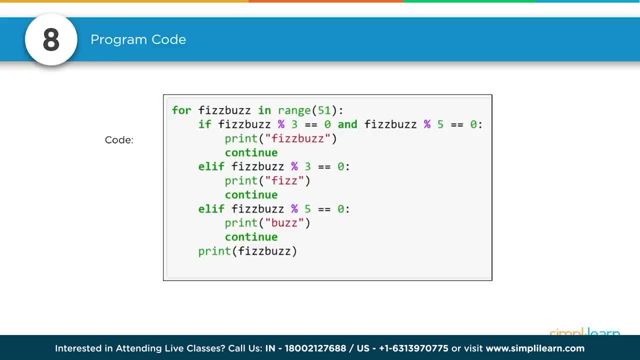 What that means is that we're going to go through all the numbers zero, one, two, three, four, and we're going to process through this loop. If the remainder, fizz buzz divided by three equals zero and fizz buzz divided by five also equals zero, then print. 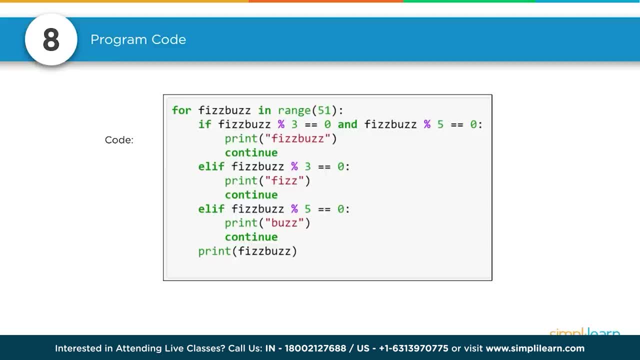 fizz buzz Continue. And else. if fizz buzz divided by three equals zero, then print fizz, Print fizz continue. Else if fizz buzz divided by five equals zero, print buzz continue. and print fizz buzz. You print the answer, In this case fizz buzz. 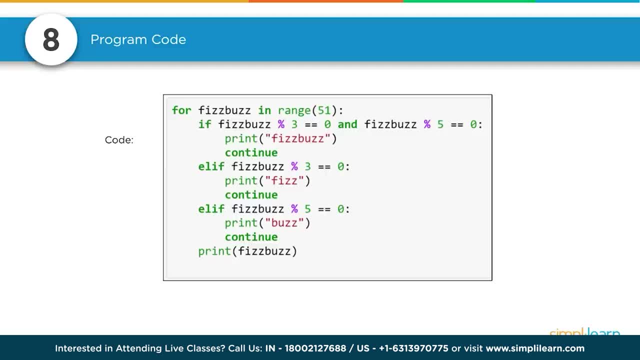 is either going to be the number we generated, which is zero, or it will be the fizz, buzz. fizz or buzz. That's a mouthful. Now, if you didn't catch the error in the code- which is always a fun game- find the. 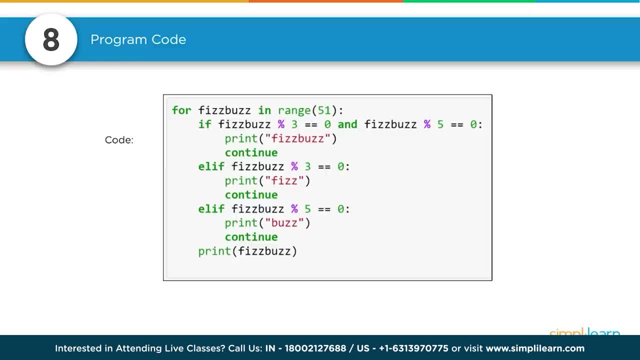 error. it has to do with the range And it's important to remember. the range here says range to fifty one. That's zero to fifty one, which is correct. We want to go to fifty one because it stops. It gets to fifty and it stops. 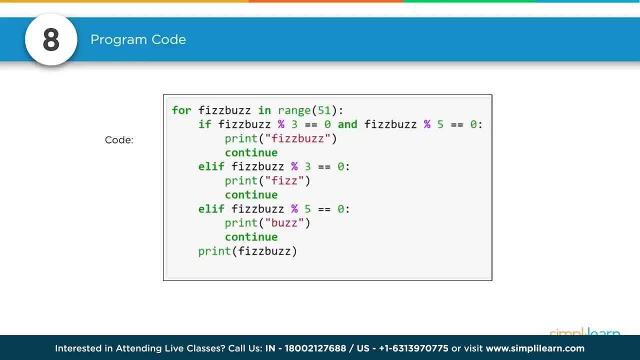 So that's zero to fifty. But if you remember, the question asks from one to fifty. So the range should be one comma, fifty one, not just fifty one, which does zero to fifty one. In this particular script in Python, you can leave out the continue. 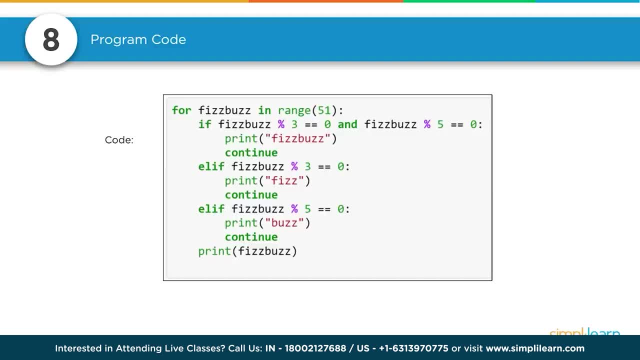 But the continue in this script skips the next else, if so, it doesn't keep processing it going down, And in programming a lot of scripts you don't need the continue in. so this would depend on what script you chose, And there's probably some other ways to do this. This is a lot of fun. 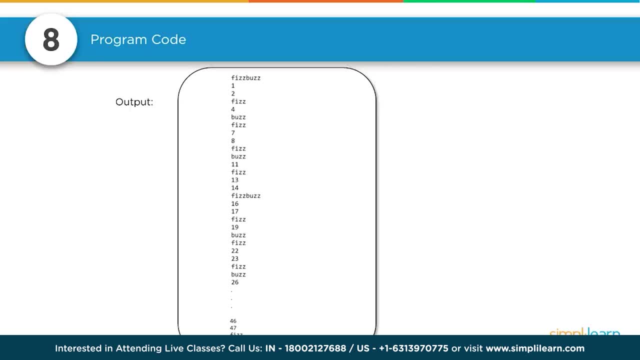 And you can see here from the output, we end up with fizz, buzz for zero, which shouldn't be there: One, two fizz, four buzz, fizz, seven, eight fizz, buzz, eleven fizz and so on. Sounds like a drinking game from my college days. 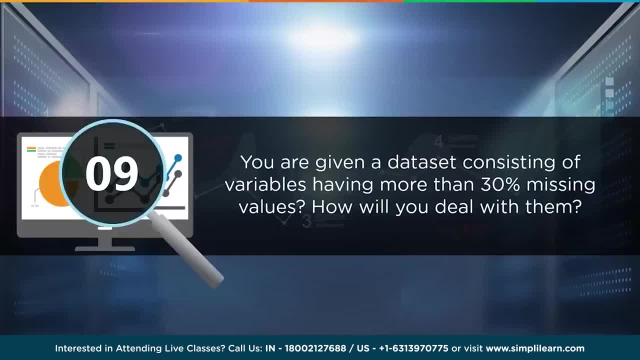 So long ago, many decades ago. You are given a data set consisting of variables having more than thirty percent missing values. How will you deal with them? The joy of messy data coming in. Ways to handle missing data values. Data set is huge. We can. 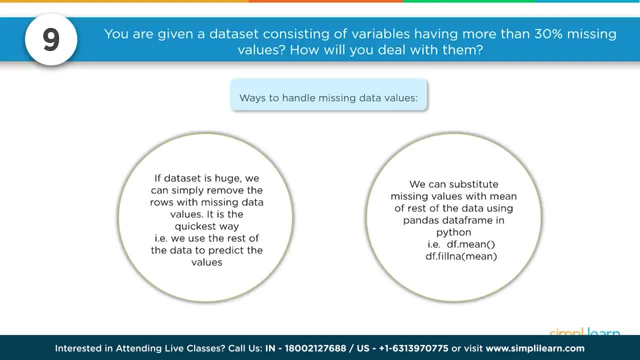 just simply remove the rows with missing data values. It is the quickest way. Ie we use the rest of the data to predict the values. You just go in there and say: any row of our data that has a NA in it, get rid of it. That doesn't work. 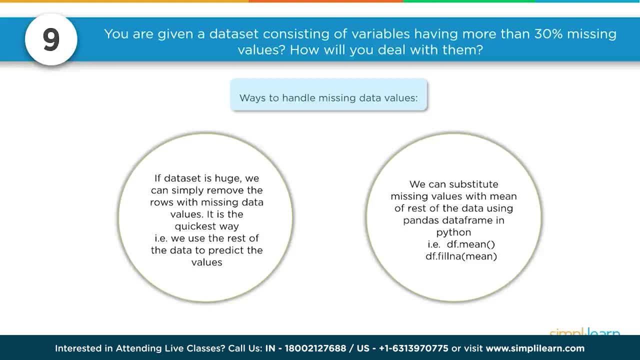 with smaller data. So with smaller data you start running into problems because you lose a lot of data, And so we can substitute missing values with the mean or average of the rest of the data using Pandas DataFrame in Python. There's different ways to do this. 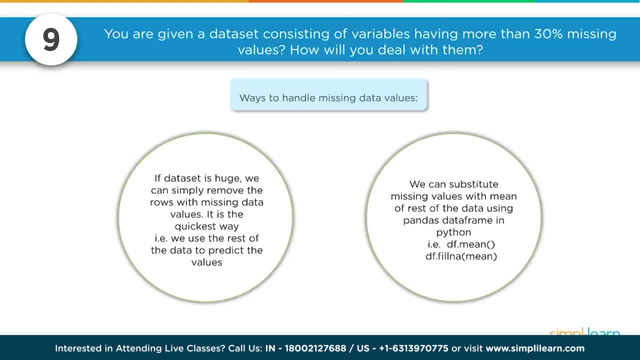 obviously in different languages and even in Python there's different ways to do this. But in Python it's real easy. You can do the dfmean so you get the mean value. So if you set mean equal to that, then you can do a dffillna with. 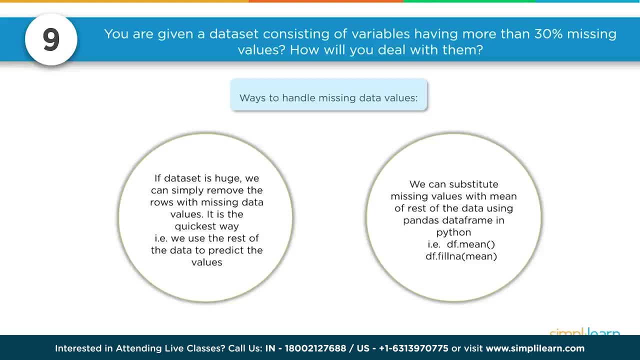 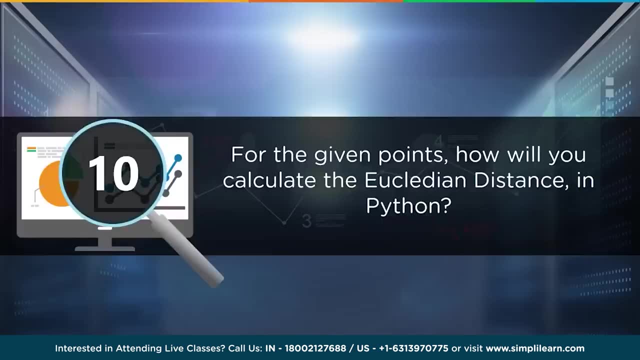 the mean value. Very easy to do in a Python Pandas script And if you're using Python you should really know Pandas and NumPy Number Python and Pandas DataFrames For the given points. how will you calculate the Euclidean distance in? 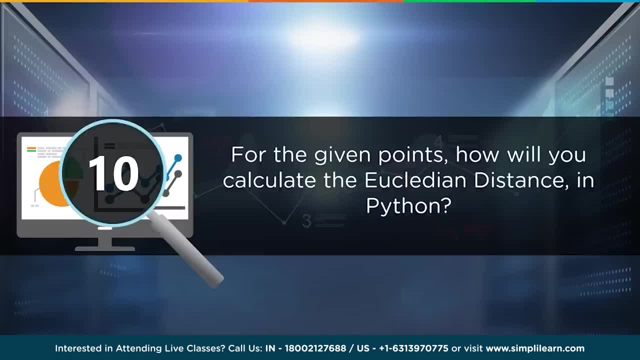 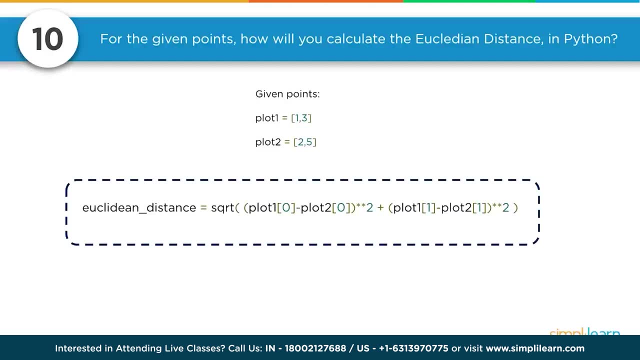 Python. So back to our basic algebra from high school. Euclidean distance is the line on the triangle And so if we're given the points, plot1 equals 1 comma 3,, plot2 equals 2 comma 5, we know that. 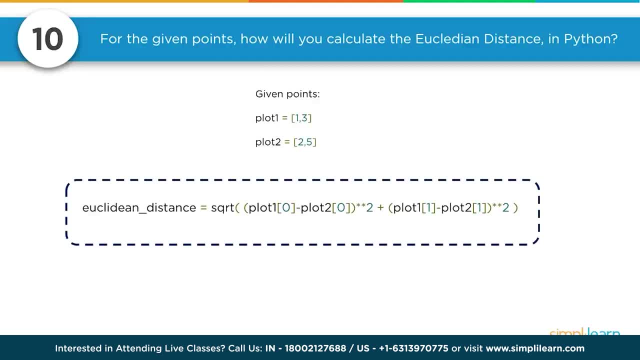 from this we can take the difference of each one of those points, square them and then take the square root of everything. So the Euclidean distance equals the square root of plot1- 0 minus plot2 of 0 squared plus plot1 of 1 minus. 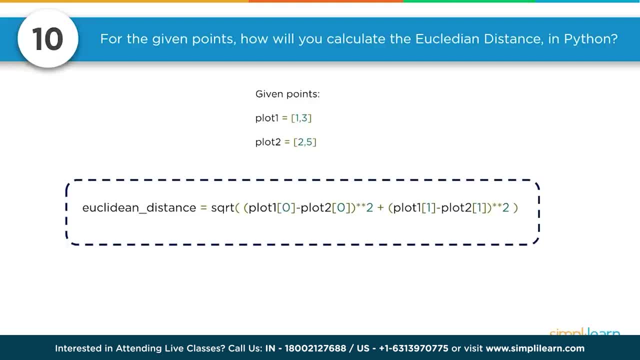 plot2 of 1 squared Mouthful there And you can remember. if you have multiple dimensions that go past two dimensions, you could have. plot3 can simply be the distance from plot1.. You only need to do one side of that Or plot2. you can do either. 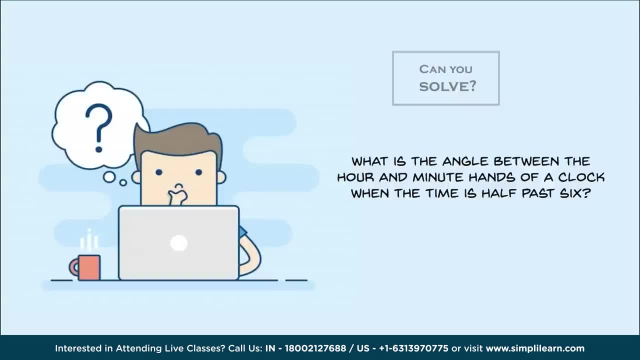 way and square that and take the square root of that. Another mind bender: How to calculate, how to figure out the solution to something? What is the angle between the hour and minute hands of a clock when the time is halfed past 6?? So you want? 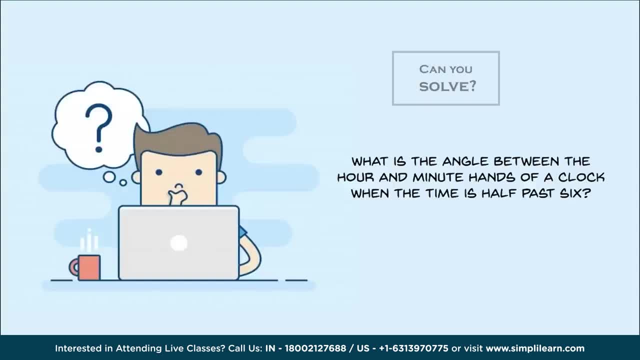 to kind of imagine that clock where the large hand is pointed down to the 30 and the other hand is going to be right between the 6 and the 7 because it's half past 6.. There's actually a couple ways to solve this, but let's take a look and 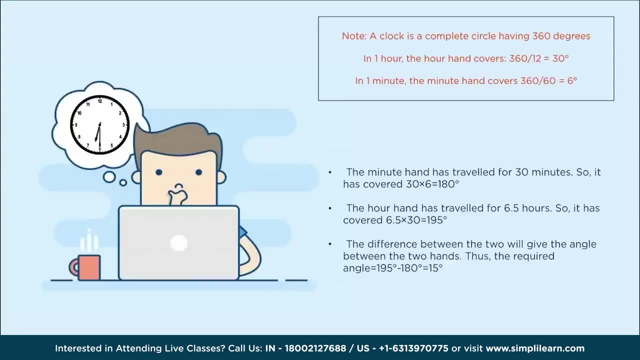 see how they did it. Note: a clock is a complete circle having 360 degrees In one hour. the hour hand covers 360 over 12.. So it equals 30 degrees for each hour In one minute. the minute hand covers 360. 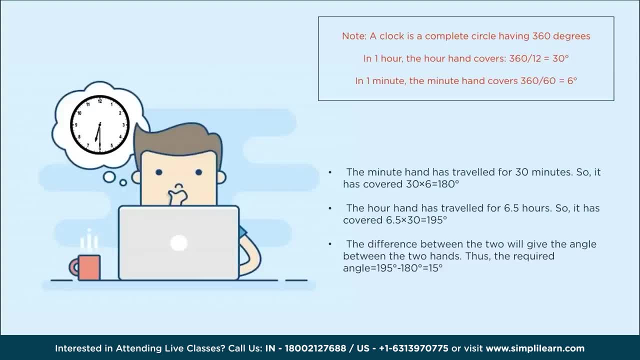 degrees over 60 minutes, or 6 degrees per minute. The minute hand has traveled for 30 minutes, so it has covered 30 times 6, which equals 180 degrees. So we know that's 180 degrees from the 12. The hour. 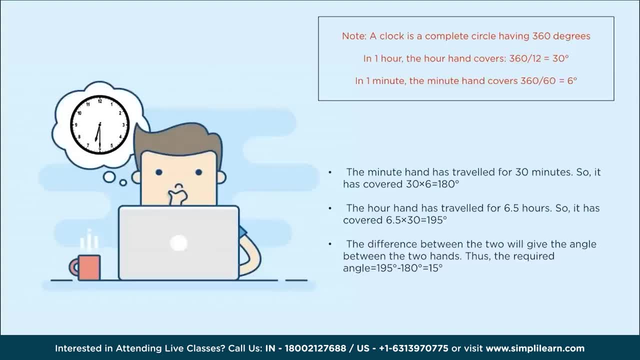 hand has traveled for 6.5 hours- 6 and a half 6.5. so it's covered 6.5 times 30, which equals 195 degrees. The difference between the two will give the angle between the two hands. thus the required angle equals 195. 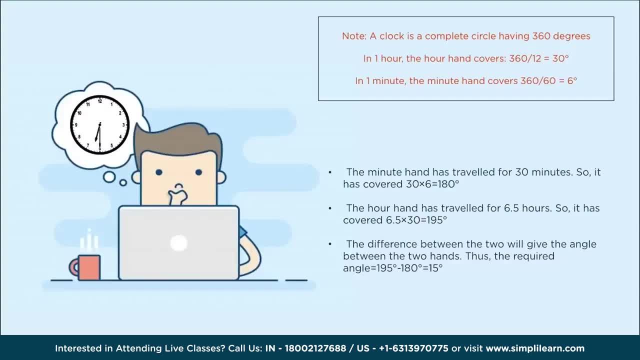 minus 180 equals 15 degrees, And this is nice the way they solved it, because you can now punch in any kind of time within reason. The hard part is on the hours, is you have to be able to convert the hours into decimals. Explain. 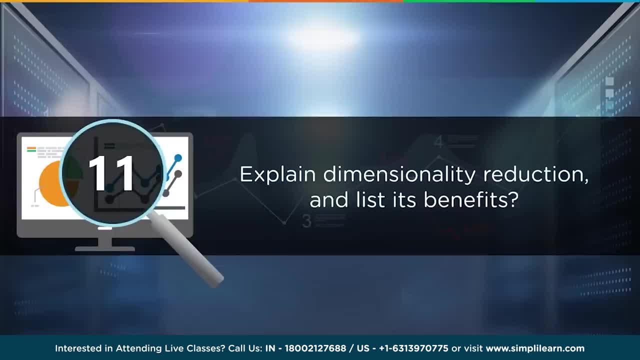 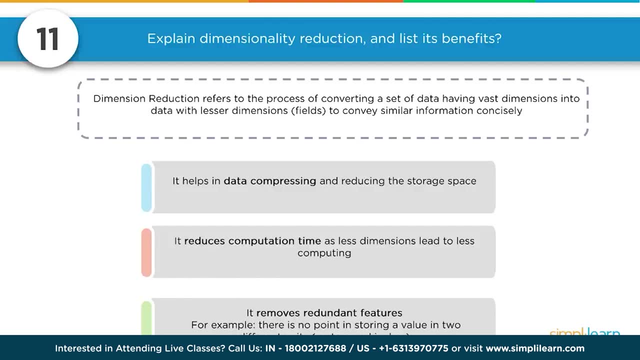 dimensionality reduction and list its benefits. Dimension reduction refers to the process of converting a set of data having vast dimensions into data with lesser dimensions. fills to convey similar information concisely. It helps in data compressing and reducing the storage space. 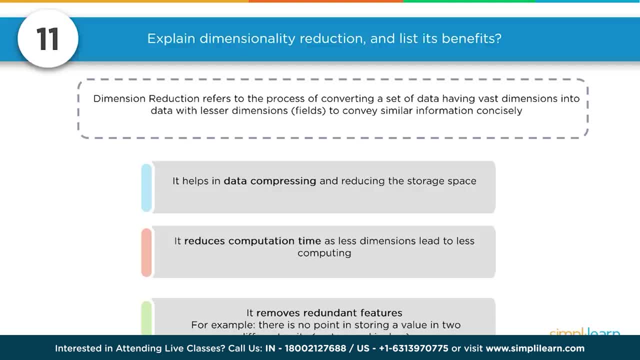 It reduces computation time, as less dimensions lead to less computing. It removes redundant features. For example, there is no point in storing a value in two different units- meters and inches. And I certainly run into a lot with this, with text analysis. I've been known to run a text analysis. 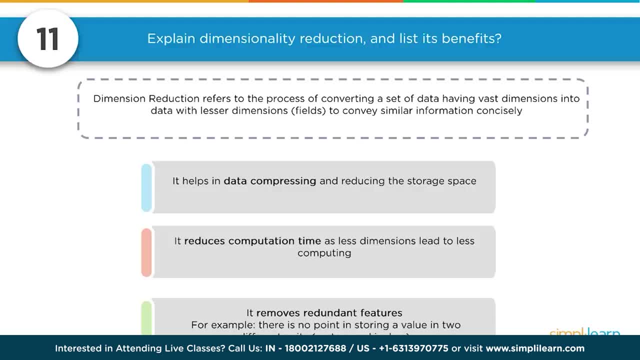 over a series of documents that ends up with over 1.4 million different features. That's a lot of different words being used, And if you do what they call a buy-connect-em, you connect two words together. now you're up to 4.8 million different. 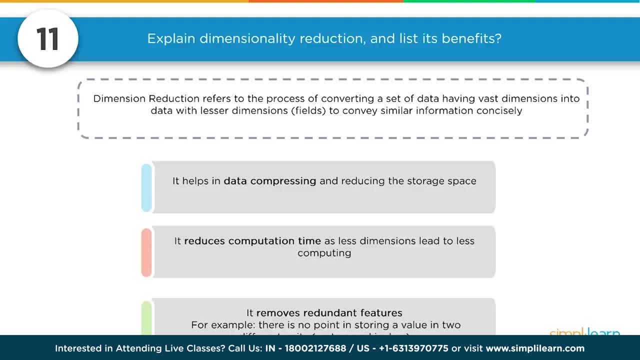 features and you start having to figure ways to bring that down. What can we get rid of That kind of thing? So you can see where that can get really high in unprocessing and learning how to reduce the list of dimensions is very important. How will you? 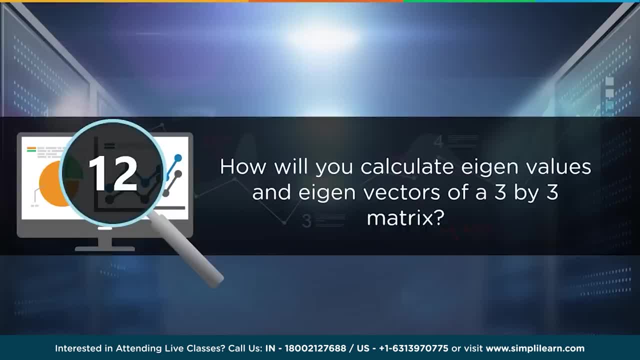 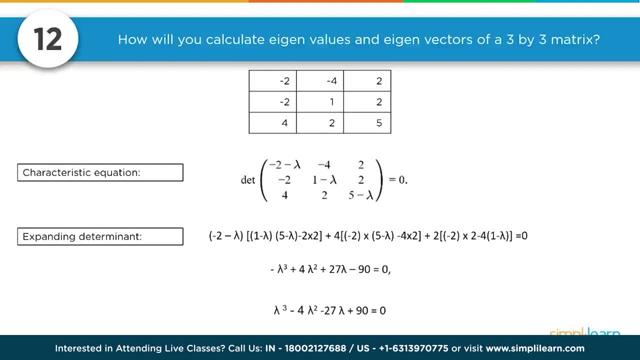 calculate eigenvalues and eigenvectors of a 3x3 matrix, And what they're really looking for here is, when you write it out for the eigen is that you know that you're going to use the lambda. that's the most common one. Obviously, you can use any. 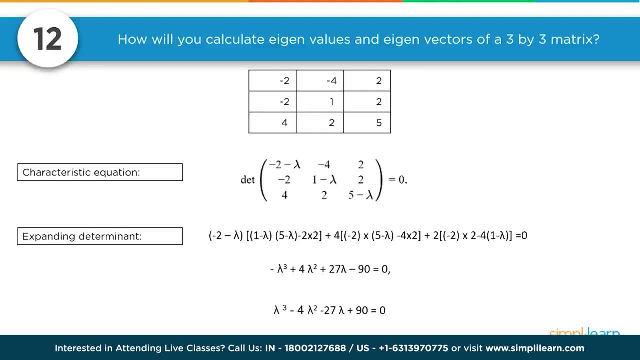 symbol you want, but lambda is usually what they use, And that you do it down the middle diagonal. And so when you take that matrix and you take the characteristic equation, you end up with the determinant and that's minus 2, minus lambda, minus. 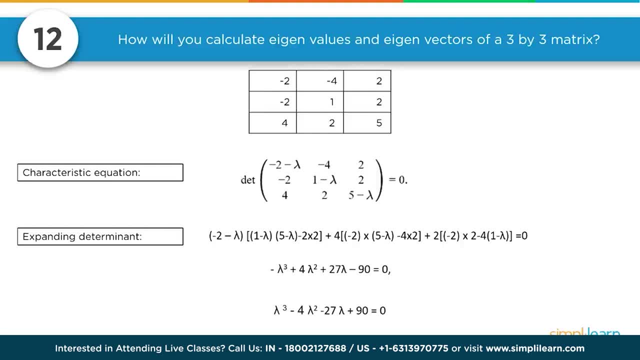 4, 2, minus 2, 1 minus lambda, 2, 4, 2, 5 minus lambda, And that's what they're looking for, and you know that's equal to 0.. So when you're, 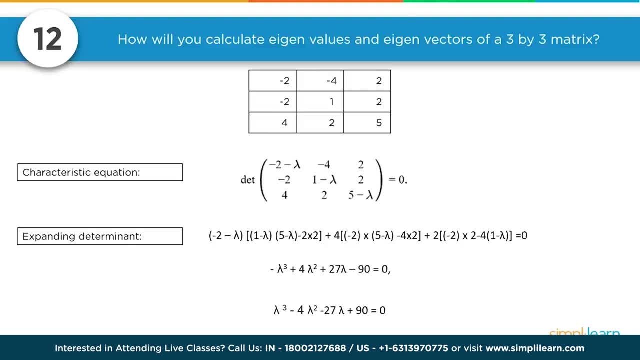 doing a matrix in the eigen setup with the eigenvectors, that's all going to come out equal to 0. And then you can go ahead and write the whole equation out so we can expand the determinant. As you can see right here, the minus 2 minus. 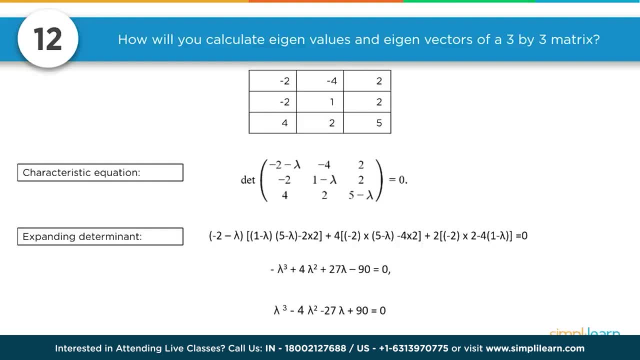 lambda times. it's a mouthful. I'll leave it up here for a second so you can look at it. When you break it down into the algebraic functions, you end up with minus lambda cubed plus 4 lambda squared plus 27. 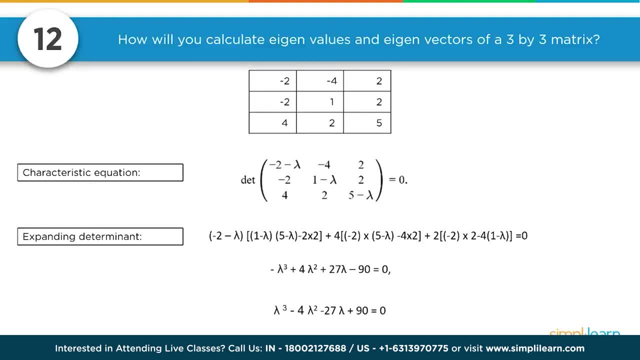 lambda minus 90 equals 0. So now we have a nice algebraic equation built from the eigenvectors. And always remember you can hit the pause button And you can also send a note. Send a note to Simply Learn if you have more questions on. 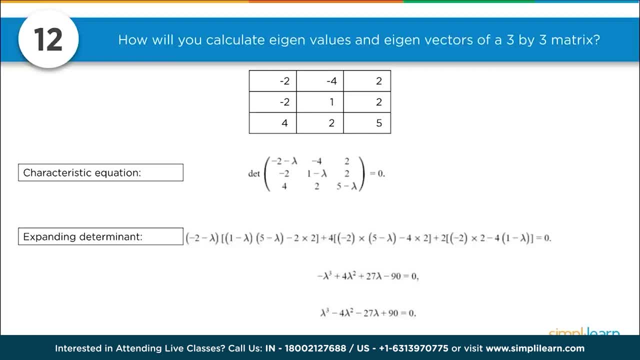 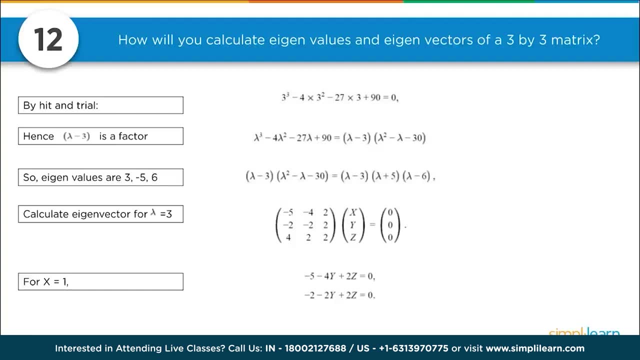 vectors or on this, Definitely have that resource available to you Or post down below on the YouTube video comments. And so when we calculate the eigenvalues and eigenvectors of a 3 by 2 by 3 matrix as we continue on down, 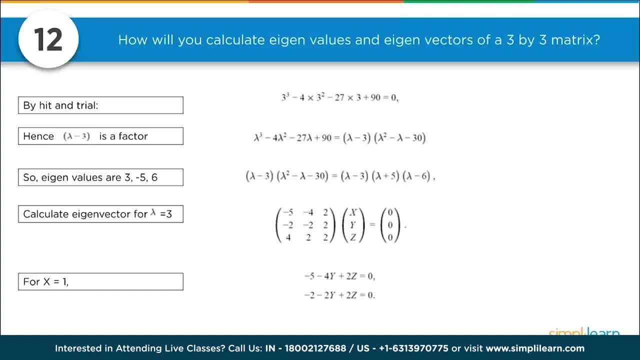 the math of this And, to be honest, I really don't like working with matrixes like this. It's important to understand the math behind it, and it's important to know the code Just enough so that you're not lost when someone's 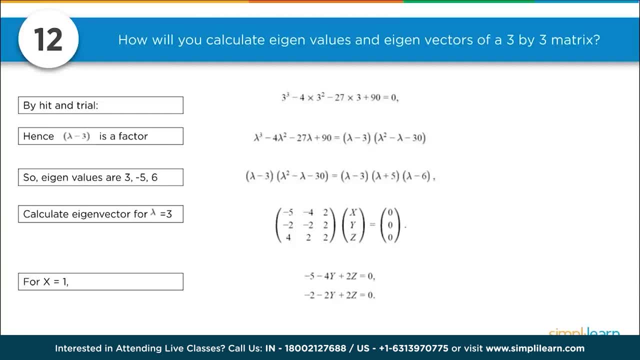 explaining it, or it comes up when I'm working on different data science models. Of course, if you're dealing with the high end math side of it, then you better know this. First is by hit and trial, So you try in different variables to solve for 0.. 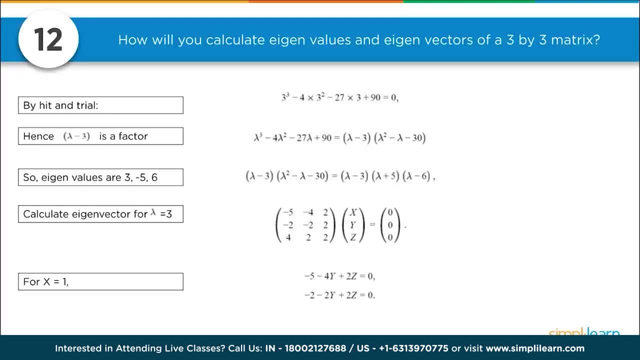 And you can come in here and you'll find that if we put in the 3 in there, we end up with a 0 at the end And substitute the 3. Hence we end up with lambda minus 3 as one of the factors. 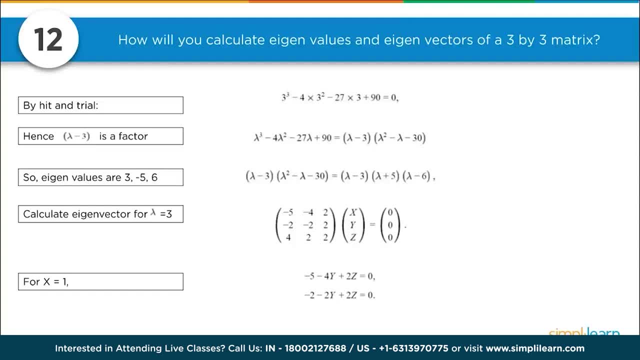 And you can do the math going out on that where we have lambda cubed minus 4, lambda squared minus 27, lambda plus 90 equals lambda minus 3 times lambda squared minus lambda minus 30. So eigenvalues based on that one are 3 minus 5 and 6.. 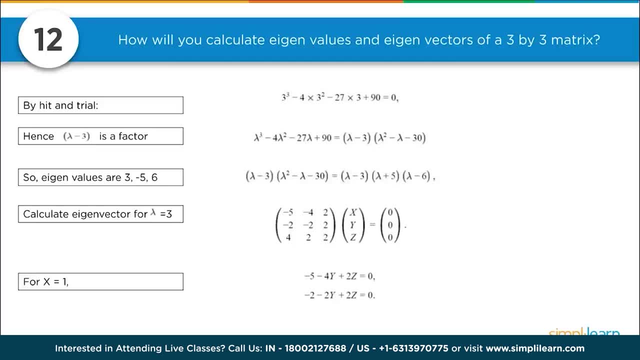 And then from there we can calculate the eigenvector for lambda equals 3.. And you can see here where the matrix as we write it out, is the minus 5 minus 4, 2 minus 2 minus 2, 4 2, 2.. That was from the beginning. 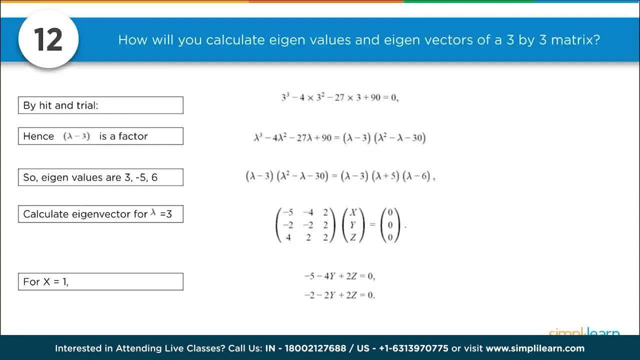 Put in the x, y and z equals 0, 0, 0.. And so when we put in those numbers and we calculate them out, we have for x equals 1, we have the minus 5 minus 4. y plus 2, z equals 0 minus 2 minus. 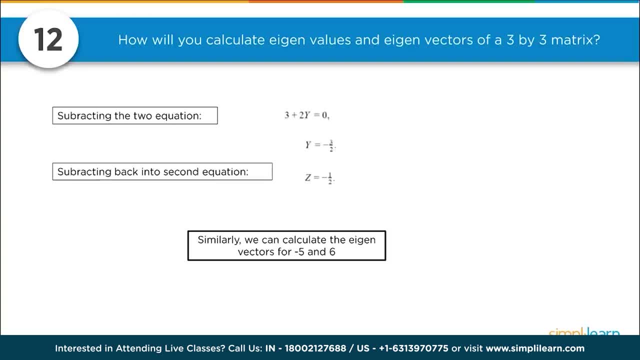 2 y plus 2 z equals 0.. And subtracting the two equations we just had, we get 3 plus 2, y equals 0, y equals minus 3 over 2 and z equals minus 1 over 2.. That's going back to the first equation. 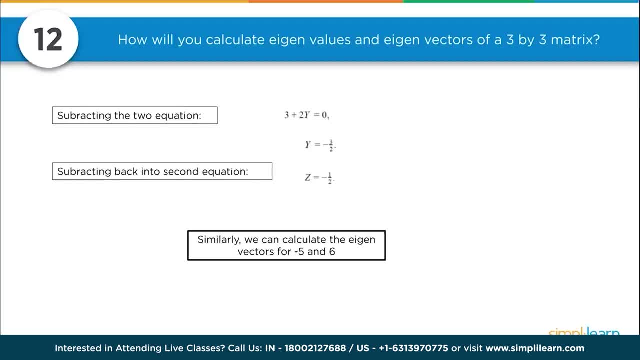 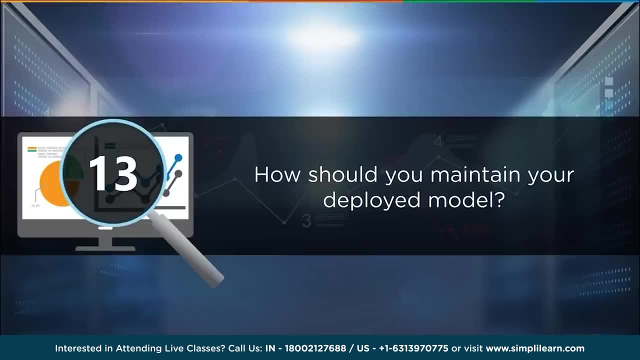 And similarly we can calculate the eigenvectors for minus 5 and 6.. How should you maintain your deployed model? Ooh, distribution time, My favorite. I spent 10 years in software distribution. So first thing- and this is true, not just- 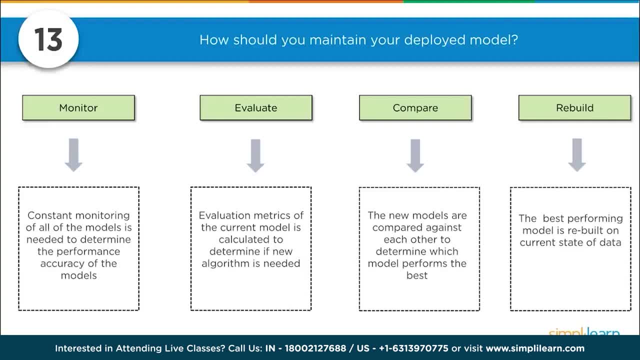 of your data science model, but of any computer code going out there. This is basic setup can work, Although usually there's little added steps in there. First we're going to monitor it So we have a constant monitoring of all the model is needed to. 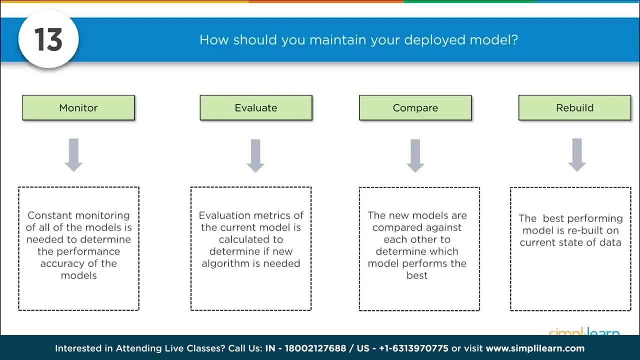 determine the performance accuracy of the models. So yeah, we want to just keep an eye on it, We want to make sure they're accurate, We want to make sure that whatever they're supposed to predict- or I threw in that bonus word- post script, where you 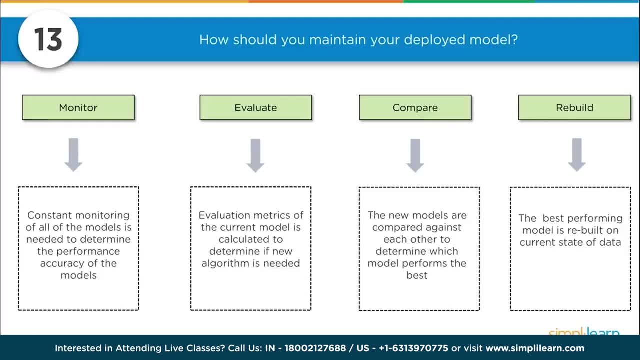 change something and you want to figure out how your changes are going to affect things, We need to monitor it and make sure it's doing what it's supposed to do. Evaluation metrics of the current model is calculated to determine if new algorithm is needed, And then we compare it- The new, 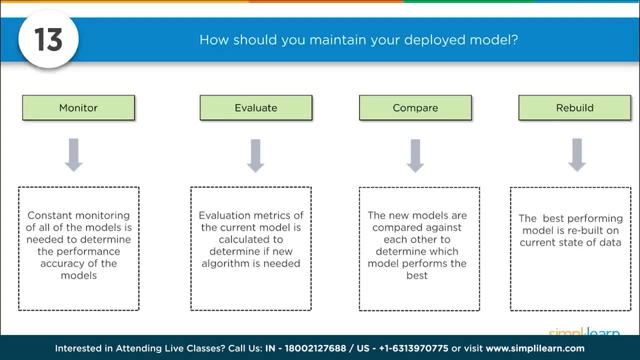 models are compared against each other to determine which model performs the best, And then we do a rebuild. The best performing model is rebuilt on the current state of data And this is interesting. I found this out just recently. If you're in weather prediction. 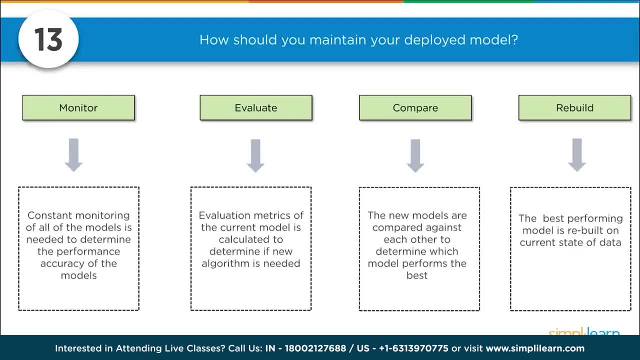 the really big weather areas have about seven or eight different models, depending on what's going on, And so you actually have almost a little forest going on there where they're like which model is going to fit best, and this is what we're going to use to predict. 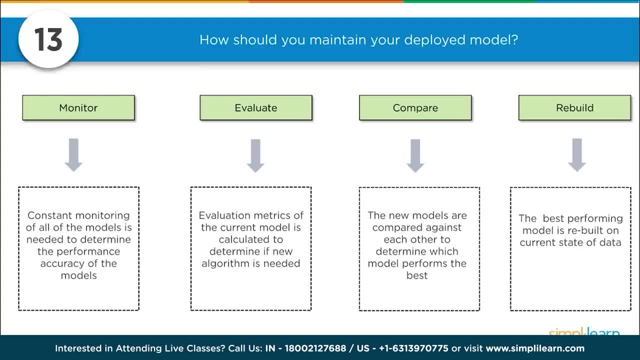 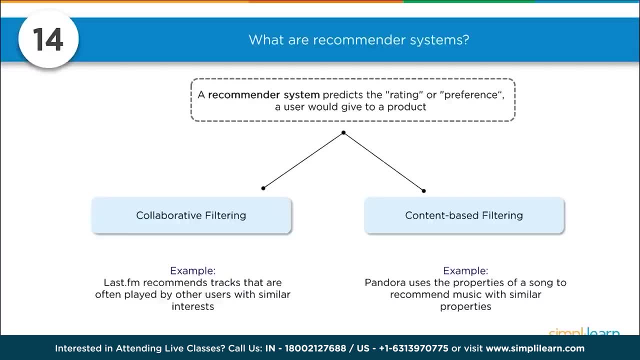 weather with. So not only do you don't necessarily get rid of the models, but you figure out which models fit data of what's going on or the current state of data. What are recommender systems Most commonly used nowadays in marketing? So very big industry. 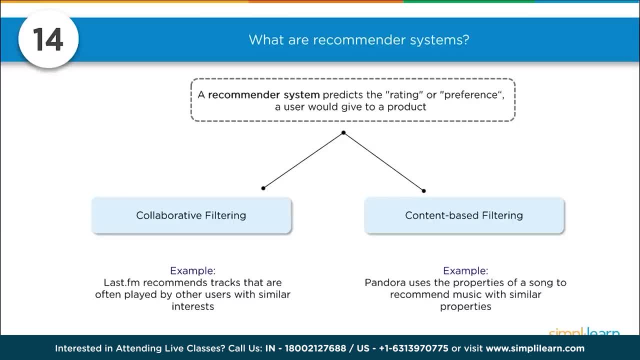 understanding recommender systems predicts the rating or preference a user would give to a product, And they're split into two different areas. One is collaborative filtering, and a good example of that is the lastfm recommends tracks that are often played by other users with similar interests. So people who 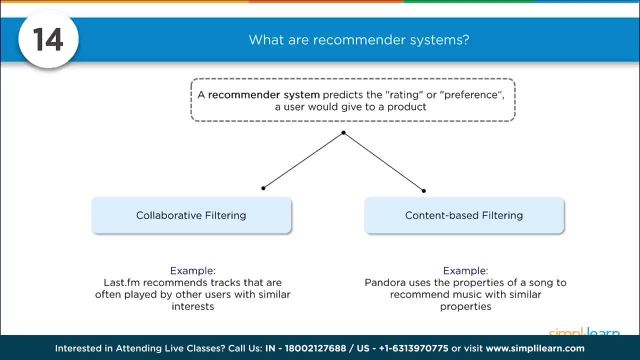 if you're on Amazon, people who bought this also bought that. It's got me a few times. And then there's content based filtering And we're looking at content instead of looking at who else is listening to the music And these example. 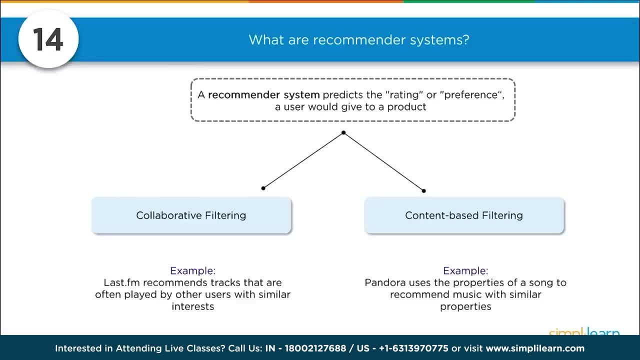 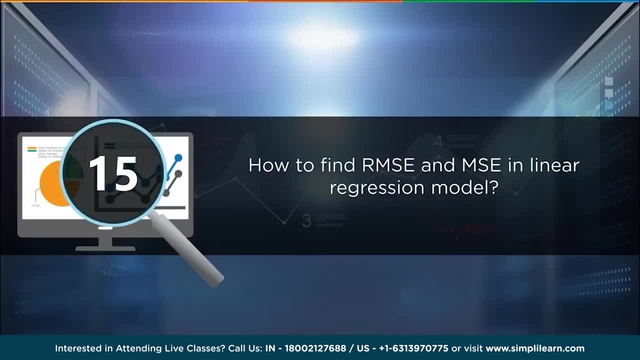 Pandora, which uses the properties of a song to recommend music with similar properties. So you have collaborative filtering and content based filtering. How to find RMSE and MSE in linear regression model. Hopefully you remember what the two acronyms mean, because that is like half the 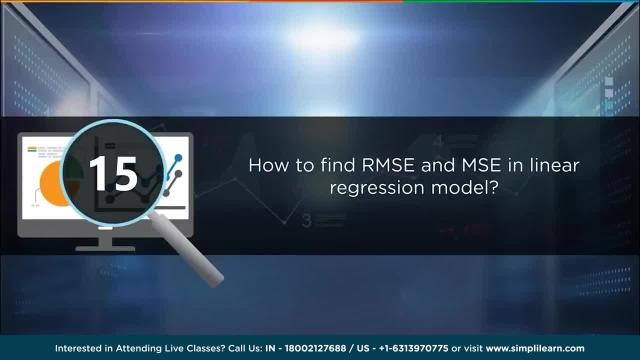 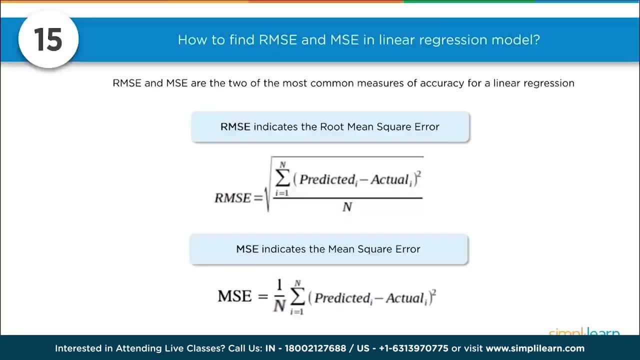 answer. We have the root mean square error and the mean square error in linear regression model, So we're looking for error. The RMSE and the MSE are the two of the most common measures of accuracy for a linear regression model And you can see here we have 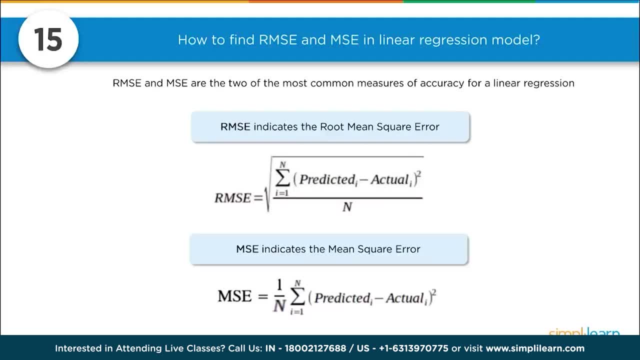 the root mean square error. RMSE equals- and this is the square root of the sum of the predicted minus the actual squared over the total number. So we're just looking for the average mean. So we're looking for the average over the end. 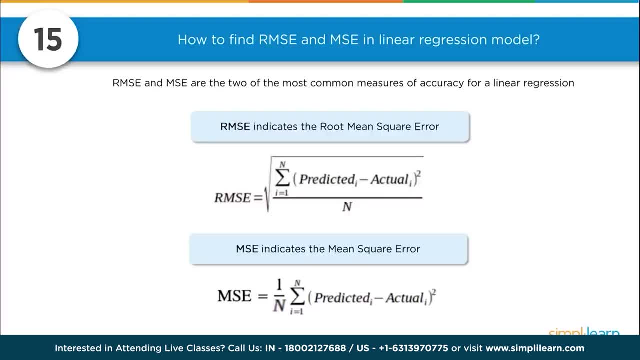 And the reason you need to know about the difference between RMSE versus MSE is when you're doing a lot of these models and you're building your own model, why do you need to take the square root of it? It doesn't change the value as far as the way. 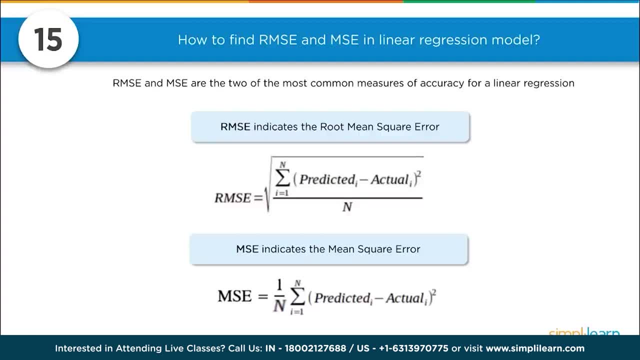 you're using it Because you're looking to see whether the error is greater or less than So why add that extra computation in? So a lot of models use the MSE, which indicates the mean square error or the average error, And it's the same. 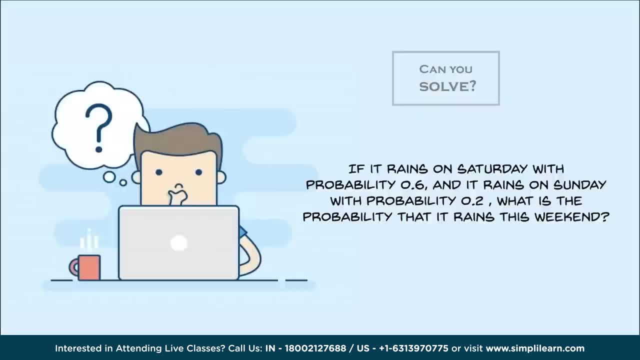 formula minus the square root at the end or across the whole thing. Another riddle to solve: If it rains on Saturday with a probability of .6 and it rains on Sunday with a probability .2,, what is the probability that it rains this weekend? 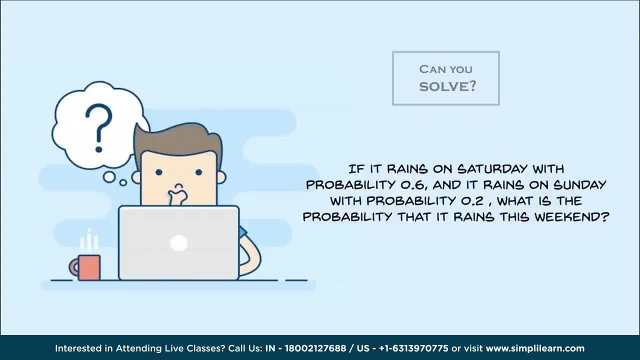 And the trick in probabilities on this case is we need to know what is the probability of it not raining, What's the chance of it not raining on Saturday, And if it doesn't rain on Saturday, we want to take that and combine that with the chance of it not raining. 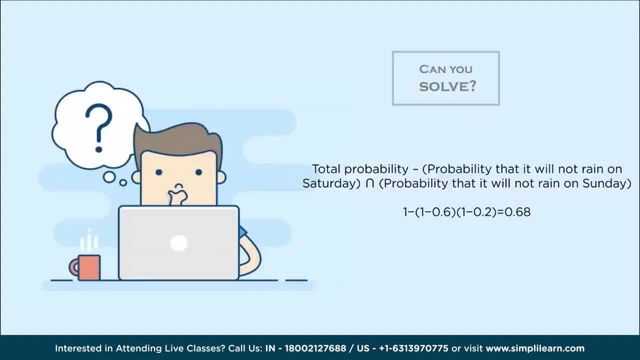 on Sunday, The total probability, which in this case we're just going to use- 1 minus the probability that it will not rain on Saturday. so that's 1 minus .6. we're going to take that as a union, which we simply just multiply them together. 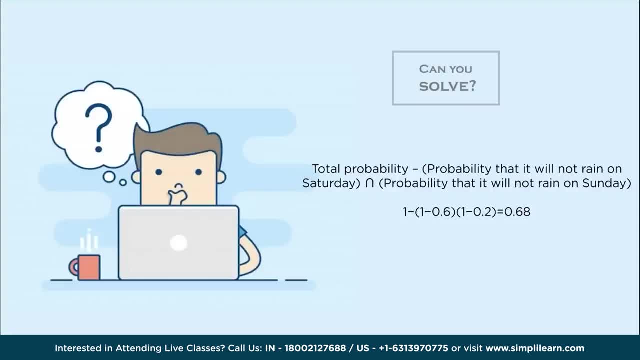 of the probability that it will not rain on Sunday And it's important to recognize the union here or the, and you can see by the formula down here. we end up with .68 or 68% chance that it will rain on the weekend And there are a couple other ways to solve. 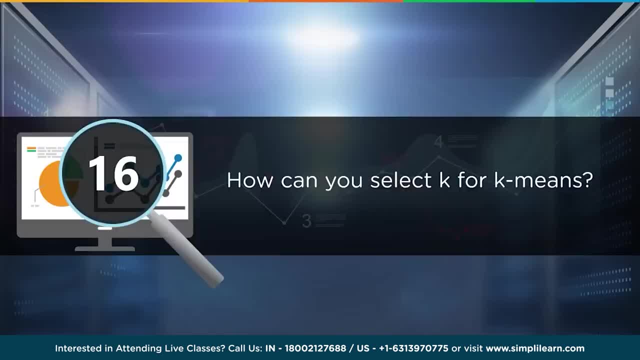 this, but this is probably the most traditional way of doing that. How can you select k for k-means? So first you better understand that what k-means is, and that k is the number of different groupings, And most commonly we use is the ELBO. 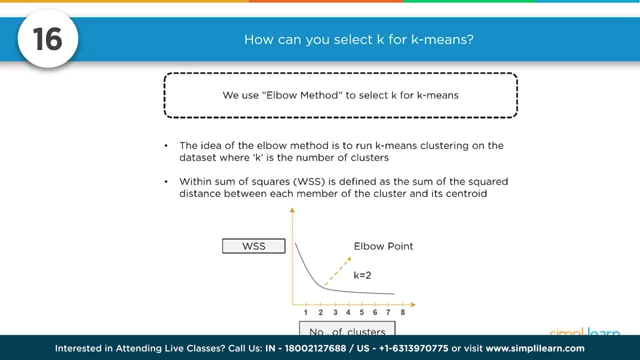 method to select k for k-means. The idea of the ELBO method is to run k-means clustering on the data set, where k is the number of clusters Within the sum of squares. WSS is defined as the sum of the squared distance between each member. 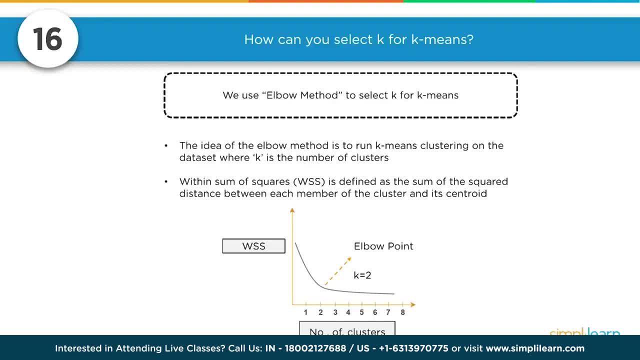 of the cluster and its centroid And you should know all the terms for your k-means on there. And with the ELBO point. and again, here's our iteration. in our code- we talked about that earlier- You iterate starting with. usually you don't start right at 1. 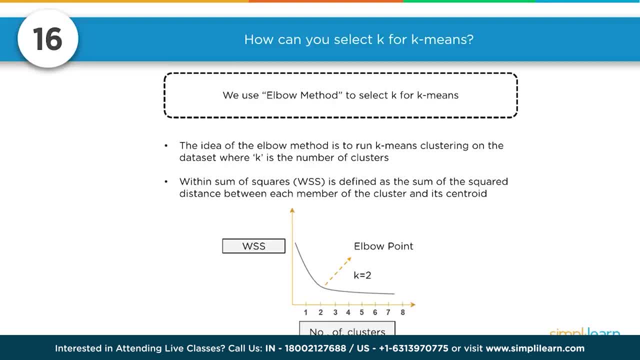 but you might start with 2, 3, or 4 and you just see where it comes out and you can see the nice ELBO there, which is easy to see graphically, where the number of k-clusters and the WSS value drops. 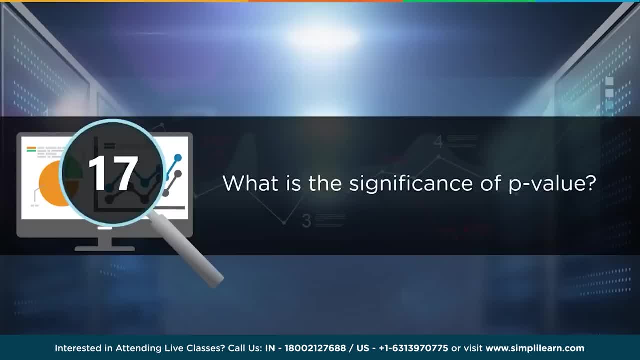 and then it just kind of flattens out and there's no reason to take the any further. What is the significance of p-value? Oh, good one, Especially if you're dealing with r, because that's the first thing that pops up: P-value typically. 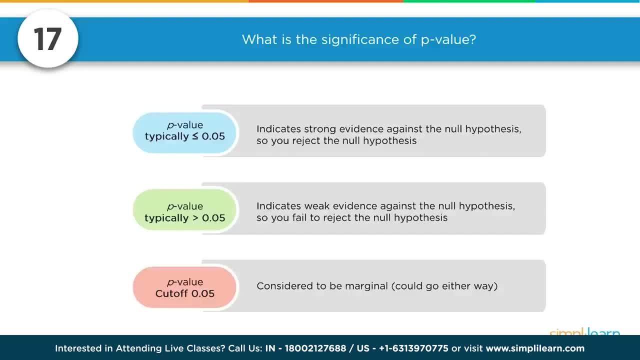 less than or equal to .05 indicates a strong evidence against the null hypothesis and you should know why we use null hypothesis instead of the hypothesis. So you reject the null hypothesis. Very important that term null hypothesis in any scientific setup and also in data science. 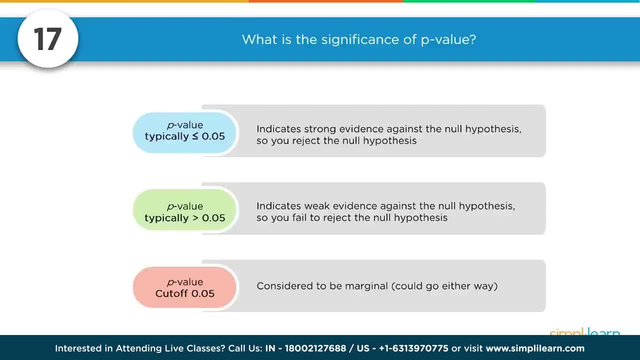 It doesn't mean that it's true. it means that there's a high correlation that it's true. So if your null hypothesis means it's not true, your hypothesis has a high correlation, that it's probably true. And if the p-value is typically greater than .05. 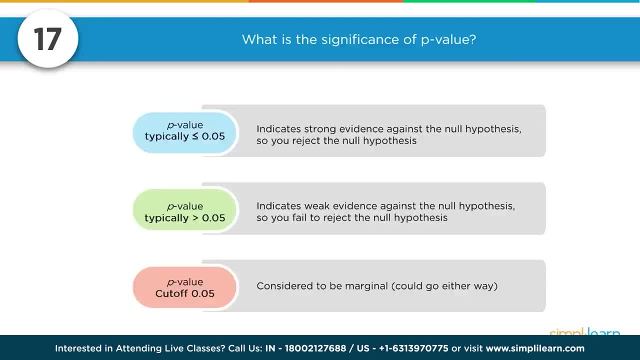 it indicates a weak evidence against the null hypothesis. So you fail to reject the whole null hypothesis and if you reject that, then your actual hypothesis is probably not true. The correlation of your data with what you think it's saying is probably incorrect And if you're right, 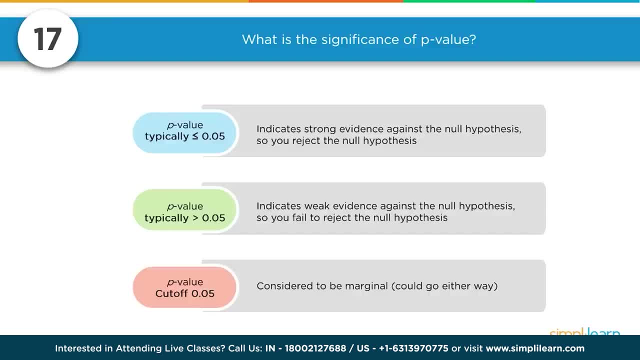 at the cutoff of .05. it's considered to be marginal, Could go either way And again you can use that p-value on different features to decide whether you're going to include your features as far as something worth exploring in your data science model. 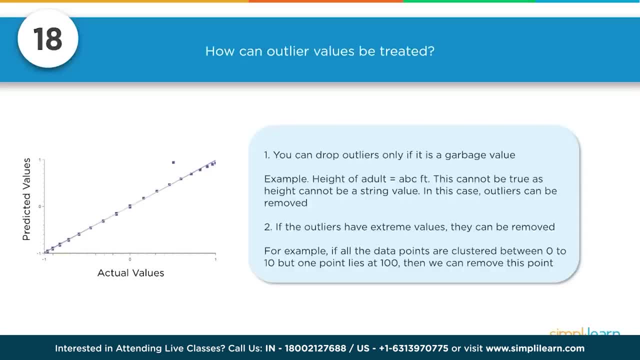 How can outlier values be treated? Ooh, good one. You can drop outliers only if it is a garbage value. So sometimes you end up with like one outlier that just is probably someone's measurements way off. Height of an adult equals abc feet. This cannot. 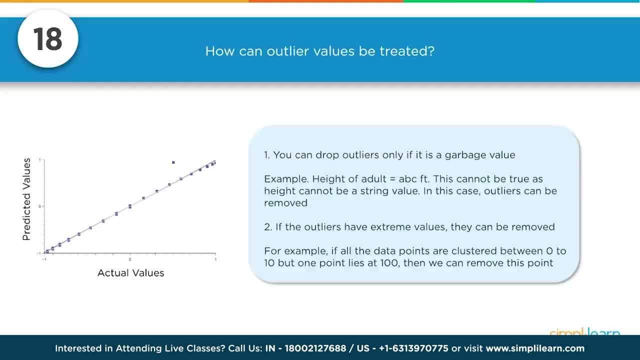 be true, as height cannot be a string value. In this case, outliers can be removed. If the outliers have extreme values, they can be removed. For example, if all the data points are clustered between 0 to 10, but one point lies at 100. 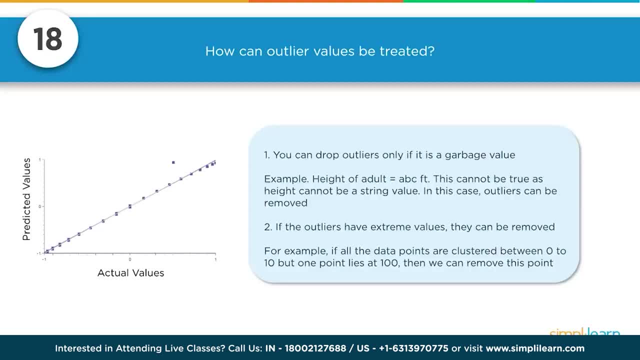 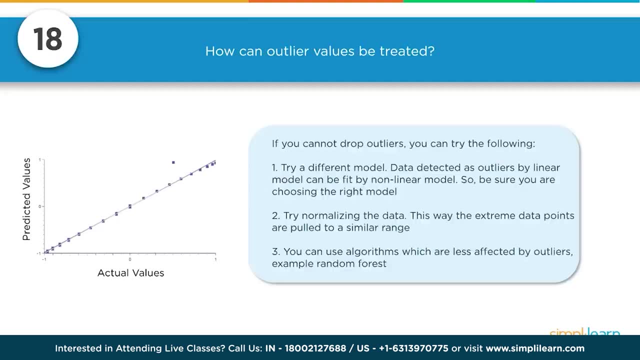 then we can remove this point. And again, sometimes you just look for the outliers so you can see what's going on. If there's something unusual there, So maybe the equipment's not calibrated correctly. If you cannot drop outliers, you can try the following: 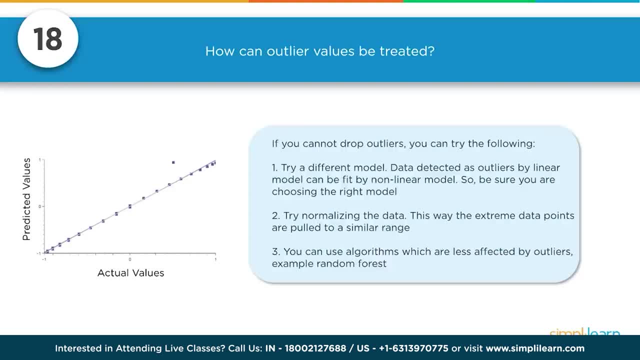 Try a different model. Data detected as outliers by linear model can be fit by non-linear model, So be sure you are choosing the right model. So if it has like more of a curved look to it instead of a straight line, you might need to use something other than just a. 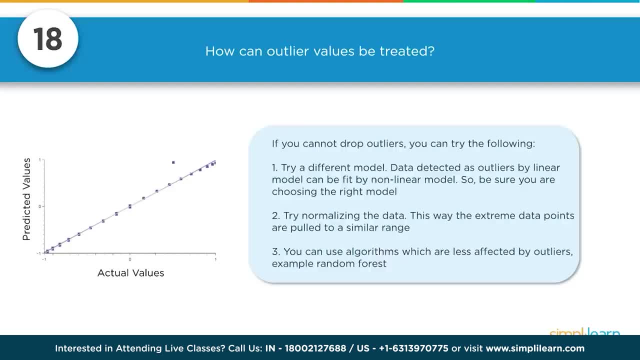 straight line linear model. Try normalizing the data. This way the extreme data points are pulled to a similar range. If you can use algorithms which are less affected by outliers- example: random forest- So there is another solution is you can come up with the random forest. 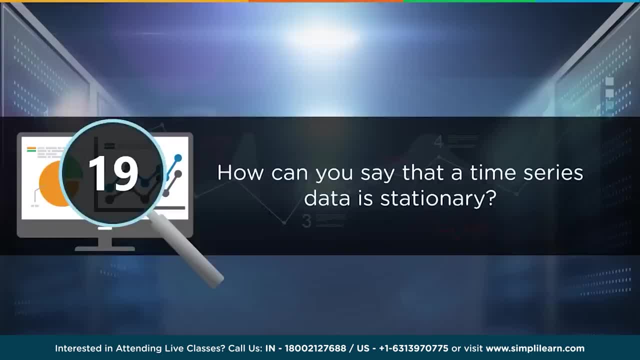 which a lot of times completely bypasses your outliers. How can you say that a time series data is stationary? Oh, that's an interesting term: Stationary meaning it's not moving, but it's a time series. We can say that a time series is stationary when the variance and 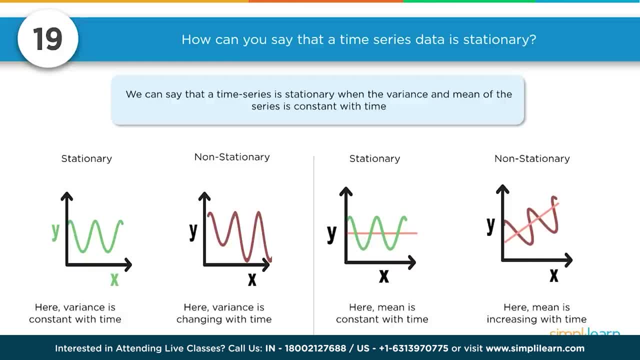 mean of the series is constant with time, And this graphic example is very easy to see. We have our: the variance is constant with time. So we have our first variable, y and x, And x being the time factor and y being the variable, As you. 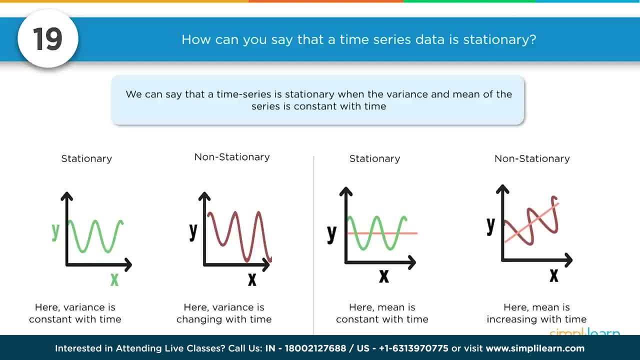 can see, goes through the same values all the time. It's not changing in the long period of time, So that's stationary. And then you can see in the second example the waves get bigger and bigger, So that's non-stationary. Here the variance is: 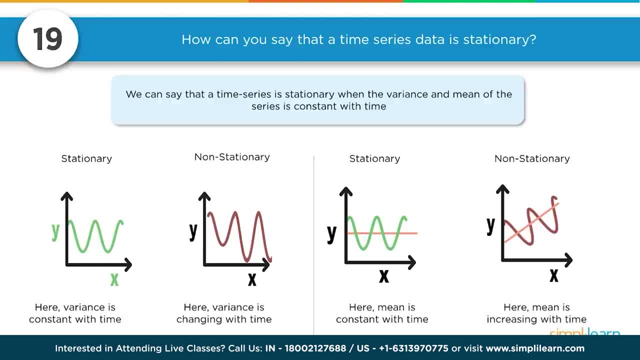 changing with time. Again, we have y, which stays constant, So that if you look at the bigger picture, it's the same wave over and over again. And then of course we have where the wave is growing in size, going up, It can also go down, So it would also be. 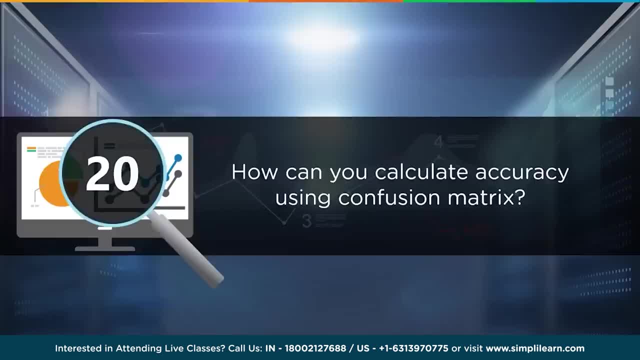 non-stationary. How can you calculate accuracy using confusion matrix? Oh great one. Confusion matrixes are so useful when you're taking that first look at data and also when you're showing the shareholders and you want to ask them for money. How can you calculate? 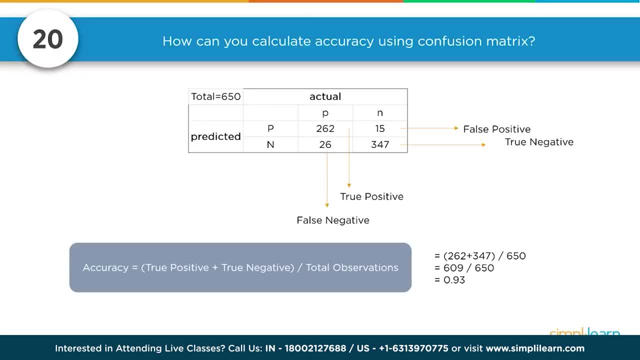 accuracy using confusion matrix. So you have your total data that we're looking at is 650, and you have your predicted values and your actual values, and you have your predicted p and your actual p. And so when you look at this, you'll note that if the predicted p and 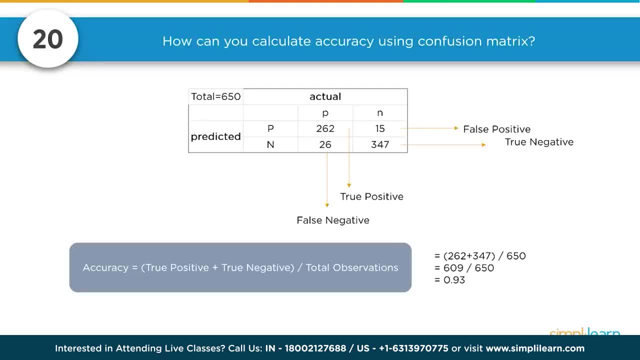 the actual p are 262 but our predicted p also had 15. that weren't correct. So you can see there's a false positive there of 15.. And the same thing with the n. You can see where n predicts n and it has a false negative of. 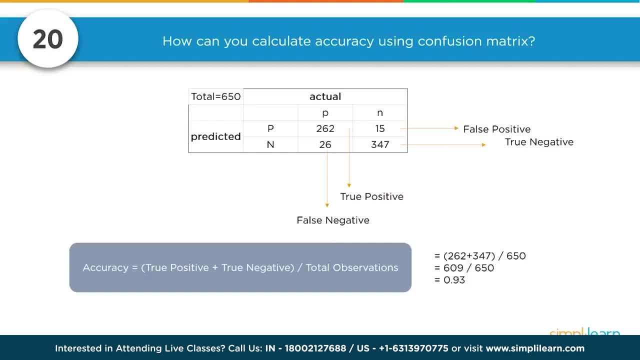 26 out of the total number of n values in there, And so we can do an accuracy on there. The true positive plus the true negative is our total observations. So you have a total of .93 accuracy, or 93%. And just a quick note. 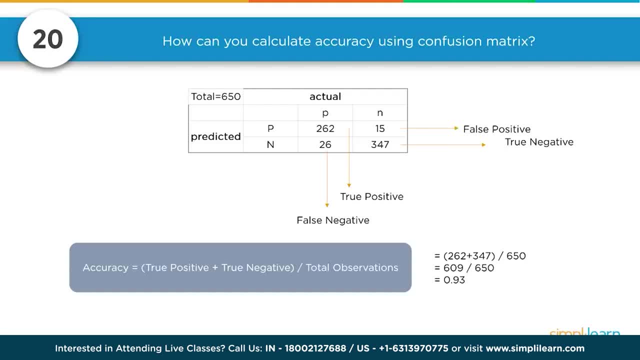 on this. This is so important because it's one thing if someone is being diagnosed with, say, cancer, You know this is life death. or is my nuclear reactor going to blow up Suddenly, if the p is the probability of it blowing up? and let's say: 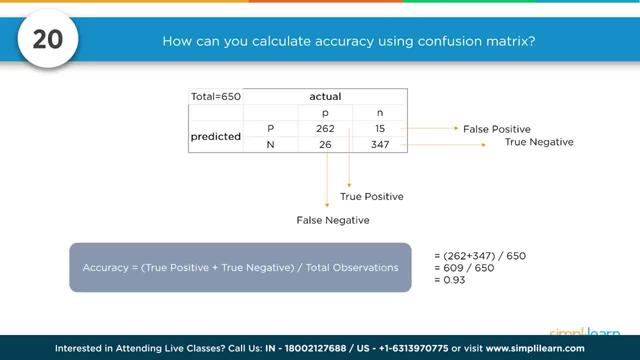 you have 15, that's a lot less than, say, the 26 chances of it blowing up. You know So. the actual domain of your data is very important. So if you're non positive, you don't really care about the predicted value having non. 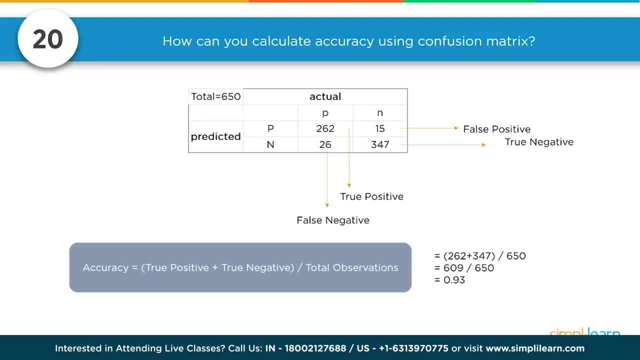 positive as positive because they're going to go do a biopsy on the cancer or whatever anyway. But you're very interested if you have a positive, an actual positive value which is looked at as negative, A false negative. That's really important in that domain, depending on what domain. 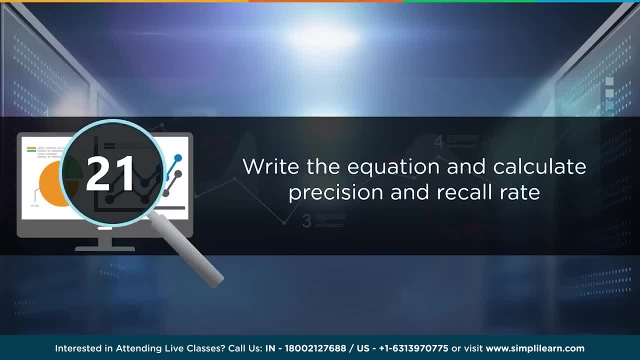 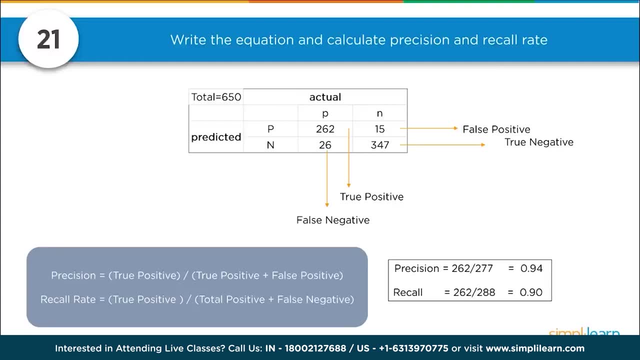 you're in, Write the equation and calculate precision and recall rate And so continuing with our confusion. matrix, I was just talking about the different domains We have. the precision equals 262 over 277.. So your precision is the true, positive over the true. 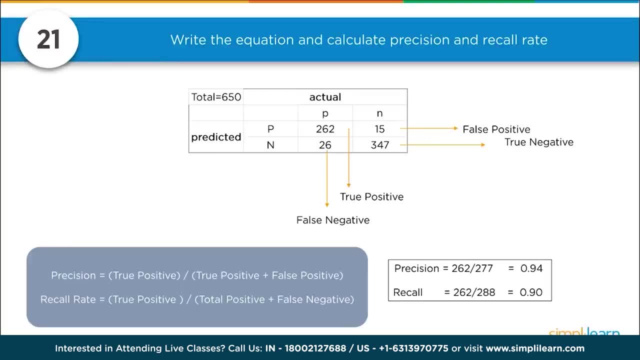 positive plus false positive And the recall rate is your true positive over the total positive plus false negative And you can see here we have the 262 over 277, equals a 94 percent, And the recall over here is the 262 over 280, which equals: 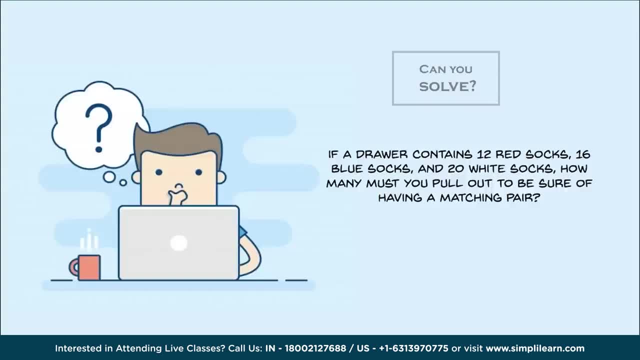 .9 or 90 percent And, oh good, we're going to take a pause for another brain teaser. If a drawer can contain 12 red socks, 16 blue socks and 20 white socks, How many must pull out to be sure of having a matching? 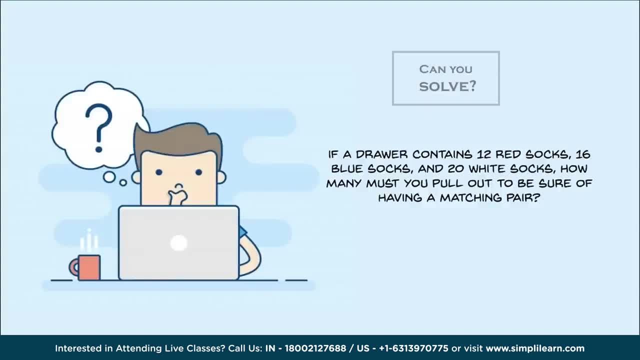 pair. The last time I went through these kind of brain teaser, things was like 20 years ago And I had six people sitting across the table waiting for my answer. That's kind of mind numbing when you're in an interview like that. 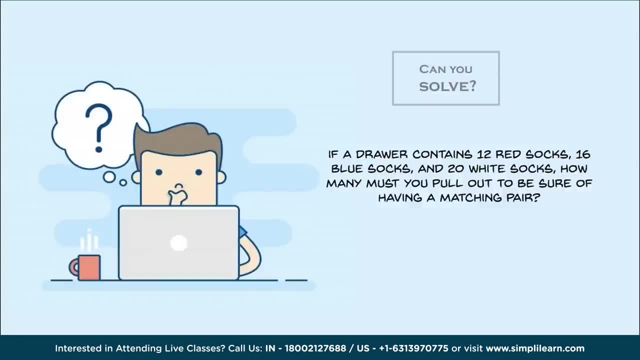 Hopefully you're not stuck in an interview like that, But on this you need to ask yourself how many different colors of socks are there, So they've thrown a lot of extra data in here that you don't need to solve the answer. The answer is four. 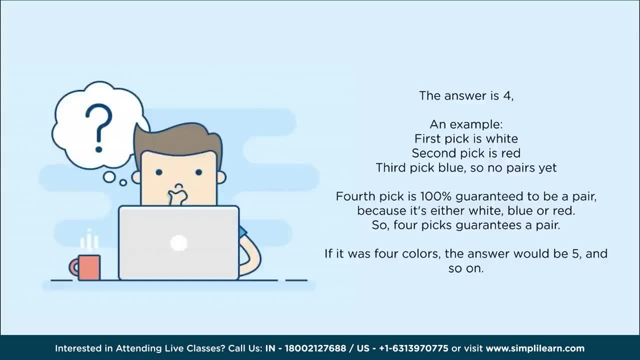 An example: your first pick is white, your second pick is red, third pick is blue. so no pairs yet And that means when you get to the fourth pick, there's a 100 percent chance you're going to have a match. 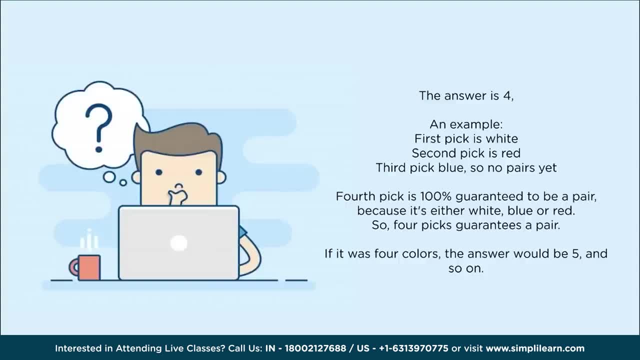 So the most is going to be four that you ever have to pull out of your drawer. If it was four colors, the answer would be five and so on. It doesn't matter how many white socks you have, or how many red socks or blue socks. 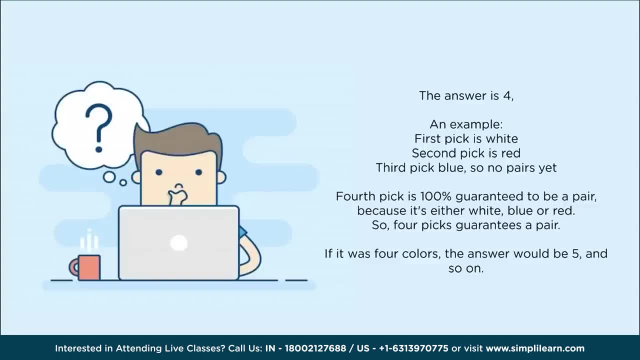 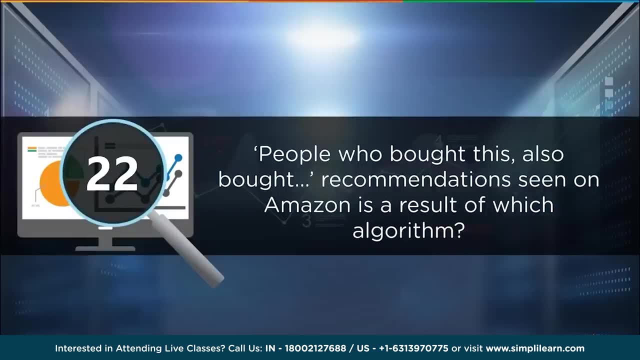 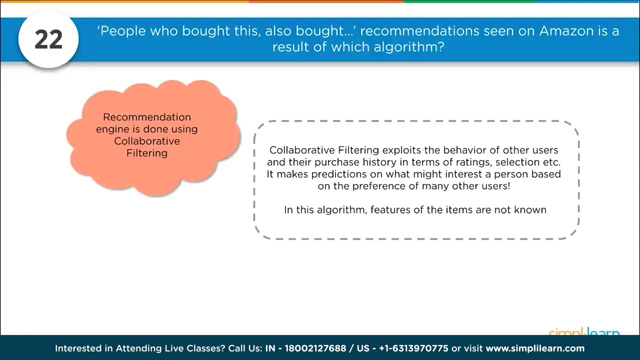 different pairs you have. It's the different colors, the number of different colors. People who bought this also bought recommendations seen on Amazon, as a result of which algorithm- Ooh, we covered this earlier Recommendation engine- is done with collaborative filtering. Collaborative filtering exploits the behavior. 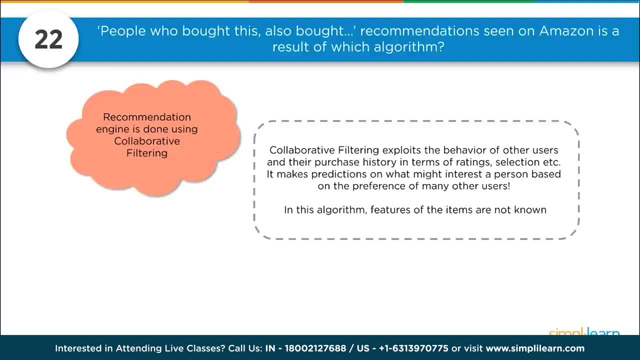 of other users and their purchase history in terms of ratings, selection, etc. It makes predictions on what you might interest a person based on the preference of many other users And this algorithm features of the items are not known, And we have a nice example here. 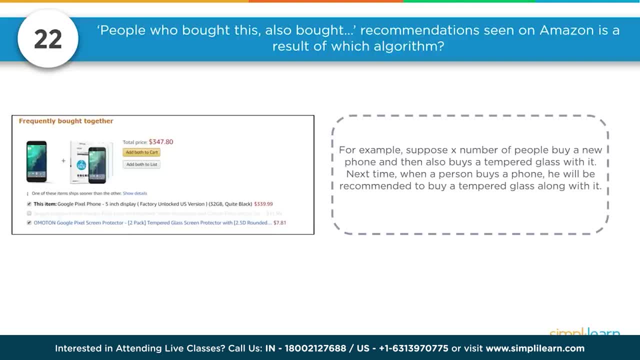 where they took a snapshot of a sales page and it says, for example: suppose X number of people buy a new phone and then also buy tempered glass with it. Next time when a person buys a phone, he'll be recommended to buy tempered glass along with it. And if you remember, 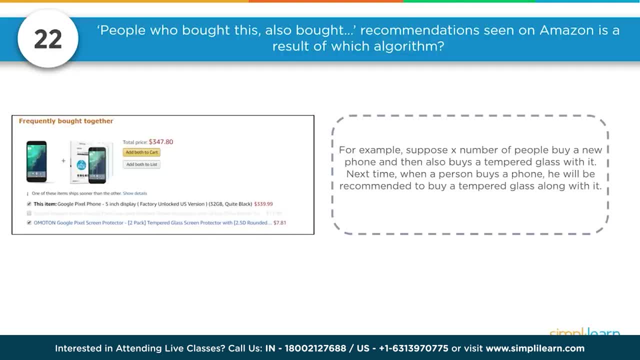 the vocabulary words we covered earlier. this is the recommendation. This is collaborative. The other word was content based. So looking at things with similar content versus collaborative, which is similar people. And remember, you know you're not going to know every vocabulary word. 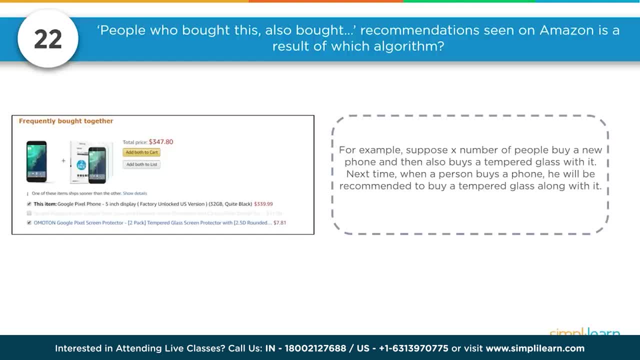 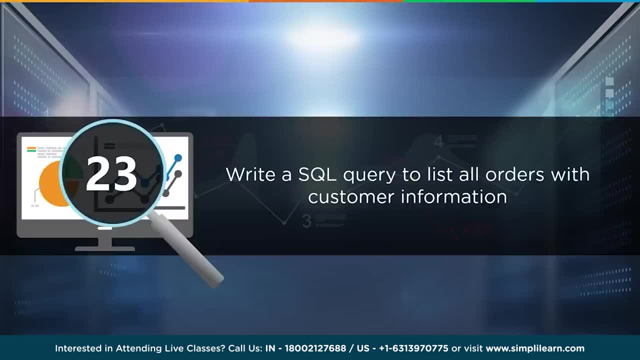 but it also doesn't hurt to get your 3x5 cards out and make yourself a vocabulary stack of cards. Buy an app on your phone for it. SQL query. I remember back in the 90s it was so important to know SQL. 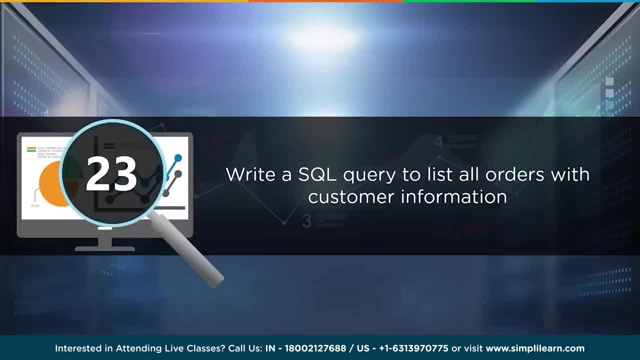 query and only a few people got it. Nowadays it's just part of your kit. You have to know some basic SQL. So write a basic SQL query to list all orders with customer information And you can kind of make up your own name for the database And you can pause. 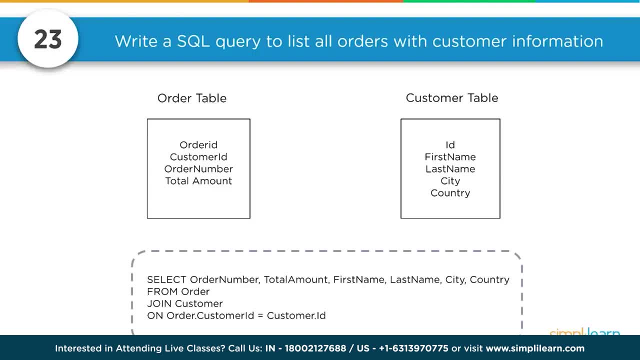 it here if you want to write that down on a paper. And let's go ahead and look at this. We have to list all orders with customer information, And so usually you have an order table and a customer table And you have an order ID. 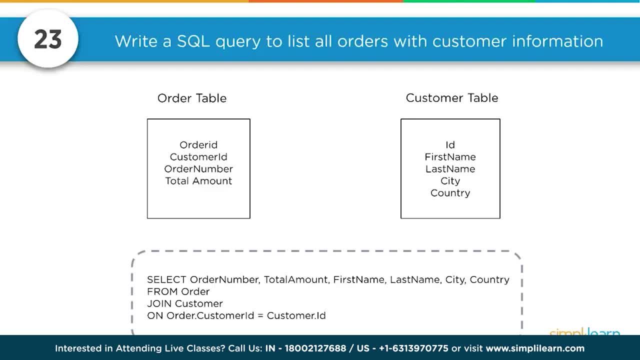 a customer ID, order number, total amount, And then from your customer table you have ID, first name, last name, city, county, And so if we're going to write in SQL with this, we're going to select keyword there for SQL. 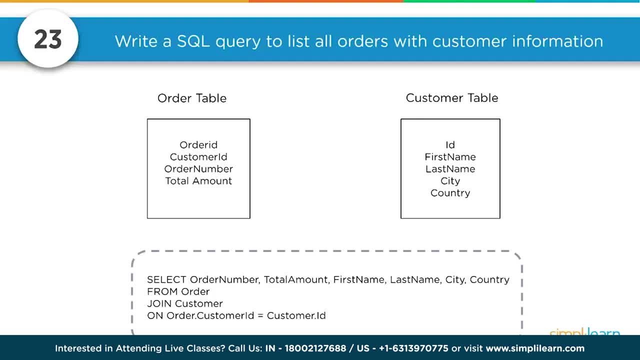 selecting order number: total amount. first name, last name, city, country. So that's the columns we're going to look at. We're going to do that from our order, We're going to join it with our customer And we're going to. 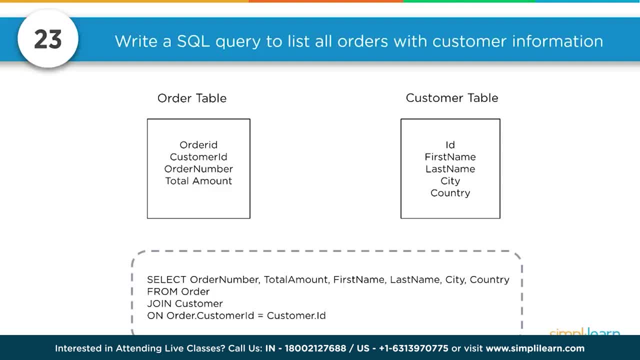 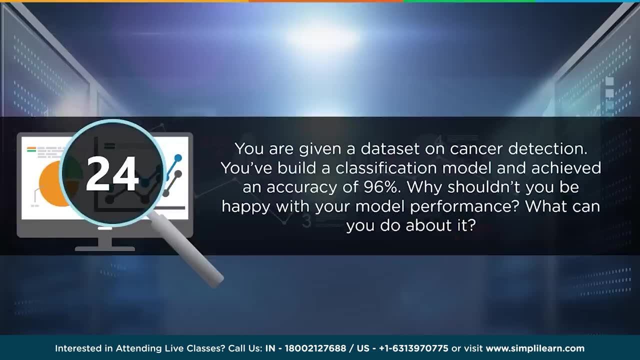 join it on the order. customer ID equals the customer ID. So this is a very basic SQL query that's going to return a table of data for us. You are given a data set on cancer detection. You've built a classification model and achieved an accuracy of. 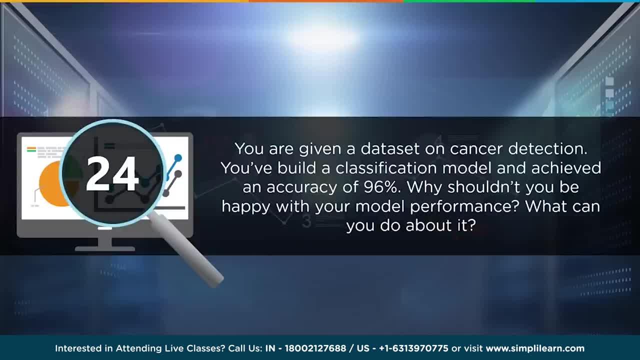 96%, Woo, 96%. Why shouldn't you be happy with your model performance? What can you do about it? That's an interesting one, because this comes up. That's one of the standard data sets on there is for cancer detection. 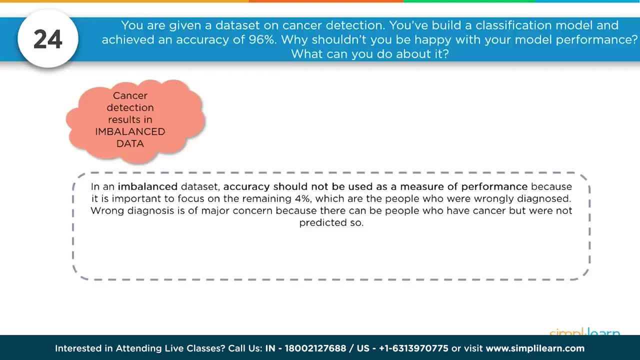 Cancer detection results in imbalanced data, In an imbalanced data set. accuracy should not be based as a measure of performance, because it is important to focus on the remaining 4%, which are the people who were wrongly diagnosed. We talked a little bit about this earlier. You have to. 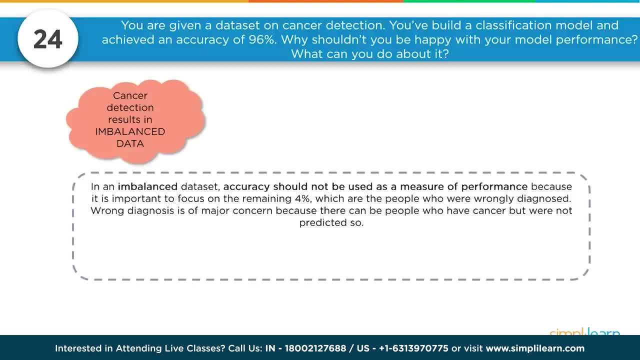 know your domain. You know this is the medical cancer domain versus weather domain. You know weather channel. they can get by with 50% wrong In cancer. you don't want 4% of the people being wrongly diagnosed, Wrong diagnosis. 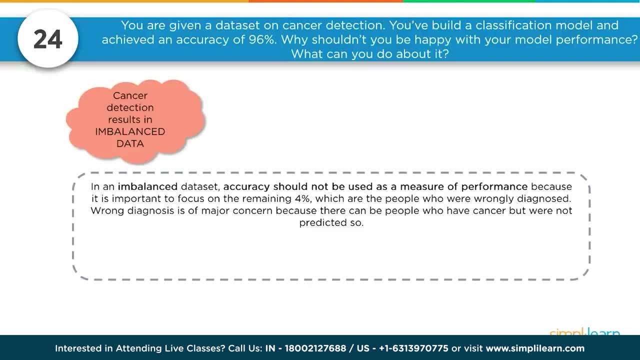 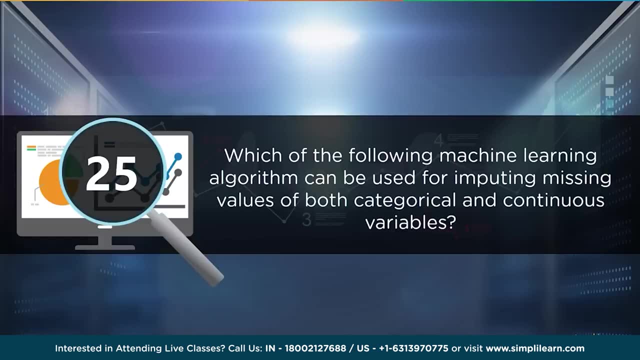 is of a major concern because there can be people who have cancer but were not predicted. so In an imbalanced data set, accuracy should not be used as a measure of performance. Which of the following machine learning algorithm can be used for inputting missing values of both categorical? 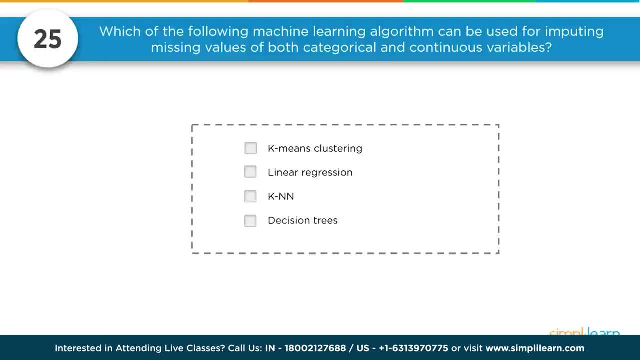 and continuous variables. We have a couple choices here. We have k-means clustering, We have linear regression, We have the knn- nearest neighbor and decision tree. Which of the following machine learning algorithms can be used for inputting missing values of both categorical: 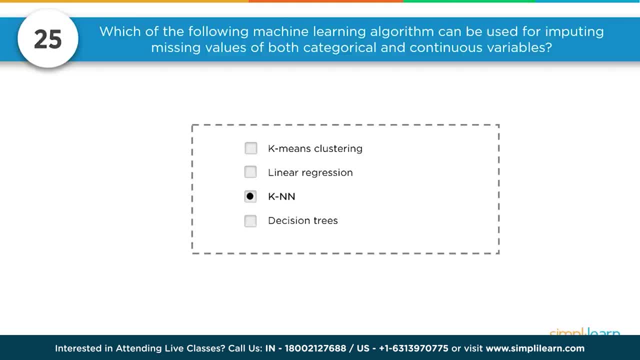 and continuous variables. Certainly you can use some pre-processing to do some of that, but you should have gone with the k-nearest neighbor, because it can compute the nearest neighbor and if it doesn't have the value, it just computes the nearest neighbor based on all. 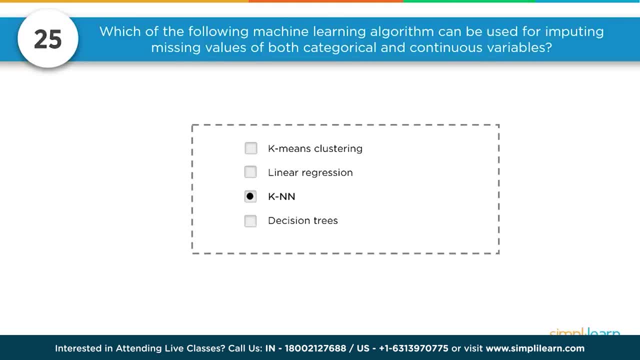 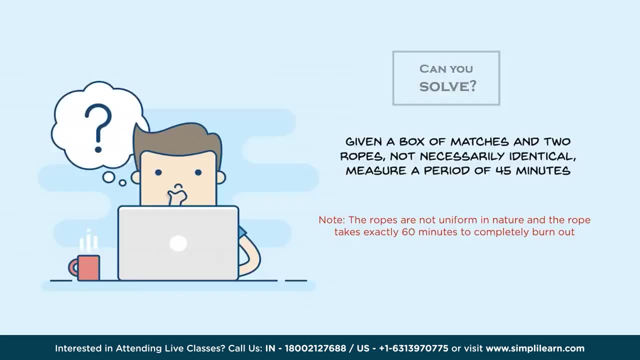 the other features, Where, when you're dealing with k-means, clustering or linear regression, you need to do that in your pre-processing, otherwise it'll crash Decision trees also, although there's some variance on that too. Can you solve Another riddle? 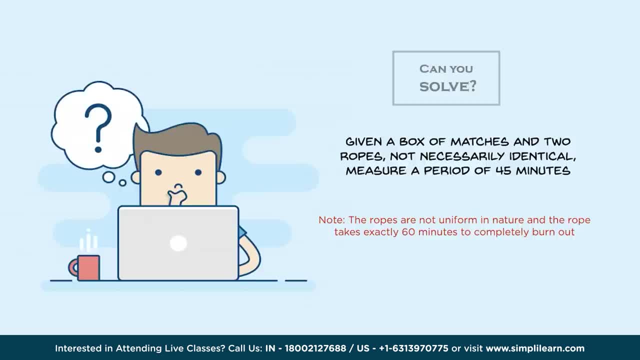 always fun ones- Given a box of matches and two ropes- not necessarily identical- measure a period of 45 minutes And in this particular setup the ropes are not uniform in nature and the rope takes exactly 60 minutes to completely burn out. So each rope takes 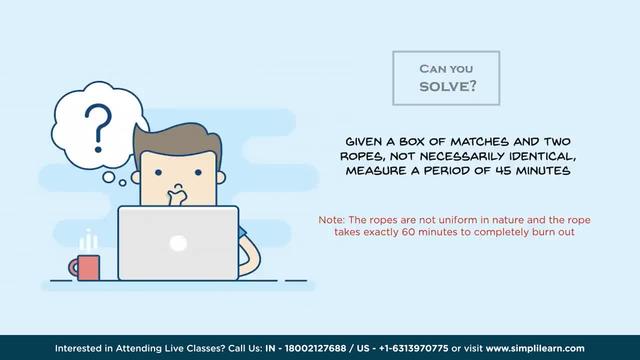 up to 60 minutes to burn out, And there's actually a couple different solutions to this, But let me go ahead, and one of the things is they're not uniform in nature, So even though they take 60 minutes anyways, let's go ahead and see what they did to solve it. 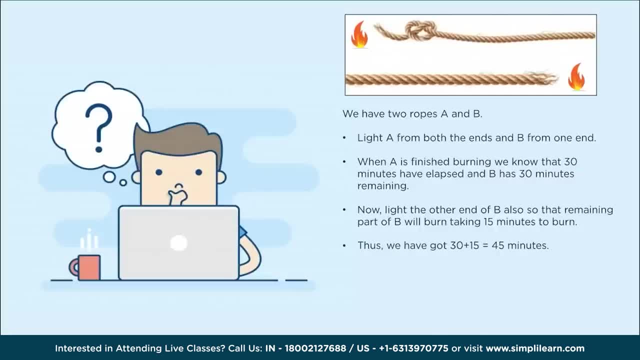 and then we can also look at different options. We have two ropes, A and B Light- A from both ends and B from one end. Okay, when A is finished burning, we know that 30 minutes have elapsed and B has 30 minutes remaining. Now light. 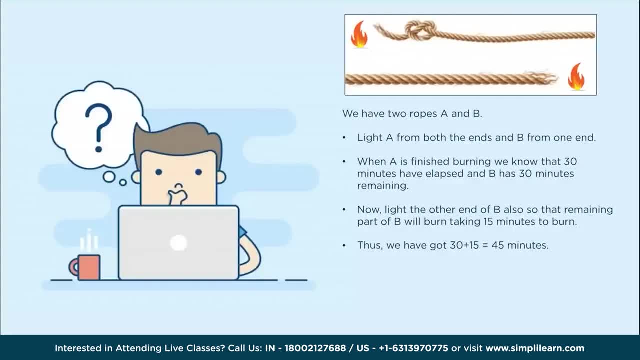 the other end of B also, so that the remaining part of B will burn, taking 15 minutes to burn This, we have gotten 30 plus 15 equals 45 minutes. Excellent solution. Mine, which I like, was to take one rope, fold it in two, so we know. 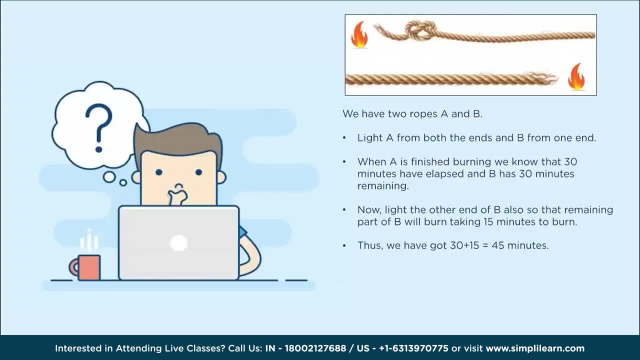 it's a half hour. take the other rope, fold it in four places, so we know that that one's 15 minutes, and then you can just connect the two and burn it straight across. I think they're trying to cover that by saying they're not. 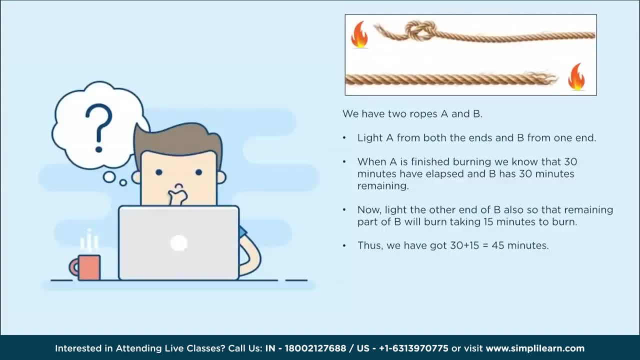 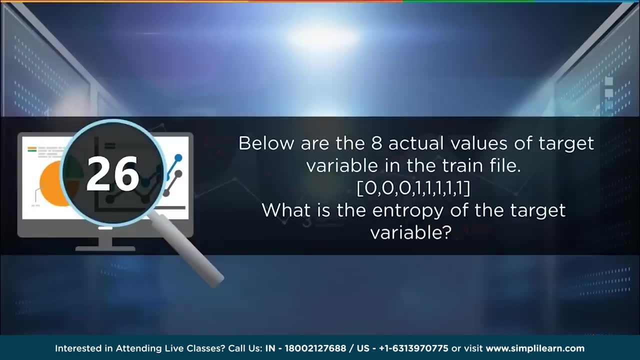 regular. the ropes have some irregularities. Maybe that's what they meant by that is, you couldn't do something like that, But that's my solution. Below are the eight actual values of target variable in the train file. So we have a training file. 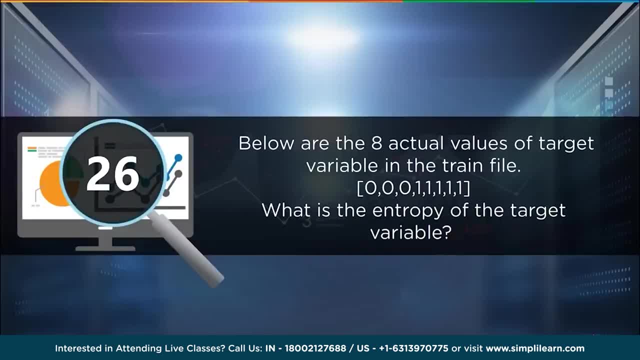 not to be confused with the train on the tracks We have 0, 0, 0, 1, 1, 1, 1, 1.. What is the entropy of the target variable? We mentioned earlier that you should know. 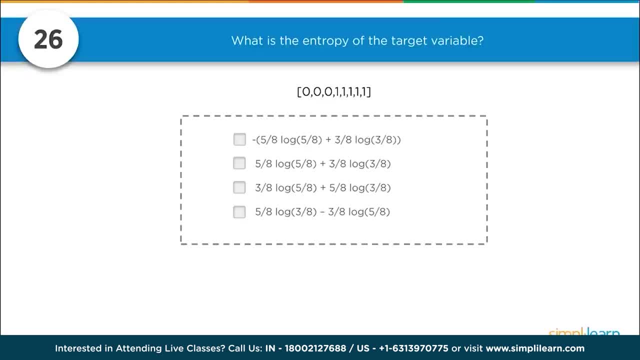 your entropy and how to calculate the entropy. What is the entropy of the target variable? So we have a couple options here. We have: minus 5 over 8, logarithmic of 5 over 8. plus 3 over 8, logarithmic of 3 over 8.. Okay, 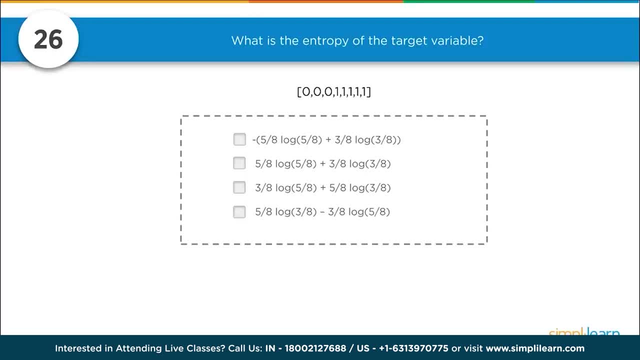 let's just see where they got those numbers from. We have 1,, which is going to be 5 ones, and 3 zeros, and then we have a total of 8.. Okay, And then we have the option of 5,. 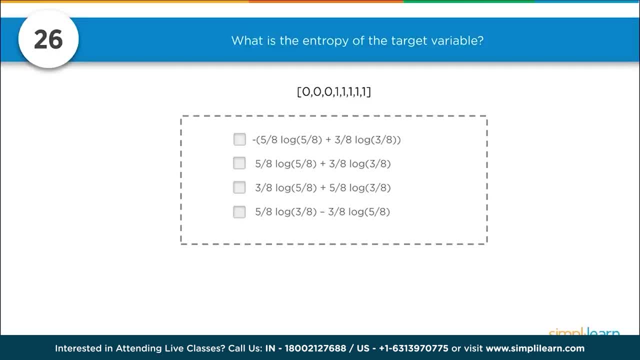 which is the number of ones: 5, 8, logarithmic of 5 eights, plus 3 eights, logarithmic of 3 eights. And we also have 3 eights, logarithmic of 5 eights, plus 5 eights, logarithmic of 3 eights. And 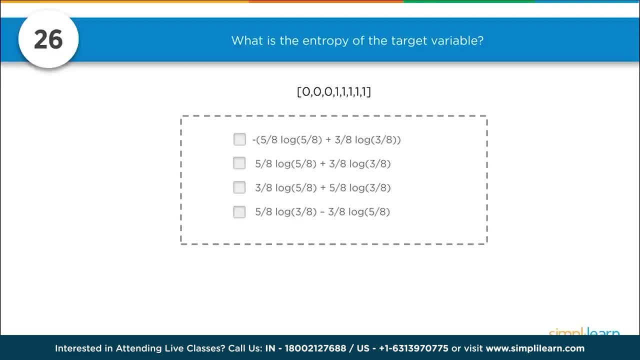 then we kind of reverse those numbers around And let's see what you're going to get here. Which one did you think it was? You should have checked the first one. So what is the entropy of the target variable? The key there is the target variable. 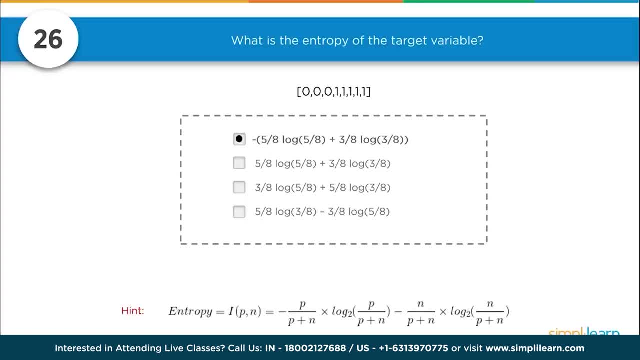 So we're looking at, the target in this case is going to be 1.. Usually that's what you're looking for, And so the entropy of that one we want to subtract out the entropy of the non-target variable. Whoops, I had that backwards. We're looking. 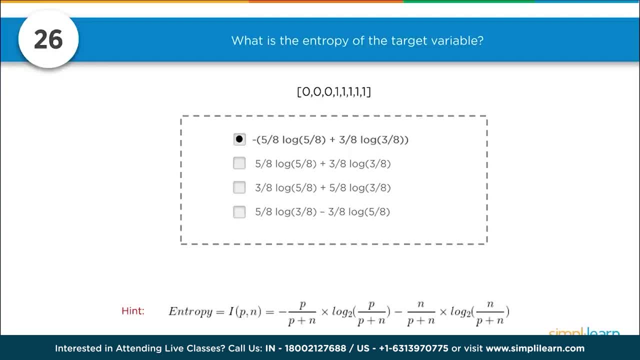 at 0, so we want to subtract out the 5 eights from there. So 5 eights logarithmic of 5 eights, or negative 5 eights logarithmic of 5 eights plus 3 eights logarithmic. 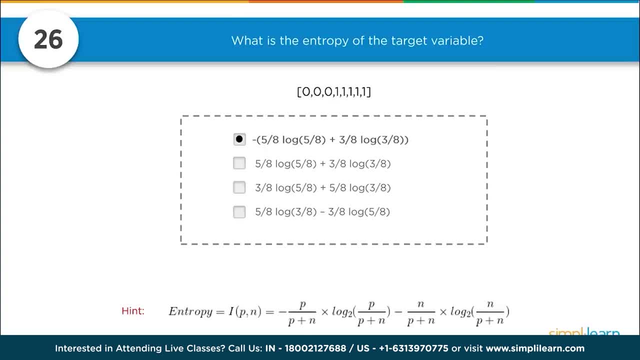 of 3 eights And they have a hint on the bottom entropy equals i of p of n. So we have a negative p plus p and n times the logarithm base 2 of p over p plus n, minus the n over p plus n times the logarithm 2 of. 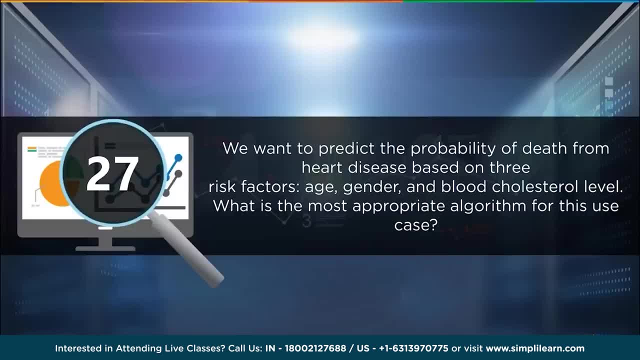 n over p plus n. We want to predict the probability of death from heart disease based on three risk factors: Age, gender and blood cholesterol level. What is the most appropriate algorithm for this case? So we have three features and we want to. 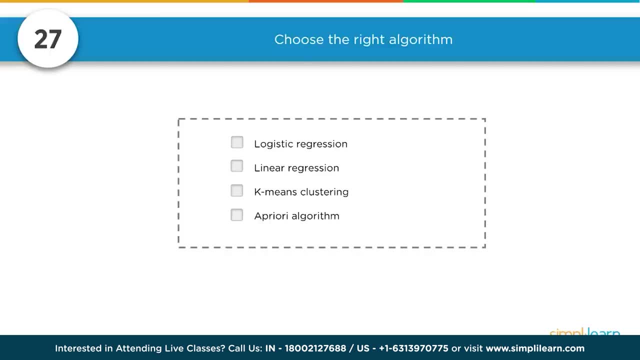 know the predictability of death. Okay, a little morbid there. Let's use the right algorithm. Do we want to use logistic regression for this? Linear regression, k-means clustering or the Aproria algorithm. And if you selected logistic, 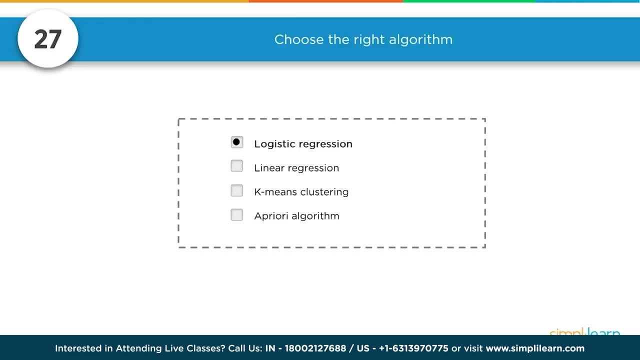 regression, then you probably got the right answer. Linear regression, remember, deals with like you take your line and draw a line through the data, and of course, you don't necessarily have to use a straight line. there's other means for that- But you're dealing. 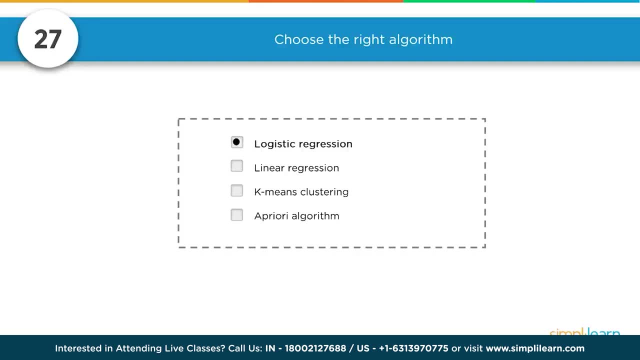 with a lot of numbers And k-means means we're just going to cluster objects together With the logistic regression, though you can mix those things together in buckets. So really the logistic regression is what you want to use in that model would be the most apt fit. 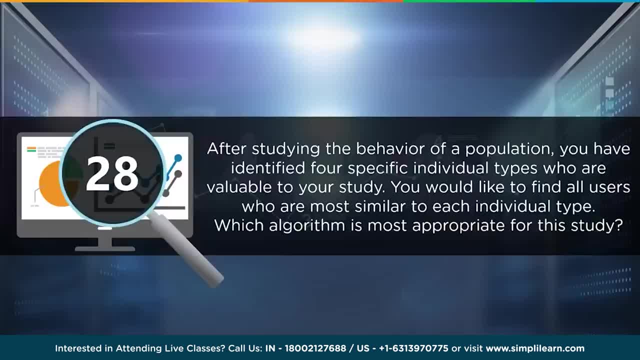 After studying the behavior of a population, you have identified four specific individual types who are valuable to your study. You would like to find all users who are most similar to each individual type. Which algorithm is most appropriate for this study? Certainly, identifying census in just about a lot of different markets is common. 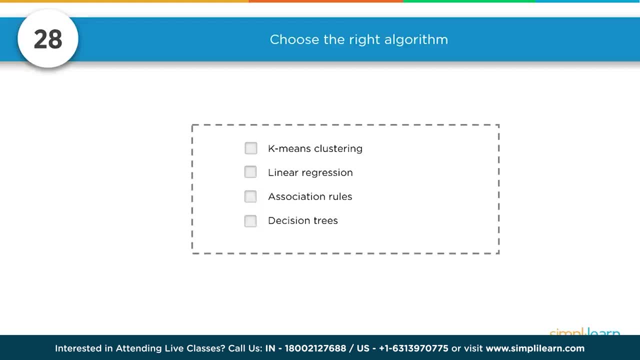 so maybe they have a census or whatever it means. But let's take a look at some of the different algorithms we might use on this. We have k-means, clustering, linear regression, association rules and decision trees, And I'll give you a hint: we're looking. 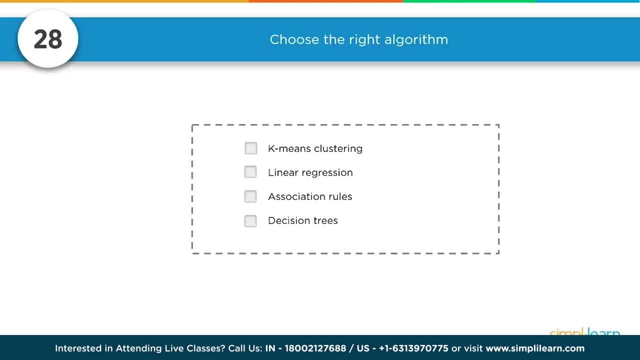 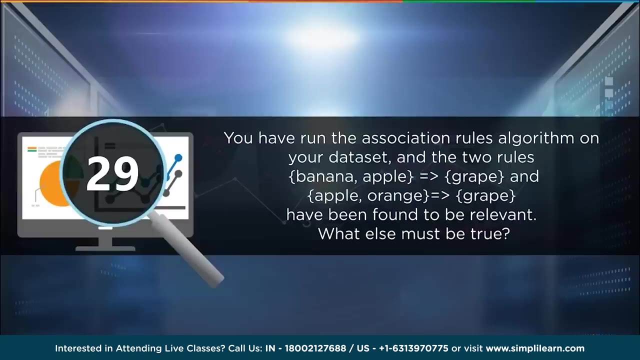 for grouping people together by similarities, and by four different similarities, so very specific. They gave you one of the values, specifically the k-value, So k-means clustering would be great for this particular problem. You have run the association rules algorithm on your dataset And the two 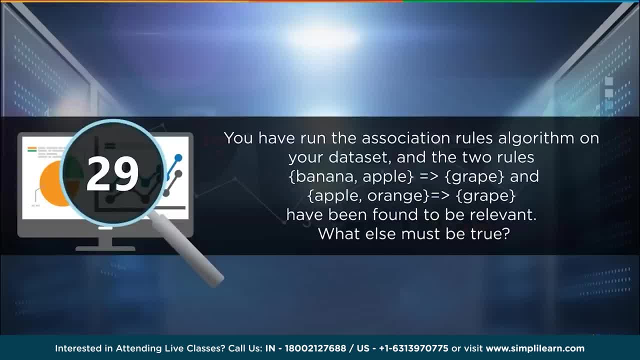 rules. banana-apple is associated with grape and apple-orange is associated with grape. They have been found to be relevant. What else must be true? So this would challenge you to understand association rules. You could picture in this particular one, you're going. 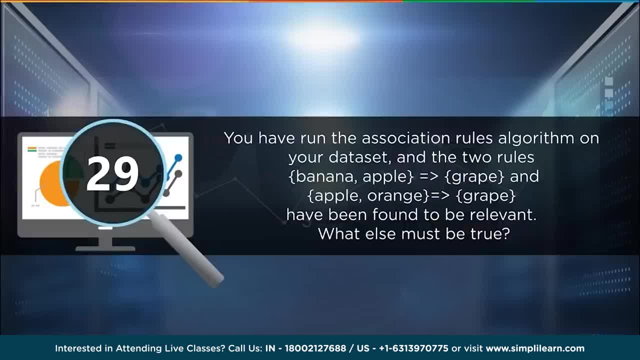 shopping and you almost always see somebody who has bananas. they usually have grapes in their bag also, And somebody who has apples usually has grapes in their bags. And then apples and oranges is also associated with grapes, And let's go ahead and take a look at that And we have a couple. 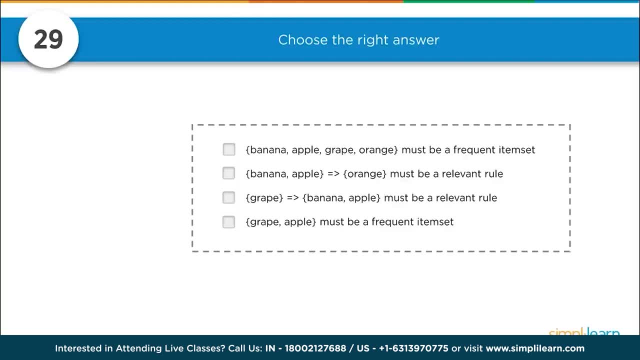 different options here. First one is: banana-apple and grape-orange must be a frequent item set. Not so much Banana-apples, oranges must be a relevant rule. Grape is common with banana-apple. must be a relevant rule. And how about grape-apple? 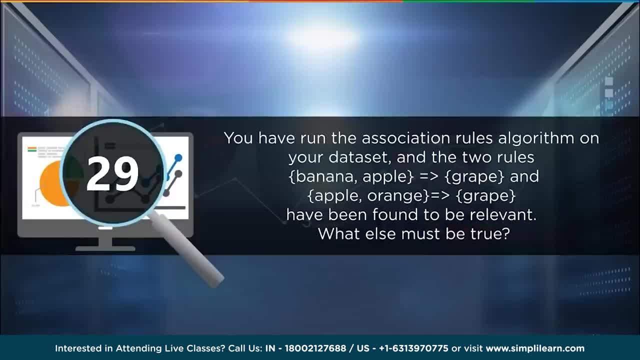 must be a frequent item set. Let's go back and take a look at that And we notice that we have bananas-apples to grapes, We have apple-orange to grape Boy. there's a lot of grapes and a lot of apples in there. 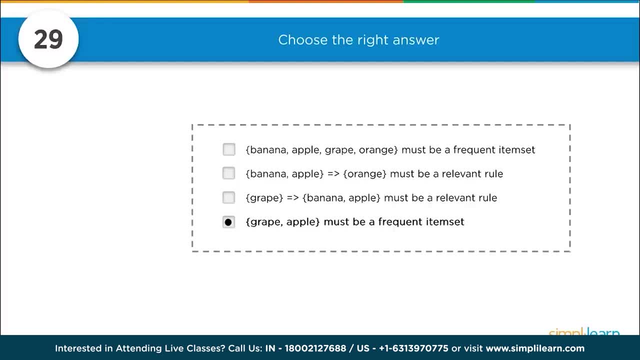 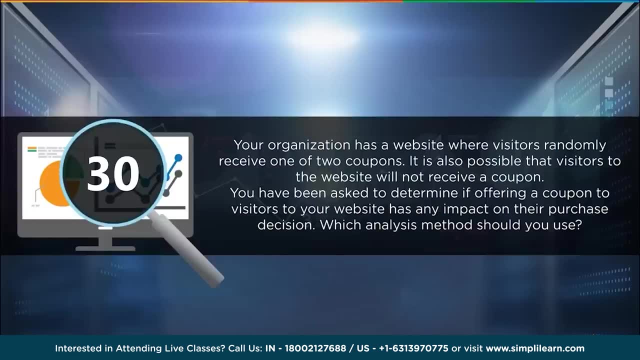 And so if you said the last one- grape and apple- must be a frequent item set, then you got it correct. Your organization has a website where visitors randomly receive one of two points coupons. It is also possible that visitors to the website will not receive a coupon. 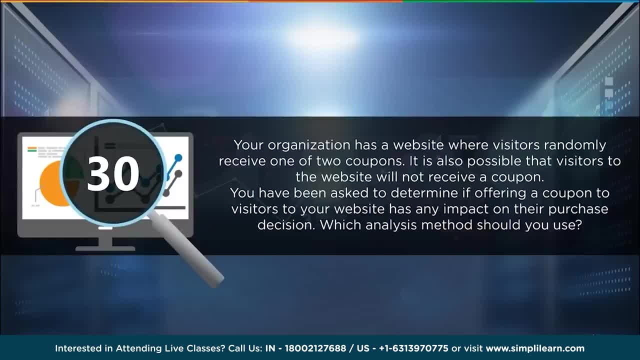 You have been asked to determine if offering a coupon to visitors to your website has any impact on their purchase decision. Which analysis method should you use? And so let's go ahead and start by giving you another hint and give you some limiting your selection. 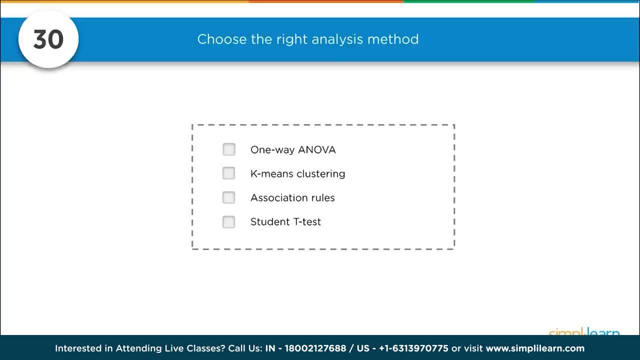 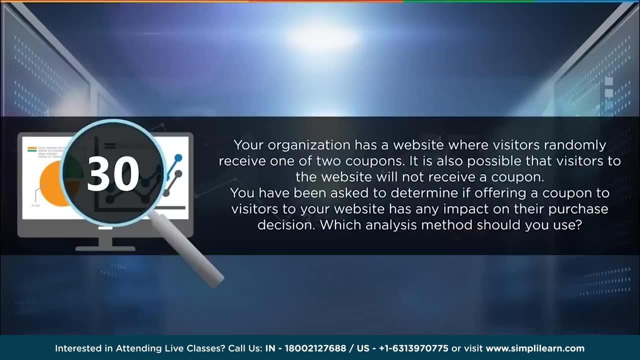 We have a one-way ANOVA. k-means clustering, association rules and student t-test, So obviously you should know what each one of these means, but let's take a look at the question again. So you want to know which method. 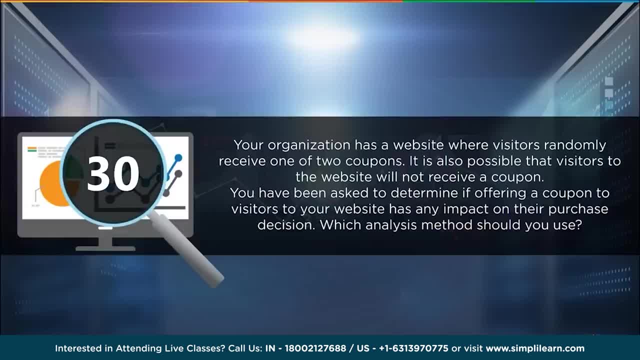 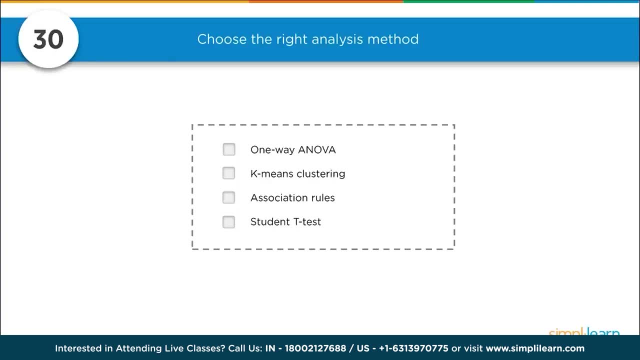 should you use to see if the coupon's valid for their purchase? While we're not clustering, we're not associating things together. we want to know the end result. Student t-test: also drawing the little t in boxes and switching them around. There's really only one answer. 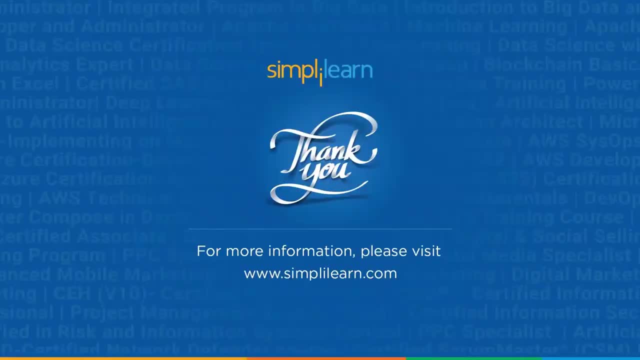 that works in here and that's the one-way ANOVA, And with that we have reached the end of this advanced data science full course. If you have any questions, please feel free to comment and we will have it answered as soon as possible. Until next time. 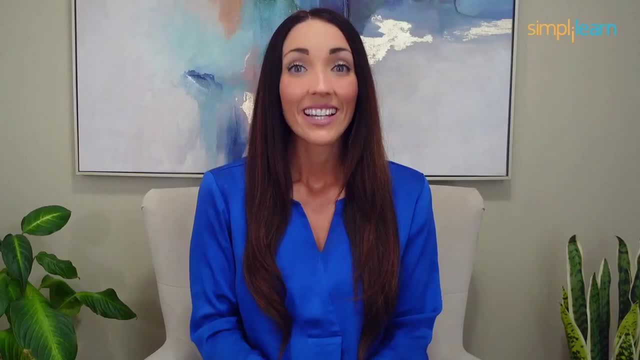 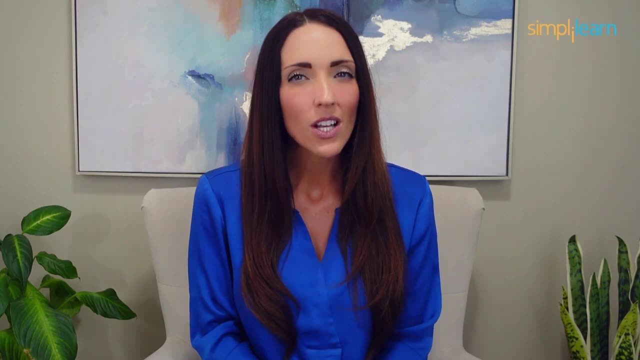 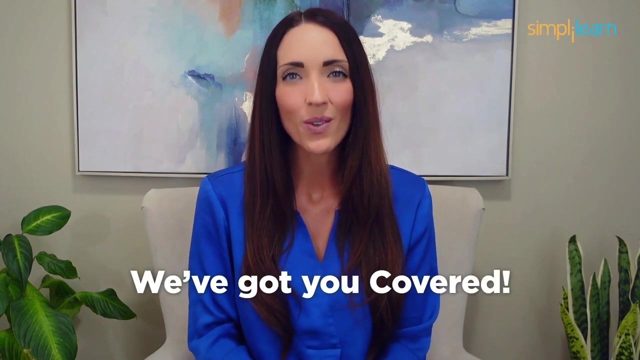 thank you for watching. stay safe, keep learning and get ahead. Staying ahead in your career requires continuous learning and upskilling. Whether you're a student aiming to learn today's top skills or a working professional looking to advance your career, we've got you covered. 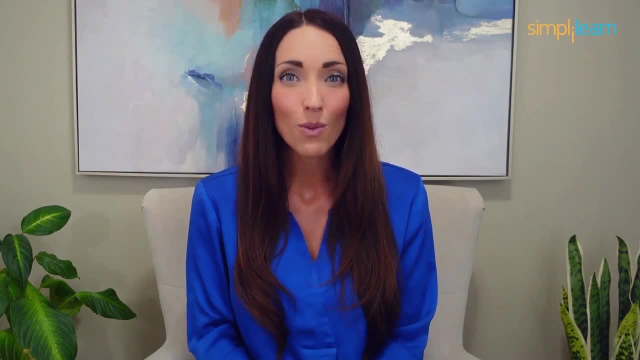 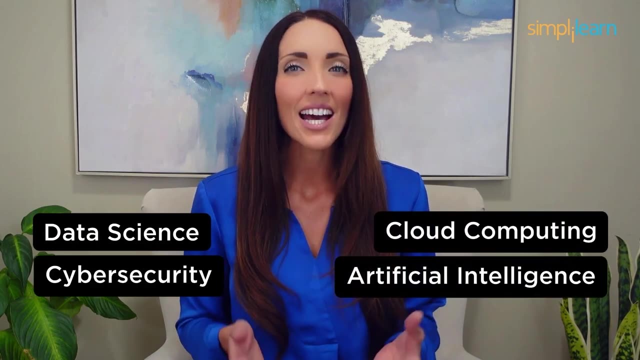 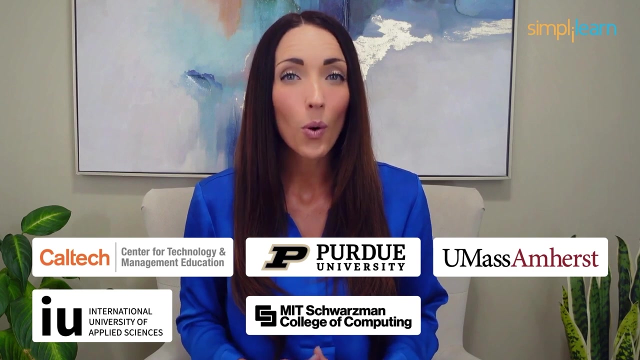 Explore our impressive catalog of certification programs in cutting edge domains, including data science, cloud computing, cyber security, AI, machine learning or digital marketing, Designed in collaboration with leading universities and top corporations and delivered by industry experts. choose any of our programs and set yourself. 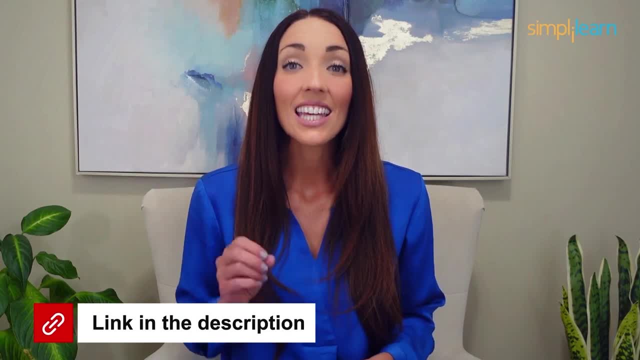 on the path to career success. Click the link in the description to know more.